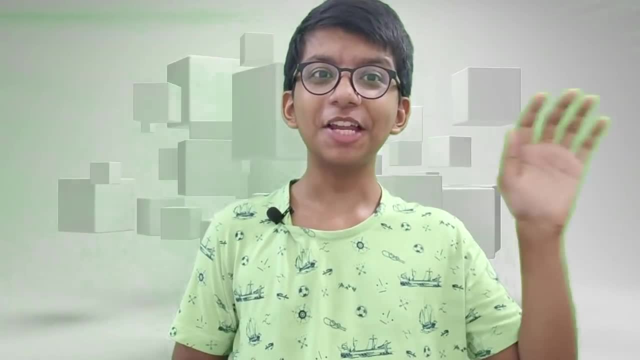 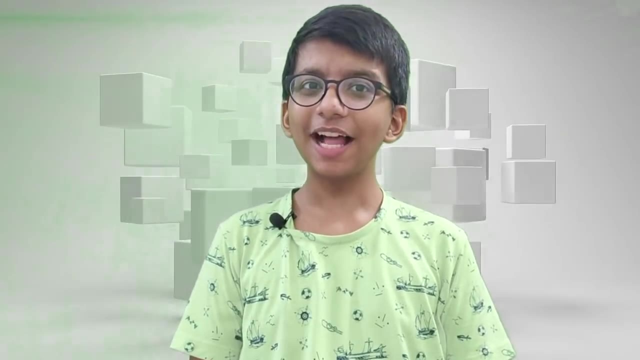 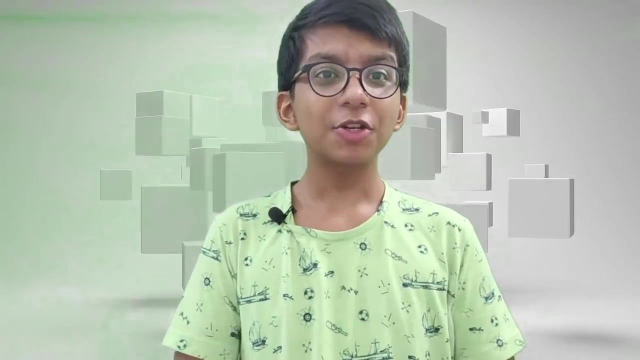 machine learning from very basics to an advanced level in machine learning. In this course you will be having both theoretical, practical understanding of machine learning algorithms and building real-world AI projects. After this course, you will be able to build your own machine learning applications and real-world applications in many domains. 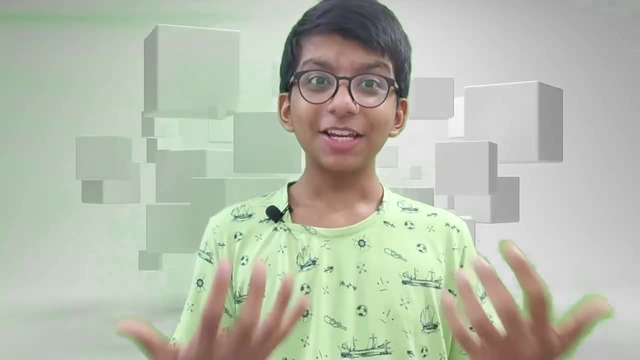 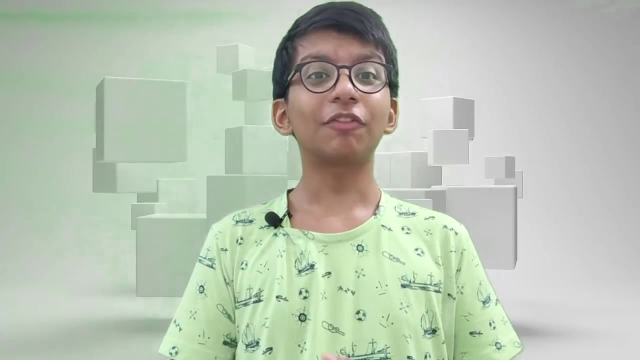 But wait First. who am I? My name is Ayush and i am A data scientist at Artifact. I am from India, standards 9.. I have worked on various applications of artificial intelligence, like machine learning, deep learning, artificial intelligence, and we operate in one whole academic. 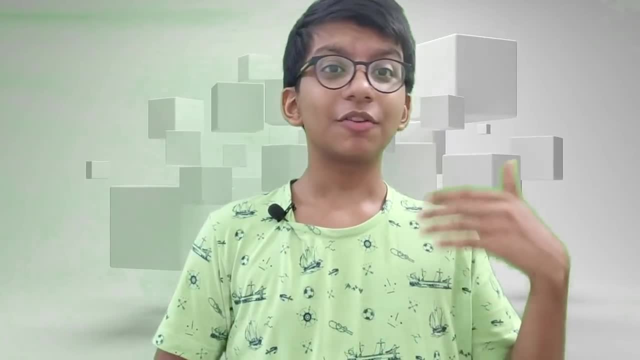 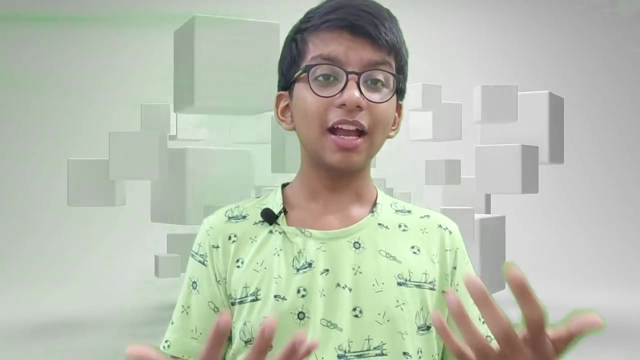 diaphragm. This course will be a�iudeane of AI project. From this course and after, I've worked on various domains of deep learning, which is known as computer vision, generative adversarial networks and natural language processing. I've also contributed to the large AI process and a team by Undana. 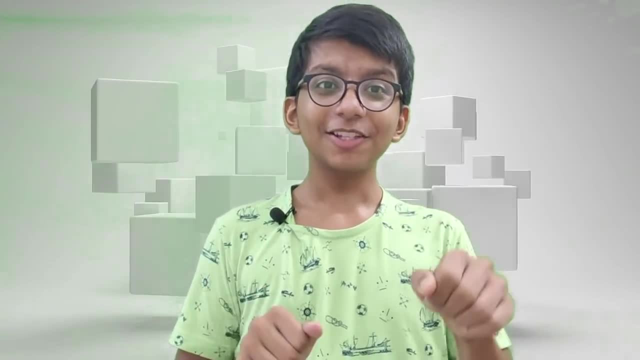 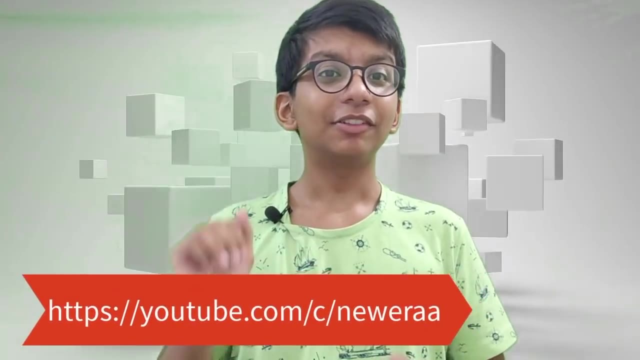 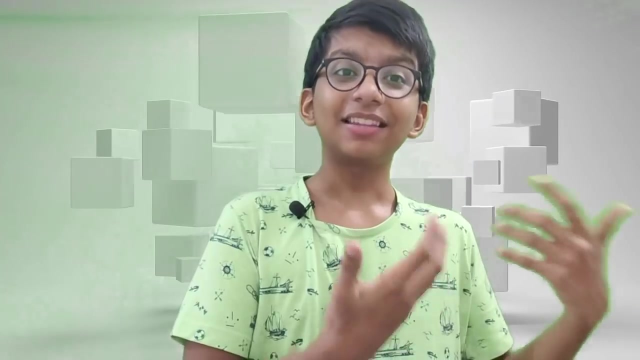 Okay, so this is my basic skills And also I run a small YouTube channel- which is not as big now, not as small- a big YouTube channel which is around we have 500 members, where I make a content on machine learning, deep learning and various AI things. 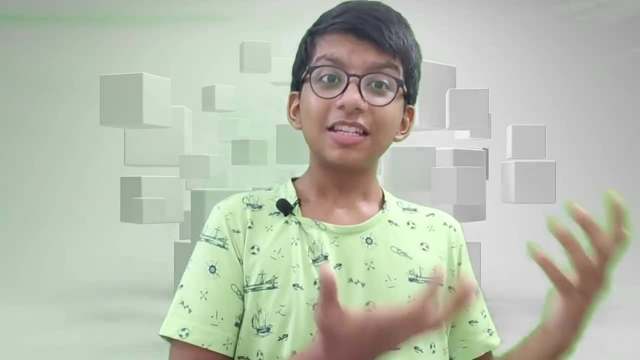 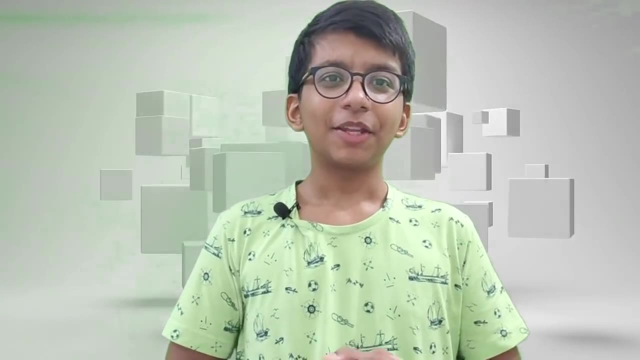 And I put end-to-end courses there. Currently, deep learning course is being launched, So you can start coaching after this completing this course, that deep learning course. Okay, so that is from my side, And you can connect me on LinkedIn if you want to know more about me. 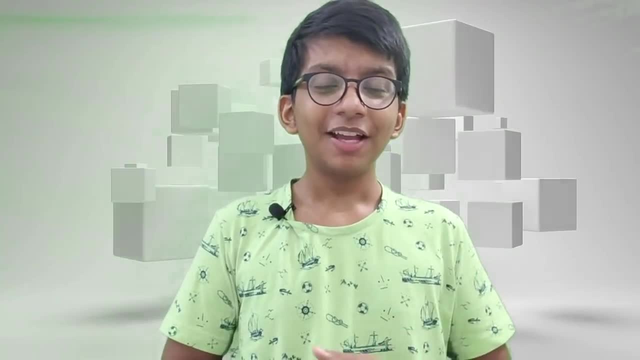 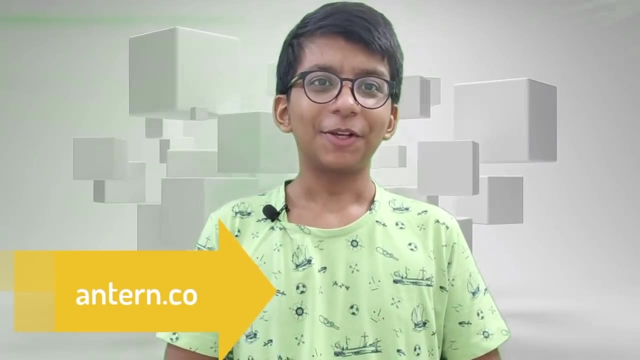 And I've also cleared some Microsoft exams, so you can get to know more about me. Okay, I'm also a founder. I'm a founder of Android, an AI tech platform, and also a product-based platform. Okay, so that's it from my side. 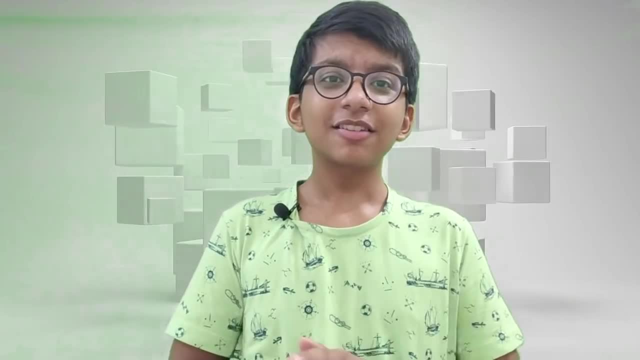 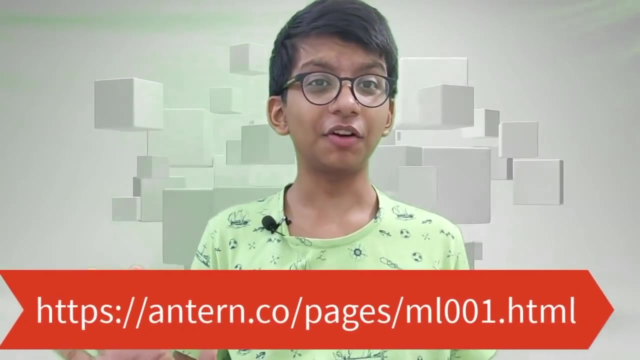 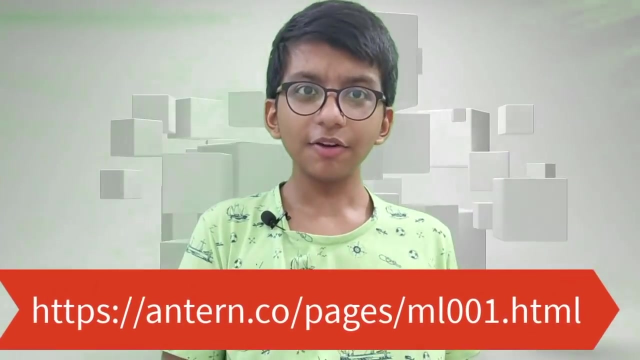 And I hope that you will get a lot more from this course. Now let's discuss the syllabus of this course. We will start with the very basics of machine learning, covering the fundamentals of machine learning, into section number one, And then we will go further into understanding some algorithms like linear regression, logistic regression, support with the machine. 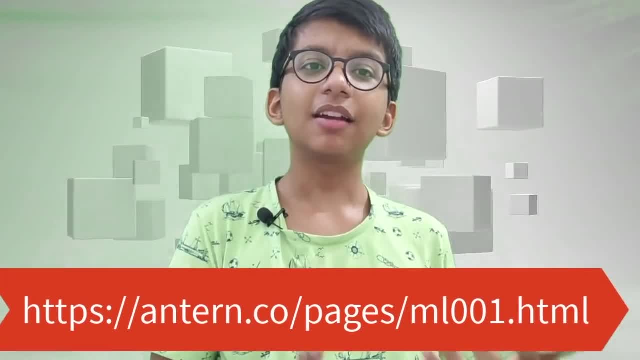 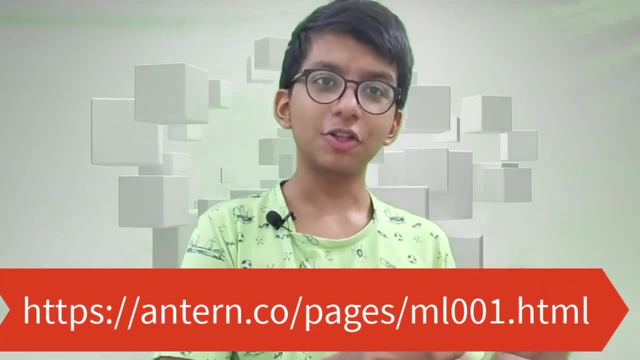 principal common analysis learning And some ensemble learning methods like bagging, boosting, stacking, cascading, and then we'll talk about unsupervised learning And you may think, hey, Ayush, what do you want to teach this much? 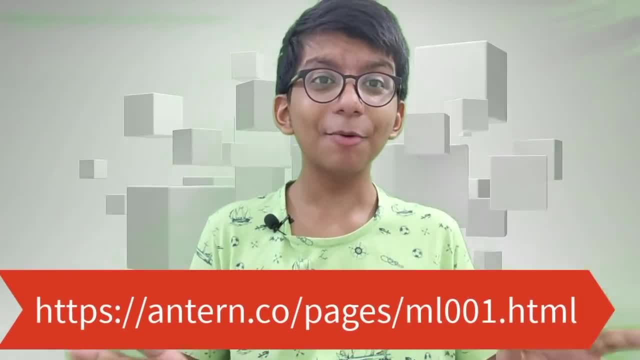 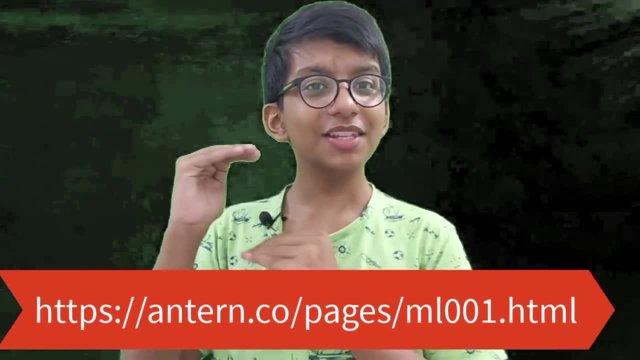 No, absolutely no. This is a 10 plus hours, of course. So absolutely, there is a lot more content. So this course is divided into sections and each section has different subsections. So I have made a full list of sections. 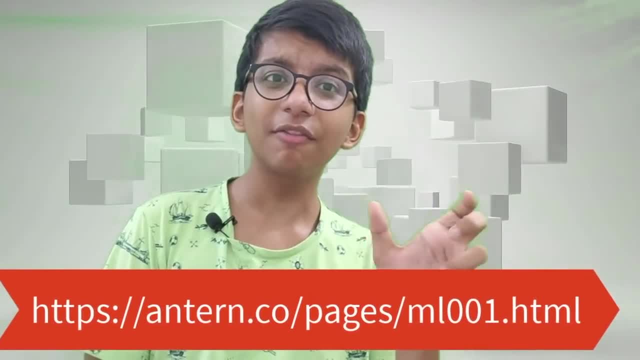 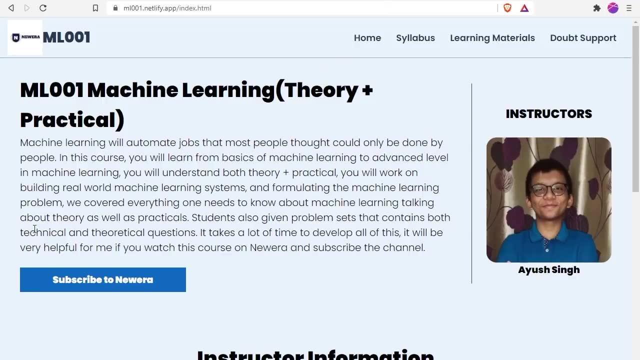 So I have made a full list of sections. I have included all syllabus talks what topics I'm going to cover in each of the topics or sections divided into subsections. And you can assess the syllabus by visiting the course website. 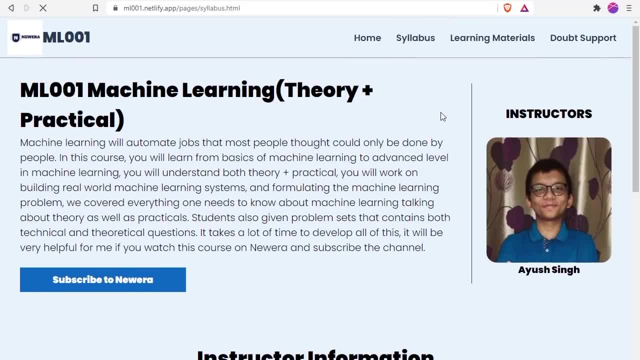 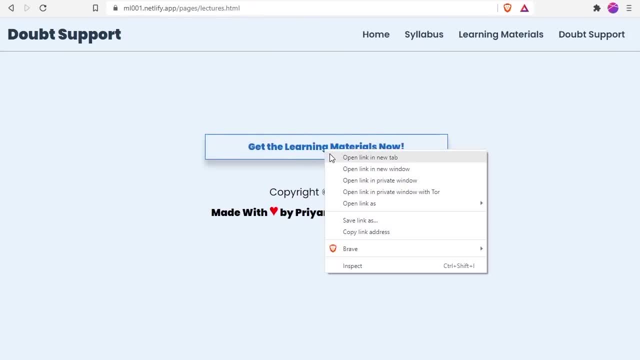 The course website I pre-made with. I made with my friends, friends of Antwerp, so you can definitely go there and assess all the syllabus, all the problem sets of this course and each and every section. you'll be having one problem set. 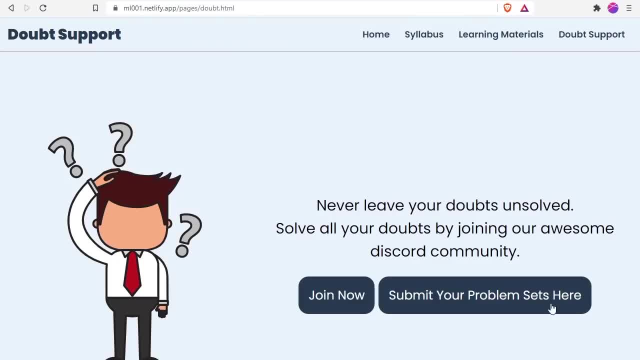 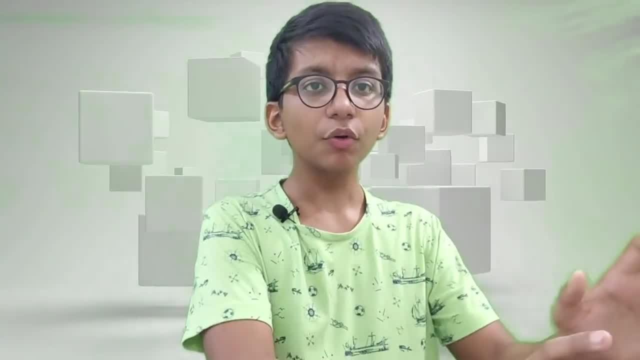 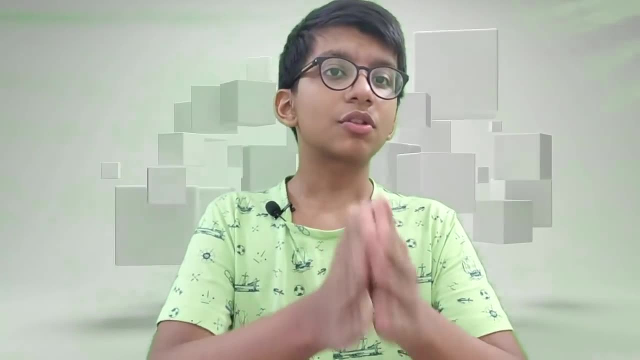 And all of these is in the description. All of these is in the description down box below. okay, all of where the time stamps, as well as the course notes, okay, so are all available on the course website so you can go there see what's assignment are there, complete that and join our discord server. to just to, 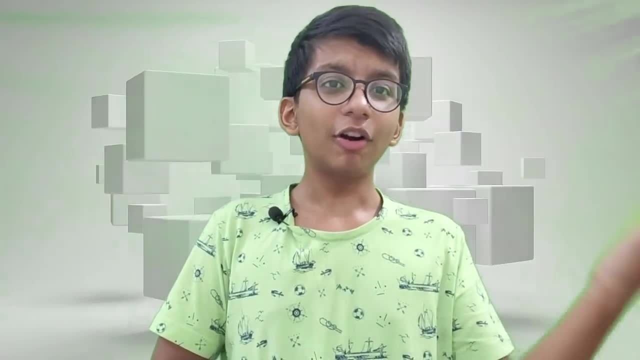 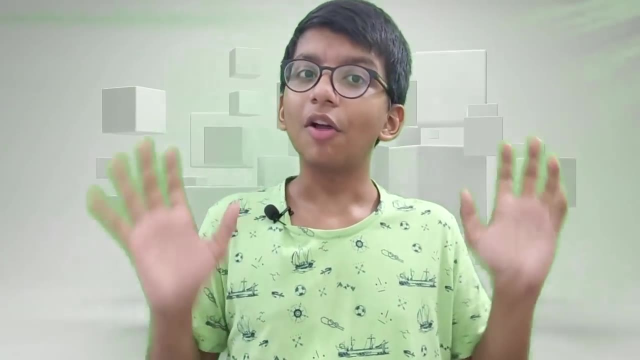 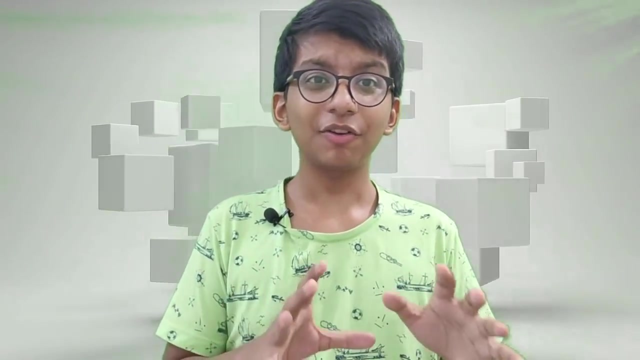 discuss your assignments, and you can also submit it through forum. okay, so this is the basic syllabus that we are going to follow and I really hope that have worked a lot in preparing the materials for this course, teaching you all and the blackboard and understanding you, helping understand each and every. 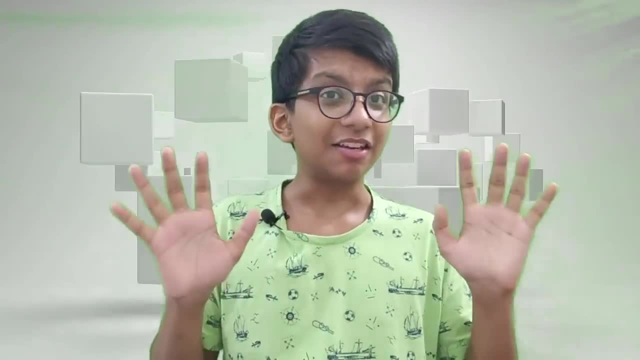 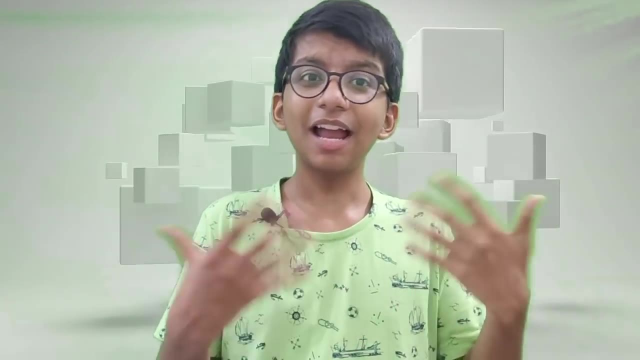 topics of machine learning, and a very, very, very easy way. and this course has extensive syllabus, a very good syllabus, to which I have, which I haven't seen on you full YouTube okay, so please be sure to see the syllabus, what we are going to. 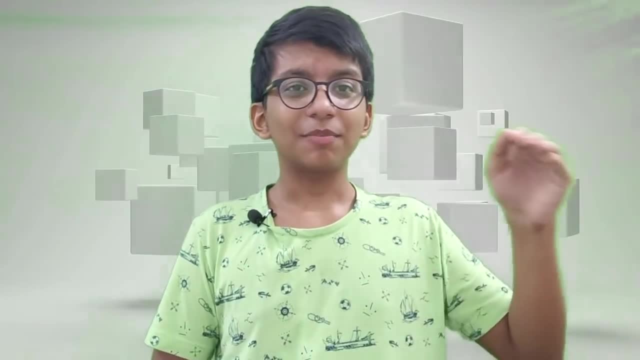 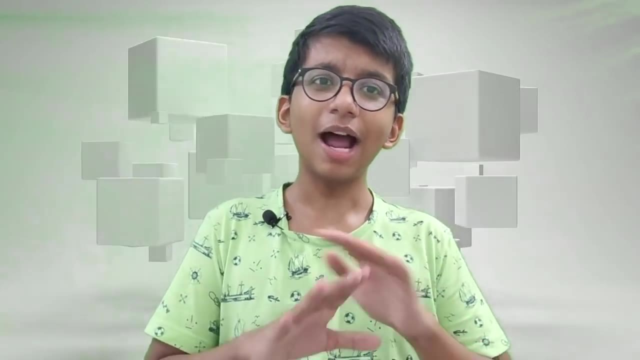 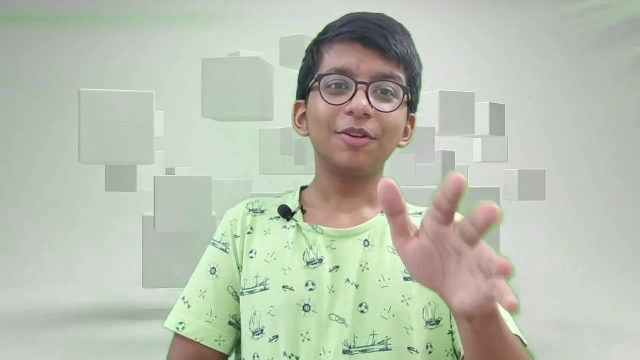 cover. just have told you in just shot. the reason is I want to just start with this, this video, so I give it a shot. you can see the syllabus by visiting our course website. for absolutely free, everything for absolutely free. you can go to the course website, which is the link in the description down box below. so let's 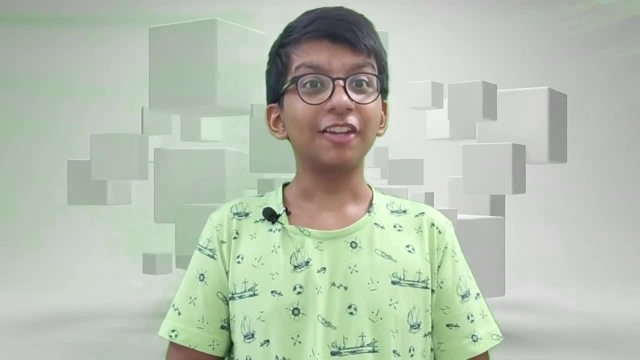 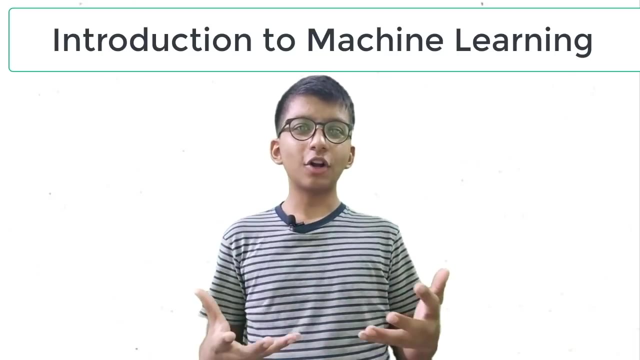 start with the section number one, fundamentals of machine learning. okay, so now we'll start with machine learning. in this section you will get introduction to machine learning and we'll talk about introduction to machine learning, types of machine learning and their types, and we'll see some full application. 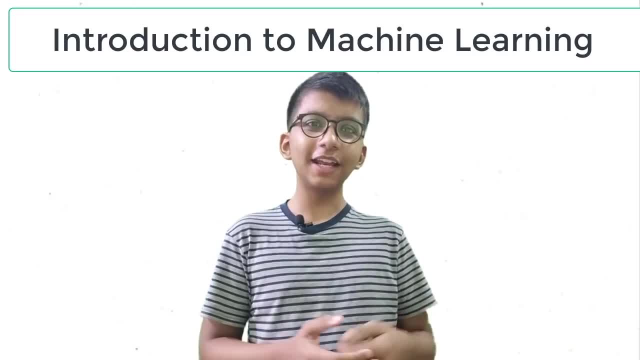 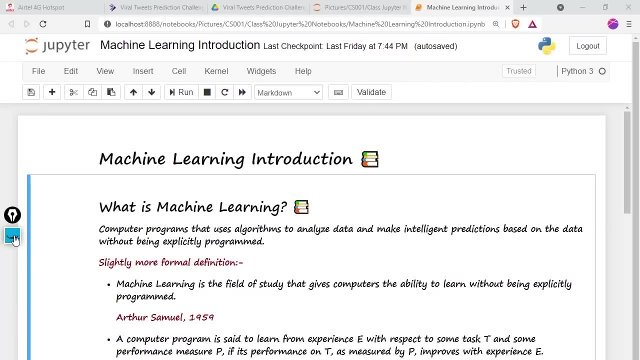 and then we will see some problem of overfitting and underfitting, and then we'll wrap up this section, okay, so let's start. okay, so now we'll answer a question: what is machine learning? and you may ask: hey, Ayush, can you tell what actually machine learning is? yeah, you will get to know more and more. 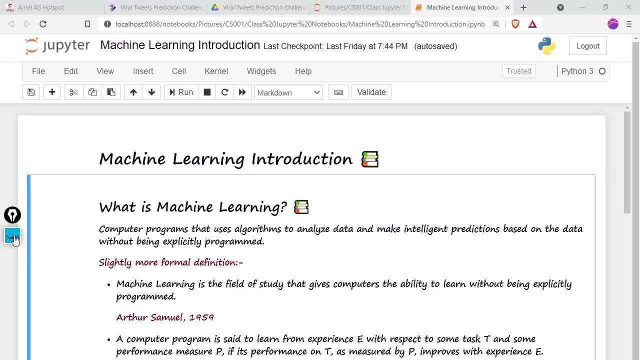 about what actually the big picture of machine learning means. you in depth, when, when we will go through this course. but in simple terms, machine learning is like this: computer programs that uses algorithms to analyzes the data and make intelligent predictions based on the data, without being explicitly programmed. and you might think, hey, Ayush, what is kind of? 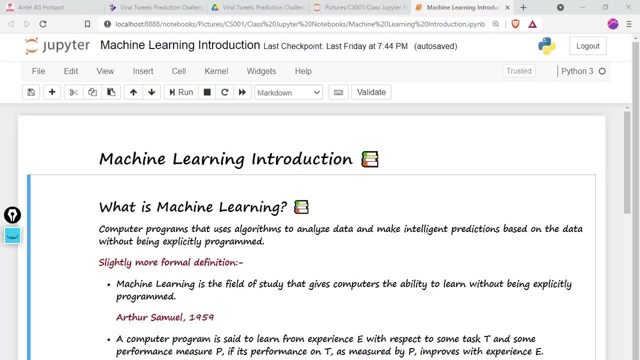 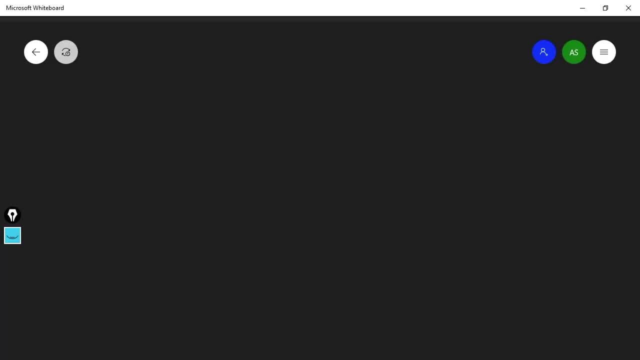 this. I'm getting a little bit confused, no worries. so let's, let's get into this and let let me explain you what I'm saying over here in this black boat. so you're given a data, you're given a data, okay, and then you give to the algorithm. 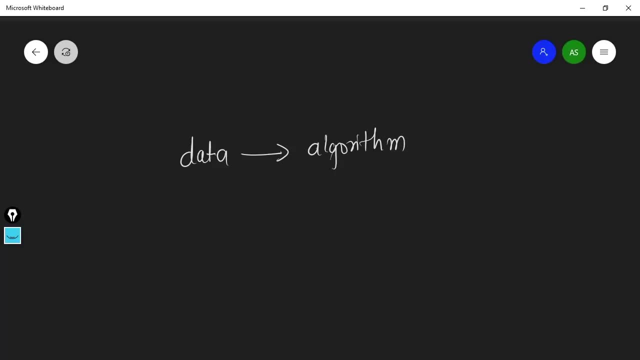 the algorithm. the algorithm analyzes the data, analyzes the data, analyzes the data and whatever he has analyzed or learned from the data, it makes predictions based on to that. it makes predictions on to that. okay, so, specifically, what we word or what what we are doing, we want to make a function X that maps out input. 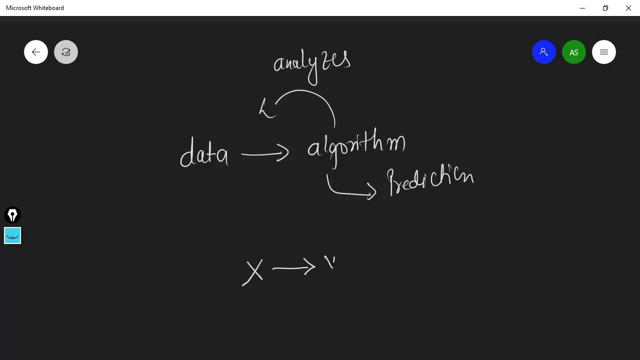 variable X to the output variable Y, Y, And you may think: yeah you sure, confusing me. What is X, What is Y? No worries, X is the input feature. X is the input feature means, um, let's take in a problem statement, or predicting: 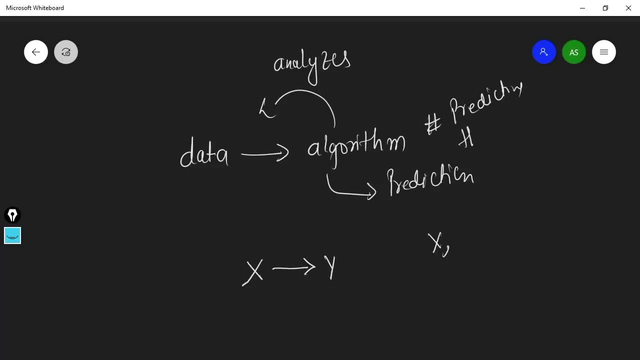 the house prices. predicting the house prices. Okay, So you want to do this, So uh, here, on the basis of the size of the house. So, uh, on the basis of size of the house, you want to predict the price of the house. Okay, So you give input variable X and you get output variable Y, Okay, 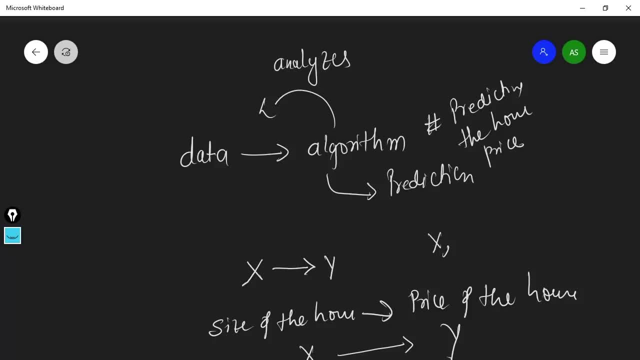 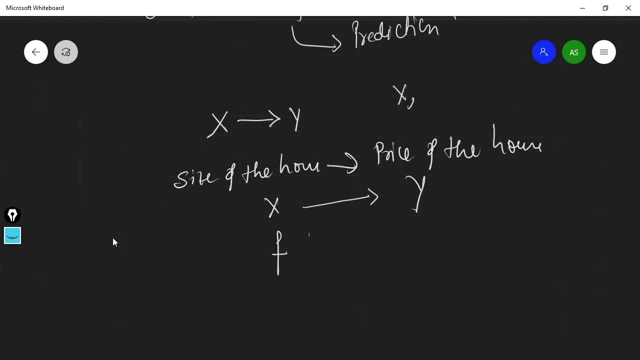 So, on the basis of the size of the house, you want the price of the house. Okay, So you wanted to make a function. So you wanted to make a function F that takes input X and maps that to Y. And that's the definition of machine learning. That's the. 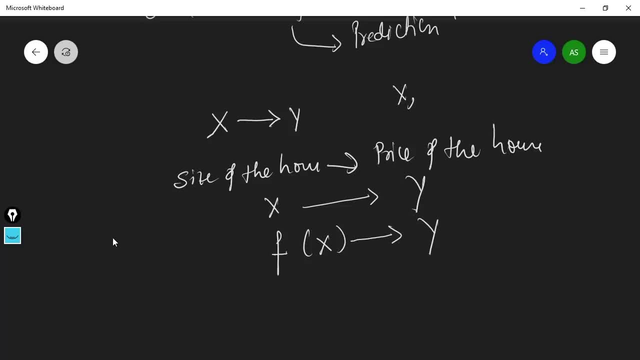 beauty of machine learning. So what you were doing, we are. we want to, we want to map our input variable X. Maybe it can be, maybe the size of the house, maybe the- uh, the number of fans of the house, maybe the number of our bedrooms in the house. So I'm denoting with a subscript one. 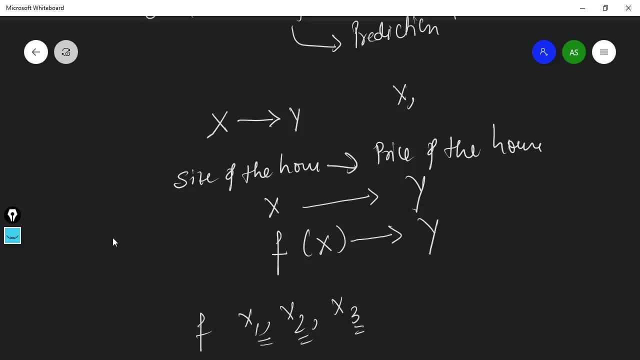 subscript two, subscript three: and we want to make a function that maps this input variable to the output variable, which, which we did denote with Y, which is the price of the house, And that's and that we are doing, and we will, and we will learn how to make this functions. Okay. 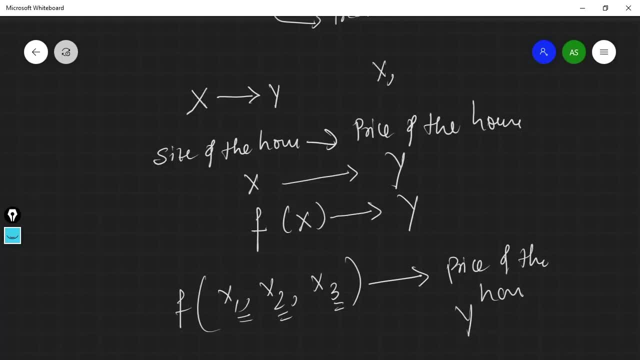 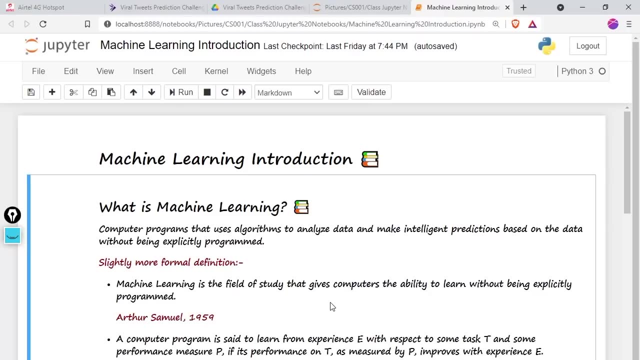 So that's the beauty of machine learning which you can see over here. So let's see some of the more formal definitions which you, which you will see you more over the internet. And the machine learning is the field of a study that gives computer the ability to learn without 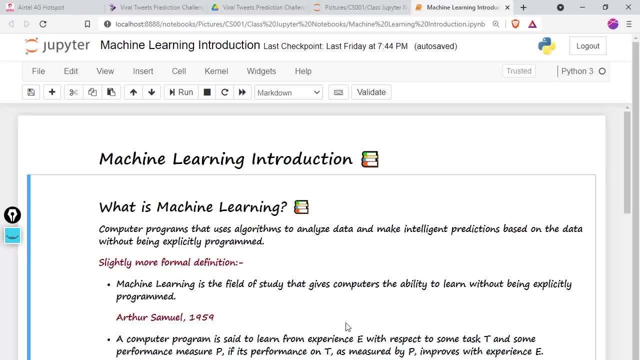 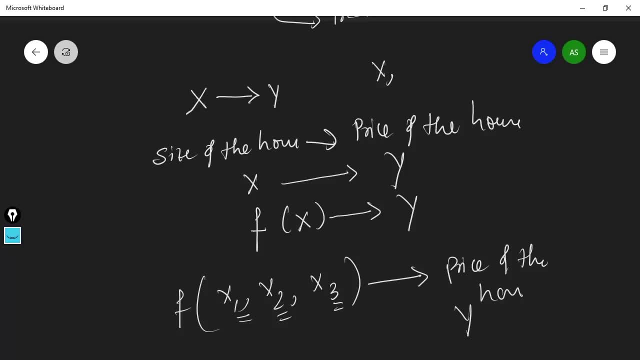 being explicitly programmed, saved by Arthur Samuel. But one definition that I've said to use totally means: if you, if you, if you. if someone asks you Hey, Hey, whatever your name, uh, what is machine learning? You just ask: Hey, I know a better way. 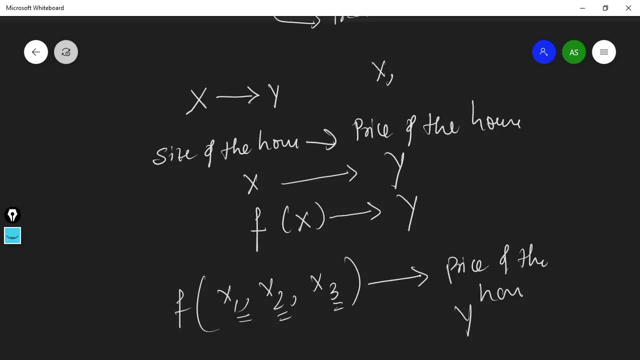 to define a machine learning, You just make a fun to you, just to make a function that maps your input variables to the output variable. Okay, And that's the beauty, or that that's called the machine learning, And I hope that you, that you, that you got it What I'm, what I'm trying to say. 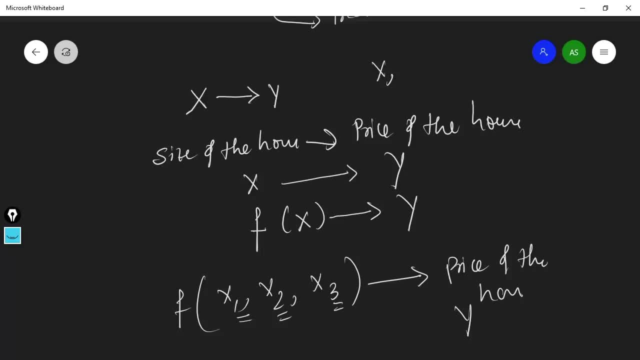 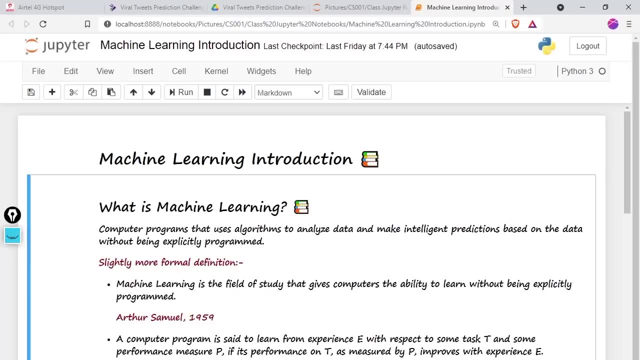 you're here and X's are the input features that you, that you want it to. basis of that, these are the input input features and the basis of that you want to predict the price. okay, the another definition of machine learning is the computer program is say to the 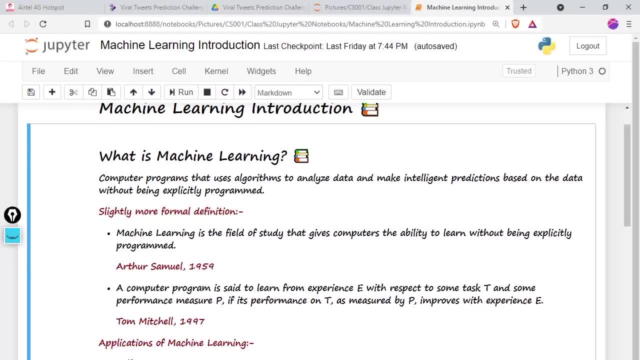 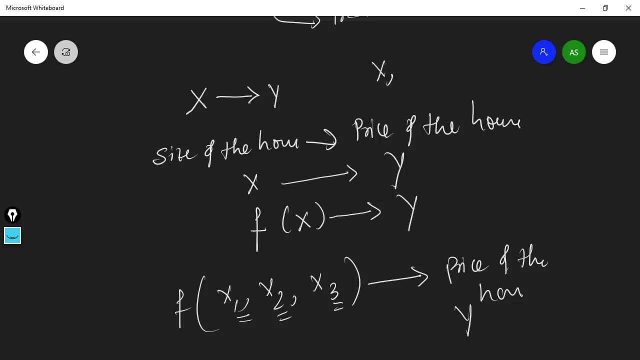 learn from the experience e with respect to the some class of a task, t, and some performance measure by p, if its performance on t as measured by p, improves with experience e. and this may seems a little bit intimidating, but let me clear this definition. it's very, uh, my, my favorite definition. 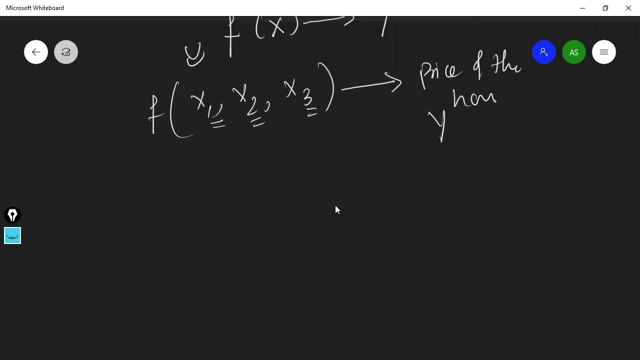 although this, this is my favorite definition that i've shown to you, but let me tell you what the definition tells you. the definition is so, before that, let me take one example, which is: uh, let's take an example of: uh, checkers. okay, playing checkers, playing checkers. i hope that you. no, no. 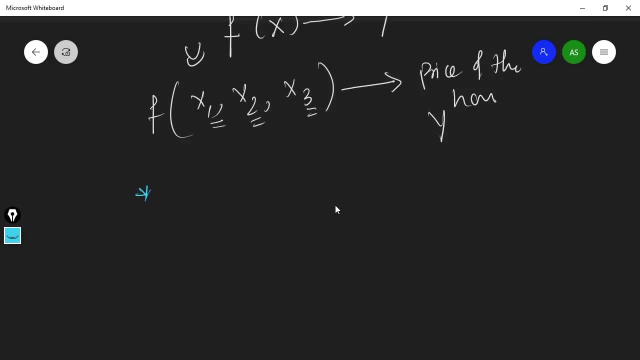 no, uh, let's, let's take another, because many other people do not play checkers over here. okay, so let's take a. a and email spam detection system: email spam detection detection system, which you will make in this course. yeah, you will make this course. you will make this into the course. okay, so this is a. 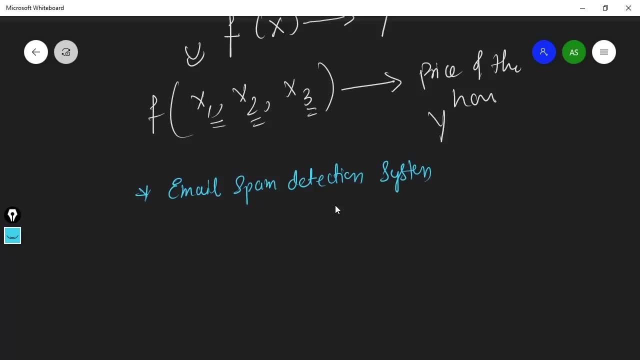 problem statement. and what's the? what's the? let's fit that definition onto this problem. here. t is the. detecting the emails means detecting whether the email is a spam or a not, so let's let's denote zero as detecting a spam or one as a uh. 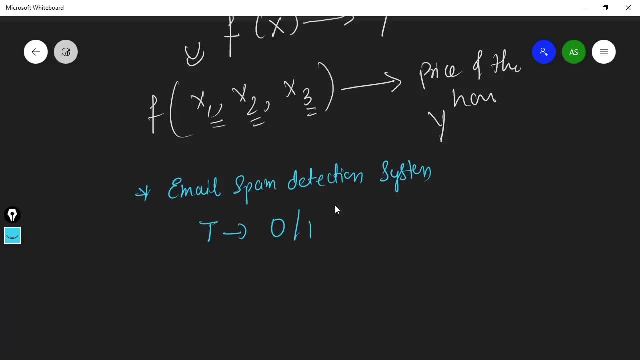 ham. okay. so let's say, let's say ham and e is the experience of this. prediction is the experience here, e is the experience of detection and p is the performance. how much performance increases upon to the experience. so in this way, higher the experiences, best uh system is. but i think this is more formally. 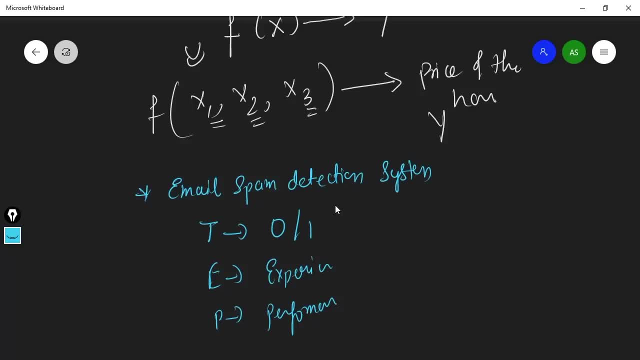 fit to something called a reinforcement learning, which will not see the advanced learning. but again, uh, e, a, p, q, ten, s. the definition which you have to take is: you wanted to make a function of function f that maps your input variables to the output variable, and that's machine learning. and or you can say: 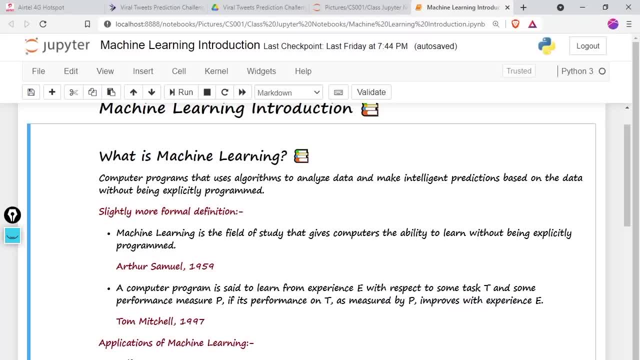 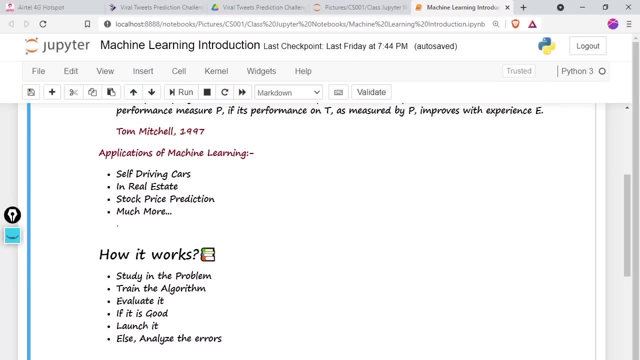 that's the beauty of machine learning. okay, so some of the applications of machine learning there is um, i've just listed on few, but there are a lot more: self-driving cars, real estate, stock price prediction in medical we have, or coven 19 detection, uh, maybe using chest radiographs. 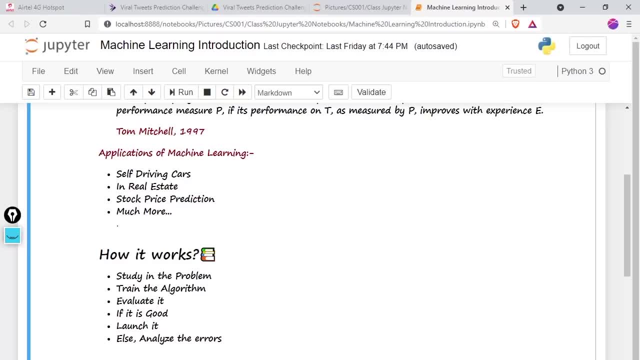 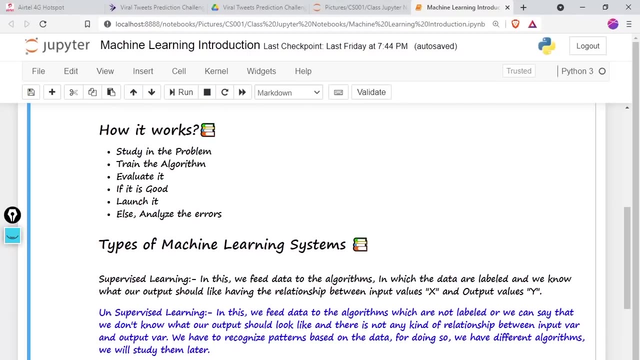 and then uh, disease prediction, cancer detection, etc. and then it's just a boom and i highly encourage people to get into this field and try to contribute to the world in a unique way. okay, so you can see how we had some, some of the applications of machine learning, so how it works. 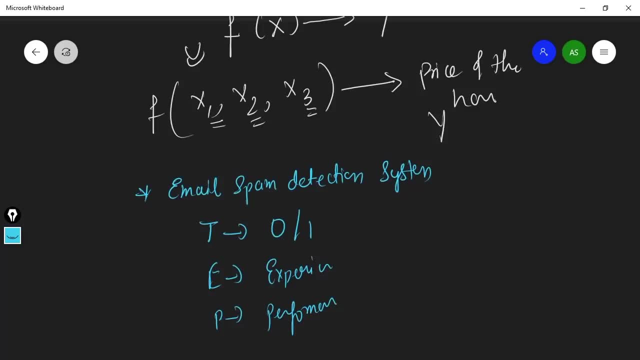 so what you do? uh, let me get to get back to my boat and how it actually works. so all this how it works, it's kind of a very easy how it works. uh, first you study a problem. so okay, let's, let's take in a problem. let's take a problem of again a spam detection. spam detection. 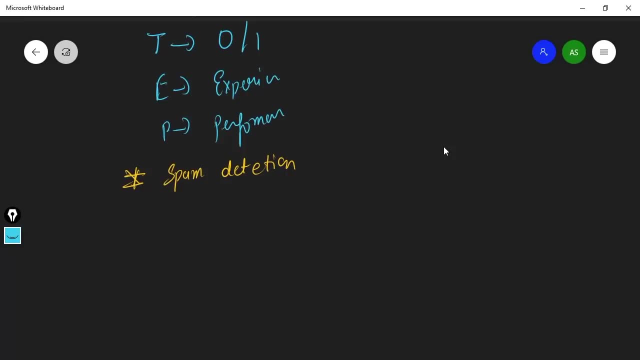 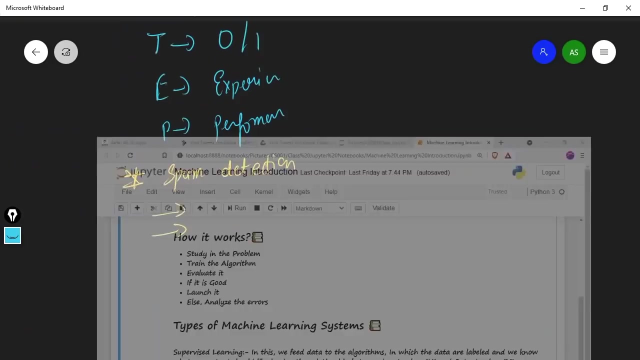 detection system. okay, i think the c okay, so to make a spam detection system. so first you study the problem. you have a look at the data. how much of the data is okay? so first you do this. the second thing is the basic workflow. the second thing, you train algorithm, and algorithm is just a function. it's just a function. 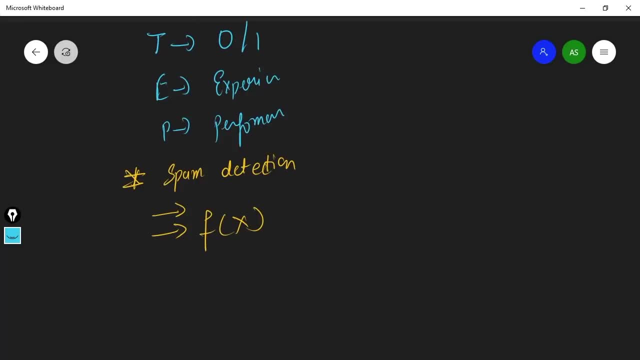 okay, f of X, which you will. how it is defined you will see later on, but you just have to have a function which is algorithm. this is, this is the algorithm, algorithm and you train with this algorithm and then you go further into evaluation. evaluation you evaluated into you give a new train, new emails and 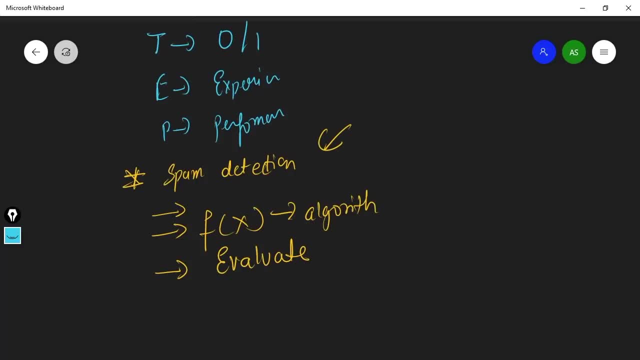 check for this correcting for correct or not, and then, if it is good, then you launch the system. then you launch the system, launch the system otherwise. otherwise you analyze some error, you do error analysis, you do error analysis and then you go further into tuning your, improving your algorithm or evaluating. 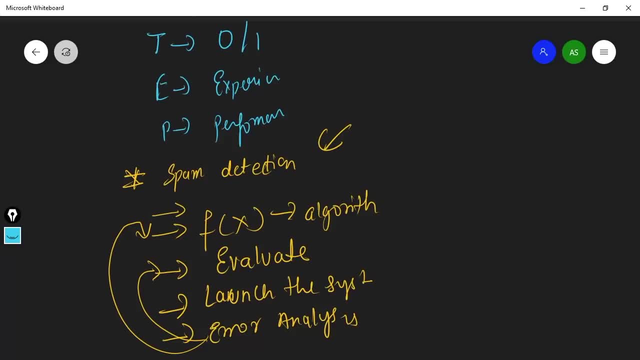 your and then you evaluate. then again, do that, do like this. so that's what machine learning is called. ML is very, very it iterative process. iterative process, which you will see in more in MLOops, why it is termed that. but but if beginner don't worry about it, okay. but 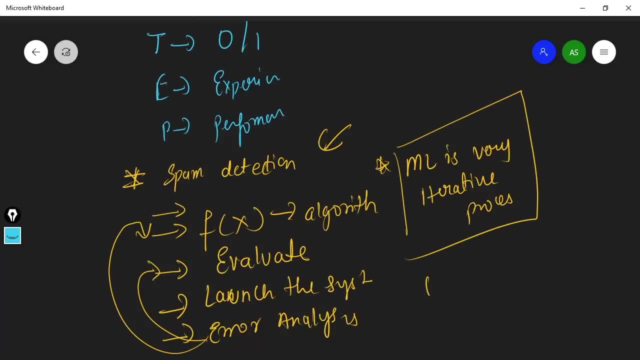 if you want to get it, after this course, you can get to my GANs course, or maybe the deep learning course, or maybe another course which is DSA, which we shall talk about, why it is very important, and then you can head over to the MLOops videos. okay, so this is the basic. you can. you can head over to that. 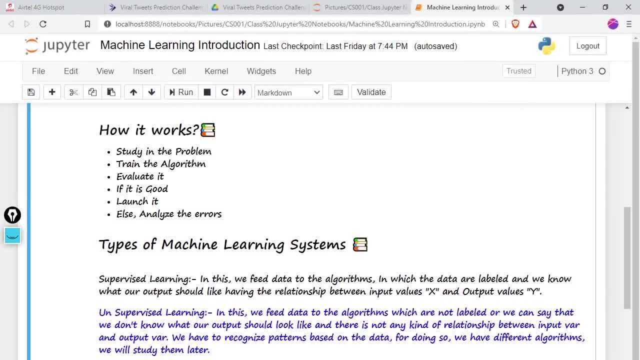 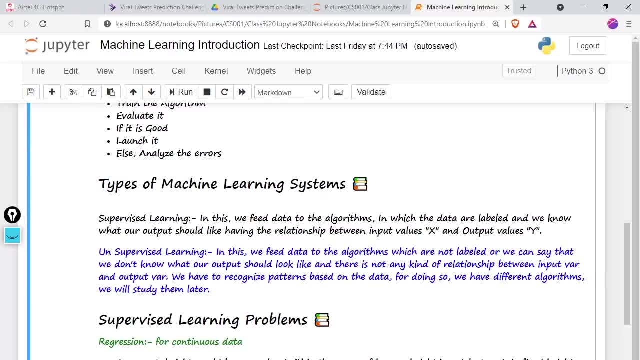 and learn something new from there. okay, so what are the types of machine learning systems? since there are, I think, three types of main main machine learning systems have three types: supervised, unsupervised, reinforcement learning and, although there is a few more, which is bash learning, transfer learning, active learning, passive. 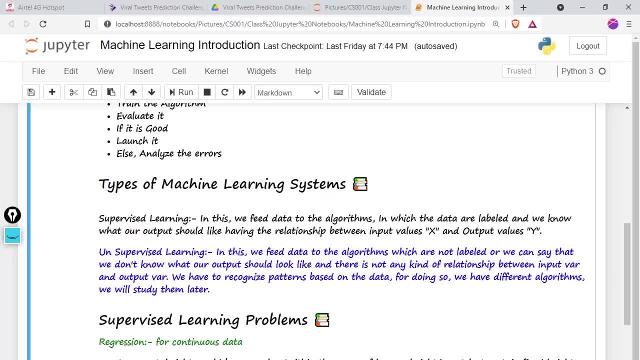 learning and so on, which you, which you can learn, obviously when you go further, know, when you go further means into more, into machine learning- then you will see that how you're learning these all and you learn a grasp, each and every concept. a few minutes, okay. so what I? 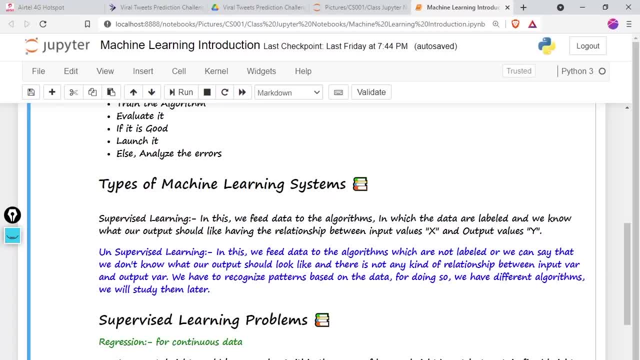 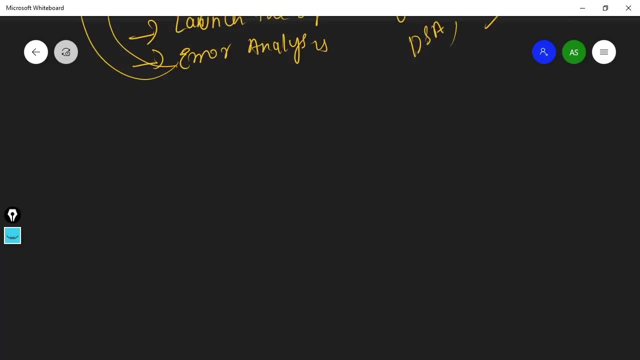 supervised learning. supervised learning- let's list. let's go get back to my boat again and let's take an example of another example which is my favorite. no, I'm not not my favorite, but yeah, that's a house price prediction. so I'm just reminded about the house prize prediction. prediction wrong, I just 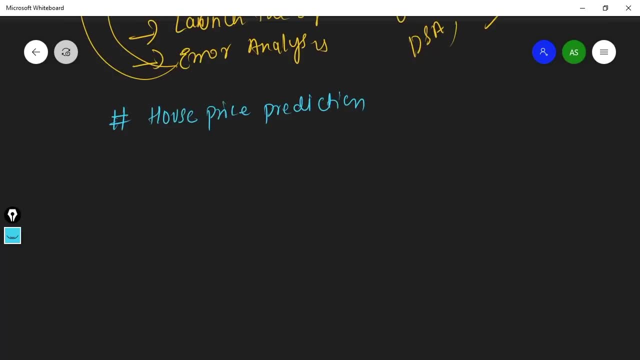 resistant. okay, this is a house price prediction. so you have a feature. let's, let's, let's denote that two on the bases of the size of the house. size of the house, and just taking example, because, and reveal all the size of the house plus the fan, number of fans in the house, number of our bedrooms in the house. on 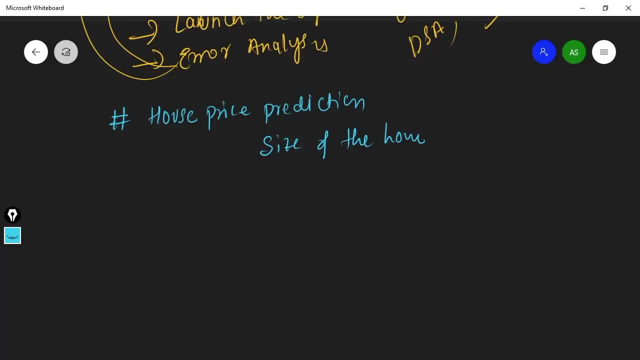 the basis of. but just for now, for predicting this, from the size of the house, you point the price of the house. you want to predict the price of the house, which is which we denote as a Y, and whatever we give, whatever we take as a feature, we 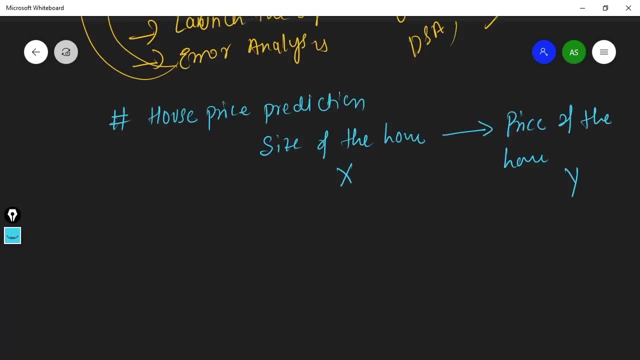 denote this as an X. okay, so there is. we denote there is only one, one feature, which is X 1, and only we are getting a 1 output, which is Y. okay, so we are. we provide X 1 means the size of the house and we are getting the price of the. 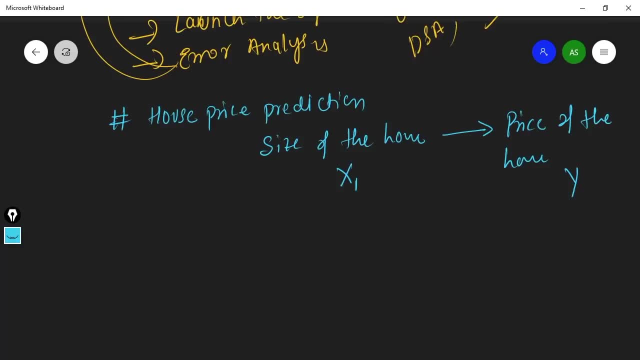 house as an output. okay, so you can see over here that we have size and we have a labeled means, we have given the price and the model can learn from this house. the trend is how's? the trend is on a. it can recognize patterns. okay, so you can. 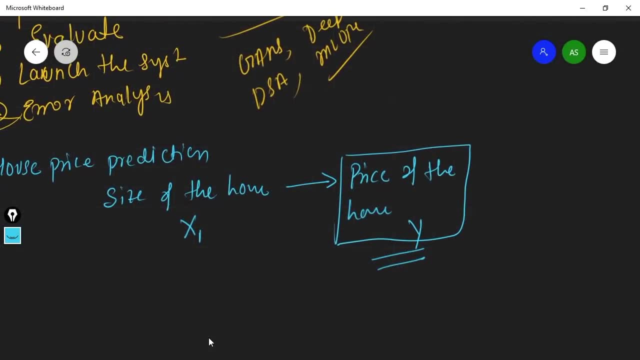 see over here that our data is labeled as a Y means we know what our output, so it learned from their label and input. that's called a supervised learning. how you can identify the problem is supervised because you see the target variable, which is called the target. this is called a target variable and this is 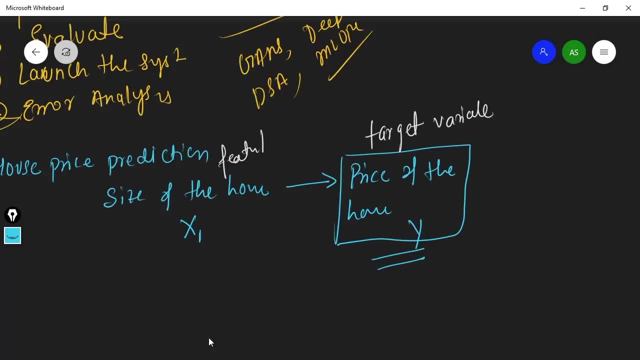 called features, features or variables, okay, and the one we want to predict is called the target variable. so we, this is the features or variable. so you see that there is a relationship between your input value X and output value Y, input value X and output value Y. what I'm saying, it has some 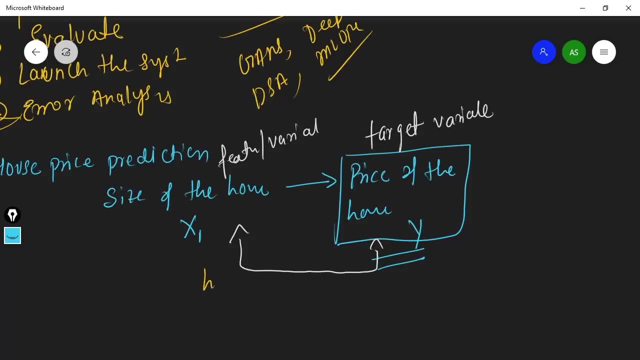 relationship because you can see over that we are given the size of the house and we will predict the price of house. so you can see over the entire ease that they have some kind of relationship and we know what our output should look like. in this case, we know what our output should look like. 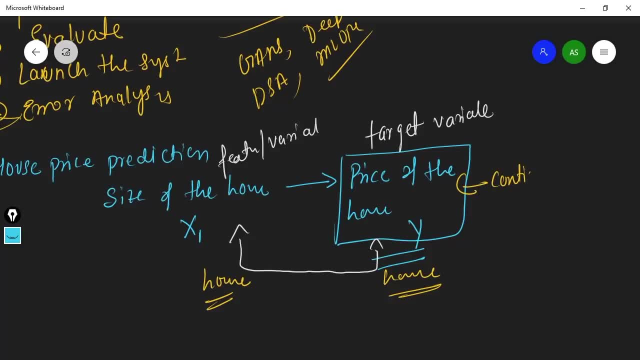 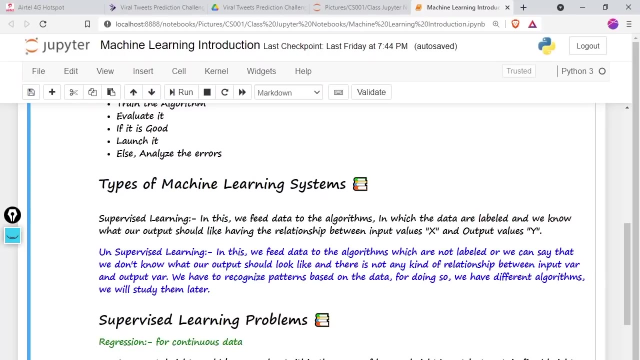 Derek's came back again sabah. Oh друг bennett. bennett, i think it's going good- means you're understanding what i'm saying. so in simple terms, you can see the definition of a hill. we feed the data and this- the data are labeled- means that the output variable. 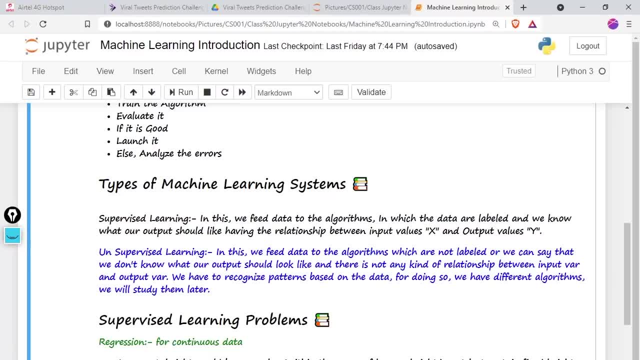 which we denote as a y are labeled and which we give, which has some relationship between our input value x and the output value y. okay, so, in the unsupervised learning, uh, which which i'm not going to go dig dive just now and further i will, i will be digging dive into this. so we, the data, 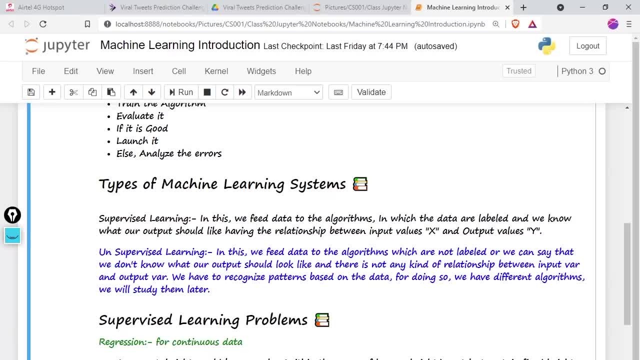 are not labeled and we can say that we don't know what our output should look like and there is not kind of any relationship between what are what will be our input variable and what will be our output variable and we have to recognize our patterns based on the data. for doing so we have 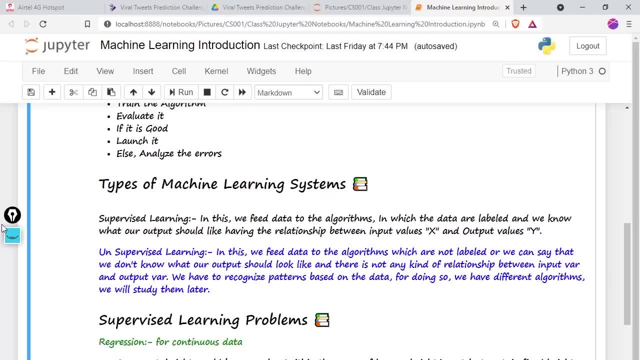 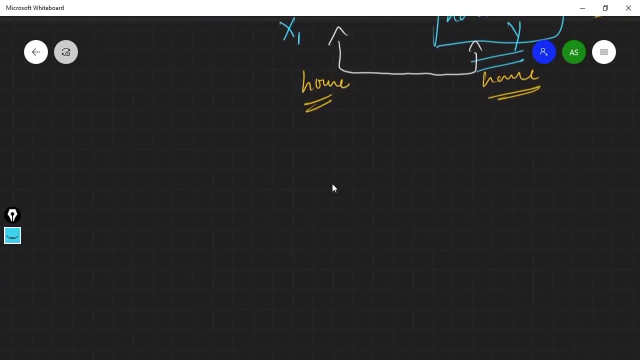 different algorithm, which we'll study later. okay, so i'm just um, not digging, digging type, but in simple terms, uh, but in simple terms, what i what i'm saying, that let me tell you what i'm, what i'm saying, okay. so, uh, let's say you this: these are the t-shirt sizing you want to you have a different, different? 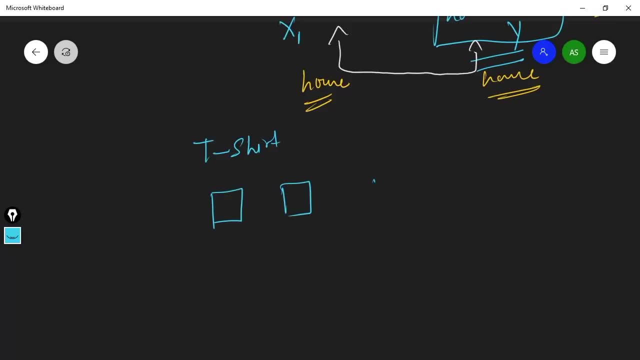 t-shirts and denoting this as t-shirts. so we have a different, different t-shirt and what and super, and this is our data. this is our data and you have to. uh, then you have to simply classify or cluster it up. so what i what your model will do? it simply make this as a l, it simply makes this as xl. 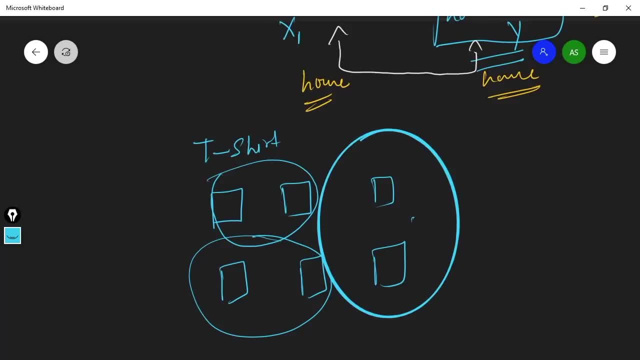 and simply makes as a m okay, so it's just a make clusters. it makes cluster xl and l and for now i don't recommend to brainstorming these things because we will. first we have to understand fully supervised learning, then it will most much clear: uh, unsupervised learning. so i don't want to dig dive into unsupervised learning for now. 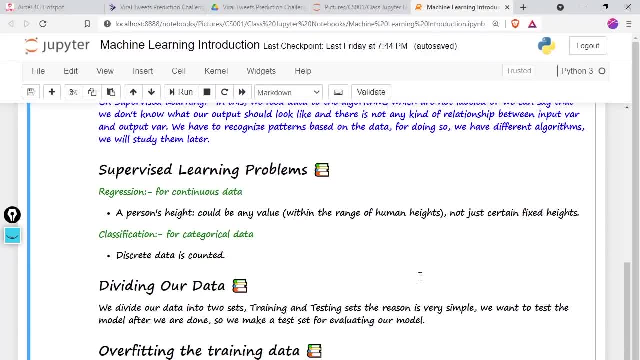 but you can see what the definitions are cut to cut okay. so let's say, let's keep that deep diving into supervised learning. so what are supervised learning? so in supervised learning, um, we know our output variable and input variable, etc. that's what we're going to talk about in this video. so let's. 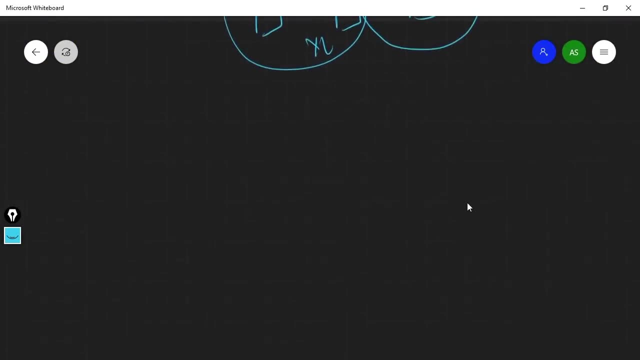 uh, that i would just explain your house press prediction. so in supervised learning we have two types of problems. the problems of supervised learning can be classified into two types. so let me write it: a supervised learning problem. supervised learning problem can be classified into regression problem, regression problem and it can be classified into classification problem. 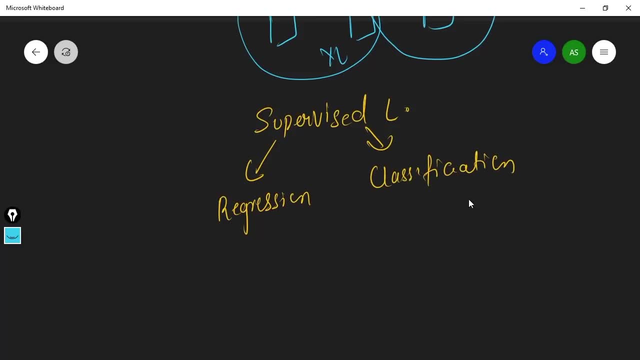 classification problem. okay, so let's keep talking about what is regression, what is classification? so i'm going to take take one example, which is a house price prediction. which is a house price prediction means house price prediction and we can see over here that our output will be in continuous value because super supervised learning and we know what our output is. 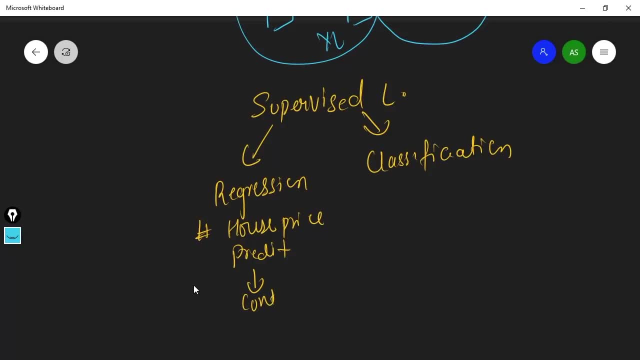 so you can see over that, output will be in continuous value, continuous value. okay, so your output is is in continuous value and in classification. and in classification, uh, let's say, given a picture, x means the often- uh, you want to classify an image of a picture as a cat or a non-cat, or a non-cat. 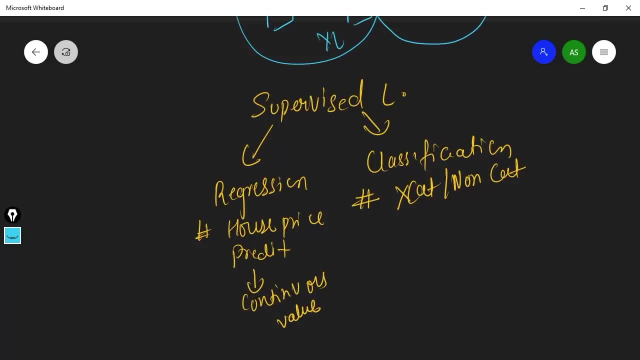 okay. so, um, you're gonna picture x. um, you wanted to uh identify that as a cat or non-cat. okay, so you can see over. that is a binary, it is only two. it is. it is a. it is called a decreed value. decreed value means we can now classify that in regression if our output of the problem is in. 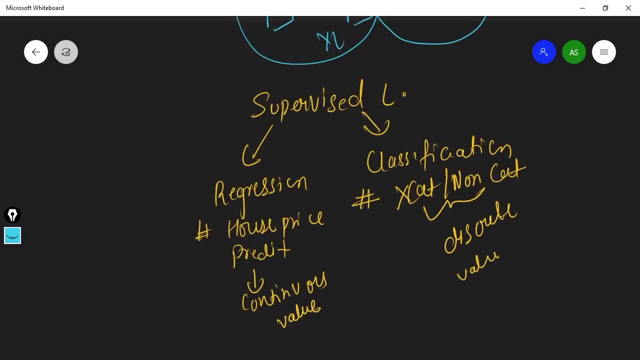 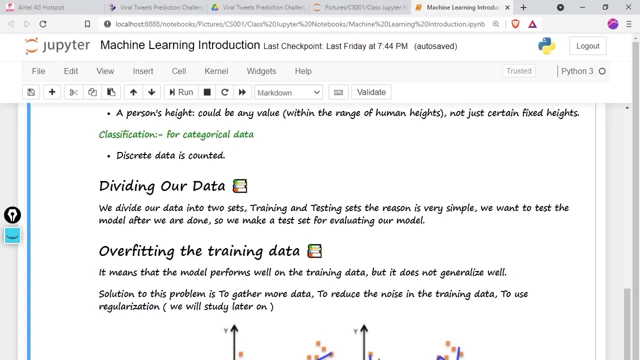 continuous value, that's called that's, that's, that's. that is a regression problem. if our output of the particular problem is a decreed value, we can classify that as a classification problem, and you can see over here: the definition is the same, okay, okay, so why we need to divide our data. so 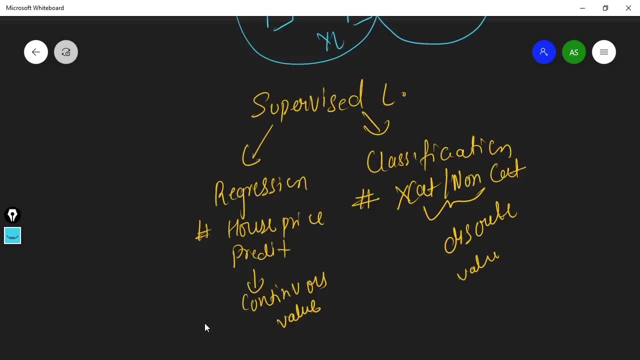 let's let let me talk about- because i'm talking too much about- data. but what is data? that's this question arise. a very good question that i want to ask by myself is data, are the they? how does data looks like um in data? let's do, let's take an example of an application, uh, system. that is a. 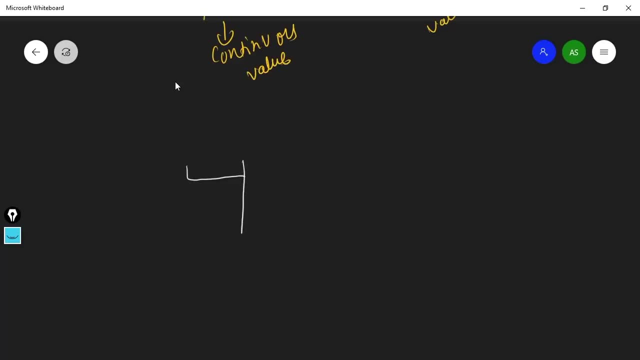 price of the house. uh, house price predictor. okay, so the data will look like this. so i'm just just making a data frame. so you have a size of the house, then you have a number of fans, then you have a number of bedrooms, then then it's the target. 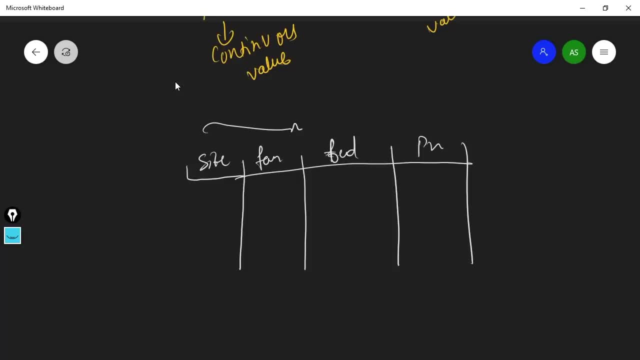 variable, which is the price. so these are your x, these are your x and this is your y. okay, and what you do? uh, let's, let's take nine square feet, two to twenty two. i'm just taking as a thousand, et cetera, just a thousand dollar, i'm just taking as an example. don't think that is a nine, it's a nine. 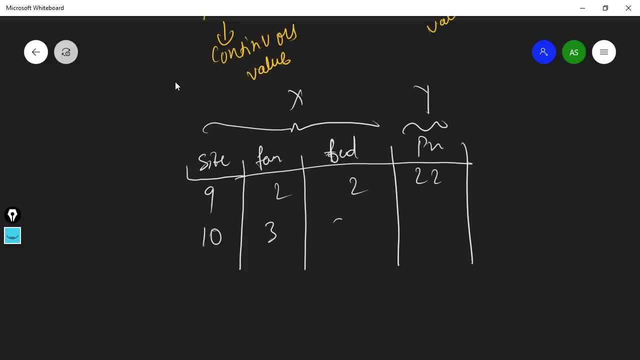 square feet size of the house. don't, don't think like that. okay, so, uh, this, this is the kind of thing. and so this, this is kind of thing, and we have a size and we have a number of fans, we have a number of bedrooms, okay, so, uh, what you do? uh, here, you can see over here that we have a. 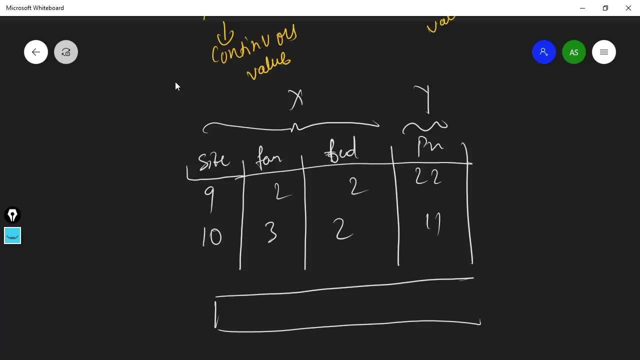 data. we have your data and what you do. you divide your data into training, into training and testing set, into test, training and testing set. so let's say you have a hundred percent of data. you take a hundred percent of a data for testing. the reason why you take this to evaluate your model? because 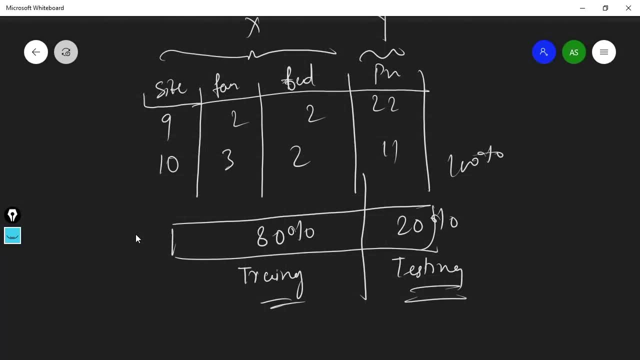 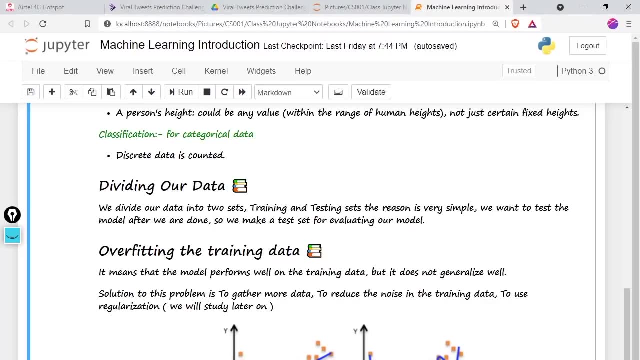 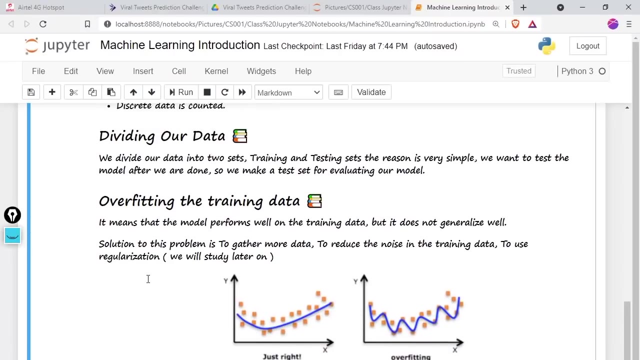 you from here you will get all those uh for testing, so you just keep 20- 20 for evaluating, to check how, how best your model is. okay, so this is the deviation of the data, which you'll see more later on. okay, so there are two problems that i want to highlight. is uh overfitting and under. 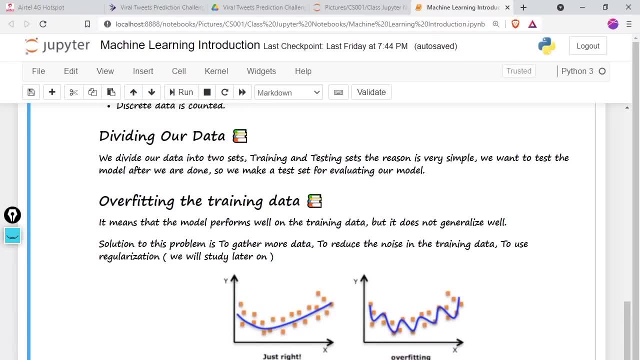 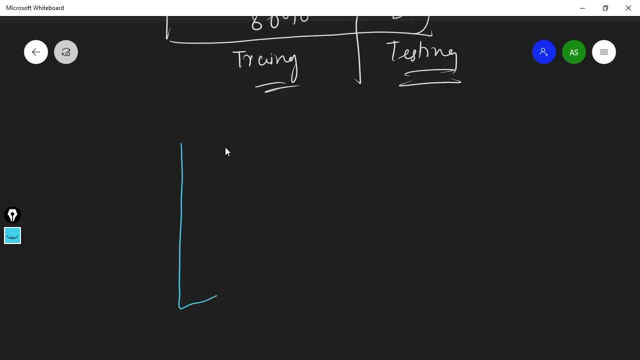 fitting, okay. so what is overfitting? so let's take an example again. i just, i, just, i just believe in, okay, so here is your x and y plane. i hope that everyone remembers in in in their school days: oops, what has happened? i hope that i draw incorrectly. okay, so you have this. 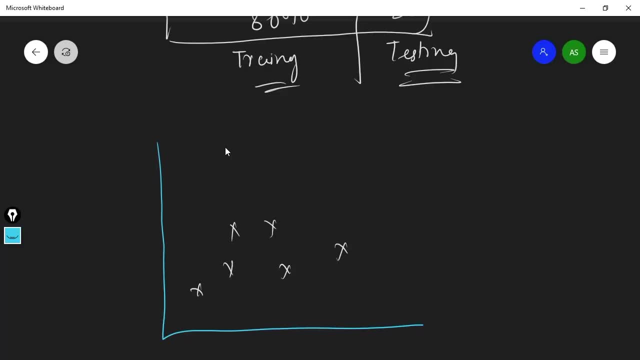 uh, these features. let me draw it very quickly. these are your data points and what you do? you simply draw a straight line. you simply draw a straight line to make predictions. okay, so let's, this is your input, which is x, so it's a 2200 square feet. 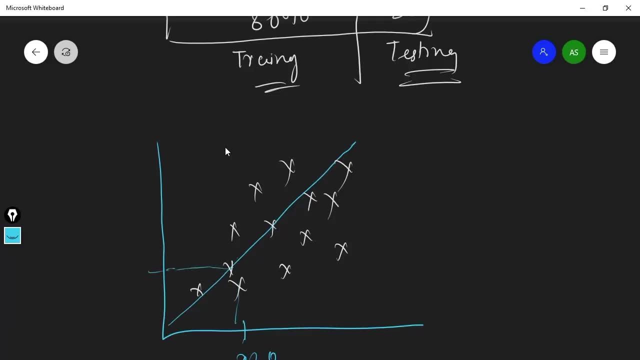 So it will go over here and check what is the price, so it will give here: Okay, so like that, it will make prediction which you'll see later on, so you can see over here that In under fitting and under fitting and under fitting, what happens if your model, if your model has not performed. 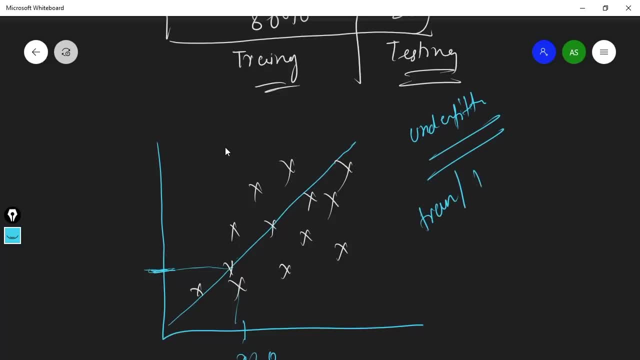 well under the training data as well as when testing data means in under fitting, your model does not perform well under training and the testing data Means your model is performs bad under training and the testing data. It means because you don't have a large number of in a large number for data. 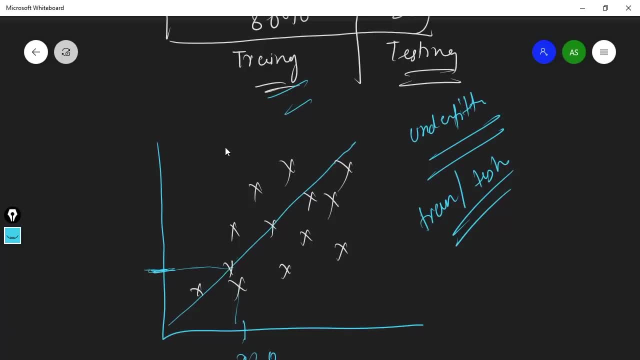 You can. you can simply add more data, Okay, but what happens in under fitting? and then you will tell me what happens in under fitting. So let me highlight this little bit. Let me So in under fitting. if your model has learned too much, This is because when you have too much of features, 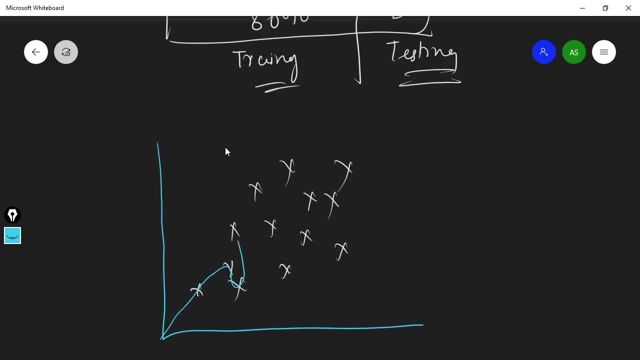 So let's say your, it will try to touch each and every point. It will try to touch each and every point and This is called. then you can see if you, if you have a, if your model learn too much and it is generalizing very, very well. 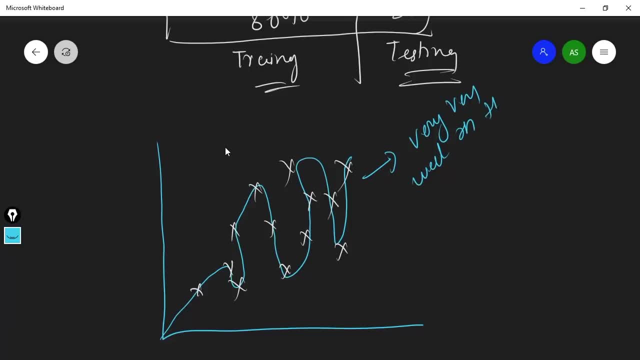 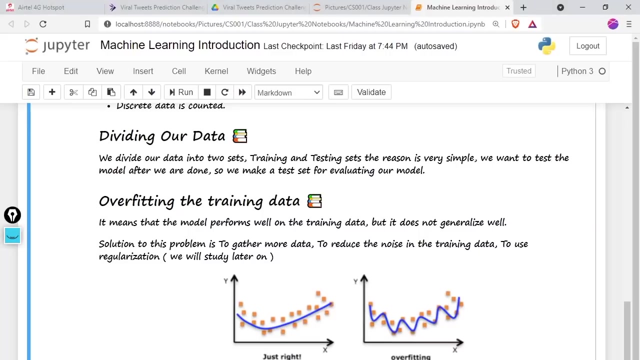 Very, very well on to the training data, on the training data, but it fails to generalize well. Fails to generalize well on testing data, Testing data. then you can say that your model is overfitting. Okay, so you can see over here that that diagram is over here. 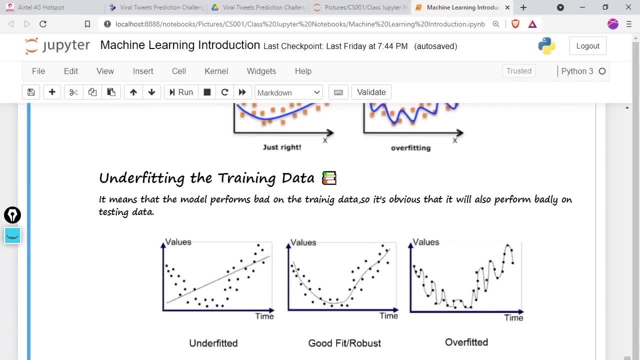 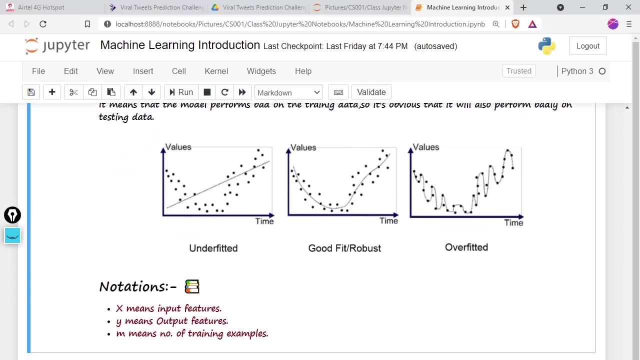 And you can see over that, on under fitting which you does does not fit a straight line, a very good way and good fit, It's good, good, good model. You can just fit a straight line and in a bad fit, over fit it. Okay, so the solutions of this, which you'll see later on, but before that we'll touch some algorithms and again, some notations. 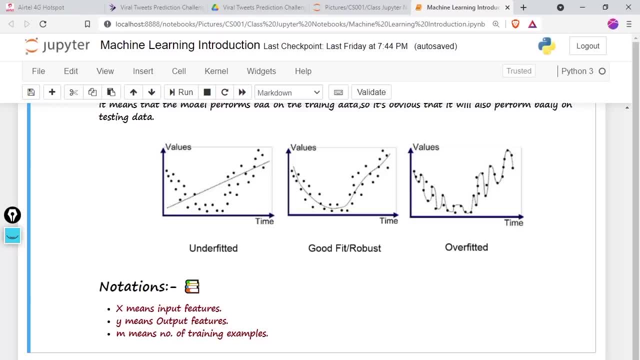 Which I've already taught you. X is the input features, X 1, X, 2, all the way down to the X n, Y means the output features, M means the number for training examples, and here let's a 600 training example Which you will get to. 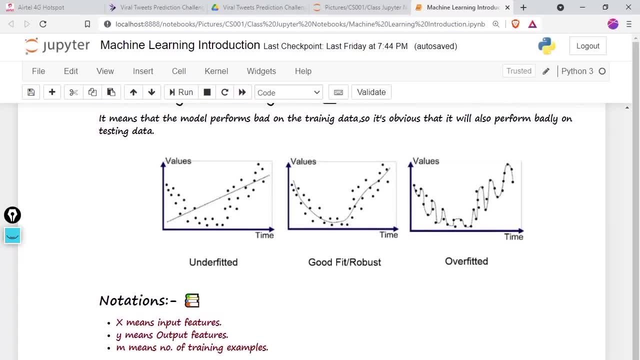 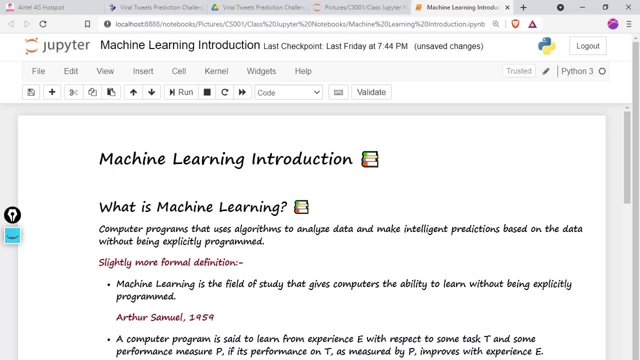 Know more for the which when, when we will go more further into this course. Okay, so now you're done with this introduction of machine learning and I really hope that you enjoyed this tutorial, and in the next section, We'll be talking about one of the algorithm, which is linear regression, and I hope that you will really enjoy that. 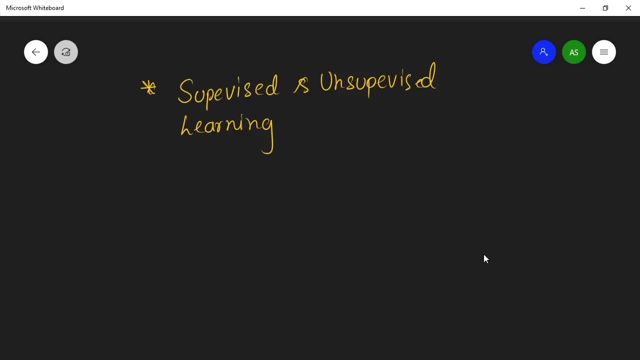 So let's meet at the next section. Okay, so now we will briefly talk about supervised and unsupervised learning, with Adaptation and some cases, studies and data Set, so to fully understand what happens in supervised and unsupervised learning. Okay, so let's start. 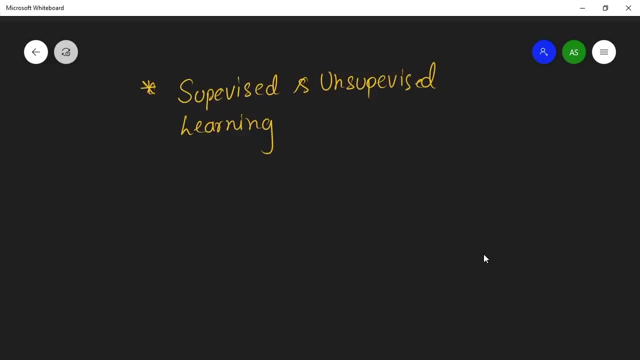 so What happens in supervised learning and supervised learning, as the names are guessed, Someone is supervising over here. I will take an example of a data set to help you understand better. Okay, so in supervised learning, What I have told you in the in the previous section is wrote in machine learning that you in in supervised learning. 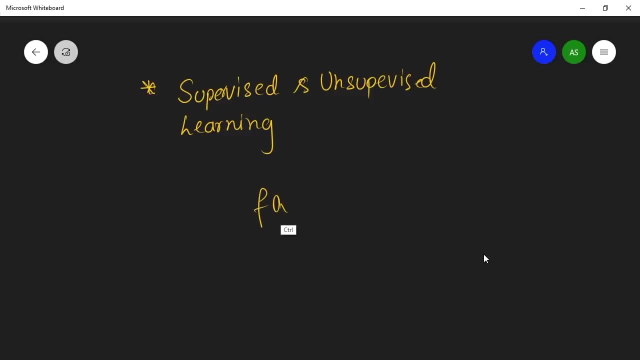 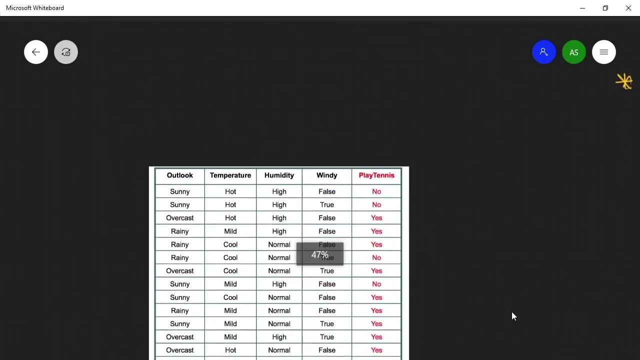 We make a function f of X that Maps your input variable To the output variable. okay, So here in supervised learning We have the input date up, input data as well as the output data. Okay means here as an example, that we have this data set, We have this data said. just assume that we have this data set and here we have this out. look feature. 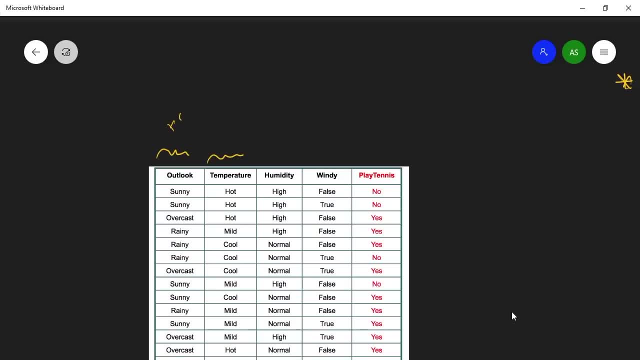 feature. temperature feature means x1, x2, then we have a humidity as x3, windy as x4. okay, and here this, the red one, play tennis. so here is our problem: statement is given on these features: outlook, temperature and humidity and windy. we have to predict whether the whether that boy will play. 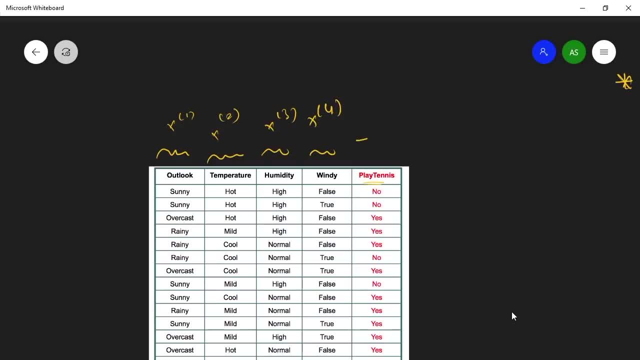 tennis or not? okay, so this is your target variable, this is your target variable. or or the variable that you want to predict. okay, this is the target variable, or the variable that we wanted to predict, that we want to predict, so it is given in this case. so it is given in this case. so here we have. 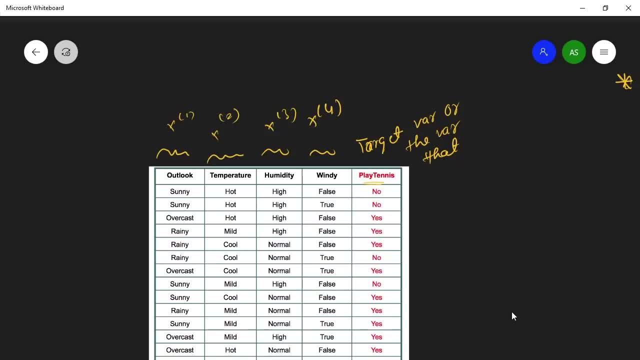 our x variable as well as y variable, as well as the y, okay, as well as the y variable. okay, so we're going to make a function f of x using this data that maps our input value, all these features, x1, all the way on the x4, uh, to our y variable. okay, so we'll give input whether. 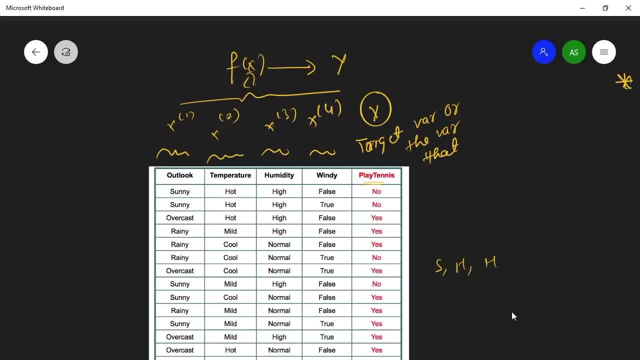 it is sunny, or whether hot or high or false, and given on this feature, the function will give you output, whether it will play no or yes. okay so here- and this is a superman's learning problem- because we have our, so we have our labels, which you can see over here. okay so, and you can also see that we have a some kind of relationship. 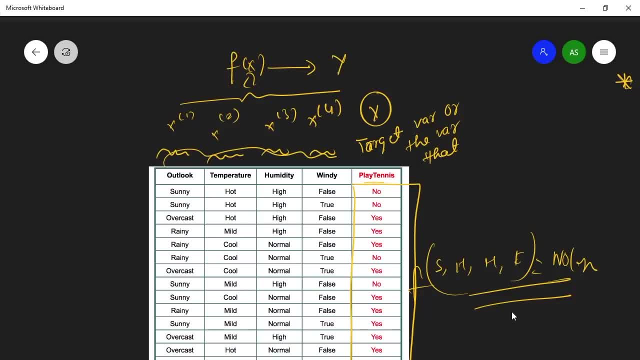 between our input value and our output value, y. as you can see that and these- uh, there is there is some kind of relationship, like a male stylistic example of house price prediction. so, given an input feature size, you want to predict the price of the house, of the house of the house. so it is on. 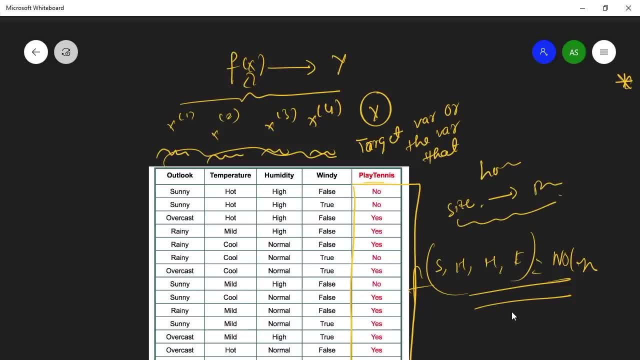 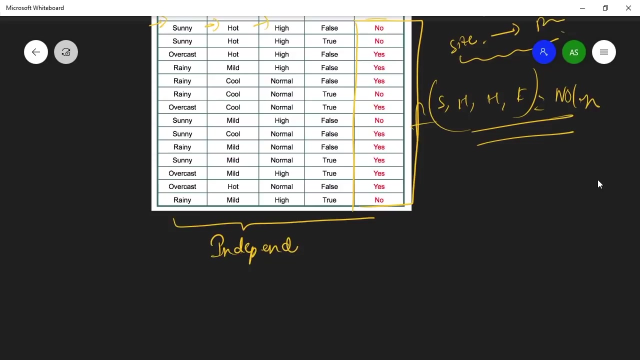 a shame name. so there is a some kind of relationship between our input feature x, output feature y. okay, another another property of supervised learning is that these features, which are input features, are co, are independent features, are independent features, are independent independent features. what do i mean by independent features? they do not have to depend on any and any feature. 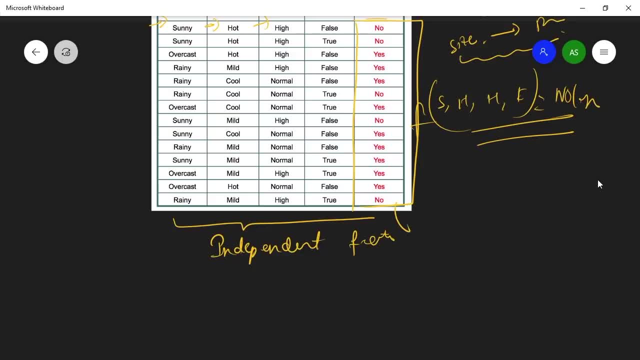 they don't don't have to depend on any feature. but this target variable y is dependent feature because the target of y is depending on these features. it's depending on these features to be mapped and the is depending on these features. so that's why x 1. 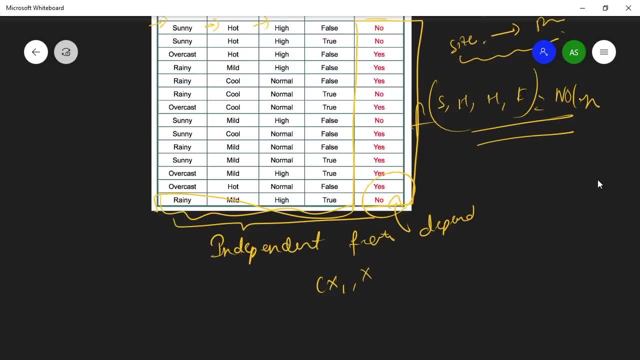 x 1, x 1 all the way around to the x. i i equals to 1 all the way around to the k means x, 1, x 2, x, 3, x, 4 is a independent feature which equal usually gets indian independent variable or feature and y is your dependent variable or feature. okay, so that's it. 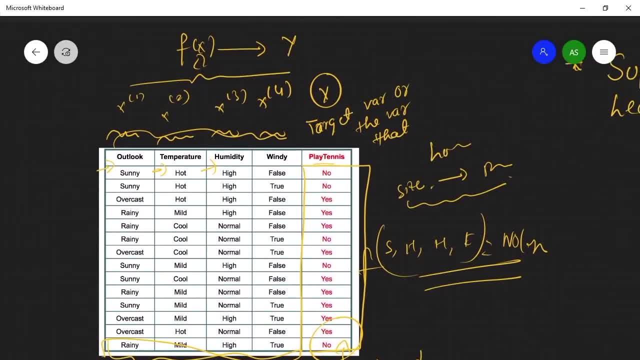 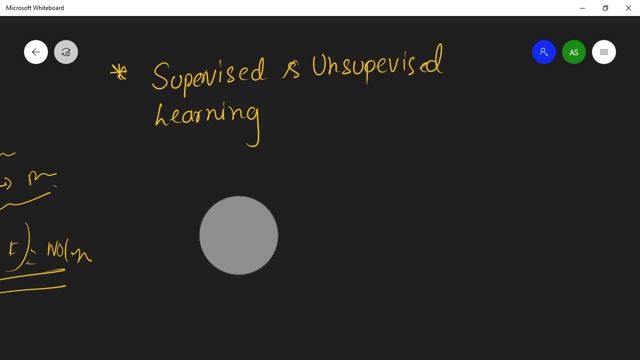 the, that's, that's called the features, the supervised learning. so let's, so let's. let me write a basic definition, or a good definition, of supervised learning. what, what is supervised learning? a good definition, okay, so the good definition of supervised learning is here. in supervised learning we have, we have our 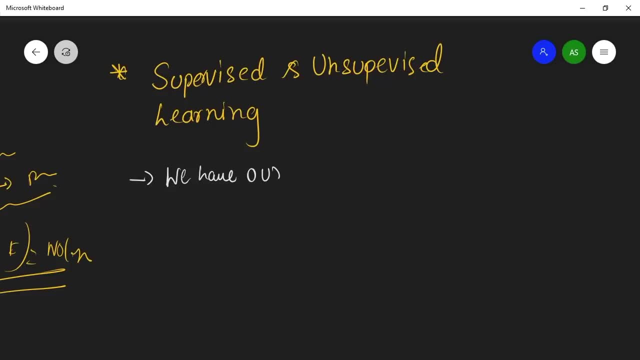 input features X. we have our input. we have our input features X. we have our input feature X, large X. and just assume that X, large X is contains all features in a vector, all that under the X I, okay, okay, so we have input, if you have our. 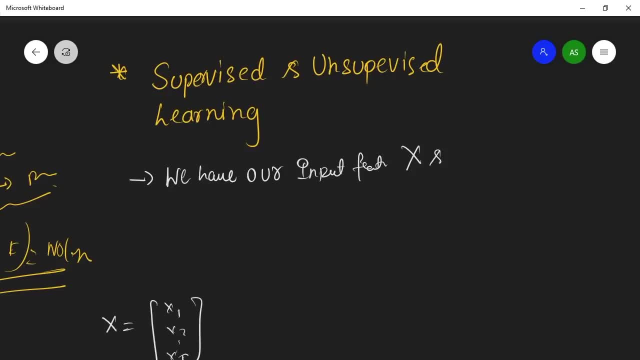 input feature X, and also we have our output feature Y, we have our output feature Y, output feature Y, Y, and there is some kind of there is some kind of a relationship, some kind of relationship, you you, between the input value X and output value Y, and and x is called. 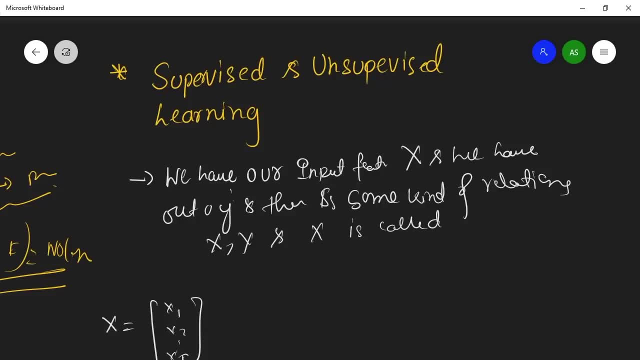 independent feature. xx features are called independent feature and Y is the dependent feature because it is dependent on: do the input features? okay, so we have seen you, so shown you an example, that there is a Y. there is a Y that is used to train using X. okay, does that using X and Y? 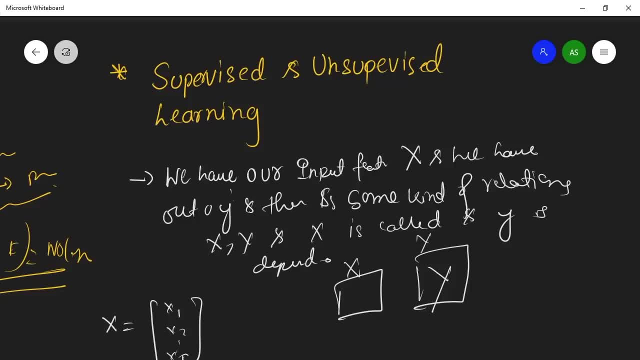 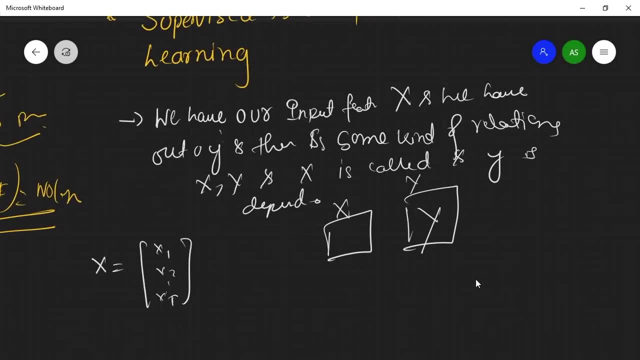 So we'll be able to predict our model. So we will see in the next section how we make a predictive model as a part of linear regression. So let's see some of the so. but before that I want to. I wanted to just show you that there are two parts of supervised learning. 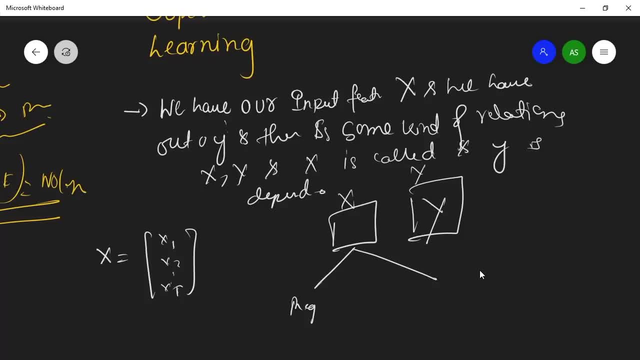 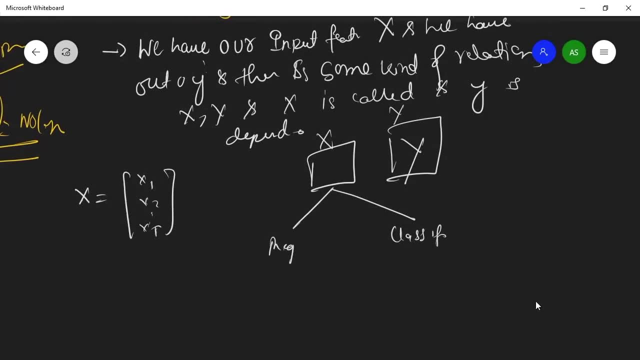 First one is a regression. Second one is classification- classification. So what do I mean by regression? You know what your output will look like, because here we know that, what our output, because we have already seen our data, So you can see the output is in decreed value. 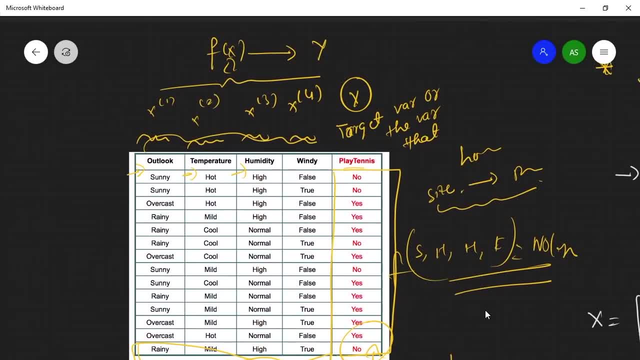 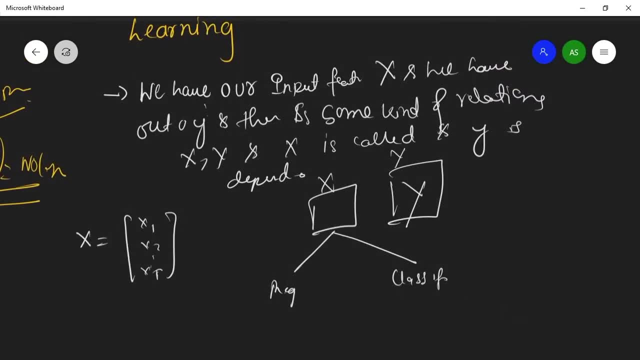 What do I mean by decreed value? Your output is in finite means. either it will be yes or no. So here, if it is in decreed value, if you know that your output is in decreed value, then you, then you, then you consider that as a classification problem. 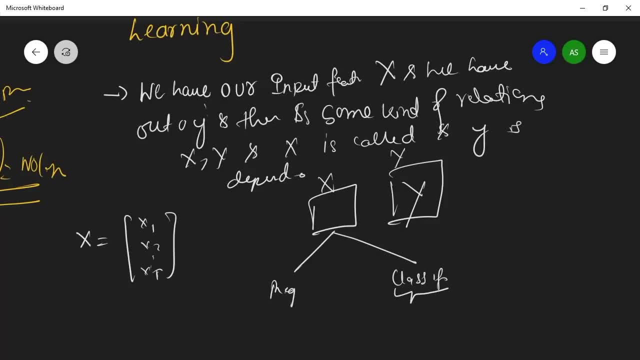 How you identify. that is a classification problem. when your output is in decreed value And when your output is in continuous value means it's not finite. maybe the age of the person, maybe the stock prices, that is a that is continuous, OK. so that's why if your output is in continuous, then it's a regression. 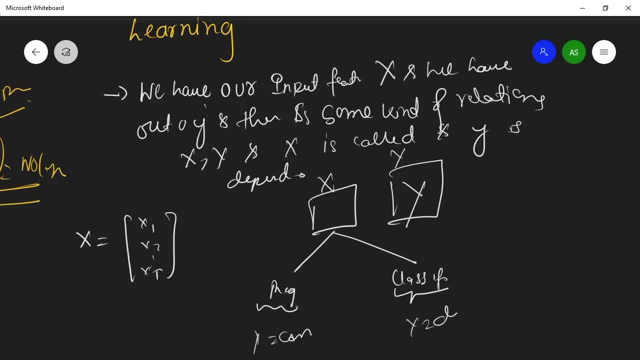 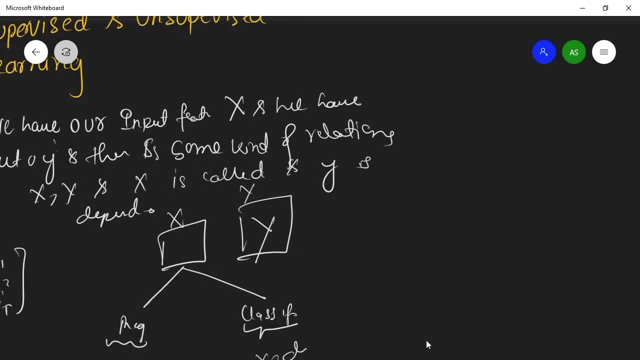 If your output is decreed, then it's a classification, OK. so let's see some of the applications of supervised learning to help you understand more, better, to get the feel of supervised learning. So in supervised learning we have Our favorite and supervised learning. 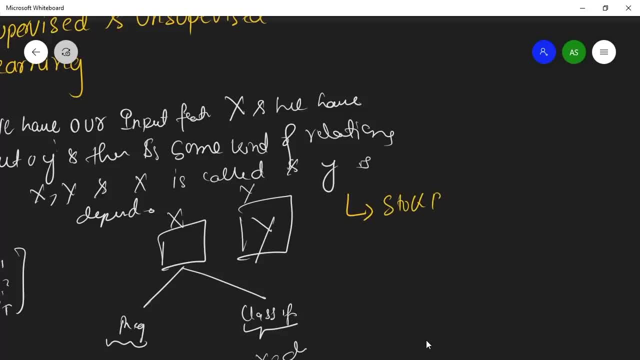 We have maybe the stock price prediction. stock price prediction We are. you are given closing price high, closing high, then et cetera, maybe some volume and predict what is the stock price and maybe the you want to predict this. You can consider C, close as a target variable going to predict what? what will the closing price basis on high and volume? 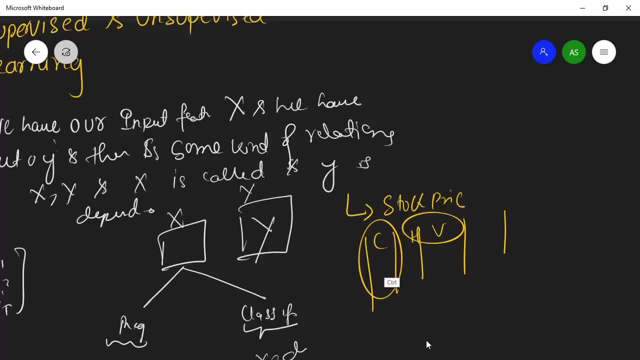 OK, so high and volume are your independent feature and C equals C will be your independent feature. It will be the Y. next is maybe the house price prediction. Maybe you want to basis on the size. like that You want to predict what will be the output. Y, and maybe that's the example of a classification problem giving you want to identify whether the person has a diabetes or not. 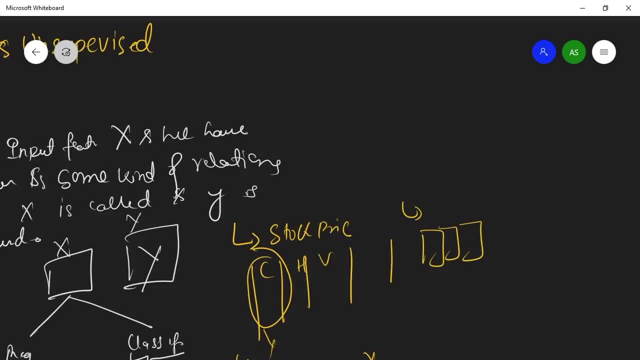 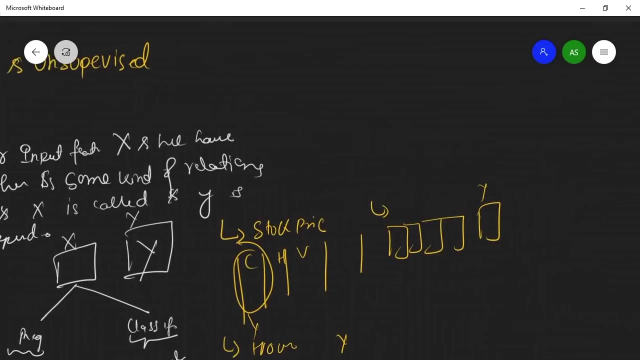 Basis on maybe the age, gender, BMI, et cetera. OK, so we have this output of Y. OK, so these are some of the applications of unsupervised- Sorry, supervised- learning. OK, so now let's see unsupervised learning. as I'm not going to go deep dive into this unsupervised learning, 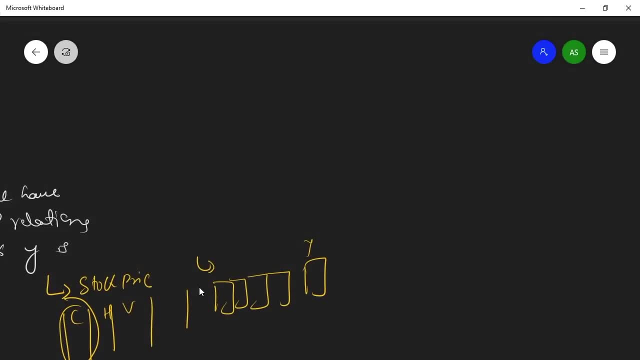 There is a next section, that there is a particular section of a supervised learning. We'll cover the in-depth about unsupervised learning. But the core idea behind unsupervised learning that in this case in supervised learning, we are given XI as well as YI, for for each, for every, I equals to one. 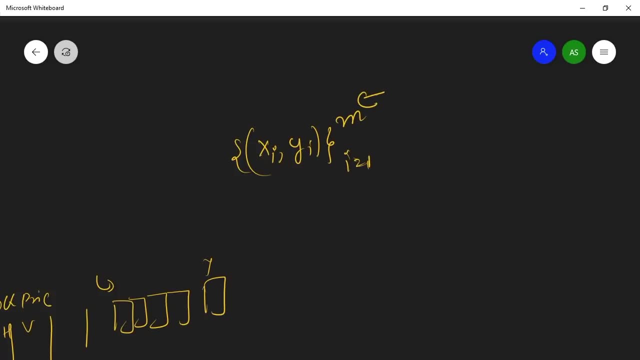 All the way down to the M And M. here is the number of training examples. OK, so that's it, And here is the means we have, for we are given. I, OK, so here, in super supervised learning and supervised learning, we have this in unsupervised learning, the unsupervised learning. 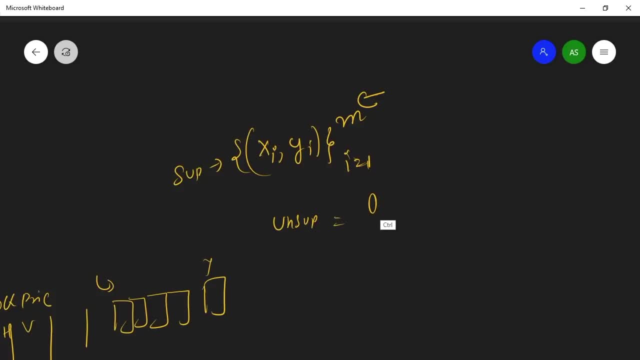 We have only XI's. We have only XI's. We don't have YI's, We have only XI. We have X1,, X2, X3, all the way down to the XM. OK, we don't have the label YI. 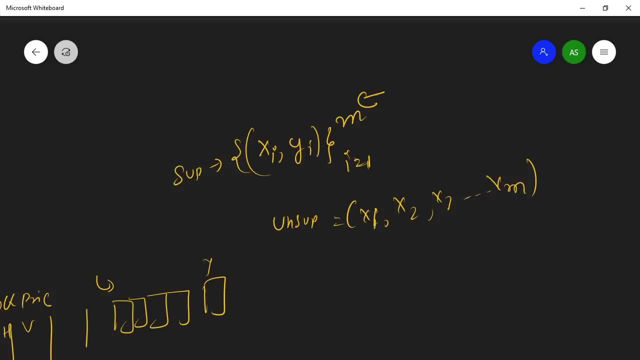 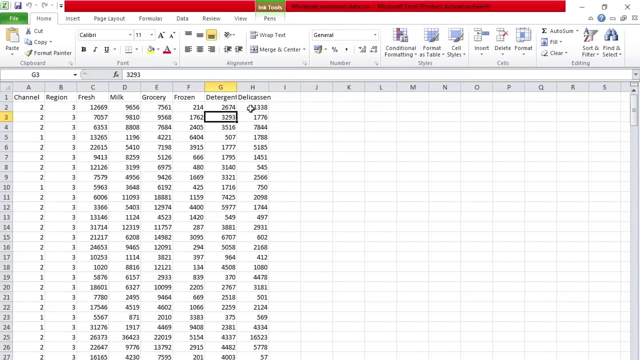 There is no supervisor that will guide you, OK, and what you have to do. let's take an example. You have, you have this, So here is your data set. So here you have a channel reason: fresh milk, a grocery frozen detergent and and that is gasoline. 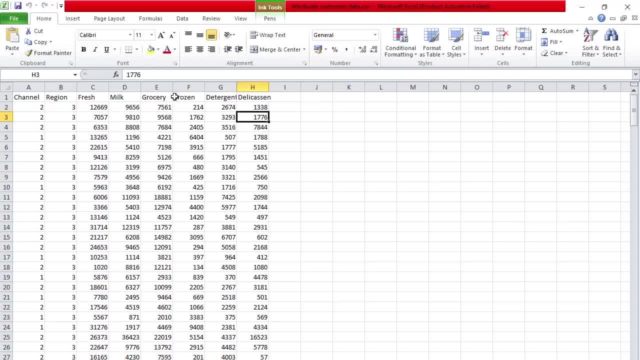 So let's take an example- that unsupervised learning is used in markets, market segmentation, segmenting your customers. So you have these features and you don't have the weather, The person with You, what you do, you just cluster the person which has similar nature you have. 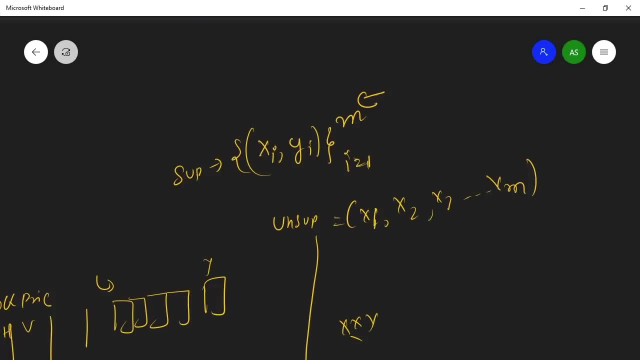 You just cluster the person. Let's take an example that these person use used to eat milk. these person used to that. So you cluster this out. you cluster this out, OK, then you can hand code it. OK, these person used to eat meals and then you can send promotion to these people or big deal another thing to these people. 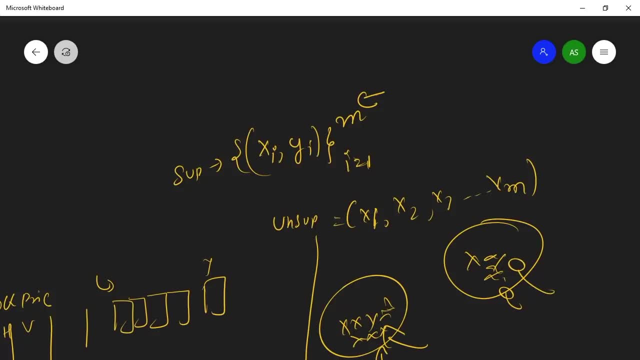 So you can identify your business needs et cetera, from these clusters either. I'm not going to give deep dive- I've been to the application et cetera- but I will go deep dive into the application, everything. 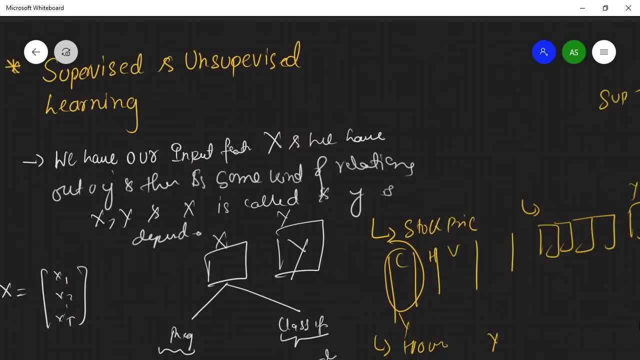 But as of now, I hope that you understood supervised learning in that. OK, so that's it for this, Just a small video on supervised learning and unsupervised learning, And the next section will be starting with actually the math, and then we'll dive into the machine learning. 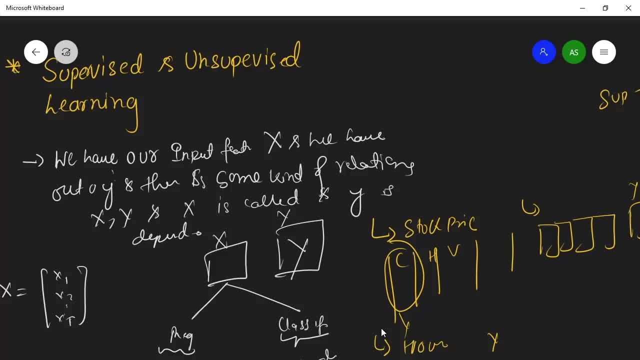 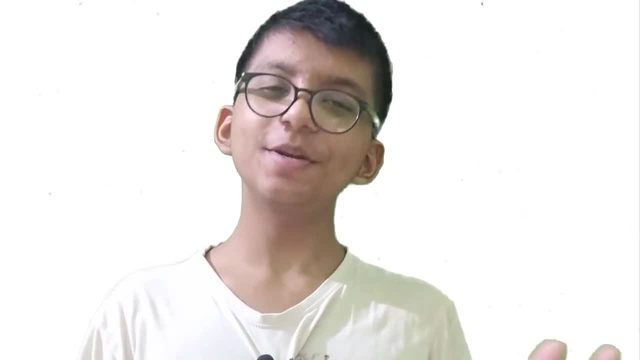 The beauty of you will see the beauty of machine learning. OK, so let's meet at the next section. Till then, do the problem sets. So now we have seen an introduction to machine learning And I hope that You had really enjoyed that section. 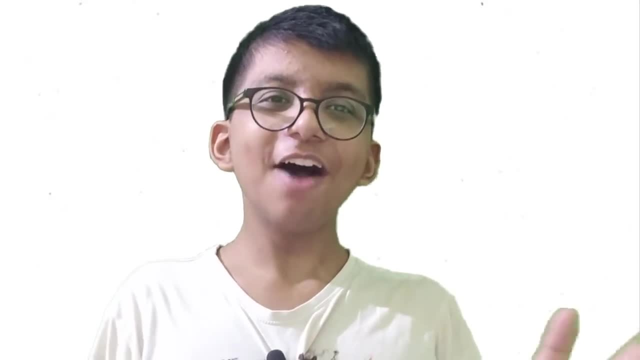 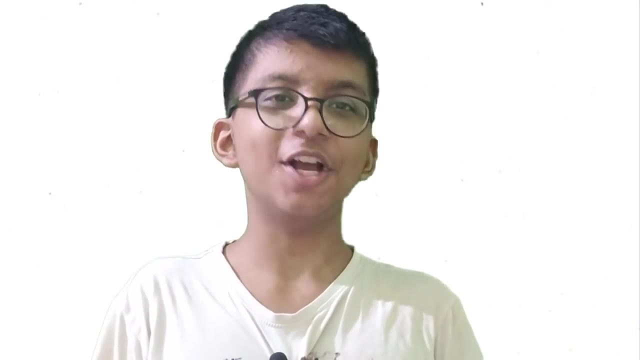 Now it's time for getting the hands- you are dirty- into the maths. Now we will see some learning algorithms, which is linear regression, And then we'll do one project, which is Boston hotspots prediction. So I guess I'm very excited to have your first learning algorithm in a toolkit. 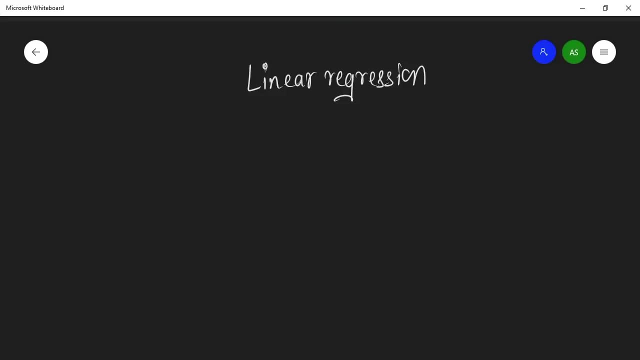 So head over to the next session. OK, so now we will see one algorithm, which is a linear regression, which is a learning algorithm. as in the previous section We have seen a machine Learning and an introduction to machine learning. Now we will see how to make that function. f of X, that maps. that maps your input variable X to the output variable of Y. 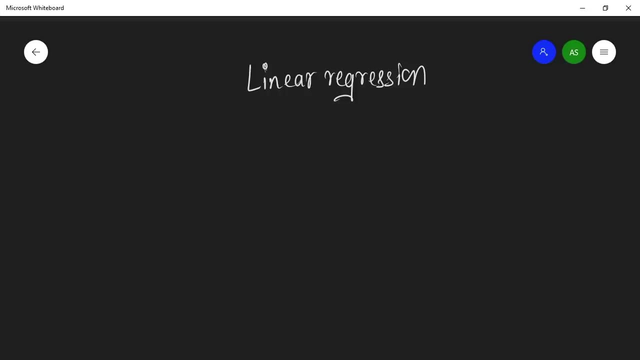 OK. so before that, I want to recall something which is in supervised learning and super wise learning We are. we were having two types of problems. First one is a regression problem. The second one is specification Problem, as you might think. 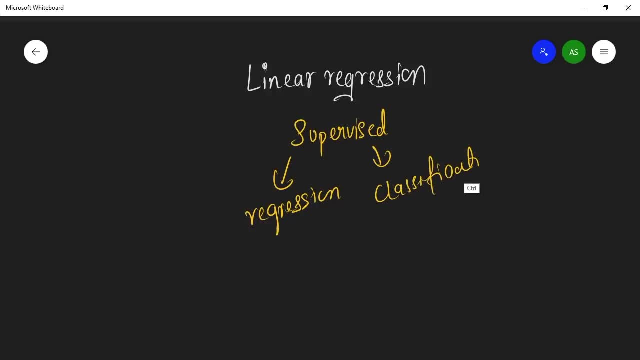 OK, so linear regression. as you know, as you can see from the term regression, it's a regression algorithm, So it's a regression algorithm that will study today, OK, And this section, OK. so let's recall what is regression. 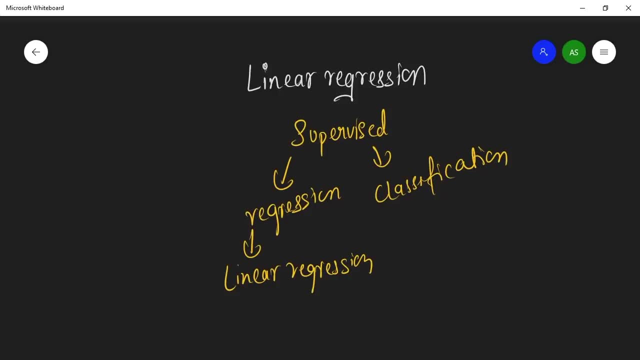 It's a, it's a type, It's a type of supervised learning, and so supervised learning algorithm, And here we know our output will be in conjunction- Continuous value. Our output will be in continuous value means let's say, let's- let's take an example- that you want to predict the price of the house. 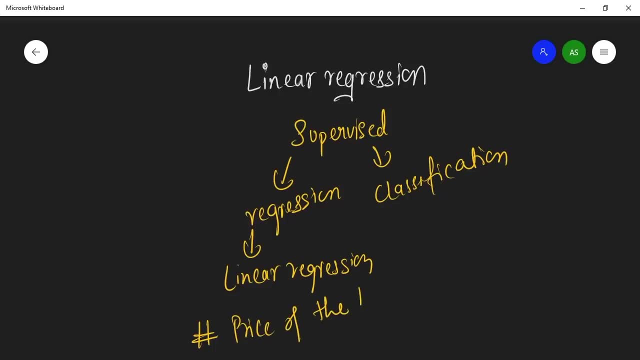 Let's say you want to predict the price of the house. OK, so you can see over here. the output of this particular problem will be in continuous value. We don't have any kind of decreed value, so we can identify that this problem is based on to the linear regression problem. 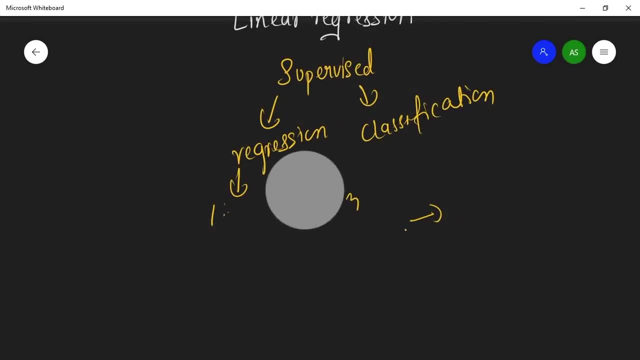 OK, so let's, let's, let's start See, let's see, Let's see how this algorithm works in much more detail, so that you could get more intuition about and you can ace an interview on a linear regression. And also I'll be putting some interview questions over here of what someone can ask you and what someone not. 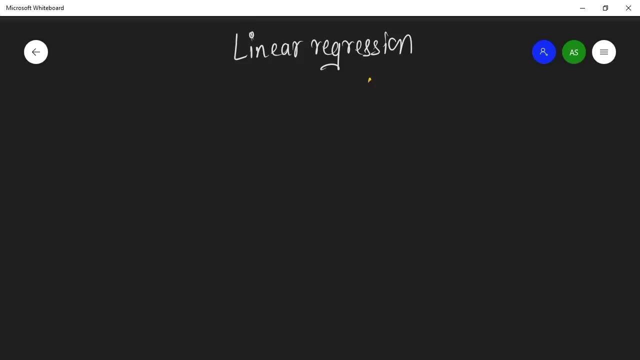 OK, so let's assume that we have a scattered data. So let me make one X and Y plane- I hope that this is good, Pretty good, And let me make that one. OK, so I'm just going to make the scattered data. that looks like: 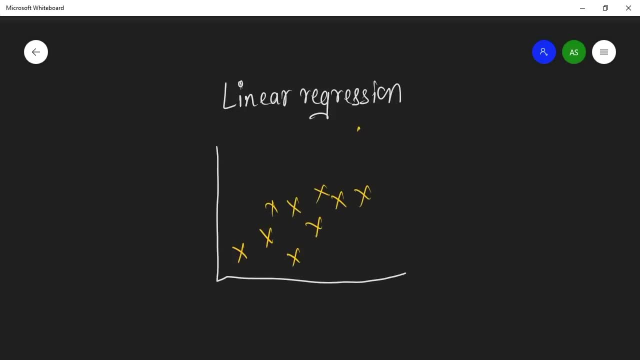 This. OK, so this is your data And let's take as a problem statement. as, like this, Let's take a problem statement which is predicting the price of the house based on the size of the house. So let me write that: predicting the price of the house, predicting the price of the house. 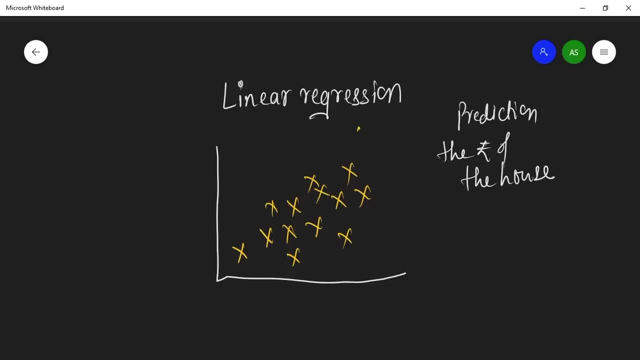 And this is the end in rupees, So the price of the house based on the size of the house. OK, so you will give X, which will, which will be the size of the house, And you will get the Y, which will the price of the house. 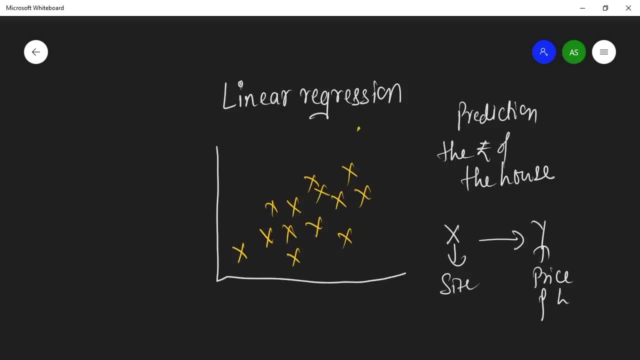 OK. OK, so we have the scattered data and an X axis, We have our size, which is our input variable, And in Y axis we have our price. OK, so what we do? we fit a straight line If it is straight. in linear regression. we fit a straight line like this: 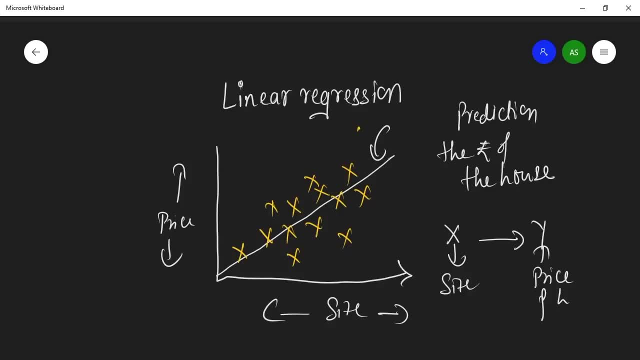 We fit a straight line, which is called the hypothesis, which is called a hypothesis, And regression term is called a hypothesis, which will see how we can compute the straight line. So we make the straight line and you can see over here that after making the straight line we can make predictions. 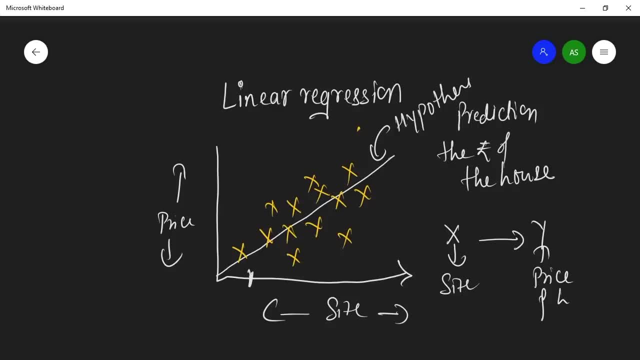 So let's say that this is, this is the size, And based on this we are making the prediction like this onto the Y axis: OK, so, and again, let's say the price. let's say the size of the house is twenty two hundred square feet. 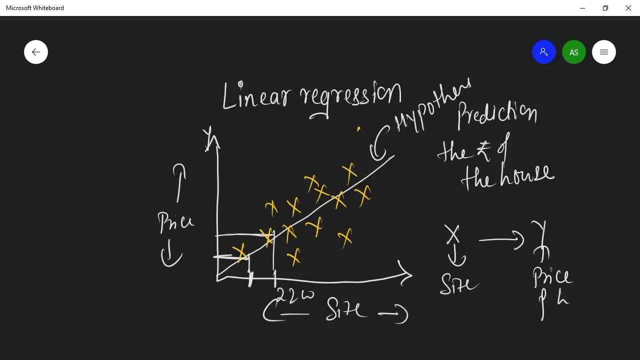 Then the price will be like this: to twenty two thousand, et cetera. So, like, like, like this We are making predictions, OK, and you can see how we are. This line is a little bit far away from the actual data point. 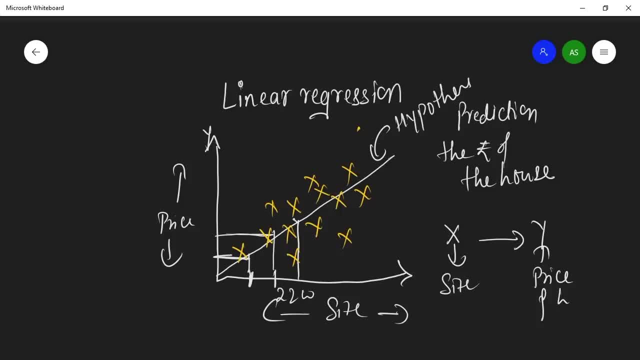 So that's the issue that that we'll see later on. But you just construct a straight line that touches each, that that closely touches each point, or that that is closely passes through this tree of scattered data points. OK, so let's see how we can compute the straight line, because linear regression, as you know, linear means it constructs a linear line, that's. 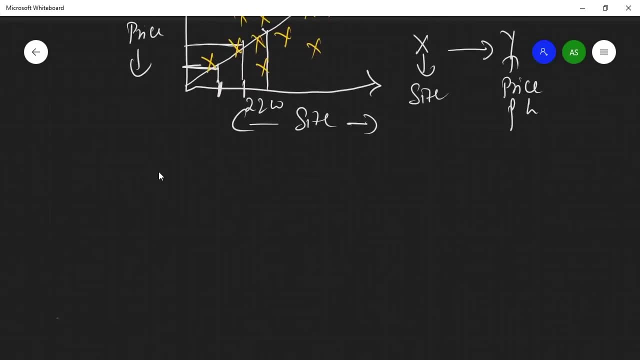 intercepts the data. OK, OK, so let's see how it works. So in for making the straight line. as I have already told you, it's called a hypothesis, So how we construct hypothesis, So this is called the hypothesis function. 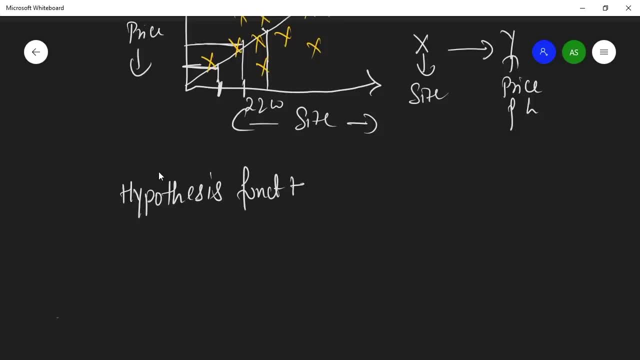 We compute hypothesis function like this: We have weight of every features. So let's say they are zero times X, zero plus theta, one, data, zero time times X, zero plus theta. one times X, one plus theta. two times X, two, all the way down to the data and times X and OK. so you are summing it all up. 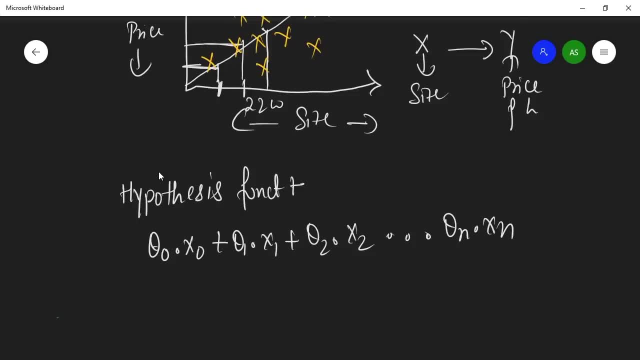 So what, what I, what, what you can see over here, that what you can see over here, that we have the status and we have these features. This is, this is the- let's say, the size of the house. Let's say, this is the- maybe the number of fans in the house. 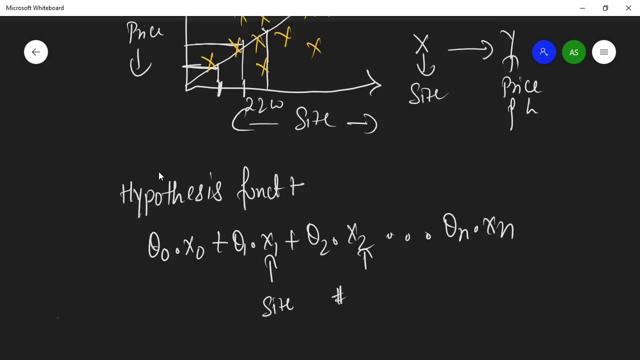 I'm just taking those problems. I'm predicting the price of the house, So so that's five. number of fans in the house and and et cetera. OK, so these are the features: X one, X two and X zero. is the bias term? is the bias term or the Y intercept, or the Y intercept? 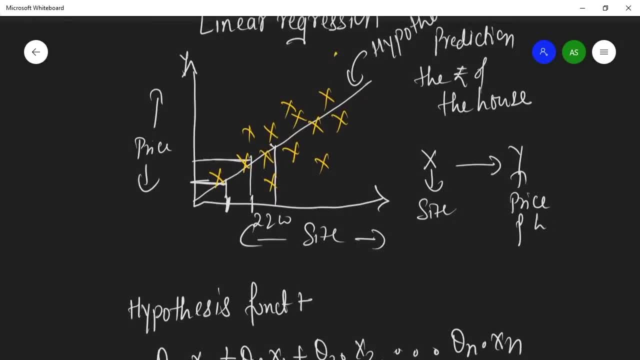 Maybe if you know about. intercept of Y means if X zero equals to zero, then your line will be crossing from the origin. If X zero equals to one, then it will be from one. If X zero equals to two, Then Then it will be from two. 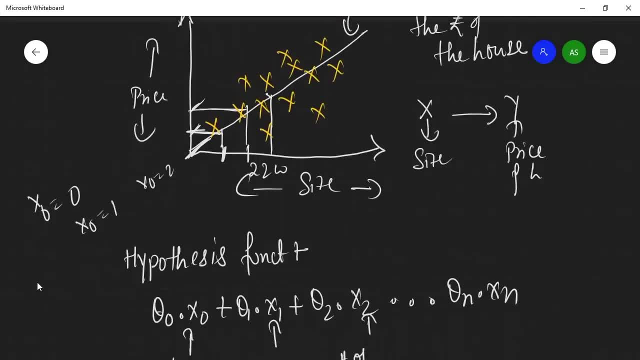 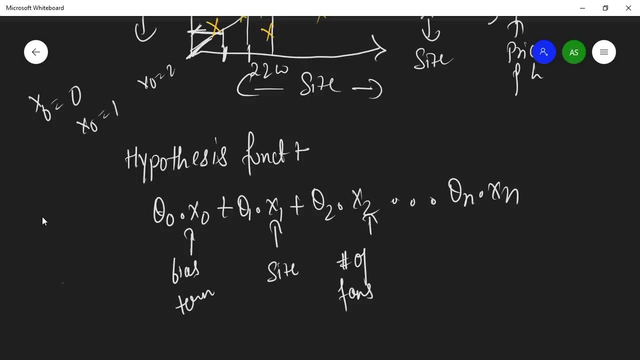 OK, so it determines the Y intercept from where he wants to make a straight line. OK, so we have this: a theta zero times X, zero theta one times X, one. theta two times X, two, all the way down to the theta X times X, X. and let's take a particular problem statement and let's understand that. 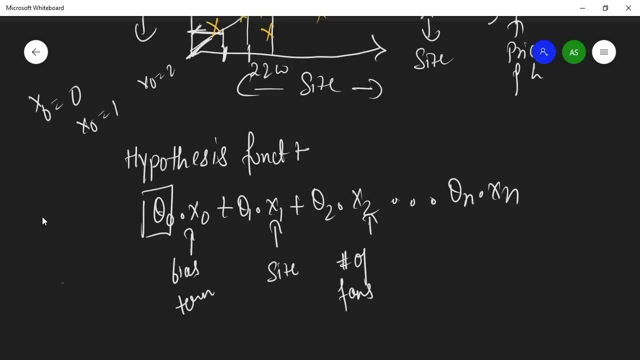 But before that you may think he I use for this data here. What is theta here? We only have to learn machine. Well, we have to learn this data machine. Well, we have to get. We have to get the best data. 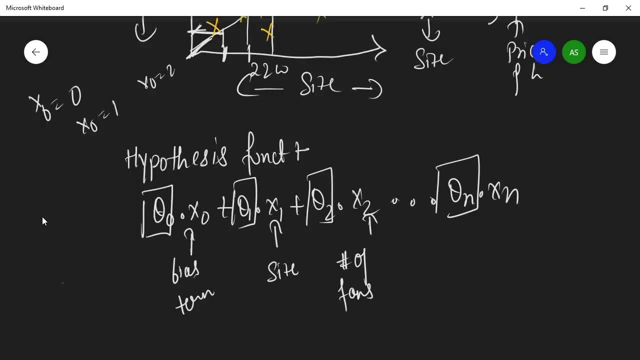 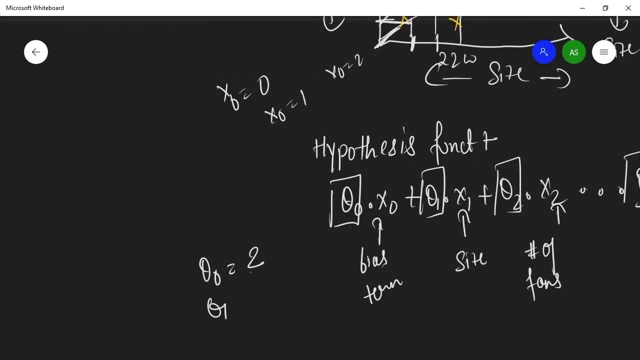 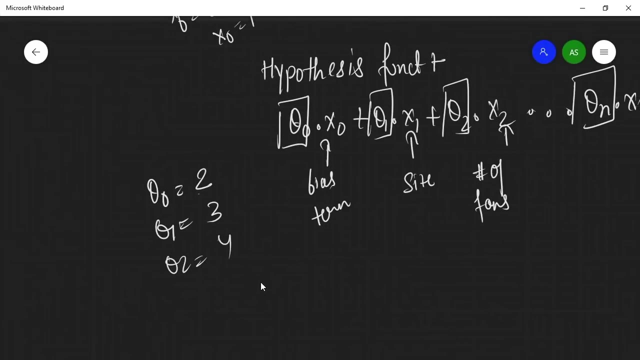 Now we are able to make prediction. Now let's say, we take theta zero, Let's take, we take theta zero to be two, OK, and theta one to be, let's say, three, theta two to be four, OK. so just just, I'm taking only two features and one bias term, which is: this is the bias term. 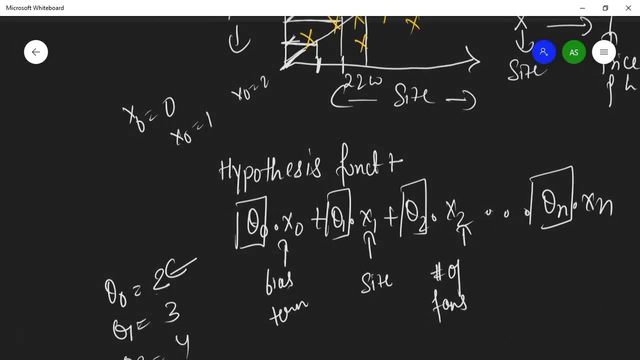 And these are the two features. and X zero, is obvious, is always equals to one. X zero is always equals to one. So that's why we never Write X zero OK. so that's why we never write, We just write theta zero plus theta one times X one. 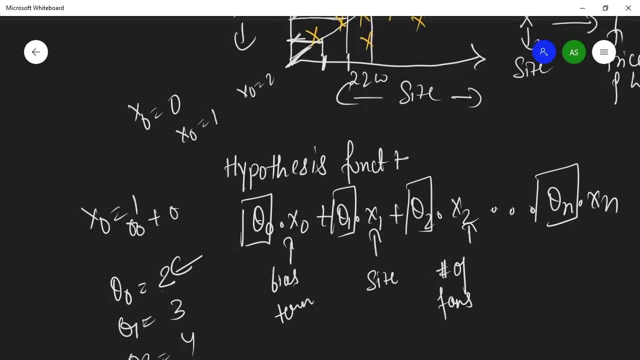 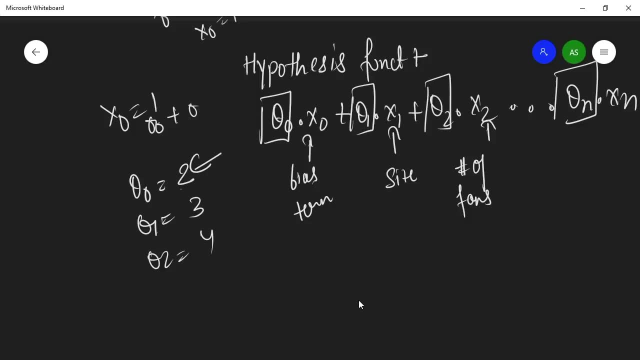 We did not write, but I just just I've showed you so for a clear reason of those things. OK, so you can see over here that let's let's take an example that this: we have two features like the size of the house and the number of fans. on the base of that, 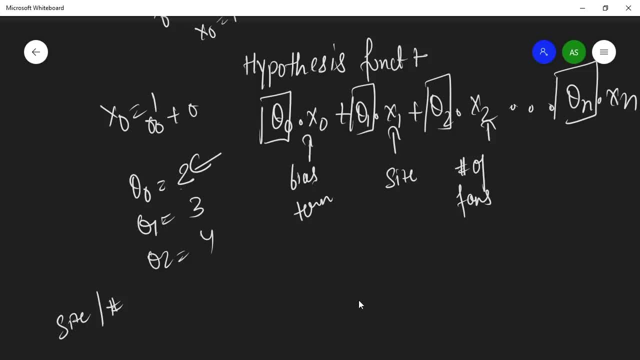 You have to predict the price. So for each feature, we learned of eight These. these are called the feature rates. These are called the feature rates. So we learned this and if we get the best feature rate, we will getting the best prediction. 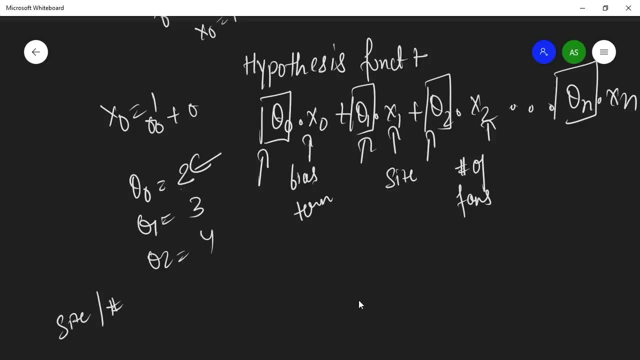 If we get the bad feature rate, we'll be getting bad prediction. OK, so let's say: let's, let's construct the problem. So let's see your theta zero to be two times X zero, which is X, where X zero equals to one. 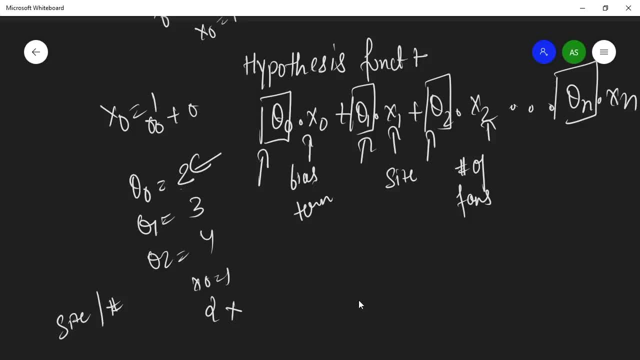 So it's obviously two plus theta one, which is, let's say, theta one is three as of and times the size of the house, plus the data to be four Times the number of fans in the house. OK, so now this. now, using this, you can make the prediction. 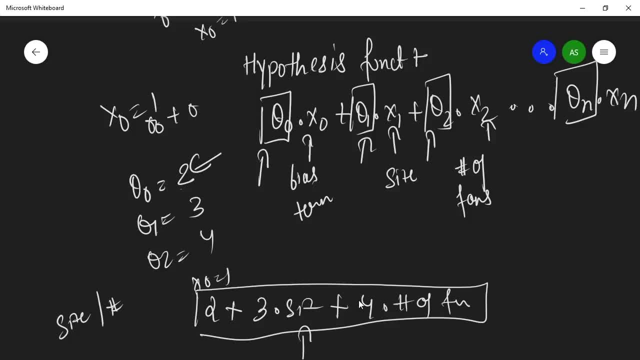 You can just plug in the size and you can plug in the number of fans and you will be getting your desired output. Why, OK? so just now you may think he machine learning is not the. we are not it. We are only using it as a computational power. 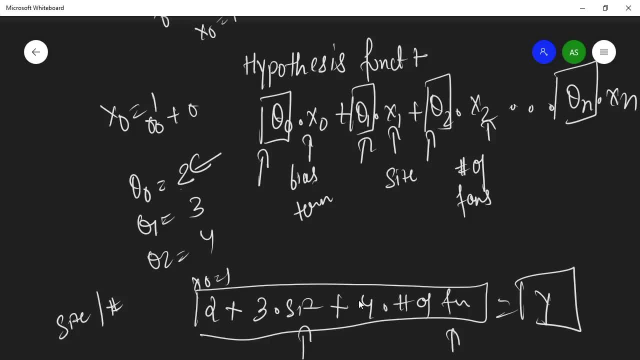 And you can see over here that how it, how it learns theta will, which we'll see, because machine learning is totally based upon learning Parameters. OK, so you will see how the heat out, Lauren. So let me tell you theta's, we have to only learn theta. 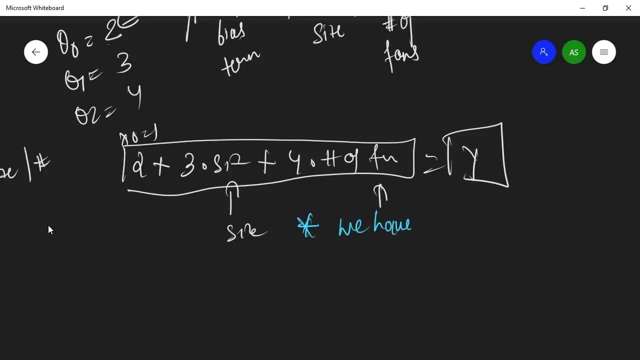 We have to only learn, which will see the techniques where we have to only learn theta. You have to only learn theta, And if the theta is bad, then then you. then your hypothesis is that a function is bad, So this is your function. 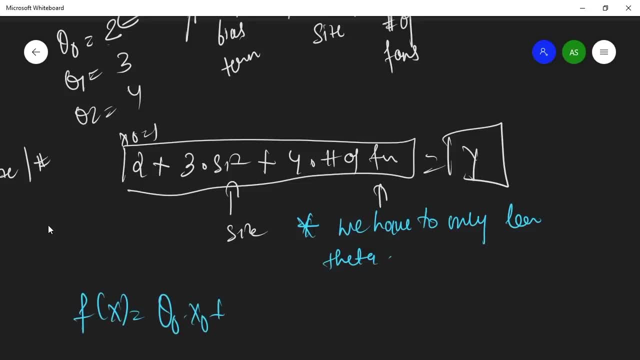 This. this constructs your function like this. They are: one times X one, Plus theta, two times X two, all the way down to the data and times X, and and, and. here they denotes the number of features and features. are the columns OK in the data? 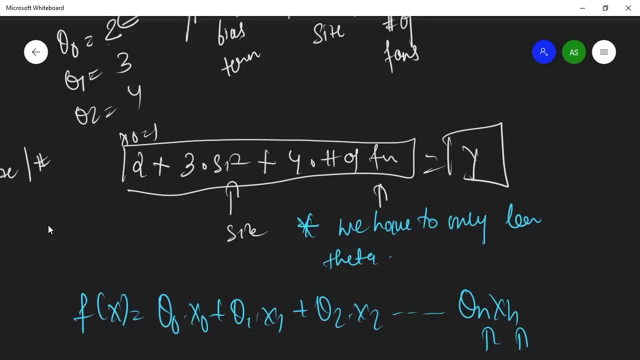 OK, so this is a function and you can use this function to map your input variable to your output variable. Why? OK, so that's, that's, that's kind of our. we have our kind of a function that maps our input variable to our output variable. 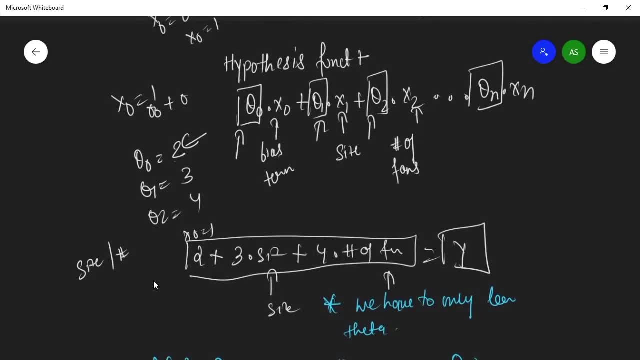 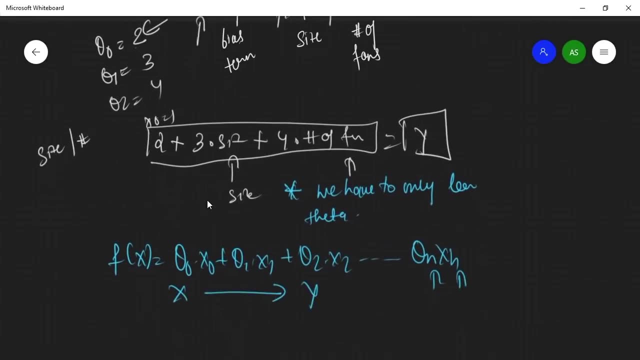 OK, OK. so now I think that you, that's, that, that's, we've got how we construct that A straight line, and using this function, we can construct that a straight line, and we have to only learn these, these, this, this is called, these are called the feature rates. 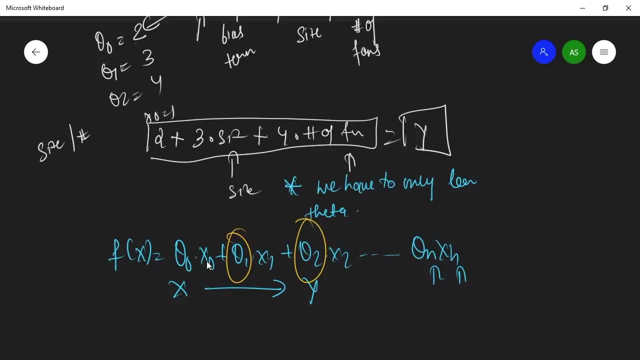 These are called the feature rates, and these are called the feature rates And this is the bias term, or the y intercept, from where the, the, the line should originate, as I've showed you earlier. OK, so now I hope that you got intuition about hypothesis function. 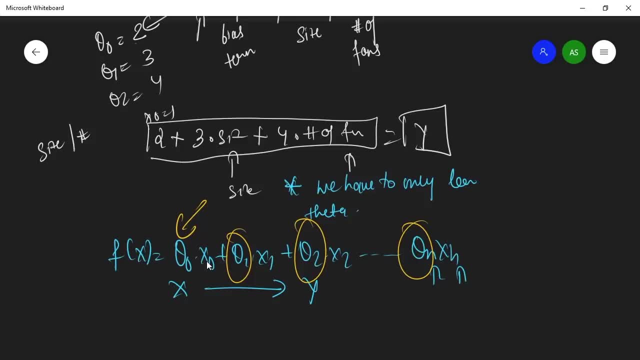 OK, So now let's keep talking about the vectorized form of this means. the vectorized form is maybe vector vector. vector vectorization means how here we are, separately computing for each values. They're computing data zero, then times X, zero data. one times X one means separately for each value. 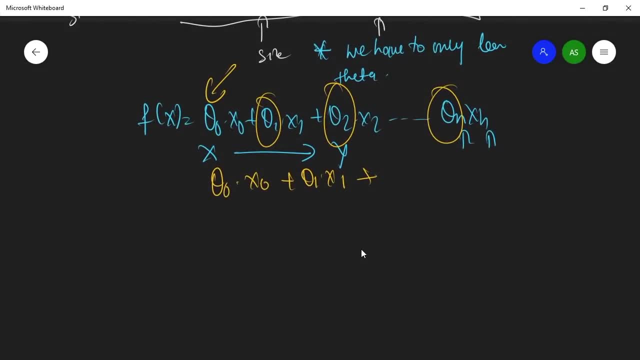 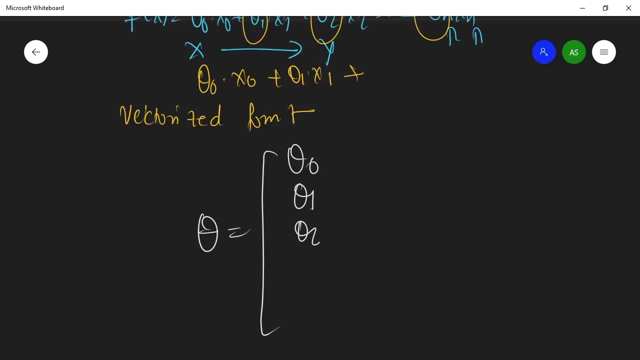 So in vectorization we do at once, we do at once. So what we do, we put our all the thetas, So we put out, So I'm just writing vectorized for them, vectorized for him. So we put our all data, we put our all data to be in joint vector data. and let me do this: data, zero data, one data to all around the data and data, these data. 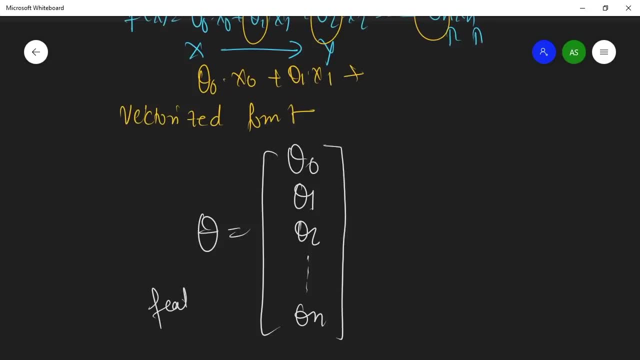 This is the feature vector. This is the feature vector which, which is all the weights. You will further see that, Yeah, we have to only learn this. Then you would believe me that, Yeah, we only have to learn. But it's a neural network, but it's a machine learning. 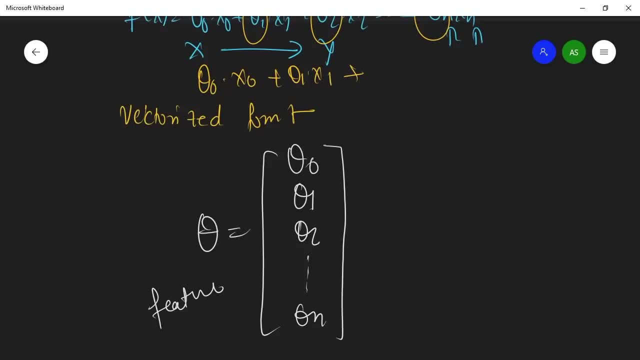 OK, so you have this base data in the joint vector data and you take a giant vector X and you store all your X's over there: X, zero, X, one, X, two, X, three, all the way down to the XN. 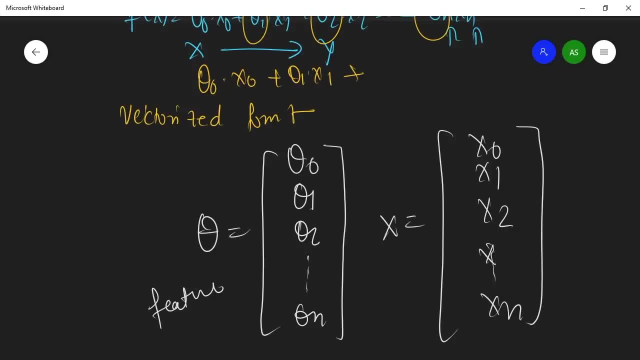 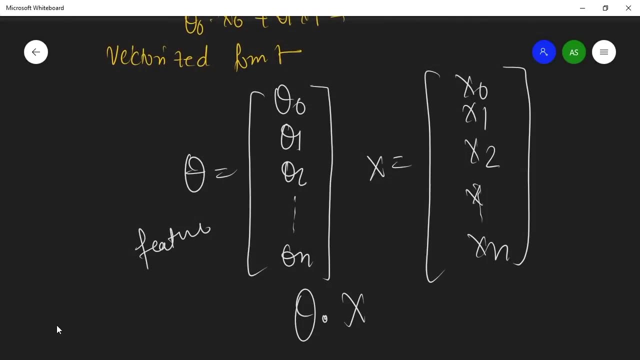 OK, so you take this and then you take out the dot product. OK, so then you take out the dot product and data times dot product. OK, so now your hypothesis effects will be like this: OK, so you just give this function and tell us what what it will do. 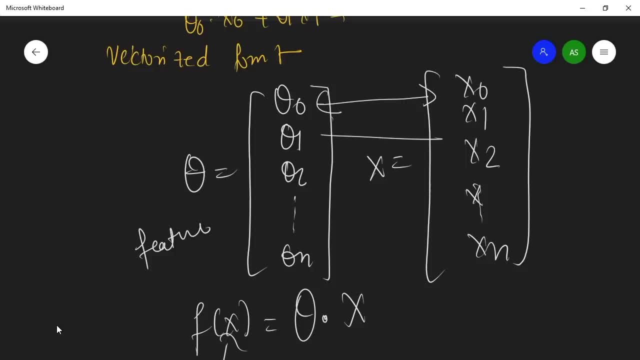 It will data zero times X one, data one times X one. It will sum, sum it all up. data one data to like, like this: broadcast it OK and it is computing at once. OK, so you can try and then some sum it all up. 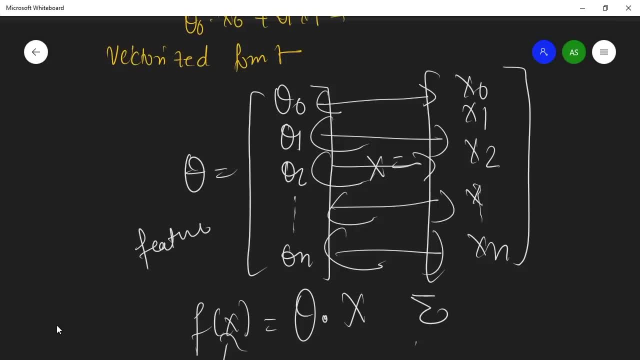 OK, so you can. so you can write in summation format: equals to one all the way down to the N, or equals zero all the way down to the N data data: I times X. Let's say I. OK, so you are doing is a vectorized form of that. 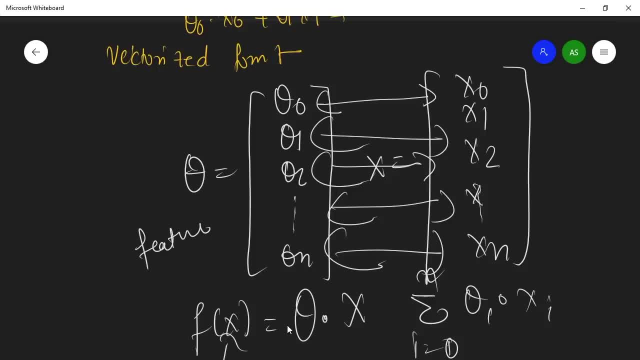 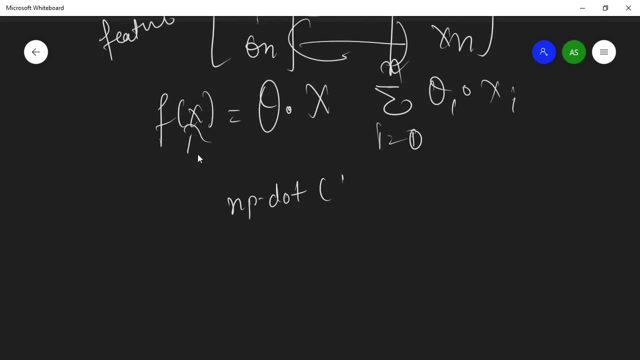 And you can see over here: in Python is very easy. Just one line of code like like this: You just do like this and be dot, dot, data and X done OK. so it's very easy in Python. So don't worry how how we can code this all. 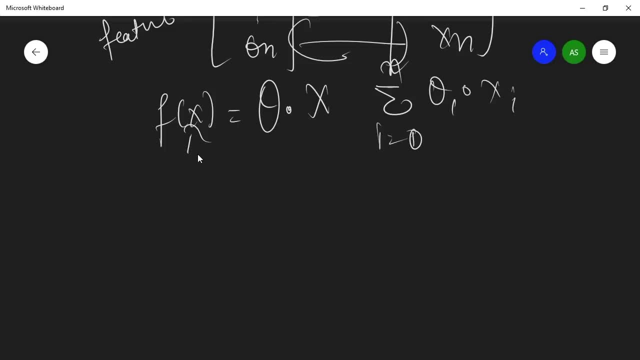 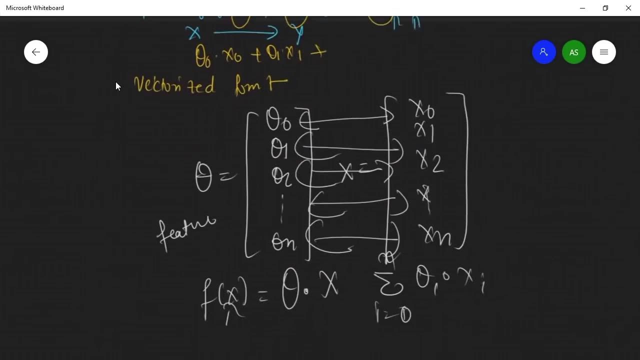 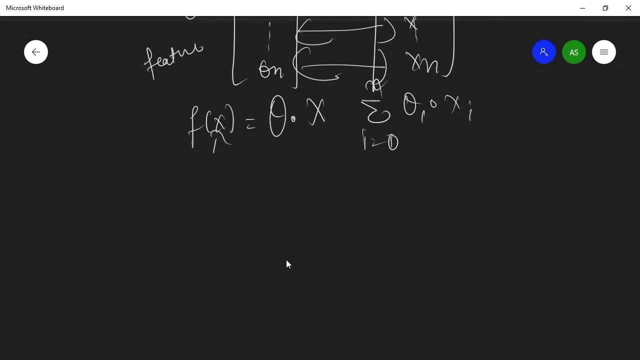 It's, it's quite easy. OK, so now we have seen the hypothesis and then we have seen the vectorized form of this Linear regression. OK, so you may think, hey, I use how I can get this data, But before that, how we can evaluate your data is best means your data's are good. 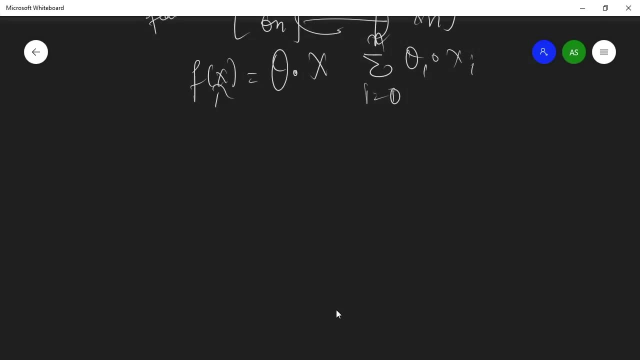 Your data are good. So for evaluating your model, we have something called cost function. We have something called cost function. OK, so why we evaluate a model? to check how are the if our data is good or not. OK, so we check, because using that data, we are making prediction. 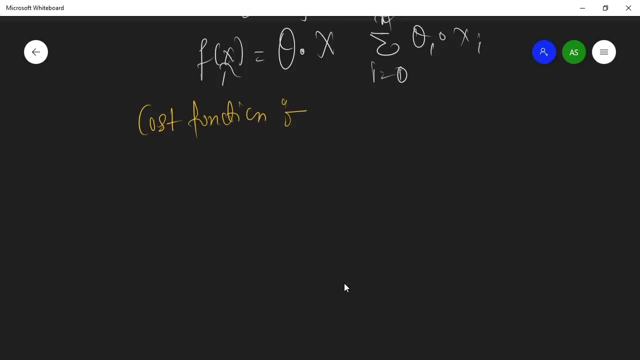 We are multiplying with the features and we will get feature these, the size we will get from the user. We will this game fan number of fans get the user and we multiply with the weights and then sum it all up And then we give the result. 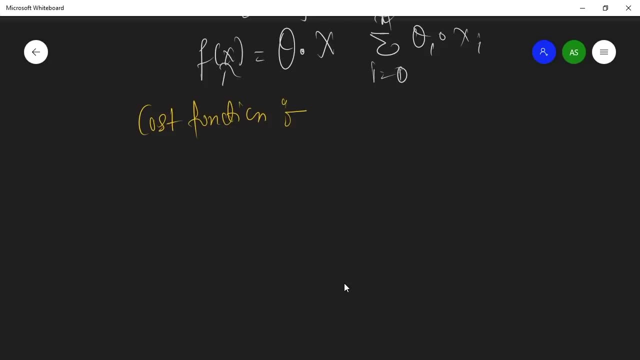 OK, so this is the cost function. And here what? why? why we use cost function to evaluate a model. OK, so you will get to know how, what, what we do. So let's say we have a scatter plot, So let me plot on a scatter plot like this: again the same. 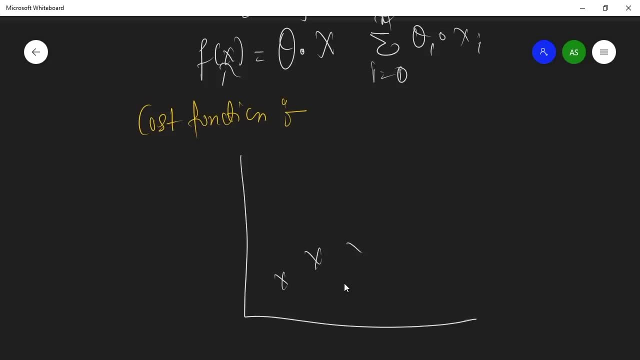 I'll be doing the same, but this time a little bit more crunchy. Yeah, I think so. OK, so this is this is my plot And what we do, and we simply draw a straight line. This is your hypothesis. This is your hypothesis, which is F of X. 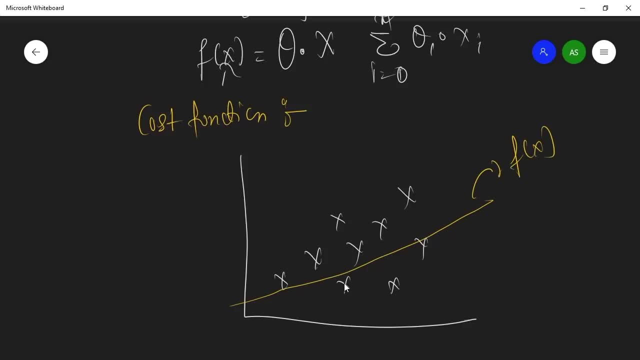 And what this cost function will do. this is your. this is your actual data point. These are your actual data point And these, these are your actual data points. These are your actual data point. It will. what did you simply know? It will simply take out the distance between predicted this. 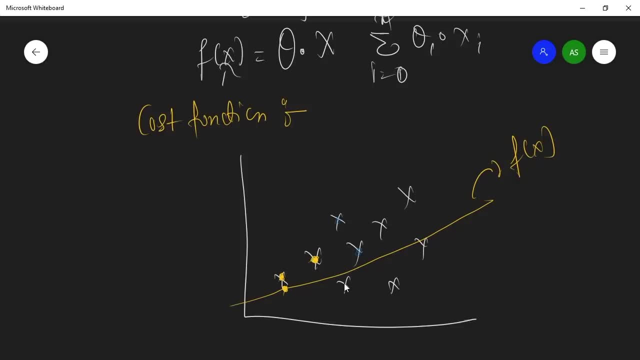 This is the predicted, I'm highlighting, and this is the actual OK. So this is the predicted, This is the sorry. this is the predicted And this is the actual. This is the predicted, This is the actual, OK. so you said how the difference between the stakes are: distance between like this, like this. 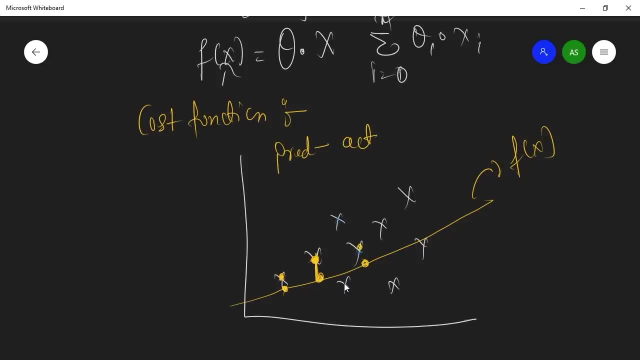 Red composers: actual value: predicted: minus. yeah, like this. and, and then sum it all up, means higher, the this, uh cost function will be barrier, more or less higher. the cost function will be barrier model will be: and uh, less the cost function will be: uh, good, your model will be the reason why. if your, if your points are on this. 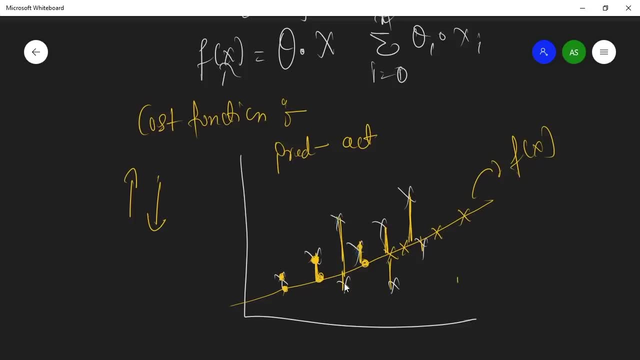 line and your cost function will be zero, because the predicted will be zero. sorry, let's say, predicted will be all the same and actual will be also the same, so it will be resulting in zero. so just what? what we do? we? these are called the residuals in terms of cost function, so we just 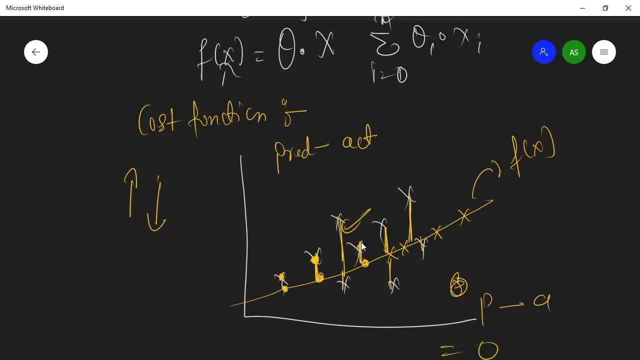 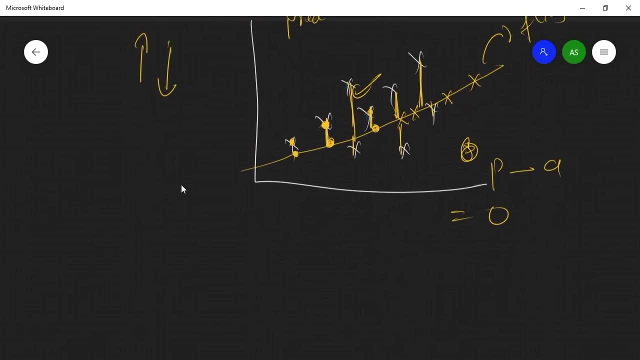 take out the distance between predicted and the actual value for all data points. okay, so this is the cost function. okay so, uh, let's try, rest for formulate this in a formula. let's formulate: this is the formula like this: uh, let me show you how we can formulate that. yeah, so you just take out a j of theta and just. 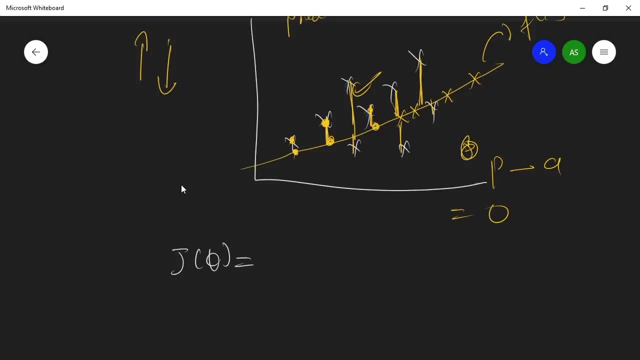 denoting j of theta will be like the uh short form of cost function, because we are checking how our theta is good or bad or not. okay, because it only determines whether your model is good or bad. one over m, one over m and m. here is the number of our data points: 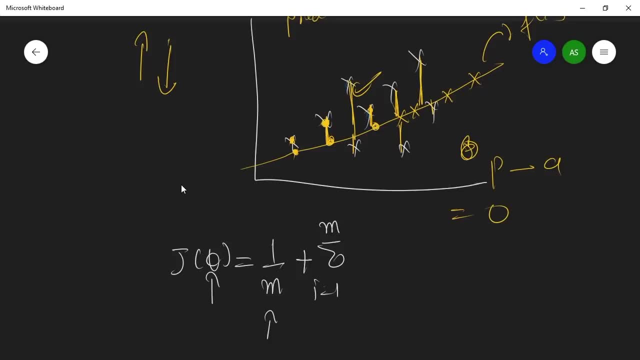 plus i equals to one all the way around to the m and you just model prediction, the value. let's, let's denote the model predicted value by y hat and how, how we have, we have, we got y hat. yeah, we have got y hat like this: y hat equals to uh f of x, equals to theta times x. 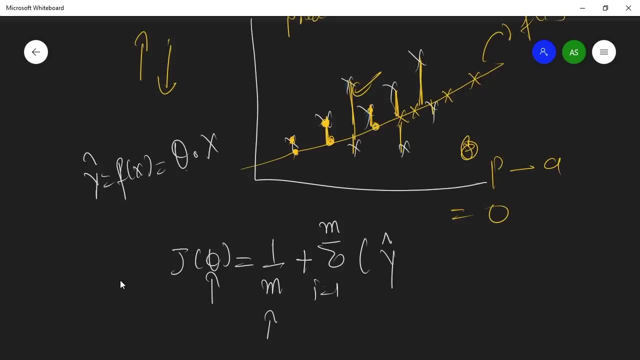 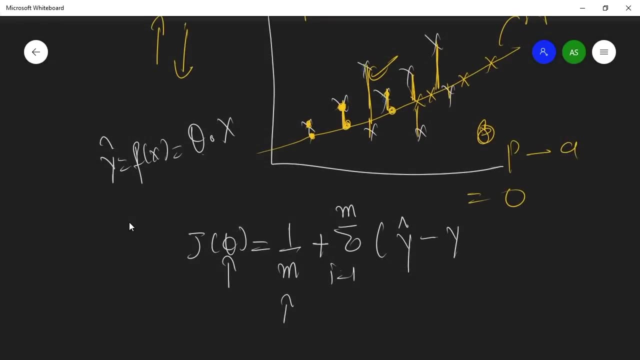 means dot, product of the theta, and x, which is equivalently equals to the hypothesis. okay, so we let's let's note as a y hat minus y, okay, and in other words, we can write this out like this. in other words, we can write it, write this out like this: theta transpose x i minus y, i, and this is this is just a. 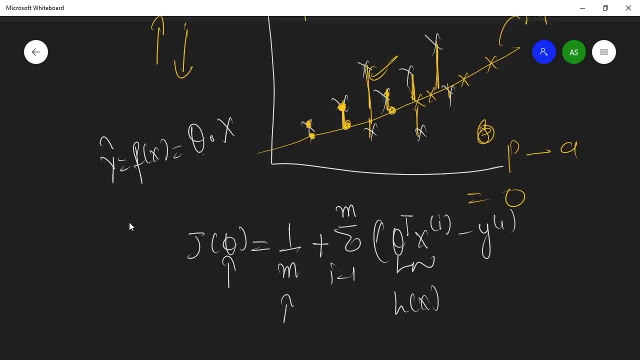 hypothesis h of x. okay, and transpose like this: uh, you, you, your, uh, x will will be like this. so you make this: uh, theta will to be like this: okay, so it will be easier. like this: okay, so the. so that's what this transpose is doing, but if you can do or not, just just we are doing the, this, uh, let. 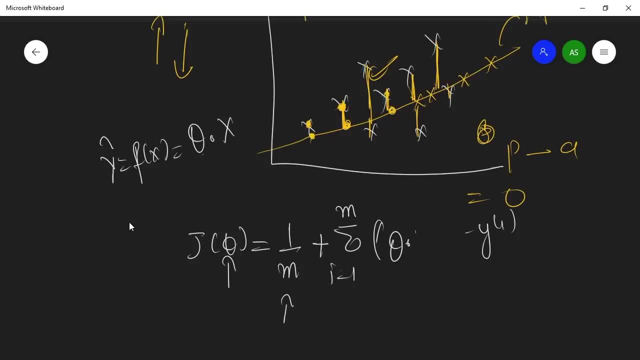 me write that theta times x. okay, the dot product between theta and x minus y i. okay, minus y, i. for each and every day data point. we are taking out the difference between predicted and the actual value and then we're squaring. we are squaring here because it help us to. 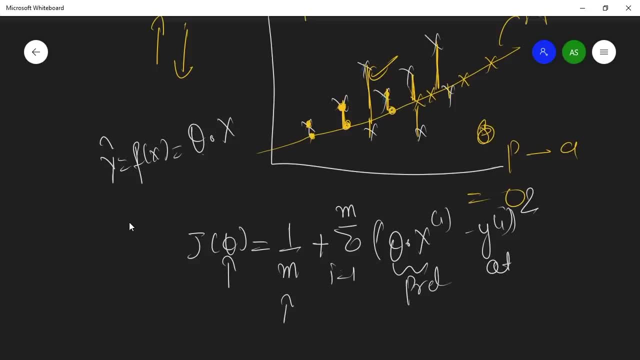 infer the call, something called the gradient descent. okay, for easily derivation of this cost function. you will see why i'm taking the deviation term over here. okay, so in other words, is this this? this this is called the loss function, which is known as mean square error, m, s, e, okay. 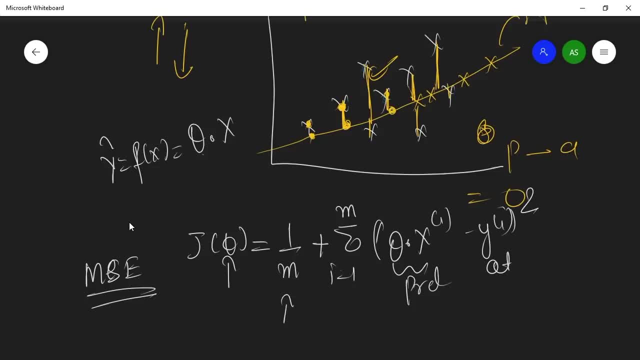 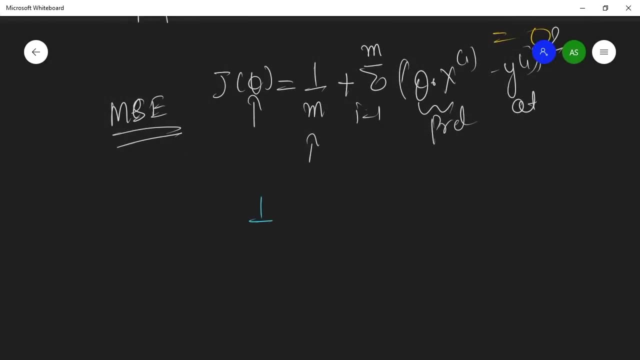 which is called the mean square error. if you square root this, if you make this, uh, let me show you what i'm telling. if you square root over 1, over m plus i equals to 1, all the way down to the m xi minus y, i squared. if you square root this like this: 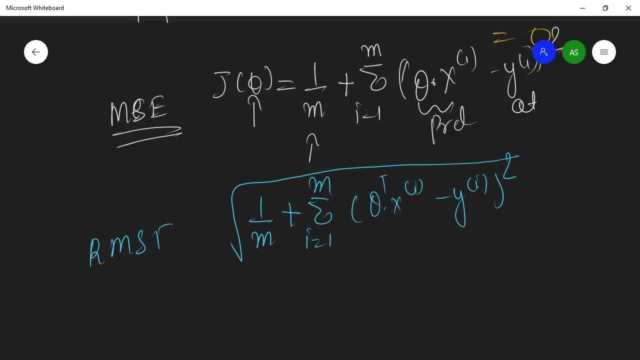 okay, this. this is called the root mean square error. root mean root mean squared error. okay, and hire this and battery model this, okay, okay, that's just just, we are taking the square root, okay, but we'll stick with this. um msc, but in real world, emily and kaggle competition they have given. 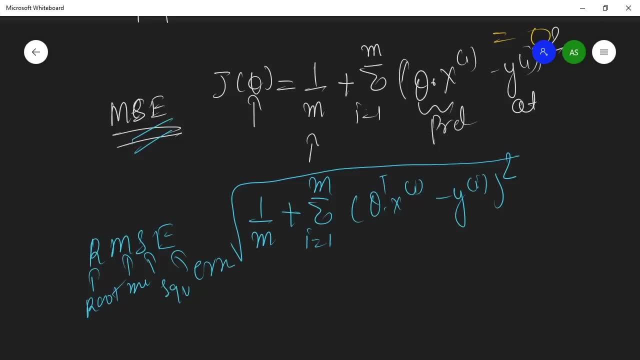 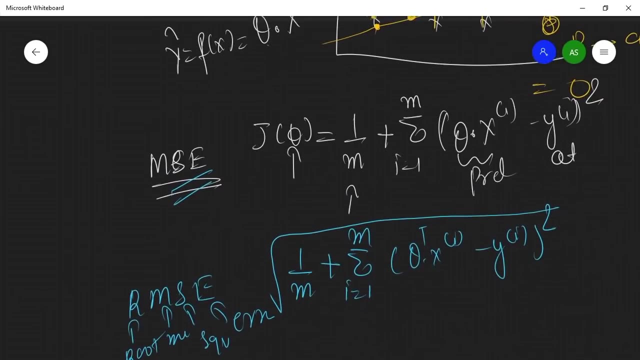 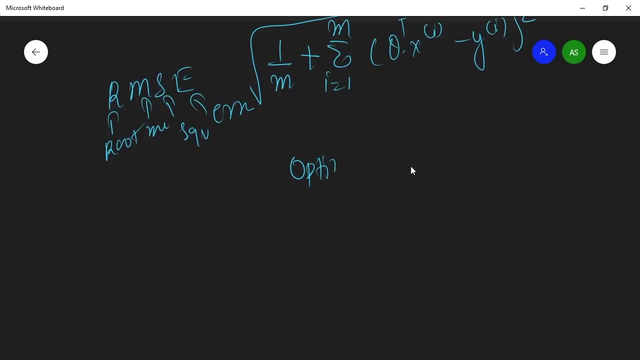 what they're going to use mainly. i have seen rmsa to be used very much okay. so, uh, after we got our function and it tells: okay, your model is that good or that bad. now, if your model is bad, how you can optimize, or how how you can get to optimal theta means best theta, how you can get the optimal theta. 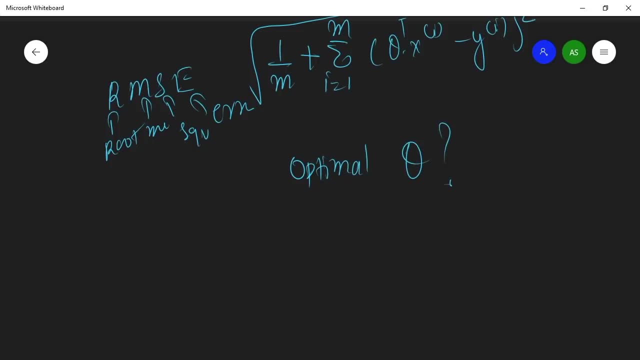 this is the great question to ask. okay, so how are you, how you're going gonna to get this optimal theta for getting that? we have something called gradient descent, something called a gradient descent algorithm. gradient descent algorithm, which is known as the optimized gradient descent algorithm, is known as the optimization algorithm, which is known as the optimization algorithm, which will 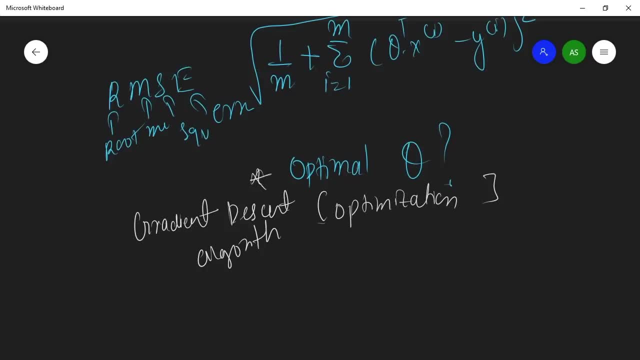 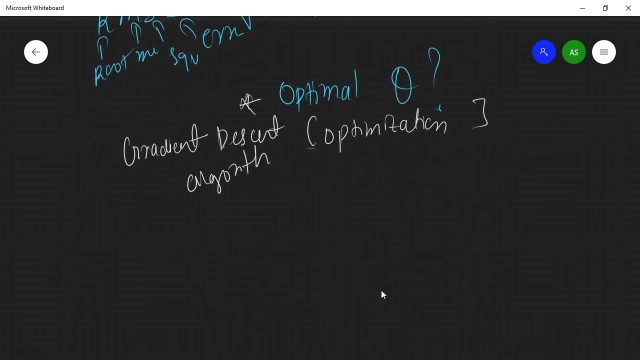 help us to get the best. theta, okay, optimization algorithm, okay. so, uh, let's, let's dig dive into this algorithm and let's understand how we go get this kind of thing. so, let's say, our the visualization of the cost function will be like this: okay, just just for the sake of an example, i'm visualizing. 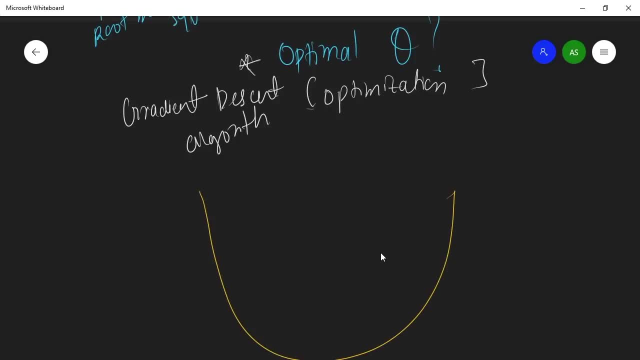 like this: okay, so this is, this is your cost function. i'm just writing as a z of theta this: this is your cost function. and now your cost. uh, cost- here use is your theta, where the cost function is very high. okay, so here is your theta. okay, so what gradient descent does it? tweaks the theta. 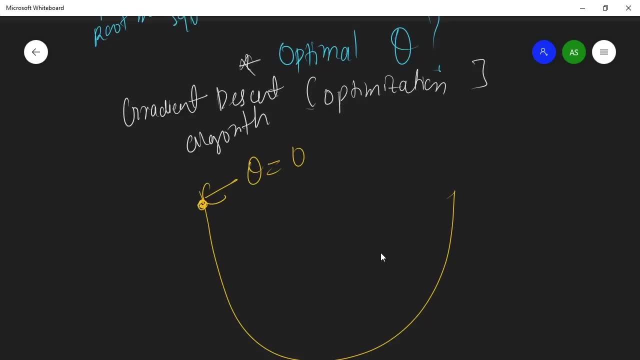 means let's say your theta is zero, then simply let's say: it's makes theta a little bit to 0.2. okay, it tweaks the theta, it changes theta a little bit and if the cost function decreases, then updates the theta to be not like this, to be like this: if the theta go down means the cost. 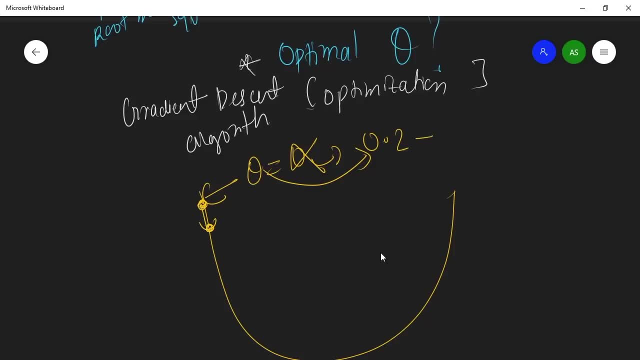 function little bit decreases, then it changes again 0.3. if the cost function decreases, then it's: do not make this, then it's uh. update this theta, okay, then again. it simply tweaks checks if the j of theta going down. if yes, update the theta. okay, until and unless your uh cost function is. 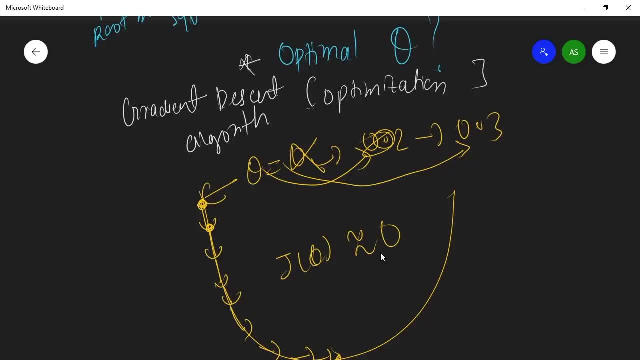 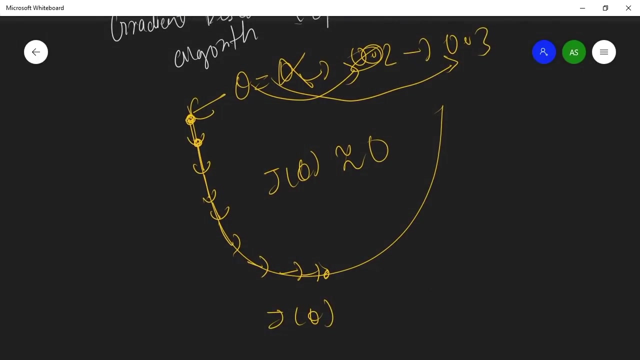 until, unless your cost function is approximately equals to zero. okay, so that is simply the gradient descent, and it's very, very simple. that i've just shown to you. so let's, let's formulate this mathematically, because it's very, very simple when we formulate this as a mathematics. so how we simply. 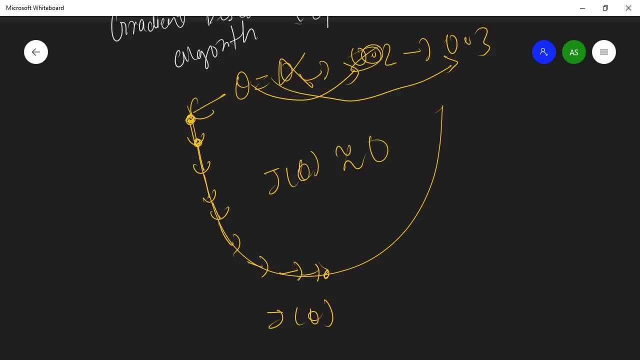 what? what we do for tweaking these things? for tweaking the theta? we take out the partial derivative. we take out the partial derivative of your cost function j of theta. now you will think: hey, i wish you have um. why? why you have taken the calculus name. i'm not a calculus student. 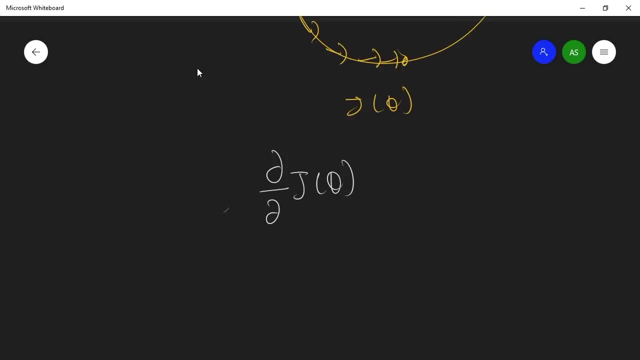 i'm not kind of that, don't worry at all at all. it's kind of it's. i just want to give you one definition of a partial derivative- partial, what if? what it does? it simply tweaks your theta. it simply tweaks your theta and checks if the cost function decreasing okay, and it's just like the slope it's. 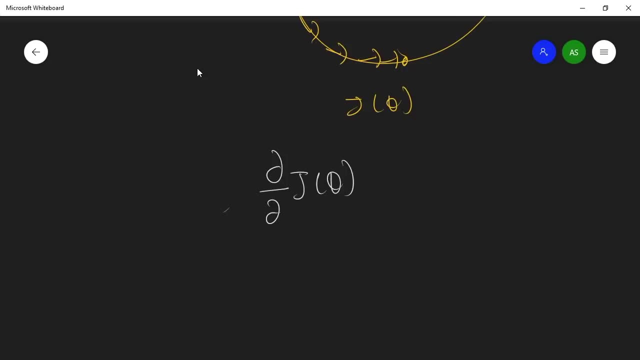 just like the slope, but you don't need calculus, you don't even need calculus. yeah, if you want to go on a research level, then you obviously need, but for now, for machine learning, you don't need calculus, even you don't need calculus, just um, just, you can. just what, what this equation is doing? it is just. 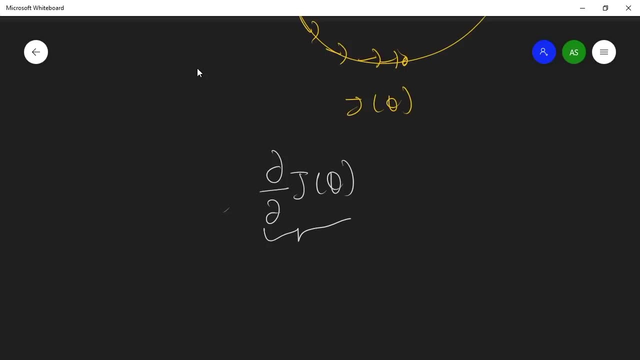 it is just: um, uh, tweaking your theta, tweaking your theta little bit, so it gives us like this: 2 over m. so it gives us 2 over m plus i equals to 1, all the way down to the m and it's a y hat minus y squared. okay. so this, the after, after deriving this partial we, we get like this: 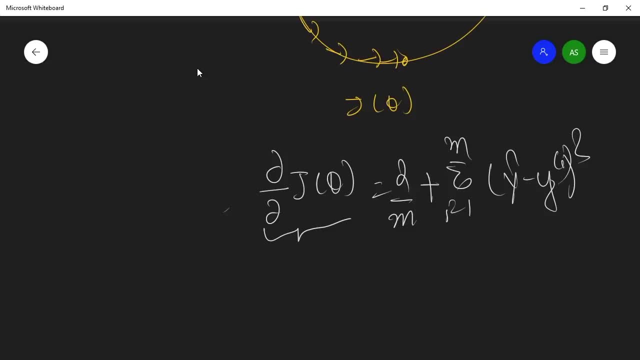 okay, so now after this we do, uh, we do- we take out the partial derivative for every theta, means theta 0, theta 1, theta 2, theta 3, all around the theta. and we do for all theta. we take out a partial derivative of all theta and then we up and then we update our theta. so here is a full gradient, decent. 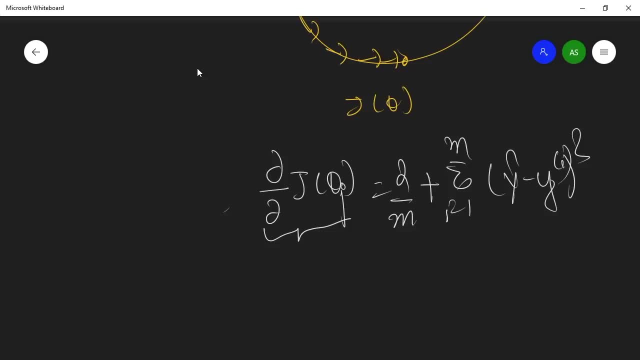 algorithm. so what? what? what we do? we simply write: theta z- this is the update kind of assignment, theta minus the learning rate alpha and the kind of a partial derivative of your- okay, partial derivative of your cost function, okay, so what we are doing, this is our, this, this is our. 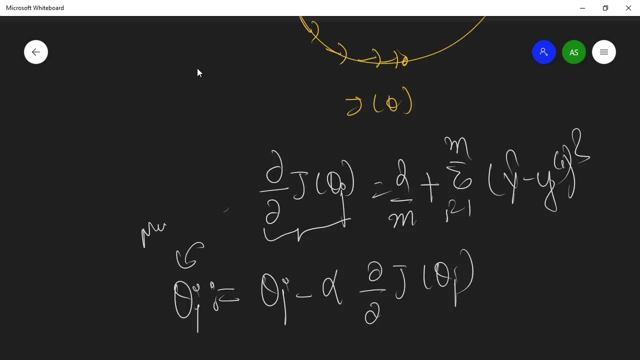 this, this, this will be our new theta that i've just shown to you. we update the theta, so this- this is your old theta- means the bad theta. this is a learning rate, and what rate? your um, this is the hyper parameter, which i will talk about in just a second in detail. but what we are, 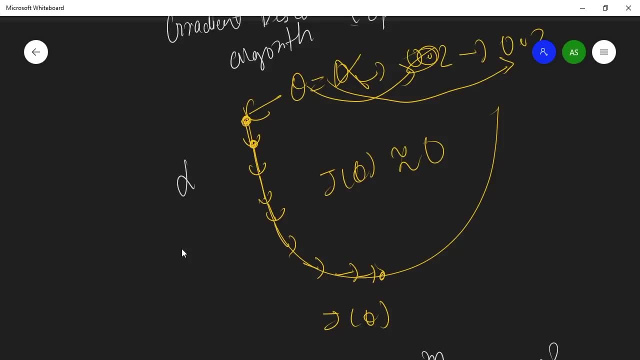 going to be doing is menged until i get a full version. because, um, this your alpha less than the nucleus. and what alpha is in the 균? it is actually called the beta. so in general it is like this in one space than it is in the nucleus. so from that bins that you can use. 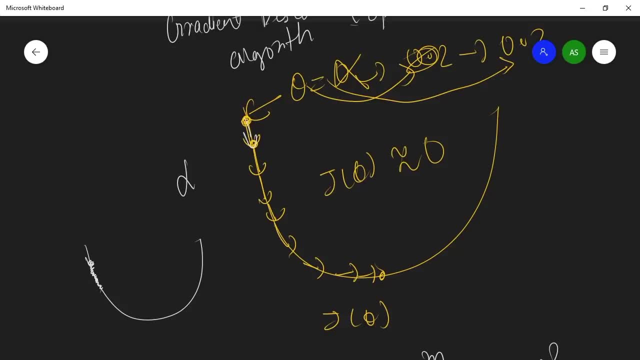 on system like a system like a dc, a zero, zero, zero and the delta野r theta, but, of course, okay. so are we starting to make this comparison here? yeah, we are starting to make this evaluation and everything we have talked about is: there's a great things to think about and let's go ahead and 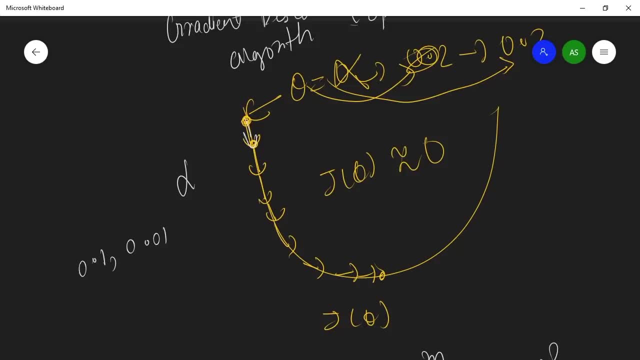 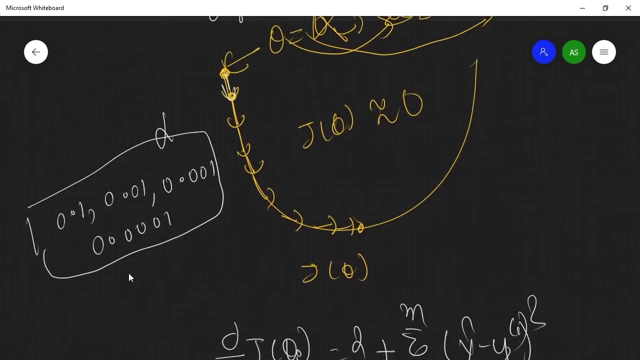 0.001 for- okay, for a little bit smaller- medium data set, 0.001- a little bit more smaller, and 0.0001- okay. so these, these are the optimal uh for me i have seen so far is these uh alpha, but you can tune it. you can tune it using um grid search cv or randomized search cv, which we will see later. 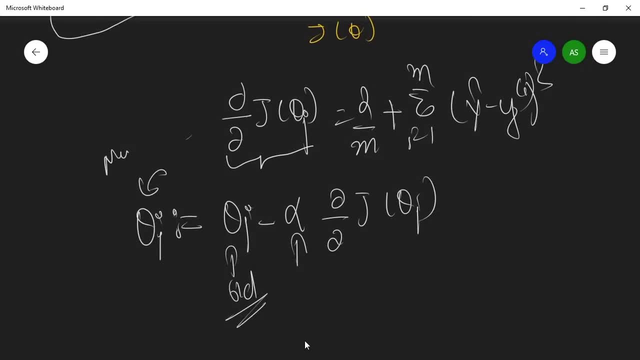 on, okay, okay. so i i just say to you why, by this theta, it just determines the rate of your, uh, tweaking the parameter, okay, just going down, and this, this, this gives, this is the simply the partial derivative of your cost function, and we are updating this, this, this will be our new theta. 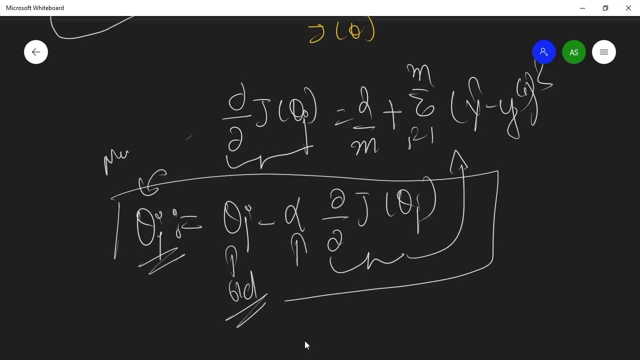 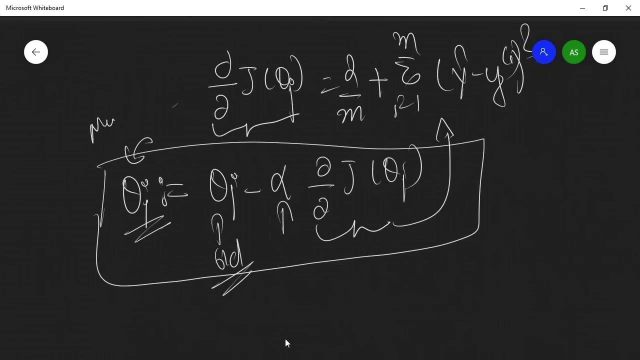 and this is whole learn, uh, algorithm of gradient descent. okay, okay, this is just just just equations, tells us the whole algorithm for gradient descent. okay, so now again, i'm going to talk about the gradient descent and i'm going to talk about the gradient descent. okay, so now again i'm going to talk about the gradient descent and i'm going to talk about the. 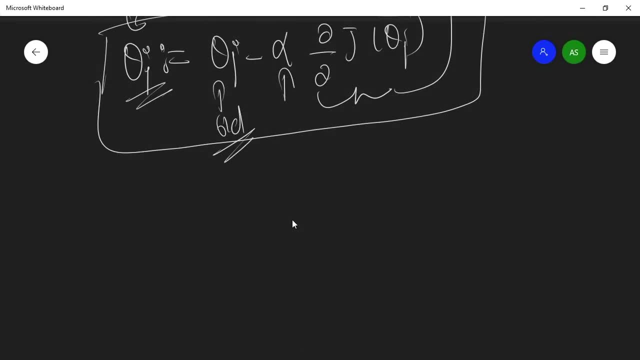 uh, vectorized forum, how we can vectorize this? okay, because i i totally believe in vectorization. so, let's uh, what, what, what we can do. uh, here we are in the pre. previously we are taking out the partial derivative of theta zero and then we are taking out the partial derivative of theta one. 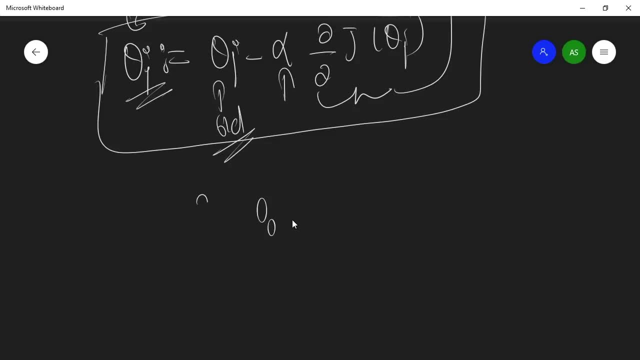 separately what we can do, what we can do and we can simply put that into: uh like, like this partial derivative into a joint vector, theta, into a j of theta with respect to zero, kind of this, and like this all the way down to the end. okay, so you just put into the joint vector. 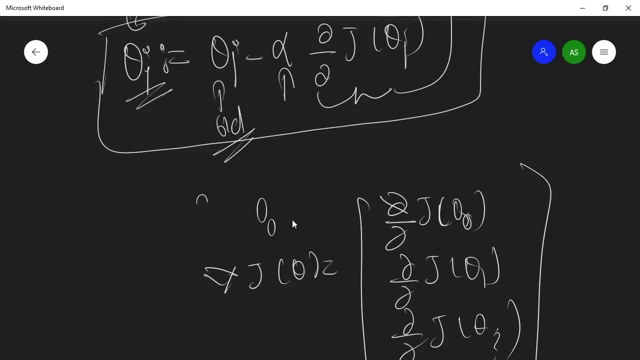 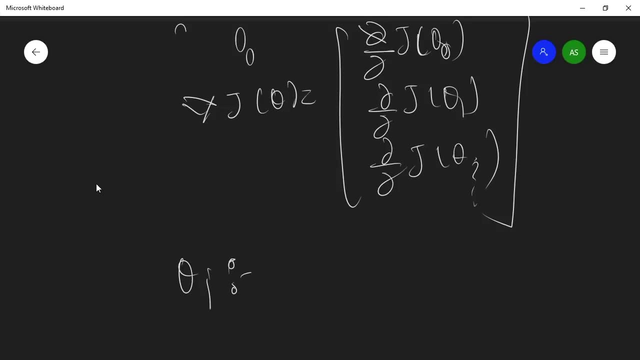 and you just take out the partial derivative, whatever you want to take out, and then, and then you just uh write the vectorized forum: theta z, theta z minus the learning rate alpha, and that gives us, uh like like this: 2 over m times the x, transpose x, theta x, theta minus y, and this is your. 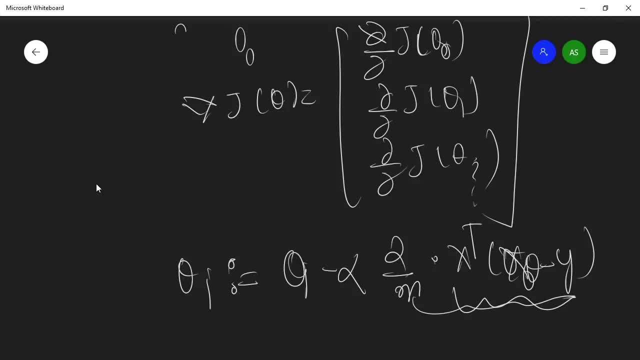 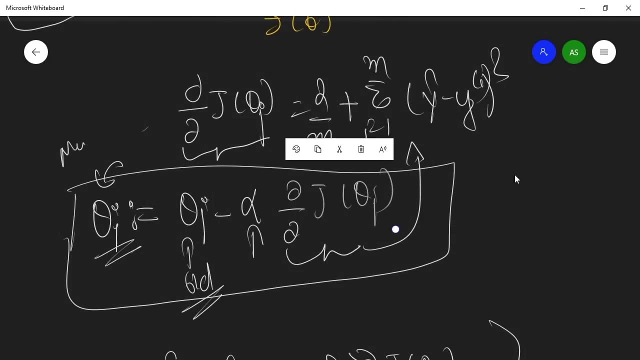 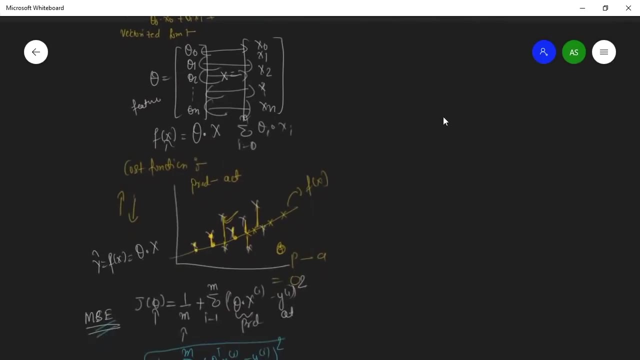 new um derived equation, which is a vectorized form. okay, and yeah, yeah, yeah, you can definitely use any any kind of this. this is totally okay. but for the vectorization you can follow or not, it's your point. but for computational power, just just, i've told to you. okay, so we have seen so far. 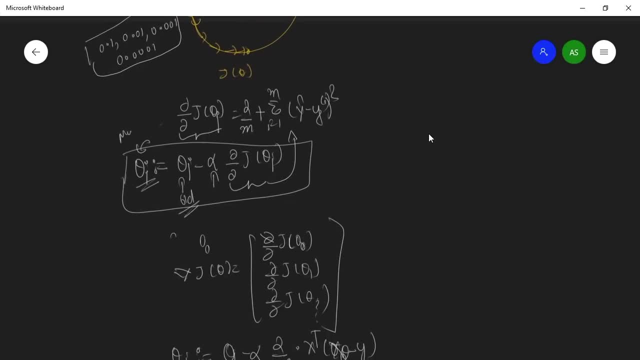 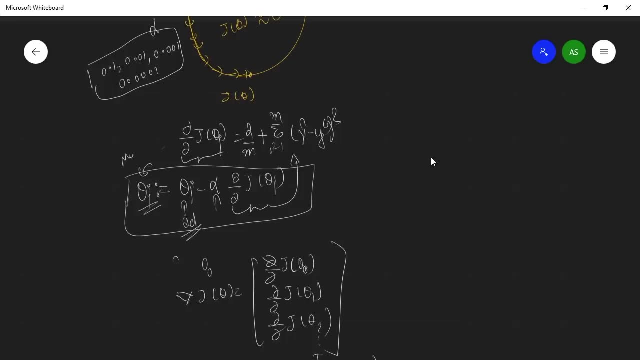 and now we are done with this. we have developed our lane integration model. we first have to develop the model from making predictions and then then we have moved further to check if our theta is good, then we have seen how to how to get optimal theta. okay, but you may think, ask here you see. 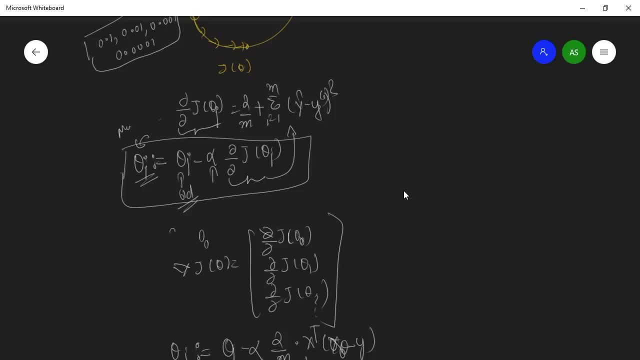 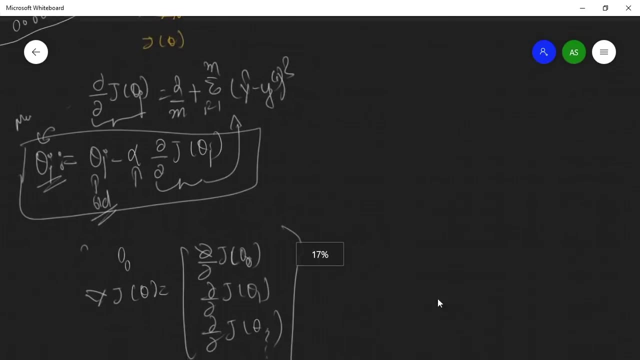 i have to do these kind of things. yeah, you have to do these these kind of things for getting your and and if i did, if i say truth, uh, the truth is in scikit-learn. you can implement this in three lines of code. you can implement this whole algorithm in the three lines of code. 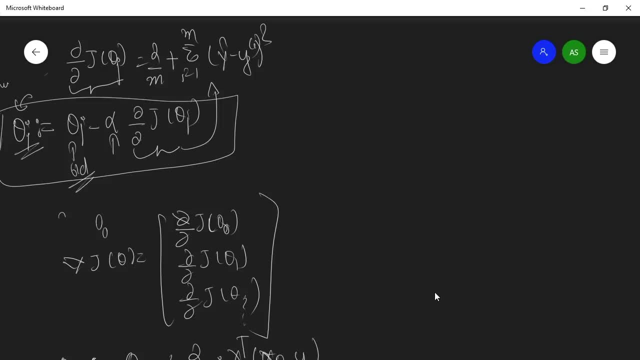 in some library but in programming assignment you have to implement from scratch this algorithm so that you can ace any kind of interview, okay, okay. so, um, you may ask: there is something called a normal equation. there is something called normal equation. that that i'm going to highlight a little. 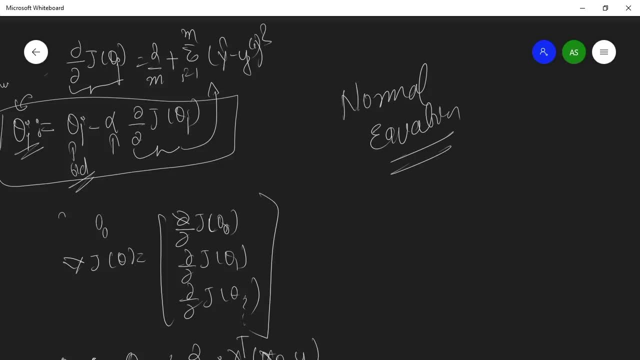 bit. normal equation gives you a better theta in just one way means: normal equation gives you a theta, optimal theta, in just one equation like this. so equation is: x transpose x, inverse of that, x transpose y, and from by you by using this and x. here is the data points, it means the features. so you can simply use this uh formula for getting the. 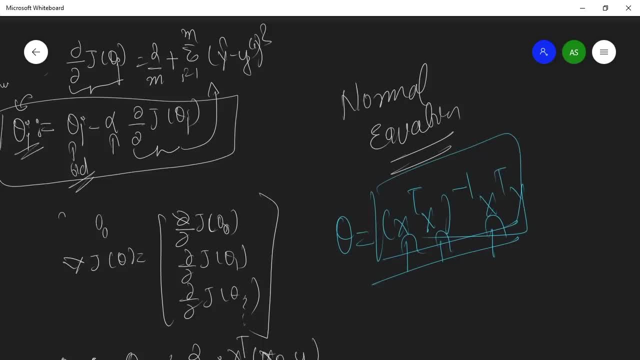 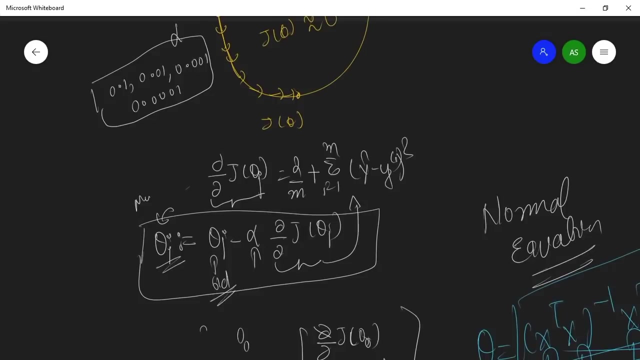 for for getting your optimal theta. okay, this is just the same as doing this, but not in every algorithm. it will work. it will only for linear regression. the normal equation is only for a linear regression and i hope, but having a good intuition of all those- because in interview they usually ask this, they don't, they usually talk about 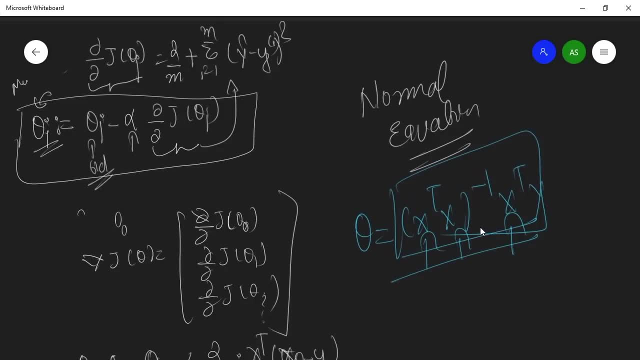 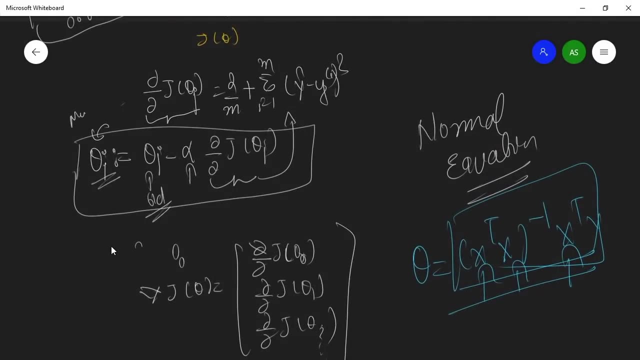 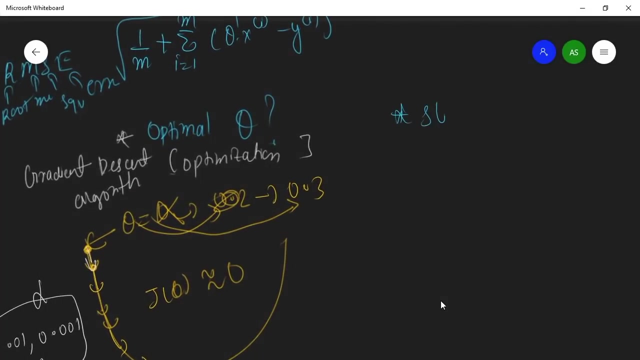 normal equation. okay, they don't all talk about normal equation. they usually talk about this gradient descent, etc. although there are too many optimization algorithm, some as like gradient descent in gradient descent. we have this and then we have a stochastic gradient descent. we have a stochastic which is called sgd. we have an atom optimization algorithm. we have rms prop, rms prop. 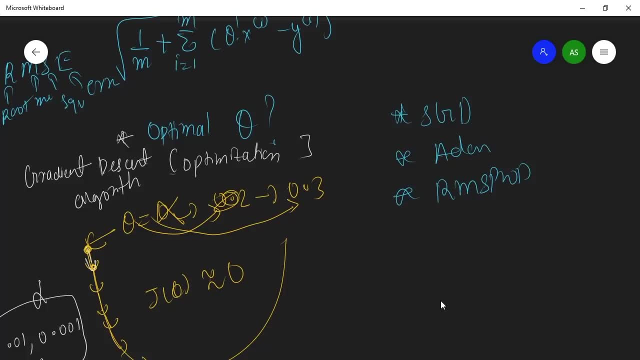 and then gradient with momentum, which will you, which you will see advanced level in- uh, i will talk about sgd, but atom, rm, rms, prop and some more optimization algorithm or convex optimization advanced, which you will ever see in deep learning. okay, okay, or you can head over the new era with the deep learning courses currently learning and 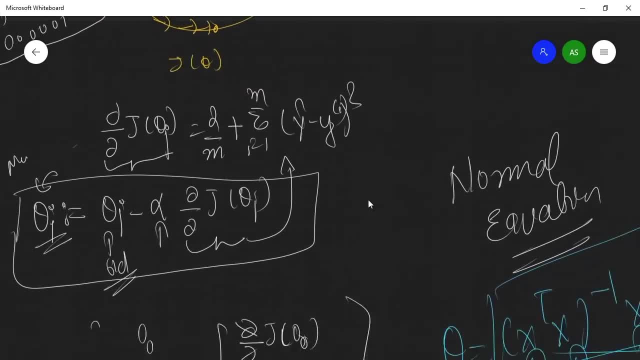 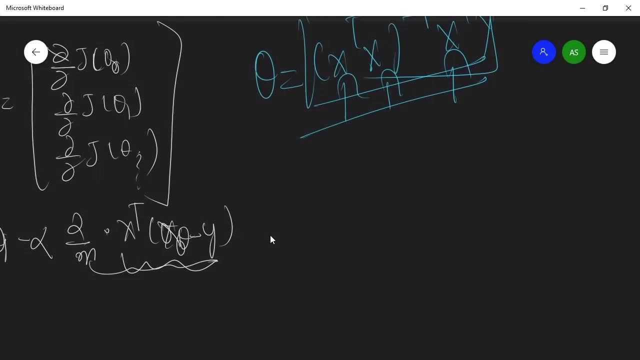 you can learn from there, okay. okay. so now we are done with this and let's little bit- let's a little bit- spend some time on to some assumptions of linear regression. okay, because in interview they usually ask why you wanted to choose this algorithm instead of this algorithm, or what is the assumptions of? 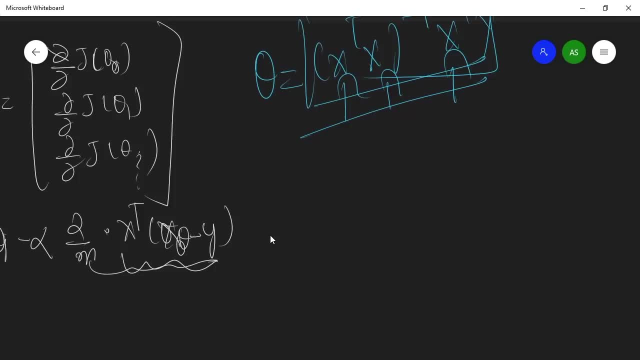 this algorithm, etc. so the sum of the assumptions, um of a linear regression it the issue. it should have a lean, linear relationship, linear relationship, the data should be linear, the data should be linear and no or little multi-collinearity. the co, the correlation between uh variables would be. 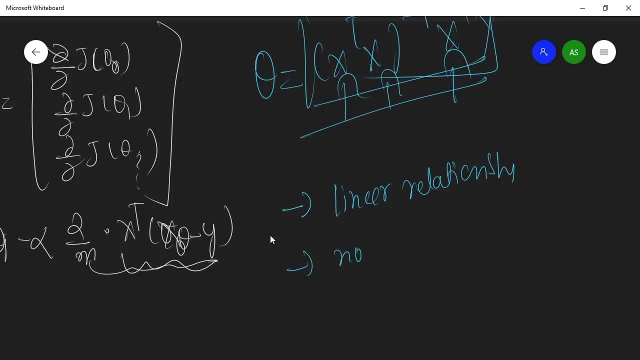 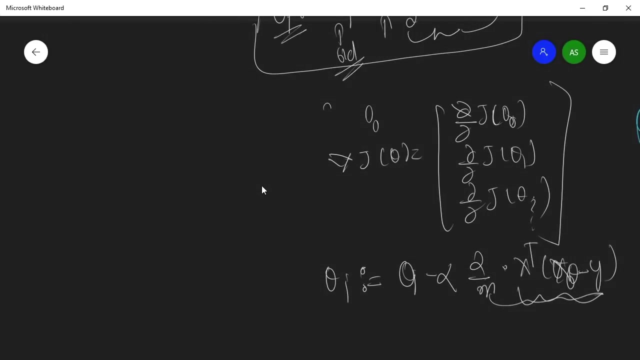 uh, no, nothing, okay. no, or little multi-collinearity, multi-collinearity- okay, you can see a seo internet for more. okay, so now we have seen some assumptions, but i want to, just i want to give you the things what is independent and dependent feature. independent means the size of the house, the pr, the number of 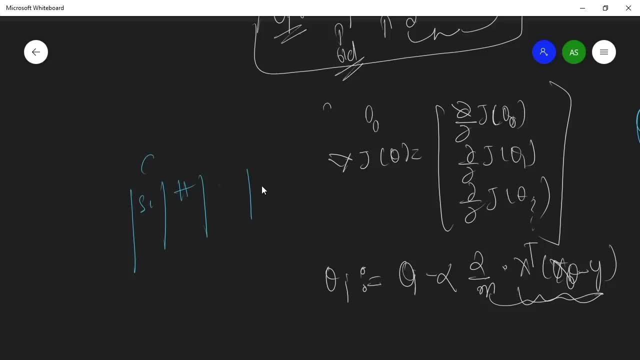 fans and number of, let's say, the bedroom. so these are the independent feature, because they are not independent to any feature for the kind of any value. but the target variable y is dependent on feature, so that's why the target variable is called independent- sorry, independent. and these 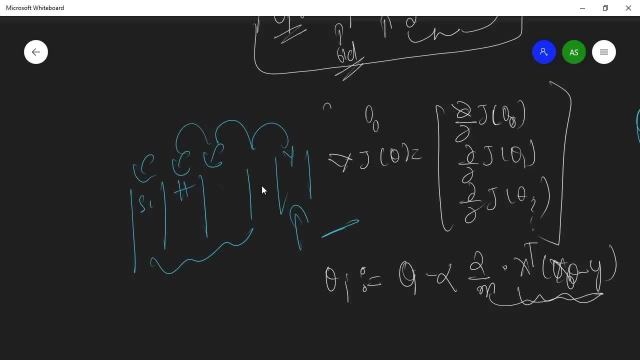 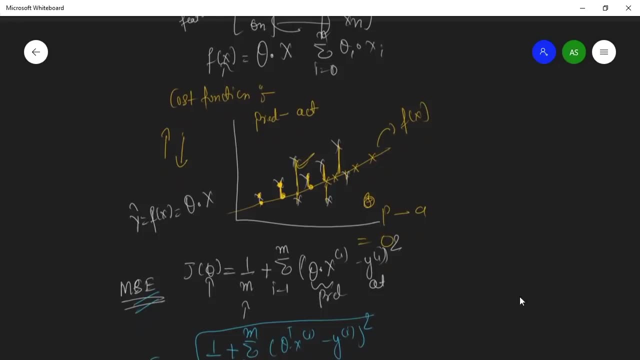 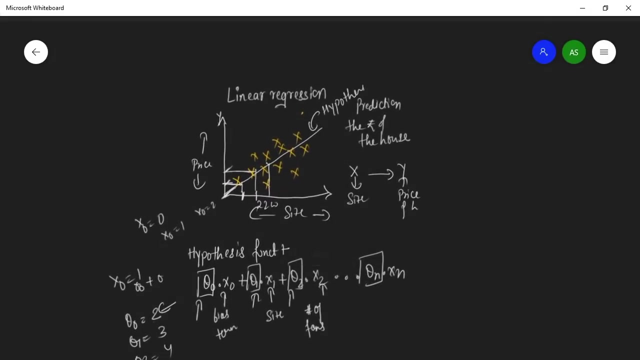 are called independent. okay, so this is just a casual information to know, because everyone talks about this. okay, so now i think that we have talked very, very much in small amount of time and i hope that you really, really enjoy this tutorial, and i'm putting all my effort. then you can go on to. 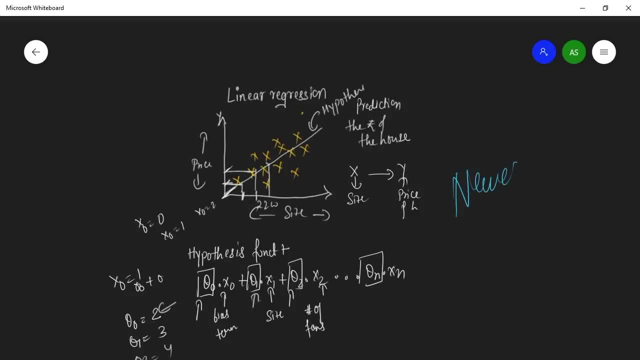 my youtube channel, new era, new era, and you can subscribe that youtube channel if you want, okay, okay, so, um, now we have talked that and in the next section i'm going to go over, uh, in theory pattern. i'm going to go over polynomial regression. but let's spend some more amount of if i have time. 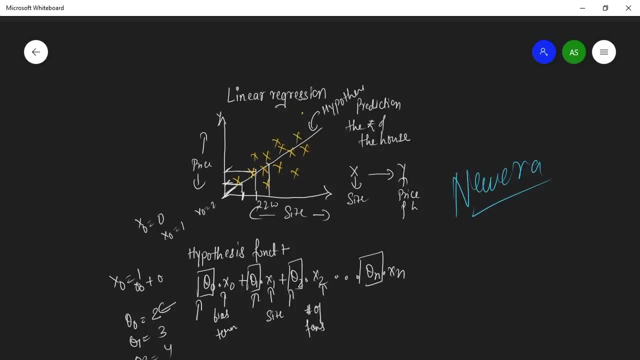 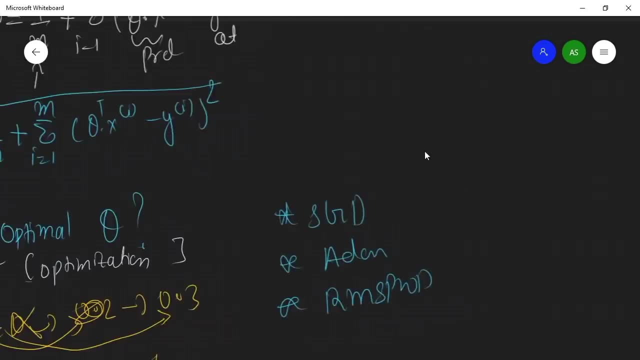 let's spend two more minutes on the polynomial regression. okay, so there is something called the polynomial regression, as we have seen. the assumption: the data should be linear. but let's, our data is not linear, then what we do? okay, then what we do. so let's say, your data will be like: 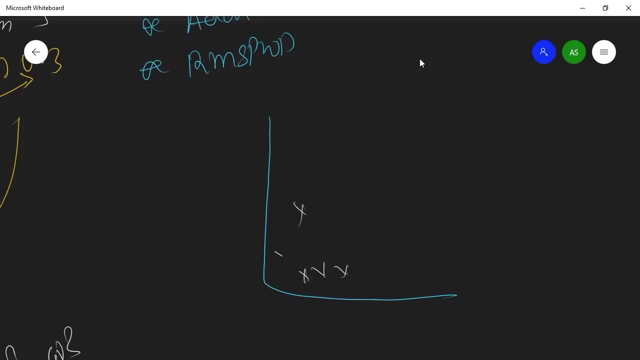 let's say, your data is like this, your data is like this, your data is like this. so you, if you feel fit like this, then it is obviously overfitting. so what you do? you just simply transform your data. you simply transform your data to be like this into: 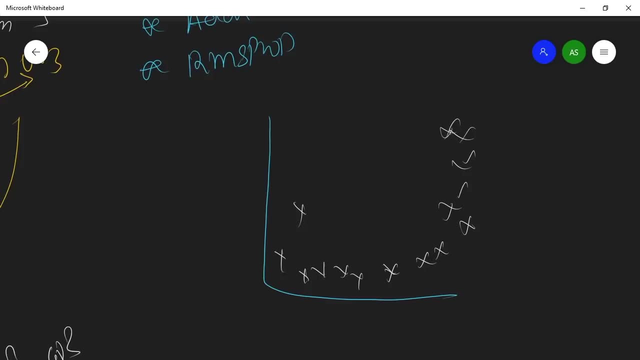 the quadratic form. you enter the quadratic form to be, you just simply transform this one one degree to the two degrees, so it will confirm like this: okay, so you two will be transformed as, let's say, four and six, three, maybe transform as a nine and whatever, but it was just so. I'm taking an example. okay, 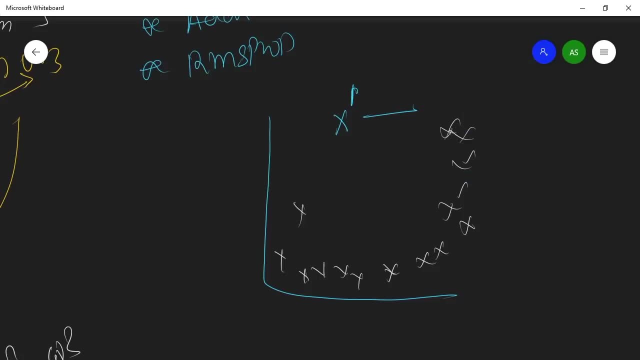 if you transform your data to be fitting over the linear, so you transform your data to be fitting over linear. now your algorithm will be fitting like this: okay, so now I hope that you have gone everything about Polly. now we will talk about it and do some Boston house class prediction and then 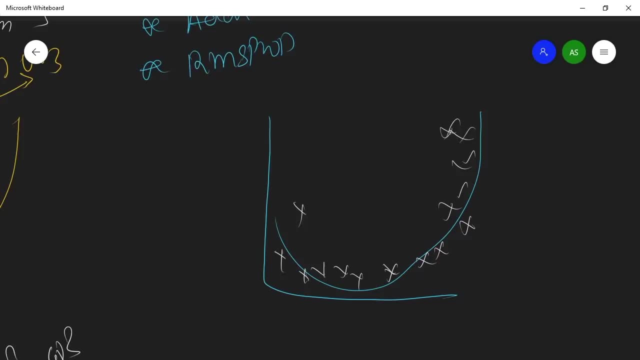 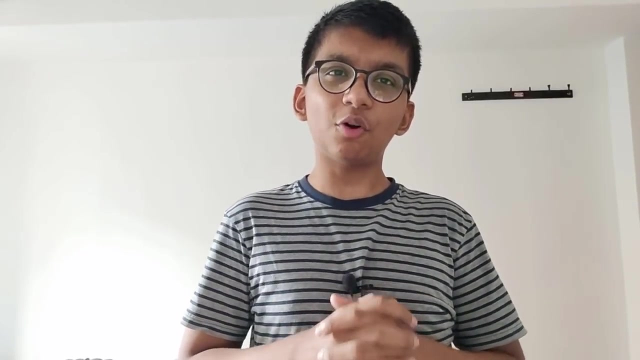 we'll move on to the regularized linear models. okay, so let's head over to the Boston house prediction and then we'll move on to be the regularized linear models. okay, so now we have seen linear regression and we have done one project. now it's time for getting your hands dirty in the programming assignment you. 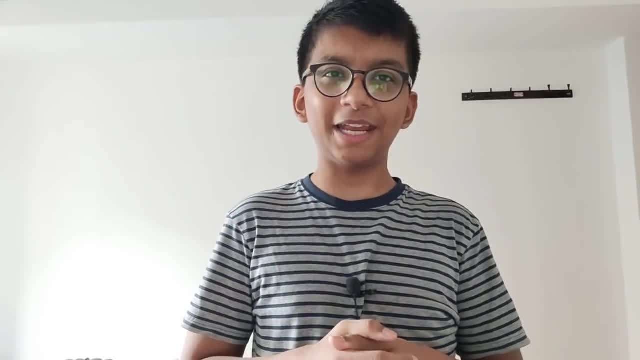 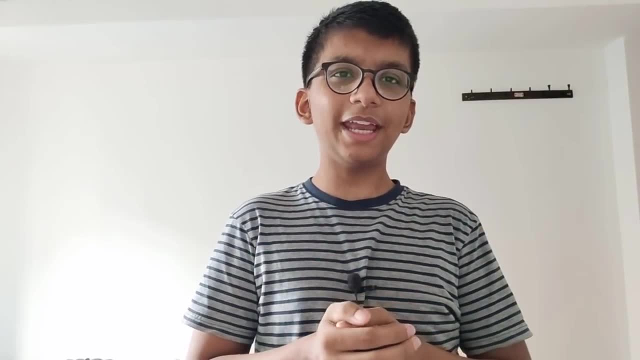 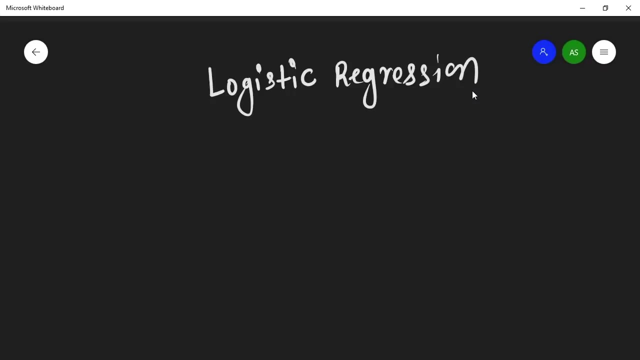 will be able to find the programming assignment description that marks below in the assignment page. okay so, And now we will start with logistic regression after doing assignment at the command command game and follow up with this course. so now we'll talk about logistic regression, and I hope that you will really enjoy this. okay, so now we 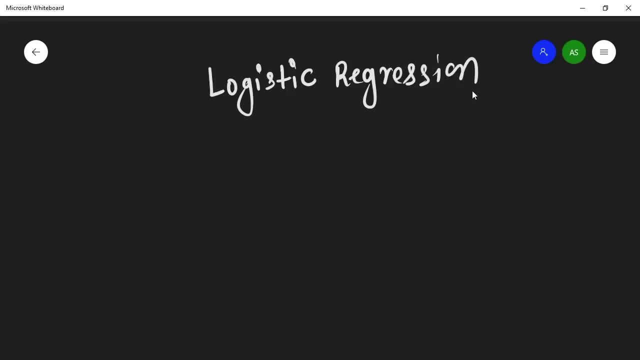 have seen linear regression, which is one of the regression algorithm. now we will see one classification algorithm, which is logistic regression. don't worry, don't think that this legend reaction is a regression algorithm. know, it's a classification algorithm. so, because the name is logistic regression, regression- because the underlying working of this algorithm is same as is. 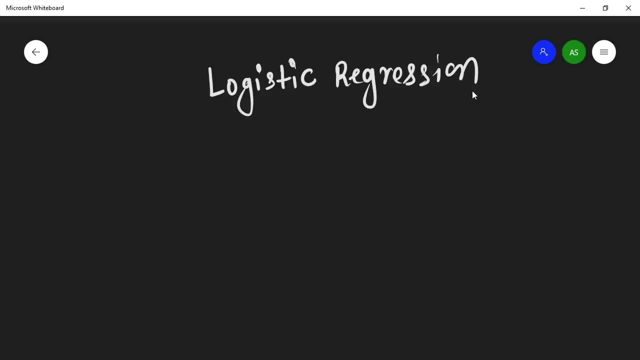 is something similar to linear regression, okay, so you will get to know about this, how it differs from linear regression, okay? so before that, let's let's be clear about- we are on the same pace about- classification. what is classification? okay? so this is a great question to ask to yourself: what is? 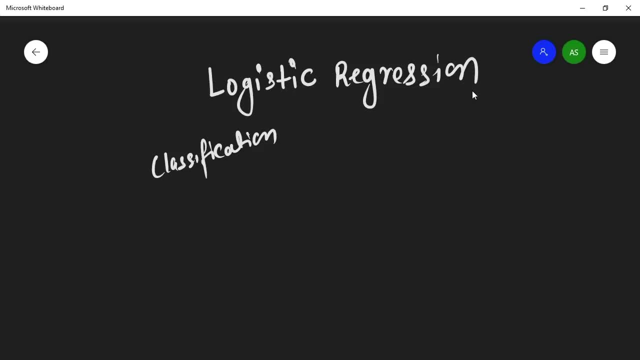 classification. so let's see an example: when, given a range X, you want to classify this image as a cat. if it is cat, then we will name it a zero. if it is non cat, then we will name it as a one. okay, so this is a decreed value, our. 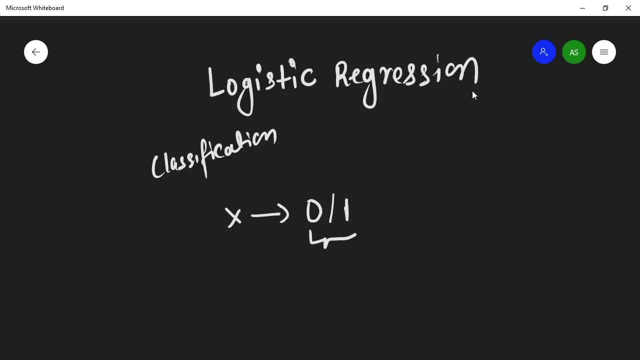 output is a decreed value and the classification is a supervised learning approach. so this algorithm is a supervised learning algorithm. so here we know what our output should look like. so here our output is a decreed value, so we can classify this as a classification task. okay, so that's the classification and something called the binary. 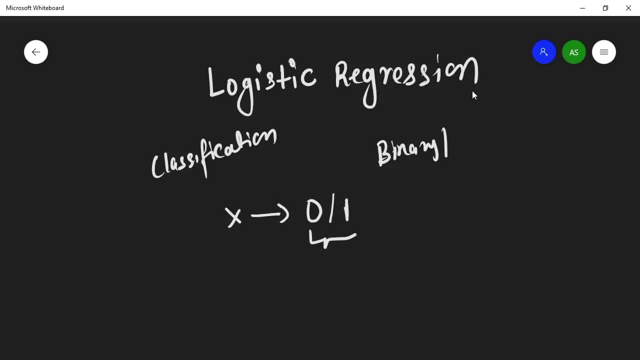 classification and we have a multi-class classification, also called a multi-class classification means maybe the person has a cancer, person has a pneumonia, etc. this means a decreed value. your output is a finite value, value. okay, so we have this classification and this tool, so now it's time to study about. 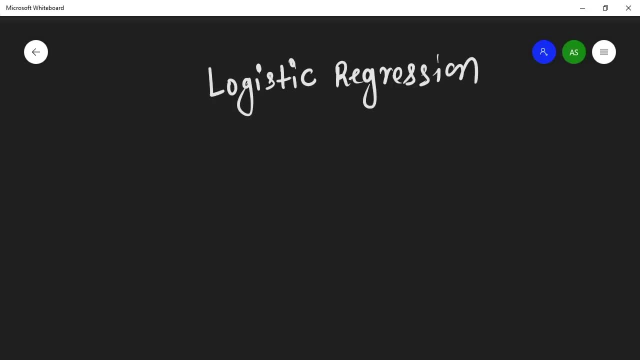 legislation in detail. and so what we do in legislation, we classify the data, we classify in the data. so let's start with hypothesis. in linear regression we have a hypothesis which is H of X, so let's denote as Hf x equals to the n legislation. we also do the same: theta0 times x0 plus theta 1 times X, 1 plus theta 2 and theta 3 and theta 6 and theta 7 and theta 8, and in the third symbol we have similarly an intersection popped in idols. we are identifying which is behavior on the path ofiani, because that'sмотр of GT, what schools are means, what means it. remember he 수 Behavior, we. 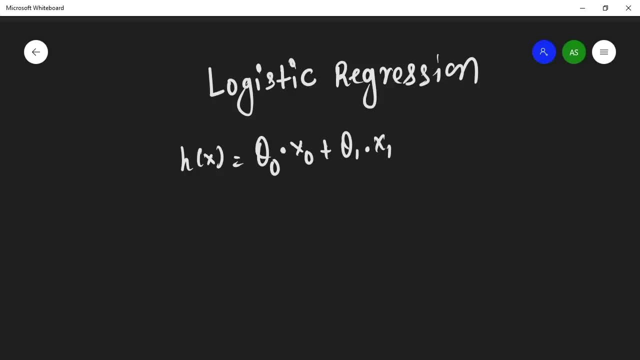 plus theta 1 times x1, plus theta 2 times x2, all the way around to the theta n times xn. okay, so in linear regression we are doing the same for drawing a straight line, and here we are also doing the same for a function, and this is, and this, this, this will be for linear regression. 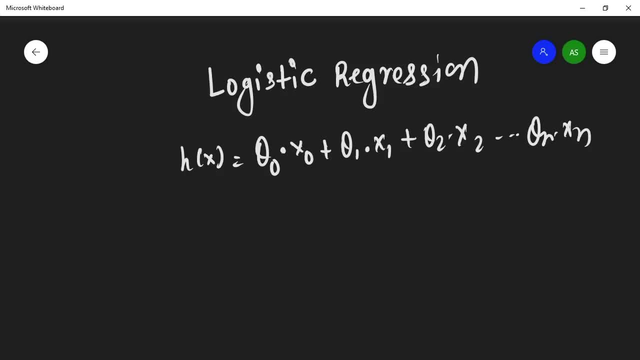 and the same for a logistic regression, and this is the step. this is the first step for hypothesis, and the second step of hypothesis means the model predicted value equals to the sigmoid of h of x, so let's denote this as a short form of z. okay, so this h of x is g, and g here is simply h of x. 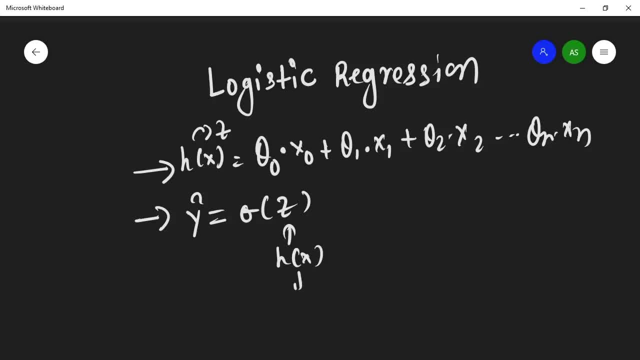 and h of x is here theta 0, all the way around to theta n, so you can name it as a theta transverse x. okay, so you just here. you just do the sigmoid of your h of x, which is: which is your um prediction function. so you just do do the. 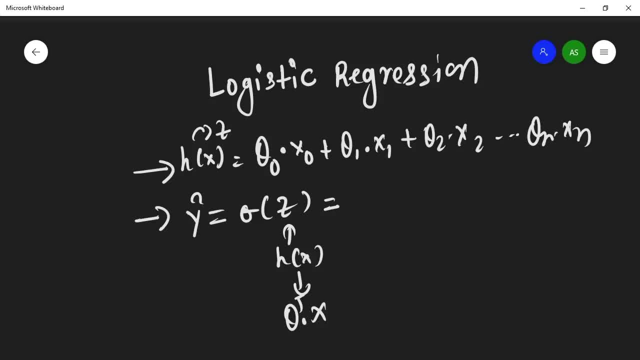 sigmoid of this z and you get your output and you get your output. so let's say what the sigmoid does? you get your output from logistic regression and this output makes the out this, uh, the this, whatever the output came, let's say 22, 22 to between 0 to 1, then the sigmoid, the if, if you 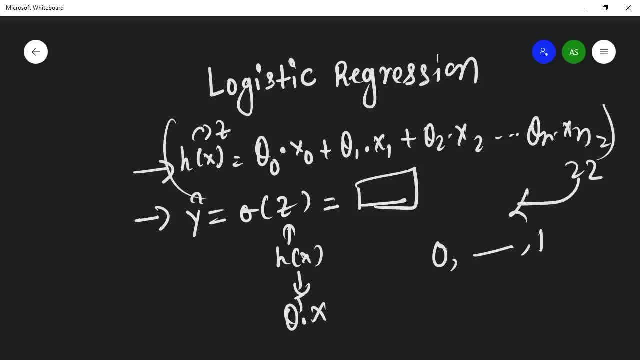 apply sigmoid to this. you apply sigmoid to this, then it. then it makes your output between the range of 0 and 1 and you and you set the threshold. if, and you set the threshold. if your, the model particular y hat is greater than uh y hat is greater than 0.5, then this picture is a cat, okay. 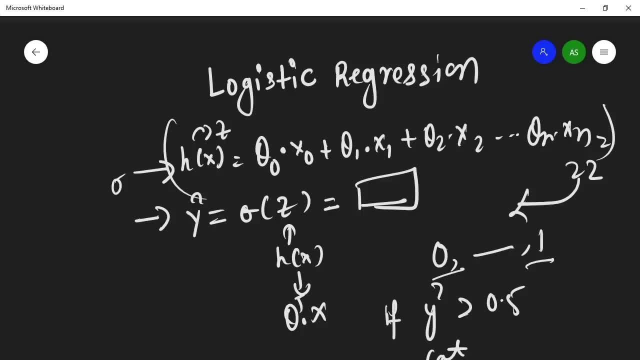 otherwise, if it is more than 0.5, then it is a non-cat. okay, and this is what it. this is what we are doing in linear regression. we are just. this is this, this was our hypothesis, but in addition, we add this to the logistic regression, which is the logistic regression, which is the logistic. 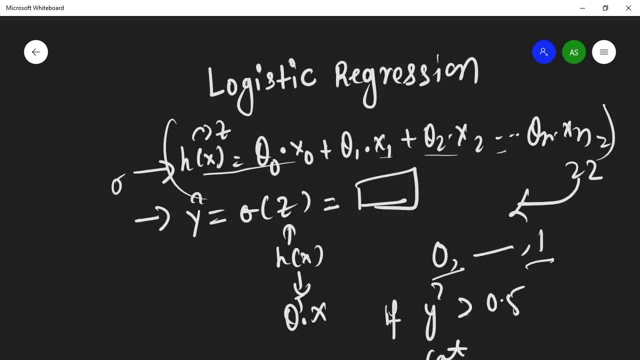 add a sigmoid to our h of x. and the reason why we add sigmoid it's it's totally because that we want our output between 0 and 1, in the range of 0 and 1, so that we can make prediction like this. so you just you apply sigmoid- and formula for sigmoid is 1 over 1 plus e- to the 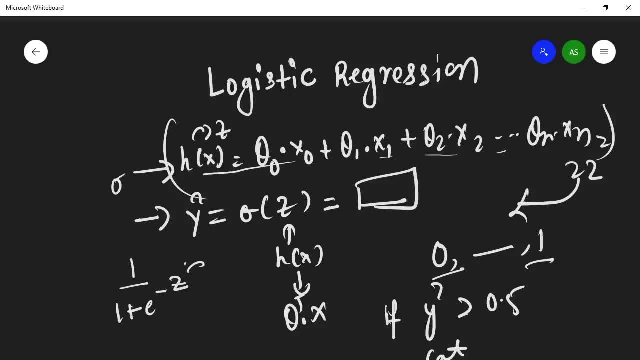 power minus z and z, here is h of x. okay, so this, this, this will be your whole hypothesis, this is your prediction function. okay, now you just put the z and theta. you have to one: learn theta. you have to learn these thetas, which is called the parameter weights, again the same as a. 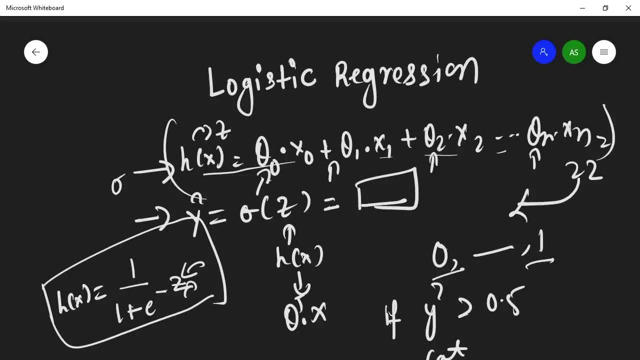 linear regression. okay, so what we are doing, we are just doing the same as a first, the first step we are doing same as a linear regression, and then we are applying a sigmoid at that h of x and then we are getting the output, which is the which is in the range. 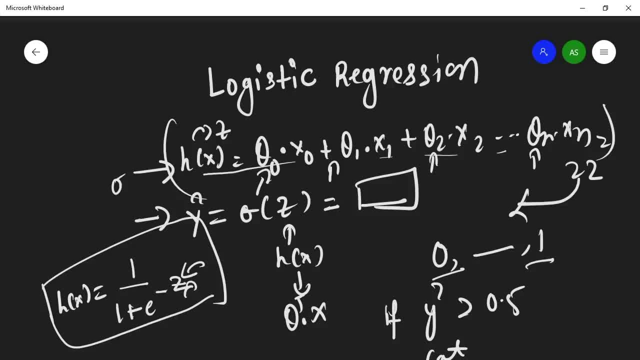 of 0 and 1 and we set a threshold. 0.5 is a threshold and if the particular, the model predicted y hat from this output between the range is greater than 0.5, then it is a cat. otherwise, with smaller than of 0.5, then it is a non-cat. if you want to be a more strict, then 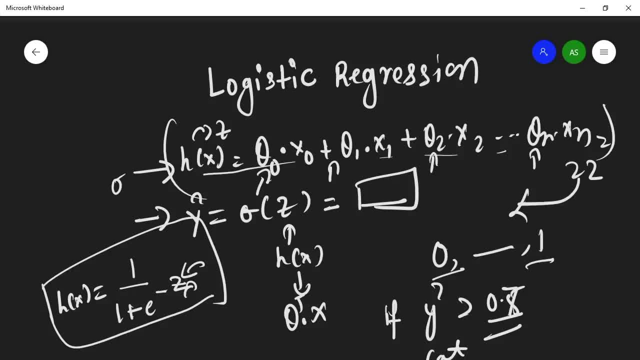 you can make 0.7. the probability is greater than, as it is, 70%. okay, so let's say you're more output like this: zero point of 80. okay, so it's two is equal to zero point seven, and then you get the 80%. your model is saying that particular, this image is a 80% accurate, that it is a cat. okay, so. 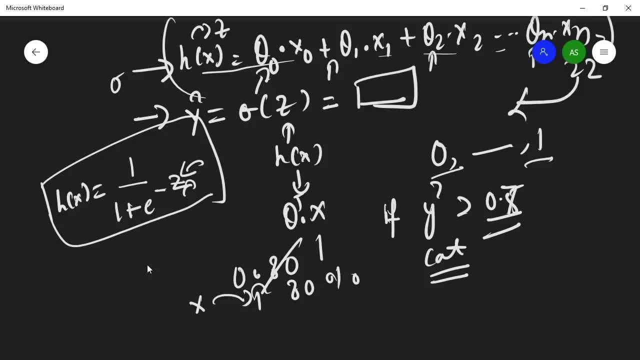 you just make it as a one round of two. one means it is a cat, otherwise, if it is a 0.40, then it's 40%, that is so you make it as a non, okay, so this is the basic thing that you should understand is. 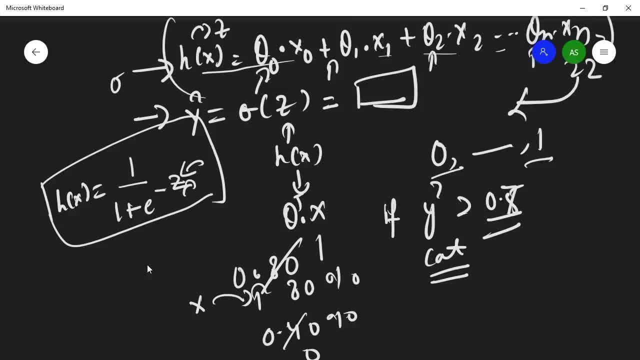 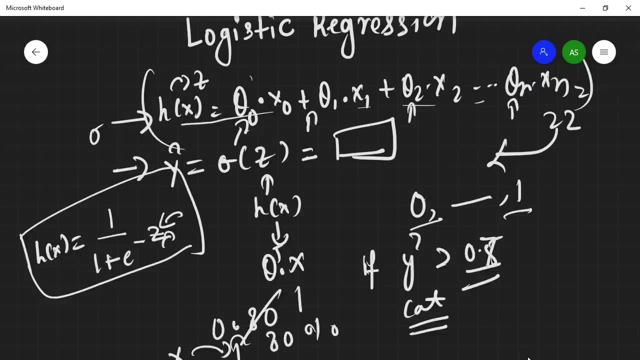 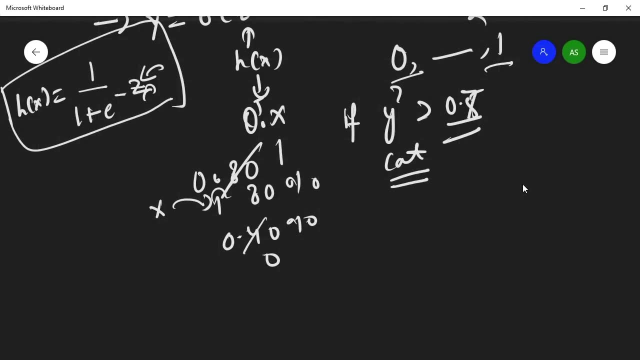 a prediction function that we have made and, again, you have to only learn these thetas. it means we have to get these three, these thetas together to get our good output. okay, so this, this was a legit regression and I and the hypothesis for legit regression, okay. okay, so now in linear regression, we have seen something called a cost function. 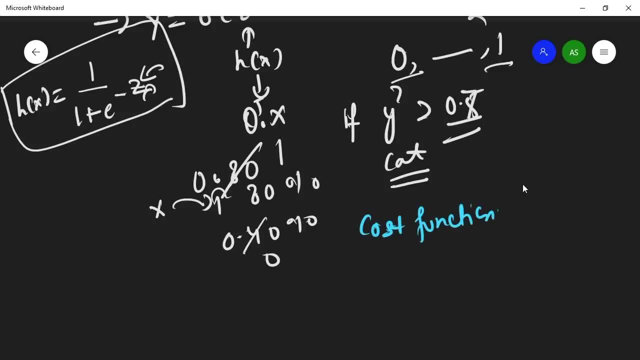 something called as cost function, and cost function simply what it does, it simply say, gives you the accuracy of their model. means if the cost function is very, very high, then then your model is very bad. if your cost function is load, then your, then your, then the new model is good. Okay, so it helps us to evaluate your model. Okay, it's the. 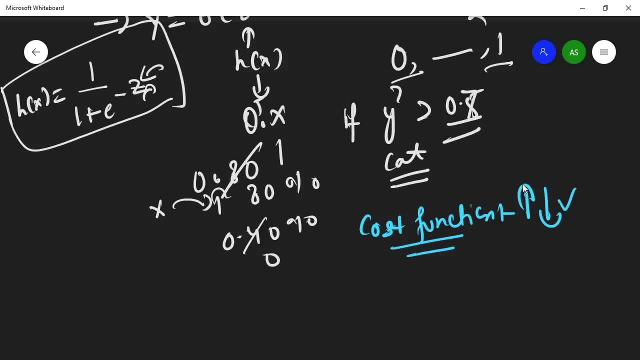 loss function. It should be on the cost function. for a good, for a good model. your j of theta means the cost function should be approximately equals to zero, Okay, okay. so in legislation we have defined a little bit different this cost function like this, Let's do for one. 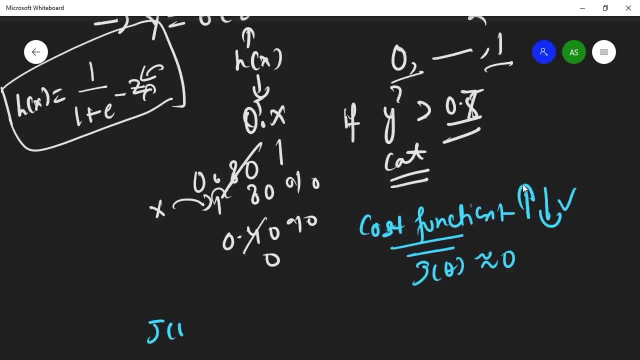 training example like this: j of theta. j of theta equals to minus one times yi. the log of edge of xi. edge of xi plus one minus yi. one minus yi. log of one minus edge of xi. Okay, so this, this is your cost function for for one training example, and you can see over here that we have a cost. 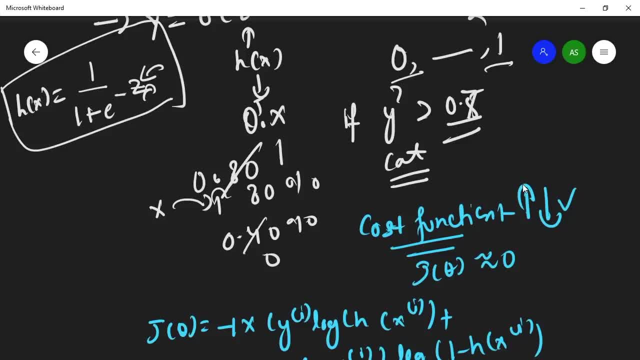 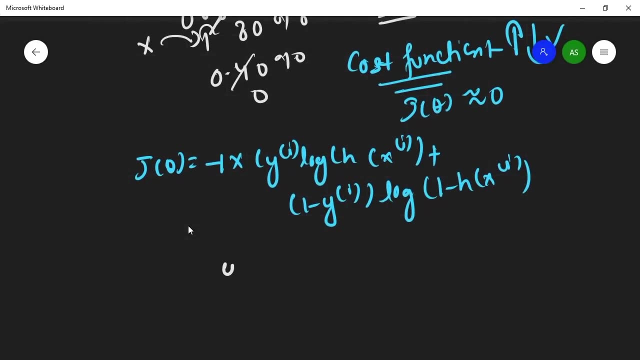 one minus yi One times the yi times the log of edge of xi, and one minus yi times the log of one minus edge of xi. So what we are actually doing. so let's break down this equation and let's understand step by step. Okay, so what we are doing Here? we are doing yi is the ground. 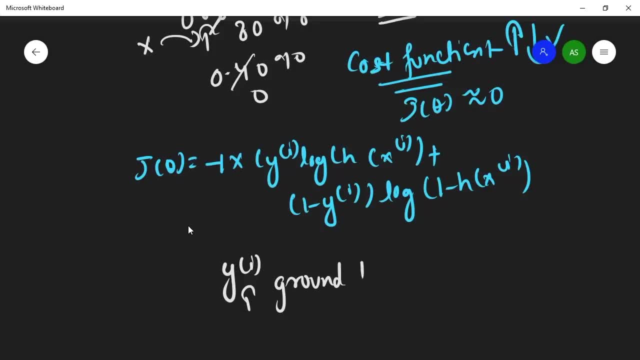 truth is the ground truth, ground truth and edge of xi. edge of xi is your model predicted value, which is the model predicted value, And it's just taking the log of your model and multiplying with the yi. Okay, so let's say your y is equal to zero, your y is equal to zero and your model predicted y hat is. 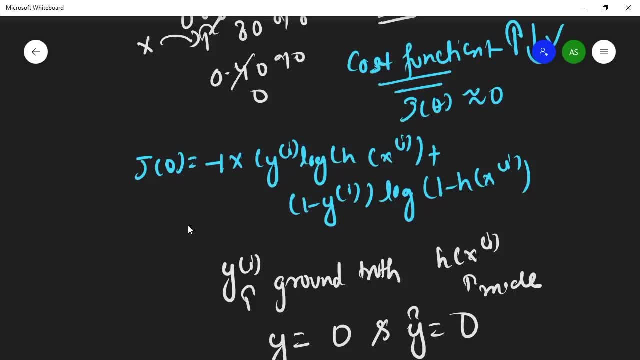 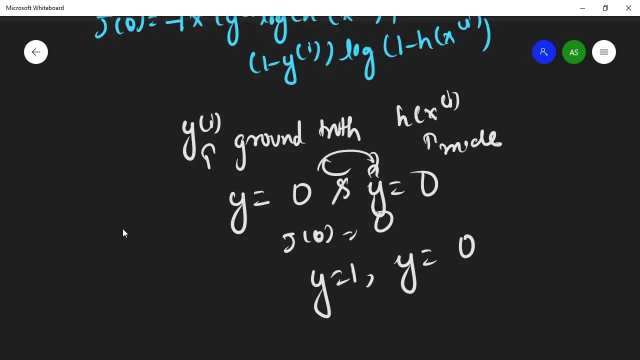 also equal to zero, Then your cost function will be approximately equal to zero, because they both are the same. So your cost function will be zero. Okay, it will be low. If, let's see your ground truth is one, your model predicted is equals to the zero, then this, this is a mismatch. the 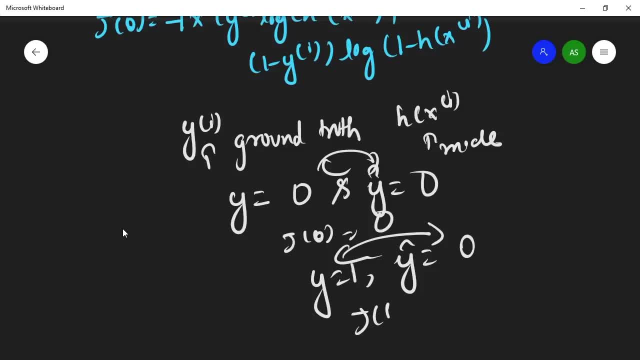 your model done very bad, so your cost function will be very, very high. okay, so this is what the basic integration behind this cost function and this is a basic formula, and again you can see over here that we do this kind of for oops, what is okay? so let let me write the equation for M training example: we have 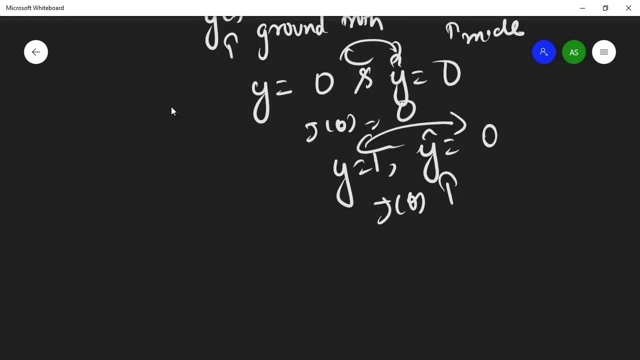 done for one training example, so let's do for M training example. so let let me write the equation for that. so you have a J of theta, you have a J of theta and 1 over M. 1 over M, I equals to 1 all the way on to the end. why log b fondo? 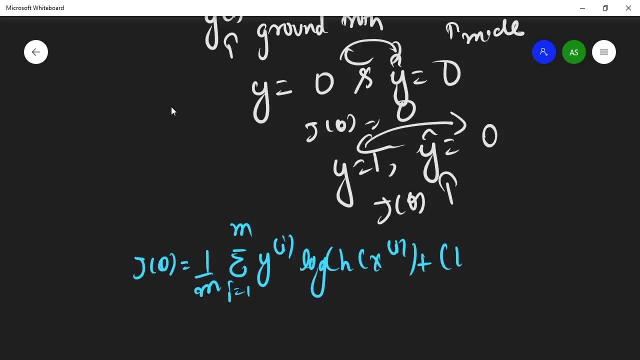 of Liu Victor plus 1 minus y. I the law of 1 minus edge of x, I okay. so this is a long loss, this reduced sum sometimes called s low log loss, exp. despite a three-pertussis equations. Example: my simple cat and vice a. 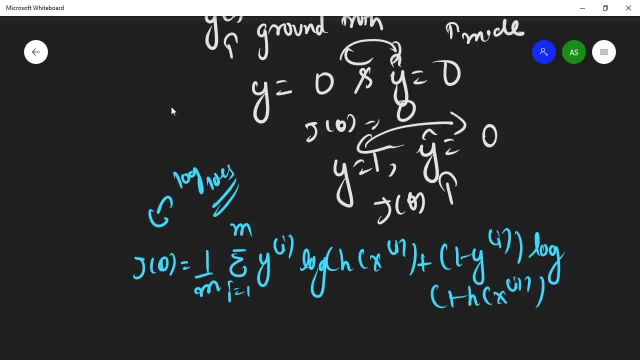 sort of frugal rule in lower either matrix or other different arguments given loss in terms of machine learning. So this is your cost function that is used to use as a loss function. that we have seen so far And I have given an example- when both the 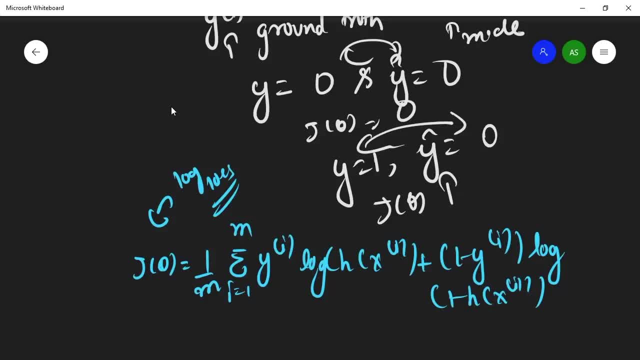 output is correct ground truth and your model predictor is equal, then your cost function will be zero. Otherwise, if it is different, then your cost function will be very, very high. So this is the cost function for your legitimation model. 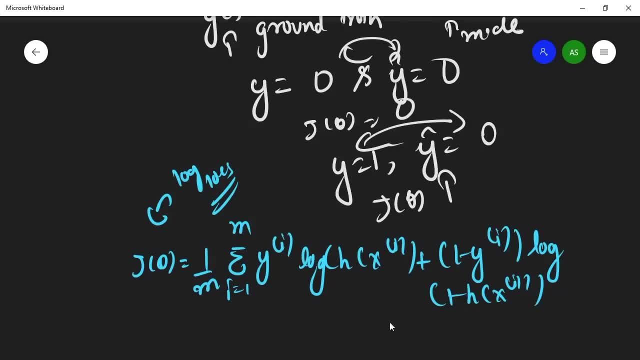 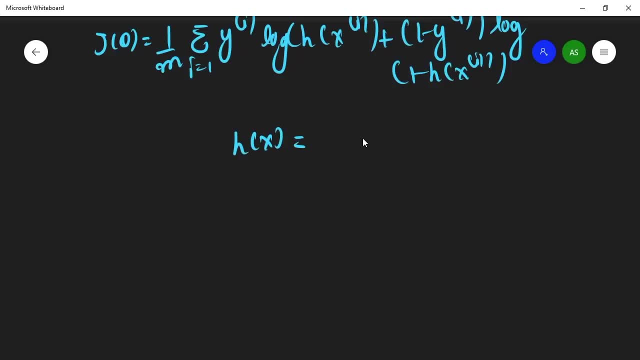 So let's recapitulate the two things: the hypothesis and your cost function. So the hypothesis is that h of x equals to the sigmoid of z and z. here is theta transpose times x. The dot product is in transpose times x and you just take the equation which is similarly. 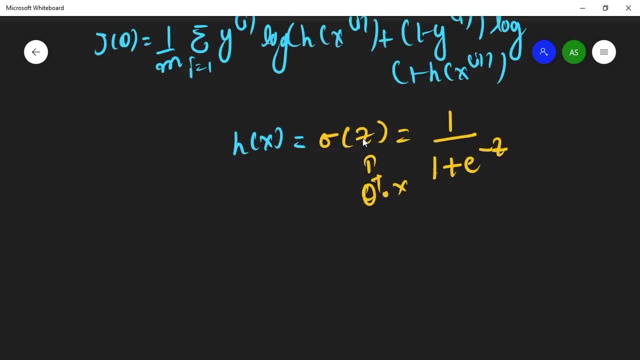 equals to 1 over 1 plus e, to the power, minus z And z. here is just theta. transpose x, So the theta contains the parameter weights and x contains the x1,, x2,, x0, x1, all of them. 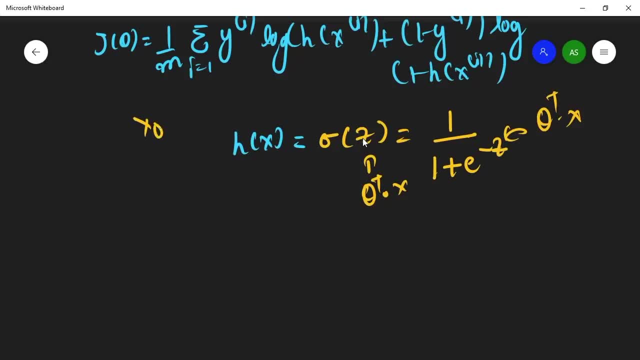 to multiply And by convention we are using x0 equals to 1.. You can rewatch that linear regression section once more if you are getting a little bit confused because I have gone a little bit slow there. So the gradient is important for getting the good, for reducing. 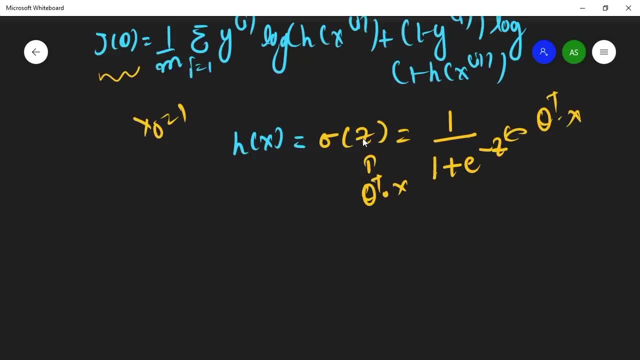 this theta. So the gradient is important for getting the good, for reducing this theta. So the gradient is important for getting the good, for reducing this theta. So the gradient for being that j or for getting the good optimal parameter, we use gradient decent algorithm and gradient descent method does the same. Here is your theta. we have the. 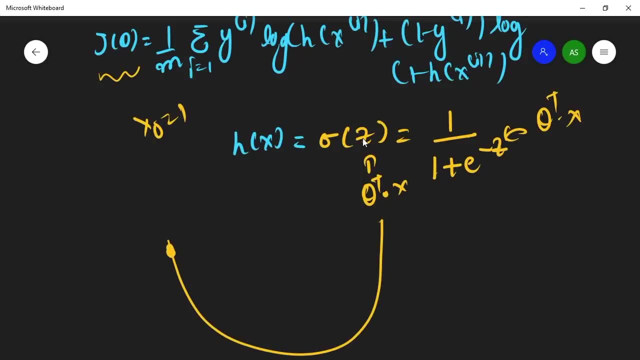 cost function very, very high. This is your cost function diagram. So your cost function very, very high when your theta is here. When you change theta, your cost function little bit decreases. over here Again, you change, again. you change. This means you are taking. 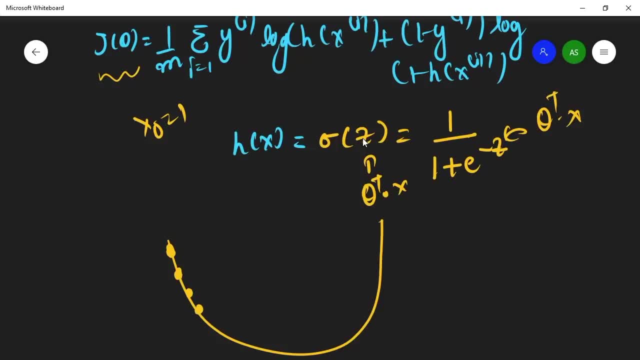 out the gradient of your cost function and checking if it is going down. If it is, then you just update your parameter. Let's say theta zero was here to be theta 1, to be zero. 2. then you update it out. want to be little bit 2.1. then you cost and 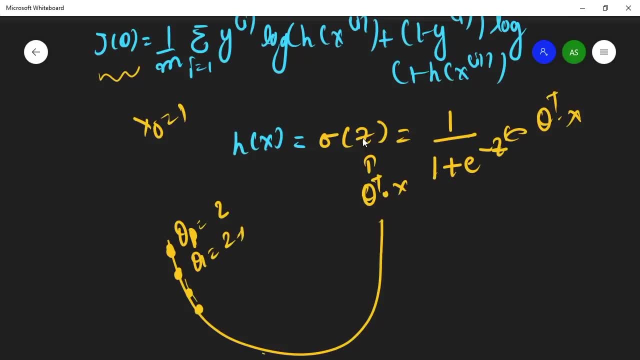 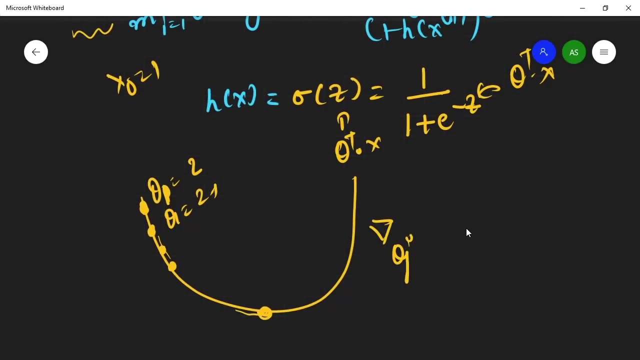 decreases. then you do the same for getting into the global optimum over here. okay, like this. okay, so here's an equation for the same. so how's the equation? you just, and I'm doing it here: theta J for J is just means the taking of the partial derivative J of theta equals the 1 over M. this is the. 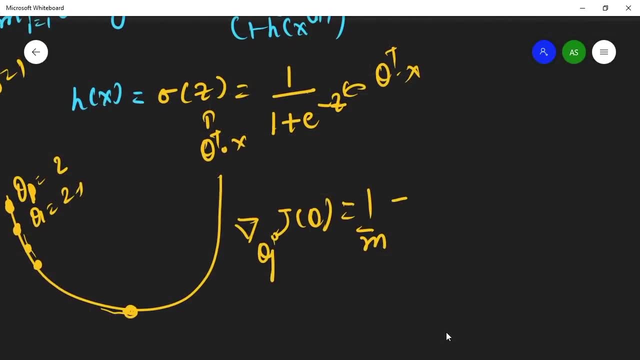 equation after deriving from cos function. this is the equation forms: I equals to 1, all the way down to the M, X, I minus Y, I, okay, and then you just add up some some kind of X G times, X G, okay. so this is your cos function, that's it. 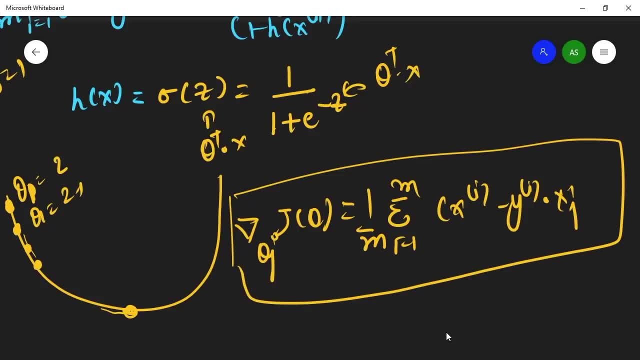 this is the taking of the partial derivative, although it might change little bit because everyone has a different kind of about this, but it's similar to memory of that. okay, and then you just take out the partial derivative of your cos, function J of theta, and then you 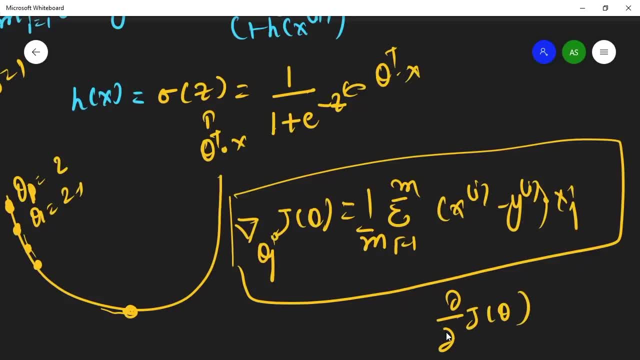 update the theta by taking out the gradient. then you update the theta like this: and theta J minus the learning rate alpha, and this is your previous theta and this is your new theta means updated theta, and you're taking out the partial derivative of your cos function and it's just the same. you just 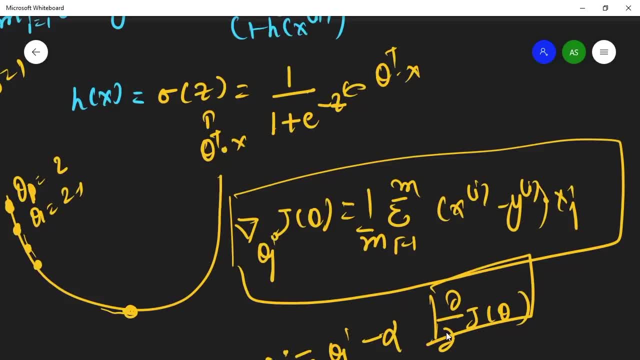 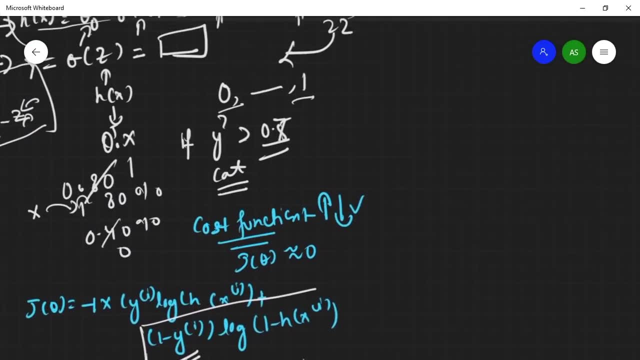 tweaks your parameter and checks if your cos function is decreasing or not. okay, okay. so we are done with the less information and I really hope that you enjoy it. so let's recap, recap and then little bit go for the end of vectorization of this code. okay, so what's for? you're seeing, we have seen. 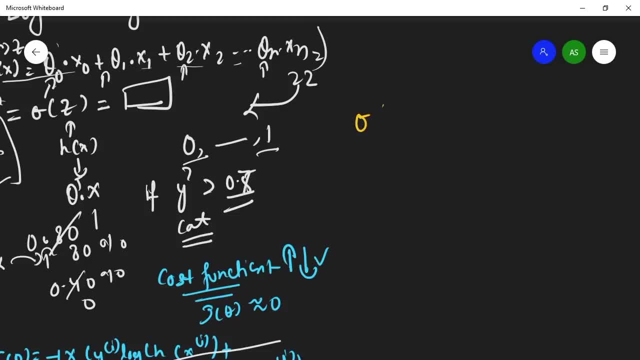 hypothesis. and the hypothesis is given by the. this segment of C and is a simple 1 over 1 plus e to the power, minus C and Z. here is theta transpose to X. okay, and then what you do? you have a cos function for getting the X to different. 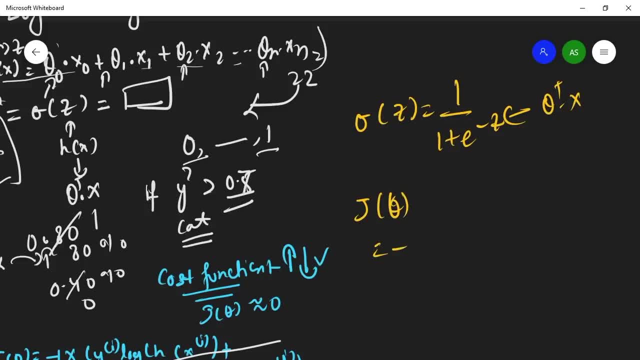 model this: J of theta, which is equal to the minus one times Y, I, and then you just get 1 over Venus to x��� de ta, transp Guide ce. the law of this is that you see far and and for entering example, you have that and the gradient decent. you just update this, will you just a bit of data and 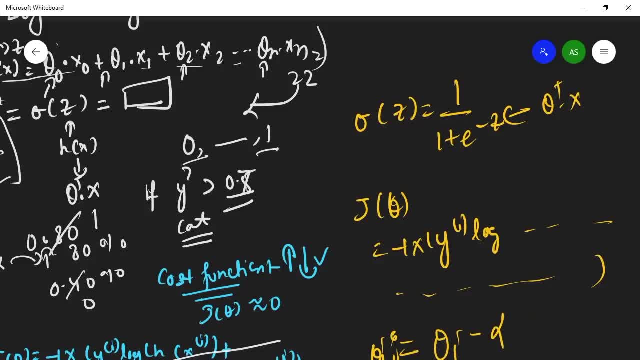 data say, minus the learning rate alpha and is: take out a partial derivative of your cost bunch of J of theta, okay, and the alpha here is simple: the datum is the range of learning that we have seen in linear regression. okay, okay, so we have seen so far and now it's time for getting into more detail about 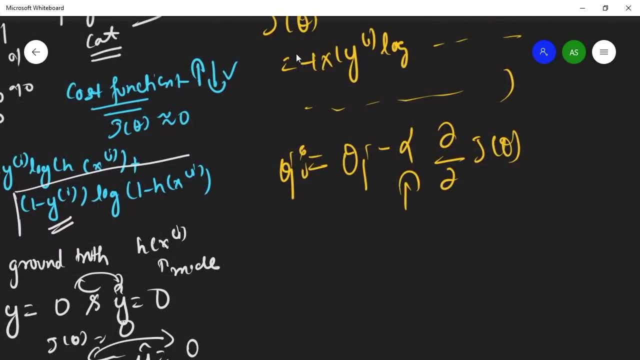 vectorization. what's the vectorization means? so vectorization means is you just do you here you are taking some amount of time, but if you want to do at once, if you want to do all the calculation at once, so here is a vector, vectorized code. 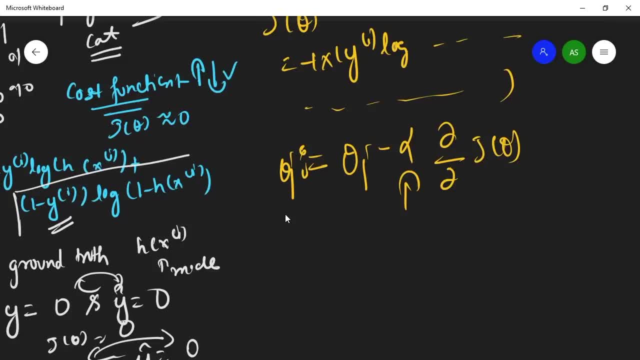 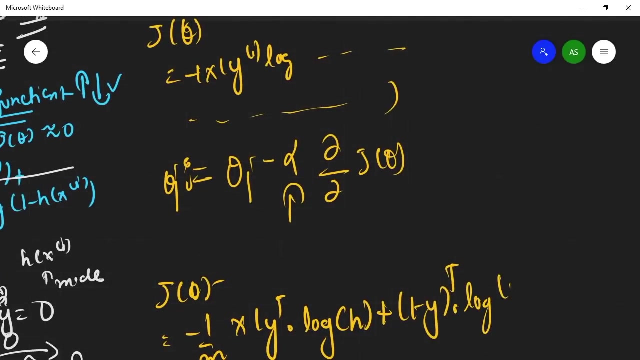 for when the cost function. okay, so I'm right writing for cost function, which is a vectorized code. so here it is: minus 1 over M times Y. transpose times the taking a dot product within Y. transpose dot H plus 1 minus Y T. the transpose dot log of 1 minus H. okay, and H here is your model predicted and Y here. 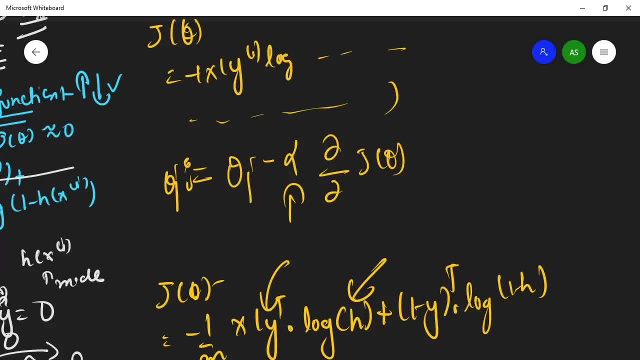 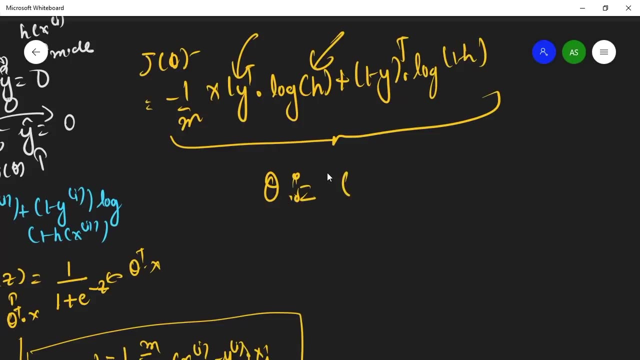 is a ground truth okay, and we had just vectorized the code little bit to get your job job done. okay and a good way okay. so that gradient descent also a little bit vectorized. so here is the gradient descent theta: this theta minus the learning, this ciones derivative, all the learning rate, alpha and times, X transpose dot X minus. 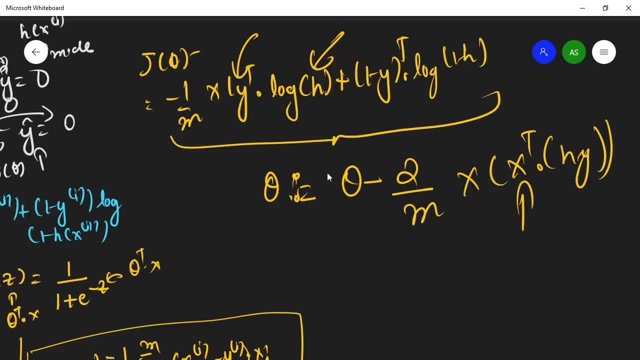 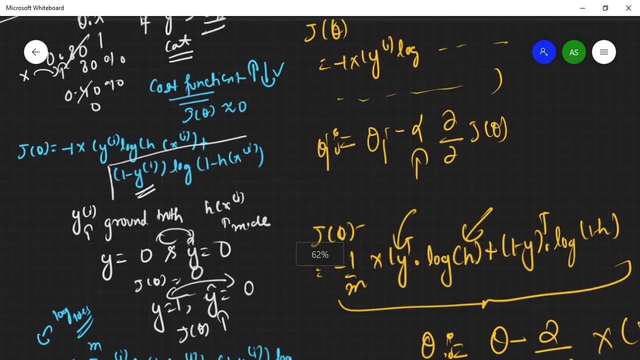 Y. okay, so this is then. this is what you get after deriving your partial derivatives. okay, so this is the basic thing that you should give a mind about when performing logistic regression, and I really hope this will have enjoyed till now and And now, if you can see, let's summarize a little bit so that you can get a better feel. 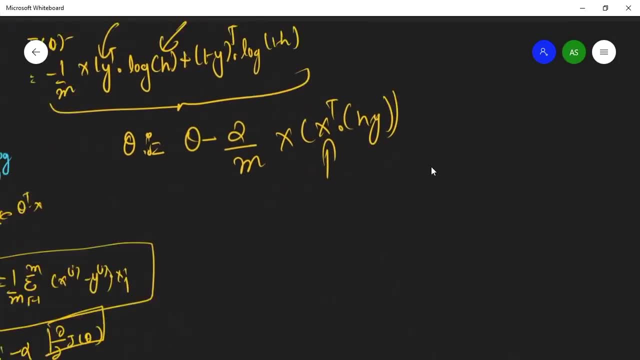 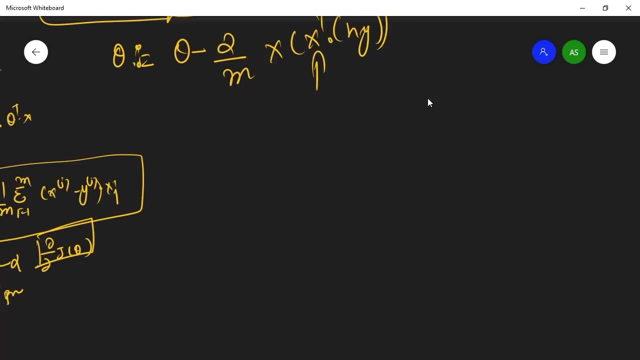 what we have seen so far. Okay, so the G-situation is a classification algorithm that will classify our example, that will give the probability. after you just apply the sigmoid to the Z, then you get the probability means in between 0 and 1, you just get between 0 and 1,. 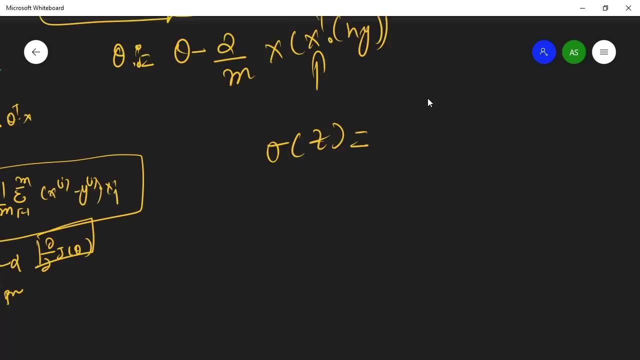 and then what you do? you simply take a threshold, means if your output is greater than 0.5, then you make it as a 1,, otherwise you make it as a 0,. okay, As a convention, we take 1 as a positive indication. 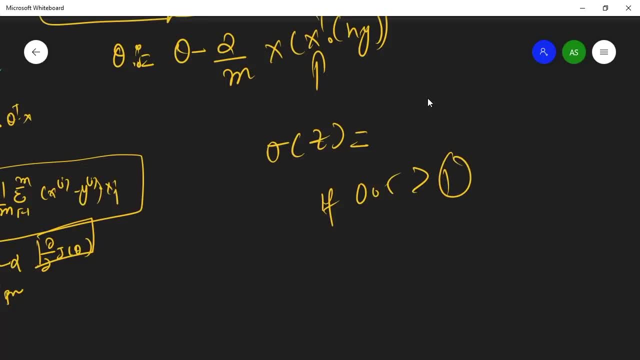 means the image as a cat is a positive indication and 0 as the image is a not cat, then it's a negative indication. okay, You can take anything, but for convention you do this kind of thing. Okay, pretty much you see what I'm trying to say over here. 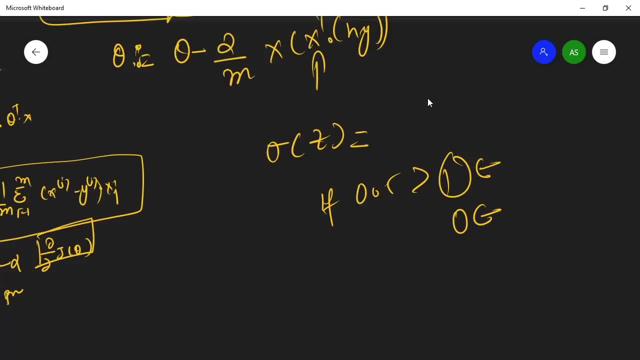 Okay, so we have the hypothesis and we have a cost function for checking that convention. We have a ratio from R and we have a gradient descent for getting your best optimal theta. And again, we are only learning theta over here using the gradient descent algorithm. 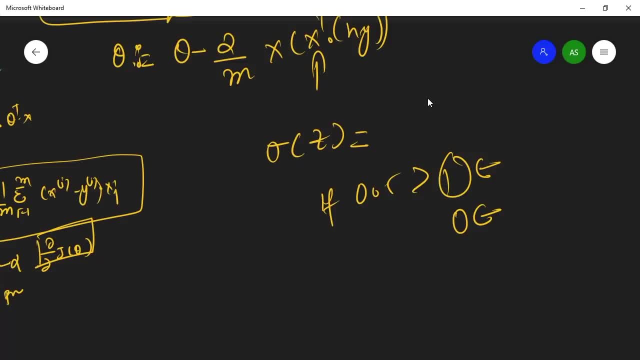 Okay, so now I think we are done with the logistic regression and in the next section we will go over to PROZECT, which is Brees Cancer Detection System, and then we'll go a little bit further into understanding the support vector machine. okay, 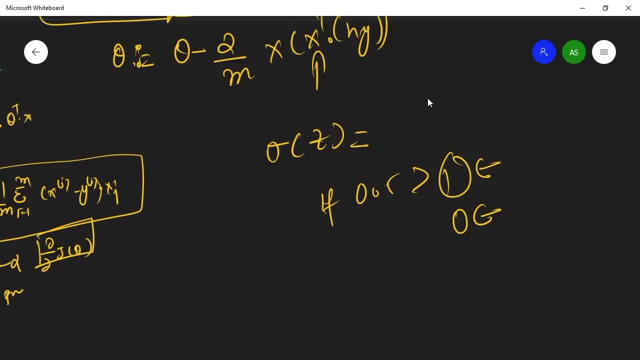 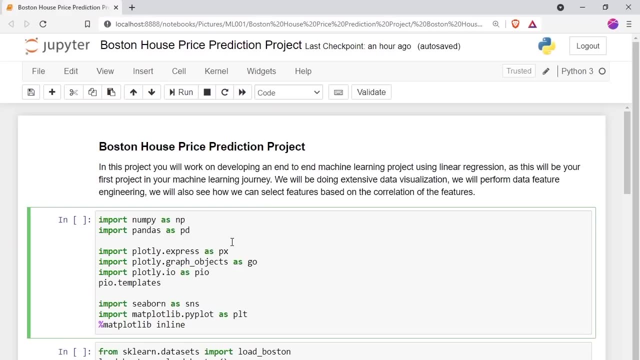 And I really hope that you will enjoy that section also. so let's meet at the next section. Okay, so here I am on my Jupyter node and I'm going to show you how to download a Jupyter notebook. And you can download a Jupyter notebook by searching online. 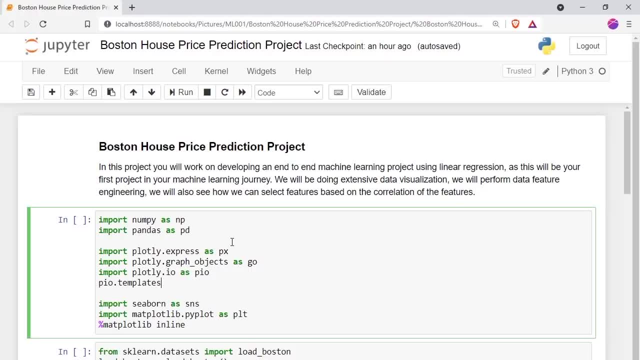 how to download a Jupyter notebook and you can follow the tutorials to download a Jupyter notebook. Okay, so what we will do? we will first start with importing the libraries, then we will load the data. we will understand what data we are working on. 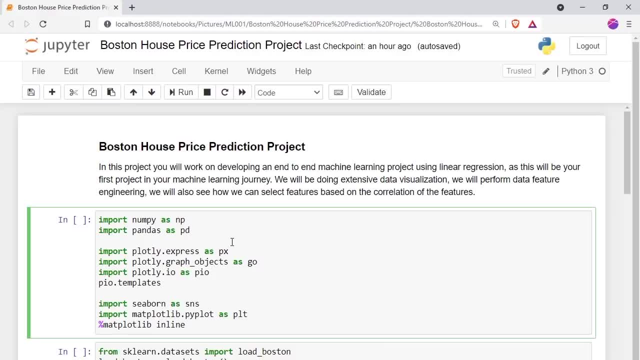 and then we will follow the feature engineering. then we will see how to select features. we will do expiratory data analysis, like data visualization, data analysis, and we will perform feature engineering and then we will see how to select the features. 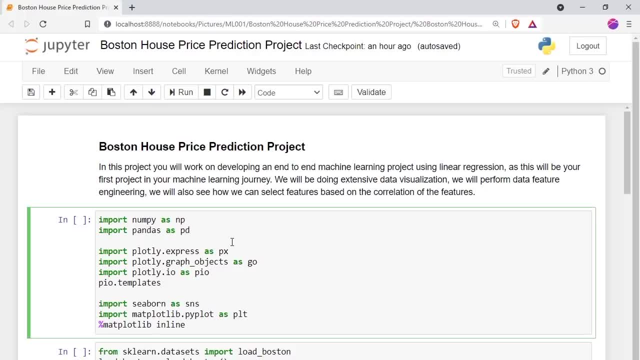 from the correlation of the features, and you don't need to have any kind of experience with Pandas, although you can have a look, if you want to, in detail- but you don't have to be expert in all of these. This is just a beginner project. 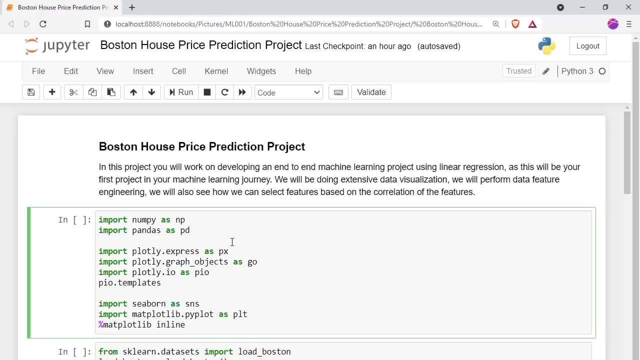 You can also modify it and put it on your resume and make some changes And what you can do. you can save this model and simply deploy it, Okay. so let's go ahead and start. Let's first try to deploy it over a website, okay. 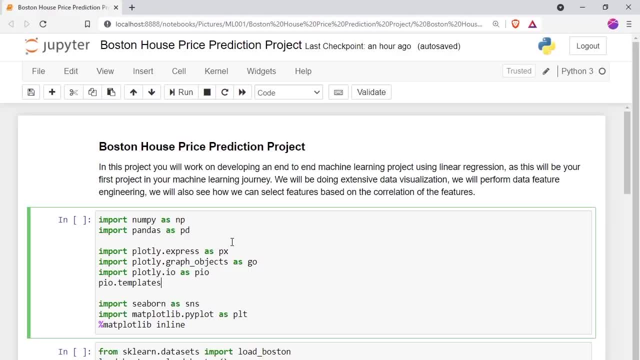 Okay, so I will talk about deployment later on, but before that, let's walk through. let me make you walk through this project. So, first of all, we are importing the libraries. First we are importing the NumPy as NP. 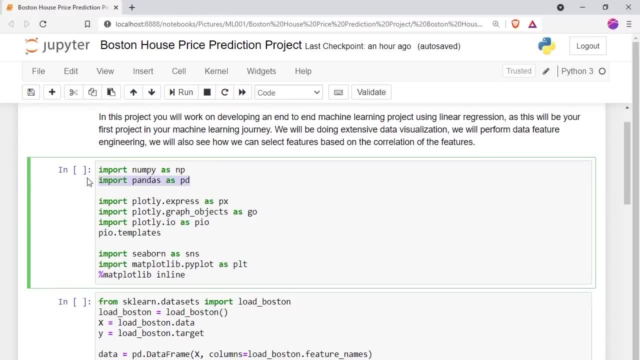 and we are importing NP as a liaise, Pandas as PD. PD is also a liaise short form of name. Plotly is another great visualization library, but I rarely use it. I don't want to use it for now. 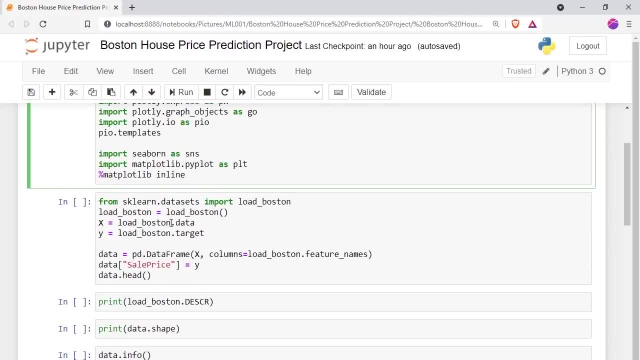 but in future you can use it plotlib. we just just want to show you i uh seaborn, which i'm going to use it here, and matplotlib is also a visualization library that i'm going to use over here, and this matplotlib in line tells you to use a matplotlib in the back end. okay, uh, it's kind of a tells matplotlib to choose the. 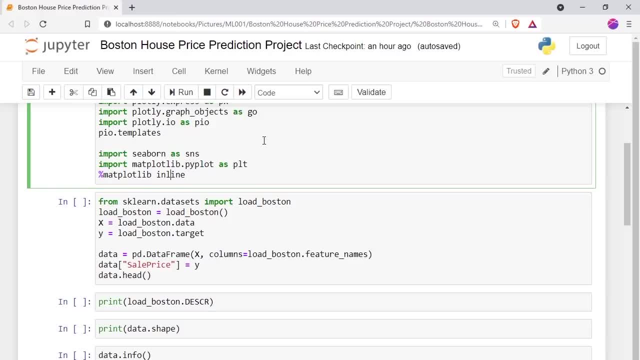 to plot the images in the back end. use use the jupiter notebook as a backend. okay, so, uh, first of all, uh, this is the learning thing, so we will load the data from the scikit-learn library. scikit-learn library is a famous library for machine learning, so we'll load the datasets from. 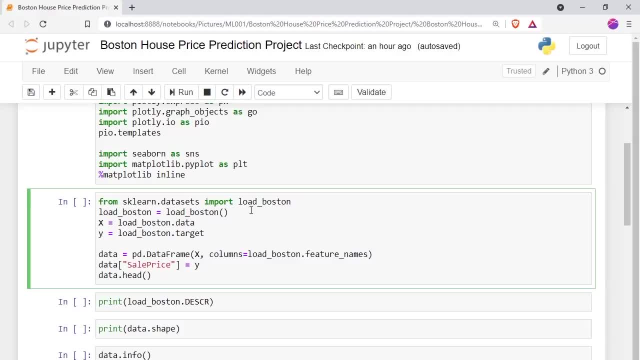 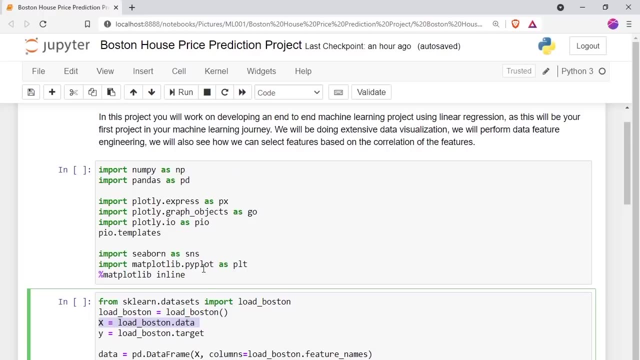 loadbuster, which is a boston house price prediction. we'll make boston hospice prediction, so you. so we want a data set of that. okay, then we instantiate our load boston and then we take out x, which is the data. i will tell you what is x and y over here, and y, which is a load bostontarget in our 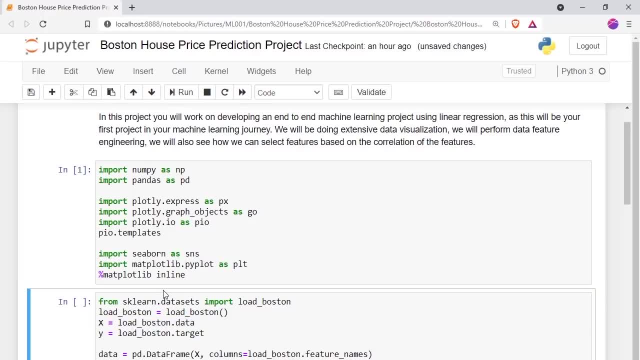 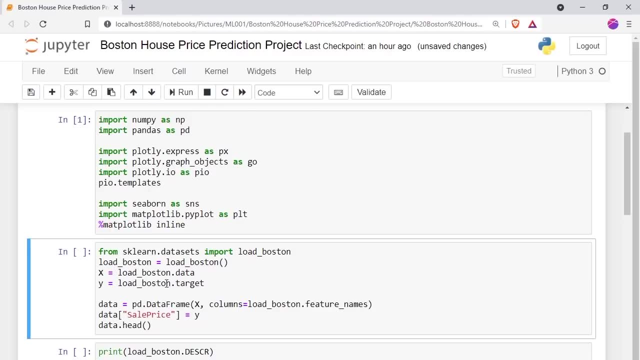 previous tutorials. in the introduction to machine learning, we have a talk about x and y variables. x variables is the independent features which we, which which we use to predict the model, and this is the y, which is the target variable because it's unsupervised. so we know what our 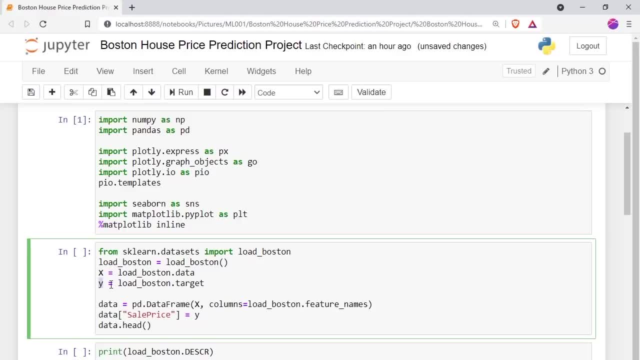 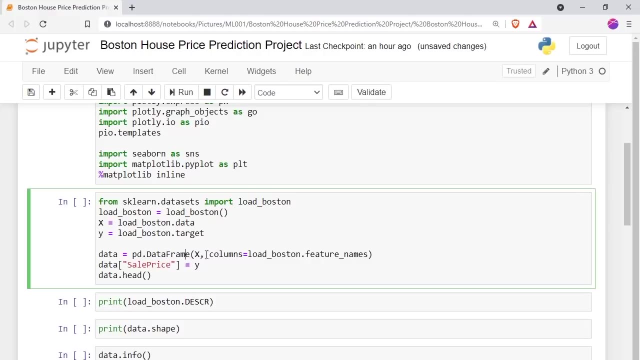 output is. we know what our output label y is okay, so, um, we will be given this. and x, y is the target variable which will be in case. in this case is the sales price and this is the features. okay, and then i call pd, dot data frame and it can constructs a data frame and we give. 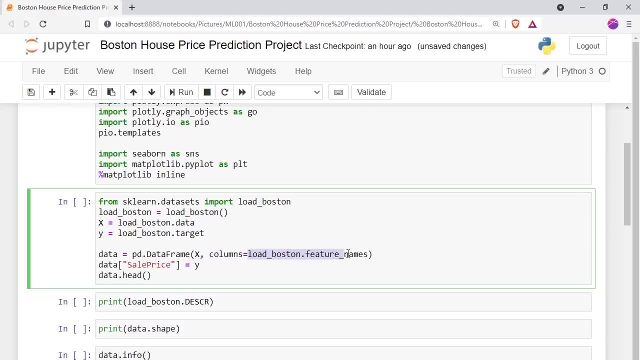 x, which is the features, and we give the name of the columns- dot feature names. there is a dot attribute, dot feature names to get the names of the columns automatically. okay, and then we make one column. here we are making one column, which is a sale price. we are making a sale price and then 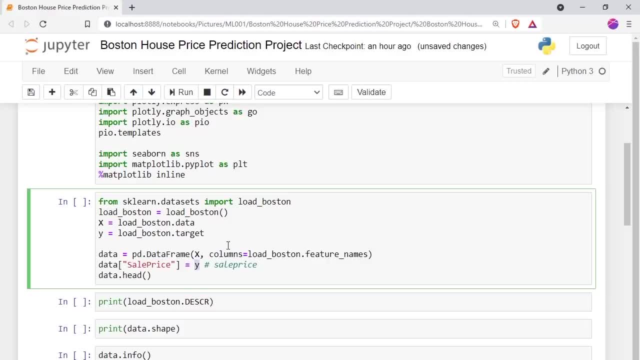 we are making it y over here. okay, my y y means load boston dot target. either you can make this also like this, either you can make this also. it's just the same. okay, y is just a target variable and if you just run this now you can see this is the data. 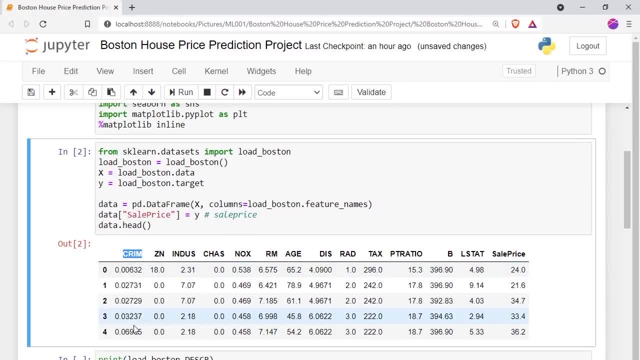 frame. um, here you have a crime rate per capita, that let's see the column distribution. so i just first see, let me show you what we have done. these are the x variable till s ls that. these are the x variable and this, this is the y variable that you use to predict, and you may think, here i use 24.0. 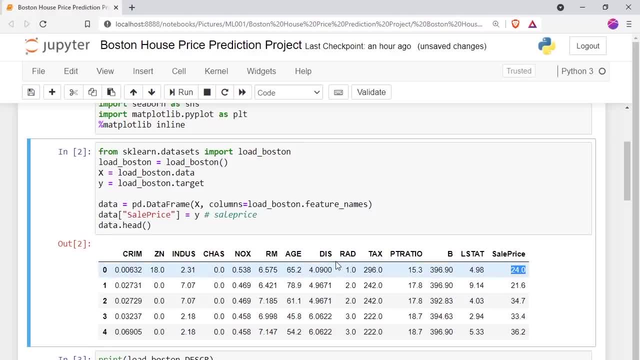 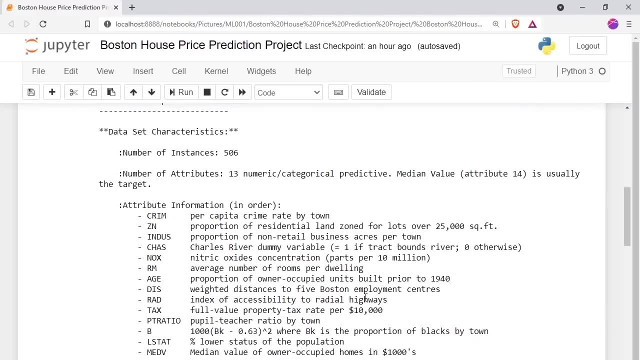 means 24.0 is the dollars, is just the price of the house? no, the price of the house is given 20.0 thousand dollars. okay, so you can search just just just. we will see the whole thing just in second. okay, so this is the data frame that we. 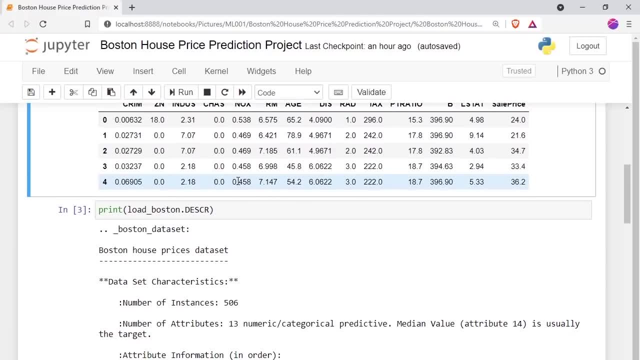 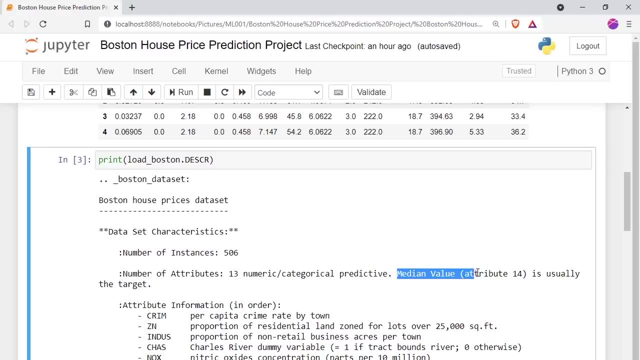 constructed okay, so now let's take a look at the what data we are working on. so there are 506 rows and there are 30 numeric and categorical columns and with the median value, attribute 14, which is our target variable here. i'm giving given is a sale price name, but you can give us a median value. 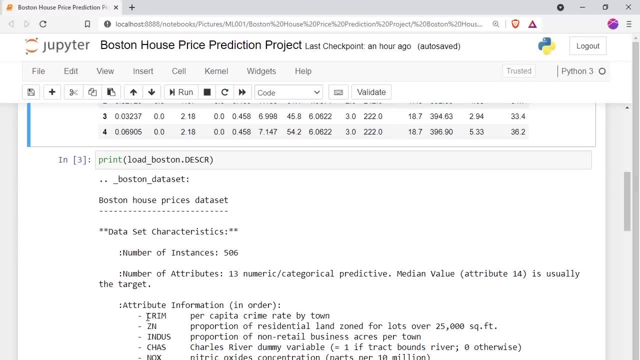 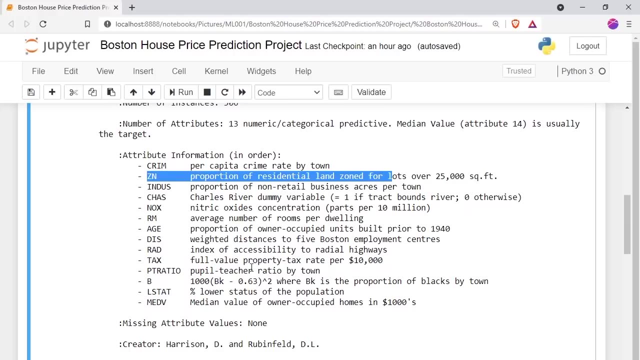 it's usually the target variable. okay, so here is the column name. is the crime? is the per capita rate, then proportion of a residential land, proportion of a non-retail business, which are knox age, uh, what's the proportion? uh, average number of rooms per dwelling, etc. you can read over here. and the last, which is: 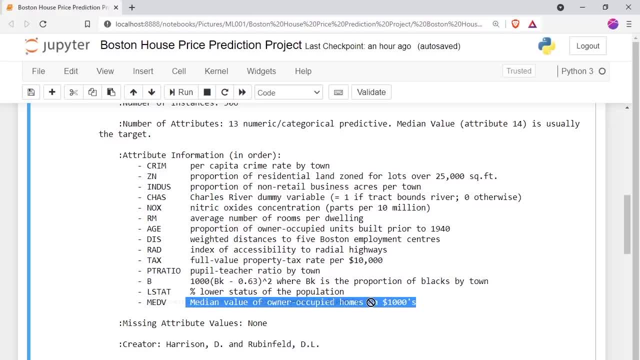 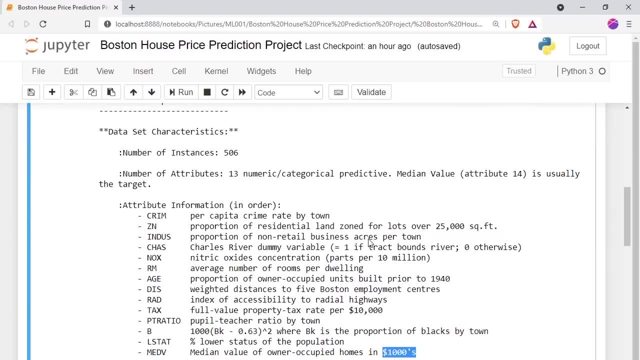 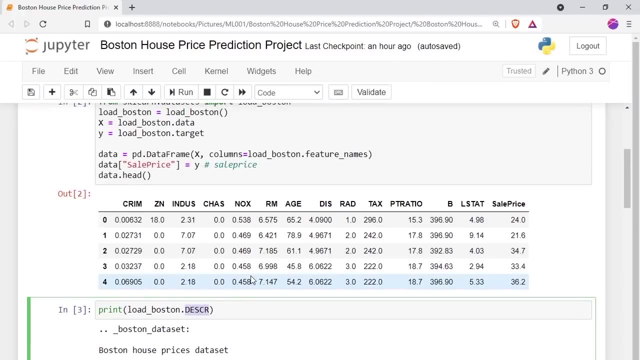 the favorite, uh, the target variable, which is the median value of the, which is the sales price, in this case in a thousand dollars, so twenty four thousand dollars. now you know your dream has gone out. i think so. okay, so you're gonna read it over here. just just you can use dot d c e d e s e r. 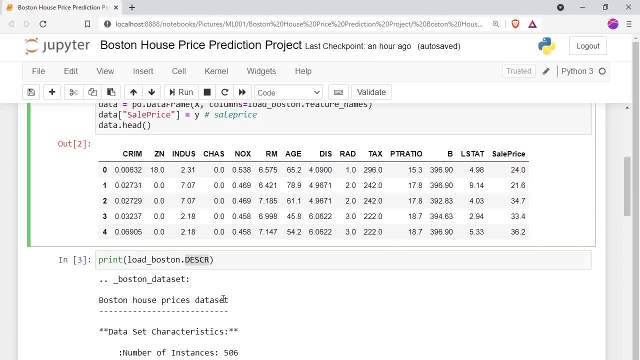 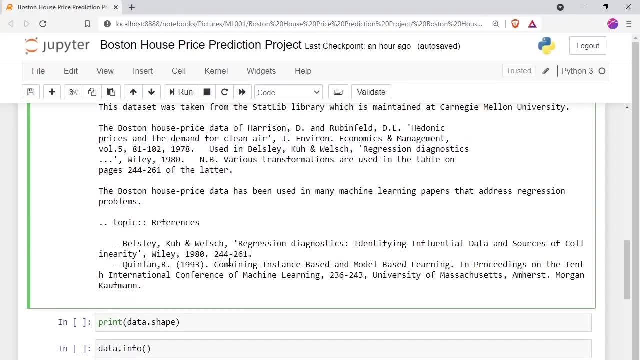 because this is available in the scikit-learn, so you have this kind of thing to see the information about the data set, but in real world we will work on real world data set, so you will see how you we download, how we process, etc. okay, so let's understand a little bit more about the data. we look at the shape of the data, which? 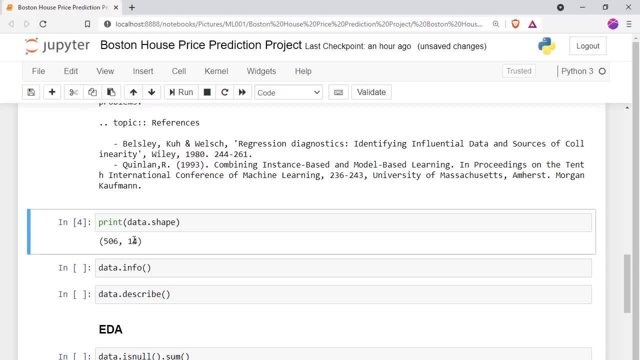 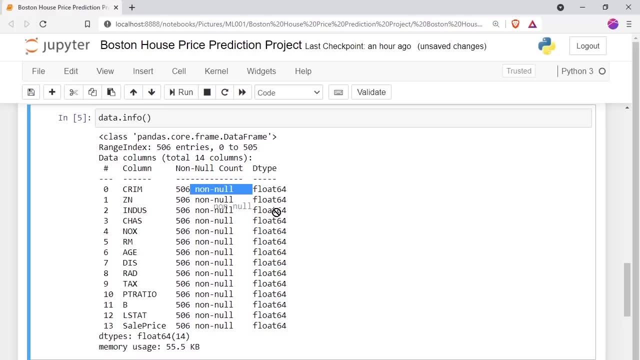 is 506 rows and put in columns means rows and then columns. then your dot info tells us the information of your, of your data, which is non-null. values means what are the data types and is there any null values into that. null means missing values into that column. 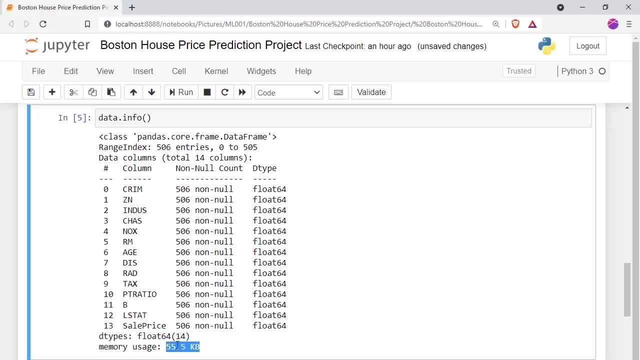 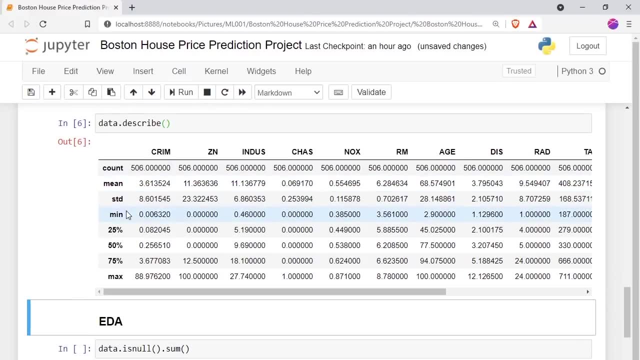 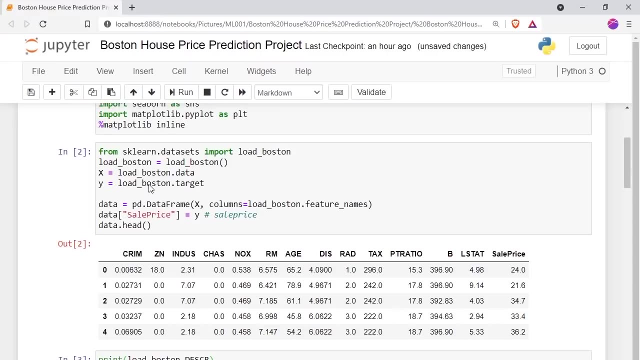 okay, and all the data sites are float. what is the memory usage, etc. okay, and let's uh dot describe, will tell you the mean of that particular column: the standard deviation, the minimum, 20, 25 percent of that, 70, max count, etc. okay, so we had seen how, what data we are working on. these are the features. 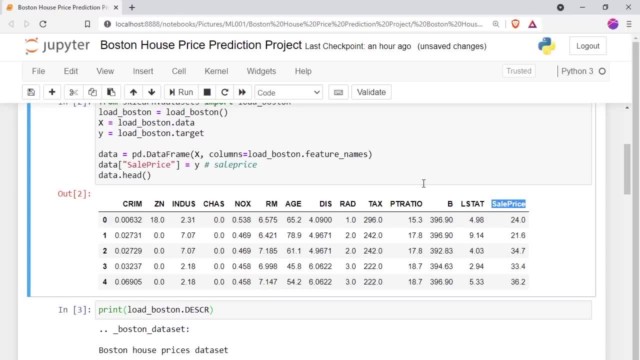 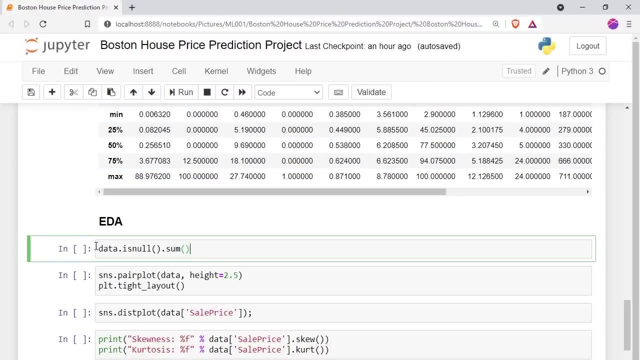 which is the x variable, and this is the target variable, which is y, which is a supervised learning problem, as we can see over here. okay, okay. so let's just take a look at the null. you can use the null and we can use data. dot is null, dot sum, and you can see over here that we have the zero, zero, zero. 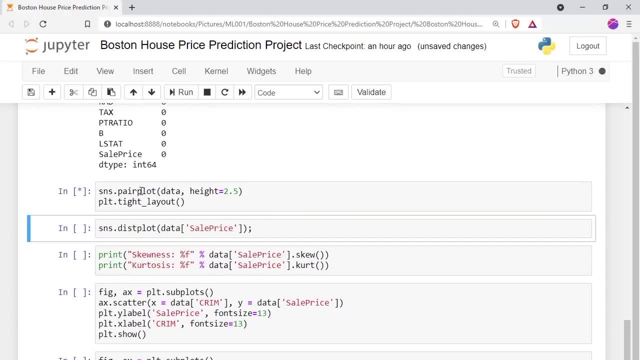 all the way. and then we can plot a pair plot, snspeerplot, which will plot all the things which with respect to every feature. so you can see over here that we are just plotting the peer plot. uh, you can see, but if you, we, we do not get a lot of information from this peer plot. 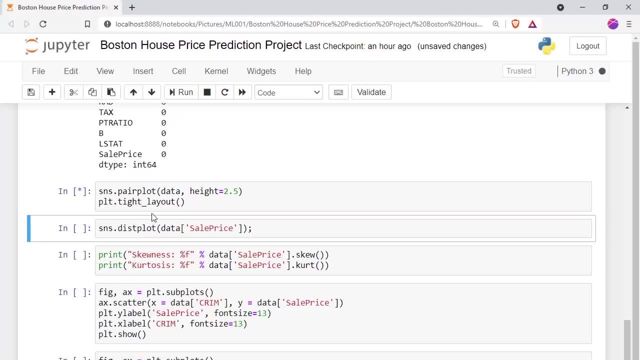 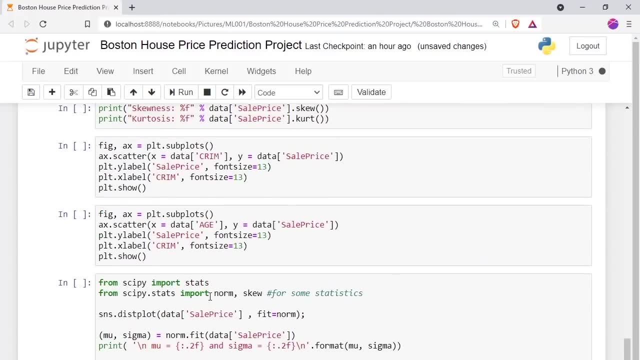 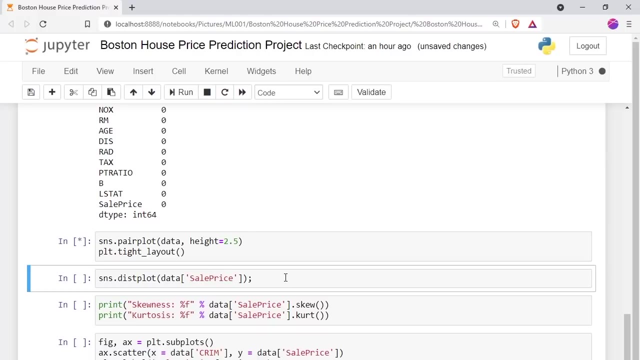 because it's very kind of small and we cannot see what data is it is it pointing on, etc. okay, so we have to definitely take care of that to to uh, visual visualization that i made. okay, just wait for a few seconds, then it will show up, okay. 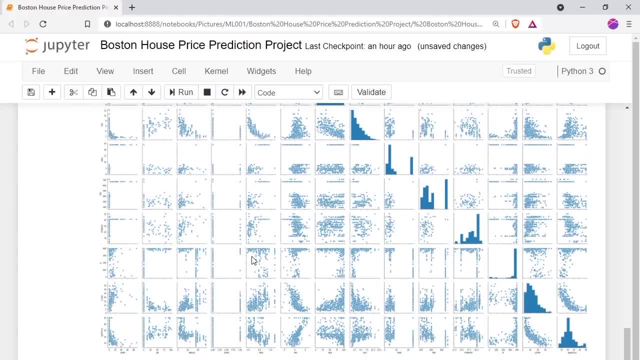 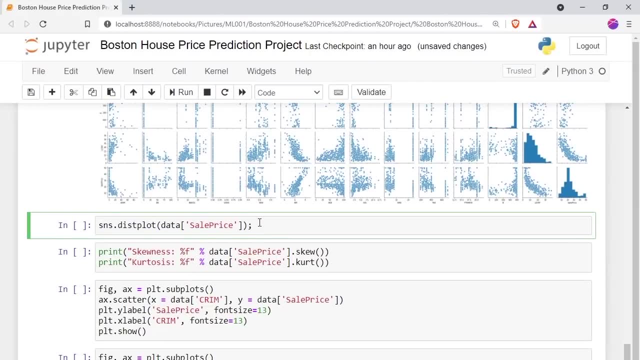 okay, so it's plots and we are unable to see this kind of thing and we are unable to see. so it's very hard to see this. so what, what we do, let's let's take out, and let's just take out the inferences from the sales price, which is: this is the target variable. let's do. 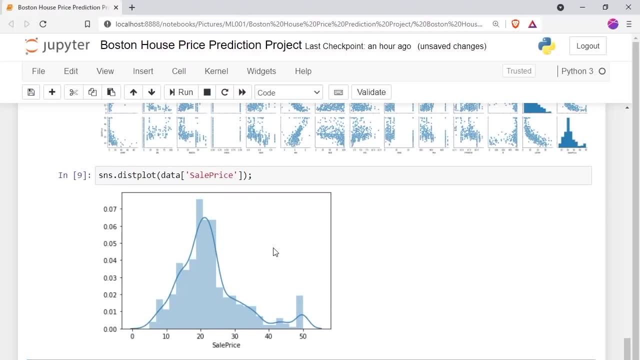 some analysis. so we plot a distribution plot and you can see over here this little bit skewed we want it is. we are seeing over here this positive skew, but here we can, uh, add some transformation. so what's the secret? skewness and woroodsome could do this. so here we have one, a. 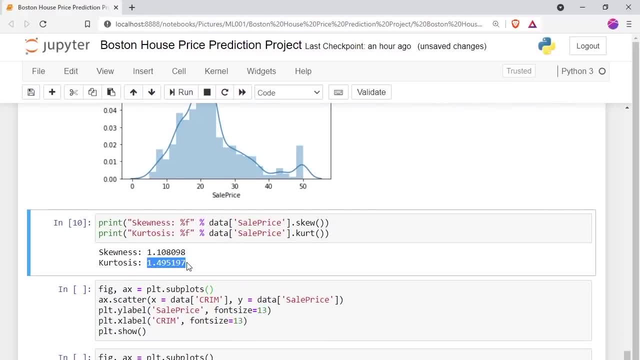 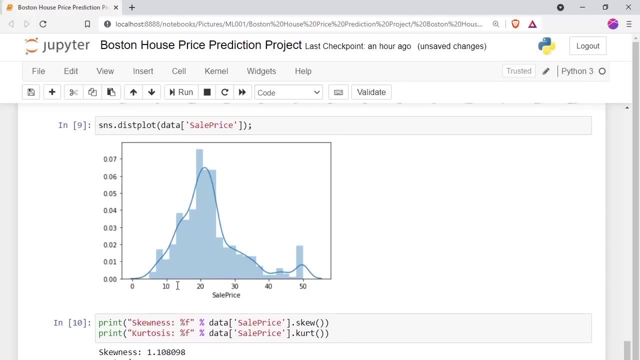 point one, zero, eight, zero, nine, eight and one point four, nine five, one, nine seven, which this? this will help us to find outliers, and outliers are those who are far away. let's say that you are working on uh age. okay, so uh age is 20, uh, 20 years old, 50 years old, but let's say 150 years. this is the. 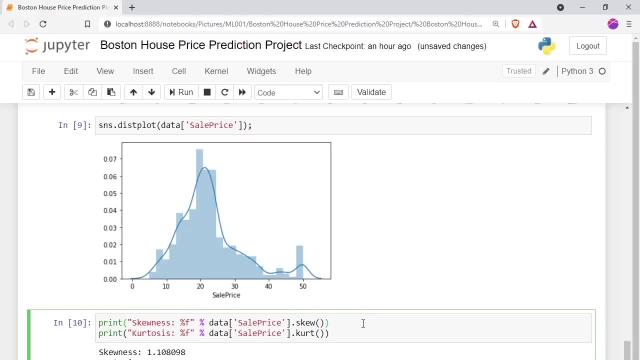 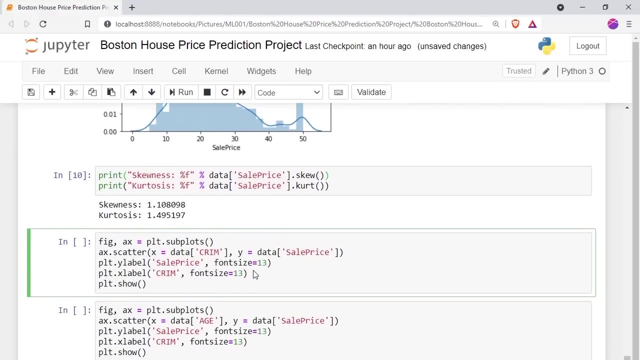 outliers: okay, these are the outliers. okay, those who are exception, those were exceptions of the data frame. okay, so we have to take care of this. but before that, let's see some relationship with each and every column. one. you have taken two columns. you can try different, different columns. 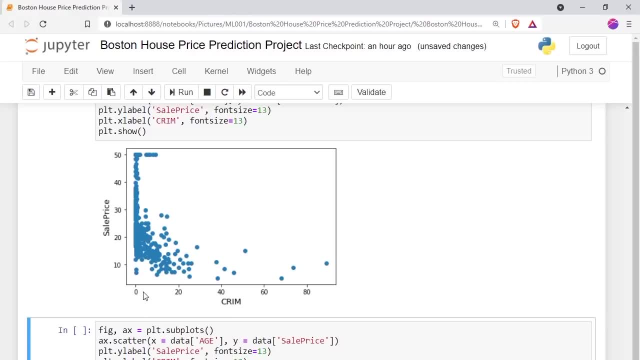 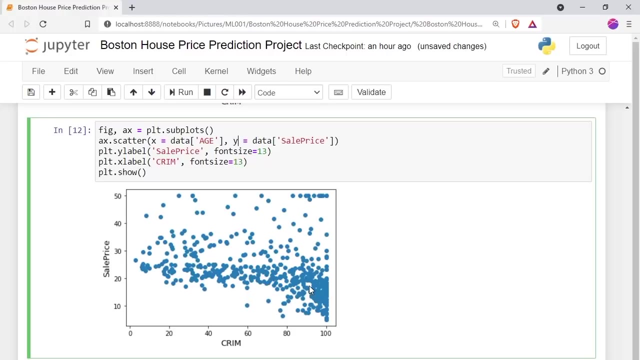 so there there is a little bit crime, there is the sale prices very high. when there is a lot more crime, there is sale prices very, very low. okay, and what's the age? you can also see, and you can see over your 100 years old has been sold uh in a smaller rate and uh, 20 years old has a little 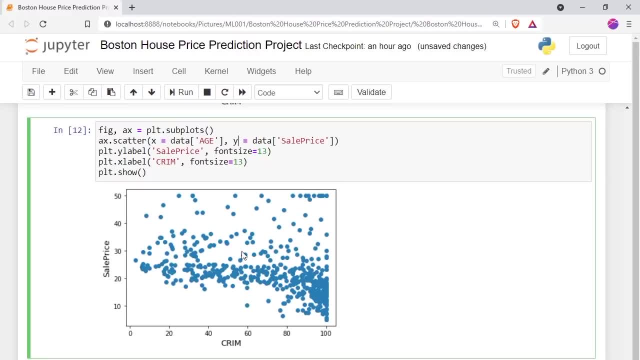 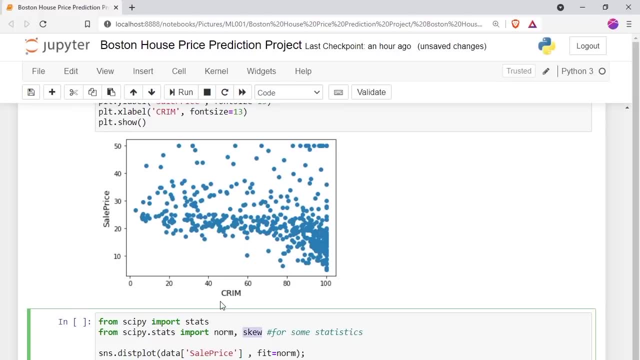 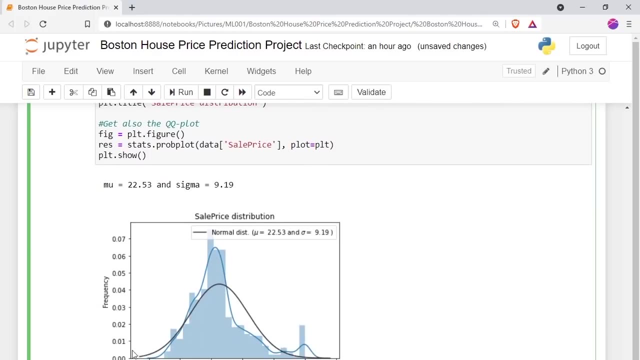 little bit higher way and you can see the data visualization over here. okay, and you can see over here that i've imported psi, pi, which is again the like num pi. i'm just taking out the norm and the skewness. so you just plot a distribution plot, for seeing this kind of thing means uh, for a normal distribution, if you know. 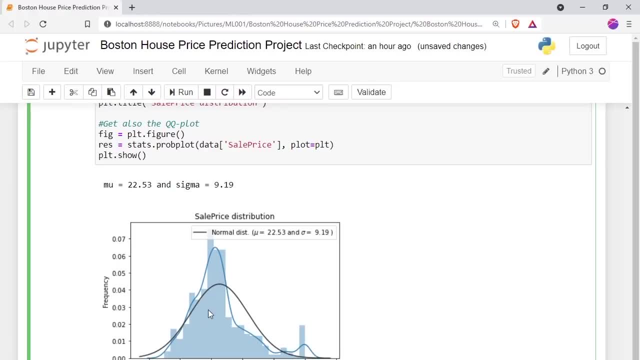 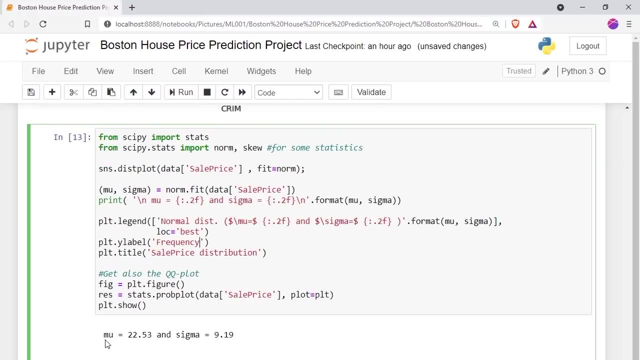 what normal distribution. you are just plotting the normal distribution and we, and this is your actual, this black line, and you have this blue line, so you have to transform it a little bit. so your mu, which is, uh, mean, is 72.53 and sigma is 9.19. okay, so these are some. if you know what python, you should know about these. 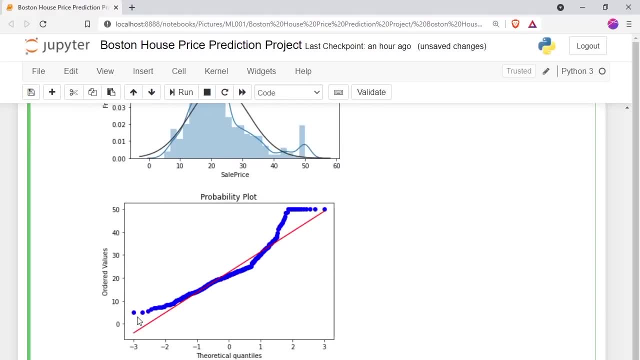 kind of time for formatting, etc. okay, and this is the qq plot, which will help us to see the quadrant quantiles, which is uh order values. you can search more on the internet or uh go on wikipedia to learn more about this, but our main, main focus will be this: uh, sales price means. 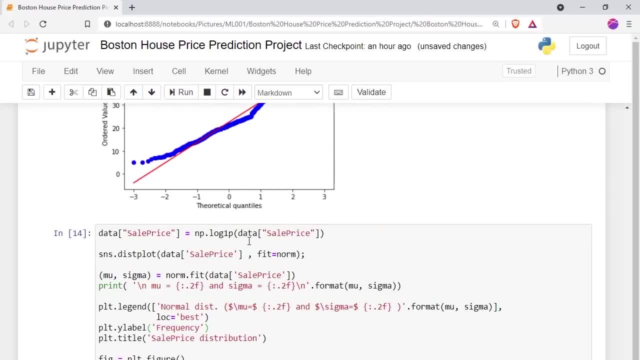 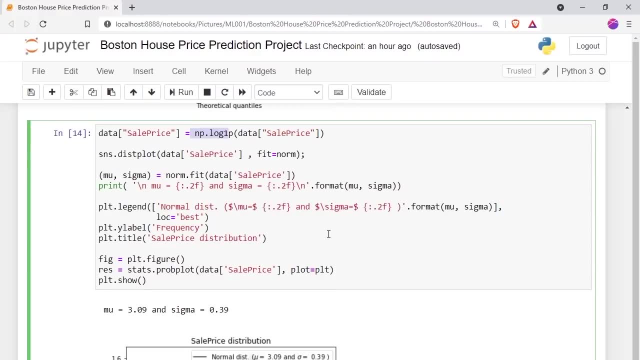 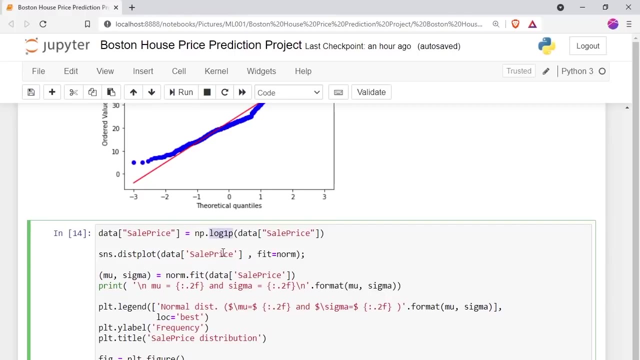 distribution plot. okay, so let's run this, let's try, let's add, let's add a log, let's, let's uh, let's uh, transform our sale price to a little bit more accurate. so now you can see over here that is, askewness is over now. we have just applied a transformation over here, log1p, and it's now good. 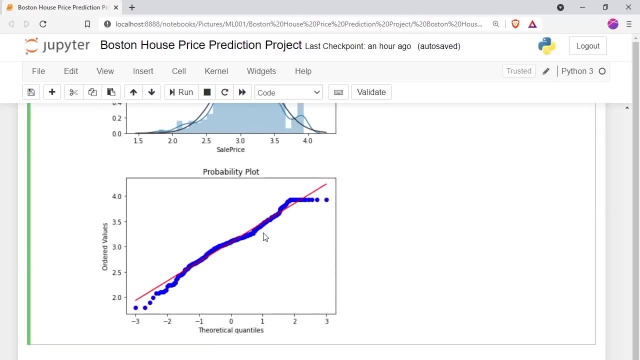 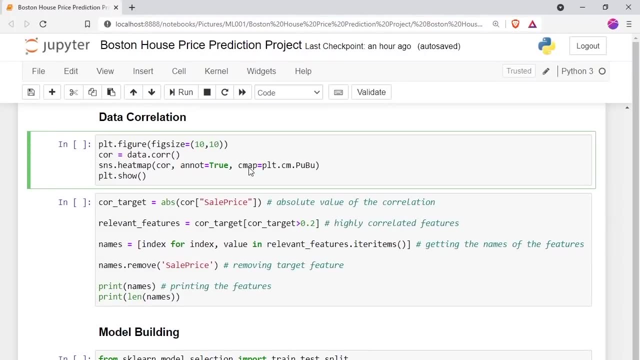 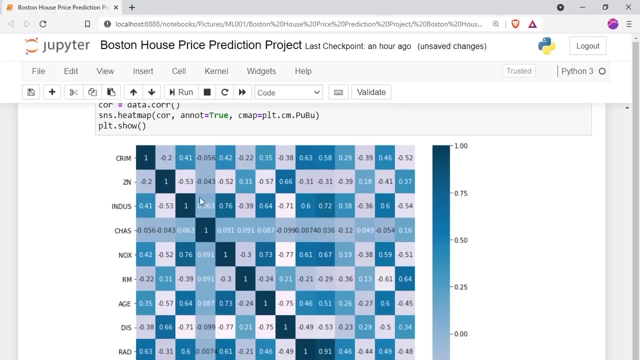 okay, to avoid outliers. okay, and this quantity is also removed. okay. so data correlation: what a correlation? first of all, correlation is the? is the relation between features? okay, so if the, if it is one, then it is um positive correlated, then it's minus one very negatively correlated. you can search more. 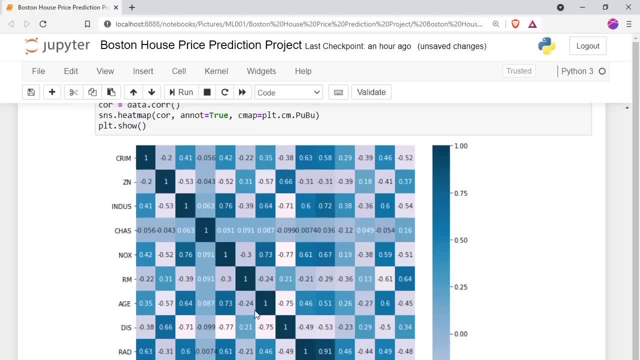 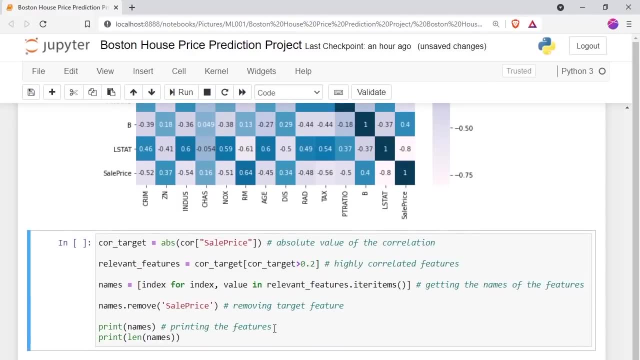 internet about it, because it's not a statistics class. so you see away, if the diagonal is one, all the features are perfectly correlated. okay, so how do we select the features which are highly correlated? okay, the features, how we select, if we have taken the absolute value of the sale price and we are taking the highly correlated feature from this uh statement? 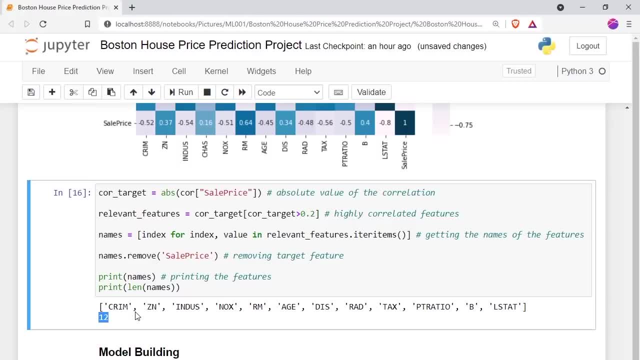 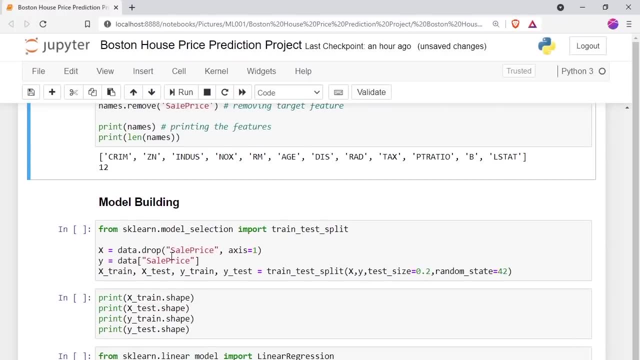 and there is 12 feature that we get that is highly, highly correlated. you can choose this, but i'm not going to choose. you can either, um, delete the rest of the columns except these 12. okay, and let's just start with model building. so you just employ important split and train. 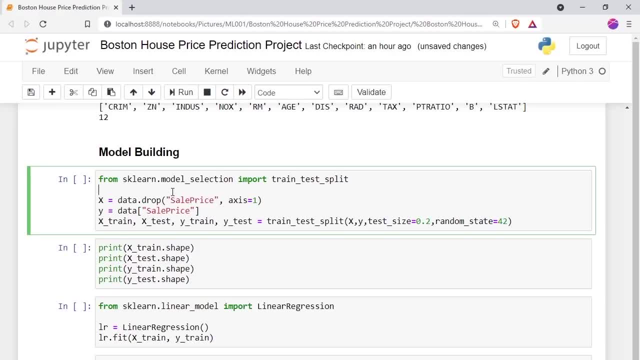 test place. simply divide your data into training and testing means: um, let's say you have. you have 80 of the data, so sorry, 100. so it will take 80 for training and 20 for testing and use drop because you don't want x to be sales price and y to be the sales price, okay, and then you test size. 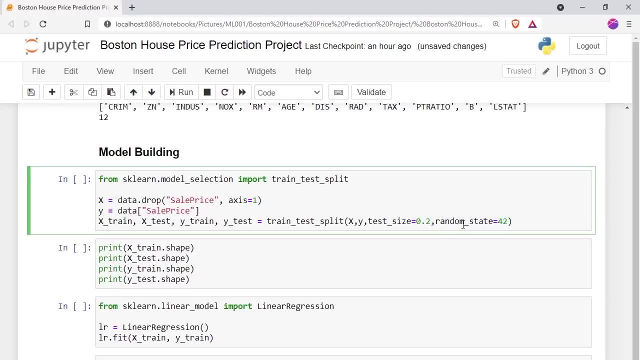 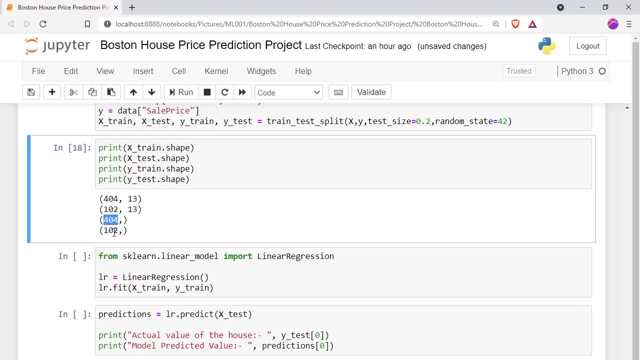 then the van van random state will tell you the uh means every time you run the data should not be changed. okay, so if you run this now let's take a look at shape 404 and 13 columns for a training and 402 for testing and 400 for labels and one or two labels. okay, so, let's, let's start with uh. 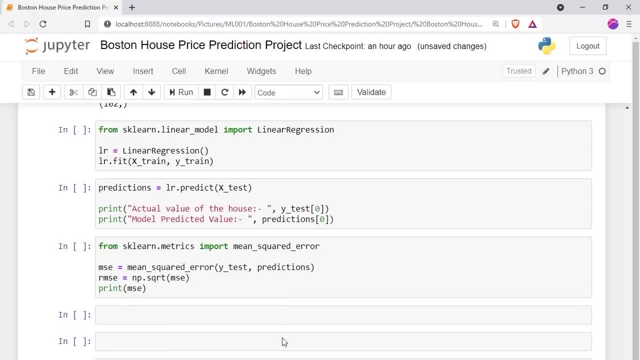 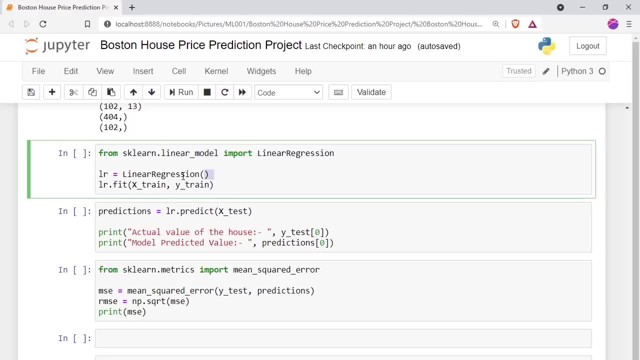 let me make one little little bit more uh, so that it should be clearly visible. okay, so you just uh a linear regression and you just instantiate it and then you fit the model x train and y train which we have used for training and y training, x train are the. these are the input and this is the. 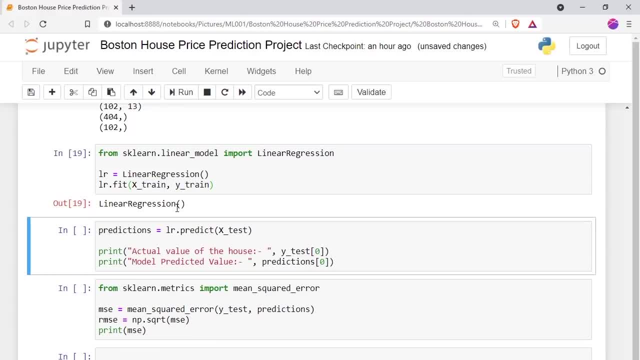 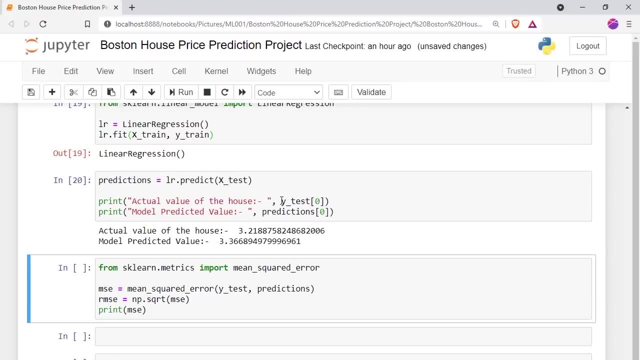 y target variable and then if you run this, now it's instantiated, now we can, now we can make prediction. okay, so you can see over the actual label, because we know, we, we know what y test 0, because this is actual label and this is the prediction, which is 3.36 is a predicted value. 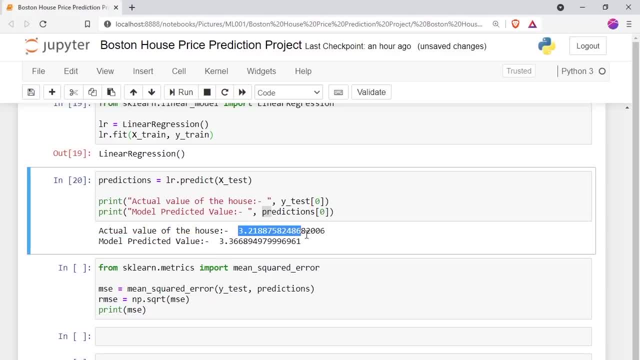 from the model. and three, point two, one, oh, eight, eight, eight, eight, seven, five, eight, two, nine, is, et cetera. is the is the actual value, which is a little bit uh different from this, but it's um good performed, very, very good in terms of linear. 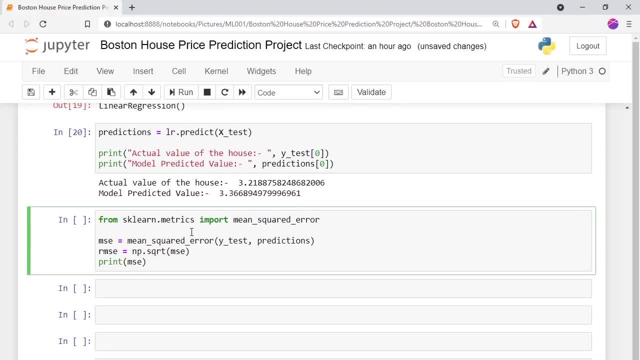 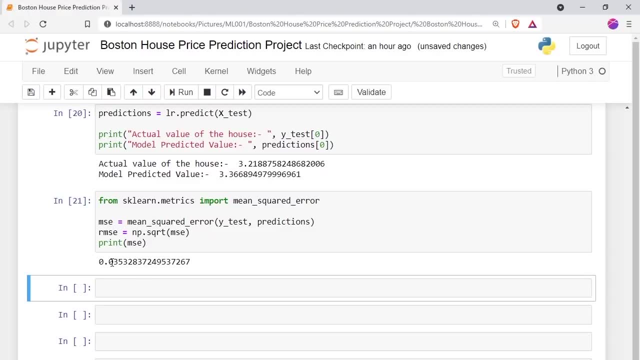 regression, as we have seen so far, okay. now, if you want to check the accuracy- for checking the accuracy, we have seen a cost function. you can run this- and msc mean square error. and let's say, if you want to see msc, there is 0.035, which is good, and if you want to take out the rmsc, the square, 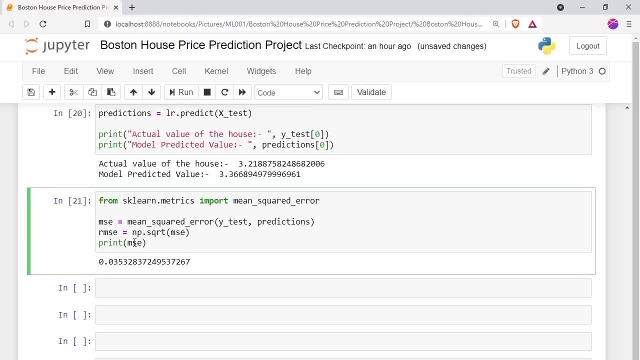 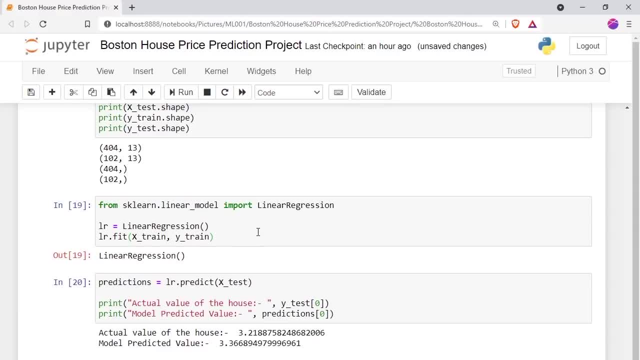 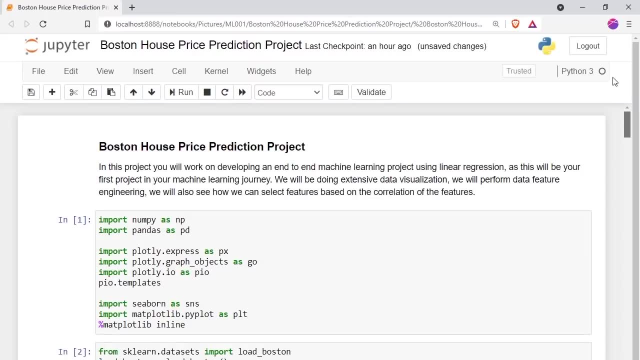 okay, and you've seen it's pretty much good. okay, you will learn more about how we can improve this by using xg, boost, bagging, boosting, etc. later on. okay, now we have done our full prediction project, the code will be in: uh, my github, which is in the description down box below. there is a lot more. 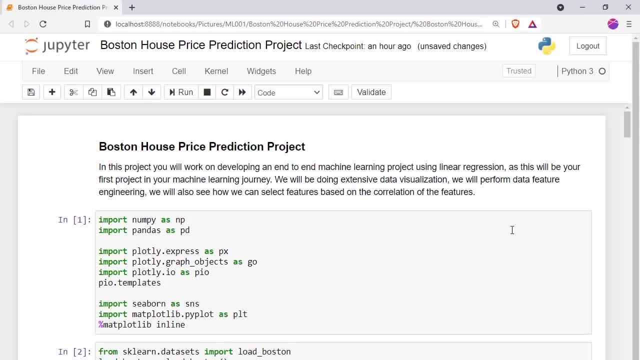 project which which is available in computer vision, natural language processing, which you can take a look, if you want, to my projects. okay, so now i think i have not quoted just now because there will take a lot of time, so i just written up and just annotated each and every line of statement. 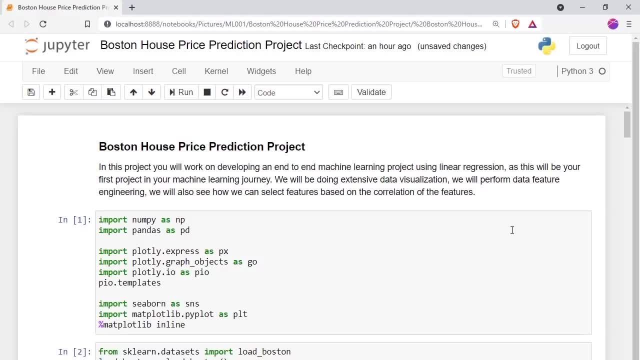 okay. so if you have any kind of problem in search on internet because you have to master google to if you, if you have encountered any kind of problem, and in the next tutorial we'll be talking about a regularized linear models, which we'll talk about lasso and which which we'll also use in this- 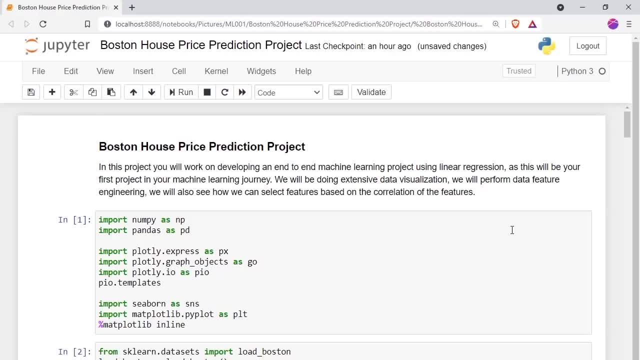 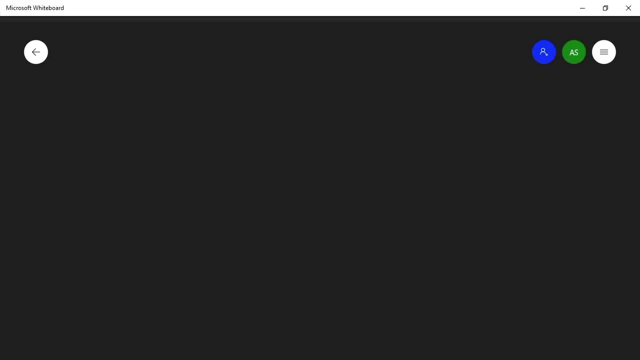 to check. uh, as a last one, regression and a ridge regression. okay, so let's, let's get into the next section. okay, so now let's get into the next section. okay, so now let's get into the next section. okay, so now we have talked to talk, talked about a linear regression, and we have made one project. now it's. 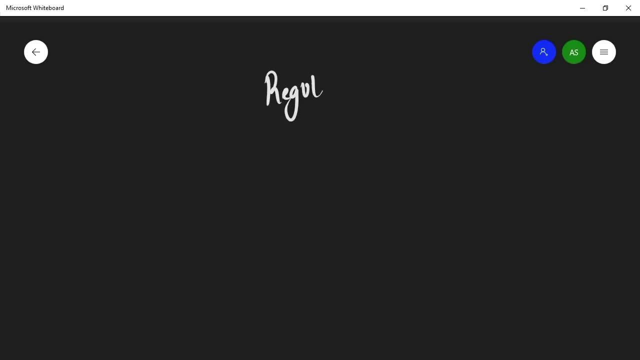 time for getting into the regularized linear models. linear models, okay, so, uh, if you remember that we have a pointed out or some problem which is, uh, overfitting, which is overfitting, which we have pointed out earlier, okay, so, how does overfitting happen? let's say, if your model has learned too. 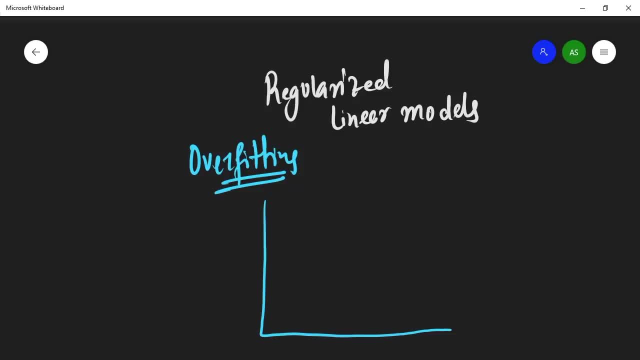 much so let me draw one uh x and y plane and let me draw some data points. okay, so this, these, these are the data points. and let's see, or you have a complex portal, which is a complex function which maps your input variable to output variable. so you just uh, make the complex function like this, which is: 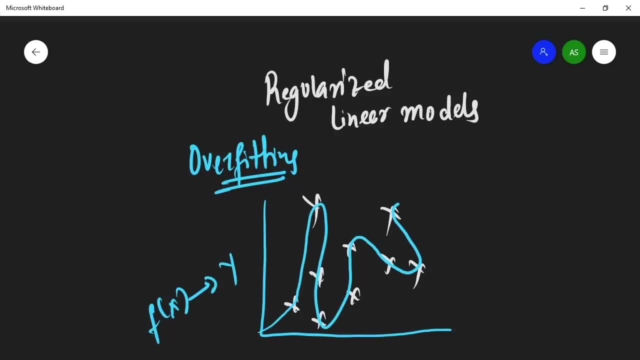 which is touching each and every line. so let's say, a new uh example comes in and it's making a bad prediction, so you can see it learned too much onto the training data which are in a trend and it's it is very going bad it is. it is uh not generalizing well onto the new examples. okay, so that's, that's. 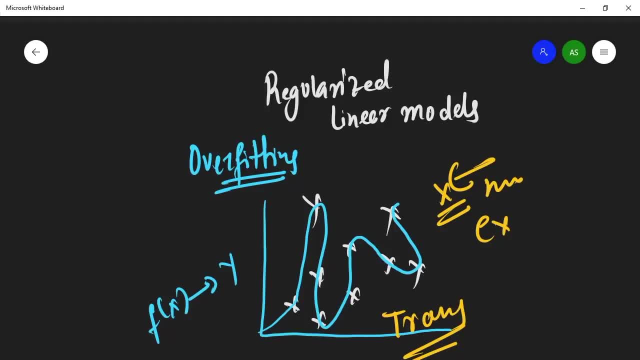 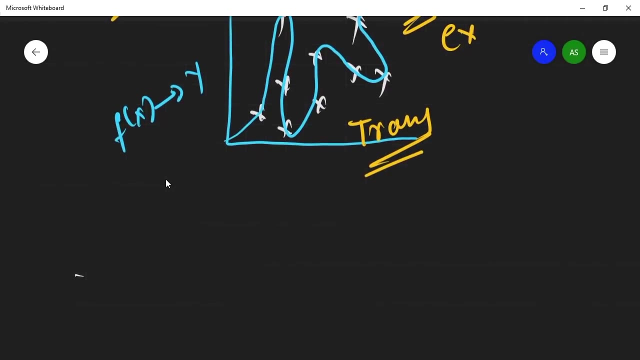 called overfitting. if your model working better, best, 100 accuracy on the training- and working worse on the validation accuracy, then your model is likely to fit overfitting. okay, so how it is caused. let's, we have a lot of features and you, um, let's say, a thousand features. 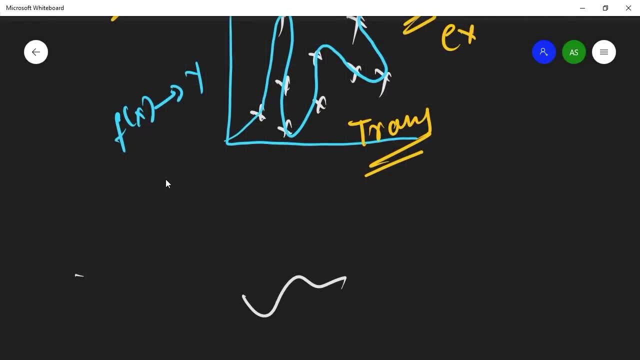 and so it will learn, obviously, the complex functions and then it will perform very, very bad. okay, so for that we have some solution, and the solution are: either you reduce some features, reduce some features, reduce some features. this is you can do this. another thing in what you can do, you can, this is the same as like this, regularization in simple terms. 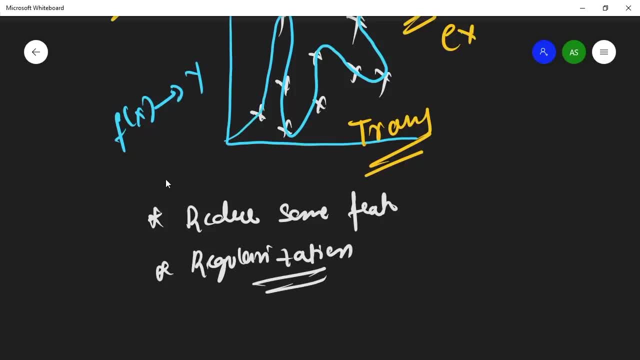 regularization is just eliminating the features that are not useful. okay, so it is just equals to this. so we give another name, which is called the regularization. so let's see some of the regularization techniques. so the first one is last regression. so let's see a last regression. 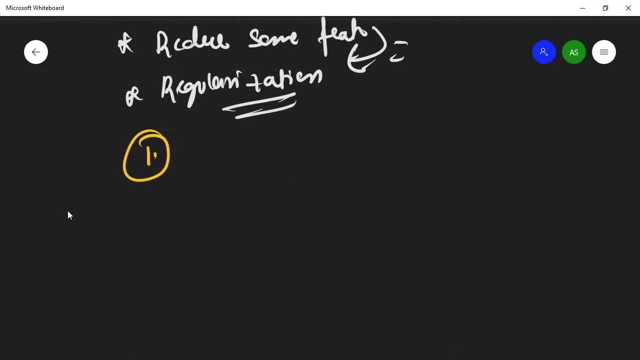 so what is last regression? last regression is a regularized linear models. what we do? we just add a simple term with us, a simple regularization term at the end or at the end of the cost function. let's say this: this term lambda, 1 over 2, i equals to 1, all the way. 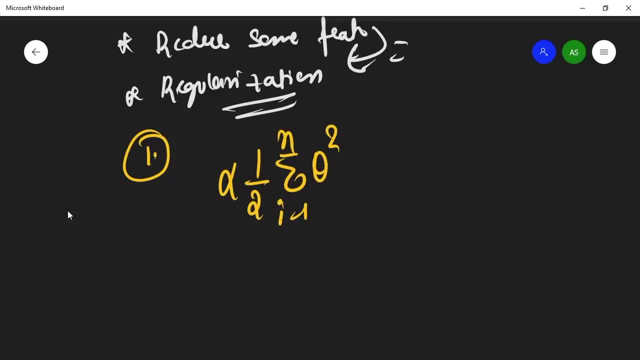 down to the m theta squared. i, okay, so you, this is. this is for a ridge regression. this is for a ridge regression. okay, so, this is for a ridge regression. i will talk about lasso just just after this. okay, so just you add this at the end of the cost function. so your now new cost function. 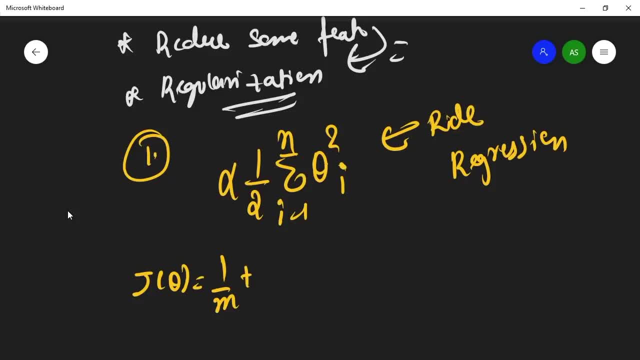 will become like this: 1 over m plus i equals to 1 all the way down to the m. theta transpose xi and this is the model predicted. minus y squared plus your regularization term: uh, this one i equals to 1 all the way down to the. 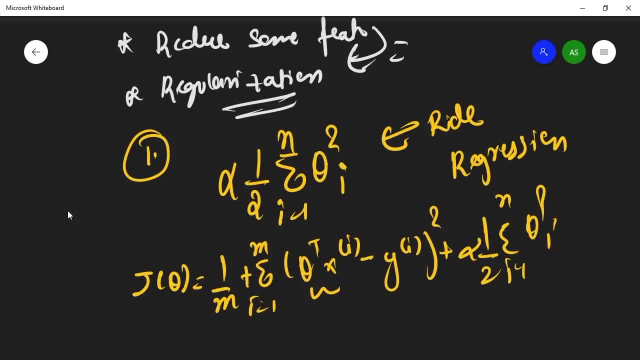 end theta squared. i okay, so you can do like this now. uh, let's, let's understand what it's doing. it is just: uh, let's say you have some piece features, which is the, let's say, the size of the house, let's say the price, um, let's say the number of fans, number of bedrooms. 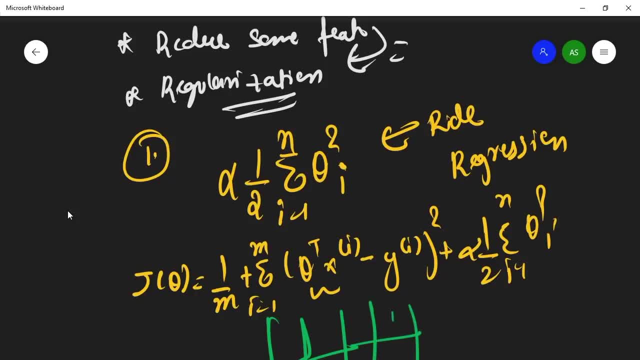 and a number of uh uh grass- okay, number of grass. so you can see this, this. this seems to be a less important feature, so it will. it will save you a lot of time and you can do a lot of shiny things in this. so this will simply make the theta means the parameter. 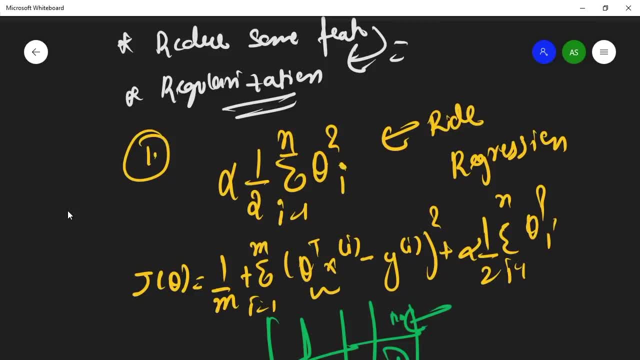 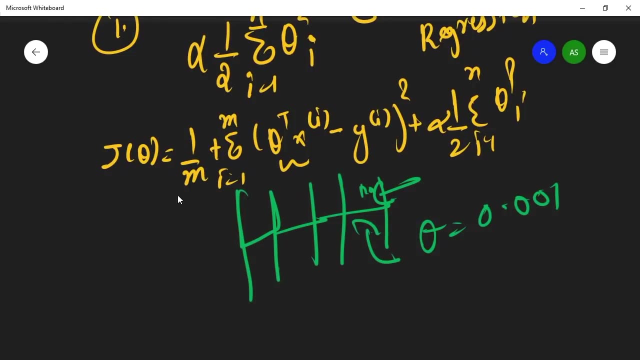 feature means the feature weight of this column to be zero. okay, so it simply penalizes or closer and closer to zero. in ridge regression it makes the feature weights closer and closer to zero. okay, so what it's doing, it is a. whatever the less important features are, it's just. 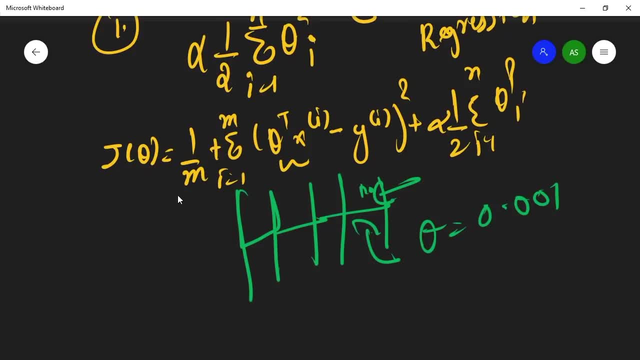 penalizing the theta of that, and the theta is the is used to make prediction and let's say, theta times the number of fans. okay, and let's see it's given a new feature which means theta x 2 or something like that. it will make the idea of doing a physical function like 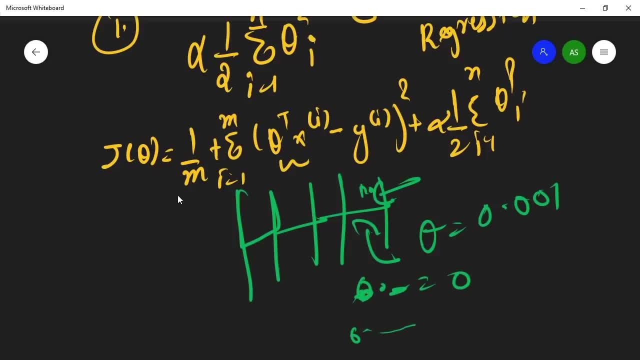 grass equals to prediction. So this is a very, very, very, very small. Okay, so it's just penalizes your theta. Okay, so that's a rich regression. is doing just penalizing or eliminating the or LA by how it eliminating? just making theta to be equals to zero, Okay, but if a but in region regression. 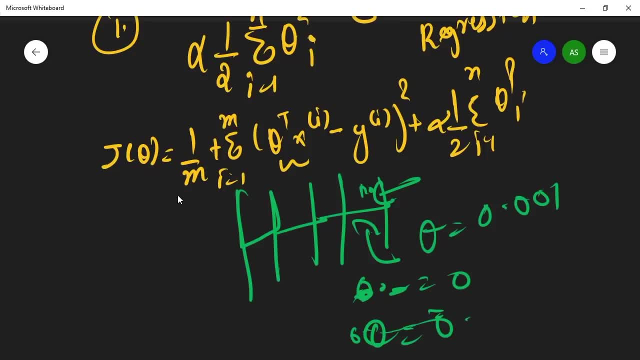 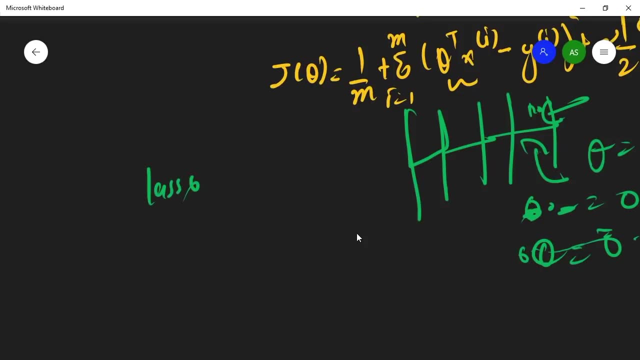 it is. it is making closer and closer to zero, But in case of lasso regression, it is simply. it is same in case of lasso regression. in case of lasso regression, I'm talking about lasso regression, it's, it's whatever the less important feature are. it simply makes it simply eliminate. 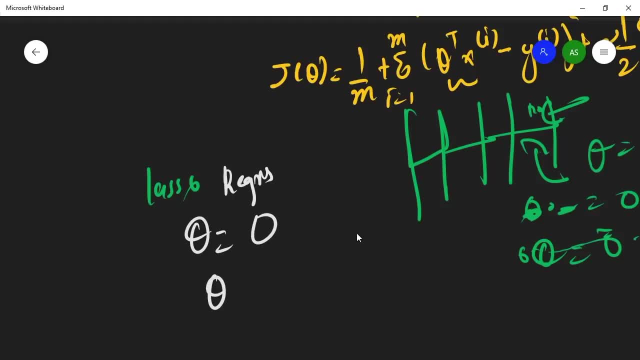 it simply make the theta zero, So whatever. let's say theta times the number of a grass. So theta equals 00 times. let's say seven is equals to zero. So this feature says: eliminate negative, So that's a lasso, is very strict. Okay so these two and you, just just you use l two norm. 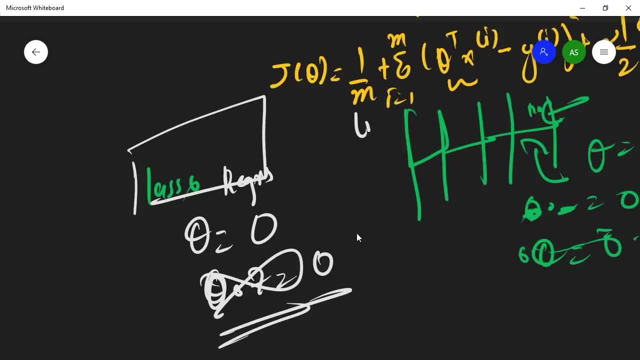 And in that case, in rich regression you are using l one norm, but in lasso you're using l two norm. okay, just as the regularization term, which is like this: at the end of the cost function I goes to one all. 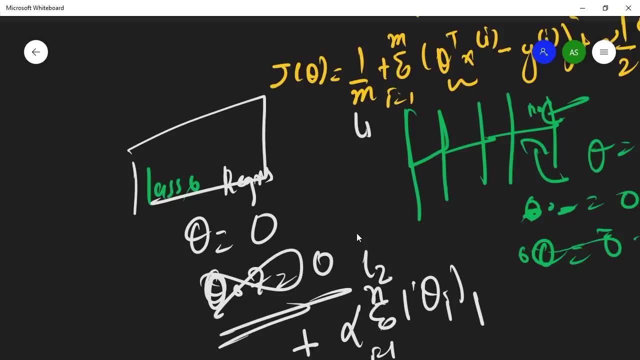 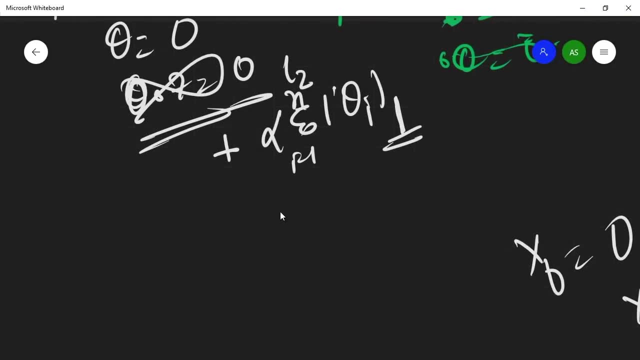 the way down to the end. the absolute value, I and one, yeah, this, this one, okay, Okay. so, but one, one more thing that you did. you can see over here- that we do not penalize our theta zero, which is 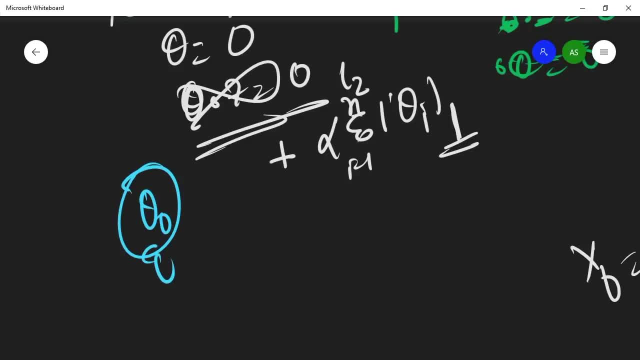 the bias term, which is one of the bias term, So we don't want to penalize this. So we start with I goes to one. So we start with I equals to one, rather than starting with I equals zero. So we do separately all the things, Okay. so what we're going to do is we're going to do a little bit of a. 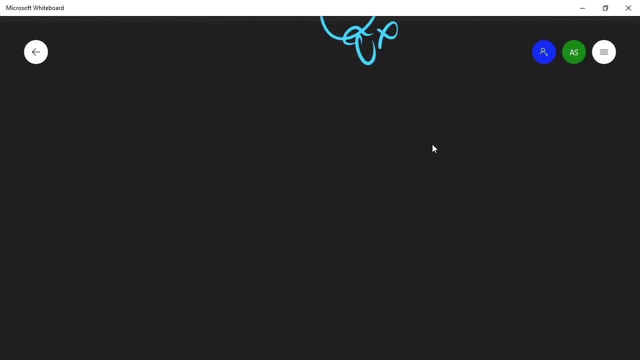 what, what, what we do? we just take, we just start to pay. the i equals to one all the way down to the j, which is the theta, will be separately do zero, okay, And then I think it's very clear, Let, let me. 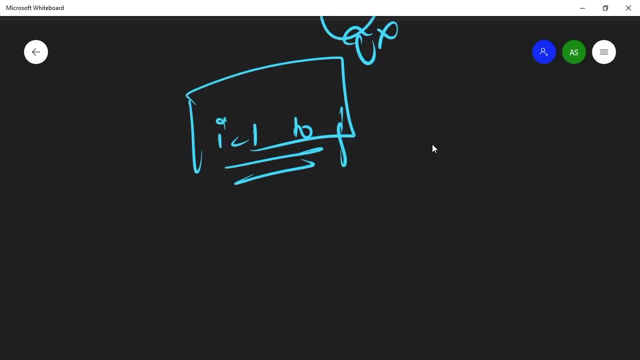 make you clear what I'm saying. I'm saying that you do for, let's say, for theta zero, j of theta zero. you do separately this. you'll do separately this, without the regular regularization term, without, okay, but the whole thing. So what do we do? So you do what we do, and then after that, so we 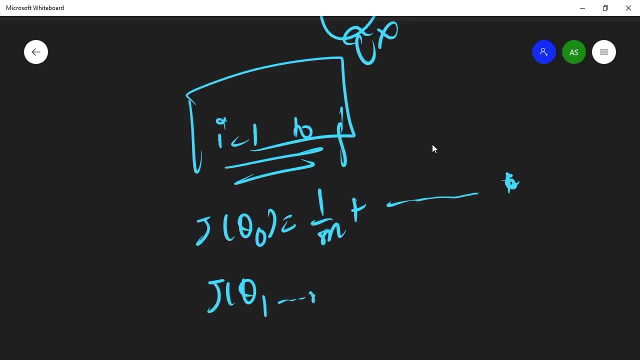 get to the next part. what we do is: we do, we do this, and then after that we do this, we do this and thenamperally for other other thetas, one all the way around to the J: you do, you do at the regularization term, at. 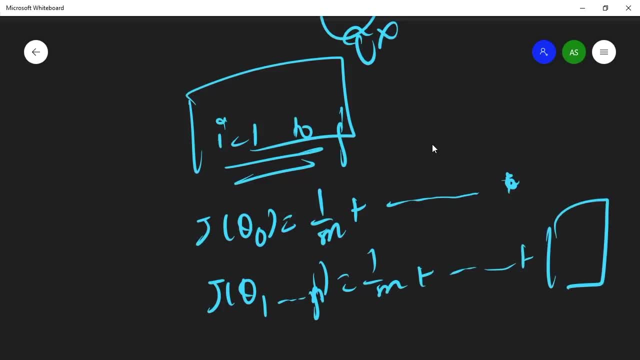 the end of the equation and then you separately update this also, this theta 0, and you separately update this theta 1, and you just take this as a gradient of this theta for theta 1 all the way around to J and this gradient, this, the gradient of this cost function, theta 0 for updating or. 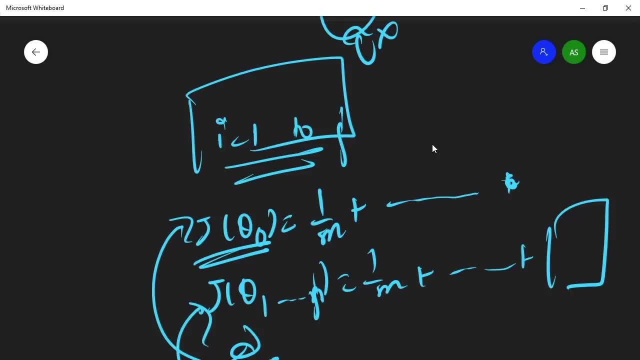 theta 0 and getting the best theta 0. okay, so you do not want to penalize, because only the bias from you don't want to penalize this, okay. so I think that is very clear to you. and again, for recap, regularization is just penalizing or eliminating the less important features by making 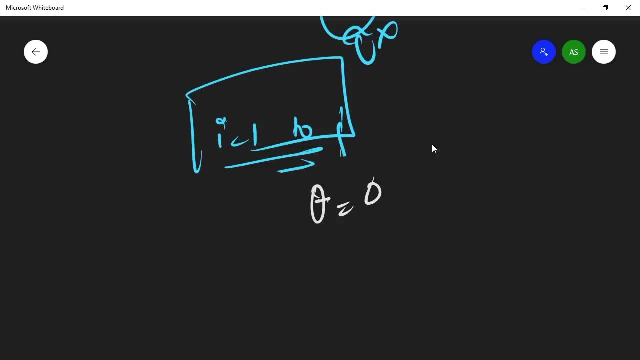 the parameter weights equals to 0. okay, now we hope that's pretty much clear. now we hope that is very clear and in the next tutorial we'll be working on to last regression, with a sorry logistic regression, which is the. now we'll start with classification, which is which will cover. 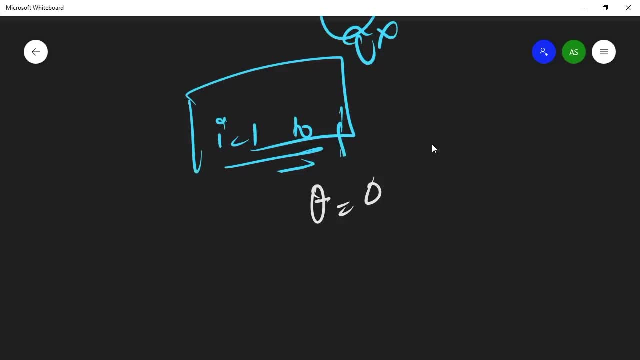 logistic regression as the same as a linear regression, but this is a classification, not regression. okay, so let's, I will be happy to see you in the next section. okay, so now we'll talk about regularization, one of the favorite topic that I like to talk on. I will take around 10 to 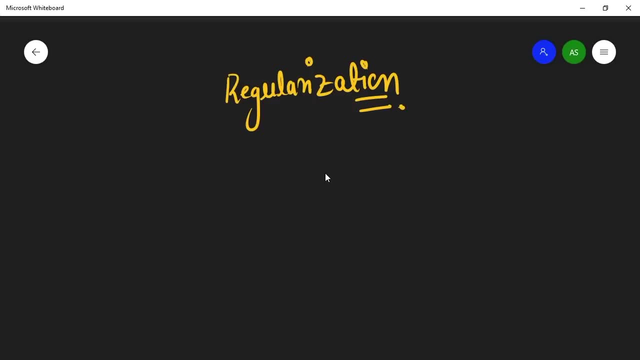 15 minutes to complete something called as a regularization topic, and I think this is one of the most important topics that I like to talk about, and I think this is one of the most important topic in machine learning, or maybe you go to deep learning, okay, so we'll learn about L1 norm L1 and L2 regularization, which is often called a little. 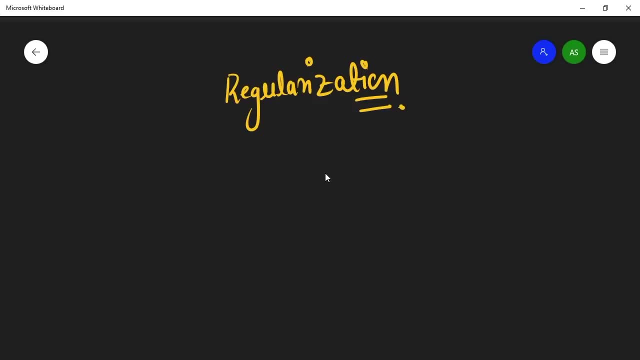 rich and last. so or regularization, and I hope that you will understand that, and why. what is a regularization? so, first of all, this is the problem that should come into mind: and what is and why regularization? I think these two questions must be your first question over here. so, but we're going to talk about that after a couple of minutes on the topic. but be familiariy with just to have a nice memorizing some things, because if you're learning something carefully that it might be hard to learn, and if you learn something small, that maybe you might get mad at that, maybe you might get mad at it, maybe you might fail at example. you know, but if you're 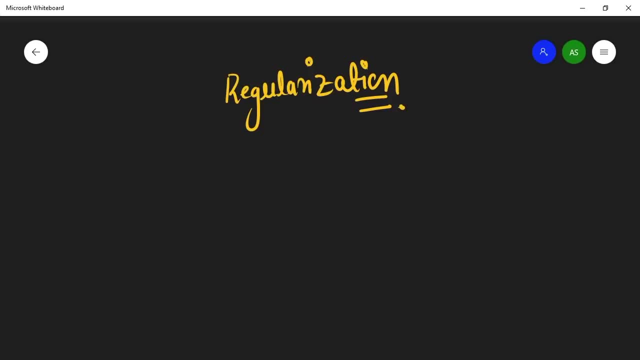 over here. so, but before that, I'm going to highlight one, something called as overfitting, and I think overfitting you all know, but just as just to those who forget about it, let's revisit that. so let's assume that you have an X and Y. 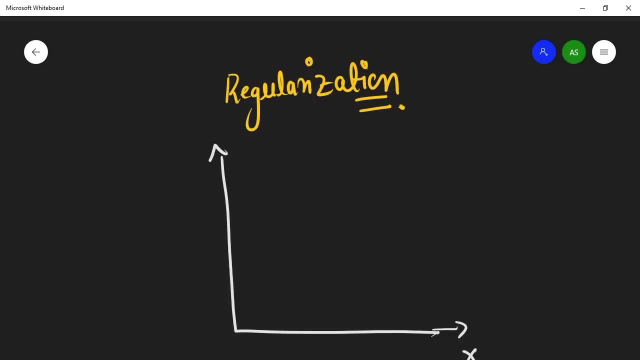 plane X and X here and Y here, okay, and here is here. you have a data point, okay. so you have a data point like this, okay, and you fit it and your model learns a lot. your model learns a lot means your model is performing very, very best on. 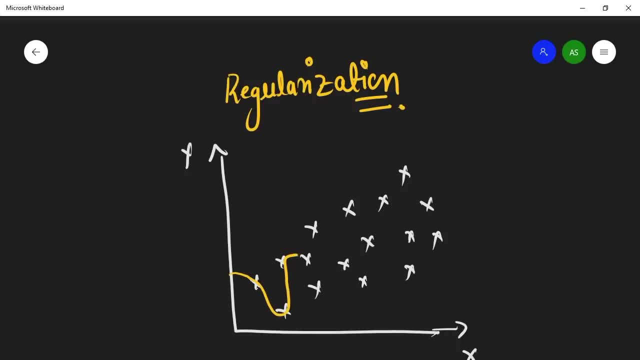 the training set. let's take an example that it performs. it is. it is the, the error. the cost function over to here means that the residual error or the cost function over here will be approximately or very, very low to zero, and the accuracy or on the training set will very, very high. 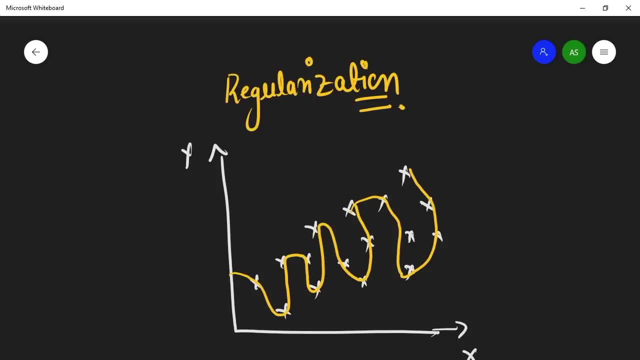 okay. so you have a data point like this, okay, and you fit it. and your model learns a lot because it tries to touch each and every point over here. okay, and here your cost function means the difference between your predicted and actual value. submission over I equals to 1. all around to the end will be approximately equals. 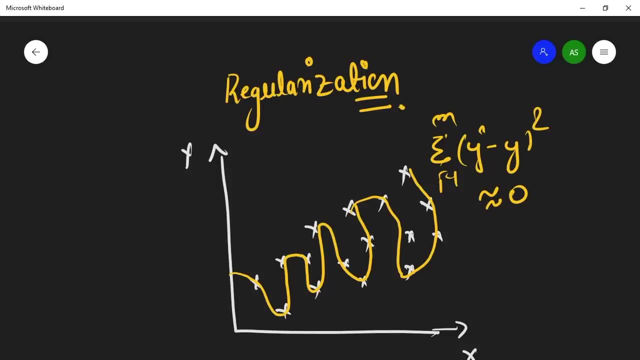 to 0 and if it is, if it is, if you, if it is touching each and every point, so it's obvious, that is, it is very, very best on to the training set on which it is trained. so it has, it has learned a lot, but let's, for the sake of example, some example come over here and some example. 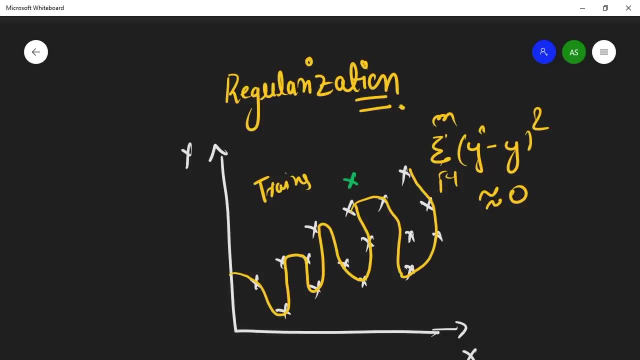 come over here. so what will happen, though? your model will fail to generalize well under the testing set. okay, so that's why I'm telling that your model will fail to generalize well on testing set. so you can assume that that this, this, this, you can see, you can say that this, this model is on overfitting. 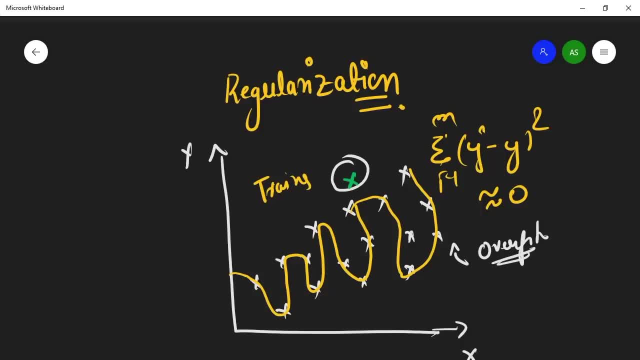 because you find out that your model is performing a very, very best on a training set and then, if you evaluate it, then you will see that your model is performing very, very bad. okay, so that's the sign of overfitting. so we always wanted to reduce the overfitting. so how we? how can we reduce our overfitting? we? 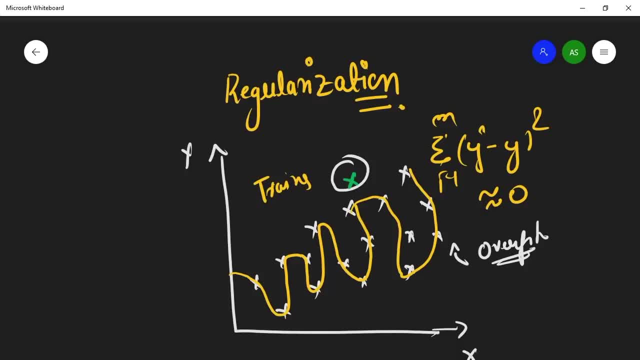 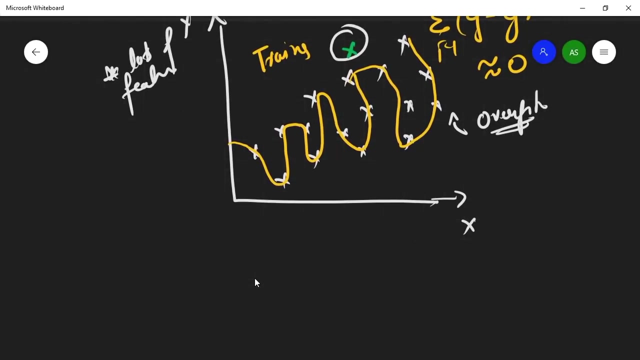 have something called as a regularization and how it happens. it can happen if you have a lot of features, lot of features, lot of features, or your polynomial degree is very bad- high if you're using polynomial regression. okay, so the major cause of problem is lots of features, okay, okay, so now let's see how we can remove this. how. 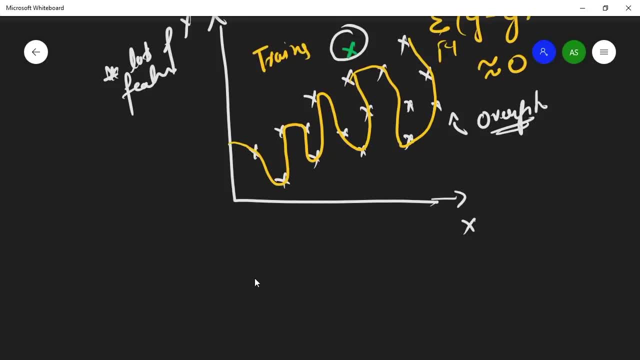 we can prevent or how we can make our, our model less prone to overfitting. so so we have something called as regularization. regularization will help you to eliminate, to eliminate the features, to eliminate the features which are less important. so again, I'm saying it will help you, it. 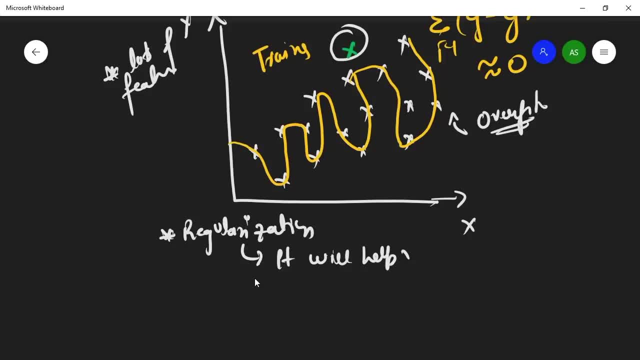 will help you. it will help you to eliminate, to eliminate the features, to eliminate the features which are which are which are less, which are less helpful, or contains a less and less information. okay, so it will eliminate that. so that's how we can reduce overfitting. 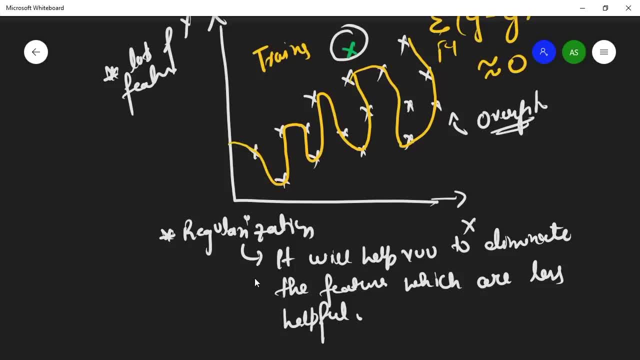 how we. that's how that's what the regularization is doing. it is saying that if the feature is less important, remove that. okay, or make the make their respective and make the respective hyper parameter to be equals to zero: okay. make the respective hyper parameter to be equals to zero means I make, make the 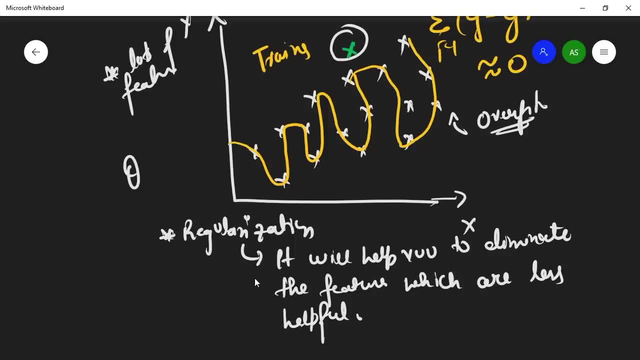 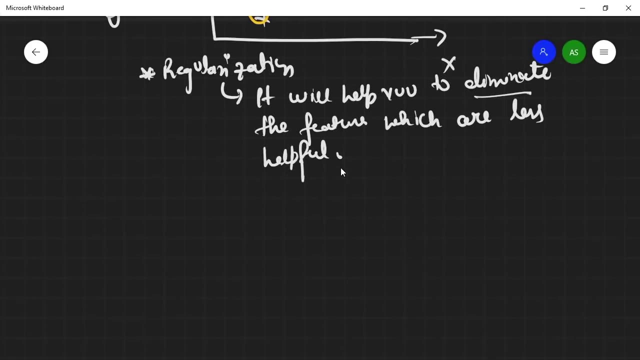 respective, not a hyper parameter. make the respective theta to be zero. so we will see. we will see how what it will do. just just for as an example, let's assume that it will help you to eliminate the features which are less helpful. now let's see how, how, how, how it will do. okay, so let's assume, let's. 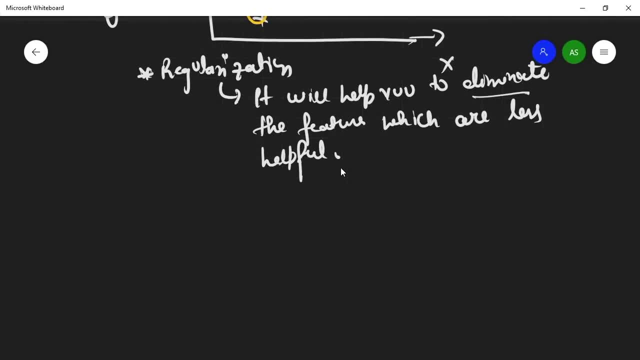 assume that you're working on, uh, some problem which is house price prediction. okay, so so you're working on house price prediction and there you have some features. so here you have x1, so maybe the size of the house, my favorite size of the house. okay, then x2 is maybe your favorite: the number of fans in a house. number of fans in a house. 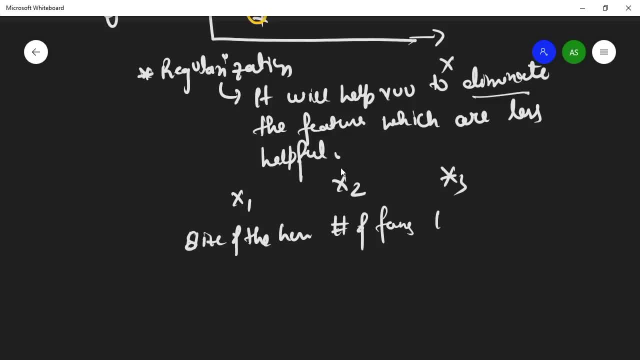 okay, number of x3, maybe the number of bedrooms. number of bedrooms, maybe another feature, maybe another feature. number of, uh, maybe some fan, no, no, fans as well. maybe ACs, okay, air conditioners. so here we have four features, okay, and let's say: and now what we'll do? so we so, for each, for each. 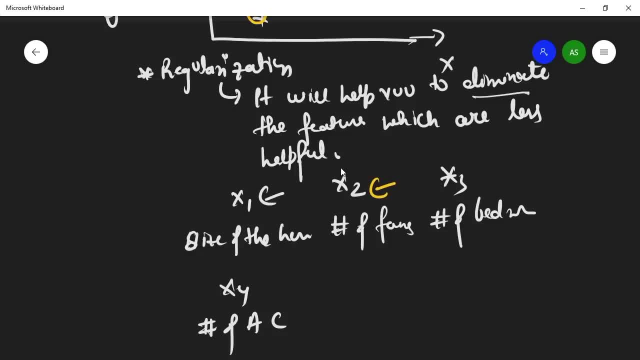 feature. for each feature. for each feature: x1, x2, x3, x4. we'll be having some primary weights. we'll be having some primary rates like theta, theta 1 times x1 plus theta 2 times x2, plus theta 3 times x3, plus theta 4 times x4, and you can see over here that we have this. this is this. 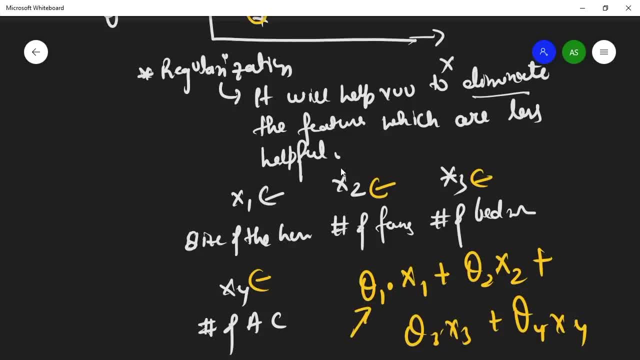 is called the hypothesis function. so here these, the only we did. these are the weights, these, these are the weights of these features, and we only have to learn these weights by just tweaking it. okay, by just tweaking it. tweaking means: let's take an example. I hope that you've already seen a linear regression, just as an overview that. 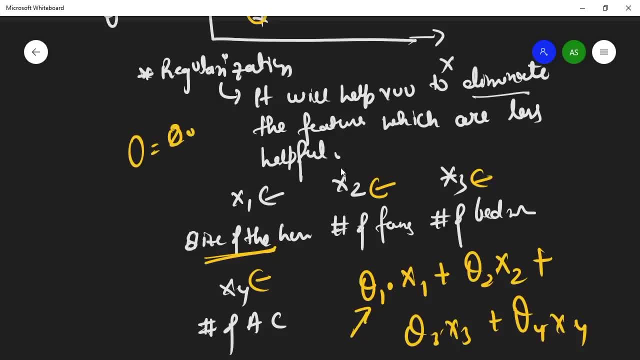 your data was: this equals to 0 to 2.1. theta 0 equals to 2.1 previously. and you just take out the partial derivative of your cost function with respect to this theta and then you update the theta. okay, why? and just see the linear regression part, you all, all will be very clear, okay. so here, if you, 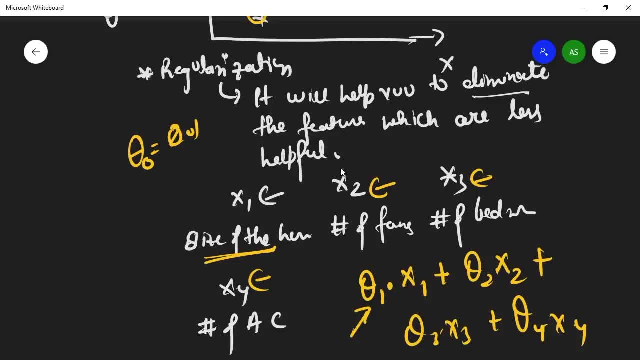 if you're. if you're, if you are being confused, please go to the linear regression, part um. you will be not able to further continue, so, please, please, go back and lay in your regression if you're not able to understand why, what is theta and why it is okay. 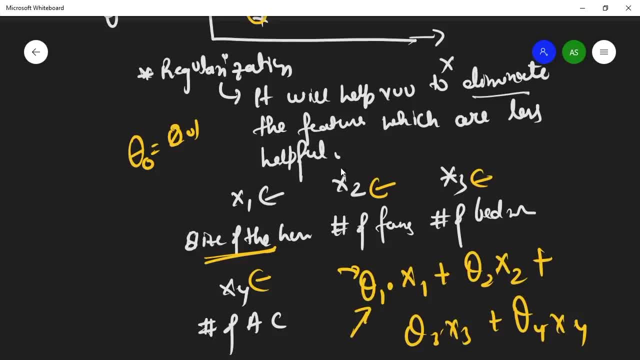 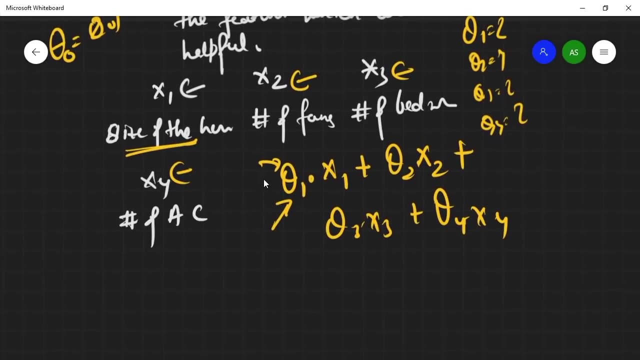 so this theta is a weight for the feature and we can simply give- let's take an example- that our theta one is equals to two, theta two equals to four, theta three equals to two- okay, and theta four equals to two, okay. so we can simply multiply. so these feet, if these thetas to be learned, okay. so 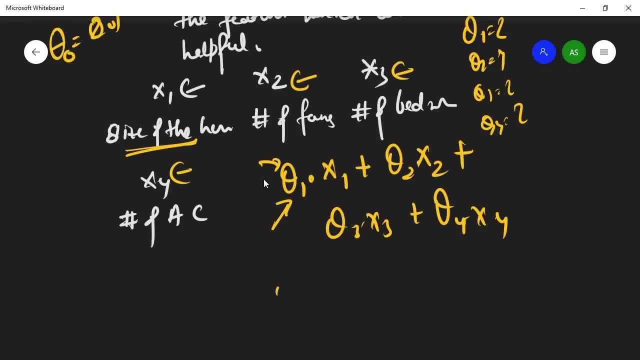 this will give input that listed the size of the house. so two times size of the house, maybe 24 square feet plus uh, then number of fans, though. so four times number of fans, maybe four plus number of bedrooms, two times, because here we have theta, three equals to two. let's assume that the user 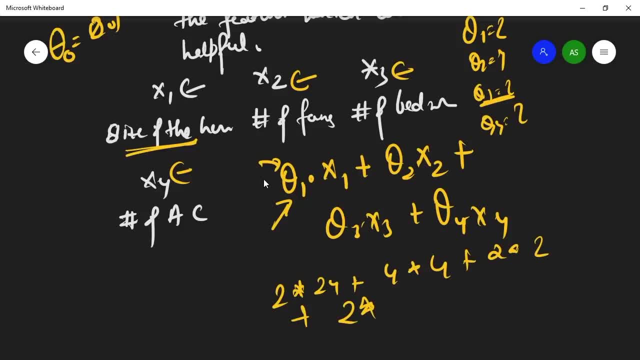 given two plus uh, two times two times, uh, maybe number of acs equals to one. okay, and this, this is it. so here, you learn some weights, you learn some weights, and usually you do the same. you have some parameter weights. you have some parameter weights which you learn by, by tweaking or by changing, and 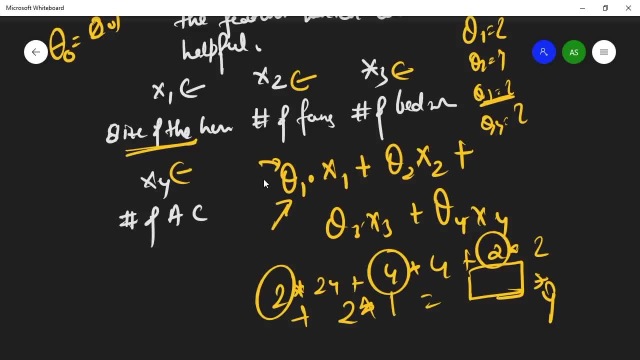 taking a look, if it is, if you, if your model is performing best, and we just take out a partial derivative of our cost function with respect to this theta and then see if our, if our cost function decreasing. if it is, then we update the new theta, then we update our old theta with the new theta. 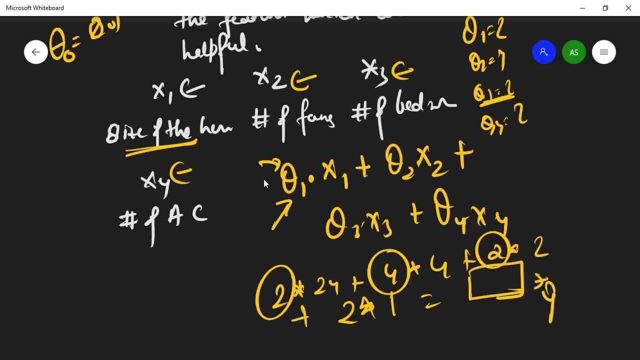 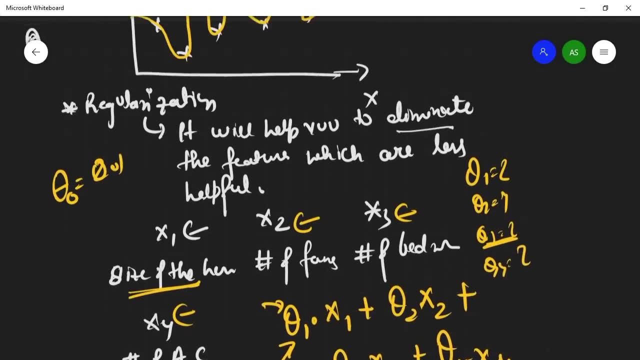 so this is what we are doing over here and I hope that you are understanding what I'm trying to say you over here. so, just for an uh, just for this intuitive examples, I hope that you understood what I'm trying to convey over here. convey you over here, okay? so let's assume that you have this. 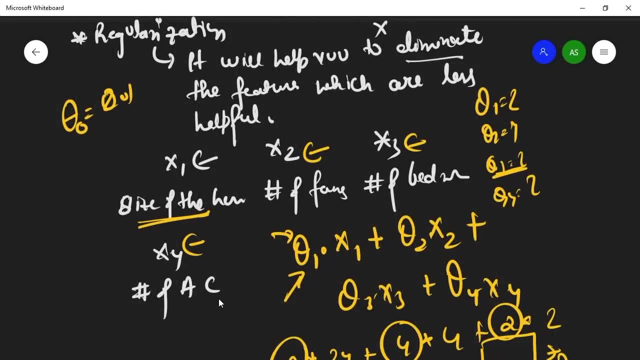 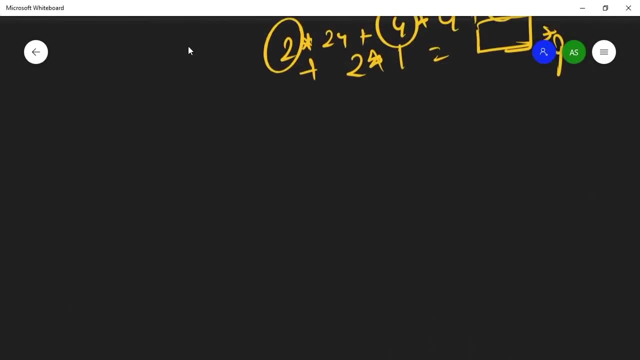 now let's assume that this number of uh, like your model, is overfilling. okay, so what you do in regularization, you apply something called as uh, rigid. so let's see the rigid regression, what it does: Ridge regression, Ridge regression. okay, so the the equation for this regression is: 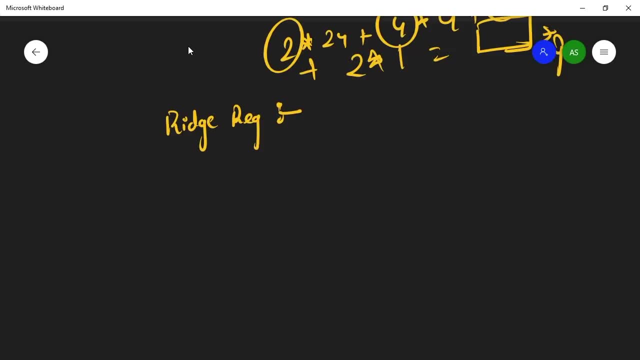 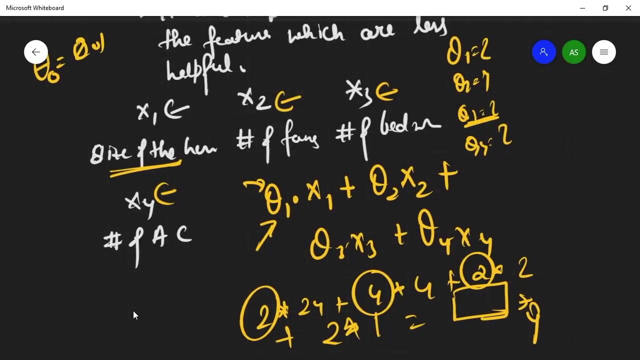 just add, it's just add- a regularization term at the end of the cost function. okay, at the end of the cost function. so again, here we have theta zero. also here we have- oops, what happens? here we have theta zero. also here we have theta zero times x zero, just a biased term because an x is. 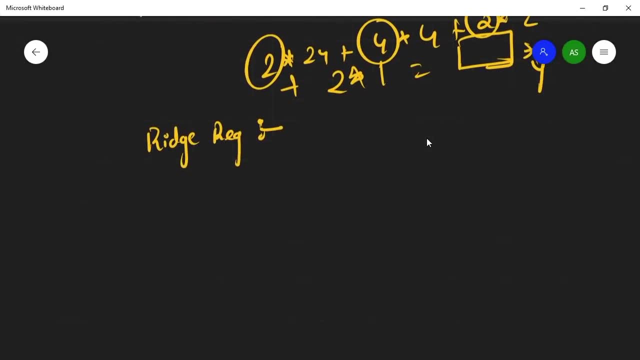 equals to one. okay, so in the rigid regression, in rigid regression we add a regularization term. so here, here's what I'm, here's what I mean. so J of Theta, J of Theta equals to one over M, one over M plus one over M. plus I equals to one. all the way around to the M Theta, transpose three dot. 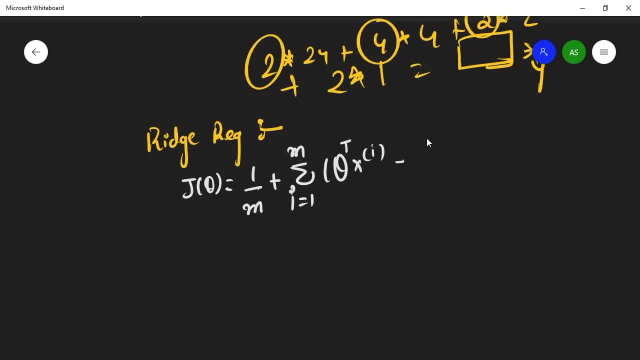 transpose X I theta. transpose X: I minus Y, I squared plus, I'm saying plus. and here we have something called as learning rate and this is just Alpha, okay. so don't assume that is the learning rate, this is just Alpha, uh. or you can have someone can write it as a Lambda, okay, so it is just a Greek letter, uh, just we denote, okay, so don't. 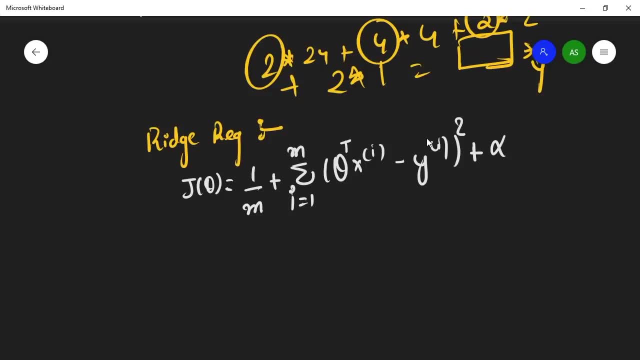 don't compare with that uh learning rate Alpha. do not compare. here I've I will tell you. I will tell you what is this, what, what this Alpha does. one over one over two, I equals to one all the way around to the M Theta squared, I okay. so here we have added a new uh a. 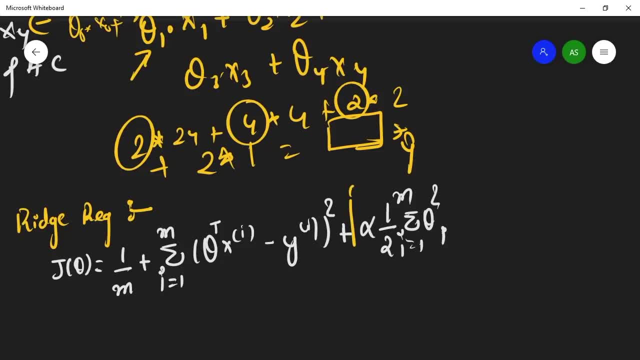 new regularization term, a regularization term over here, a regularization term over here. so what is this? so this is simply what it does. it's simply. it simply make it simply take the features which are which are less important and make that parameter weights closer and closer to zero. 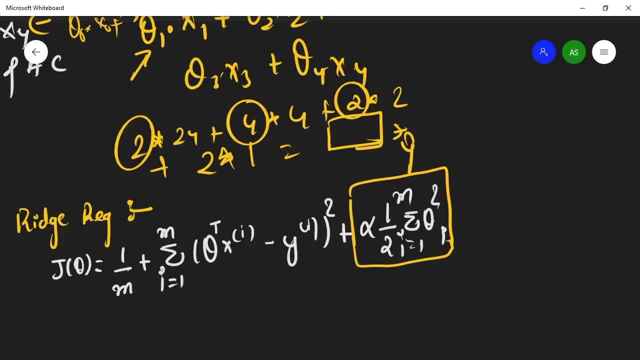 okay. so what do I mean with this? so, for an example, let's, let's assume, let's assume that, uh, that you, that the number of a, your model, this, you, using the, this, using this equation, this is the L1 norm, the it is the L1 norm, okay. so let's assume, sorry, L2 norm, this is L2 norm, okay, in registration, we. 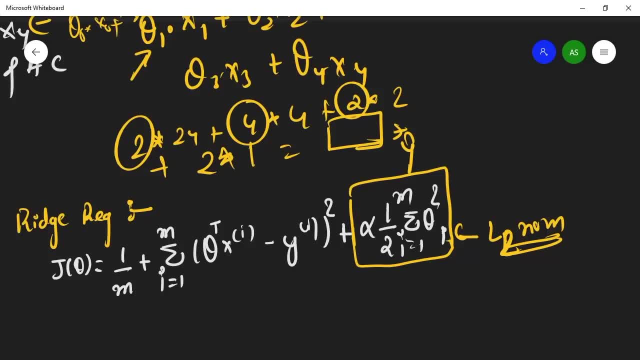 have L2 norm and here it's simply penalizing your Theta, who is very less important. so let's assume that the number of AC or model find out that the number of AC is less important, so what it will do. so, Theta 4, our indicating the 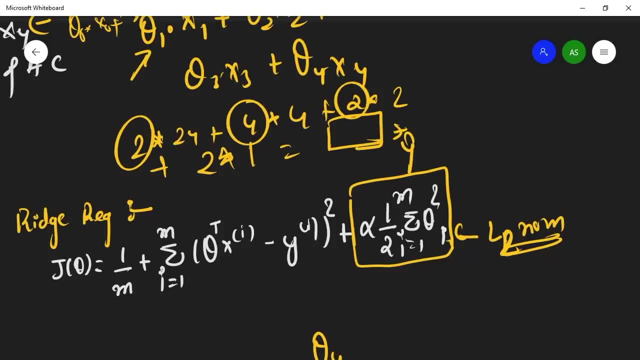 number of AC. the Theta 4 is the weight of our number of AC. then it will make Theta 4 to be to be closer and closer to zero, zero point, zero, zero, zero, zero, zero one. okay, so it penalizes your Theta. it penalizes your Theta as it found, as you, as it found, that your number of AC is less important. so 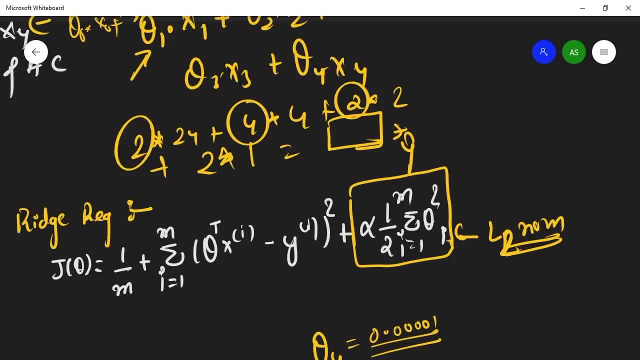 it penalizes your Theta and whenever you are multiply it penalize, penalize, times the number of AC, then it will be also very, uh means low. okay, so that that just helps you to less prone to overfitting. okay, so it is not doing anything with your, with your input. 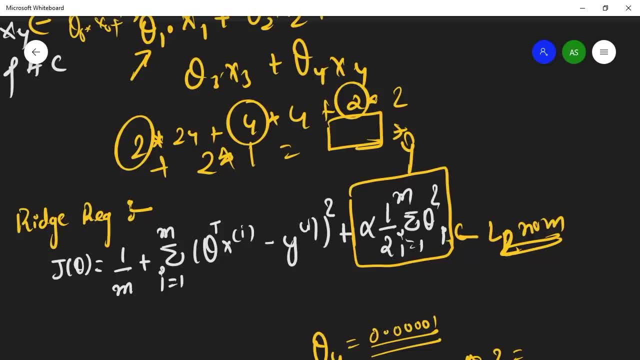 value it is doing because if you multiply 0.0000001 with whatever the number of feature, it will be approximately 0.0000001. okay, so, like, like that. okay. so what is does? simply, it simply eliminates or penalizes your Theta value by just making closer and closer to zero. okay, so this is the 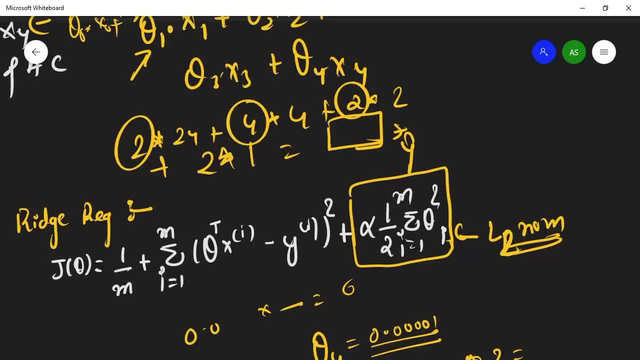 L2 norm. okay, and here we have something called as Alpha and Alpha contains. Alpha contains how harsh or how strict to be onto the certain feature. so let's assume that we have said some Alpha- obviously we don't touch Alpha inside learn, but here let's assume that your Alpha controls the strictness. okay, 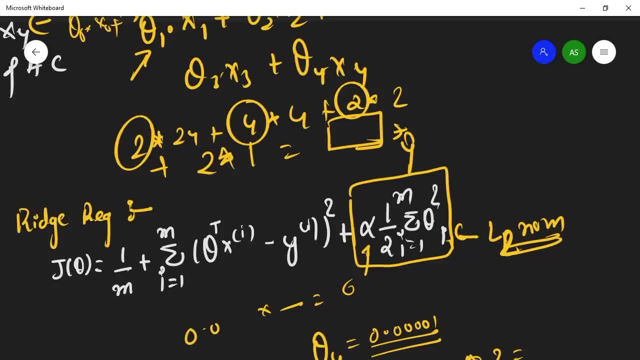 now is a large, I think so if your Alpha is large or Lambda is large, um, some people may write this as a Lambda also, okay, so don't don't be confused. so if your hand Lambda is large, then it will make it. it is making close and closer to zero. now it will make Theta 4 equals to zero, fully zero. okay, so it. 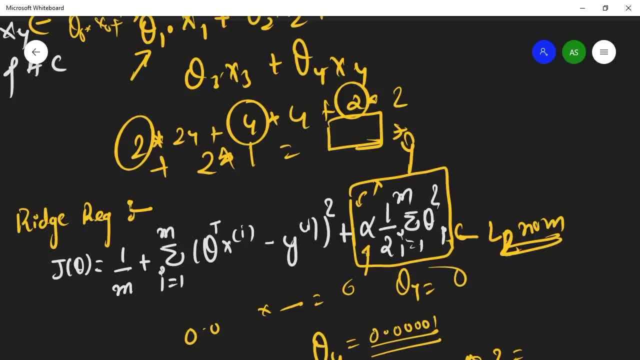 simply eliminates it. if you add: it is very strict. if you keep this, it is very strict, okay. so it controls whatever. I think okay. but I think what I like to remember is: controls the strictness, okay. so, and here you can see that you are taking the L1 norm and you are not taking off Theta zero. you are. 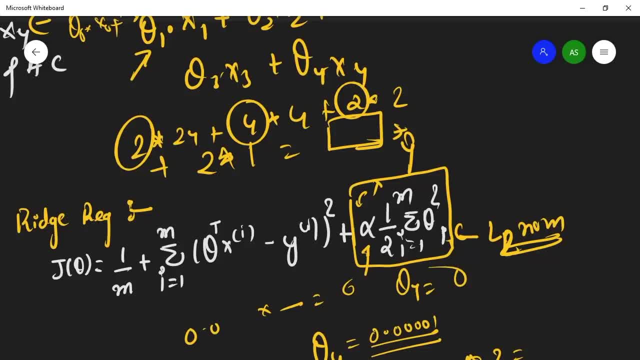 explicitly doing for Theta zero, because Theta zero is your bias term and you do not want to penalize your Theta zero, Theta zero. okay, so we are not penalizing. we are going from Theta i equals to one all the way around to the M. we are not going to i equals to zero. we are going to each and every. 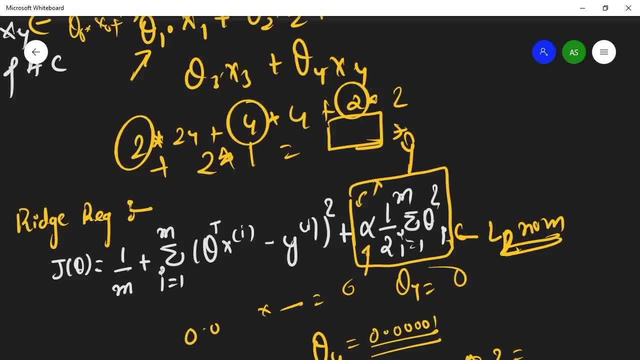 so we are not going to Theta zero, so we explicitly do for Theta zero and we explicitly tween to tweak our Theta. or do we take out the derivative of our Theta explicitly? okay, because we don't want to penalize our uh bias of, sorry, it's uh, our biased term. okay, so this is the rigid regression, okay, so 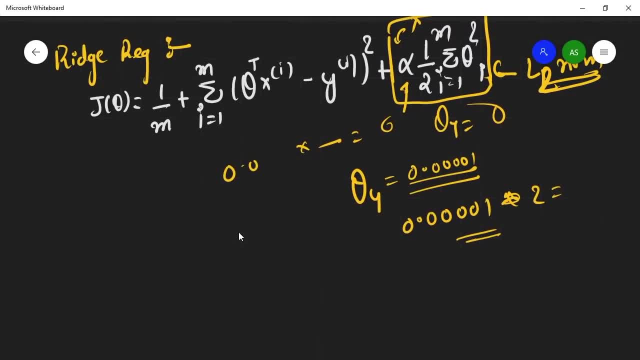 we have something called as a lasso regression, lasso regression. lasso regression means a lasso regression. it's very, very it's it's. it uses L1 norm instead of L2 norm. it's just the same. it's just the same. it's also penalizes the Theta value. but what it will do, I will tell you. okay, so Theta, zero Theta. 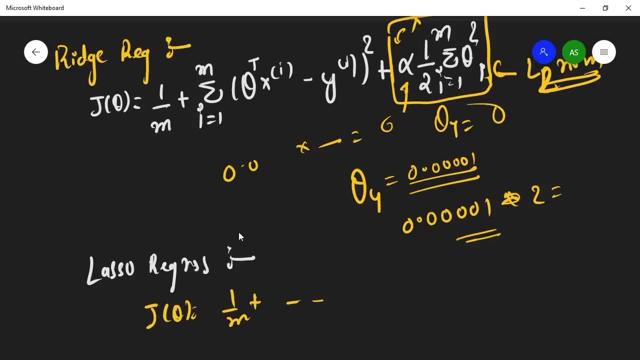 zero equals to whatever your cost function will be. I'm just putting one, two, three plus. now I'm right to regularize. now I'm writing the regularization term. i equals to one all the way around to the M. you are not penalizing again Theta zero, the norm of the norm of Theta i. 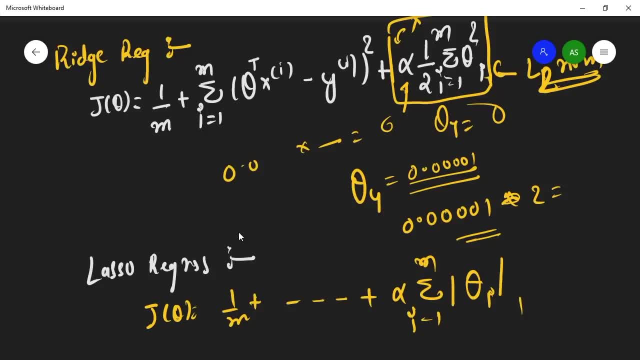 okay, so this, this is what you, and here you are taking the l1, or? okay, so taking the norm, or yeah, you're taking the norm of your Theta, okay, so here, what if here you are applying the l1 Rome, so what it does if he, if, if lasso regression is very strict, just assume it is very strict. 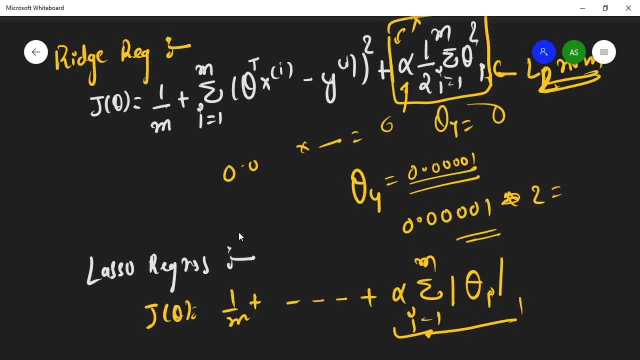 whatever feature he finds, whatever I'm saying, I'm taking the gender as a he, okay, or whatever this, this lasso regression finds whatever feature that less important he finds, he will directly make that theta 4 to 0. so here we assume, here we take in: theta 4 equals to closer and closer to now. then 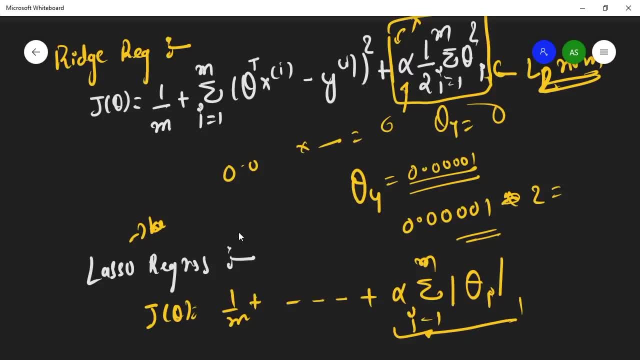 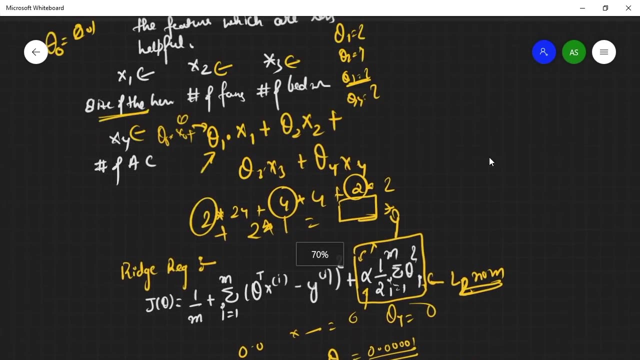 in lasso, it will take it directly to 0, okay, so it is very harsh. so the both have specific use cases, okay, so these are the. this is called the l2 l1 norm and this is called the l2 norm. okay, so here we have studied about regularization in detail and i hope that you understood very, very clearly and 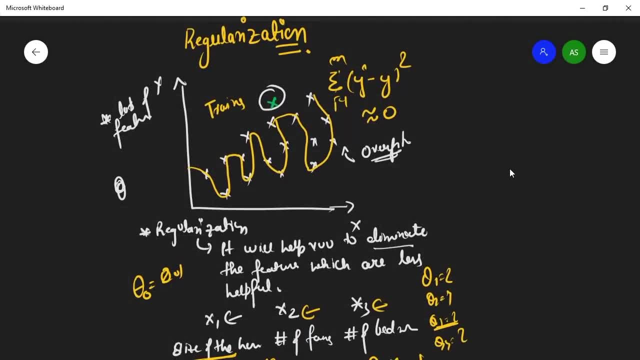 uh, we have talked a lot and there is one more, which is elastic net, which you don't need to worry about now. it's very kind of a just combination of both of them, but it's not used in industry, as we use this l1 and l2 norm. okay, so thank you for seeing this video about regularization. 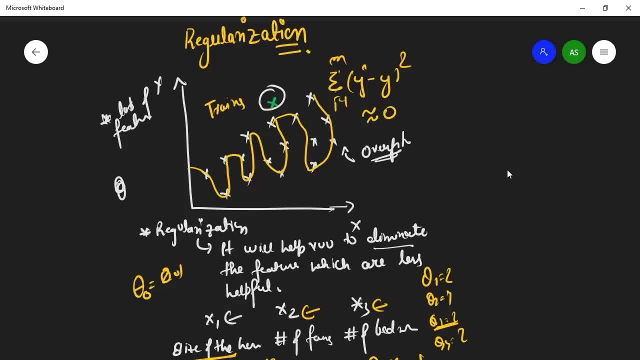 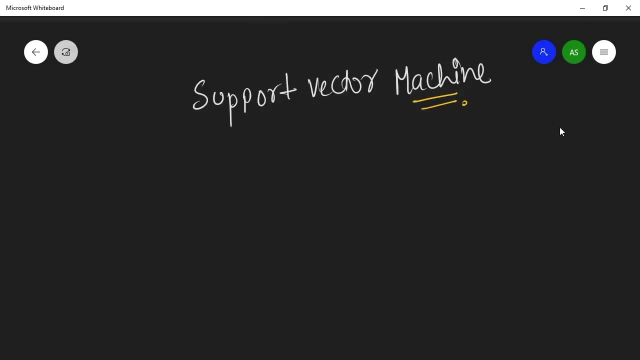 and, and you can head over to the next section to learn more about more about machinery and completing this course. okay, so thank you for seeing this video. head over to the next section. okay, so now we will talk about support vector machine in detail so that you could be more powerful in machine. 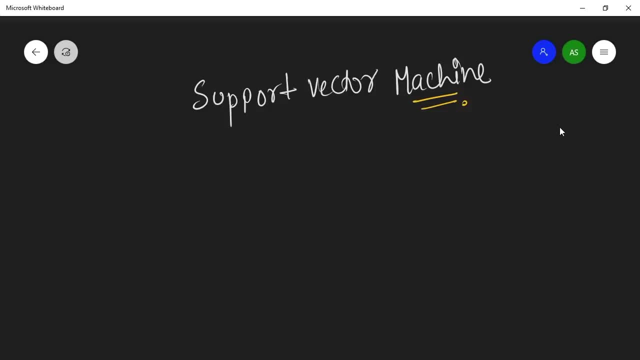 learning or you or you will be having a powerful algorithm in your toolkit of machine learning. so support vector machine is a supervised learning and learning algorithm which is a both for classification and regression. we have seen logistic regression and legislation is for classification and linear regression is for regression. so support vector machine is for both. 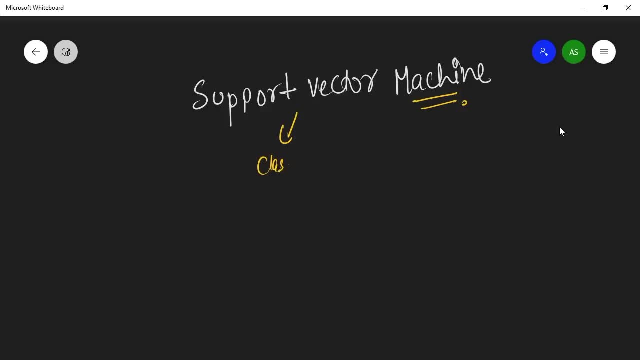 which is classification, which is classification, and one more which is, uh, regression task. okay so, regression test. so, support vector machine can be used in classification, either your output and degree value, or it can be used in continuous value. okay, okay. so, uh, let's, i will dig dive into support, like the 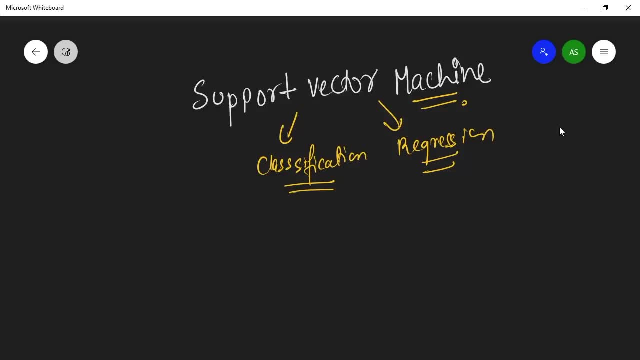 machine. but before that, uh, let's, let me tell you what we are going to study in this section. so we'll use. we start with the introduction of support vector machine, then we'll go further into what svm do, and then we'll talk about linear hard margin, then we will go further into non-linear 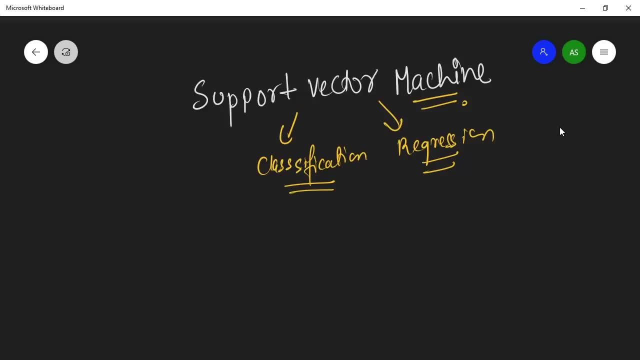 classification, and then we'll talk about empirical risk minimization and then a semi-supervised transductive svm, and then we will talk about svr, which is support vector regression- okay. and the next section: we will do one project, which is stock price prediction project- okay, okay. so, uh, what is svm? what actually svm does? it's, it's, it's simply just what is like this. so let me. 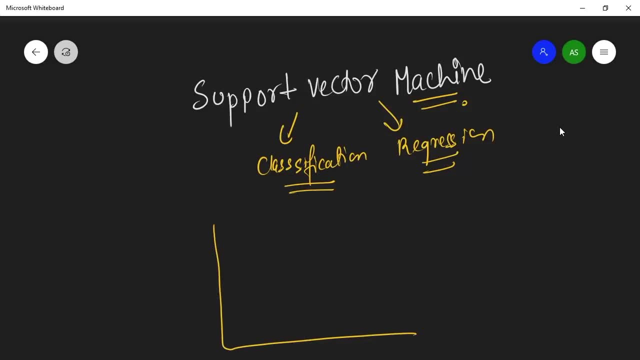 draw one x and y plane. so here is my x and y plane. i hope that's, that's beautiful. so here is my x and y plane and let let me make a linear data, okay. so here we have the one data point, and another data point is over here. 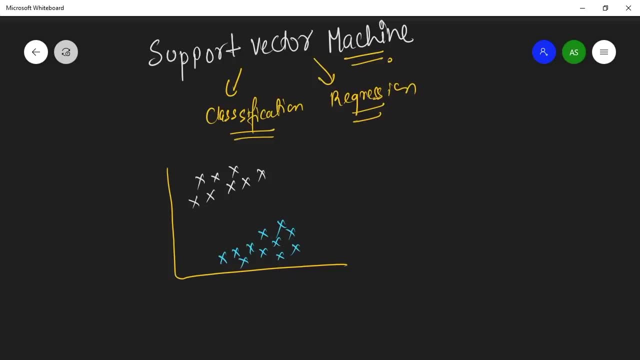 so we have like this. okay, so we have like this, and then we have this data. okay, so let's assume that that you're working on cat and a non-cat- uh, antique coffee cognition system. okay, so you're working on cat and non-cat recognition system. so what actually svm does is here you can see over. let's assume that white color. is for cat images means the labels are cat and blue color. let's take a look now. if you choose to do it with the PRODUCT COORDINATOR herself, then what you do is: if you choose to do it with the PRODUCT COORDINATOR itself, then they And check the ugly flux property you. nuel körter and compare and tell us how to do the same, so that way you can start toiving more visible parts of the block and similar the articulating model and save too much weight. you get better performance and us, as finnish, remember till we get back to movement of our 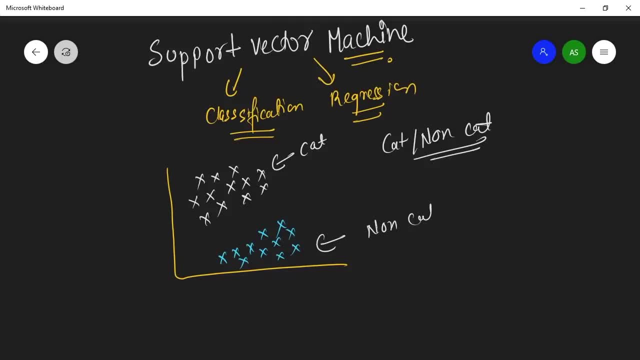 let's take as a non-cat. Okay. so these are data and what SGM does it makes: it constructs a hyperplane. it constructs a hyperplane like this. It constructs a hyperplane like this: Okay, and now, whatever new point come on or beyond here, then this example will be cat. Otherwise, if something come here, then it will be non-cat, Okay, so 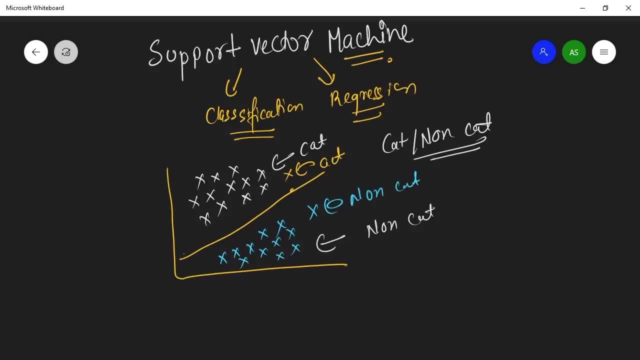 this is what SGM does, But this is not the full procedure. I will tell you. But here what it does: it simply constructs a hyperplane and two parallel hyperplane, and one, two parallel hyperplane, two parallel hyperplane. this margin- Okay, these are called a margin, So it always tries to maximize that margin. So it may sound a little bit confusing. So let's draw it again to, let's. 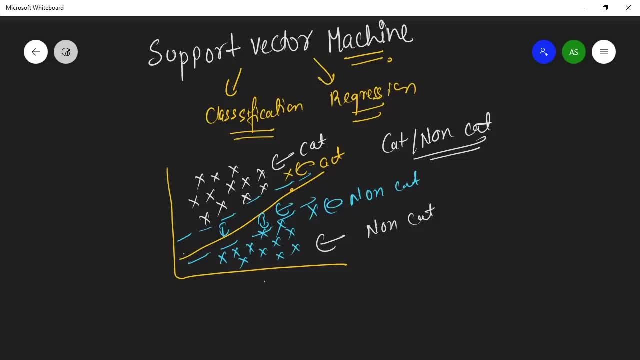 let me show you once more time what actually it does. Okay So, here is a white examples And here is your blue examples. Is it non-cat and non-cat? So what it does is construct a hyperplane and a two, two parallel hyperplane over here, two parallel hyperplane like this. Okay so, and this is called the margin. This is called the margin And SGM. 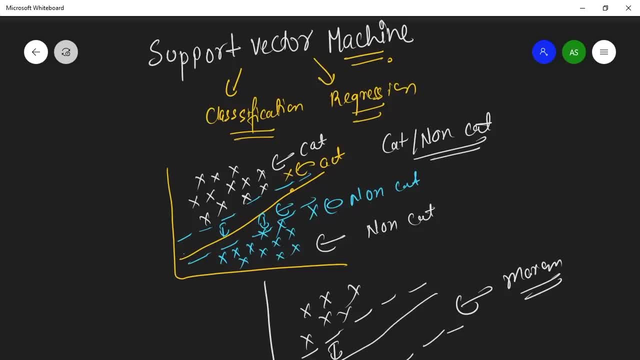 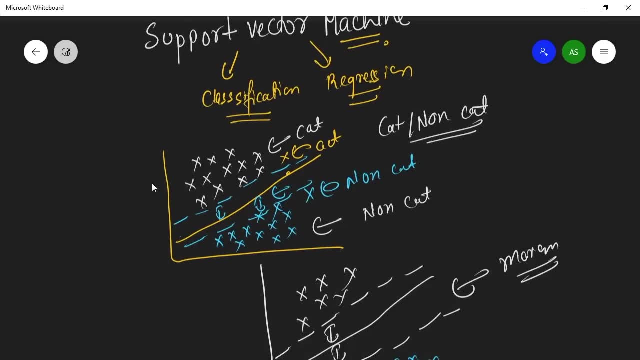 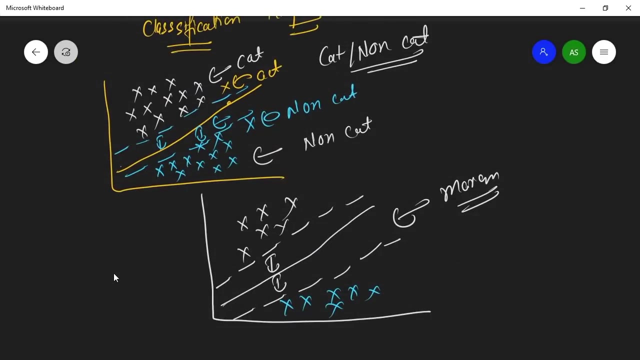 always tries to maximize this margin, keeping away the nearest data point, far away from the hyperplane. what I've said is very crucial to listen what I'm saying. I'm saying that what SGM does? it simply construct a hyperplane and two parallel hyperplane. that separates the data. 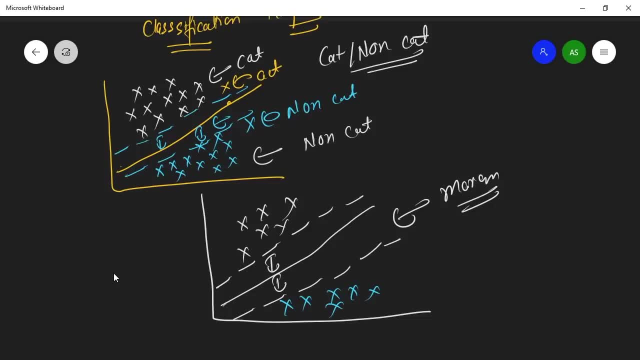 point and at a maximum margin. Okay, so it always wants to, SGM always wants to maximize that margin and such a way, in such a way, in such a way, such a way so that the nearest data point, so that the nearest data point, let's say: 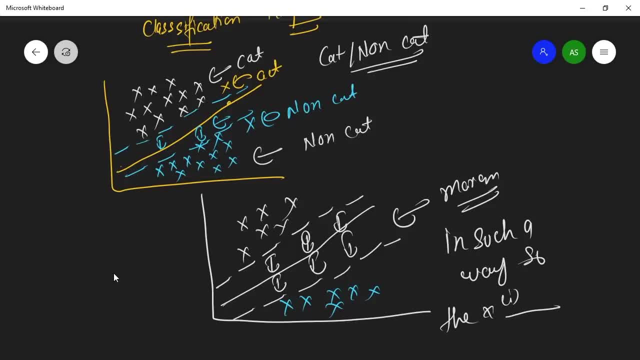 xi is far away from the hyperplane. this hyperplane, okay, is far away from the hyperplane. so that, so that it would be easily, so that whatever comes here, then it would classify as a, as a non, as a non-cat, whatever comes here or here, it will be classified as a cat. 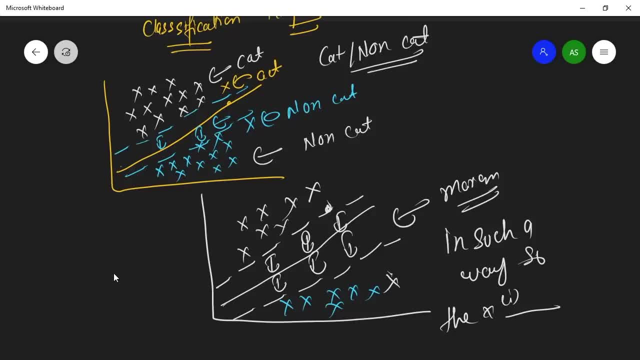 okay, and and and what I am saying, that the nearest data point and the nearest data point is far, should should be the far away from the hyperplane here. okay, so it would be here. so these are called the support vectors, who are the nearest data point from the hyperplane. 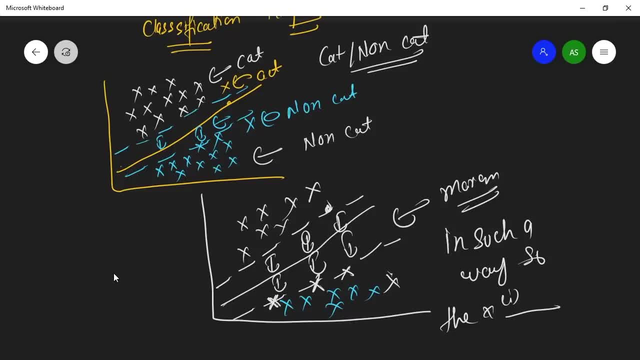 okay, and that is supported by. these are the support vectors which supports this parallel hyperplane. to separate this? okay, Again, it's me. It may sound a little bit confusing, so let's revisit this again in a more detailed way. 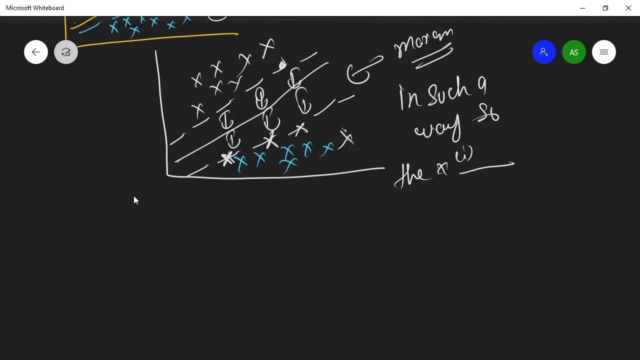 So let's say: let let's take another, another example that we are building. a person has a cancer or a non-cancer, I think the original. let's say a non-cancer. okay, so you build xi plane, so let's build one xi plane, and then you put this blue example which is: 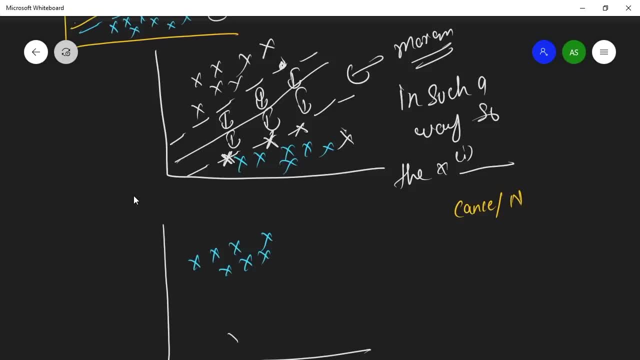 which indicates as a cancer, and this white example, which indicates as a non-cancer. Okay, So what is the? simply construct a hyperplane like this. oops, it simply construct a hyperplane and a two hyperplane like this and a two hyperplane, and this is, this is called the. 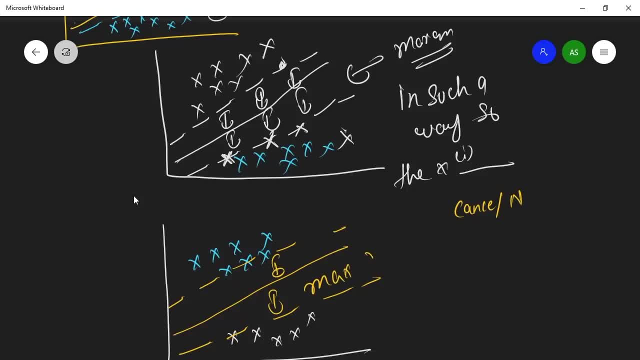 margin and it always tries to maximize this margin so that in such a way, in such a way that the nearest data point is far away from the, from the main hyperplane. okay, so you can see over here that this, this is the nearest data point. it's far away. so these are called. 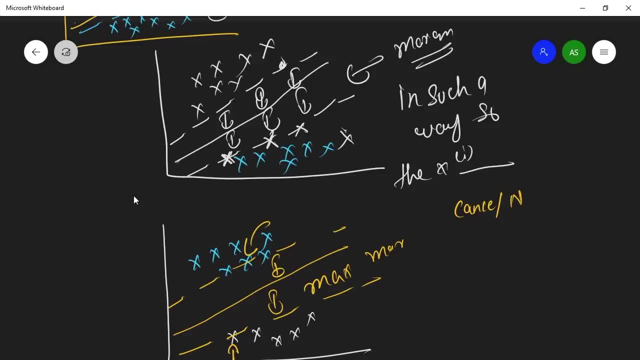 these are called the support vectors. these are called the support vectors. okay, pretty much easy. now I think that's it's much clearer. we have- we have taken three examples. now I think this is much clearer. okay, So it's. it may sound to you like it's. it's like a linear regression. you have a linear. 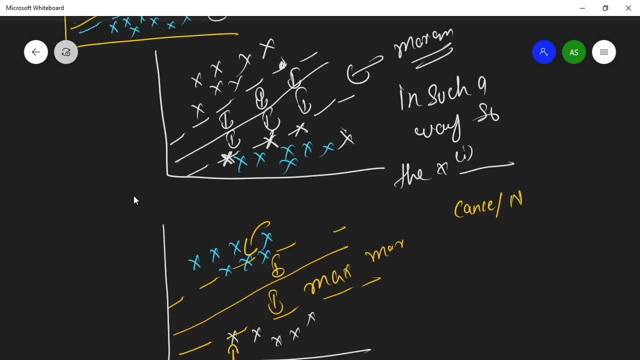 data and you're just filling a straight line with two hyperplanes. what does it mean? it obviously means like linear regression, but if you come to the more in detail, the data are not lean, not linear. okay, the data are never linear. 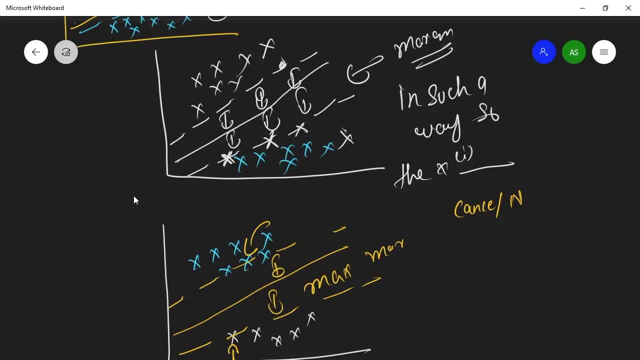 So there are two kinds of SVM there. the first kind of is hard margin classification and soft margin classification. okay, so let's visit, visit hard margin first and then we'll revisit soft margin, okay, okay, so here you can see over here all that. this is just. 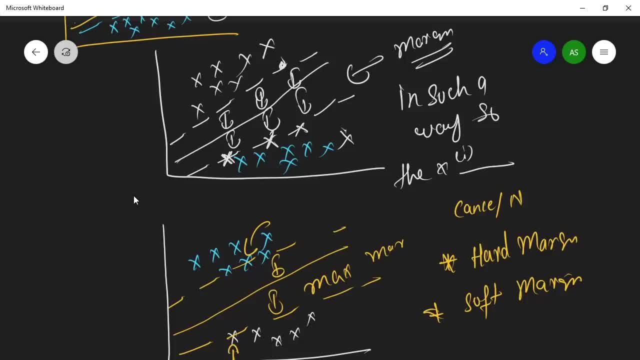 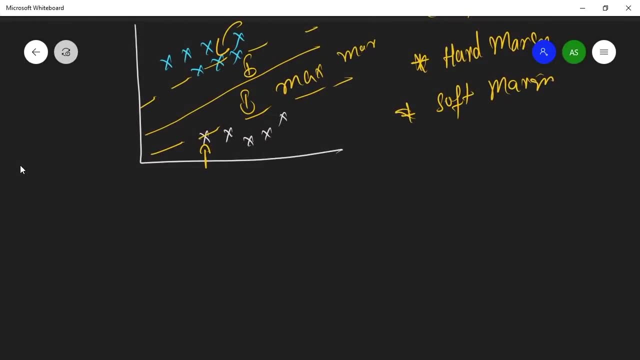 like linear regression, but wait for a few seconds, few few minutes, then you will understand why it is not like linear regression, Although it seems like that you have simply constructed a straight line, but the equation and it's used for classification, it's quite, quite different, okay. 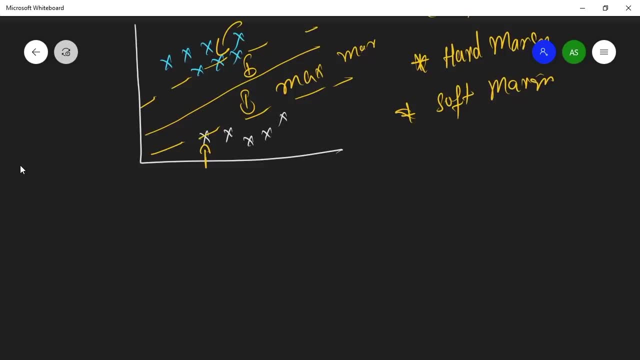 Okay, so in it's called a linear SVM. the word we have seen is called linear SVM. we are here constructing a simple hyperplane and separating two data points. okay, So what are hard margins? Hard margin means that we are not allowing any data to be generated. 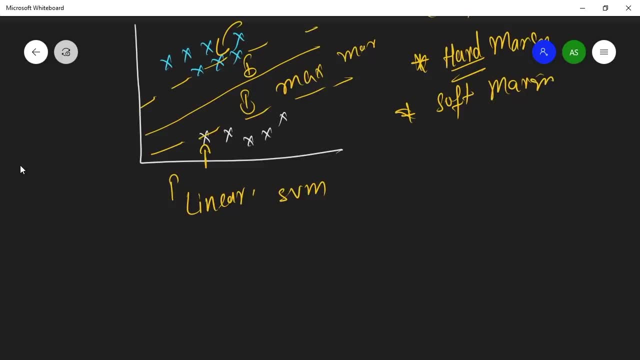 Okay, Okay, Okay, Okay, Okay. So we are not allowing any data point to come into that margin. okay, that's called the violating the hard margin, sorry, violating the margin. so we are not allowing any data point to violate that margin. so in that way we end up being an overfitting, or in that. 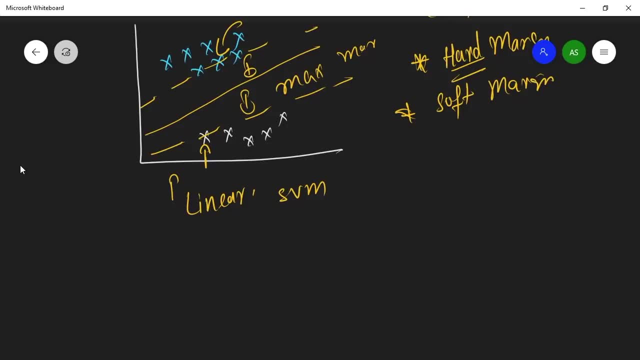 way. we very much. we, our, our model is being started overfitted. So let's see what, what I'm trying to say over here, over here. So let's construct a hyper, let's, let's construct one X and Y, and we're going to. 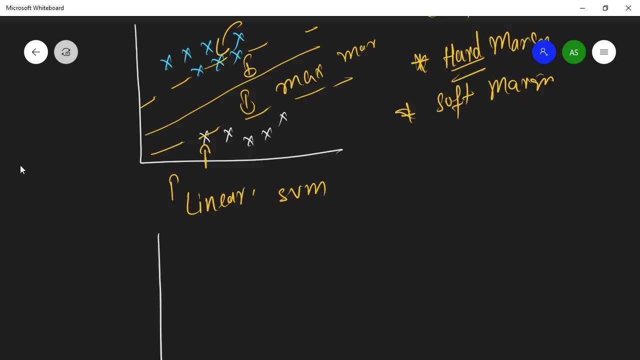 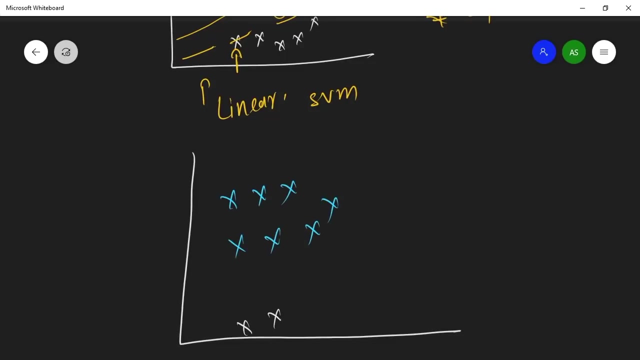 construct one X and Y plane again. so let me construct one X and Y plane. oops, here is my X and Y plane and let's let's just draw two data point again. let me draw two data point like this: okay. and let's draw a Y data point like this: okay, okay. so and 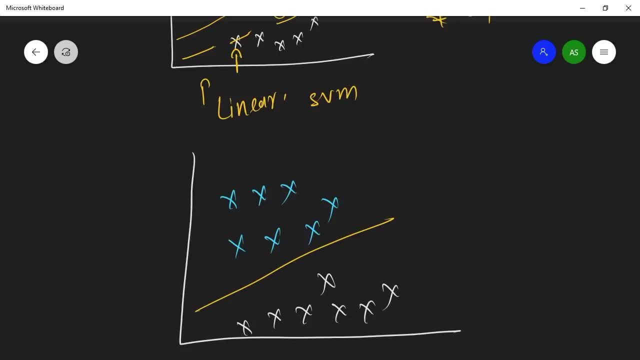 now what SVM does: simply construct a straight line with two hyperplanes, okay, with this hyperplane, Okay, Okay. so in hard margin, we are not allowing any data point that it comes under in. so we simply kind of do like this. we simply kind of do means we simply minimize this. 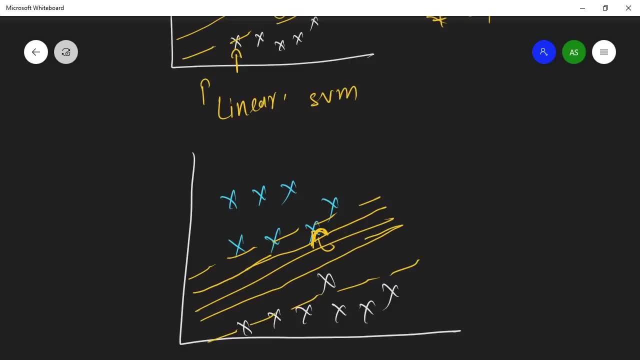 margin like this. so we are doing like this, all it. it is very strict. hard margin is very strict. hard margin is very strict. the reason I'm saying it's very strict because it it does not allow any data point to come into that margin. but in soft margin we allow. 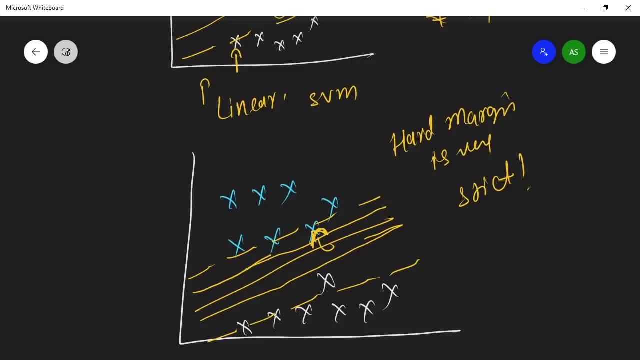 some data points to violate that margin to avoid over-fitting. okay, so that's what the soft margin and hard margin means. Hard margin, it means we are not allowing any data point to come into that margin, and soft margin means we are allowing a little bit of data point to come in that between 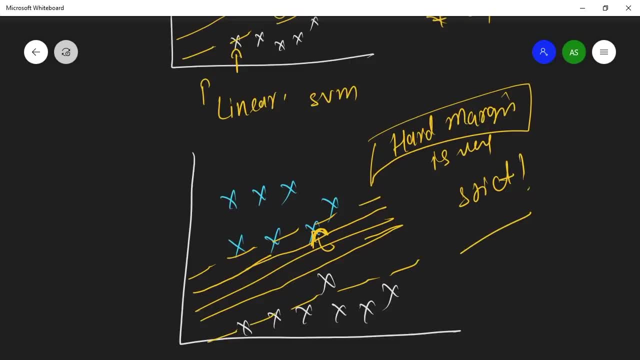 and the width is and the width of the margin. this is the width. we are showing the width right. All right, the margin is adjusted by C. okay, so if C is very, very large, then your width will be very, very small, like this. okay, let's say C equals to zero. this is 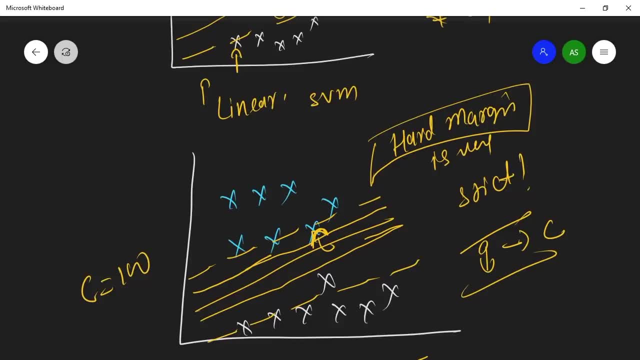 the margin, my margin. so this is my margin. so let's say your C hundred C equals to hundred, so your margin will be very, very. the width of the margin is is kind of a low means. it's very slow, kind of it's very small. but if, if, if C. 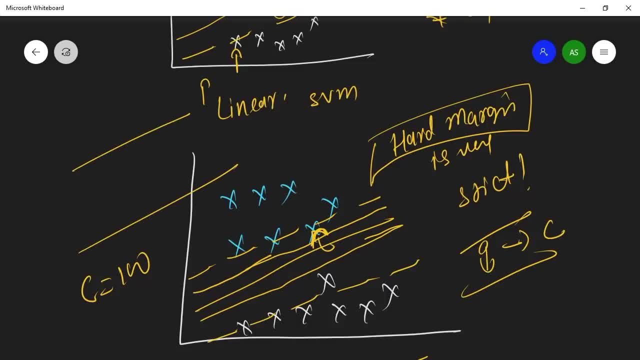 equals to one, then your the width of the margin will be very, very large. okay, like like this. so it's just kind of any. it's kind of a very awkward thing that you can see over here, but that's what the convention site. okay, so we have seen. 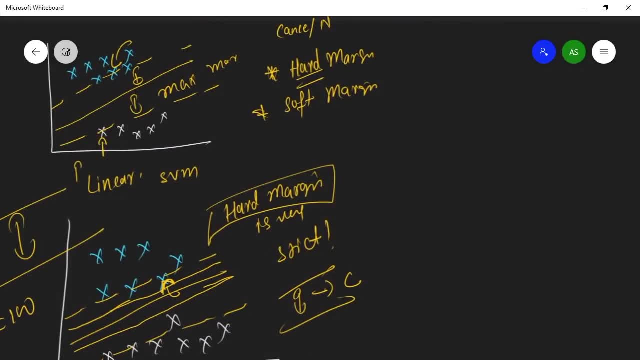 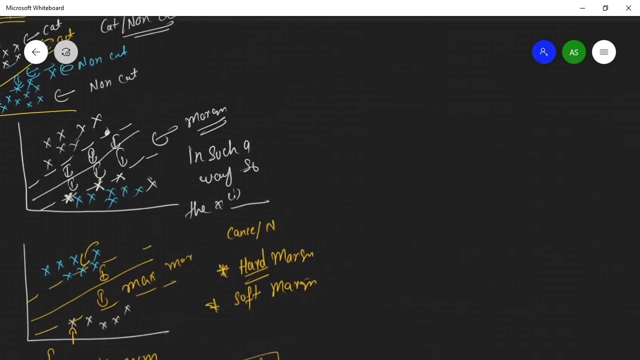 there's this kind of thing and maybe you will see sometimes C to be named as lambda. okay, it's just, it's just the same. lambda and C are the same, just as convention. we give it a C as a name, okay, so let's just to get so. now is you, now you've got the overview of this hot. 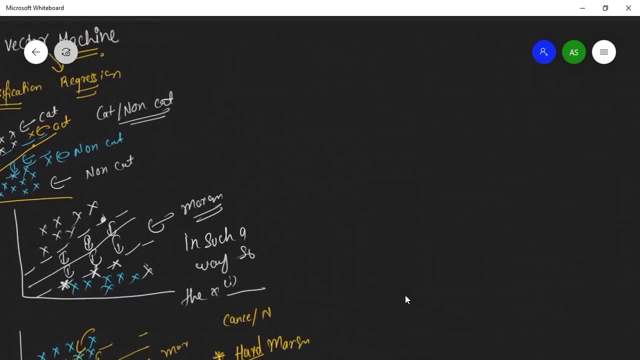 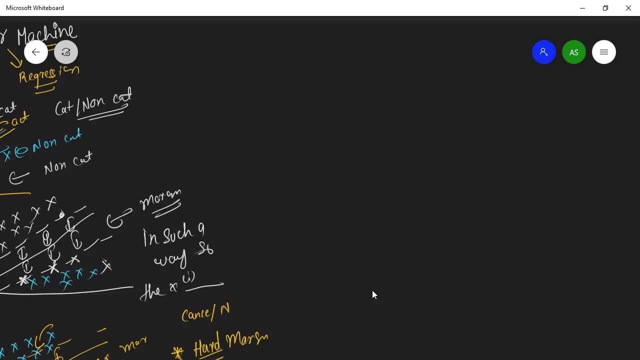 margin and SVM. so we have seen a lot more things. now it's time for getting into the little little bit of mathematics, which is how do we construct a hyper plane? in linear regression we are just making the straight line, and this is theta transpose X. but this was our favorite equations, like this theta. 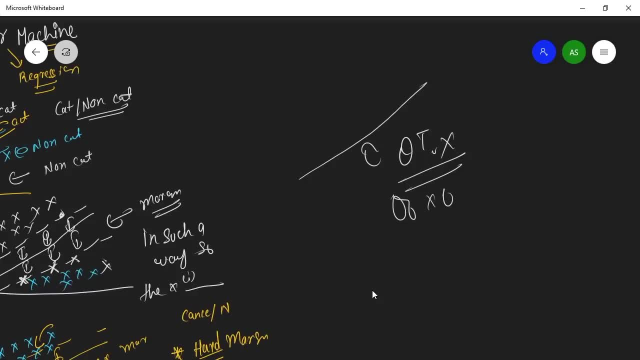 0 times X, 0 and in legislation we are just doing the sigmoid of Z. so these are our hypothesis. so this from this equation we are, we were making our straight line or maybe the sigmoid. so what happens in case of a support machine we have, our hyper plane is due, is due. our hyper plane should, if is defined by: 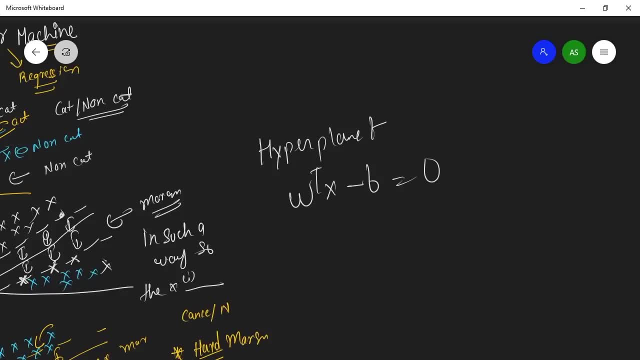 W. transpose X minus B equals to zip. this is the condition that our hyper plane should satisfy, okay, okay, so what is that this? this W is our parameter weight, is our parameter weight in this guy in linear question we have seen, is theta and B is our biased term, which is in. 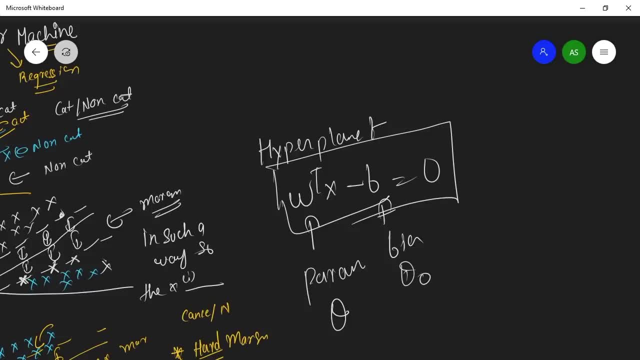 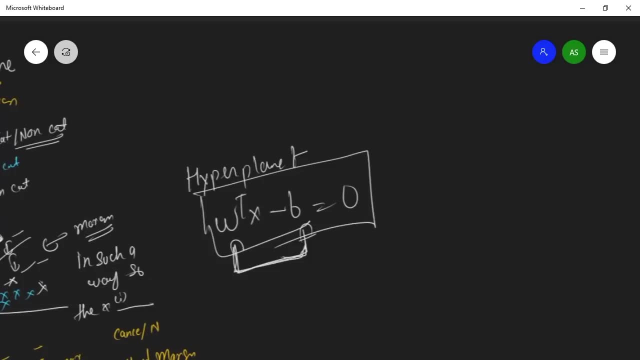 case of linear and logistic, which is theta 0. okay, so we have just just given over the new name, which is W and B. okay, and it's okay. so we have made a W, transpose X minus B, and this is our hyper plane that we have made as a W. 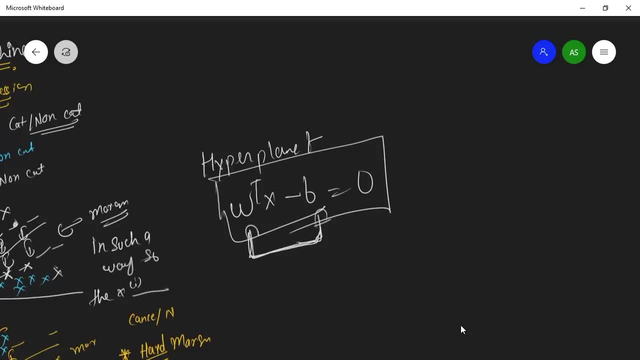 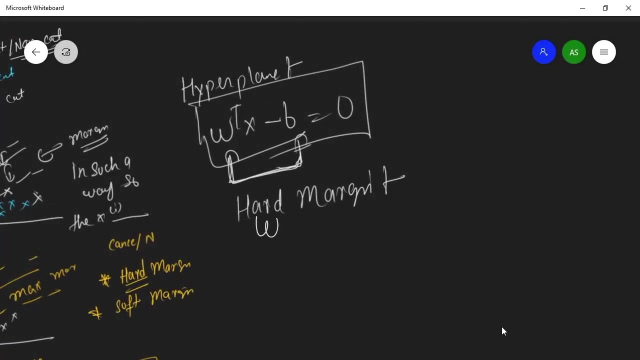 and B are the parameter weights. okay, so we have just just given a new name and transpose your own linear algebra and this is: W is a parameter vector. okay, so let's define some constraints in for hot motion. so let's define some constraints for hot margin. how hot margin make predictions? okay, so whatever, whatever. 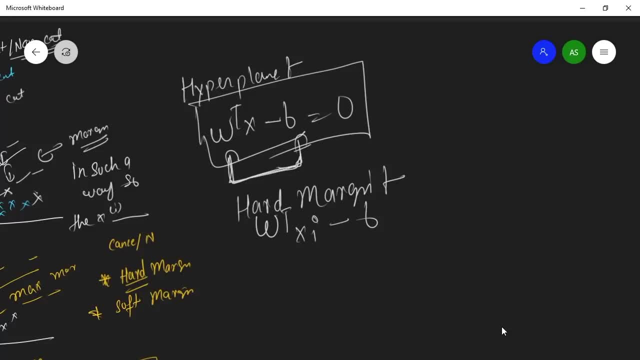 the output of your model minus W, transpose X minus B- is greater than or equals to 1, then anything on or above this margin will be regarded as 1. in this case it will be capped, okay. why I'm seeing like this is, let's see, you have 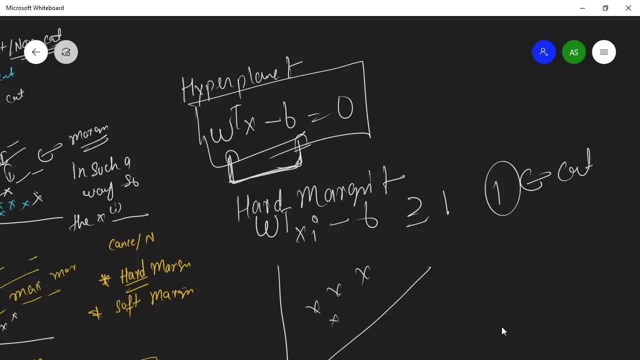 this straight line and you have this, and you have the data point and the one, these two parallel lines, and again here you have. so whatever on this margin or above, this margin is regarded as 1, means the positive attention, so it is regarded as a cap, as you, as you know, okay, and whatever. 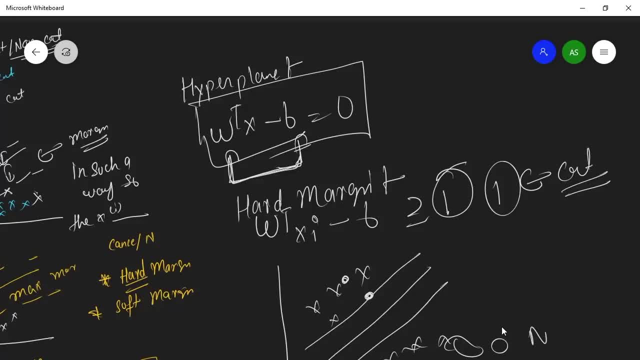 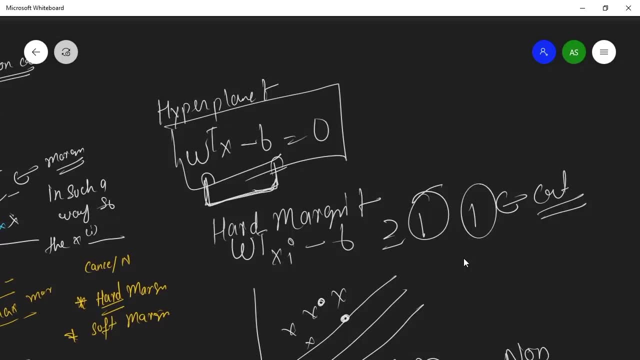 this is regarded as a 0, okay, as a non-cat, okay. so let's, let's, let's write the equation for that and it's quite easy, it's quite um and remember, rememberable. like W transpose X minus B, whatever on or beyond this margin. this: 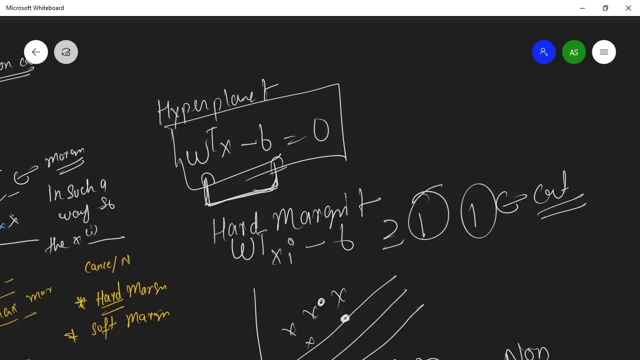 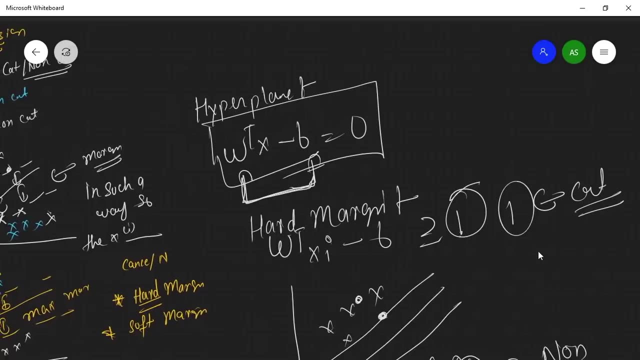 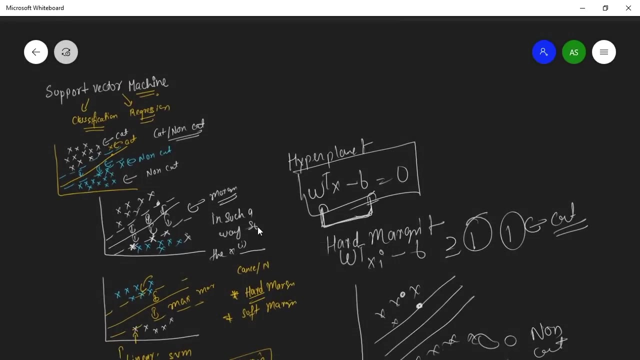 motion will be regarded as 1. whatever below this margin will be regarded as a 0. okay, as a negative attention. so that is the hot margin constraints and that's that. that's how we make predictions on support vector machine. okay, frame. pretty much clear what I'm trying to say. 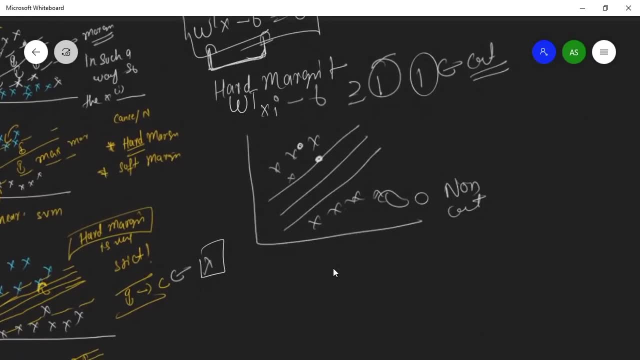 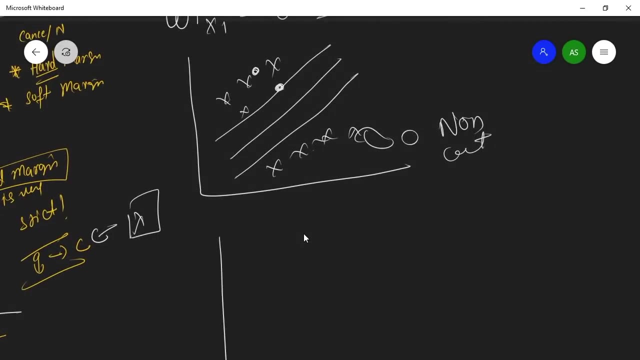 over here. okay, so now let's dig, dive into some little bit more further into math- is: how actually is it? it is being constructed like this. so let's say you have made a straight line and this, this margin you can see over here, this, these margin, is written by: this hyper plane is the main hyper plane is rated by W. 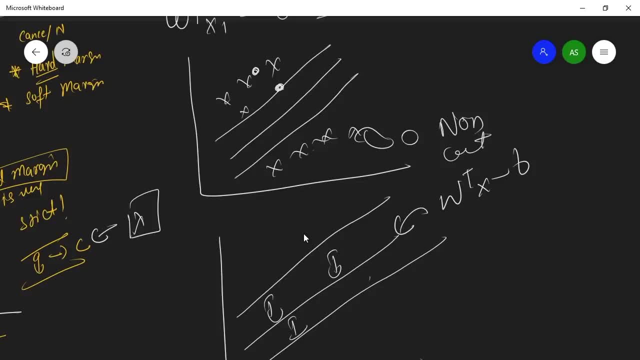 transpose X minus B and this margin is equals. this margin is equals the 2 over the norm of W. so to maximize this margin, we wanted to minimize this motion and minimize with W. okay, if you want to maximize this margin, because FZ, as we have always. 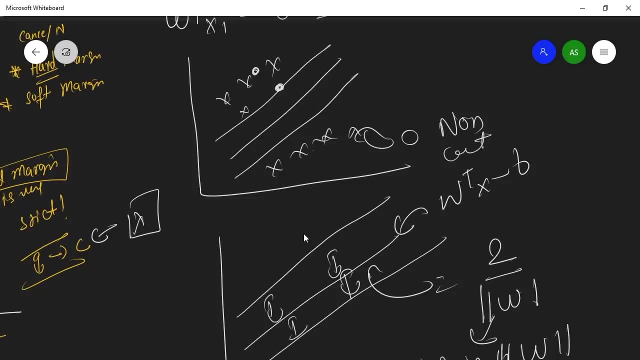 starts to maximize this margin. to maximize this margin, we have to minimize this norm of W and this margin is written by 2 over the norm of W. okay, and so, as you obtain that, as we always to maximize, so that set is written by the 2 over normal W and to maximize that, go to minimize the norm of W, so we can. 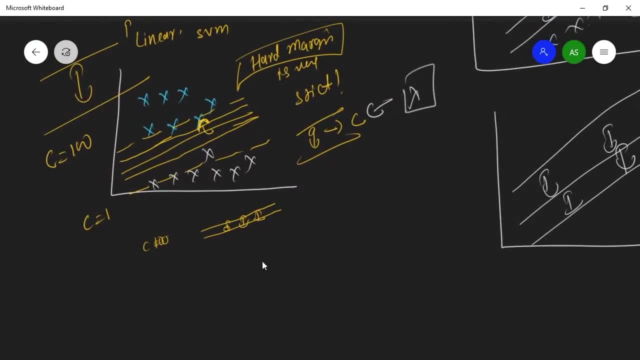 write an objective function, we can write of object a problem like like, like this: the distance between two hyperplane, the distance distance between two hyper plane to hyper plane, is written by 2 over the norm of W. so to maximize that margin we want to minimize the norm of w with: subject to subject to yi, w transpose xi minus b. 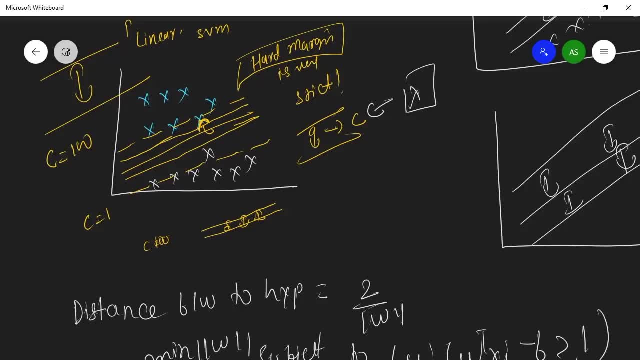 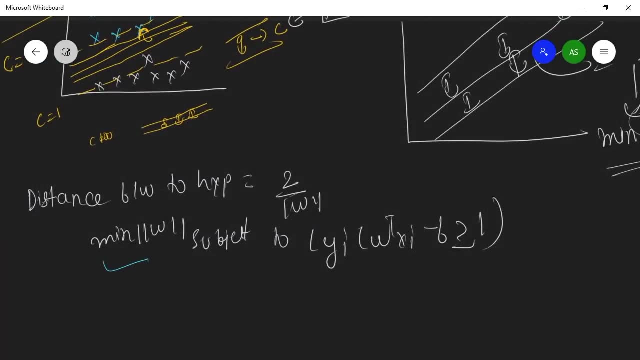 greater than or equals to 1. so what i have said, so let's understand this equation a little bit more further, what i have written over here. so for maxim, this is the minimizing means we want to minimize, to maximize that margin with respect to yi, which is your ground. truth means actual. 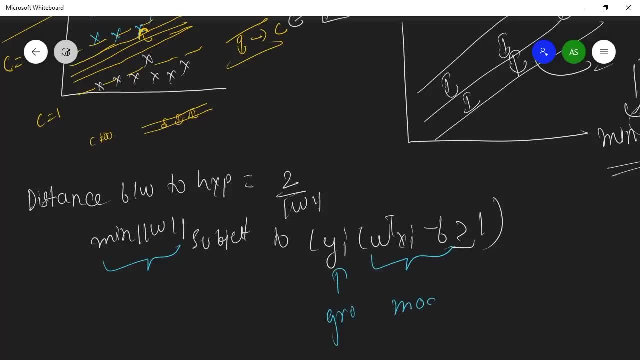 label and this is your moral predicted value, moral predicted value, and you can show here if it is on or beyond this. it will be one, otherwise it will be zero. so if yi is equals to your moral predicted value, then your cost function will be zero, then your loss function will be zero. otherwise, if it, 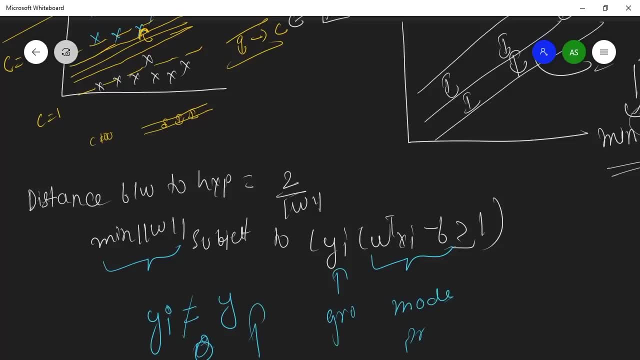 is not equals to y, then the new loss function will be very, very high. so you want to minimize this norm of w to get the good predictions. okay, so we have started this- and i really hope that you had understood the concept that i explained to you- and we can write our cost function in a hinge loss force. i'm talking about a soft margin, so 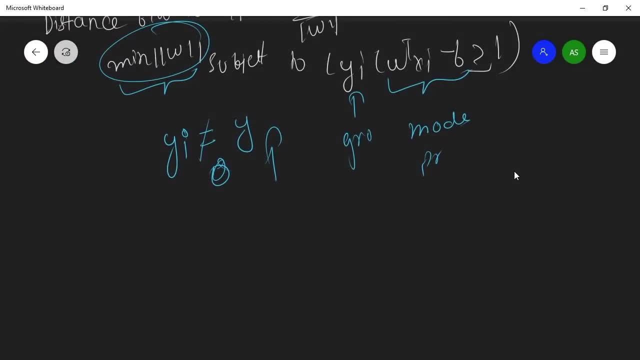 we can write our soft margin like this so we can write the loss function, the cost function, the loss function. you can write our loss function like this: 1 over n plus. I'm going to each and every training examples: max of 0,, 1 minus y, double transpose. 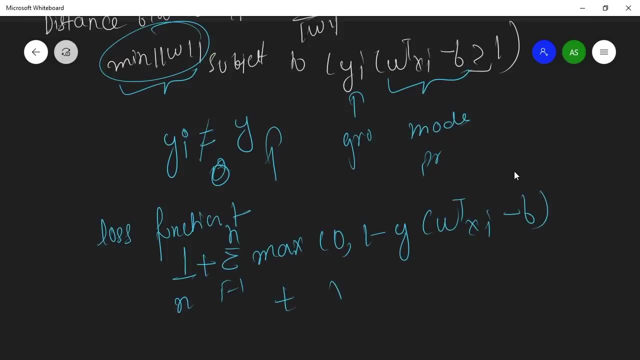 xi minus b, plus regularization, plus lambda, over times the norm of w squared. So this is quite confusing a little bit, but let me try to explain you in more detail So you can see we are going to each and every training example. but take note of: 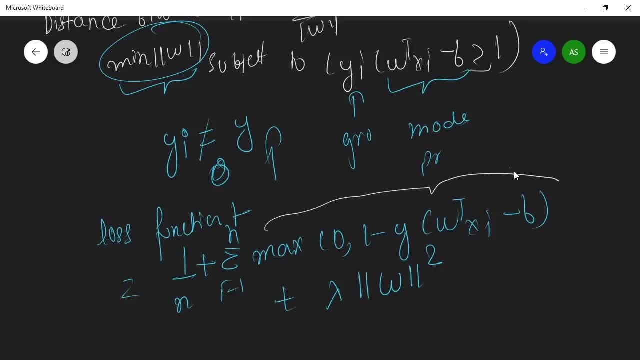 max and this is the hinge loss. if you can see, this is called the hinge loss. If you want to get into more detail about the hinge loss, you can have a look at some Wikipedia pages for knowing about hinge loss. And this is your model. 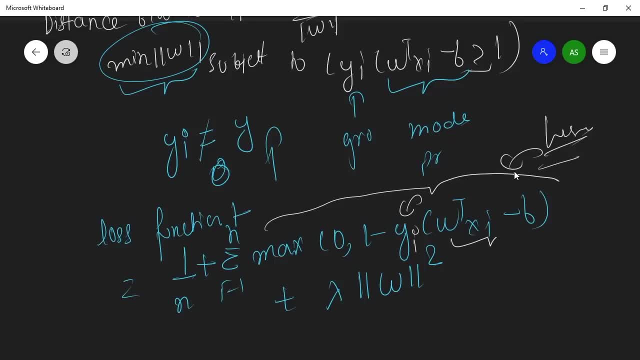 predicted value: yi, and this is your ground truth. yi and this is your model predicted value. and this is the lambda times. you can write it c also. you can write c also because it helps you to adjust the width of that margin. So that's. 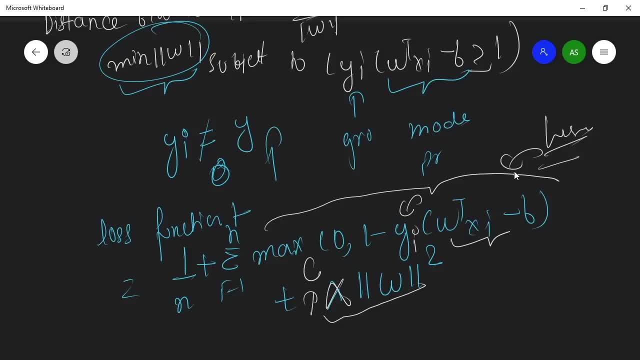 why it is a very, very important hyperparameter. okay, And times the norm of w squared okay, Okay, so we are done with a kind of a linear classifier. we are laying here SVM- it's linear classification, so we have made our good loss function. 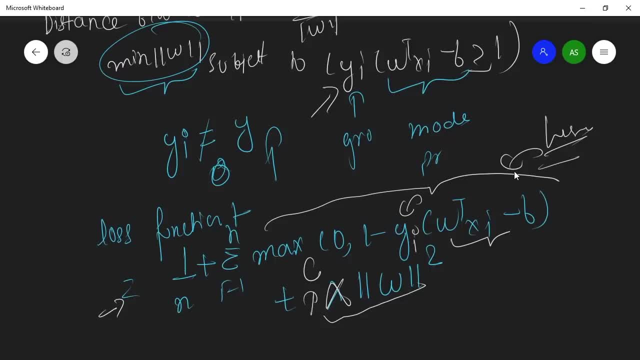 so we have made a prediction function and now it's okay, we want to minimize this norm of w to get the good predictions, okay. Okay, so we have seen only the linear SVM. so let me formulate one example, which is like this: 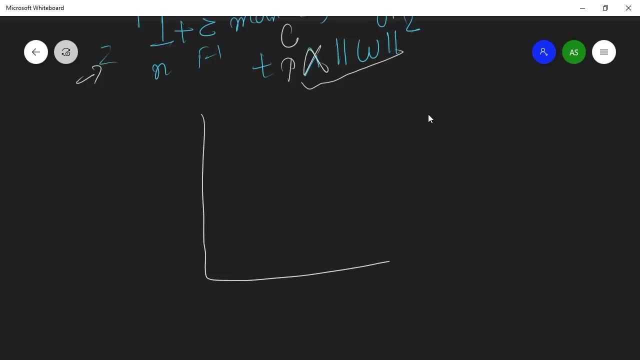 let me make one again: x and y plane. I'm making too much x and y plane. it's best to have this kind of thing, so let me make one non-linear classification like this: okay, So you have this kind of data and this kind of data and let me make 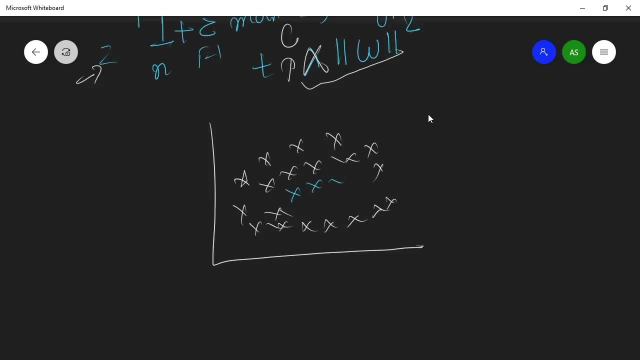 these white examples are cat images and these white examples are non-cat images. So now, if you can, if you want to make the straight line, you will be not able to do. that means you're not able to kind of classify it, so it's very bad. So what you? 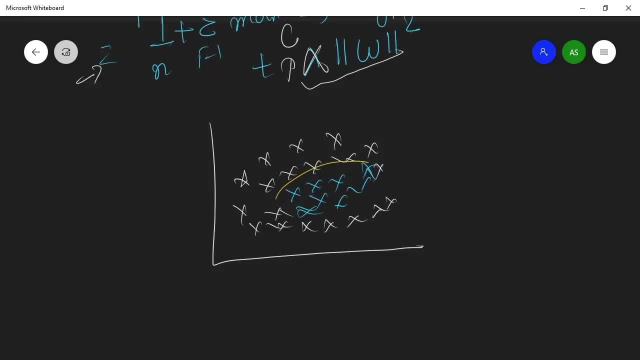 have to do. you have to make a non-linear, you have to do the non-linear classification like this: Now it will be okay, Now it will be okay. so SVM also is also is very kind of powerful in non-linear classification with something called as kernel trick, something called as kernel. 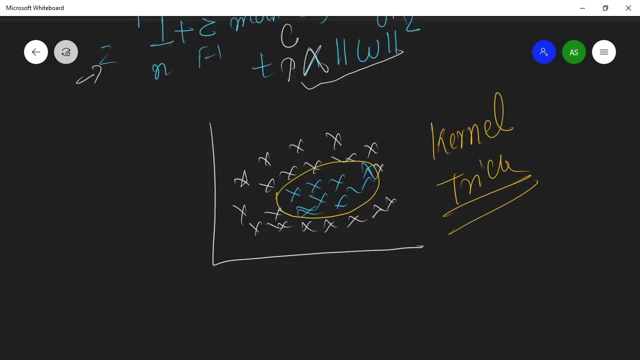 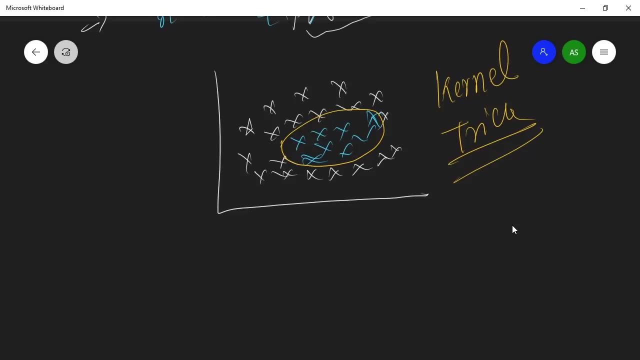 trick. So we will elaborate kernel trick in detail. so let's start with kernel trick. So what? what we do in kernel trick? so let me write an algorithm. so what you do? you write an algorithm in terms of x. you write the inner product. 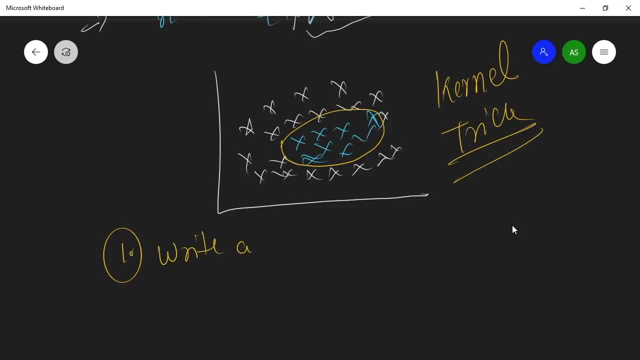 let's say, let me write, you write an algorithm. you write an algorithm in terms of the inner product of x and z and the these x and z are two data points, are two data points. So what you do? let let me tell you what. 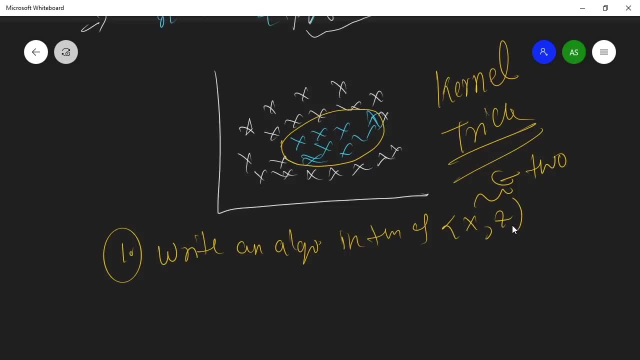 what? what we do in non-linear classification? We take our data, we take our data x and we transform our data to some more. let's say, we have one-dimensional data to a two-dimensional data in non-linear classification. Okay, so we transform our data to from one-dimensional to two-dimensional, like. 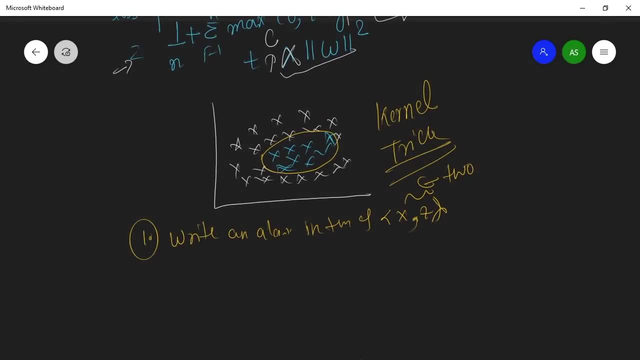 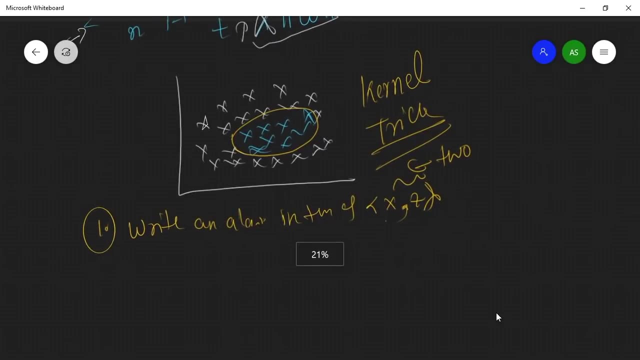 like this. okay, so we write an algorithm in the form of x and z, and x and z are the data points. So in simply in kernel trick, we transform our data to from one-dimensional to higher dimensional space. So you will get to know what what 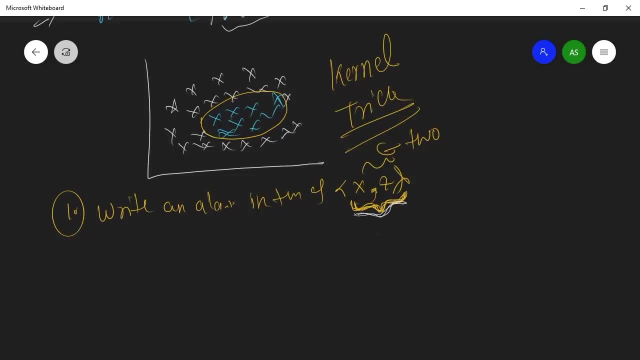 we are doing. So let's let let me write these steps. So, after we have written our algorithm in terms of the inner product of x and z, now what? what we do? we map our input input in this X without I write. we map our input X to the Phi of X. 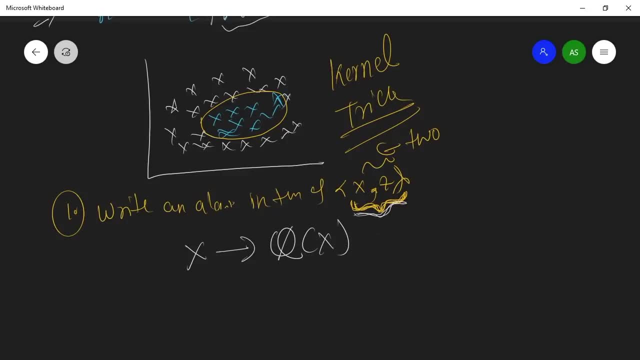 okay to the Phi of X. so we are. just, I will tell you what this function is, because, okay, so we write our function V, that we map our X to the Phi of X. I will tell you what, what we do in this case. so we we find a way to map our this, we find 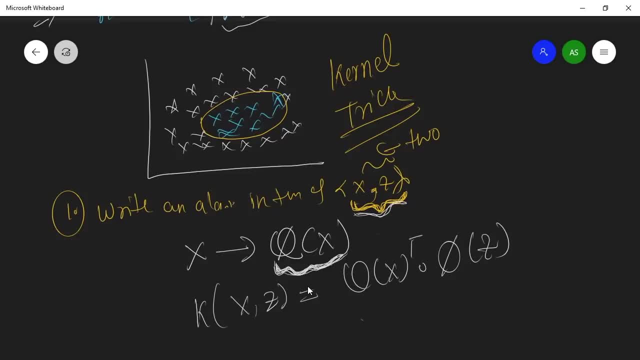 if we find a function, so we map our X to the Phi of X, so we write a function or you find a way. you find a way so we find the X to be some Phi of X and it will transform your one-dimensional data to the maybe and in any kind of your. 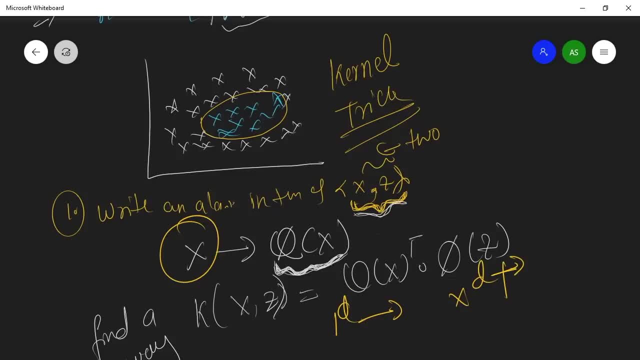 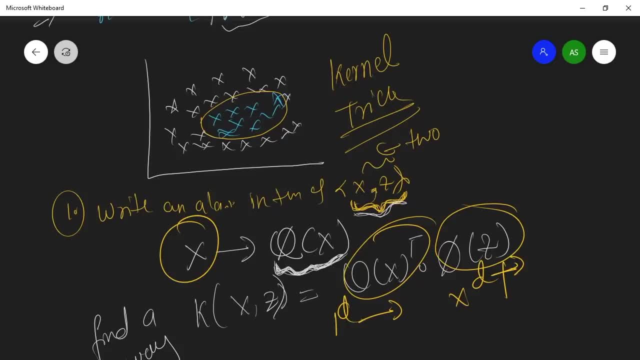 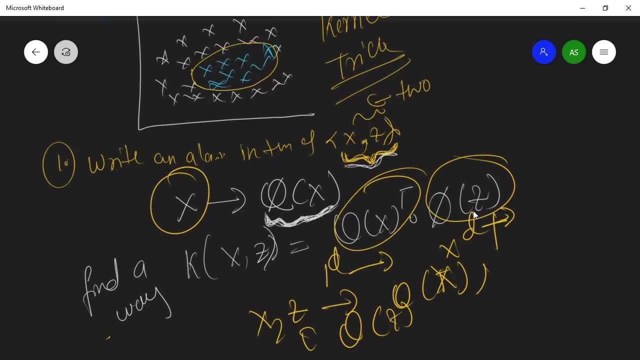 what is does with that help an example. and then what we do. we replace our X and Z with our transform data, which is Phi of X and Z, to be the be the Phi of Z. okay, so this is what we do. so let's see some how what is does and and what. 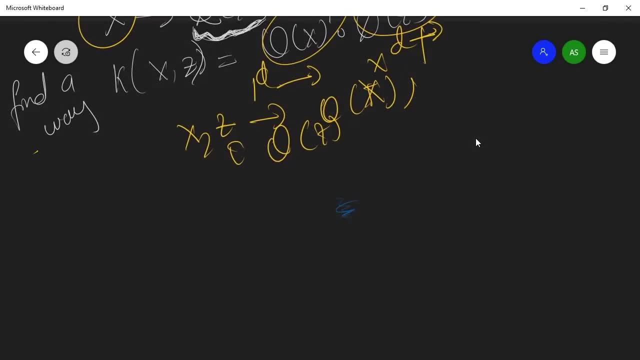 face. so we write the kernel functions are one of the famous kernel is our RB of kernel that will transform your data, x and z, to the high dimensional space. so the kernel function is written by the RB of kernel function. written by k of x, comma z, exponent of minus. 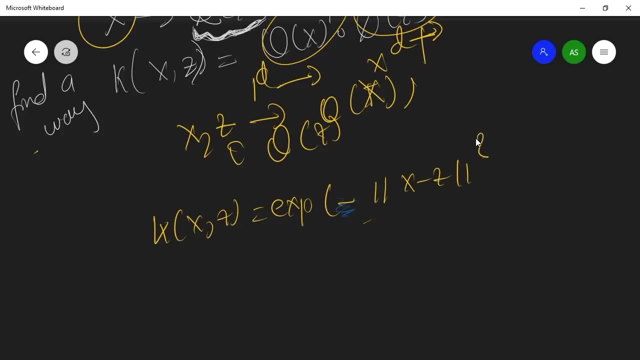 norm of x minus z, squared over 2 over the sigma, squared okay, and the x and z are the data points. okay, great. and some more kernels are, which is polynomial, homogeneous, polynomial, inhomogeneous, which you can search on internet, but the most famous one is RB of kernel which is widely used. 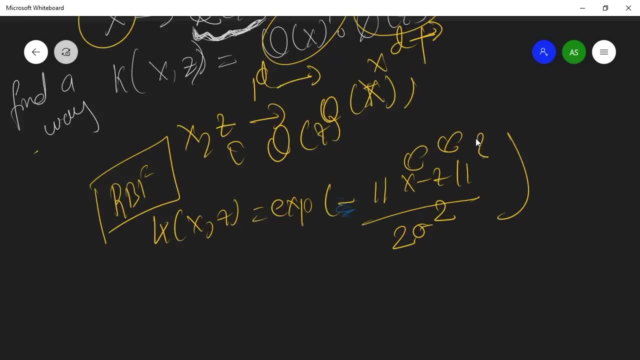 in the industry, okay, okay. so we have seen now various kind of things and about kernel trick, how we do the non-linear, the transformer data. you are able to do the non-linear classification. so here are some. we will discuss one, two kind of one parameter problem which will help us to state. 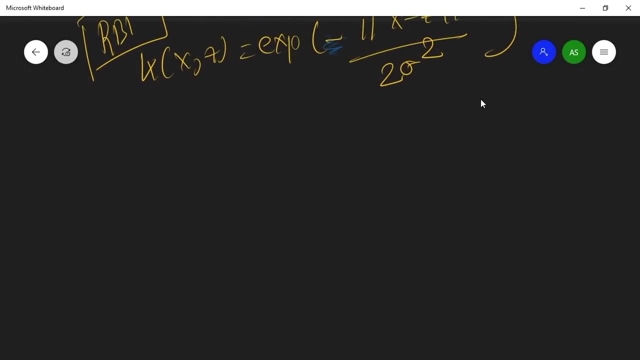 our optimization objective and then we will see the sub gradient. okay, so why? I am talking about primer problem? it will help you to formalize your objective function. so it will help you to formalize your objective function. so it's just the same, just as written. we write that. 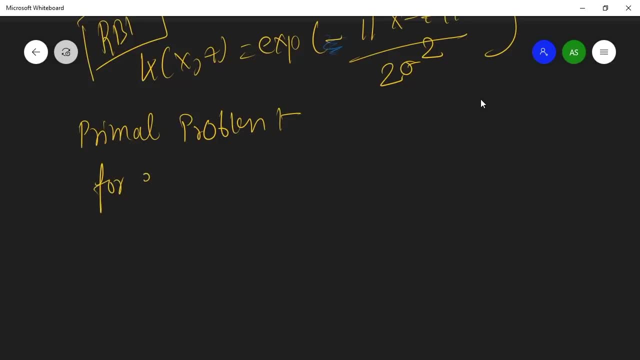 so for each i, for each i be the member of 1, 2, all the way around to the end. we introduce a new variable Zeta. we introduce a new variable Zeta where Zeta I, where is equals to the max of 0 comma 1 minus Y I. so we reduce a new variable Zeta I 0 comma 1 minus Y I. 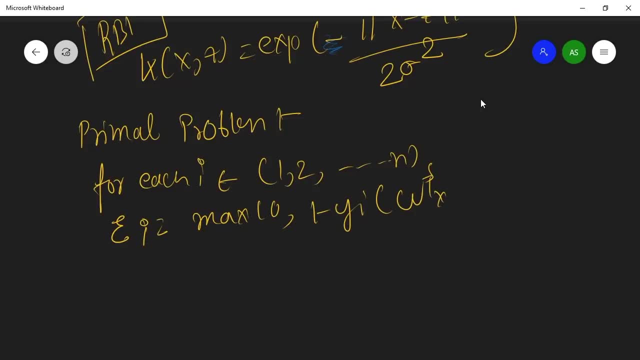 okay, and then in that we write W transpose X minus B. okay, so this is just a hinge loss where we introduced a new variable that range losses is storing. okay, try the images, see what I'm trying to see you here. okay, so then we write our function like this: we want to minimize, you want to minimize 1 over N. I. 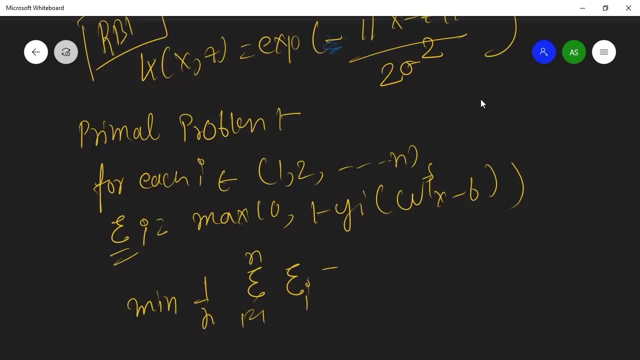 equals to 1, all the variety n Zeta I plus the regularization term. see the norm of w squared. okay, with respect to or subject to, subject to to yi w transpose x minus b greater than or equal to 1 minus the zeta i. time is just where. 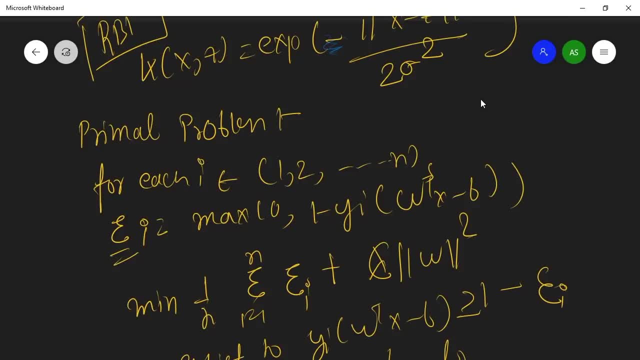 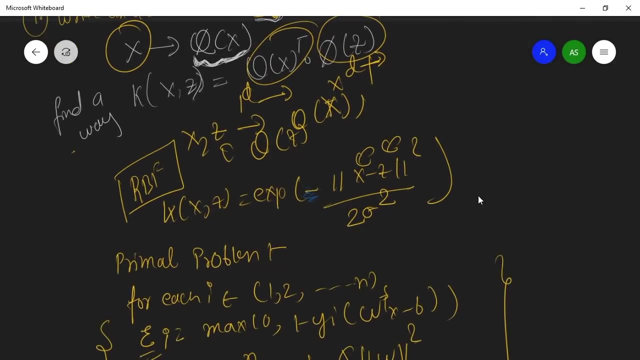 zeta i is greater than or equal to b for all i. okay, so we have just formulated one problem. it is just equal to the hinge cross that we have seen we want to minimize. the objective function that we have seen so far is just equal to that. so we have formulated in such a way that you can. 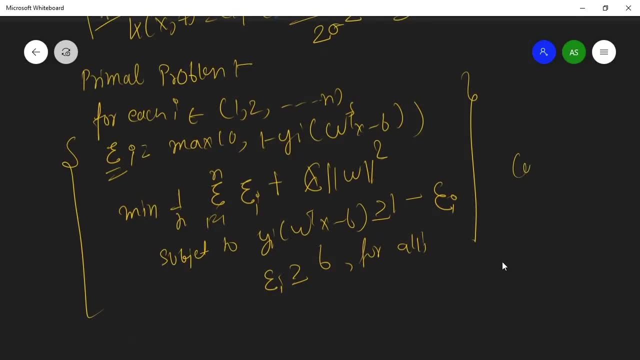 use this. okay, so we have an objective function which is our cross function. now we can now some something called a sub gradient, something called as sub gradient descent, and which what? what we do we? we make a convex function f of w and b. we take out the sub gradient of our, of our function. we 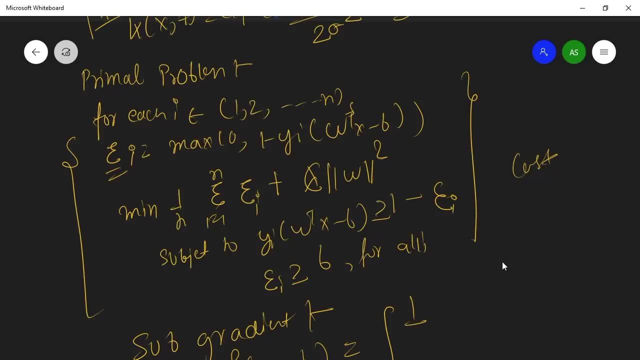 take out the sub gradient of our cross function and then we update our parameter w and b. okay, and that's the sub as the gradient descent what what we are doing? okay, so it's little bit different than gradient descent. here we are taking the sub gradient of our cross. 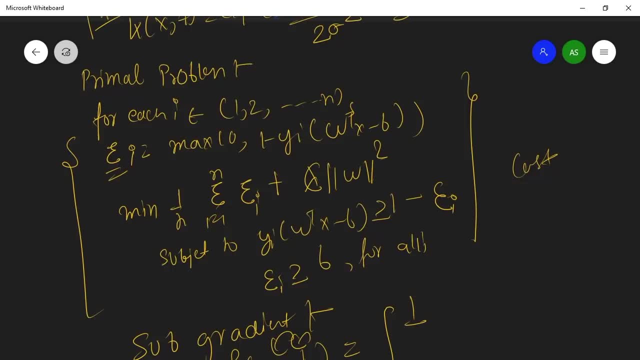 function okay. so this is what we are doing. this is called the primal problem, and then we, with this, we we take out the sub gradient of that primal problem. okay, pretty much is what i'm trying to say over here. okay, so one more thing that the that is very popular among beginners, or learning theory. 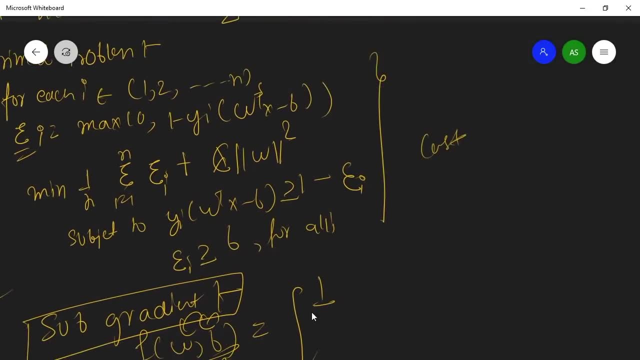 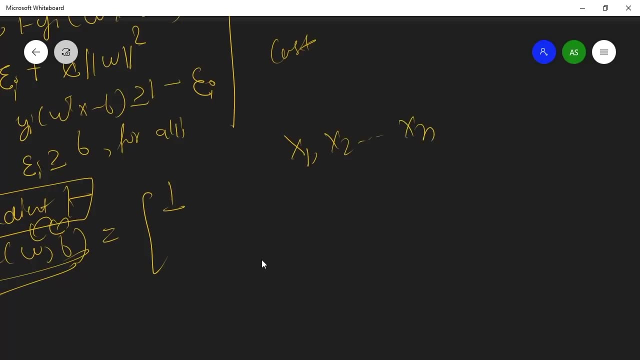 something more or less empirical risk minimization. what do you mean by empirical risk minimization? okay, so, person you are, whatever you have, personal information i can give you. i don't know whether it's your first time either or not. well, but it's okay to give it a first, your will, but apply it. 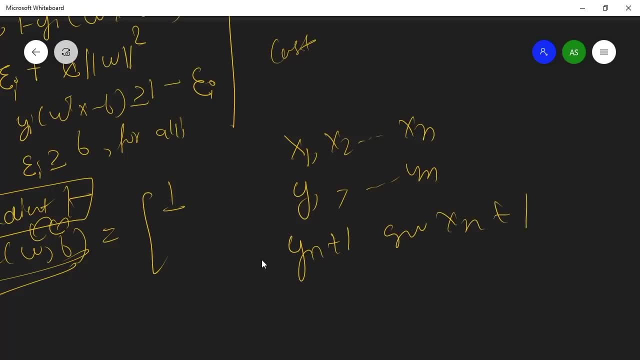 alright, so i just remove it usually, so that way you don't give it a second and in some cases you could some other use it, but it's okay, because it's eating. how to explain to people some of their aqueles with an accuracy level and projet a a goal used as they just utilize this exercise now. 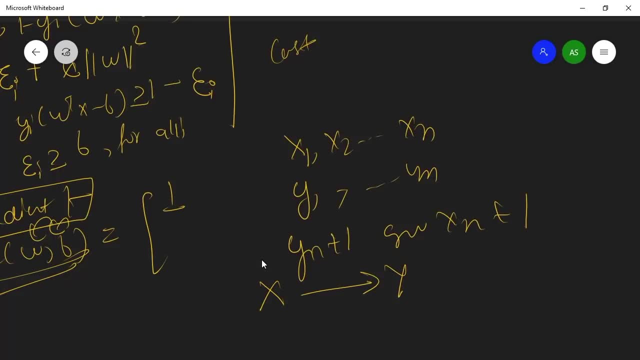 they put- i just leave that out- when they include all of this right here. then back into the next area, minimize. So that's the empirical risk minimization which we have already seen. So we just have to know the definition for it. What is S? 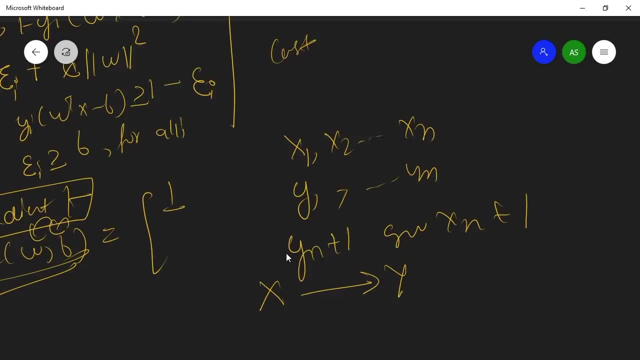 Okay. so, as we have talked about non-linear and linear, now it's time for getting into the support vector regression. I'm just going to give you the equations. It is kind of quite easy. You want to minimize your 1 over 2, the norm of W squared. 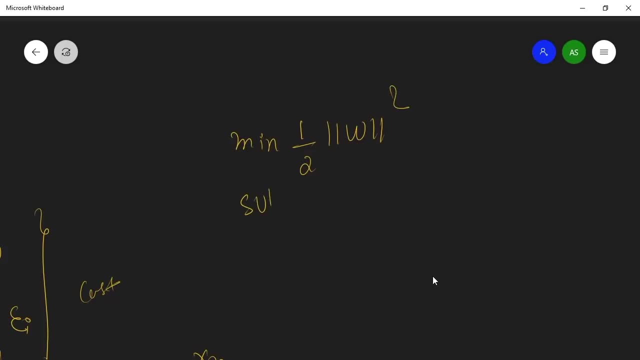 You want to minimize this, to get your output with respect to or subject to the YI, the absolute value of YI minus the inner product of W and XI and P times B, and it should be greater than or equal to the sum epsilon, and epsilon be the smallest. 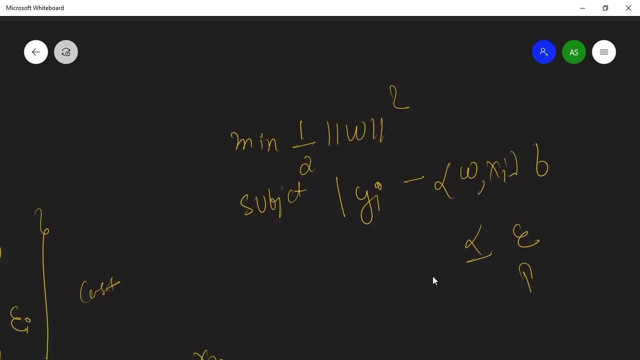 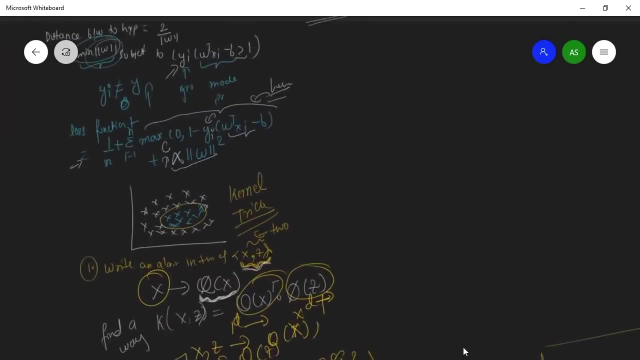 positive integer, So just to be comfortable with that. So I hope that is quite clear and this is for regression task And we will see them implementation in our next section. So I hope that you really enjoyed this tutorial, this section, and we will be carrying out this. 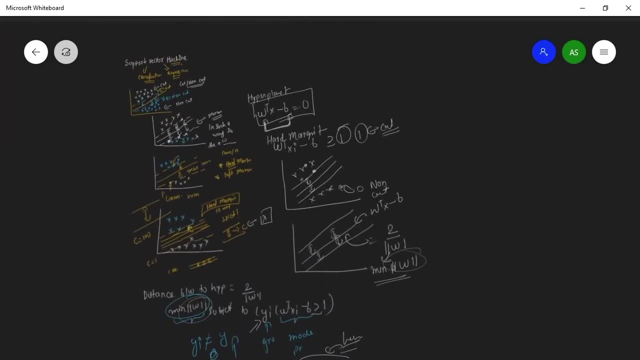 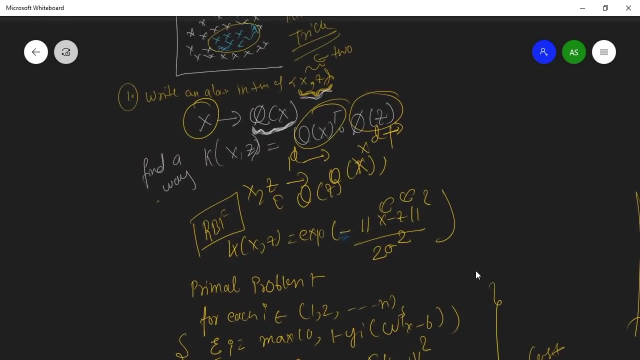 more into detail Now. we have gone too much into math. but if you haven't understood any one, please feel free to put your comment in the comment box. I'll be very, very happy to take your comment and provide you answers over there. I will be taking a look at your questions and we will. 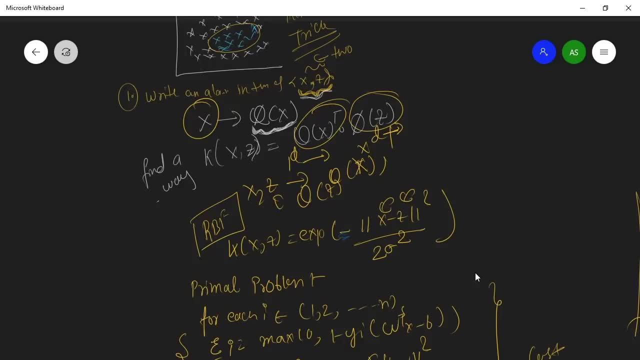 be answering soon. at that point, Just put the time stamp, Okay, So that I could know where you have a problem. Okay, so I think that we have gone in too much detail. If you haven't understood primal problems or gradient, don't worry, It is not required for beginner machine learning. 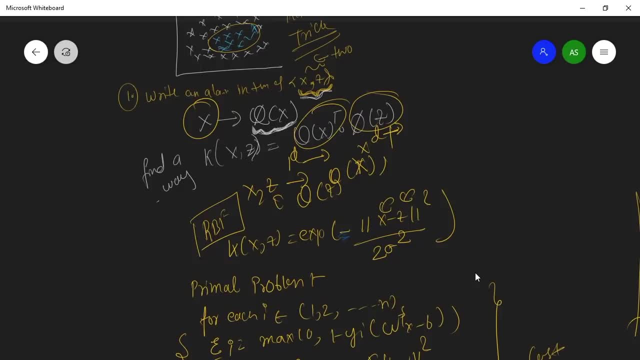 So if you have, if you, if you learn too much in machine learning and gone into deep learning, now you can come back to this primal problem to understand what I'm saying. But it's quite easy to understand, and the kernel trick, what I've said, etc. 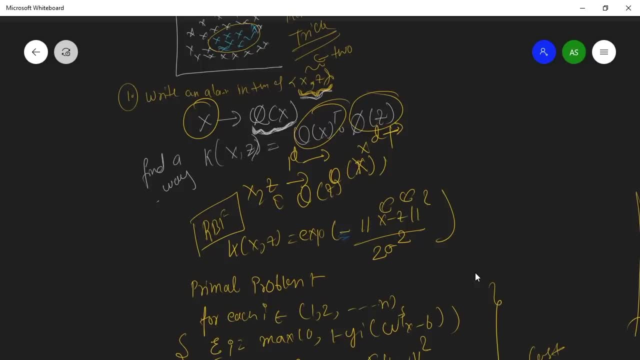 Okay, so thank you for seeing this video. Sorry, thank you for seeing this section. I'll be catching up your next section. Till then, you can do the program assignment. Okay, I'll be catching up your next section. We'll be making one project, which is stock price predictor. 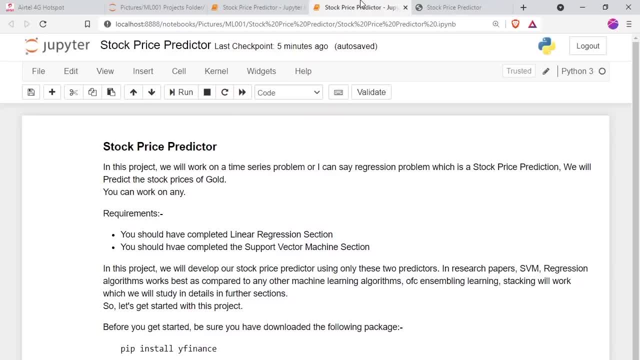 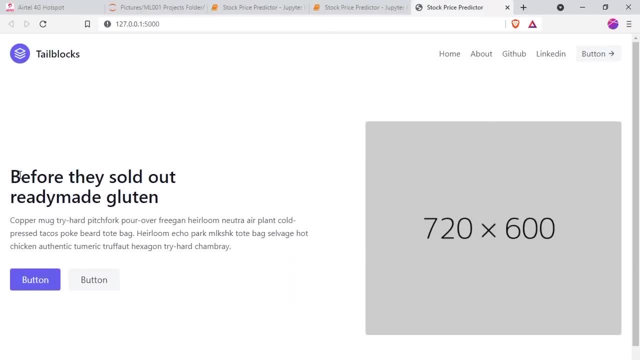 Okay, thank you. So now we will make a stock price predictor, which is our end-to-end machine learning project, And here's a demo and you can see over here that I have to use. You can just remove the tag. I will show you where I have taken all those things. 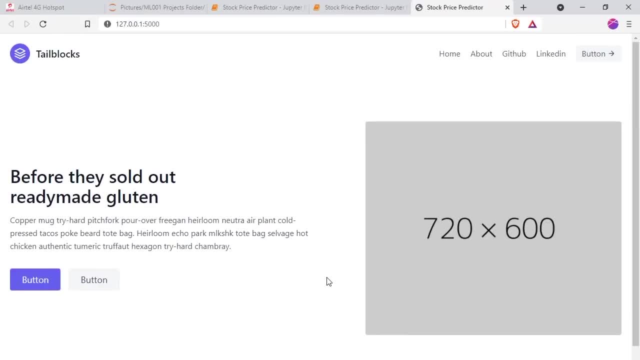 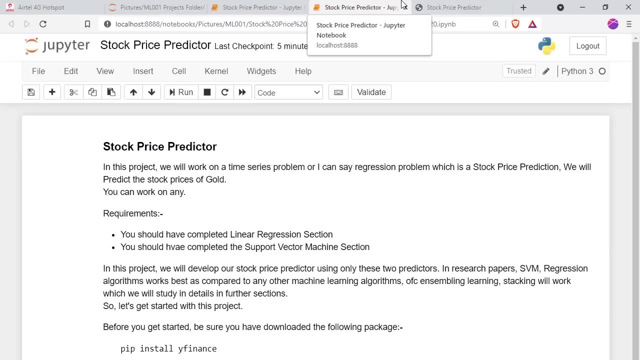 Just I do. I'm not a web developer, but I had made a good front end of this and also I made a back end using flask. Okay, so we will code, As I made a stock price predictor, and I will show you how you can build the same website, like me. 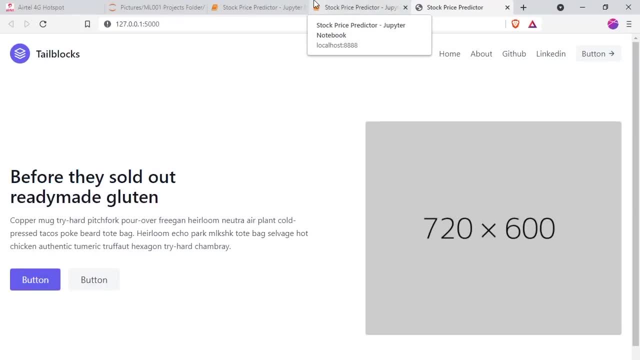 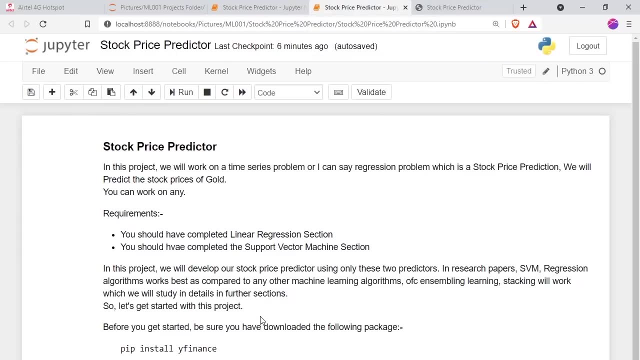 And you can also make a beautify if you're a web developer. Okay, so here is my, here's my Jupiter notebook, And here, first of all, I'm going to download the data from Yahoo Finance and you can simply pep install my finance. 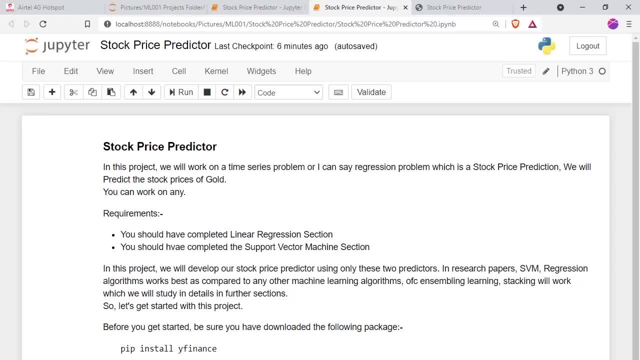 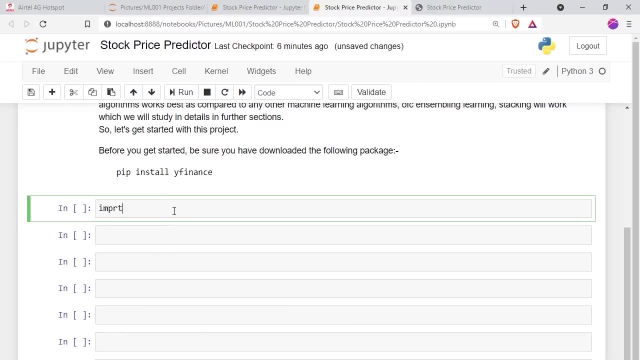 I've already installed that. you can install that. So you just want to import first of all the basic libraries. Let me do that. So first of all, you want to import the basic libraries like this: First of all, I will import numpy as NP. 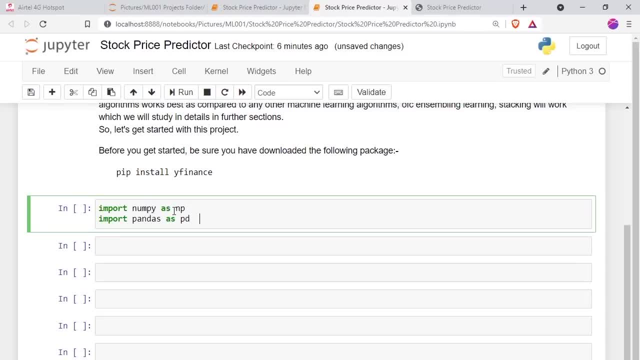 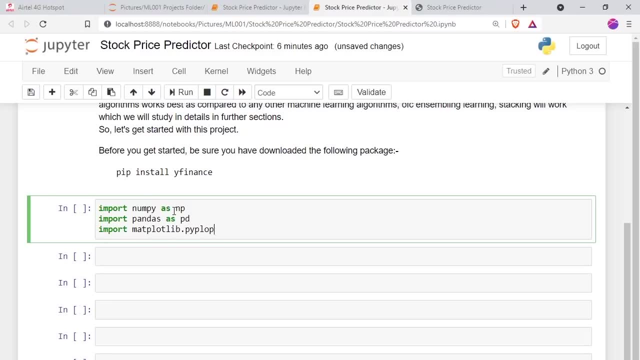 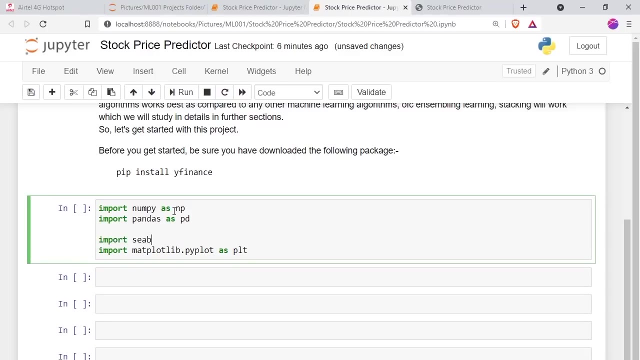 Then I will import pandas as PV, And then I will import matplotlib and import matplotlibpyplot as PLT. Then with that I'm going to import the Seaborn, because I'm going to use Seaborn now in this case as a visualization library. 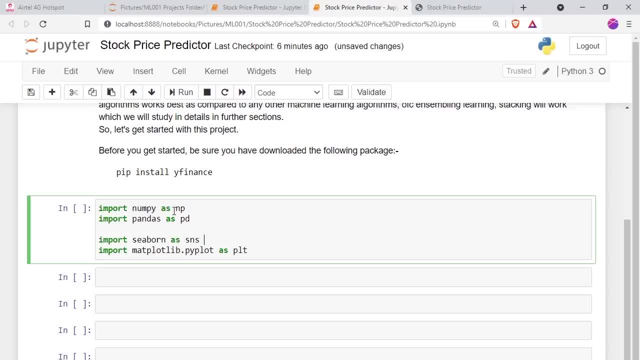 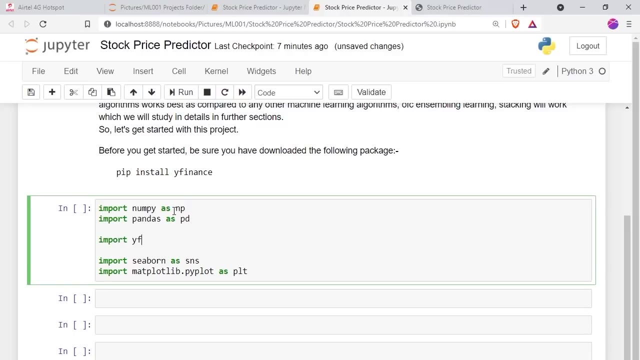 So numpy is a scientific library, Pandas is working with the data, The Seaborn is a visualization library and matplotlib is also a visualization library. Okay, And one more thing that I want to import is for my data, for my data, which is import Y Finance as YF. 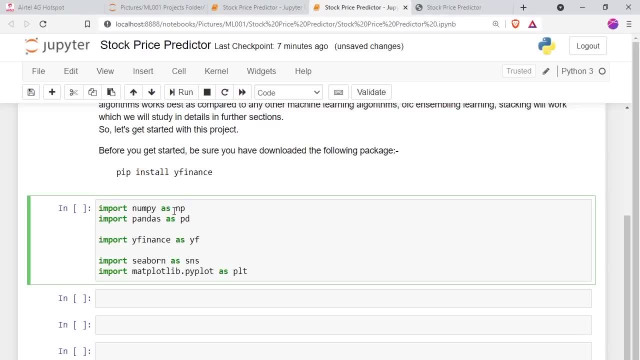 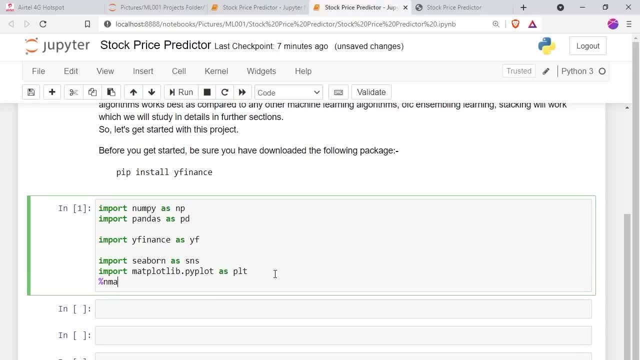 Okay, as YF- and YF is just Li, It's given to that. Okay, let me run this out and yeah, I can to add: this is optional what I can to add over here like this: matplotlibonline- matplotlibonline. Okay. 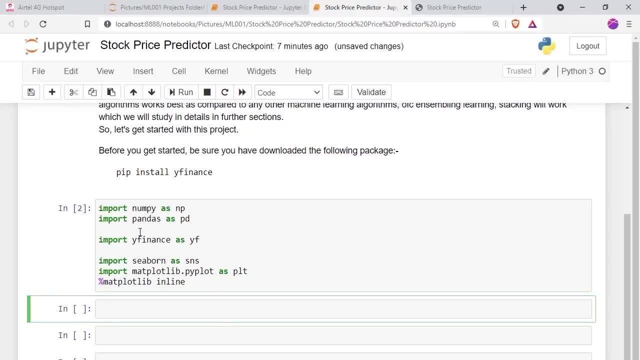 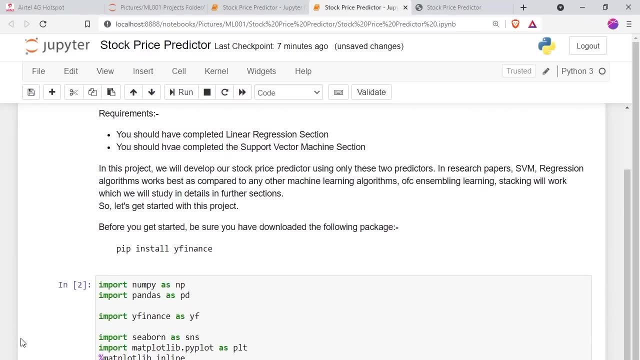 Now it should work fine. Okay, So we had done with importation of our all the libraries and now it's time for getting it a little bit more detail about the data, how we can load our data. So first of all, I'm just going to use 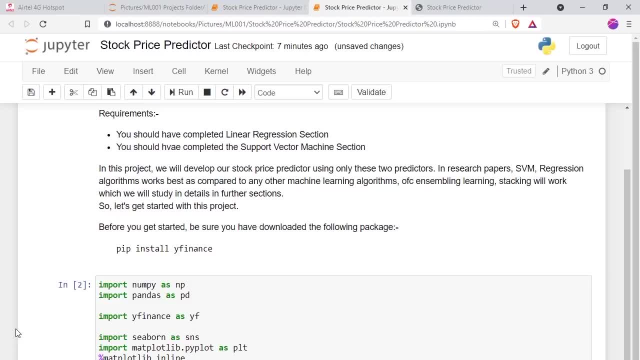 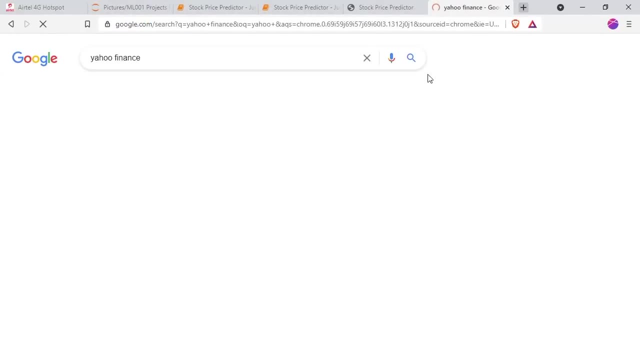 i just want to. i'm in this project. i will make a stock price predictor of natural gas, okay, and you can do any of like gold, silver. just go head over to the yahoo finance, just head over to the yahoo finance and just head over to that and just to search whatever. let's say i want to go for gold. 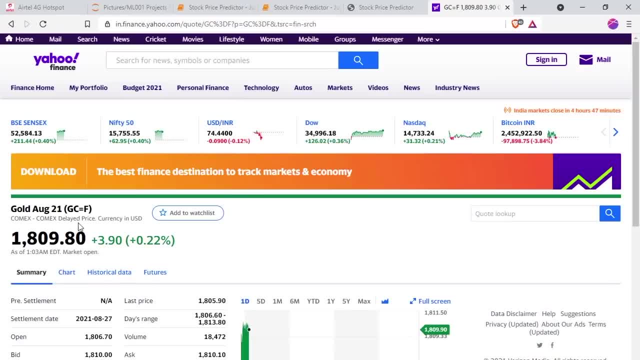 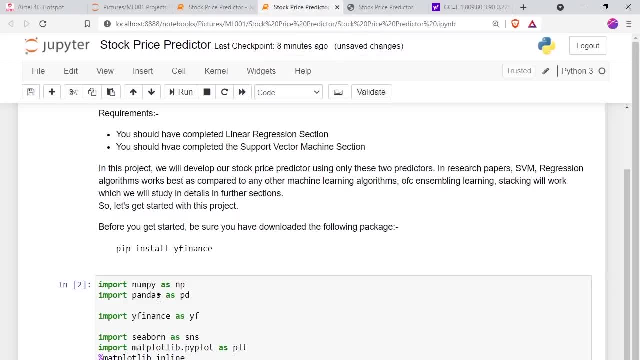 so if you go over gold, then you will see over here that you have a gc equals to f, which is the code of that. okay, so you just take, take, copy the code, and here's just all. i will just show you how, what you can do. first of all, i will take input. i will take input which is: enter the code of the stock. 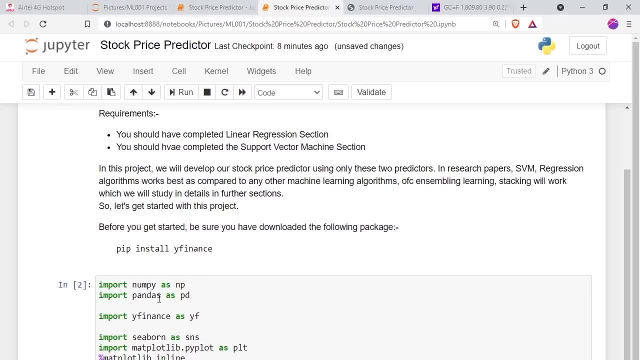 enter the code of the stock to download. enter the code of the stock to download. okay, now it will take an input. now i will just uh, make a variable. now i'll just make a variable: yfdownload, and it will take off the code from the stock. 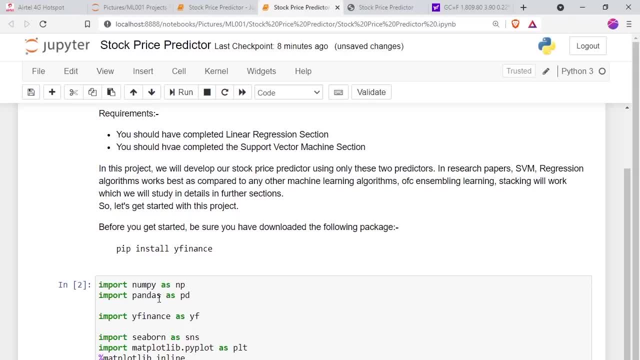 box, okay, and it will download from uh. it will download from, let's say, 2008. it will download from 2008, uh, in january- to one till uh. it will down it download till two, two, two, zero, two, one till uh, zero, let's say, let's say two, let's say one and tell 18.. okay, so this is the favorite. 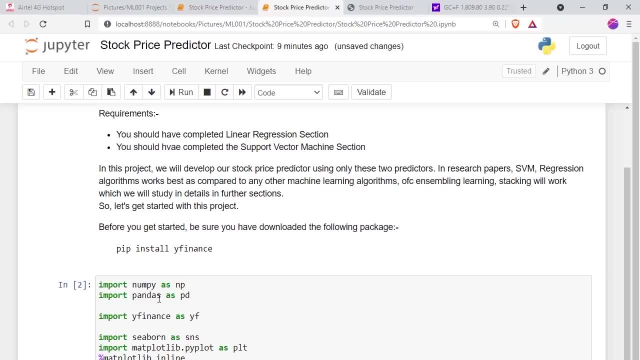 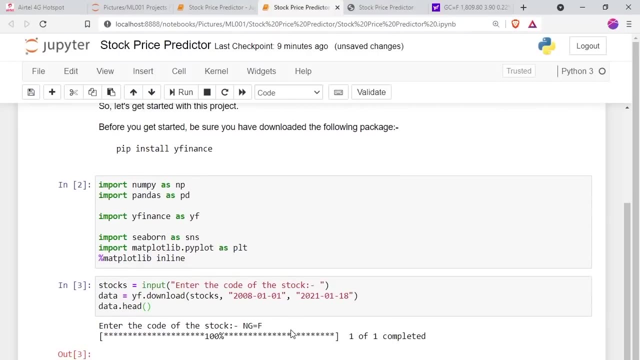 thing. and now what you can do. we can simply do this kind of thing and let me run this and let's ask the code of the stock. okay, so you just give the code of the stock. so let me give the natural gas equals to f. this is the code. so it will download a stock like this and then it will simply tell you the data. 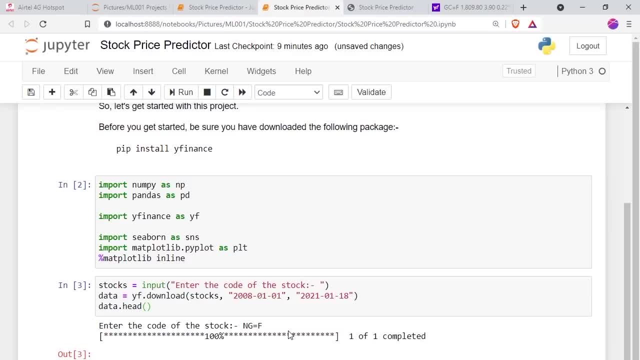 how it looks. okay now, if you can see, see over here that you have open, high, low, close, adjacent close and volume. okay, so one more and one more thing that you just that you can do. you can write auto adjust or to adjust equals to true. what is just is to adjust your uh, all of. 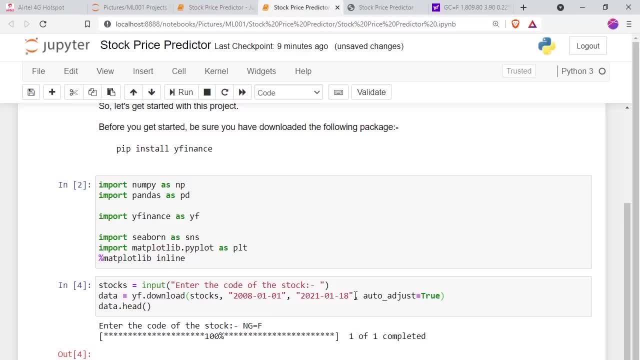 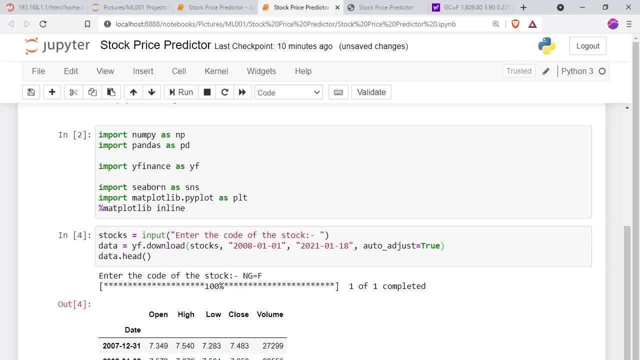 the kind of for day data frame and then you can see over here like this: okay, so that's what it's doing till now. okay, so we are done with this. now it's time for getting into a little bit more detail about uh. now we have loaded the data. now let's take a look at the shape of the data, like that: 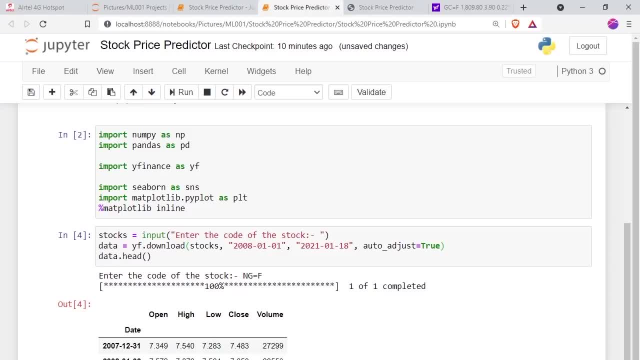 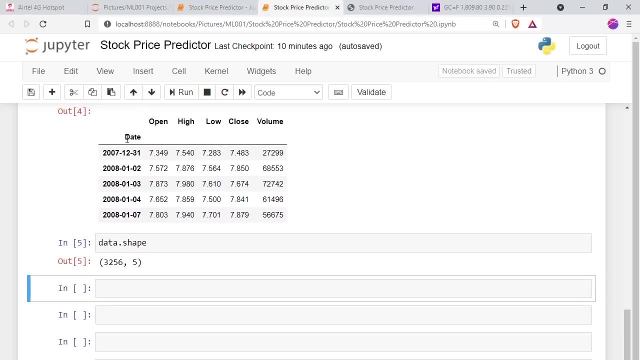 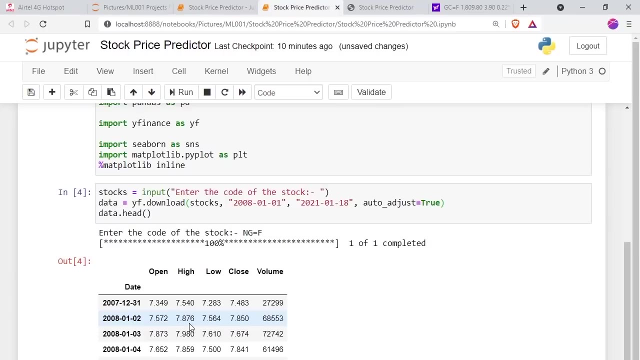 so data dot shape and to tell us that we have a total of 3256 uh training examples and five columns including date one, two, three, four. uh three, two, four, five. we have five columns and information about the data. you can take a look. we have a non-null values. we have this, we have that. what's the data type? 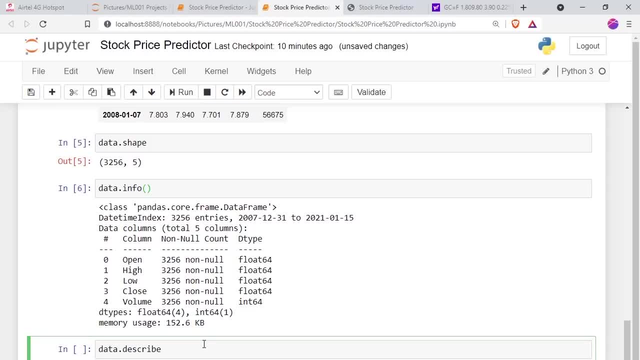 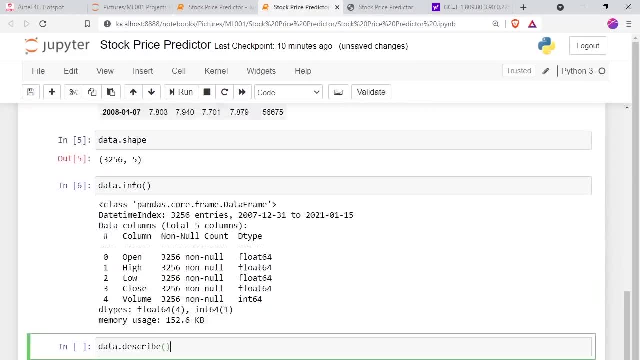 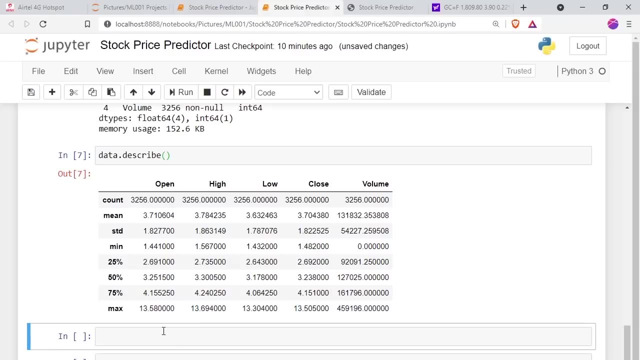 you can also take a look at the mean standard deviation, maximum, minimum of all the stuff. so let me do that, okay, so you just uh see this and now you can see that you have a all of the count, uh, the minimum, mean standard deviation minimum, 20, 25 and etc. okay, now, if you wanted to take a look at the 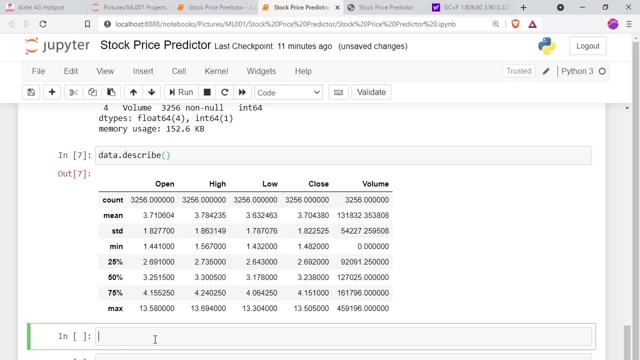 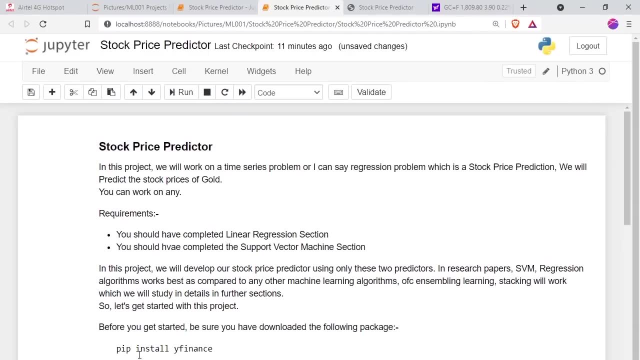 now we are done with data exploration. now let's let it go further into how it. uh, because stock price prediction is very, very non-linear. okay, but one thing that i want to mention over here: they do not use it for personal purposes. this is only for educational purposes. 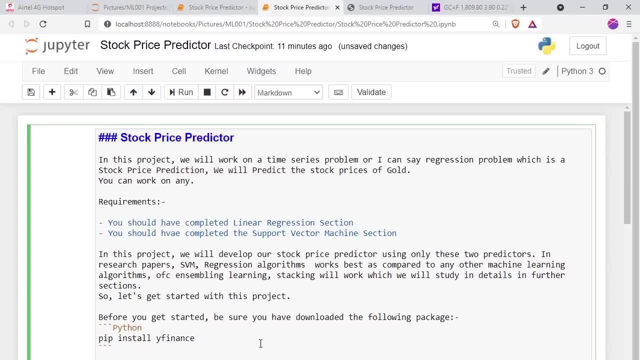 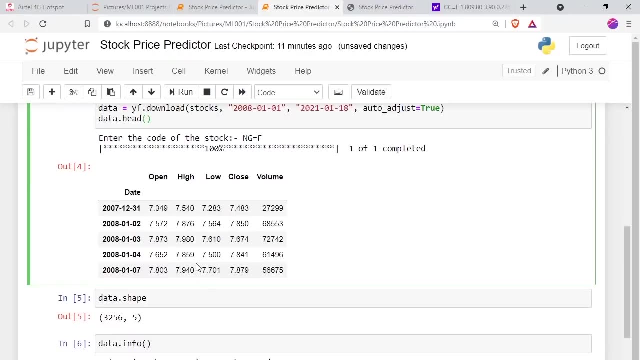 okay, only for, uh, educational purposes. the reason why it's very non-linear and you can't uh, and then you and you can't depend on your algorithm to to simply predict the output. okay, it may give you, uh, the wrong output, i don't know about this- very, very non-linear, so 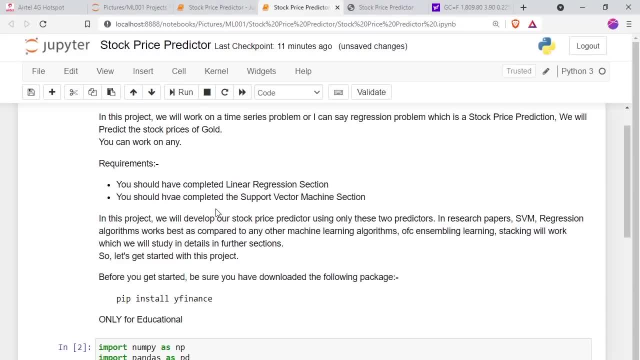 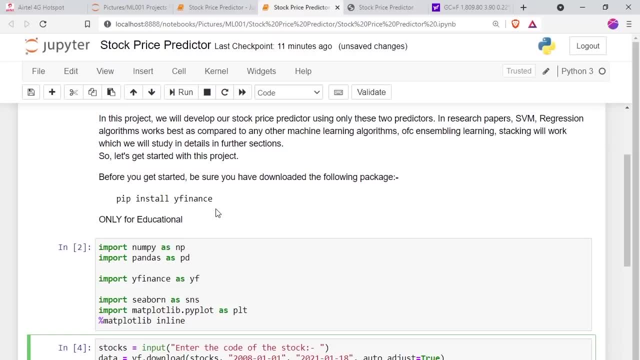 be sure to not use it just for educational purposes, not working company. you're just making a simple project so that you could get a concept of how you implement, how the whole looks like. okay, so don't implement by yourself, um kind of, uh, use one in yourself and 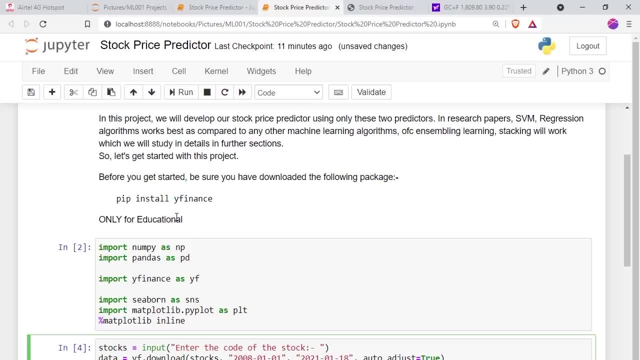 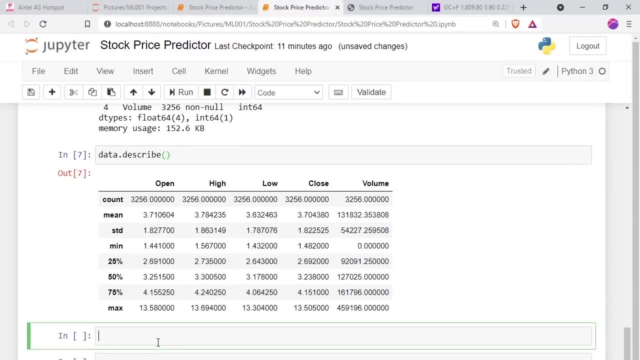 do not kind of, uh, make a website like that, do not. it is only for educational purposes. okay, now, if you're done with this, now we can analyze our data. now, if you want to and analyze our data, you can write this close dot plot. you can just plot it out. 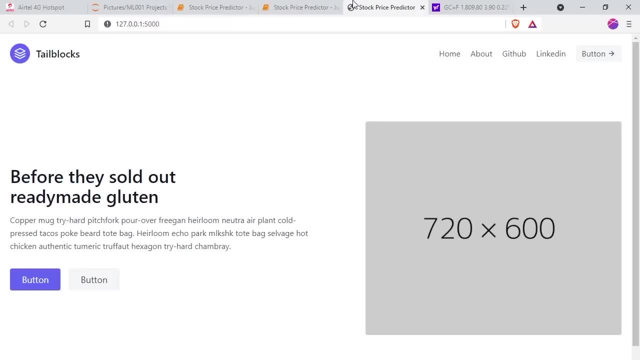 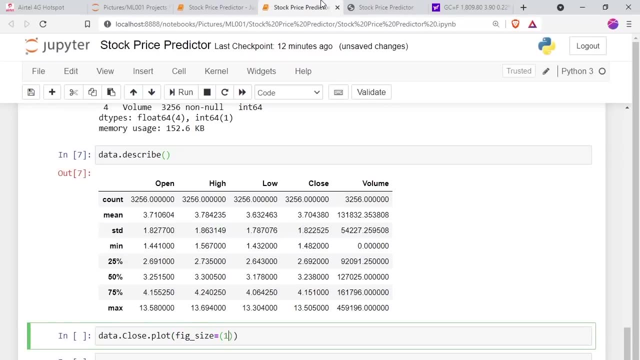 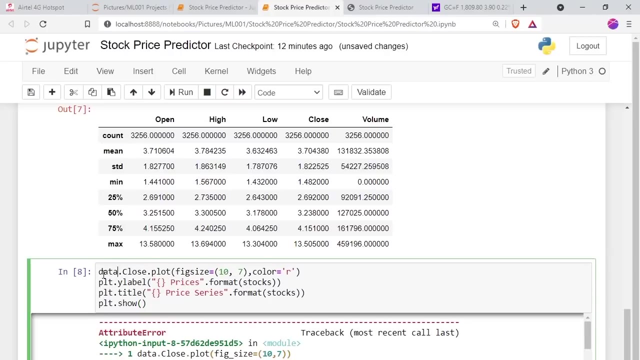 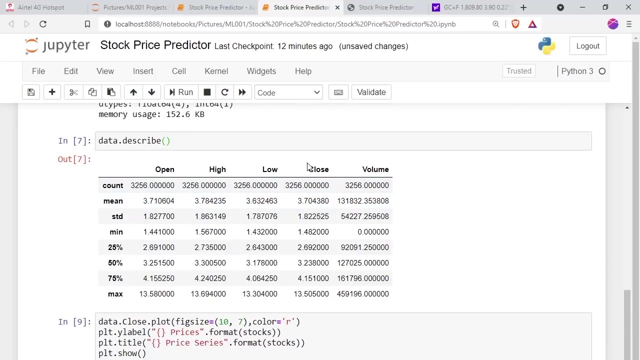 and now it will look like this: oops, you can fix size. let's say, i'm just going to make it 10, 7, and we have this. and here our target variable is close. okay, our target variable is closed, and uh, means we? it will just tell you the direction of the stock. let's say: 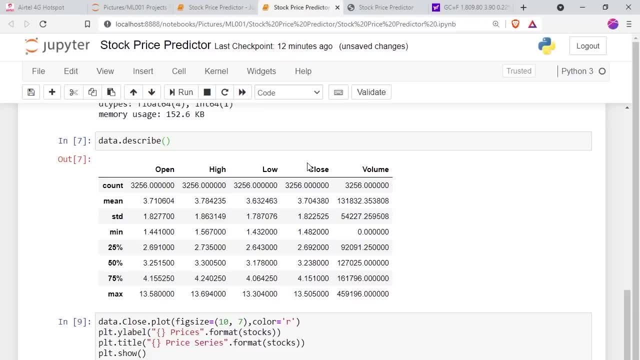 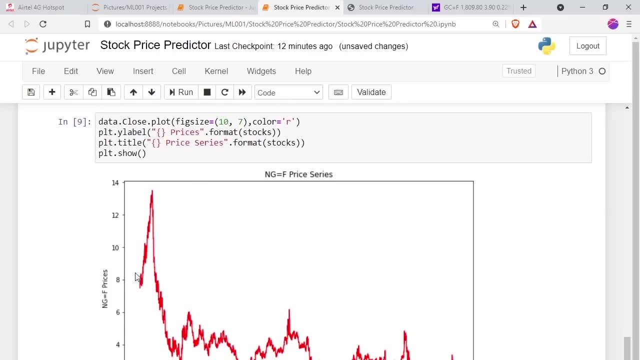 if the close is very high, then your direction of a stock is very high means it will the close will very hard. so here's very non-linear. so it just starts in 2008 in very low way and up up in 2009, then gone drastically down in 2010 and then kind of that. so you can see the 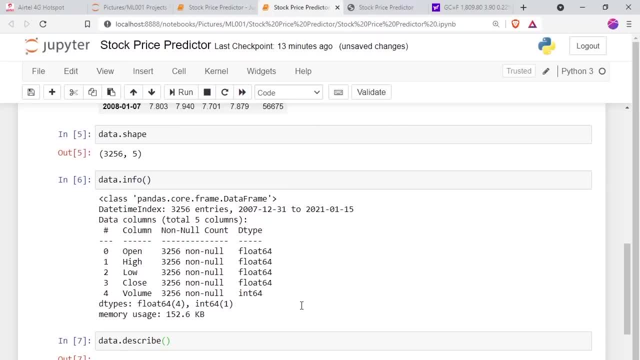 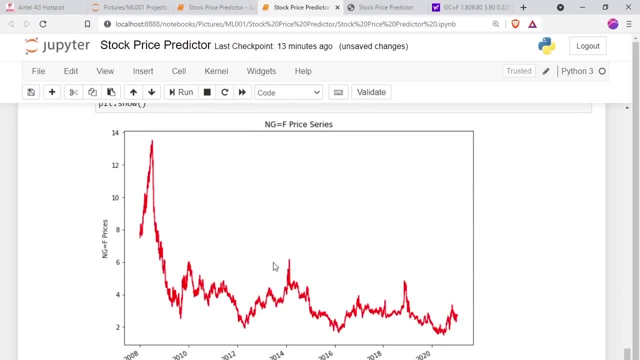 non-linearity like this. so it's very, very non-linear and it's not. you can, you can, depend on this algorithm or this predictor to predict your output in a good way. okay, so now. now i think that we are done with everything. now let me see, uh, what i have to do. okay, now let's take a look at. 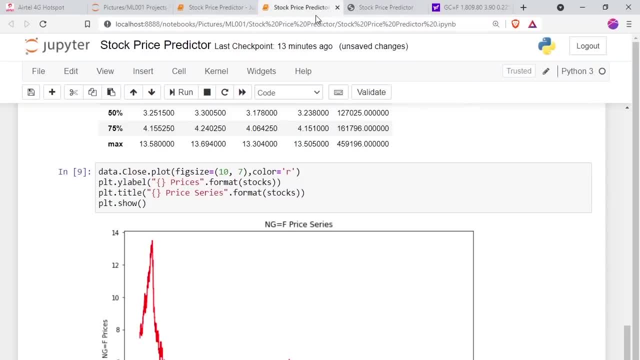 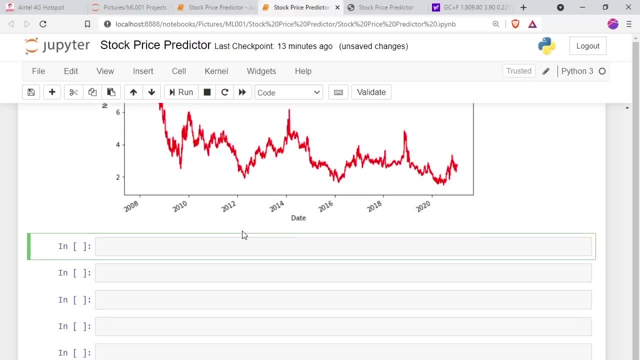 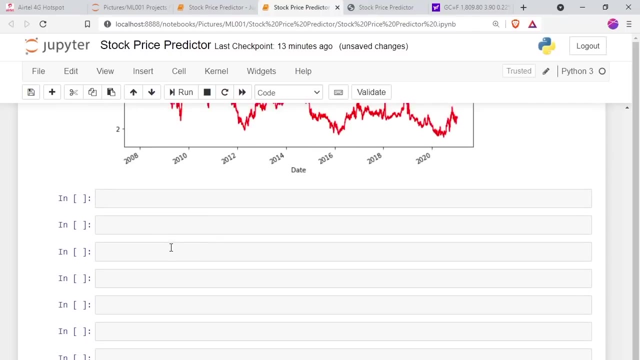 the this: how we can plot the distribution plot. was the distribution plot of our open, then what's the distribution plot our close? okay, so it will give us a more feel how we are, uh, proceeding with our data, or it will help us to choose the algorithm, okay, so here's the thing that i wanted to mention. 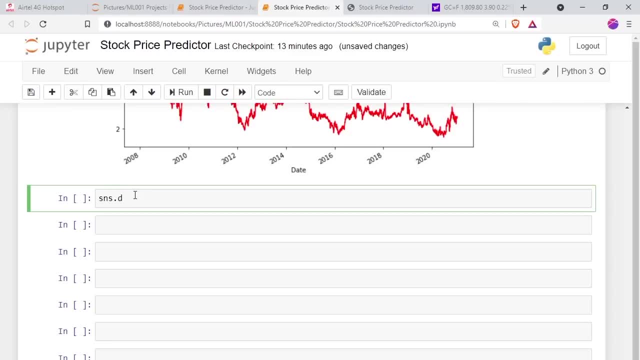 so first of all, um, just i'm going to use as seaborne and just i'm going to use seaborne, and then here i'm going to name as a data. i just want to name as data and i'm going to put over here. 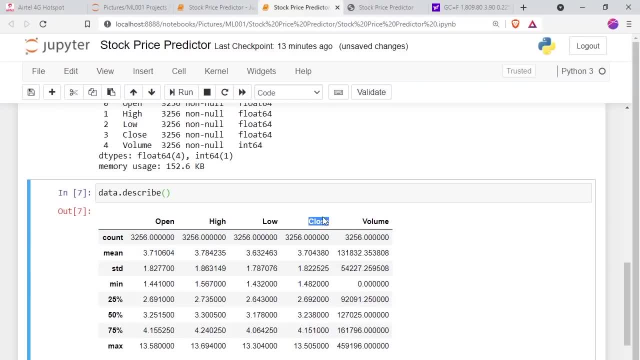 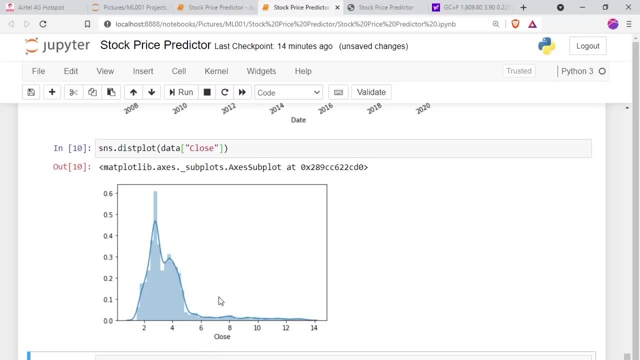 this open, let's say close, okay. so we will see if this is normally, if this is non-linear, etc. to take a little bit more feel okay, so you can see. obviously it's a little bit non, non, it's just. it's a non-normally distributed okay. so you can apply a log transformation, that's. 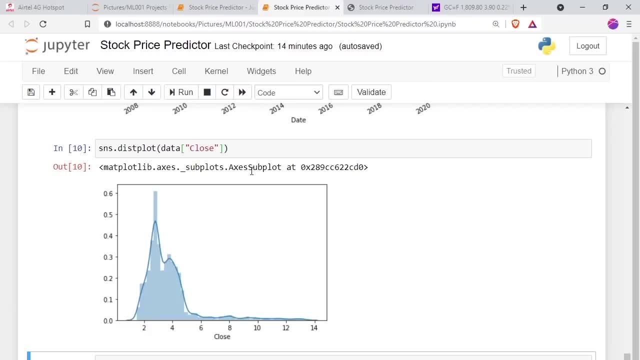 called feature engineering, but that does not work well in this case. so we should leave like this and then we will take a look at this plot and then, if you wanted to take a look at the open, then you can see that it's a little bit more like a normal distribution. so we can do the same for the other. 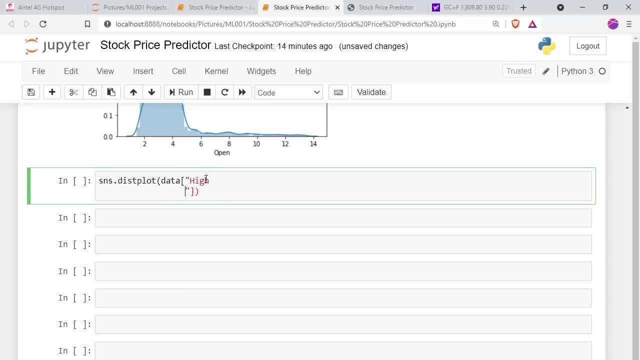 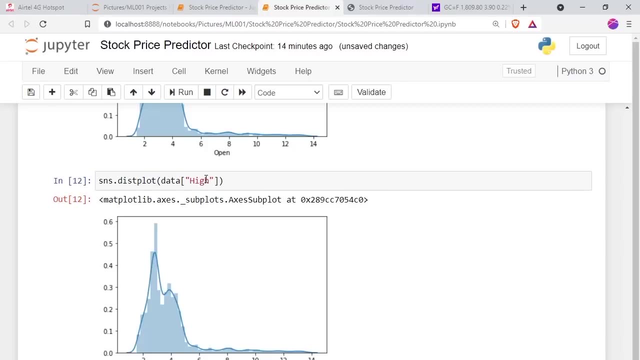 things. to get the feel what we are doing. let's say we are, we have done for high. let's say we are done for a high and if you take a look at the highest, also like there's a squid. okay, so we are done. uh, we are done with you. can, you can play with the data visualization and take out the inferences. 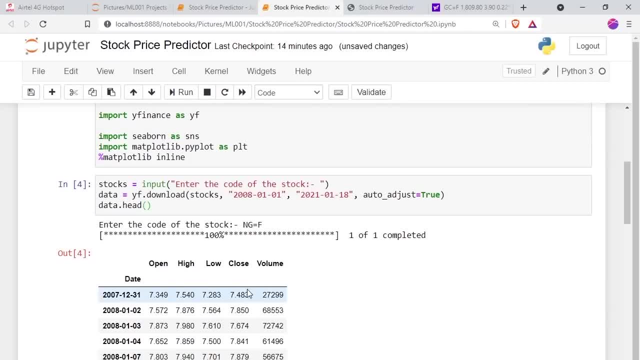 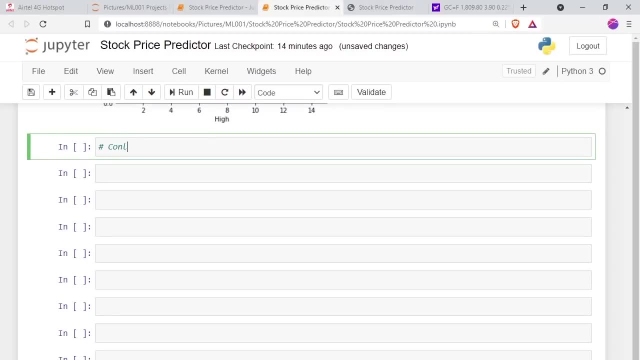 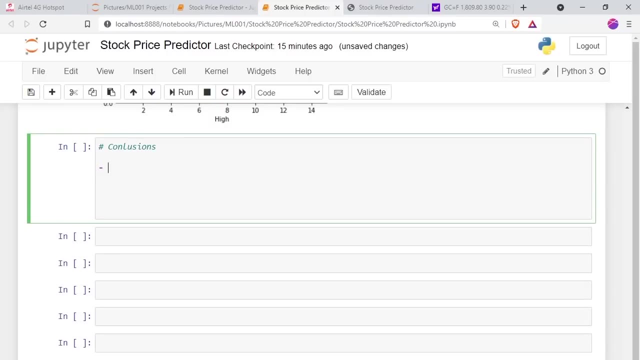 about the data and about the data inferences. okay, now we have understood the data, what we have. okay, let's uh, write the conclusion: what we haven't understood till now. so we have understood the first and first foremost is the shape of the data, shape of the data. and then we have understood. 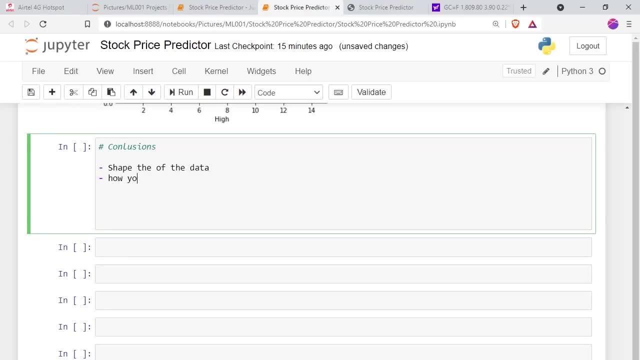 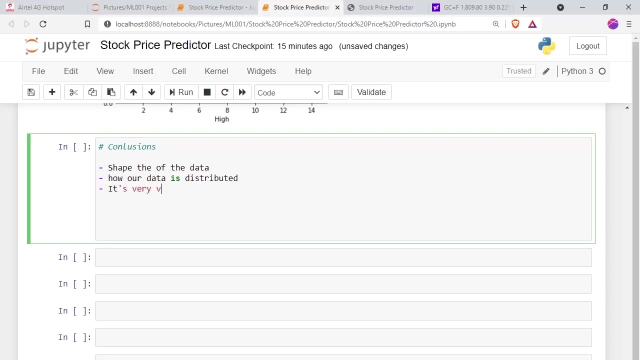 the how our data is distributed, how our data is distributed. our data is distributed, then we have understood that. then we have understood how our- uh, it's- it's very, very non-linear. it's very, very non-linear. okay, so you can cannot use for our own purpose. 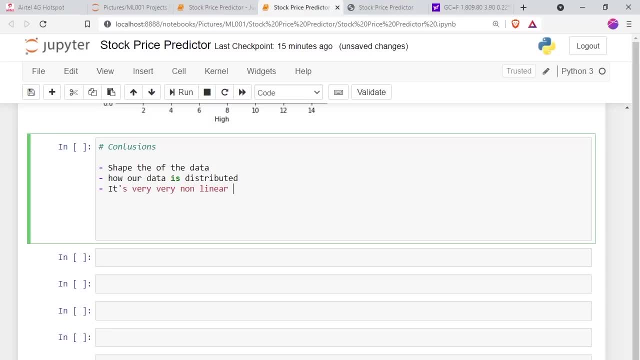 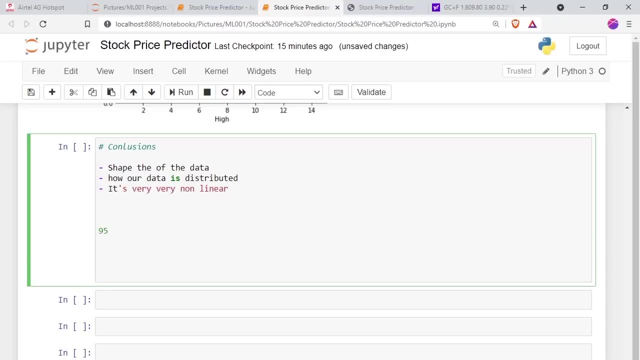 uh, maybe you can use deep learning architectures like lstm to get the direction of your stocks. and let's say, if you, um, maybe the 99.95, that works correct, or remember, 80 works correct, or maybe 775 works correct. uh, so you can have just some now. do not use linear regression. 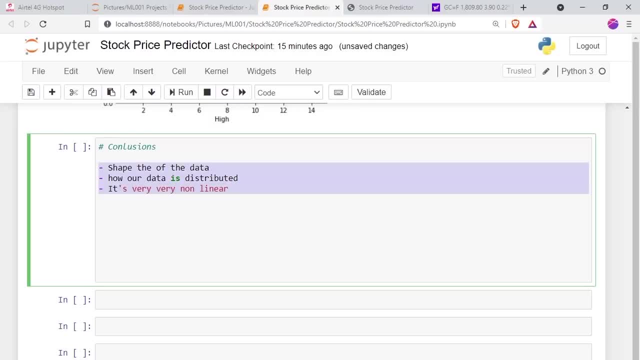 or and any kind of things to make your own use. but definitely in future let's see what the reason is. but definitely in future let's see what the reason is. but definitely in future let's see what the reason is comes with. uh, for stock price predictor, because stock price prediction. 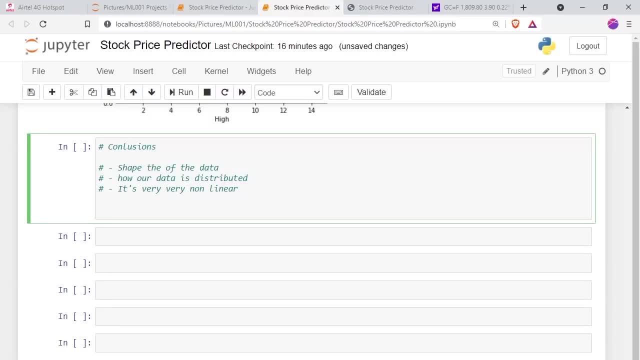 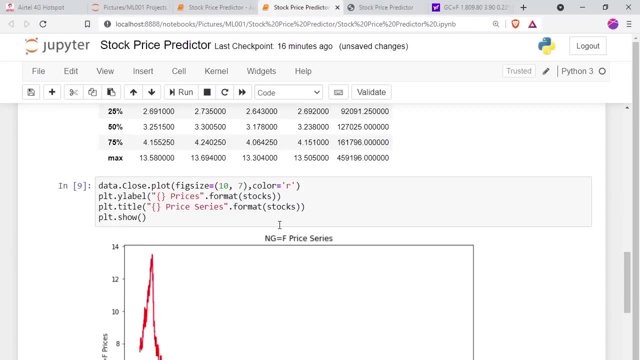 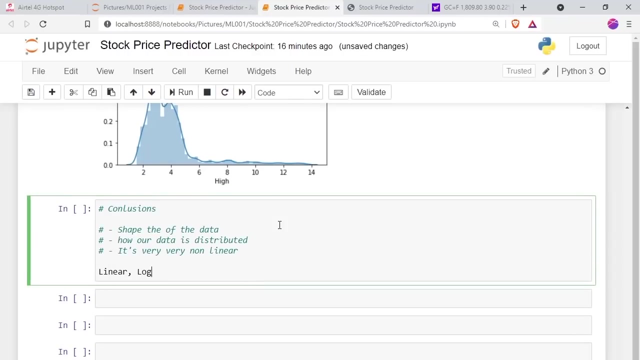 is also a competitive uh project to work on because it's very, very non-linear. okay, so we are done with this and now it's time for we have started how much algorithm. we have started linear. we have started linear, then we have started logistic, then we have studied some regularized linear models. 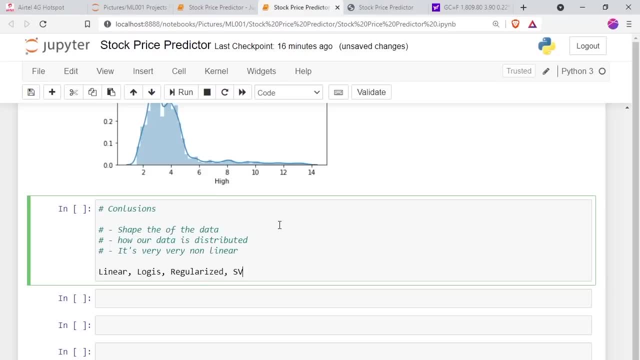 regularized linear models. then we have started support vector machine. then we have studied common analysis, which will study, uh, which we have not studied. so we should study principal common analysis and then, for the moment, okay, so we will use support vector machine, we will use support vector machine, but we will see that linear regression and regularized linear models. 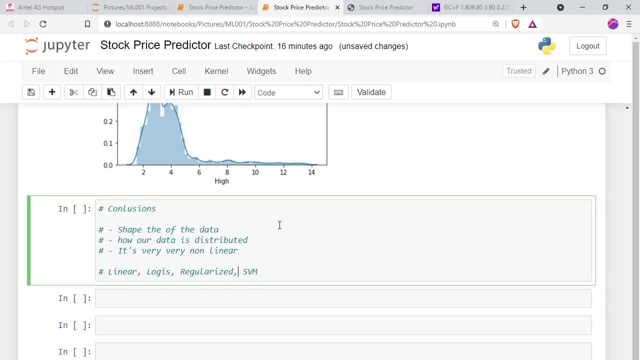 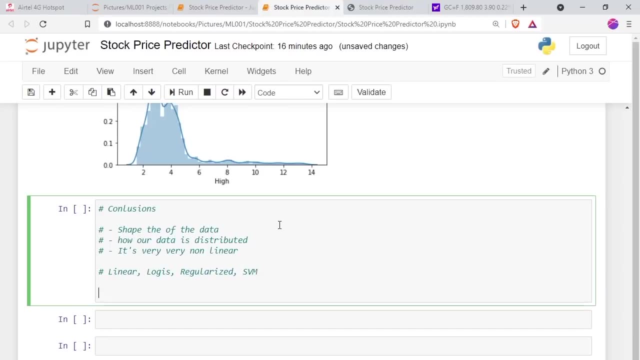 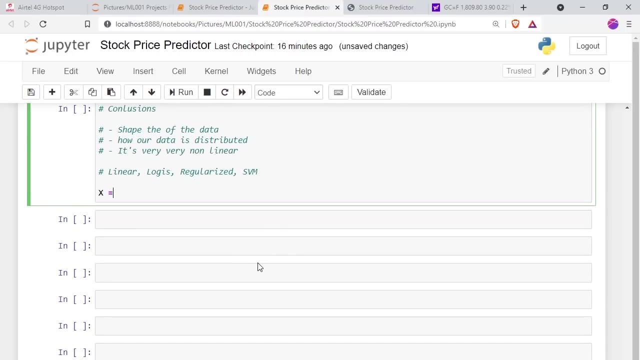 works best in this case and we will go with, or saving the model of regularized linear model. okay. so let's start with linear regression, but before that let's split our data into x and y and then the training and testing set. so here i am. um, just i'm going to x like my convention, so i'm just 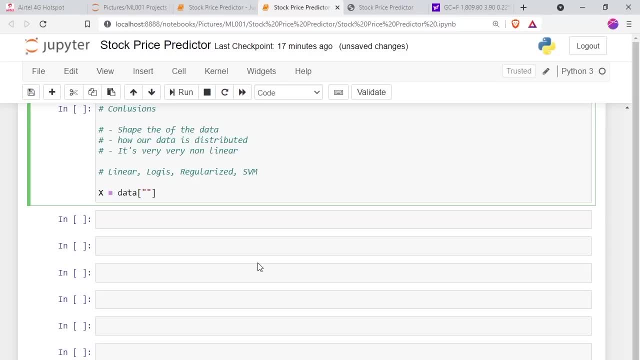 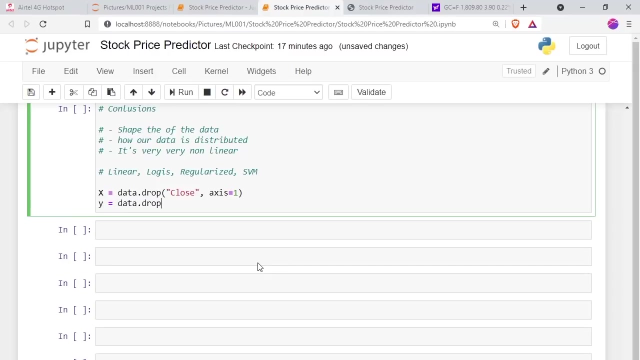 going to make it like this and our x variable will be all the except close. so i'm just going to remove this and then in: x is number one, and then y equals to data, then y equals to data, dot drop, i'm not. it says we will not drop it, we will just give, simply give the close. okay. 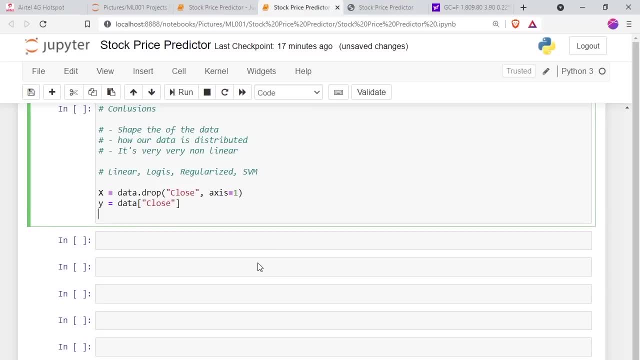 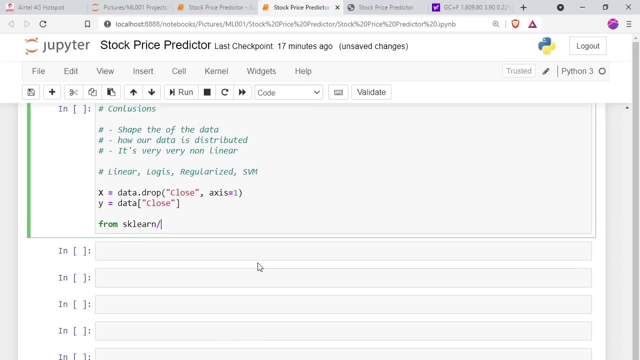 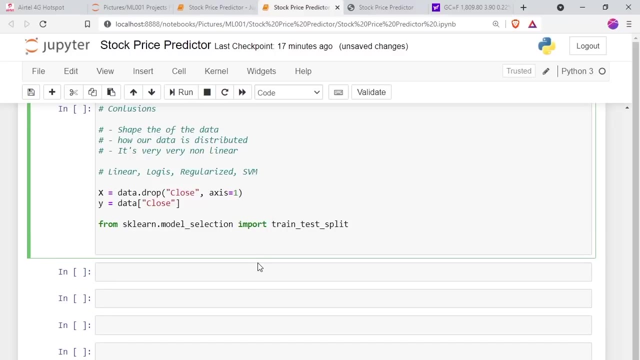 now, if, uh, we, we are done with this. now, x and y data to drop close x and y. now we are done. now, what, what we can do? we can simply uh, import more, uh, kind of a model selection, uh, which is trained to split. we'll import one thing which is trained to split, which, let's say, you want to split your. 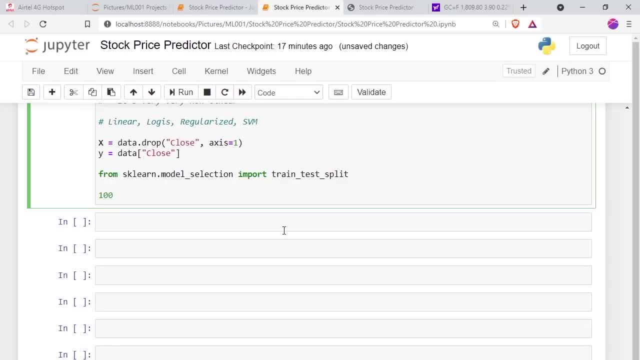 data. let's say you have 100 percent of the data. so you will uh split your data- 80 for training and 20 for testing- to validate your model. okay, so here i'm doing what i'm see you can see over here: x train, x test and y train, y test. okay, so this is the. you can make the variable and all the. 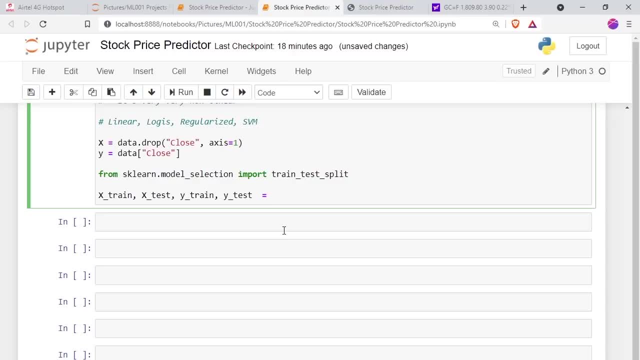 training and means the labels of x train will be in y train and label of x test will be in y test, like this: okay now, if you, now you have just give x and y and just give the size of the test set, which is, let's say, give the 20, 20 percent, means you just want to use 20, 20 of your whole data. 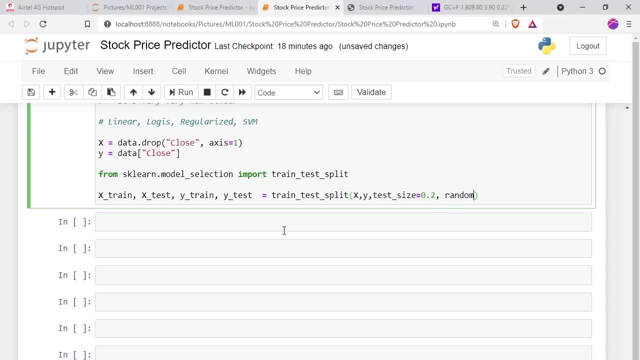 for testing. then you want to do just random state and you think, here you, what strand randomness does? it's simply, um, let's say, uh, if you, if you run it one more time, then your data will not be changed. your shuffle, because shuffles also, so your data will be. 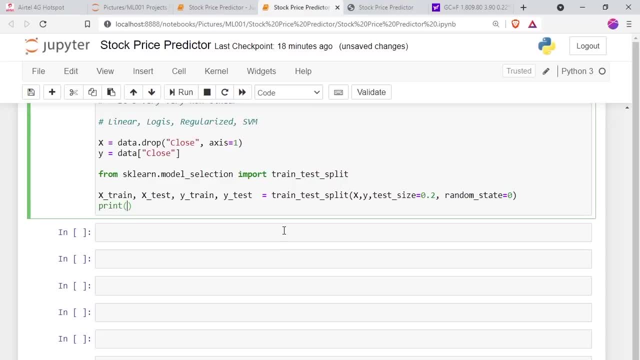 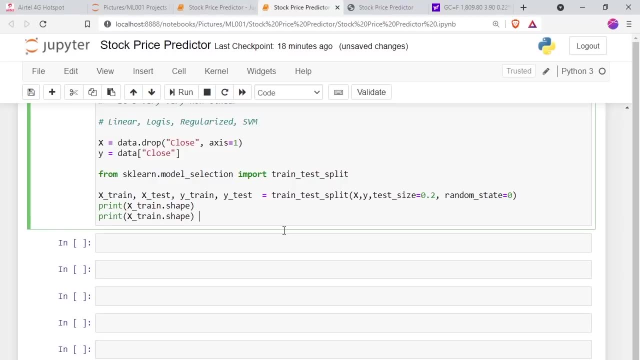 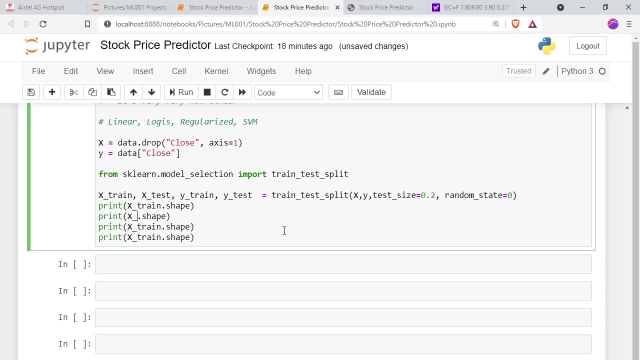 not changed. okay, so we will take a look at the shapes of that so that we can get a more feel what we are doing, so you could understand what to whom we are working with. uh, let me just copy and paste it over here and just going to make it like this, and then i'm just going to 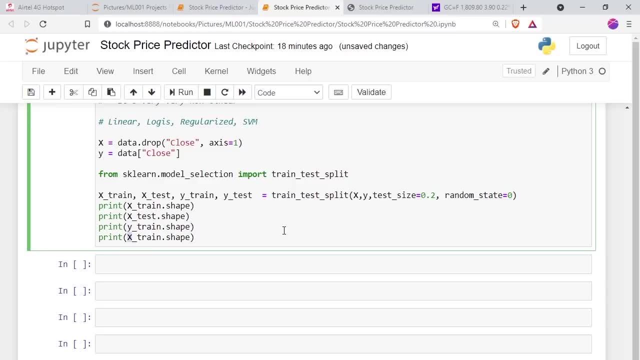 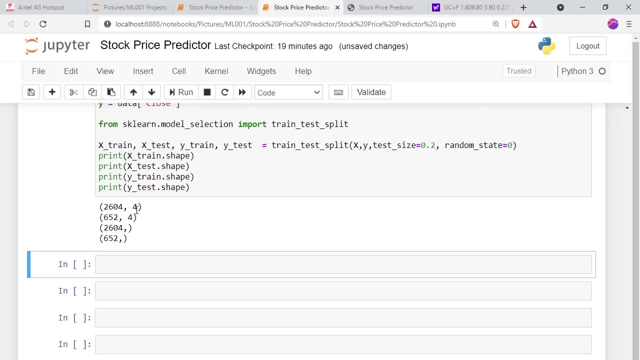 make it y train and this one by test. okay, and just meant to make it a little bit more detailed. okay, when you run this, you can. you're going to see over here that you have a 2604 and four columns, and the fifth column is two, two thousand. uh, this the labels of y. okay, so that's the thing. and now 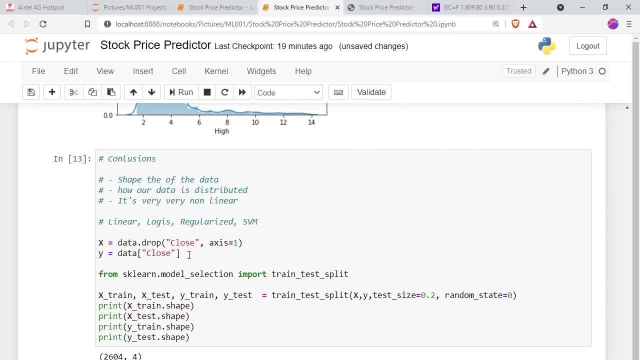 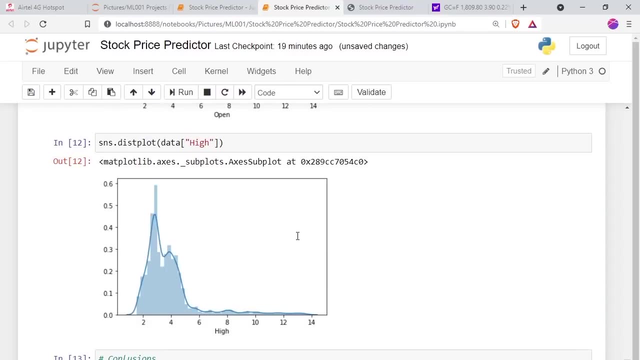 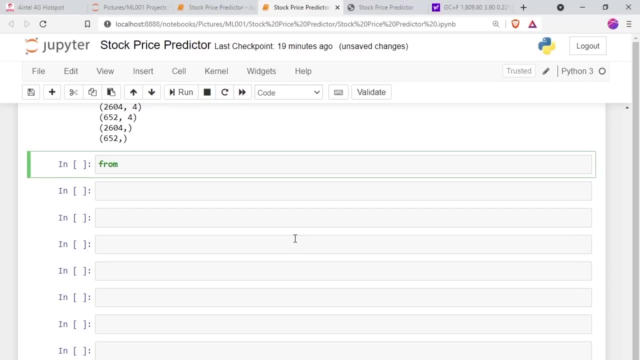 what we can do. we can go further, and we have taken the close as our target variable, which will tell us the direction of our stock stocks. okay, okay. so now we are done with splitting, now it's time for getting into a little bit more depth, is uh? modeling part means we are going to, first of all, i'm going to import the linear regression. 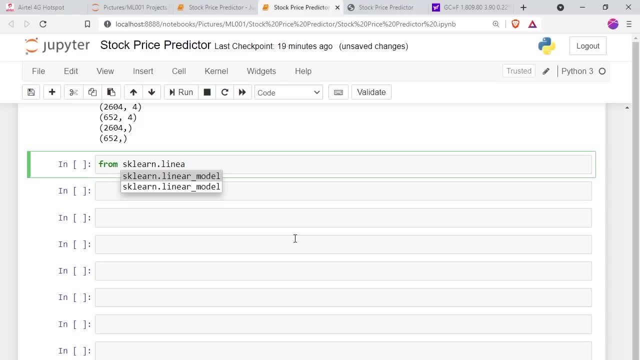 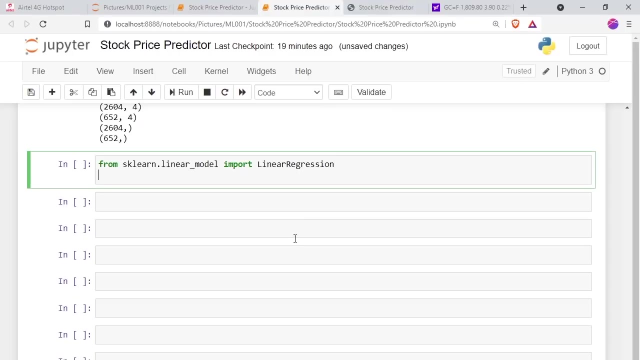 because every everyone thinks the linear regression is very bad, but let me tell you it's very powerful algorithm when it comes to linearity, but here we don't have a linearity, but still it works best when you apply a polynomial, etc. question. okay, but let's uh keep. 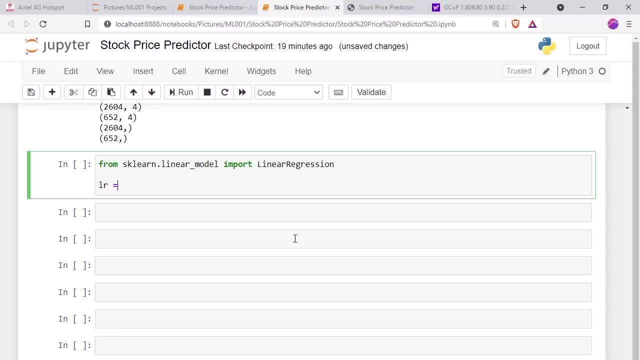 let's use the logistics- sorry, linear regression, and you can see over here that this is the regression problem and so supervised learning problem. so we cannot use logistic. it will be very, very bad for us, okay, so just i'm going to instantiate, just i'm going to incher: instantiate, instantiate. 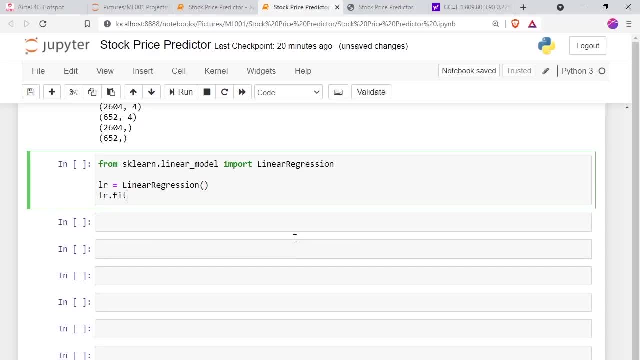 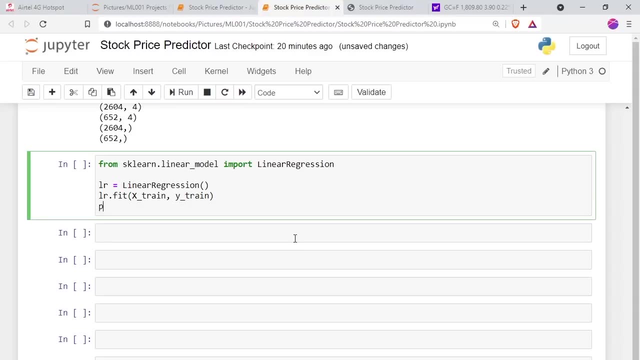 and i'm just going to call lr dot fit and i'm just going to give x train and the labels y train, which is the labels of x train. okay, predict one means i'm going to use that lr, which is train model, to predict my X test. okay, now, if I run this, now, if you see the predicted, 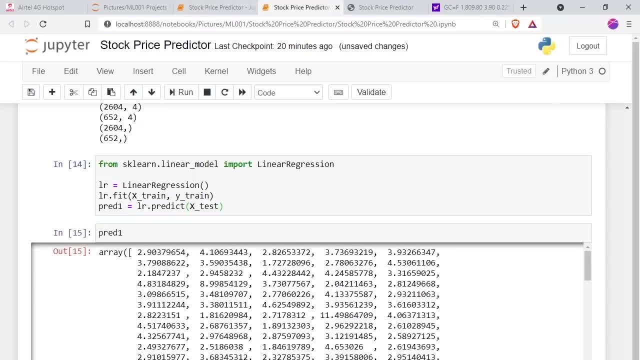 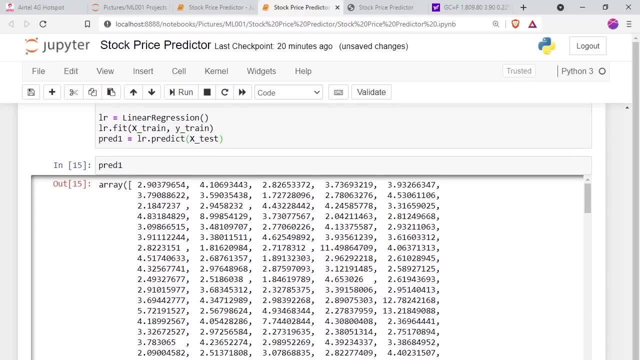 output. you can see over here that the let's see the first training sample. so you can see over here: oops, this y test huh. so you can see over 2.918 and the predicted is 2.90 and the actual value is 2.918. okay, see the things. that is. 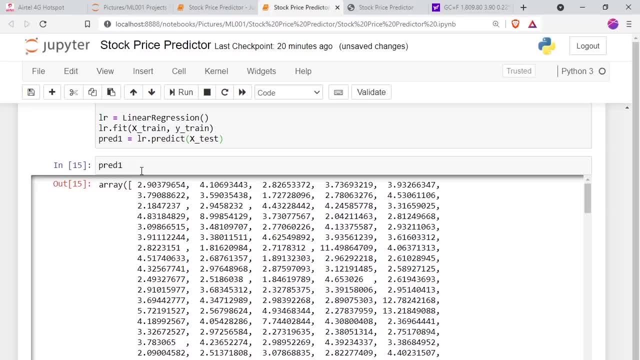 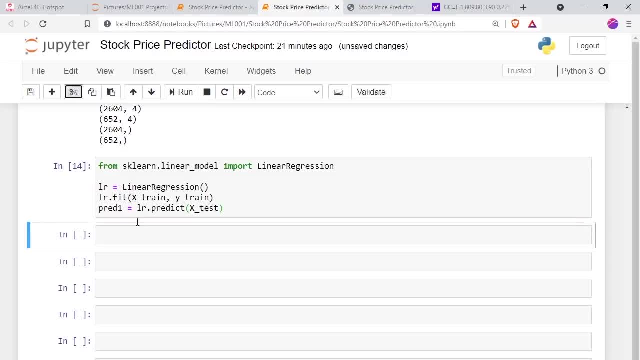 over here. this quite, it's quite, very, very good because you can see over, that's quite working very, very good. and yeah, linear regression works out as best. but it may happen that may over fit your data. but let's see, let's calculate a matrix. so we are going to use some matrix, which is ma. we are going to use 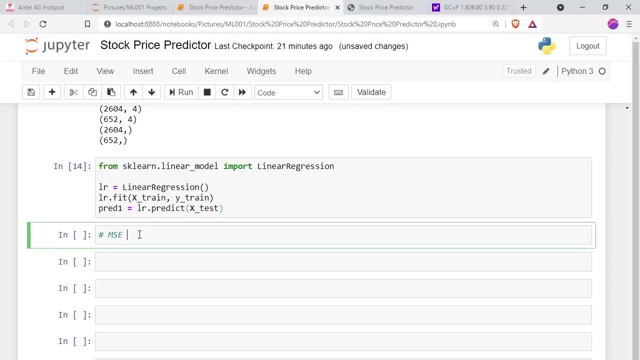 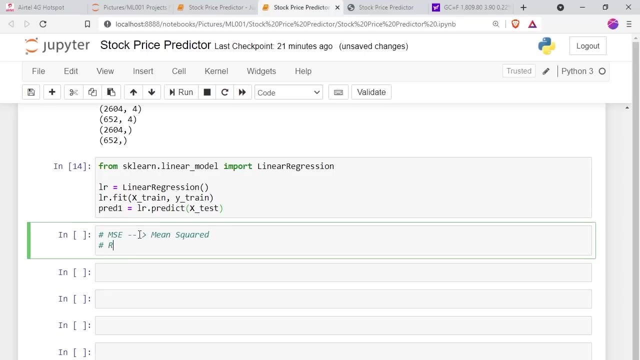 ma, which is a sorry MSC, which is a mean square error, which is a mean square error, which we have talked about, the cost function for a linear regression. and then we are going to use, then we are going to use RMSE and simply it does simply the square root of a square root of mean square error. and then what you 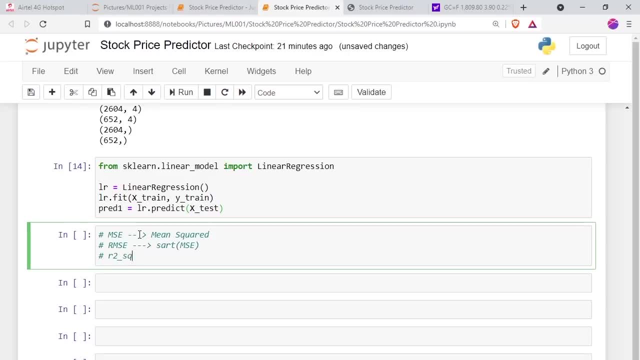 do here and then we will calculate the R2 square, okay, and you can see. if you want to get into mathematically, we'll talk about some matrices- matrix later on. but the best output of R2, if your model giving output is R2, equals to 1.3. 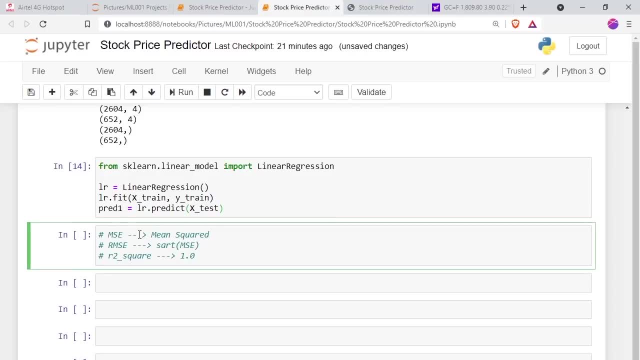 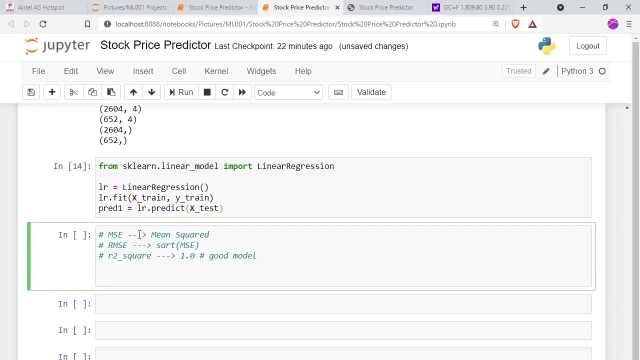 then you have a very bad, sorry, good- model and it's a good model if it's, if it's giving good, okay, so we'll see how much our R2, etc. so I will write one helper function like this, right, won't helper function, calculate matrices? I will 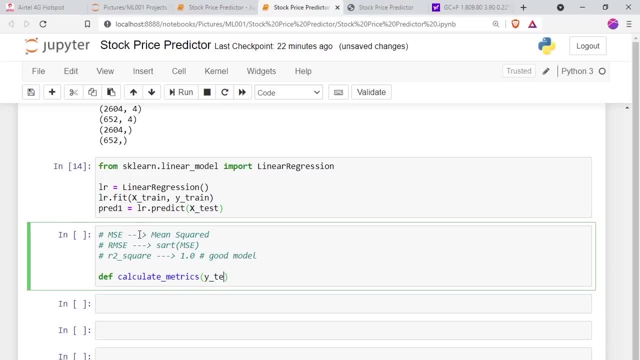 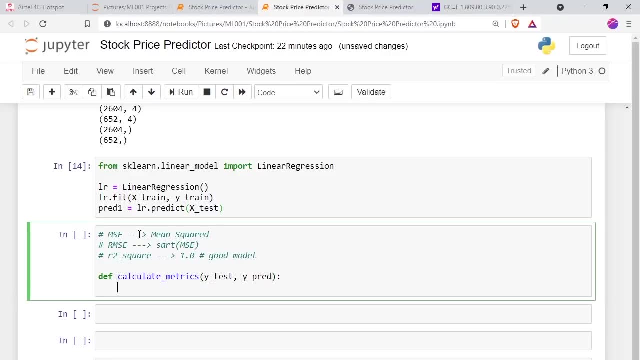 just write a matrix and then it simply takes the actually value, which is a ground truth, and it simply hace the predicted value of your model to cal, calculate. and then, first of all, I'm going to calculate the MSC, and it's just first of all as a 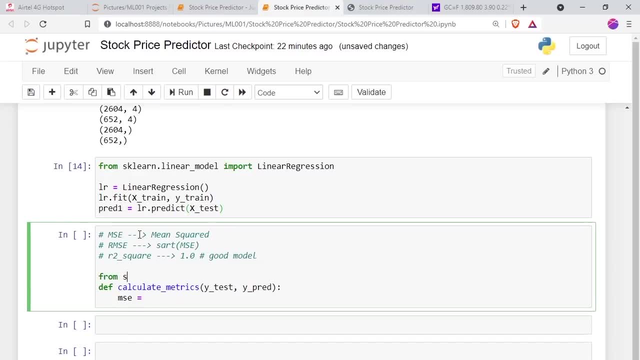 to import because you can also make your own function. but it's better to use vectorize or scikit-learn because it's already provided to you. but you know, it's very kind of easy if you wanted to define msc, so you just write and define msc and just uh, take the sum of everyday data. 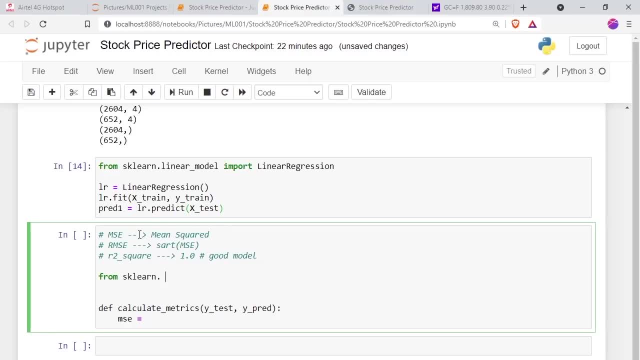 point and the residuals, and then just, uh, square them up and then like, like that, you can do that. we have already- i think you have implemented programming assignments, okay, so you can just make it import. uh, let's say: oops, i don't want to, i just want to import the matrix and i'm going to. 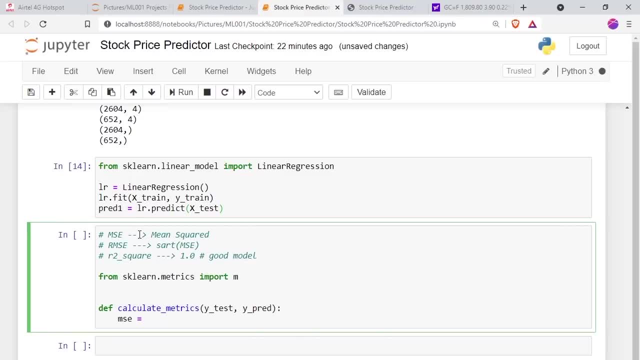 import msc and mean square error. obviously we do have mean absolute error, which you can also use, but for now i'm going to use these two. but, by the way, we don't have rmsc. we have to code rmsc by yours, by ourselves. okay, we only have r2 squared. so first of all, let's uh, do this kind of thing. 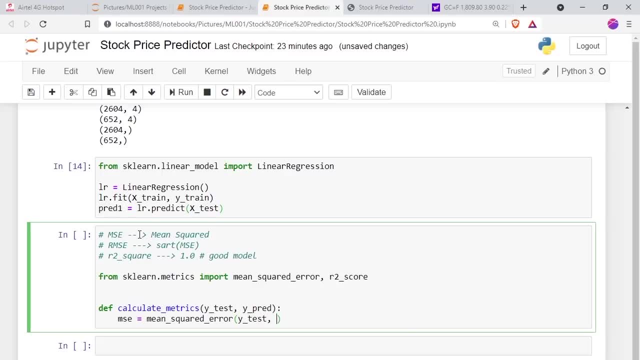 means mean square error, giving the our parameters y test and y and y fret, and then rmsc. and you may think here you how, how you can calculate the root. mean square error. just write np dot. square root is just taking the square root of msc. okay, 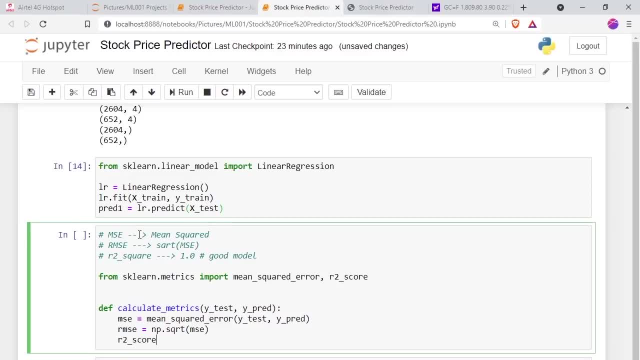 that's easy. so r2 score, which is r2 scores i'm just going to write: is doing a spelling uh wrong, because maybe it will cause some error if you have a reserve keyword or like. that's function okay. so you have r2 squared and then 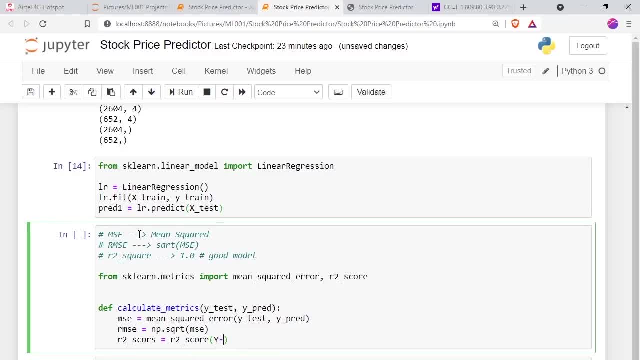 rmsc. just give it a kind of function of rmsc. and then rmsc, data circle- butterbox, kid one there- and rmsc u t is p quarter and f quarter t. now when you say these things, rmsc is your y test and here it's the gates frick. uh, it's your score. and now you just give y test. 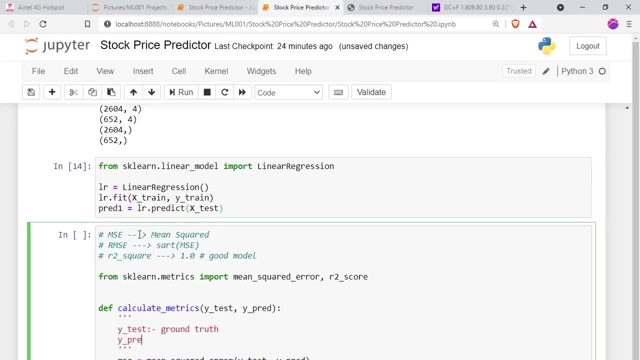 now you just give y test. sorry, yeah, y test and y fred. okay, and these are y test and y fred are. just let me write that. what is this? oops, i'm. i think that i'm doing wrong. uh, you can see the spelling okay. okay, so we are now. 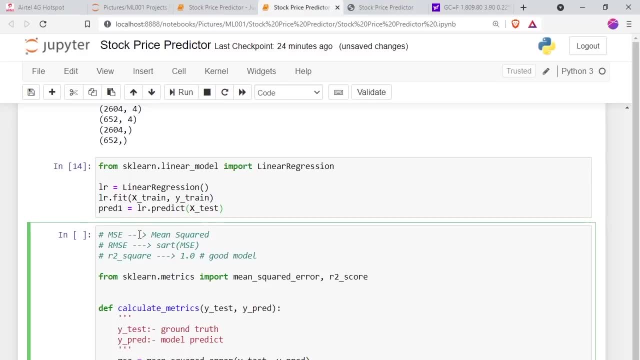 what i'm, what i will do. i'll just print it out: msc, then i will print rmsc, then i will print rmsc, then i will print r2 okay, r2 scores okay, and this i'm just gonna do: msc. uh, just want to. 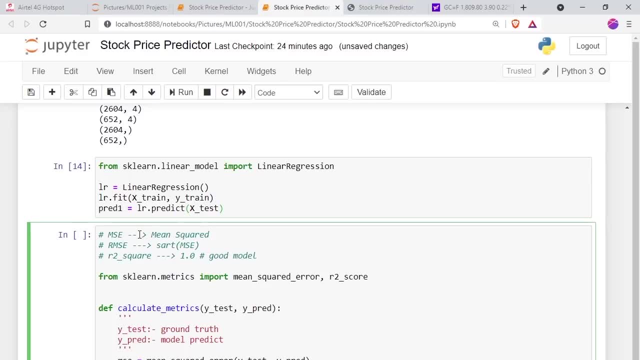 make it msc like this, and here also i'm going to make it rmsc okay, and here also i'm going to make r2. square are to score. sorry score, it's score okay. now i think that it should work now. we are done now, if you wanted to. now we are done with. 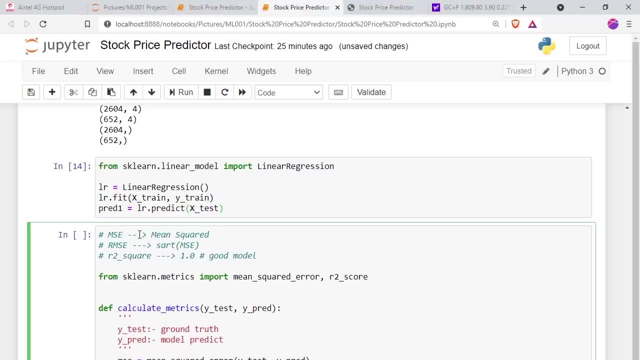 helper function. now we're going to calculate the matrix, so you where? we will just calculate the for a linear regression, so we will just give a y test which is: i would ground truth, which I made. oh, it's about while splitting our data. now we'll make. 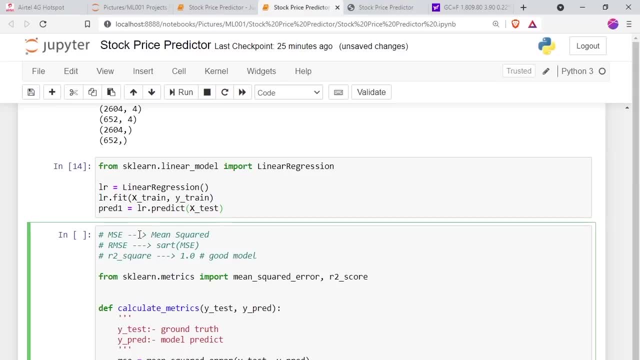 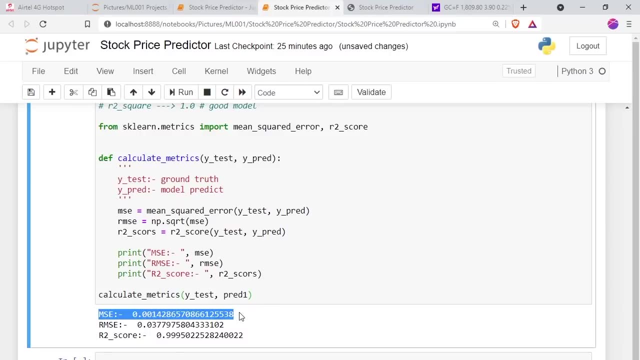 a Y prediction. Y prediction- and sorry, it's a prediction- one that that we have made in linear regression predicted okay, so you can see, the MSC is equal equals zero means approximately equals zero is quite good, because and cost function- your cost function should be very, very approximately equals zero. your root miss. 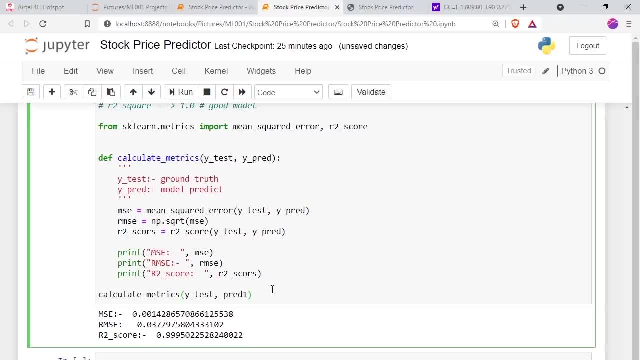 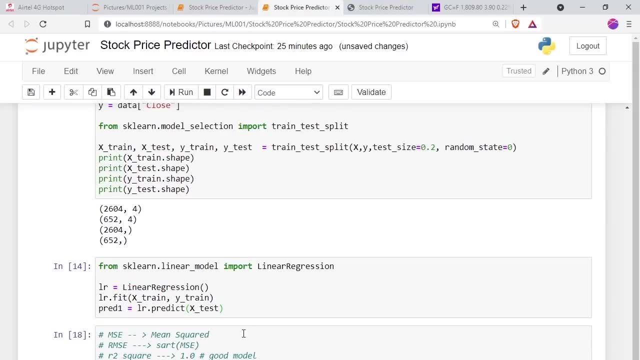 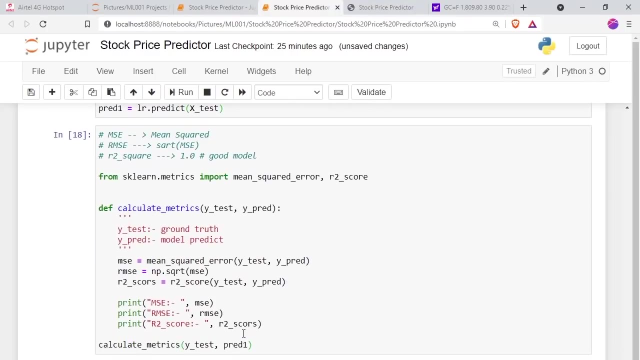 square is also and your R2 is zero point nine, nine, nine misses, and misses approximately equals to one point. oh, okay, so it's quite good. lane linear regression performs quite good. okay, now let's a little bit let it go go further into some regularized linear models like rich and lasso. so let's use that from. 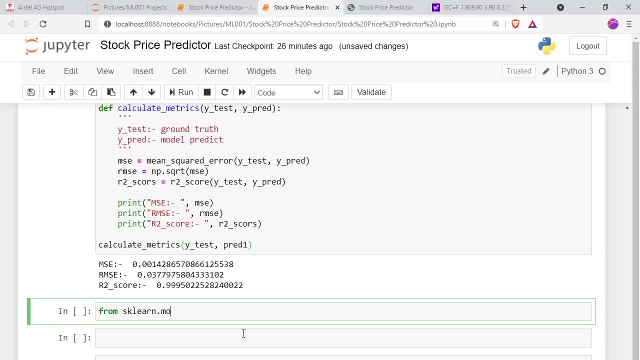 SK learn, SK learn dot model. sorry, linear models, linear model. I'm just going to import lasso and you, if you know, if you name, may know about this. lasso and rich. lasso, what is? or simply eliminates the less important features, simply eliminates the less important features. and rich is just a penalizes your less important features. 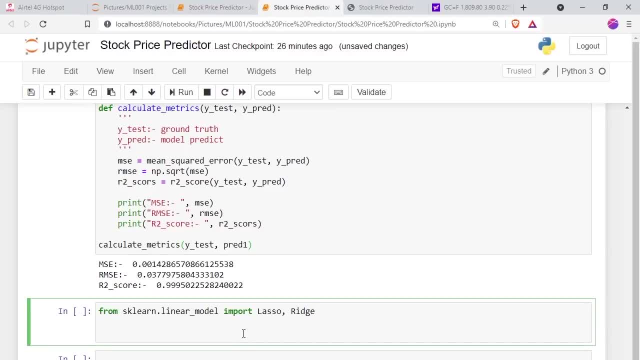 okay. so now let's make, though, two of them, so let's say la as a lasso. so I'm just going to fit it over like: this is a short form giving the X, x-ray and y-train is a short form for doing that, and then I will do for the. 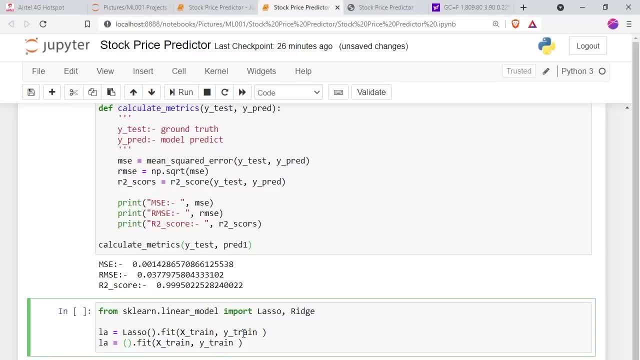 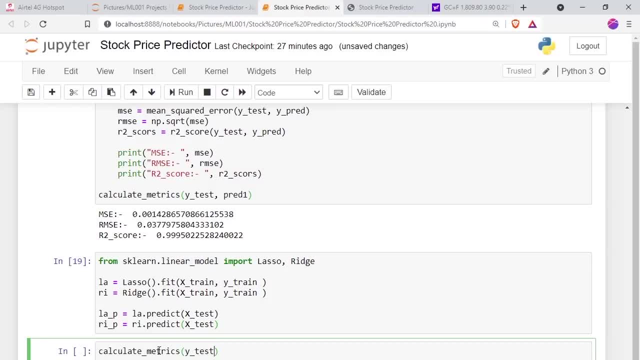 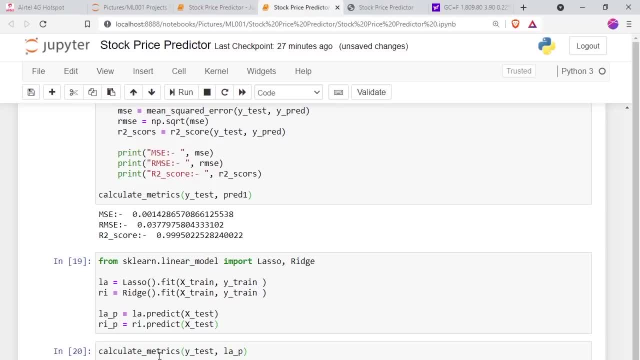 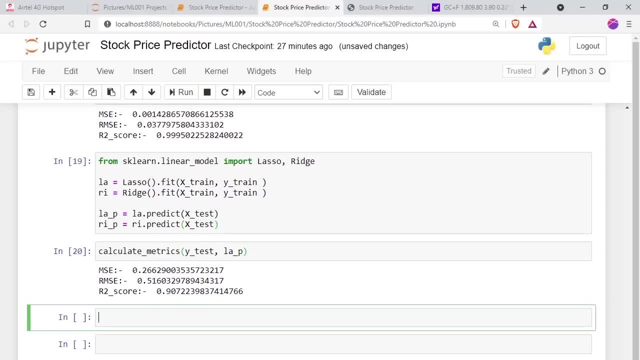 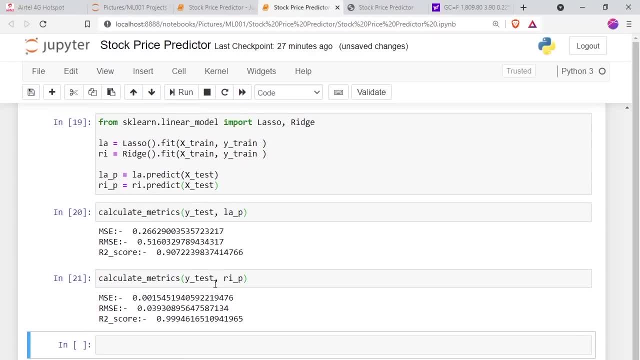 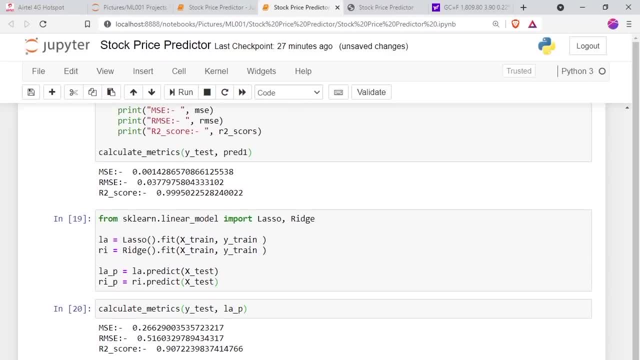 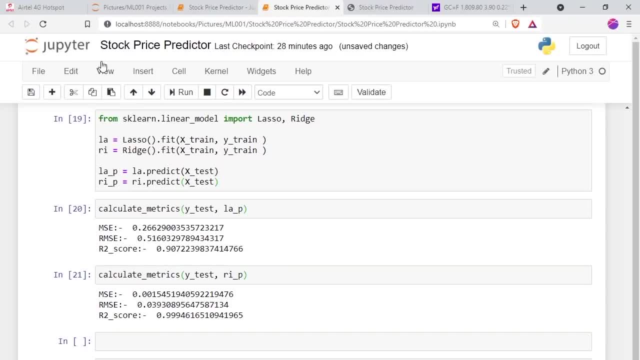 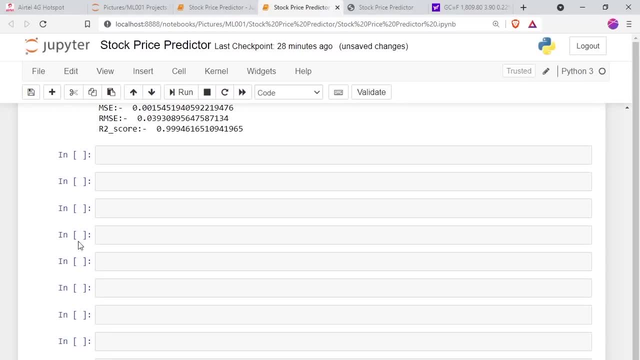 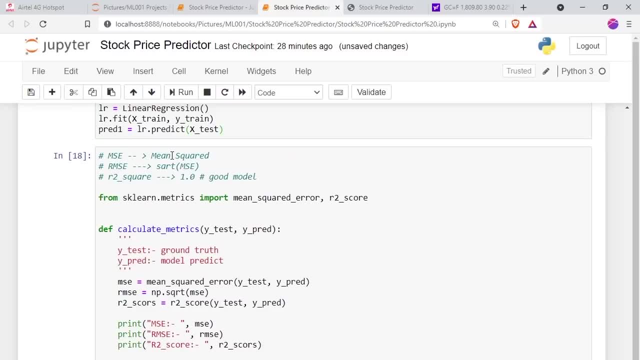 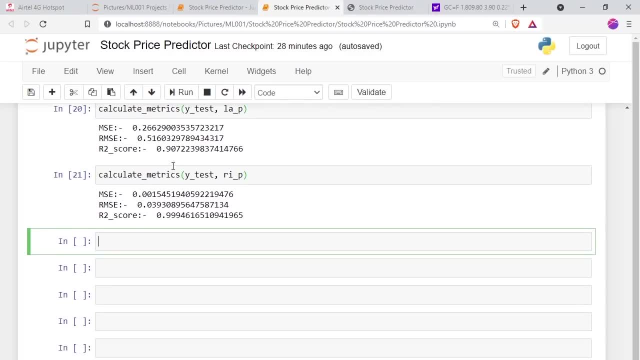 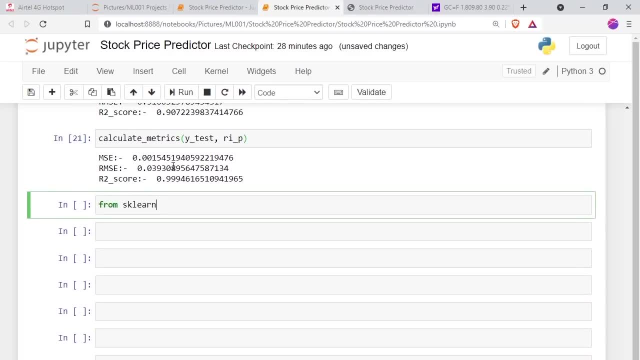 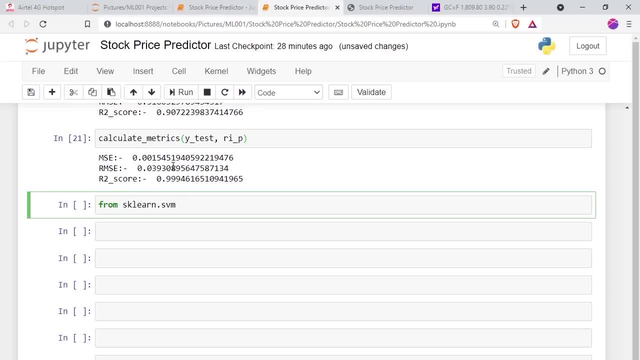 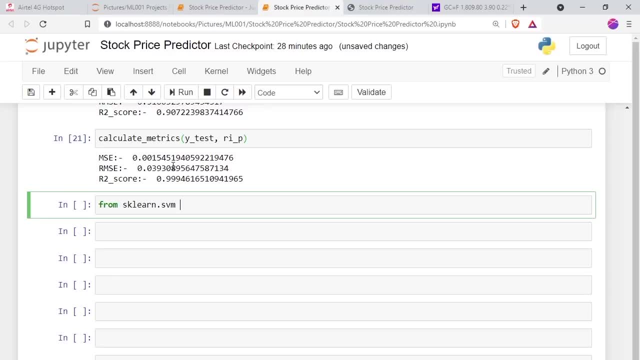 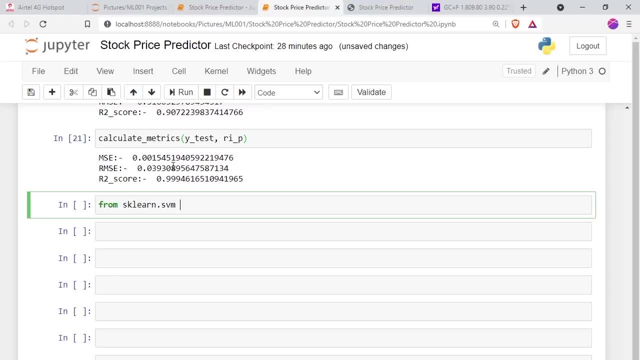 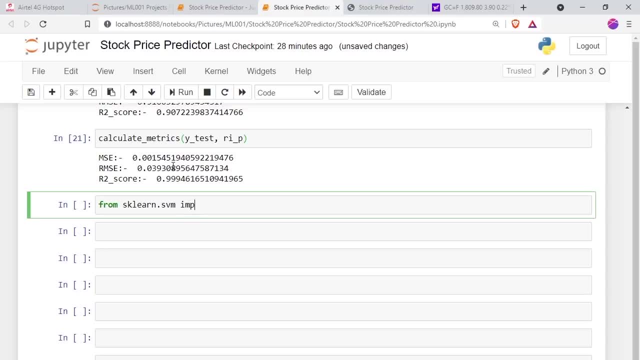 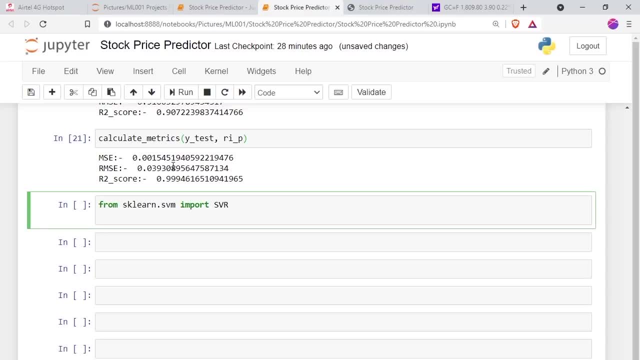 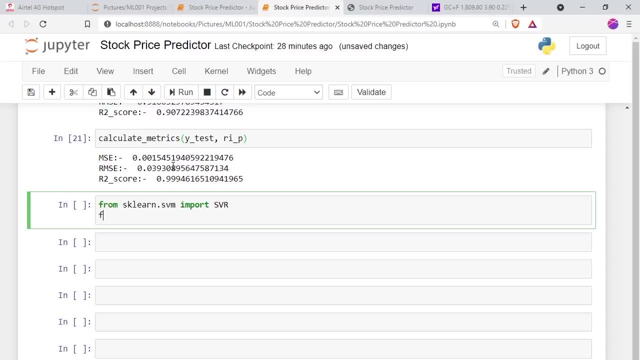 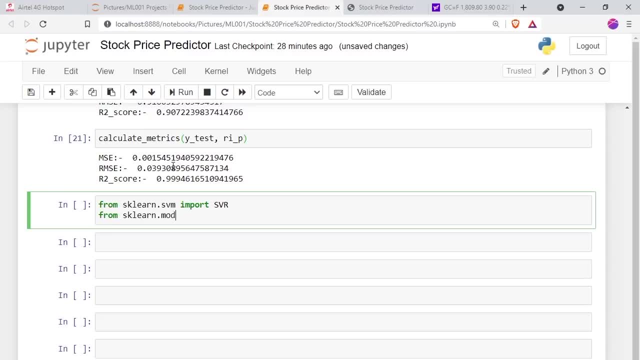 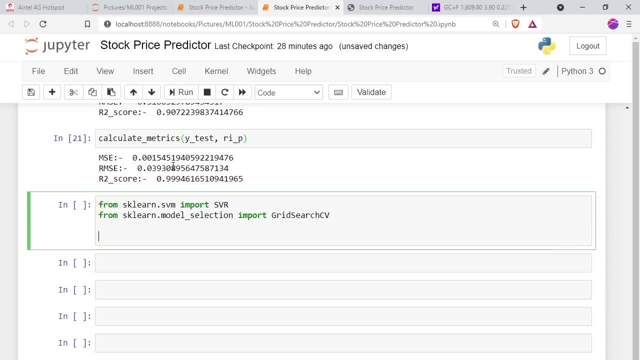 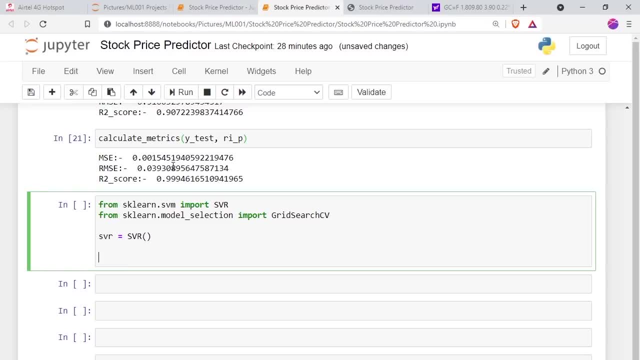 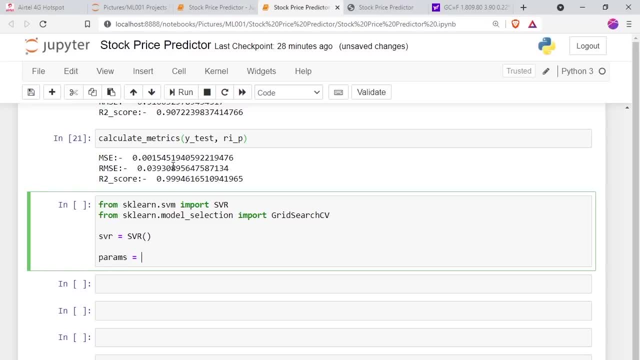 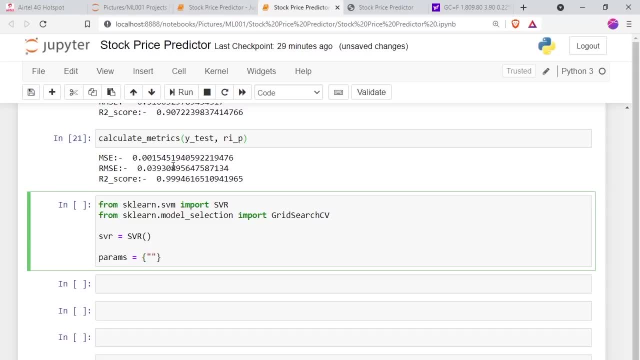 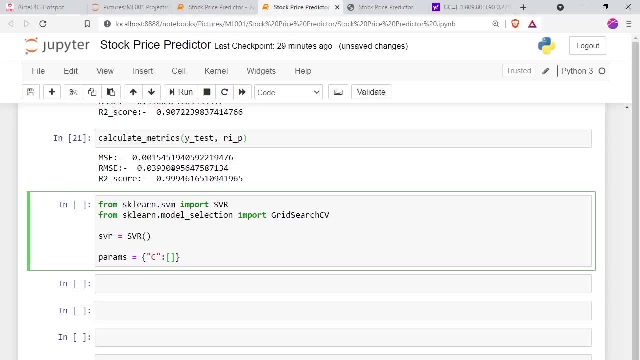 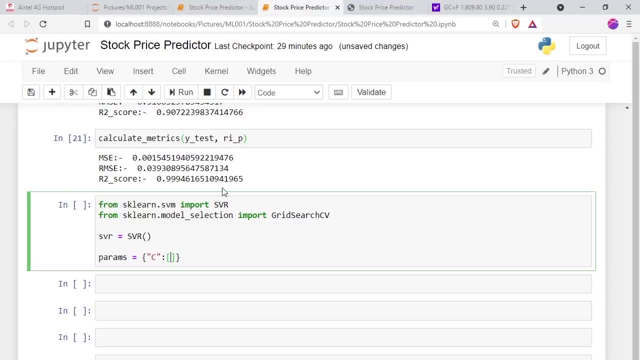 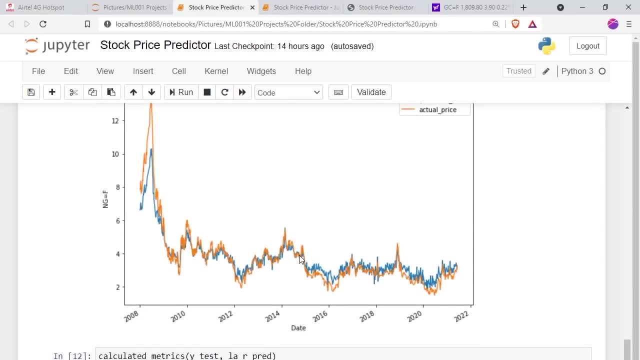 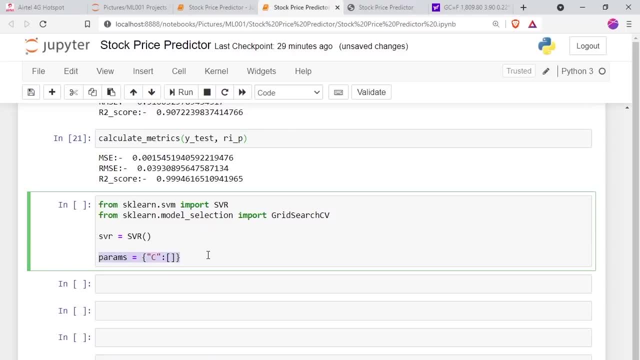 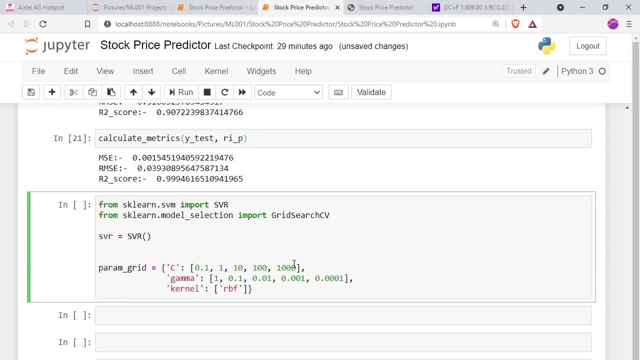 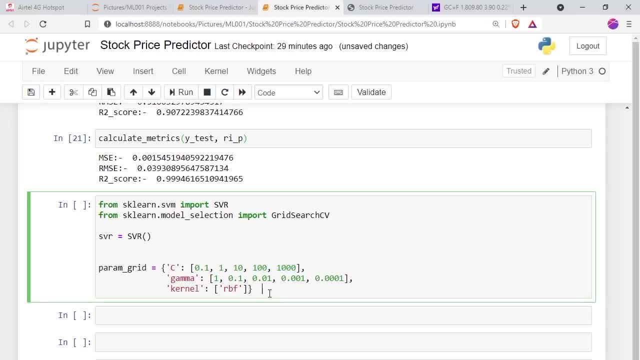 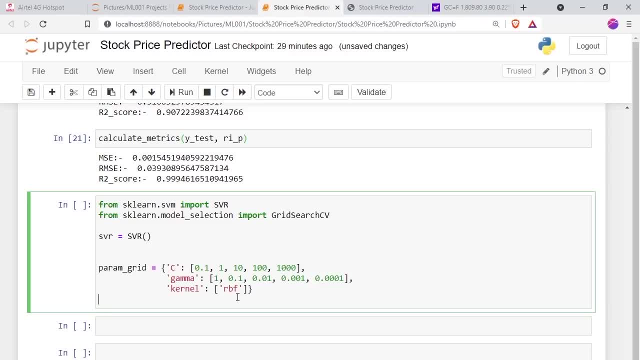 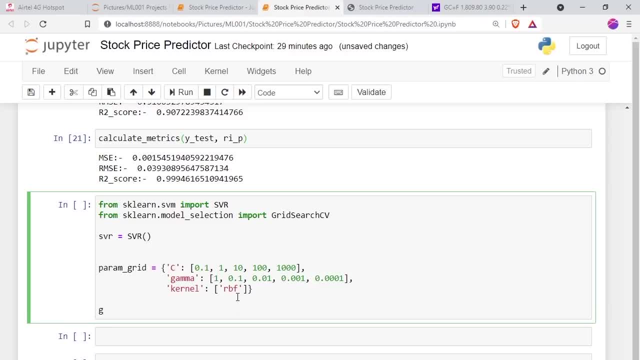 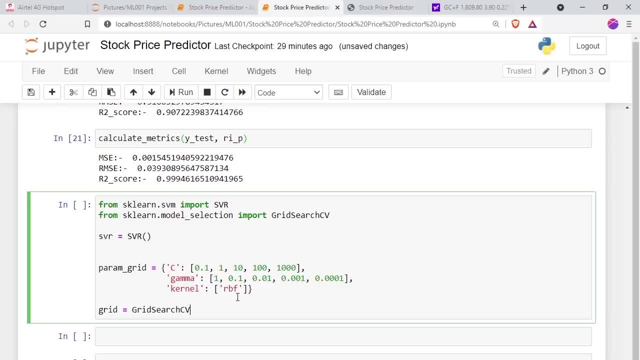 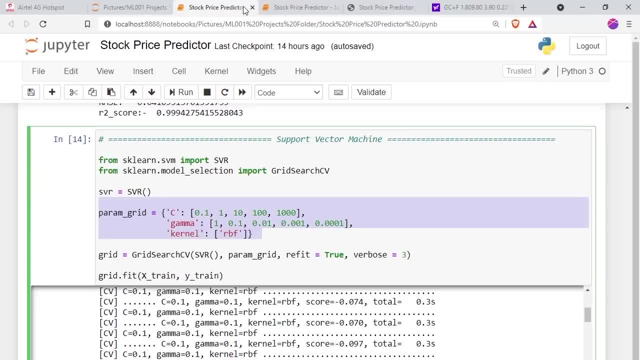 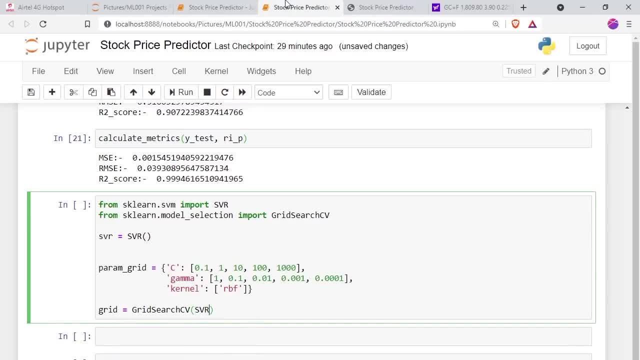 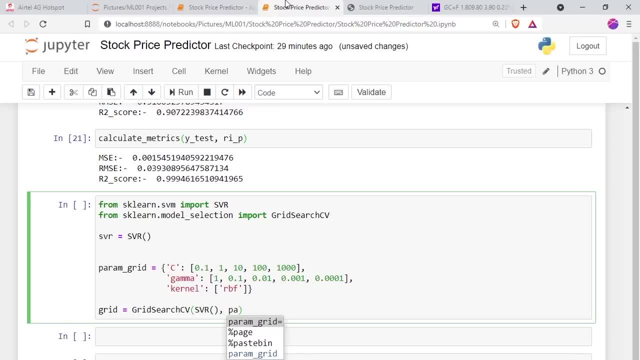 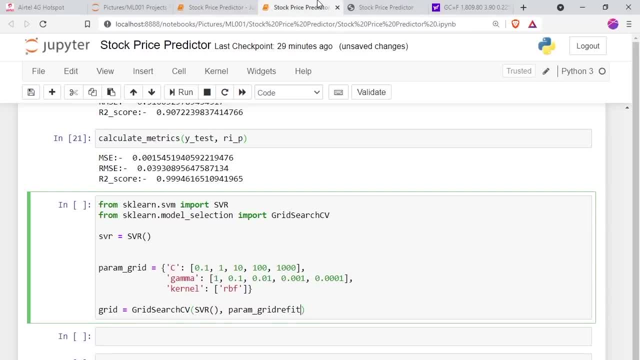 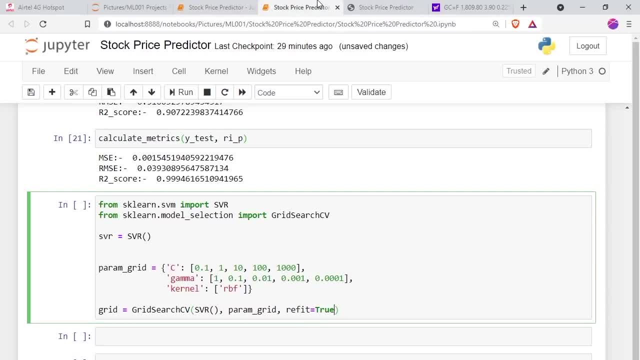 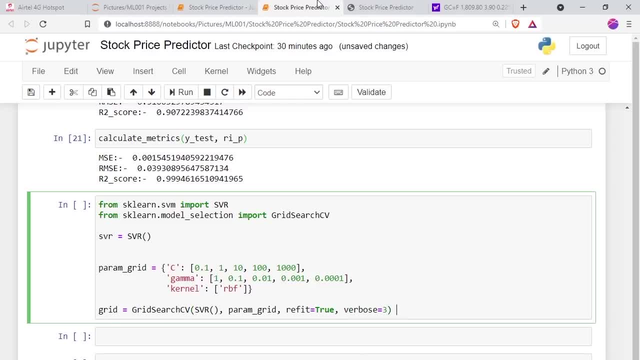 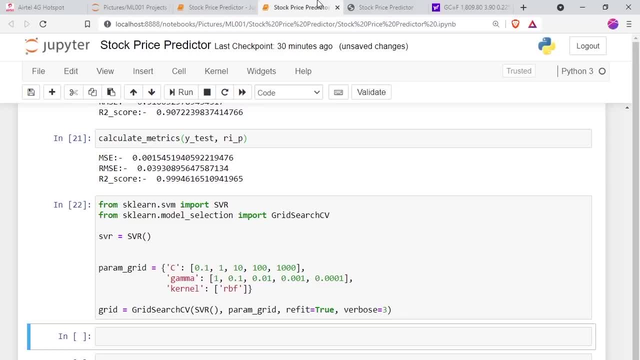 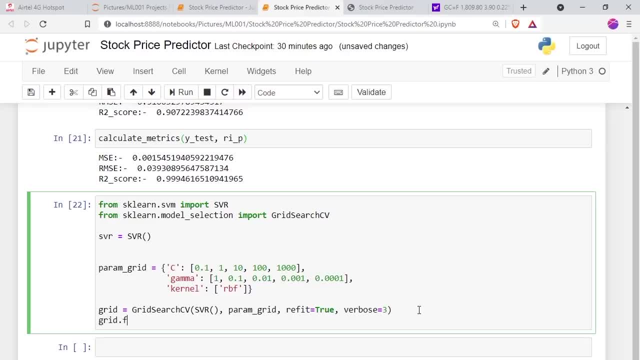 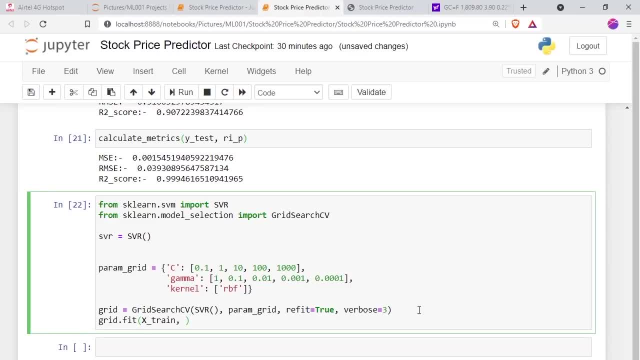 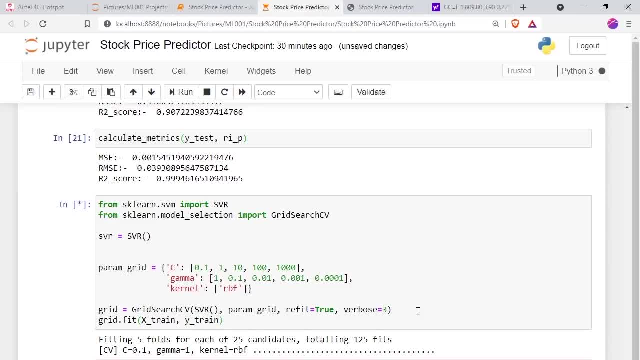 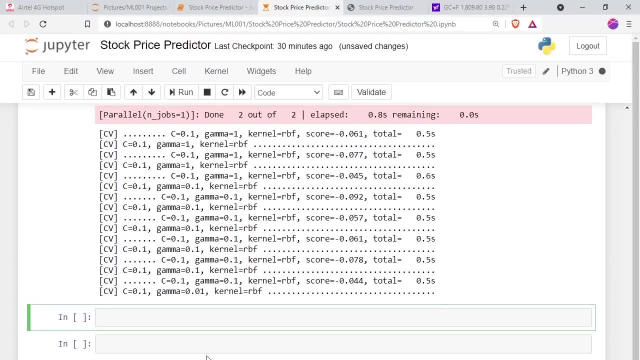 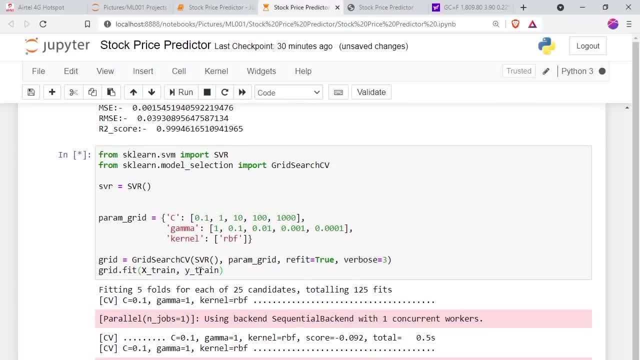 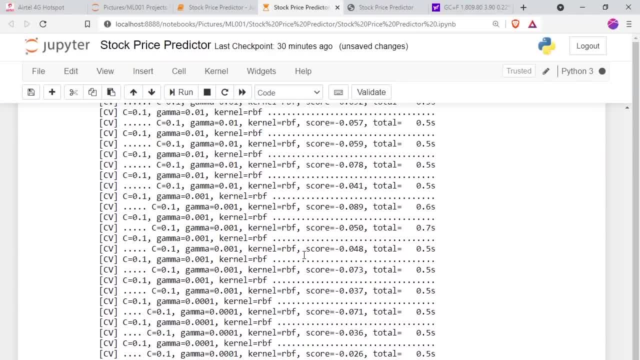 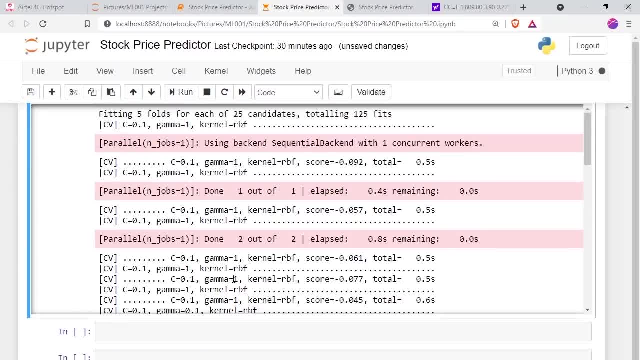 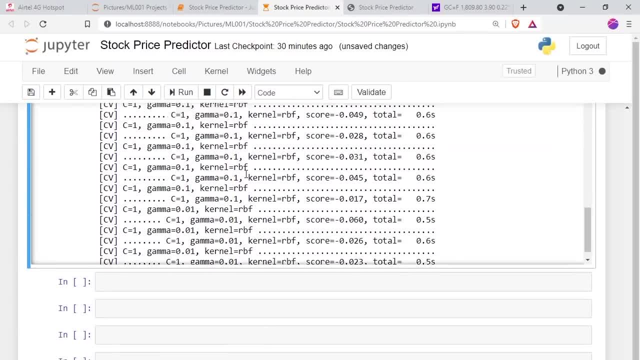 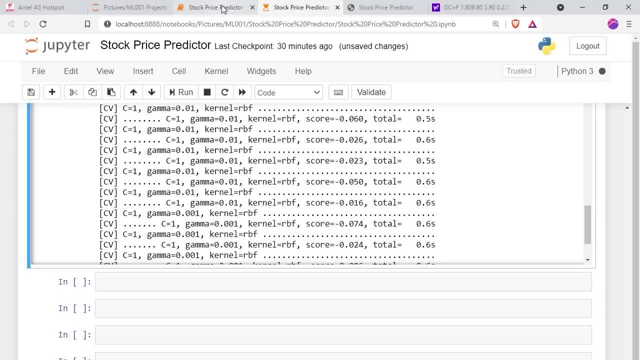 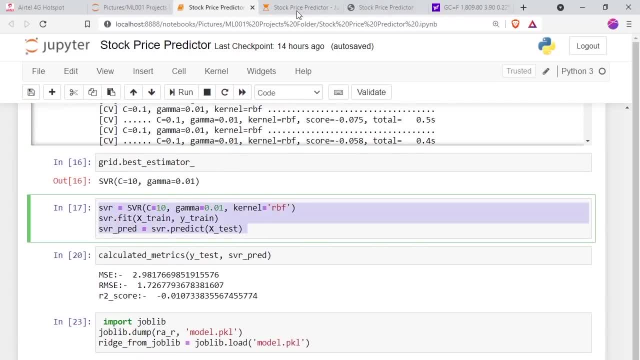 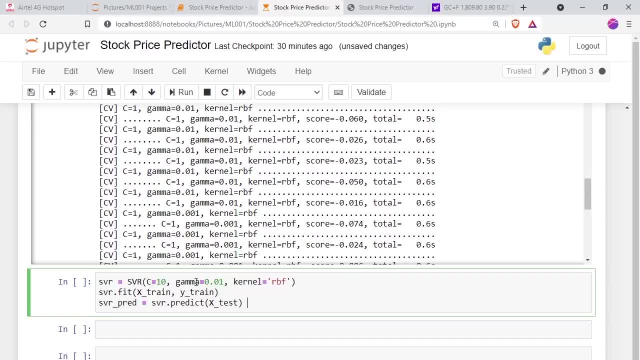 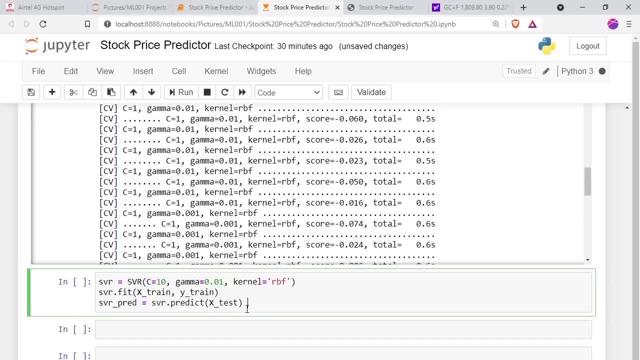 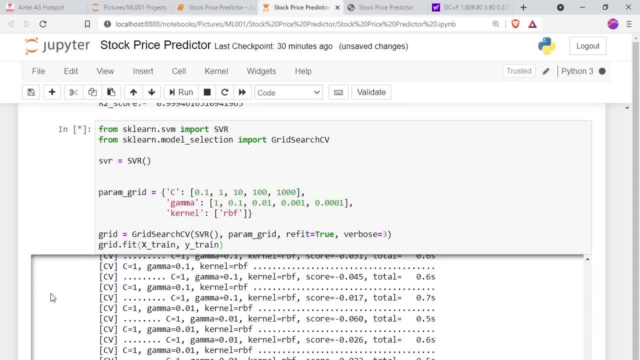 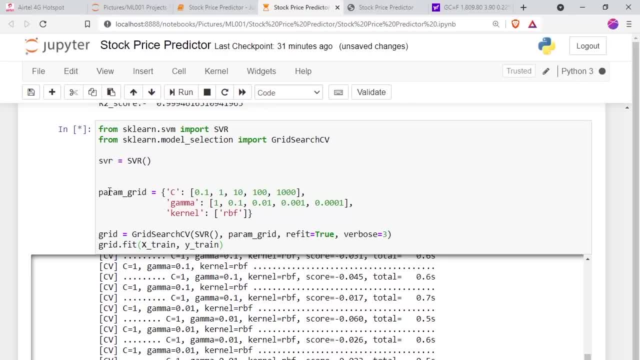 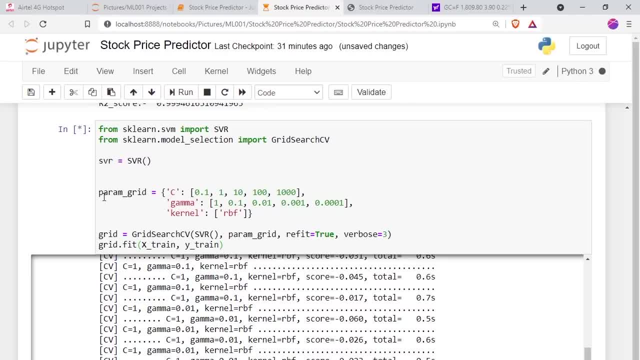 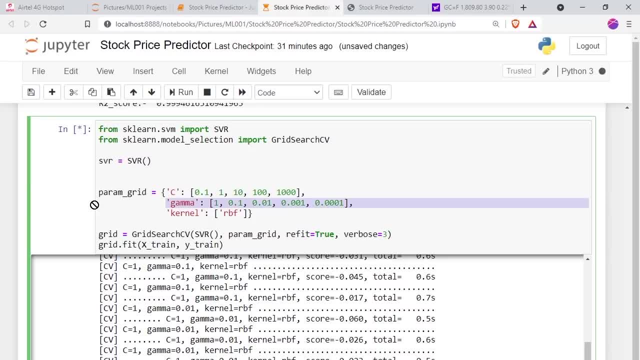 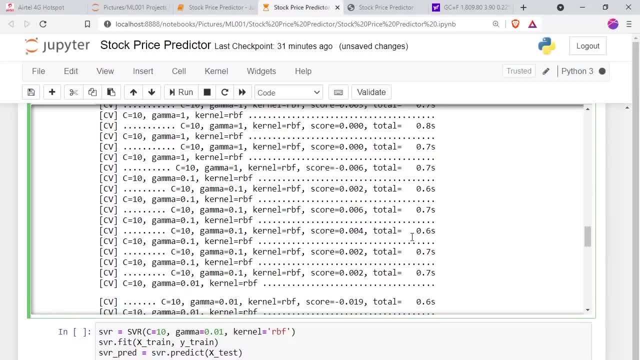 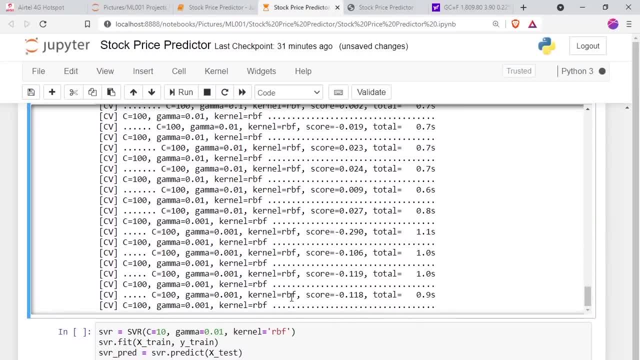 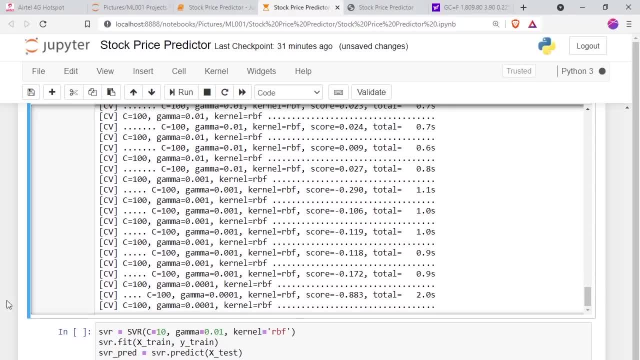 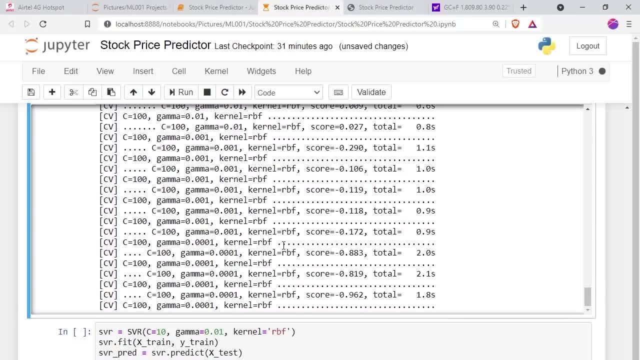 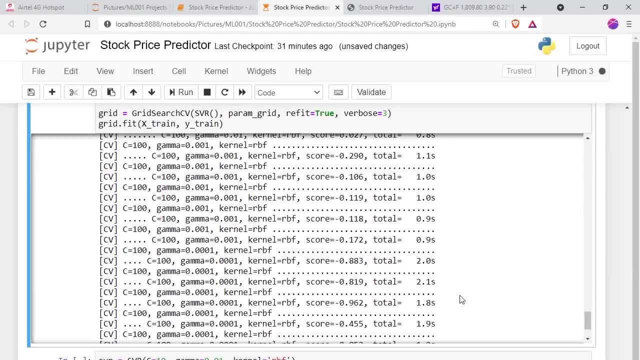 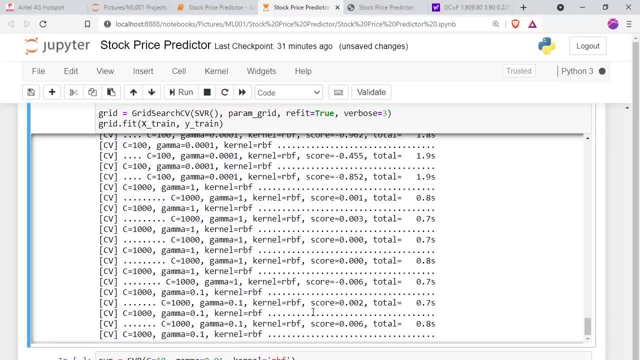 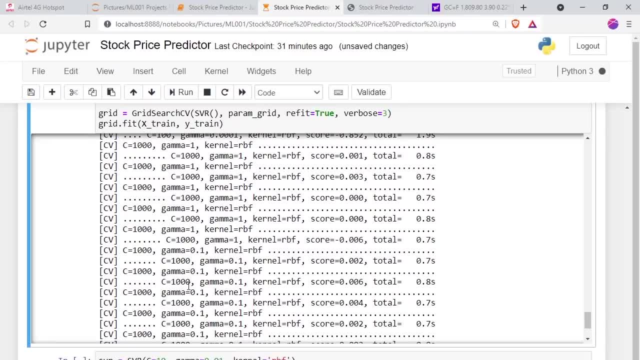 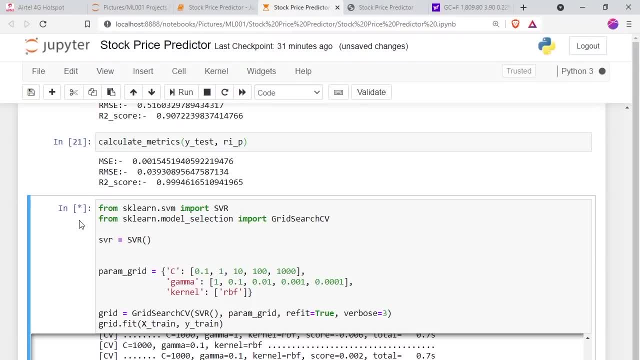 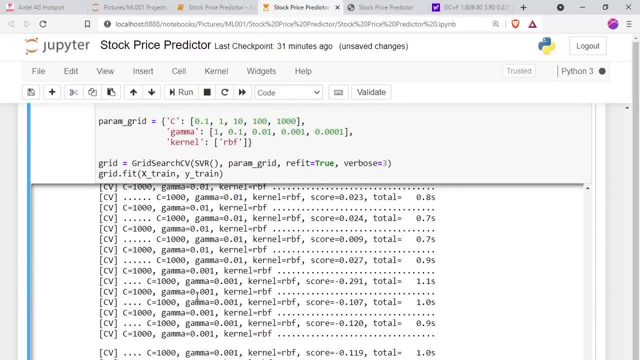 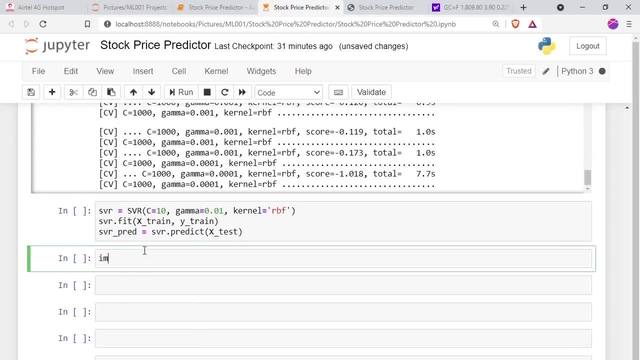 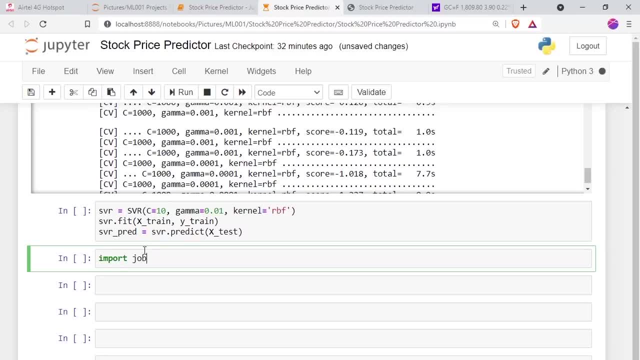 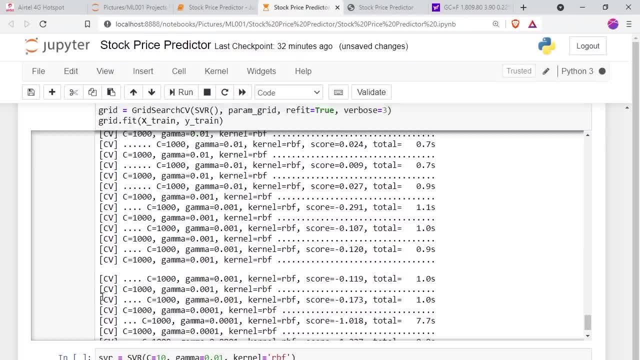 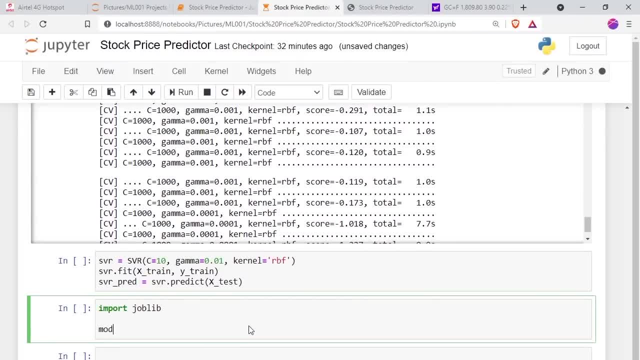 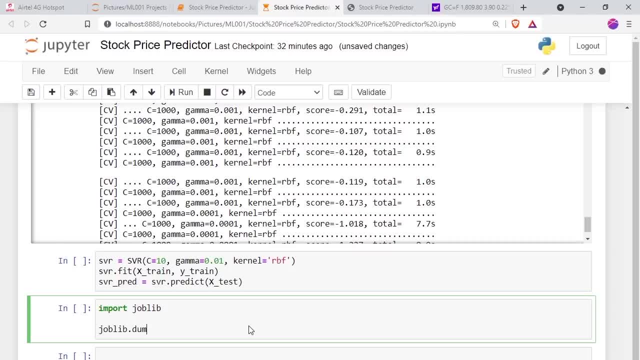 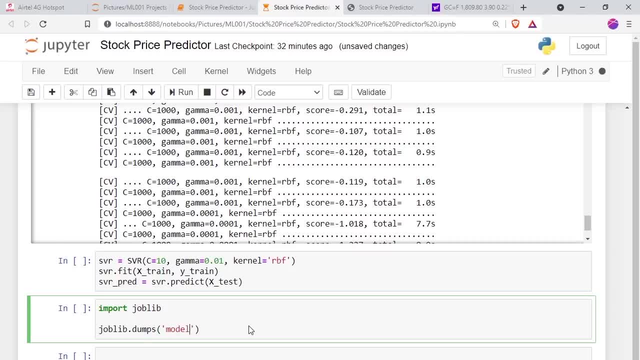 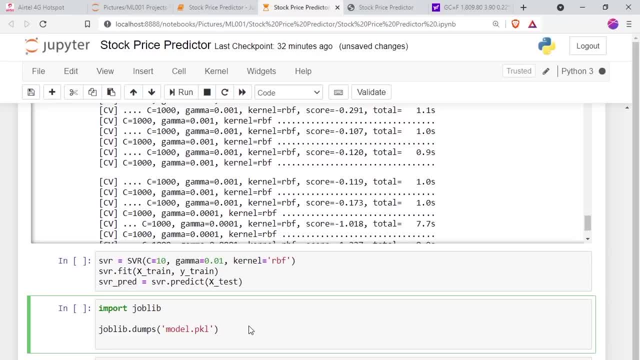 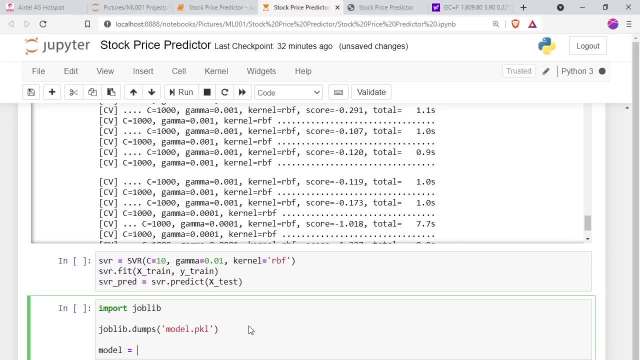 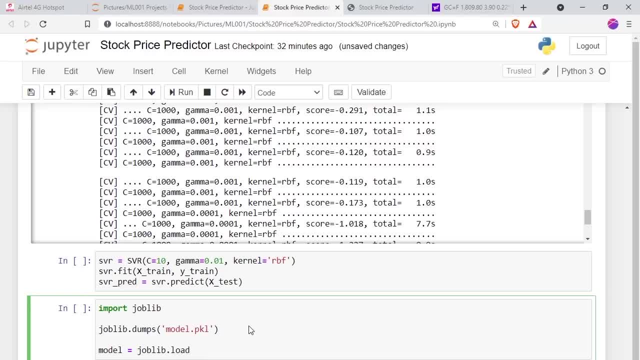 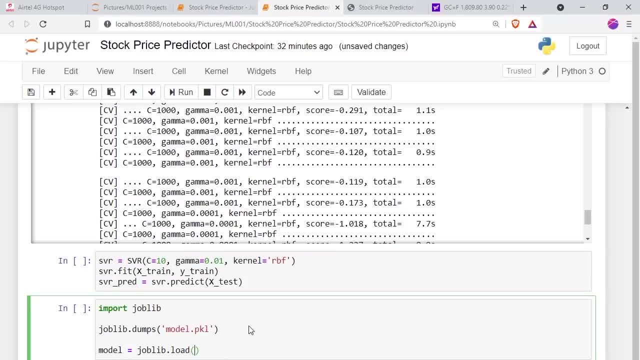 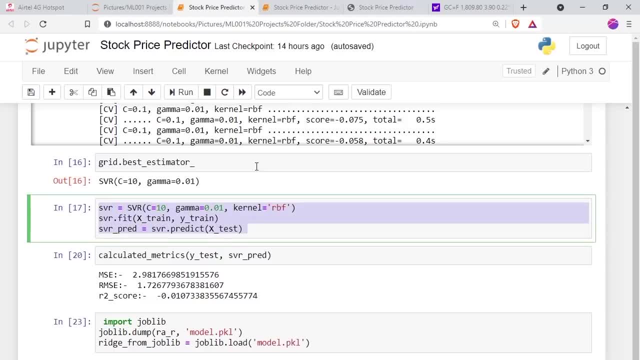 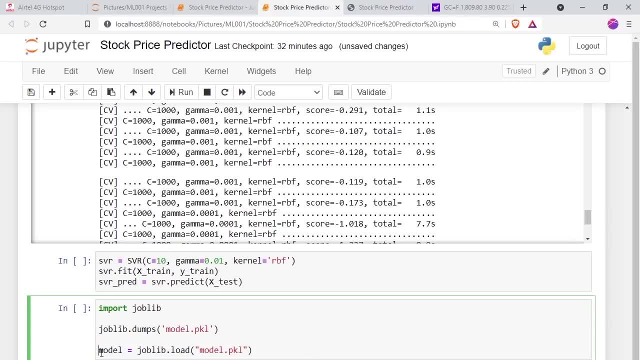 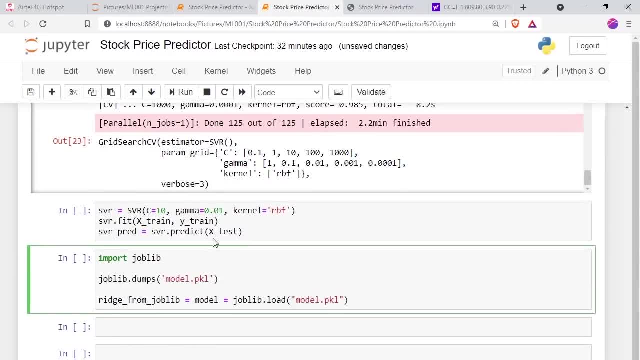 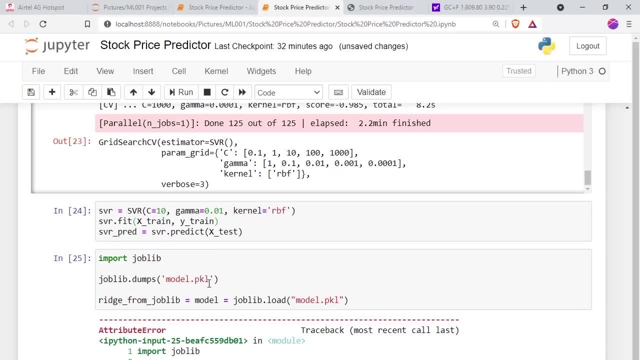 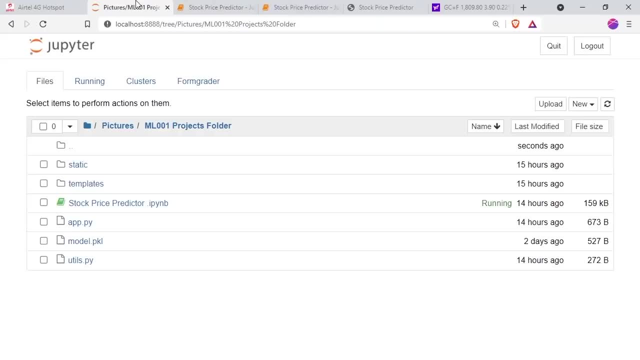 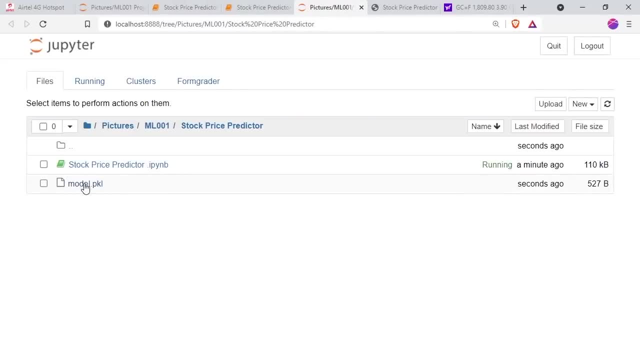 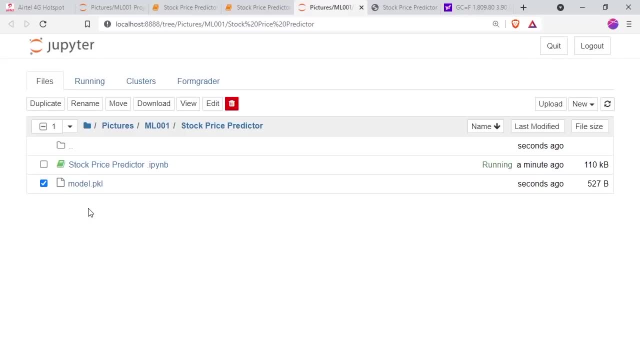 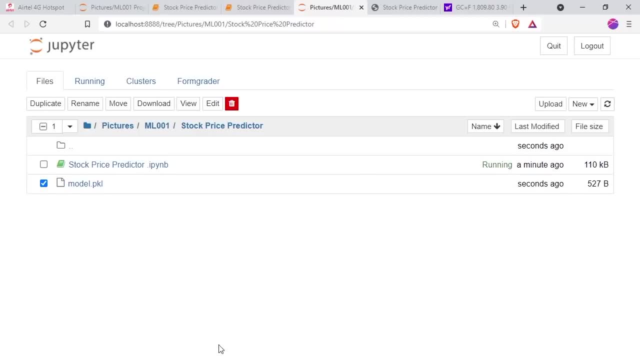 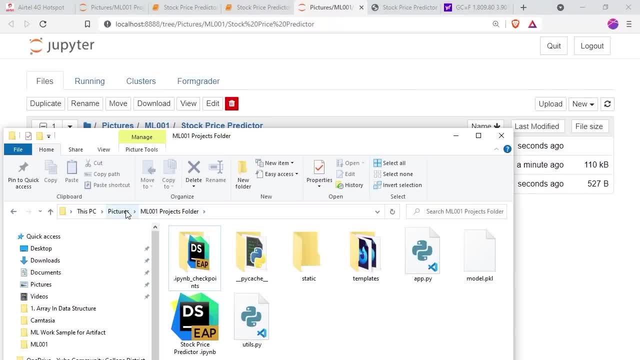 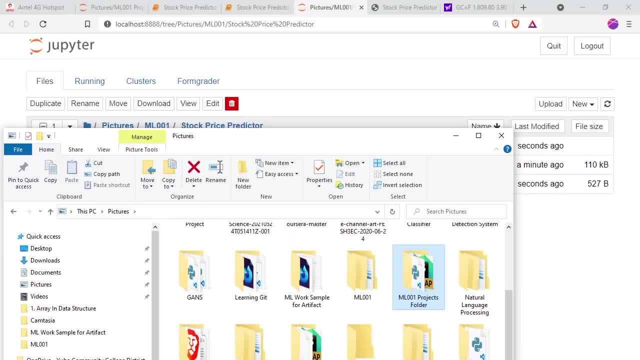 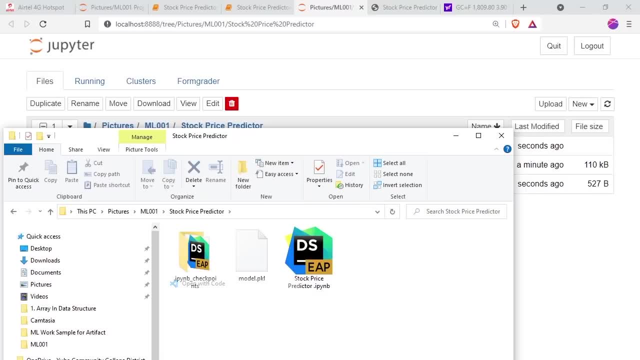 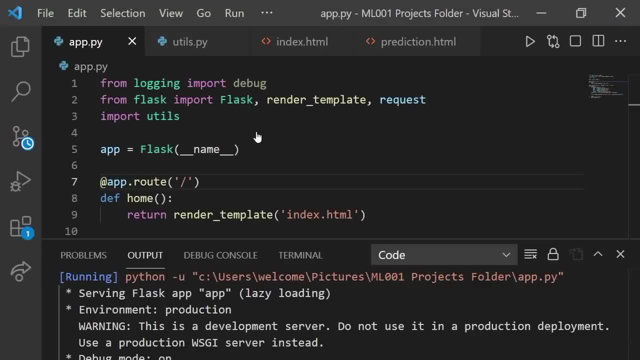 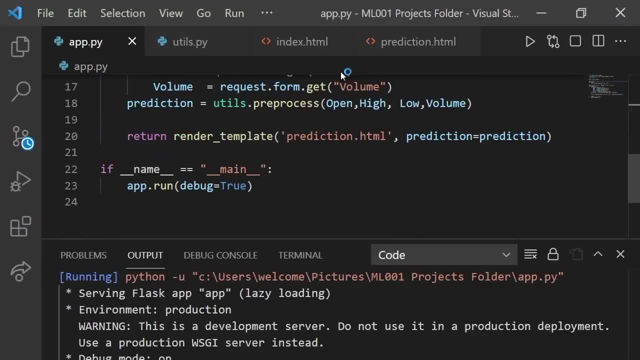 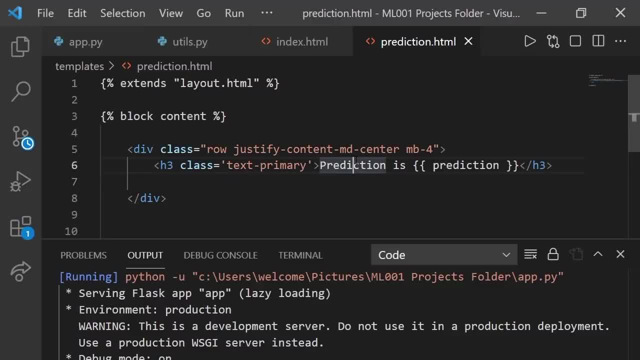 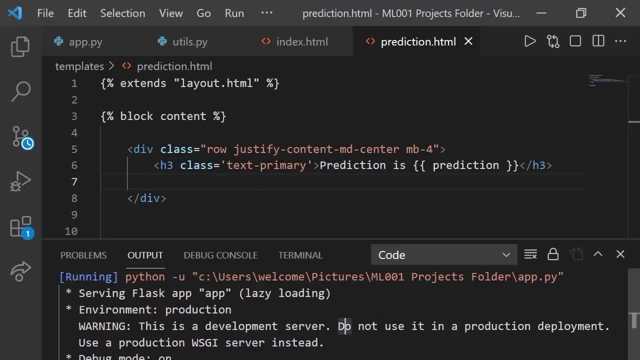 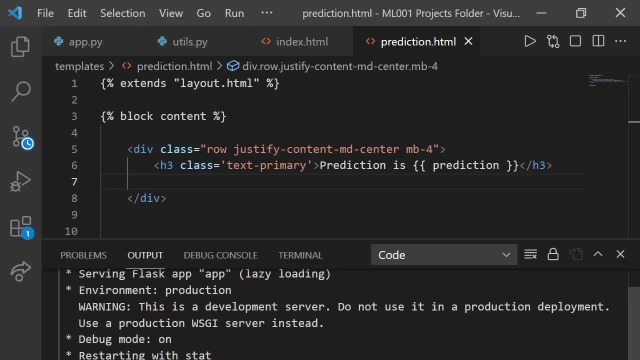 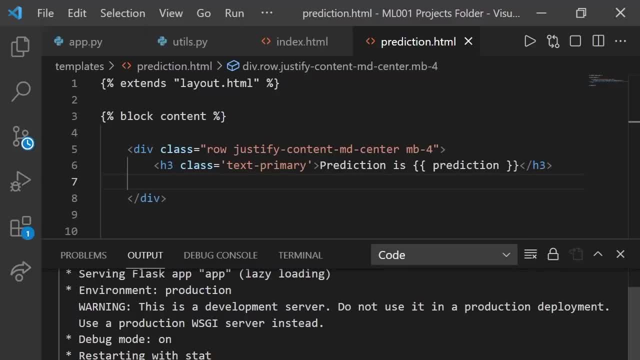 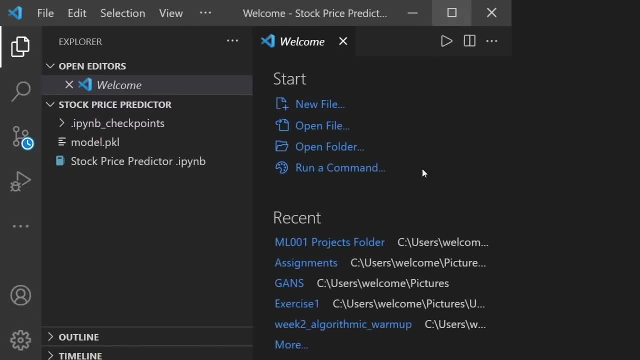 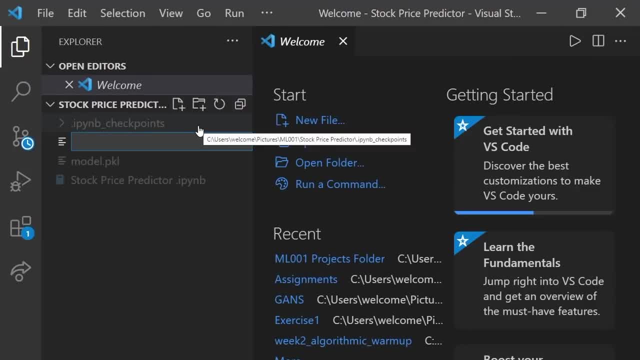 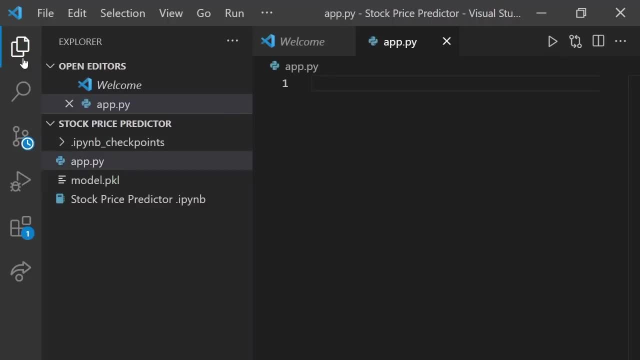 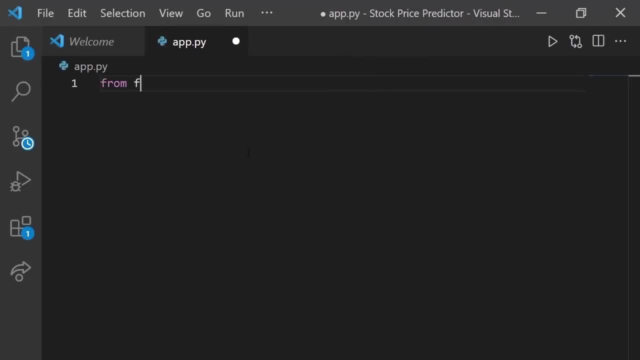 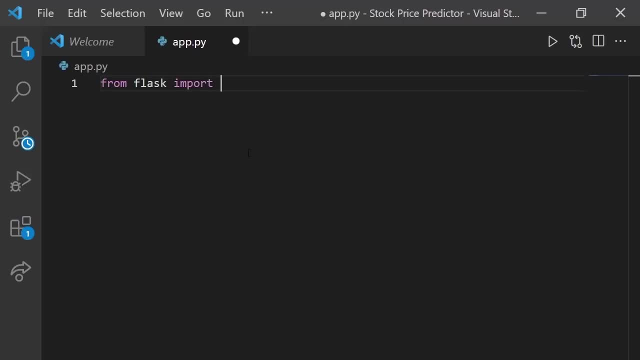 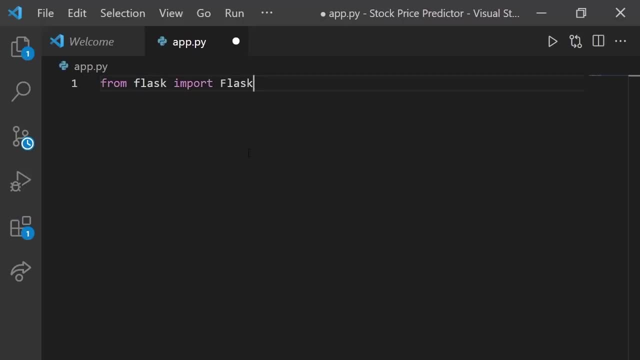 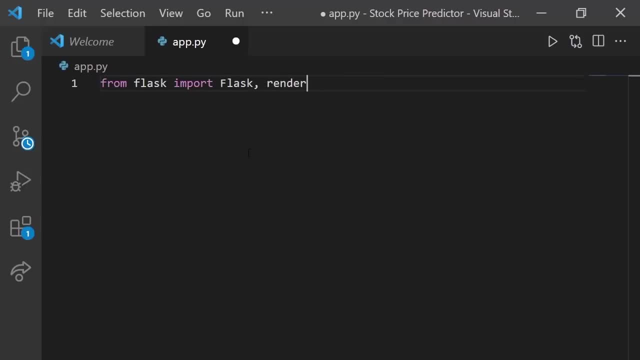 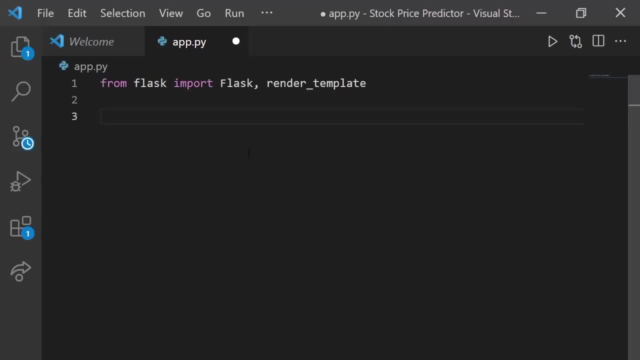 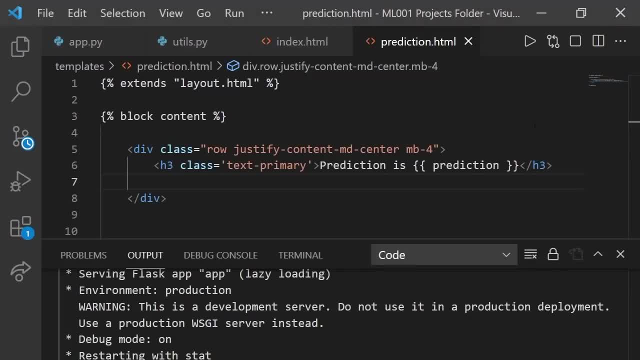 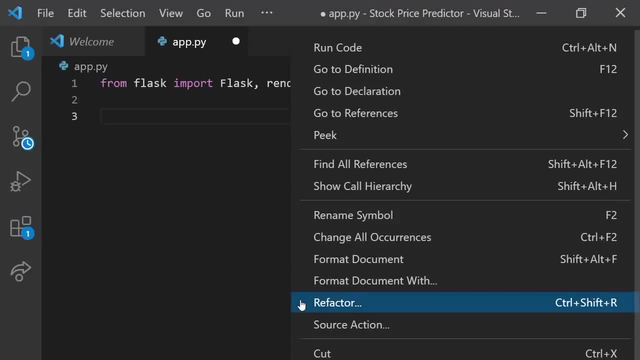 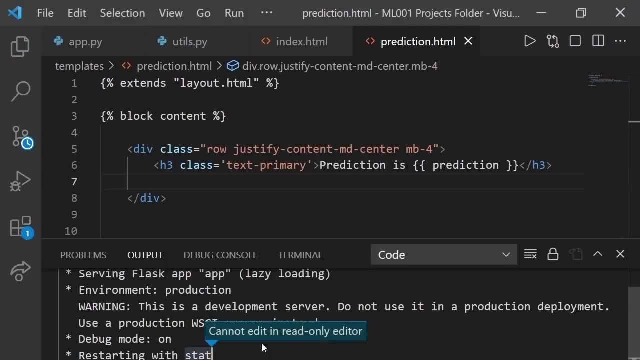 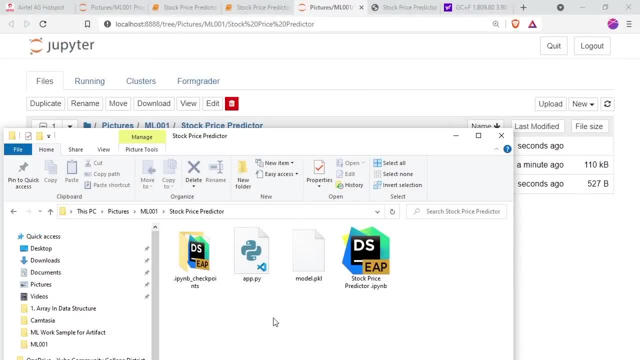 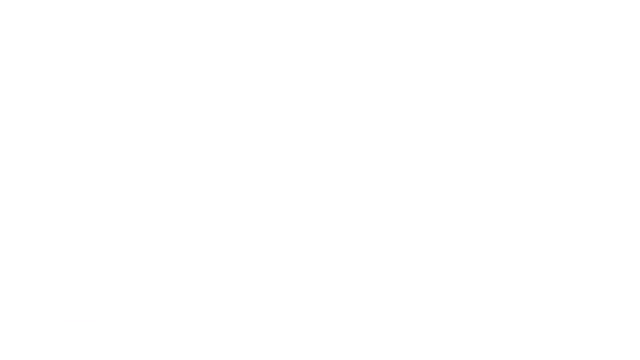 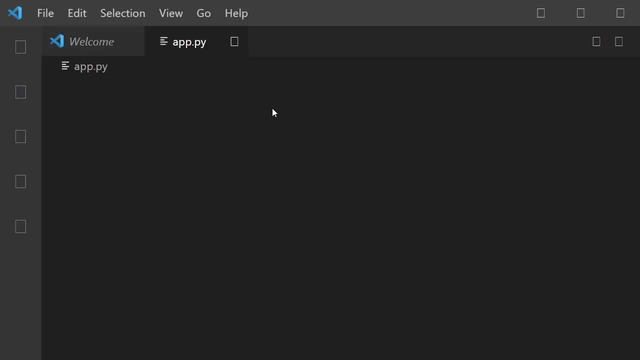 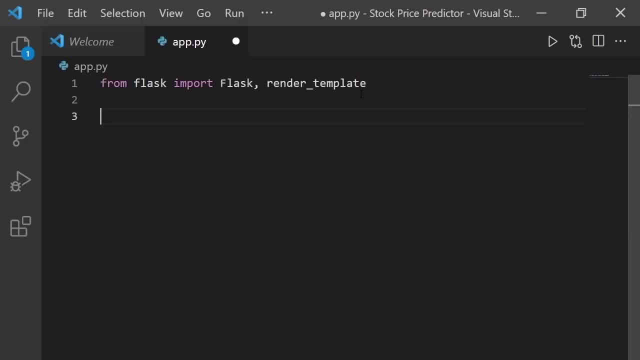 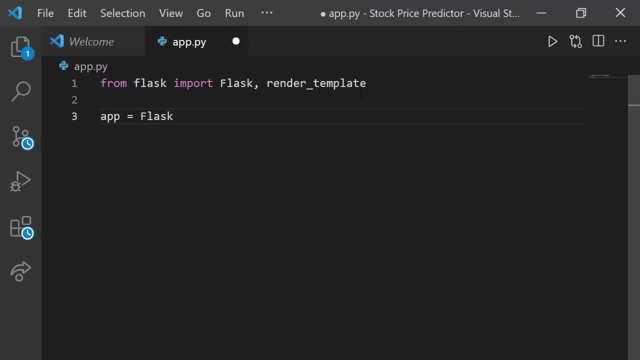 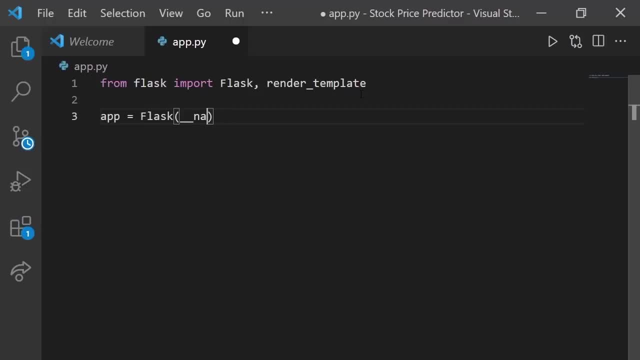 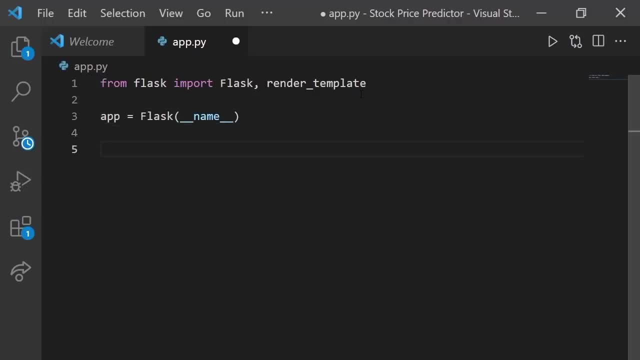 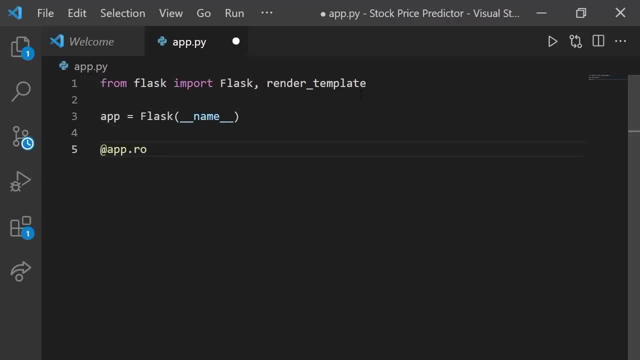 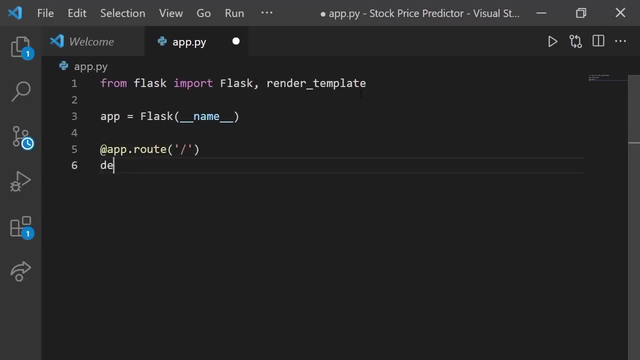 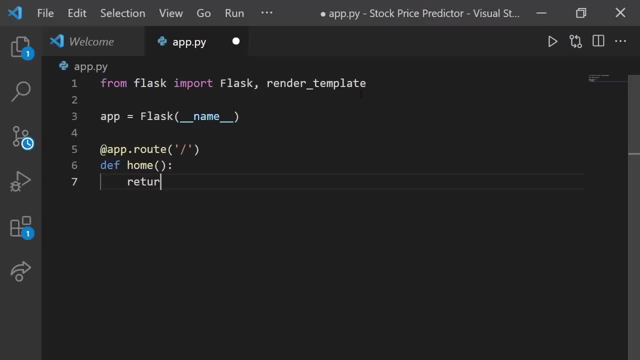 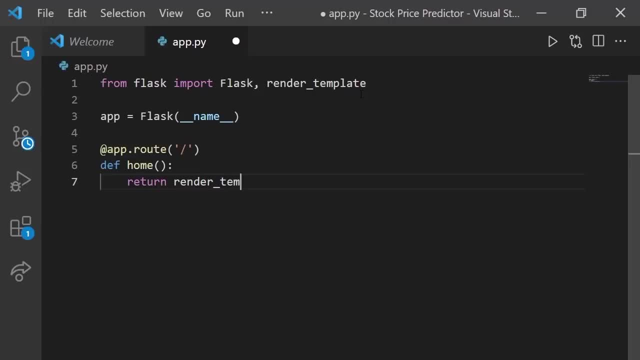 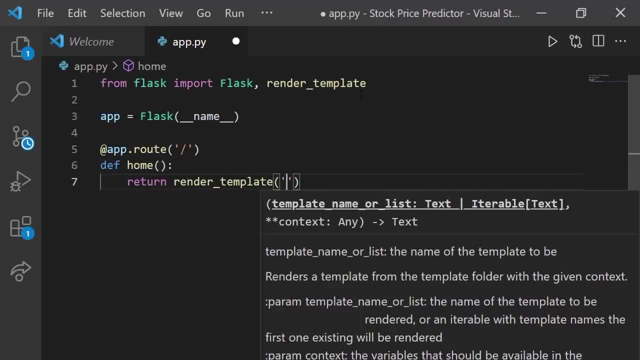 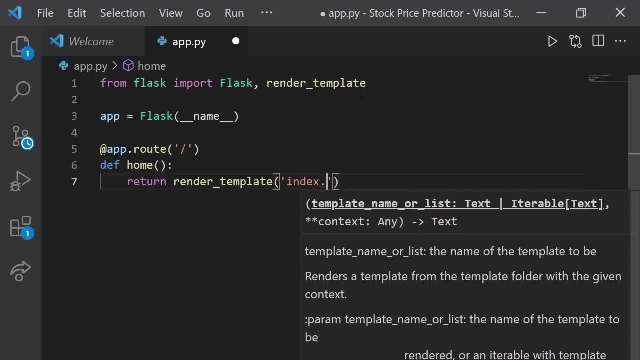 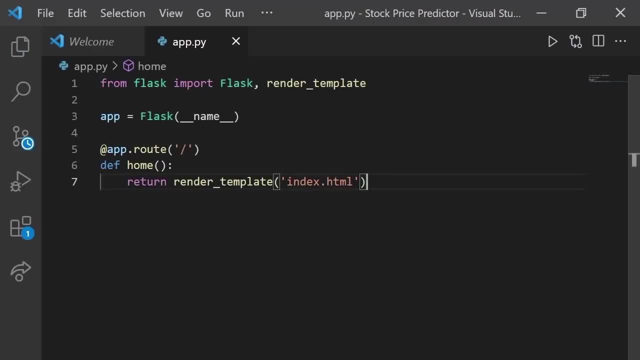 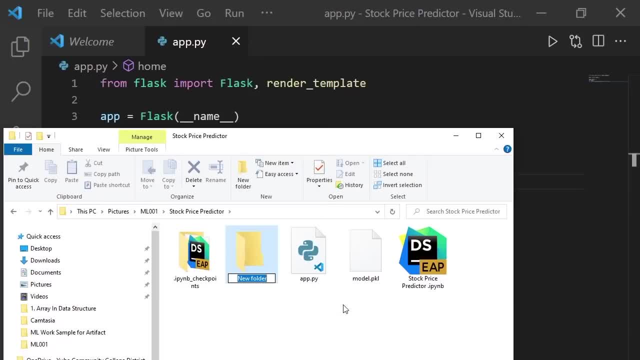 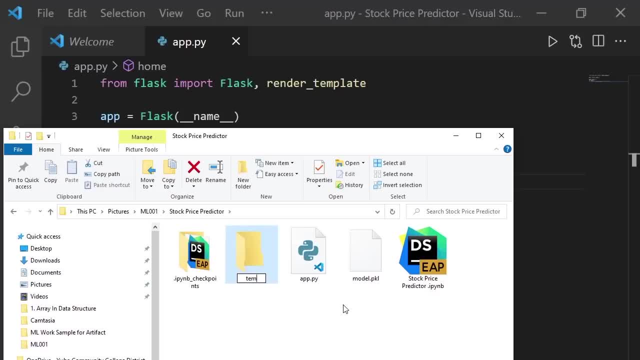 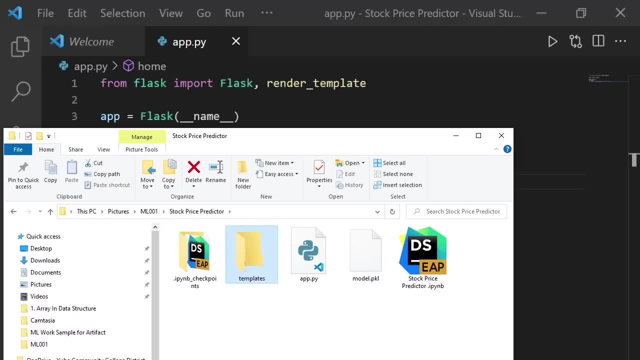 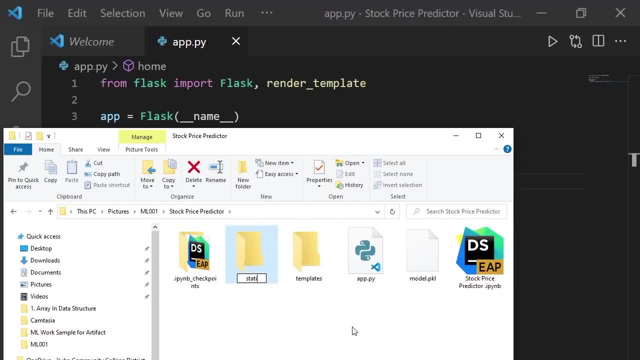 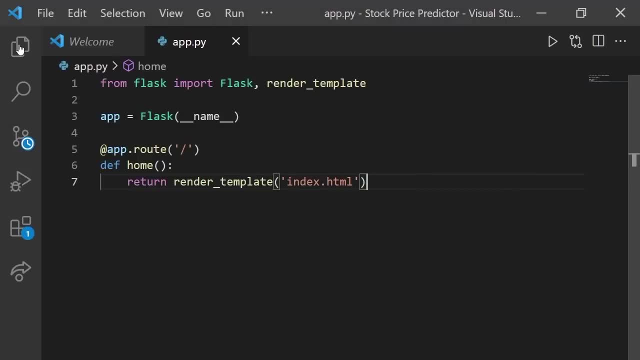 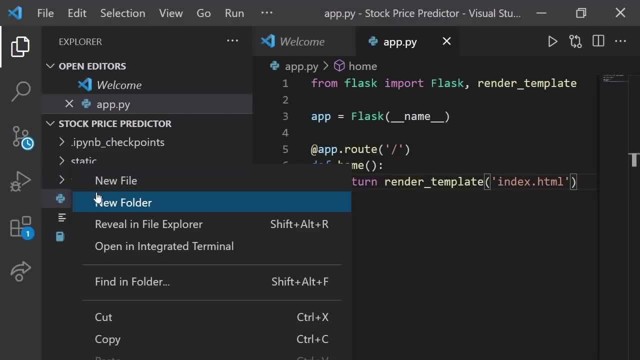 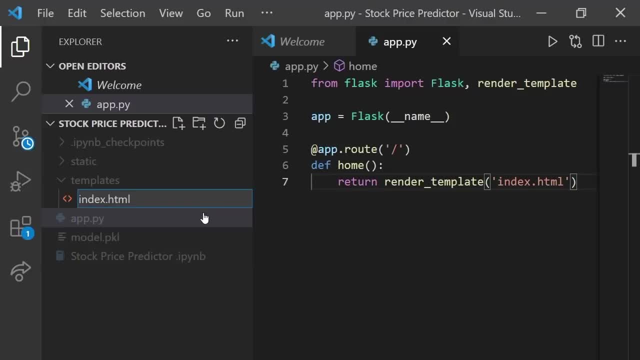 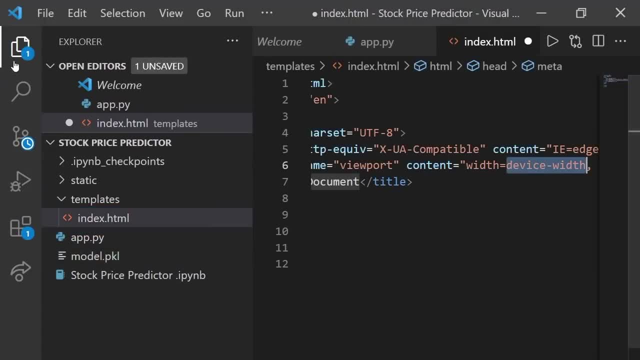 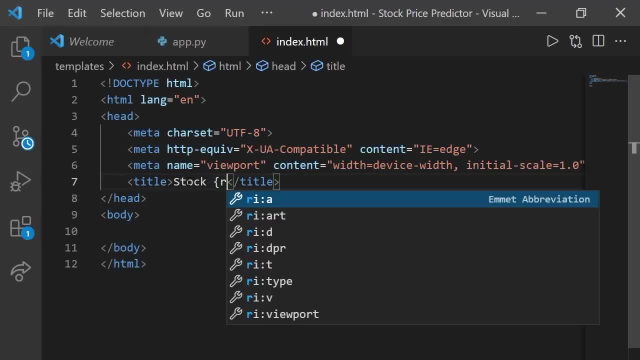 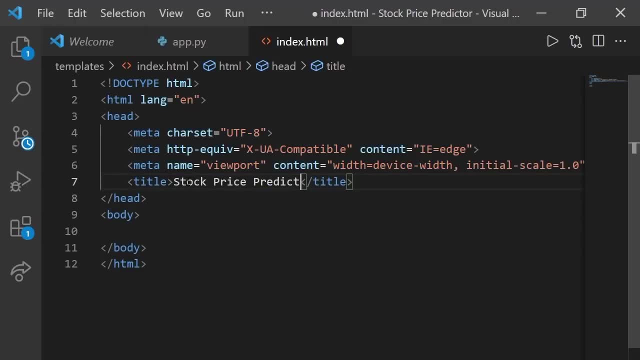 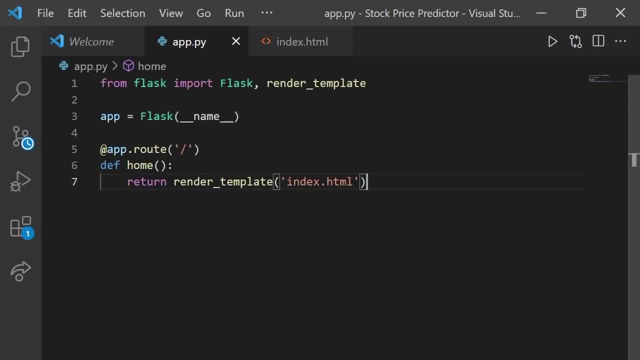 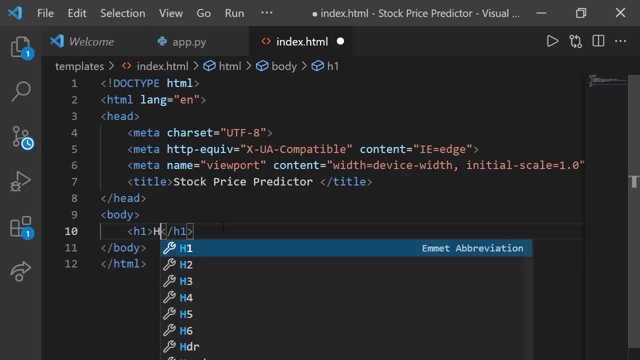 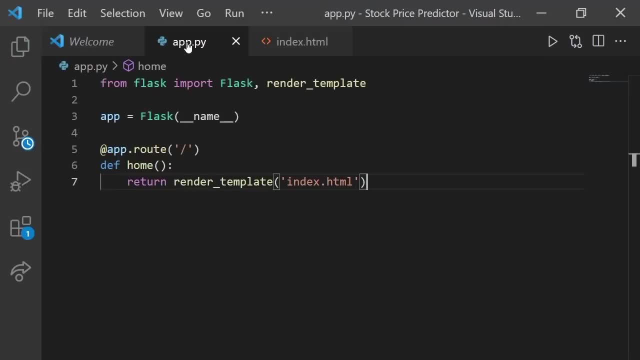 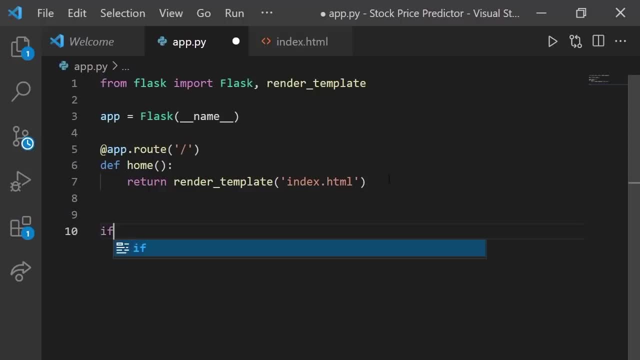 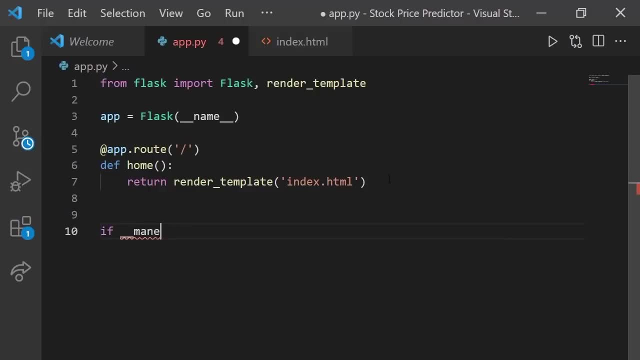 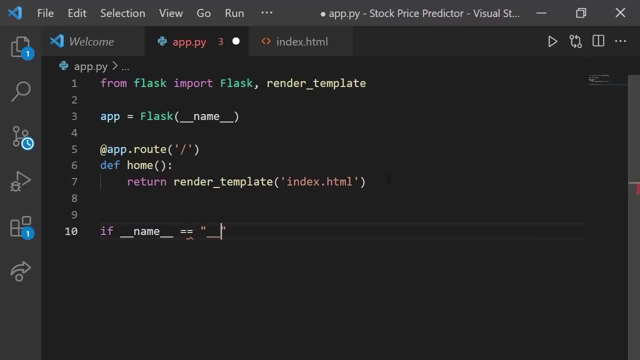 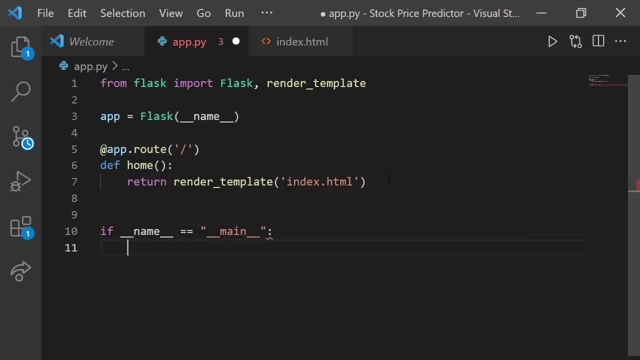 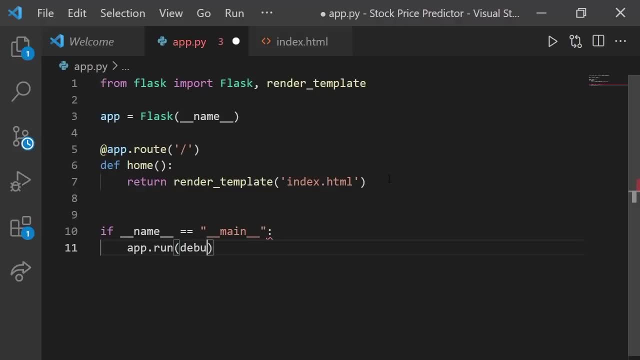 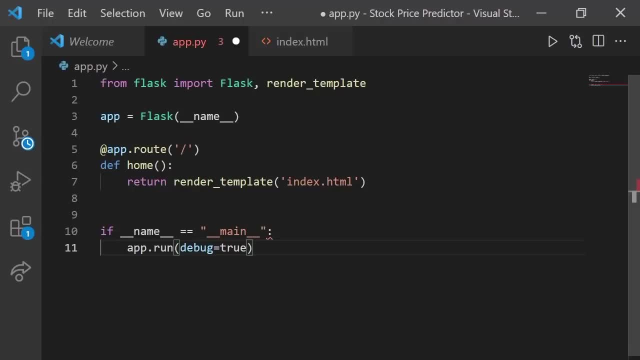 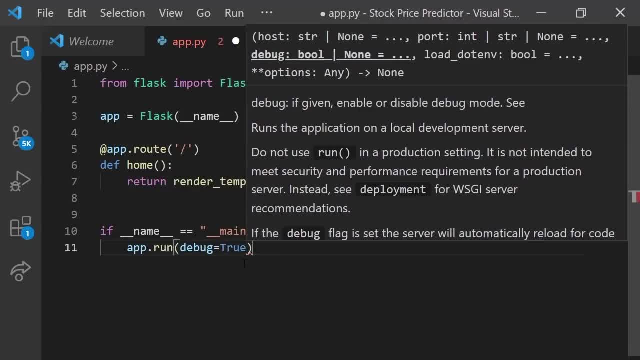 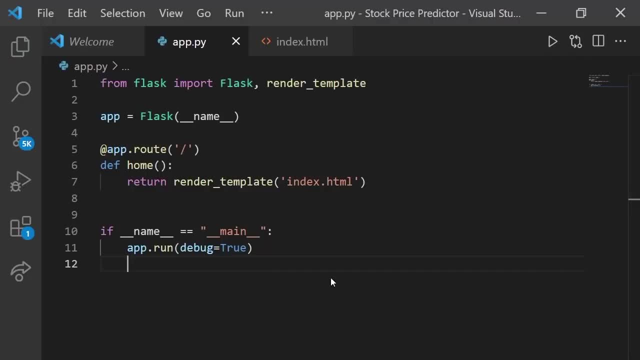 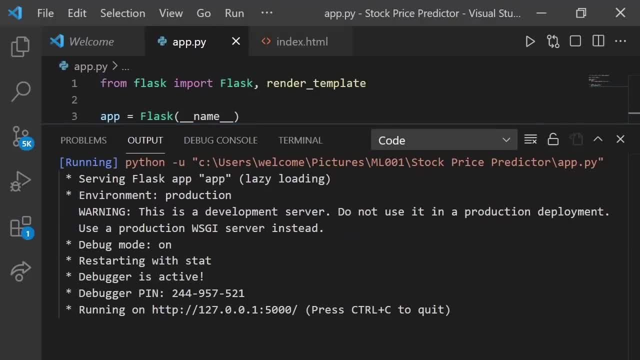 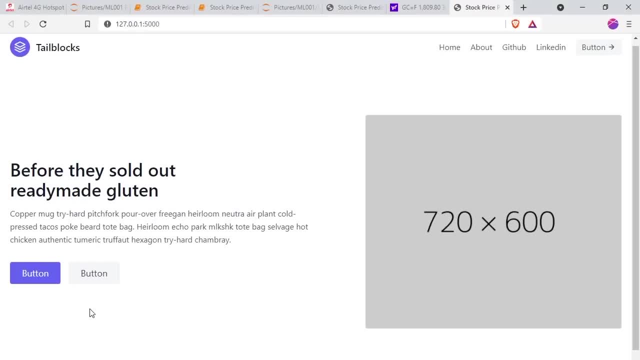 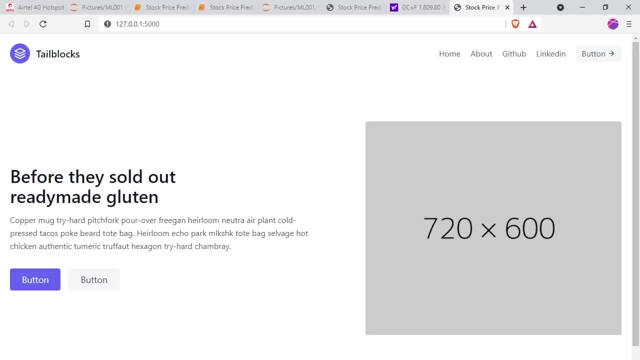 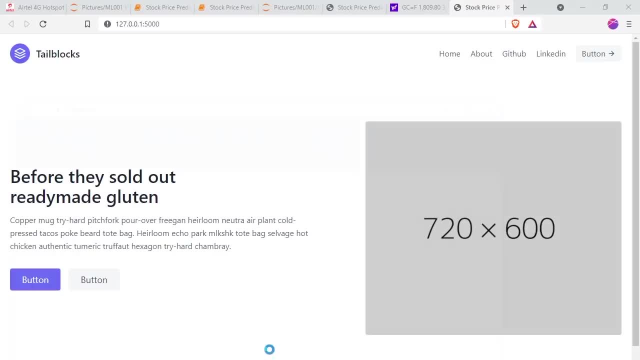 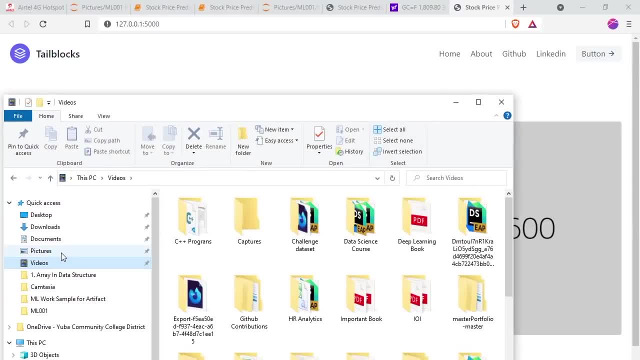 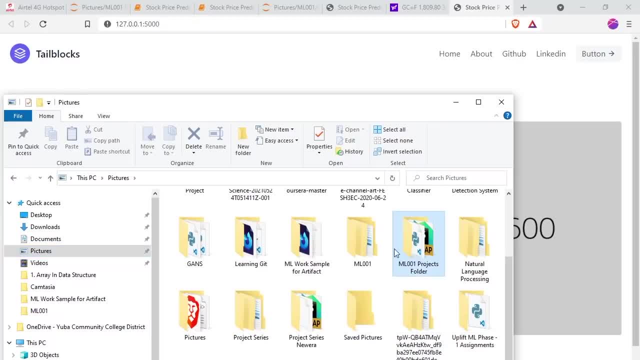 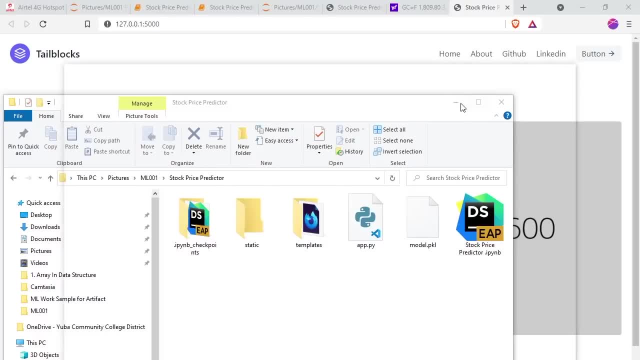 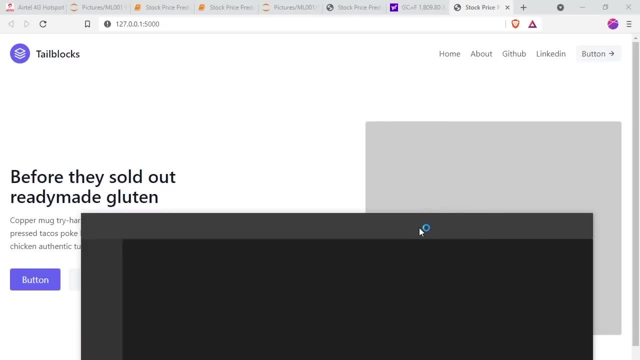 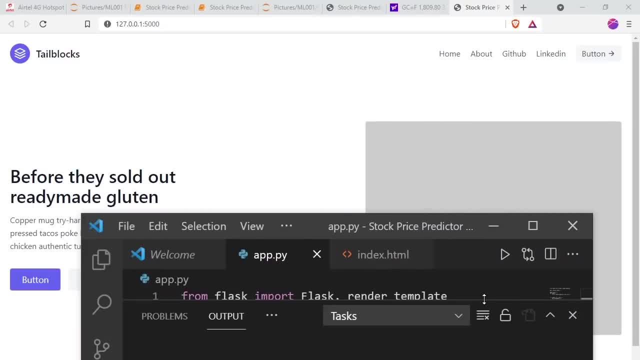 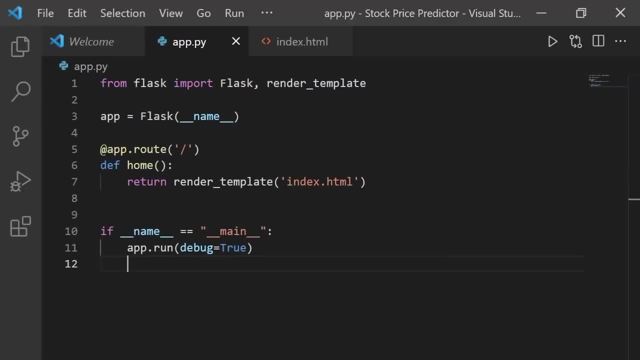 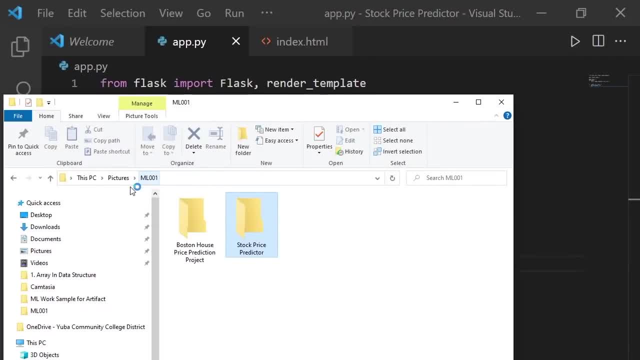 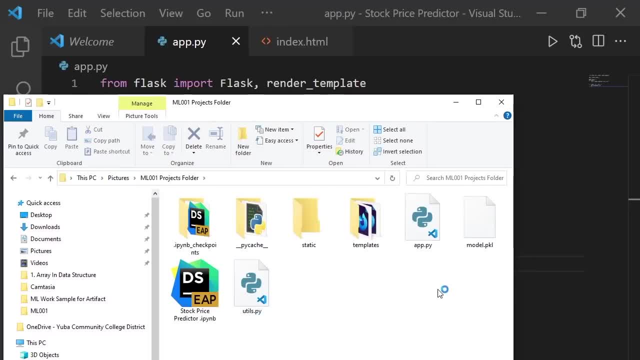 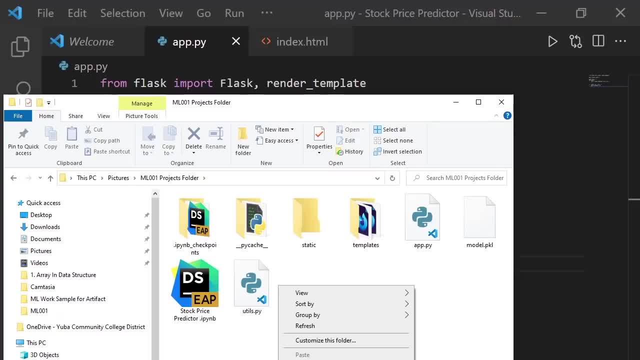 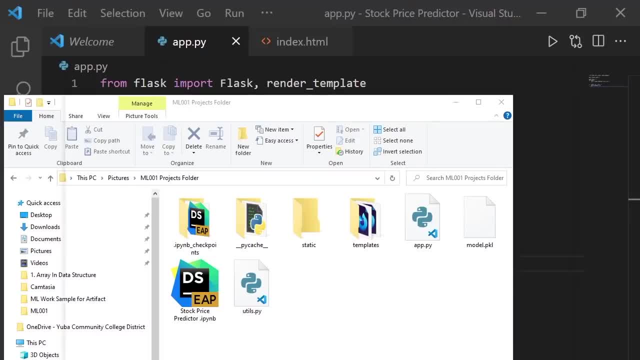 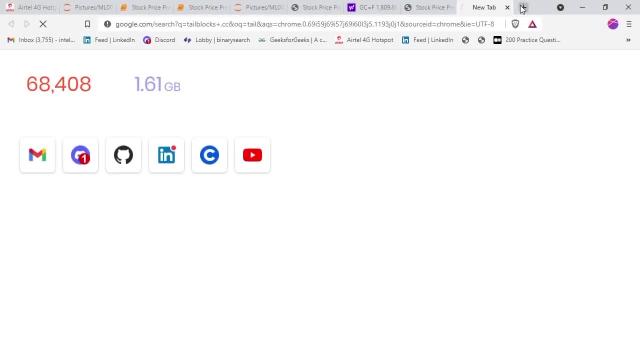 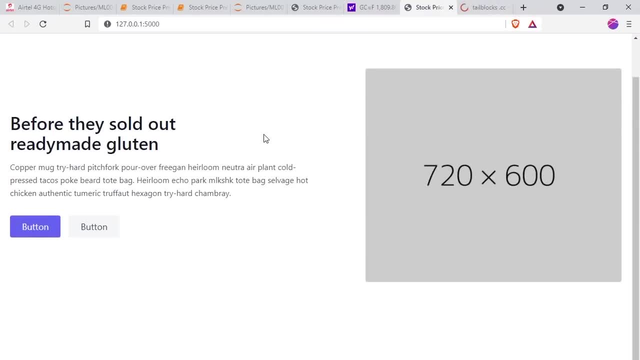 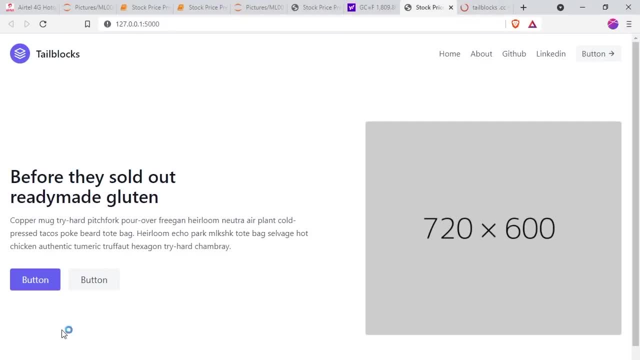 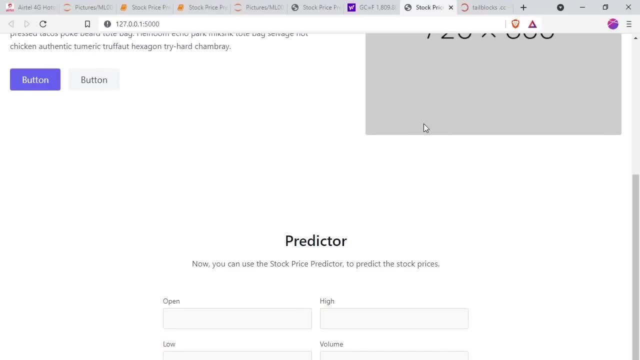 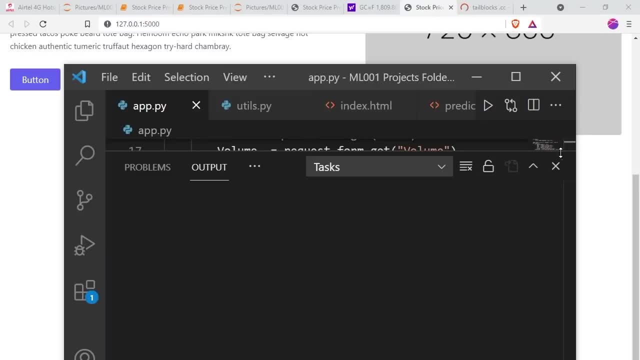 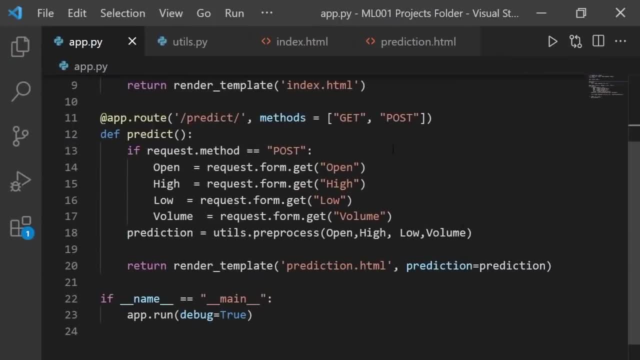 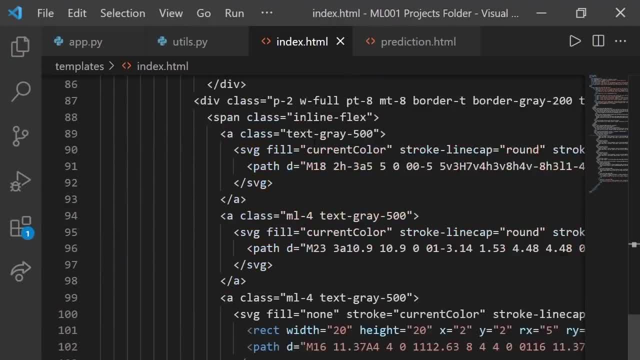 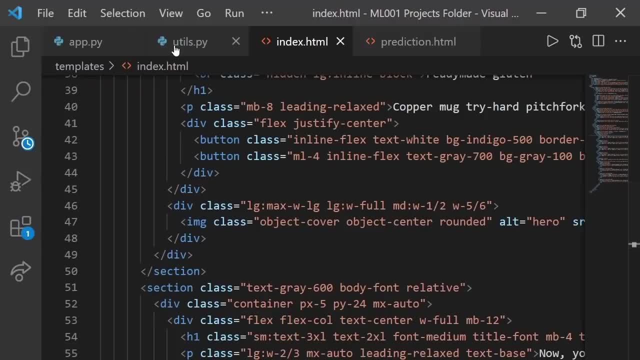 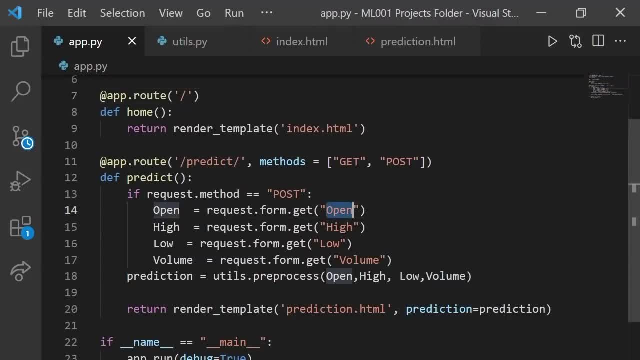 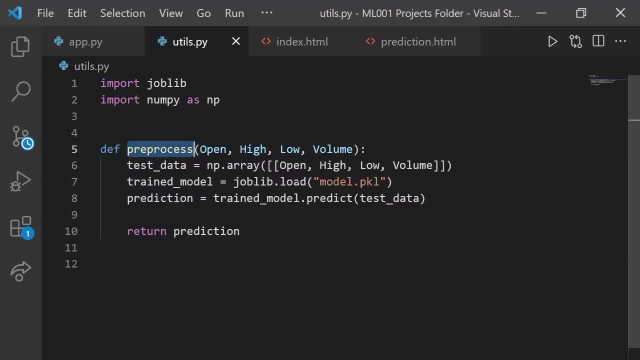 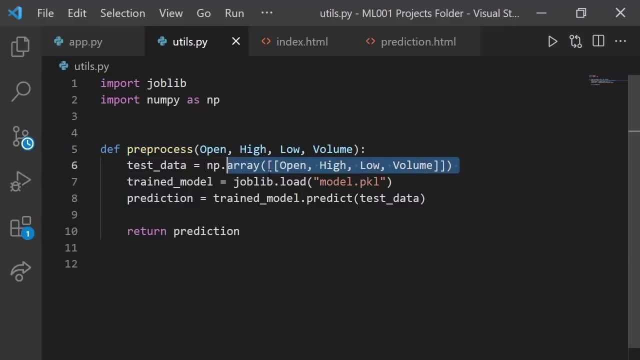 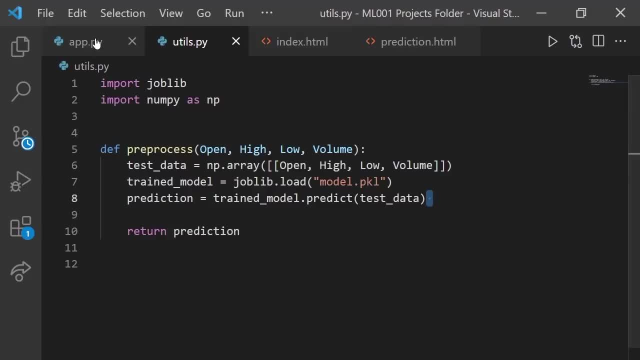 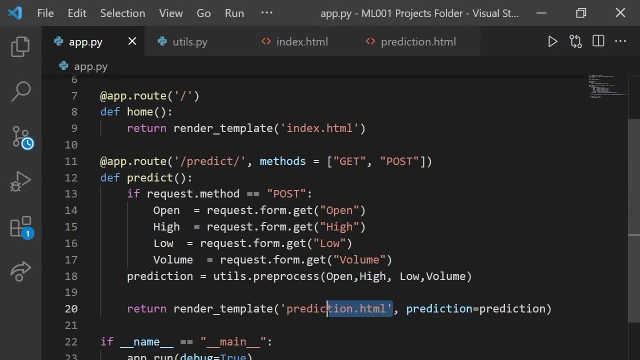 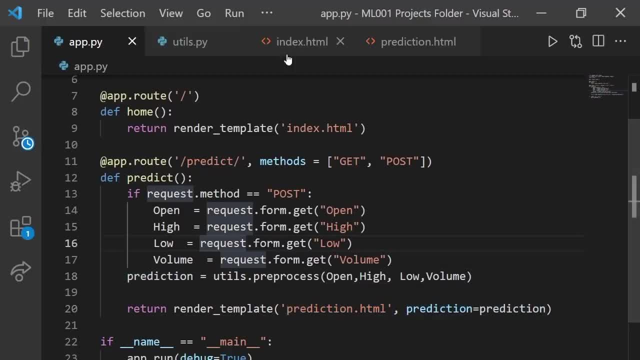 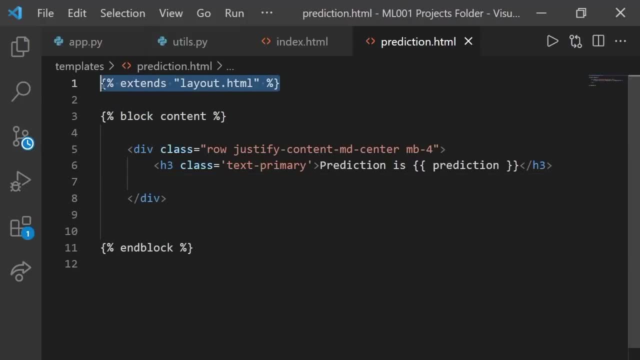 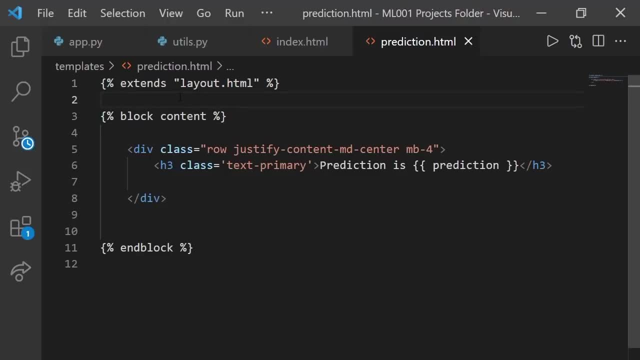 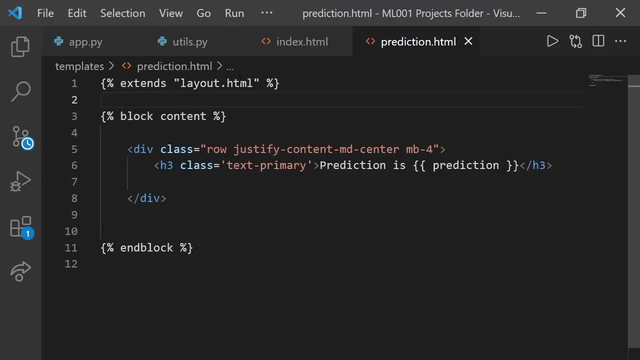 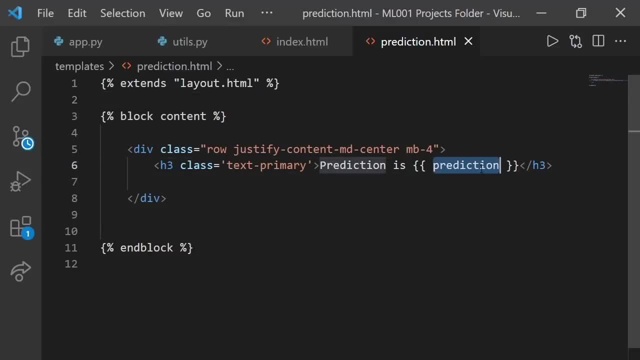 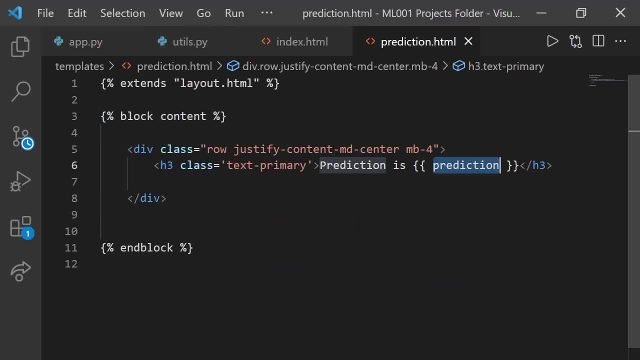 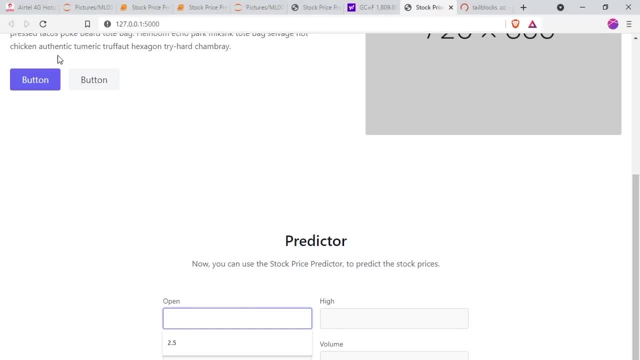 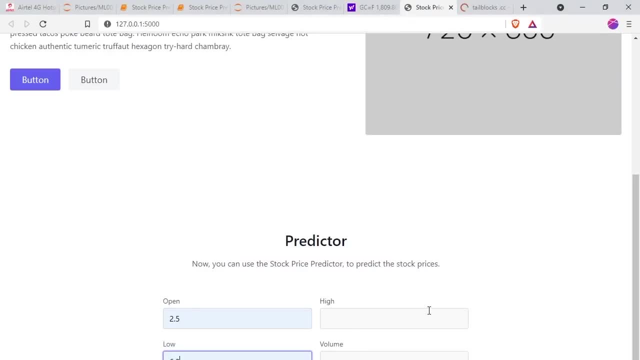 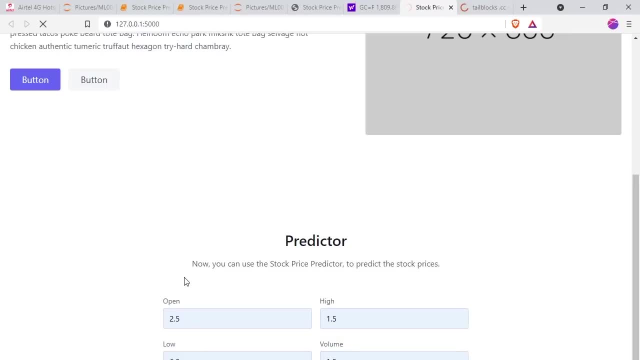 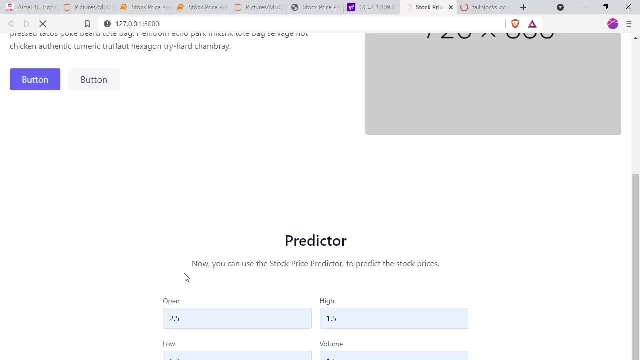 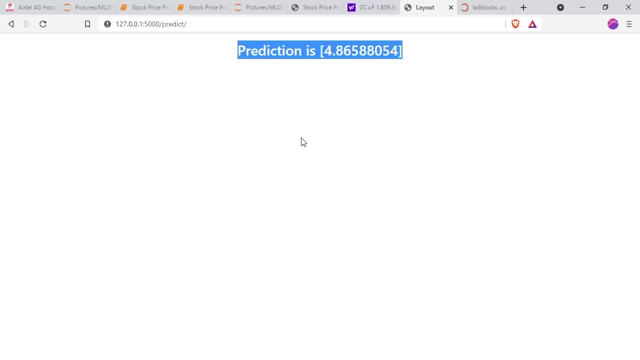 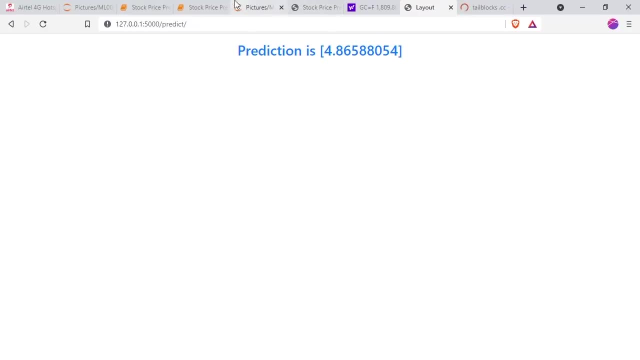 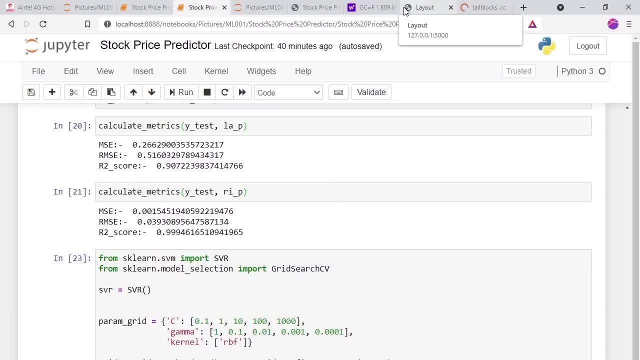 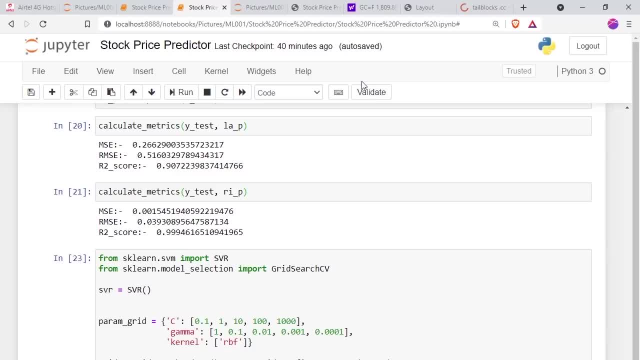 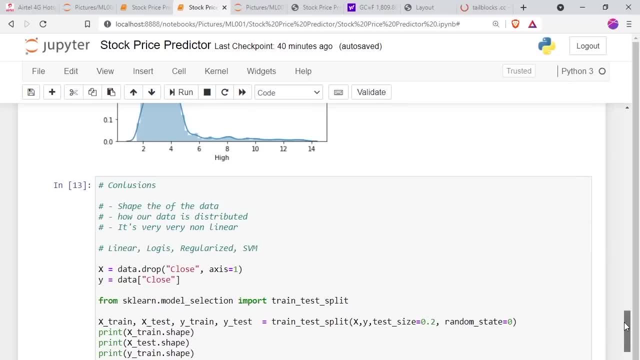 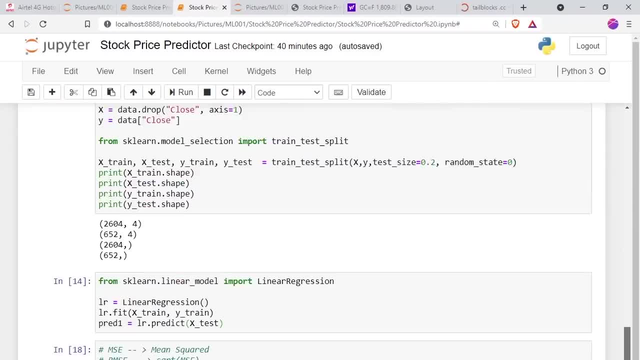 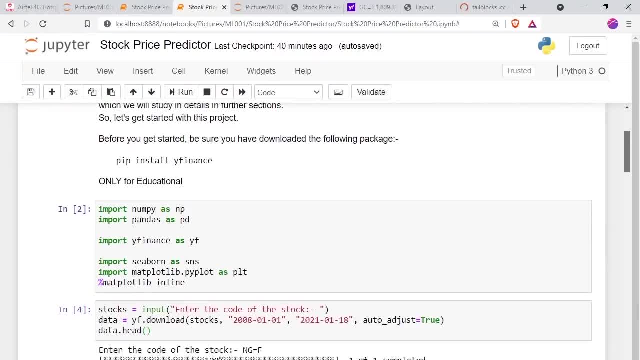 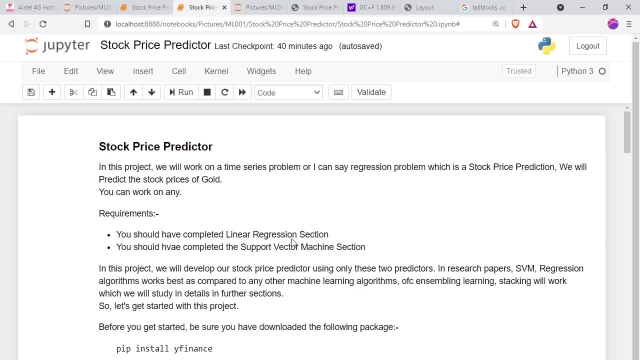 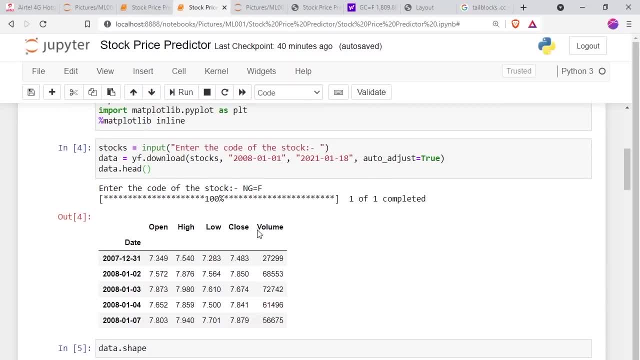 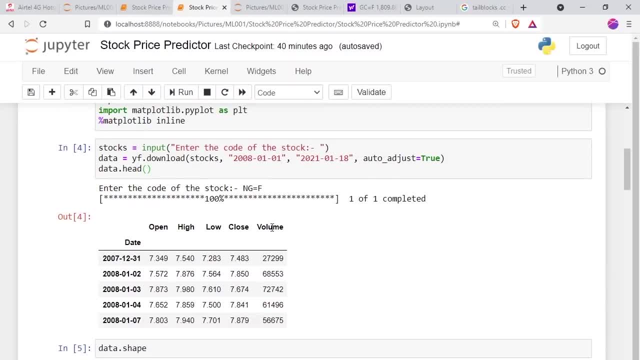 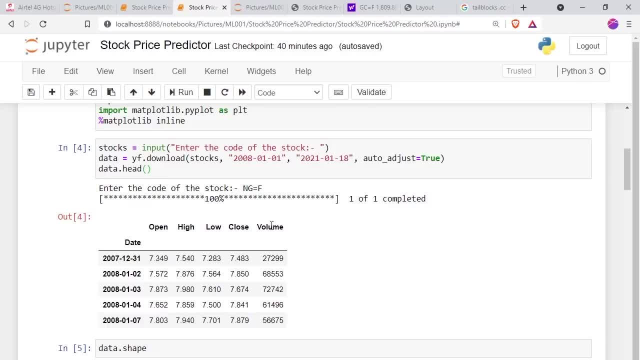 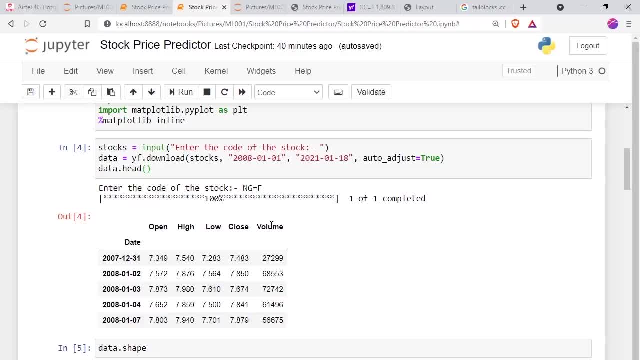 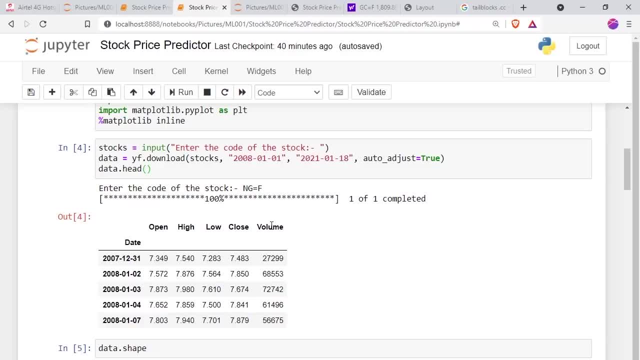 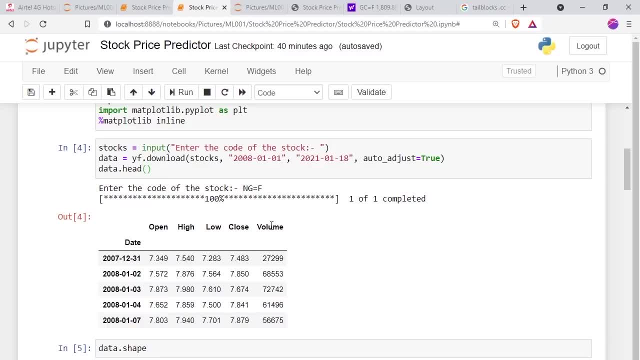 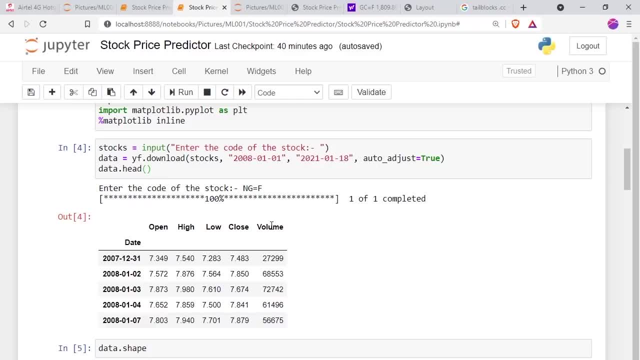 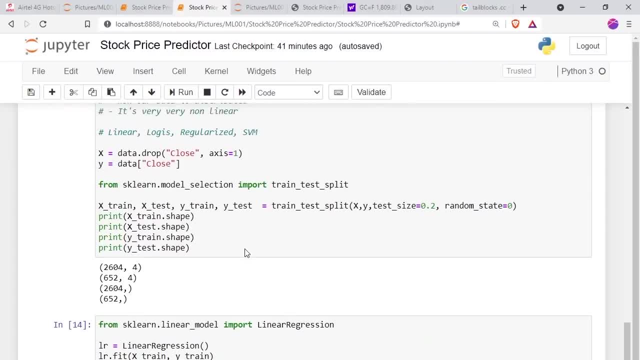 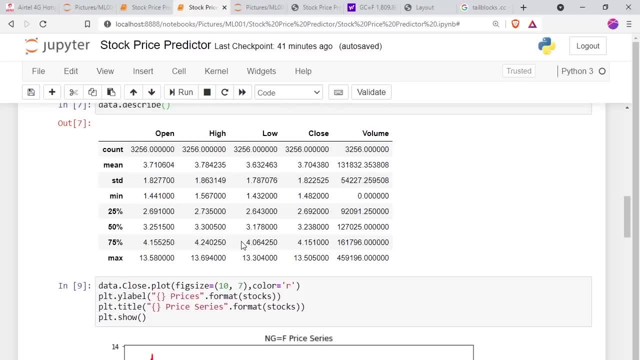 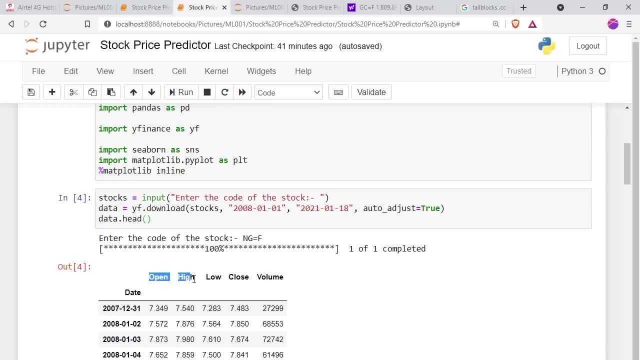 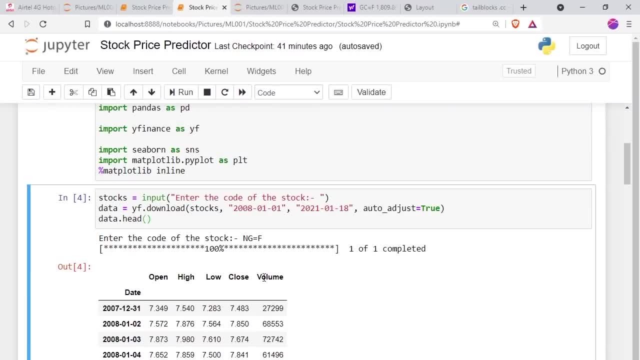 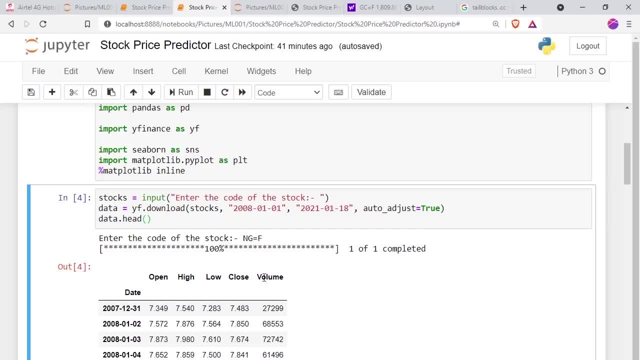 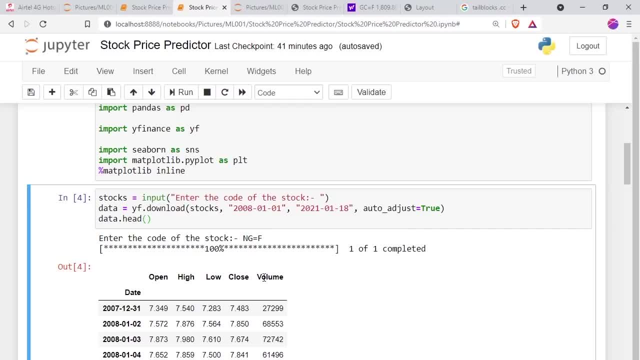 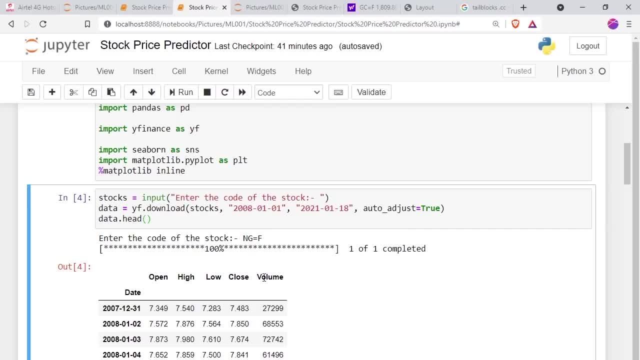 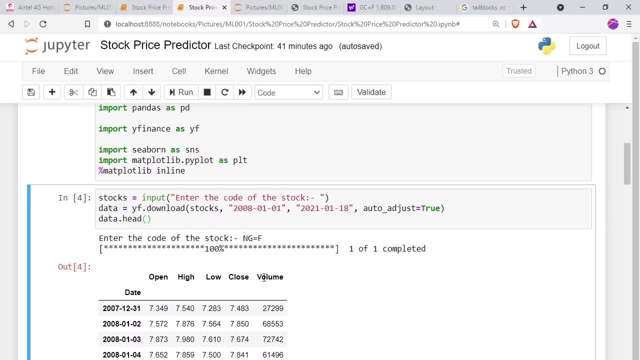 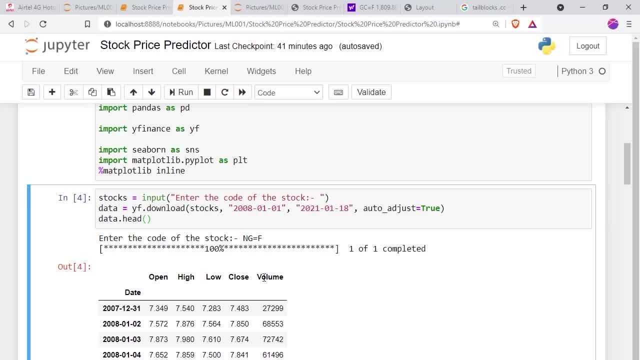 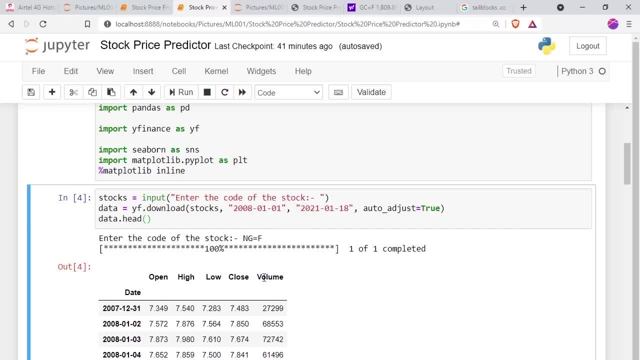 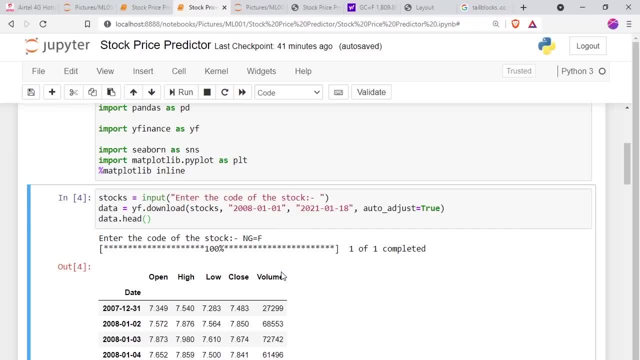 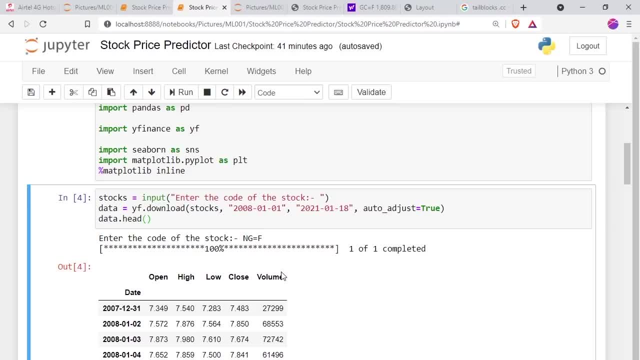 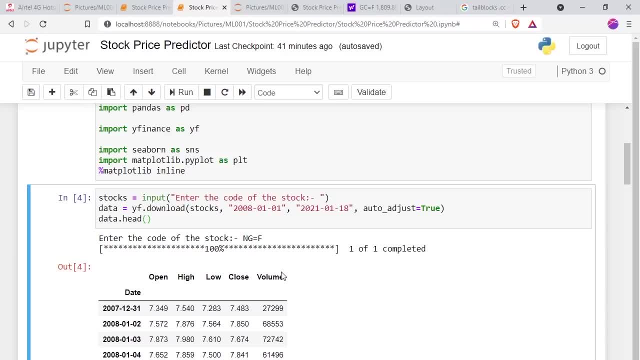 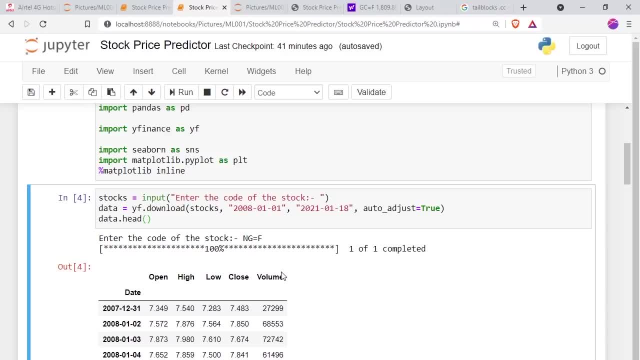 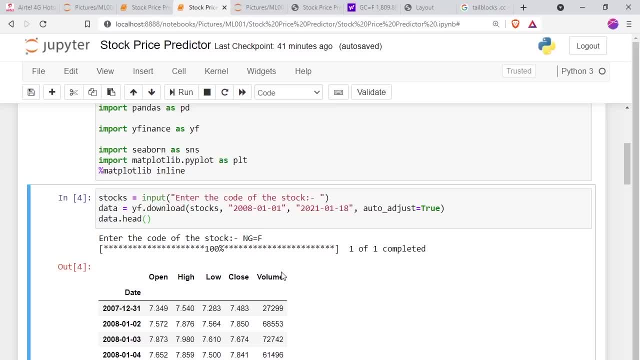 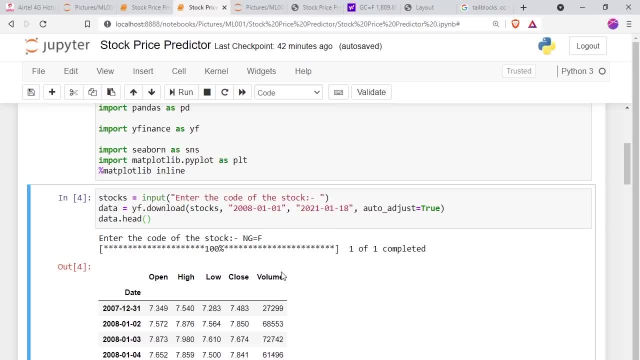 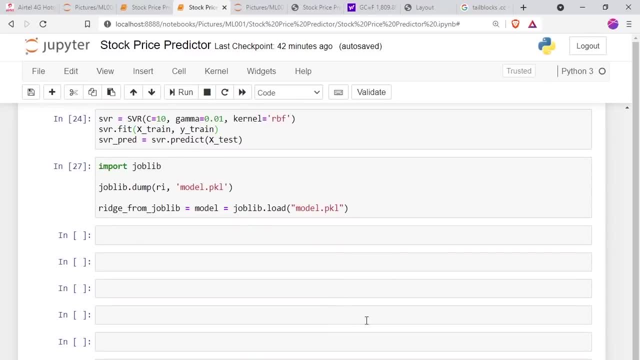 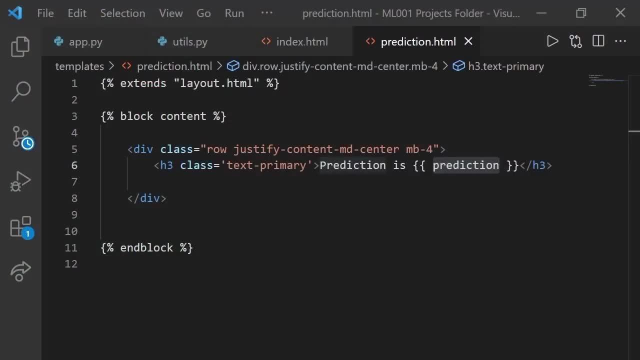 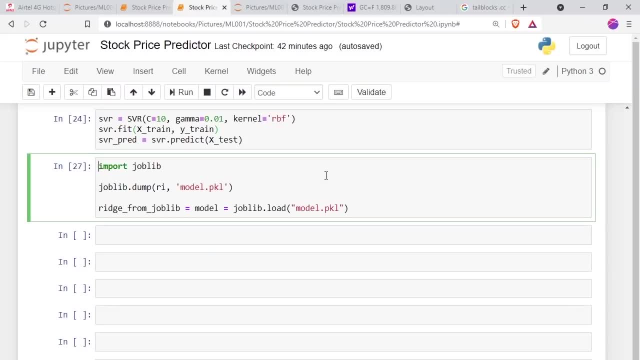 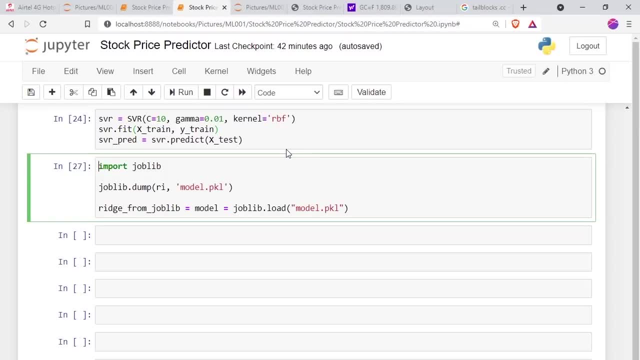 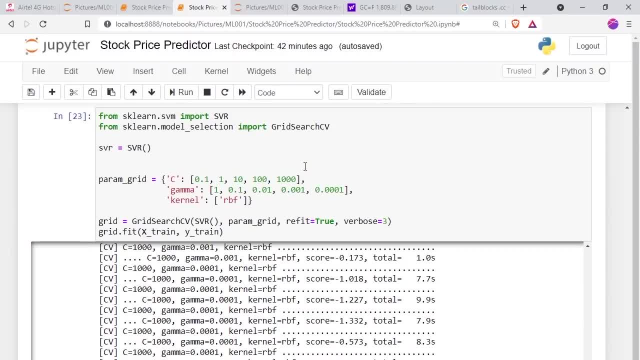 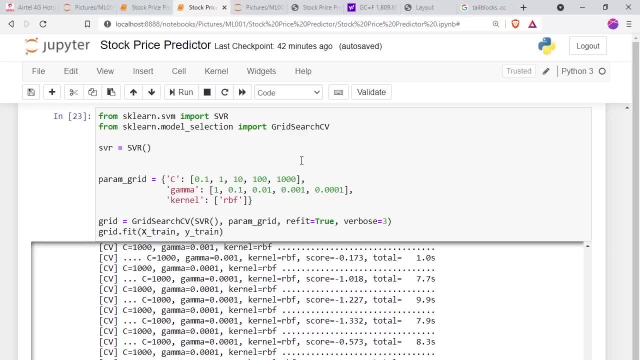 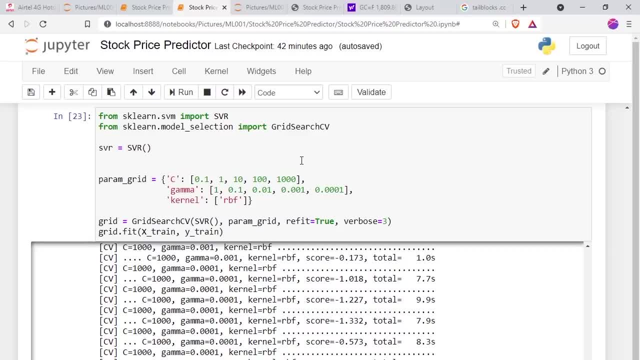 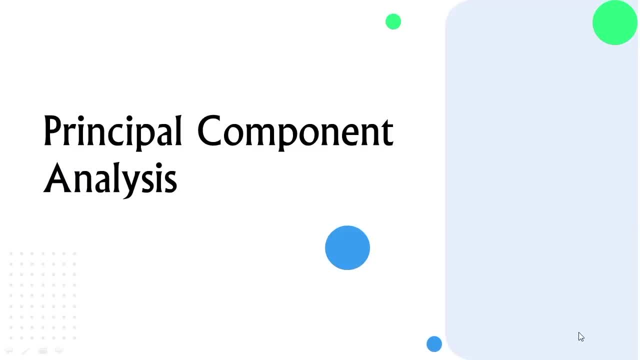 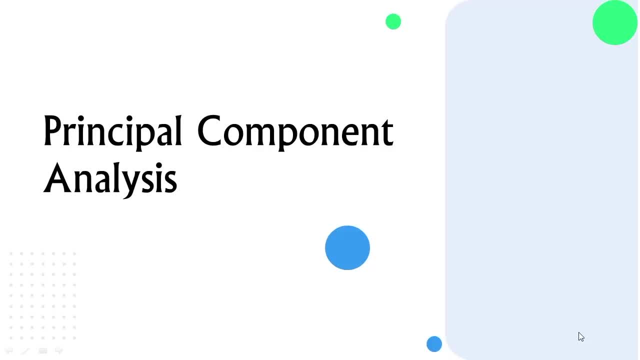 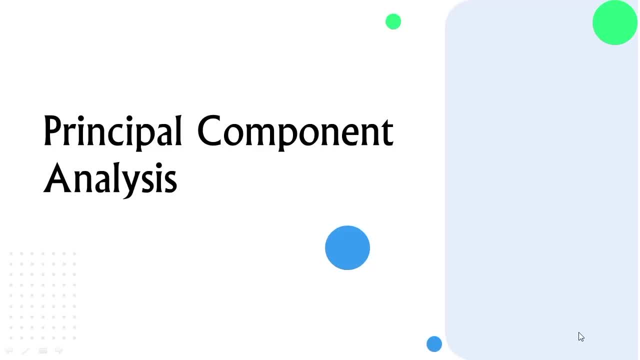 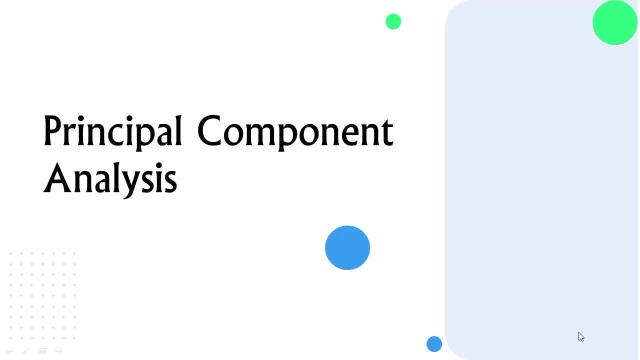 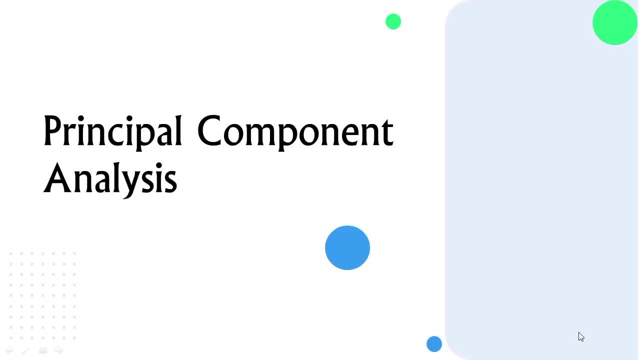 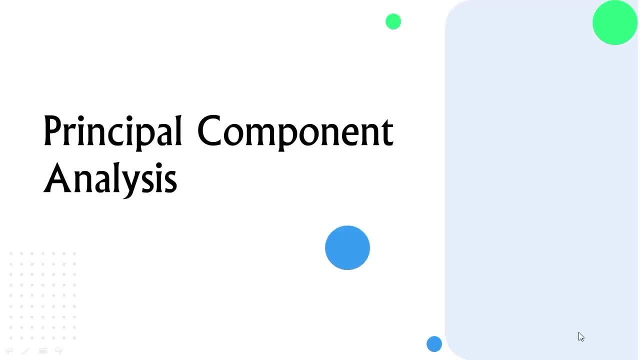 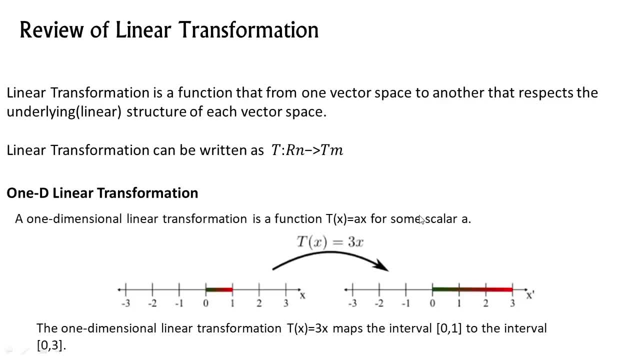 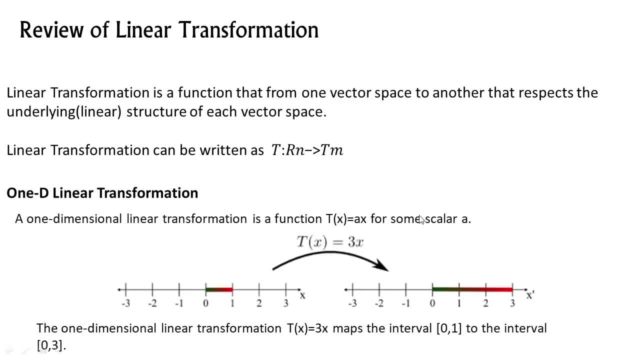 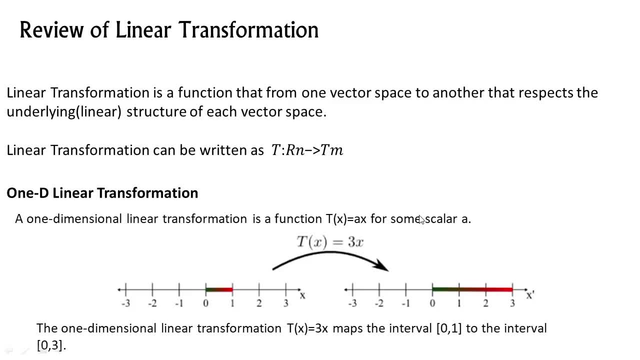 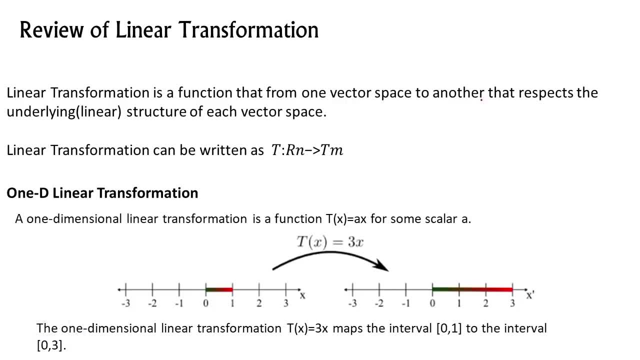 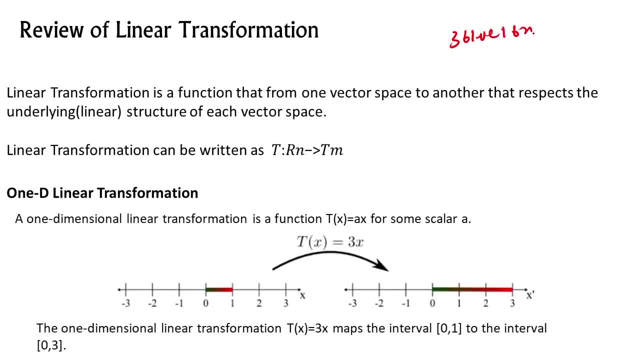 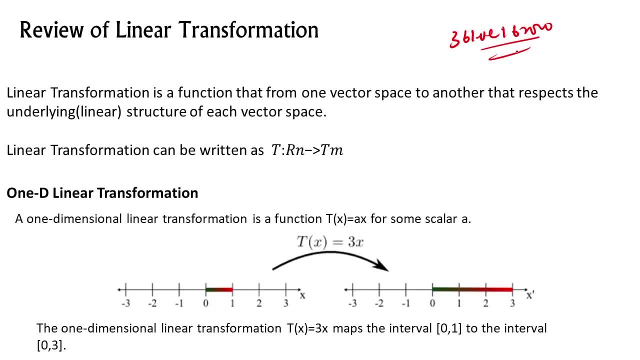 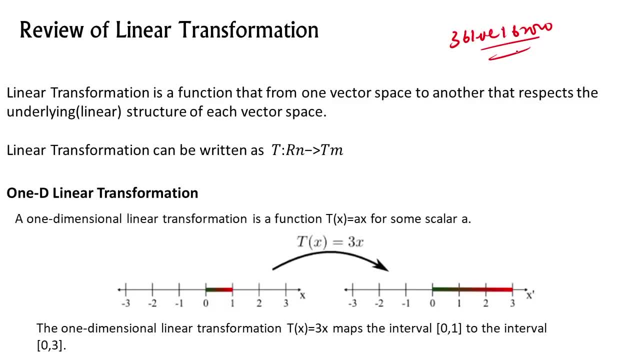 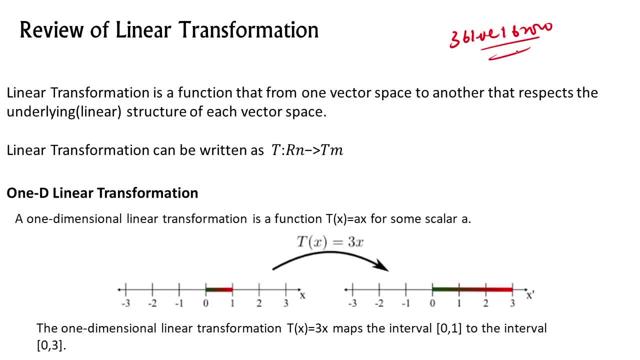 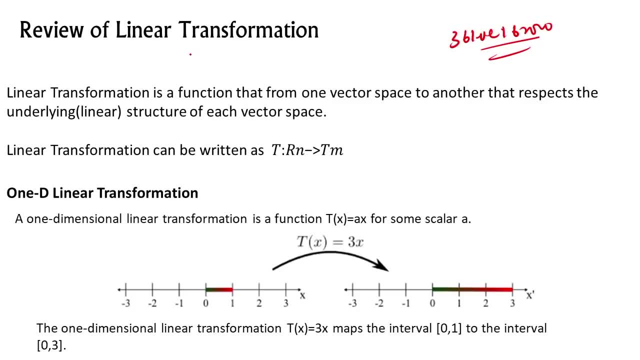 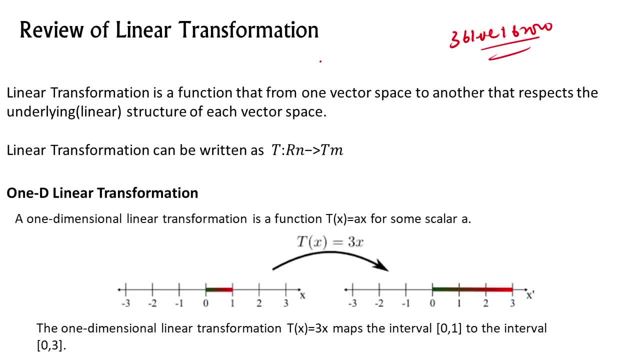 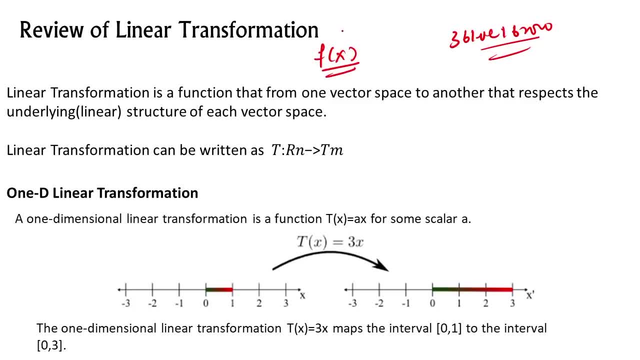 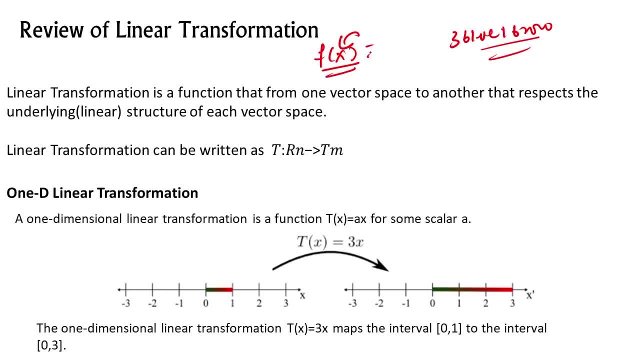 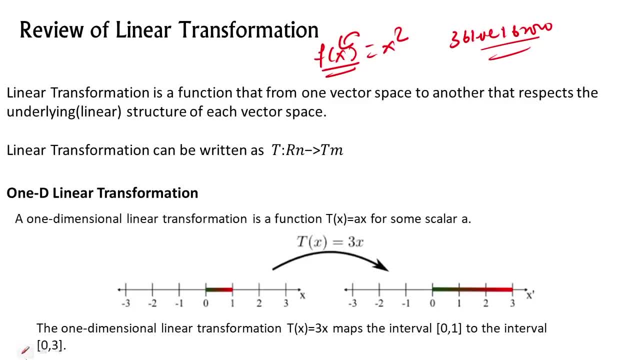 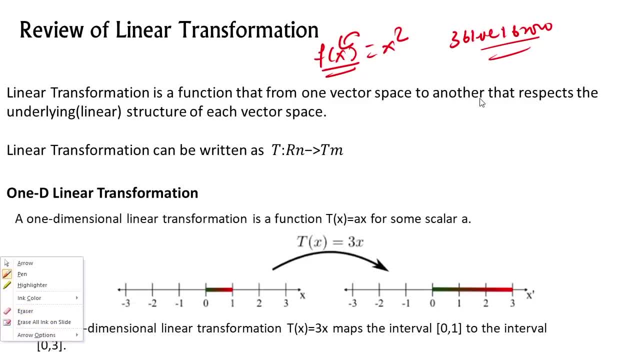 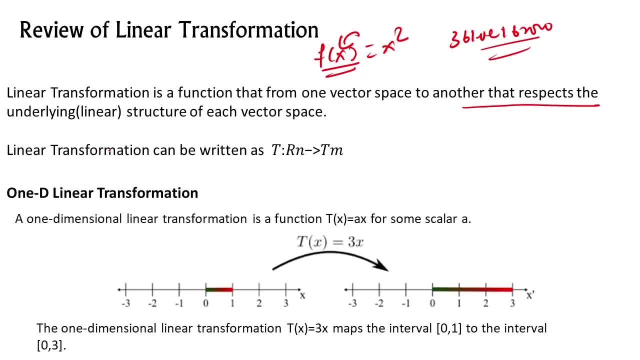 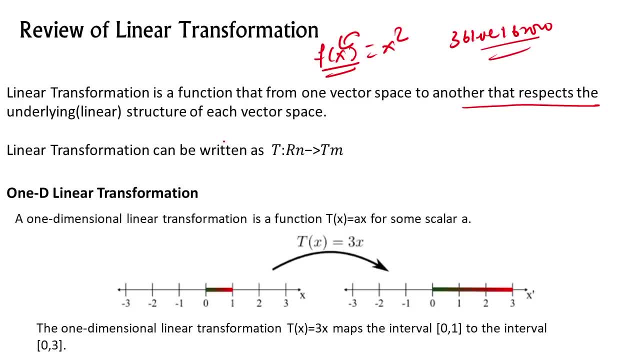 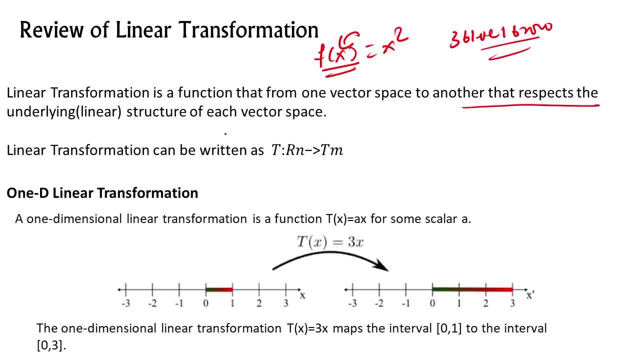 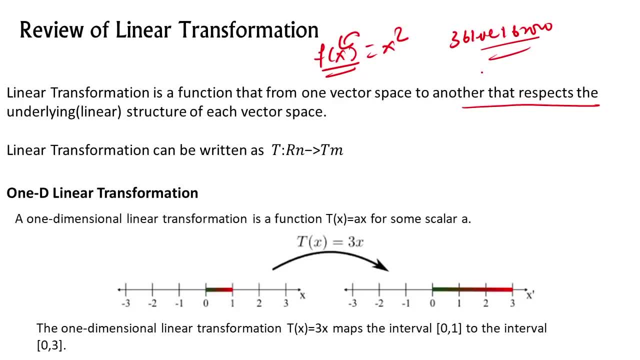 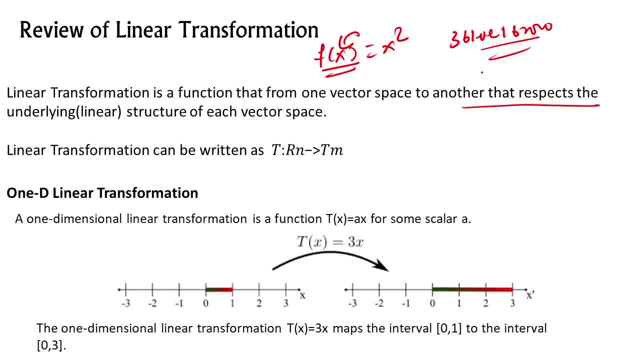 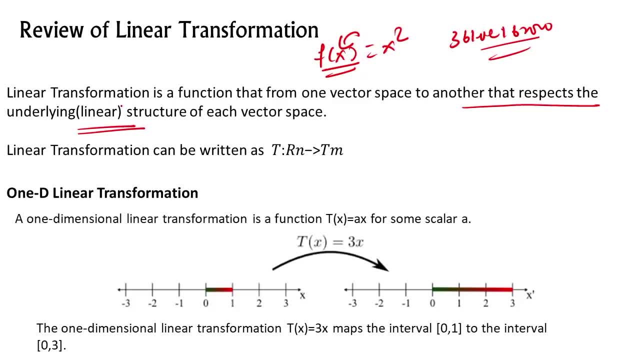 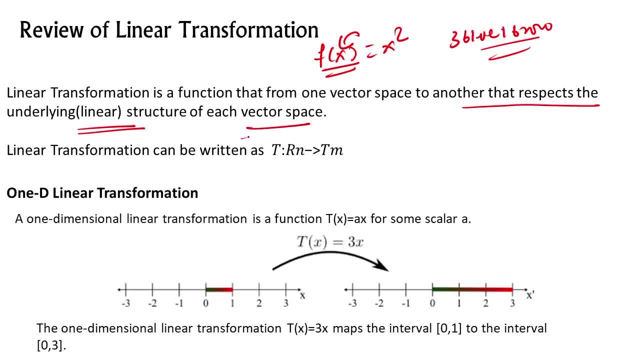 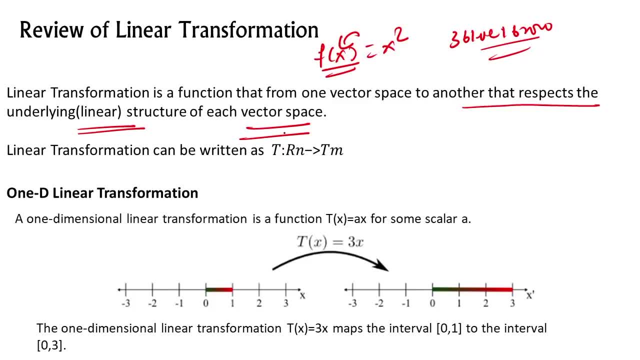 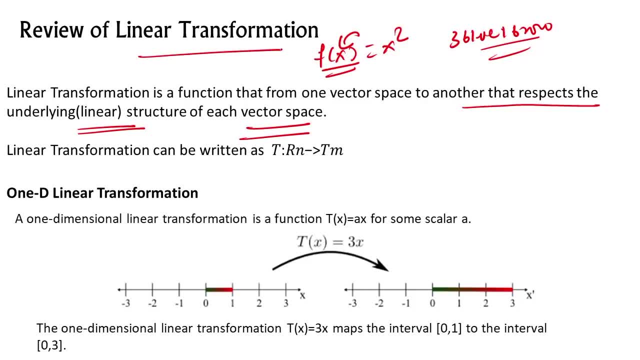 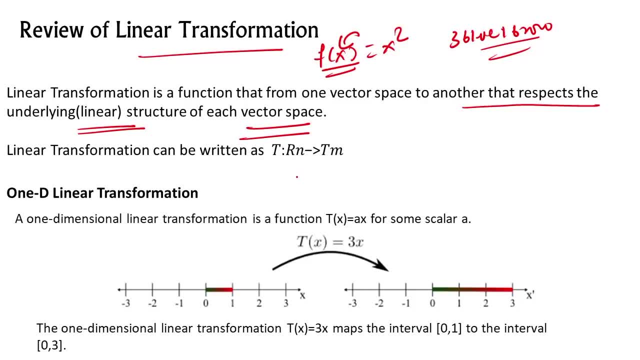 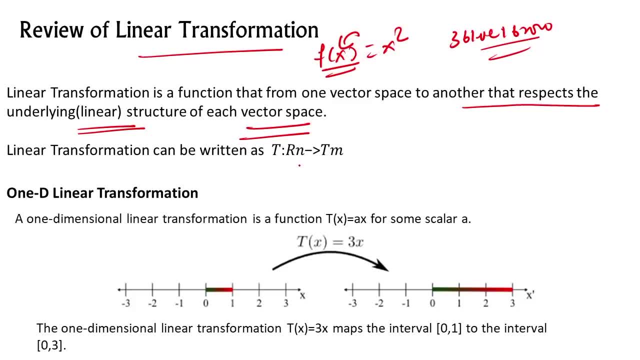 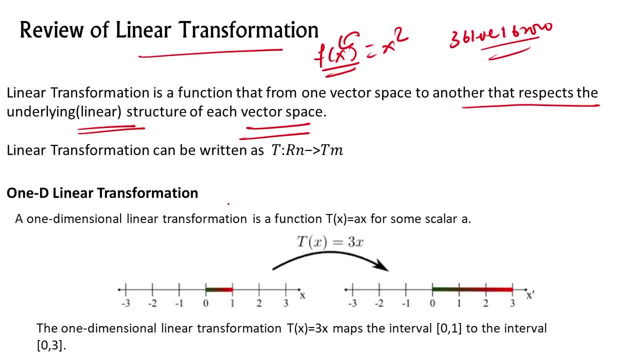 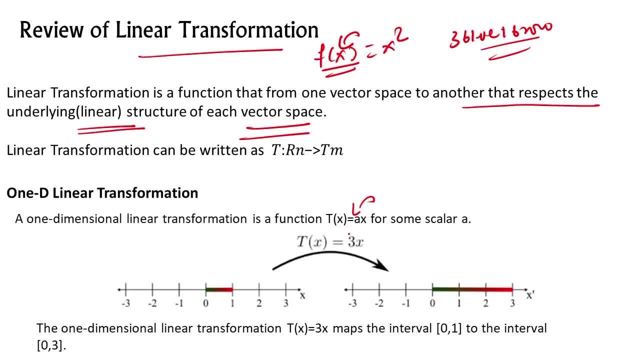 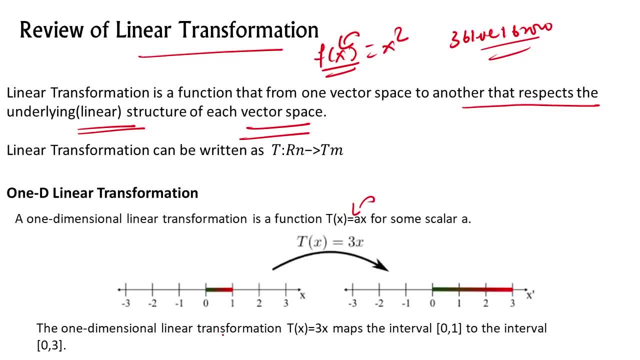 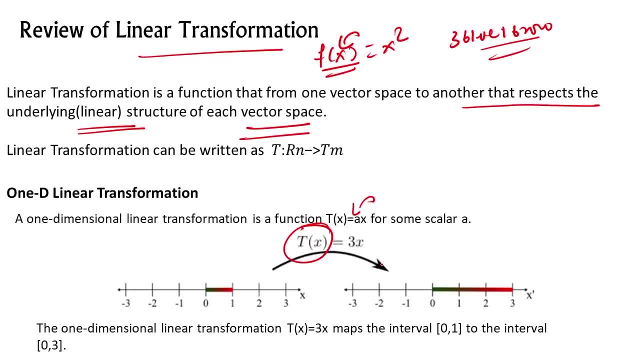 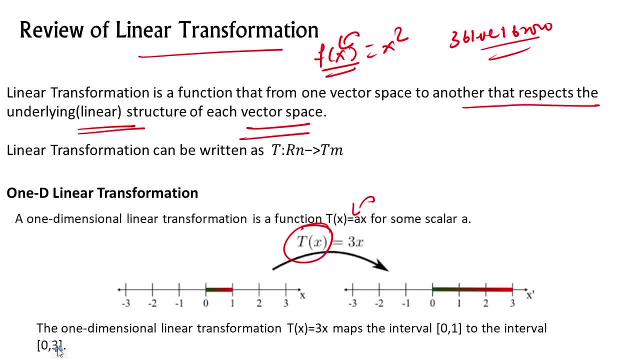 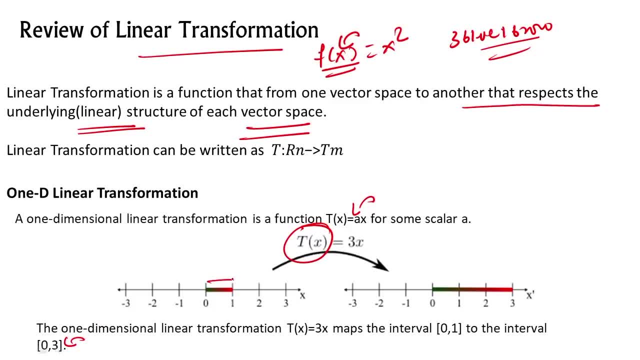 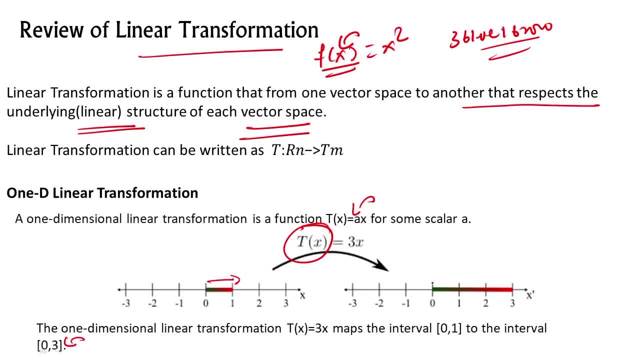 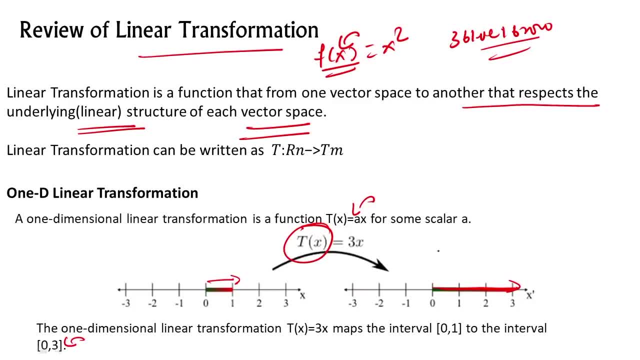 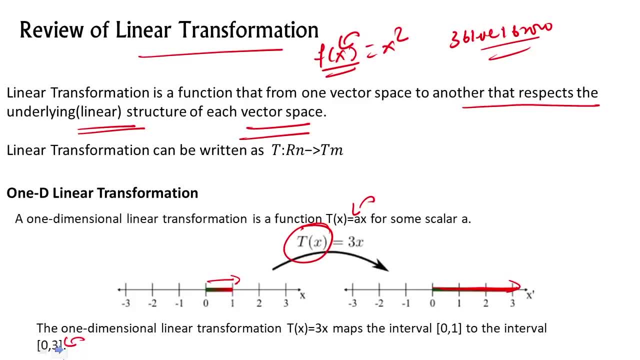 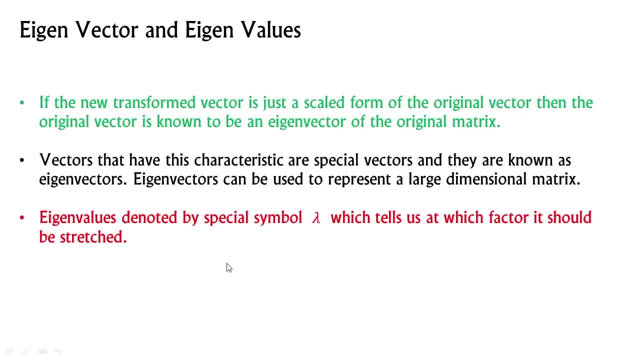 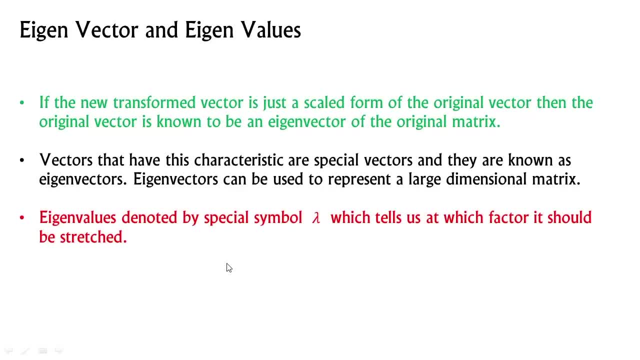 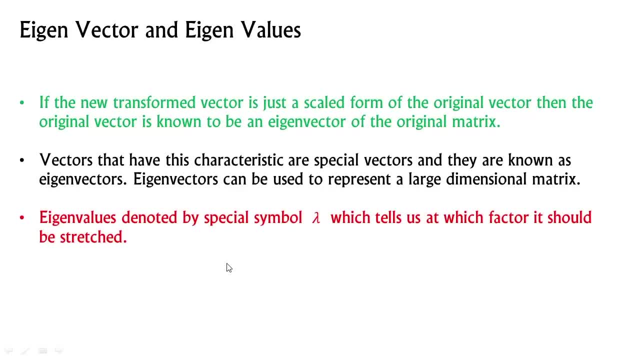 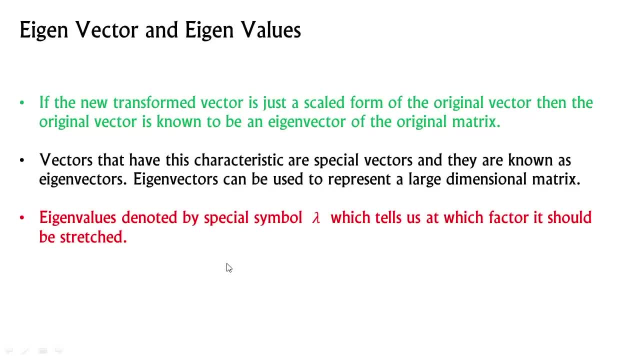 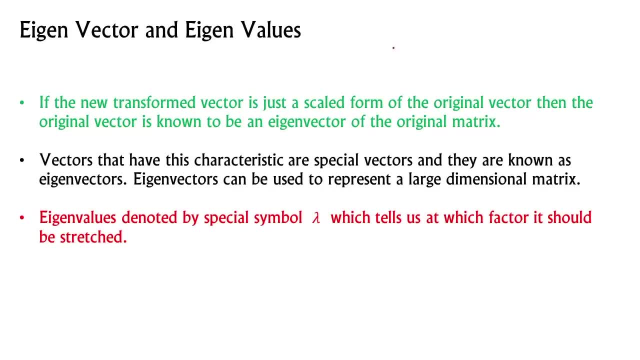 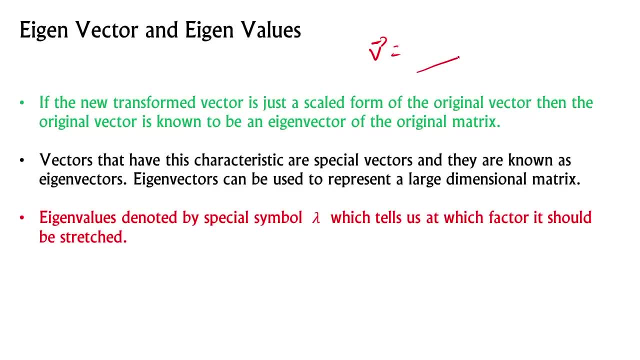 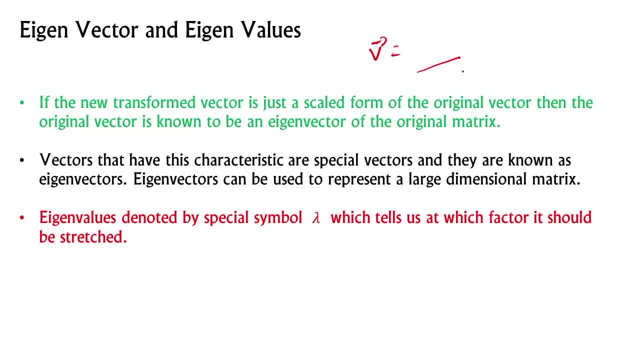 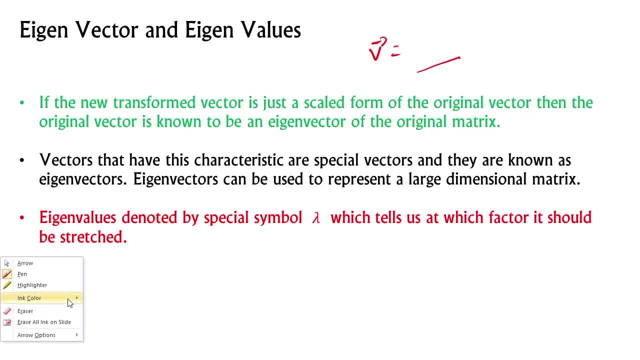 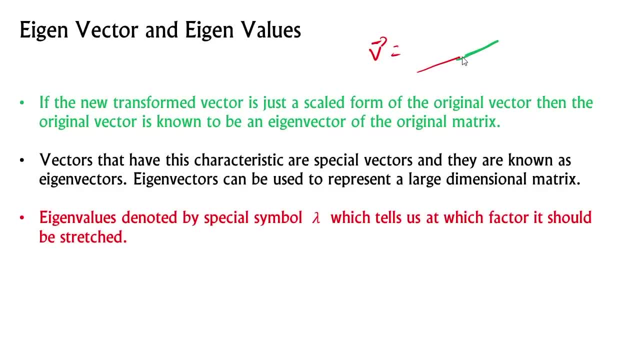 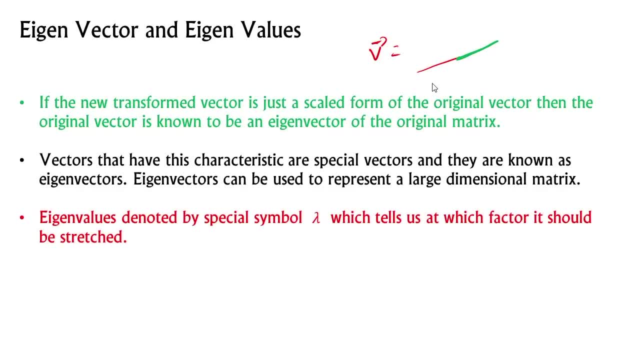 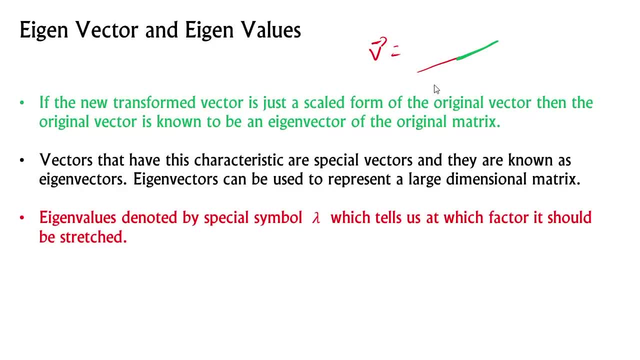 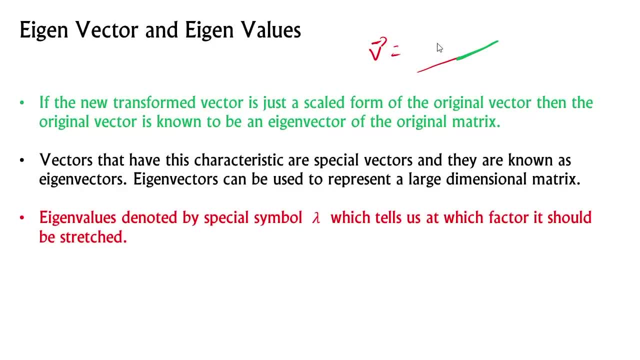 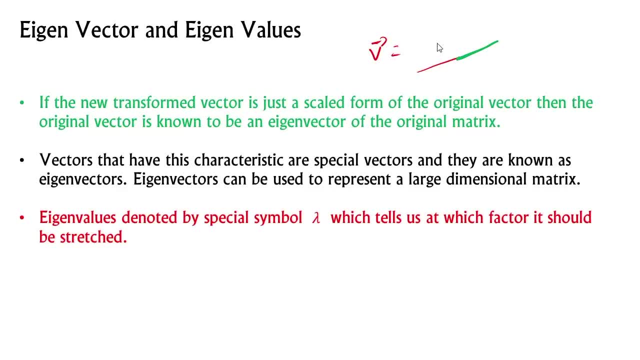 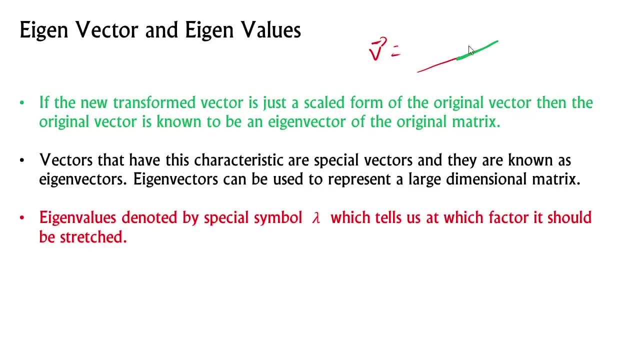 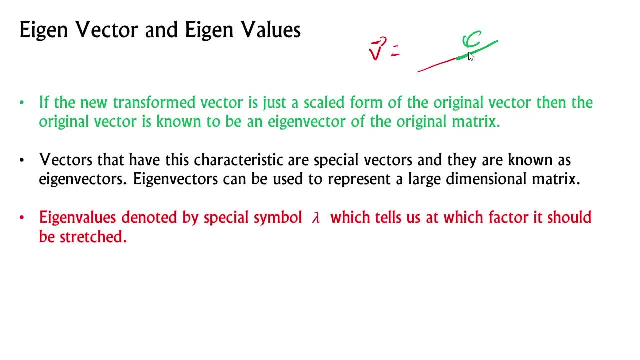 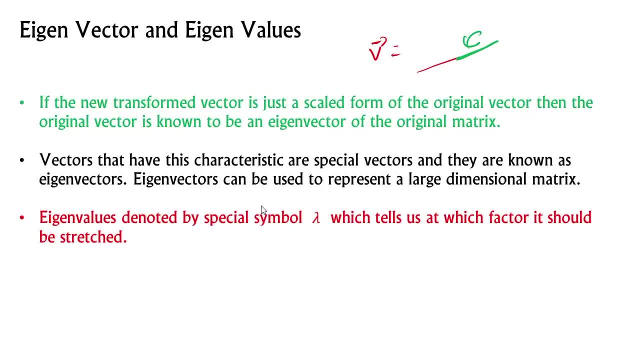 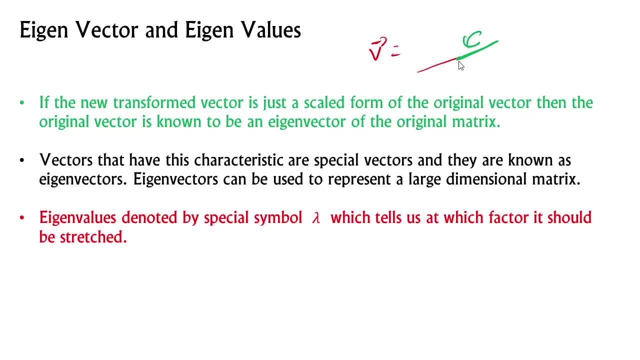 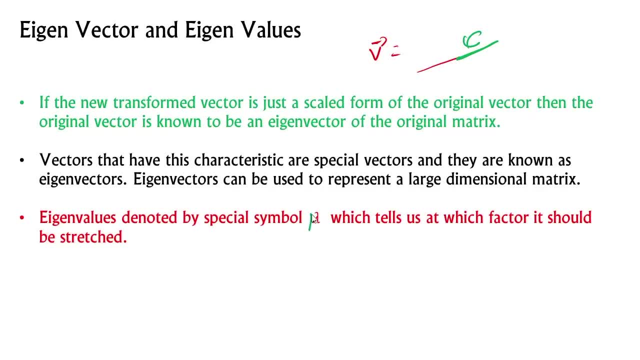 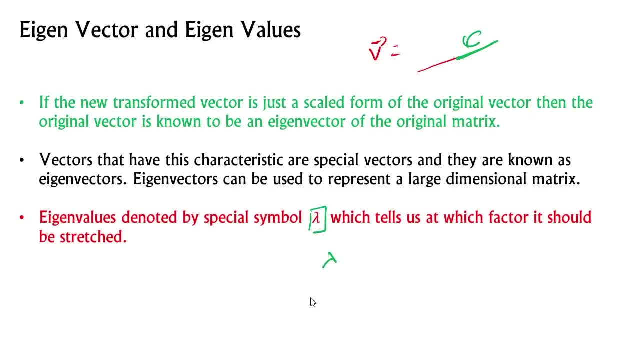 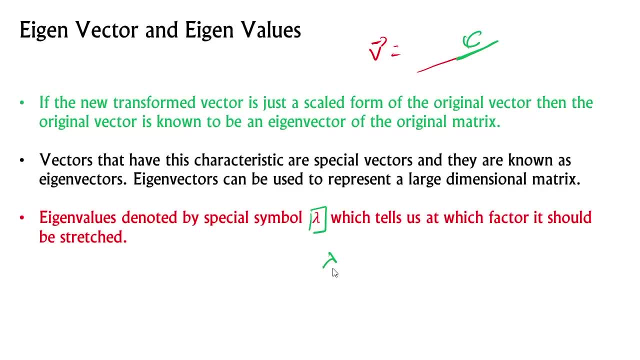 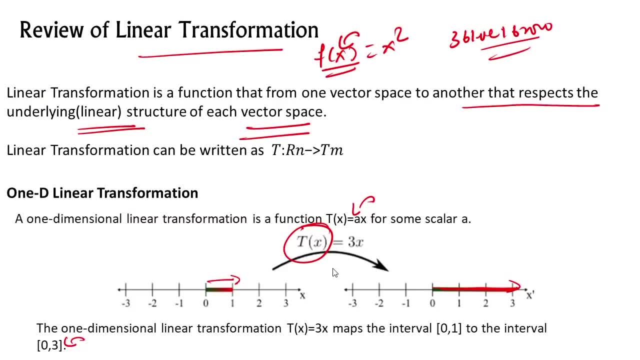 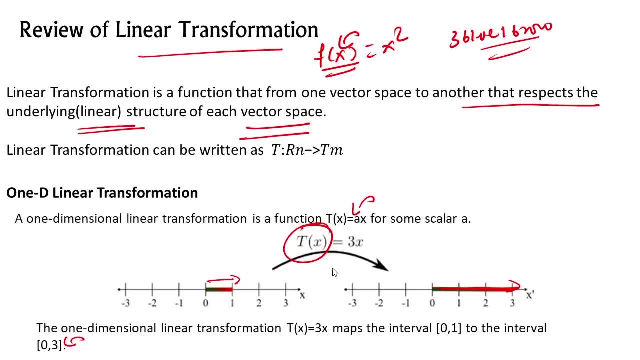 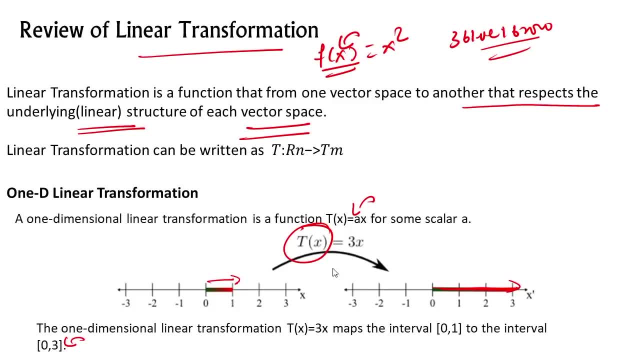 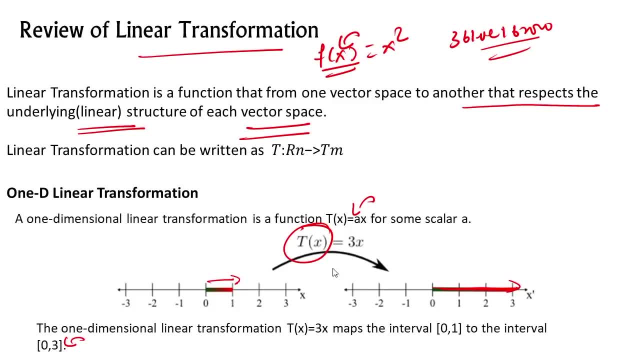 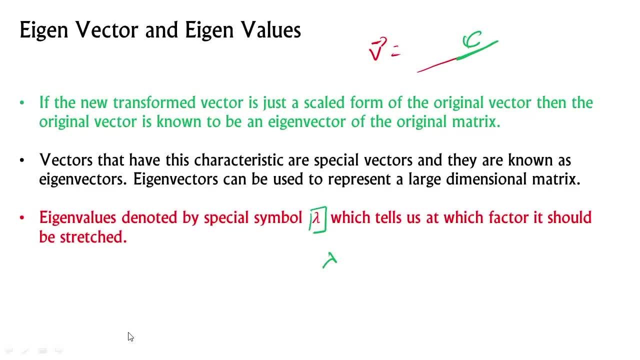 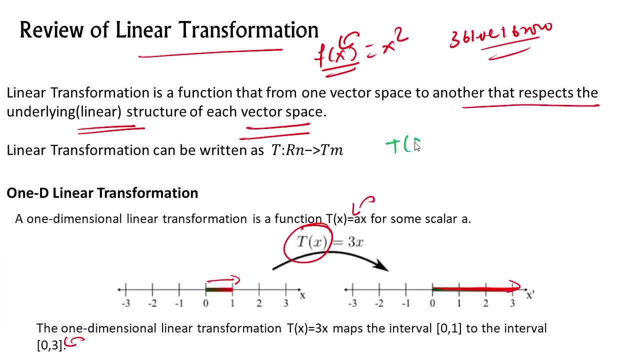 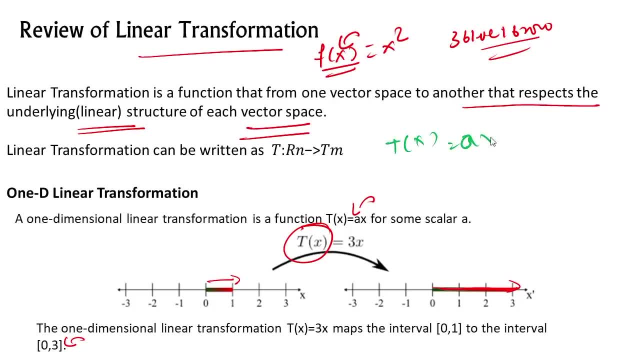 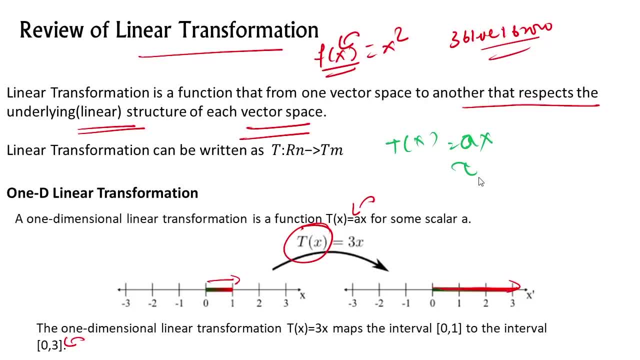 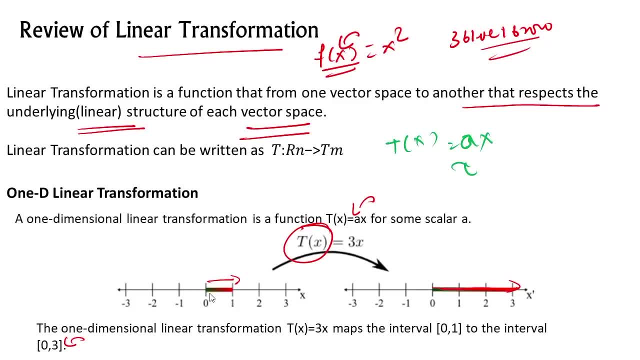 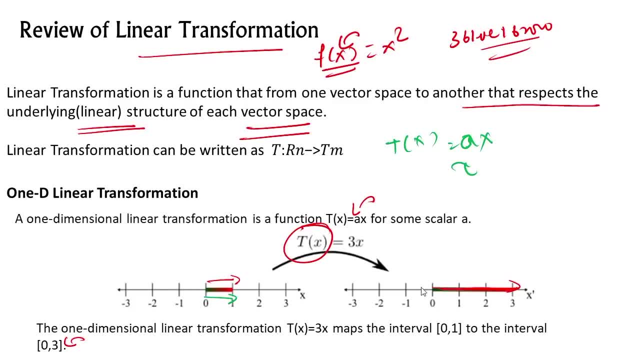 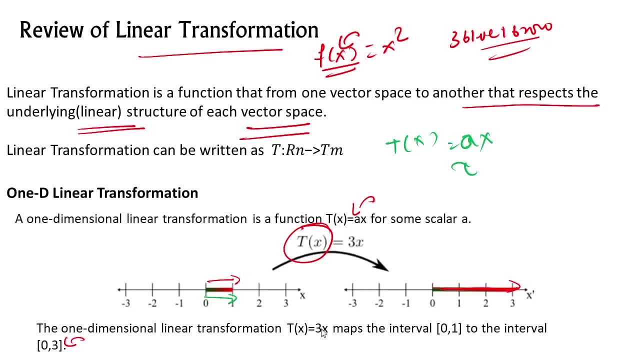 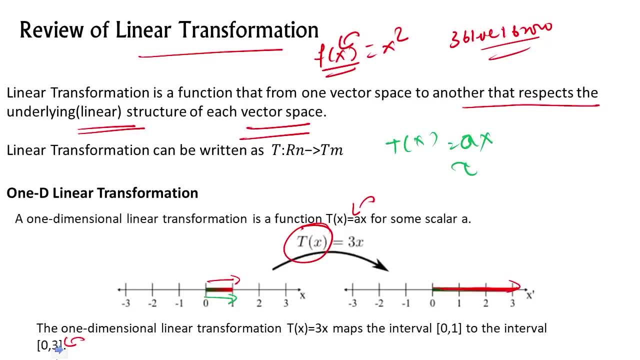 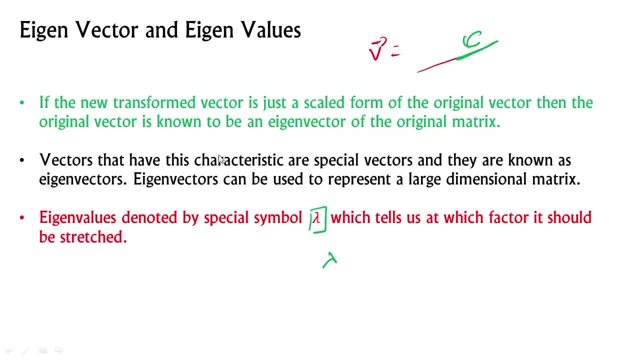 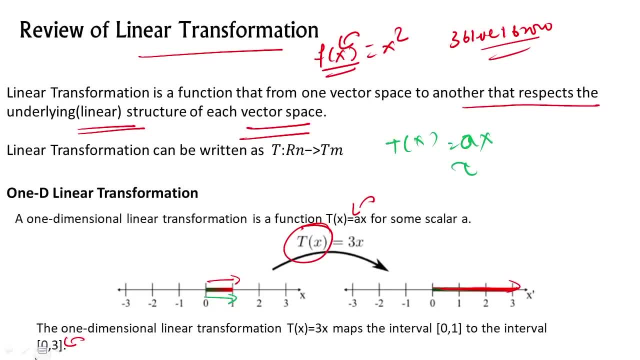 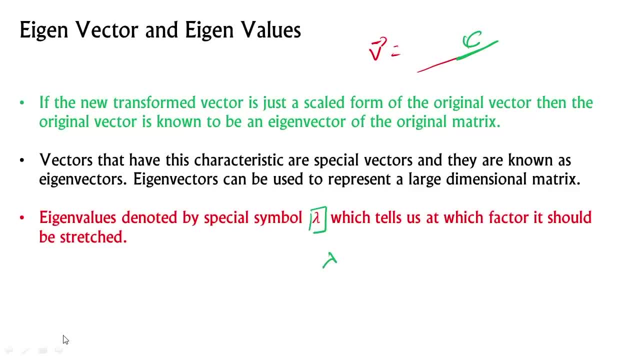 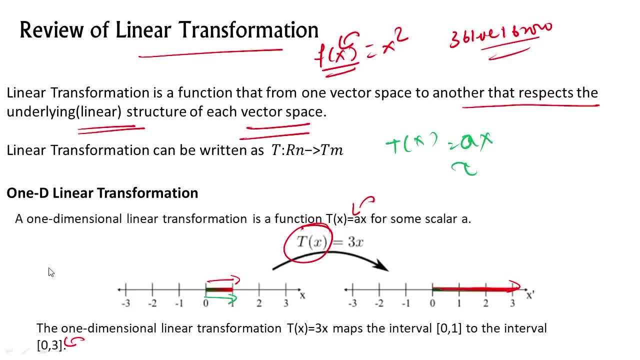 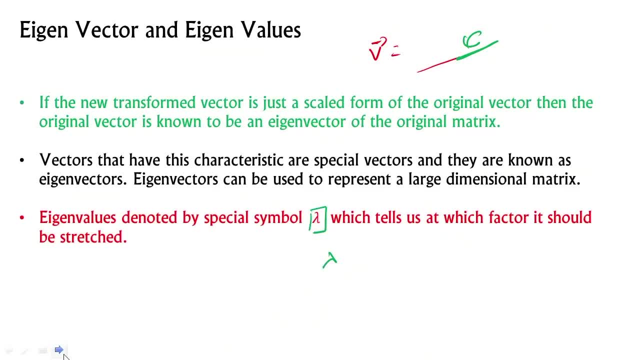 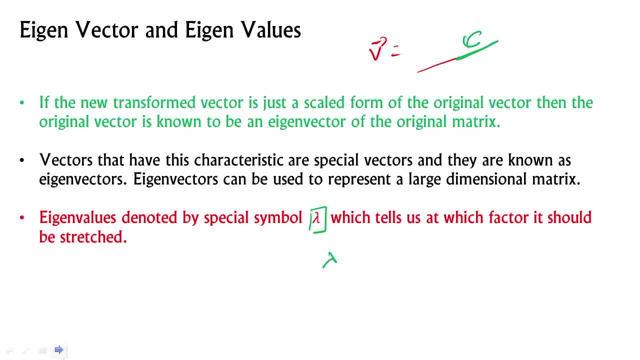 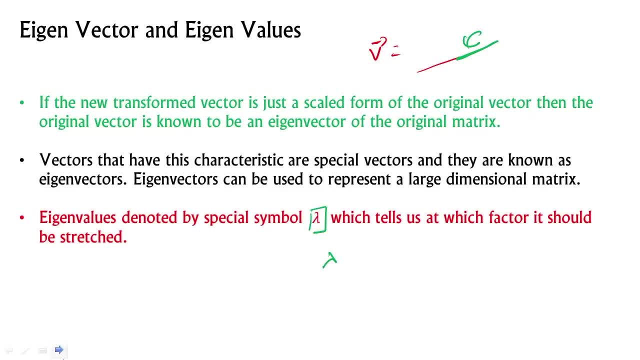 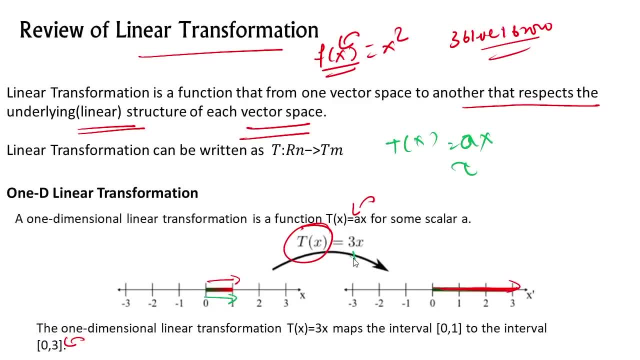 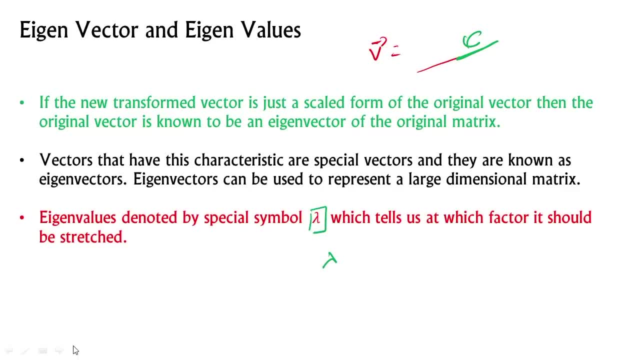 And the factor by which it is scaled here is 3,. the factor by which it is scaled here is 3, then the 3 is your Ison value. Okay, This is what the simple Ison vector and Ison values are. Okay, Pretty much is what I'm trying to say here. 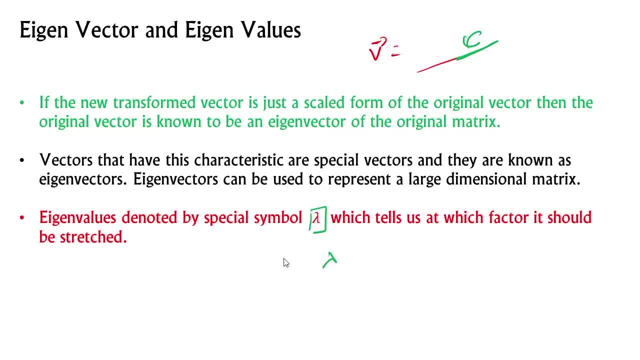 Okay, If you want to get in more detail, there is a video by Gilbert Strang. Gilbert, I think that's correct, Gilbert Strang. Linear Algebra videos are a book by Introduction to Linear Algebra- Introduction to Linear Algebra. You can have a look by Gilbert Strang or you can have a look for a quick look at 3Blue1Brown video. 3Blue1Brown video on Linear Algebra on YouTube. Okay. 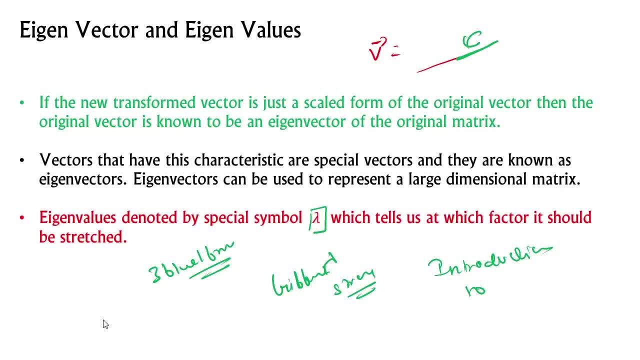 So that's the video. If you want to learn more about Linear Algebra, you can have a look. We'll do that later. We'll do that later, But for now, if you know this, then you're good to learn about principal covenant analysis. 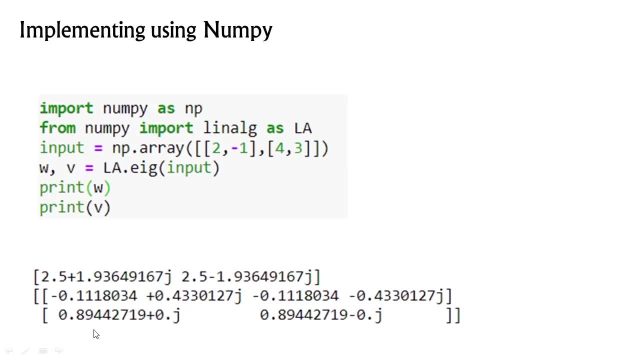 Okay. So you may think, hey, Ayush, I don't want to do so much of math et cetera. So you have a library known as NumPy, which you can have a look, which I have given the notebook in the description down below about NumPy Pandas, so you can have a look. 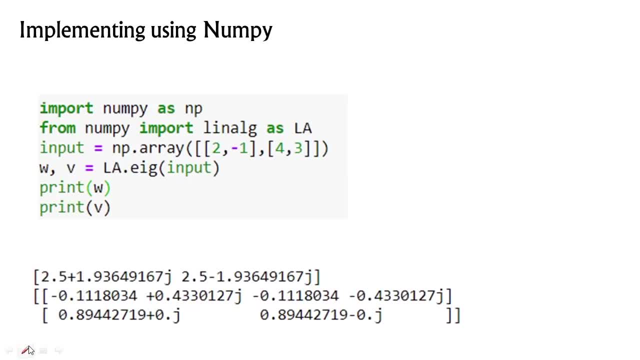 So you can just implement. You can just implement by this: La La Pal is alive. la is alive as a linear algebra. we are taking out the eyes, eiz of the input and input. here is our vector, okay, and this is your. the is in vector and. 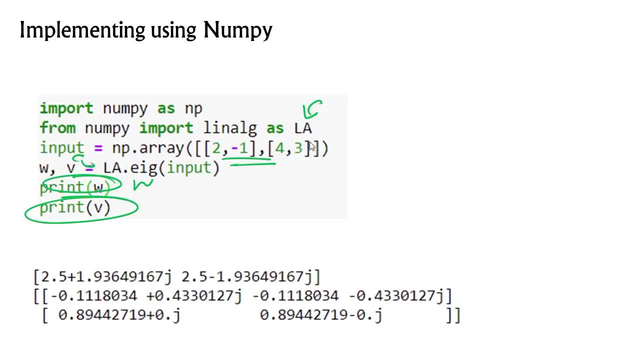 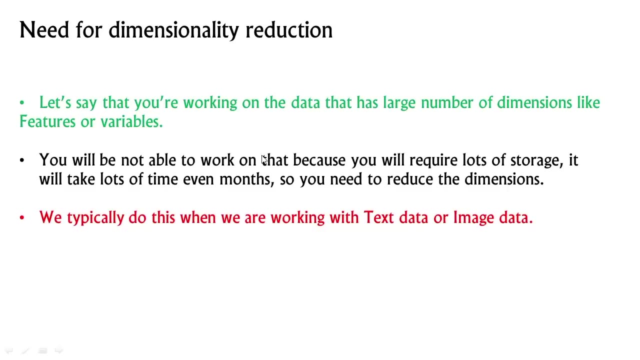 nice and value as in vector off the earth. this matrix, sorry, yeah, this is a matrix, okay. so, and this, this matrix is just a 2 comma minus 1, 4. okay, that's the matrix of 2 by 2 matrix. okay, so we have studied about linear algebra, that is. 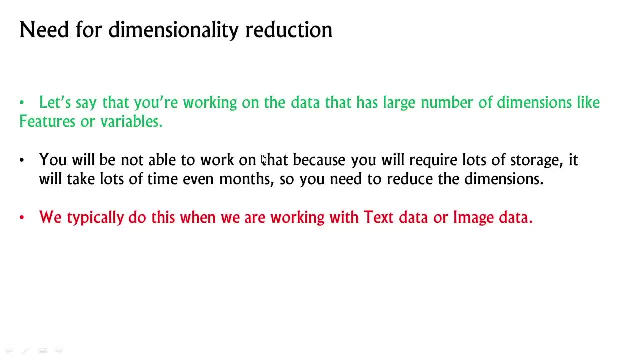 required for us for a principal common analysis. now it's time for understanding why we are starting this all and why- why we need dimensionality reduction. so let's say you're working on kind of a large amount of data set, so this is 3,000 dimensions, and what do you mean by dimensions? it's like the size of the. 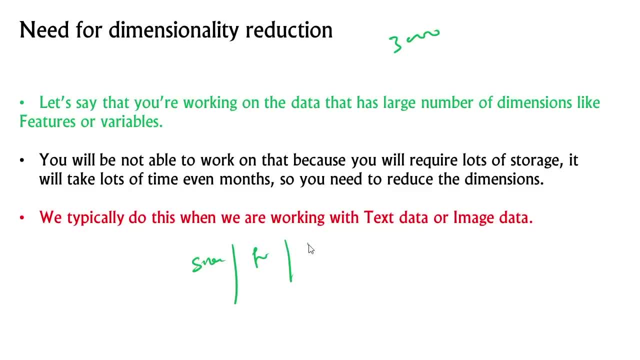 house is one dimension, then floor of a house is second dimension, then number of fans is a third dimension, then etc. so I like, like that, we have 3,000 features. okay, so we have 3,000 features. so for that, to give you, first of all, it will cost storage, second, it: 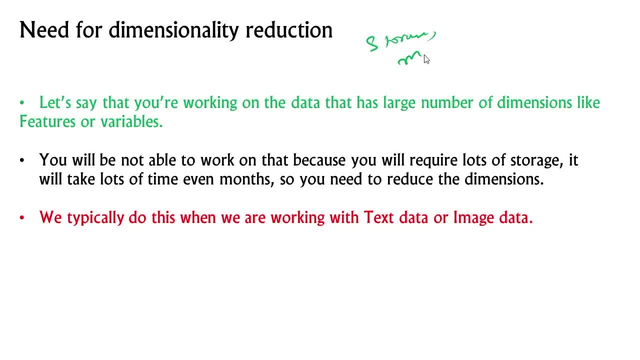 will cost time. it will even take months to train your model. so it may even take months. so you don't have too much of computer resources. okay, so that's why. but in real world, we have a millions of dimensions data available. so well, what we do? we simply use dimensionality reduction method or technique, which is a 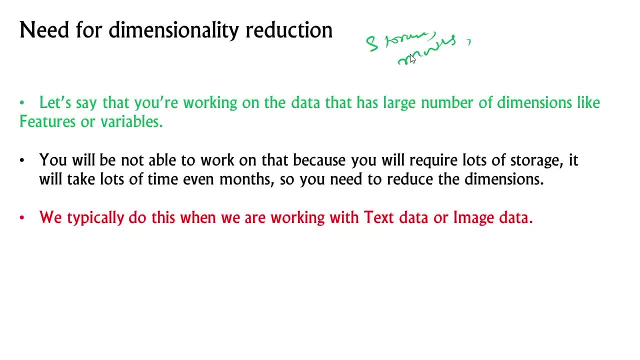 PCA to reduce your model feature with data features or variables. okay, and we typically see this in text data or image data. so let's say you have some image. let me draw one image of mine, so here's my image. so it will. the eye has one dimension and it may be a millionth of dimension, data set, only one millionth of. 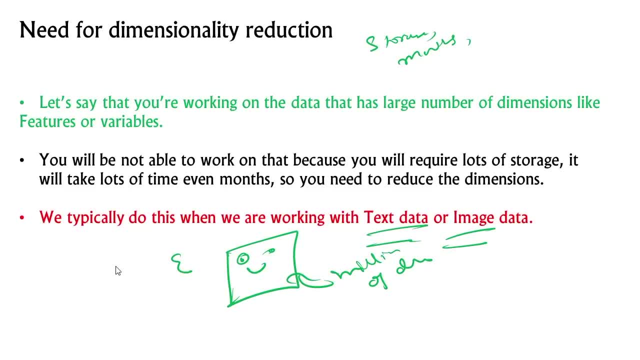 dimensions. one image I have work on- I have work on that- which is, which has 75 dimension, 785 dimensions, so we have what we have to work on. this typically be seen on your text data, where you will working on national and processing like what embeddings or image data we are working. 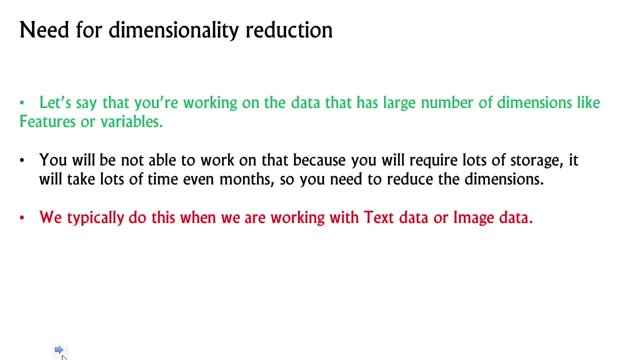 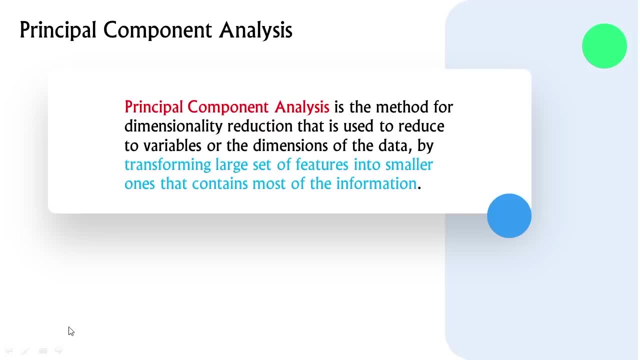 on images. okay, so you need the principal common analysis. okay, so what is principal common analysis? principal common analysis is a method for dimensionality reduction that is used to reduce the variables or the dimensions of the data by transforming large set of features, last set of features and the smaller ones. that contains most of the information. so 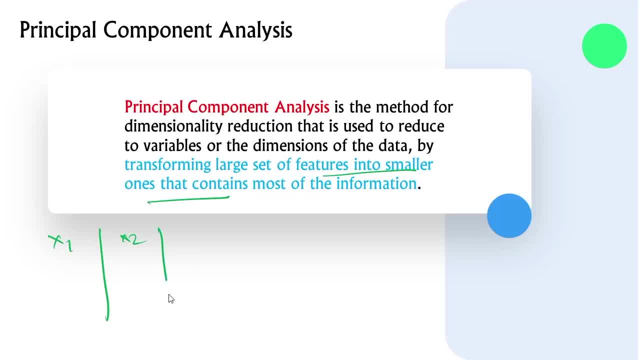 let's see you have x1, then you have x2, then you have x3 and all the boundary. let's say X, well, 40, let's say 50, okay, so what it does? it ask you a component. let's say you have given a two component, so it will try to put. it will try to put. 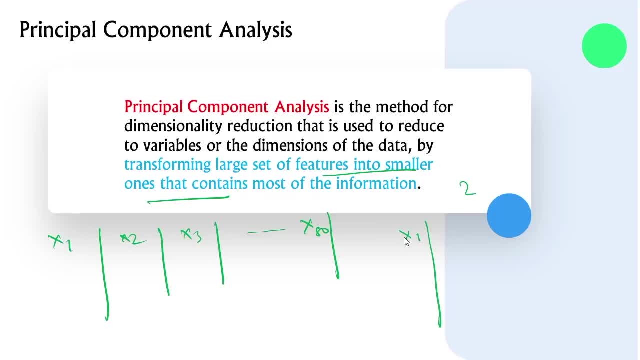 most of the information into the first component, x1, and it will try to put, let it be one, and and and in a second component, most trying to do most of the information in these two component, because we have, say, to reduce from 40 dimension to two dimensions. okay, so so it will simply compress that, like that. 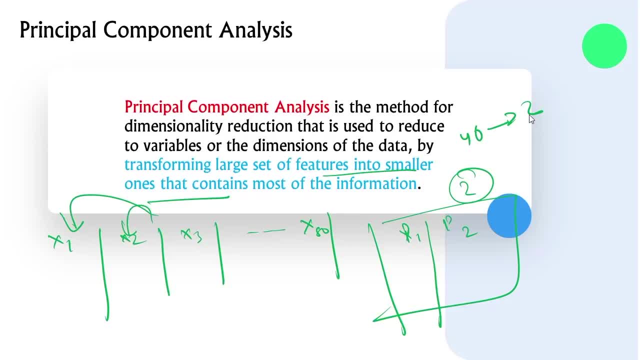 or put all the information into the first data variation, first and second. if you say it is one, so it will try to put every most of the information, the first component, and then move this all. so obviously you will lose some information from the data, but it's good to have not more than dimension. okay, I will give a 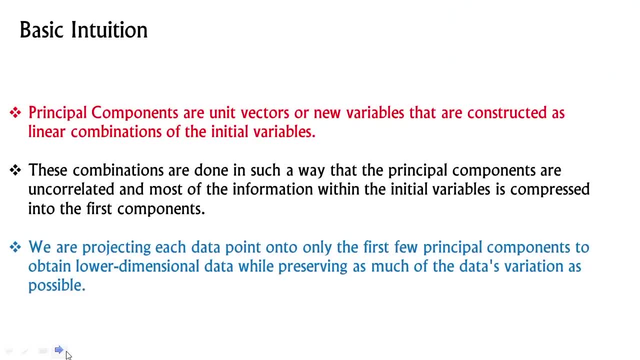 tip when you have to work on principal component analysis. okay, so what is the basic intuition? basic intuition behind principal component analysis is that we have a principal components which is a new variable. which are the new variable? like, let's say, I have, I've given you the P 1 and P 2. they are the new principal. 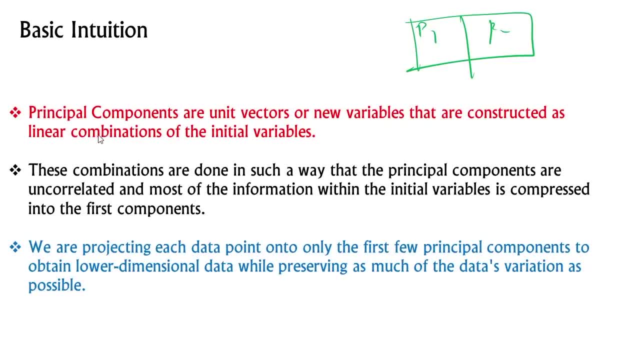 components which are new variables, okay, that are constructed as a linear combinations of the initial variables, okay. so what? what? what we do? let's say we have x1, x2 other than the x40, so we just try to put in all the first and second. so means we is a hyper parameter. 2 is a number of. a component is a hyper parameter. 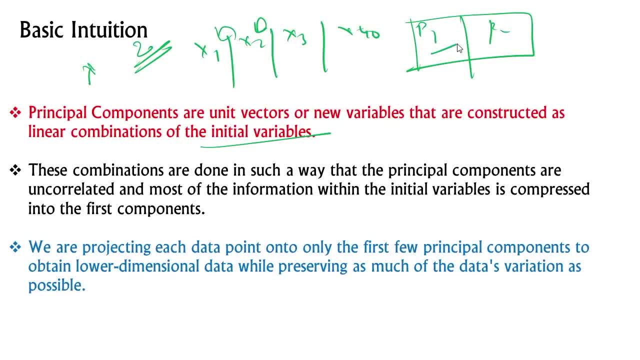 so let's say we have taken 2. okay, so it will try to put most of the information into P 1 and P 2 and these are the new vectors, or the unit vectors or the variables, like this all and it's just a linear combinations of these variables, okay, of the initial. 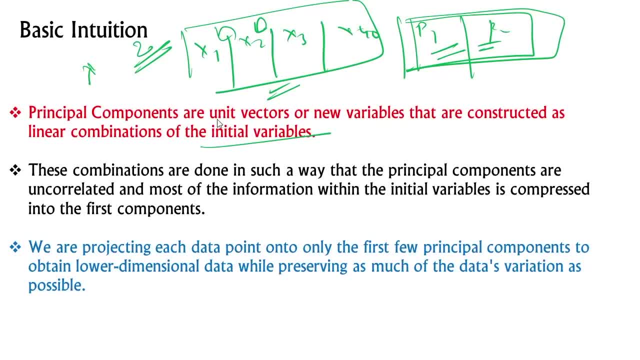 variables. okay, you will get another through visualization what I'm saying, and these combinations are done in such a way that the principal components are uncorrelated. they are uncorrelated and most of the information from this variables- I mean size, price, etc- will be compressed into the first components and so on. okay, and you're projecting each data point. 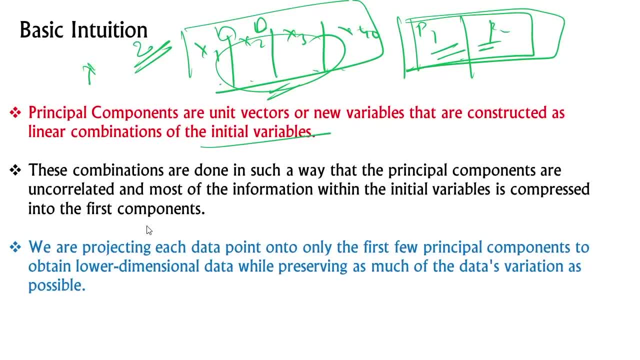 onto one, onto only the first few components, to obtain a lower dimensions of data, preserving as much as of the data variation as possible. so what is this? we are projecting, etc. if you have seen, orthogonality concept into an linear algebra. orthogonality so what it tells. so here's the visualization of that. 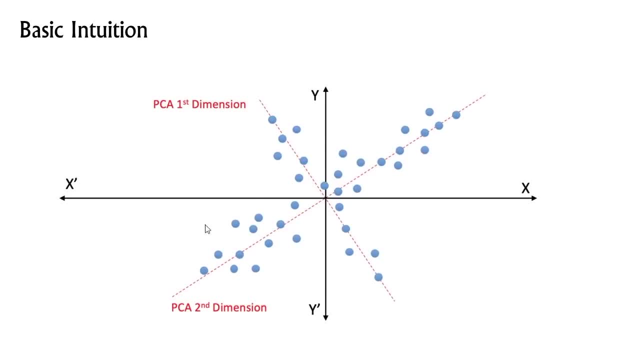 so what it tells. so here's the visualization of that. so here we have a data and what we do? we take out the true complex. if we have two components like this was dimension, and then we have a second dimension like this: okay, so we have a second dimension like this: okay, is these? these are the 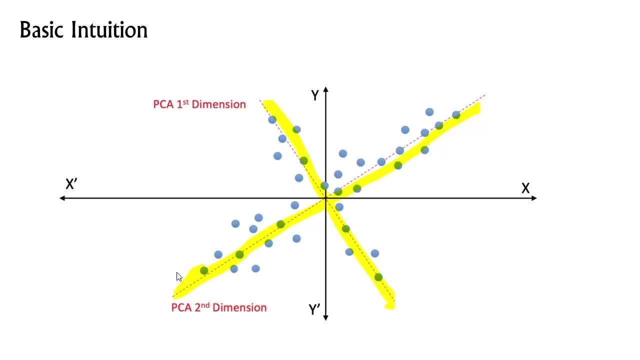 principal components which are constructed, which is, which have constructed as the linear combinations of the initial variables. so what is what we do? we project our data point onto this, we project our each and every data point onto these diamond principle components like this, and now our data point will be on this. so here's the vezes baseline addition which is showing: 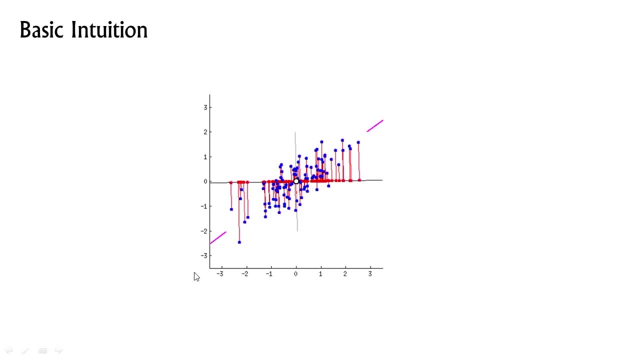 more about this. so we are projecting each data point onto the two components. here we have first component and here we have second component. okay, this is the basic integration behind principal components. so basically, we have a. let's say this and let's say this one, and you have a. 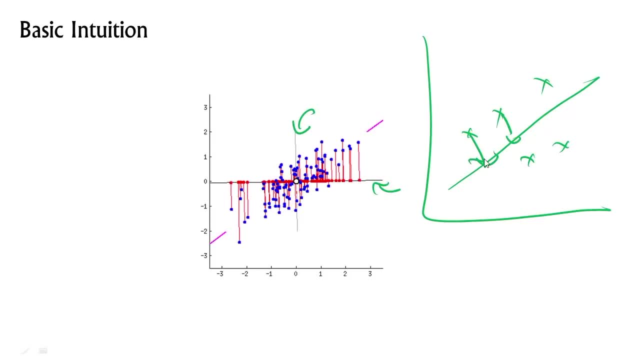 data point like this: okay, so you just project the data point onto here. you project data point under here to reduce the dimension of the data, preserving as much as the information as you can in the first component. okay, so we will see the algorithm. so let's start seeing the algorithm to understand a. 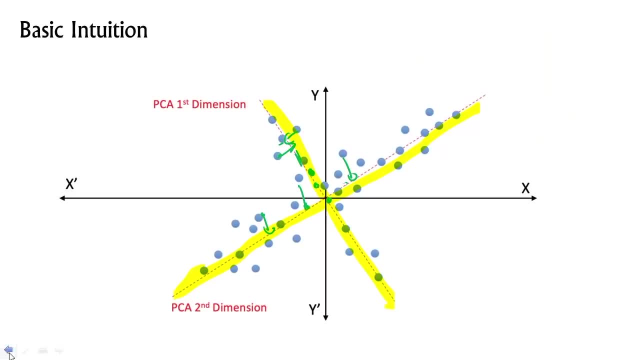 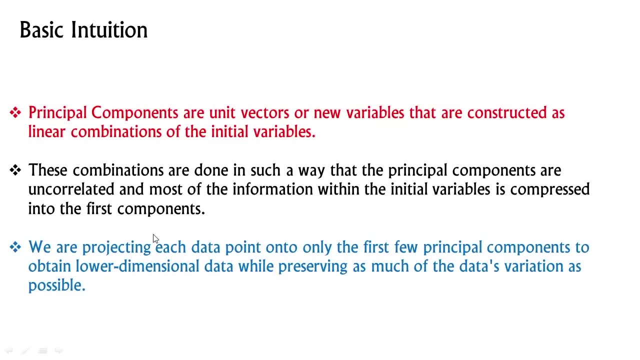 little bit more detail what what we are doing. okay, but for that let's review sort of concept from previous sites. okay, so principal components are the unit vectors. means they are the unit vectors, like the new variables that come out of the p1, p2, whatever he all the Pn, Pc is the number of components as constructed. 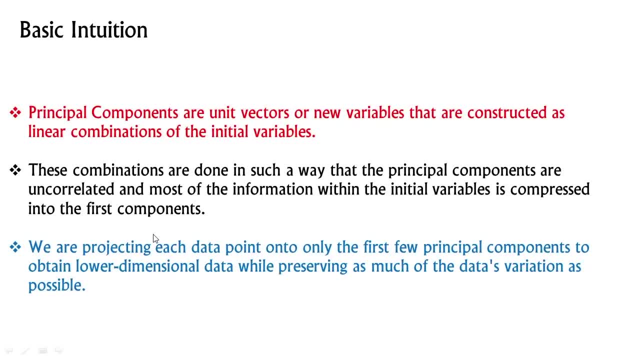 because from the linear combinations of the initial variables and these combination on combinations are done in such a way that the principal components are uncorrelated. okay, you will see the algorithm i design: correlated etc. and most only information within the initial variables and just in a compress in the first and then second, like this number of components you are. 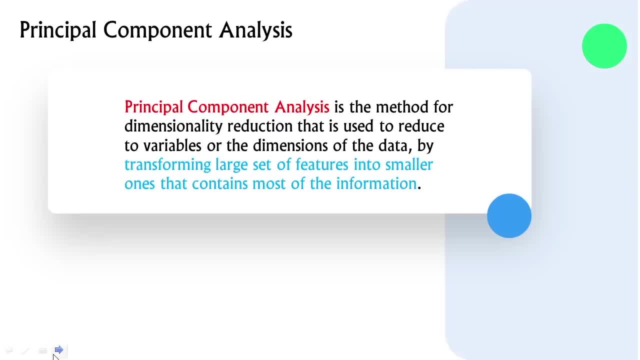 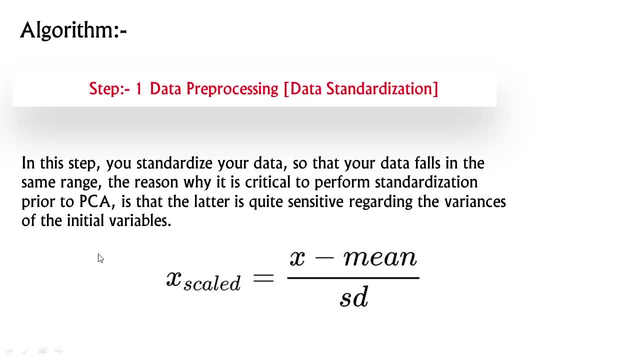 given. okay, pretty much is what i'm trying to say. you here, okay, and we have seen the basic intuition. now it's time for getting into the algorithm. so the first step and the first and foremost step of this principal component, analysis, is data pre-processing. what do i mean by data pre-processing? 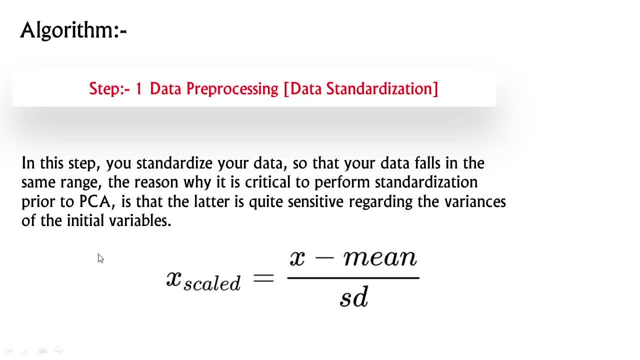 means we have to standardize our data. so in this step, you standardize your data. it simply means that your data should be falling in the same range. okay, so let's say you are working on a some system like, let's say, the age. uh, like the one one, one where you have one variable which is 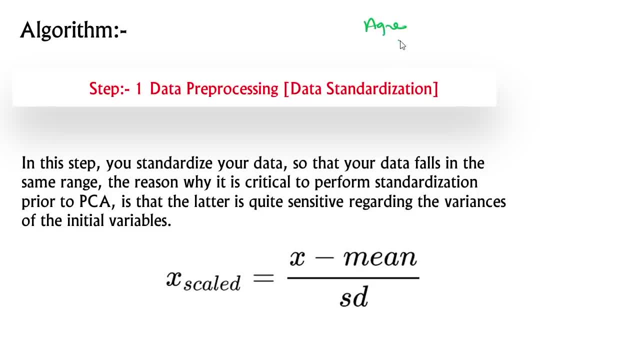 the age. so you have an age and let's say the first person is 20, second person is 40, like like this. so let's say a new person is 1 200. it's far away or far different from these entities. it's called an. 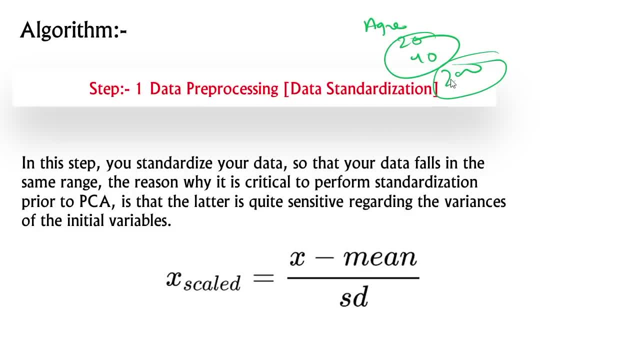 algorithm liar. it's called an outlier, which is which, which is which is not in the range of age- okay, and it's which is not in the range of the common ones- okay. so let's say your data is like 20- 40, it's a two. 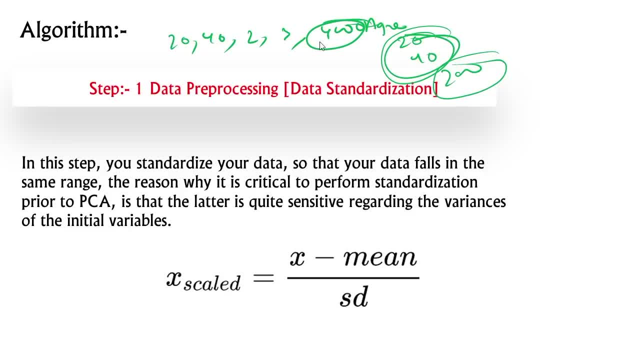 three, so let's say it's a far four, four thousand. so you, this is, this is kind of a outlier and principal common analysis is sensitive to outliers. okay, so what, it would do so for them, for so, uh, so that's why we do the standardization of the data. some sometimes we do normalization. 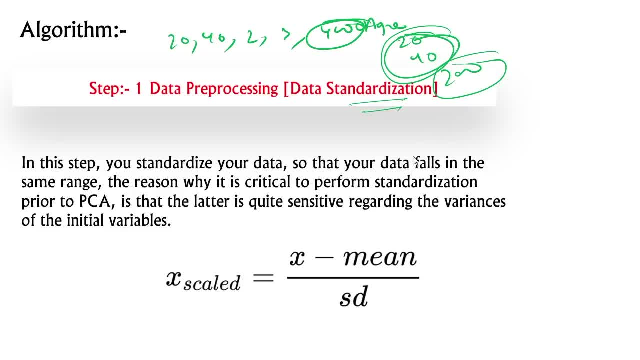 also so we do the standardization of the data, so our data falls in the same range, and the reason why it's critical to perform, because it's quite sensitive. regarding the variances of the initial variables, okay, if you have seen the variance and mean of here, and the formula for this is x scaled. 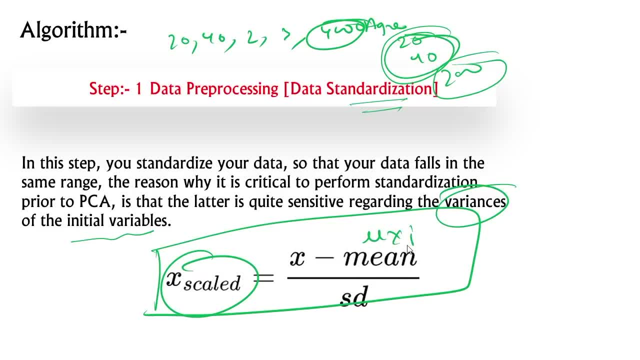 equals to x minus the mean of XI by the standard deviations. okay, standard deviation. and then you will get this scale formula of your day data. and don't worry how to implement this. you can also implement this just by coding in Python. so let's, we have made a. 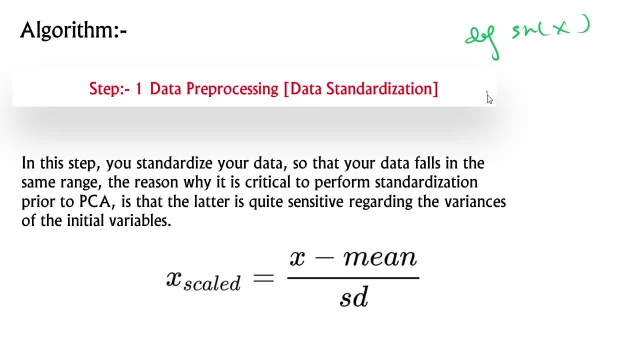 function. this is standardized. it takes the value of X. then you try to make a new variable like scale. then you subtract X minus the mean. is NP dot mean of X divided by the NP dot standard deviation of X. okay, into this. but if more formula vectorize code is in scikit-learn, you can use scikit-learn to. 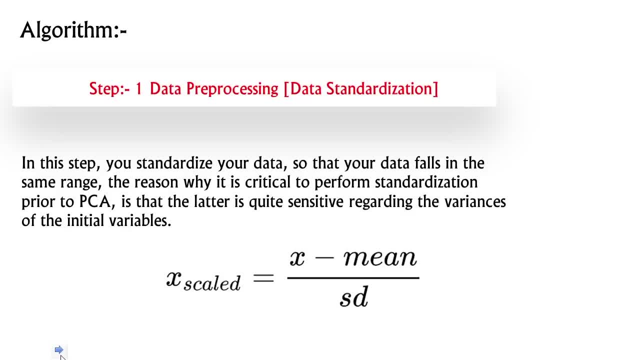 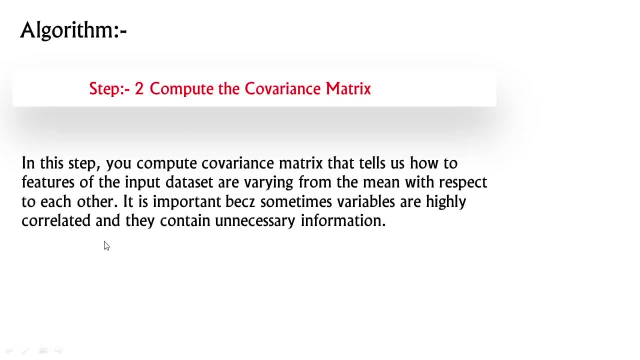 implement it. just three lines of code. okay, don't worry if you are, if you are not able to implement from scratch. after first step, after we standardized your data, now it's time for getting into the computing your covariance matrix of your data. so what do you mean by covariance matrix? 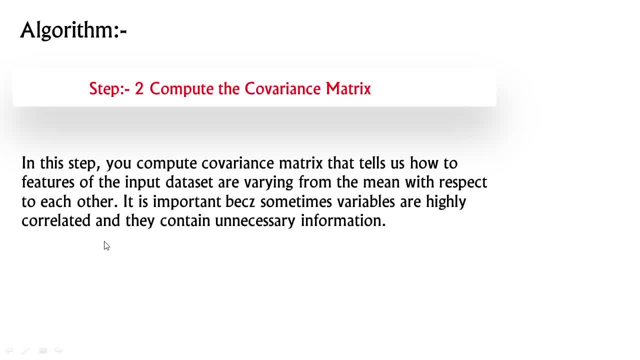 in the is covariance matrix, a p-by-p symmetric matrix where the diagonal are the variances of whatever the data. but if you will tell you can have, I will go to internet whatever. what is covariance matrix? but here, after taking out the covariance matrix, it will tell you that that that tell us how to feature, how the 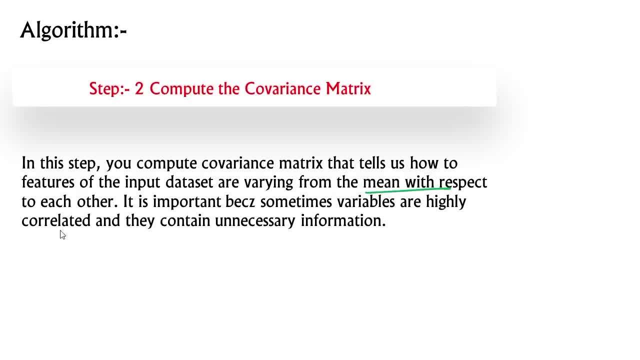 features of the input data set is varying from the mean with respect to each other. okay, so here's test the core. okay, correlation like that. it's not a really correlation, but here you have an input data set like X and it's that out of how much the input data set are. 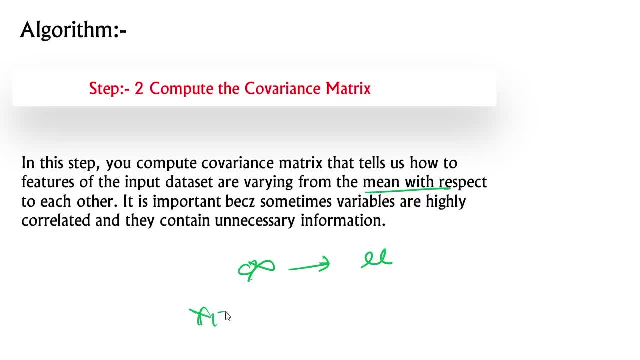 varying from the mean with respect to each other, means the X 1, how it's varying from X 2, etc. it is sometimes important because there are some variables highly, highly correlated and they contain unnecessary information to work on. okay, so you should review have to do. you can remove that. okay, so that's how we come to. 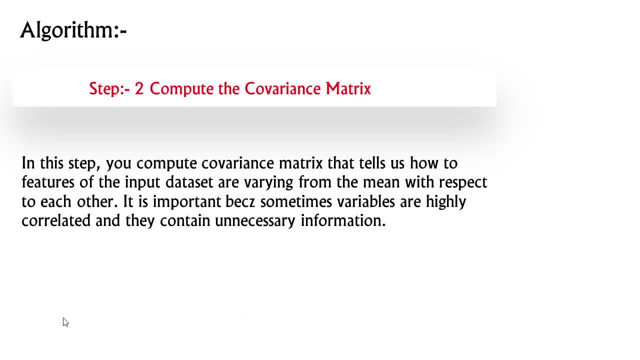 view the covariance matrix pretty much is. you want to try trying to save here. okay, so you just should denote covariance matrix with C and for implementing covariance matrix you can use the again numpy for the scientific numpy, that NP dot cough, and you just give the data as your features. it's X and 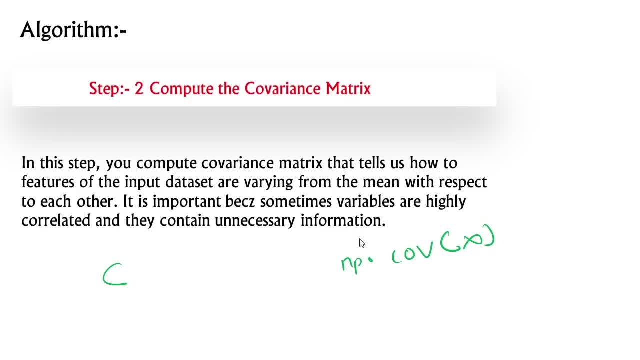 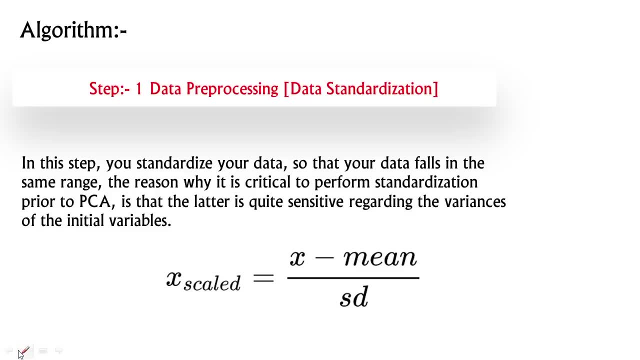 you'll get your output at the covariance matrix. okay, pretty much is you. I'm trying to say you here. so let's see what I have seen so far. we've seen: first we have to pre-process your data like a state of standardization or normalization. then we 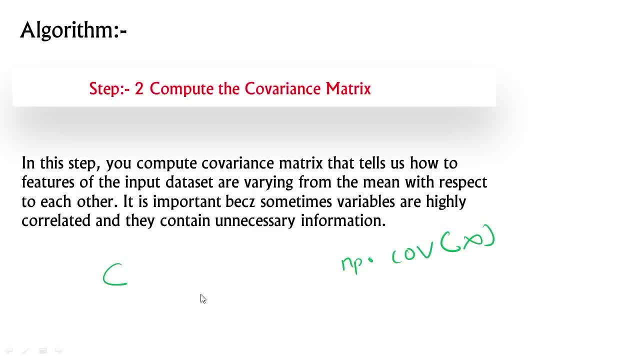 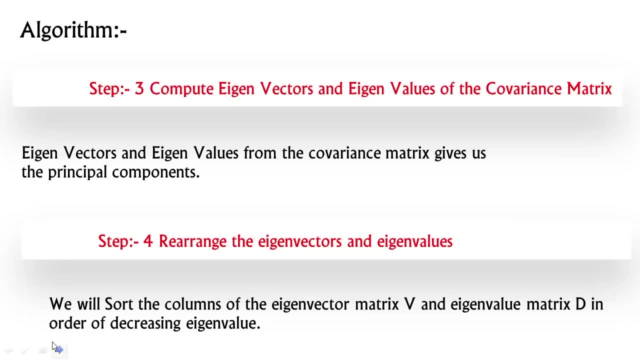 have to compute the covariance matrix of your data. it tells you how the input variables are varying from the mean with respect to each other variables. okay, because it's sometimes important, because some variables highly correlated and they contain unnecessary information. okay, the next step is computing. the is in vectors. 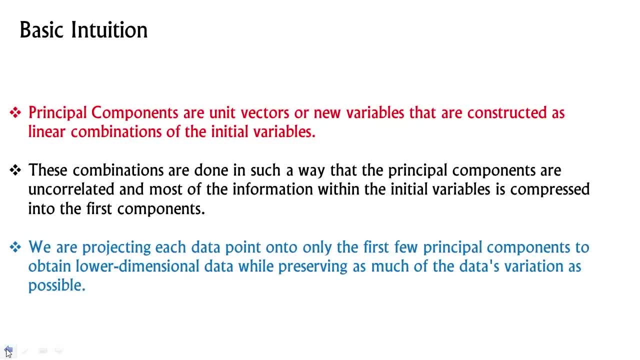 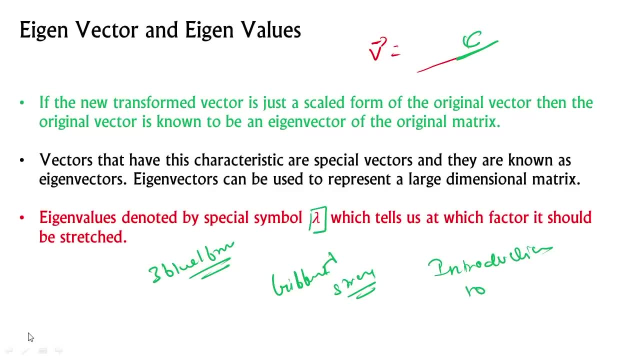 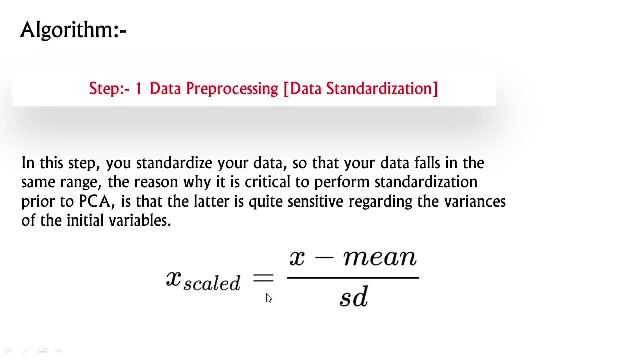 and is in values of the covariance matrix. so let's review what we have seen so in is in vectors. we have seen that if our new transform vector is just a scale from the original vector and the factor is called the is in vectors and the factor by which is stretched is known as is in values, okay, so that's the is in. 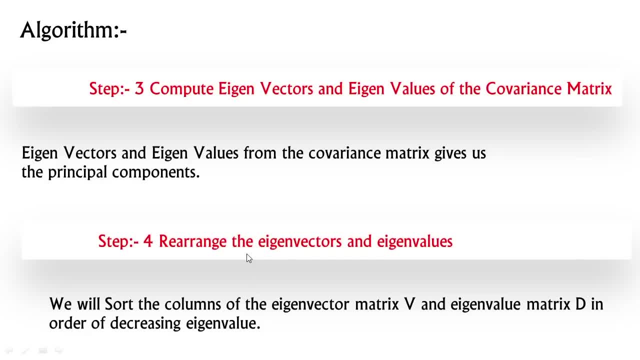 vectors and is in values. the reason why I made this PPT is if I write in blackboard, that will be not beneficial for you because I would receive same. so I had made it known so you can have a look on in the future also to see. 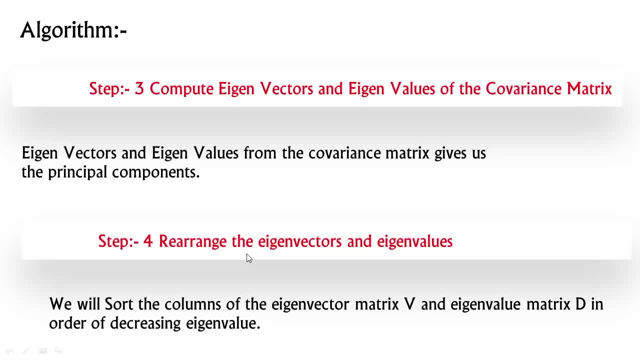 how it's working and it's better to have a text onto the screen to while you are listening, okay, okay, so what we do? you compute the is in vector and is in value of the covariance matrix means you come from. is in vectors are the transform vector from the original vector and the factor by which the is stretched is. 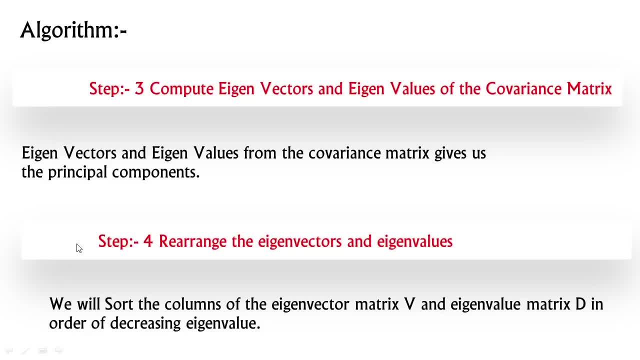 called the is in values. okay, you can easily compute the is in vectors and is in values in Python. and then what you do you sort the columns of: is in vectors- matrix V- and is in value- matrix D, in order of decreasing value. what do you mean by the step four? let's say you compute is in vectors and is in values. 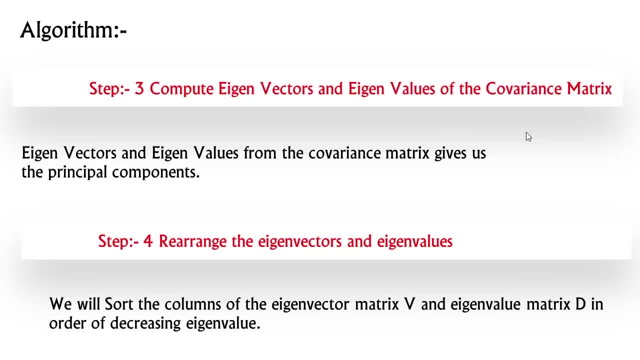 and those who has high means, high information or high numbers. so you just sort them means the larger were in the first and larger were in the first and larger the second, second, third, fourth, fifth, sixth, seventh, like this: okay, and then after that, what you do? you simply, you say: oops, let me do. 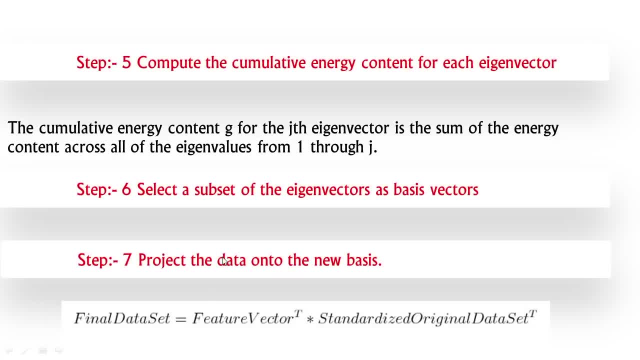 that you simply compute the cumulative energy content, how much the content is. each is in vector is having okay, and then you select a subset of is in vectors as a basis. vector means, let's say, and you are in cyclone, there is a sorry in any other. you should choose how many, how many number of components to use and 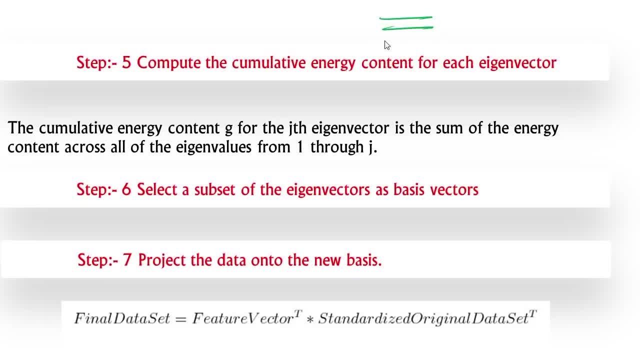 okay, that's the meaning. so what you do? you simply sort in decreasing, decreasing order and you come to the content of each item vector and then you select who has the high energy or content from the top, and if it is to be of, if you choose a principal component to, then only two highest, two highest will be. 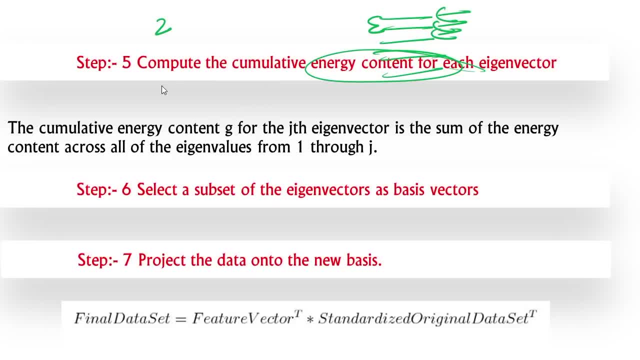 choose those who have highest number of information, okay, and then you take this, and then you take this to and to project on to the final. you project data on to the new basis, okay, so you, you have a large amount of again until, and then what you do? you remove this or you project this principal component on this. 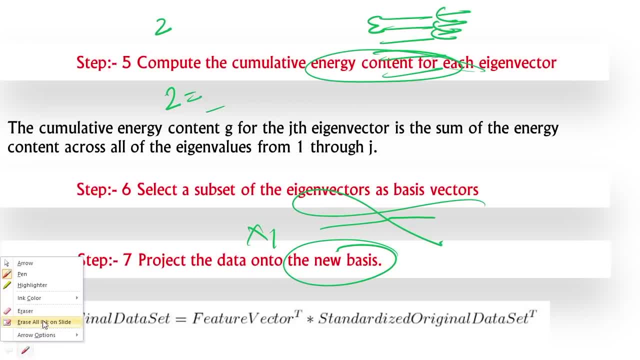 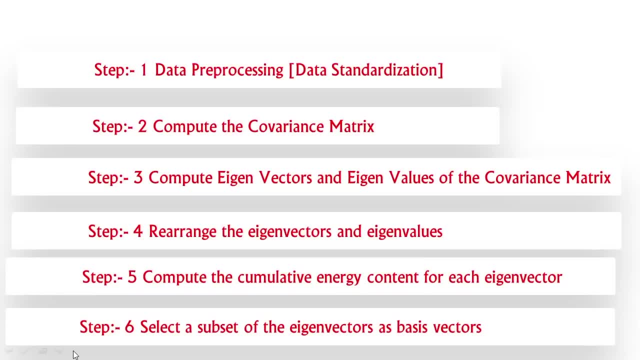 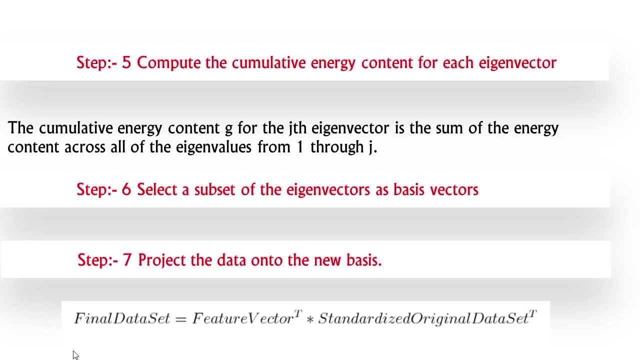 as a vector on to the new vectors. okay, and this is the formal analysis, randomized, and this is the feature vector to transpose. okay, so we have seen so far and here's the steps. what were the algorithm of steps? and I have not written last step, which is: 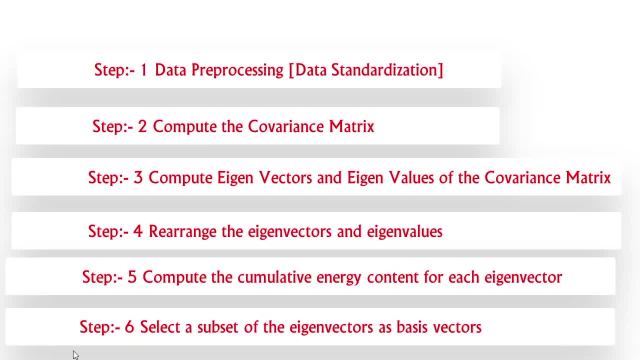 projecting the data. you can have a look, but because my kind of what's not fitting okay. so first you cross, pre-process your data, then you compute the covariance matrix, then you compute the Ison vector and Ison values of the covariance matrix, then you rearrange the Ison vectors and Ison values, then you 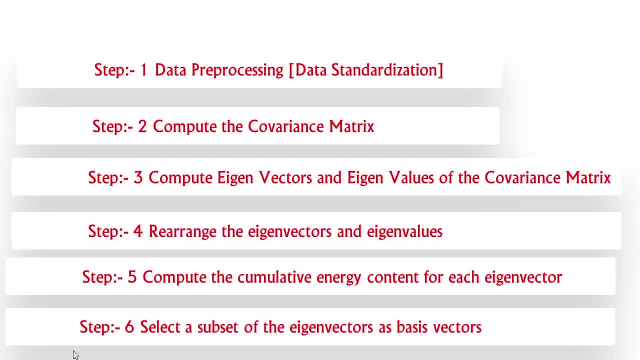 compute the cumulative energy content of each Ison vectors, although it is not necessary, because we, when you sort the decreasing order, you, the top, will be having the highest information, and then you select a subset of the Ison vectors as basis vectors. okay, so I think that we have seen so far and I 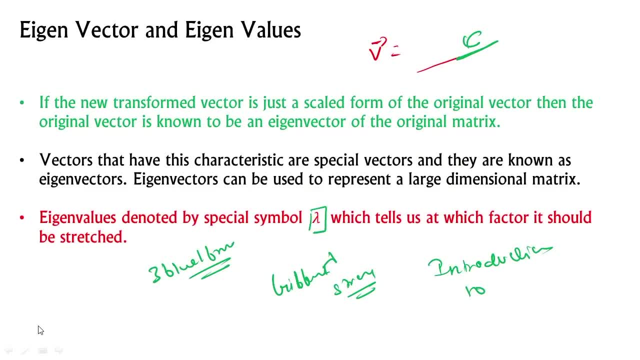 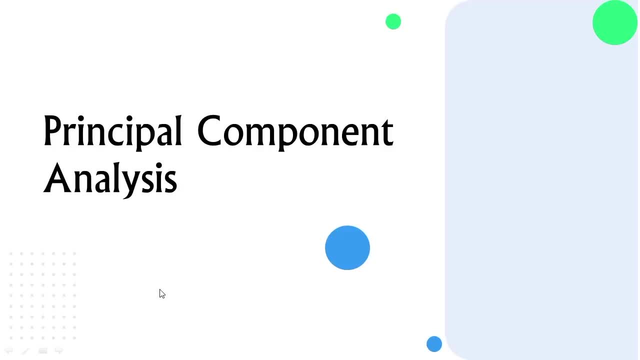 really, really hope that you have enjoyed this tutorial and in this section previously I think you may find is quite intimidating. now I think that you are able to grasp that concept of linear regression, logistic regression, support vector machine, principal, common analysis, and then we have coded projects and then 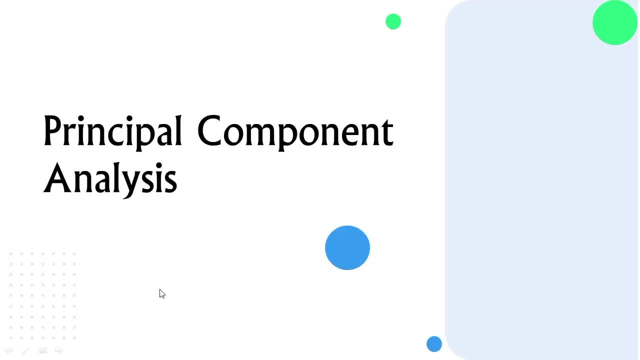 you have coded Boston house price prediction, stock price prediction classification project. you have coded logistic and linear from the scratch. now in the next section we will code principal component analysis from scratch. we will do by with ourselves to get the more feel of the principal component analysis. okay, so I really hope that you have enjoyed. I'll be catching up your. 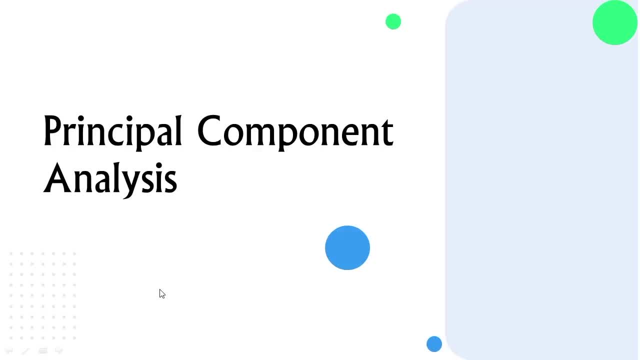 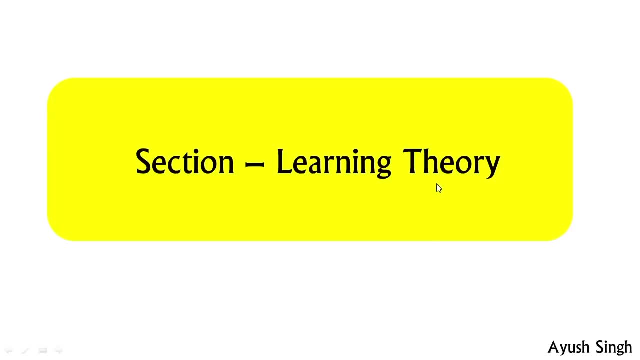 next section. so let's start with the next section to learn something new. okay, so now we'll start with learning theory. again, one of the most important concept to learn in machine learning- and, I think, gaining some something or less- we will see the topics which will study in this course, in this section- is: we will see why it is. 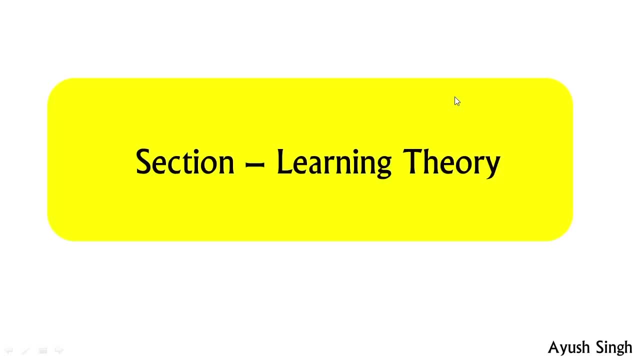 very important means. maybe it might look a little bit more nonsense over here, but maybe if you are going to deal advanced version of machine learning like deep learning or NLP or computer vision, it should surely make sense type that learning theory actually works. and in learning theory in this section we'll 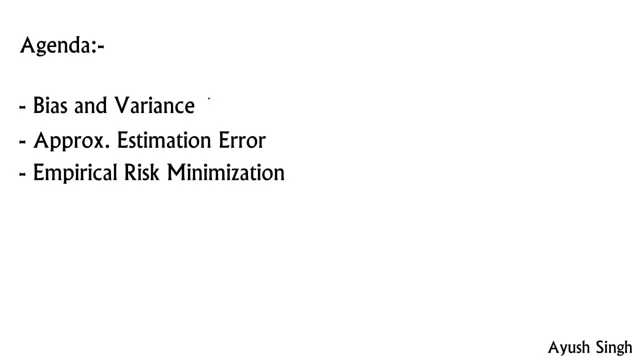 learn about these three topics, our main main, communicate main, talk on to this, like bias and variance, trade-off, and then it will move on to approximation, estimation, error, then we will move on empirical risk minimization and this, this will be our new concept, this, this, this, this will be, this is, these are two. 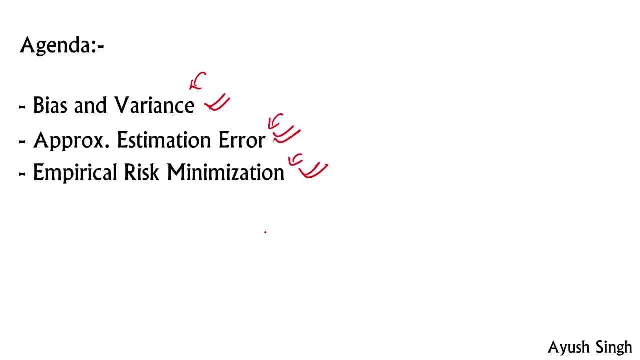 just a definition, just I didn't just just a, just a problem framed. okay, just a definition which, which is, which is needed because in many of the research papers they have listed empirical risk minimization or approximation estimation error. the reason why they have maybe some in history they may might be have different- 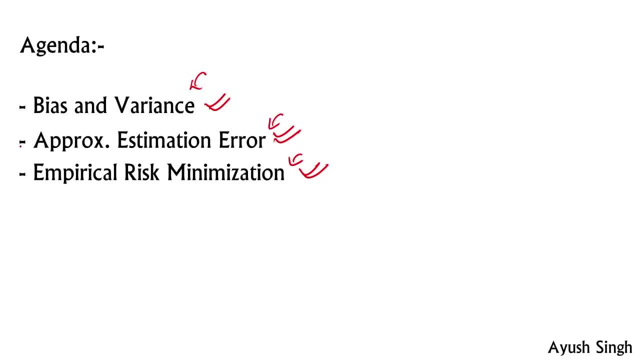 something out of different choices. okay, so we will study and we will just see the definition of this, and, and it will surely make sense, but if it is not, please be sure to ignore it for now, continue with this course and you are free, feel you feel free to come again. 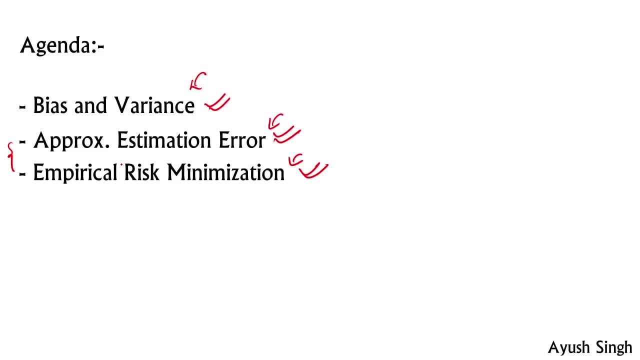 okay, you're feel free to come again and then watch this to concept, because it will surely make sense. okay so let's start with bias and variance. okay so, in bias and variance here, we will study about bias and variance, trade-off. and here is a warning: warning is is, warning is is. this is one of the easiest concept. 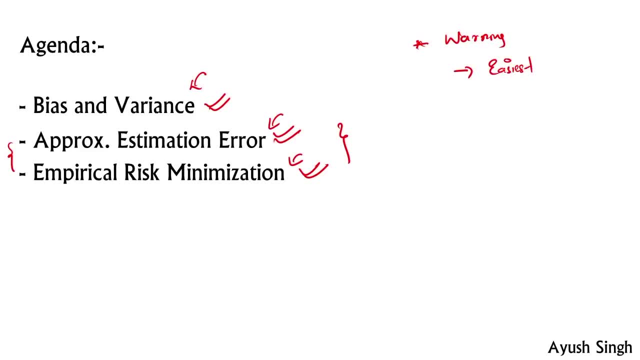 to learn as instructed by. even. however, I heard that is easiest concept to learn and it seems the easiest, but it's a very hard to master, very hard to master, and I hope that you heard and you're done saying this, and I think this. this actually makes sense. if you're a beginner, then it might not because you 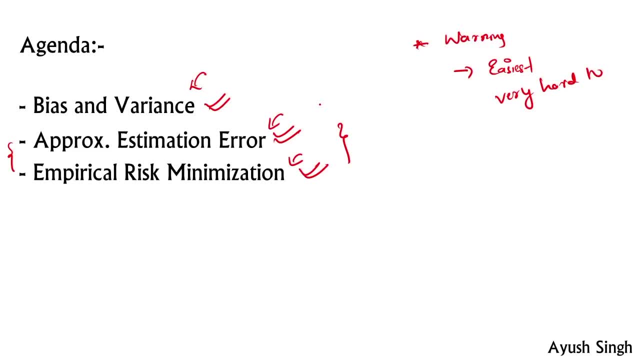 will understand everything but it when you really are actually developing the product. it's a very, very important to keep track of bias and variance, trade-offs- and it's asheron, okay. so let's start with bias and various. before that, we are going to recall our two problems, which is a 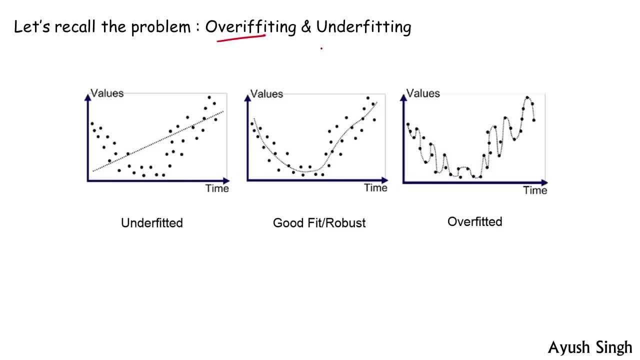 My favorite over fitting. oops, not my favorite, It's a over fitting and under fitting. okay, so here is my favorite diagram from the Google. so here Let's assume that we have a time and x axis and values and y axis. Okay, so maybe some kind of problem, okay. 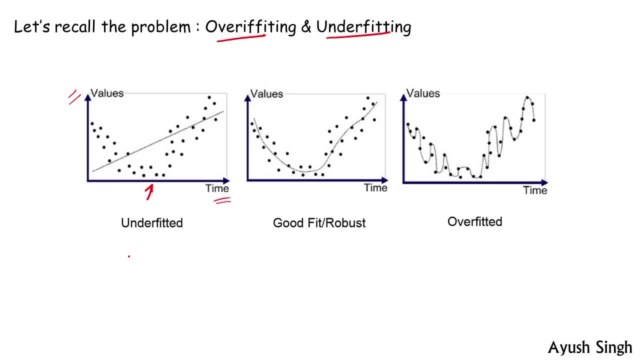 So here you have these data points, here you have this data points And what do you do? you just fit a straight line means a simple linear regression. simple, simple Linear Regression. okay, you just fit it a simple way in your regression, which is just theta 0 times. 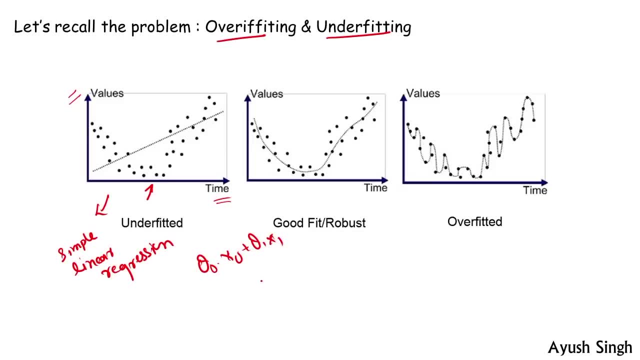 X 0 plus theta 1 times x 1- okay. so plus theta 2 times x 2: okay. so Here you just assume that we have a straight line using a linear regression. Okay, but you can see over here that the train it is not performing well on a training. set also means 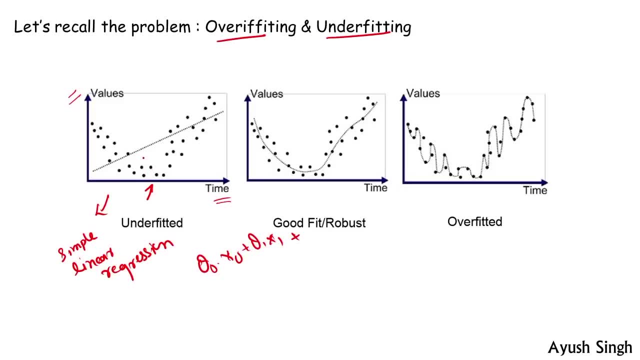 This is my training set, so it is not performing well. the residual error or the cost function will be very, very high. It will be very, very high, Okay, the cost function, which is J of theta, which will be very, very high in this case. so we call it as an under fit. 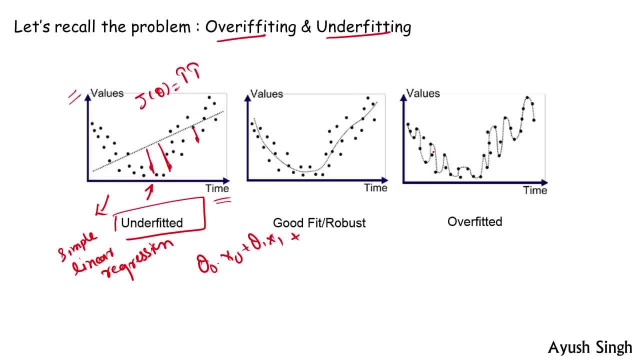 Okay. so the major problem, major, major, major problem that make this problem occur- is That we have a low amount of features, low amount of features, Or you have low amount of data, or you have a low amount, or you have a low amount of data. okay. 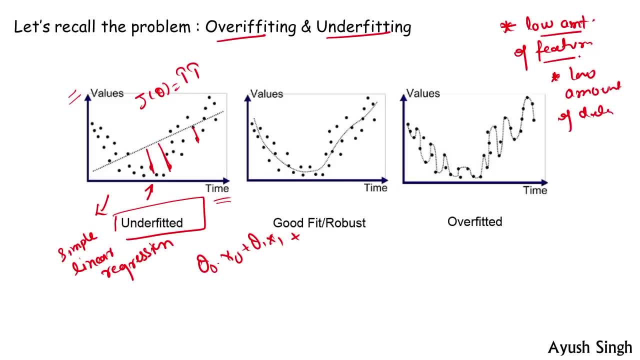 So these two causes the problem. so you low amount of features, low amount of data- Okay, and that can be good, that that can be sense using just by Adding more data or adding more feature. or if you don't have feature, you can do feature engineering To generate more features. okay, so just to do not focus on feature engineering for now, because it's not a dead data science course. 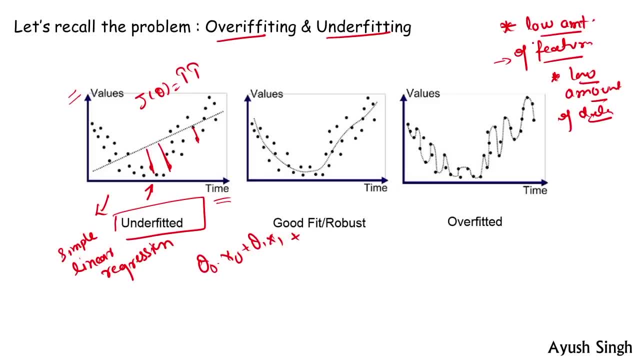 But obviously you just need a simple feature. engineering means it's just generating more features based on our feature. So let's, for an example, that you are building a spam detection system. So let's assume that that you are building a spam detection system where you have a one column. 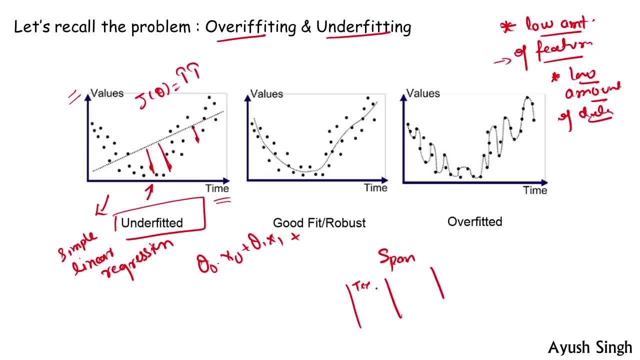 Which is of text. another column which is the label, whether the in, whether that text is a spam or ham. So it is a label. okay, So you can generate more features Like length of the text, what is the now, how many number or what is the number of a text in that? 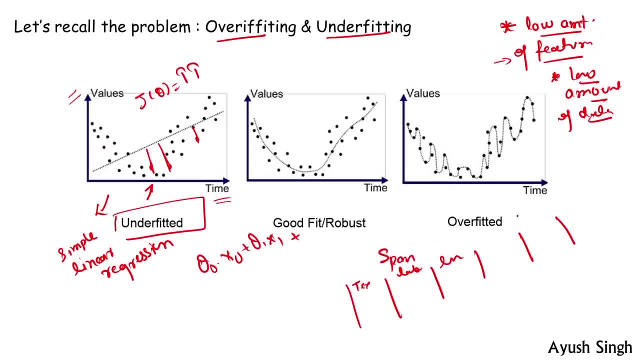 What is the number of a words in that text? What is the number of a character? so you can, you take, you, using this, this, this text feature, you generate more, three features And that's called a feature engineering. okay, So I think we, if you, if you see, are they very happy to make a video on a feature engineering, okay? 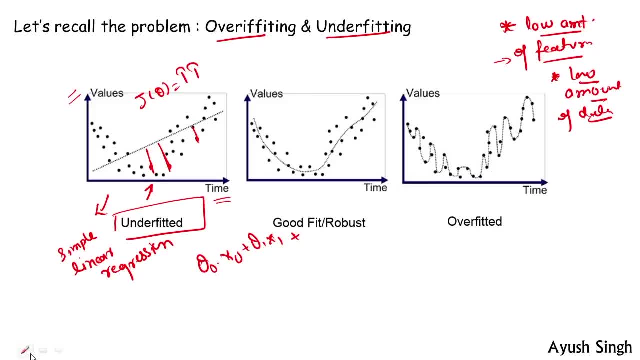 It will be. it will be a full place day data science course. okay, so here after this, We have our simple In your question, which is just like this: now This is called underfitted, and major root problem that I've seen so far in my experience is a low amount of feature stack that we have. 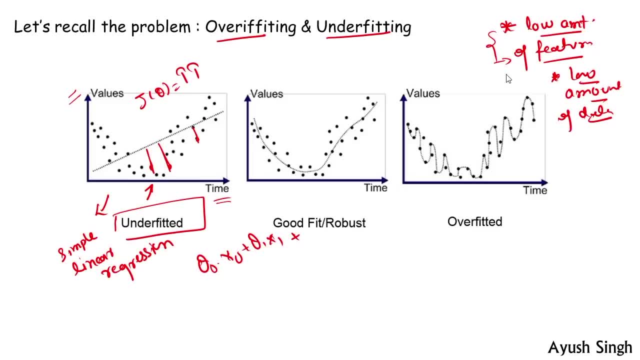 Okay. so in general, the underfitted me. the under under fitting means is just that your model is not Performing well on the training set and it's obvious that will not perform well on the testing set, So that's why we call this an under setting. okay, the next picture of here. 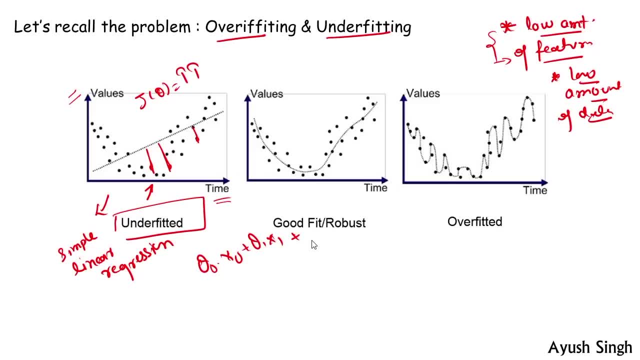 Is good fit. slash a robust, robust means it will. it will be very robust. It is a very good fit. you can see you, it is a very good fit. the cost, the residual error is low. the residual error Is low and it says we have a very good polynomial kind of thing. 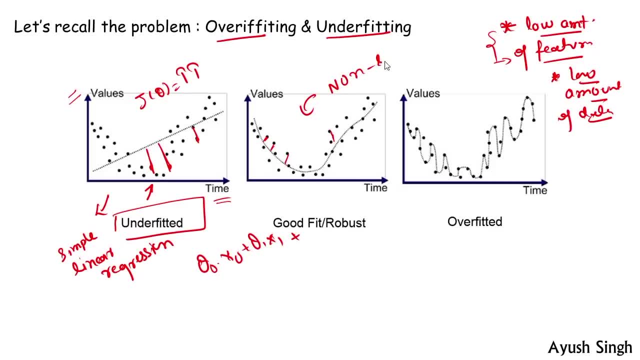 Non-linear or- or I can see I've against a nonlinear or a polynomial regression. over here we have applied polynomial regression and here's what we get the as a Hypothesis. okay, so here you can see, that is a very good fit and this is this is the robust model. 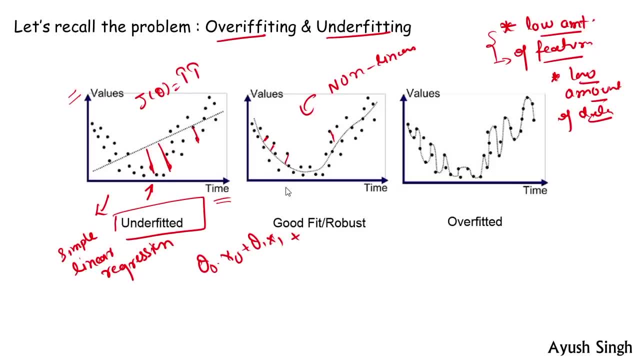 Okay, so we can say that this model is performing well on the training set as well as on the testing set, because whatever Example will come here, the residual error will be low. okay, so likely that is. the is a puffing well on a training and testing set. 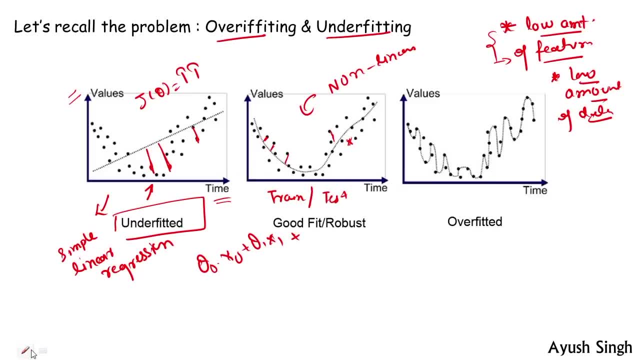 Another picture which tells you about overfitting. what do you mean by overfitting? overfitting simply means that your model performs very, very well. or I can say that your model wants very, very well on the training set, where your cost function, your cost function of J of theta is. 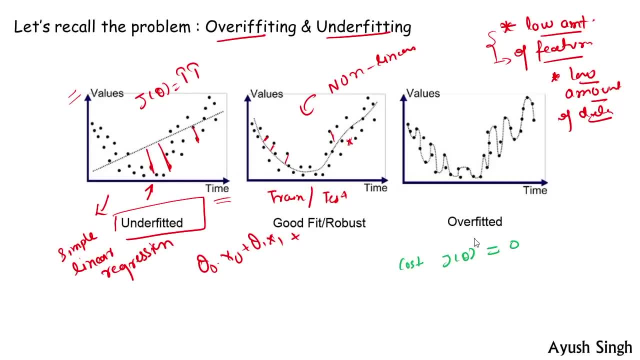 Equals to zero. okay, there you, you don't have any residual error. or approximately equals to zero, okay, So your cost function is very, very low. so you can assume that your model learned a lot. So, just touching each and every example, your model learned a lot. So that's why your cost function is very, very low. and cost function is just in order by the submission over I equals to one. 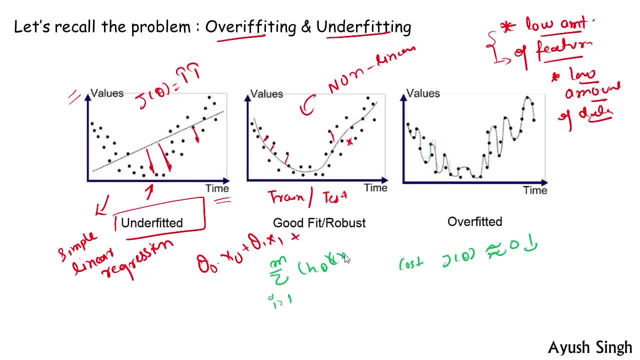 all the way around to the end, at a H of X, I, H of X, I Minus Y, I squared, okay, And just taking out the difference between the predicted and actual value. and here the Predicted and actual value are on the same line. so here you your model on the very nonlinear. 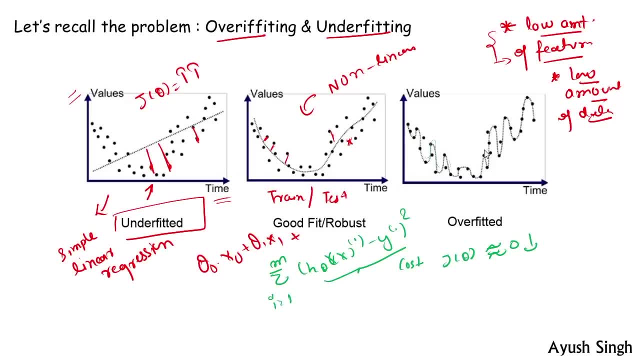 Hypothesis it all. it happens that if, if you have a lot of features, lot of features, and Here you have a low features and here if you have a lot of features, that happens okay, and Maybe you have used too much a degree in polynomial regression. 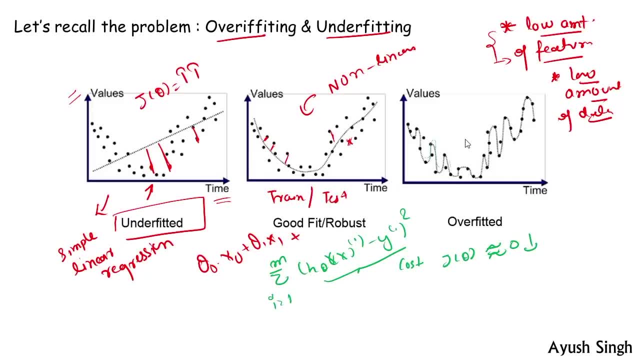 So that's why it happens, or maybe something that of a rather not a very kind of complex architecture, Or you have, or you have made a very complex function of effects with the highest degree Explorer, etc. like that, like that. okay, So this is, this is the, this is the problem for overfitting, and whatever new example come over here, your model will be very, very high. 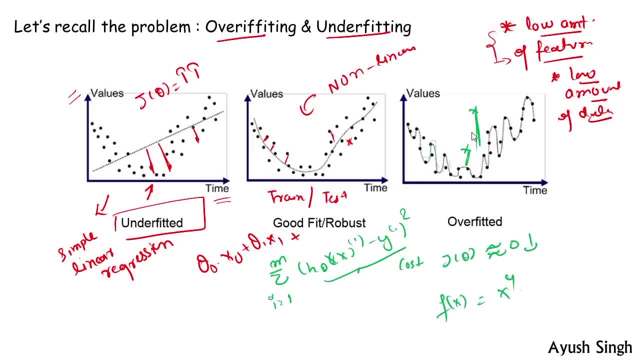 Whatever come here, the residual layer will be very, very high. okay, so your model will fail to generate Generalize. well, on to the new training examples. okay, So the in general overfitting means. over overfitting means that your model perform bad, Or or against. here model perform very, very well on a training set in which your cost function is low is 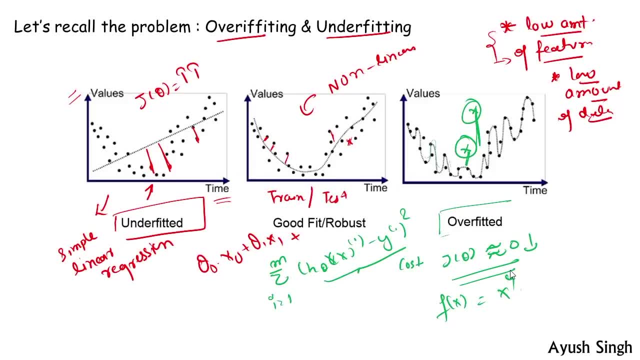 Is equals to zero, which is actually good, but, but you, you may think it is good, But just just wait that your testing set error is very, very high. okay, so that indicates the problem of overfitting. so We can prevent overfitting by selecting some of the important features. 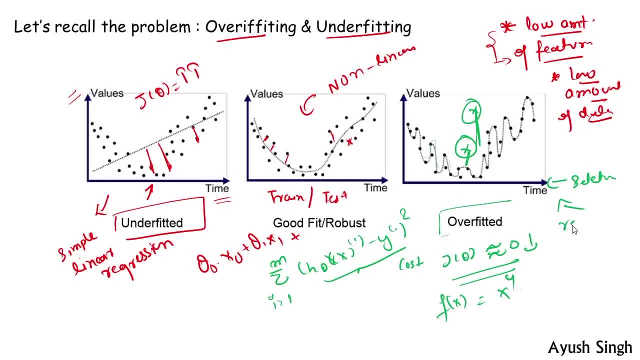 selecting important features or Regularization. so regularization is just an advanced version of selection of features, so let's see what it does. okay, so I Have already told you about regularization now in our regularized linear models, and I hope that you understood that. okay, so now we will. 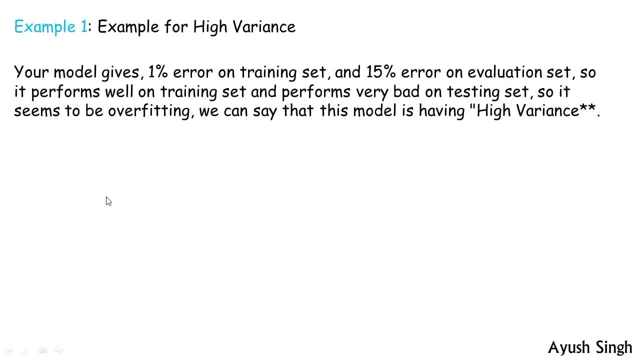 See the bias and variance Straight off by taking a look at some scenario of your model. okay, so let's assume that you are building some model. Okay so you are building some model and your model gives one percent error. one percent error on a training set. 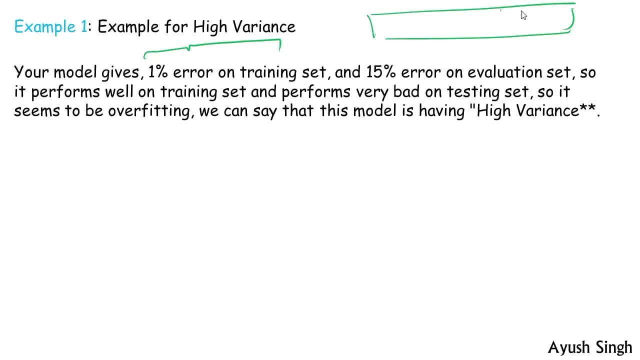 So you have one training training set like this, and you divided this training set into training and Evaluation set, so you have this whole data. you have this whole data and you divided this in training and evaluation set. okay, So what you've done? 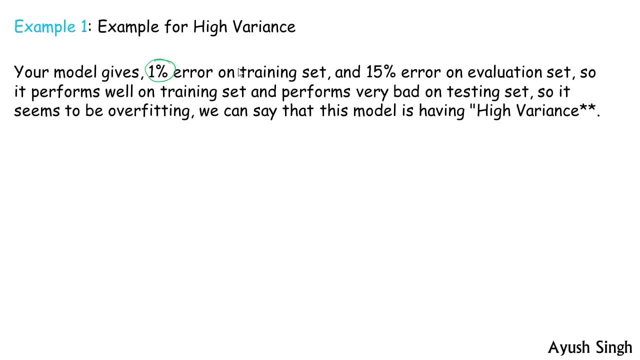 You've taken a one percent error on a training set. one percent error on a training set, which is, if you see, oh yeah, you one percent error, one percent error on a training set and Fifteen percent error on the evaluation set, so you can assume that your model is. you can see that your model is overfitting because 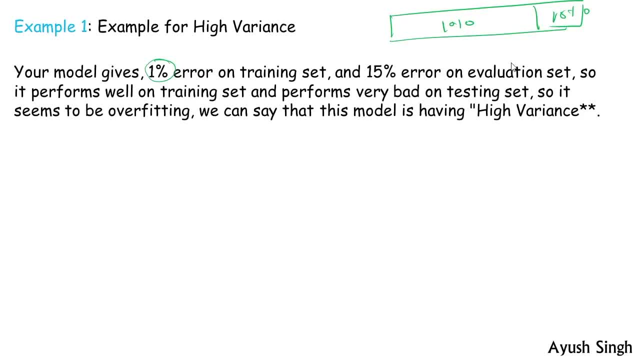 Your error is very, very low in training set, but your error in validation set is actually fifteen percent, Which is very high. okay, according to this. okay, So it Is performing a very, very well on a training set, but it fails to generalize well on a testing set. so it is. 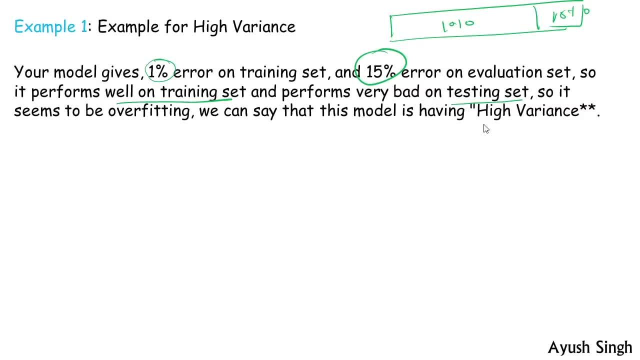 Overfitting and in this case, we say that the model is having high Variance and we use bagging. we use bagging to reduce high variance, Which you will see in ensemble learning methods or sections. so don't don't worry, you can come back again to this section to watch this. 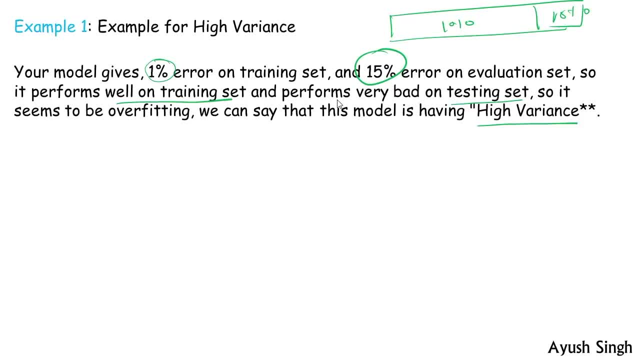 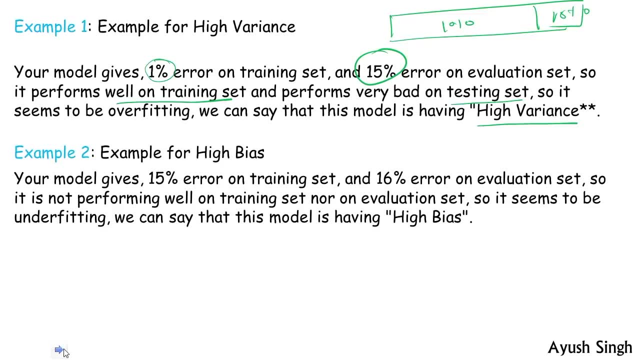 Okay, so this is this is how you added: identified if your model is having high variance. Next next is that let's assume that your model is giving a fifteen percent error on the training set, on the training set. Okay, Fifteen percent error on training set and sixteen percent error on it and on evaluation set. 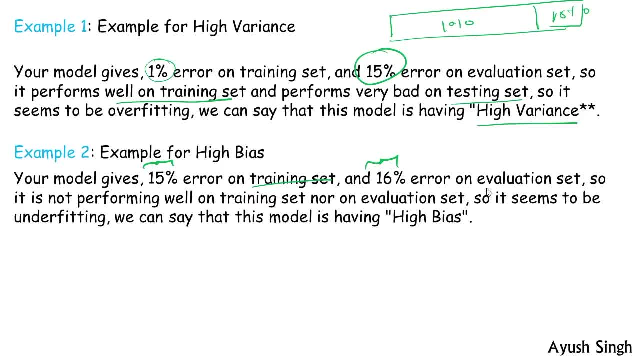 So it is not performing well under training set, obviously to not perform well on an evaluation set. So it seems to be under fitting. so here it has high bias and use boosting. use boosting to reduce bias. Okay, so this is this. this is what I'm saying, and 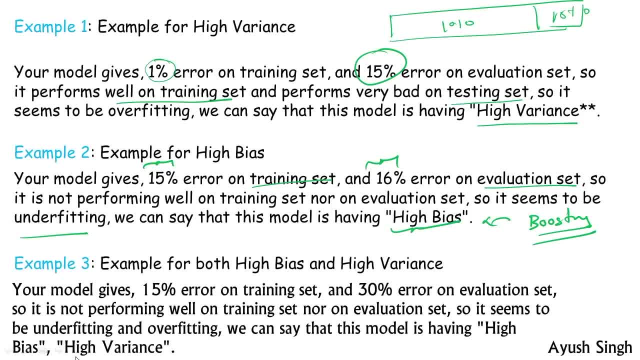 Let's take. let's take for that, for the sake of an example, again example- that your model is having both high bias and high variance, where you have a Thirteen percent error, which is obviously high variance, and 30 percent error on evaluation, which is obviously high bias. 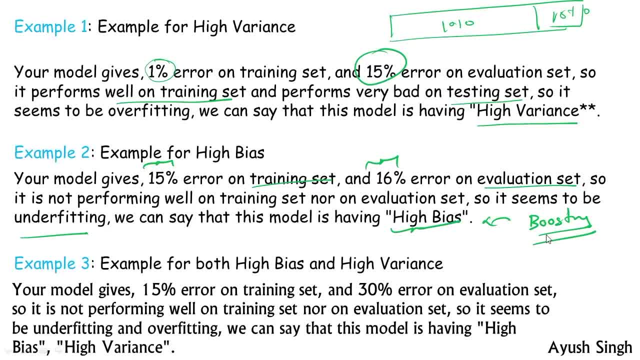 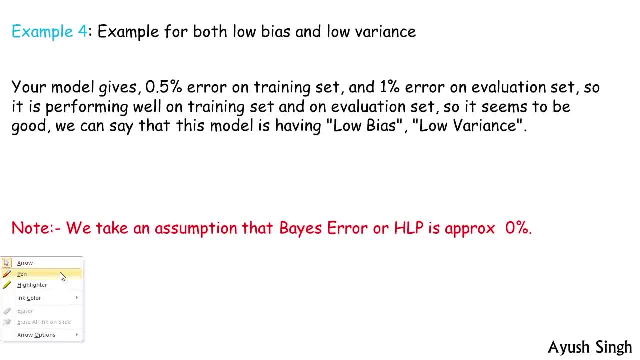 Okay, so it is both overfitting and overfitting and obviously it has a high bias and high variance. Okay, the next, our favorite, last example of this bias and variance trade-off is: Your model gives 0.5 percent. model gives 0.5 percent or training set and one percent on the strength testing set. 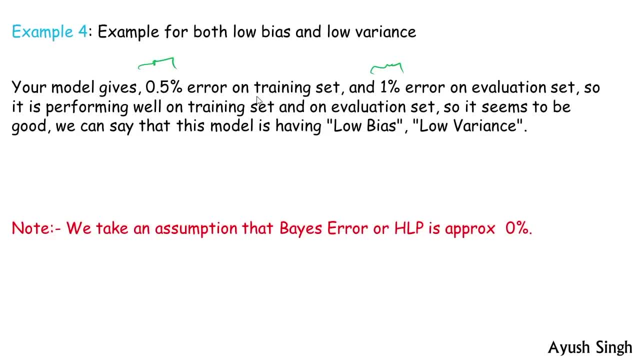 So it seems to be a perfect model or a robust model. There is not learn too much on training, certain book. It is very robust and good model. Okay, here it seems to be a good, so we can say it is. it has a low bias where it has a very small. 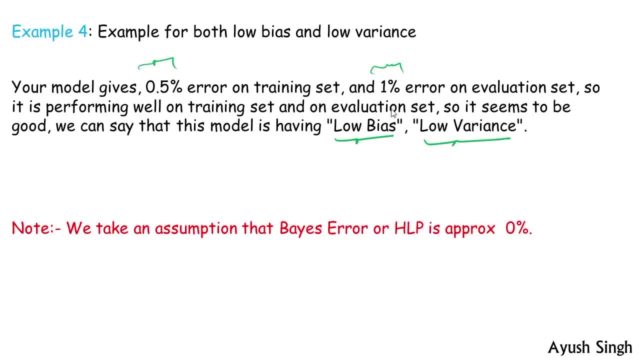 Error and it has a low variance where it has on training set is a very good Okay. so this is this is what we consider for low bias and low variance And all of these, all of these, we take assumption. Do you know what assumption hopes? you don't know, but because you're watching. but 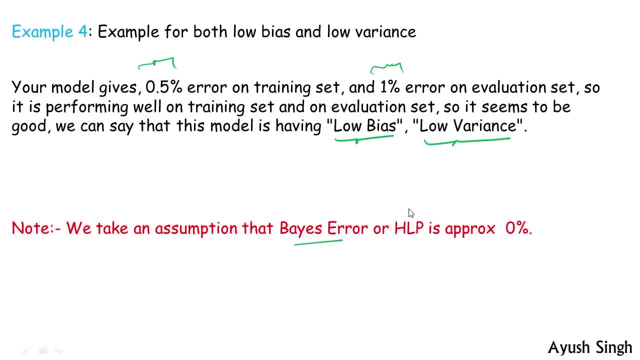 we take an assumption that base error or human level performance, or human or human level performance, human level performance is Approximately equals to 0%, as approximately equals to 0%. So what do I mean with this assumption? I, what, what? what do I mean? 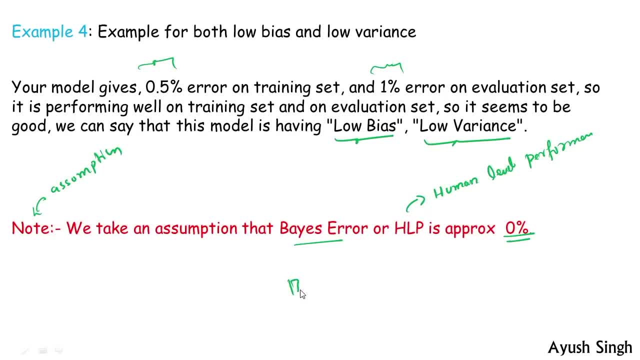 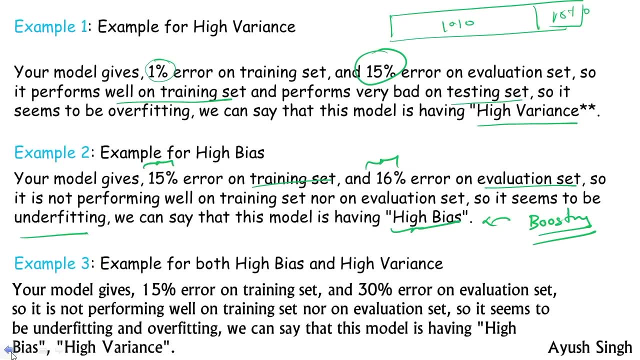 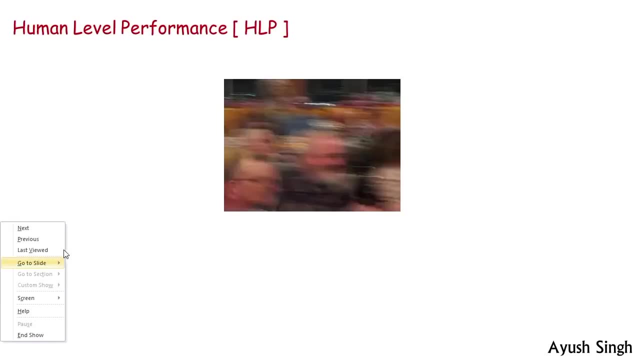 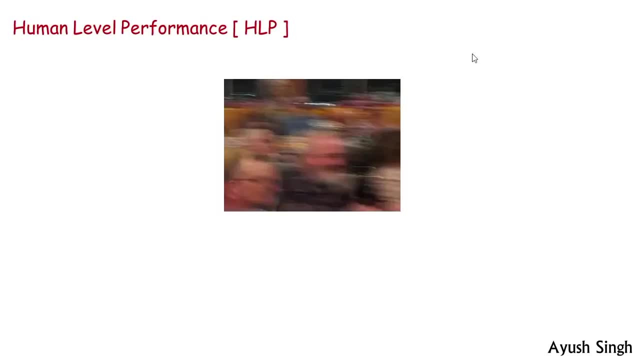 a some Classification model, or maybe the face detection model. okay, so your, bill, your, you have built a face detection or face recognition, our real-time facial cognition. so your, our Algorithm. even you will fail to identify this person. even I will fail to identify this person. the reason why? because it's very blood, very, very, very blood. okay, 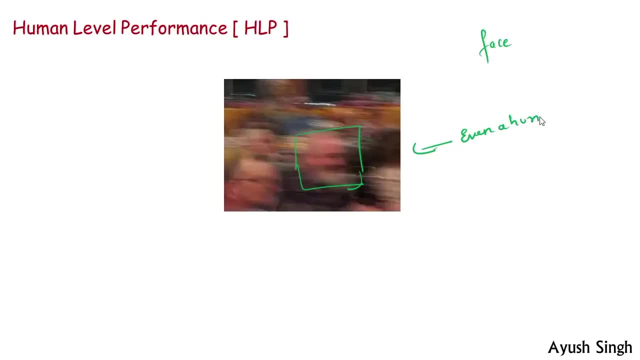 So, even a human, even a human Human error, okay, HLP, you, even in human error, will be very, very high, very, very high, because it will be not able to. He will be not able to either Identify who's this person is. okay, so, so so, and then you can cannot expect. 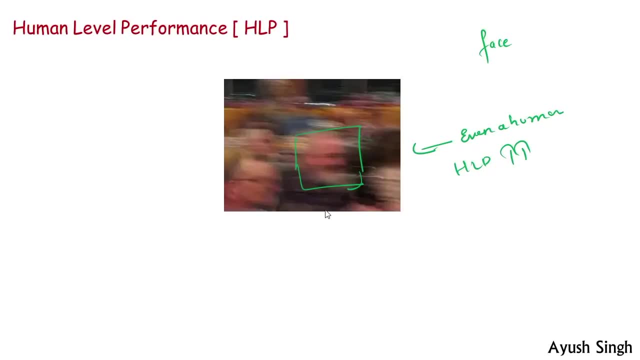 that your Model should be a very great over y'all, you can expect that your model, as very Your, your model- is also giving the same error as you are giving, because you are also not able to identify as well as your Model also not not able to identify. and actually this is not. this is here the HLP. 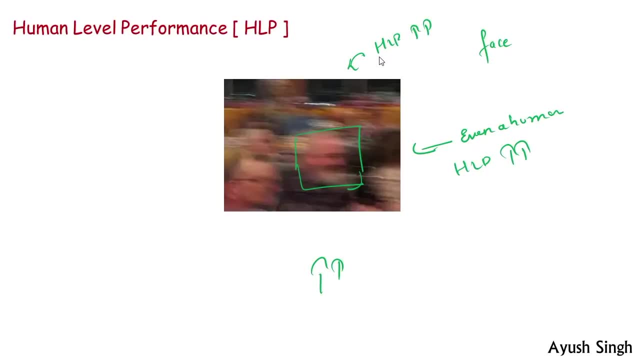 HLP is very, very high, or I can say the base error is very, very high. so we can say that here You can. you cannot expect your algorithm to work best, but let's assume that that you have a fresh image and Here the HLP is equals to 0, means human level performance is equals to 0 and you, now you can expect your algorithm. 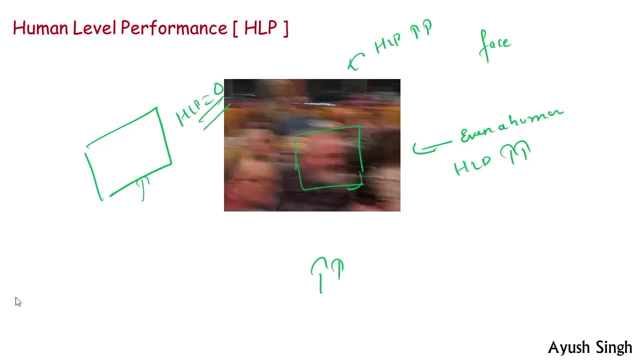 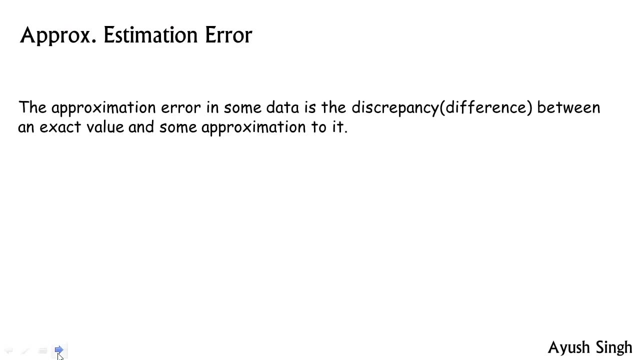 Performance to be good, because it is the human of performance is equals to 0, so that's called the base error. I mean, and I hope that you understood the next: We have talked about bias and variance trade-off. you can again rewind this video to understand again. 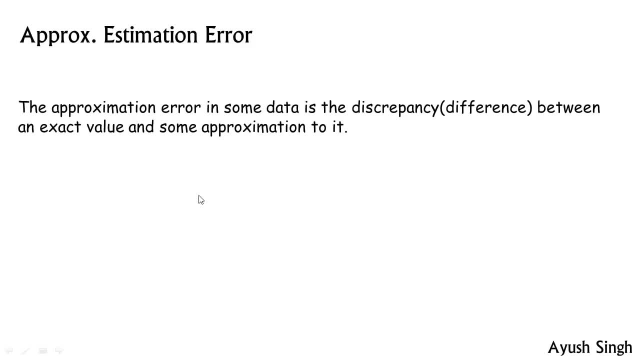 But what is that approximation, estimation error? This is just a definition. so the approximation, the estimation error in some data is the difference between exact value and the approximation of it. and this Approximation indicates your f of X means the outputted model, the output from the model. 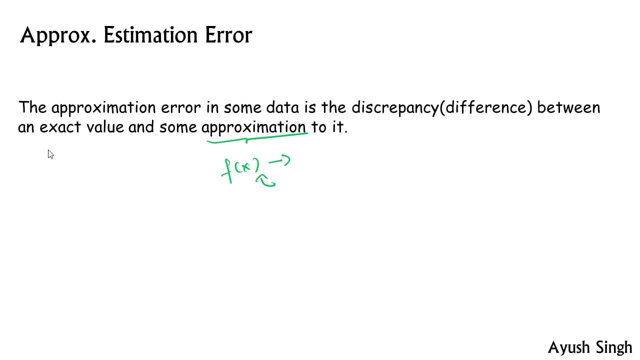 So we here your f of X given some approximation, and this is a ground truth, which is why I have: okay, So difference between these, both is called as Approximation error. okay, so here I've taken one example from Wikipedia. again is a scale example, but that's that's, that's general. 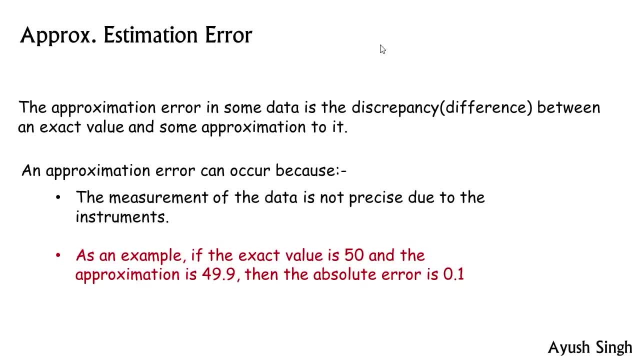 We mean I already told you nine cost function. you take out the difference between. that's an approximation estimation error. okay, So it's just like this: if the exact value is 50 and the approximation is for 49.9, Then the error will be 0.1. 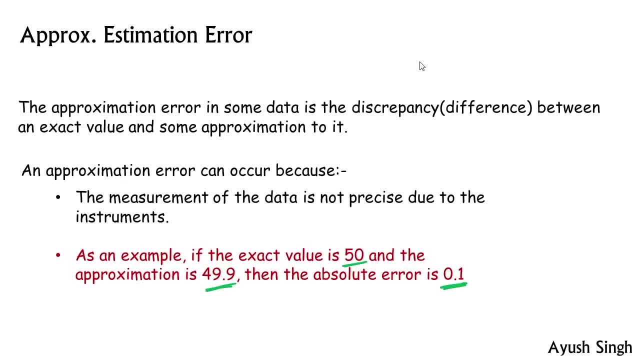 And that's actually what you do when taking out the error. for one training example, You just subtract this and the regression problem. what you do, use a subtract y, hat minus y and then and you get your answer Okay, and then you add some mission for every I, for every I. 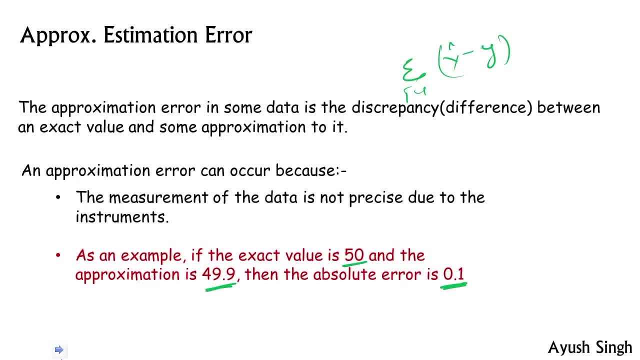 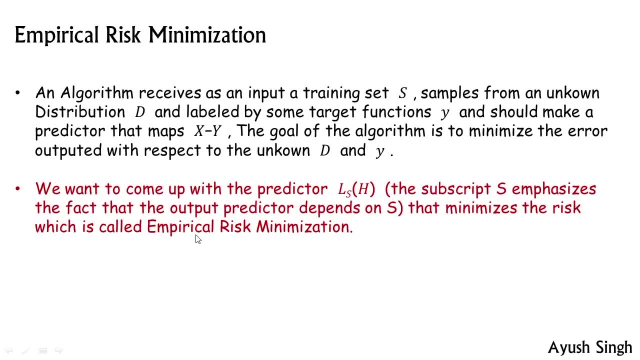 Okay, so this is what you do and this is just a definition, because you will see a lot in your research papers. Okay, next one is empirical risk minimization. again, We have seen so an algorithm receives, as an input on a training set s I'm going to adjust, I make you familiar with this what I'm saying, that an algorithm, 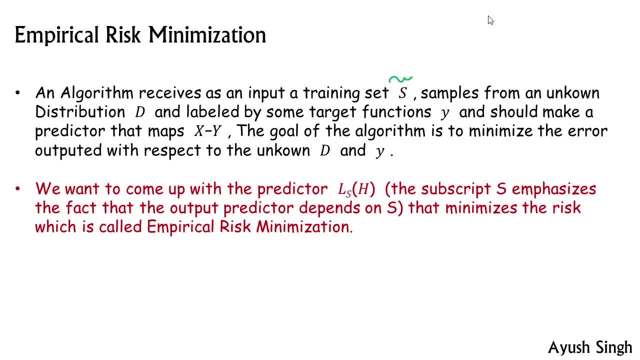 Receives as an input. a training set s means We get and we get our training set, which is a sample from the large distribution D okay, So we get our Sample from the distribution beam is large. We just take out some example and labeled by some target function: y okay, 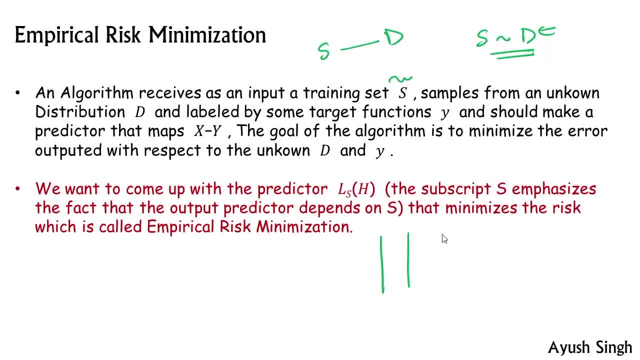 So here we have our training set as well as we'll be having the labels for it, because this is a, this is framed on Supervised learning. okay, so here we will be having label, as well as the samples for each training example. Okay, and should make a predictor. 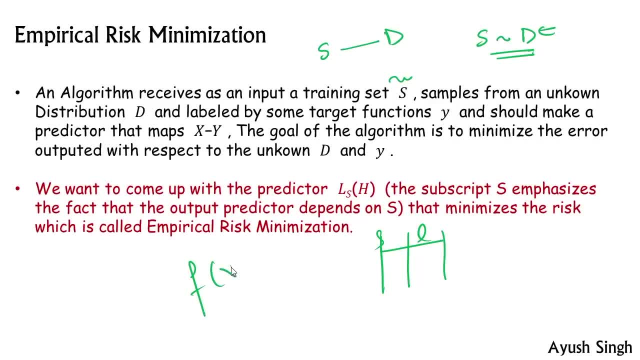 We should make an F the predictor that maps our input variable X. is these features to the output variable Y? okay, and the goal of this algorithm is to minimize the error output. it, with respect to the unknown D, means now we will feed a new example that a model has not even seen, and your model should be very 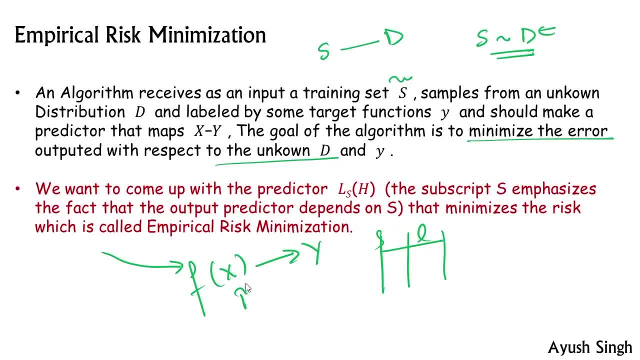 Minimal, or your audio or your model should be, or your model error should be very minimal. okay, So this is what the full definition is saying, And it simply means that we want to come up with a predictor, l subscript s s. we want to Come up with the l of edge with sub subscript s, where s emphasis is the fact that output predictor depends on s. 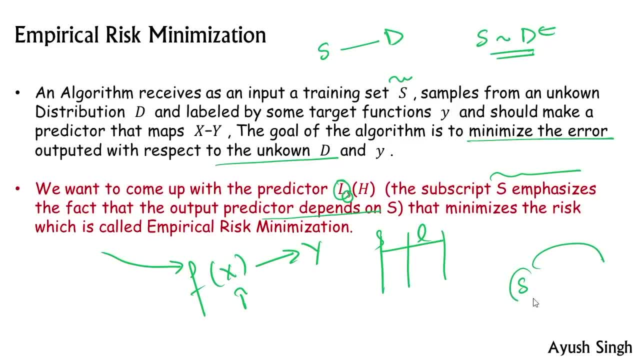 Okay, so, whatever the output will be, it depends on s, because we have taken, we have learned, We have learned the weights, we have learned the w, we have learned the theta 1, theta 2, all around, theta n, From these s. so that emphasizes, that Minimizes the risk or the error, which is called the ERM, which is called the empirical risk minimization. okay, 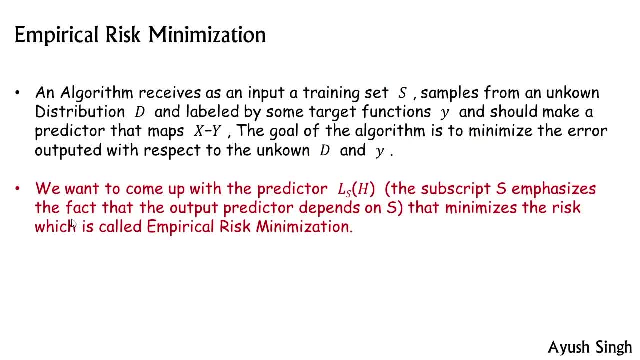 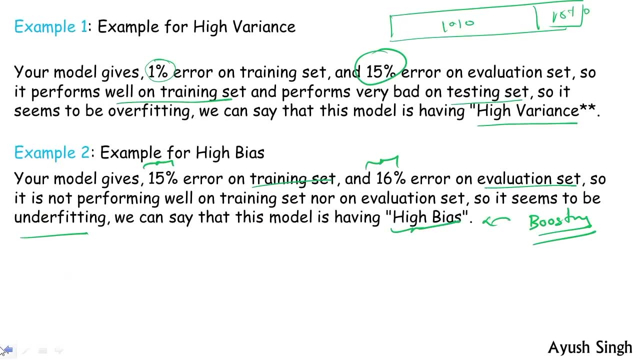 So I hope that you understood this concept very much clearly and I really hope that you had enjoyed seeing this section, and We- I have talked a lot on empirical risk minimization, Learning theory and etc. so I hope that you will utilize this way, and we have already talked about 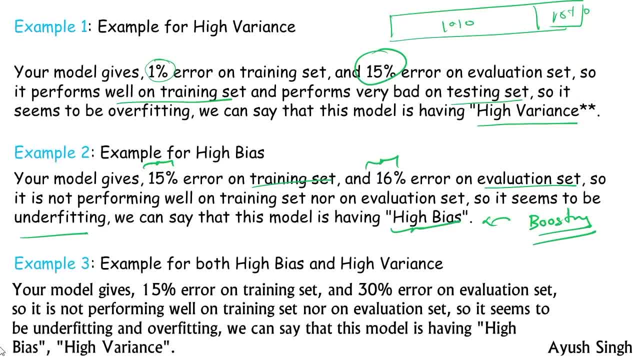 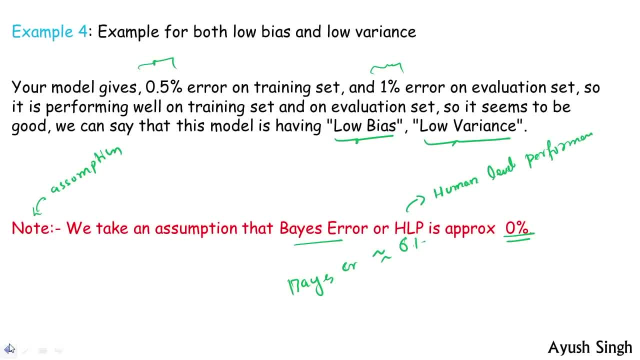 The job and now you can continue further if you. if you haven't understood anything, you can feel free to ask in the comment box below. I'll be very happy to take your doubts and be sure to have a look at the course website, Which is already available in the description. 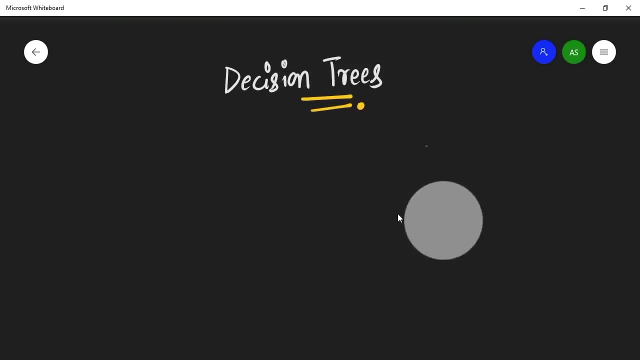 The box below. so meet you in the next section. Okay, a very warm welcome in this section. and in this section We will be talking about decision tree, one of my favorite topic to talk on, as I will go in depth of decision tree to Make you understand everything in decision tree with intuitive examples, with solved examples of decision tree, as I have seen. 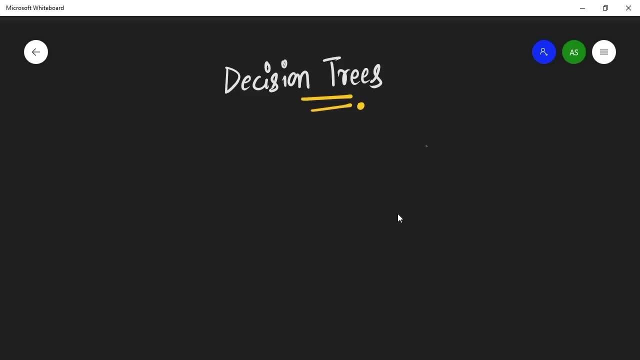 On YouTube that they are the. some instructors are doing great job, But they are not doing that. into decision tree means for free, so I just want to make you familiar with the certain tree. whoever is watching this tutorial into depth, And I really hope that you will enjoy this section. 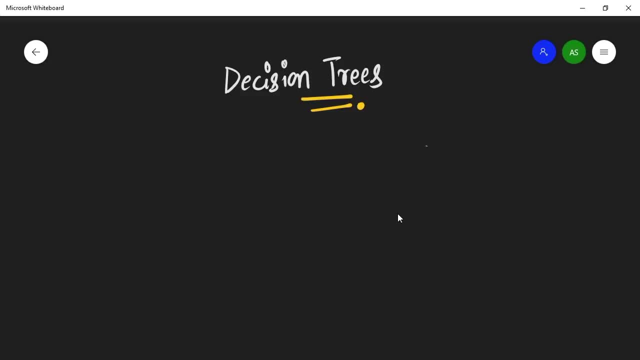 but before that, what we are going to cover in this section are as follows. first we will start with Introduction, geometric intuition, a basic intuition about decision tree, what actually decision trees are, and Then it will go further into How we building that decision tree. so for building, we will learn some sub tasks of concept, which is 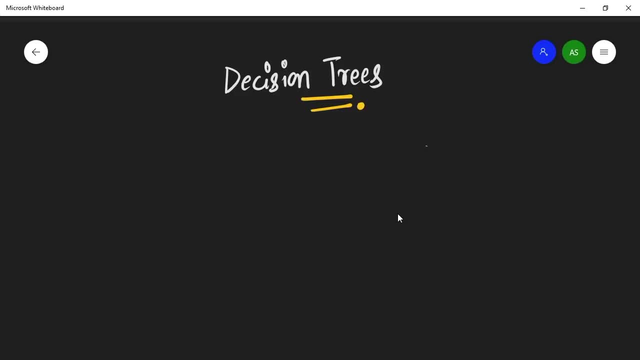 like entropy information gain a guinea impurity. okay, then after that we will build our own decision trees and then i will show you the implementation of decision tree. okay, but before that, let's uh understand the basic intuition of decision tree, as there will be more topics which 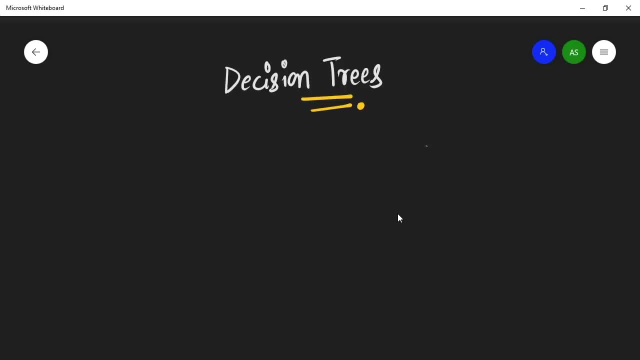 we will cover, as i will discuss later on. okay, okay, so let's start. so, uh, first of all, what is decision tree? this isn't. three is a supervised learning algorithm. okay, so it is a supervised learning algorithm, and what do i mean by supervised learning? is that we are having our 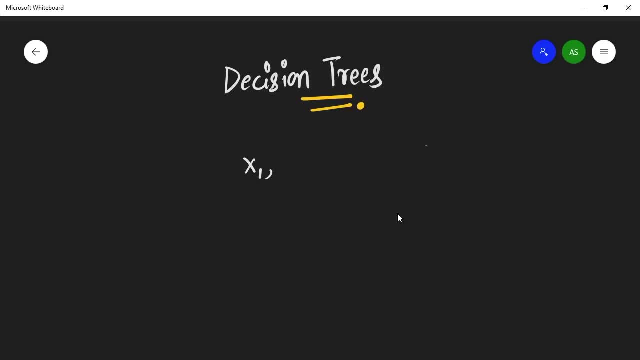 xx1 with our label y1 all the way around to the x2, then we have y2 all the way around to the xn and we have y. okay, so ever having labels. so it is a supervised learning algorithm and it is used for both like support of. 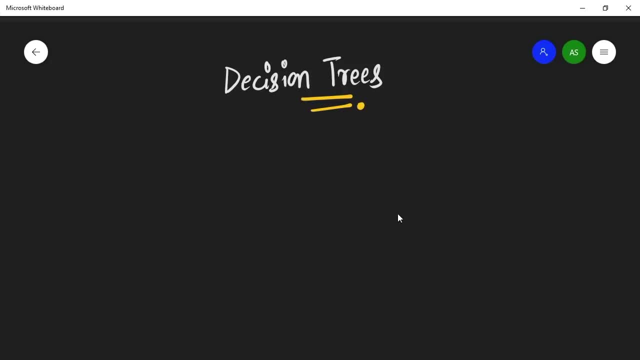 the machine is used for both regression, classification, so it is used for both classification and regression, okay, so, uh, you will see how we do, how we construct the decision tree like that. okay, so let's start with um the basic intuition of decision tree, so the definition of 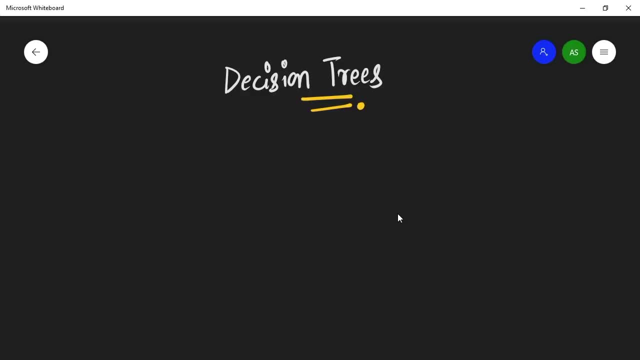 decision trees that they are nested if and else statements. okay, if you're a programmer, then you will be relating this concept, which is if and else, and the python is a prerequisite, or any programming language is a prerequisite. so what is decision? true, it is just a nested if and else statement. 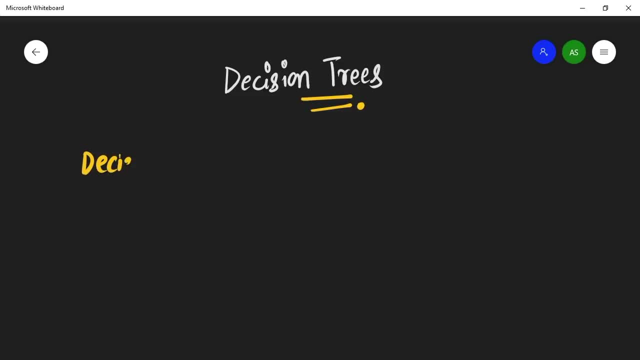 so it is a nested. it is a nested if and else a statement, so i don't know why it is so bold. so it is a nested if and else statement. um, so is what is just? you just ask a question and it splits the data. okay, so let me write the. 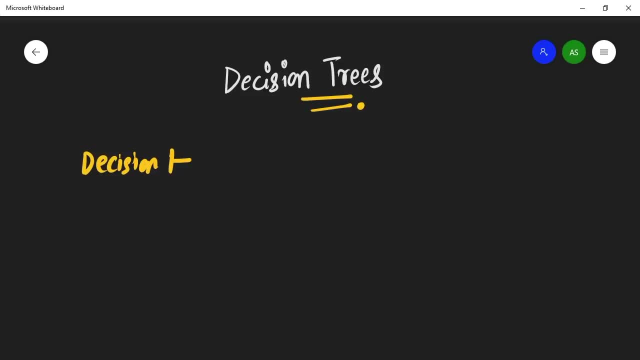 form of definition to make you more. uh, into which intuition behind. so they are nested, nested if and else statements. okay, so we just ask questions, is just ask questions is just ask questions and splits the data. okay, so it's just question and splits the data. so let me take one example of iris data set. let me take one example. 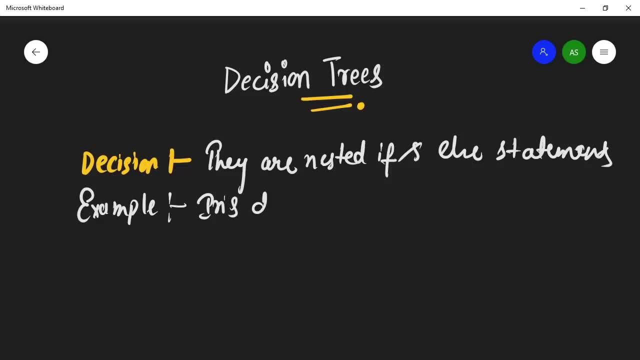 of iris data set. okay, so, what we do in iris data set. so, but let what? let let me make you familiar with what is that, this data set, to make you more clear understanding of this topic. okay, so, iris data set is simply like this: you have a data set which has four features like sepal length, sepal- 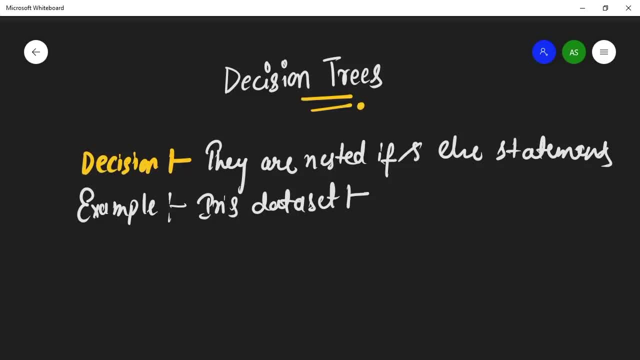 width. petal length. petal width: okay, and you have the label, which is the species of the flower. okay, so this is a task of flower species detection onto the basis of four features. okay, so this is a classification data set, binary classification data set. so you are having a like. 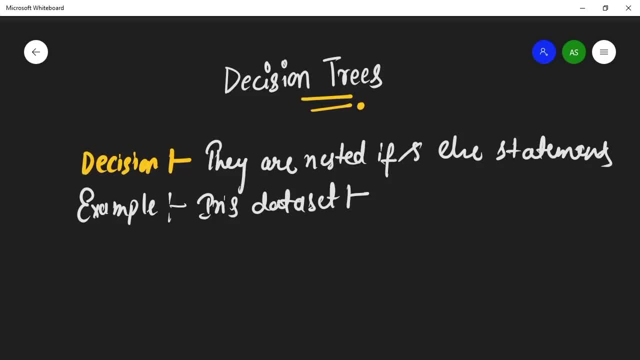 this, so let me change my color. i don't know why it is so bold. okay, so you, you have like this: uh, first you have sepal length, sepal length, and then i- i i hope that you understand what is sepal and what is petal- so sepal width, then you have petal length and then 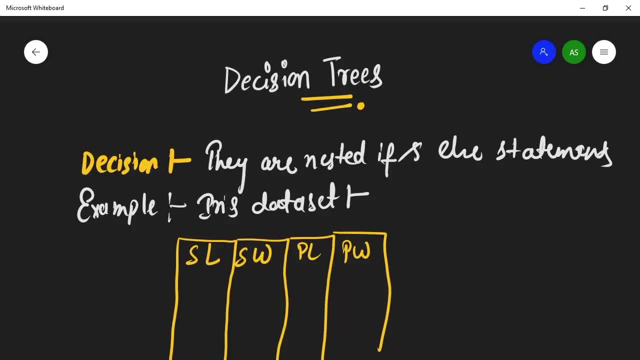 you have a petal width, okay, and then you have a one more column, which is the label, which indicates what is species. so let's take an example: 2.2, 4.30, let's say 3.2, 4.6, and the label is: 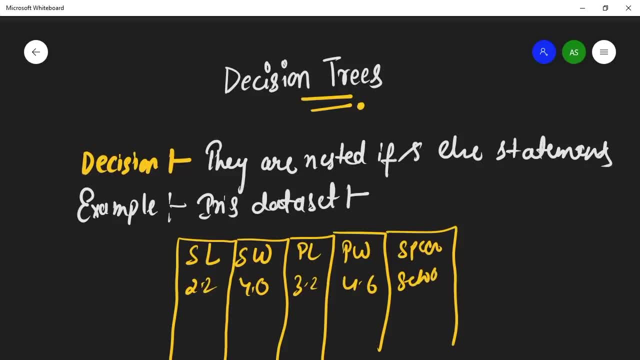 um, satosa, satosa. okay, so you have three classes in this data, set as a label, which is satosa, which we label as one, sorry, zero, versicolor, versicolor, which we label as one, and virginica, virginica, which is labeled as two. okay, so the output will be either zero means satasa, then either it will: 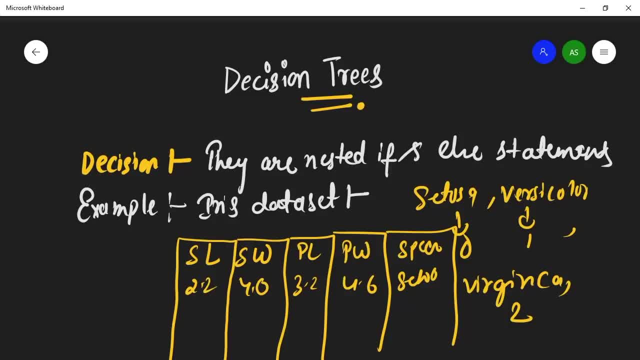 be one means versicolor or virginica, as in quote, versus two. okay, so that's the iris data set that i had just make you familiar with. okay, so let's what? what we will do. we will not make use of any library. we will not make use, and then anything we 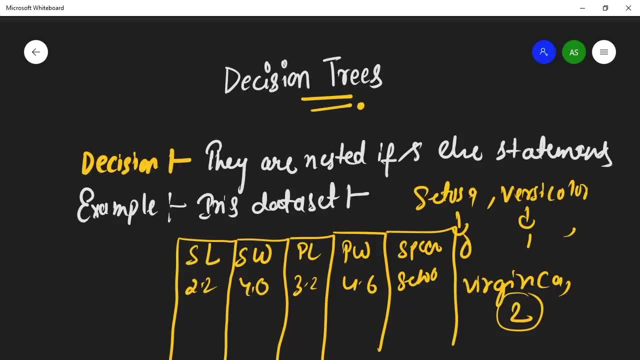 will simply what what we will do. we will simply make a decision tree by yourself, by making just if and else condition. okay, so we'll make a simple classifier. obviously it is not so formal, but we'll make a simple classifier that will simply classifies your flowers. okay, so that's what. 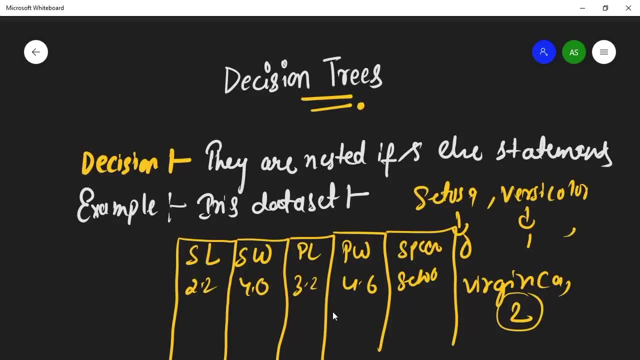 we are going to do so let me remove this and i really hope that you understand what this data set is and more uh understand. if you want to more in detail about what the data set is, you can search online. this is a famous data set, like iris tape data set, which is just for flower species detection. 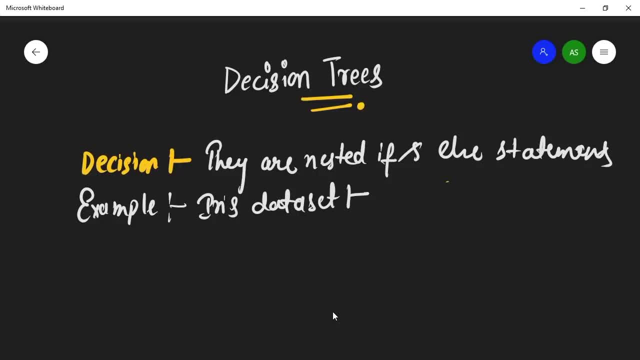 system. okay, so let's start. so first, uh, uh, here we have an um variable axis, here we have our axis and this is how we are gonna target the flower species, we are gonna make our data set and we have these two types of values. uh, they are sepal length, sepal width, parallel length and parallel. 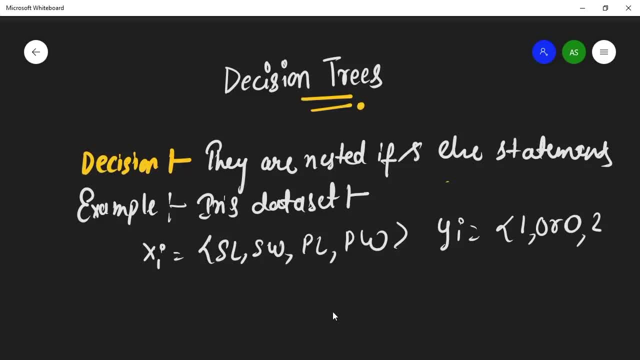 width. okay, so we are having these features and we have a y i which indicates either one or two or two, or zero or two. okay, so that's the basic intuition, uh means of the data set part. we are given this data set. now what we will do? we will make a classifier like this: 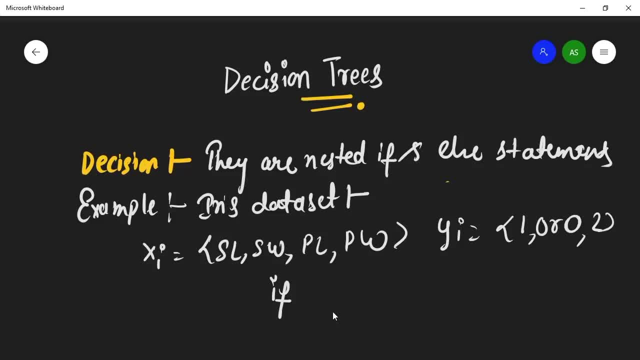 i should choose a better pen, like this blue, okay. okay, so if the petal length is smaller than some, a and may, a may be some number. a may be some number, let's say, let's say 2.3 a may be some number. if petal length is smaller than a, then consider y to be, uh, versicolor. okay, so let's. 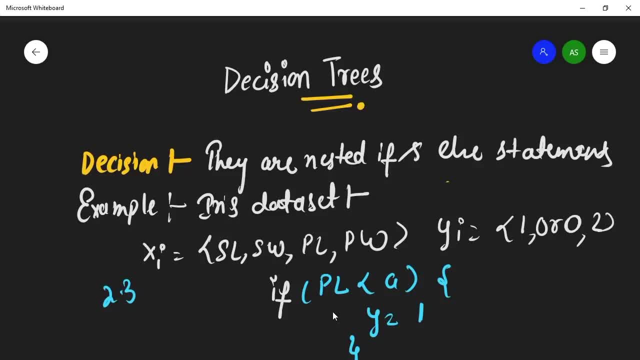 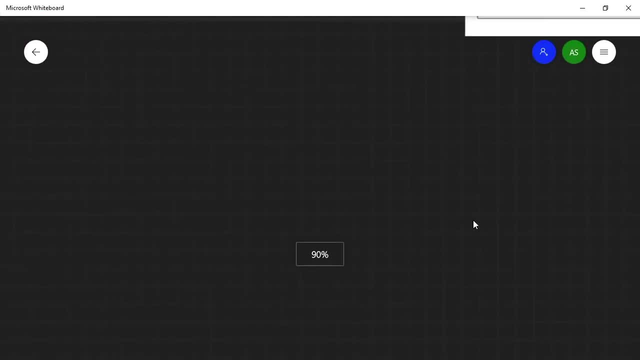 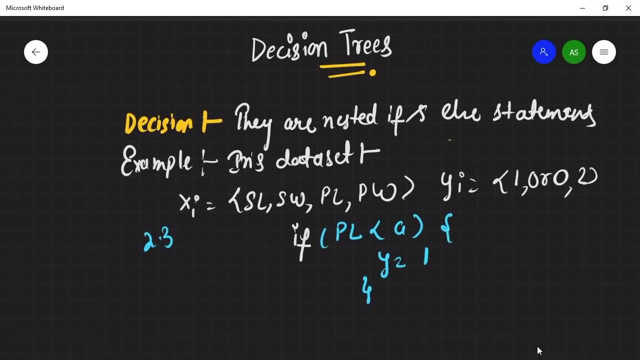 consider y to be one. okay, if not, if it is petal length is greater than a, then what do what? what to do? oops, i hope that it is getting not clear what. what happened? i have to buy my new computer. why do i don't know what, why it is so much lagging. okay, so you'd, if it is smaller than a, the petal 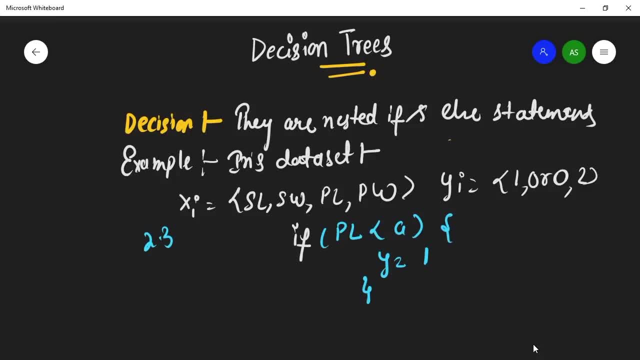 length, then consider your flower is means, uh, a versicolor, and we have, we have made one one. and if, if it is petal length, if your petal length is not, is greater than a, then what you will do, you will write else. if sepal length, you take again one feature. you take again one feature and says: if 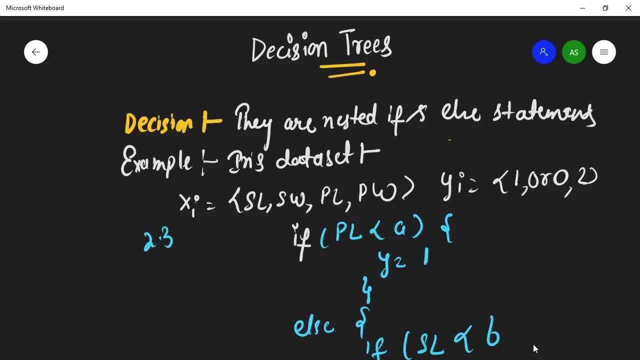 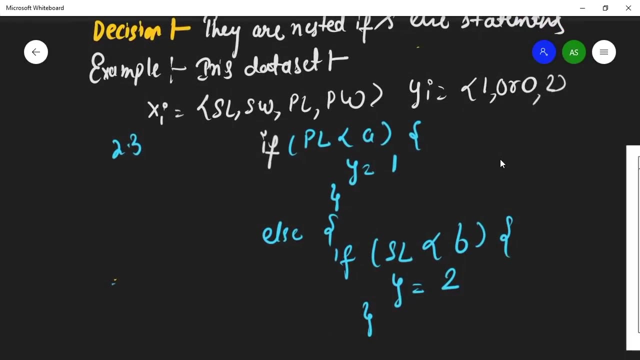 it is smaller than b. if sepal length is smaller than b, then you will. you consider your y to be: uh, virginica means two, okay, if it is not, if it is not, if both is both condition fails, then say: if both condition fails, then say that your output is citosa, okay. so here is our simple decision tree. we're using two features. we 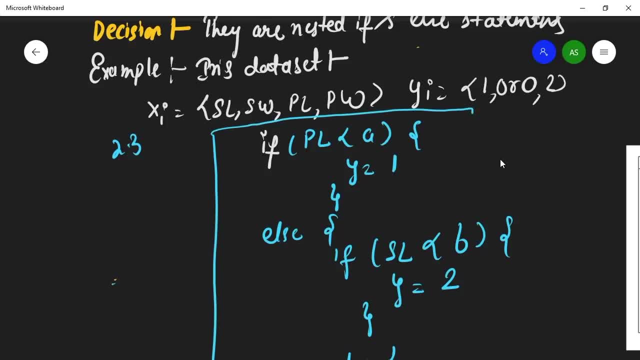 have made the decision trees using two features, so let me make it more intuitive. i i i hope that you are able to understand, okay, so so that's why i'm speaking very slow. so here let me tell you what i'm if petal length. here we are, we have taken two features, which is petal length and sepal length. 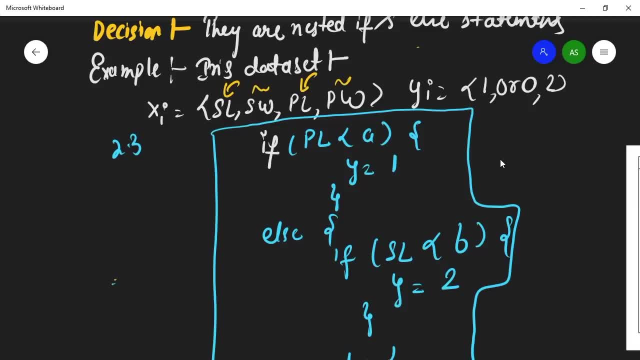 okay, we had not taken the petal length and sepal length and the sepal length. okay, we had not taken taken this, this, two features. okay, but you can make that. but this is not a formal decision tree. this is just for an example. this is obviously not correct. 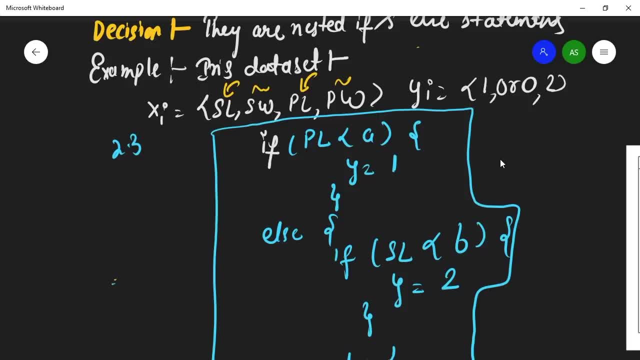 okay, so you had to make made one if condition that if the parallel length is smaller than some, a and a can be anything: 2.3, 4.3. that that is usually I'm taking, anything, but it is usually taken, which will see in one of our data. 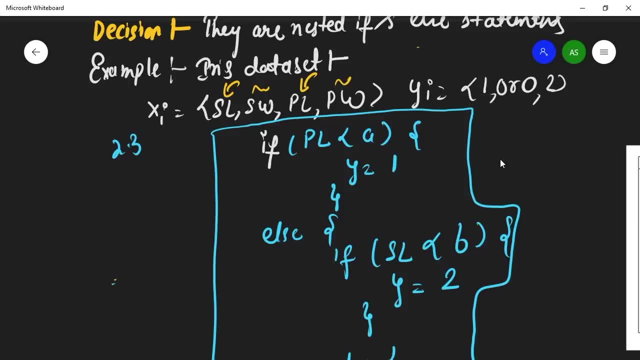 set. we will see how it is chosen and you will obviously see how it is selected. okay, so if it is smaller than a parallel, and then consider that y to be equals to one. if it is not, let me check. that is, the recording is on here, okay, regarding 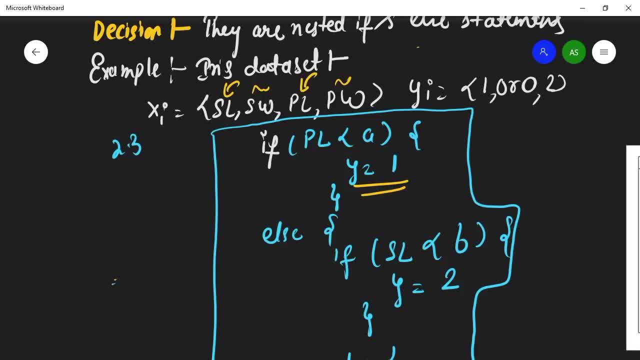 is on. okay, so we, if the parallel and smaller than a, then we consider our vibe to be this versionica. okay, if the parallel is greater than a. or is it this? this? this condition fails. this condition fails. It then goes to else condition and in else condition it. 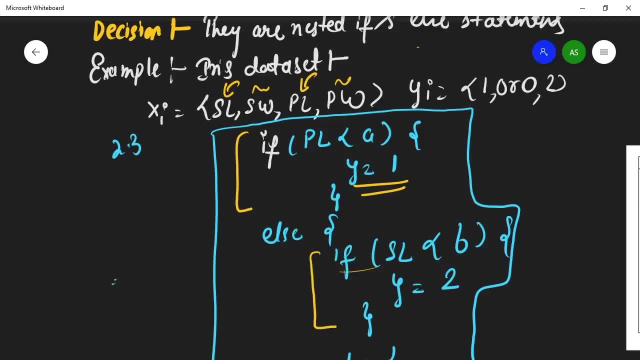 This is again a nested loop, and nested- sorry, not loop- if an assist control flow. So check if your sample and is smaller than B. if it is, then you say that y equals to virginica. Okay, and otherwise, if this condition also fails, Then it says: else, your y means y should be setosa and you have this hole into the this. 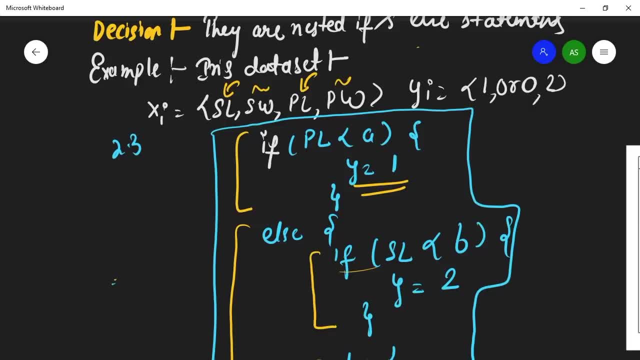 And nested loop in this and you have this whole classifier and this is your whole classifier, So that this is the decision tree. Yeah, so let me make this diagrammatically in the terms of decision tree. so, In terms of decision, true, we can write this: equal air, this: 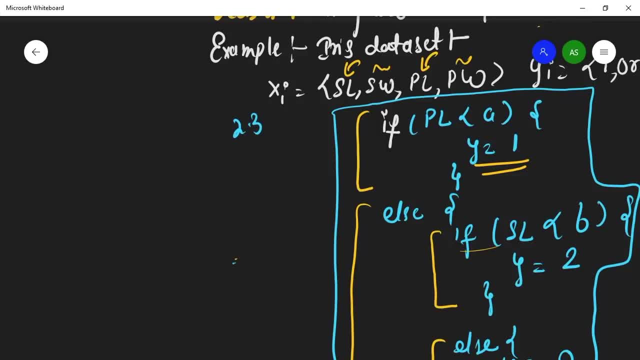 This if-and-else statement. first we have our root node, this we have. first we make our root node like this: Let me make one root node here: We have our root node with this condition: If a parallel length, parallel length, is smaller than a, okay then if it is. if it is yes, 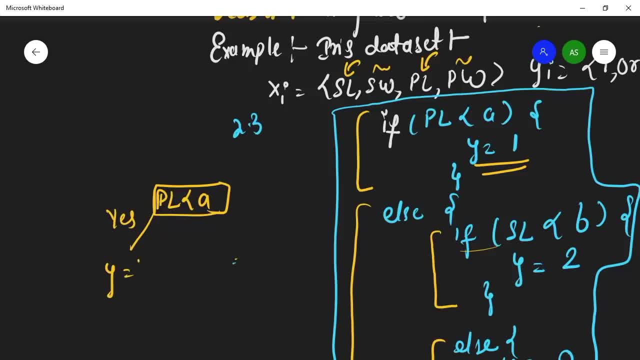 Then you say your y to be 1, okay. if it is no, if your parallel length is no, Okay, you consider. you again make one more condition, Which is: sample length is smaller than B. if it is yes, Then you what you do? you classify this y equals to 2, if it is not. if it is not, 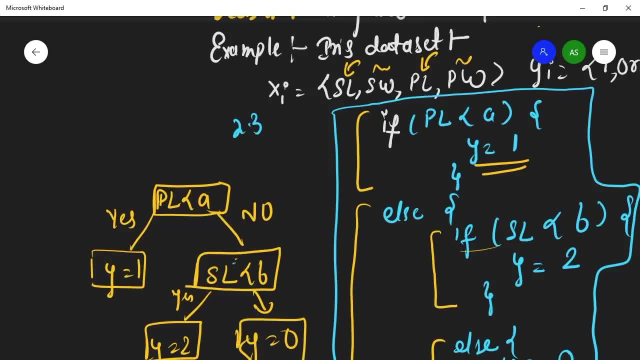 Then you take it as a 0 and Your whole. three variable, target variables are covered And this is the decision tree and this is whole. this is the decision tree. I am made in yellow. This is the decision Tree is. just ask a question on the dataset. if the parallel is smaller than a, if it is, then you consider y. 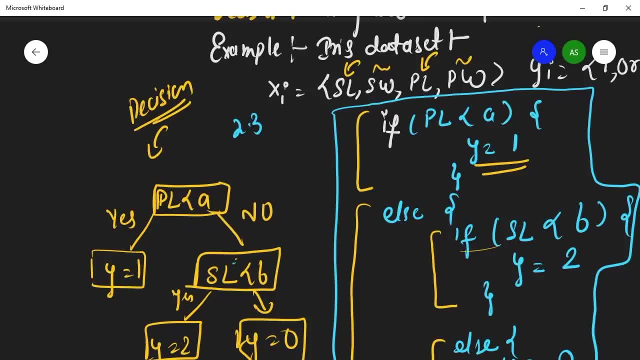 Goes to one. if it is not, then again We have made another issue, another decision, and then we: yeah, if it is yes or if it is no, like this, okay, So that's the. this is the decision tree. It's a. it's damage like that. 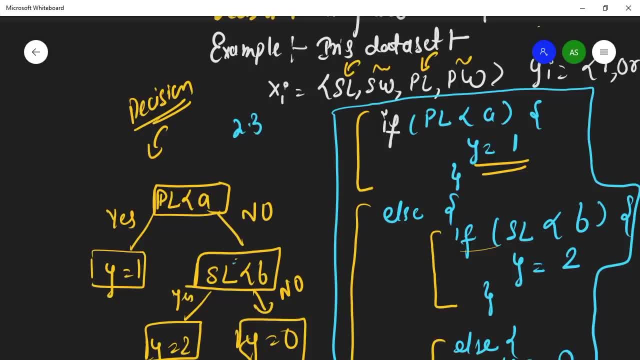 this okay. so here again, I'm saying: this is what you do. just believe me. yeah, we had. this is the decision tree, and how it is constructed, we will see. okay, so we have made this. if an L statement, that's true, if an L statement like this and 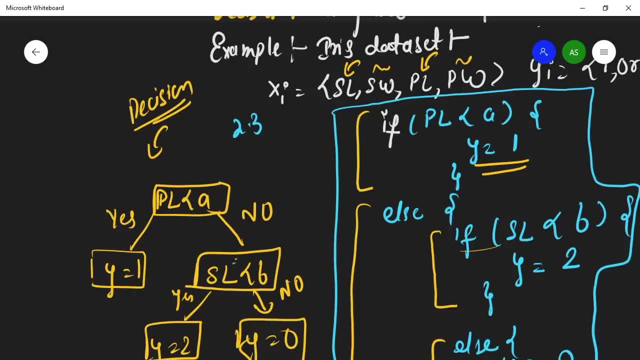 this is what the decision tree is. so here are certain terminology that we will be will have to see over here. so here are the details that we should know. okay, so the the first node, or head node, is no. is known as a root node, is known as a root node or parent node. okay, this is. this is a root node. obviously this is. 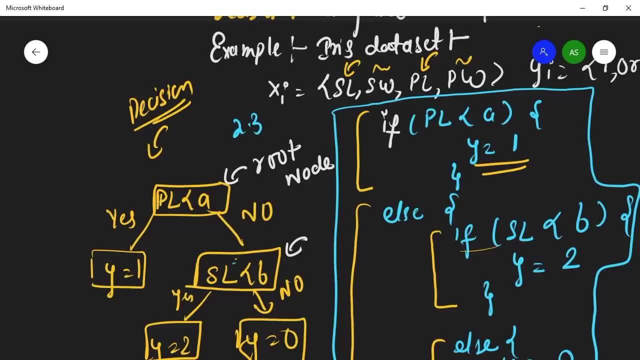 also a parent node, and these are the child node. these are the child node, okay, child node. and this is the parents node and this is also the parent node and this is the terminal node. this is the the terminal or a leaf node, because you are not splitting this node into further. 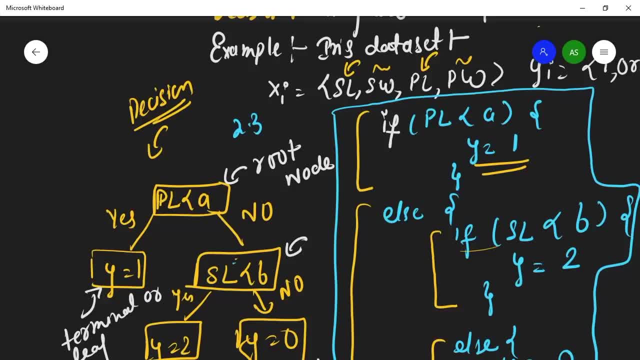 nodes. so this is called the terminal and this is also a terminal node. this is also a terminal node. okay, this is also terminal or leaf node. this is some sometimes called a leaf node, when you are not splitting further. okay, so this is a leaf node or you consider is a nice leaf node. this is the whole thing is. 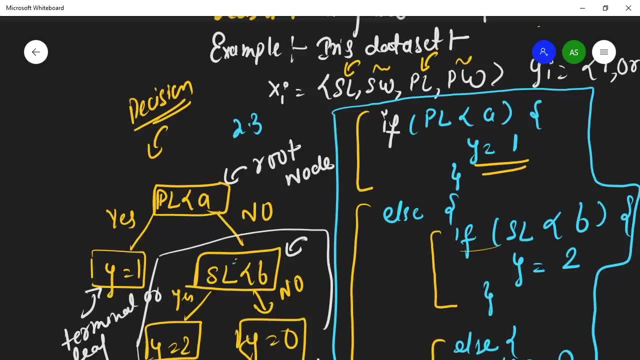 called branch. this whole thing is called branch. use this, not a branch. have lar yaşa. it's all branch thisрать, branch have, which make us the convergent of store. serve 크 mercy. this whole thing is called branch. okay, and that's the basic terminology of this. okay, and this is the 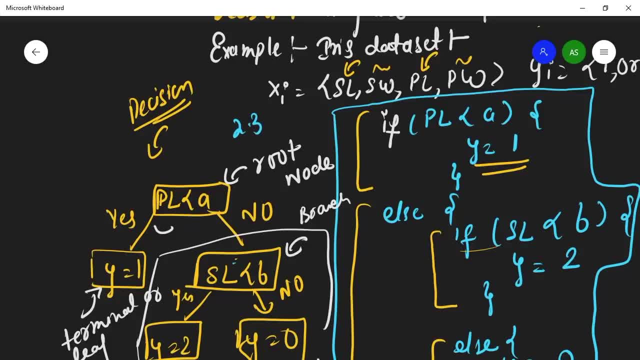 splitting of your data. okay, this is the, this is what you are doing, which is splitting. okay, if you're removing some node- let's take an example this- then you are pruning it. okay, then you are pruning this node, but we are we don't know, we don't want right now. okay, so that's the, that's. 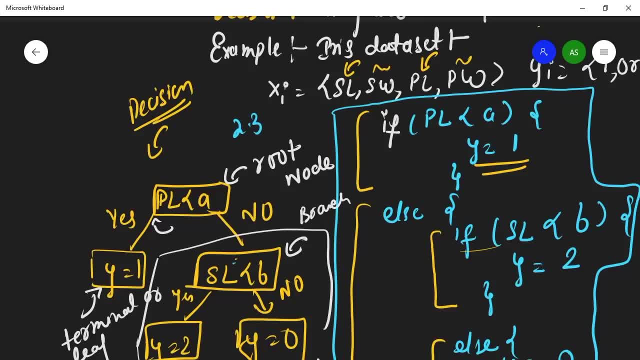 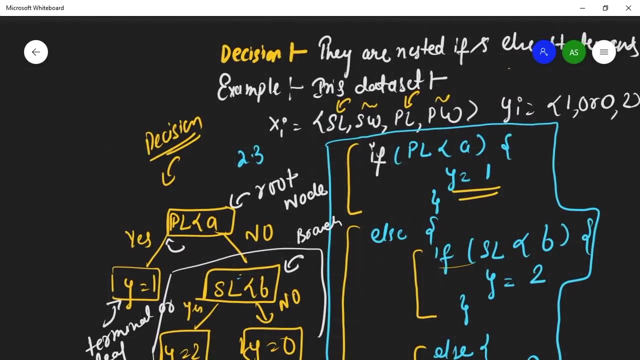 what that's the decision tree, and i hope that you under understood this example clearly and i really really hope that you will- uh, that you got a very good intuition of decision tree in much smaller span of time, in much easy way, okay, so i hope that you remember this terminology either. i will make 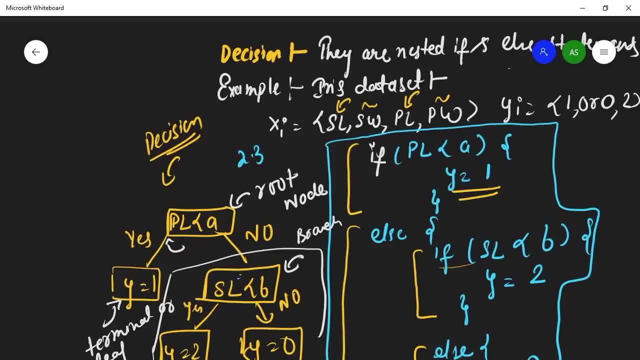 you familiar with terminology by the time. also, if it is not required for remembering all those things, okay, but this is it's it's best to remember. take a paper and a pen and write notes with me whatever i'm writing, okay, and just listen me carefully. after listening me, you can make notes, okay. so now let's see what's the decision. boundaries. 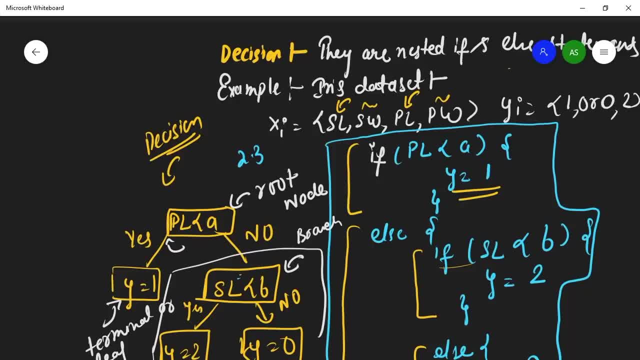 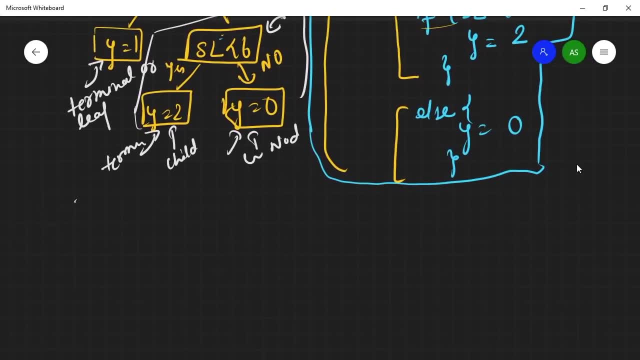 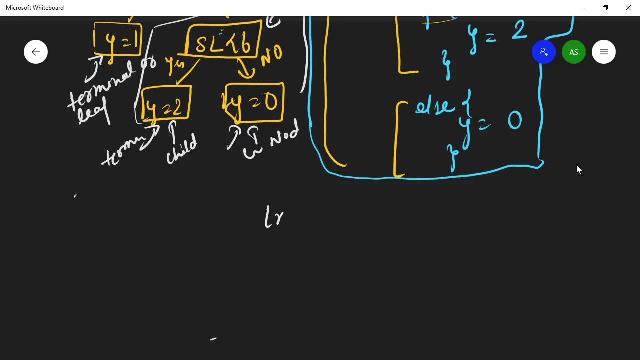 will look like. okay, what's the decision boundaries will look like? or the hyperplanes will look like, but what do i mean with hyperplanes? i mean with hyperplane, decision boundary is- let's take an example of linear regression. in linear regression, we are making a straight line. this is called the hypothesis decision boundary. then we 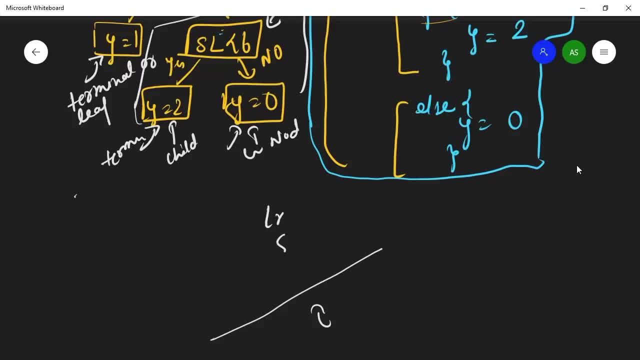 have a hyper plane. it's called a hyper plane in support victim machine. we are also making hyper plane and logistic regression we are also making. hyper plane means a decision boundary. so in the decision decision tree we also have the decision boundaries. okay, or hyper planes. so let's see how. 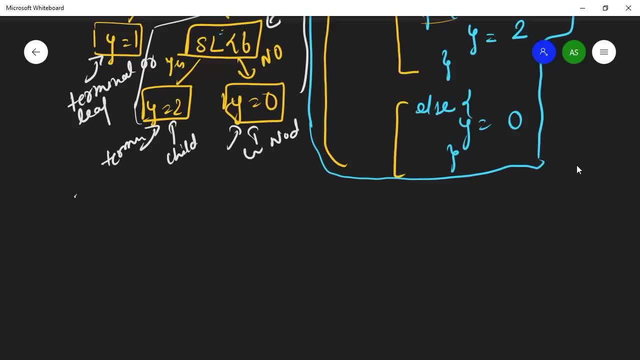 it is constructed. so i don't know i will be able to make that image or not, but i will fully try that. okay, so here, uh, uh, let let me make one x and y, plane x and y. oops, i'm uh. please anyone help me to make this. 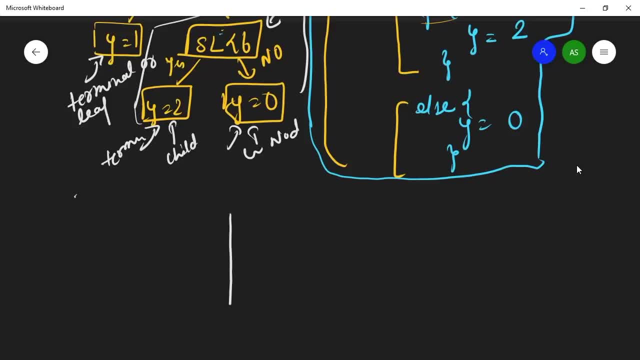 okay, let me do that. oops, i'm just freaking out. let me do it again. yeah, okay, great. so i made one and this is my x-axis. this is this is my x-axis and this is my y-axis, and we have two features: which is sepal length and, uh, pedal uh length, i think so. yeah, so we have paddle length and the x-axis. 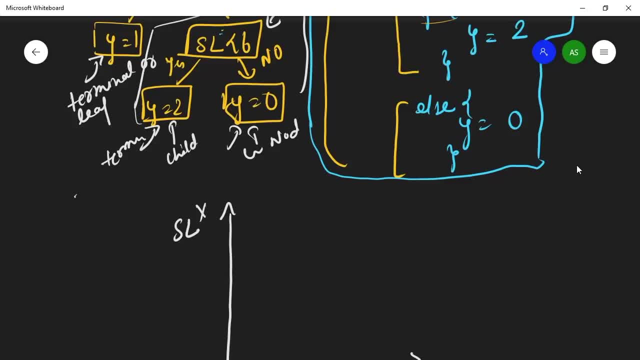 and we have sepal length in the y-axis. okay, so we i i have just made it. you can remove this y-axis, maybe it will confuse you. and in our axis we have petal length and y-axis we have sepal. and because we have taken only two features in this example we have, we are not taking more features like 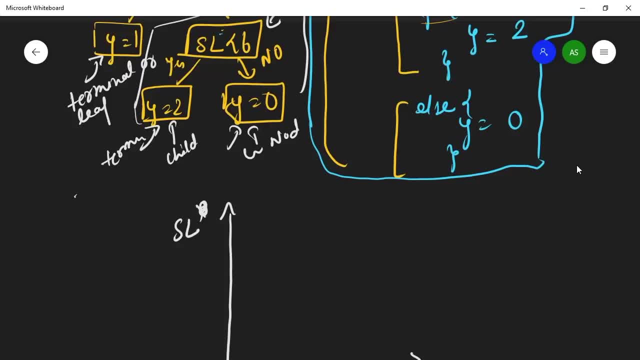 petal width and sepal width. okay, so what? what we consider, what we have done, we have consider, we have consider this full reason, we have consider this full reason, this full reason to be y equals to one. okay, this hyperplane, this hyperplane list, let's name it as a. 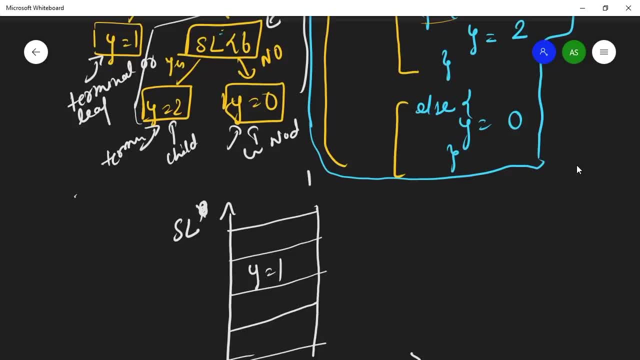 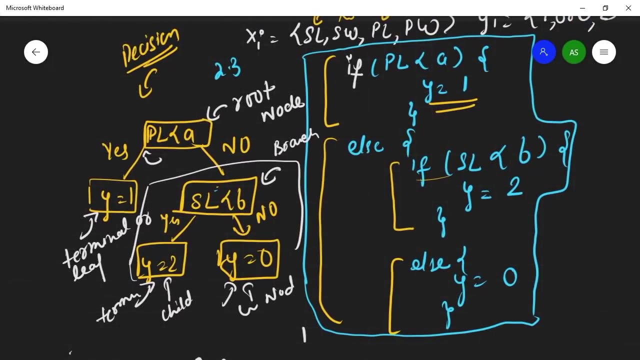 first type of plane. so this full reason is our: y equals to 1 means whatever data point will come is considered, y equals to 1.. and this is just this is just the if statement that we have seen. if per length, if length is more than a, okay, then y equals to 1. so that's, this is the full reason. 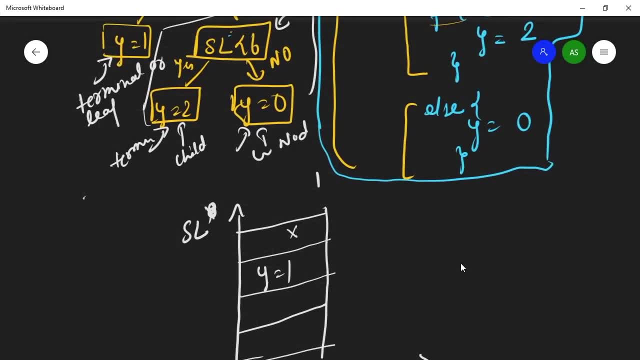 okay means we have not for this bit, so it is just a full reason. we are: y equals to 1. if that condition passes, okay, then another hyperplane we can construct. let me choose another pen, another hyperplane, we construct that. this reason, this reason would consider y equals to 2. ok, y equals to 2 if the sepal length is. 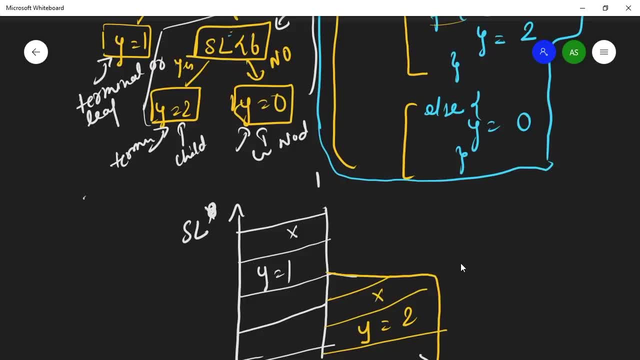 smaller than B. if the points could come in this reason, then it will consider y equals to 2. another. we have hyperplane. let me take another pen. and let me take another pen. let's take an example of blue. ok, another Bears term. we can consider that as a. y equals to 3. 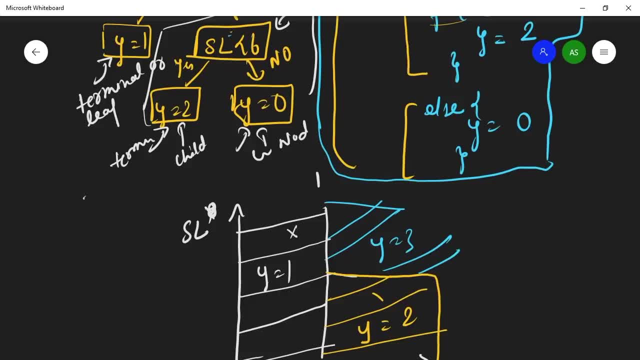 ok, if that, If that falls in this reason. so here we are constructing hyper planes And if some with something come here, then it's going to control y goes to 1, It's y goes to 2 or y goes to 3 with these two features. 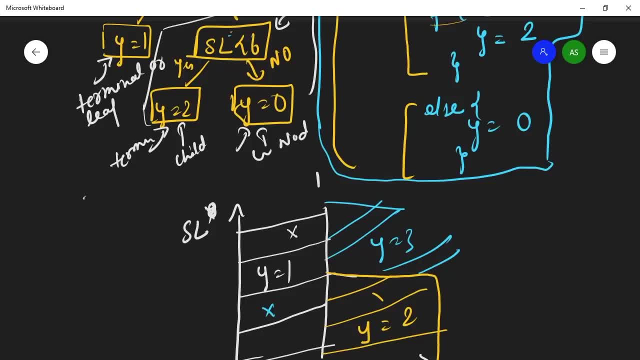 Although obviously it will be more dimensionally high when you plot the four features. Okay, so you can see that you have a hyper planes where we are able to make predictions- Okay, and we have made a simple classifier- Okay, but in something to note over here, that all your hyper planes are: 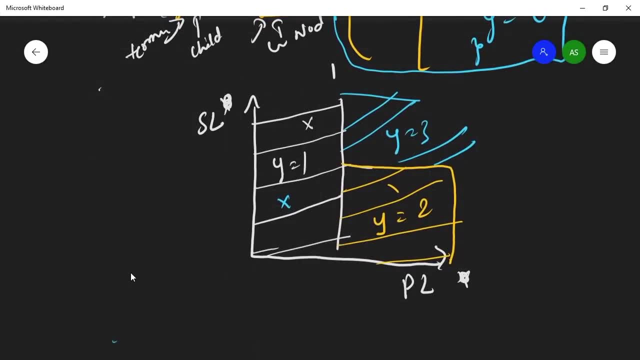 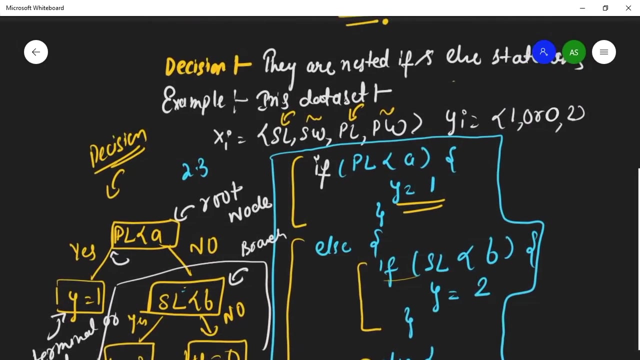 X's Parallel. okay, our X is parallel means this is parallel and this is parallel. So you can see over here that all the hyper planes are X is parallel. okay, so that's the. I hope that you understood. decision trees in that and This is the basic. 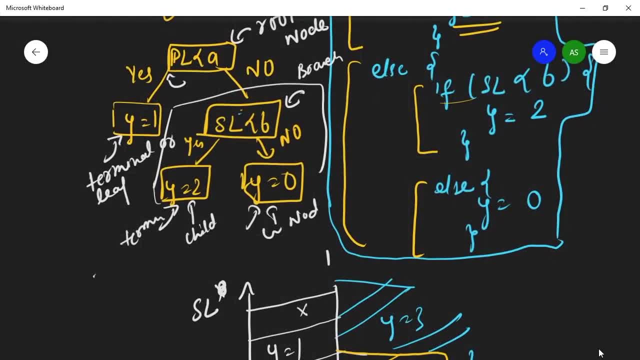 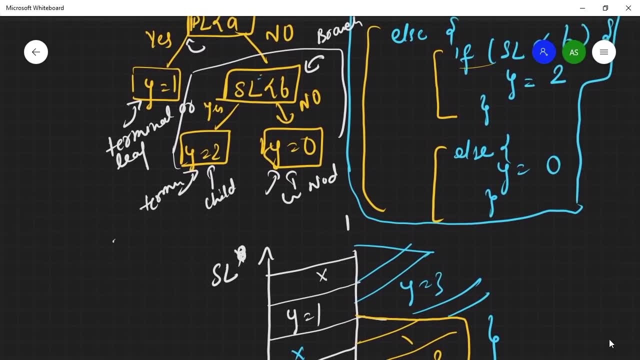 Intuition that I want to give it to you, in more Sophisticated way or not sophisticated, It's just a good thing, Okay, Okay. So, as I've tried it to keep it as simple as I can, and I kept it, Okay, so let's. 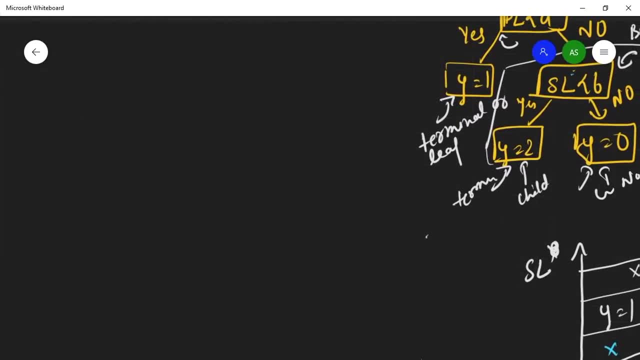 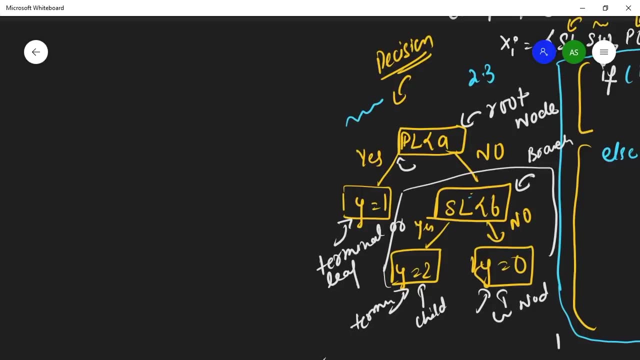 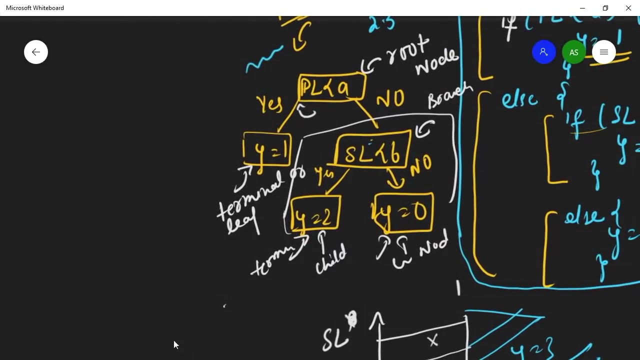 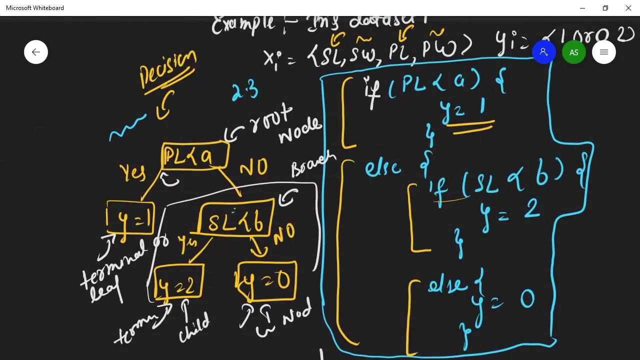 Let's let's start building, or let's start with mathematical region. That's how we construct these kind of decision trees, these kind of decision trees, how we construct. Okay so, But before that we have what, what, what we do we? How we choose the variable, or how we choose the feature to be the root node, or the brand, or this, this, how we split. 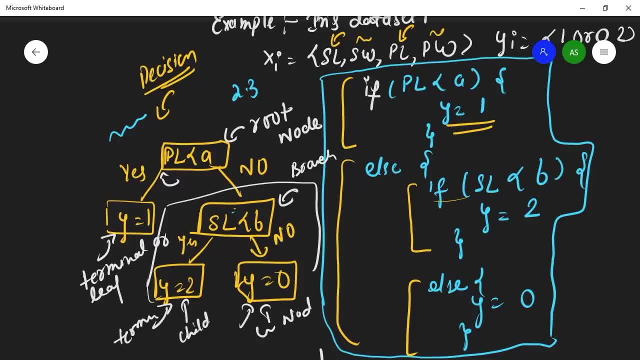 so We have an attribute selection measure and you give, if you select around randomly, like I have, choose a petal end of you. if you choose It around randomly, then you will be ended a very bad model. So we have different attribute selection measure. We like entropy, information, gain, gain, impurity, which we'll see in detail to understand the how we select that. 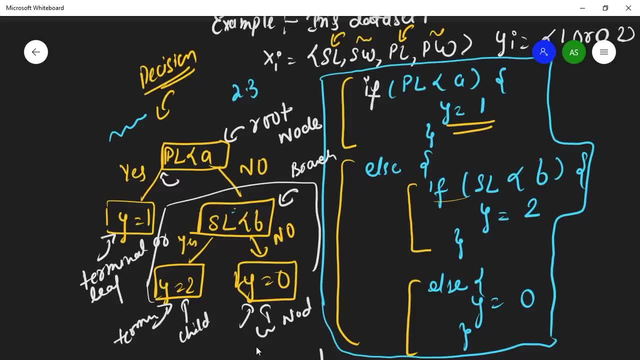 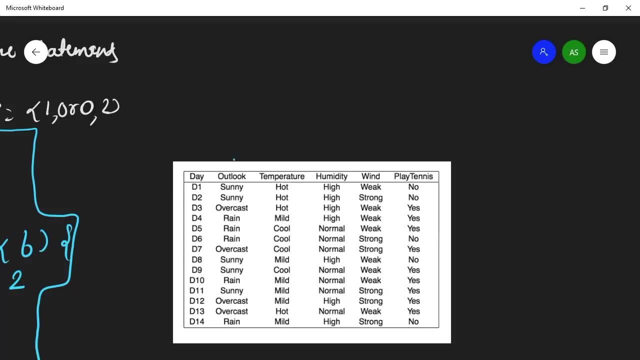 So we want to give you an attribute to be as a root node, or like this: Okay, So let's take a. let's take an example of this data set. if you want to split this data set, what feature you will use? you, What are you going to use outlook as your feature? 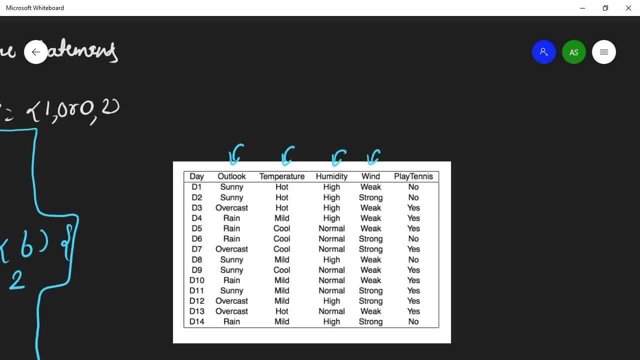 Root node or temperature as a root, nor our humidity as a root node or when as a root node. Okay, and play it in. this is our label So which you will use. if you choose around randomly, Maybe you will be end up ending up with a bad model. 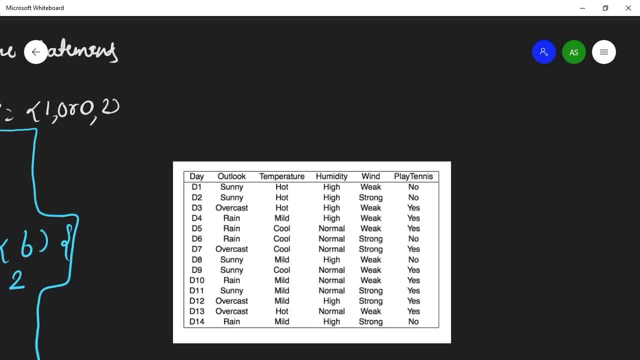 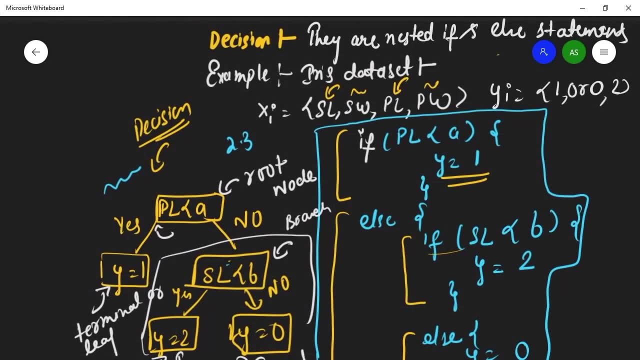 have to do that kind of thing. no, so we will be scientists or researchers, have done a very great job. even you all have to do all this kind of thing, research, and please keep contributing to the ai community. that, uh, maybe, and i'm also doing research in machine learning and definitely will. 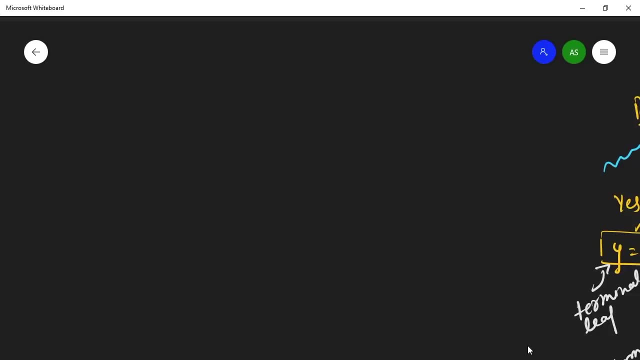 come up with something extra. okay. so, um, different measures, different measures are, uh, different attribute selection measure are entropy. we have entropy. then we have the second number. we have information gain, information gain, information gain, which we usually write as ig, ig. then we have guinea impurity, then we have guinea impurity and simply, uh, i g. okay. so we denote like this: 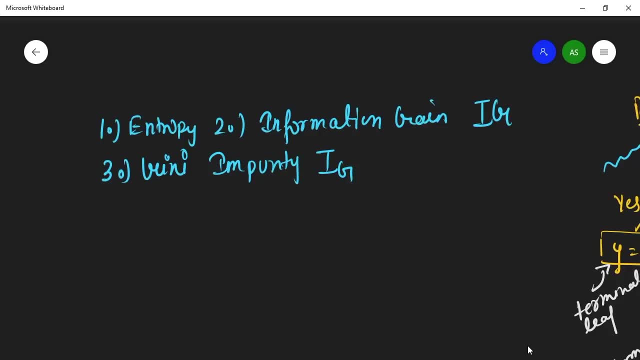 okay, so, uh, we will, we will talk about all of these three and i, and i hope that you will uh understand each of them. okay, so, let's start with entropy. okay so, uh, entropy. let me write it more formally. yeah, so what? first of all, what is entropy? entropy is an attribute selection measure. 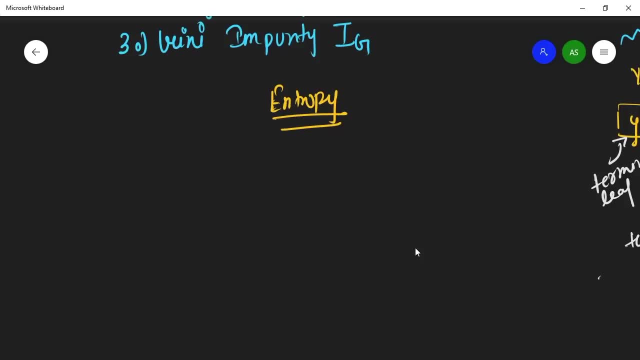 it's the measure of a randomness. okay, how pure or how pure that attribute is to be used as some notes or a root? no, okay, so it's the measure of randomness. so let me write the definition, because definition is also important, and if you want this kind of all my notes, you can simply 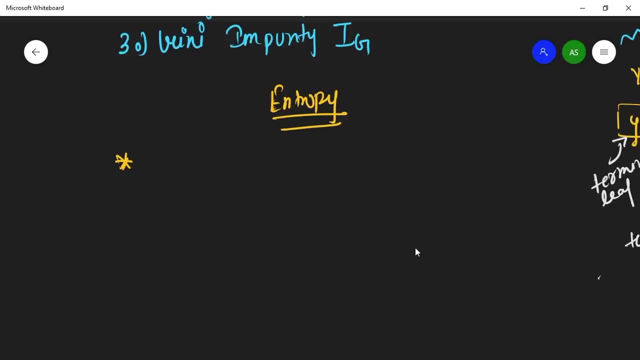 write me or write with me along. either you can comment or um. join the newer community discord community and ask me there i will be able to give. okay, so ask me there, i will be able to give all this entropy, etc. is the measure? is the measure of randomness? 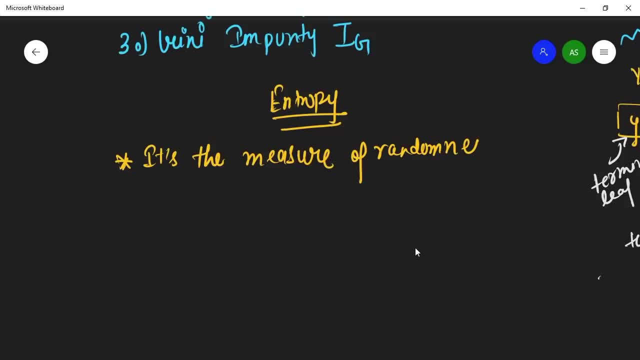 the measure of randomness. okay. the higher the entropy is, the hot the. the higher the entropy is, the harder to draw any information from them. okay, so it's. if the higher the entropy is, it's very hard to break your uh node, okay, or to choose the node, so our entropy should be low. 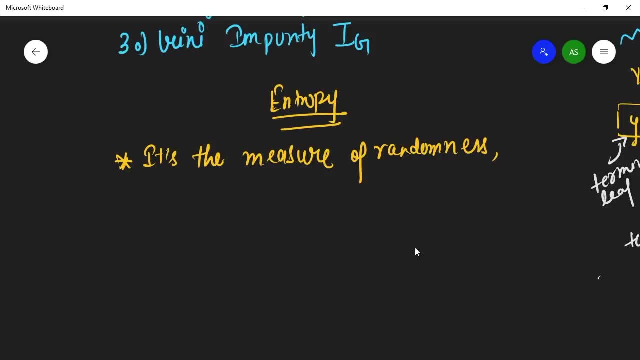 to to be considered as a leaf node. but still, don't, don't worry, i will dig directly into the, into the cases, to make you more understand. what do i mean with these terms? okay, but first of all, uh, let's take in, i will show you one equation and then i will show you, um, how some? first of all one. 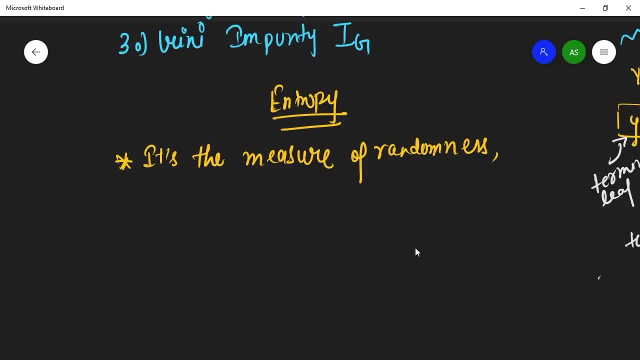 example, and then i will show you properties of entropy. okay, so first of all, uh, let's take an example here. you are given, you have y to be, maybe, uh, y1, y2, all the way down to the yk, and in this case you are not. this is not examples, this is a this. this is like maybe citosa means what is the. 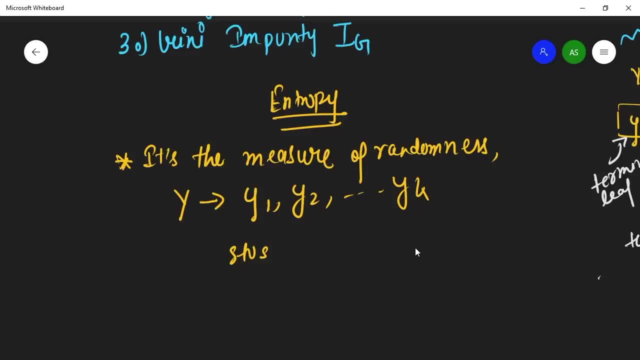 number of classes you have. okay, so maybe you have binary classifier or you have a multi-class classifier. okay, so you, what is the number of a classifier? so maybe you have in the, in the iris, citosa, we have here's uh versus citosa, virginic and versicolor. so we here, we have y equals y. 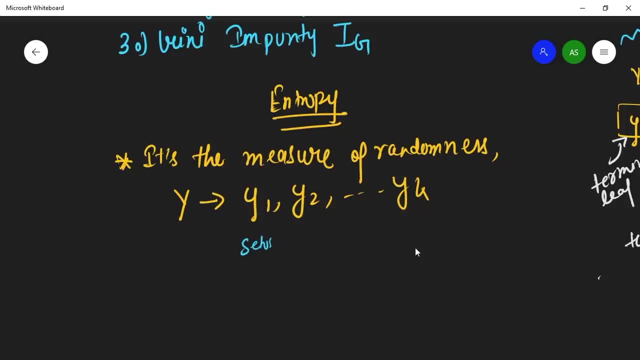 equals to y1, to be citosa, then we have virginica, then we have versicolor, means three y's. okay, so that's what i mean with this. okay, so let's, first of all let me give you um, let let me give you the equation. okay, so the 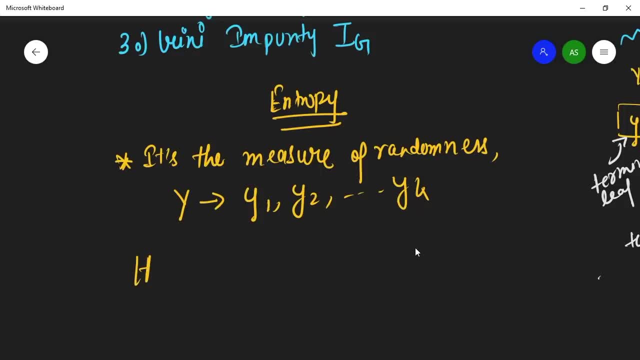 equation is defined as like this: uh, h. we define our entropy by: h equals to. let me choose white color because i will. i like white much. okay, minus many. uh, this is this. minuses very important. minus the submission, i equals to one. all the way around to the k. 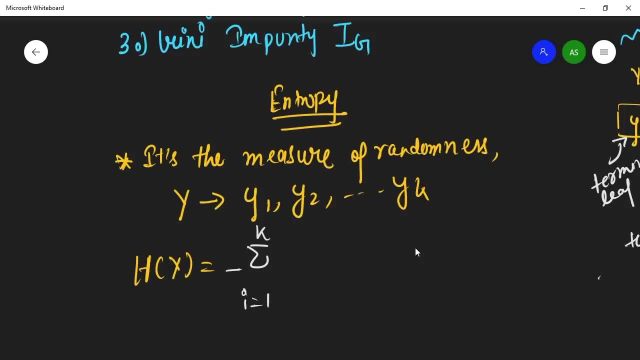 and k. here is the number of your. what is the class? what is the number of a class? okay, p of y, a probability being y, i log of base, and b is usually taken as 2 or e. okay to 2.713. okay, so b is usually taken as 2 or 3.713.. 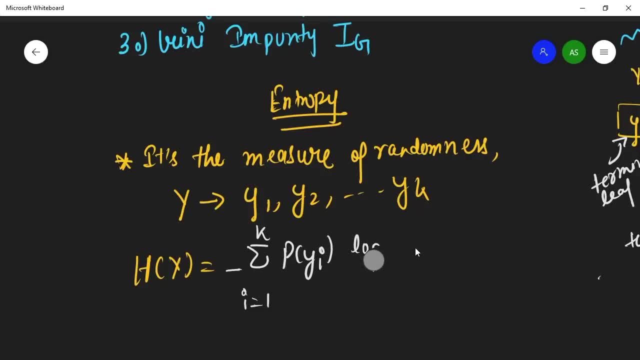 But we usually take B as a 2. so if you were taking P as a 2, then you can consider it as LG. if we're taking B as a e, then then you take as L and natural logarithm and you have a Log to base, a log to with the log, with the base 2.. Okay, this means LG. Okay, so you take log of. 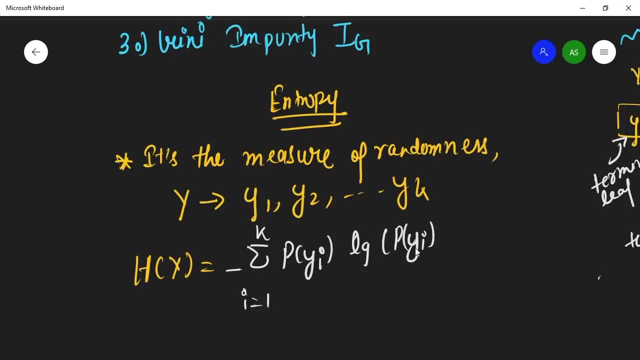 P of Y, I. okay, and that's the full equation of your entropy means it just measures their randomness, Okay, so, let's, let's take one example, because it is I, I. I know that is making no sense to you, And I know that is making no sense to you, but I will make sure that it will make sense, Okay so. 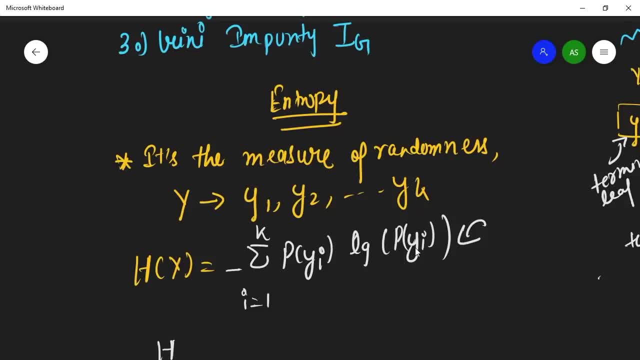 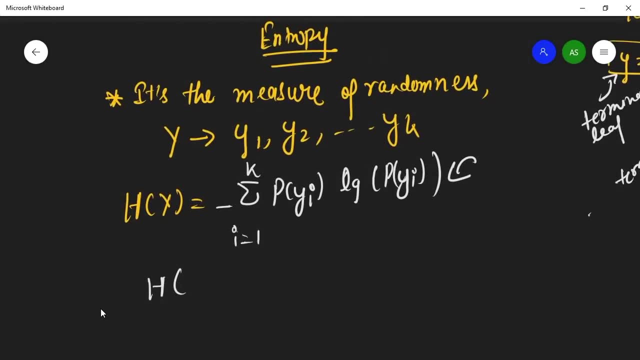 first. yes, You, we want to measure our randomness for playing golf. Okay, you want to measure Your randomness for playing golf, Okay, so let me write play golf. Oops, let me write the data set first. What's the data set we'll be using? so we have this: play goals, data set, play. 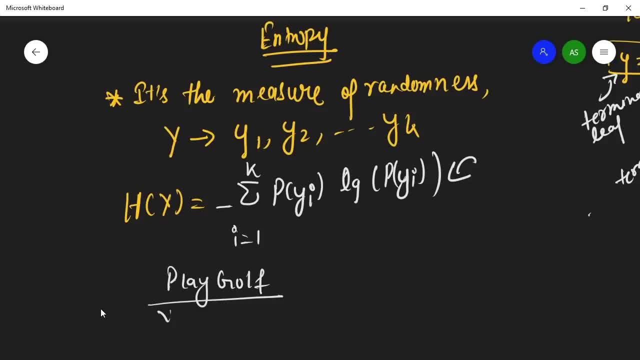 goals data set We are. if it is, what is the number of yes, which is nine, and what is the number of No, which is five? Okay, So this is our data set, like this, And let me make this also: Okay, so this is our day-to-day data set, and you want to take out the entropy of playing goals. 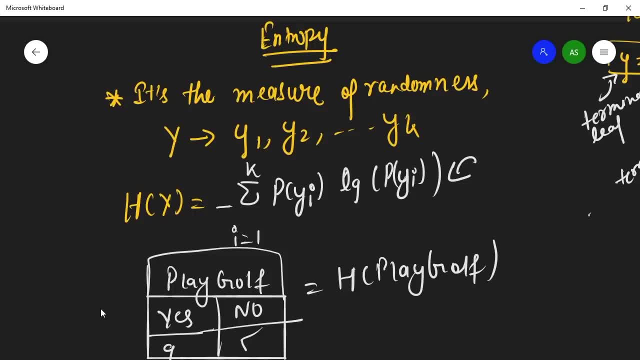 Okay, playing goals Okay, and here we want to take out entropy of being no, being no and being yes, Okay. So what you do? first you take out the entropy: entropy of zero point three, six log two. zero point three, six minus means this is your first. this is your first. 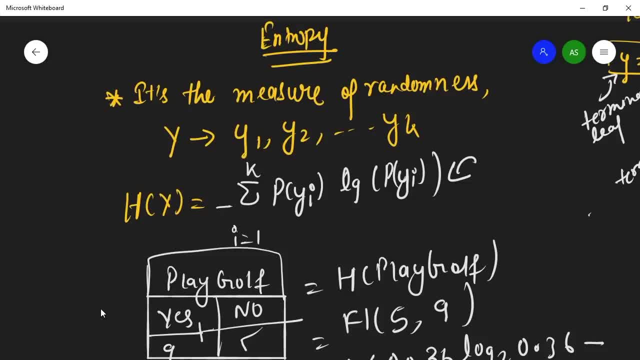 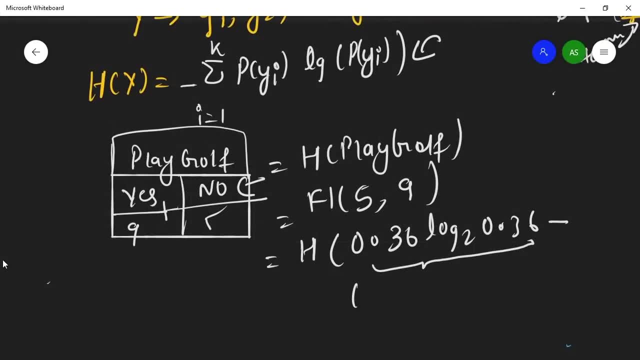 Y I, this is your first. y means yes, sorry, no, this is for no and minus. let me make it up: Okay, minus zero point sixty four. log base two: zero point sixty four. Okay, This is what you, and the answer is 0.95. 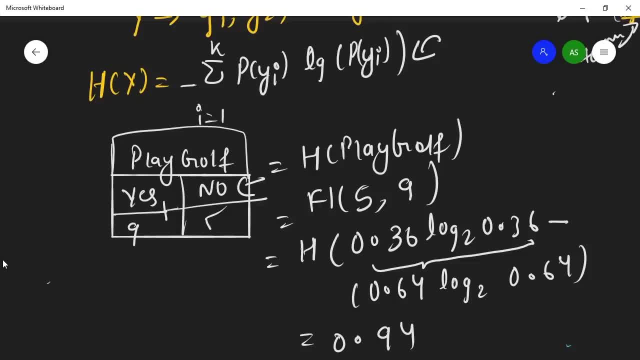 Okay, so here, what three, what? what we are doing over here? that first we are writing this, this equation P Of y, I times the log of for no, and then we are writing for yes, okay, and there is subtracting and we have a Entropy at zero point ninety four, and it can be further split, Okay, Okay, So this, this, this was the. 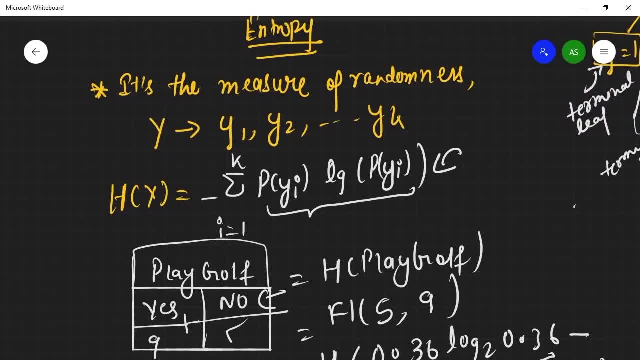 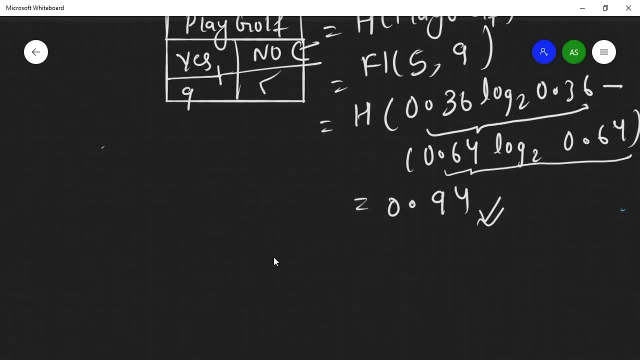 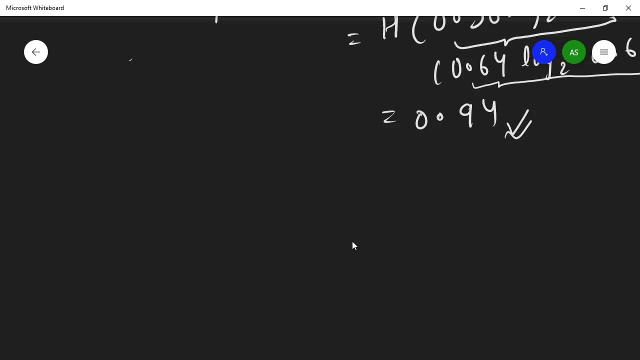 basic calculation of it, entropy. but let's see some cases of entropy to make you more sense of this entropy. and for attribute selection measure. okay, so we will see some properties. so let's consider, let's consider that we have y to be two class means we have a binary classifier where we have two class. 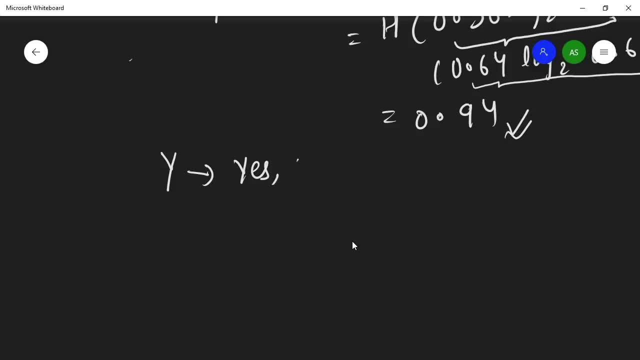 one is yes, one is yes and other one is no. okay, any kind of yes or no, whether it is playing tennis or etc. it's yes or no, okay. so let's take an example of let's let's take one scenario, let's take one scenario, number one. okay, so here is our scenario which tells: here is data, here is your. 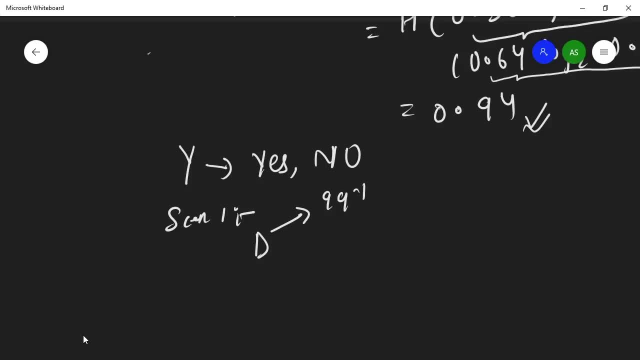 data and number of a yes is a 99 percent. number of a yes is 99 percent. in your data means these are the your y labels. so we have two unique values in your y labels. so here you have yes and no. so in that case your yes is around 99 percent and your no is about one percent. is about one percent? okay? 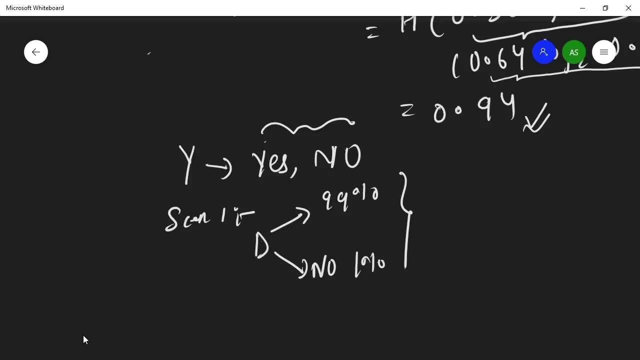 this is your case one. so let's take out the entropy for this h of y minus you're taking minus 0.99 means 99, log means lg. i'm writing log, not two. maybe i'm writing a log of 0.99 minus this. this is for my yes means this is for my yes because we have added a submission for each for. 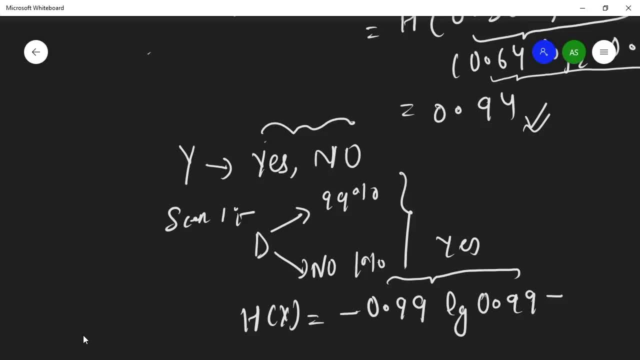 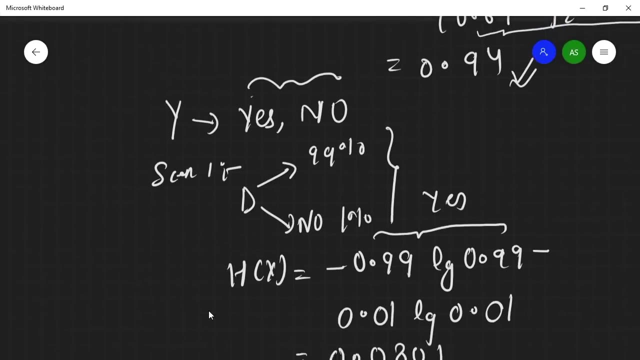 each uh y variable. so we are, for we are doing for each, for each y variable: okay, minus 0.01, the log of 0.01 and your output is 0.0801. okay, so that's the your entropy. okay, so let's take one more. 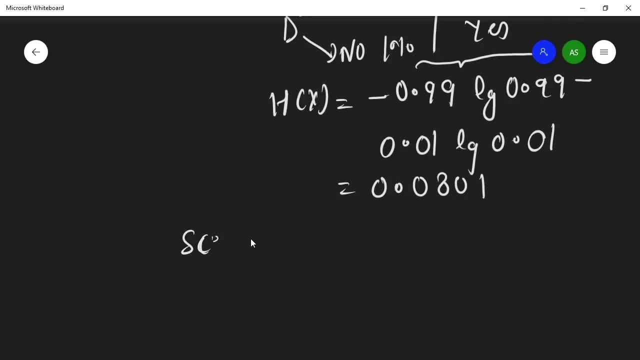 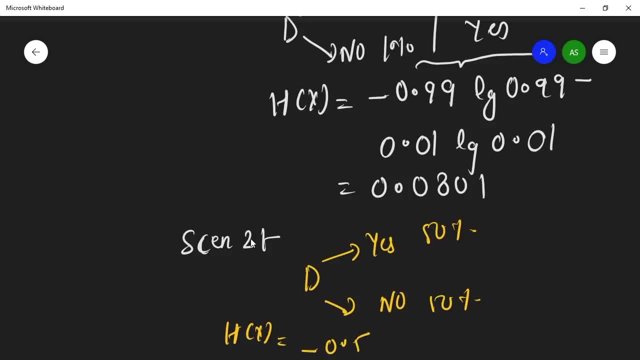 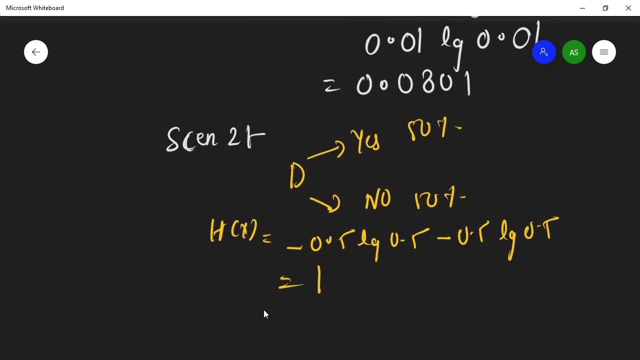 this: if you take out entropy of this, minus 0.5 log of 0.5, minus 0.5 log of 0.5, which is equal to 1, which is equal to 1, and the maximum maximum entropy is one and it is, and it is very. 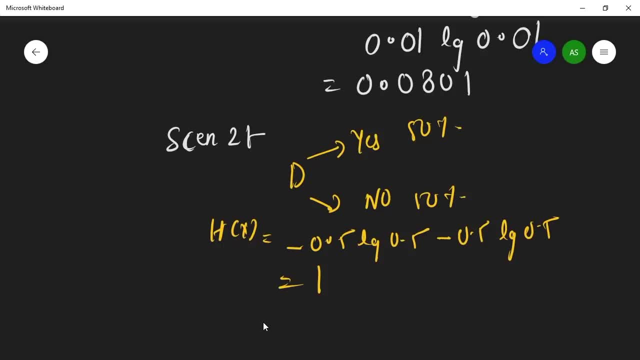 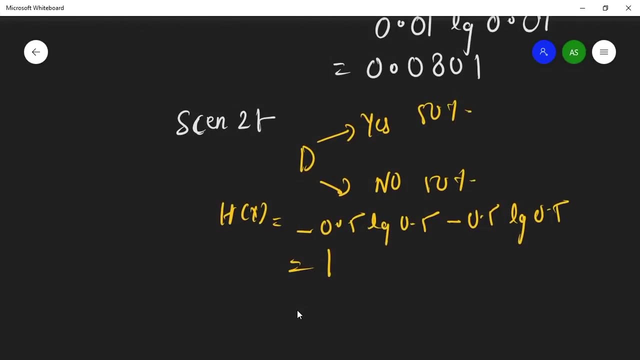 very hard to air, to split this, to split this it's very, very hard, okay, so its maximum entropy is one. let's take another scenario and if you have a binary classifier- i'm taking an example- your maximum entropy is one if you have a binary classifier. if you have a multi-classifier- 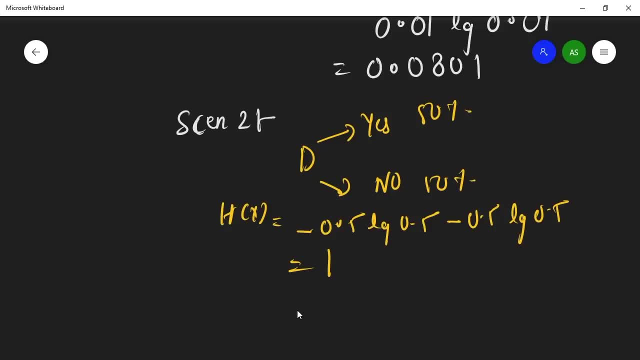 then the equation changes. okay, which you can see on internet, but most of most of the cases, if you understand binary, you will be able to understand multi-class. okay, let's take another scenario, scenario number three. okay, scenario number three tells you scenario number, tells you that your d. 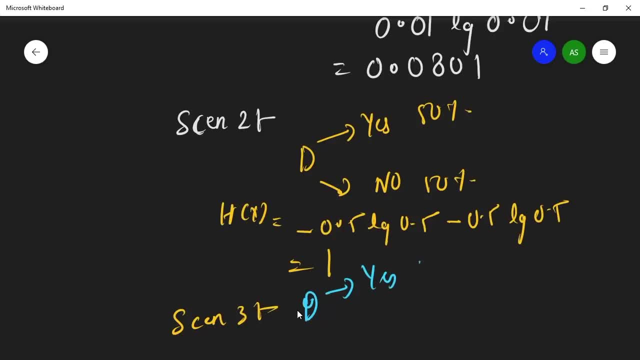 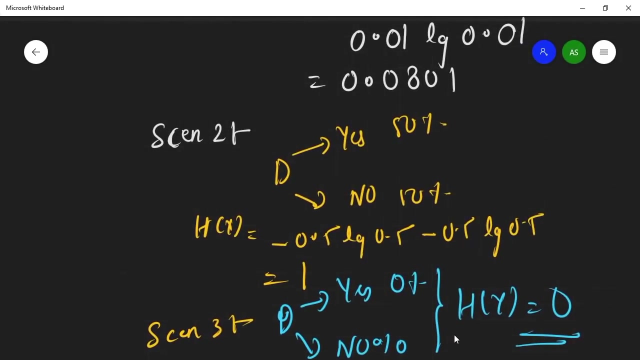 which has yes to be around zero percent and you have no to be around 100, so your entropy over here would be zero. okay, your entropy will be zero and the minimum entropy is zero over here. okay, so you can see some cases that this is: if you have id3 follows, if you have um, if you have a, some algorithm means. 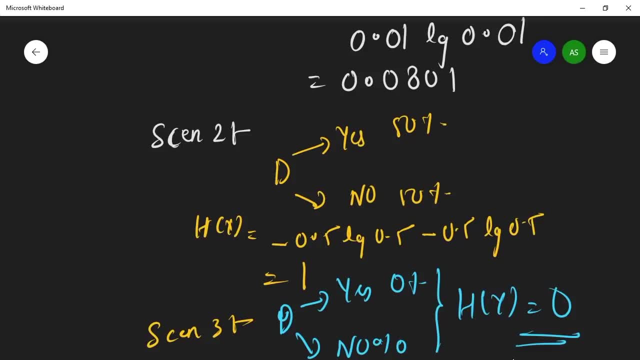 and decision tree follows that if you have entropy equals to zero, then you consider that as a leaf node. and what is leaf node as a your prediction? if your entropy is zero, then you consider that as a leaf node. if your entropy is one, then it needs further splitting. or if your entropy is big, means uh, your entropy for binary. 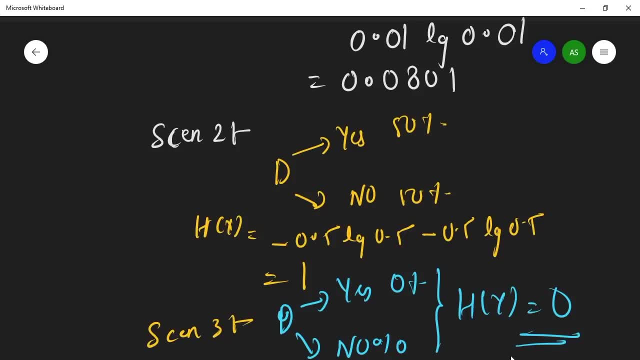 is generally, uh, greater as like this. your entropy is generally like this: entropy is in between or equals to: okay, so your entropy will be in in this range. so, um, some means, algorithm follow id3. there is one, one algorithm called id3, subset of addition tree algorithm. so id3 follows. if your entropy is zero, then you consider, or is: 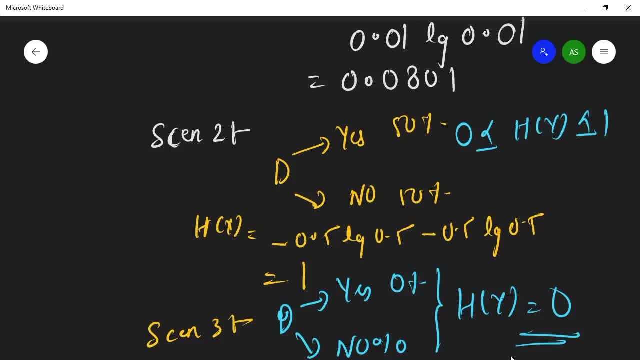 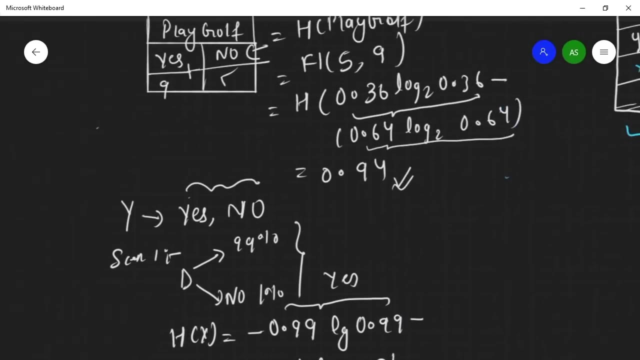 small, then you consider as a root a leaf node. if it is one or large entropy, then then you then it needs further splitting. okay, so that's the entropy and I really hope that you understood entropy in detail. so let me make you familiar with what, what we have seen so far. so we have talked about 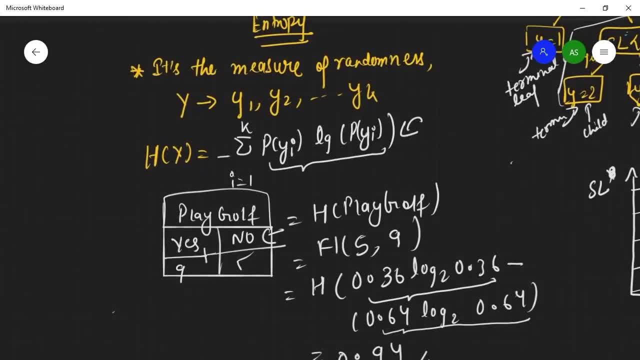 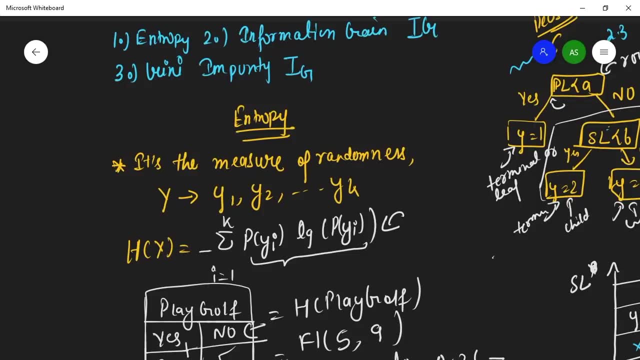 decision tree, which you can reverse back to see more, but I'm going to, uh, recap too late the entropy. so what do I mean by entropy? entropy is the measure of a randomness that measures if your attribute needs further splitting: or it's considered as a root node, or it could consider as a leaf node. 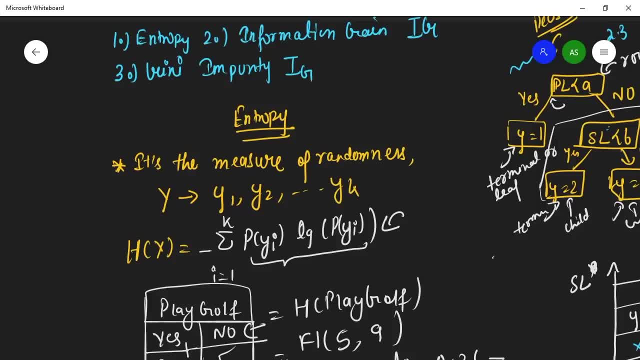 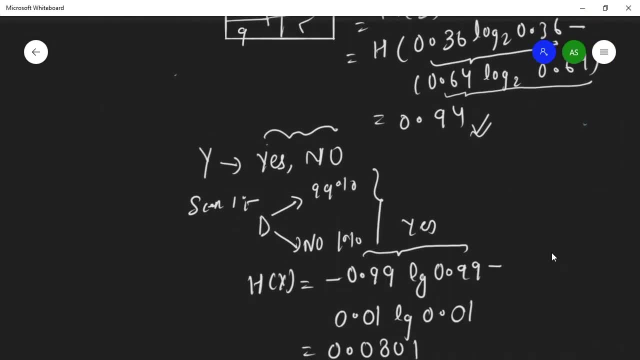 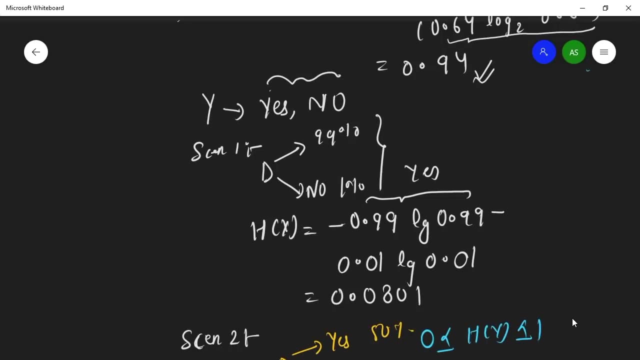 or like that. okay, so we have taken one example of playing golf and then, uh, and then we have taken some three scenario where we have seen that it is very hard to split. it is very hard to split if you this is. it's very hard to this um get you get information, for entropy is high so it needs for. 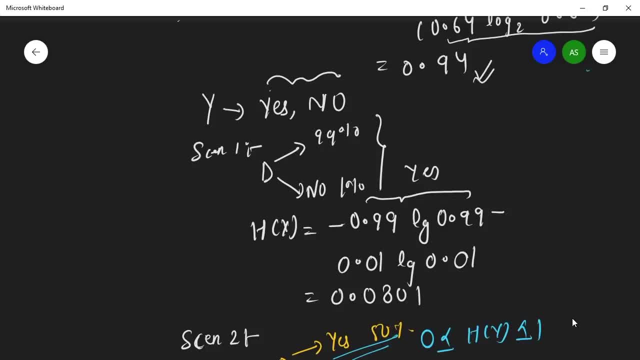 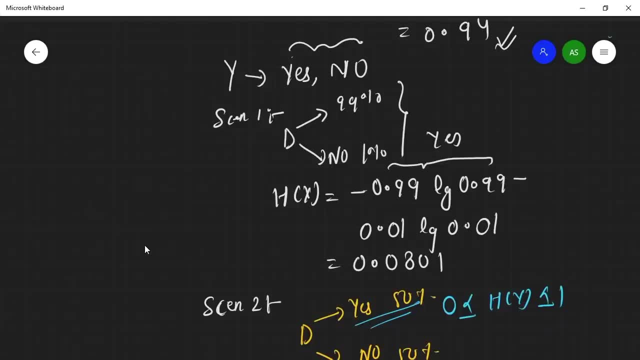 the splitting. okay, so if you, if you have yours to be a 50 percent node to a 50 percent, then interrupt, it will be one. if you have another scenario there, then it will be like this: I can um, just see the calculation. you can see the calculation if you want to be a to understand. 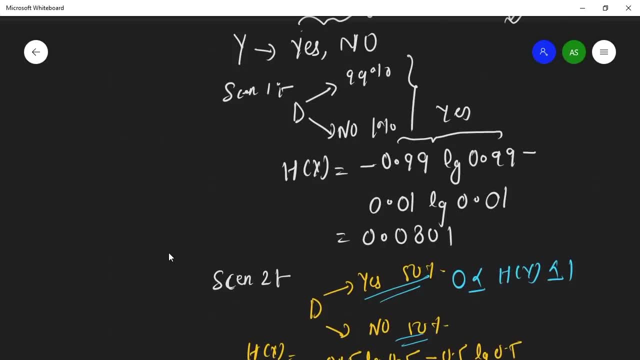 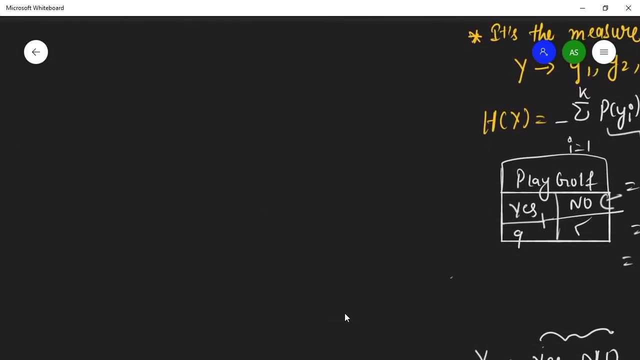 it much better. okay, so that's what, uh, these entropy is. but let's see the diagram of entropy visually. it's a bit interesting. okay, it's a bit interesting. so let me draw one diagram of entropy. okay, so here we have our. let me draw one, let me draw a good one. so here we. 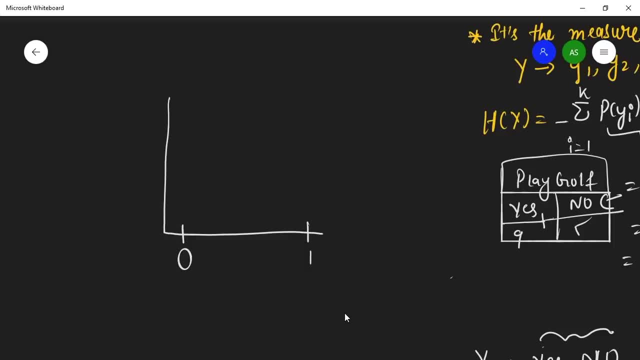 have zero. here we have one. okay, so I, I hope so. I'm I'm not able to draw it, but let me try at least. okay, and the highest entropy is one. the highest entropy is one. okay, is one, and this is the diagram of entropy. this is the diagram of entropy. okay, so the highest 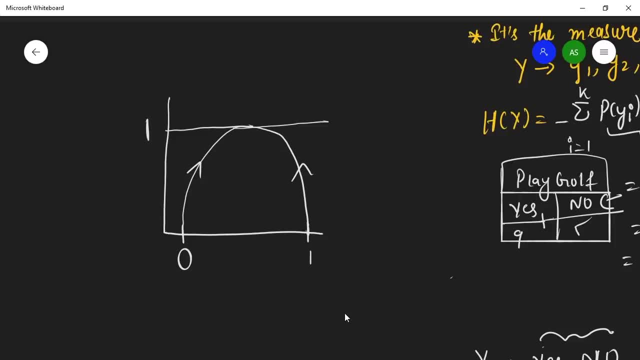 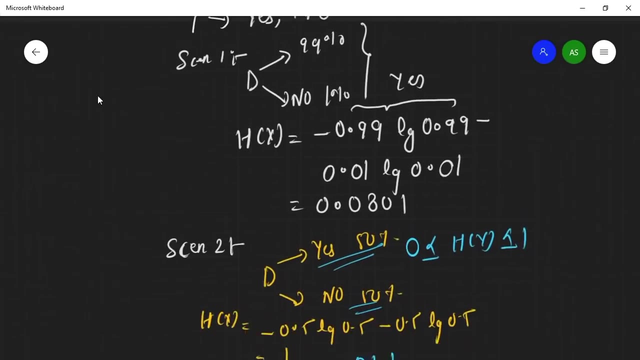 entropy can be one if you're taking with this equation. okay, I have already showed you, approved you, so this is an example of entropy. okay, great, so we have seen the entropy, which is the measure of a randomness. so now let's talk about the another attribute, selection measure, which is information gain. okay, we'll talk about information gain, let. 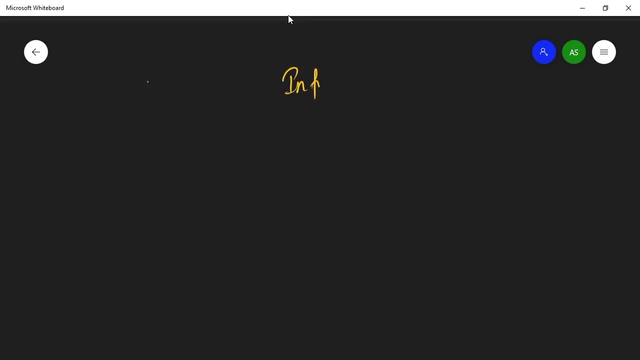 me write it down: information gain, and I will take an example of I. I will explain you information gain with the help of one data set, which is all I have already showed you. I thought I will give you a surprise with that, but I've already showed you. let me show you a little bit more of that. 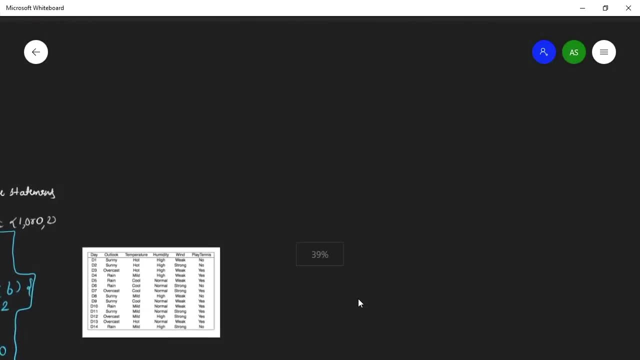 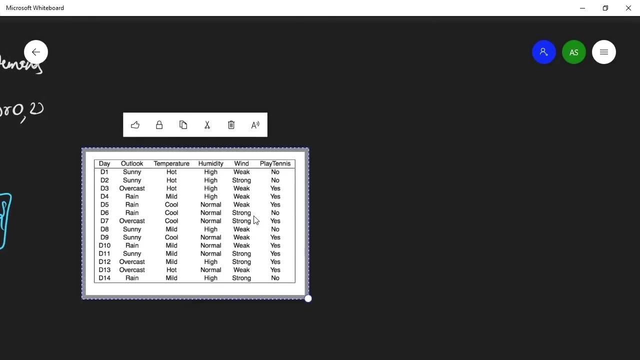 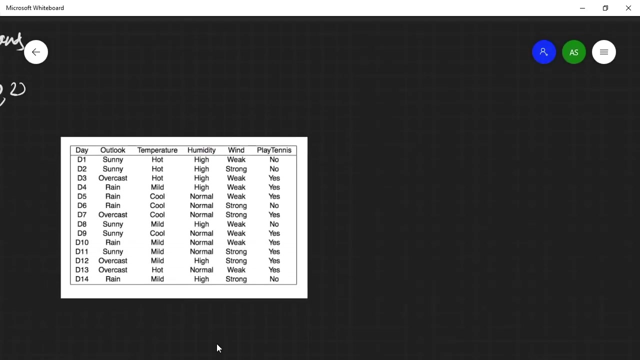 show you again. so here we have that data set. let me show you. yeah, here is our data set. okay, let me draw back. look at this, okay, so here is our data set which is played tennis. okay, um, this is a play tennis data set, and what you will do, we will, I will make you familiar. uh, just, 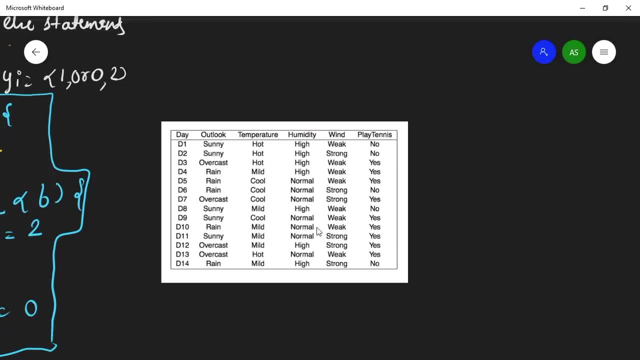 see this data set. a look at this data set. I will be looking, I have already looked at. okay, so here you have a plate and this is a target variable and you have these features. so we will see which feature to use or which feature to not. okay, so here, um you, you can just see what I'm. uh, you have around one, two, three, four, five, as 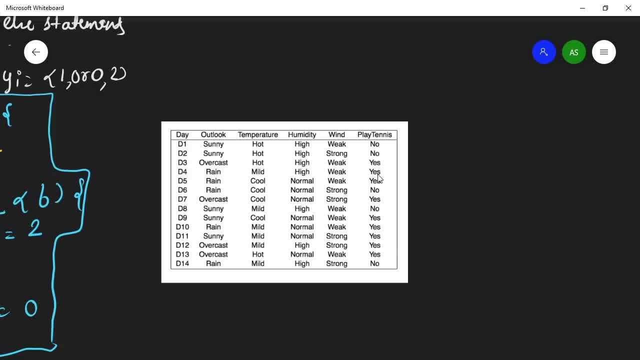 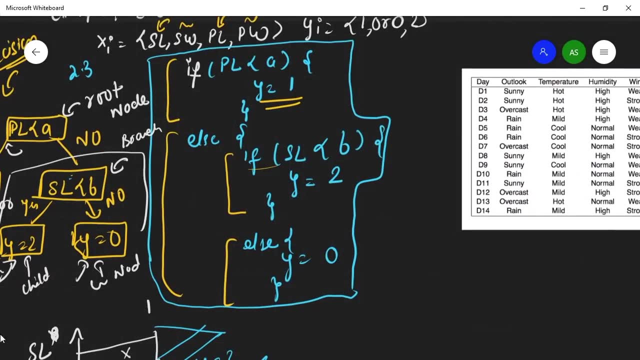 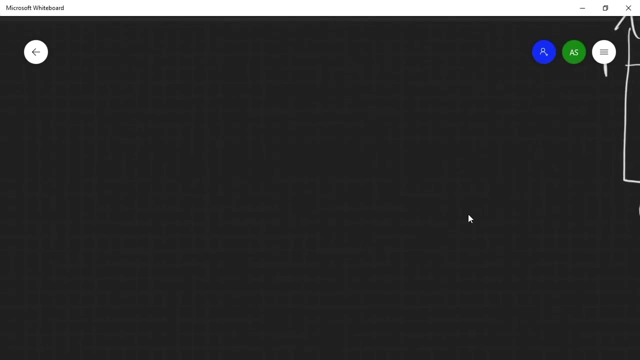 a no and one, two, three, four, five, six, seven, eight, nine, nine as a yes. okay, so we will. um, you just succeed, see this. and now let's come back to information game, you understand. first I will give you an overview of what information gain is, and then we will dive deep. oops, where is my? I don't. 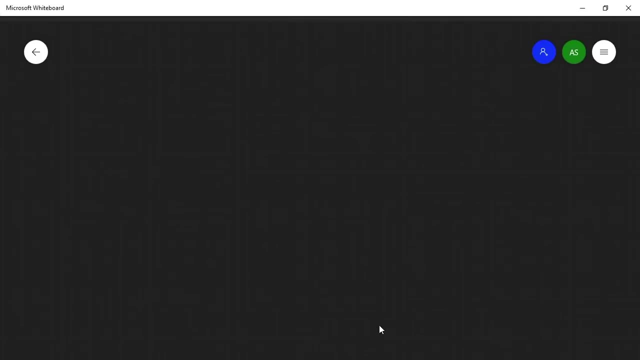 know why my computer is lagging? just give me a comment why it is very lagging, okay, so here is my information game. okay, great, I know that everyone is able to see. yeah, okay, great. so let's consider you have the data set B. okay, so you have the data set D, like this. let me consider this: 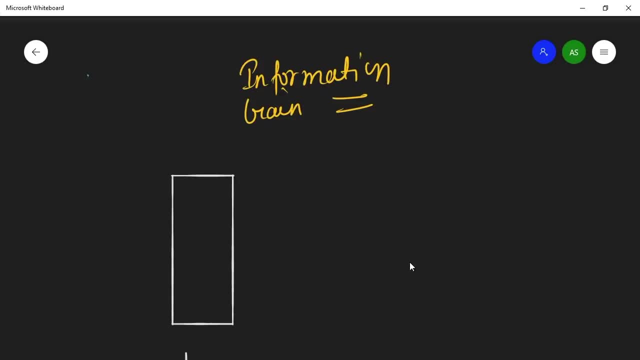 as a data set. let me consider D. oops, wow, it's. we have a data set which is D, and what you do? you further divide this data set into your- uh, further data sets, further, smaller sub sub subsets of this data set, and how you will divide the subset of this data set. it means that you divide this data. 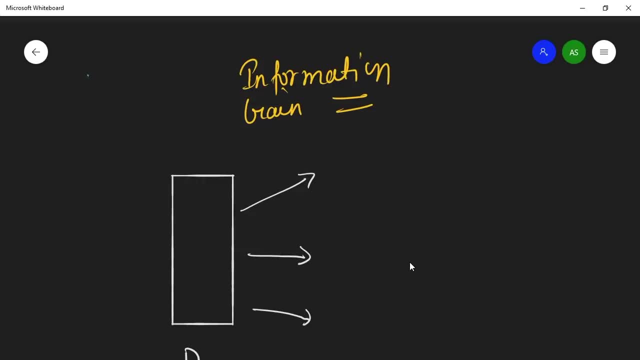 into versions, and what versions may be. let's take an example of Iris data set. okay, so what you, what you do, what you do, you divide this setosa, versicolor and virginica into three data set, which concerns setosa, versicolor and virginica. okay, so, whatever. examples of setosa. 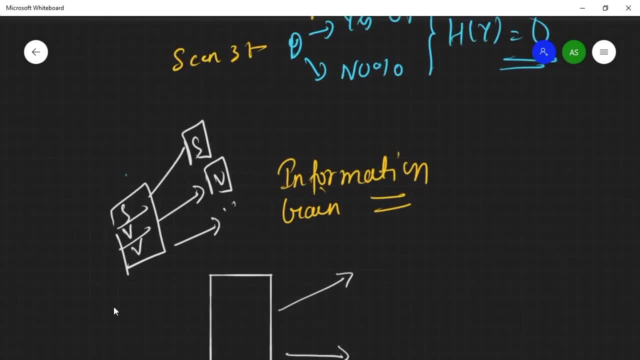 will come will go in this data set. whatever examples of virginica will come, will go in this data set. whatever, uh, whatever- examples will go, versicolor will go in this data set. so that's who you, what you do. you divide your data basis on the number of a label. 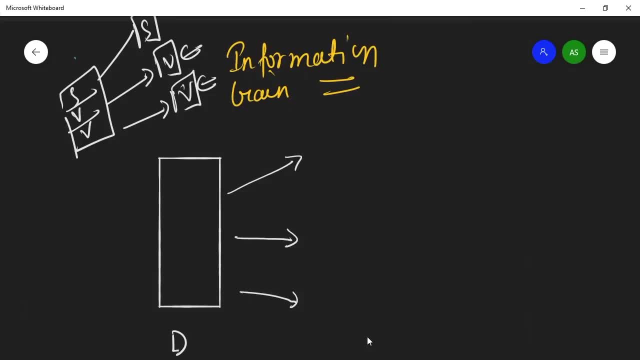 and I'm talking about binary classification for classifier or uh, classification task over here. okay, so what you do? you divide your data set, first to divide for dv1, then you divide for dv2, then you divide it for dv3. okay, dv3, okay. and what you do? you take out the entropy. you 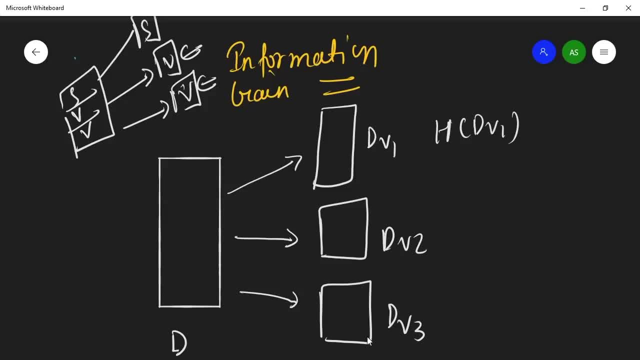 take out the entropy of this dv1, you take out the entropy of dv2, you take out the entropy of dv3- okay, and maybe there's this kind of setosa versicolor virginica. you take out entropy and then you take out the entropy of your whole data distribution, okay. 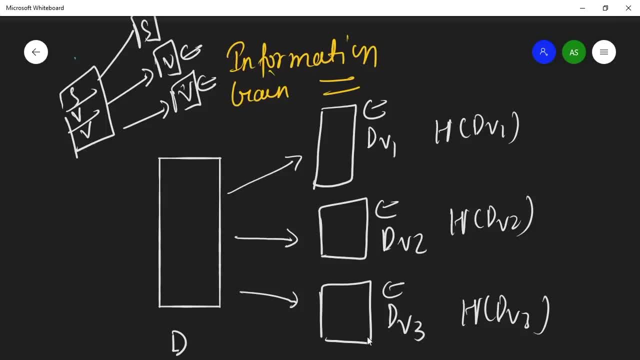 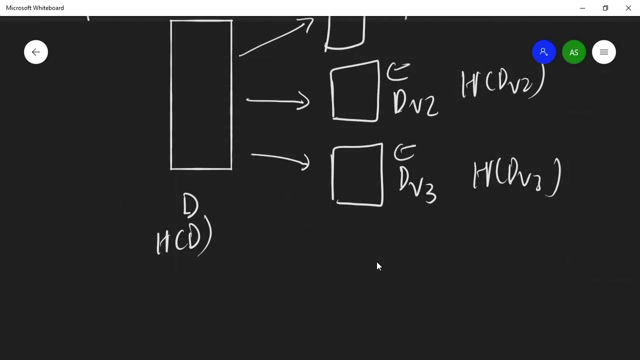 before splitting. so you take out the entropy before splitting and then you take out the entropy after splitting. okay, so take out entropy before splitting like this: okay, after that, you, you minus it, you subtract, you subtract your uh edge of D, which uh the function. the entropy means previous entropy means previous entropy, this entropy edge. 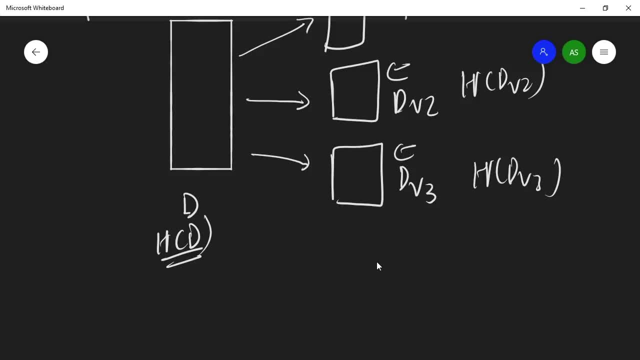 of D, which is the entropy. before splitting minus minus, let me write it down: minus the weighted entropy, which is this, which is whatever the weighted entropy will come. so let's see how we that have. a help. help of an example what what I'm talking about? uh, this, how? 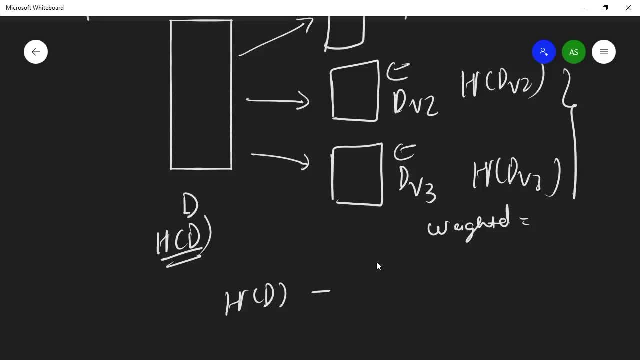 do you calculate? one example to make it more familiar: uh, weighted entropy. how do you take out the integrated entropy? so you just multiply, uh, minus it with the weighted entropy. okay, after splitting entropy. after splitting. so let's see how it is done in more detail. okay, so I've just given you, give you what. 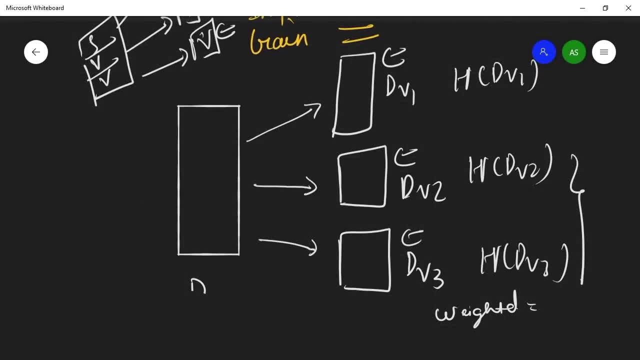 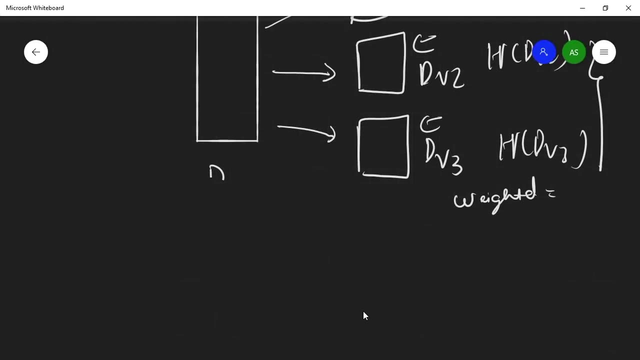 the. what the formalize is just to divide your data into subsets of your data, like the divisions, and then you take out the entropy before the splitting and then you take out the entropy after splitting. okay, so let's see. so, uh, first let's take out the entropy of division number one. of division number one. 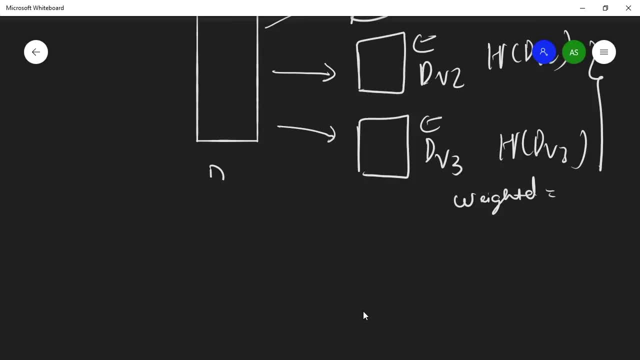 here I'm going to take out entropy of division number one with the help of that Platonist data set. okay, so oops. H of dv1, which is he there? we have three. five means first time writing for. uh. three means first time writing for yes. 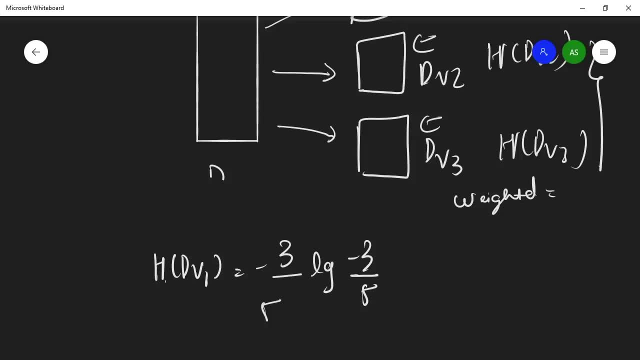 okay, first I'm writing for yes, where we have our, where we had divided our day, the data set into a yes or no. so there we are having total of five examples where three examples are yes and two examples are no, and out of five. okay, then the entropy will be 0.64. okay, but you then again. 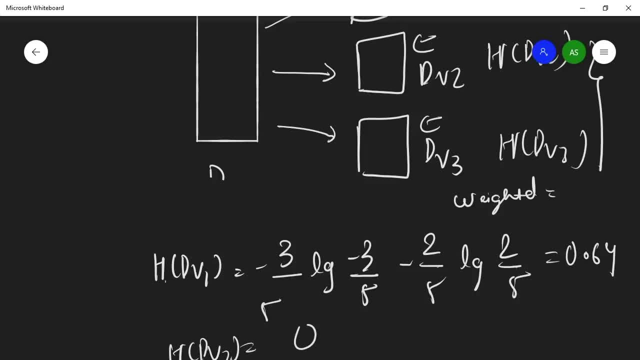 what do you do? you take out entropy of your division number two. you, it will be zero and it in the same. you take out a division number for division number three: zero point ninety seven. okay, but then what you do? you do the, you take out the average entropy and that's, that's equals to. 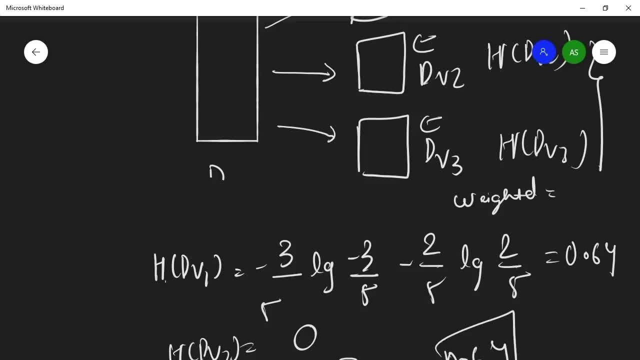 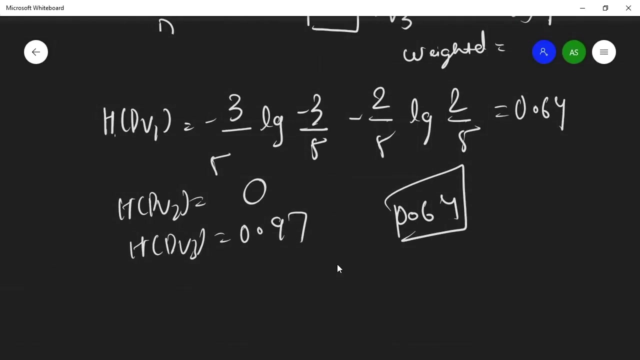 0.64, then that's equals to 0.64, and the formula for calculating your weighted entropy is like this. just wait for a few seconds. the formula for calculating your entropy, or weighted entropy, is like this: let me write it down first, what you do. you take out this. I think it says it's not 64, it's yeah, so I will just multiply. 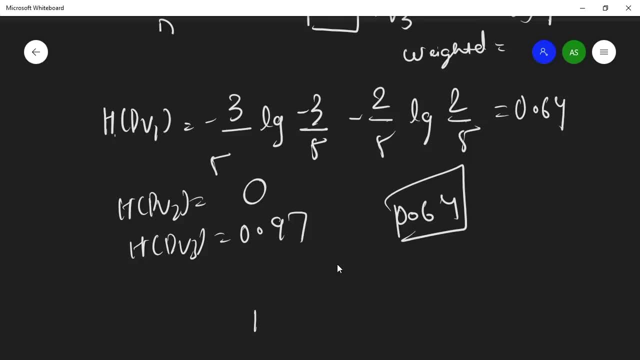 with the first division, number one. here we add d1, the norm of d1, divided by d times, the entropy of d1. then you, what you do, you plus d2, the norm of d2 times and entropy of d2, plus norm of d3, normal d3, and this is the division number three: data set. 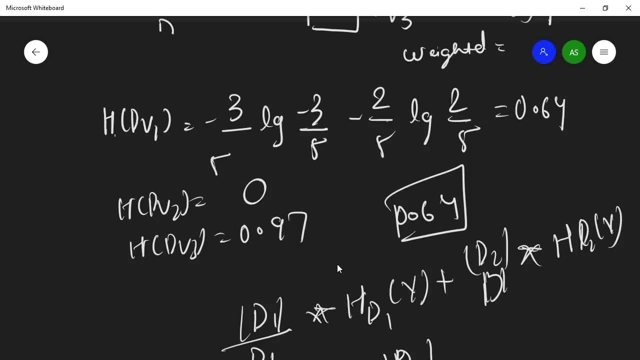 divided by the norm of d. okay, and this is your full data. this d is a full data, so you take out the size of that full data. okay, then you again d3 y- okay, and then this is your avated entropy that you get after all of this, after you've taken out the weighted entropy. 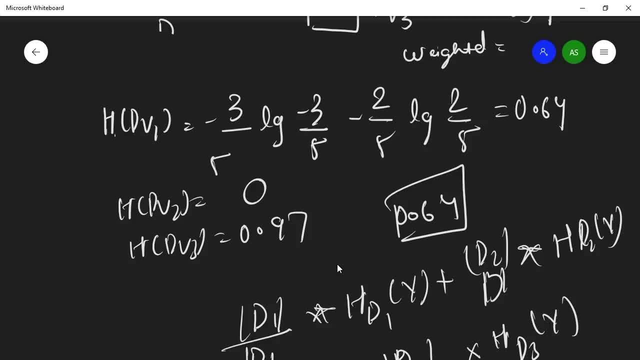 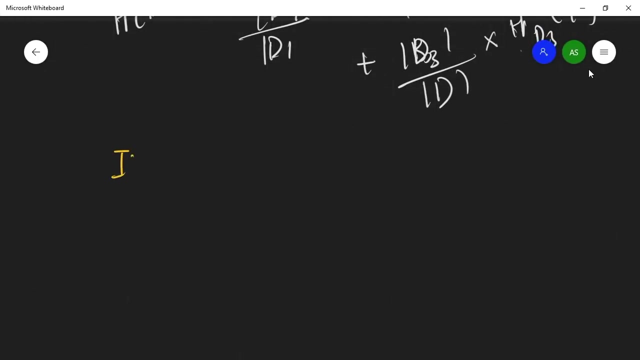 and that that will be equal to some number. and then what you do? you subtract. you subtract your entropy, previous entropy, you subtract your entropy before the splitting. you subtract your entropy before the splitting. minus, minus you get after splitting. so let me write the formal equation for IG, what you get. okay, so IG, IG equals to y and any var means variable, maybe. 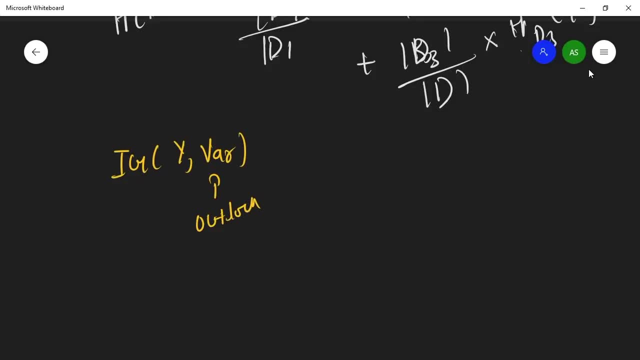 variable can be Outlook. a variable can be Outlook or temperature, temperature of that from that, or windy, or humidity. okay, so in that we will check. if, though, if the higher the entropy, a higher the information gain is, we can select that as a root node. okay, so what you do? you just. 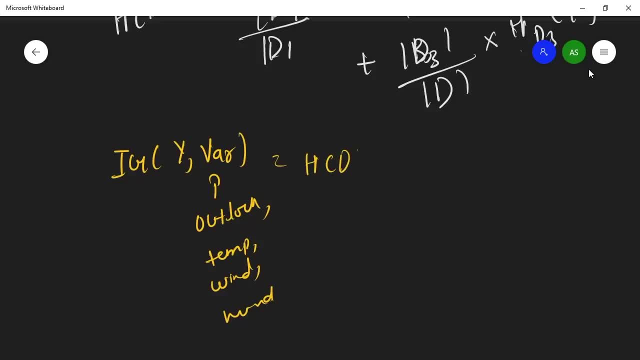 you just take the entropy of your data, full data, and then you pre pre means of your data and then this it minus i equals to one, although all the way down to the key, the norm of di means the division of your data and this is simply, uh, the maybe citasa, or then versicolor, or yes or no, like that. 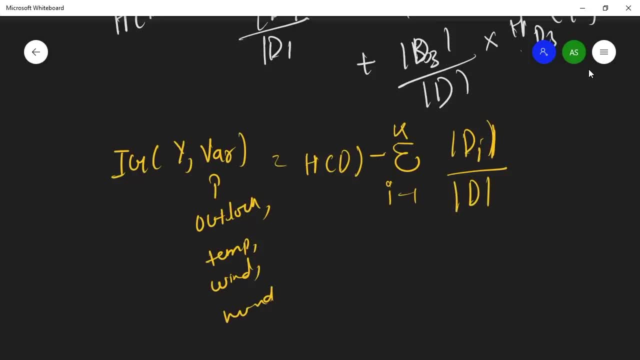 so, divided by the full, full d times the entropy of di. okay, so this is your weighted entropy, this is your weighted weighted entropy and this is your. this is your entropy. okay, before you're splitting, and then you will get the information gain for that. you for that variable. okay, so we will see. uh, one more example later on. 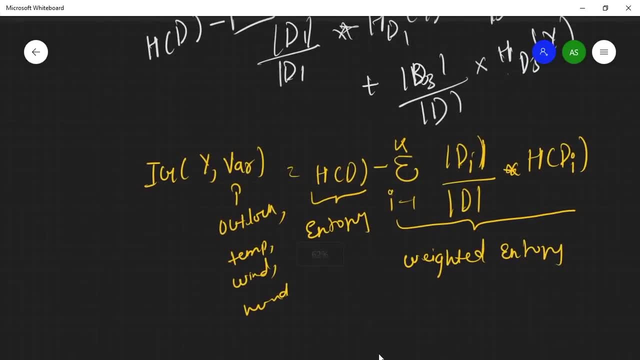 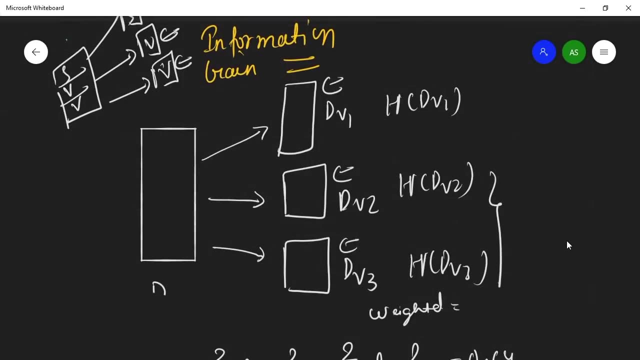 when, when, we will be building our own uh decision free by yourself, mathematically. so again, let's recapitulate what you have seen so far. we have simply seen, we have simply seen. so let's go back to that data set. let's go back to that data set. so. 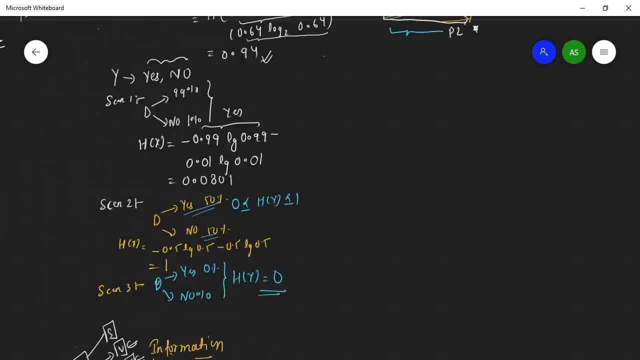 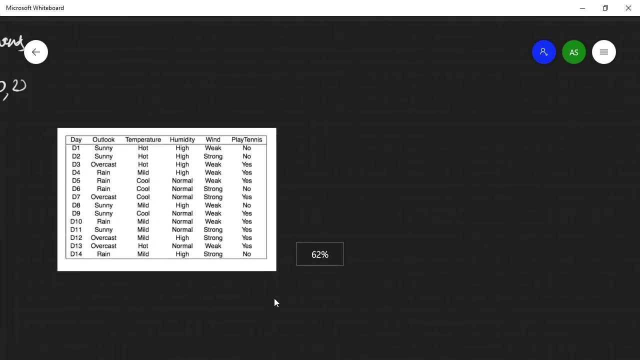 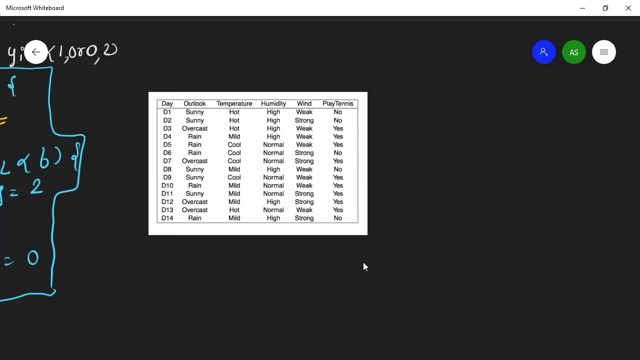 my data set. i don't know actually where. yeah, here is my data set and here what. what we do? we take this data set and we simply um divide this data set into multiple divisions, into two divisions. okay, so we divide this data data set into yes and no, okay, and whatever number of examples will come. 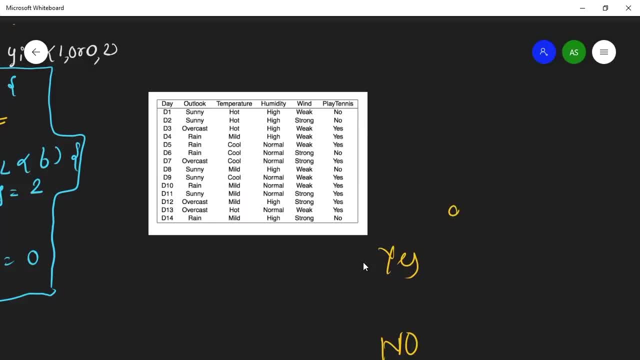 we take out. let's take an example: here we have nine over total number of data examples and here we have a five over total number of examples. okay, so what you do you? simply, nine by fourteen, log of nine by fourteen, minus five by fourteen. uh, log of five by fourteen. okay, then you will get. 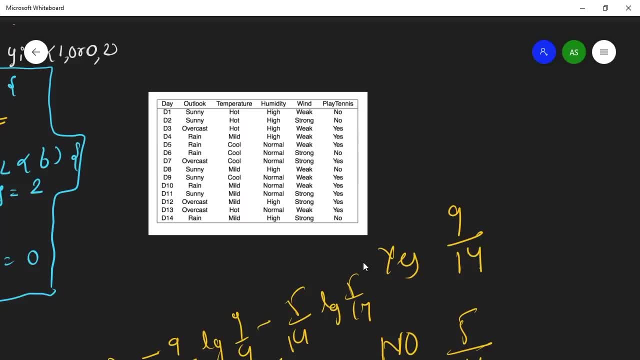 some entropy, which is your entropy of your data, okay. entropy of your data before is splitting, okay. so that's what the entropy is and i- and i hope that you understood what i'm trying to say over here- and this is your for yes and this is your for no, because you have added a submission of. 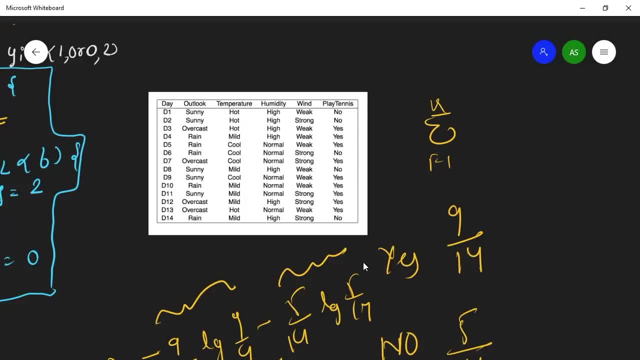 your entropy like this: i goes to one all the way down to the k, then you have a probability of y i minus the log of means, with base 2 probability of y i. okay, so that's what we are doing. you are doing the same over here, but this time you have two. so that's why you. 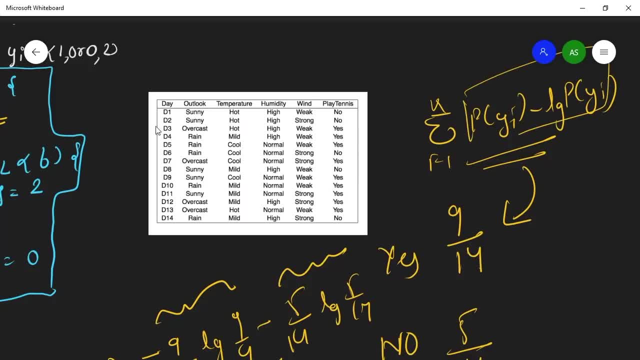 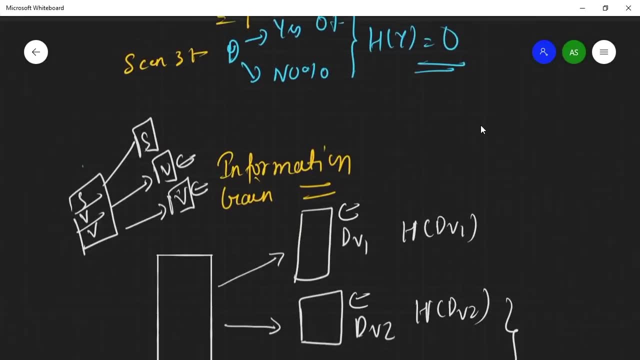 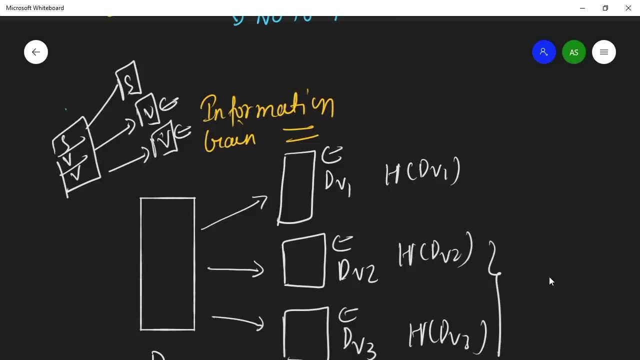 are doing two, and this is only for binary. you can see equations for multi-class. okay, so that's what the um information gain is, and here what what we do. we take out data and we divide our. first we take out the entropy of that data and then we divide our data into multiple divisions. and here 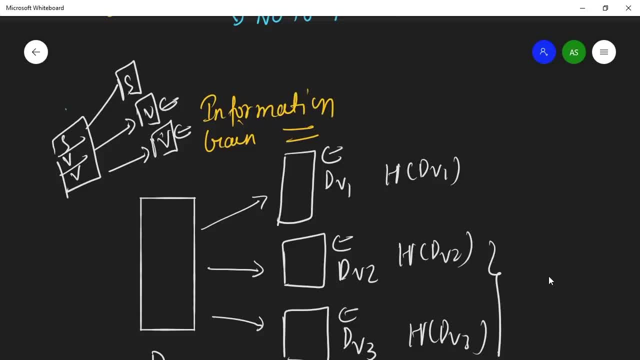 we have three classes um categories, so we divide it into three categories. if you have two categories, you can divide two categories and then take out entropy of that categories and then you take out the weighted entropy. okay, without rather taking of the average, you take out the weighted entropy of that. 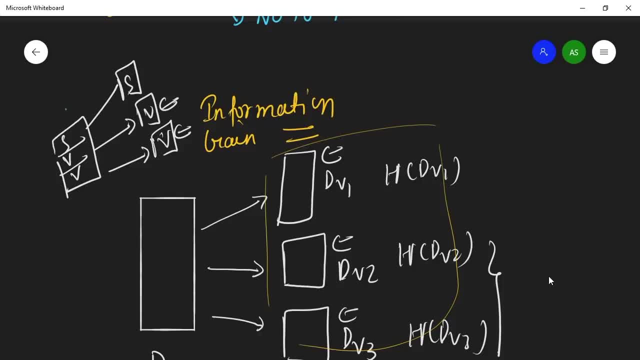 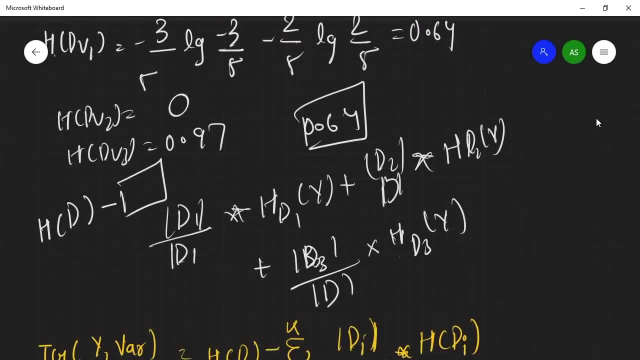 after splitting these all, you take out the weighted entropy, then you subtract, and how you take out the weighted entropy, here is an equation. i'm going to give it to you. it's just i have already given, but more formally, this is the equation for weighted entropy. okay, so what you do? you simply, it's the. 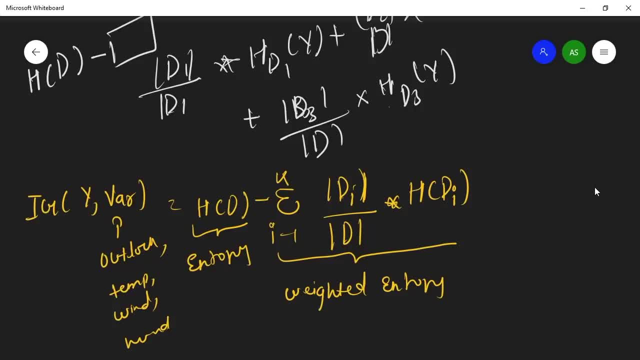 norm of d means no divided by what is the number of a full means. here we have number of a no, number of a number of no divided by total number of examples times the entropy of that di. okay, so that's why, who you, how you take out the weighted entropy. so, after taking out the weighted entropy, 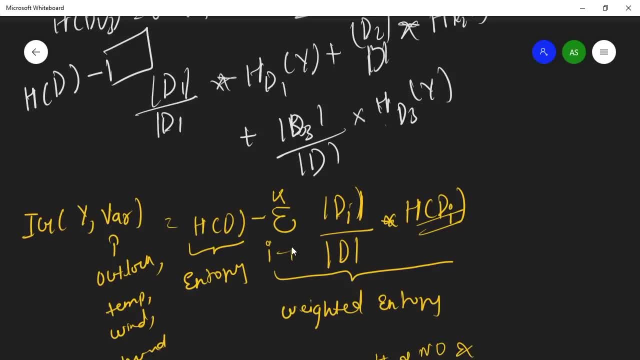 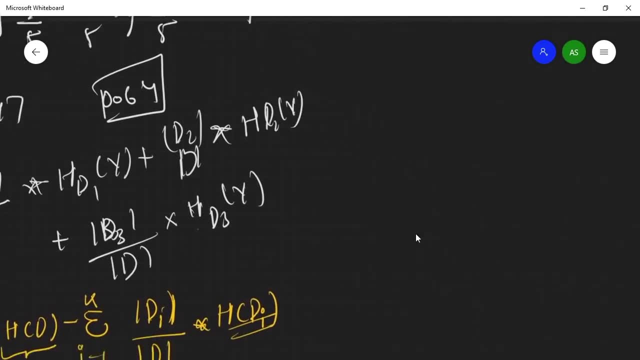 you subtract the previous entropy minus the weighted entropy. okay, so that's what we are doing. and information gain. i really hope that you understood. information gain, okay. okay, so please implement, see if on some blocks. if you want, or either you can ask me in discord, so i'll be very 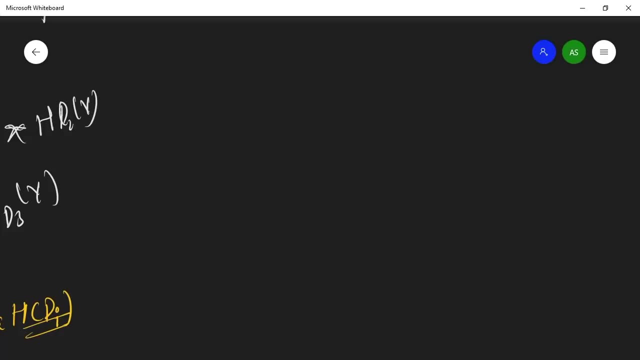 happy to help you. in the newer you can find the discord server. in any new era, new video on new era you can find at it and you can join and there is a lot more that you can. and also, if you want to support, please kindly go to new at our youtube channel. new at our youtube channel and please 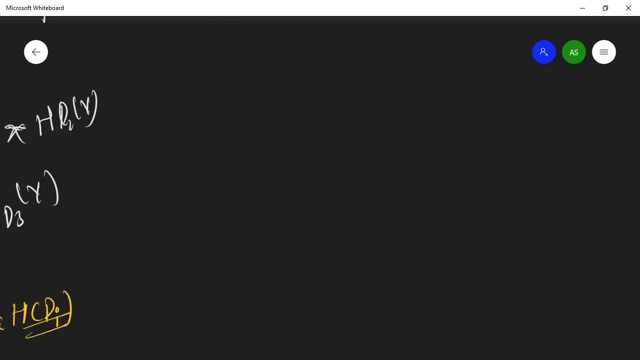 subscribe that youtube channel, okay, and if you can watch the whole tutorial on new era, okay, because you are going to get the uh whole ad free over there, okay. so, uh, now we have seen entropy, then we have seen information gain, now it's time for uh talking about uh, guinea impurity, guinea impurity. 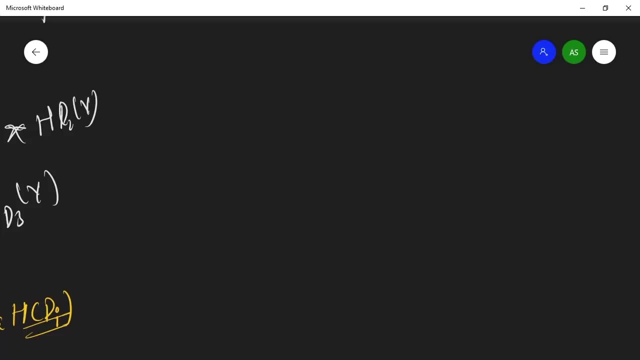 okay, so this is also the most famous. it's a most similar and most famous that is used today, which is guinea impurity. guinea impurity and it's just equals to. it's very, very similar to entropy. it's a very, very similar to entropy. let me, this is: 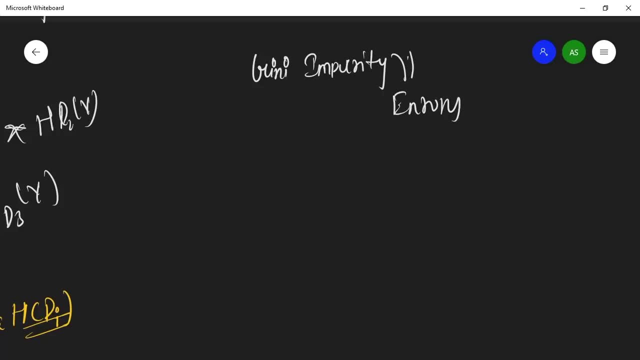 i use things very, very similar sign. okay, don't comment it like this. just i have just said it like this. it's not i using it's, just i have. it's very, very similar to entropy. so let me give you one equation, uh, the equation for calculating the guinea impurity. so i g and it is not information. 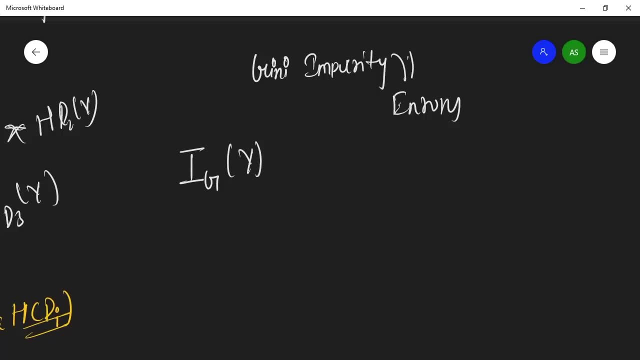 gain. this is a sign for a guinea impurity. of y equals to the 1 minus i equals to 1, all the way around to the k, and again it is the your y variable, not any anything. it's the y variable again. i have already seen: y equals 2. 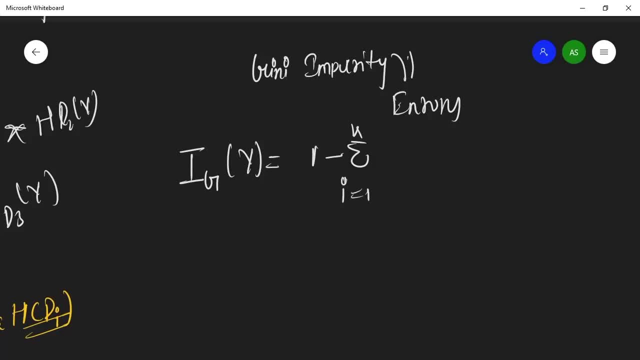 and we also know min 2 or it also vertical. so unique values in your eye times the probability of y. i squared okay. so that's the that's the thing. and again, it's if, if we take a same scenarios, if we, how? i'm saying it's if we take the same scenario. 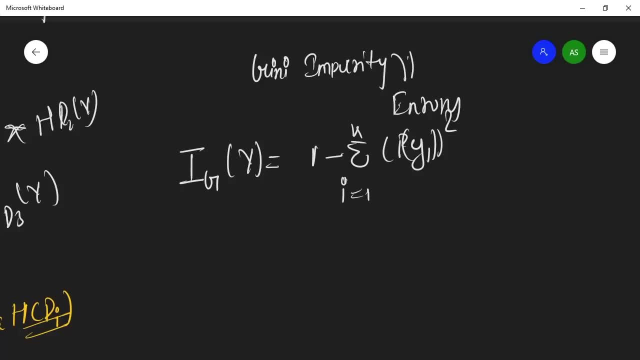 as we have taken entropy some scenarios. let's take an example of scenario number one. scenario number two, scenario number one: we are your yes, we have. let's take a. let's take, you have y to be two class category, where you have the unique value as a yes or no. okay, so what is the 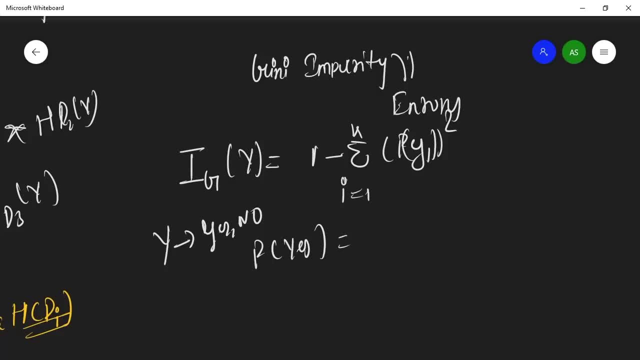 probability means what is the number of yes is 0.5 and what's the number of a no? is 50, okay, 0.5, okay, so what will be the guinea impurity gain? impurity will be 1 minus 0.25 is. 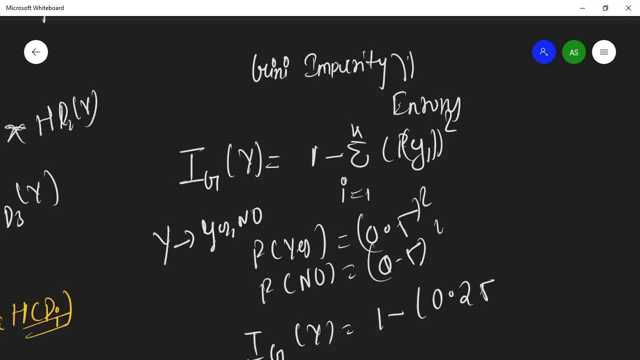 0.25. because if you square this, because here we are squaring, so if you square this and you again you subtract it, again you subtract it minus 20, 0.25, 0.25, then you are going to get a 0.5 and 0.5. 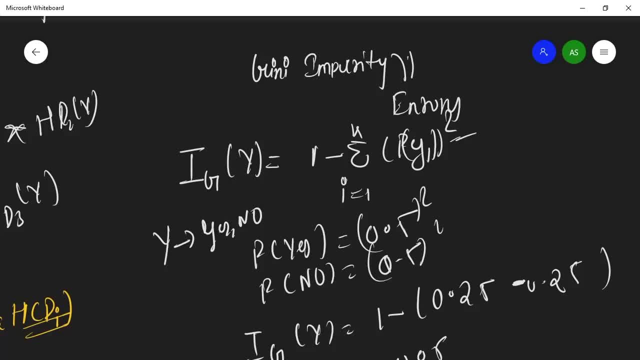 is maximum in guinea, impurity. 0.5 is maximum. in entropy we have one as a maximum. if it is this, 0.5 is 0.5, then it's needs for this pitting. if it is zero, then it's not need, if we can consider that. 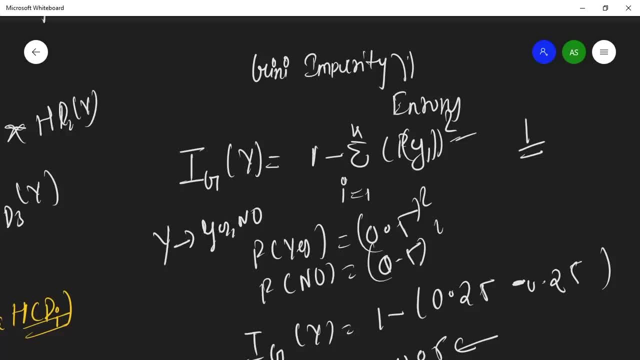 as a leaf node. okay, so that's the scenario that we have already seen in, and if it is in, in the case of guinea impurity, our guinea impurity, in this case, where you have 50 percent, yes, then it that that will be one, so we have. if you. but you may ask here, yush, what is the advantage of guinea? 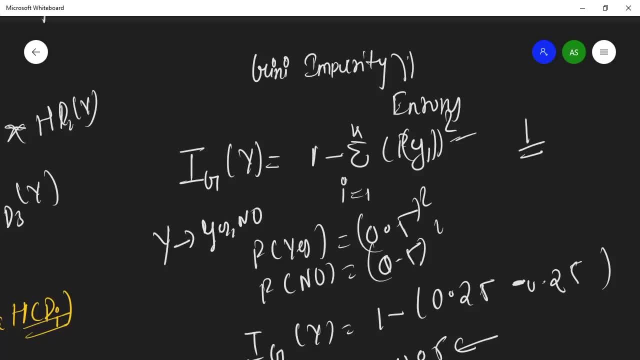 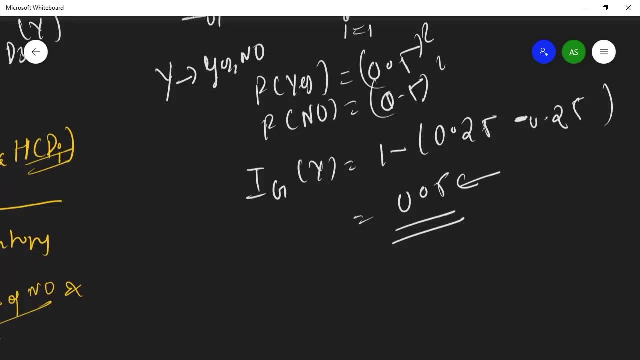 impurity user rather than using the entropy. so it is an alternative to entropy just to increase the computer, just to make it fast, because in guinea impurity, if you have seen we are just taking h of y- equals to the minus. the summation i equals to one, all the way under the k p of y i. 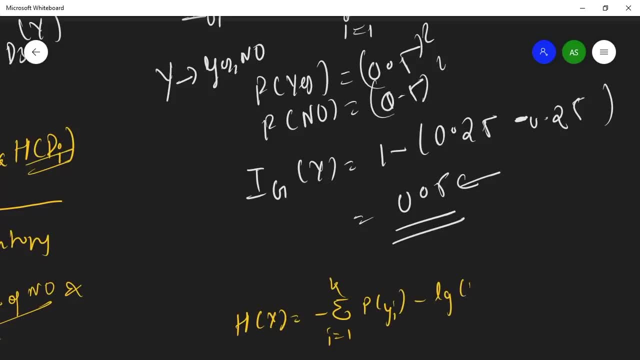 minus the log of p of y i. so here you can see, we are taking a log, and taking a log takes time, okay. so as an alternative, a researcher comes with a very, very easy way to make a log of p of y i. so here you can see, we are taking a log and taking a log. 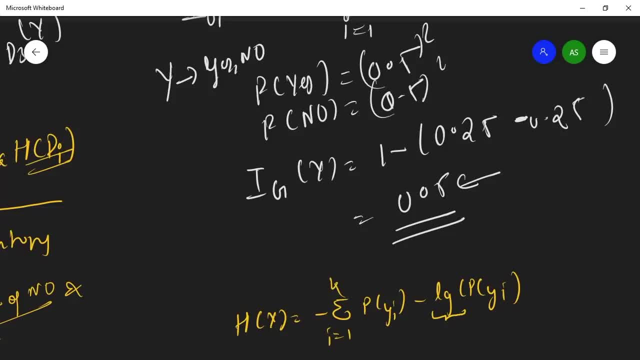 and under understandable wave. the one minus and this, these are: this can be derived, these are derived in information theory. okay, but I'm not going to go in information theory. but you can see, this is the for a gain. impurity, and this is most used as an alternative to give you it at entropy in impurity is most used. 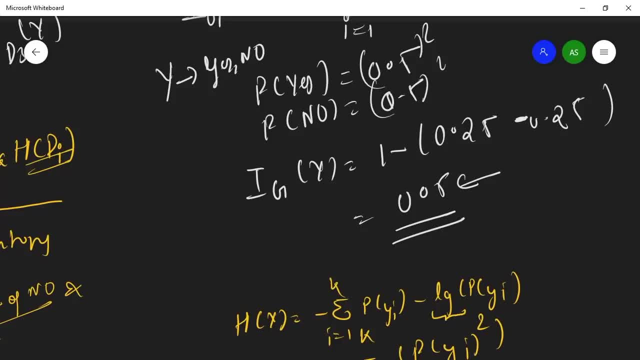 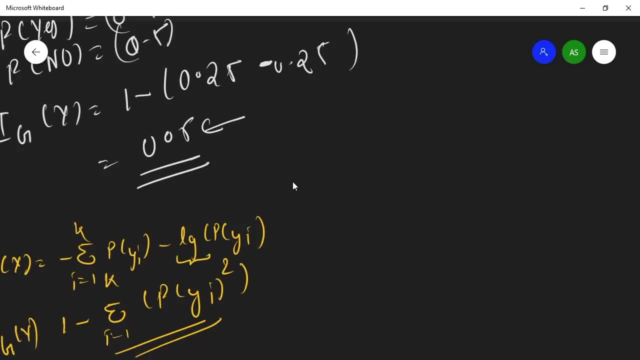 as an alternative to entropy. okay, so that's the thing, and I hope that you understood Guinea impurity also. so let's, let me make you familiar with the diagram. so here is the diagram. let me make first four gear. entropy first. here is for entropy. so here we have 0, either we have one, so here this is foreign. 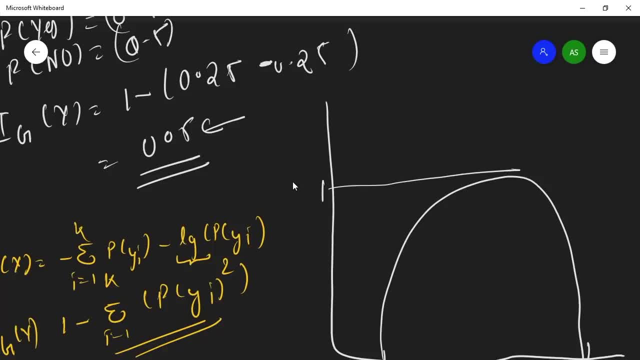 tropi. your maximum is one and this is for obviously some. something will default so. but the maximum is 0.5 in guinea impurity, so yellow one is guinea impurity, so positive. it means 4.5 in the guinea impurity. so if you take from around, 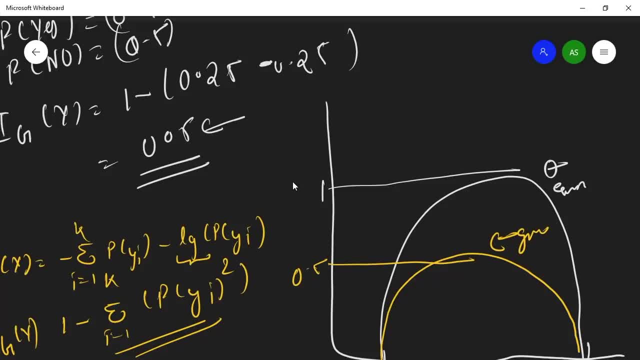 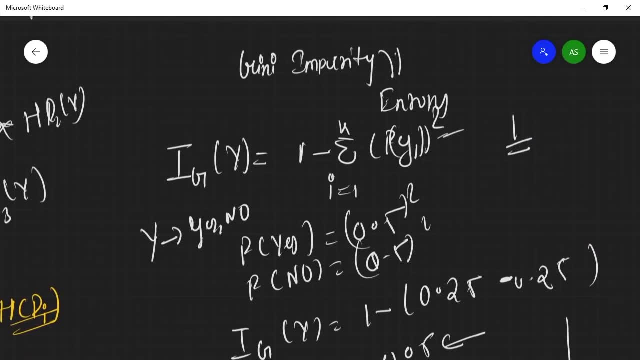 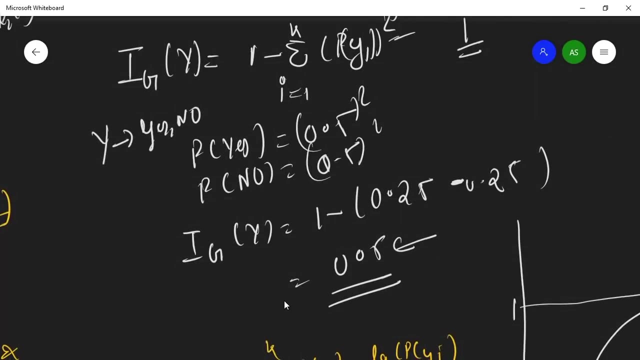 impurity and the white one is entropy. okay, white one is entropy. so i hope that you understood the why, why i'm saying: but why do you use gain impurity? because, because, just because it is more faster, because in we are taking log and that takes time. this more faster than um entropy, okay. 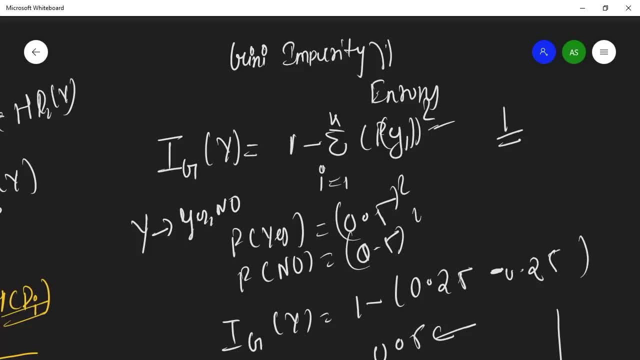 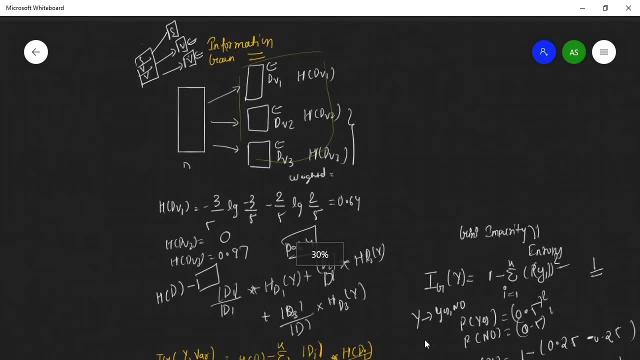 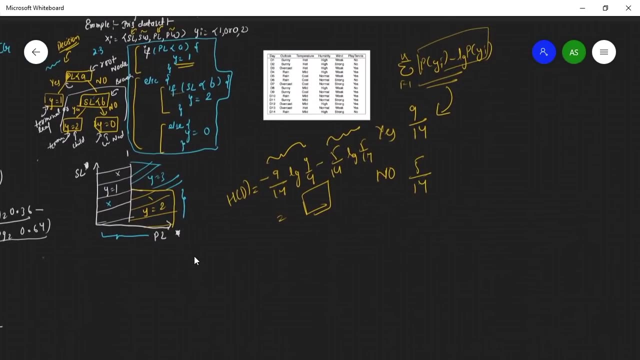 so that's the whole definition of all this, and then i'm recording till 51 minutes and i hope that you understood all of this. i hope that i have written a lot, okay. so, uh, we have learned a lot and i really hope that you understood also. okay, so now we will make one, a decision: tree classifier. 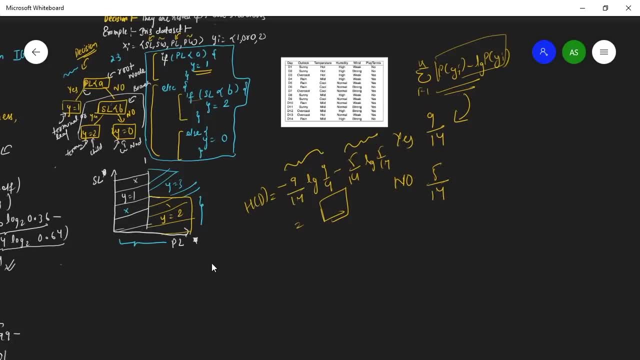 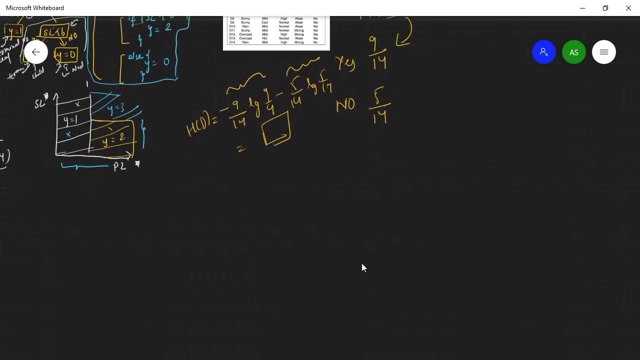 and i will show you the decision tree numerically, okay, how we do regression, task and decision trees okay. so first, uh, let's, let's do in a fast way. i, i i do have not a lot of time over here, but i will show you this data. 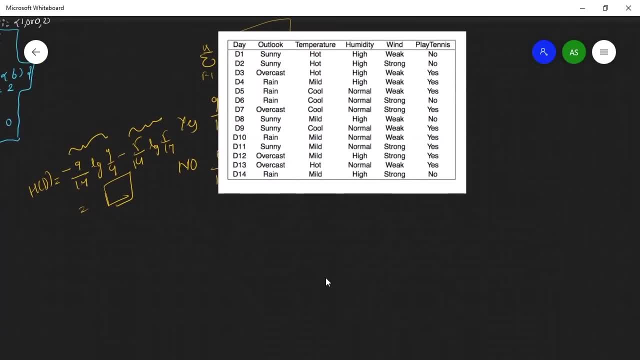 set. so here is my data set which i'm going to use. okay, so, first of all, what we do? we take out the entropy, okay, we take out the entropy. we take out the entropy of this whole data set. we take out the entropy of this data set h of d- oops, where is my pen? h of d and simply what? what we are doing. 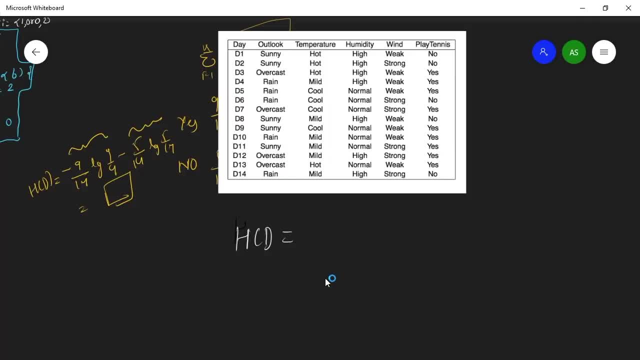 here we have two y's. so here we are taking the entropy of our data distribution d. okay, so that that will simply equals to 0.94, as i have told that you have to take out entropy before splitting. okay, for information gain. so we take out the entropy where this of this data set, as you have. 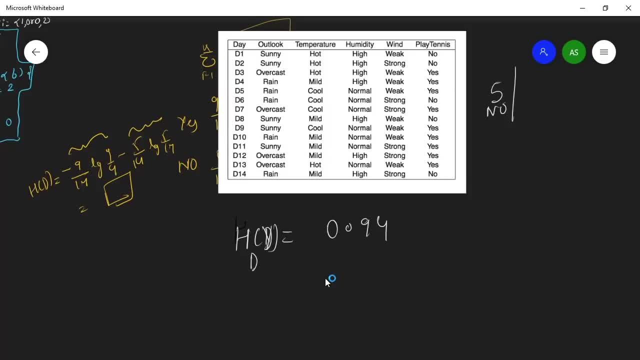 around five, no, five, no and nine, yes, okay, okay, so, and that way you can take it out: uh, if, if, if i want to make, i can simply make like like this: five by fourteen, five by fourteen, log of five by fourteen, minus nine by fourteen, log of, uh, nine by fourteen, okay, so, after you calculate, you will get this. 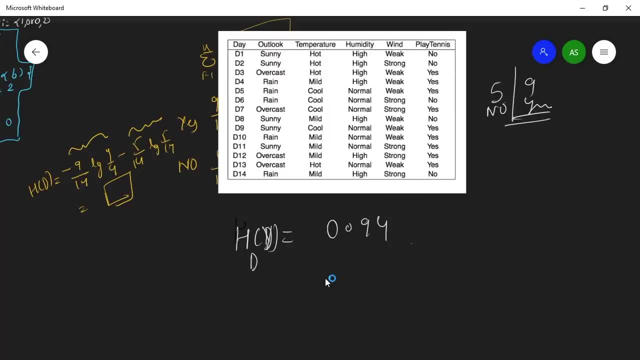 okay, so, but feel free to collect, correct me if, if i do anything wrong in calculation. okay, feel free to correct me in the comment box. okay, in mathematics we do. i'm just doing it fast you. just we have to remember the concepts, okay, so after you calculate the h of entropy of your 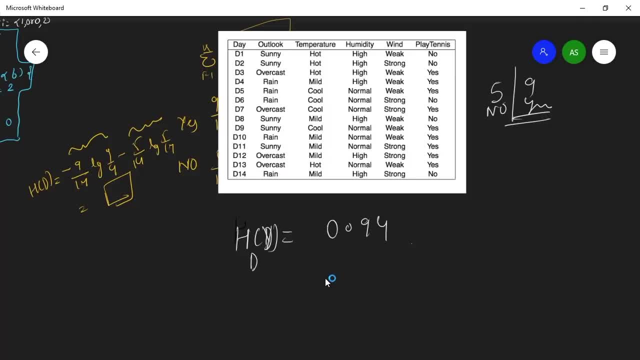 distribution. now, what you do to calculate the information gain? you calculate, you calculate the information gain, you calculate the information, you calculate the information gain. okay, how first you calculate the information gain for? you calculate the information gain for, with, for y, with respect to outlook variable means we have to check how much information that outlook variable contains. okay, so in output. 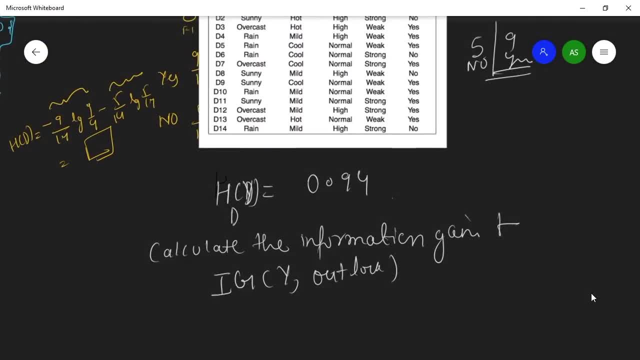 in outlook. here we have outlook. you can see over here that here we have outlook variable. so let me, let me take out. so in outlook, if you see the Y variable we have in sunny, in sunny we have two yes and three no's. we have two yes and three no's. then we have in outcast: 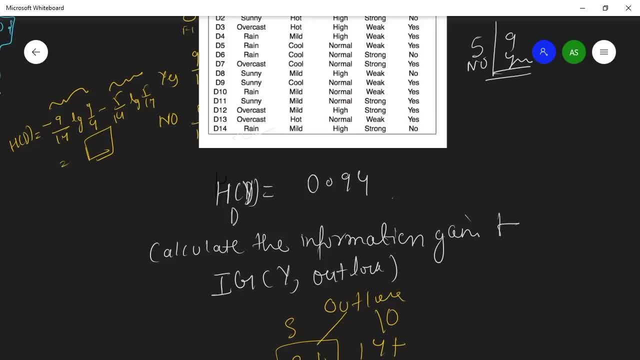 we have four yes and zero no's- okay. then in rainy we have two yes and three no's- okay. so this is their outlook variable. and here you have a two yes and three no's. four yes, zero no's. two yes, three no's. and this is for sunny, this is for 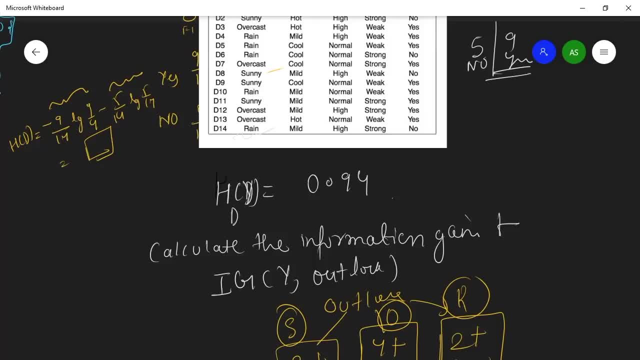 overcast and this for rainy, and you can see over here, okay, sunny, overcast and rainy, okay. so this is this: you can see that if you take out the entropy of this, entropy of this H of d2, d2, H of d2, then you will see. 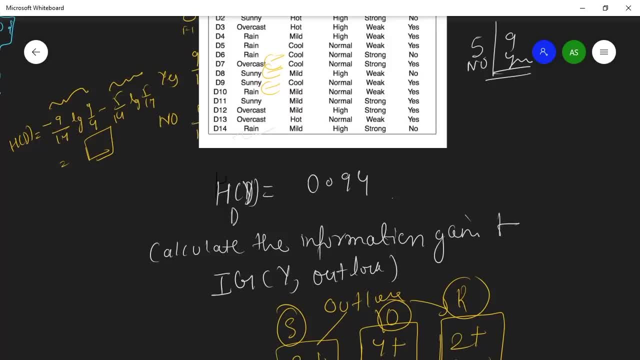 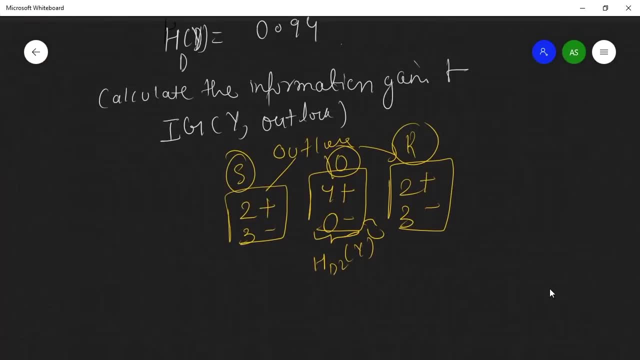 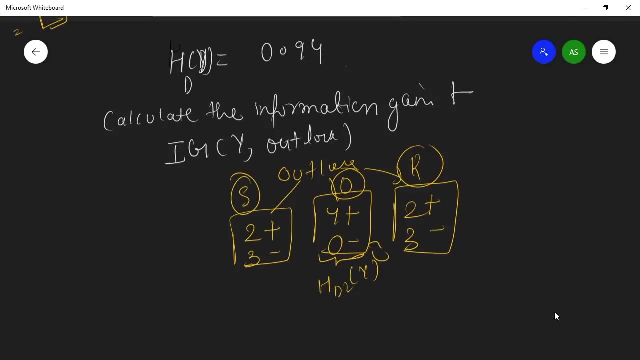 see that this is equals to zero, and you can. you can take this as a leaf node and it does not need further splitting. okay, so you can take this as a leaf node. you can take this as a leaf node because this does not need further splitting. okay, now what you do? you take out the entropy of this h of d1. 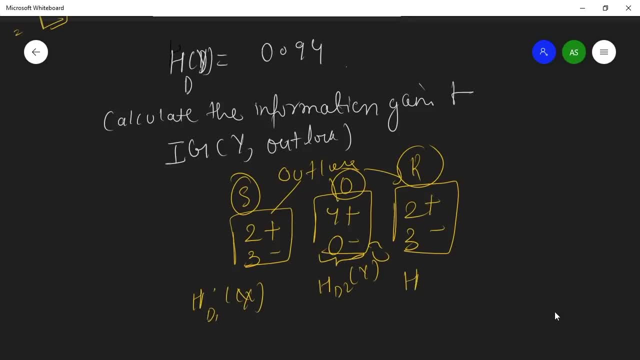 of y. okay, then you take out this h of d2, d3, y. okay, so the you have taken this data set, large data set. okay, taking this data set and it's split. you're taking this feature, split it. okay, so we have this before splitting. and then you what you will do. you take out the weighted entropy. you take. 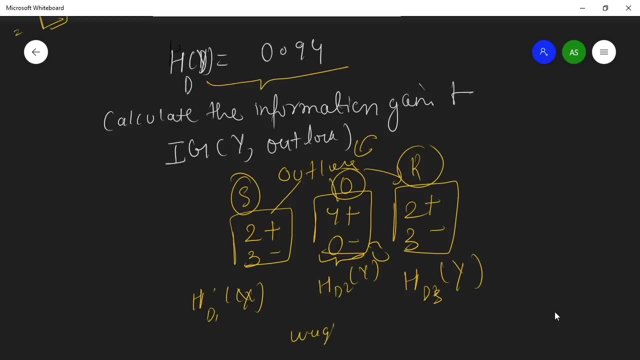 out the weighted entropy. weighted entropy, weighted entropy, which is equals to 0.69. okay, so what you would for information gain, you simply subtract: 0.94 means the previous entropy minus the weighted entropy, 0.69. okay, and weighted entropy: i've already shown you previously. 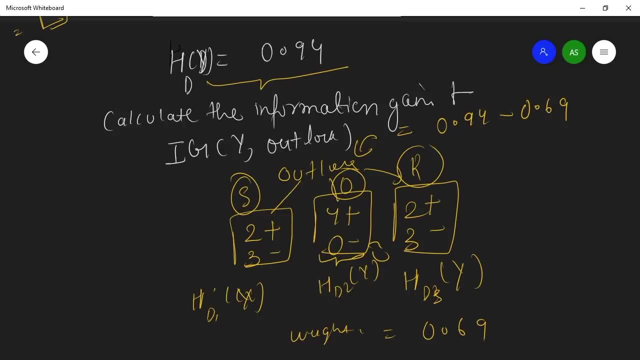 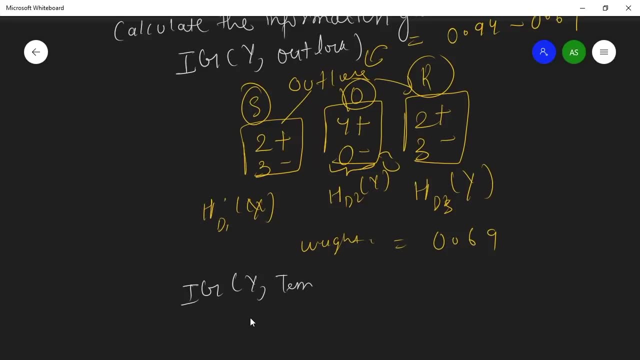 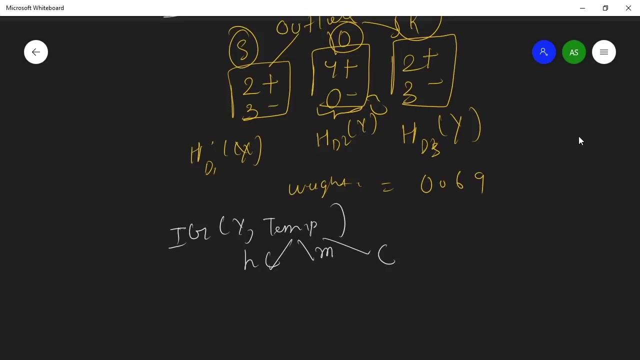 okay, and you do the same for uh temperature. you do the same for temperature, very, very in temperature you have y in temperature. where you have around in, you have three classes: high, mean, i think, mill. let me see high, mild and hot. high hot, mild and cold. okay, so in hot we have two yes and two no's. 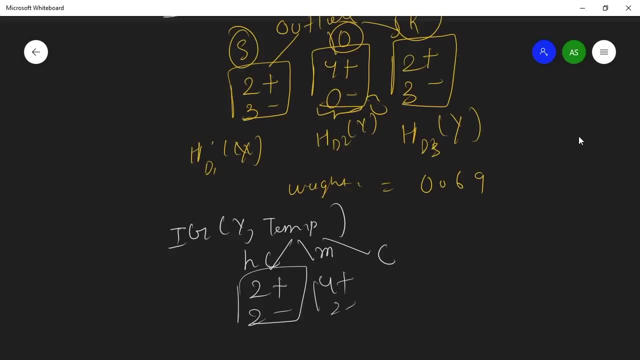 and there we have in mild we have four years and two notes, and then in cold we have three years and one nose. okay, then you take out, then you take out like this, and then you do for humidity, then, then then you do for humidity, humidity, and then you do for. 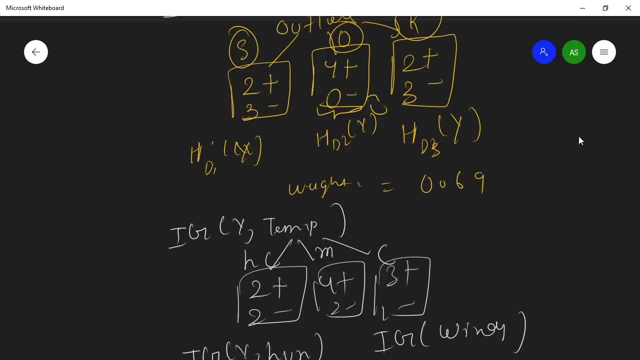 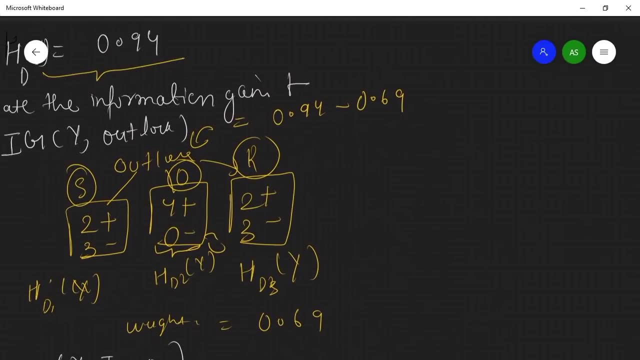 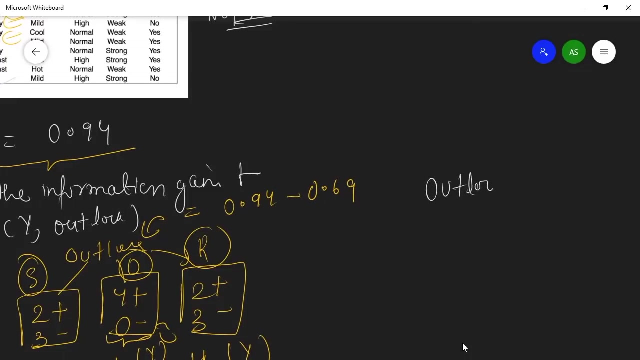 windy. okay, then you do, and it's fast that that the information gain in overall outlook is very high. okay, so, what you do? you take that into. uh, you take that one lead, that outlook as your root node as your root node. okay, then you, then you take that. 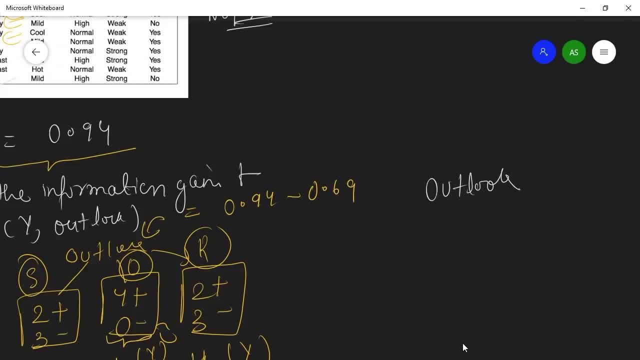 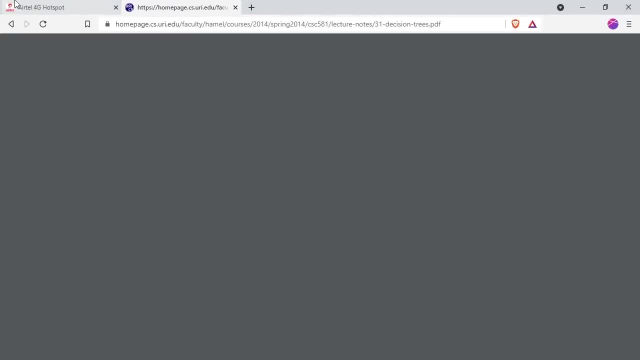 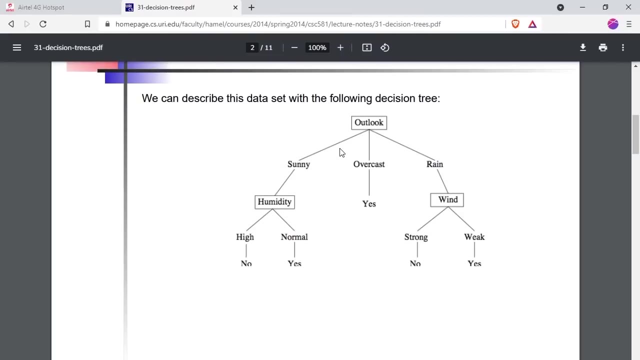 outlook as a root node, then you divide this, then you divide this. so here let me go to one of the one of my favorite decision tree PDF, where I I will just explain you what this is. okay, so you think, take this outlook as a root node. then what you do, you divide this, you divide this as we have divided into sunny. 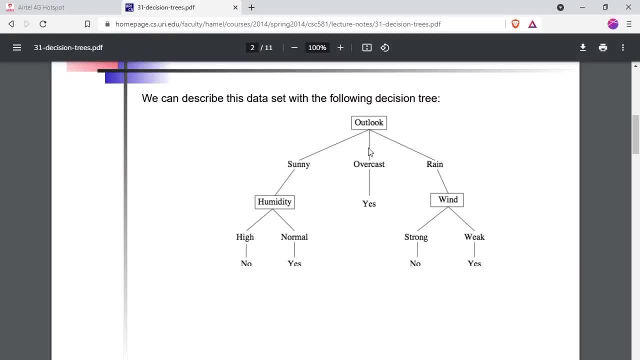 overcast and rainy. sunny overcast and rainy and overcast. you can see that we have our entropy equals to zero, so it does not need for the splitting, so we can consider that as a yes means we have four years, so we can consider that as a. 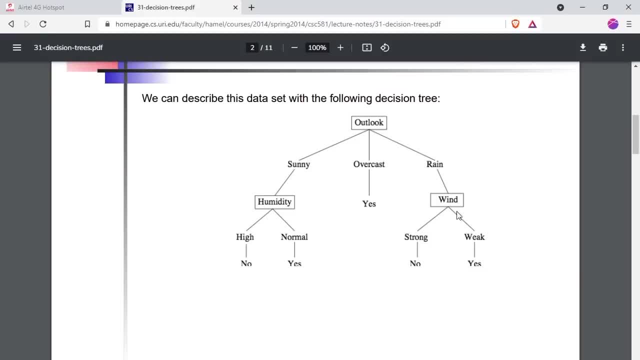 yes, because it's very pure, and then its needs for this fitting and this also needs for this fitting, and then at some point there they also become pure. where the entropy equals to zero, so, or the guinea impurity equals to zero, then you consider as a leaf node: okay, so this is how we make the decision trees and this: 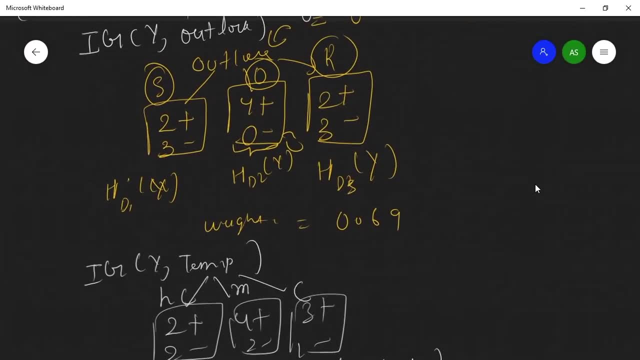 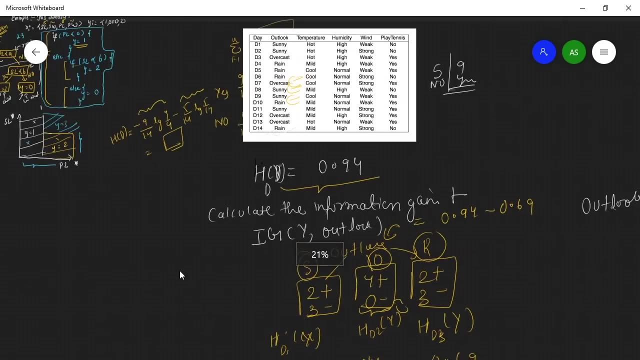 is how we calculate the information gain. this is how we made our decision tree. okay, okay, great. now I really hope that you understood decision tree, and now it's I. I also enjoy very much when I make these kind of tutorials, this kind of tutorials, and because it's 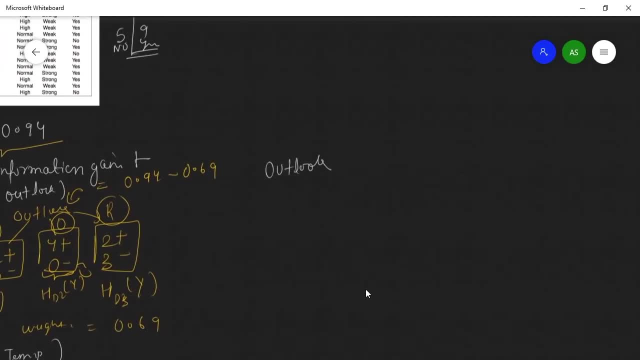 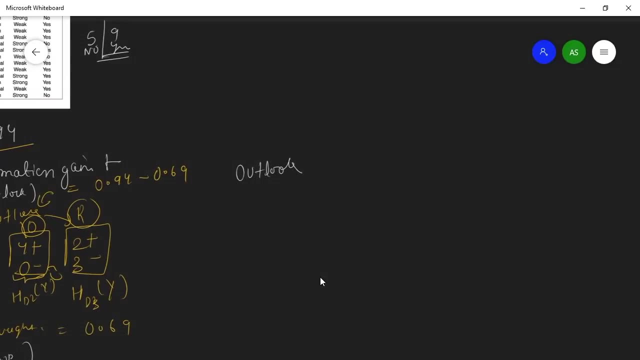 just amazing, just helping students to make this understandable things. okay, okay, great. now one, as we have only talked about classification, so as regression is not too much hard also, so in regression, let me show you what do you, what, what, what we do in regression. so let me take 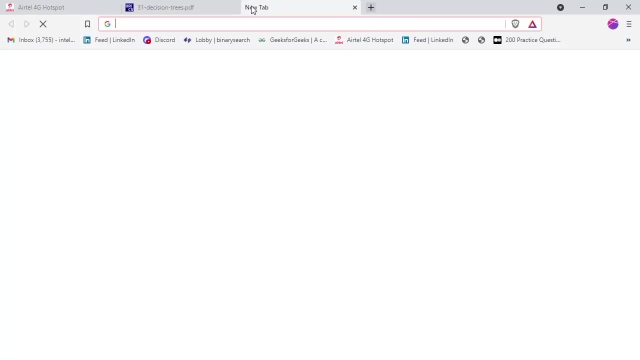 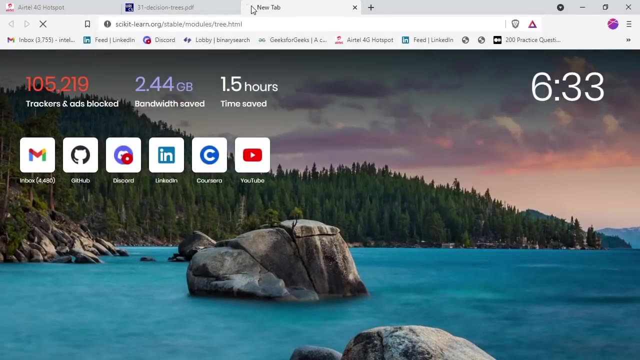 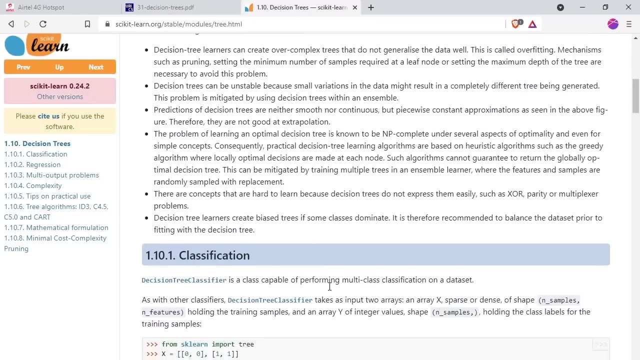 one. let me go to the cycle learn decision tree: decision tree cycle learn, I hope that stable. yeah, here it is. so it's explains very good. it's explains very in the win, in very good way. so let me make you what the what do I mean with? 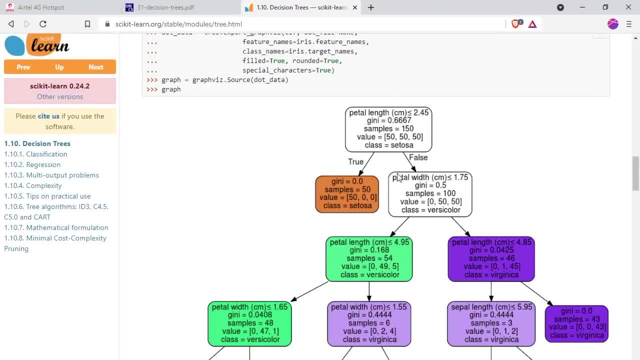 this. so let me take an example of this parallel and then pedal with so in the same way. I'm going to take an example of this parallel and then pedal with so in the same way. here you what you do. your petal length is more than or equals to zero. 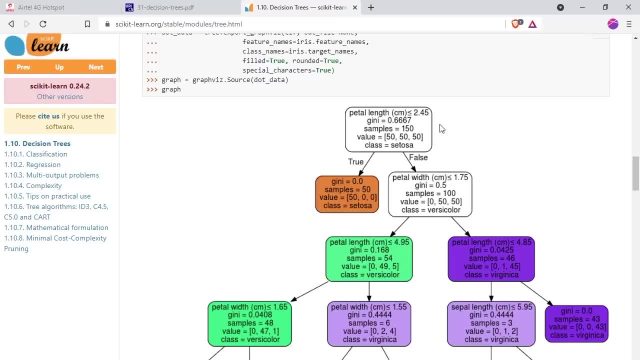 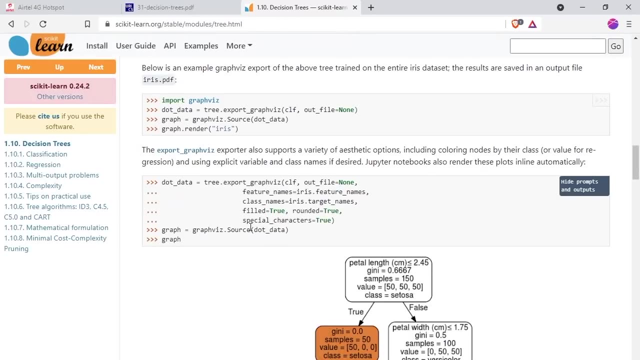 zero, two point four, five. then guinea period is high, the nude split it okay. here the guinea purity equals zero, then it does not meet for this fitting, but it is for this driftings, this trips, that okay. so here it seems to be over mistering, because if you, if you leave the decision, 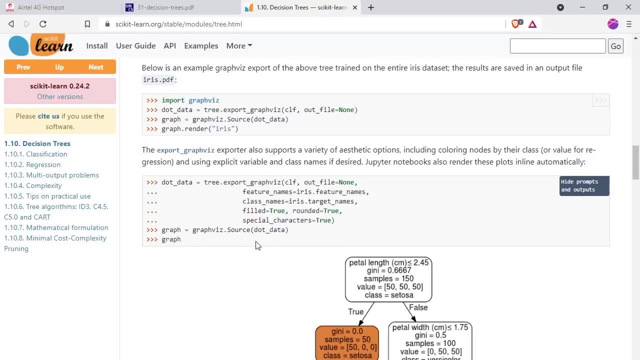 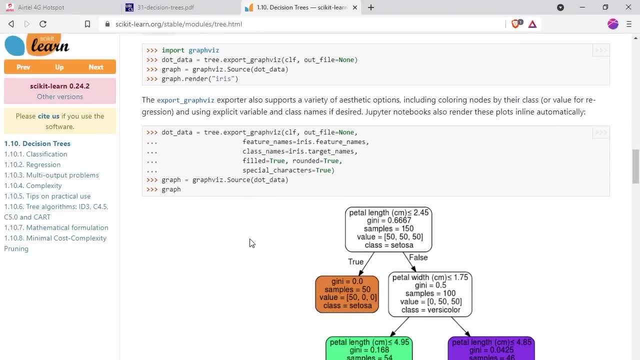 3 to be go as to ask a question, then it will over fit. then it will over fit. so So what do you do? You either stopped at certain depth. you either stop your decision tree at a certain depth to make it more robust, to make it more robust, or you prune your decision tree by removing 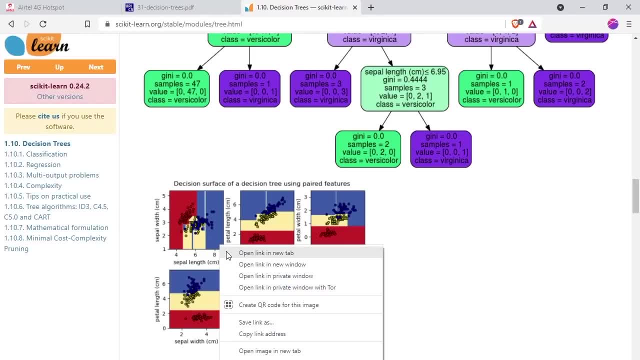 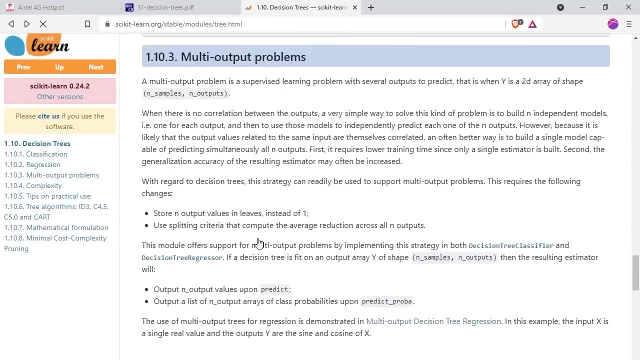 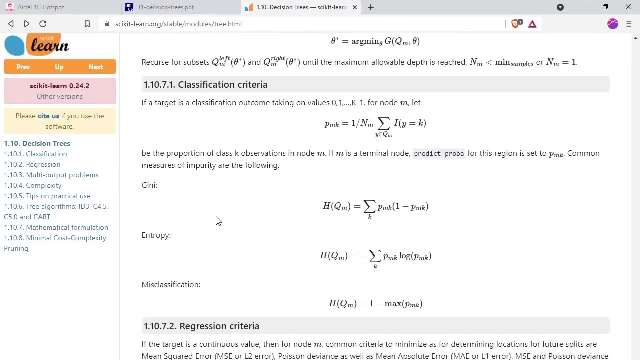 some, some branches from here, Okay, And you can see, the same way that we have seen that we have made the this kind of this kind of decision, boundary decisions are hyperplanes. Okay, great, Let's see some more hopes. I use brave as as my browser, but soon we'll get this, but soon we'll try something, some. 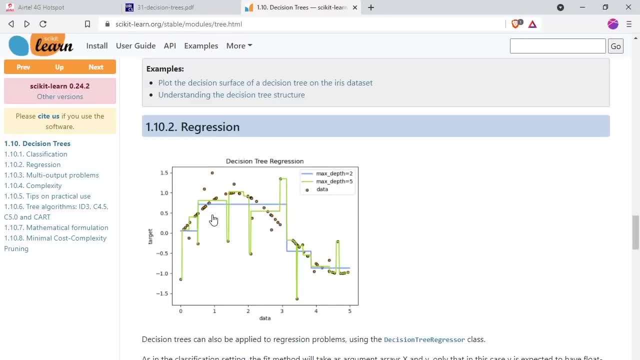 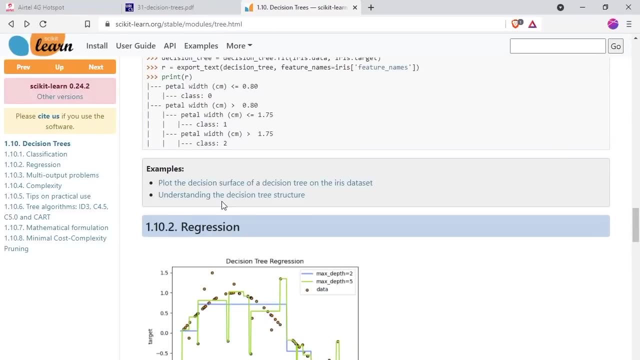 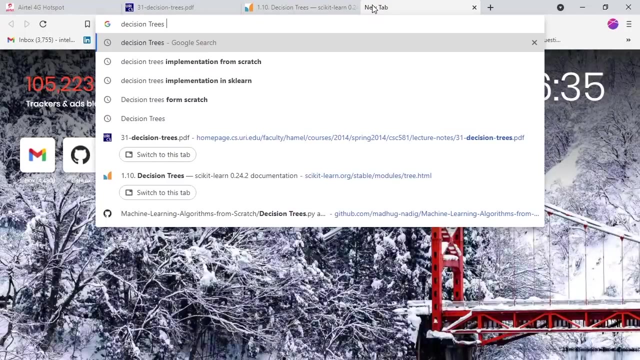 please make sure that you can put your comment below, if you. if I can see, okay and regression, what what we can apply in regression also, So you can see over here that here what, what we do. let me get back to some good pictures: decision trees, regression, regression. but I will soon go to documentation to show you. 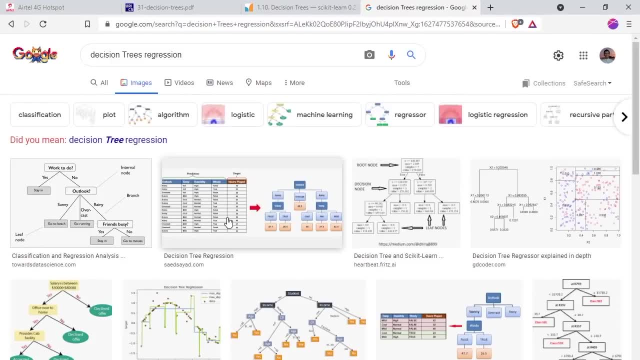 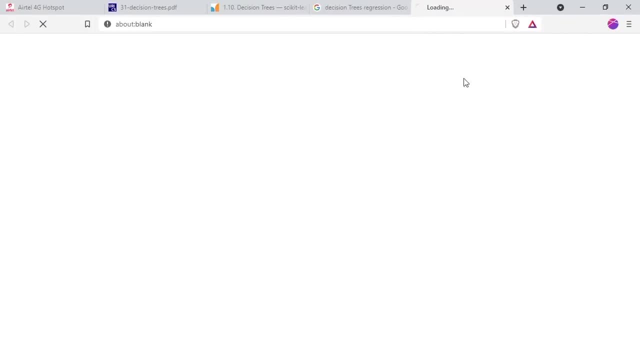 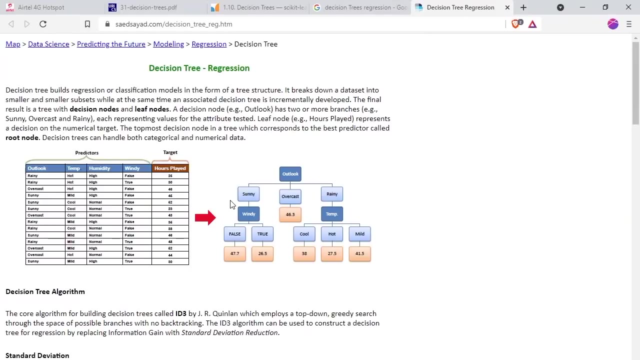 more sophistication. Okay, So here is my decision: tree regression, And let's take an example of this, As you can see from this also. yeah, so here is here. we have a good example. So here you are, predicted here with target variable. okay, 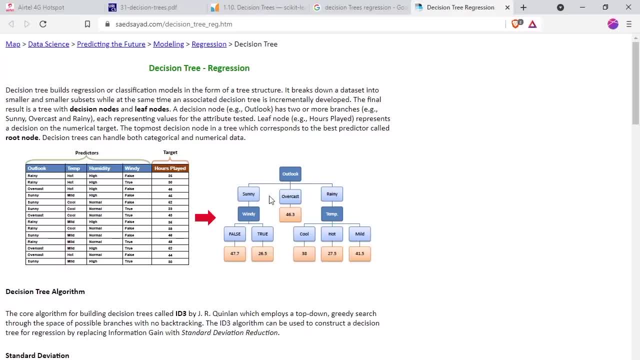 So here you what you have taken. you take an outlook and then you're divided into sunny, overcast and rainy. and sunny needs for the splitting, but overcast does not okay, so most of the time you average it and then you take a 46.3, Okay, and then you split it again. you. 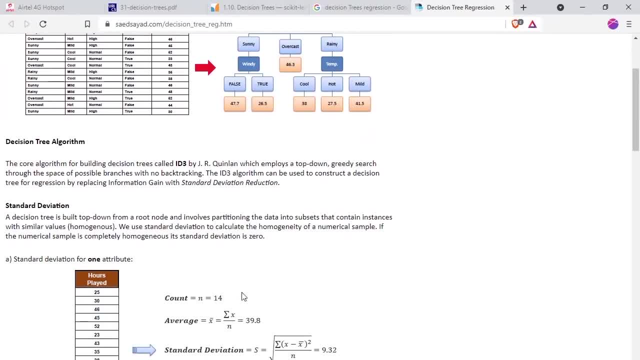 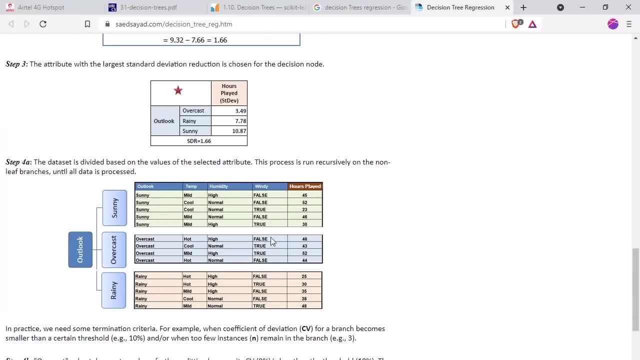 what you? what you do is split it. if you take out the average, again I'm saying: you take out the average, okay, That's what you're doing. And again, if you- if I go further into this, it is very well explained, it is very well. 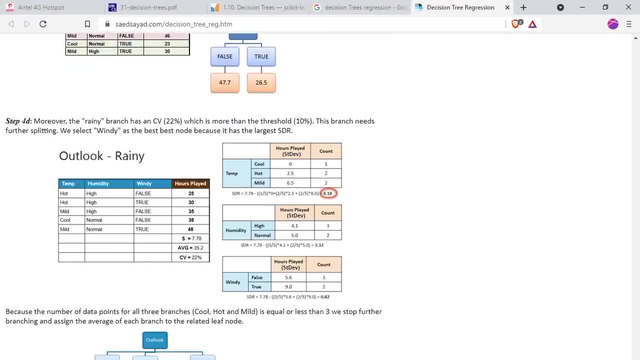 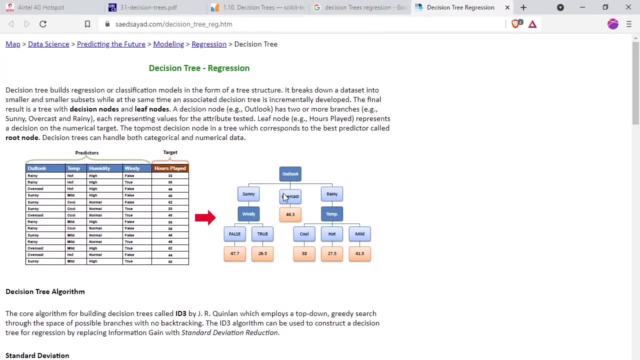 explained. you can go to this: it's very well explained, But yeah, it's only for regression, but it's so much of but what, what we do? we simply again the whole the things are same for attribute selection measure. You, simply, you can. sunny overcast and rainy overcast over over here is we have for this? 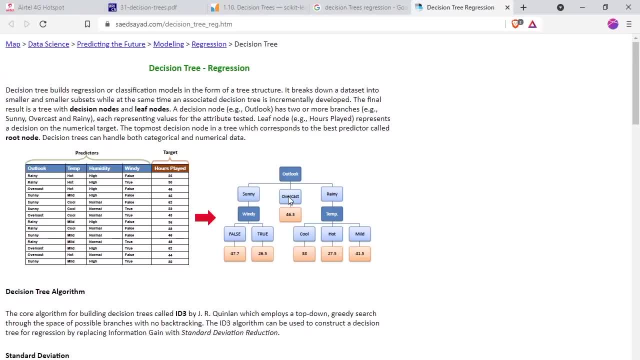 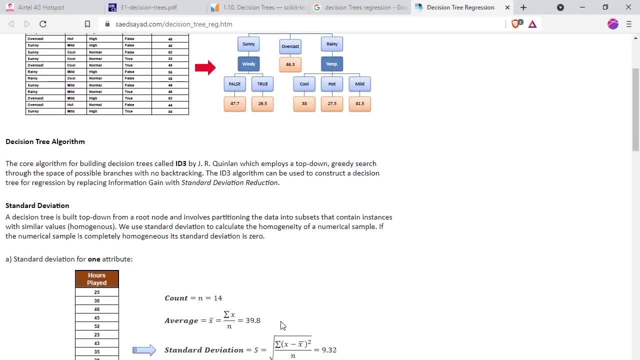 is your leaf, this is your concern. this is a superior that's just considered as a leaf. And then what do you do? you take out the average like this: you take out the average and then you take out a 39.8, 46.3 over your of taking on average. then you split your. 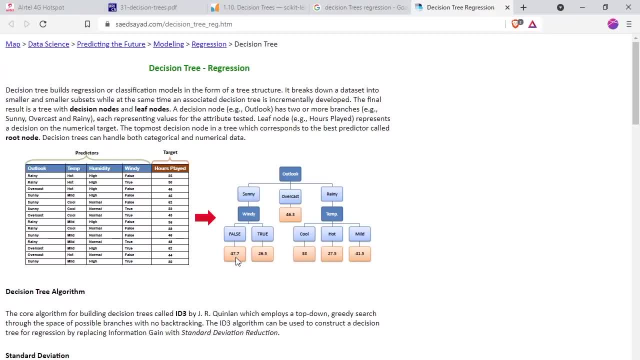 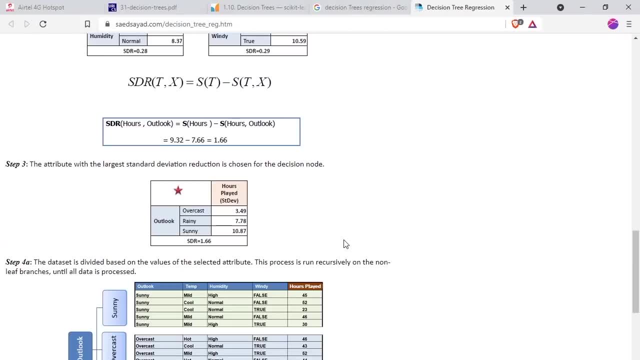 sunny into false or true, then if it is false, then your output output will be 47.7.. And if it is true, then it is 26.5. in the same way you do the regression, okay, So I hope that you understood and you can go again to understand it more detail. 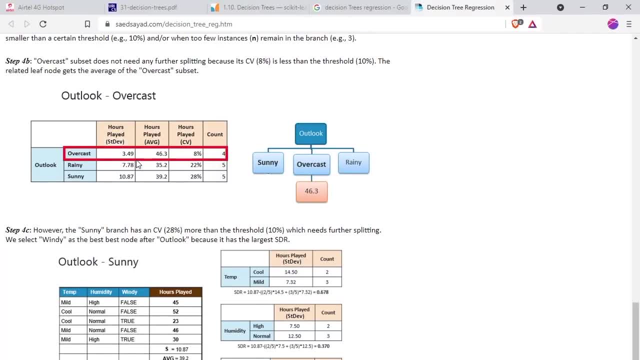 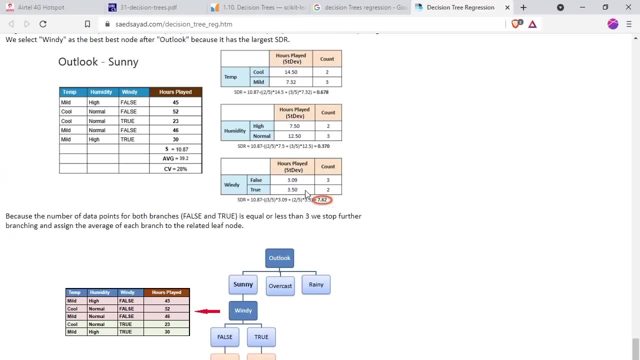 So, So what you, what you do, you take out the hours played and our average standard deviation average and hours played, and then you count it and then you simply do some calculation and that's not too much hard, Okay, Great, So we have seen so far about a decision: trees regression. 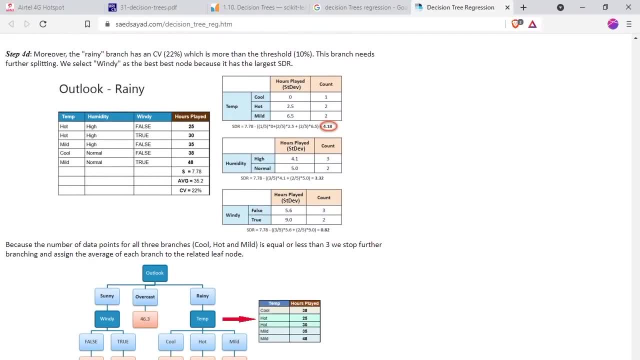 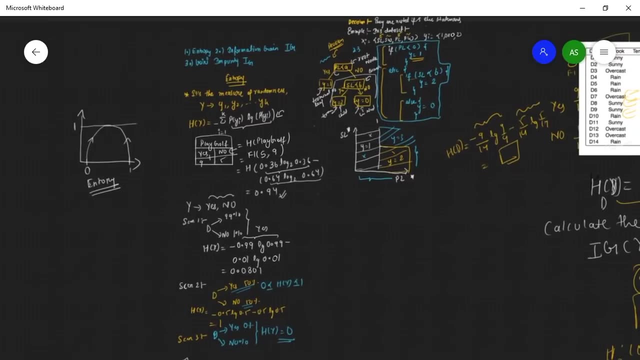 I really hope that you understood this also. Okay, so you can go to this node, this tree. this website said there's sad dotcom decision here, a grass rag. you will be able to understand the, but it's more important to understand attribute selection measure, because people usually confuse us like this, and we have taken 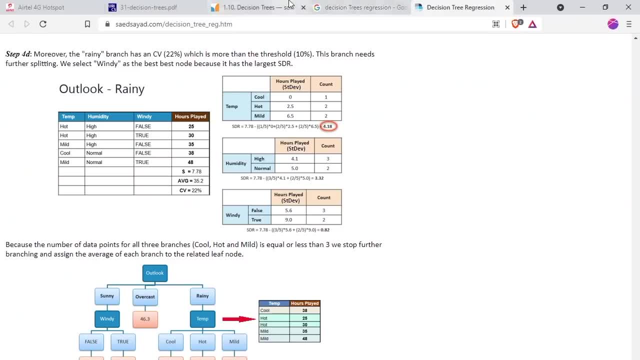 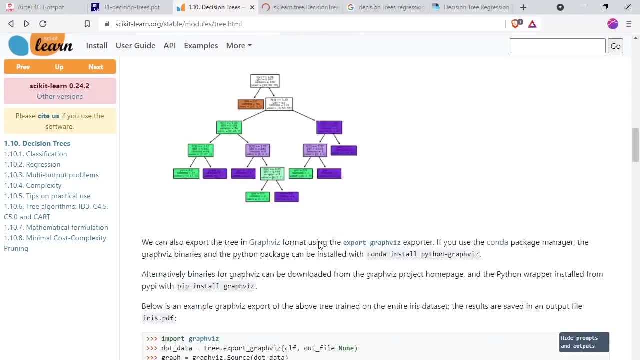 lots of examples for this. Okay, Okay, great. So now, what we will do, we will, I will show you. I will show you some. I will show you the documentation. I will show you the implementation, the implementation for decision tree. I will show you the implementation. 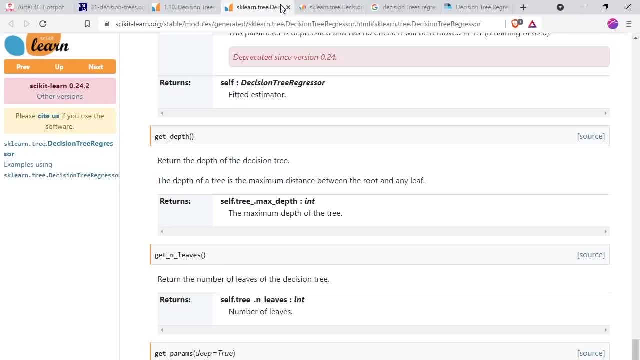 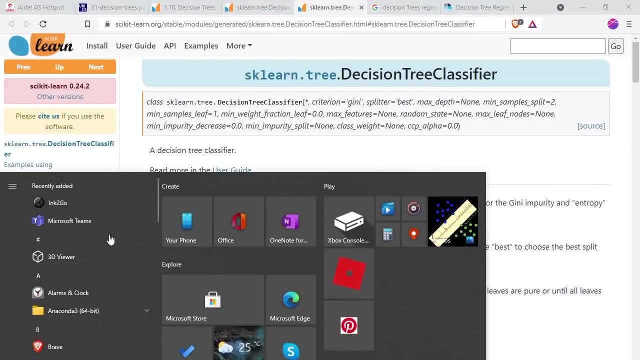 of decision tree regressor and decision tree classifier. Okay, so that you can all, because it's very important to learn from implementation. Okay, so I will explain you in more intuitive way. So let me open my ink to go. I hope that and not I'm just using it. 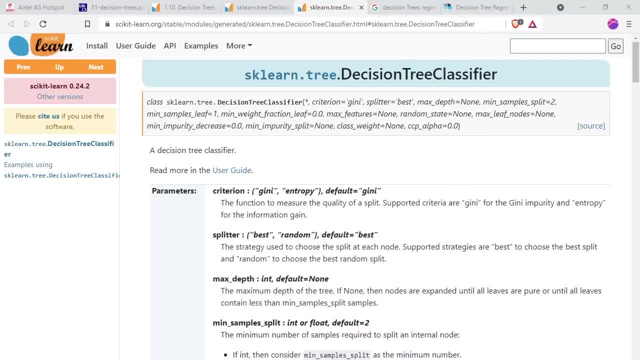 Let me see if this works for not for me or not. Okay, Okay, great, Let me choose this pen. Yeah, So you can go to this website, this tablecom, And here you will be able to find more. you can go to cycle, learnorg and documentation. 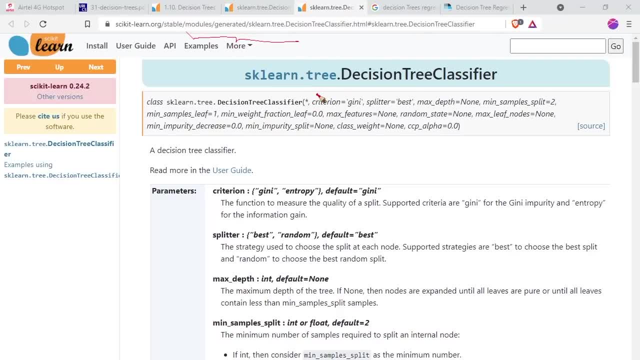 of decision tree classifier. Okay, so here again, it's just the. what is the criteria to choose the attribute? Here we have guinea and here we have entropy. Okay, so you, guinea is a default, you can choose entropy also. okay, the quality of. 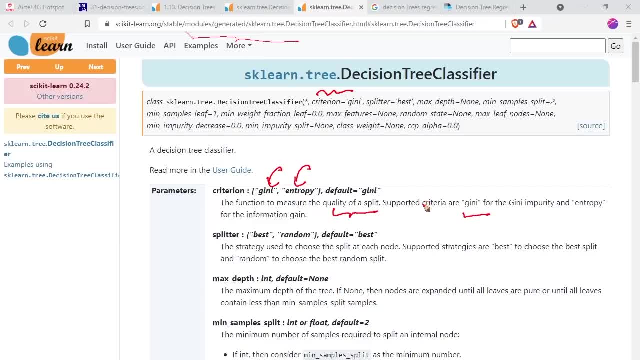 a split. supported criteria is guinea and the entropy is for the info and the for the info. Okay, So you can choose the quality of the information gain After a splitter is splitter means? do you want to choose the best splitter or random splitter? 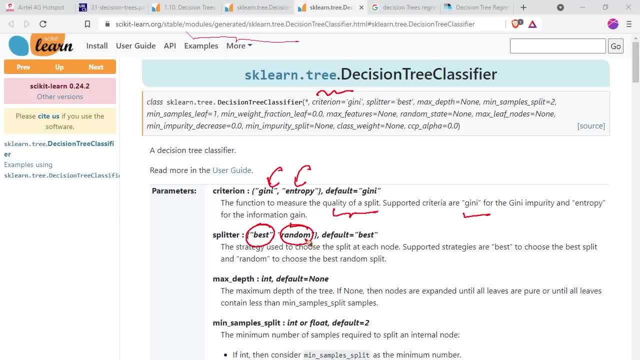 Okay, best means is we choose the best. random means: any ran randomly. okay. max step: this is very important hyper parameter which you can tune it using grid search CV. using grid search CV or a randomized search. randomized search: okay, you can tune it. 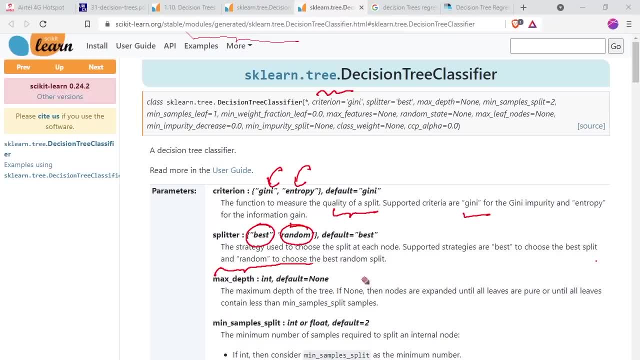 Okay, So that's what you will do And what you do. you just, you just make your decision to do. if you do not make that, it will overfill, or then the new decision will overfill. Okay, so the maximum depth of the tree? okay if it is default as none. okay if you do. 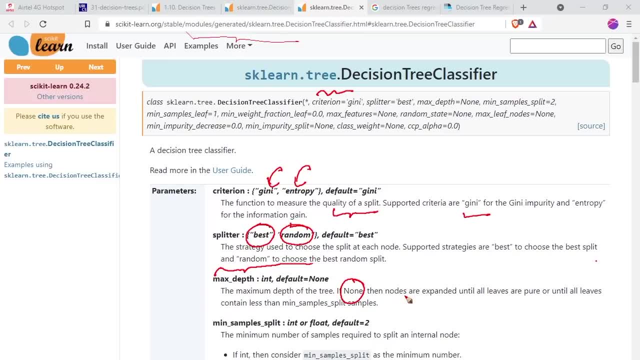 it will learn a lot. it will make a lot of decision bound. it will learn a lot until, unless its leaves are pure, Okay. so it will learn a lot. So that's why it will overfill. So this is a very important hyper parameter. 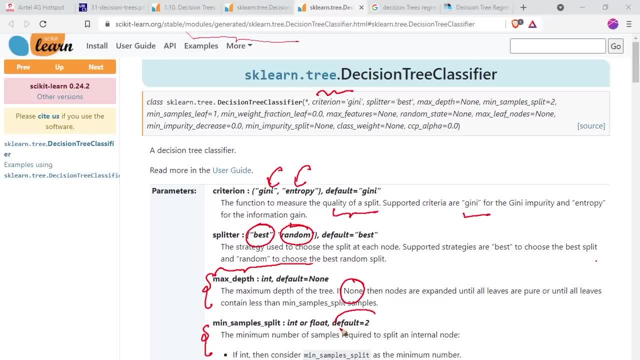 Then again you have a minimum sample. split means here the default is to again, you have to tune it again, you have to tune it. the minimum number of samples required to split an internal node- okay, and internal node is just that know, the minimum number of splits. 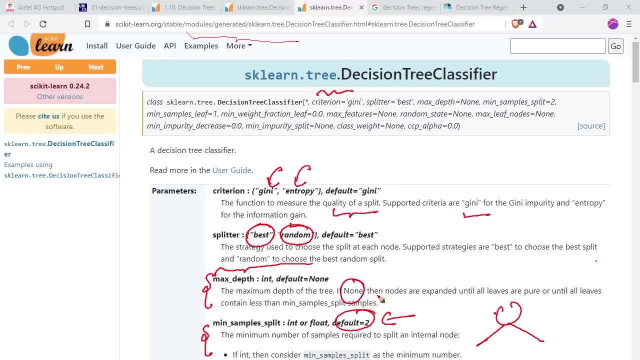 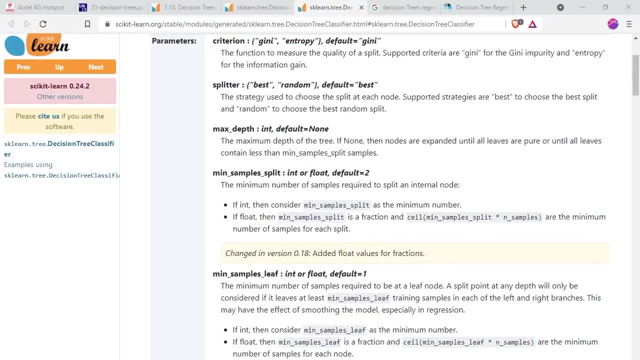 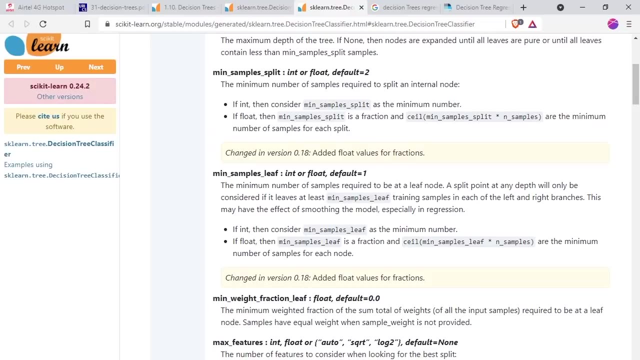 that require. Okay, this is true, but you need to be very cautious into this. Okay, then we have minimum samples split, then we have minimum samples leaf, and then the minimum number of samples required to be at a leaf node. okay, so what is the minimum? 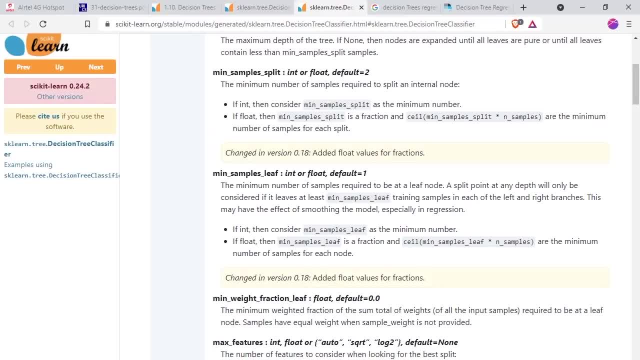 number of samples required to be at leaf node. again, it's one, but you can also tune it. but it's not bad, but it's very good to tune it using rates or CV. then we have a minimum weight fraction leaf. then we have a what is the max. features means the number of features. 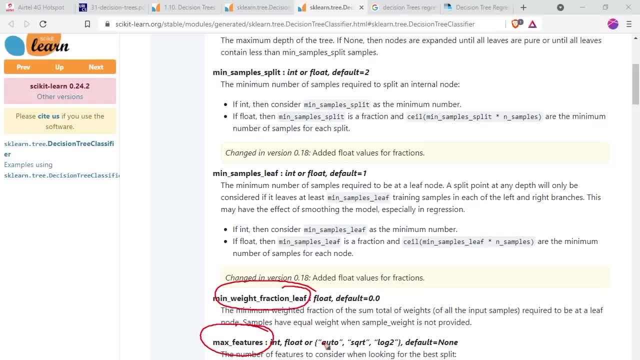 to consider when looking for the best space for a larger number of features. then you can consider as an: the default is none, but you can use this. but it also has some this advantages, okay. okay, then we have a random state. control the randomness of your estimator. 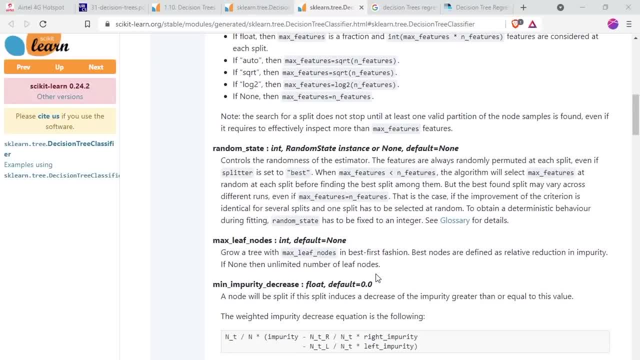 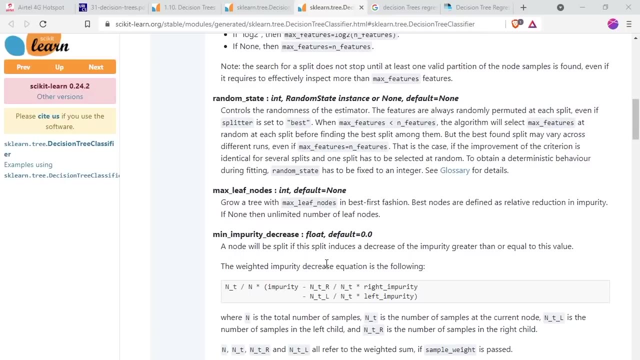 Again, it's a. you can read some more details on random random state max max leaf node, the growth between a best first fashion. it is the default and none. it's just like a max leaf node or the minimum purity degrees. the node will will be split if the split induces. 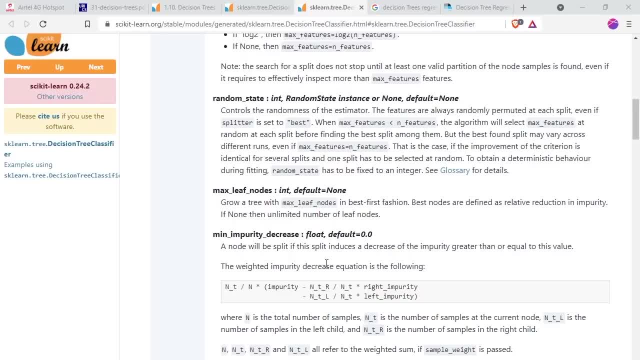 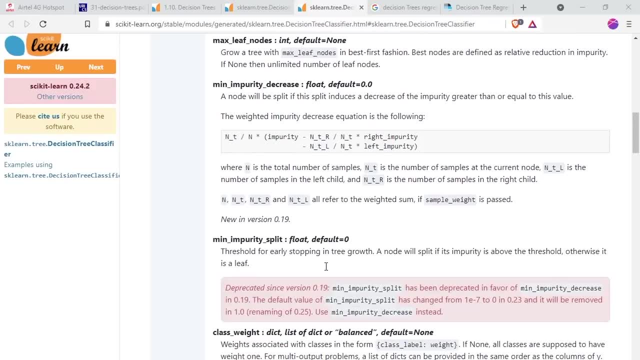 big and uses our degrees for the impurity. Okay, So you can see that the value is basically greater than or equals to this value, but I've not used it. If I say very much right, it's just a limitation that you can make to prevent overfitting. 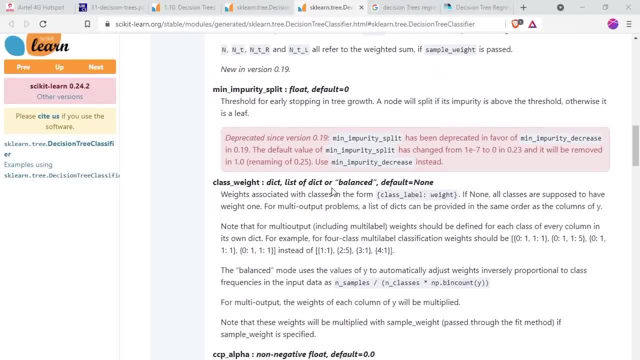 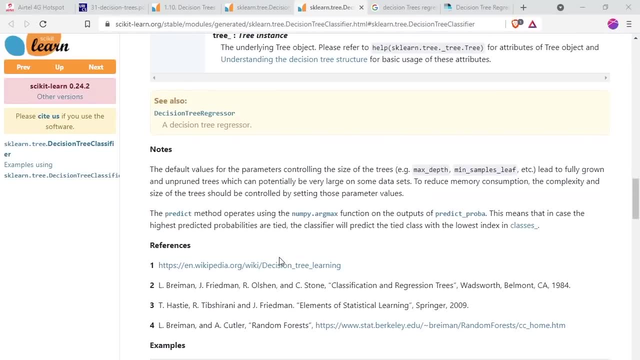 Okay, I think this is deprecated. then you have a class weight. what is the default is none, always. then you have alpha, non negative value. So that that's the basic intuition. Okay, So we had talked about this, and then you can see some examples. 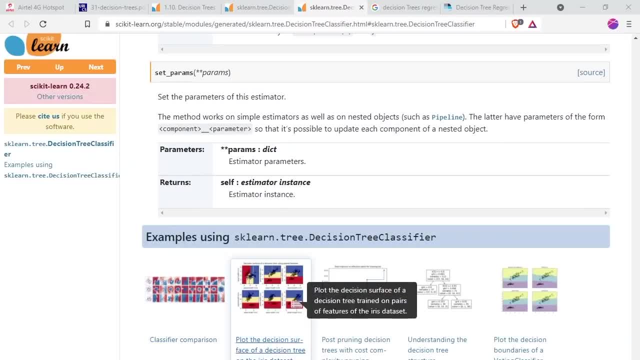 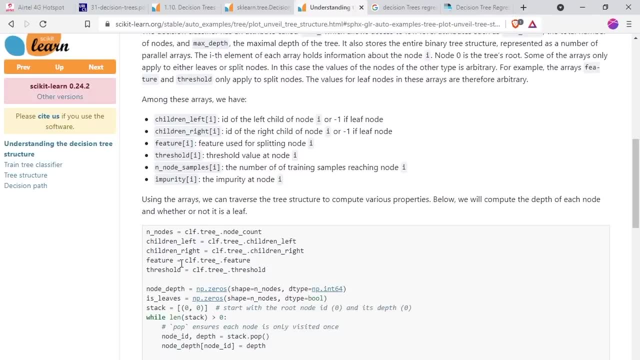 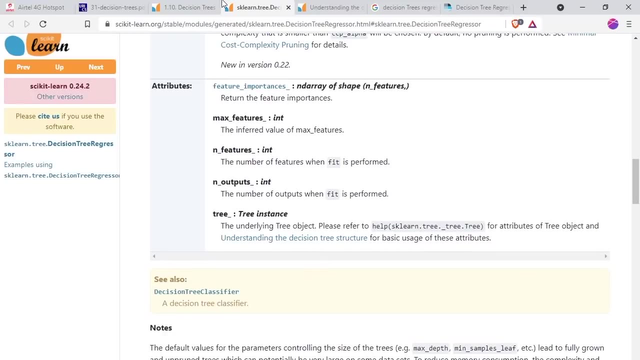 And then there is something called as. let me show you, You can also use this as a understanding decision tree structure. So I will just show you one example of this. okay, So here you can use the graphics tool. here you can use the graphics tool to plot your 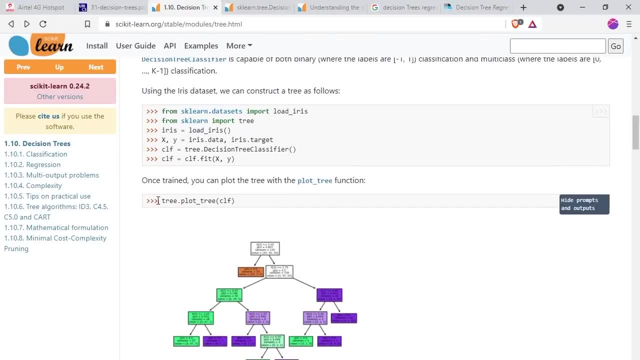 decision tree like this you can. he has used tree dot plot tree. it is plotting the tree like this. okay, because this entry has one more is advantageous. it is easy to interpret, Okay, So that's the basic intuition behind decision tree. 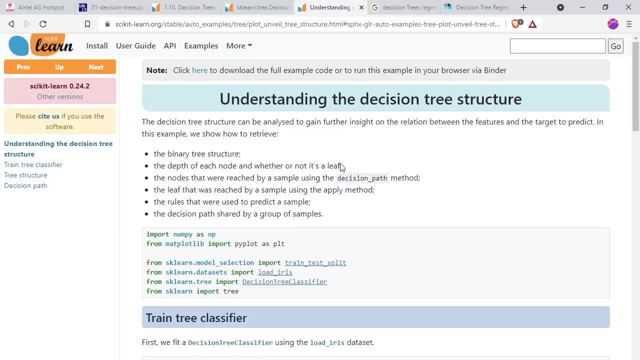 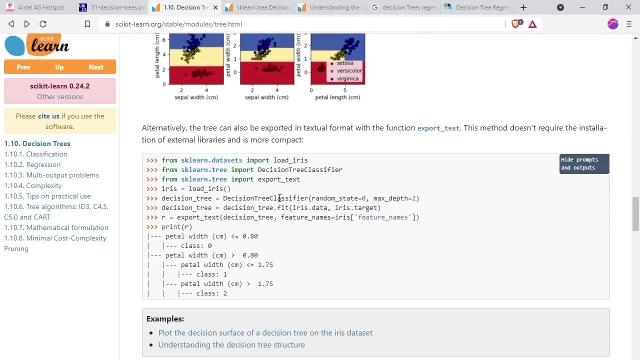 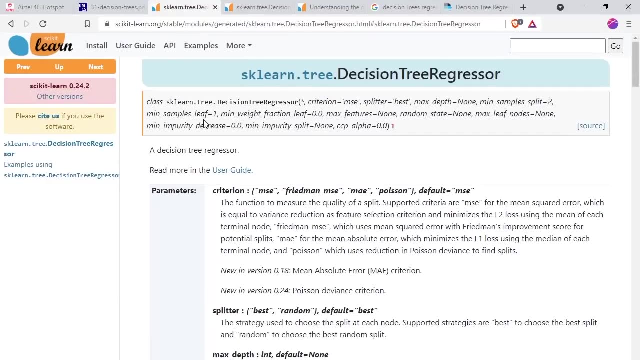 Okay, So let's go to decision tree regression. Okay, So let me see where is the regression. Okay, let me see one more Great: Where is decision tree regression? Here it is Okay. So in decision tree regression can be used for this. this is for regression task also. 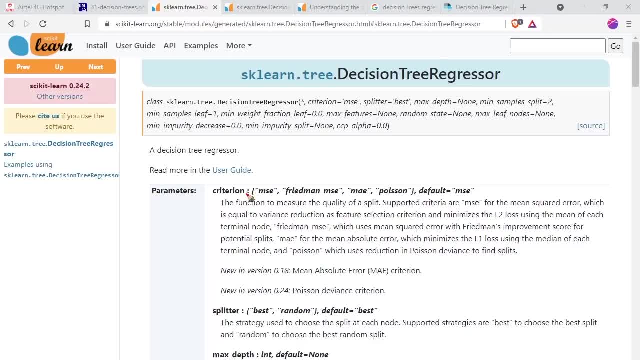 So here you have to choose certain criteria, the function to measure. here we are not using any entropy, here we are using the quality of your split. you can use mean square error means how much it, how much it differs. okay, so it means square error or mean absolute. 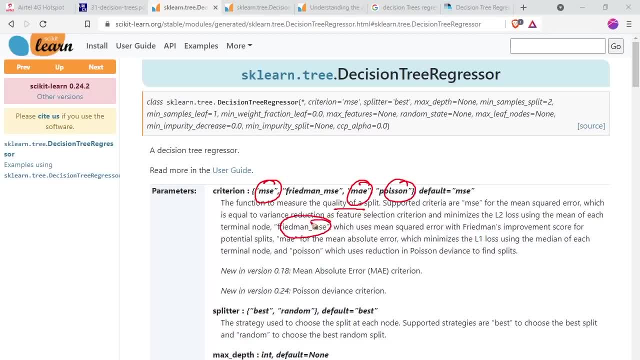 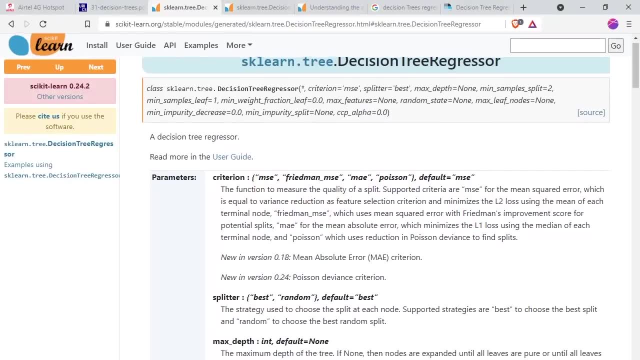 error or poison. So you can see a fine Friedman MSC but most uses MSC or MAE or RMSE. okay, it's a platter Again. it's best again the same thing: max depth, obvious, to control your depth, to prevent. 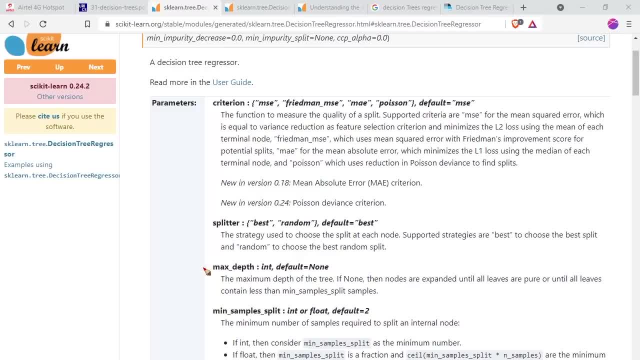 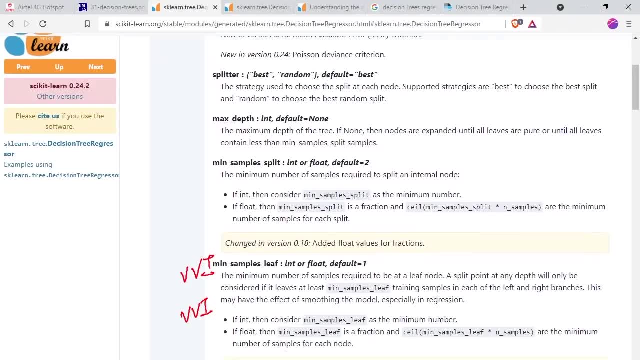 overfilling this important hyper parameter- again I'm saying this- a very, very important- VVI, This is also a very, very important Okay. Then you have minimum sample leaf and then you have the same as we have discussed. okay. 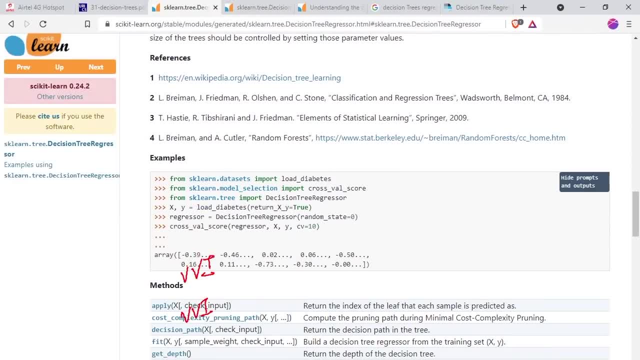 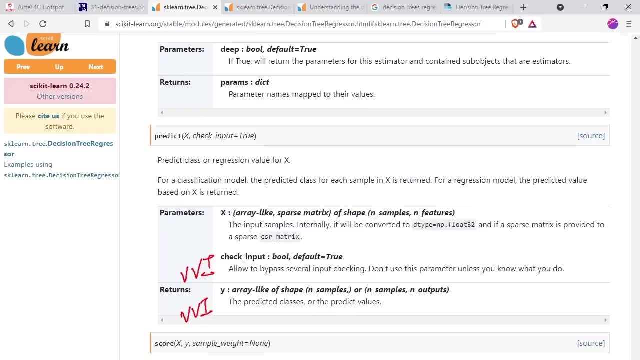 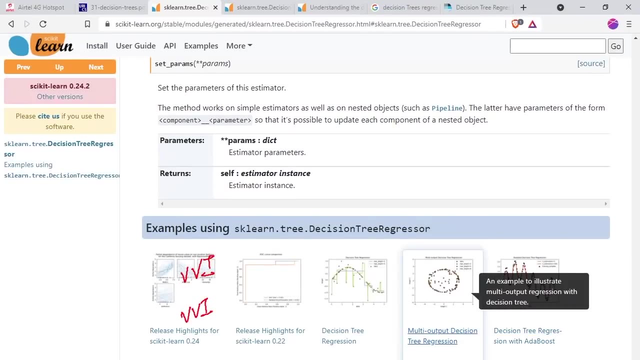 And then you can see some examples of decision tree like this: how we make, and then there are certain methods like plot or etc. Then you have some, some, some examples which you can see from here, And this is usually you can use. we will talk about a double stop for later on. 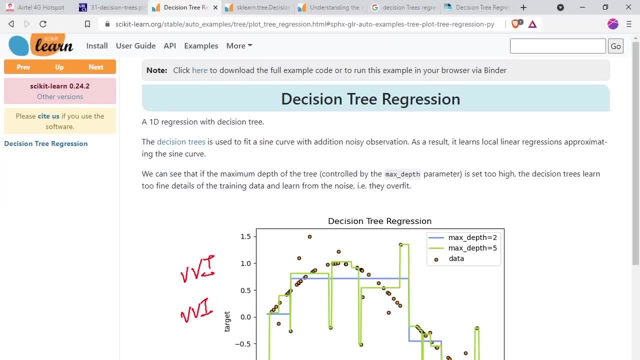 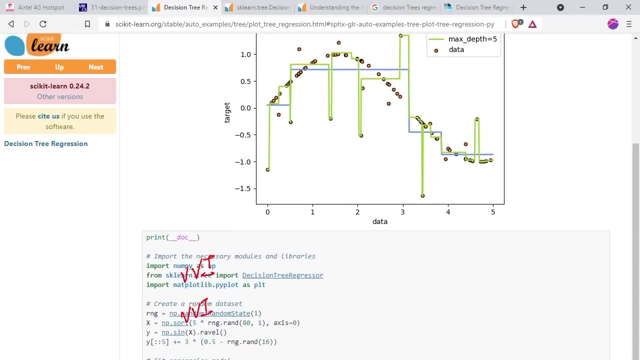 Okay, so you can see some visualization in this. This library and this entry is used to fit this curve with addition, noise observation, And it's just controlled by the depth of that map, by the max depth, And the blue line considers the two and the max depth to be five. should take then it will. 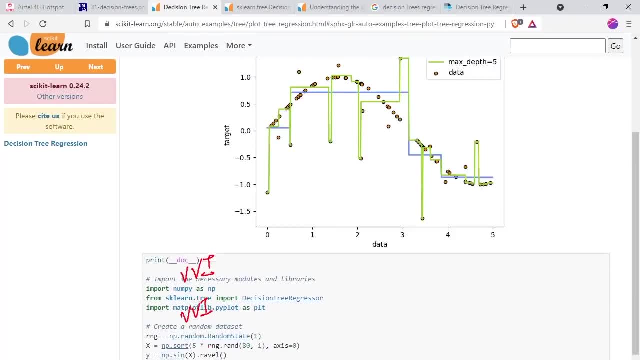 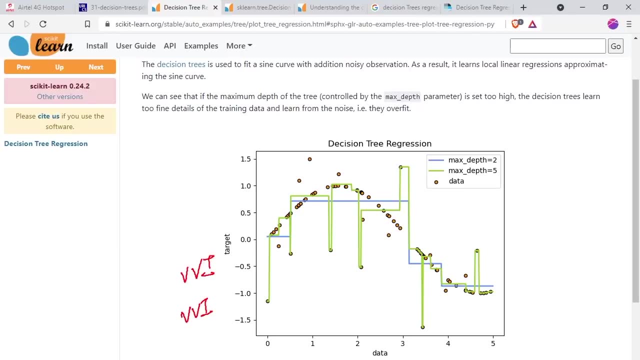 perform very, very well on training set but bad on testing set if you do not control your max depth. Okay so we have talked a lot on decision trees And I really hope that you understood decision tree in that. Okay, so in the next section, the reason why I've taken this too long to make you understand. 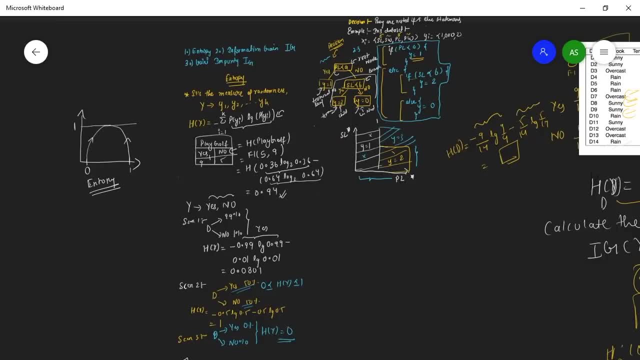 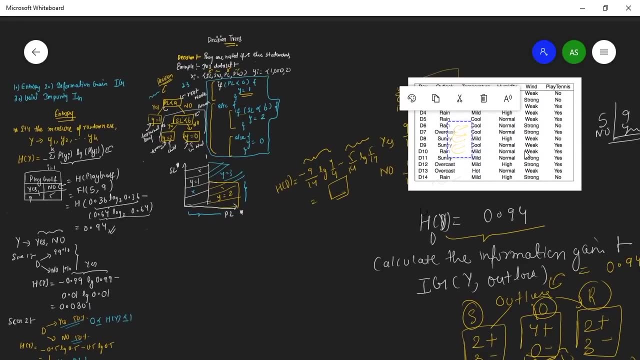 decision tree, because very, very important concept to understand and and I think it's very, very important. Okay, so you can have a look, if you want, on to this notes. okay, But you can. you can ping me on discord or LinkedIn. I will very happy to give you these. 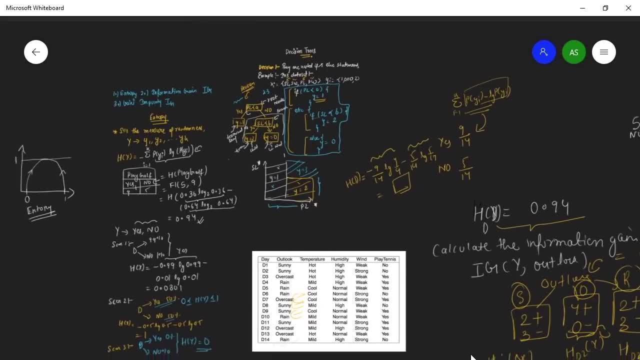 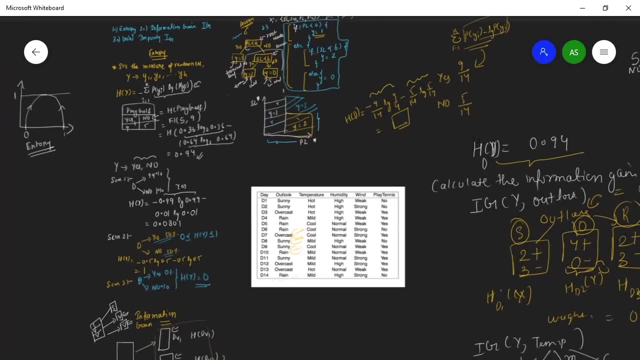 notes. if you're not able to write either, I will recommend you to write these things. Okay, I will, I will just Okay. If you have any questions, you can ask me to make this all wrong. Okay, So that's it for this video, for this section. 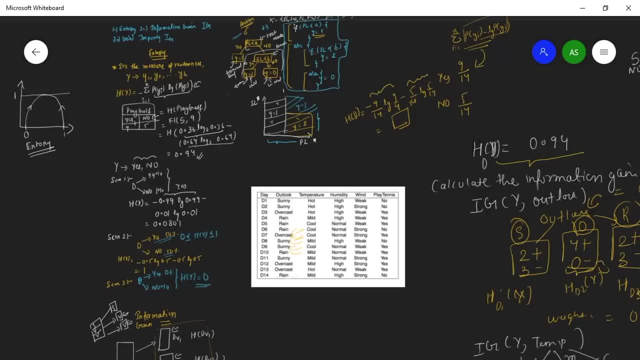 So sorry for this section And I'm my throat is also so much paining. But yeah, that's it for. that's it for this section, And in the next section we will start with ensemble learning And again then we will go to unsupervised learning. then we'll talk a little bit on 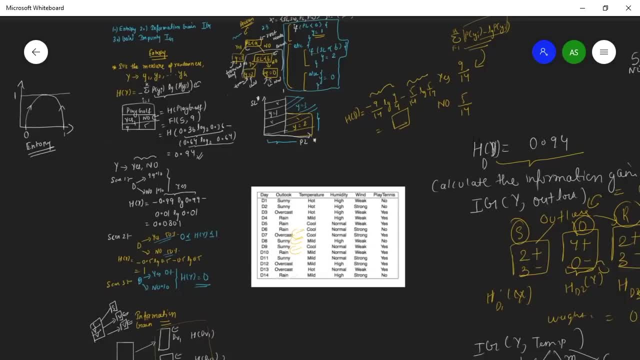 neural networks And then we will end up this course and you will be having enough understanding of machine learning to get started making projects in machine learning- Okay, And getting a job or internship. but you have to a lot of practice, okay, so you can do. 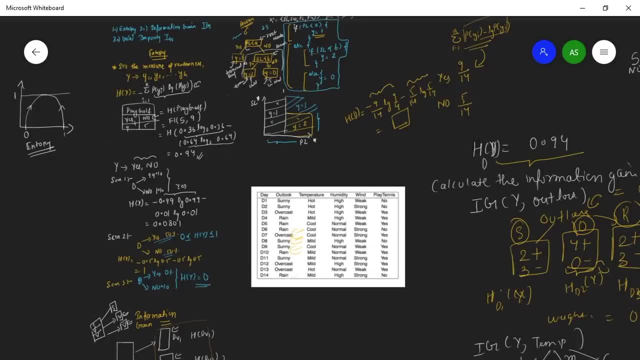 that, Okay, great. So thank you for this seeing this section. And again, if you have any kind of quotient you can ask me to, then you want to be sure to subscribe if you wanted to support this content. Okay, so let's meet at the next section. till then, 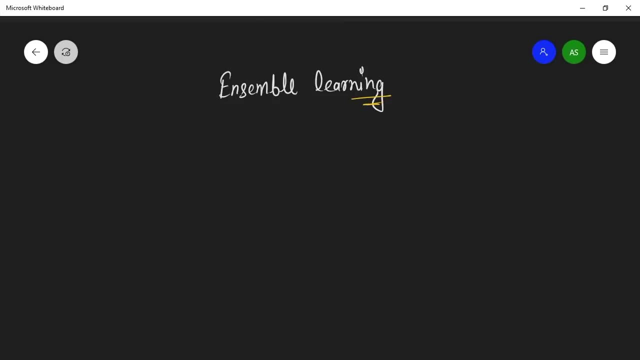 Bye, bye, Okay, so now we'll talk about ensemble learning, one of my favorite topic to teach and to use in my professional experience. So why? why? I think ensemble learning is one of the best for Kaggle competitions. for Kaggle competitions, ensemble learning methods or techniques are most popular. 99% of the Kaggle 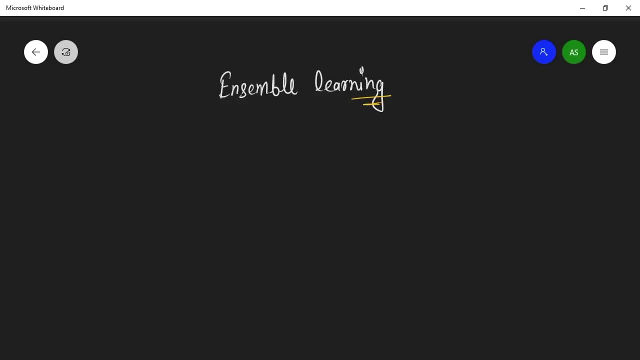 winners uses some kind of ensemble learning techniques. So that's why I think that ensemble learning is a must know technique. It does not involve a lot of mathematics, but it do involves only techniques, concepts and a little bit more math. okay, but in decision tree we involve some mathematics. 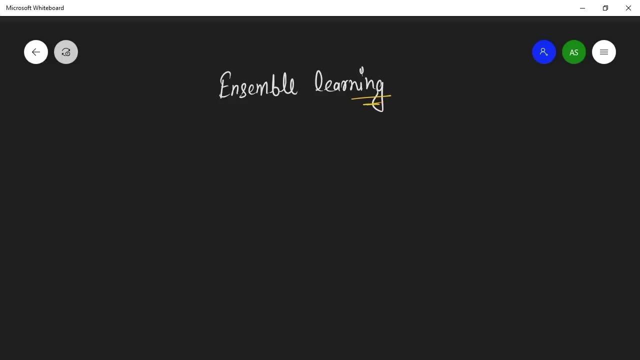 but here we do not involve a lot of mathematics. we require a little bit of mathematics, but there are a lot of techniques and concepts that we need and approaches that a particular Kaggle winners use. Okay, so it's very. we will dip dive in ensemble learning covering the four techniques three: 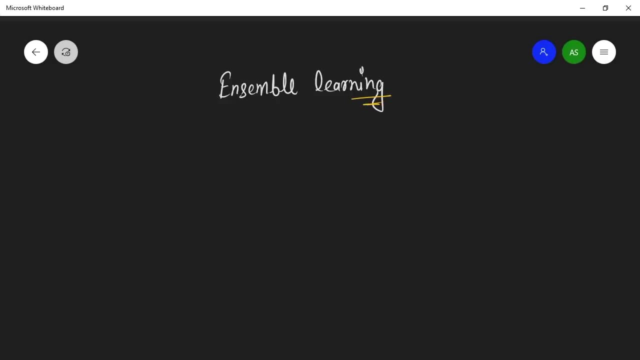 techniques, I think the three techniques of ensemble learning. The first technique will be a bagging, which we'll talk about- not it will will be in a separate section, subsections. Okay, so this is our main section And in the separate subsection we will talk about bagging. then we will talk about boosting. 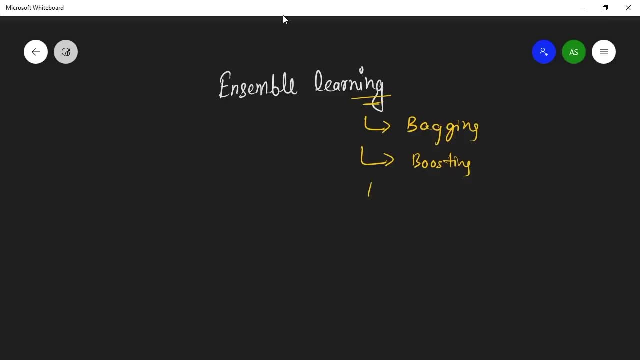 then we will talk about stacking. Okay, so these are the three techniques that we will talk about in ensemble learning And also we will see the implementation of each one of them And it and I will also show you some of the Kaggle competition winners approach, or we. 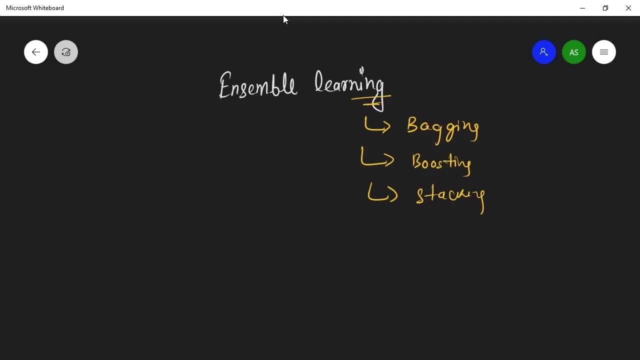 will make one model, seeing the changes for changes they bring into your system, how the your model accuracy increases. Okay, Okay, so great. But before that, let's a little bit, let me just forget about them in ensemble learning. let me recall you some concept, which is high variance concept. okay, 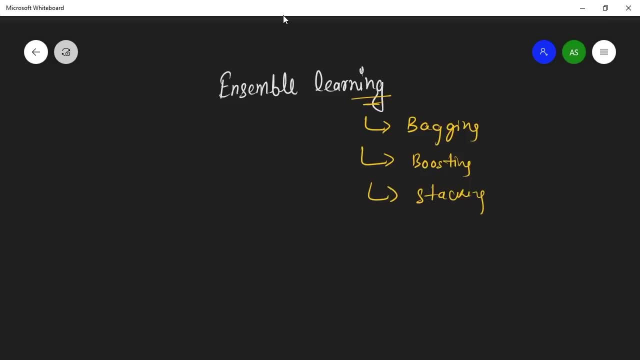 So high variance and high bias concepts, so it it should make sense to you. So let's recall: in high variance, we have overfitting model, we have our overfitting model, if I'm, if I'm correct. and high variance, we have our overfitting model. and in high 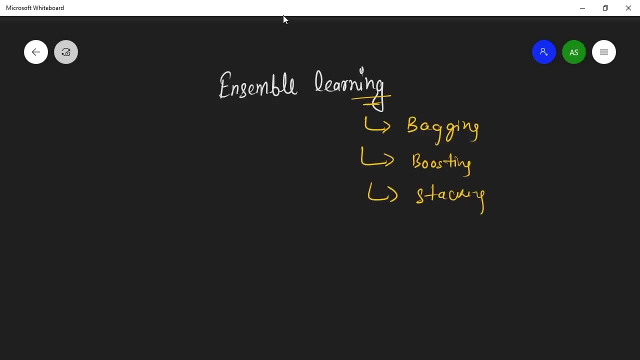 bias, we have our underfitting model, okay. So our models should be low bias and low variance, low variance model. If you have a high variance, if you have a high variance, then you have, then your model is overfitting. 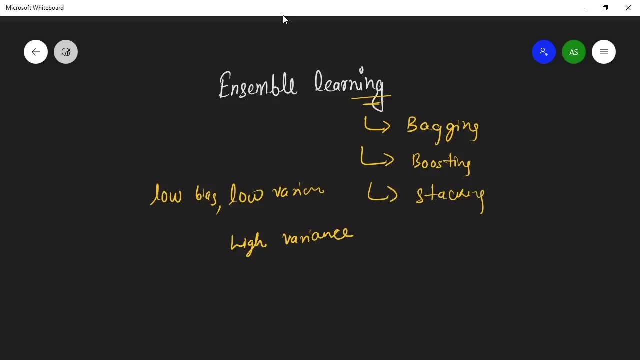 If you have a high bias, then your model is underfitting, And that's that's what the regulation that that that we need for this ensemble learning, just to make sure that that we are on the same path. Okay, Okay. So let's start with an, a simple example of, of a small example. 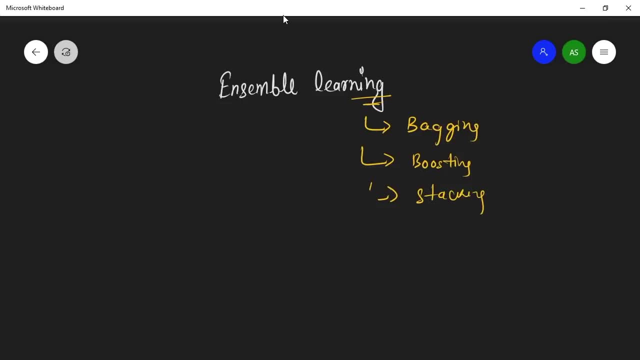 Okay. Okay, Let's say we have played some quiz. Okay, If you have played some quiz, let's. let's take an example that we have played some quiz of, maybe in Kahoot or any any kind of quiz, or if you're in competition or played some. 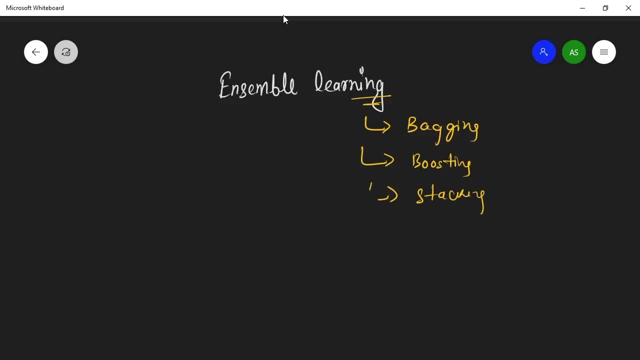 quiz. So it's a maximum percent, a maximum percentage that the- let's take an example that we have some question. let's, we have some question, we have some question here and we have some option which is A, B and C. Okay, so let's, let's take an example that the particular 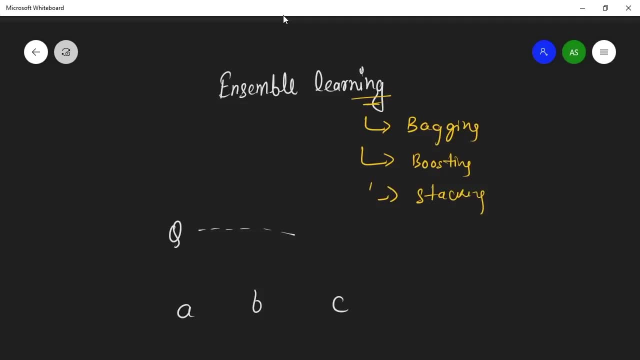 that the Majority. let's take an example: A is the correct answer. So it is. it is very obvious that the majority of the students will go with A, and if the majority is on A, then it's likely to be A be the correct answer, and it's actually the 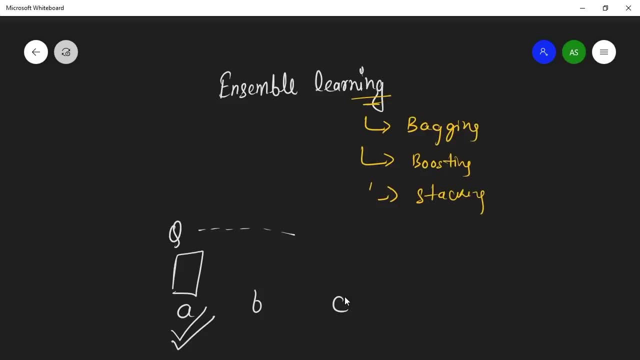 correct answer, Okay. So it's like: whatever the majority will say, we will go with that, Okay. Here the majority is saying A and in this case, A is the correct answer and if you think about the majority, Majority is more accurate than one. 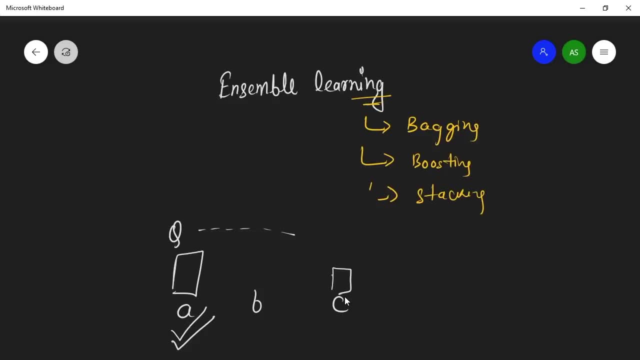 Majority is more accurate than one and in some exceptional conditions that can be different, but in 99%, the majority will win. Okay, Majority will win, if you have seen some quiz. Okay, So if you see that the option has got the highest majority and who are also into that? 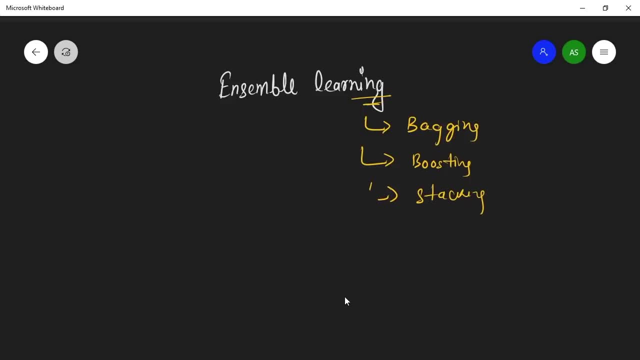 then you can think that is a correct answer. So, in the same way, ensemble learning works. Ensemble Ensemble learning is an ensemble of models. is an ensemble of models, Okay? So let's take one more example to get more feel. Let's take an example that some election is happening. 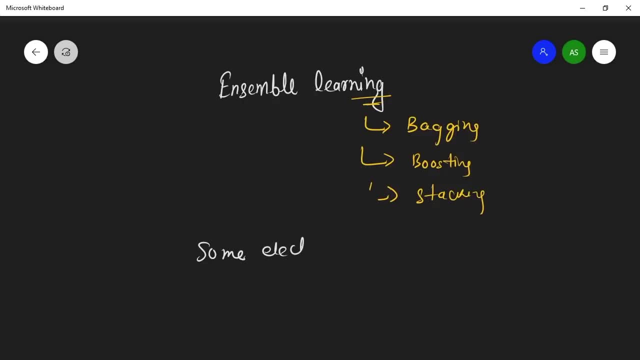 Some election is happening, Some election is happening and in that election, in that election, let's take an example- that why we do not take only one person vote and select any prime minister or president, Why we take the majority, The majority of votes, which will go on to that party that will win. 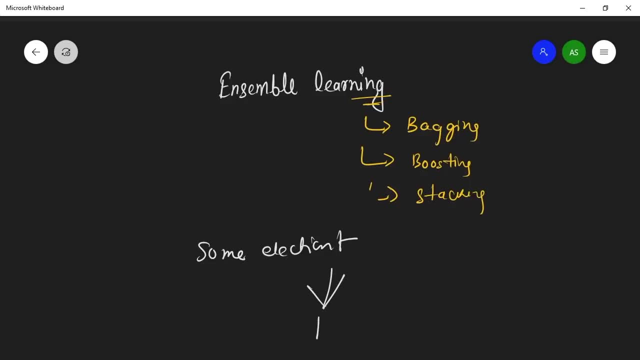 Okay, So the majority will make a right decision. Okay, Will make a right decision in most cases. Okay, So that's what the ensemble learning also says. Ensemble learning has an ensemble of models, So let me tell you what we do in ensemble learning. 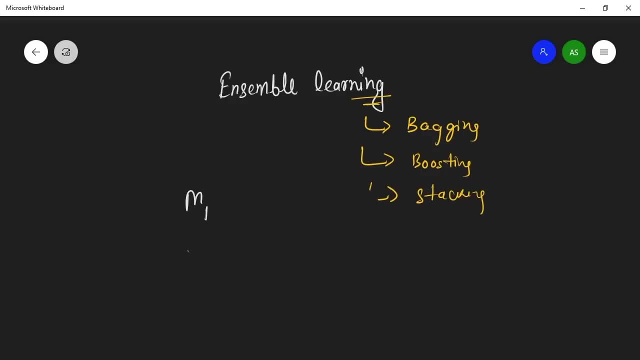 We have a model one, model two, model three, We have a model four, We have a model five, We have a model six, We have a model seven, We have a model eight, We have a model seven, We have a model nine. 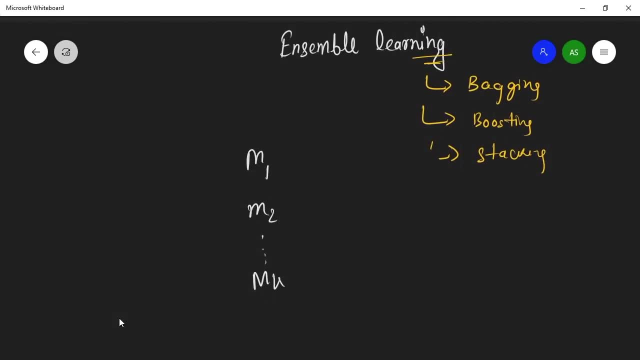 So we have the model number six, nine and 12, all the way down to the model K. Okay, So let me make you make this, make this visible here. Okay, so you have these kind of models and you train your model, you train your model. 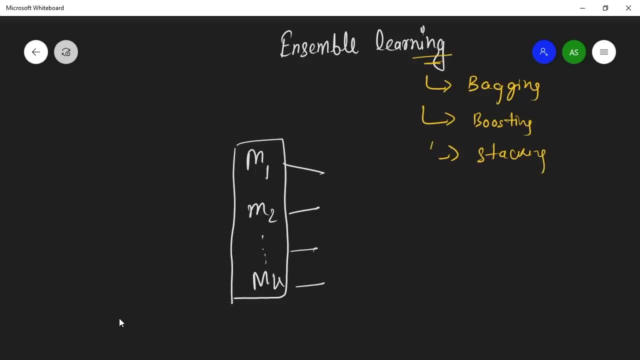 you train your model onto your data. okay, You train your model onto your data and you can you take predictions from each of the model. So let's take an example that you are trained. You are making a diabetes prediction system. diabetes prediction system. 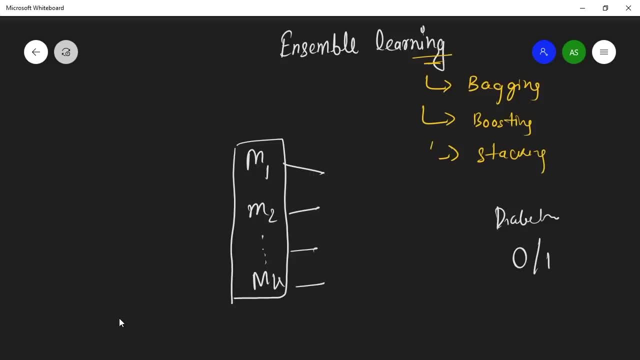 diabetes or one. okay, so let's take an example that model number one says it's it's a zero, model number two says it's a zero, model number three says it's a zero, model number four says it's a one and model number five says it's zero. so the 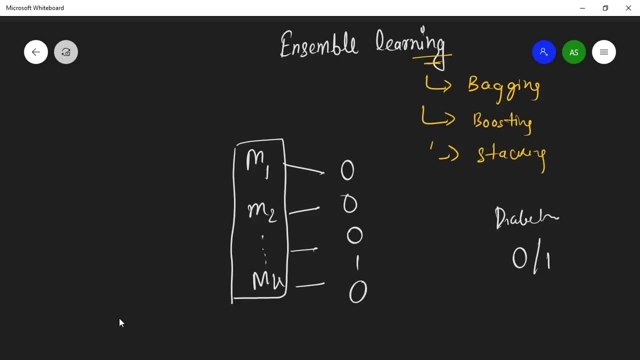 then what? what? we have a one more model, a big model, which which, what it will do? it will check the majority of votes and here the majority is zero and only one has given one and the majority of zero. so we will give our prediction as a zero. okay, so you will see how it is trained later on. 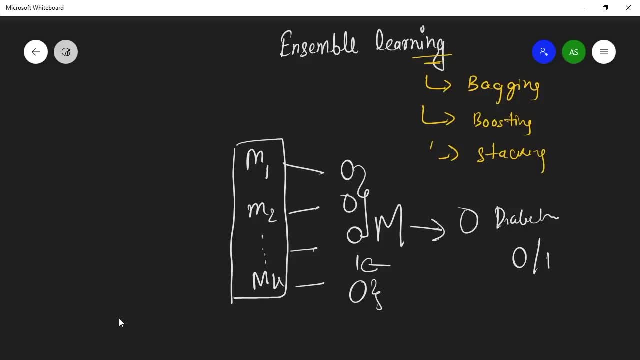 but here what the actual thing is, what is happening. we train our model and each model is giving predictions and in each predictions we are taking into classification, we are taking in plus classification. we're taking majority of votes means majority means m1 is saying is zero and two is saying zero. the 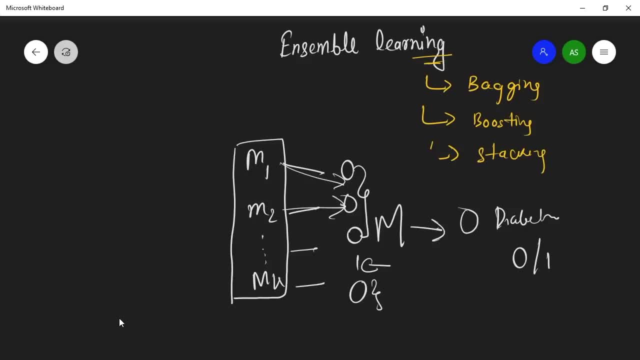 frequency of zero is more than the frequency of one, okay, so that's why our final model says it's zero and it is more than zero. so that's why our final model says it's zero and the more it is, which is y hat is equals to zero, okay, and is more. 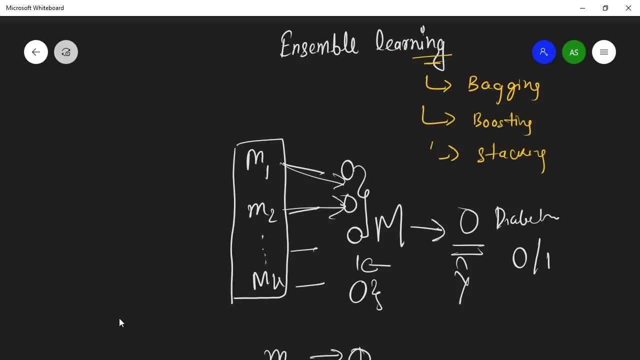 it will be. it will be high chance that if one model predicts it, one model predicts it's a 1 or 0 and the insane sample of the model the biggest is 0, then they are more accurate rather than this. okay, so that's the. that's the basic. 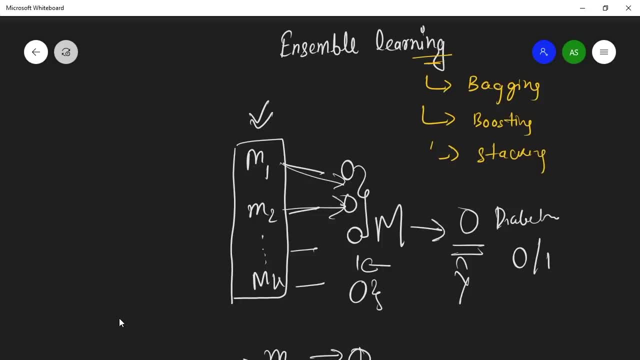 overview of ensemble learning. and you may think, yeah, use in classification, we regression. What about regression? What about regression problems? In regression problems, what we do, we take out the mean or a median of output from each model. So let's take an example that your model M1 given some prediction, which is: 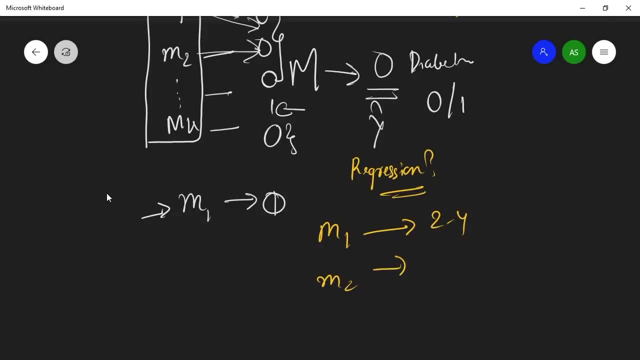 regression value 2.4, model 2 given 2.6, model 3 given 2.5.. So, what you do, the final prediction will be the average of these outputs: The average or mean or a median of these outputs. So that's what that's how we do in regression. 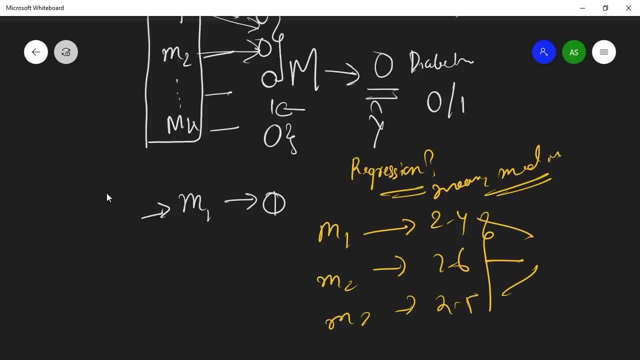 We do not take the majority, we take the mean or a median of the output from the base models and these are called the base models over here. So these are called the base models in ensemble learning. So don't be confused. what is base model? 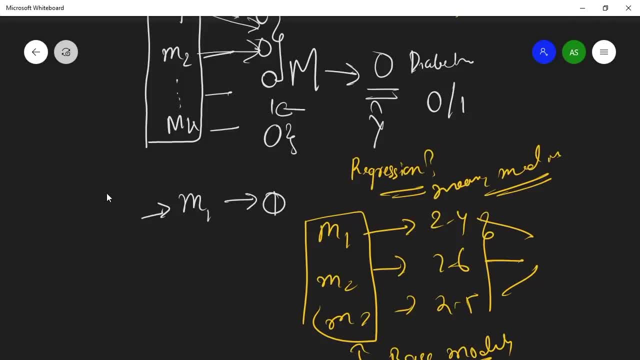 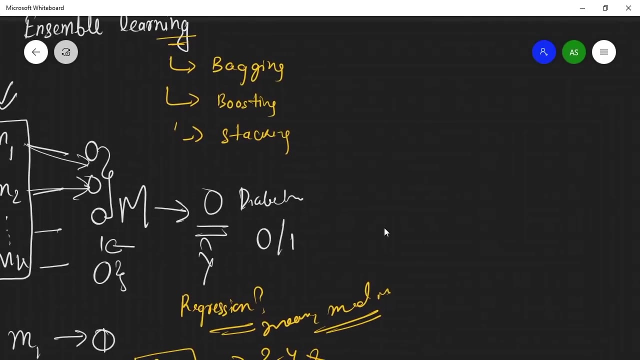 Base models are the ensemble of models that are being trained And okay, so that's, that's the basic intuition behind our ensemble learning and I really hope that you understood ensemble learning and that. Okay, so just want to make sure that, what, how we train, what are the some of the techniques used in this, used in? 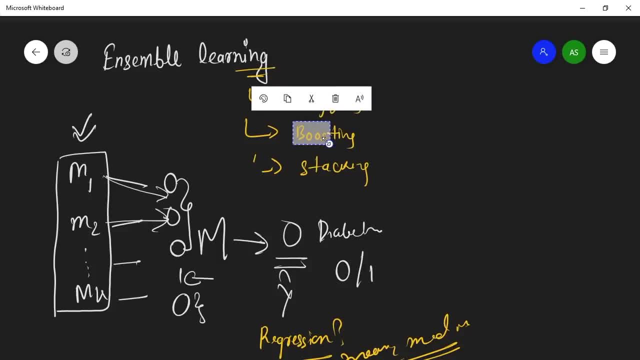 bagging, what means? what are the techniques used in ensemble learning? So we have a techniques like bagging, Then we have a boosting, then you have a stacking. okay, These are, and one more Which is cascading, which is which which you can learn, Which is not yet in. 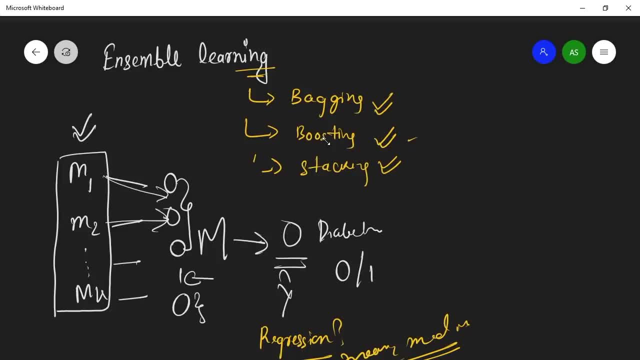 the industry yet, But in the end this is just cascading. In bagging we will see algorithm of which is a random forest, which is, which is something called a random forest- okay, Which is just an example of a decision trees. and then in boosting, we will see one algorithm which is a random forest, which is something called a random forest- okay, and it is just an ensemble of decision three. and then in boosting, we will see an algorithm talking. 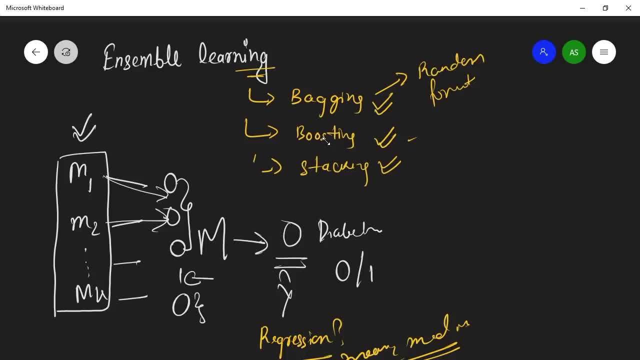 will more probably focus on, we will in boosting, will more probably focus on gradient boosting, will more probably focus on gradient boosting and we will focus on adaptive boosting, which is just a advanced of version of gradient boosting. will focus on adaptive boosting. then we will see one gaggle winner. 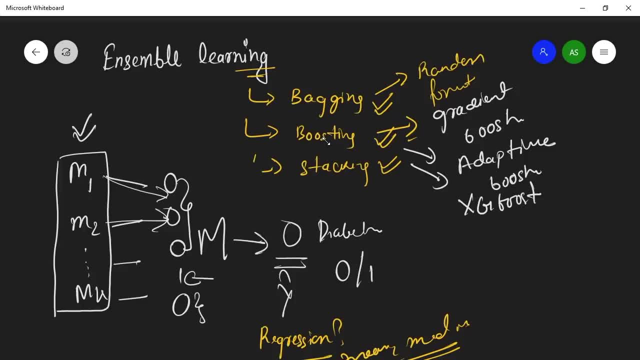 which is XG boost. okay, so we will see these algorithms or these techniques in this boosting. then in stacking we will see ML, external library, how we do the stacking and what's the intuitive understanding. and you can see there's no any kind of math, this is only the concepts. okay, so that's how, that's what. 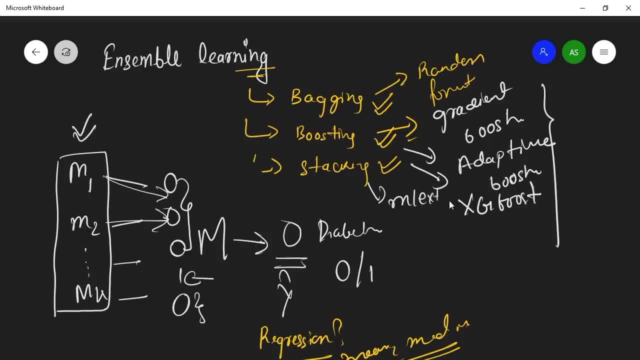 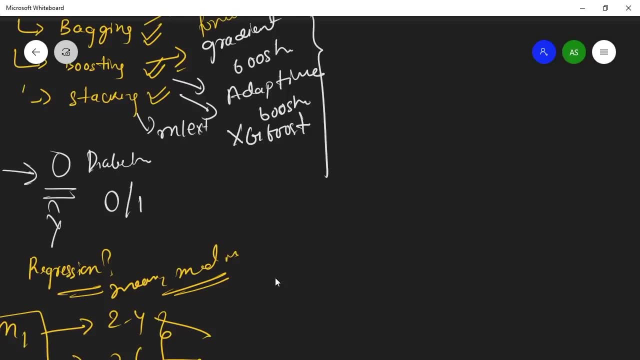 we are going to see and the study motivation for this or ensemble learning. why do we study? ensemble learning has a great reason behind them. the reason being why do we study? this is the great cushion to us whenever you do any kind of thing. why let me use this good color? why do we study? I think that is not. 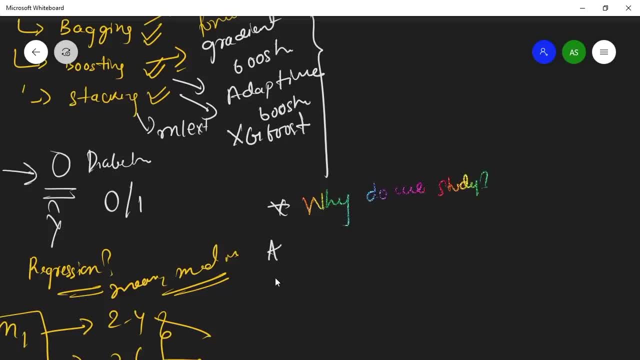 visible in most of the cases. let me stick to light. okay. so why do we study? I never study this ensemble learning. the reason being is most of the Kaggle competitions, most of the Kaggle competition winners, most of the Kaggle competition winners. competition winners uses some kind of ensemble. 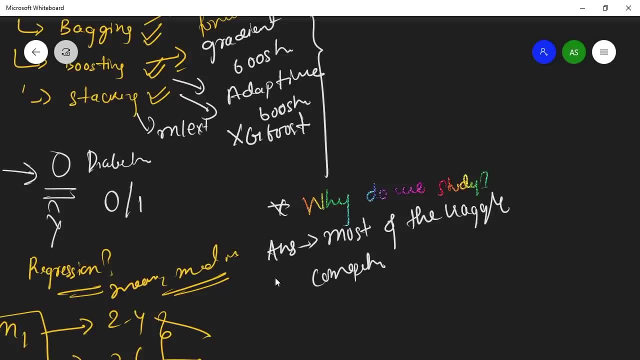 learning. either they use bagging, either they use boosting, either they use stacking, either they use cascading. they use some kind of inseitions, learning techniques. if it is a machine learning problem, if it is a machine learning problem, ML problem, okay. okay, just think that machine learning has also power, okay. 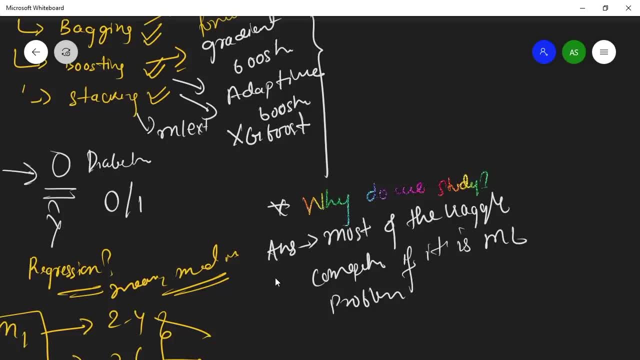 so, but there is a difference. in an Internet companies like Amazon and Google, they also uses these algorithms- XGBoost, Adaboost, Gradient Boosting- that we have a random forest in their own products of in-front production. okay, so Quora uses random forest. 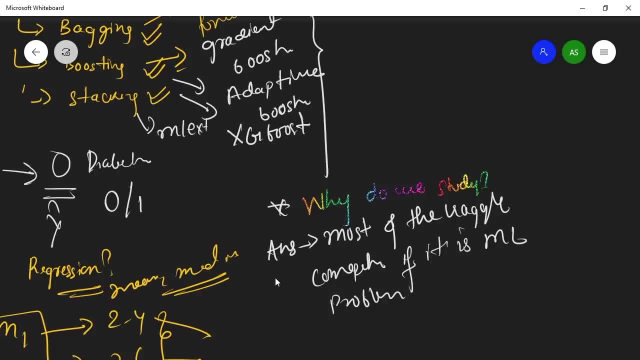 to for quotient matching. okay, so they also use machine learning, these kind of algorithms, and these are very, very powerful algorithms, very powerful algorithms which is often used in industrial, so which is often used in many kind of Kaggle competitions and around 99%. 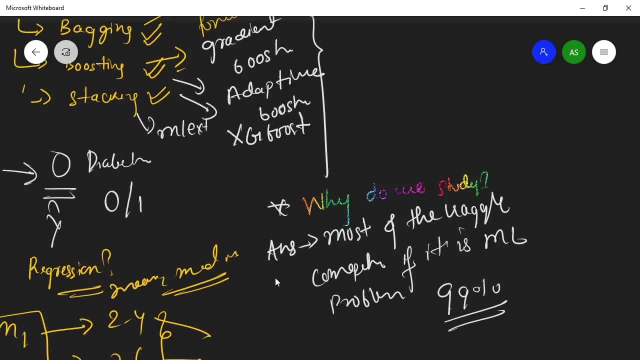 of the Kaggle competition winners are uses this kind of any kind of ensemble learning either. if it is a machine learning problem in deep learning problem, you obviously go with. if it is an image problem, you will go with CNN. if it is text text, you will. 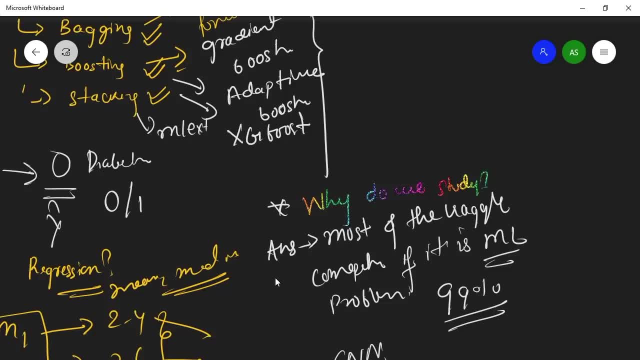 go with some word embeddings and then you can use any of the techniques and you can use RNN, so it depends. so you can use any of the techniques if you want. but in most of the Kaggle competition in the past, 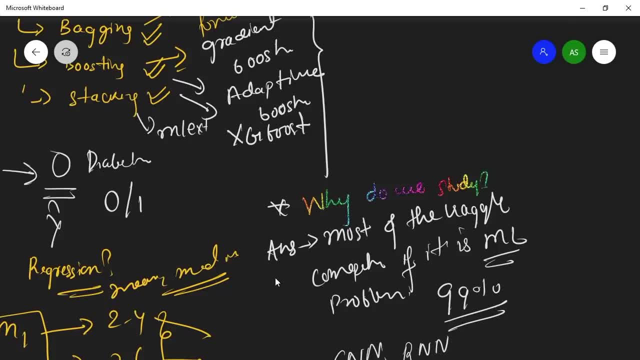 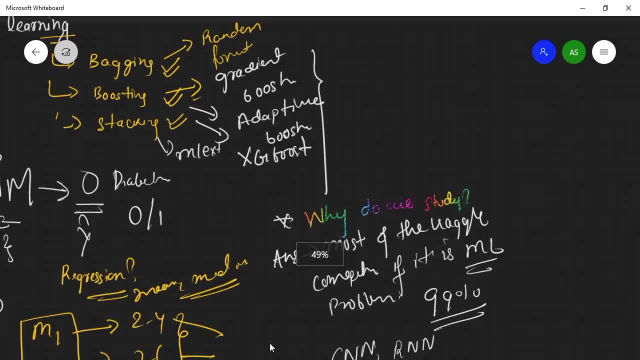 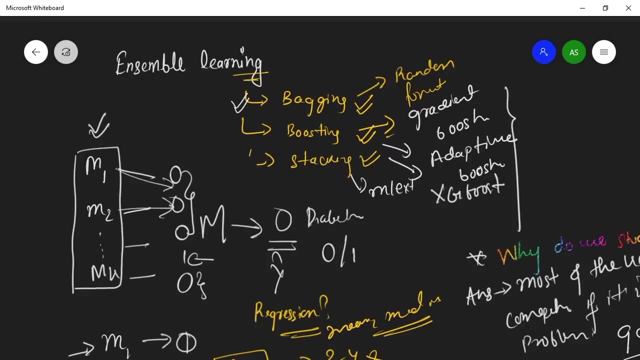 we have seen that they are the winners if they use them. okay, so you can see the case studies, if you want, in detail. okay, great, so we have talked about ensemble learning and in this section and now we will start a subsection which is bagging. okay, we will. 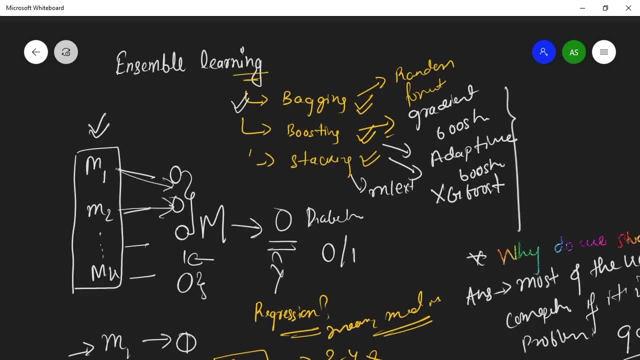 start a subsection which is bagging, which we will dive into the bagging. okay, so it's also called the bootstrap aggregation, A bootstrap aggregated. okay, so we will see a link just for a second. okay, so just. 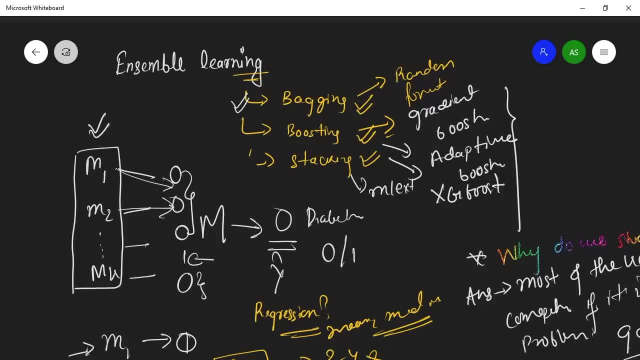 so you recall, ensemble learning is an ensemble of base models. it can be logistic regression, it can be night based, it can be supported with a machine. okay, it's a classification algorithm. whatever the majority of votes will be, it will take the majority of votes. 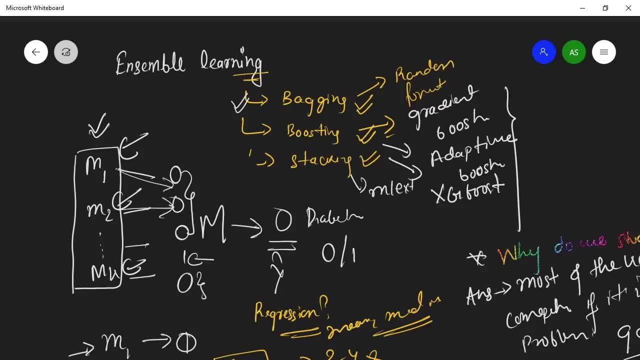 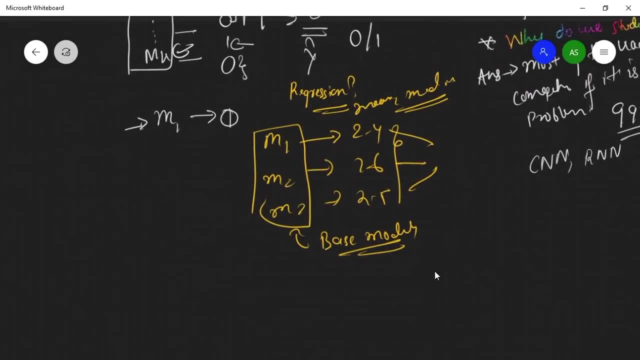 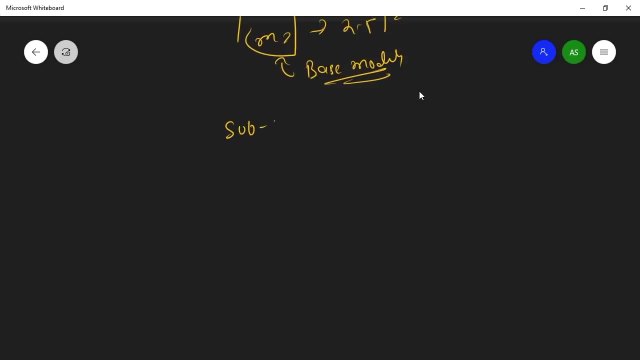 and then gives you a white hat. okay, so that's how it works. okay, so let's. and in regression, we take out the mean or median of your values. great, now we will start a subsection. now we will start a subsection which is something called as bagging subsection, which is called: 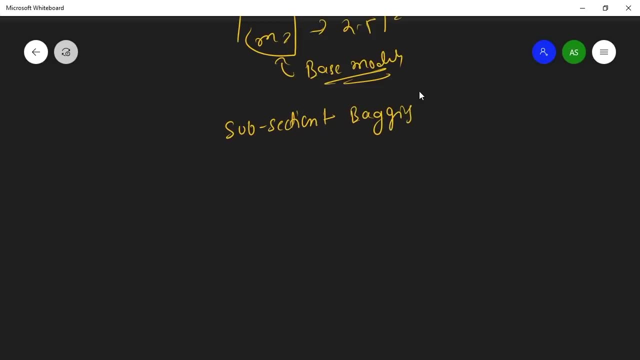 as bagging. okay, so in bagging. so in bagging it's again ensemble learning technique, and sometimes it's called bootstrap, aggregation, and from bootstrap- we deserve, we derive the word which is bagging, like this: 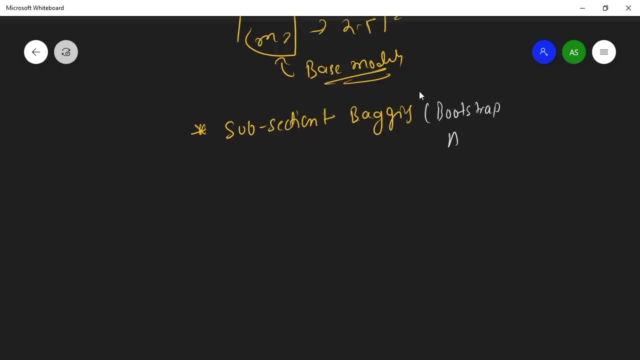 Bootstrap, bootstrap, aggregation, aggregation. okay, I think I'm my spelling is a little bit wrong, but just bear with me bagging, okay. so that's what the from the derived word from bootstrap: aggregation. just in short. okay, okay, great, so it's a statistics term. 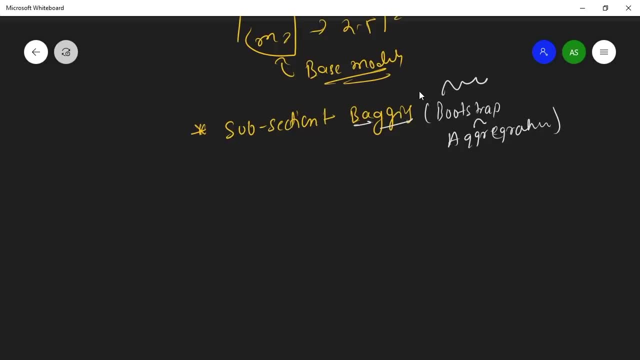 if you heard about bootstrap, aggregation means it's a, it's a statistics term. if you can relate with your statistics and probability classes, it's statistics. So let's see the geometric intuition. okay, let's see the basic overview, or intuition. 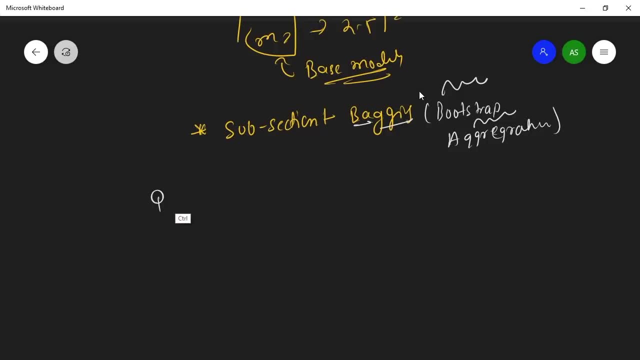 behind bagging, intuition behind bagging, intuition behind bagging: so what we do in bagging. so let's take an example that you have a data set, that we have a data set D. okay, you have a training data which is D. 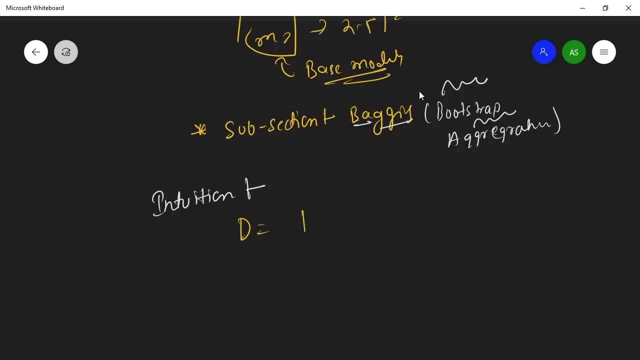 So you have a data. so you have a data like this and what you have done: you divide your data: 80% for training and 20% for testing. okay, so now what you do, just to make sure that you are on the same piece on the variation of your data also okay, so you take your. 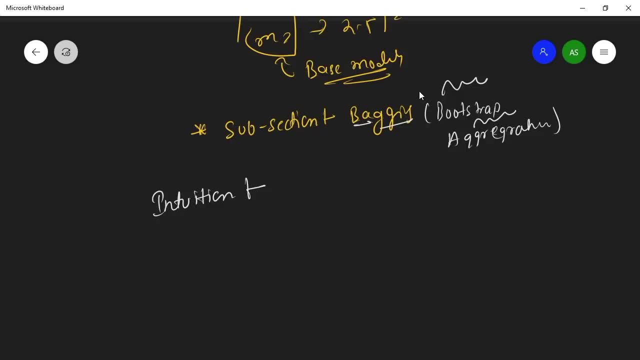 training data. you take your training data and your data is just: you take your training data like this and it's through your training. it's a supervised learning algorithm. so you do. you have xi and yi, so you have your xi with your label. yi for all. i one. i equals. 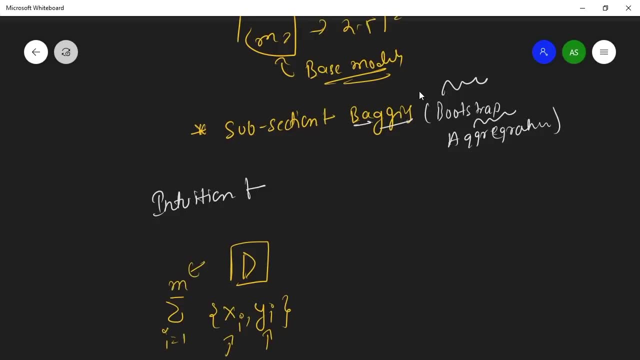 to one all the way around to the m, and m is the length of your training examples. okay, So this is your data, this is your training data. this is your training data. now, what you do? you sample some points. let's take the sample k points, or i, let's take the. 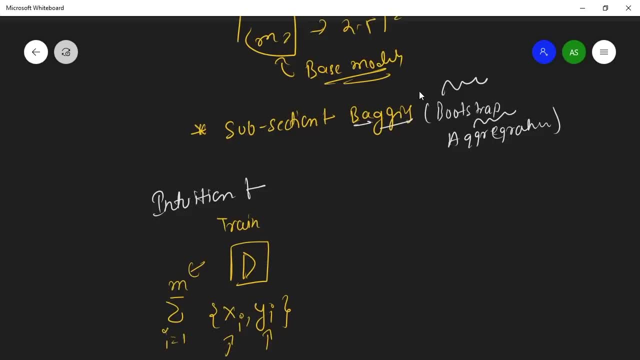 sample k point or i: Okay, Okay, Okay, Okay. example that you sample k points from this data set. you sample, you sample k points with this replacement, with the replacement, you sample k points with the displacement from this data and you feed this to this model, which is list. 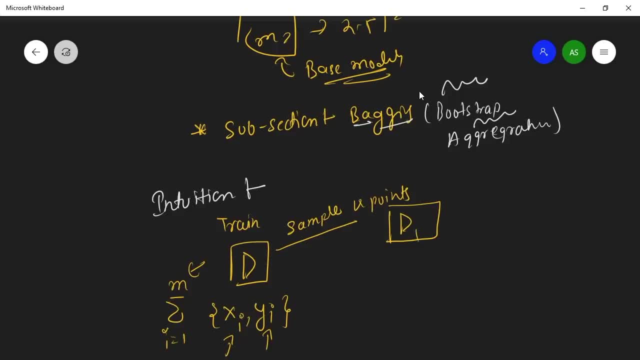 now you got D, so 1, which is D 1. okay, so you have sampled the subsets of subset of a data from this large data set. okay, sample k points. you sample k points. and now what you do? you train your model using this subset of the data. 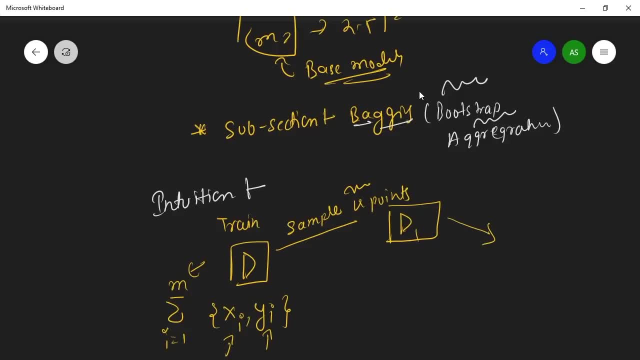 you train your model using this subset of the data and now you got your model as a m1. okay, this is your m1 model. okay. but you may think: yeah, you, can you repeat it again. it's all goes, all gone above your head. no worries, again, I'm. 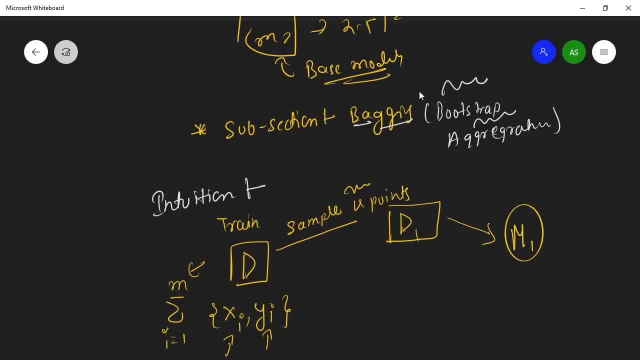 explaining. it's usually gone, okay. so what you do? so I'm highlighting I in white. so what you do? you take your training data, which is the, which is the supervisor, and problem is where you have a labels. now you take out the samples with a replacement, samples with a replacement. 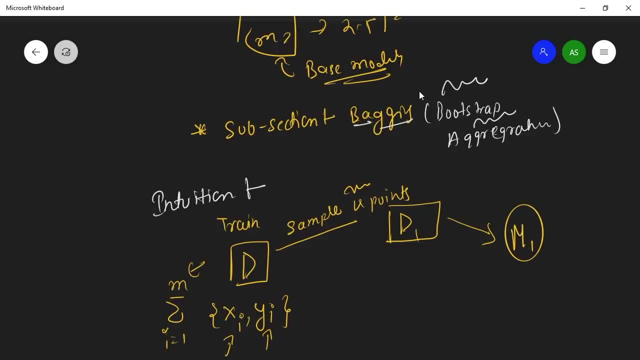 and what do I mean by sample with replacement? I will talk about Justin after I make another sample. okay, so as of now, just just trying to understand. we take out some sample with a replacement around the key points. we sample k points or m points and sample some points, or we take out a sample of a data from this. 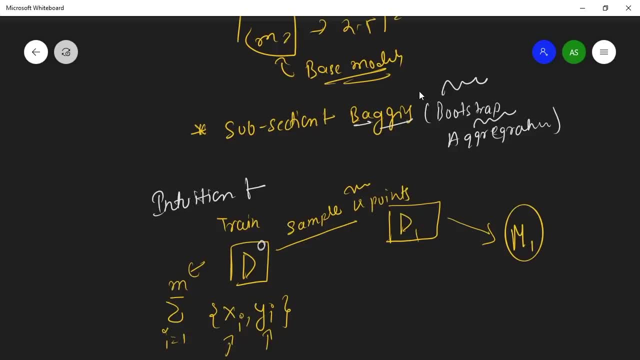 let's take an example: this, this amount of data from this, this amount of data, which any random data means, and we have, this is a hyper parameter. we have to choose the number of samples from this data and then, if- and then we call it as D dash 1, okay, then we feed to the model, means we train our model onto this data. 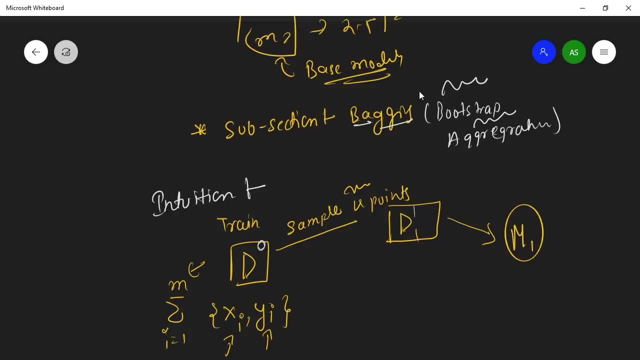 okay, then what we do? we again take out the sample, again take out the sample again, take out the sample key points with the replacement, sample K points with replacement. and what do I mean if your data is here? if your data is here means if your data is here, then 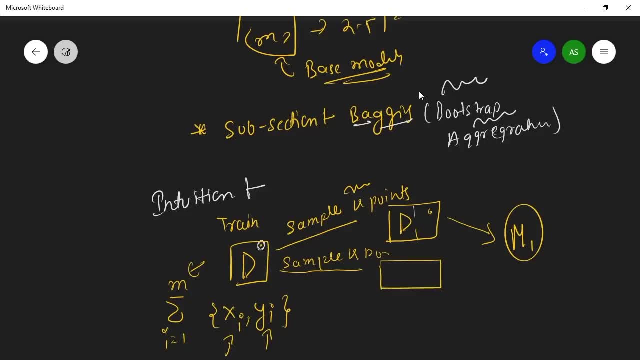 it can be also here, then it can be also. yeah, it is. it is not necessary that your data should be different. it can be same, it is. some data can be be same here and here also. okay, so that's the sampling with replacement. okay, now you samples again the random data and it's not necessary that your data 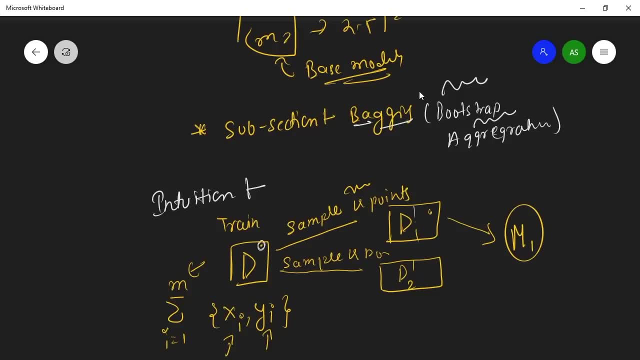 should be different from the d1. it can. some data points can be included. okay, so you again sample k points and the- and here you have a sample of a data from the large data- and then you train your model onto this data M2. okay, train your model onto this m2. now again, what you do, you think out. 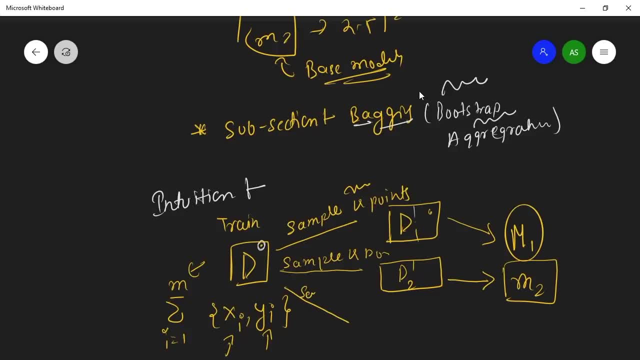 this sample. you take out the sample. you take out the sample. K points. you do it for your number of a base models means no number of times. if this is- oh, I have parameter. okay, how much we're on sample until you have your data points till K. 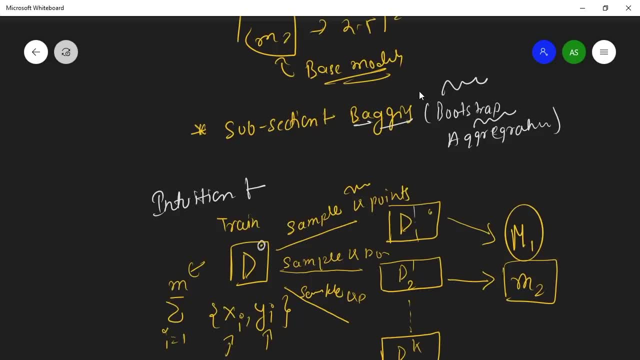 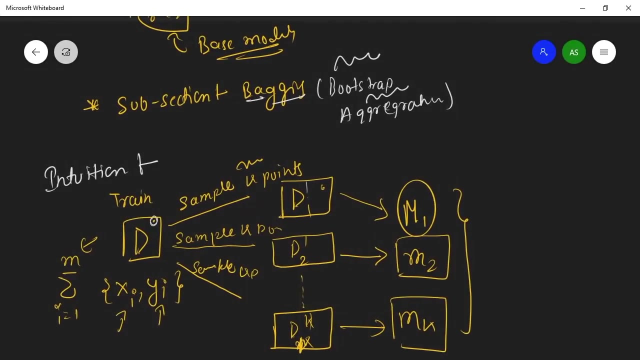 okay, till K, til k, okay. and then you train your model and go forth with the parameter you can. we'll keep going on your model till K, M, K. And then what you do? you have your K models now you aggregate this into a large model. you aggregate this into a large model, okay, M, large M, okay. And in case 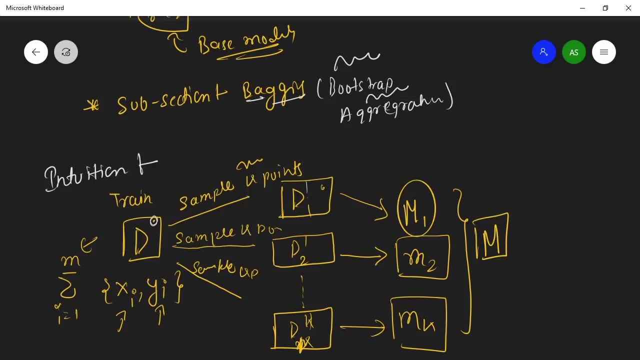 of classification: the majority of votes. the majority of votes will go as. let's take an example of ensemble learning that we have seen that. let's take an example of diabetes and prediction. okay, So if M1 gives 0,, M2 gives 0, and M3 gives 0, and M4 gives, let's take a look. 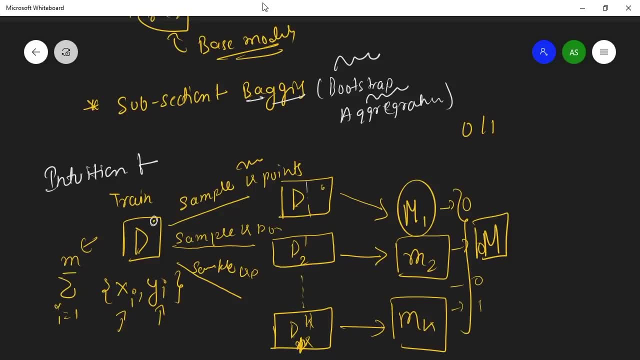 at level 1.. So the majority is 0,. so the majority of votes will lead to the final prediction by half. okay. In case of classification, we take out the majority. in case of regression, we take out the mean or a median. okay, So that's the basic intuition behind bagging, and I really hope. 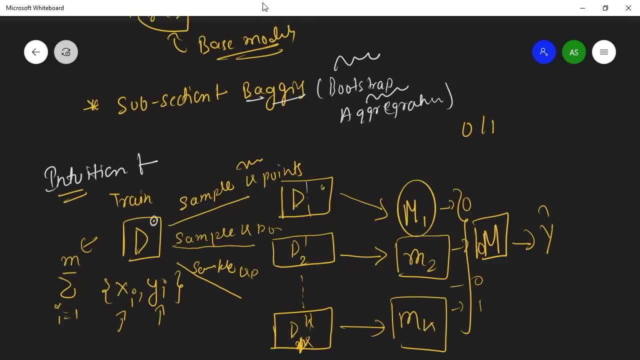 that you understood, okay. So let's take a look at the final prediction. So let's take a look at the final prediction. Let me explain it again. those who have not understood, please pause this video, if you can, because many students are still here that are not, that may not understand this. I'm going to have 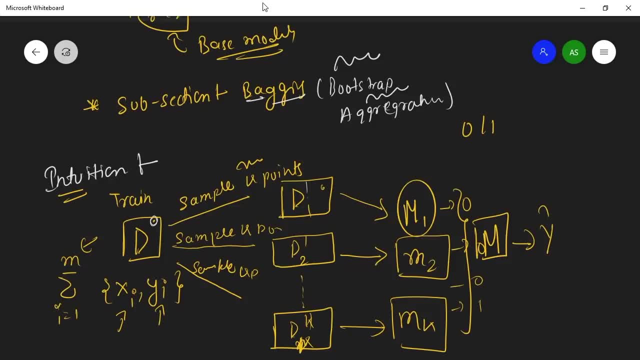 to recapitulate or give a summary of this: okay, Great. So here what we do. we have a large training data set, which is D. Now what we do? we sample our data, sample K points from that data. 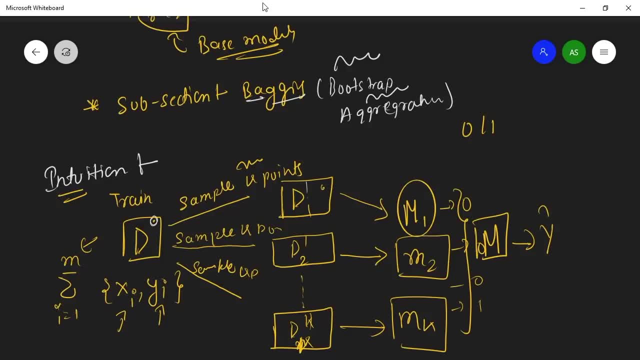 we sample K points from from that large training data and let's take any sample, sample sample of a data and then we train our model on the sample, which is M1, it can be largest regression. okay, Now we sample again K points with replacement and also it is with replacement. 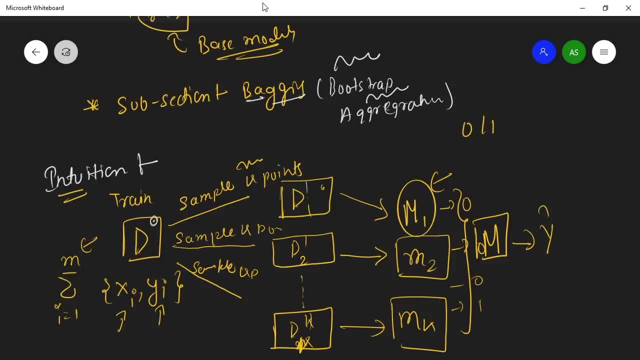 so it is not necessary that your data should be different from the D1, it can be same, or it can be some data points can be same, and then you again train. So let's take an example. you train support with the machine. let's take an example: you train 9 days. okay, 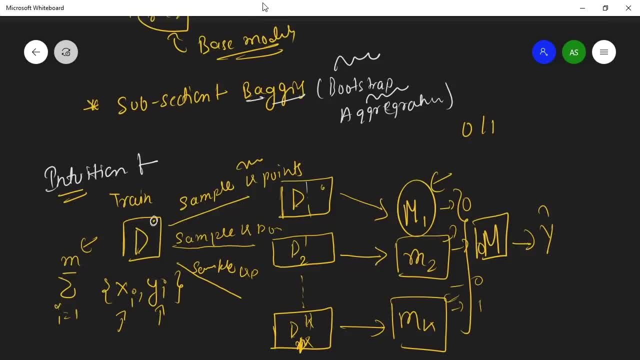 So you train, and the majority of votes is second sample learning. okay, So that's what your backing is, intuitively, and you can see that they are not involving any mathematics. Yet this is just a bunch of concepts, okay, So just, I will make sure that you on on the same days. 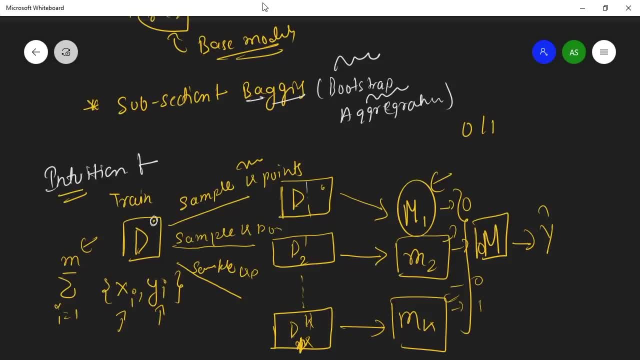 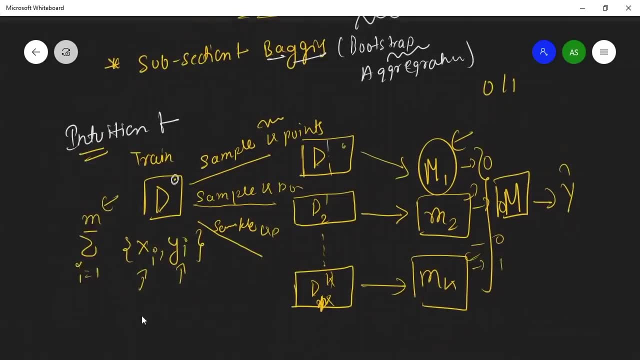 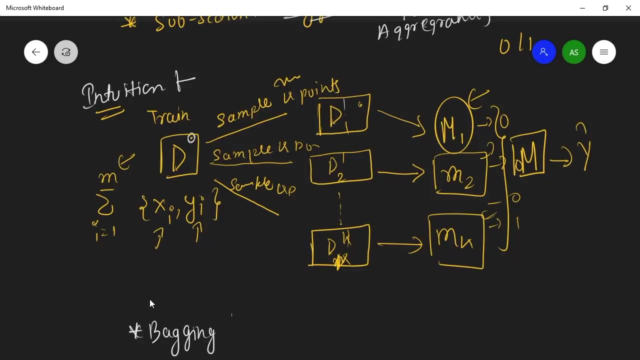 this what it helps. It is great, great version. It helps you introducing the variance Bagging. let let me write bagging. Bagging helps you. bagging helps you in Reducing the variance. It's we will discuss, of ten minutes on to this also. okay. 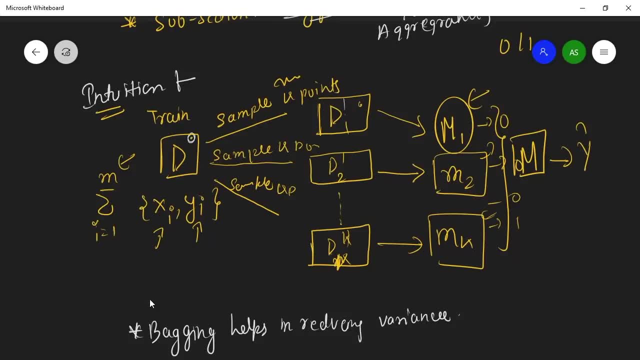 Yeah, okay, so bagging helps in reducing the variance. okay, but before that, there is one term that I want to highlight over here: that Here we have our all base models. these are our base models, and one and two and all of them of the MK. 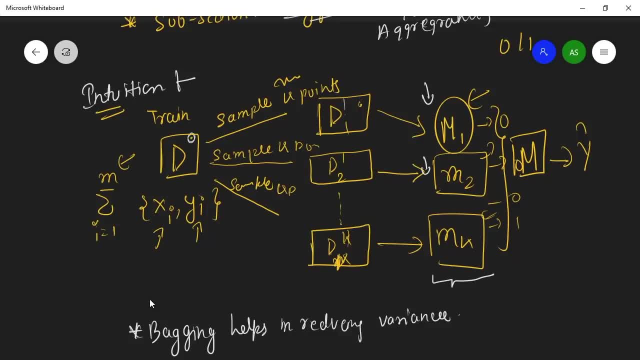 These are the base models. these base models are usually high variance model. These are usually high variance With a low bias model. with low bias model. and what do I mean by this? It is usually we do not do lot of fine tuning, We do not do. 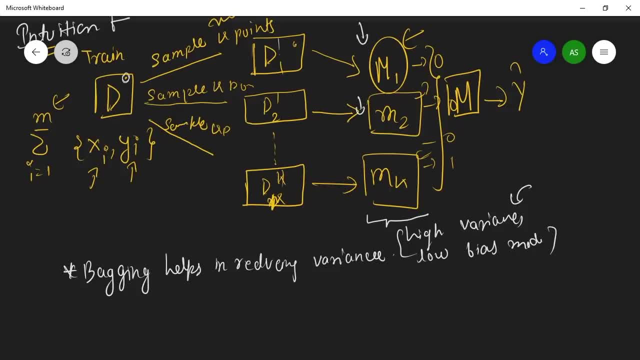 lot Of fine tuning, so that's why it is just overfitting. and we had done overfitting, so that's why just go down to any data, So that's why it is not underfitting. okay, So we have our. the base models are high variance and low bias model. 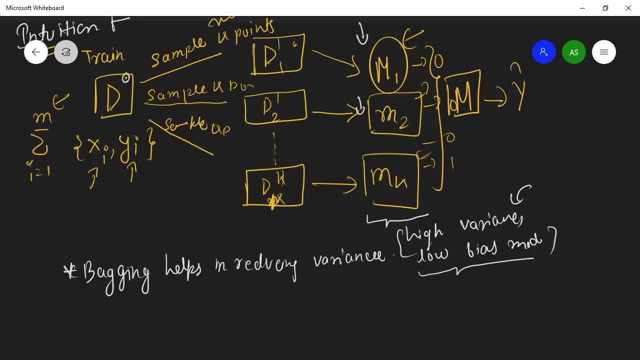 So we do not do lots of fine tuning, just we do a simple list in random for it, Which is initialized with it, with no, no number of depth. okay, It can go as much as we can, so it is overfitting, Okay. so here we have high variance model and low bias. so what it helps, what it helps. 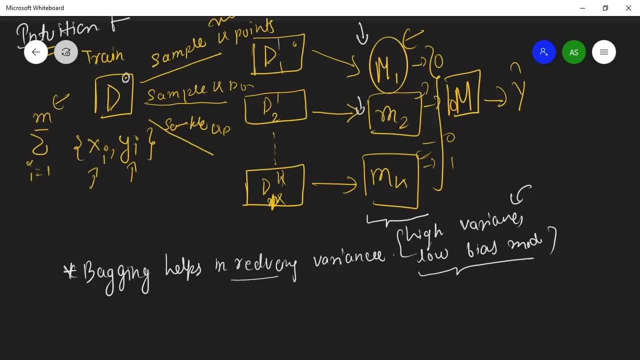 Backing helps in reducing your variance, How it helps in reducing your variance from making your model more robust. Okay, this is just a. what is does is combines them. So you have a low bias, low bias, High variance model. now, if you combine them, if you combine the majority of votes, then obviously we'll get a good amount of good. 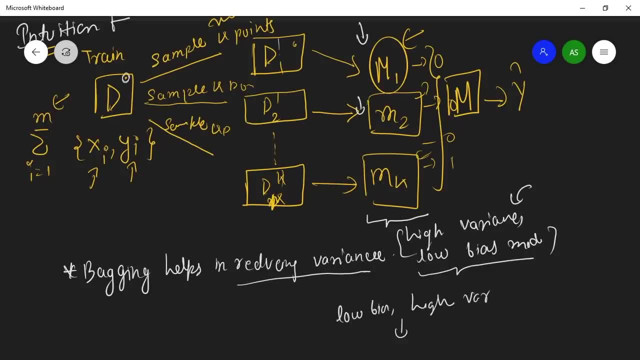 good output or a Correct output, okay, so you combine the models to combine base models to combine base models, and then you get you. then then you get low bias and low variance problem, low variance. Okay, this is what you get, this is what you get after doing back and this helps, this helps in. 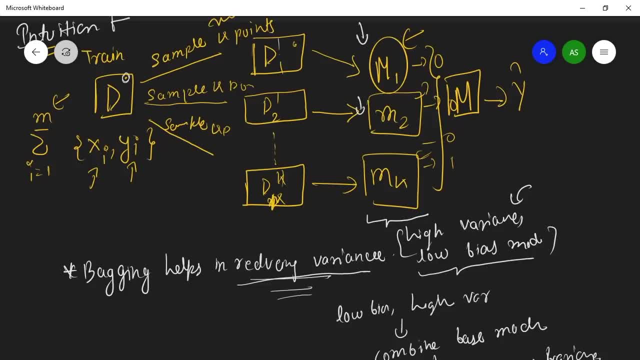 Reducing your variance and this is very good and this is very good okay. So there is some. there is some I want to highlight over here that here We are doing the call rule sampling, so just understand that this is a point: that Bagging helps in reducing your variance, because usually your base learners or base models. 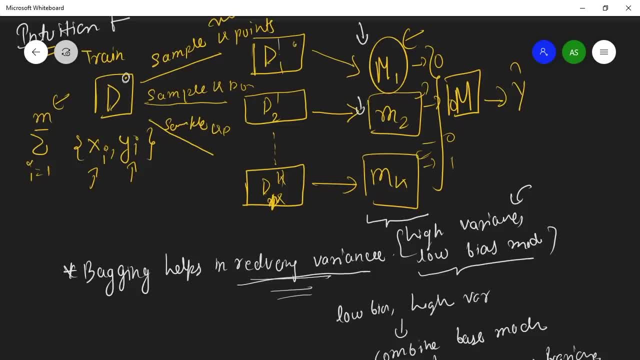 Have high variance and low bias, the bias and variance of that trade-off, that is, high variance and low bias models. So what you do, you combine them, combined base models with a line to a large model, And then you get a low bias and low variance models- low, low bias and no variance, and which is a large model. 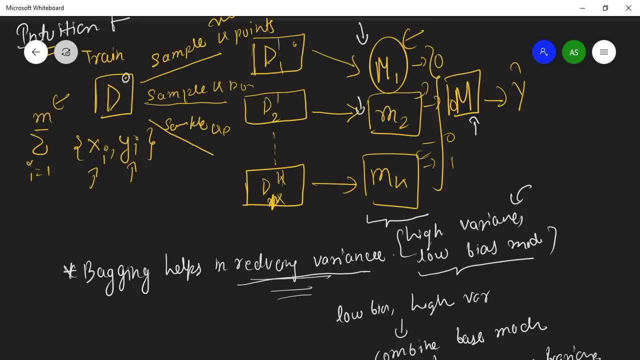 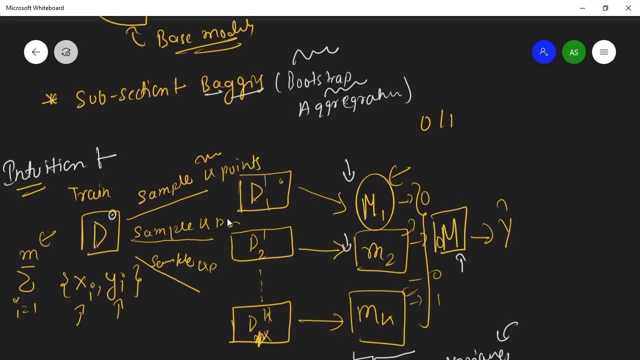 Okay, so that's the. that's the different. now I think that you understood why we call it, as it reduces variance. Okay, so here. Okay so here, What- how we sample our data. how we sample our data. okay, How we sample. this is a great topic to talk on: how we sample our data. 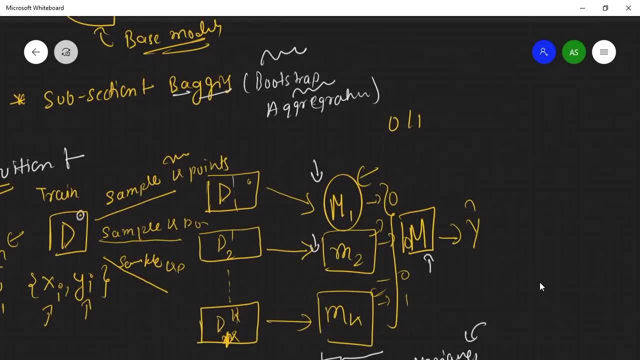 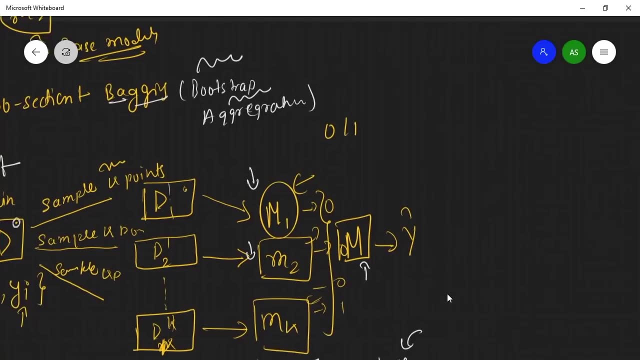 Okay, so here we have: We are doing a row sampling. We are doing a row sampling. We are not being column sampling, We are doing a row Sampling. so let me write it down: While sampling. while sampling our data from the large distribution of a data. so let's take an example. 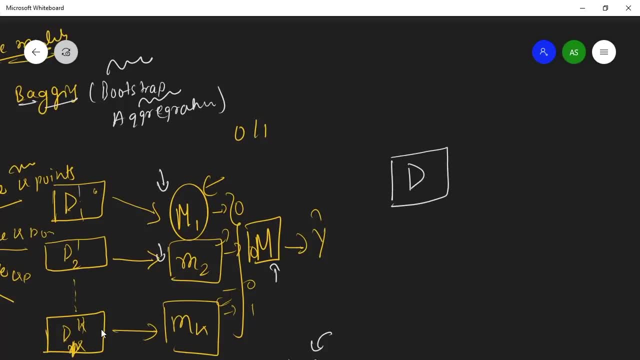 This is my large data in screening data. now, while sampling what we do, we have this: we do the row sampling, We do the row sampling, row sampling while sampling our data. Okay, so let's take an example that we have D columns, D Columns and M Rows. okay, so we have this. 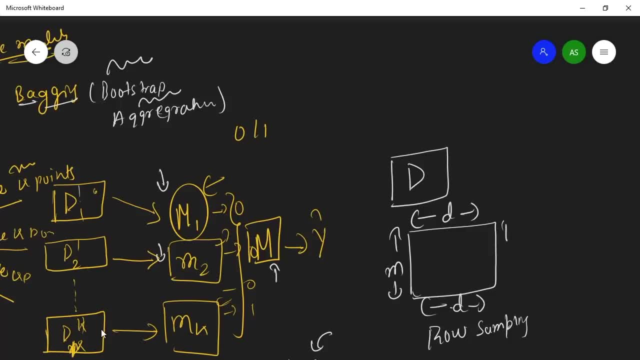 We have B columns and we have M rows- okay, so we sample only rows. in backing, We sample only rows and packing. okay. so it can be like it. can we go to t1? Okay, only rows and packing. okay. so that's what we do in, like a row. 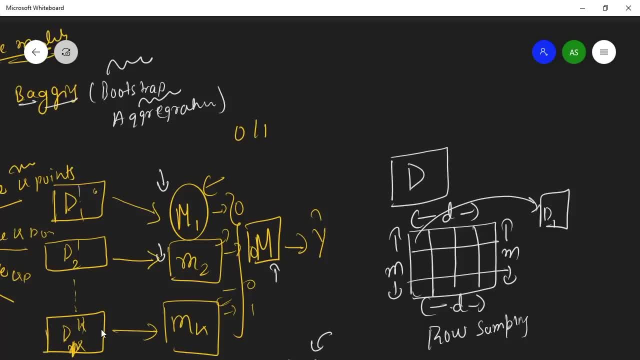 sampling. okay, so we'll see. in random forest we also do the column sampling plus column sampling. okay, and random forest, we do this, we do this, but in bagging we do not do the column sampling, we only do the row sampling. so I hope that you understood the bagging. okay, it's also the bootstrap aggregation. 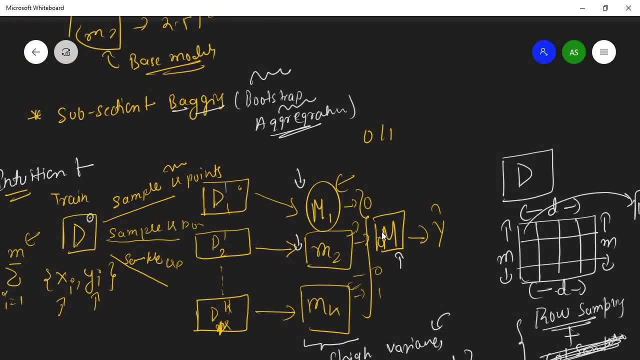 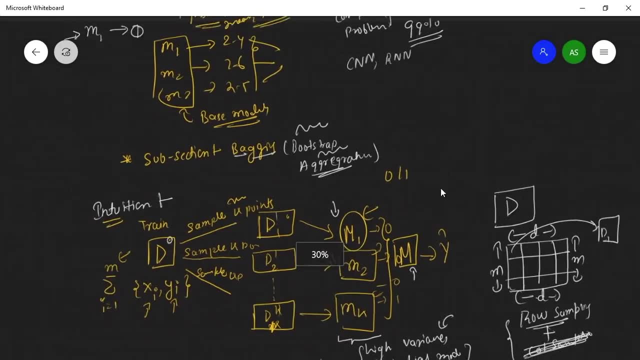 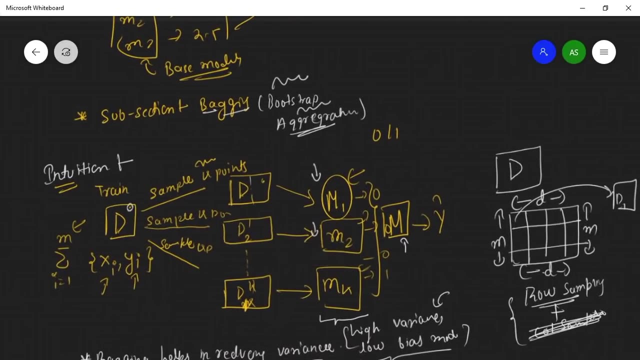 first your bootstrap and then you aggregate your base models. okay, so that's why the name it as a bootstrap aggregation. okay, so, just to make sure that you all understood. so I'm just recapitulating the subsection, as you can reverse the video to know about ensemble learning, because I don't want to just 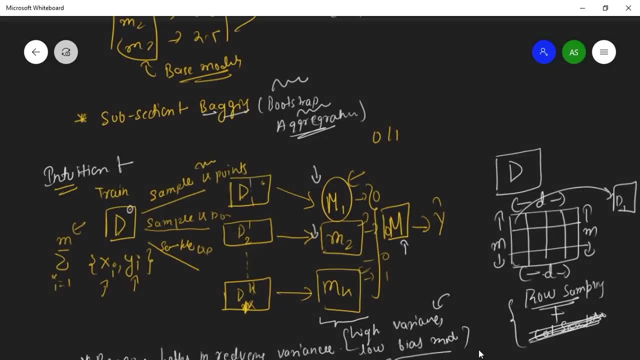 spend my time on to that. okay, so here just to go, just want to make sure that here you have your training data. here you let me see, here you have a training data, which is: you have a training data and then what you have done you'll take. 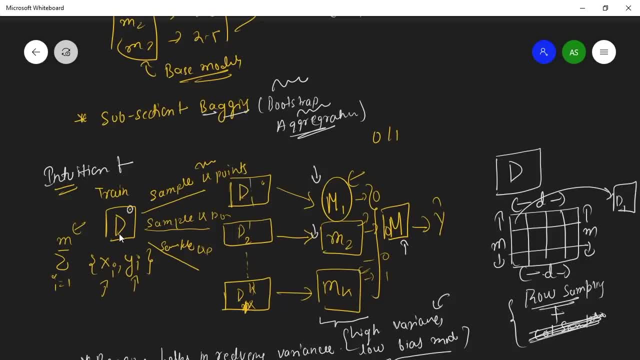 a training data and then what you have done. you'll take a training data and then what you have done. you'll take out this sample M points with the replacement okay, into your data subsets, out this sample M points with the replacement okay, into your data subsets of a data and then you train your model M1, which is your base model can. 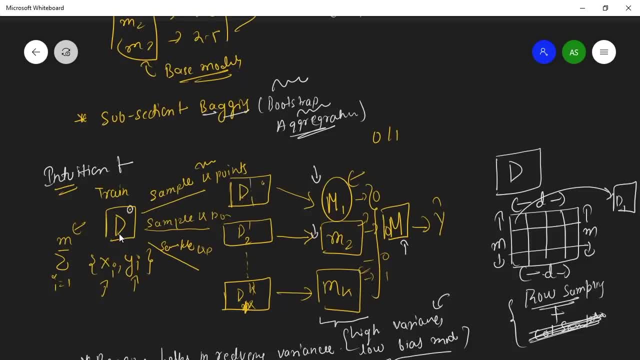 logistic, linear. okay, then you again sample k points and D2, then you again train your model on to these subset of a data. you do for K, you do for K models or K subsets, and then you combine them. as already of votes, my majority of what we 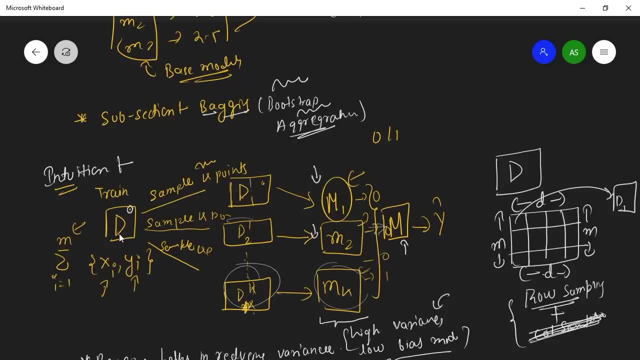 lead to classification and and if you use regression problem, we take out a mean or median of most output from the model space models. okay, ok, so that's the intuition behind Bagan, and it tells: and reducing your variance, it else and reducing your variant because you're more based model. 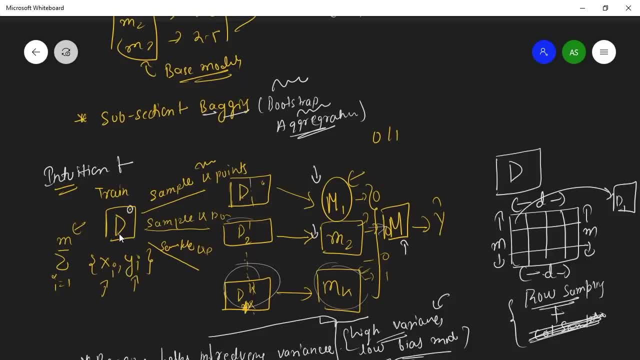 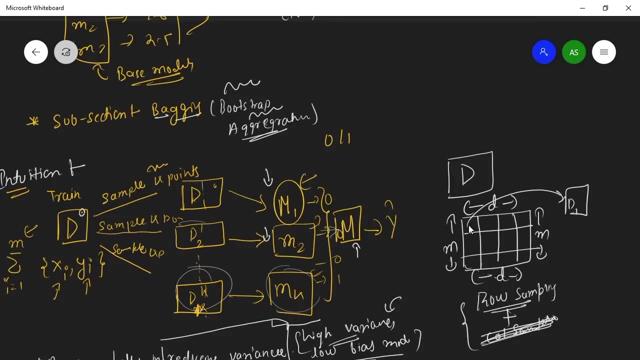 size, usually high variance and low bias model. so it combines the base models to bring up low bias and low variance model. that's actually good, ok. so and, and, and Bagin, we do the row sampling, we do the row sampling means we have a D features and we have'm column and rose. 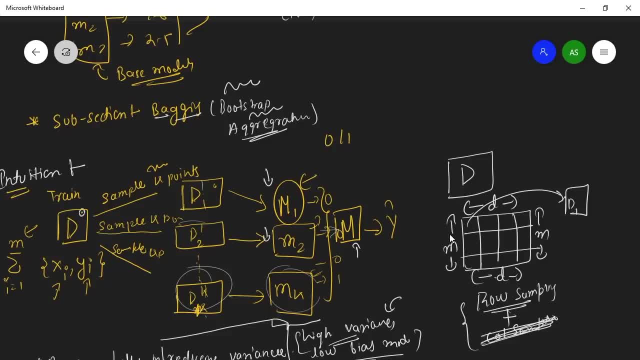 So we do sample of our m, not d, okay. So we take whole column, we take all the columns, okay, But we take subset of a rows for training, okay. So that's what we do in bagging and I really hope that you understood this bagging technique. 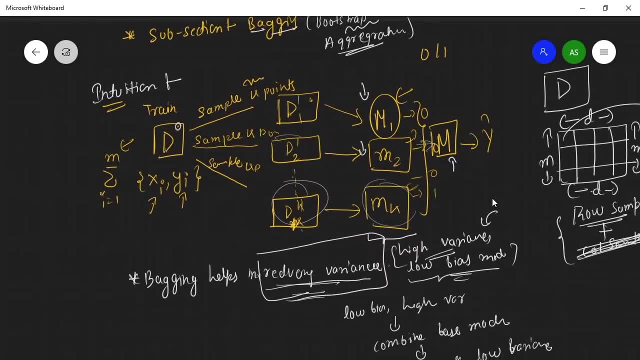 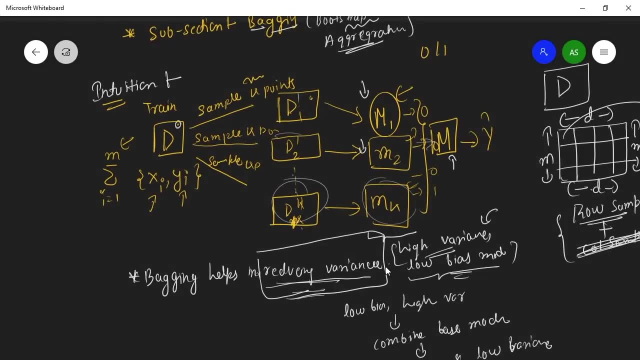 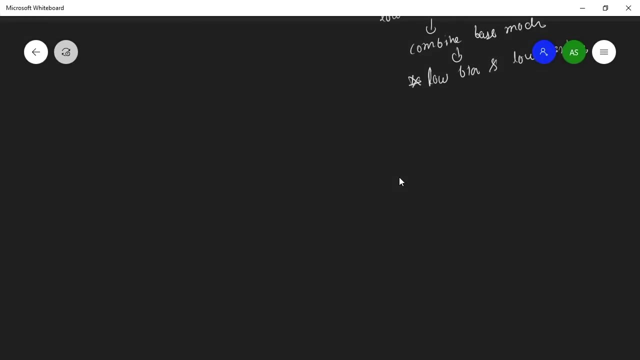 Now it's time for learning one algorithm, one good algorithm, one powerful, one gaggle winning algorithm, one production level algorithm, which is random forest. okay, Why? I think random forest is a very, very powerful algorithm to work on, is a very, very powerful algorithm to work on. let me write a random, random forest, okay. 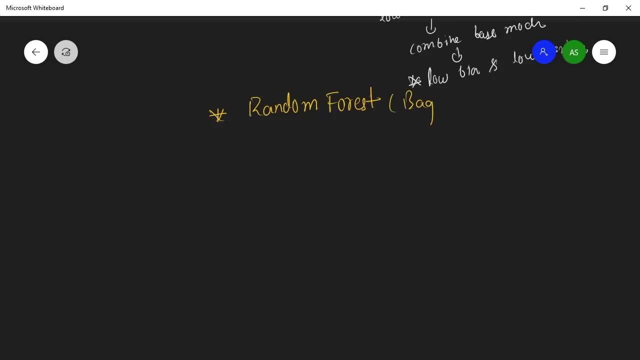 Random forest. it's a bagging algorithm, it's a bagging technique or you can call it bagging algorithm, okay. So why do I call this very powerful? Because in also my professional experience, I think that I have also used a random forest a lot. 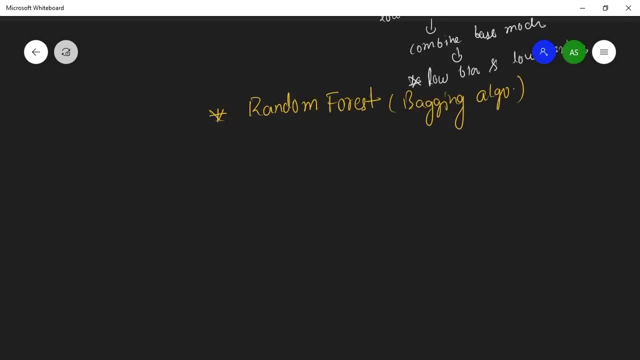 And it seems like It's a very powerful algorithm. whether you want to build a tag competition, which is a machine learning problem, or you want to make a production level machine learning, okay. So random forest usually used by Quora. then we have Google, Amazon. they all use this random forest. 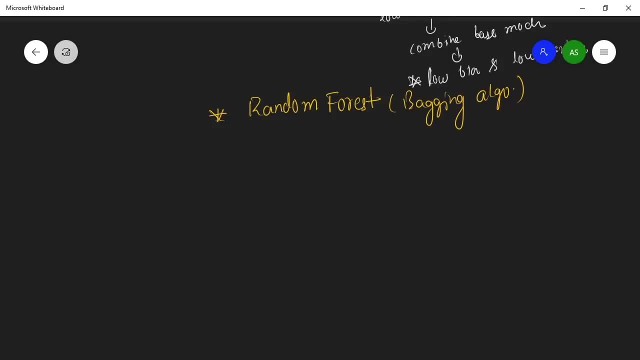 But it has some basic intuition of basic concept that instructors are not teaching and it's very, very important, okay, So, first of all, what we do in random forest, So let's recall our decision trees, Let's recall our decision trees into this. 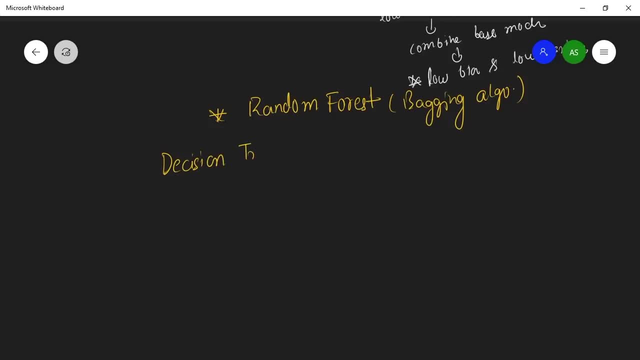 Now our decision tree will play a role. Now, here we have a decision tree, So let's recall our decision tree. So what we are doing in decision tree, we are doing on it, is a simple: it makes a decision and splits your node, okay. 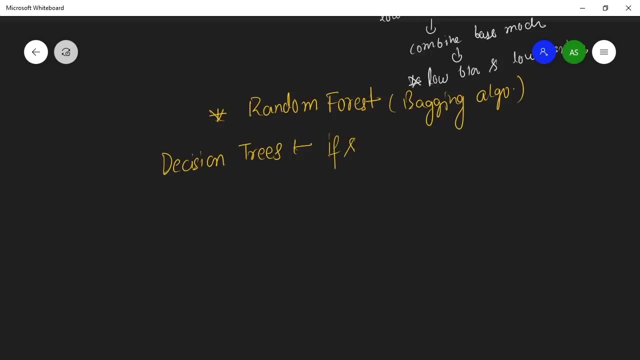 So what we are doing it's a simple if and nested if and else. statements Nested if and else statements Nested if and else. So we take: if the sepal length is smaller than petal length and you take a y equals to 1, like this, okay. 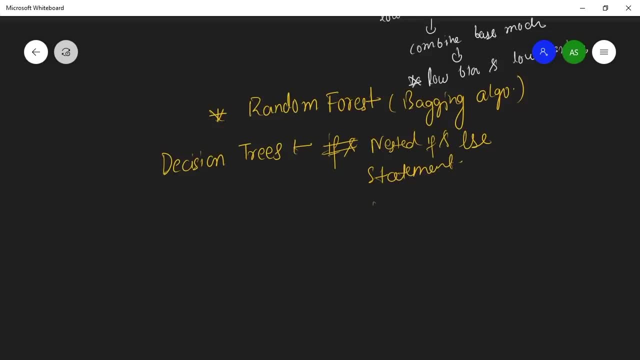 This is a nested if and else statement. It's just ask a question. it's just ask a question. it's just ask a question to the node and then splits the node, and then it splits the node. okay, So you can reverse the for the section of decision tree. 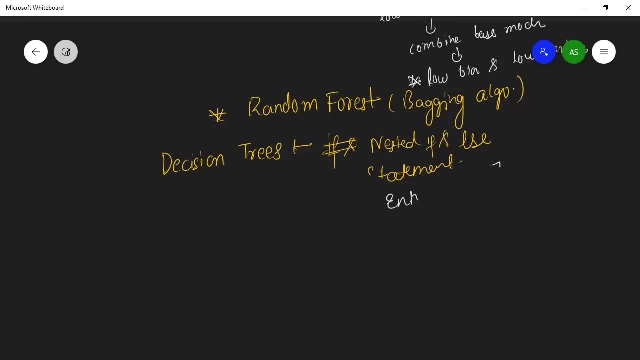 We have some attribute selection measure like entropy, Then we have information gain, information gain. Then we have a genium. here Again, in our case, it's just creating a genium. Then there is some intensity and that's why I have set it cycles and I am gonna Edinburgh's probability. 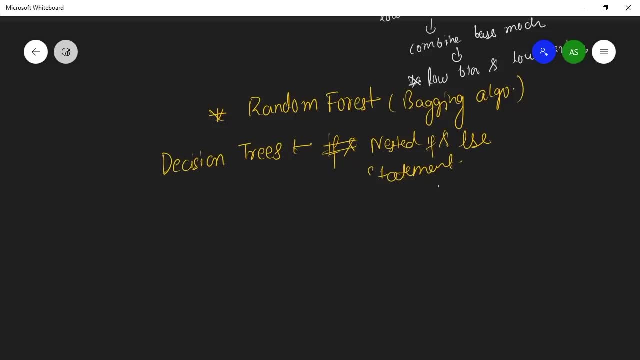 which we have seen into do in one hour of section of division tree and I hope you enjoy. Okay, So that's the decision tree. Okay, So what is random forest? Random forest, random forest is a combination of decision trees. 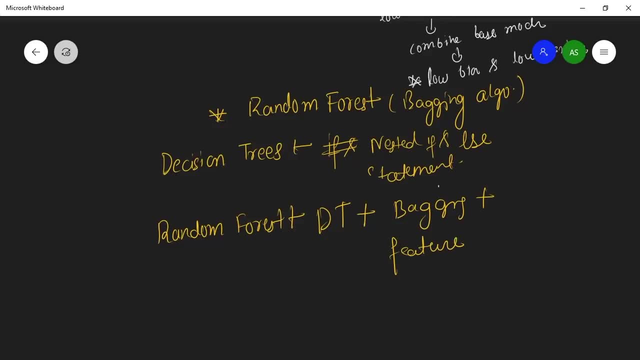 duty plus bagging, Plus bagging, Plus feature bagging, Or we call it as a column sampling, column sampling. okay. So what do I mean with this? let's understand. this is step by step, so it's it makes sense to you also, okay. 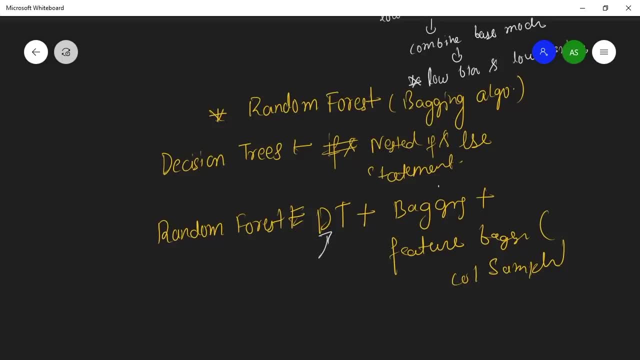 So what we do in random, for we have our decision trees, okay. So you know about decision trees, so we have there's a 500 decision tree, okay, So random forest is an ensemble learning algorithm. so we have a lot of base models, means decision trees, lots of base models. 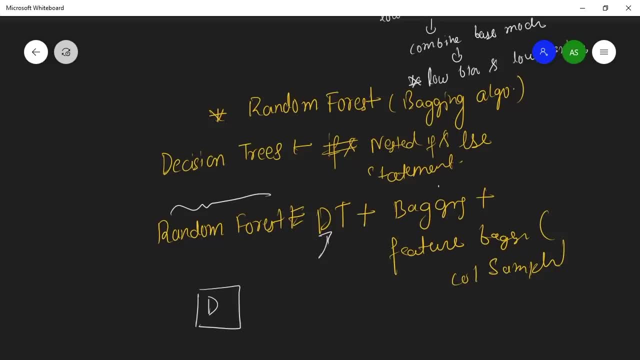 So here we have a large distribution of a data- Okay, and here we sample our data d1 and we train a decision tree on to this data. Okay, did this decision tree? then we sample the two with the replacement, then we train our date decision tree onto this subset. 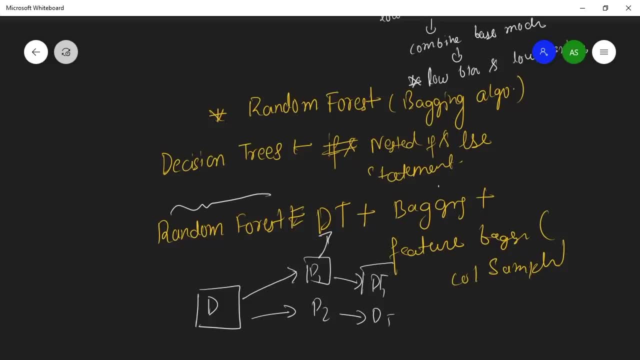 Okay. so you are not using different algorithm. You are using wallet decision trees. Okay, with the row sampling with bagging. here We are doing bagging means the sample sampling with replacement fits. here We are doing a row sampling, Okay. Plus, in bagging, we are doing the row sampling. row sampling and aggregating your model means whatever the majority of votes. 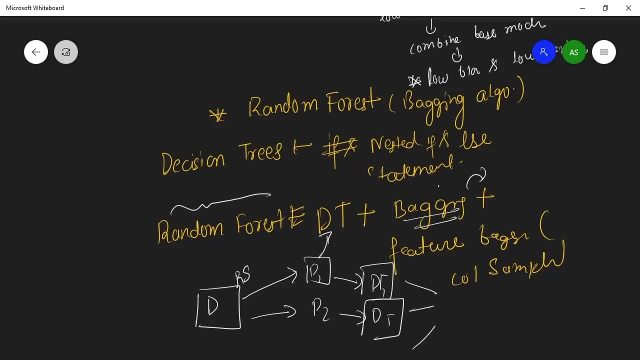 You will aggregate your model. Okay, so you are doing the row sampling plus the column sampling also. Okay so, here and this in a bagging, we are only doing the row sampling, We are taking whole column, whole features, but you are not, but you're only taking the rows. 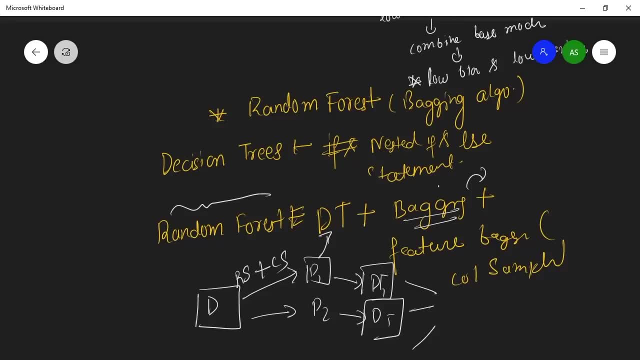 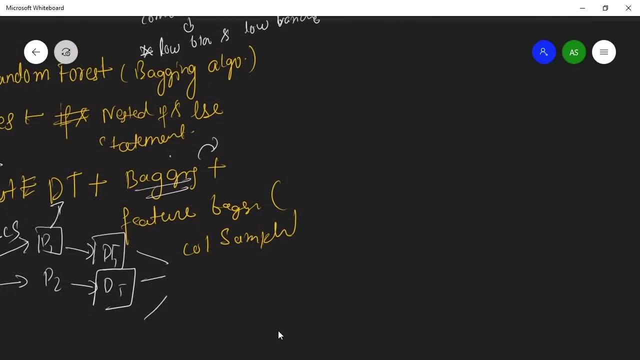 Okay, as a subset, but here we are taking, we are doing also the column sampling. Okay. so let's Understand what do I mean by column sampling or feature bagging? Okay, So the column sampling means. column sampling means that you have this, your data, You have this, your data, like this: 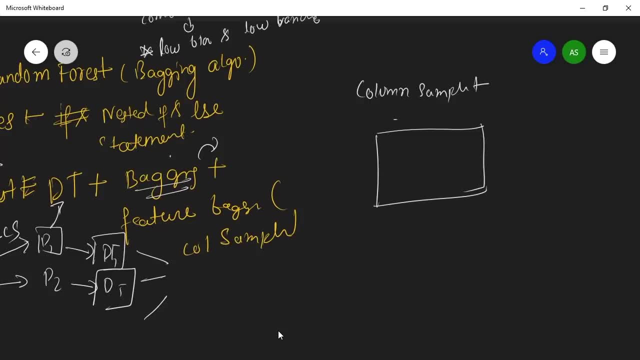 You have this, your data, Okay. Now you have these features. you have your deep features, D features, D columns like a, B, C, D, and you have M rows, M rows- Okay, we have M rows, Okay. So what you do? you for replacement? you take any rows. you sports for sampling, you take your rows. 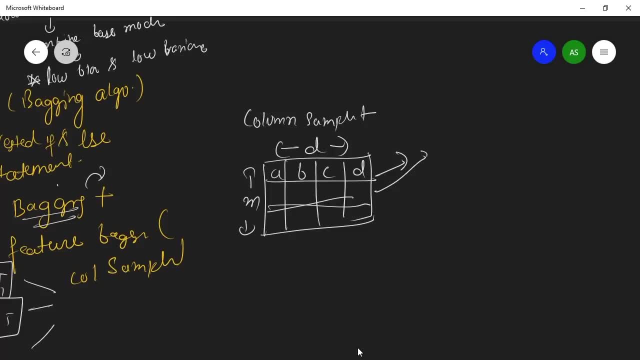 Random rows. Let's take an example. You took this row, this row, Okay, This row, and and you took a and B as your column, and then you train onto this. you are not taking full columns Or features. you have taken this a and B and in their frame, and in the next you take, you took C and D. 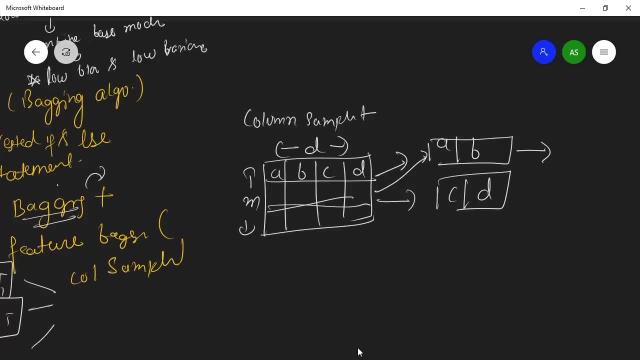 Okay, you took C and D. Okay, and then you train with one one, one rule. just an example: you're 20 century, So they're different. they are different, and if they are different, it's much higher chance that your model will be very, very good. 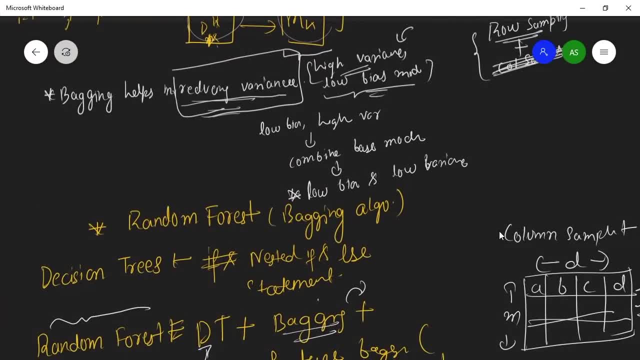 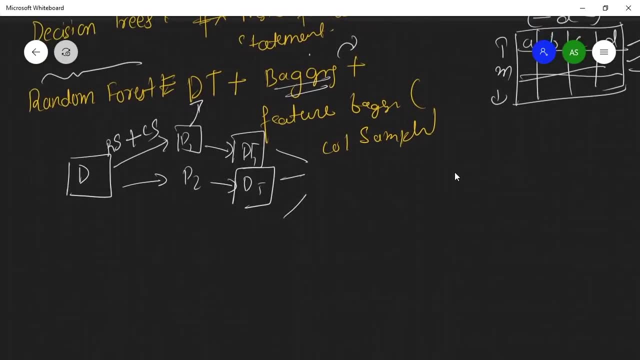 Okay, and sample learning. if your model is different, then this is, then it's very, very good, Okay, Okay, great. So That's the, that's the random forest. Okay, So we have a large number of decision-free means since base learners, as a base learners that are, 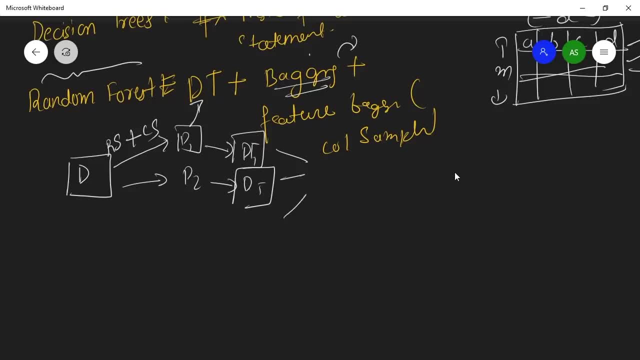 Using a bagging technique means it's sampling rules. have with the rule sampling plus column sampling: Okay, the rule sampling plus column sampling, which is column sampling, also called the feature bagging. Okay, train different decision trees and then you in majority of votes and and then you include classification. 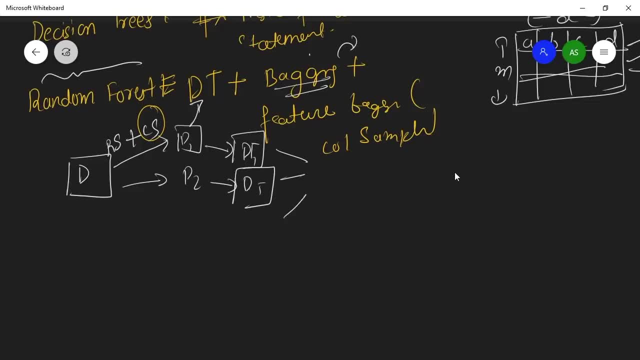 You take them as already, or in regression. you take the mean or a median of the outputs on the base models. Okay, so that's what you do in this, So that's what you do in this Random forest, and I hope that you understood. Okay, so let's understand it more intuitively. 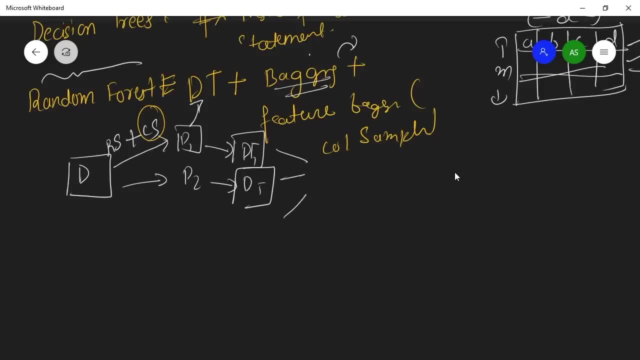 That there is something called as OOB. It is something called as OOB Out of bad points, out of bag, and this is called in back points of this, Something called as out of that point. So let me not recall. this concept is now. So let's, let's take an example. 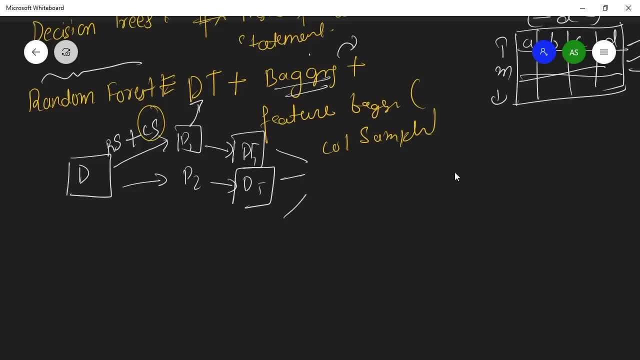 Let's take an example. Said that, what do you have done? You have this Dn, you have this, you have this large, large training set set, which is B Okay, which is D Okay. So what do you do? Let's take an example that you've taken. 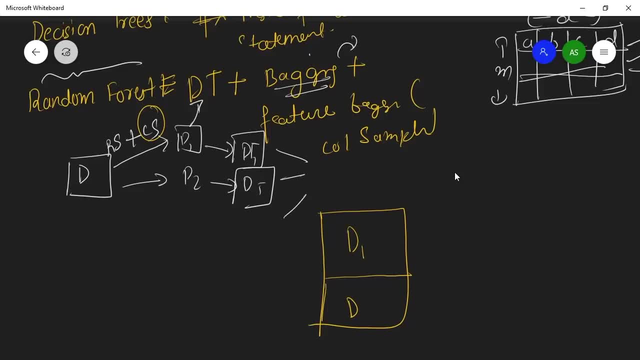 This sample of a data as a d1 and the rest of the data is called the out of back points. It's called the out of back points. So what you do, you subtract, means the training data minus the DI, and I is the sample. so these are. 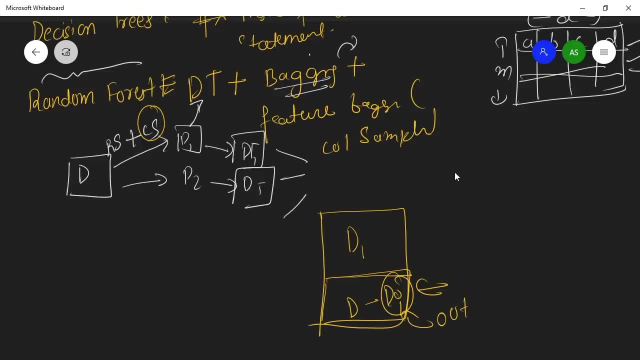 The left points after the sampling, which is out of bag as points: Okay, out of bag. out of bad points: okay, and this, this, this can be used for cross validation, for evaluating your model. Okay, So if you set o m a cycle, learn. there is a very good library which is I can learn. if you said: 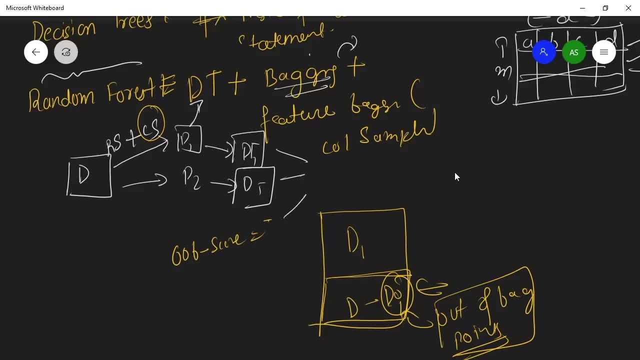 OOB score to ob is called to true. if you said ob is further true, then it will give you the ob score also. Okay, So that's the basic out-of-bag points and I hope that you understood out-of-O-B points. So now let's recapitulate our bagging and random forest, what we have seen in random forest and bagging. 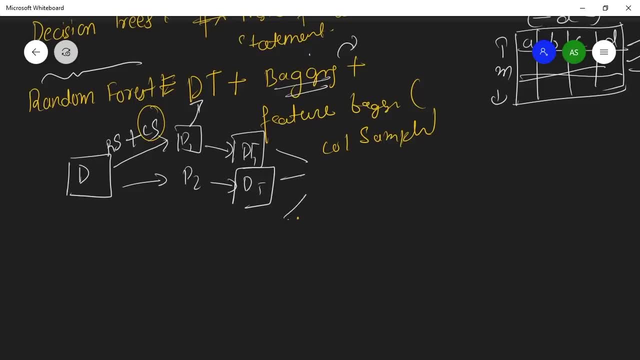 So in bagging we have seen that we have our data, we have our data D, we have our data D. What you do? you take out a sample, you sample with replacement D1, then you train your model onto this subset M1.. 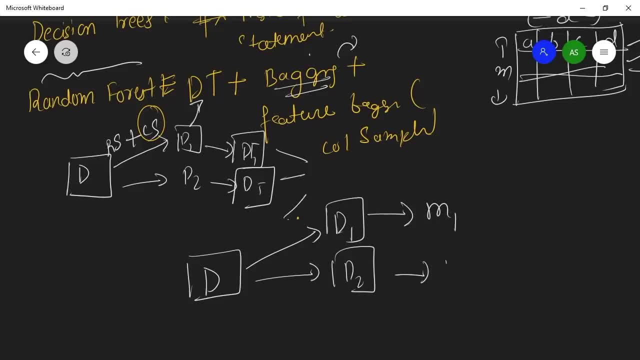 Then you go into D2, then you train your model onto D2, and what you are doing you are doing is sampling with row sampling plus volume sampling with replacement, And D3, D3, then you are getting your model D3, getting your model M2, M3.. 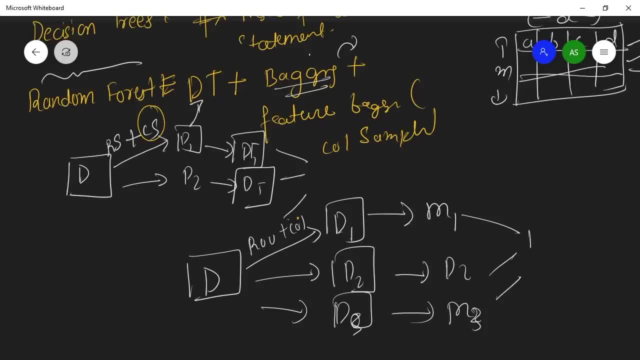 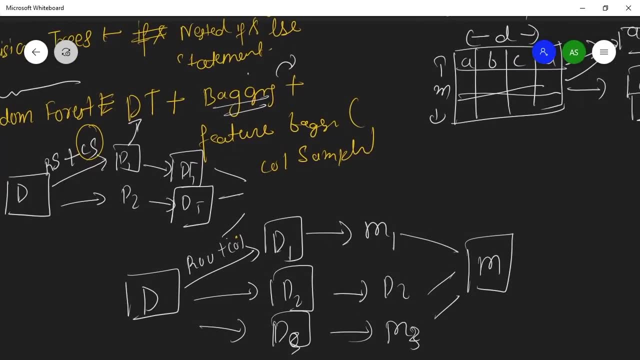 Okay. So the majority of The majority will go on a large model which is: aggregate your model, aggregate your model, and then you get your final prediction, which is Y-hat. Okay, This is the whole pipeline. So in bagging you only do the row sampling and random forest you do with column sampling, as well as you only take decision trees as your base models. 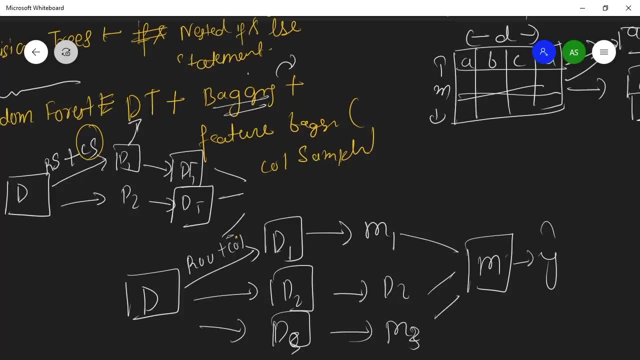 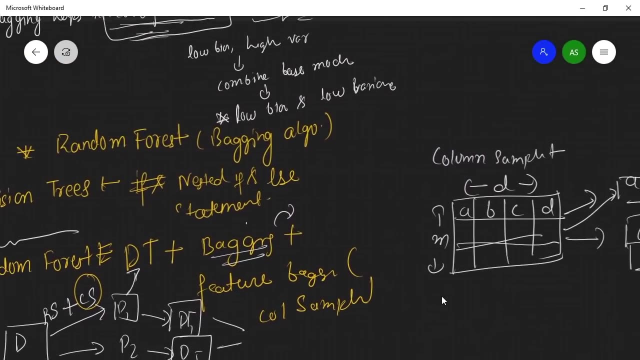 Okay, So in bagging you choose different, different kind of models, but in decision tree, in random forest, you take. You take your decision tree as your base model and decision tree as your different, different data. Okay, So that's the basic intuition behind the random forest and I hope that you understood also about what is column sampling or what is feature bagging. 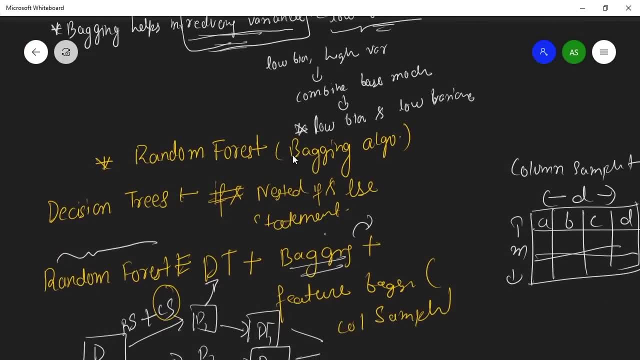 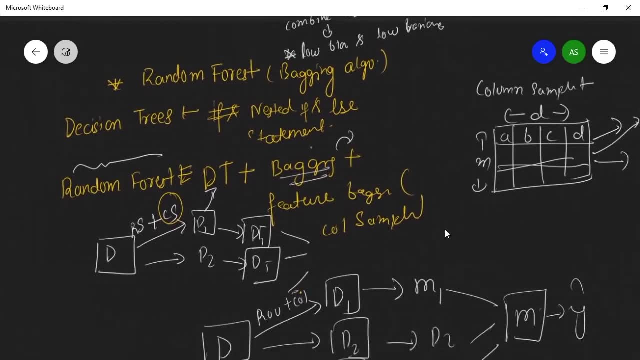 Okay, And obviously this also helps in reducing your variance, as it is a bagging technique, So obviously it will help you to reduce your variance. Okay, So that's the basic intuition behind random forest. So let's see the runtime. 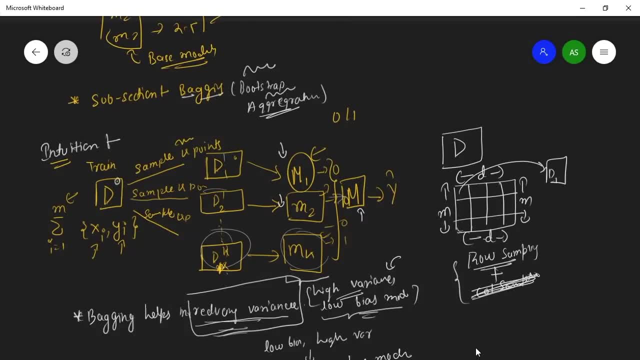 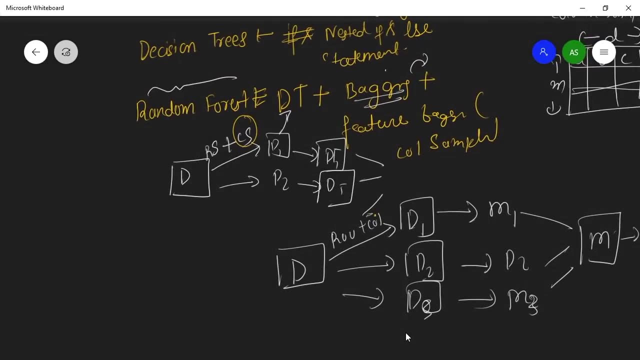 Train and runtime complexity of this, because if you, it is very, it's very required to talk about train and runtime complexity of this random forest. Okay, So, in decision trees, in decision trees, the train complexity, the train complexity. in decision trees, the train complexity. let me write. 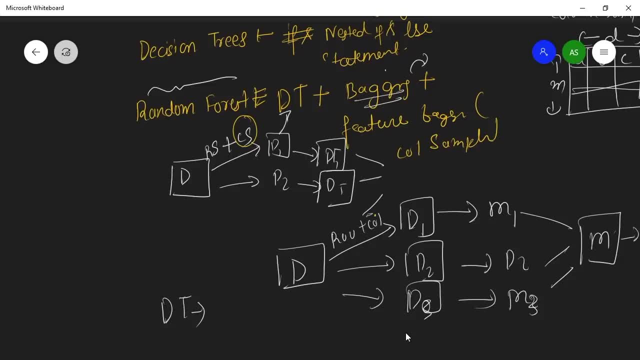 In DT the train complexity is order of N log N, N log N times, D Okay Times, D Times: yeah, So it is in decision tree we have N log N. So in random forest we have D number of decision trees, K number of samples. 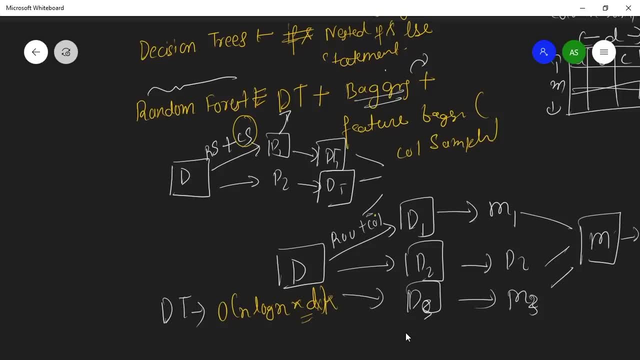 Okay, K number of models. So that's the. that's your model, That's the train and runtime complexity, training complexity of your random forest, And in decision tree it's just a N log, N. Okay, So that's the and D here is the number of cases. 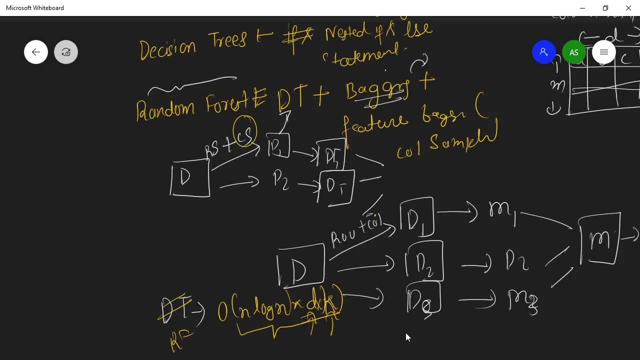 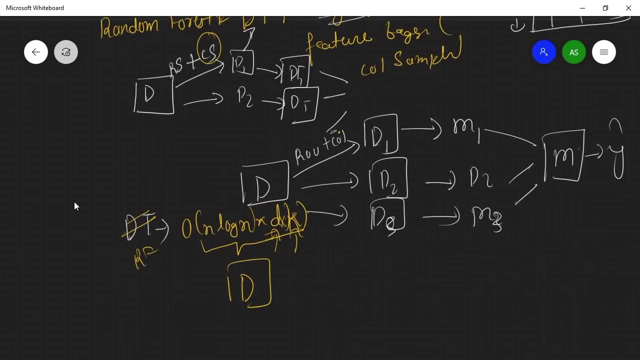 K is the number of the models. Okay, So it makes sense also If you take an example of your D as a large data set. Okay, Let's take an example that you have a D. Okay, Now you take out a sample with replacement with row sampling plus column sampling, like feature backing. 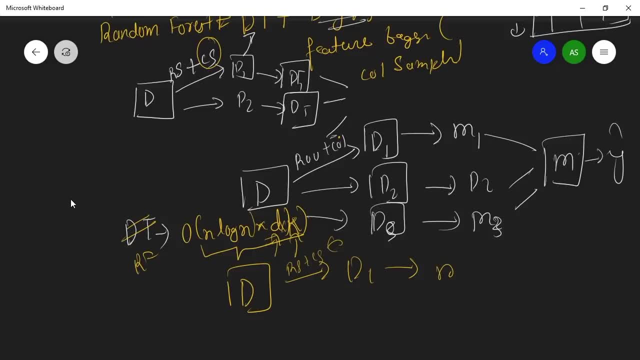 Okay, You take out a subset and then you train your model like M1. Then you again do the D2. Then you take out M2. So here, all of a sudden, the MK. here you have a K models And then you have a D decision. 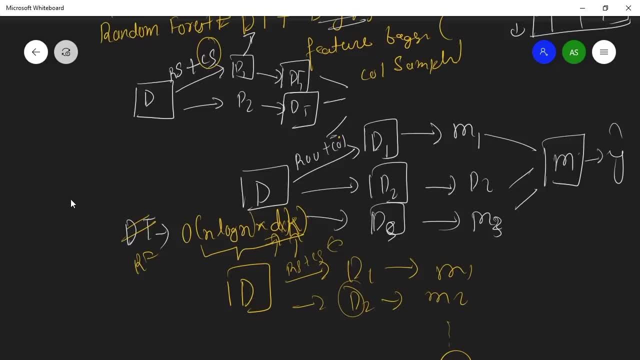 And then you have a D decision trees: Okay, So, and also, this is a trained, a trivially paralyzed. it's a trivially paralyzed. What do I mean? You can train this model onto parallely. Okay, You can train the model. 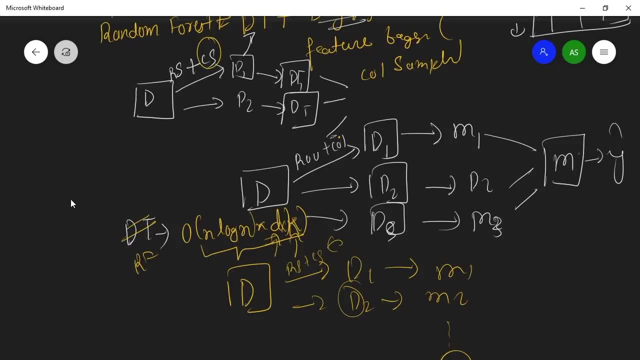 You cannot. you, you can train this parallely. Okay, You can take out a subset. You train D1 parallely, D2 parallely, D3 parallely. So this is a trivially paralyzed, parallelized, parallelized. 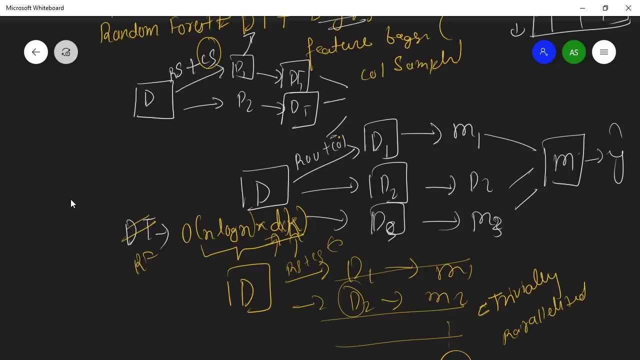 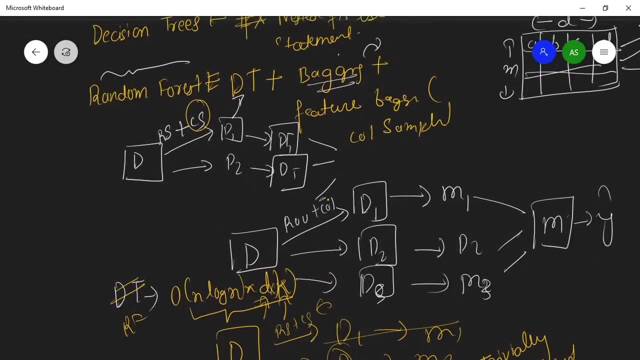 I think I'm pronouncing It's correct. Okay, It's a trivially parallelized. I can do trivially parallelized also. Okay, So that's the decision. sorry, train and run, run, run, run. complexity of random forest. 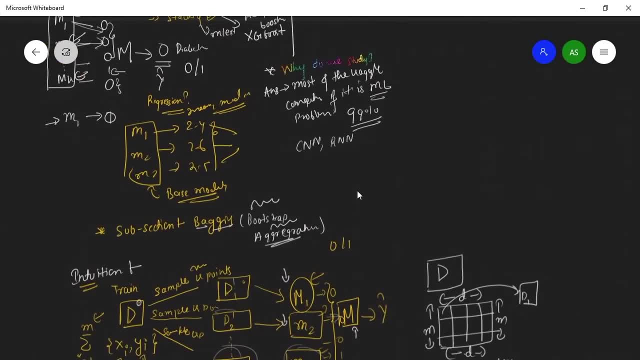 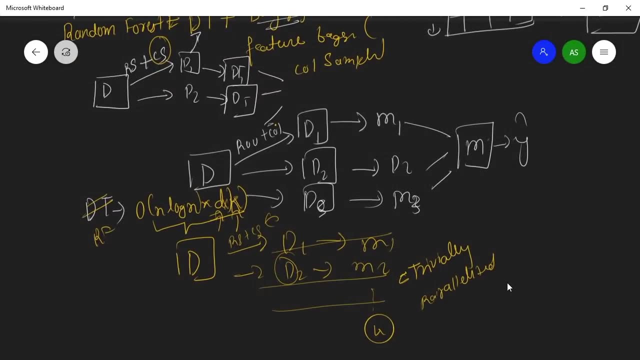 And I hope that we have talked a lot and saw the span of time, And I hope that you're enjoying this video or section also, And I hope that you are enjoying a lot. Okay, So there is one more concept that I will talk on and end this video, which is: 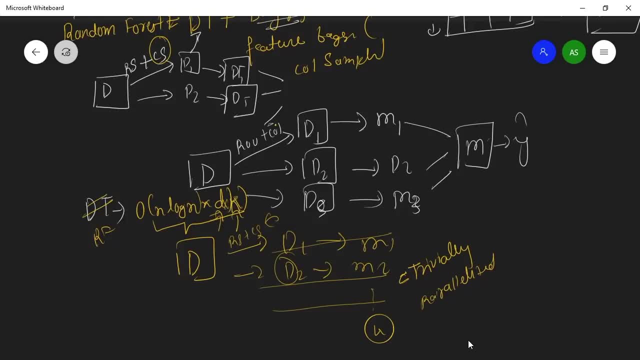 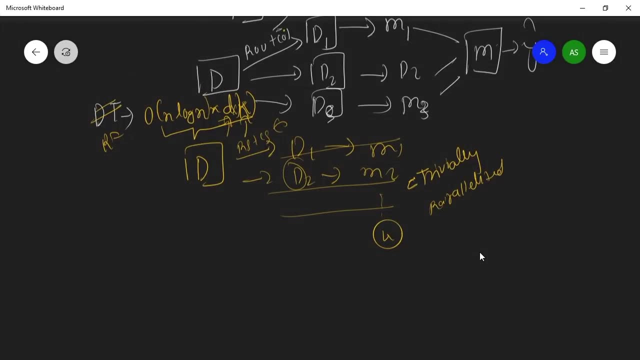 or this section which is important. It's called an extremely randomized trees- okay, Extremely randomized trees. So what we do with extremely randomized trees is they become popular after the cycle then releases its, this API, which is something called extremely, extremely randomized, randomized trees- okay, trees. 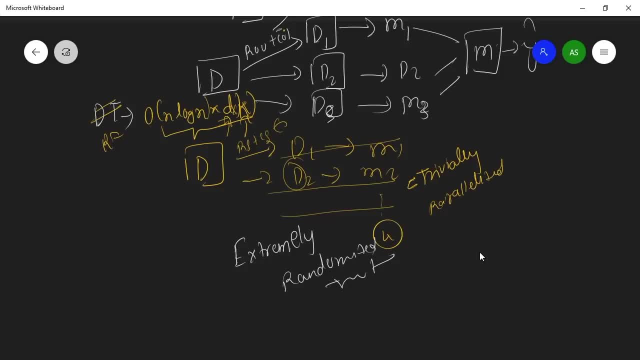 So what is this? This is in random forest. In random forest, we are doing column sampling plus row sampling, with bagging- okay, with bootstrap aggregation, with bootstrap aggregation, which is bagging, okay. So in random forest and RF, we are doing like this: 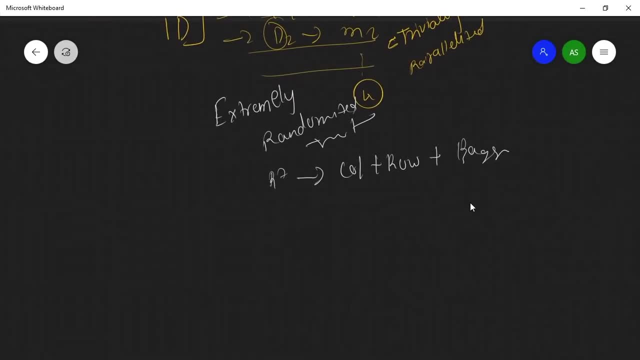 So in extreme trees, in extreme trees we try out the possible values of FI to determine the threshold means the decision trees and decision trees. let's take an example that in decision trees we have we have some epsilon and its checks is greater than or equals, like that. 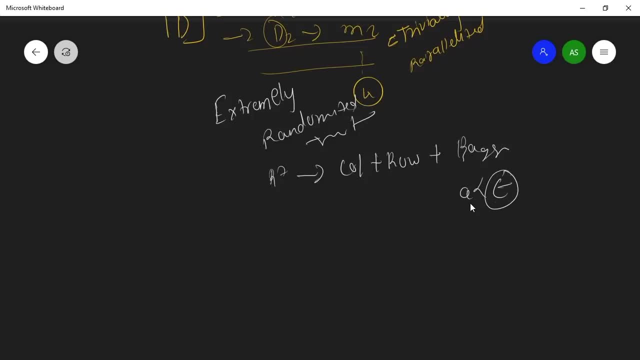 For identifying in decision tree. we are trying out every value and that is that is time. that is that is taking time. that is taking time, okay, So what we can do: instead of trying out every values, we sample. we sample some subset of column. 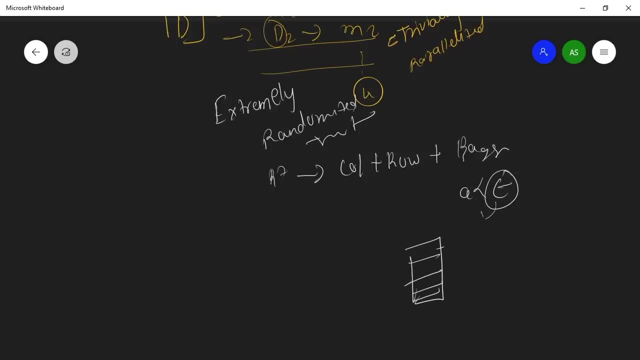 some subset of rows, some subset of rows, and check with that and choose the threshold according to that, because in random forest we have a lot of decision trees and identifying the threshold is a key over there. okay, So if you, if you take all possible values, then in that will be computationally time, complex, time taking. 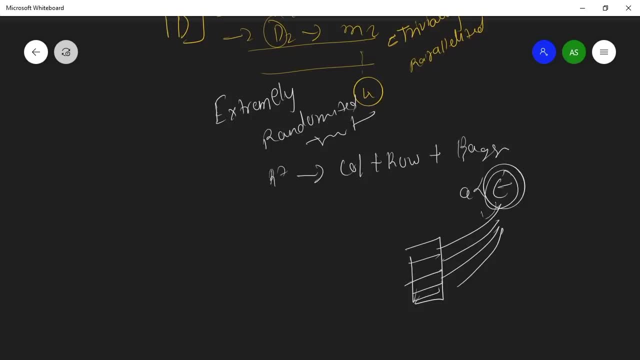 So what you do? you try out the sample of values from that whole column, okay? So then you try, and that's called the extremely randomized trees, okay, So that's what I want to talk about: extremely randomized trees. Just to make sure that we are on the same page. that what, what we were doing in random forest. 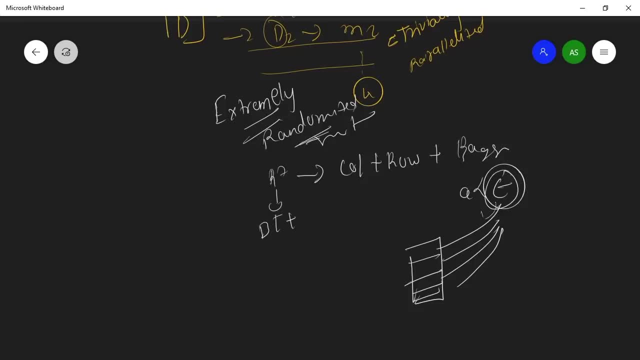 we have a lot. we have decision trees, we have column and row sampling- okay, Okay, and that reduces the variance, okay, So here in random forest we are trying out every in random forest, we have decision trees. 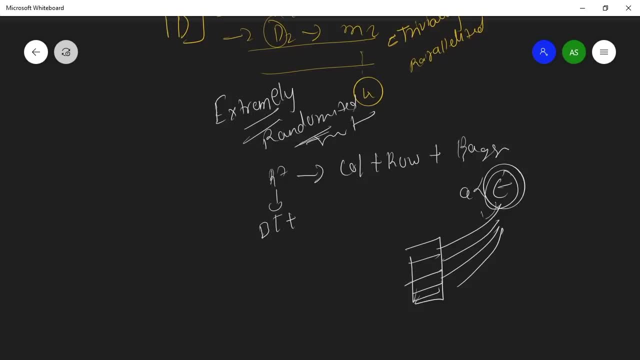 and we are trying out every possible values and we are for for that epsilon, So for, not for, for it's time time taking. So what we do, we take out the sample of values from that column and as a as a sample. 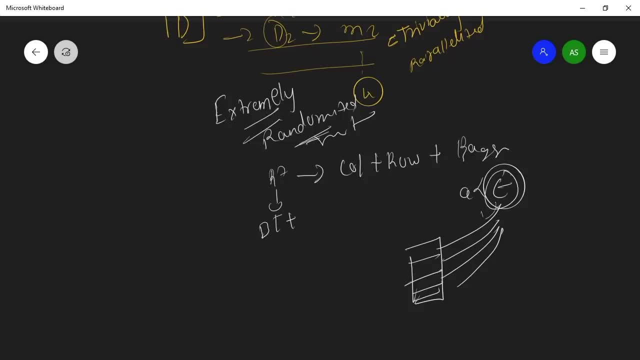 and then we check that for that epsilon to for getting that epsilon, okay. So if you're a little bit getting confused, don't worry, it's not a popular, popular algorithm which is extremely randomized classifier or regressor. it is not a popular algorithm. 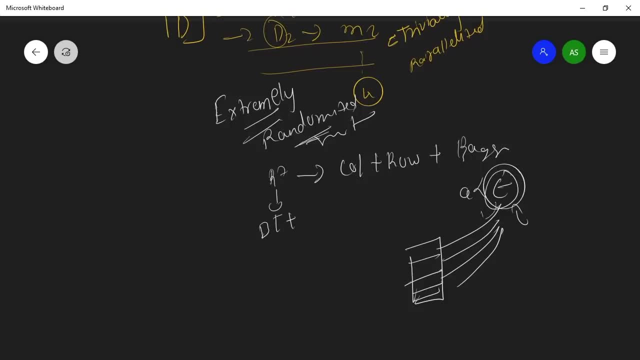 The reason being: if you take out a sample, there is lot more less chance that your model is good as compared to random forest. So we we rarely use- I rarely use- this extremely randomized forest. This is popular. I heard of this as a popular lab, popular algorithm. okay. 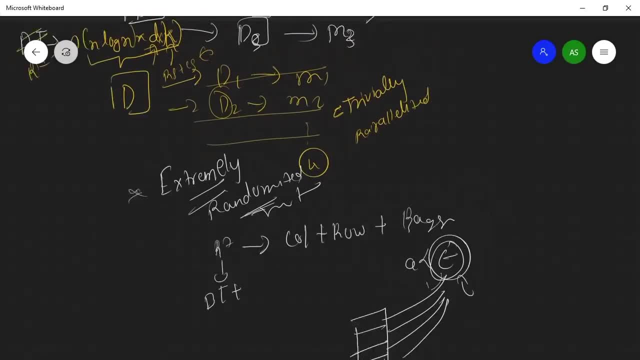 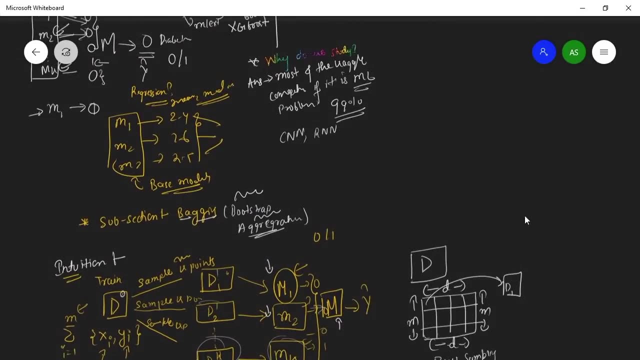 So we have talked a lot. I think that we have talked a lot on to this. Now we hope that you understood bagging, then we have understood random, random forest, then we have understood some decision tree and then we have understood the ensemble learning. 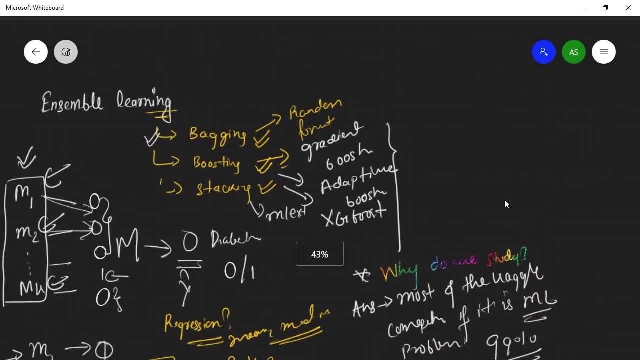 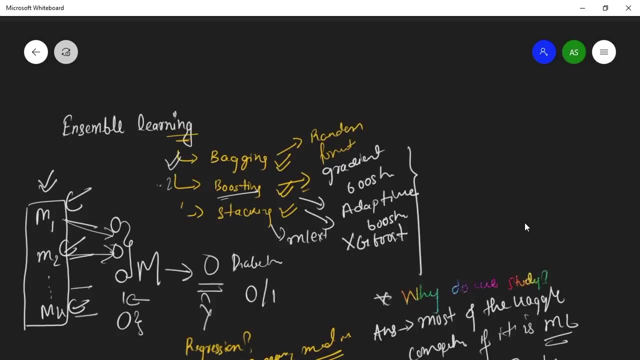 Now we have talked about bagging. okay. Now in the next section, subsection Point, a point to it will talk about boosting. Okay, and boosting will talk with the radian Adaptive XG. Okay, so we will talk about three algorithms. here We have talked about a random forest and extremely randomized, as 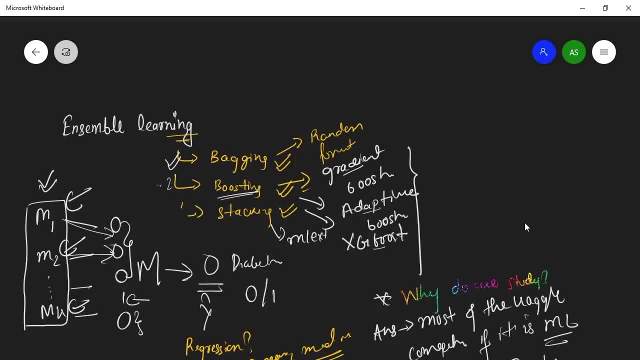 trees. so in there we'll talk about three, which is gradient adaptive and XG boost, and a gradient boosting is also called G b b t. g b b t is gradient boosting decision trees, Because they also use decision tree as their base models, only to century as a base models. 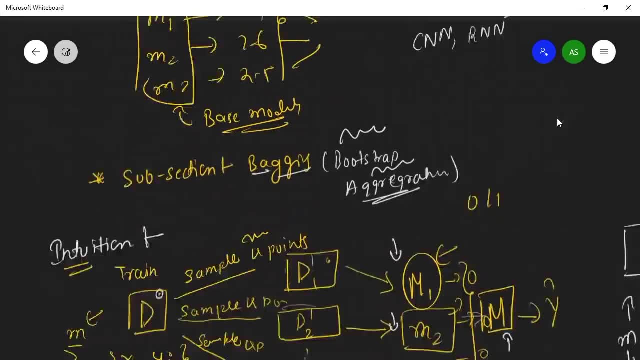 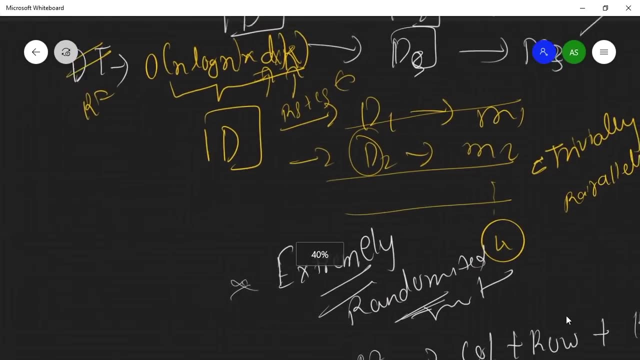 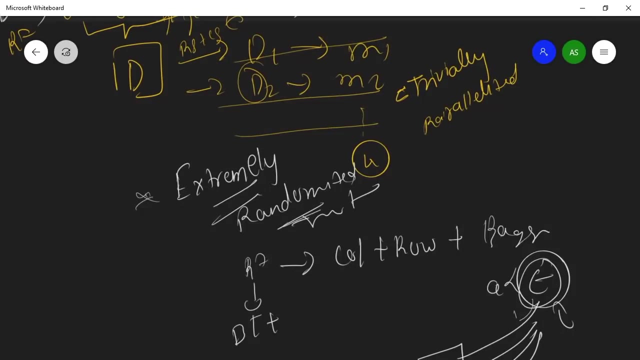 But what are the some of the disadvantages of random forest, The some of the disadvantages of random forest? that it is a very you, it is very. It is very bad choice to use, to use a random forest or decision trees on large data set. Okay, If you don't. 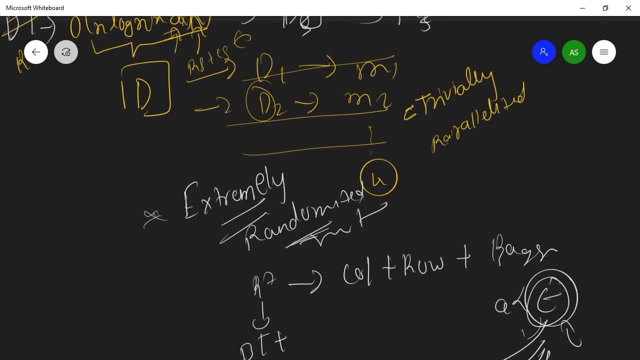 Because it's very time, complexity and taking. okay, we don't use it that kind of, but you can obviously try it out At least. okay, you can see some more assumption on the internet for this. Okay, great. So now we have talked about everything. now It's time for getting into the implementation. part of random forests. 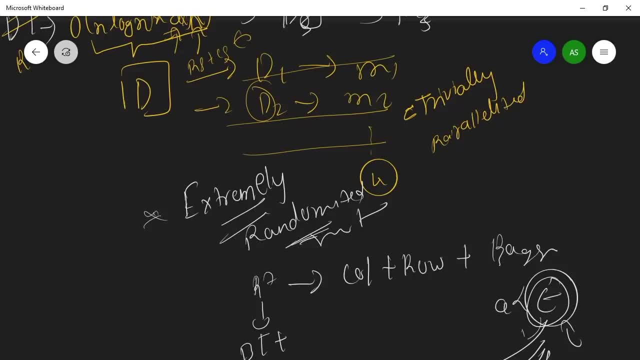 Okay, we will talk about random forests and decision trees. Okay, either way, I think that we have talked about decision trees, So I will talk about a random forest. Okay, on, I can learn it in a library, Okay, so let's, let's see the implementation. 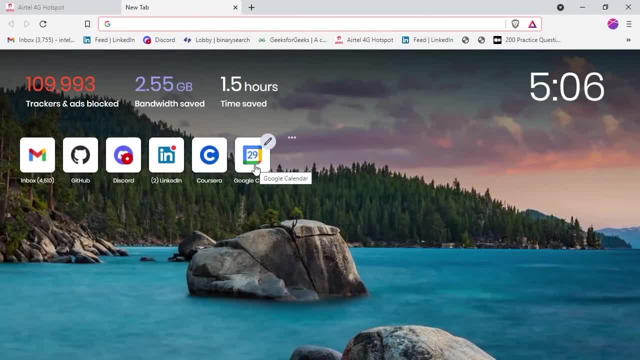 Okay, so I'm on my brief, okay. so here I will write. I will started using brave in some just just a days ago, Just some some days ago. So here what I will, what I will write, I will write a random forest, random forest. 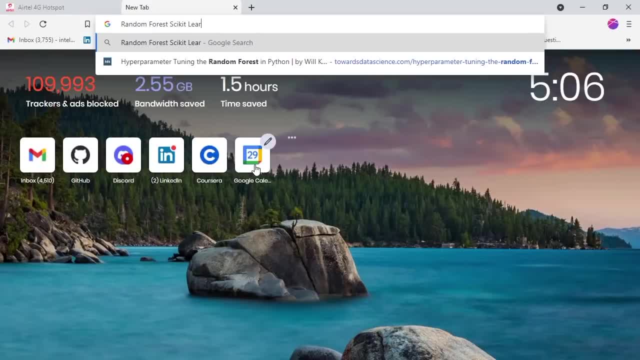 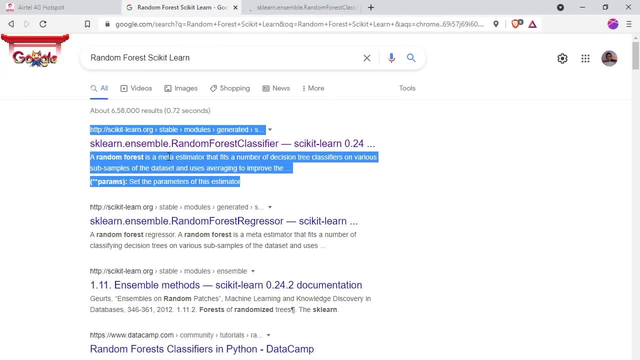 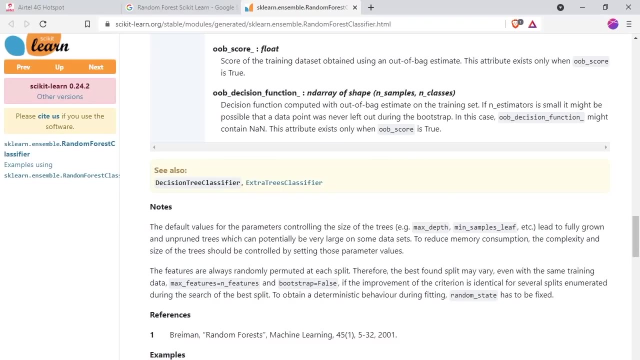 I'm citing that, Okay, Okay, and we will see one project. we will see one project which will be doing all of this Implementation with grid search, TV, fine-tuning the hyper parameters. Okay, so let's, let's deep dive into this, Let's under understand this concept. 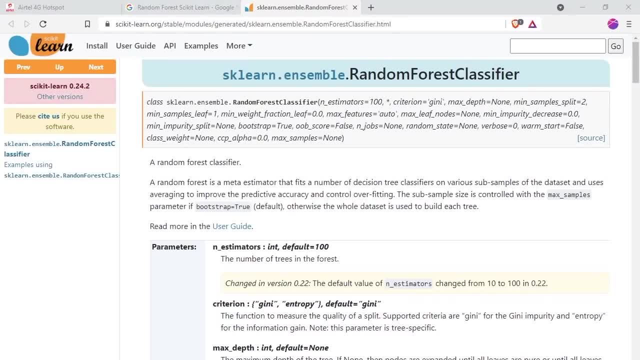 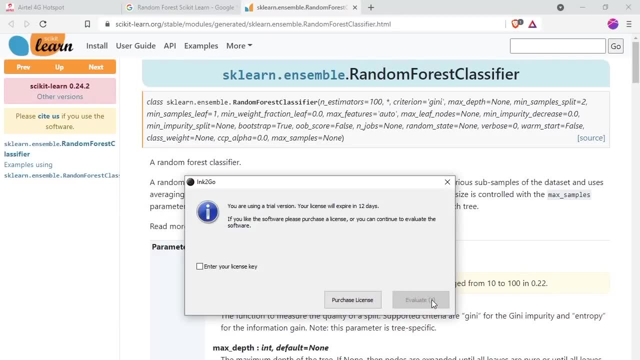 Let's see the implementation. a very finest explanation of a random forest earlier. So let me take out my ink to go again, because I it's my 12 days left, I'll do that. license expires Okay. so here I will take my pen, I will take medium. 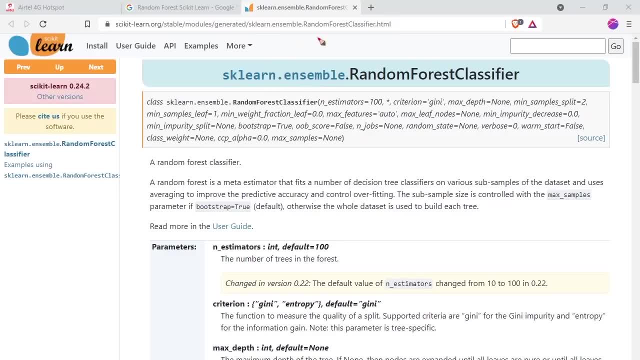 I will take a good red color. Yeah, so you can go to this API which is SK learn ensemble. You can also import by just calling: from SK, learn from SK, learn dot ensemble. from SK, learn dot ensemble. you can go with this and then you can. 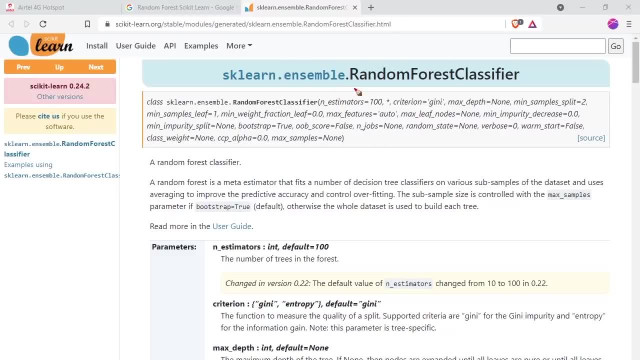 Use this API. So the first, You know you can use the random forest classifier, this. So first parameter is n- estimators. the first parameter is n estimators, and estimators is the Number of a decision trees that you want. Okay, like then, what is the number of a base models that you want? 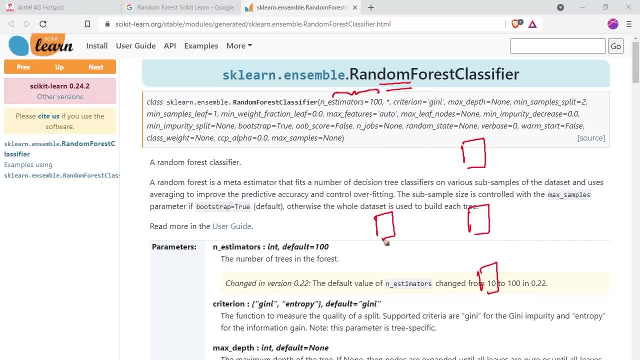 What is the number of a base models that you want? So you have this data and you take this sample, this data. So what is the number of? so you so here usually unread decision tree as a default, okay, But also this is a very important type of parameter, so you fine-tune it using a grid search CV. 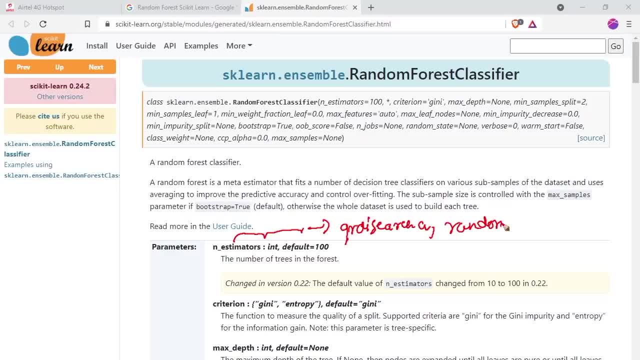 Or randomized search. okay, we will see its implementation of these two. Okay, so you can use. this is the number of addition trees After you have. what is the criteria? What is the criteria to use in our decision tree? What is the attribute selection? 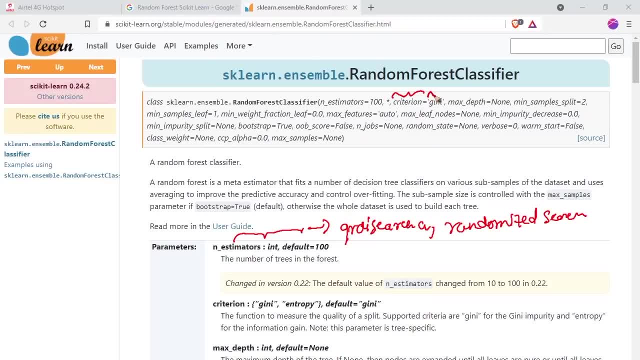 So the default is gain impurity as the best impurity. either you can use entropic, But it's computation a little bit expensive, is a time time taking. Okay, you can use. the default is gain impurity is now the: what is the number of the depth of your tree, the minimum number of a sample required to split and 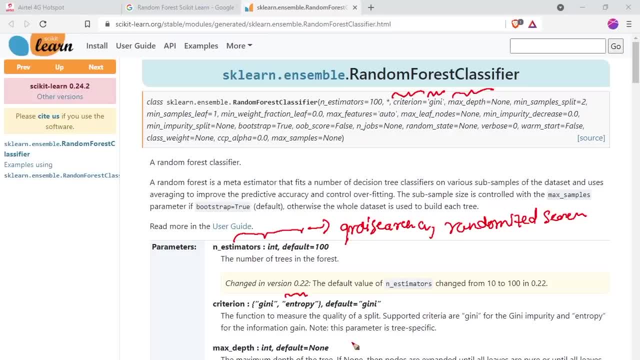 Sorry, the maximum depth of the tree to stop. Okay, then the nodes will expand means if it is none, then it will. It has a high chance that will. it will over set. Okay, Now it is also hyper parameter. minimum sample is split with number of a samples required to split an internal node. means: 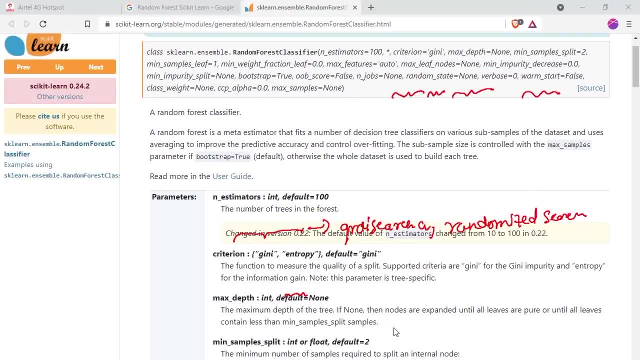 What is the minimum number of the samples to split? Okay, samples means what is the number of data points? Okay, then you have. let me delete this again. then you have, Then you have minimum sample of leaf, which is which we have already seen. Max features means what is that? 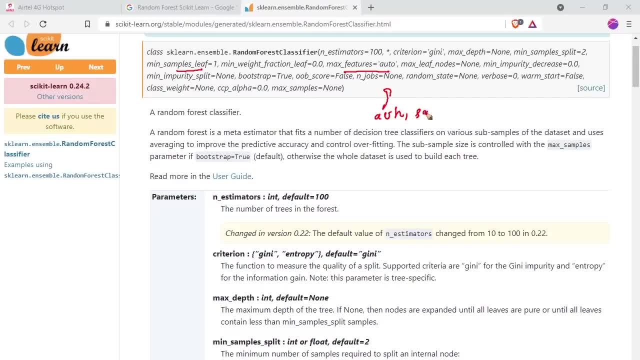 You want auto or a square root or log. you can read the documentation. impurity, then a bootstrap. bootstrap obviously equals to true. It's in both bagging where the row sampling with a column sampling OB score which is out of bag, data points, which is out of the bag after sampling. 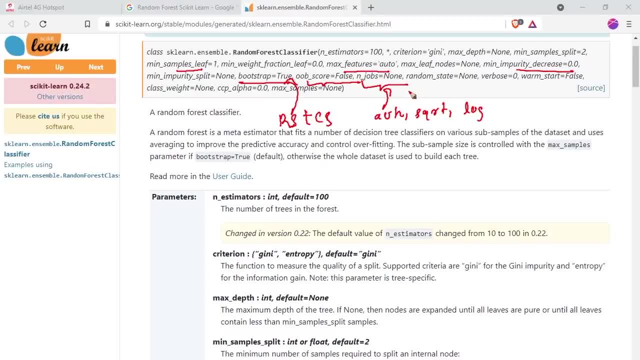 Okay, which is for n jobs. if you take this, n jobs equals to minus 1. if you take this n jobs equals to minus 1, Then it will obviously understand your course and then it will run parallelly. Okay, it will run this into parallel. It is fast. if you take n jobs equals to minus 1. usually people take okay. 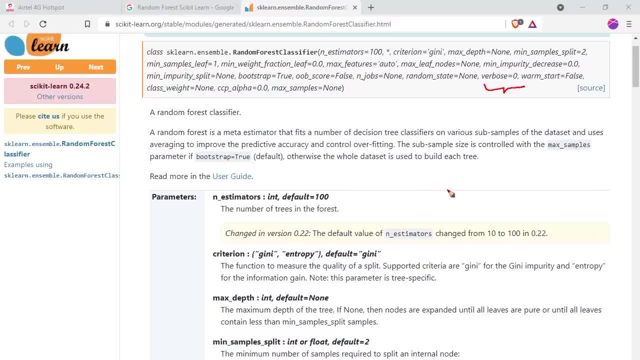 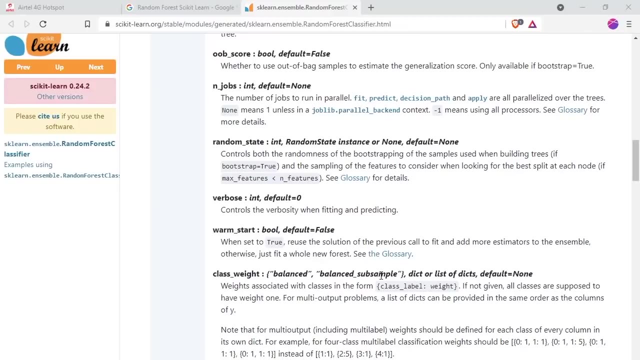 But of course it's. I think it's it's for printing out something texts. Okay, now you can see the class paid. Let me see about also far written about class weight. Let me see class weight is: Yeah, verbosity when filling and predicting class weight is just. 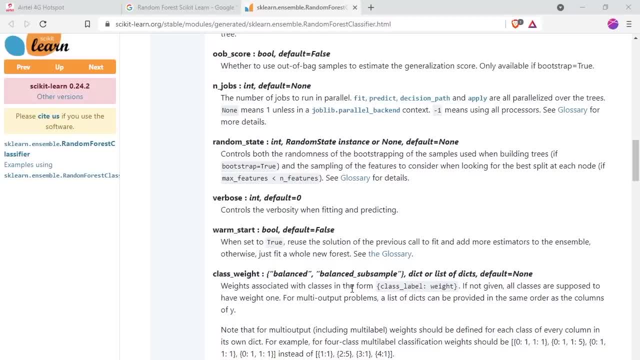 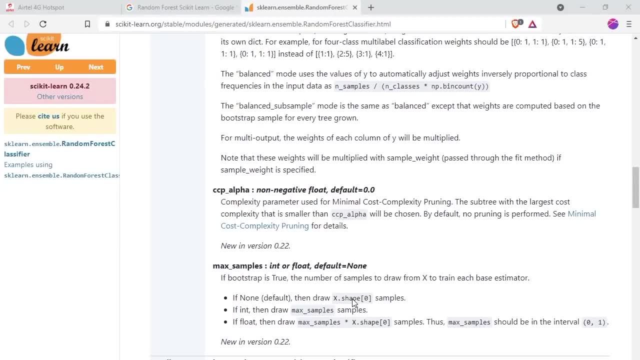 The weight associated with the class. okay, So it is obviously in the default is a none, but you can see how it is calculated. Okay, it's not max samples. it bootstrap equals to true. What is the number of a max sample if you set it in a none? 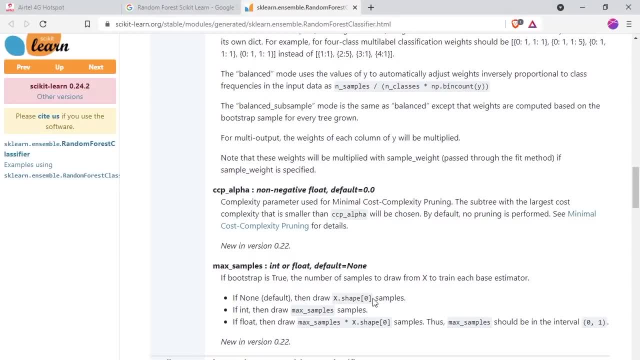 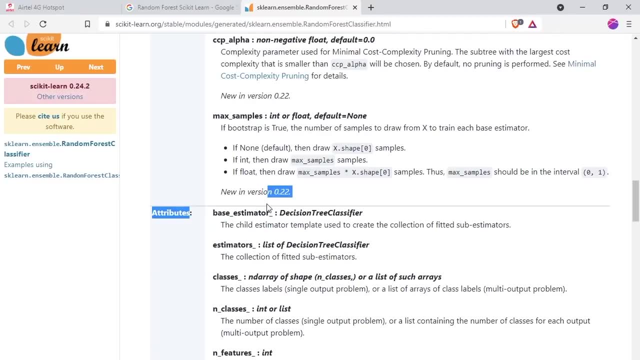 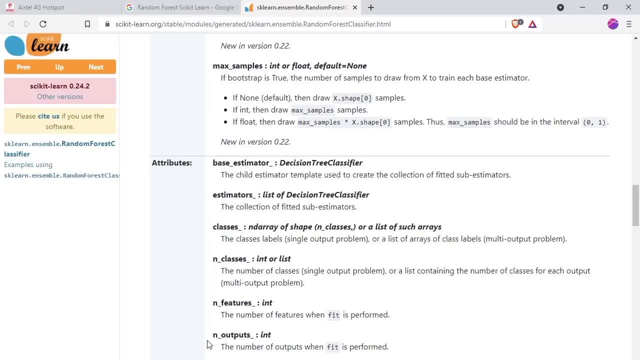 Then the default is the X dot shape is 0. the number of the samples, so you can set some max samples. Okay, So you have some attributes: base estimator, the child template used to create the collection of finished sub estimators. Then you have a number of our classes here: number of features, the number of fit, number of outputs when it fit is performed. 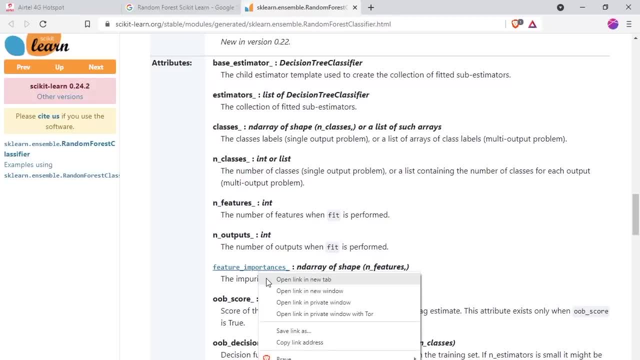 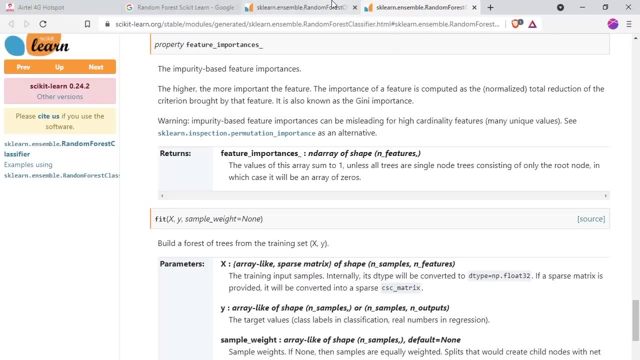 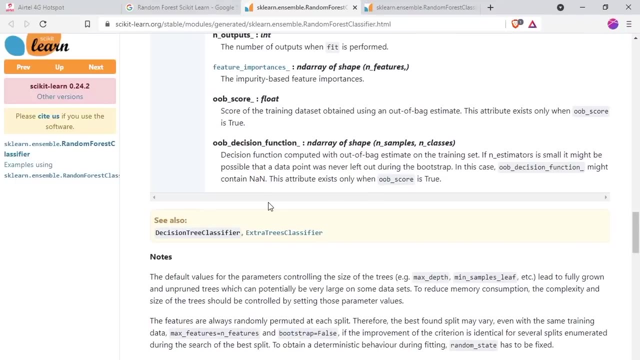 The feature importance it is. also, you can use feature importance, this attribute, to Understand what is the number of feature means. What is the importance of your each feature in your model? is columns or we score? if it's, obviously it will give you the in A float value. Okay, so that's the decision tree. Sorry, random forest, and you can see more about this. 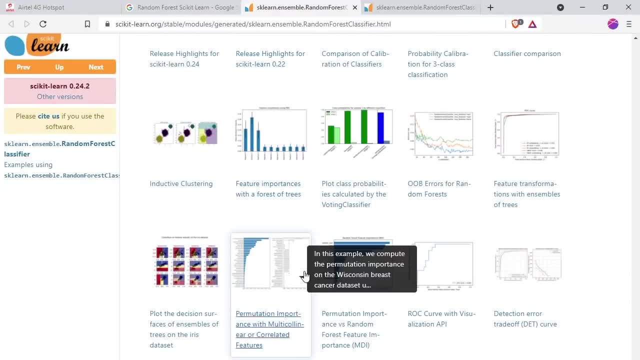 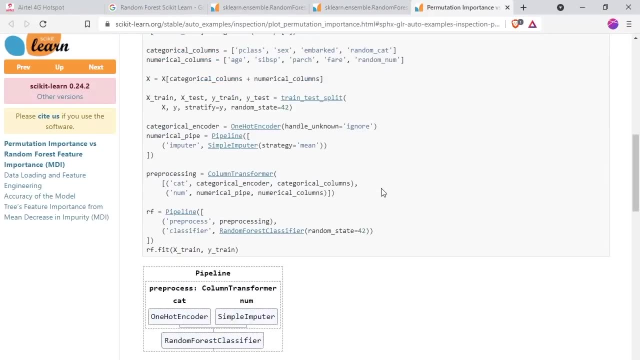 and to hear and you can really read about attributes and this is how the, this is how the Featured importance looks like. and see, you can also plot it like this. You can also plot it to so which feature? and you can use it for feature selection. Okay, great. 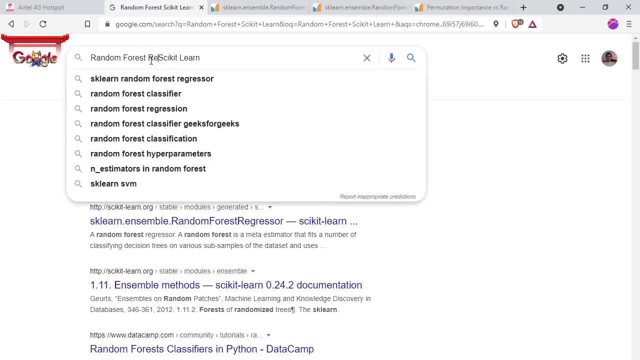 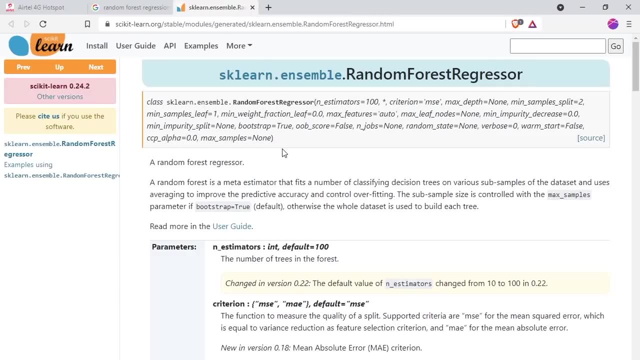 Let's see. The second one is a random forest, the regressor. Let me see. yeah, then I am under the same. Okay, So let's see again. It's very similar to classifier. It's very similar to classifier Here. here we have an estimator, which is number. let me- oops, I don't know why it is very. here we have number of estimators. criteria to be: MSE, RMSE, MAE. okay. max step. max step, minimum sample width: bootstrap equals to true. obviously. take this. take this, okay. OB score equals to false. you can take yes or no, okay. 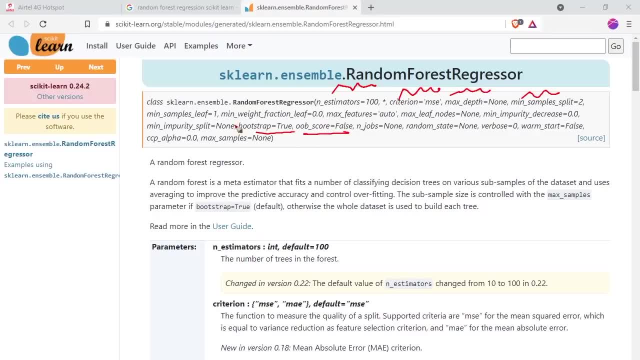 Summer default to get. it is quite similar to that And max sample is none and it sticks a default as x dot. I don't know, I don't know why it happened. Max, that is x dot shape, the shape of your, okay, of your samples, okay. So that's the basic intuition behind this, and max, the max samples, also won't have a grammar. 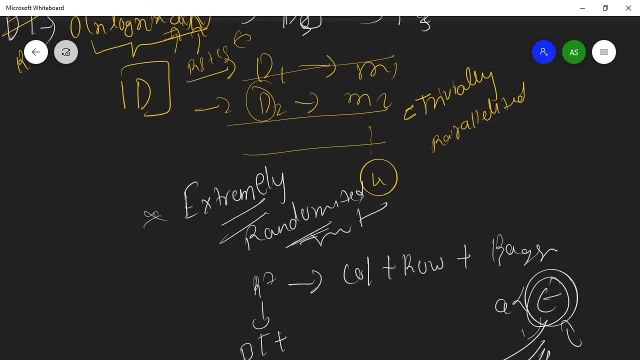 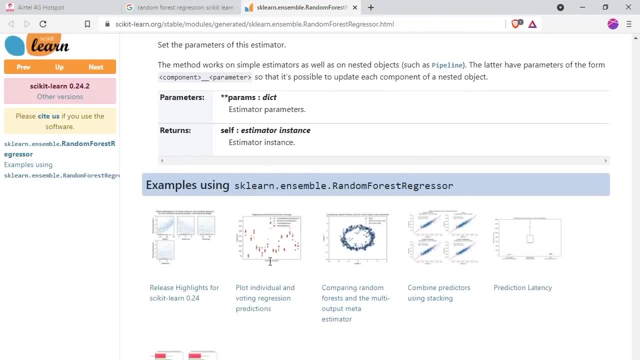 Great. So we have talked about a lot about bagging and we have spent one hour on to this. Now you can see Some more attributes. You can see some more attributes over here. You understand it much better, So let me show you uh one, uh one diagram that I found very interesting. 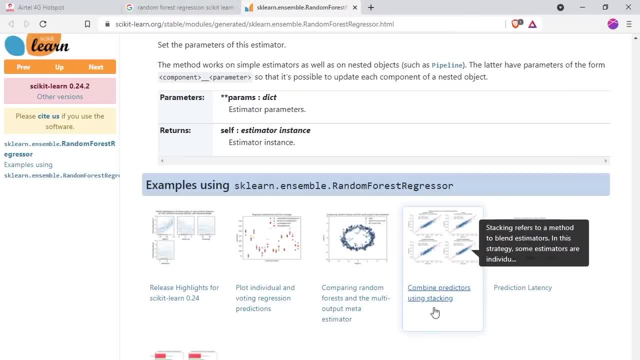 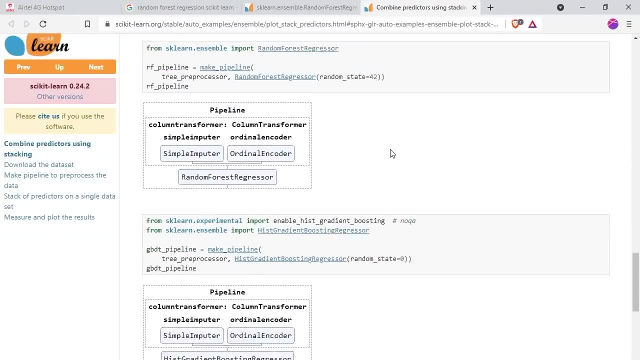 Okay, So you can see on some examples using random, for this regret regressor: uh, using a stacking, So you will also see the stacking. Okay, Stacking is also a very good technique as a gag winner- We're winning- winning technique to use. 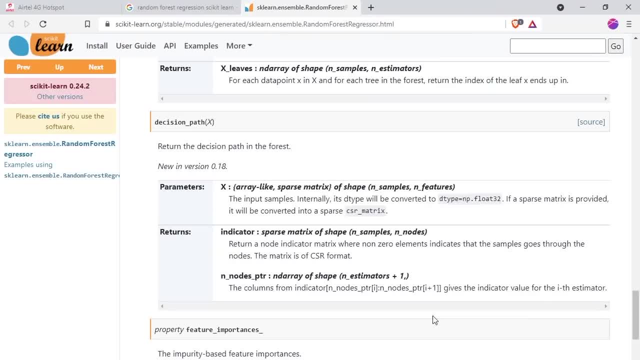 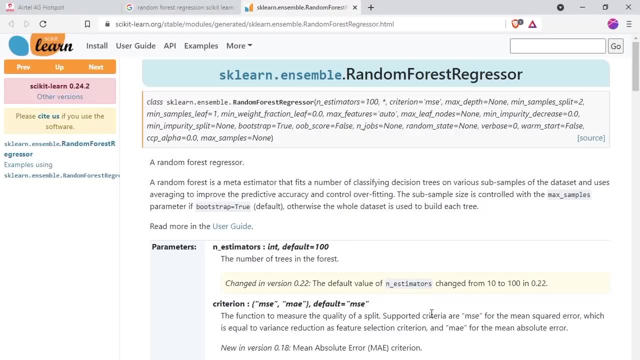 Okay, But um, here you are. Okay. here you can see that we only have MSE, we don't have RMSE. okay, so RMSE is not default. you have to make your own function for RMSE, just squaring the root, your MSE. 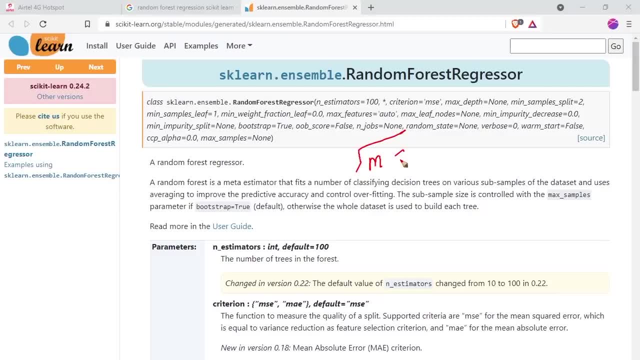 okay, but you cannot use. if you want here your RMSE, okay, you have to make your own. you have to make your own. I don't know why it is not running well, I have to complain. this, okay, I think this okay. so for RMSE. 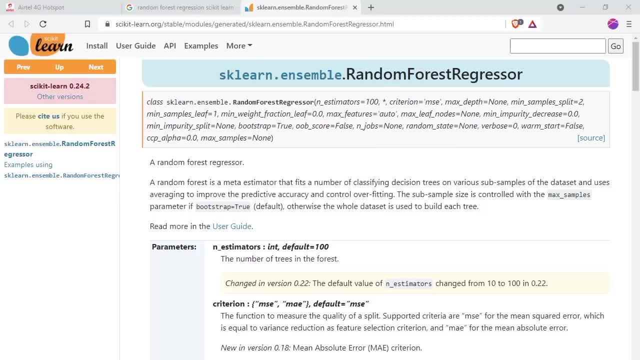 you have to make your own, okay, but here you cannot use the discovery either you can make a pull request, or on cycle or in APM, okay, just adding your own RMSE, okay, great. so now we have seen these algorithms. now we have seen. yes, I will do it. 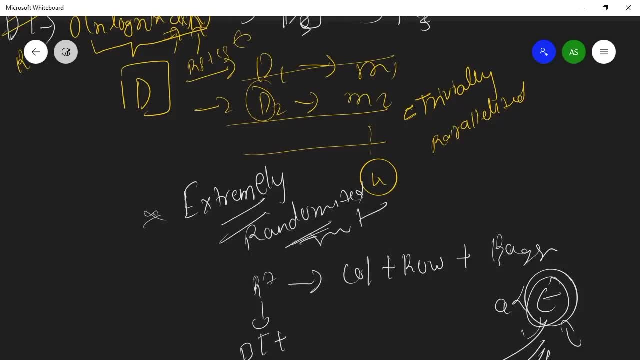 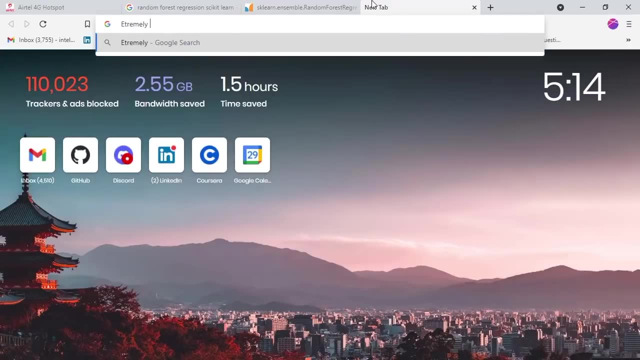 so now we have seen extremely random- there is one more left which is extremely randomized trees. I just forgot- extremely randomized classifiers. okay, so we have. we have a new release. it is called a cyclr. it is obviously in cyclr because it is a new release of cyclr. 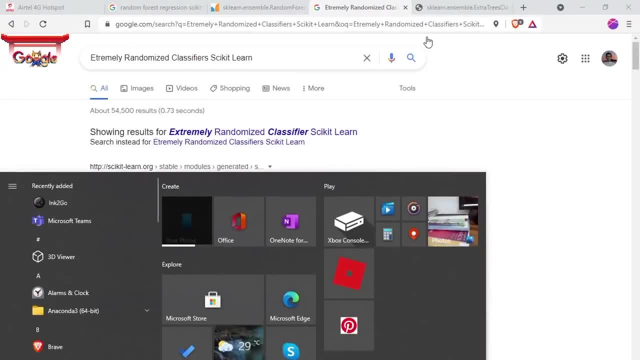 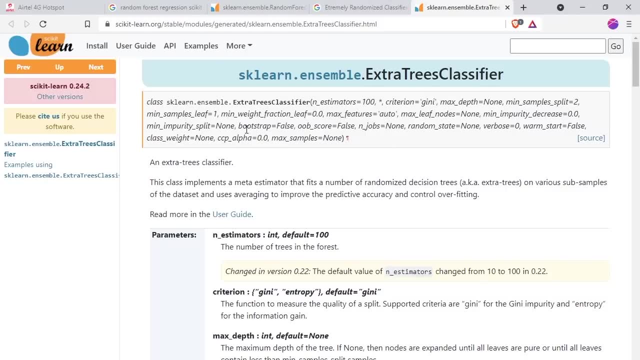 let's see this. let me open it again: integral. it is very important now. so here again, we have MST meters criteria, max depth is just the same. and then we have bootstrap equals to false. here, bootstrap equals to false. it should be true. you can make this. 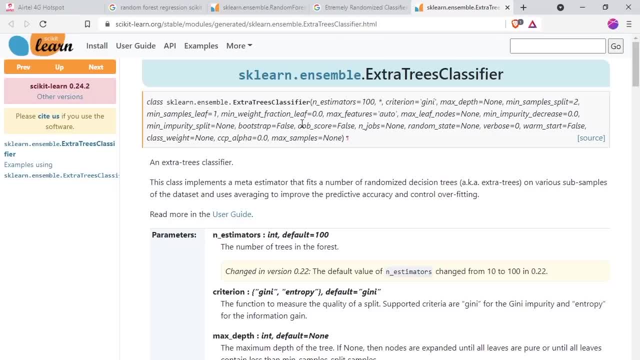 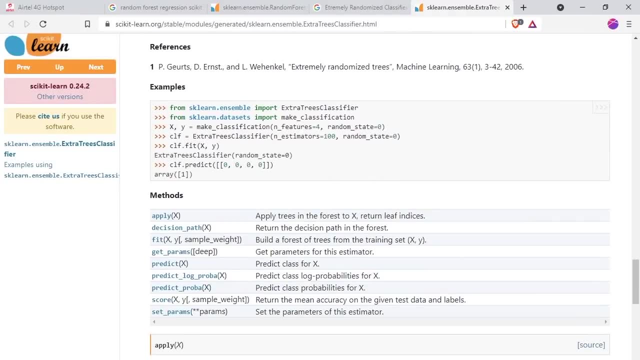 as a true. okay, then we have some more odd to square root, etc. you can, it is just the same as that. but there is some difference, and it is that I've just told you that we choose a. randomly what, what we do, we choose a. 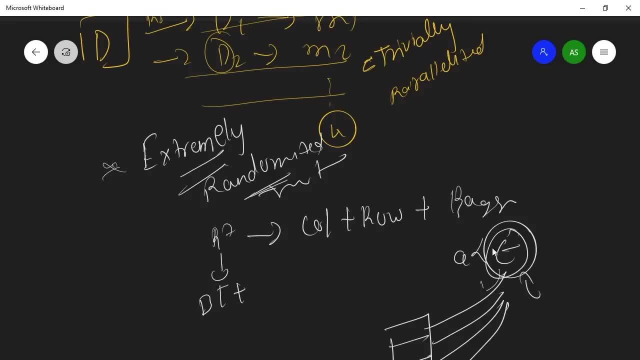 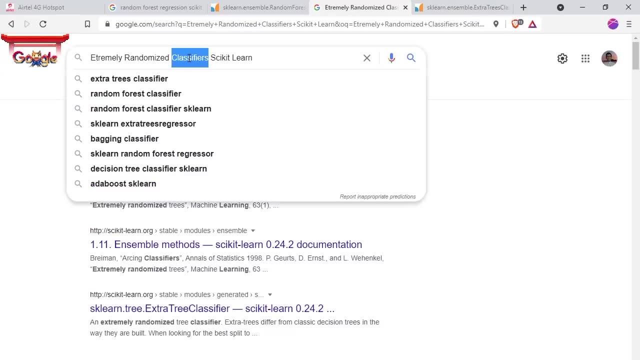 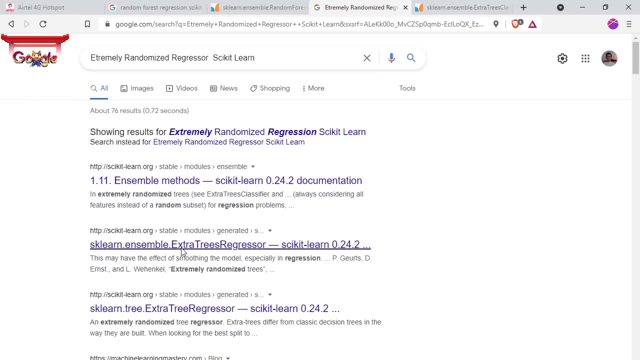 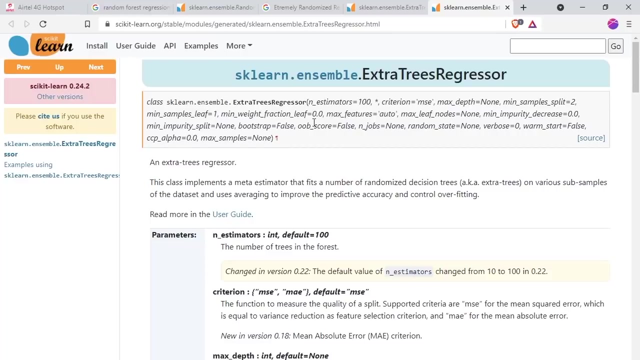 randomly, sorry, a sample, and then we take out the sample epsilon. okay, so that's what we do in a random forest or extremely randomized classifier. so let's see, for regressor and regressor is just the same. I think that I'm not correct over here. okay, let's see regressor and here the same thing over as we are. 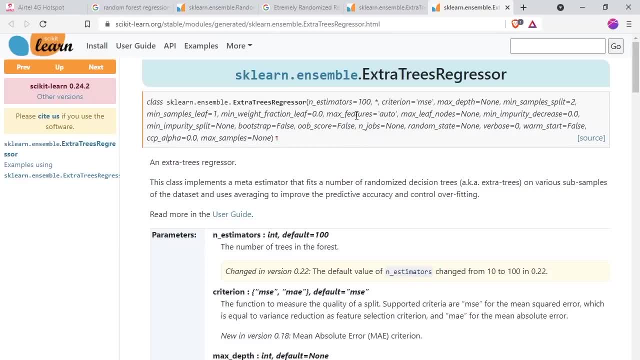 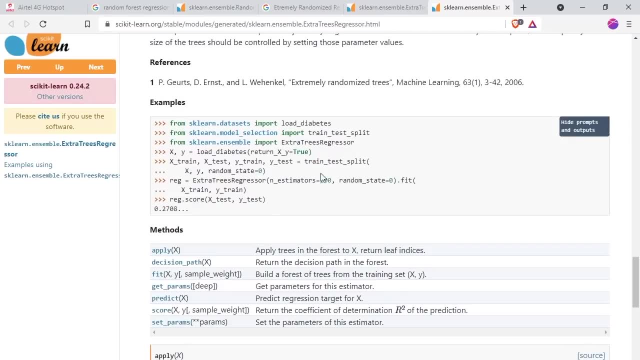 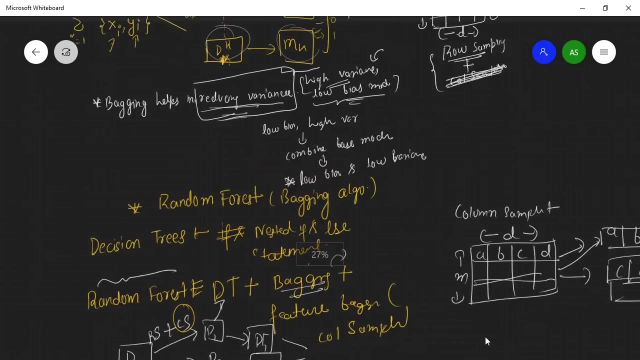 saying- and here bootstrap equals to false- you add jobs, it stops that. you understood to run previously paralyzed to create that option. okay, great. so now we have seen about a random forest and I hope that you understood everything here. okay, so now in the next subsection we will talk about boosting. now I hope that. 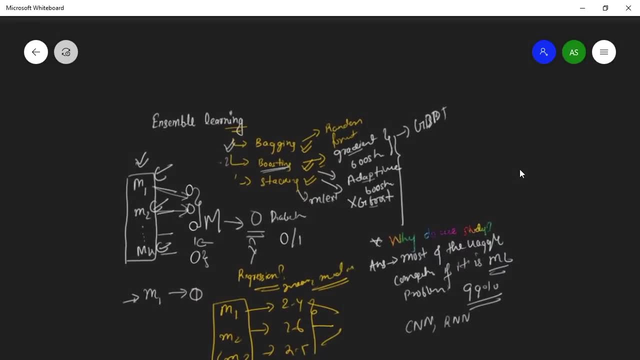 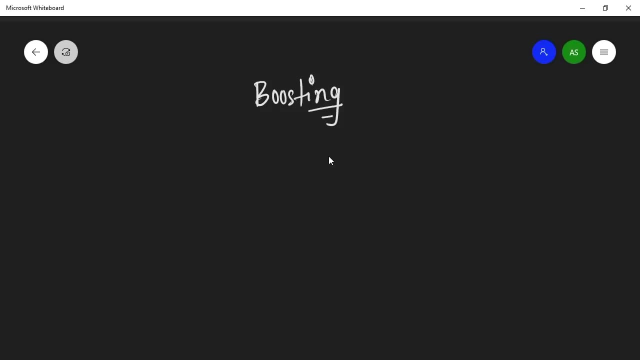 you will understand that also. okay, so let's meet at the next section. till then, bye-bye. okay, so now we will talk about another ensemble technique, which is boosting. okay, so boosting is one of the- again, one of the most popular as bagging. that we have already talked. 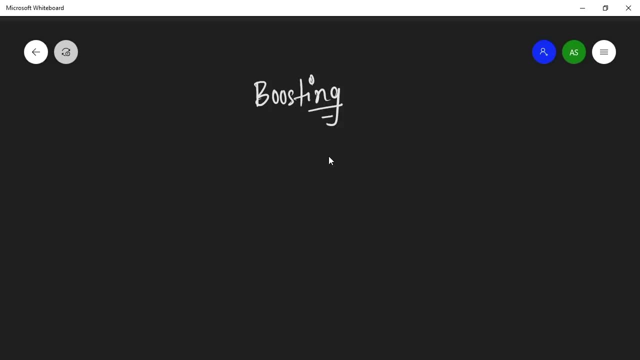 about bagging. just have a recap to late, something about bagging that is necessary, okay, so we have talked about bagging and now we will talk about boosting, which is one of the technique of ensemble learning, and I really hope that you will enjoy this section and 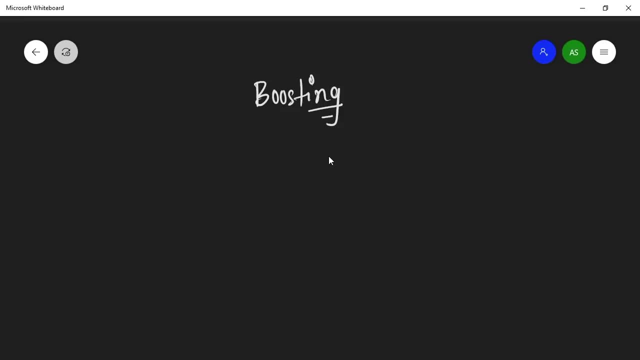 you will enjoy this section and I will see you in the next section, bye-bye. boosting you will talk about, and boosting. you'll talk about something called as a gradient boosting and gradient boosting, and then I will just give you a geometry intuition or I will just show you the 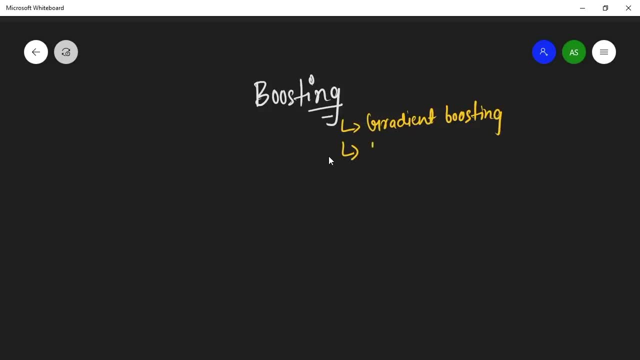 implementation of hard-to true boosting, which is often called a start at boost. okay, then I will talk about extreme boosting: egg G boost. okay. so these three algorithms means exit you to work fast, and some cases X, T boost and B trend in six positive怪 names means X G jotos work fast. in some cases X G doesn't work if you 중에, if you combine all three algorithms for installation: наг력. 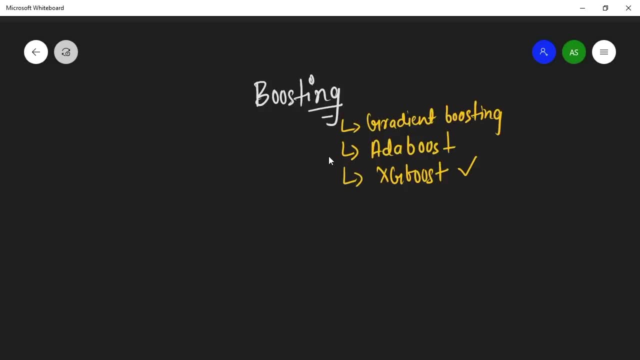 Boost works best. okay, so Gradient Boosting also works best, but I am, it is also works best. so we will see these three. okay, so let's start with this tutorial, but before that, I just want to tell you that you can do the problem set, which is on github, and you can subscribe the YouTube channel just by going to the. 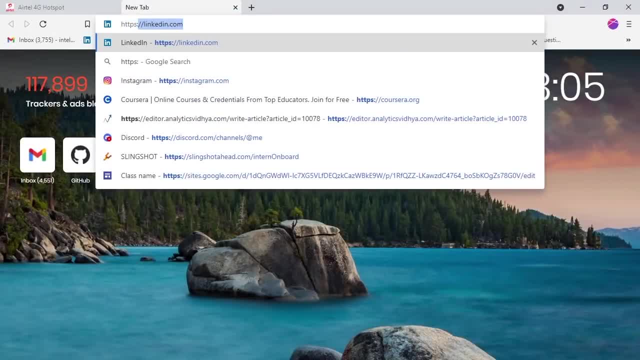 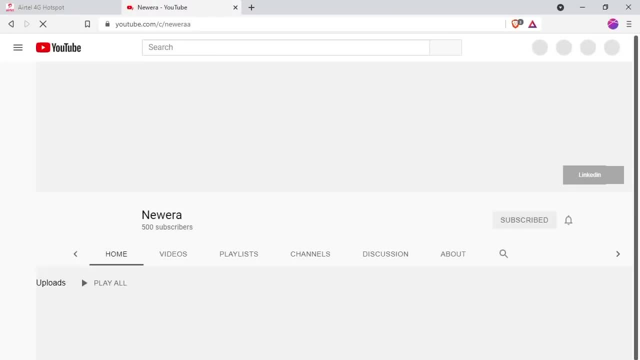 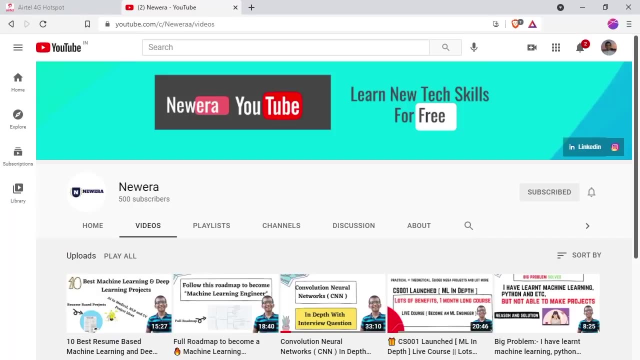 HTTPS, HTTPS, slash on youtubecom, slash- see slash. new era, because this highly motivates me to make content like this for you all, for absolutely free. okay, so you can go to this new era to subscribe this YouTube channel. it's 500, just just. I have a 500 subscribers soon putting a deep learning tutorial. there's. 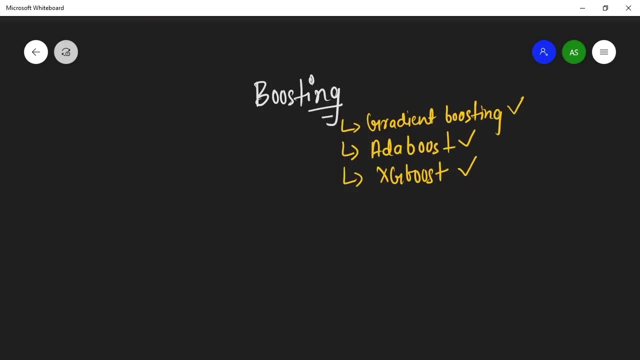 announcements coming up soon: putting a deep learning tutorial soon. okay, so let's start with this tutorial. and okay, so what is what a mobile system is? and this is reports, not that we already talked about. you can would. we was found a bind section of he won and maybe in a 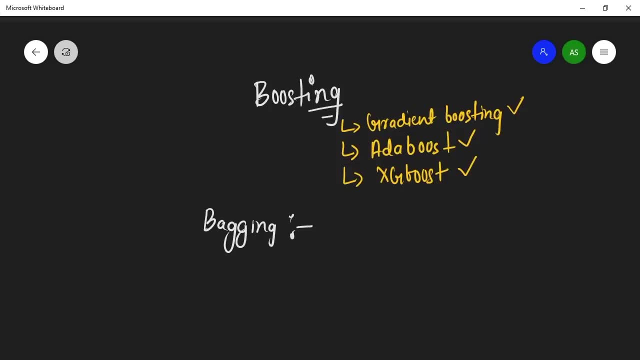 faster way. so banging and bagging. we have no bias model, we have low bias models and 여기는 high variance models. okay, so our base model usually have little small lo los, bias and high of variance. high variance means our base models usually have this low bias and high variance and using bagging. 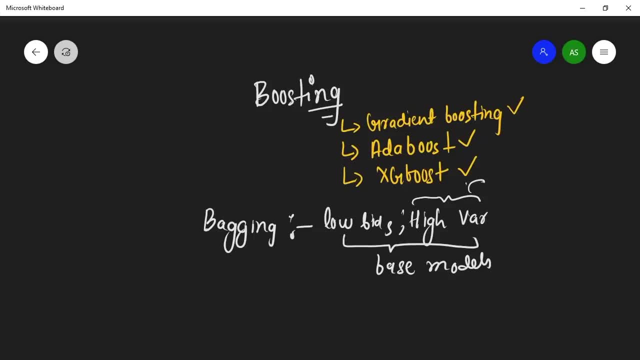 we reduce this, we reduce high variance, we reduce this variance. okay, so our output will be: after applying bagging, we have our low bias and low variance model: low bias and low variance model. okay, so what? what we were doing in bagging you? we are just simply doing the column sampling. 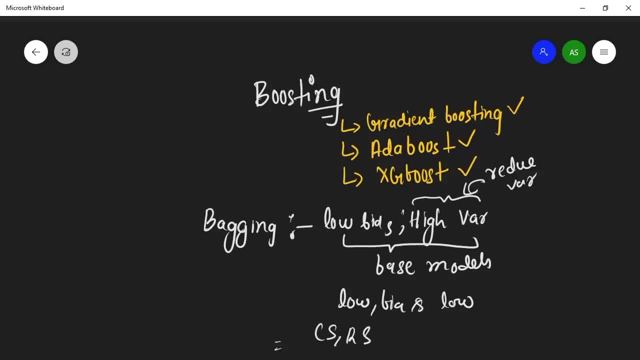 as well as the row sampling means we are doing the column sampling as well as the row sampling in case of random forest, but it just just take an example of random forest and then we do the aggregation. okay, so that's what we are doing and let's see, um, let's see, uh, just, just, uh, just a recap what we do. 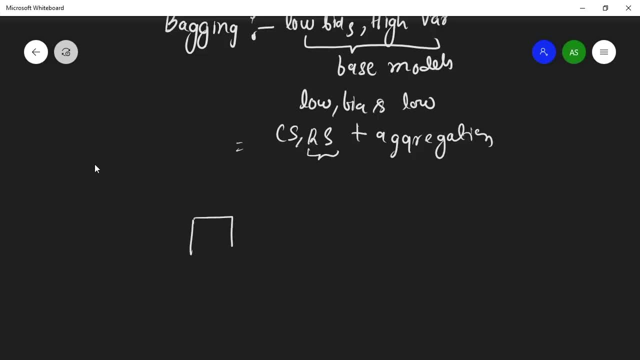 we have this large data set, we have this large data set D and and then what we do? we simply divide this data set into subset of the data with the replacement. so I hope that you remember what is bread replacement, that the data which is here, the data points which is here and it needs to, it needs not to be different. 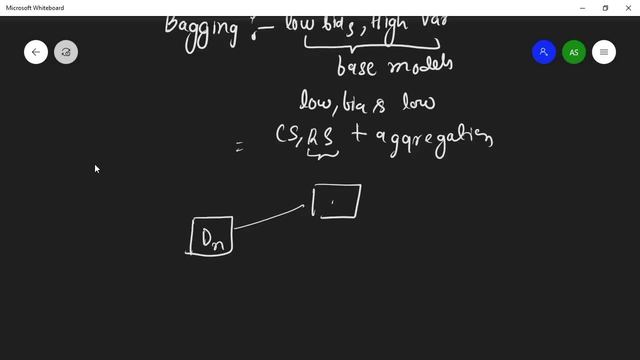 here it can be seen in the second data set also. okay, so you sample them points, then you again sample endpoints with the replacement, then you sample endpoints. so you've taken three subsets of your data and then you train your model. train your model onto this data, like everyone onto this data may be logistic regression. 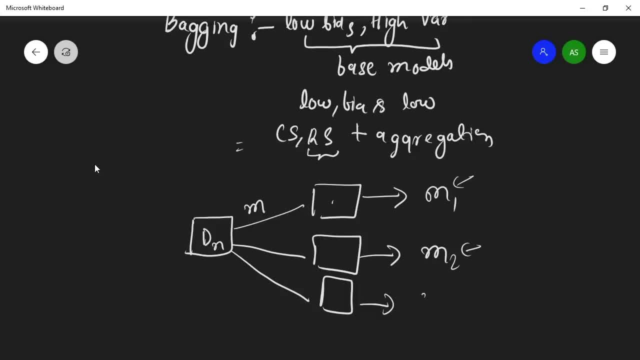 maybe linear regression or maybe support vector machine. so you have them three models, and then if it is a classification problem, you simply take the majority of votes, majority of words, that this particular example is of particular class. or if it is aggression problem, then you do the average. 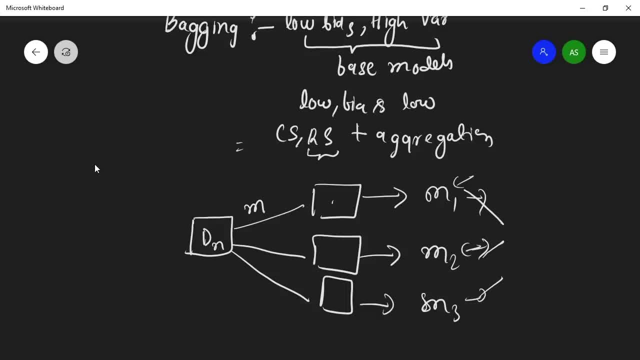 expression, or me, or you take out the mean or a median. okay, uh, in case of regression. so that's what we are doing, and in random forest we- this is these. these are called our base models, and in random forest, we have our base models as a decision trees. we have as a decision trees, okay, so the this usually helps. 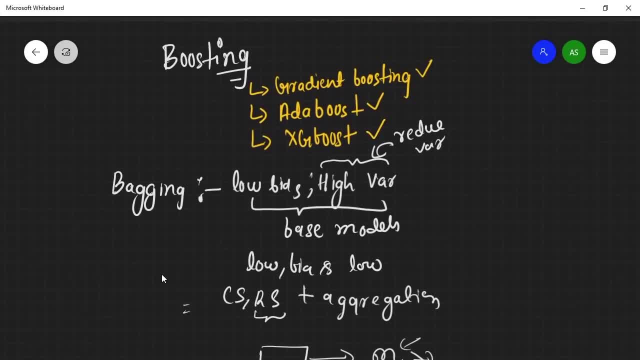 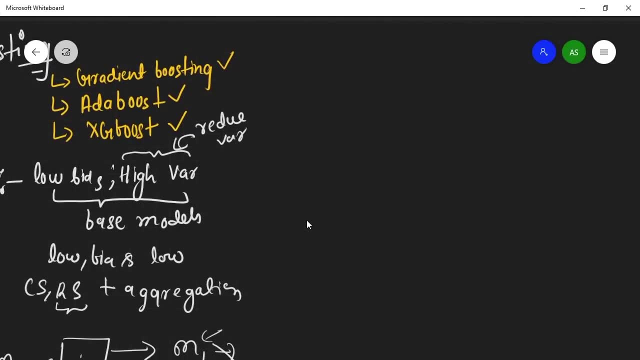 in reducing your bias and reducing your bias. okay, so that's, that's the bagging. so let's see what? what we have in? uh, boosting. boosting is just opposite in case of bias and variance trade-off. so just just now, i think that you know why we have learned bias and variance a lot. 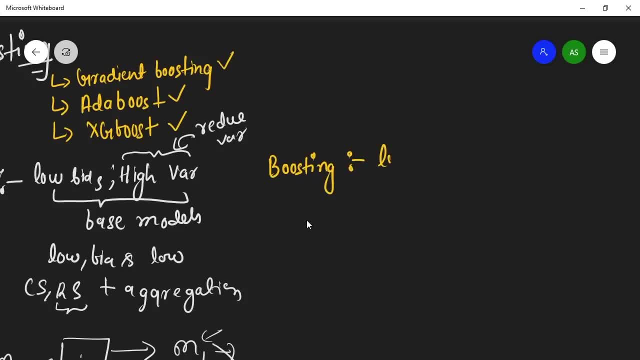 okay. so when boosting, we have low variance in the in. in this case we have high variance, but we have a low variance, high bias model. here we, our model is under fitting. we have high bias model. okay, so it is not performing well on the training set. okay, so here. 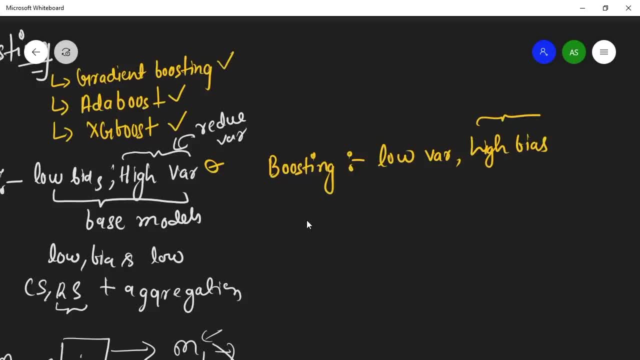 we have a high bias model, and then what we do? we additively combine, additively, additively combine. what do i mean with this? this is a very great uh question. this is: this is what we do, and here in bagging, we are doing the randomization, we are doing the bagging means. 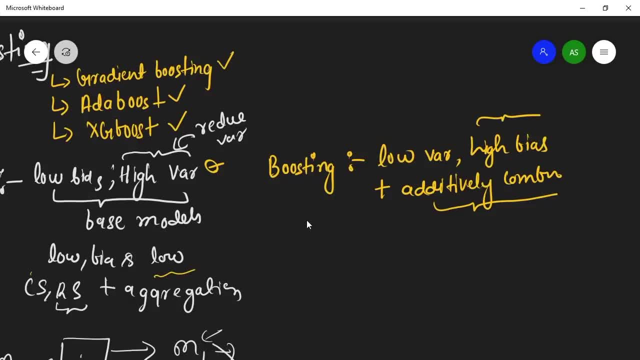 uh column sampling, then row sampling, then we have aggregating the model. okay. but in boosting we have additively combined that. here it combines the weak with, converts the weak, learners, weak models- into a strong model. okay. so different, different weak model- uh tends to be a great. 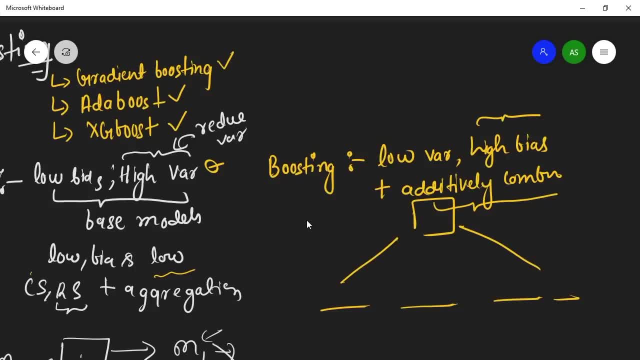 model. okay, just we will see how it tends to be a great model. so it is just combined. so let's see. let's see the core area. so the the basic idea of using boosting is using boosting is to reduce our bias. if you have a hard bias model, then you likely to use boosting to reduce the bias. 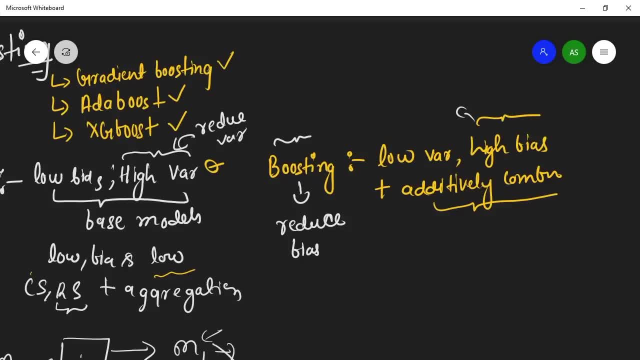 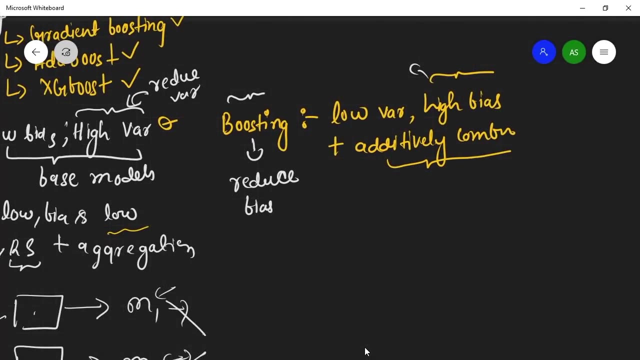 of that model. uh, yeah, there is, uh, some other techniques also that that we have already seen, but it's just we. we use boosting to reduce the bias, okay, so let's see, so let's see the, the, the basic intuition about boosting. so let's take an example that you have your data, you have your. 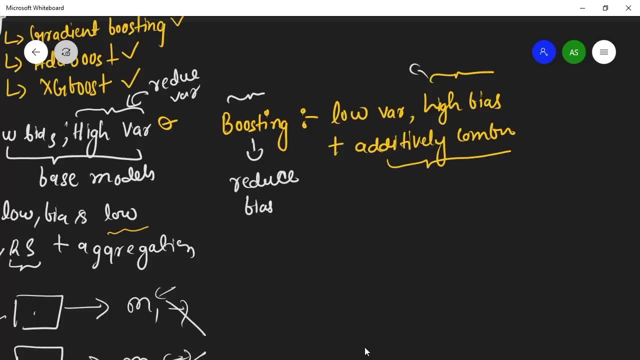 training data. so i'm just writing my training data. uh, where do i write here? you have your training data, which is your uh training data. i'm just writing train d, okay, which is usually. which is this? this is a supervised learning and a supervised learning technique. so you have xi and yi, with which is a label, and this goes: i equals to one or we can. 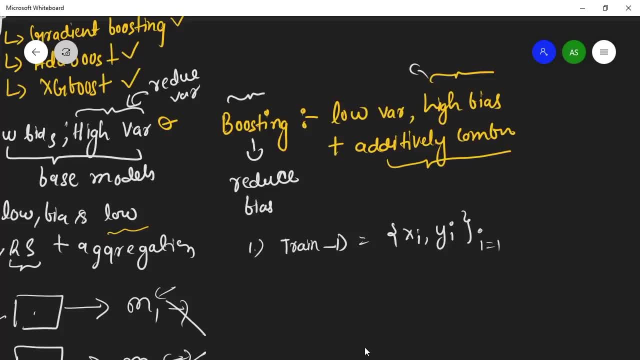 write the i equals to one all the way down to the maybe m. okay, your m is the number of training examples into that, a training data, okay, and then you make a model, and then you make a model, then you make a model at m1. so let's take an example that we have made. 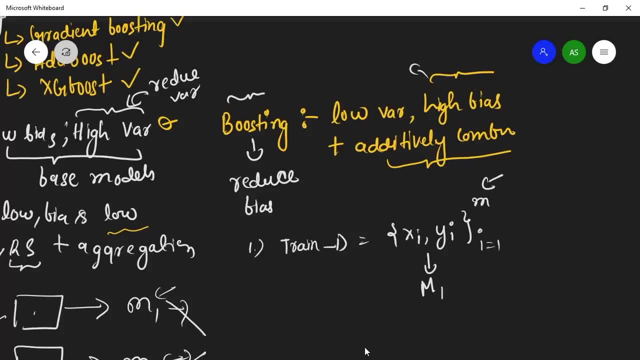 a model m1 that simply, uh, that's simply a function f of, that is simply a function f of x, which is our hypothesis. okay, so now what we will do? uh, this is the. this is the core idea behind boosting. so so we have a training data, you have your training data. like which is your training data? and you. 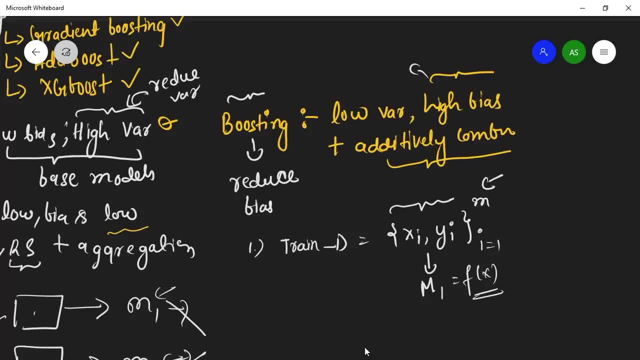 train your m1 model onto that. now, what you have seen. now, what you have seen, you simply take out the error. you simply take out the error means the cost function, the loss, okay, loss for i example. loss for i example. you have y, i, which is a ground truth, which is a ground truth. 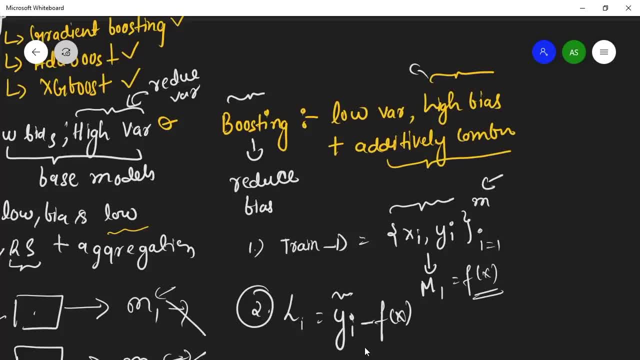 minus your model predicted value, while model predicted value is f of x, which is uh, when, when you input x, then you get your output. so model predicted value is f of x. okay, this will give you the loss. okay, the loss for if it is uh, if it is zero, then it is very good. if it is large, then it. 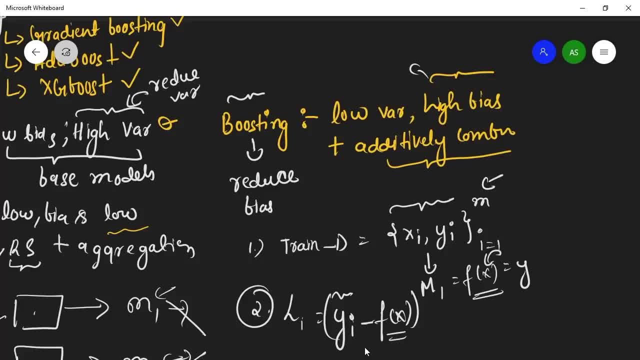 is very bad. okay, so here we are using just a simple regression. loss means just a loss. so if you over here, if you add a submission, i equals to one all the way around to the m, y, i minus f, f of x, then this is the like msc, but you do a square in msc. but now because of the gradient decent to, if 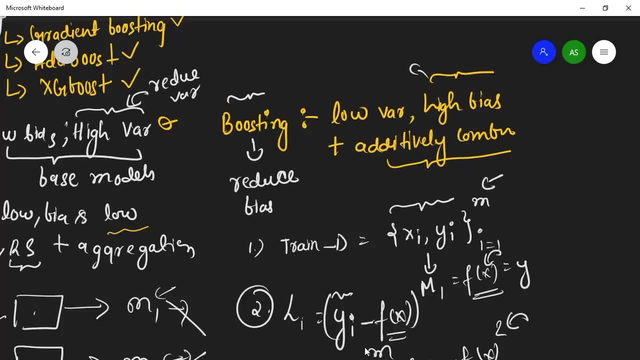 effectively compute the derivative. but here, uh, you can, you can just see, just just as a simple conversation, what we, uh, just just we, are taking the loss for each training example. so here let's take an example that we have take, take, taken a loss, and then what we do. 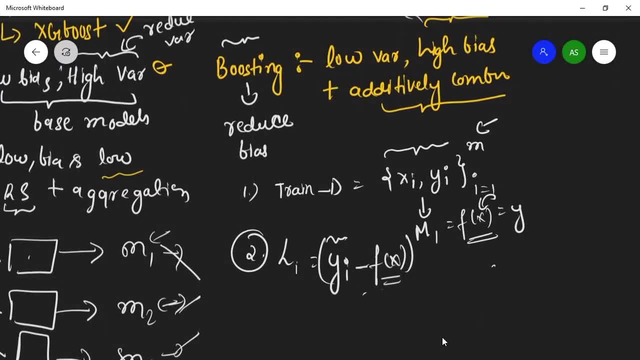 and then what we do? we train our model onto this loss means we train our model to reduce this residual error. to reduce this residual residual error, okay, we only focus, or we we more focus- onto the data which is misclassified or miss uh, which is, which has a very large uh error. okay, so we focus on that. 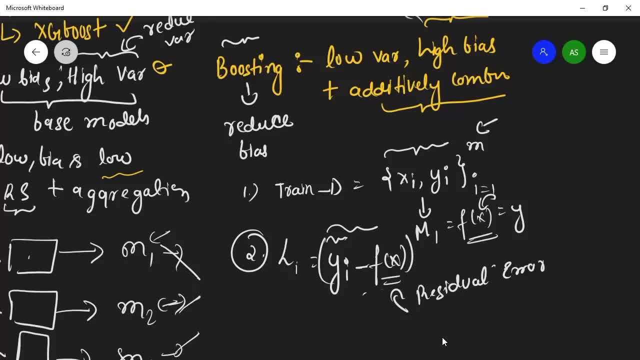 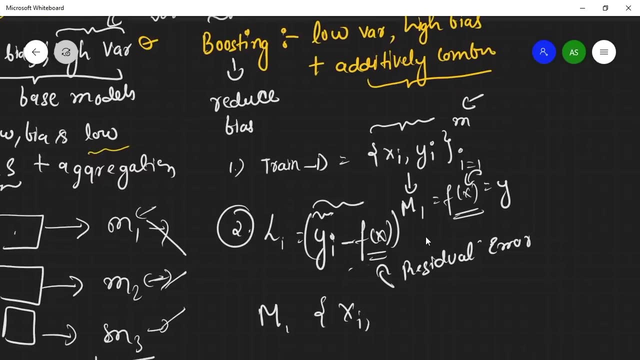 okay, so what you do so for really. so you want to reduce this error. so how you want to reduce, you want to make a model, make a model m, that that and that is given xi means you fit this residual. so let's take an example. i'm just, i'm just going to take, take, take an example to make you this statement clear, that's. 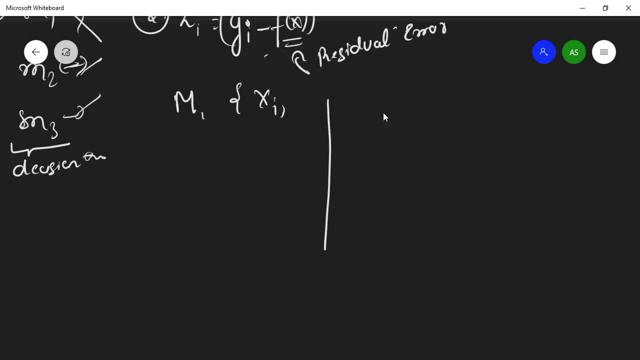 what you do. so let's take an example that you have a regression, uh, problem statement. so you have a regression problem statement. oops, i don't know why i am making a bad. yeah, why my x axis is not working. great, yeah, here is my hex axis, a bad x axis and you have an x like this: 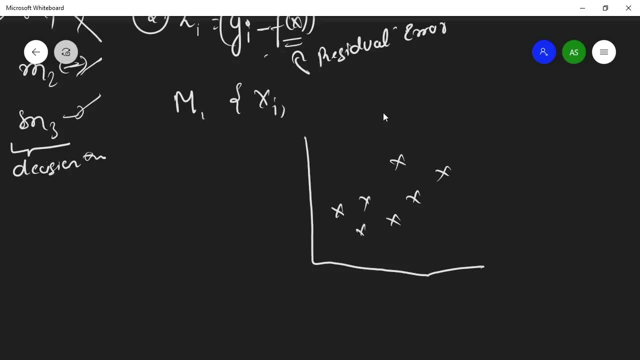 x, like this, and then what you, you have fit in a maybe this line, okay, a straight line. so here, for this train example, the loss will be very high, so it will, uh, more proudly start focusing on that and it fit on that residual covering this, okay, so maybe it will. it will do like this: okay, it will also focus more on the residual. so maybe it will do like this: okay, it will also. 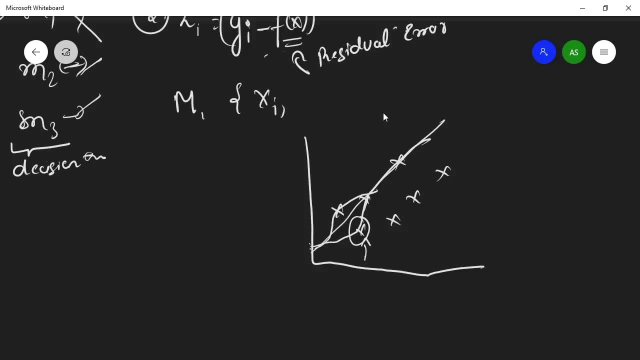 maybe it will do like this- okay, it will also cover this- if the residual is very high. so it's always tries to minimize that residual. maybe it can make a knowledge. either the example is too much a landy, but either it can make a nonlinear decision- sorry, hyperplane. okay, so for so. 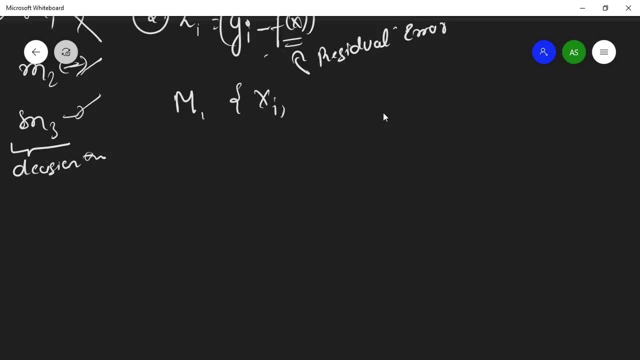 what? what we do? we fit our error, so we make up model m1 that minimizes the error by fitting onto the error. so here is where Li for I equals to 1 all the way around to the M. okay for each. for example, we are fitting a model, okay, so 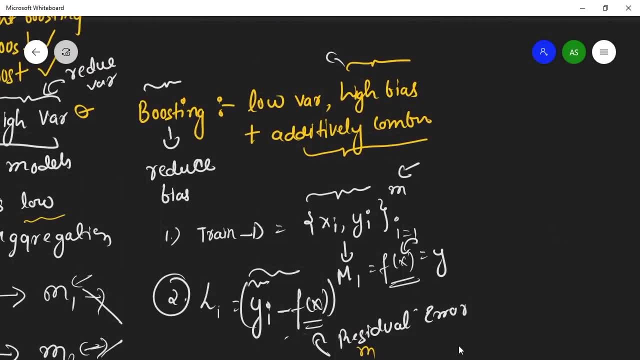 it is more probably focusing on the data which is either misclassified or which has a high, the particular MSC or MAE. okay, if it is a regression problem, then we take MSC or it is, or which is misclassified, so it is more probably focusing on that. okay, so, and that's the basic intuition, so let's, let me, let me. 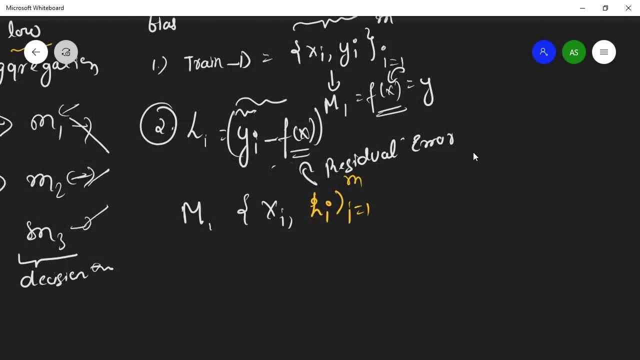 make you the full equation how this looks like. so you have, you have F, F, F, F. you have F of X. F of X with K means and some just just a model. a big, big model means F of X. okay, for each way example, I goes to 0, all the way down to: 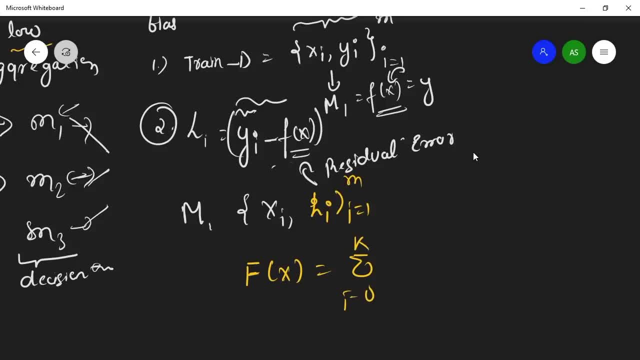 the key. okay, all the way down to the key, you have one alpha. you have an alpha times your moral I tomorrow. so you will not only have one model. you have in first model that fits them, that second model that covers that, that fits, that rest residual. then third model, that first. 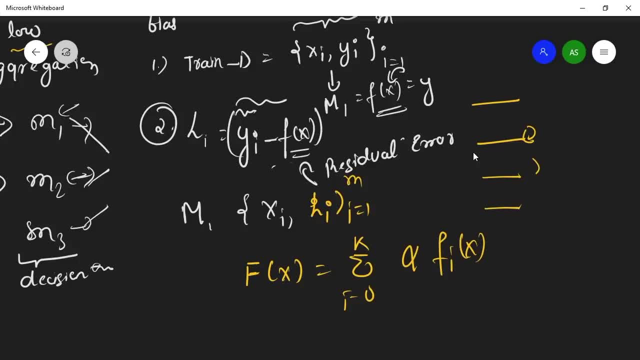 that residual from this model. fourth model: that first, that residual from this model means error. okay, so we have a different, different models. we have a large model, this K, and they go to each and every model with some lab, just as cuz assume it's a lambda. so we have this just just as of now. just consider this. 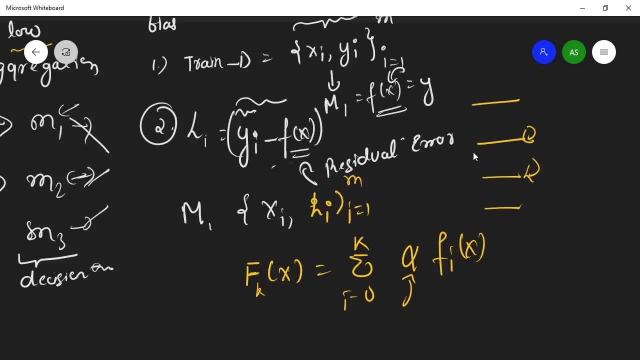 as we have computed it somehow. so we will see how it is computed. okay, we will see when we learn about some gradient boosting. okay, so just assume that we have some cons are just a lambda, a constant. okay, here, this F of I, X, that is, that is trained to fit the residual. train to fit the residual from. 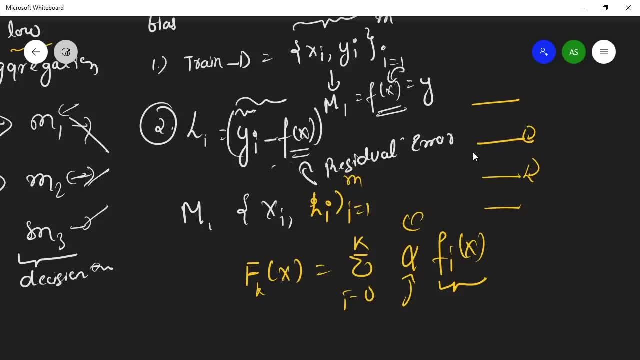 the previous model. okay, from the previous model means this model, this M, to train to fit the error we get on M 1, okay, so this, this model may have some different thing. this, this model, is able to correctly classify the error from the error from this first model. this M 3 is able to classify the errors from the end. 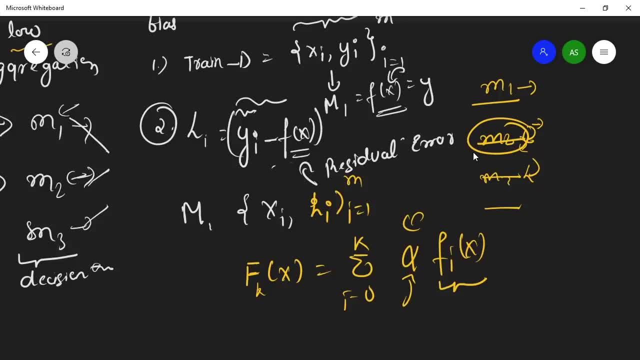 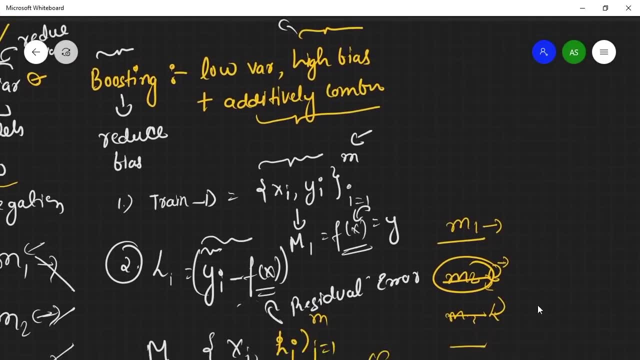 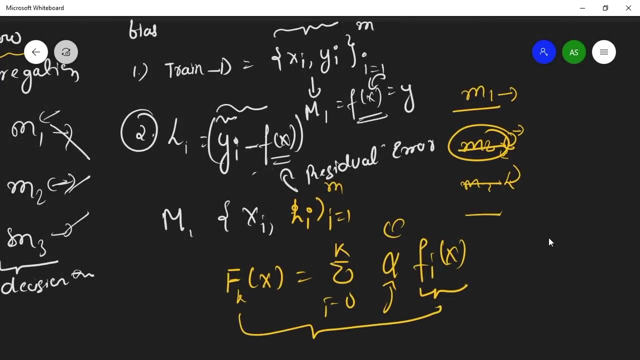 and to so like, like that. okay, so that's, that's the basic intuition behind boosting. okay, so I think that you have understood about boosting. so now this will end it up. this, this function, this function will be ended up giving you low bias, low bias and low variance- a model. 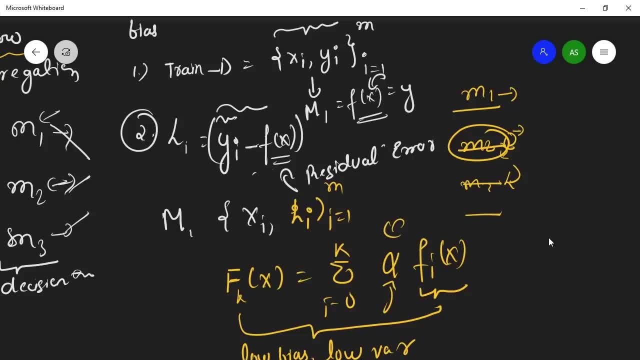 okay, but there is a problem. there is a problem. so you may think, hey, I use, can you name a problem? yeah, sure, I am here to name okay, but before that you can take a break if you want, because I'm just it will just take more one hour to. 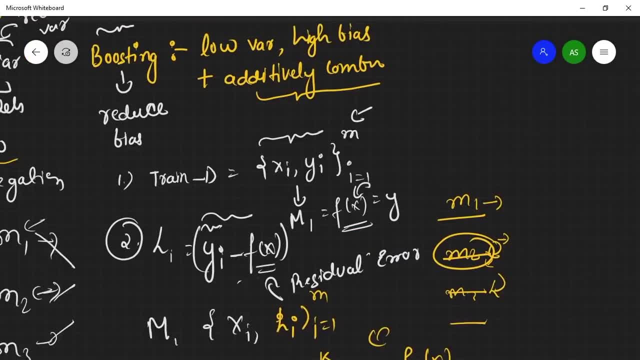 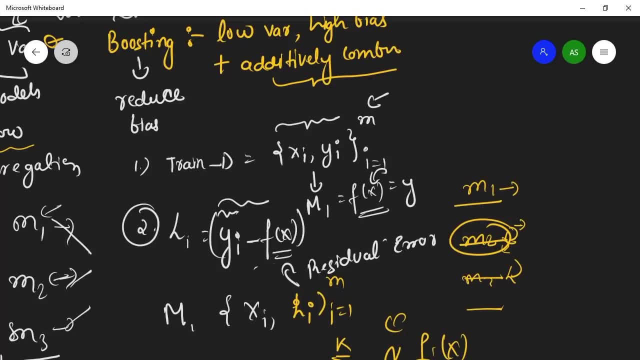 complete. I think so. it's my approximating time, so it will take one more hour. you can take a break or you can do just a prop problem set if you want, but the start to the section and then complete a section, then see the problem set, then see some challenges given to you and I get hub and I really 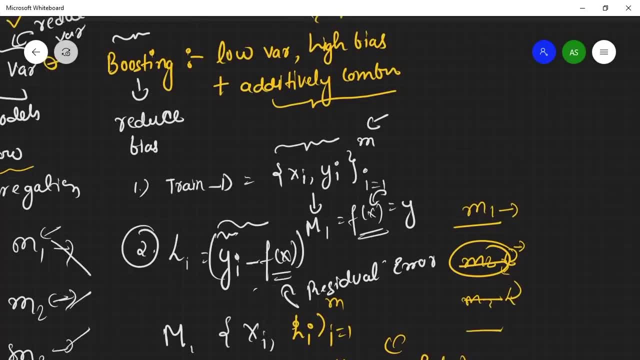 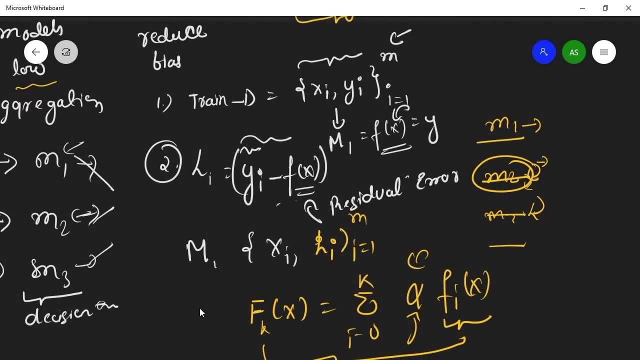 understand that you will be able to do that. okay. so here you have this one. first you have a training data, then you have a loss for loss for each way example. then each model trend, each model tend to, each model tend to fit the residual error given from the previous model. okay, and in that way they end up. 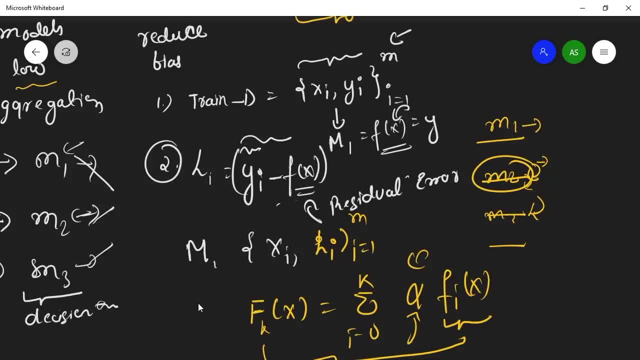 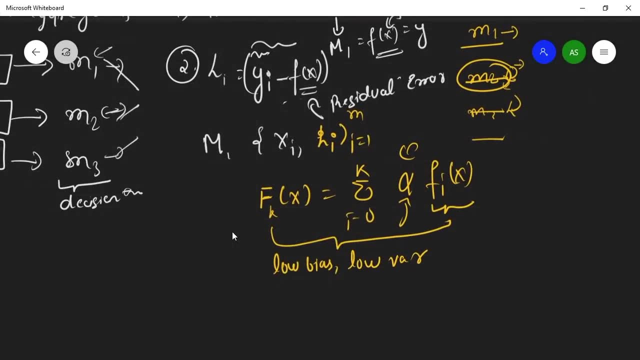 being a low bias model. it's very good on training set, but there is a problem. the problem is that if it is too much good on the training set means and only a hundred one hundred percent accuracy on training set, then what will happen? then what will happen? it will start. 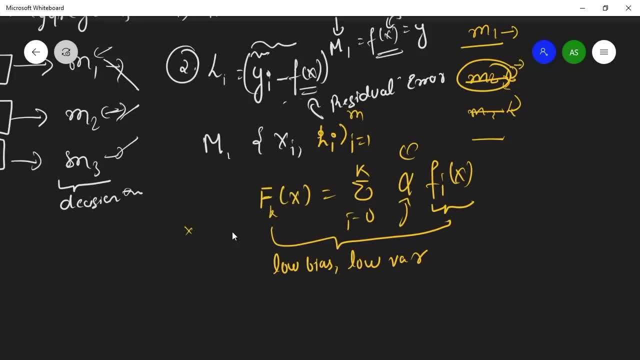 overfitting new training example will come then it will able not to classify or detect a good prediction. okay, so that's way. so that's why we have to take care how many number for base model, so that we have a lambda with it. they will understand this all. okay, great, so we have understood this, and so the core. 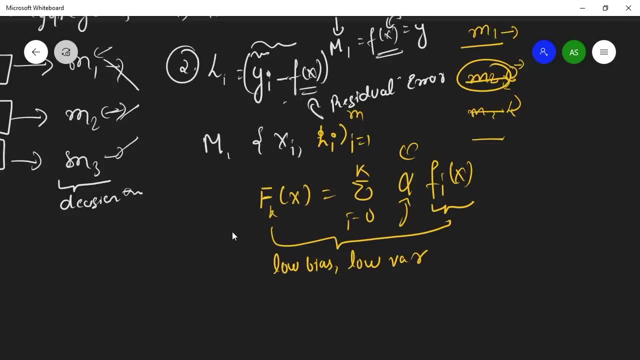 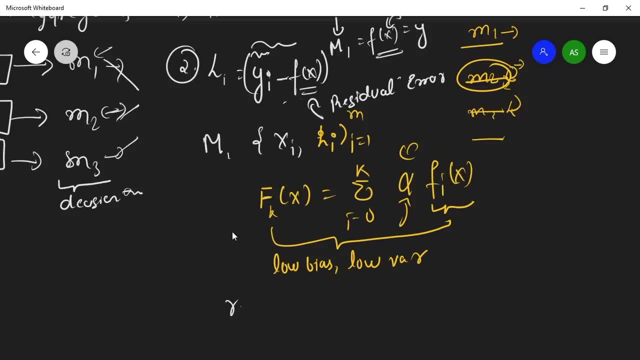 the core idea behind boosting is to reduce the bias, reduce the bias on the frame, like that: okay, this, this converts the weak learners into these strong learners and here we have a good, fine-tuned models which is converted into majority of us and then in bagging, like that, okay, so, let's see so. 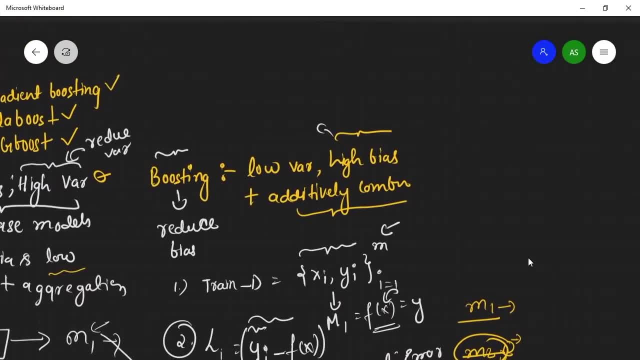 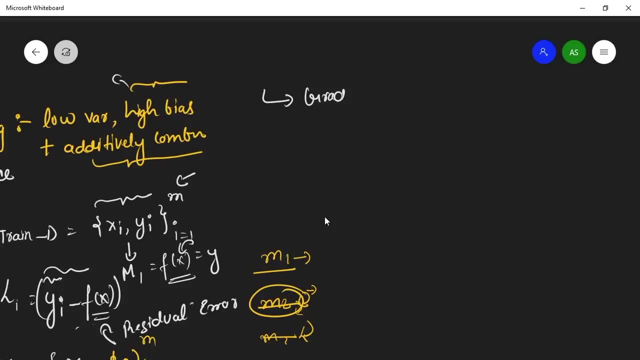 that's the basic intuition behind boosting. so there are some of the techniques that we'll study about: like a gradient, like gradient gradient, boosted gradient, boosted gradient, boosted decision trees, decision trees which is often called as a G, B, D, D. okay, this is. this is because because in random forest, 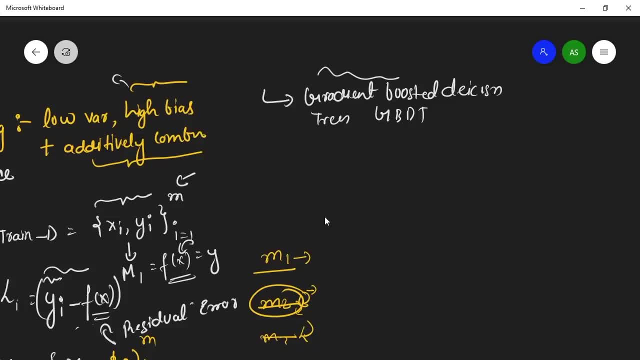 we have our decision tree and here in gradient boosting, you have our base learners at a decision tree and gradient boosting as a base learner, as a decision tree, and then we have a adapt, adaptive boost, which is often called as a dab boost, which is a little bit more advanced version of gradient boosting. 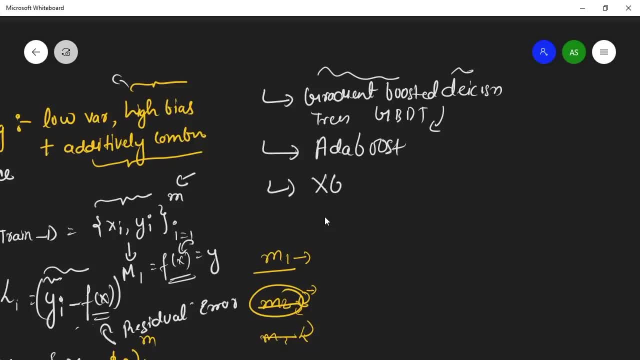 then you have extreme boosting, which is X G boost- okay, which is again a family of a good algorithm and it's always outperforms very, very powerful algorithm: X G boost, as I've seen so far, and I will show you the implementation of X G boost. 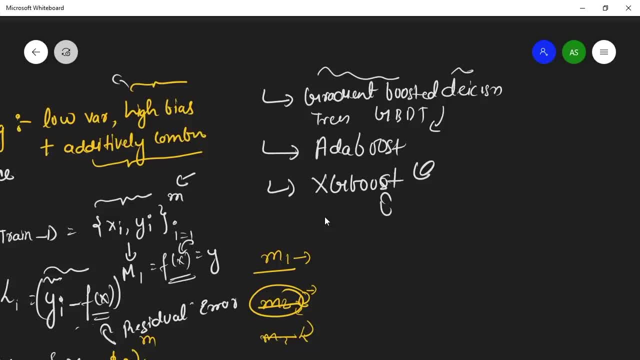 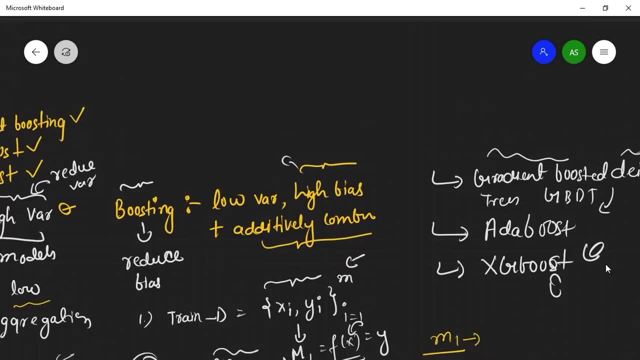 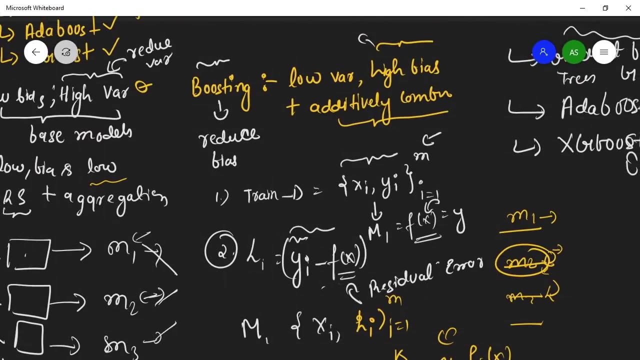 also with some. I will show you how it is implemented and everything. and there's a section Valley. okay. so, and that's the basic intuition behind bagging and I really hope that you understood bagging in detail. just to recap that bag boost or helps and why I'm saying bag up, bagging. it's a boosting, okay, so boosting. 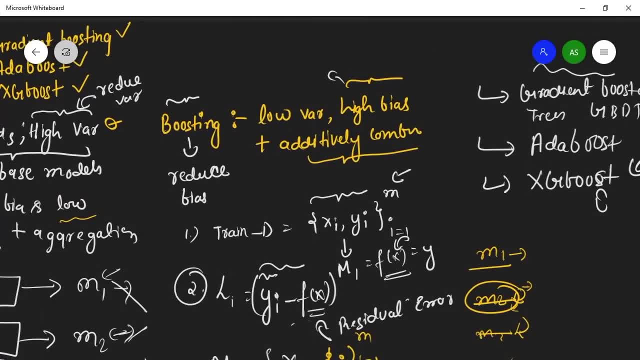 here I'm boosting. we have low variance and high bias model. we additively combined is we with in which we convert our speak learners, and with strong learners, and the core idea is to reduce the bias. it simply means that we want to improve our error on your training set. okay, so 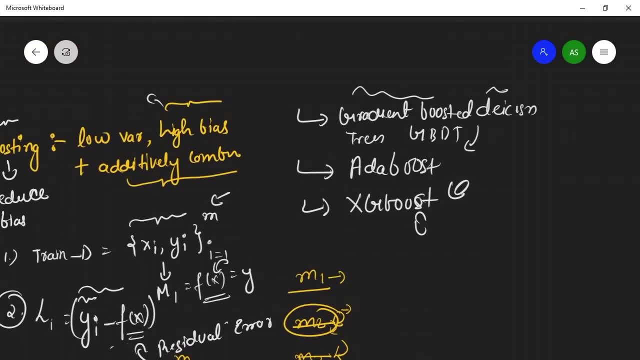 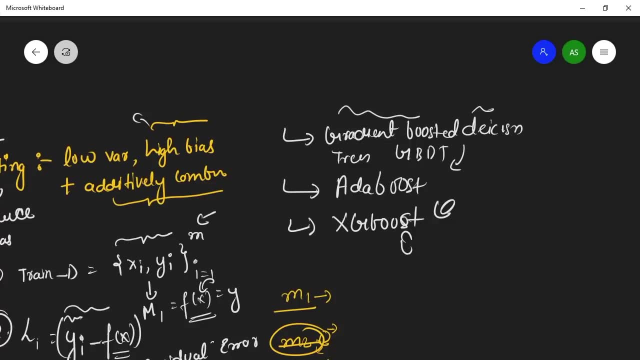 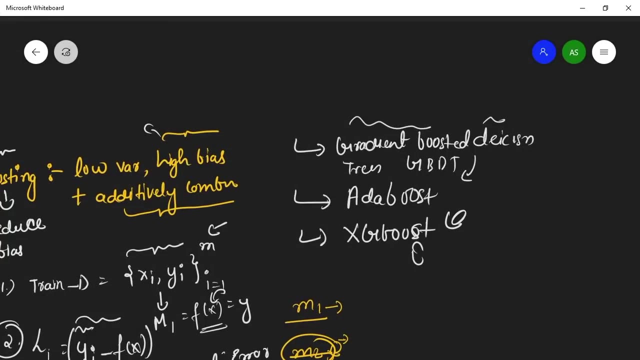 that's the basic, and we have four which we'll cover in this section, which is gradient boost to decision trees, adapt, adaptive boost. then we have an X G boost. okay, so I think that you understood about boosting, okay. so now we will talk about uh gradient boosting, which is again a good uh, a very fantastic, brilliant uh algorithm. 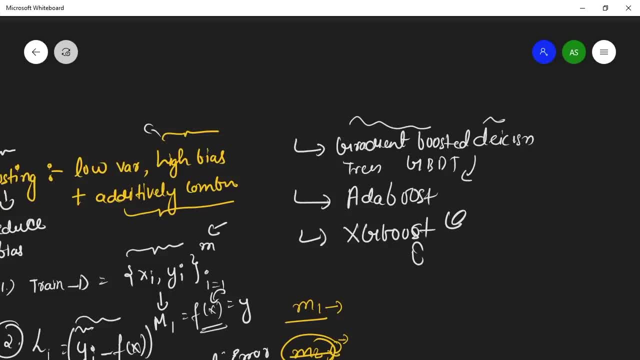 okay so, to just just use an internet companies or very big companies, which is used in ML and production, okay so, which is usually launched in 20s, these uh algorithms. okay so, we'll study in detail to make you understand each and every concept of gradient boosting, and then we will see the implementation, then we will see the adaptive boost, then we will. 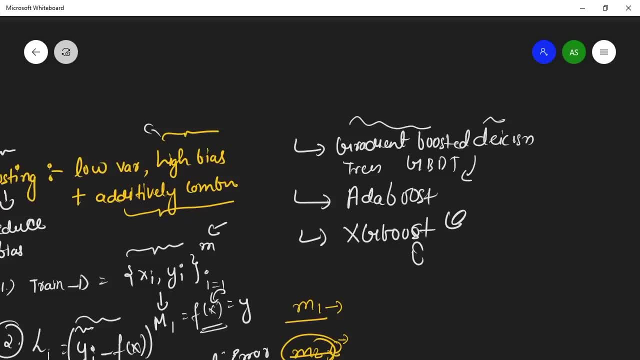 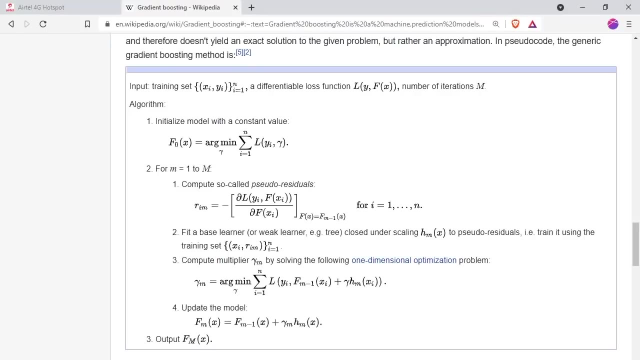 see the XG boost, and then we are end up with this ensemble models. okay, then we will go with unsupervised learning techniques, okay, so, uh, just uh, let's. let's start with gradient boosting. now we have talked about gradient, sorry, the boosting, the basic intuition behind boosting what actually? 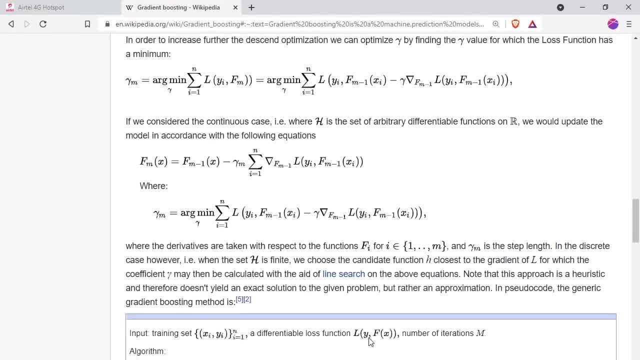 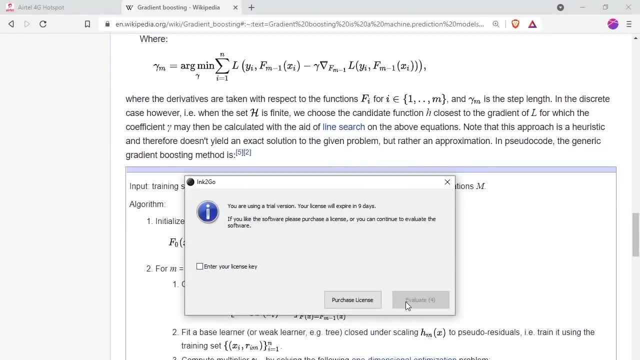 the boosting are. so now I will start talking about a gradient boosting. okay, so gradient boosting is algorithm that I've seen so far. uh, yeah, one of the most powerful algorithm, which is uh, which is yet to uh, uh, just learn, it's very to have a good in your toolkit. okay, so I'm on a Wikipedia page. I'm 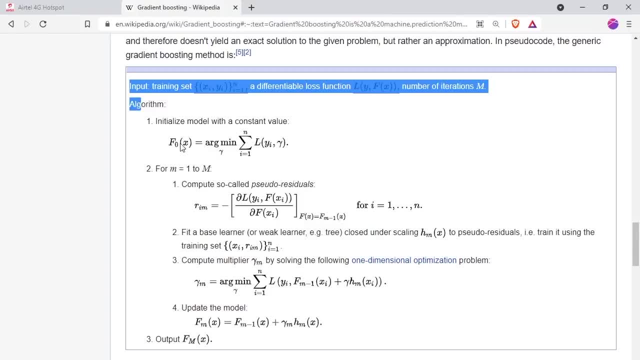 on a Wikipedia page which I found a great mission. uh, this great uh algorithm, which is again uh, which to which? which just tells you a very good of intuition behind gradient boosting, rather than just. I may make use of my blackboard either way, I will make use of my blackboard over here, okay, so, uh, so, uh, what is so? 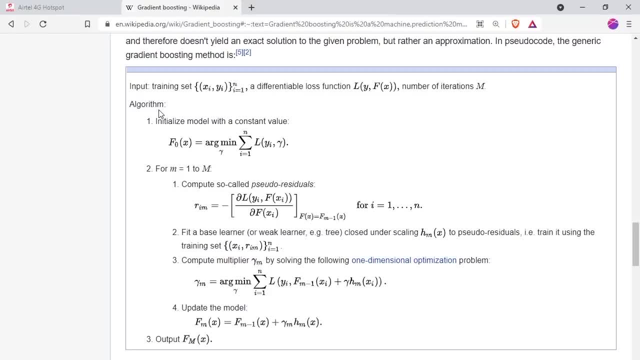 what is gradient boosting? this is a great question. so gradient boosting is a boosting algorithm that just converts the weak learners into the strong learners. okay, so let's start with in this, uh, gradient boosting, and you can search for gradient boosting Wiki and then you will see the gradient. 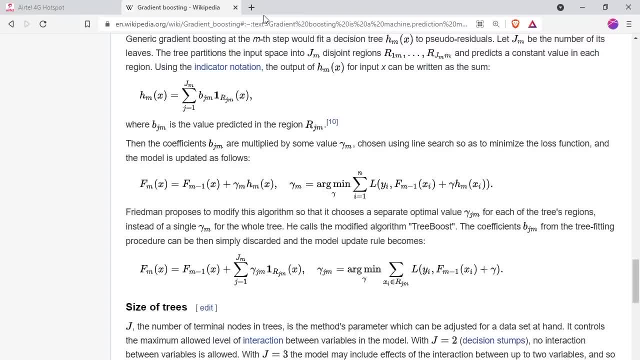 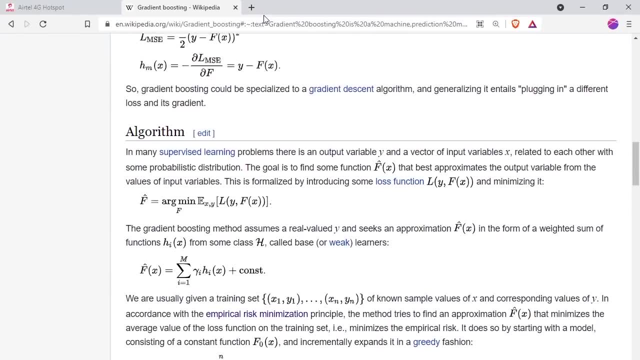 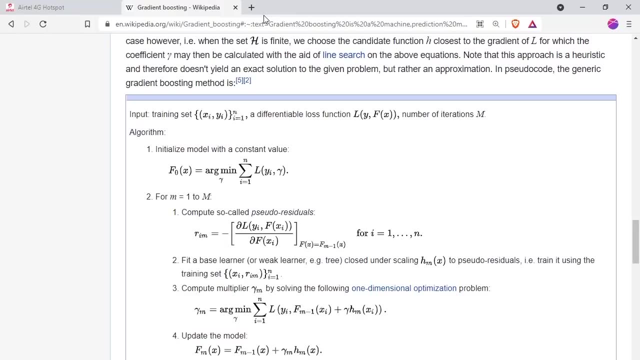 boosting Wikipedia articles and then you can read the full articles either. I will cover everything in that, uh, in sort period, period of time, but I've already covered some of them and and of my just I will cover I I have covered more than this Wikipedia. okay, so I will give you some real world. 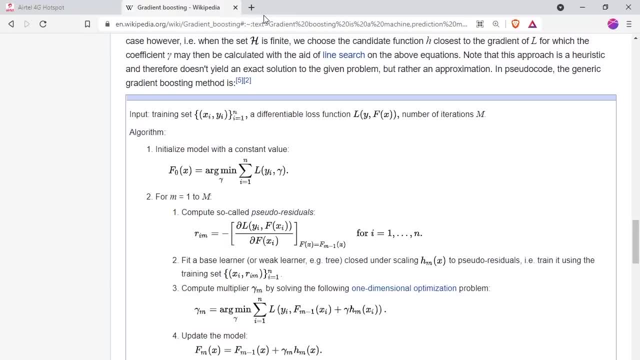 examples of gradient boosting also, where it is used and everything okay, but first of all let's understand the tro, this, the this algorithm. okay, so let me see my pen is at least working or not. I hope that this is working. yeah, this is working great, I'm just happy that my ink is working. let's try if the ink to go. if you're watching, please help me. 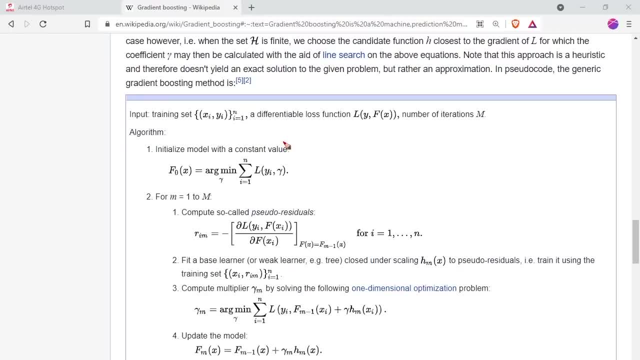 to improve this. very. it is not that much good. okay, let's improve this, but it's very good tool. it's some sometimes it lacks, but it's a very good tool. you check it out, it's very good. great, for free. okay, so you have this training data, which is a input training data. you have this three input: 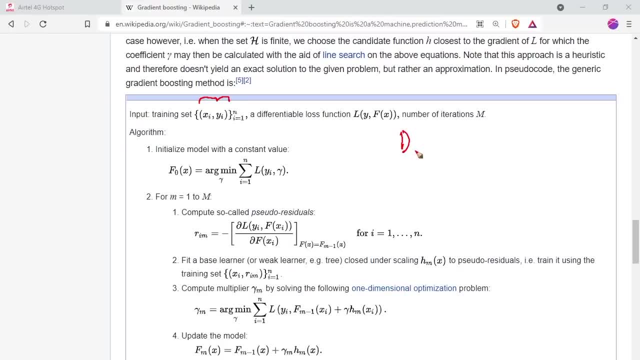 training data, which is your, which is the setup. let me write the training data, which is simply xi and yi and simply goes from i equals to one, all the way around to the end. okay, or M, which is our list. let's stick to our formal notation, which is M, which is a number of training examples, number of 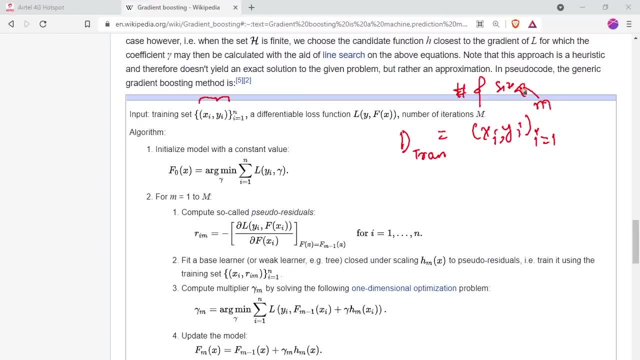 a training or the size of our training examples. okay, so that's the, that's our given data, and we have a differentiable cost function. then we have a differentiable cost function. okay, so what do I mean by differentiable cost function? differentiable cost function means that your this: 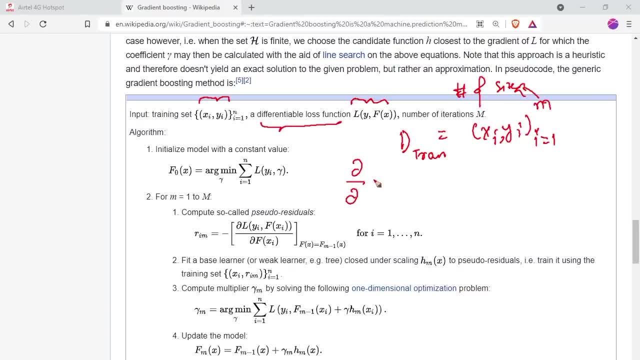 cost because we take out the derivative of our cost function. we take out our derivative of our cost function with respect to some, uh, some value. okay, so let's take, we are taking out the derivative of our J of Theta, partial derivative of our J of Theta. okay, so that's the. that's the basic about. 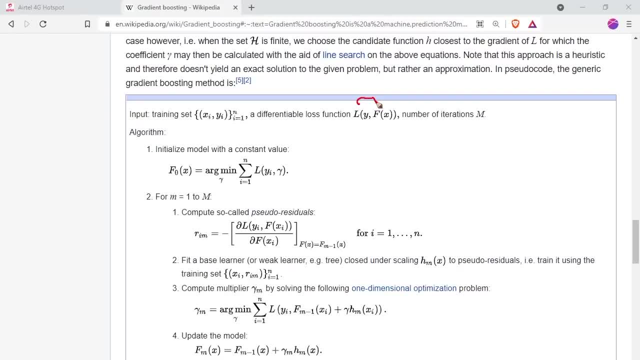 means that's the differential equation that I know. if you know, if you're a calculus student, then then you might interpret that we have a differential. but as if you're not able to get, what is this differentiable? feel free to leave this differentiable. just think that it should be derivable. okay for our gradient. 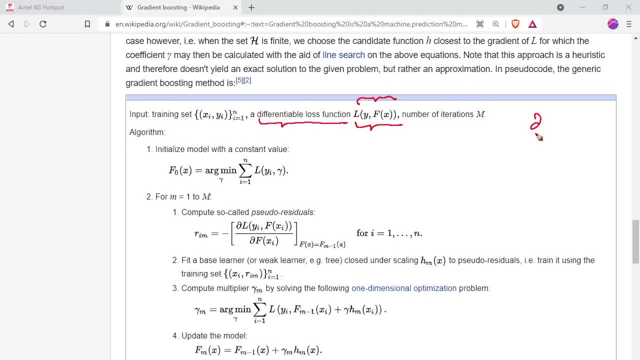 descent, or we will, because we have to take out the derivative of this particular loss function with respect to some uh weights. okay, so we, with that, if we are given training set which is train, we have a given training set which is a value- X, so xi and yi- which goes from I equals to 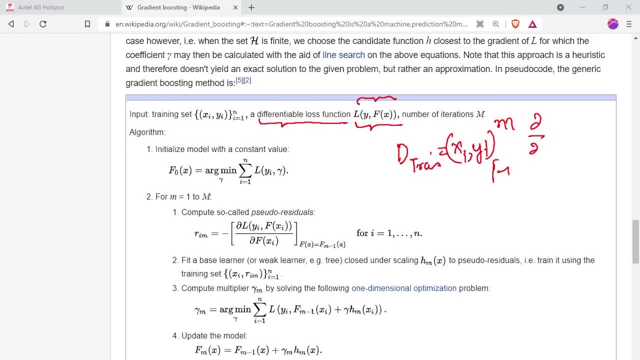 one all the way down to the M. okay, where is my eraser? I think that this is my eraser. yeah, I equals to one all the way around to the M, and then we have a differentiable equation as given. so let's stick to the J of Y, Y, F of X, and this is simply just the error. it means just a minus. 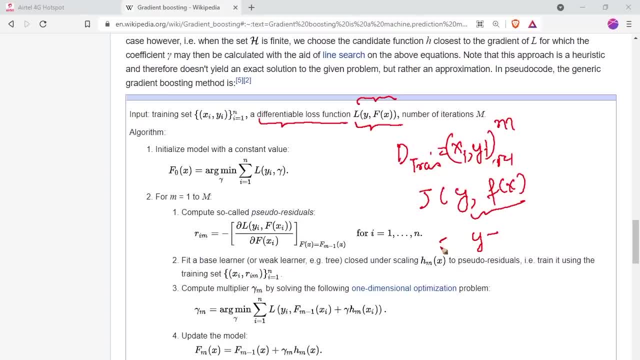 the minus your more or more appropriate value. each in a particular examples i equals to 1 all the way down to the m, and then we square it all up. okay, so that's the, that's the our cost function. maybe it can be mean square error or it can be log. 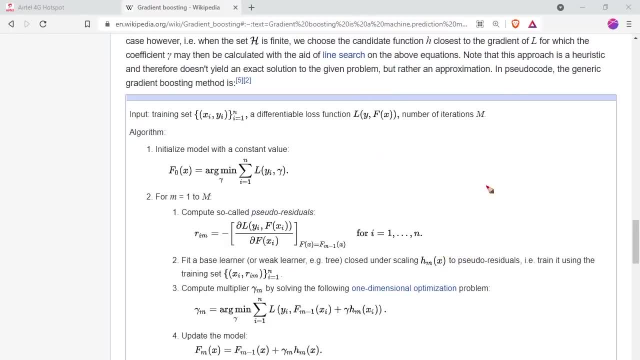 loss for classification, etc. okay, then we are given the iterations. then we are giving the number of iteration, which is m and m. here is the model: m. here is the base learners: m. here is the number of a base learners: number of a base learners. number of a base learners. okay, so this is the 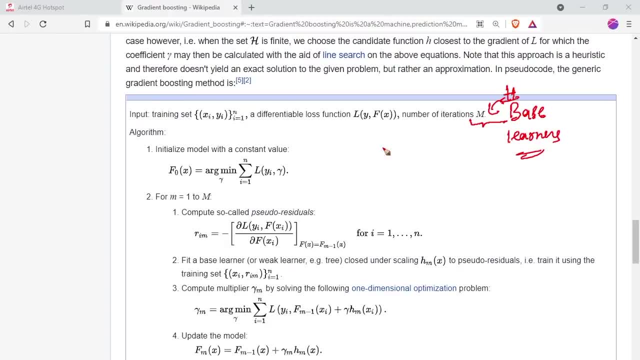 number of base learners, which is m. now let's start with algorithm. so what this algorithm tells you. so let me choose the different colors so it might make sense. so we initialize our model with some constant value lambda. with some constant value lambda in that case we have in alpha. but now we 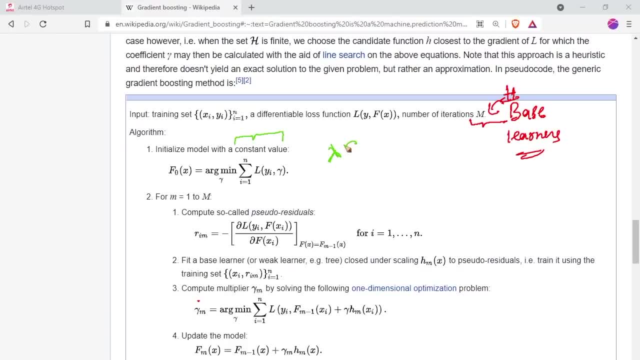 had changed a little bit, that we have our favorite lambda, okay, so we have to find lambda. okay, let's just think of it as that we have a lambda, we have a lambda that we have to find that lambda that minimizes this training error, this loss function. it should be told here, but I told you here just. 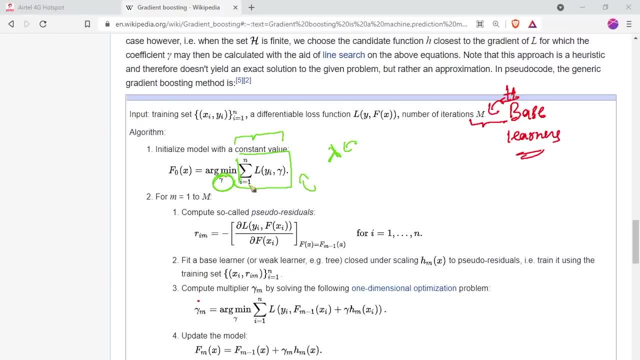 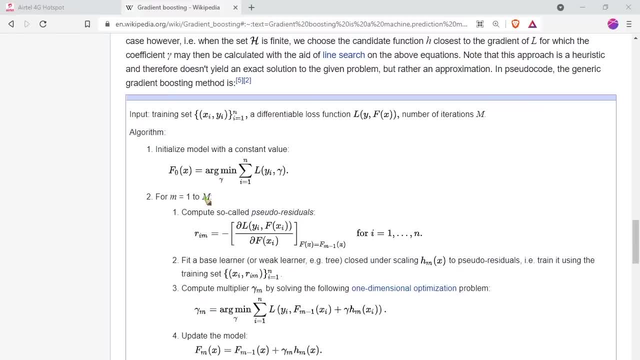 you initialize it and then what you do? you iterate through each and every model. okay, first you go. first you do this for first model, then you do again for second monuments. you apply for loop where you for m equals to one. first you 2m means you want to go 1, 2. 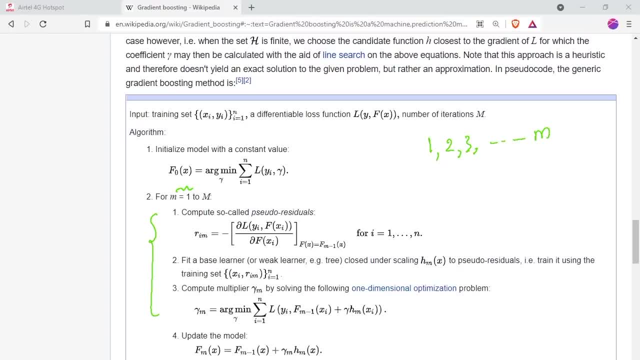 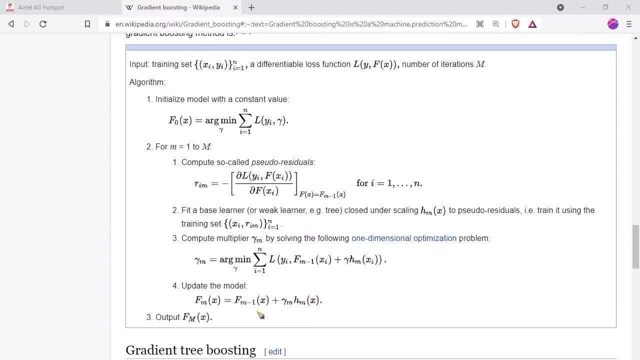 three, all the way down to the m. okay, so you do this, and then let me first of all let me. okay, so here then what you will do. then i hope that then you initialize your model, then you compute the residuals, you compute the pseudo residuals, you compute the pseudo residuals. 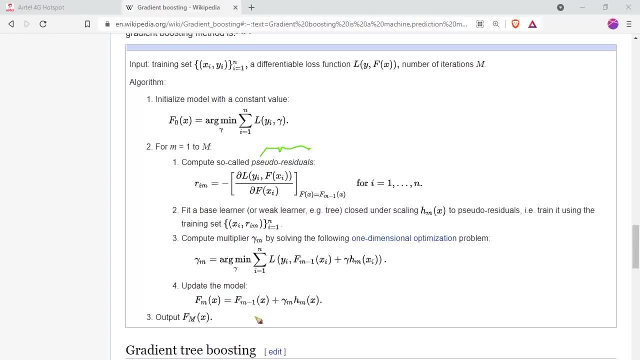 you compute the pseudo residuals, and then here it is named as r? uh subscript i and m, and m here denotes the number of which model and i here for each training examples. okay, so here you compute the inm, and then you take out the partial derivative. the partial derivative, oops. 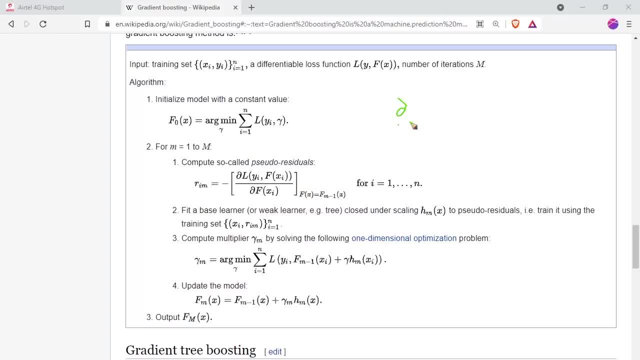 might, is not working. partial derivative- hey god, please help me. the partial derivative of your cost, function y, i of your cause, function y, i and f of x. so this is your loss function. who we're going to call the default function or the index, is here and i don't remember exactly. 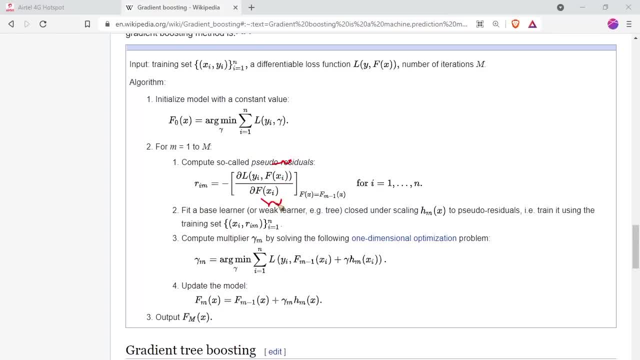 how much arrow does your arrow has a point? so here you are. you can only have one point here. which character is i and here up here and you take out of your cost? function is job. what's your with respect to this function? okay. f of x, your model: predicted value: okay. 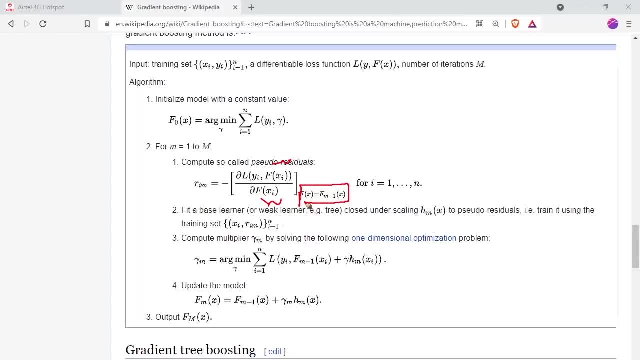 And then you want to fit your model onto your previous residual. So for you go to: i equals to one all the way onto the n. So here you take out for f of x means f means here you are fitting your model. 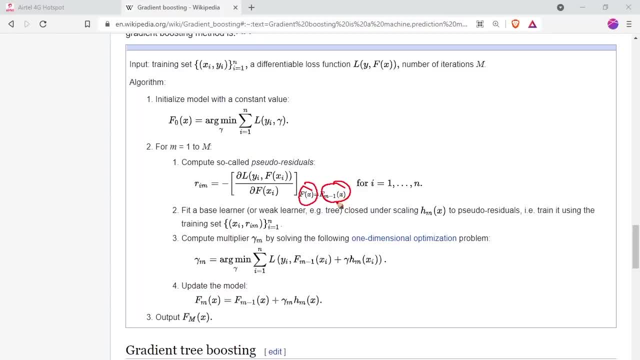 means just, you are making the model to be f of m minus one means the previous model. okay, So compute those residuals and then you fit the base learners. okay, That I've just shown you in my previous. just in a boosting that we fit the residuals. 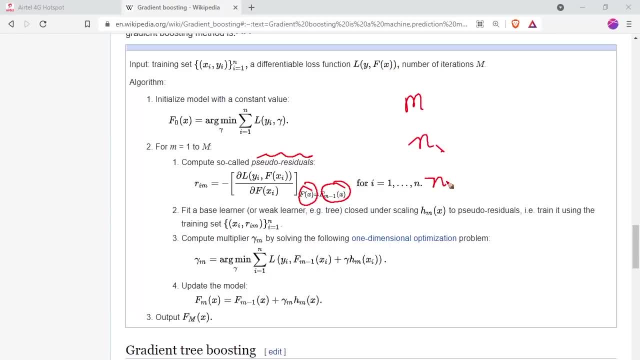 So let's take example: we have m one, m two and m three. We have taken the residuals. we have taken the residuals and here is: give some residuals. This m one is trained to fit the residuals from m one. This m two trained to fit the residuals from m two. okay, 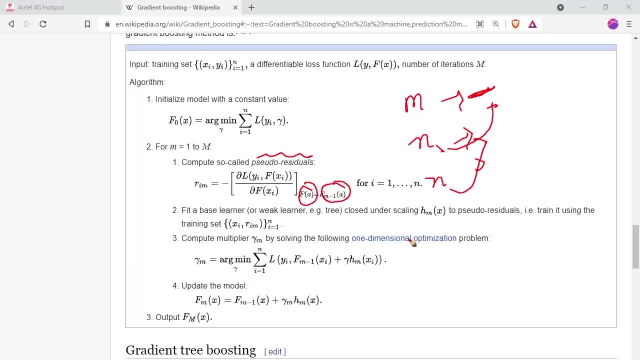 And this is m three. okay, So it is trained to fit the residuals of m m two. okay, So then you fit a base learner or a weak learner. Let's take example three, close under scaling of h of m x. 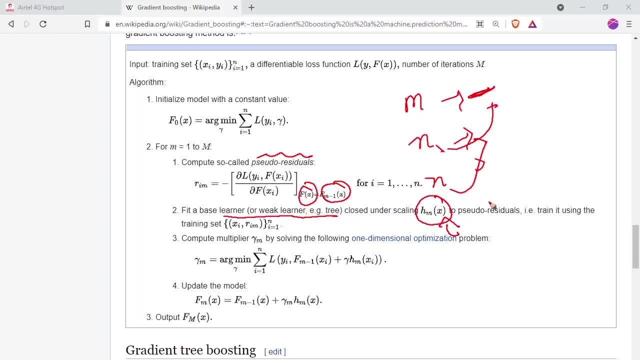 Here is your two residuals. two pseudo residuals means you fit the learner, to fit the residuals from the residuals got from the previous base learners. It is to train using the training set. this one, okay, And now here r i m is in our case, which is l? i. 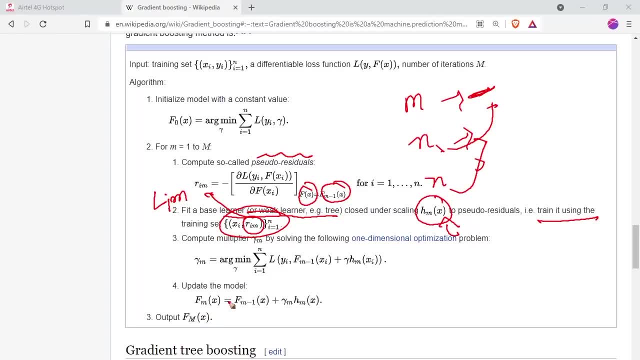 On m model, okay. So then you fit your model that I already showed you, just similar that we have seen. And then you come compute the multiplier, which is a constant multiplier, lambda m for each model. you have lambda m okay, which is a one dimensional optimization problem. 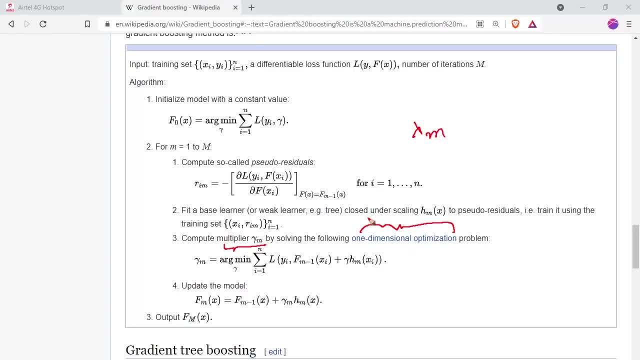 for solving the one dimensional optimization problem. So you may ask: yeah, why do we are choosing this lambda m? So for solving one dimensional optimization problem, why do we are choosing this lambda m? Because one dimensional optimization problem going into 1D, 1D, 1D optimization, 1D optimization. 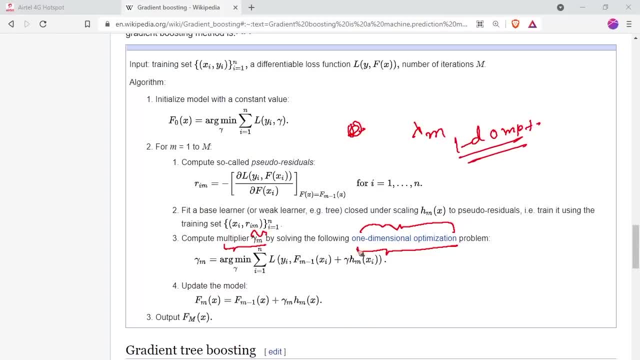 is out of the boundary course, but you can see on the link, okay, the how you compute. you compute lambda for each model. that minimizes the loss of y, which is ground truth from the previous model, plus plus lambda times. our just the model, that that we have now. 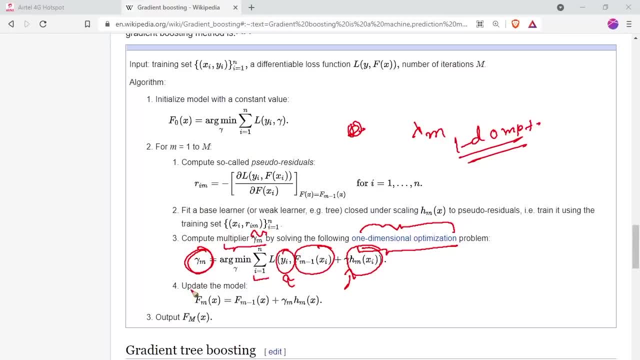 Okay, Now what you do? you update the model. Now you update the model to be to win, the model to be fitted by the, the model that fitted the previous residuals. okay, so f of m, x. here m is our model number, the means model. 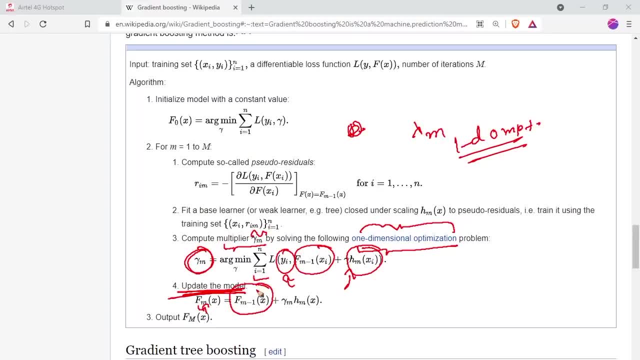 number. then we have it. then we have this: f of m, minus one previous model, plus lambda m. lambda m, which is some constant for solving the one dimensional optimization. Okay, Because we are taking the partial derivative of our loss function y, i and f of x, i, with 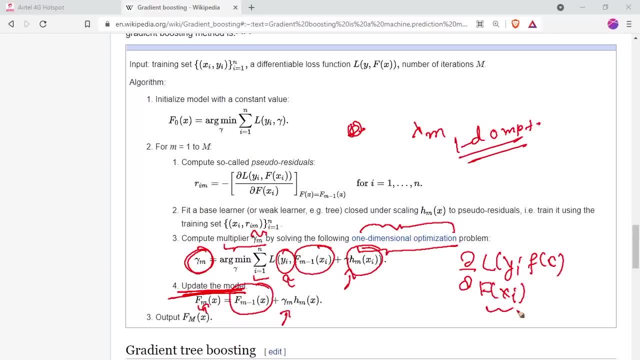 respect to f of x i and f of x i is our model predicted value. okay, times h of m, x, and then you get your output as a f big model, m, m big model to all the way down to the x. okay. So here you, when, when you cover all of this, you, when the loop is done, then you get the. 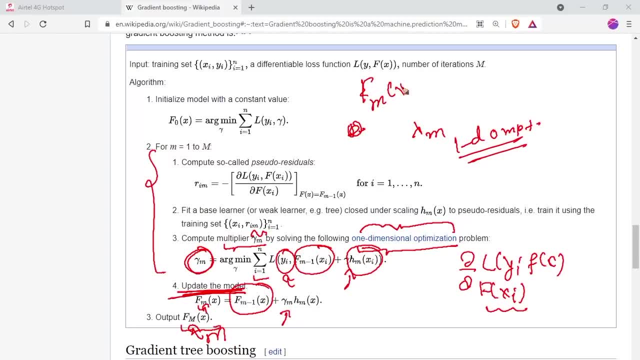 final model, which is f m x. That is simply f of m minus one x, plus the previous model. is this previous model plus the model that we got after solving this all one day- optimization problem? Okay, so that's the gradient boosting algorithm that I really hope that you understood. 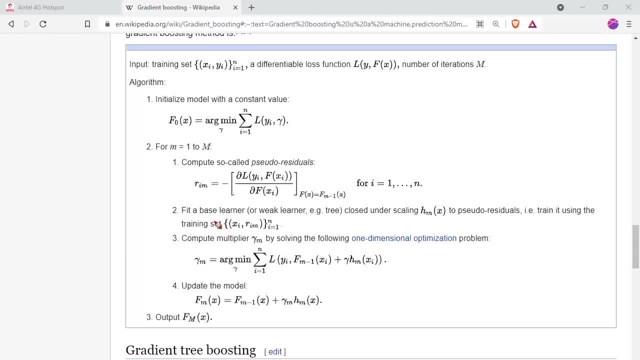 But let's- let's just just as a recapitulation, to help you understand it a little bit much better to understand this problem. Okay, so what we do, let's understand what we do over here. We simply, first, we have a given our training data, we have a training data x, i and y. i going 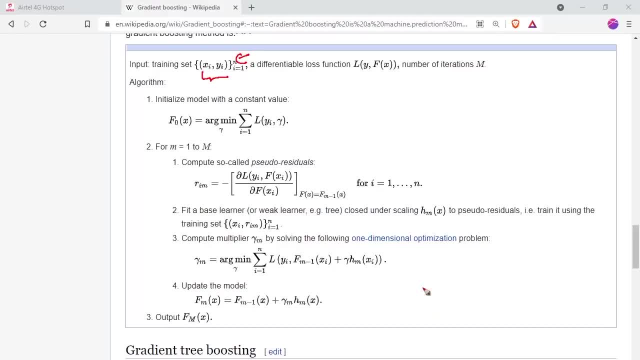 from i equals to one all the way down to the end. and n here and n here. I just hope that it should work now. And n here is your. n here is number of a training- your number, not size of your more training set. then you have a differentiable loss function with the number of base learners that you 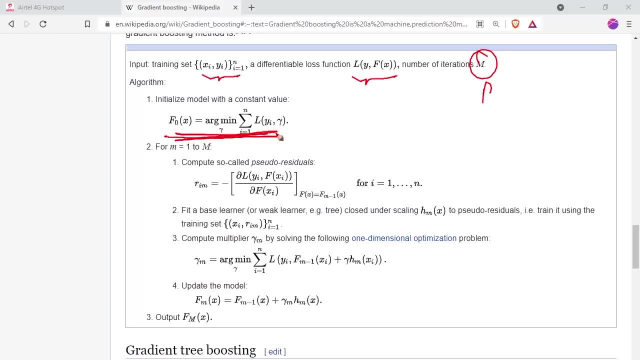 want. Okay, So you initialize the model with some constant. okay, then you apply a for loop. in that for loop, you take out the residuals. you take out the residuals for and, and then you name it as a r subscript i, which is the number of a training exam, that the index of training. 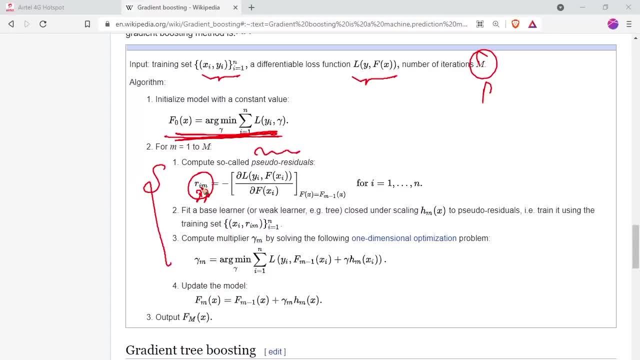 example, and m is your number in the index of your model, okay, minus the taking of the derivative or partial derivative for of your loss, okay, okay. and then you fit a base learner Or a weak learner, because they're, because it just makes you a weak learner to the strong. 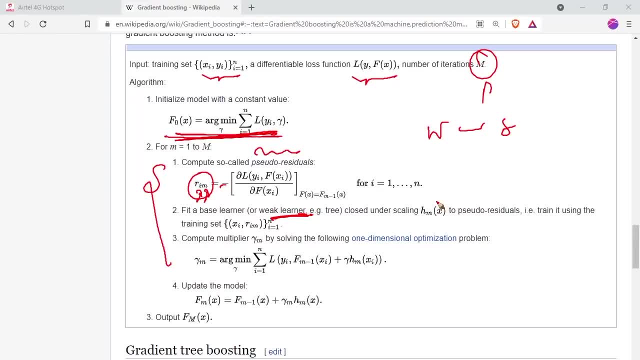 learner. Okay to closing under h of m x, which is your God, from the weak model means you just to fit the base learner to the residuals. So it's simply that you are, that you are going to fit your model into x- i and your l- i, which 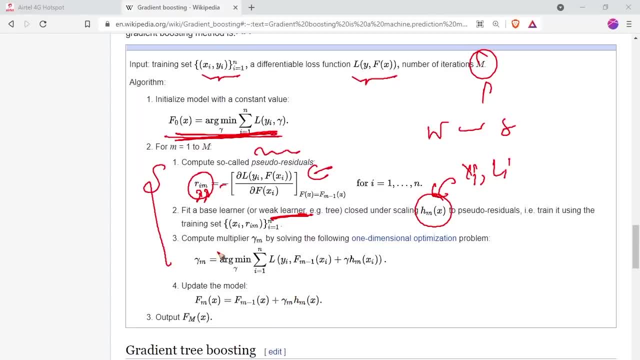 is simply l, i. is this okay? Now you compute the multiplier: lambda m, lambda subscript, and for each particular m means the model index For solving the one dimensional problem. So it's just you find the lambda m that minimizes the loss, that you get y, y, i, comma, the output. 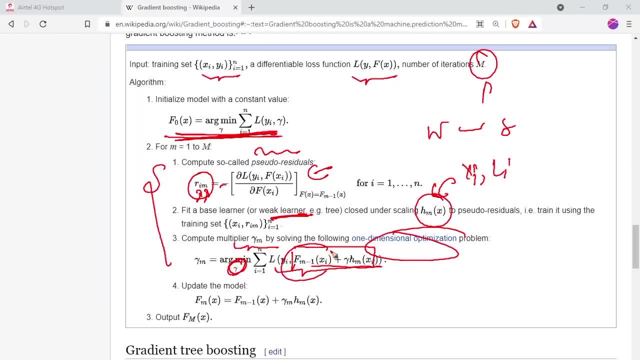 from this model. Okay, this is the whole model. now, this is a previous model, that is, this is a new model that is fitted to fit this residual, okay, and then you update your model. okay, then you have to have output a big model which is f of m x. that is simply this: f m minus. 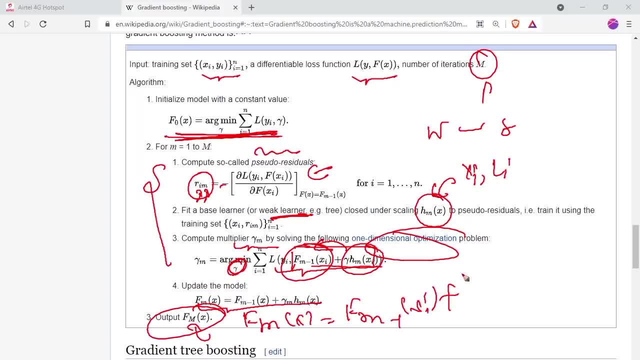 one. So you have to have output a big model which is f of m, x, i plus your big model. Now you, just after your full iteration, you'll be ending up being a big model. Okay, so that's the basic intuition behind gradient boosting, and really think that you. 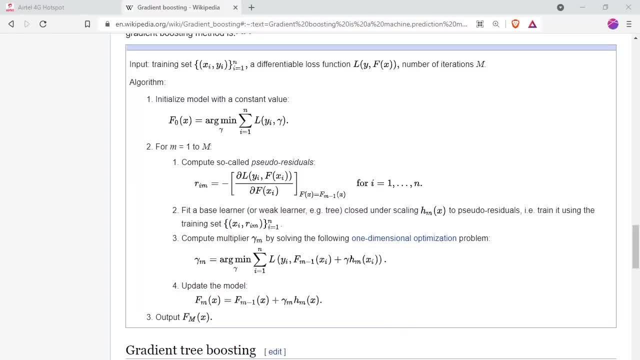 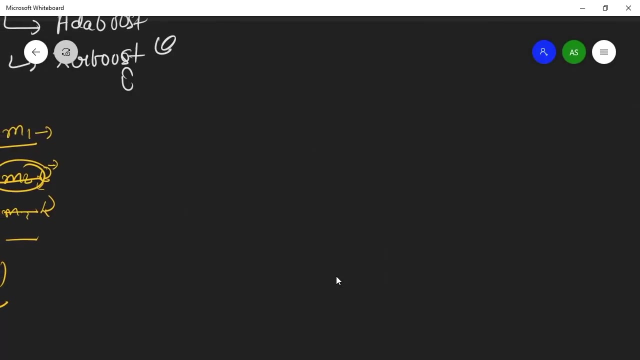 understood about gradient boosting Now. now it's time for getting into the, for getting into the, something called as a regularization and shrinkage. Okay, but before that, why do we need even regularization and shrinkage? So, why do we need? Well, as we have already talked about that, we have, and that we have in boosting. we. 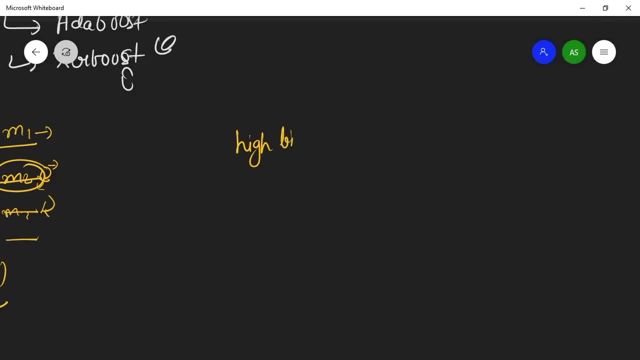 have high bias. we have high bias. Let me see the recordings are on here. Oops, we have our high bias and low variance problem. sorry, high bias. So we also we use boosting to reduce the bias, to reduce the bias. So high bias is just doing viral training set. 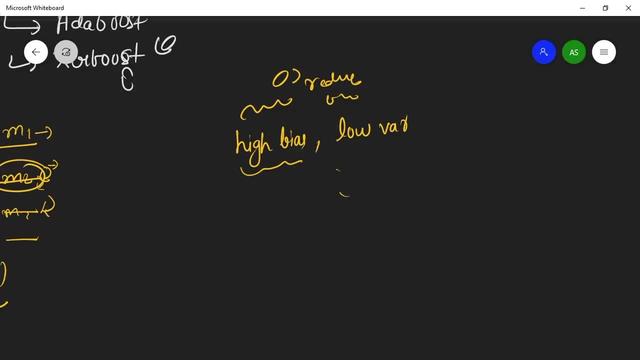 So we, just after each iteration we are fitting the previous model residual. So yeah, it is making a no limits. it is doing very, very good on training set. So very, very good on training set. So it may happen that it may start overfitting and our low by variance goes to high where 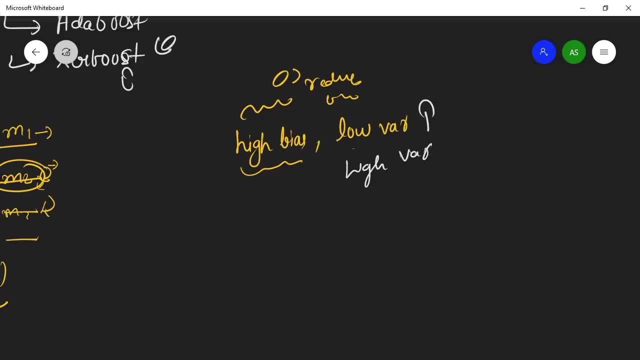 starts goes going to high variance, with our low variances start increasing and now it's converse to high variance, So that actually can cause overfitting. okay, so for avoiding the regularization and shrinkage which is again shown in the Wikipedia page. 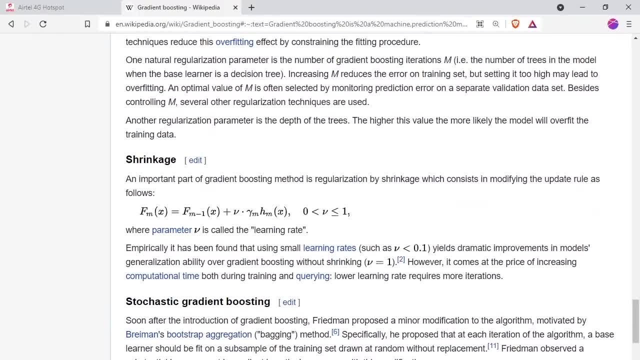 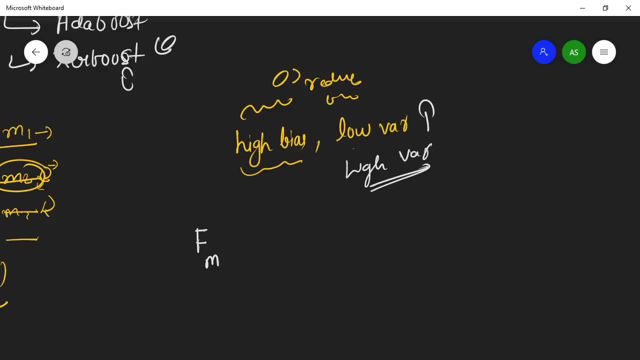 Let's see. So here, I think that I can teach you better than Wikipedia page. okay, so you have you this big model. you have this big model f of m, x, which is here. you have a, h, h, g to x, plus you do for. 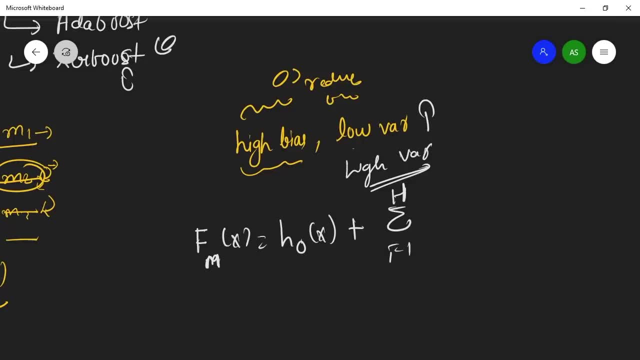 i equals to one all the way down to the edge. all the way down to the edge is number of for your model: lambda m, lambda, m, or you can see m, the number of a model. okay, h of m x, Okay. 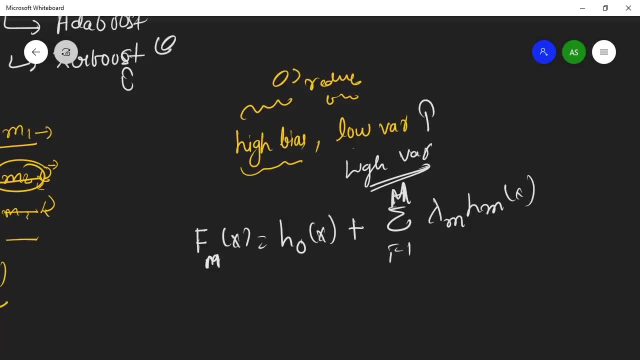 So that's your model, that the, and then what do you do then? if the number of a base models increase means it will fit more residuals, and it will fit more residuals, more residuals, then your overfit will then then over. then it will start overfitting, start overfitting. 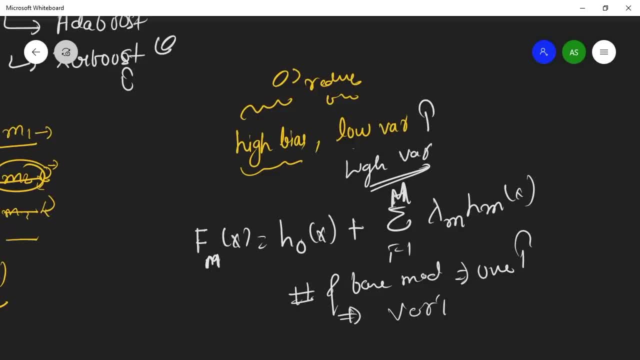 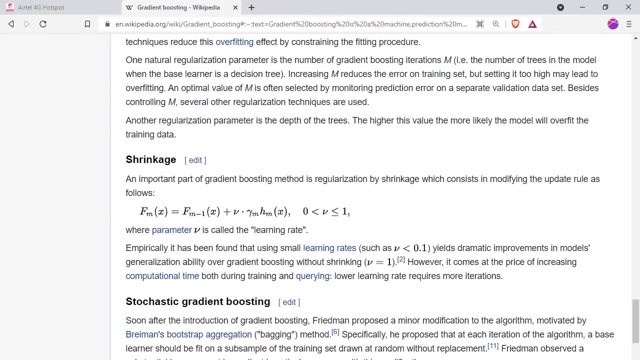 And if it is start overfitting, then your variance will start going up. Okay, so that that will cause the problem. So what you do, you shrink. you shrink by a factor of lambda. just a is a Greek letter that I even don't know. that is something called as a V, So let's assume that is a V. 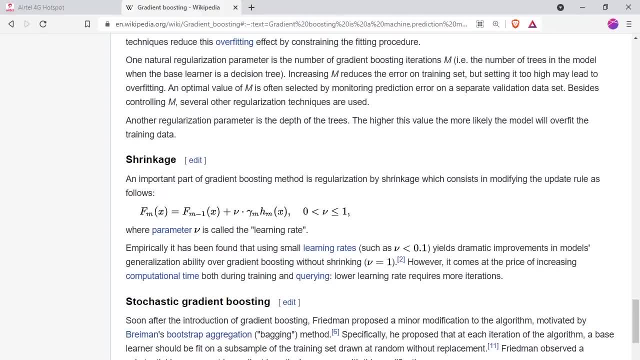 which is a parameter V. Okay, so we have a parameter, we have our parameter V, which will help us, which is just a parameter for controlling the or it's just shrinks, your shrinks, it just shrinks. to do not go. that much means this gives a weight, it is just 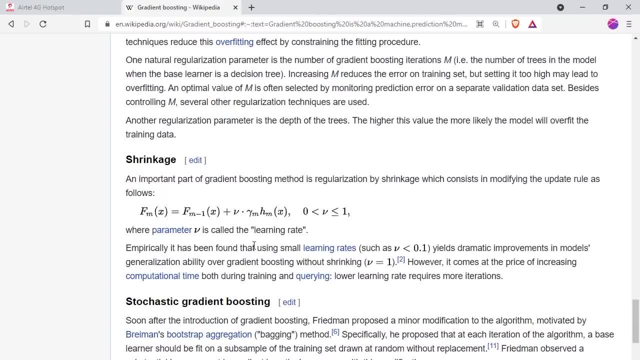 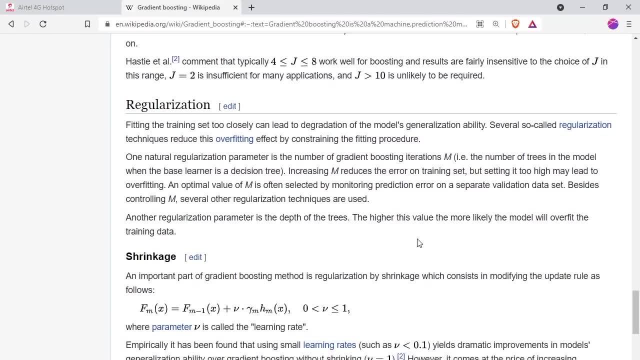 a learnable parameter just gives weight and empirical it is found that V equals 0.1, tends to be a dramatic improvements in your models. okay, so that's that's why we use this V, this V, to be 0.1. 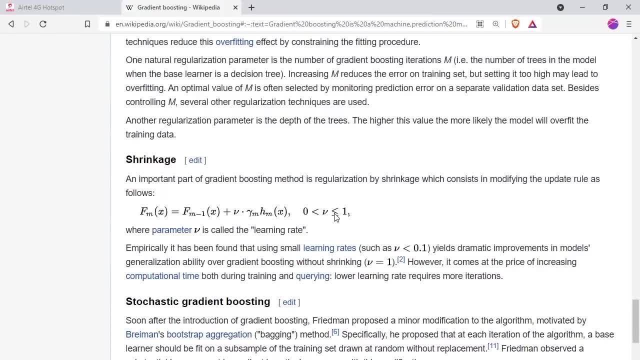 And again, your V should be in between. your V should be in between zero and one and it's found that V equals 0.1. would be dramatic improvements in your models. okay, so you add a new weightage to that model means to do this model. okay, you add weightage to. 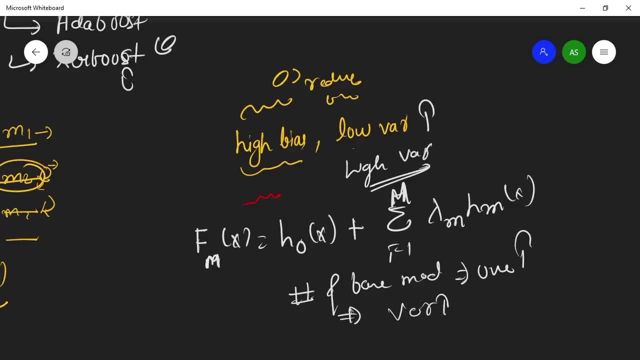 this model, Just fine. So you add a new weightage to that model that I've just shown to. you add weightage to that model And that's called the learning rate. for how, for how much time, for how much rate it should learn? 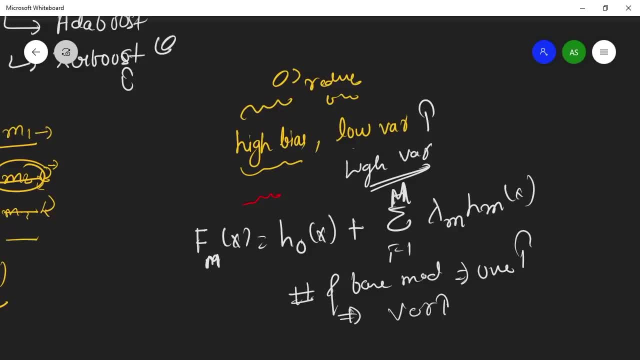 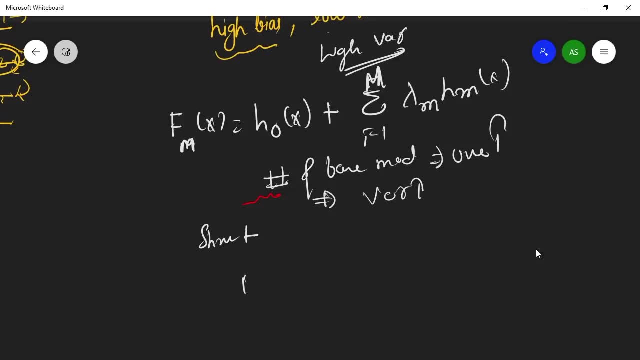 Okay, so that's the stats. we add V, that model. So let me add that. So let me add that. So what do you do for us? you just shrink your model with. shrink your model, big model, by going f of M minus one, x plus V times lambda m, h of K. 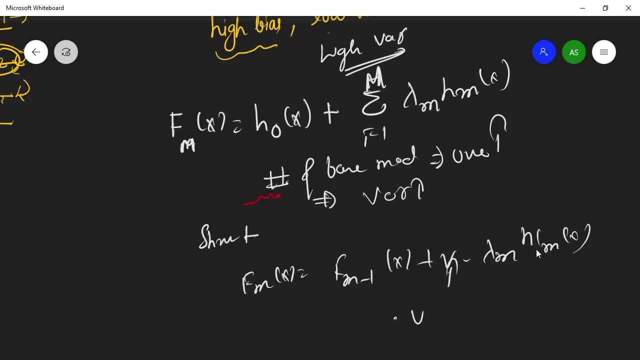 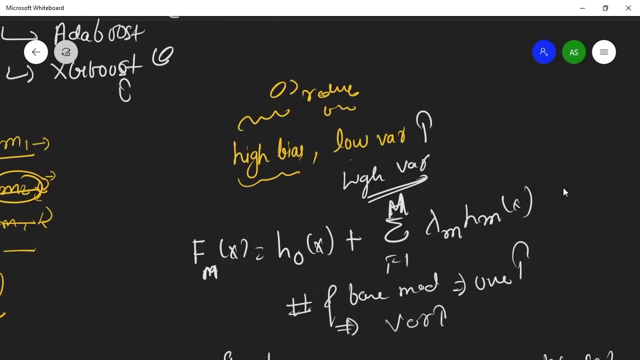 M, x, x, x times lambda, And v here is in between 1,- okay, And Periclet has found that v equals 0.1 works best, okay. So that's about gradient boosting and I really hope that you understood this also okay. 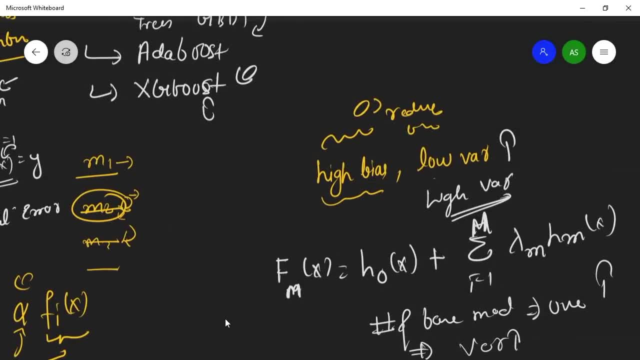 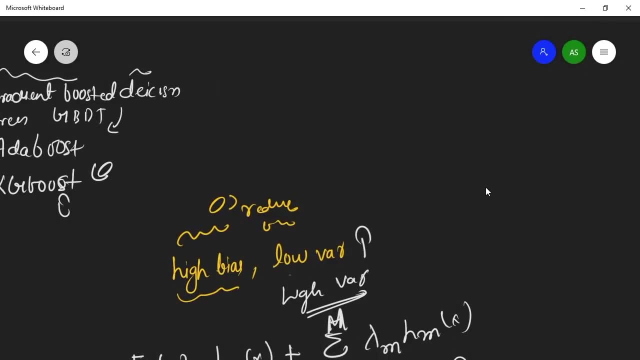 So now it's time for we will take a look at implementation. okay, So now we will take a look at the implementation of gradient boosting classifier and gradient boosting regressor. okay, But before that, let's see the train-in-time complexity of your model. 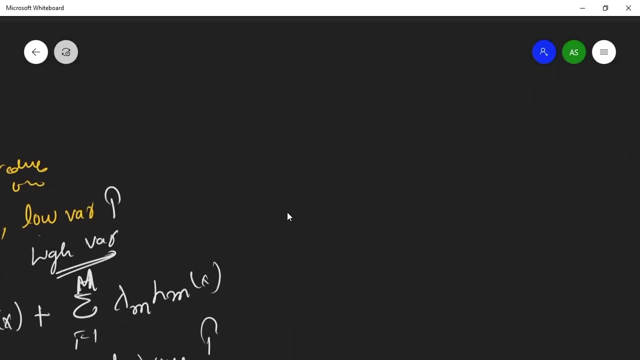 So let's take all of decision trees and decision trees. we have our train-in-run-time complexity, So here we end. decision tree dp. I'm writing dp. We have all n. oops, why am I writing this? n log d and here d and then random forest. we have o order of n log n. number of a decision tree means k, okay. 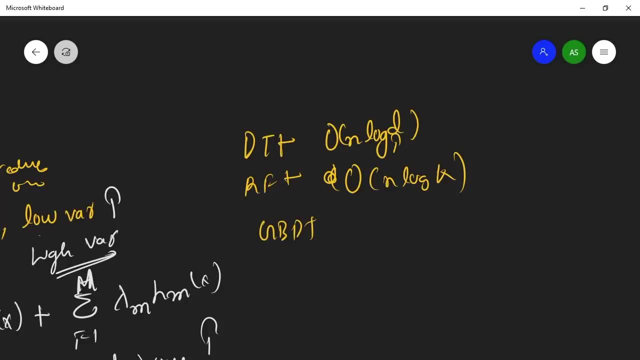 Now when group Gradient boosting decision tree means here we just take our base learners as a decision tree rather than different, different models, so we have o n log d times the number of our models. okay. So that's the basic time complexity of your gradient boosting decision trees- okay. 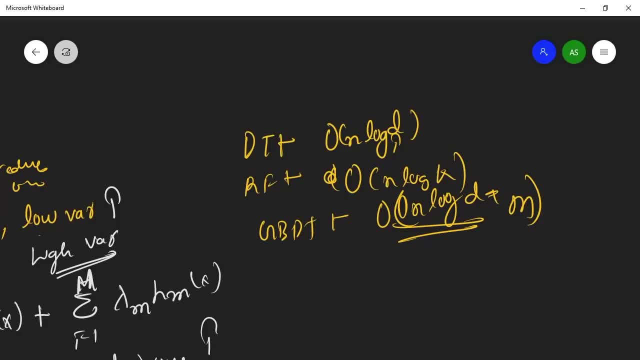 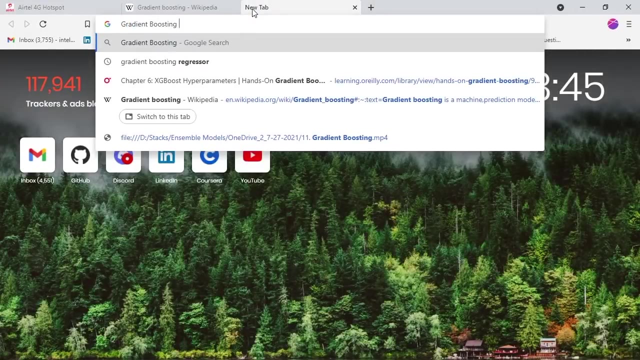 Great, Now we will see something called as. Now we will see the implementation of this gradient boosting, decision trees and CycleLearn API. okay, So let's see. So let me open gradient boosting implementation implementation. okay, And SQL learn. 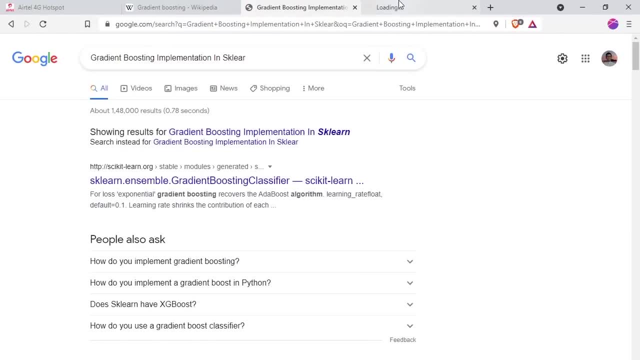 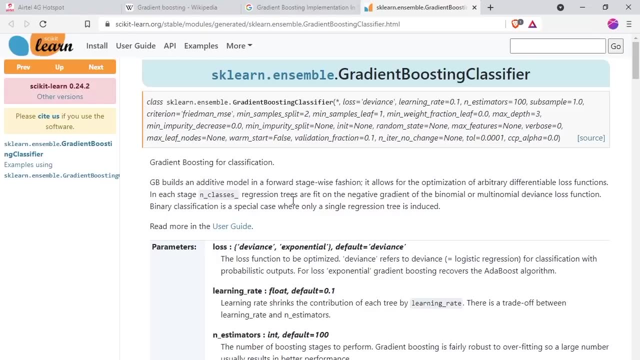 Let's see, yeah, here we found This. wait for a few seconds, it's just loading. Okay, great. So now here you are on a page of CycleLearn API gradient boosting classifier, and then you can see over here that. 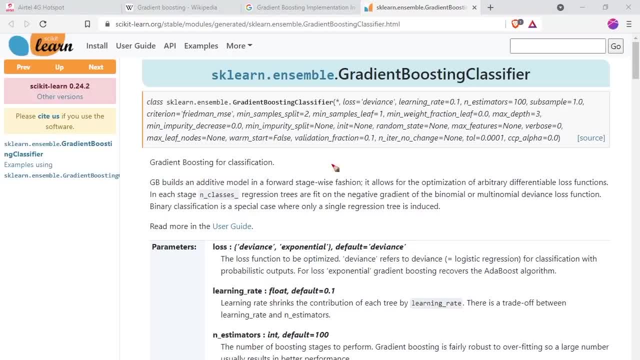 now let's see the some of the parameters that we are over here. So here that you have a loss, that you have a loss which is the deviance. deviance refers to the log loss and exponential refers to the, which is just adaptive version, which is, if you set exponential, then your gradient boosting will go, will be, as will be called as: 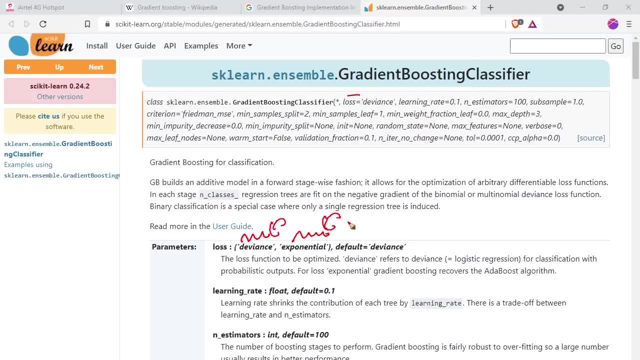 adaptive boosting or adaptive boosting: Okay, so in adaptive boosting, it is more prone, leave will see the implementation. So in adapt boost, it is more prone, only focusing on unclassified. Okay, more more prone only focusing on unclassified. but it's not being used too much. 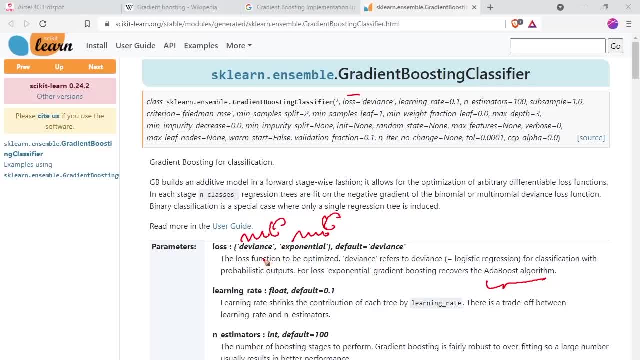 Okay, so we have a loss equals to deviance, which is it was a legislation, laws or log loss. Okay, then you have a learning rate, means the rate to string the contribution of each tree by learning rate. Okay, so this is used. 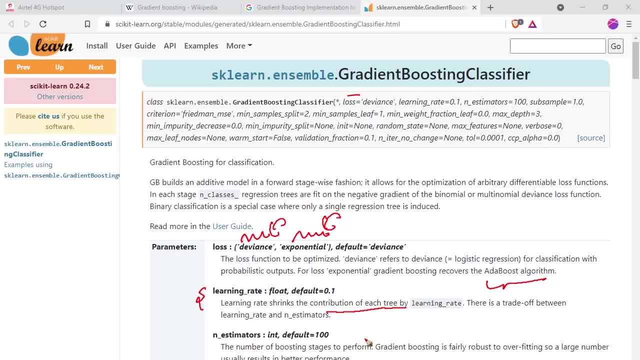 reduce your uh over uh variance. okay, so that's your model. does not start overfitting. okay. so, uh, the serial learning rate, which is default, 0.1 and leave it 0.1. okay, because it's found that muslim dramatically, that they work best in most of the cases. and then you have a number of estimators. 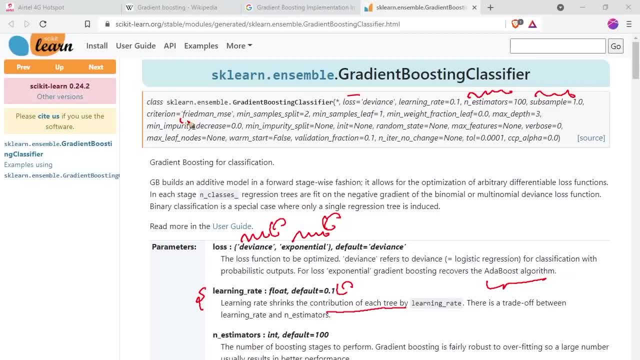 which is number of decision trees, sub sample criterion, min sample split, min sample leaf, min weight fraction, max step for each stream, min impurity. these are particularly for each trees. and then you have uh- let's see something more of uh- that we have a validation, internal change and 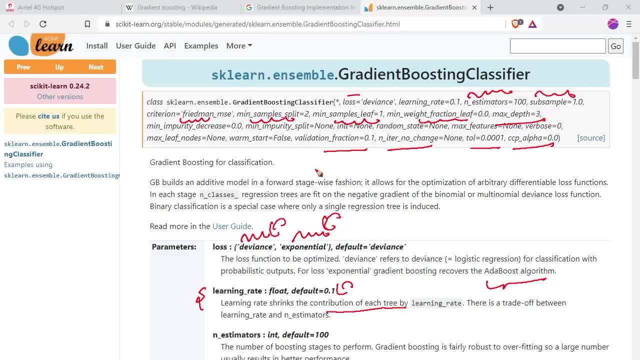 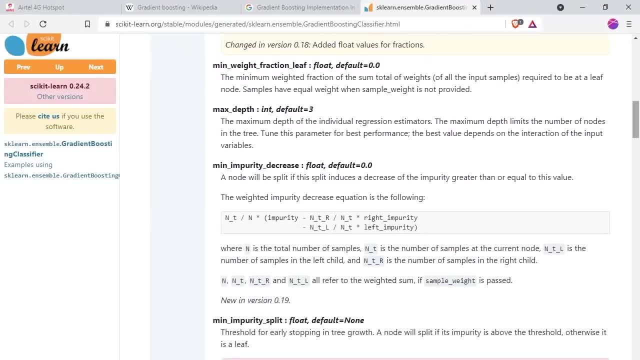 the total ccp alpha. that's not not too cool. okay, so we have this and these are some of the hyper parameters that i know that you had understood everything. okay, so you can see more about this in the parameters in detail here. but we have already talked about decision trees already. okay, 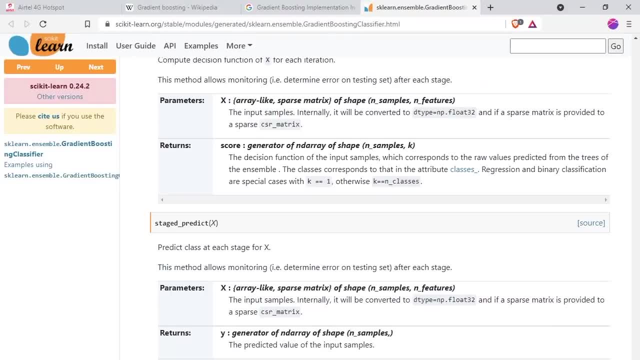 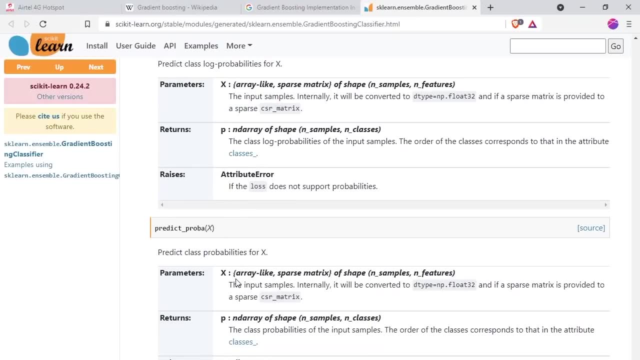 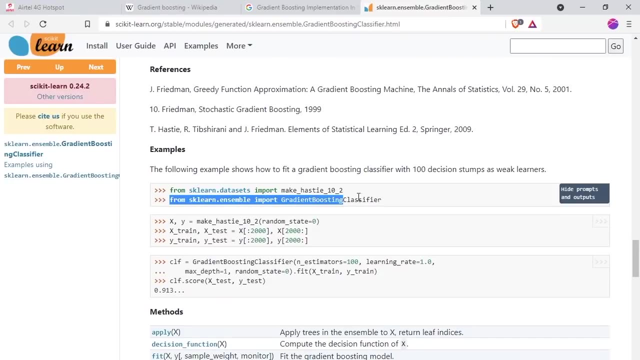 so let's see the implementation means the implementation of this. uh, gradient boosting is just one line of code which is here and you can use predict probability. it simply gives the probability of that being a true okay for that class. okay, so first you import from a scalar dot ensemble. 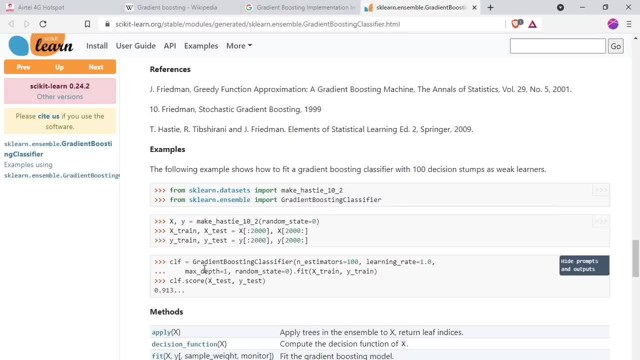 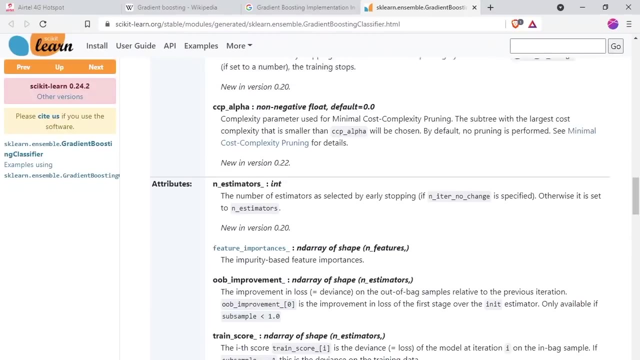 import gradient boosting classifier. here is your data means and then you call your with n estimators: learning rate 1.1, okay, 1.2, max step, random state, and then you fit it and then you get your score okay. so that's the basic intuition behind a gradient boosting. 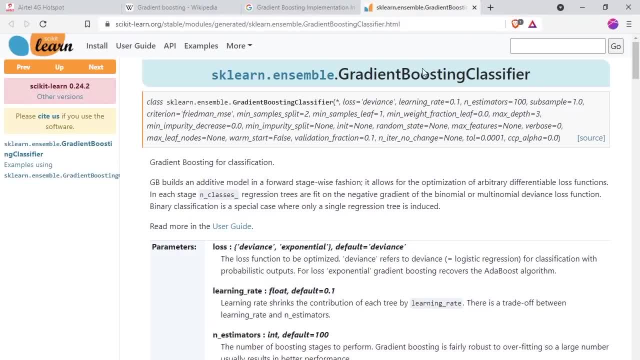 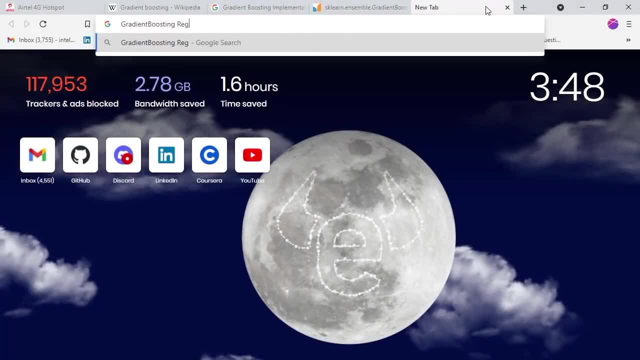 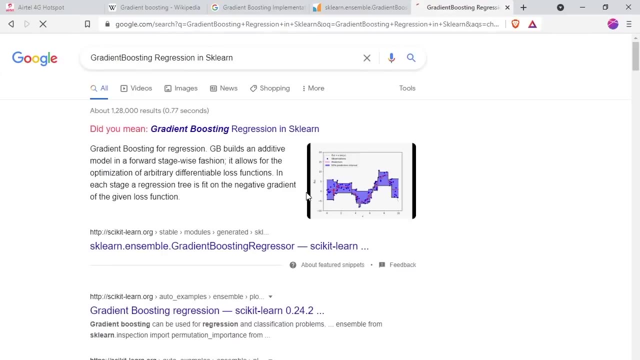 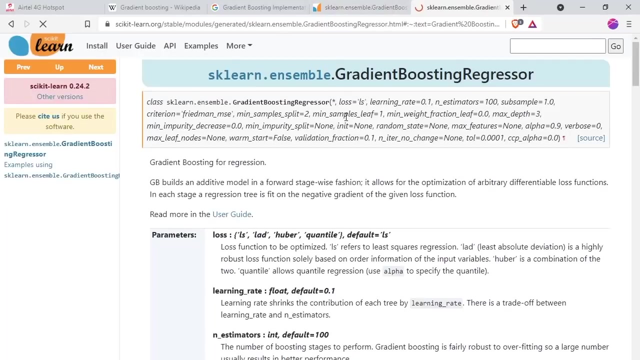 uh classifier. okay, now let's see the gradient boosting regressor gradient boosting regressor regression and sk learn okay, so this is a very good to learn from the documentation. okay, it's very good to learn from the documentation, so let's see. okay, here. here we are on uh documentation of a cycle. learn api. now what we will do. we will just uh. 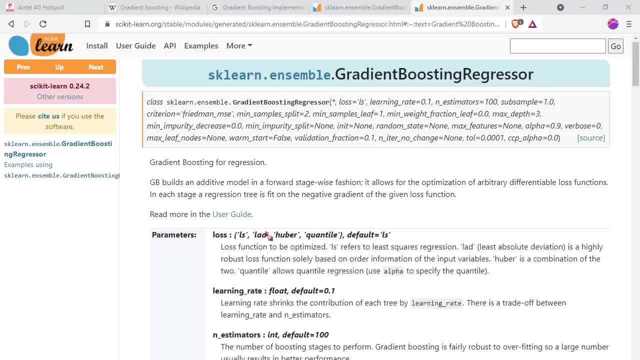 let's use the pen and then you can see over here that we have a loss function to be optimized means ls. that refers to the least squares lad, means least absolute deviation is more robust. okay. so if we have a mover, then you have a quantile, but the default is ls. okay, then you have a learning. 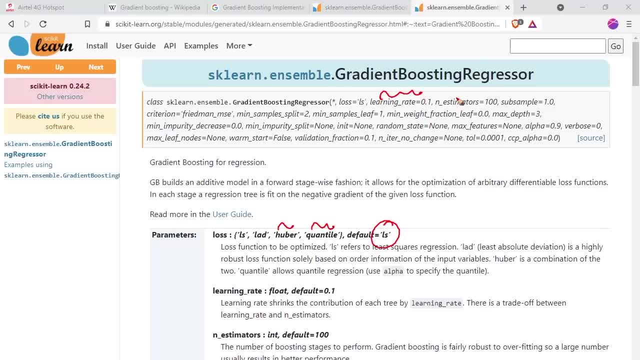 rate, how, for how much? this is a for shrinkage. then you have a number of estimators. then you have some sample criterion, mean sample split for each particular decision trees. these are for each particular decision trees, and then the same thing that we have seen so far. okay, so now, uh, we are uh. 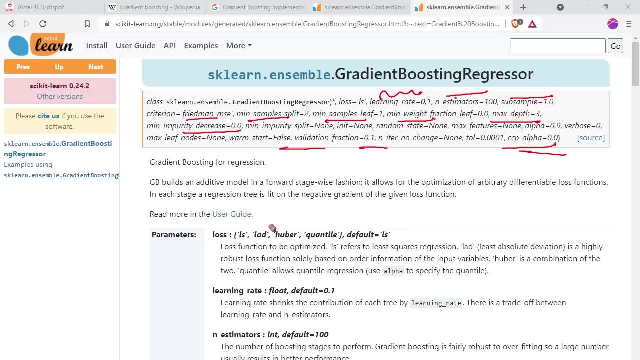 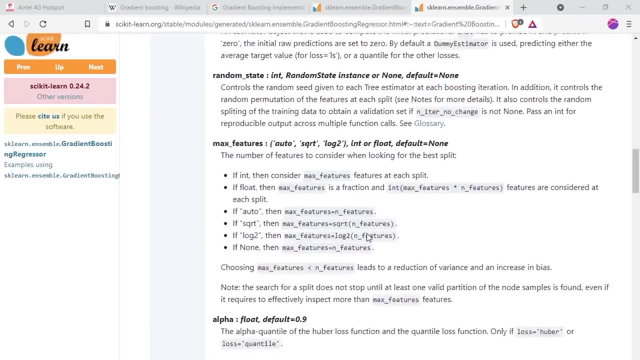 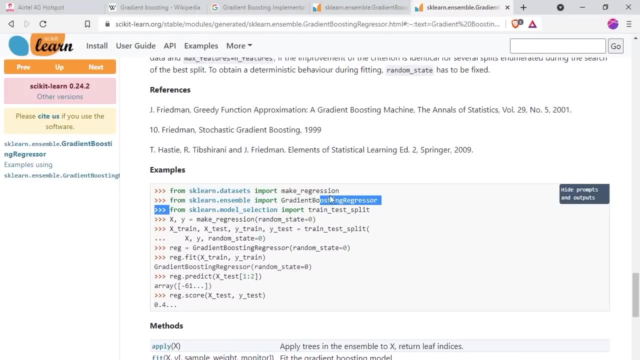 this is the basic for decision trees and i hope that you understood okay. now let's uh see the implementation of this. i'm a little bit going far because i have to teach also that xg boost and ara boost, okay, so you just call the a gradient booster dresser, then you call the your train test. 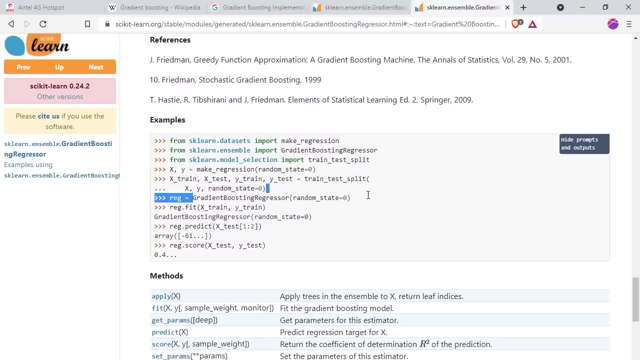 split. then you split your data and then you call your Gradient Boosting Graster with the default parameters okay. then you fit it okay and then you simply do the Gradient Boosting Graster. then you score it and it will use the sum scoring parameter means the log loss, or, I'm sorry, not. 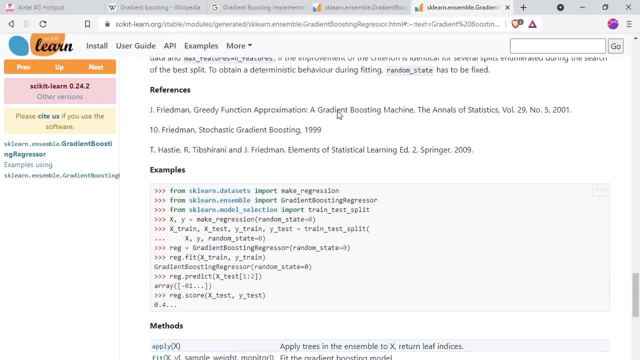 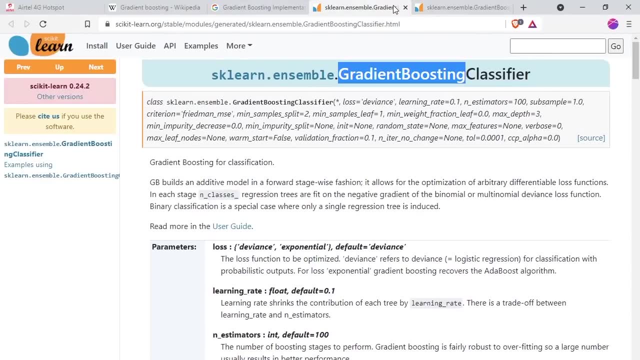 log loss. it may be it uses R2 or MSU. you can see, okay. so that's the basic intuition behind how we implement a Graster and Classifier, which we will do in project, just to showcase you how you can assess from documentation. it's very good to learn from the documentation. now it's time for learning. 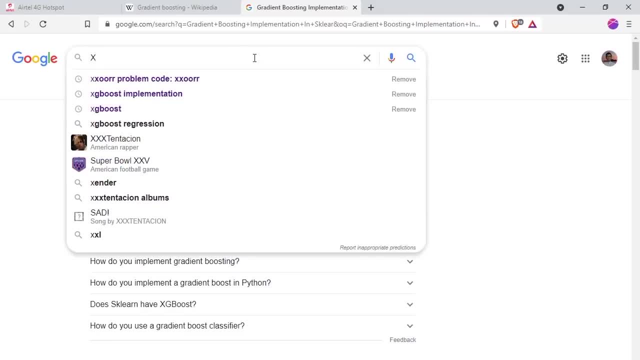 from for now. it's time for to that. we'll learn about. XGE Boost we'll learn about, but before that, let's you, let's learn about ADAPT Boost. okay, ADAPT, ADAPT Boost. so let's see the oops I 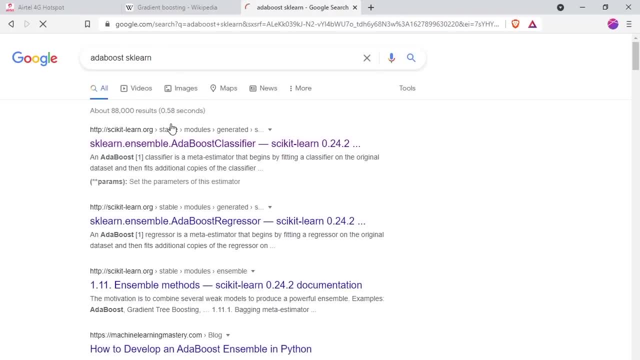 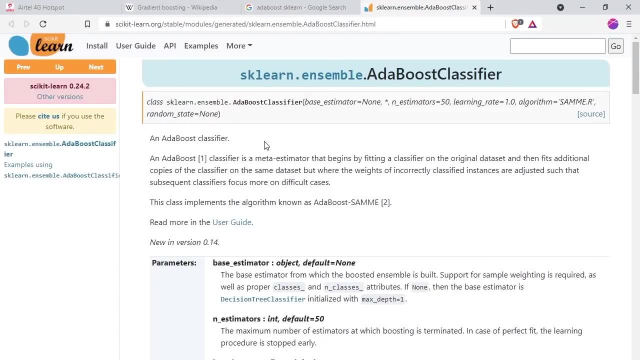 won't implement SKLearn. okay, so if you set your loss to be exponential- okay, to be exponential- then it will be equivalent to ADAPT Boost Classifier- ADAPT Boost Classifier. okay, so it will set your loss to be like this and it's just the same as that we have already. 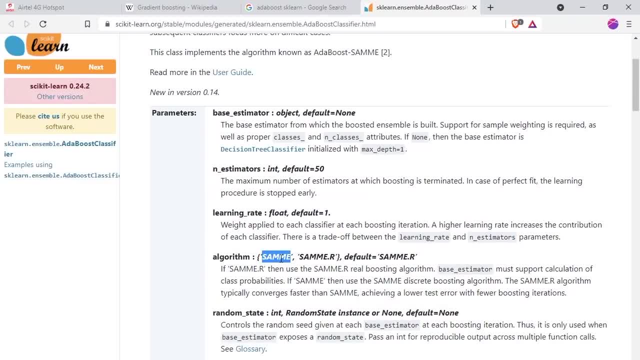 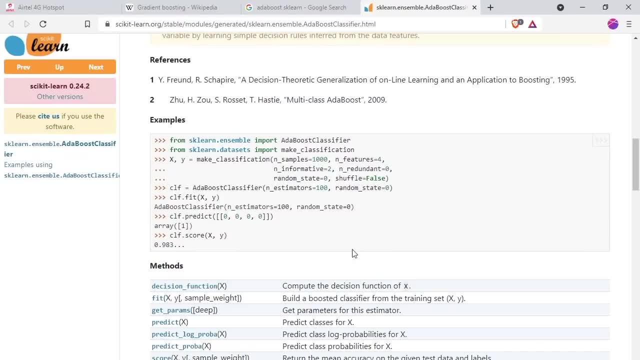 talked about. we have two algorithms given by SAMI and SAMR, which is, and SAMR, which is also for Legit regression, if you have seen as the Cycle Learned API. okay, so how you implement from ADAPT Boost Classifier, then you call this and then you fill your model and then you are done. 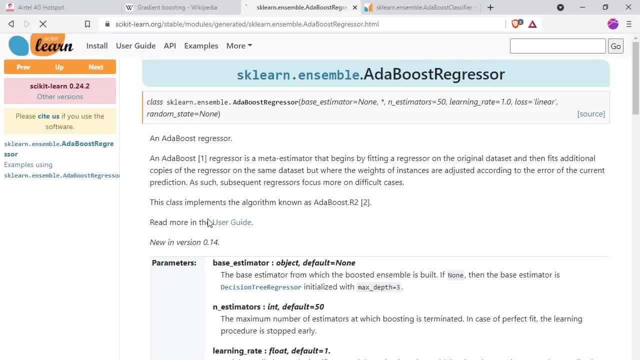 okay, it's very simple, so let's see how you implement it. okay, so let's see how you implement. I think that you but just remembering the concepts is very, very important, because it's not always you have to implement maybe your own something algorithm in your company. okay, 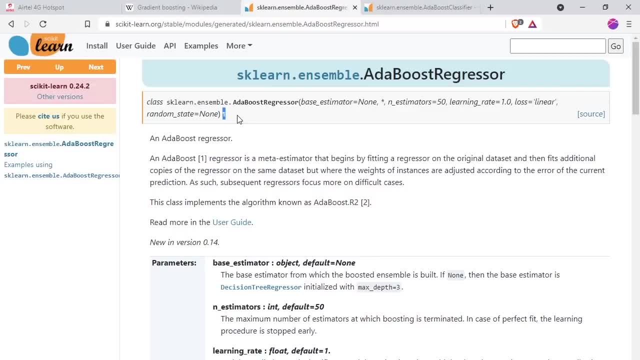 you may think, yeah, you just can't, we just study the implementation. no, no, you cannot study. okay, but Cycle Learned API is very, very slow, very, very slow, but it's great. but what you can? 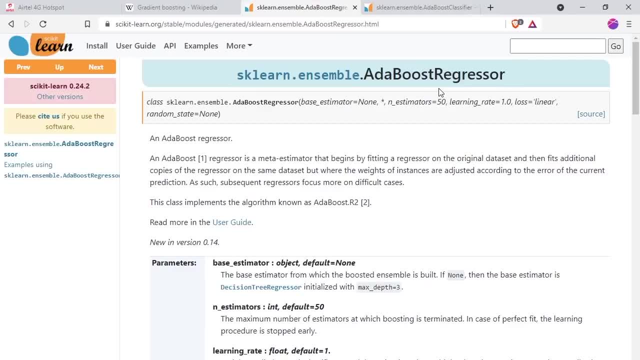 do you have to in some companies for production, because there's a Kaggle winning algorithm that we. what is happening? how we can tune the hyper parameter? okay, so here you can see again for the grasser: okay, and here you have a loss equals to linear, and then 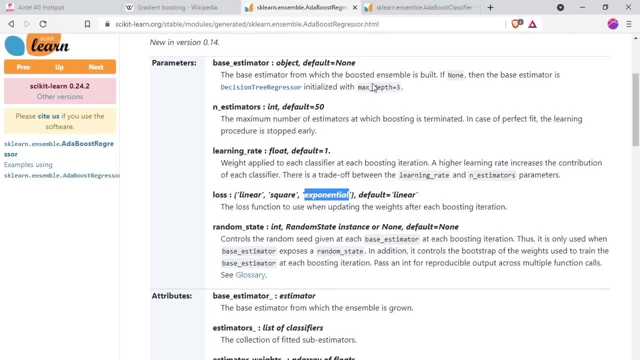 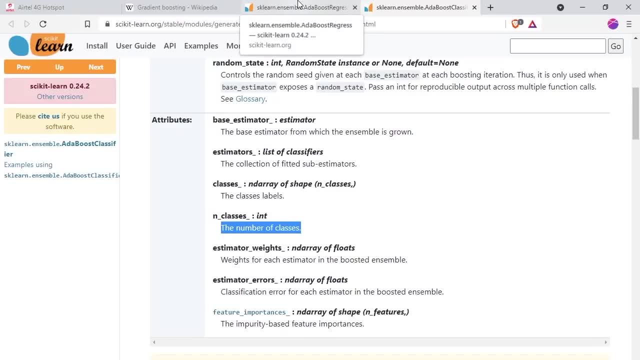 you have a square and then you have exponential. okay, and here maybe we do have a not loss. you can see, state the number of a class is how many number of the class if it is classifier. okay, so now we know about this and I really hope that you understood the following. now it's time for learning about extreme. 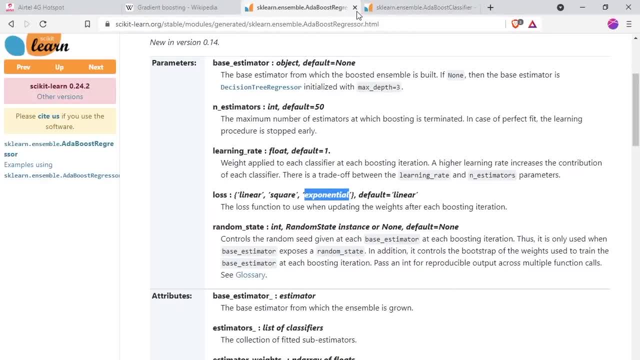 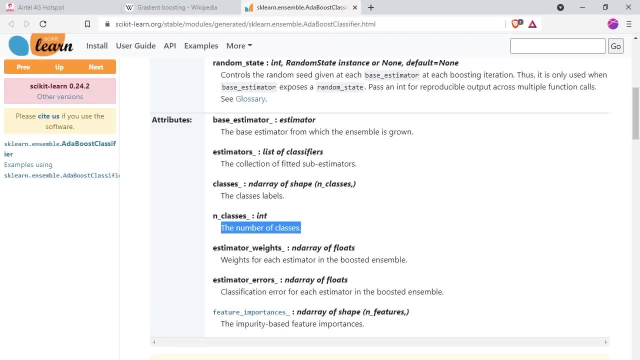 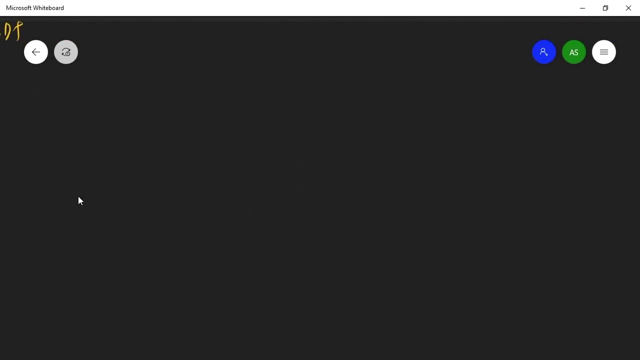 boosting one of my favorite, but I think our doubles is not used in production. many not uses too much in a production act. maybe not right over here, but I think so. okay, so now we will learn about X G boost, which is one of the most popular algorithm which I have seen so far. okay, 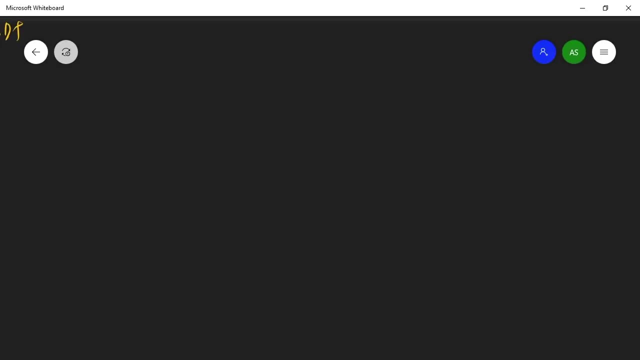 Minza RT. ok, it's good, It's a. it's a good algorithm. It's a good algorithm, but it's one of the best algorithm that wins your Kaggle competition. Okay, so now we will see what XC boost us. It's just the advanced version of gradient boosting. 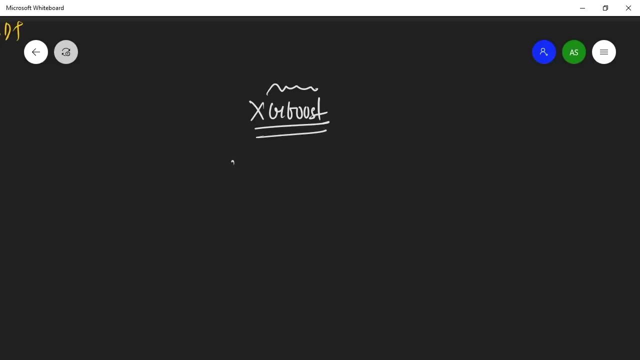 It has. it is. it does have the radiant boosting decision trees, plus it has randomization, with row sampling plus column sampling, and so in gradient boosting We are not doing this, but it's at randomization, which is row sampling plus column sampling. So that's why we name it as a extreme gradient boosting and works best. Okay, it's works. 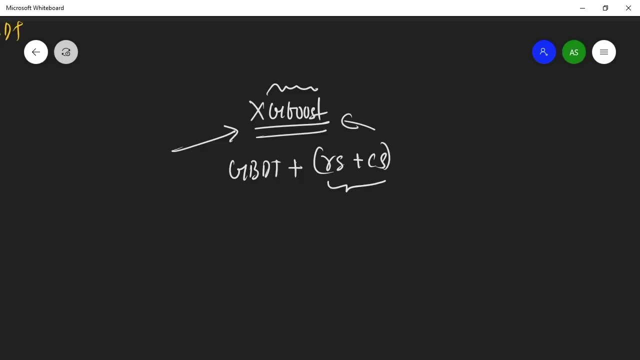 brilliantly Since some cases and machine learning problems. okay, but it needs fine-tuning a lot. Okay, so the gradient boosting decision tree. you know, you have a row, It's just how we differ from gradient boosting decision trees. you have you do the randomization. 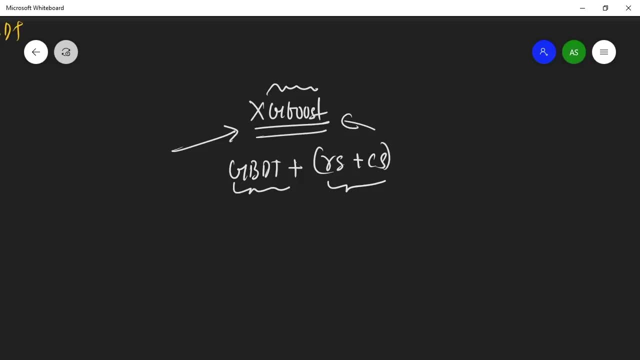 by doing feature bagging and Then you have a row sampling. Okay, and it's just for a simplicity. Let let me explain you what we tend to learn about this. what we do: We simply sample the rules as Well as the columns for our data. okay, okay, in in the specifically for bagging. We don't know columns. 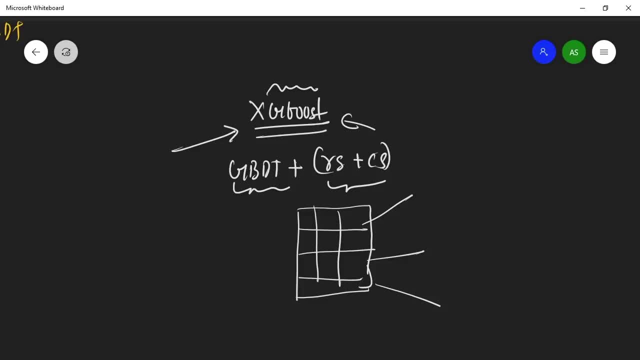 We don't do column sampling, but in a random, random forest we do both. So in XG boost we do the gradient boosting decision trees as well as a random forest plus Column sampling. Okay, so that's the, that's what we do: randomization and that's the XG boost. 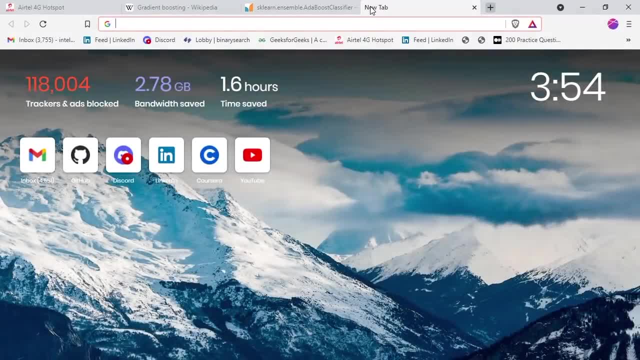 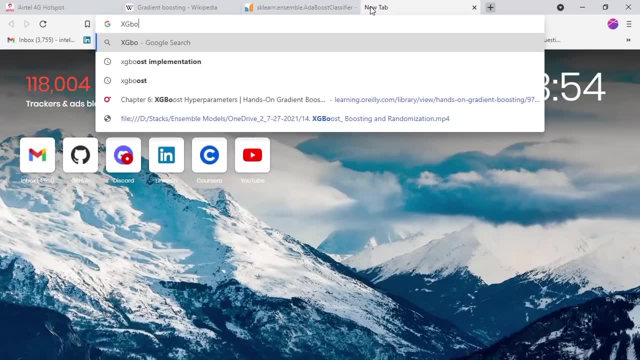 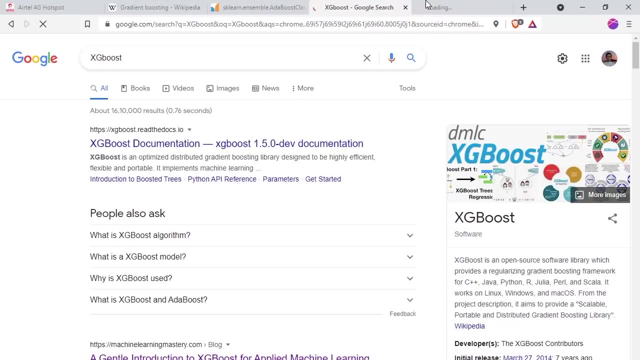 Okay, so now we will see in detail What actually the XG boost implementation. XG boost from the official documentation: Bust, but it is all. it is all. it is, of course, simply implemented in the. It is, of course, implemented in cycle or an API, but it's. 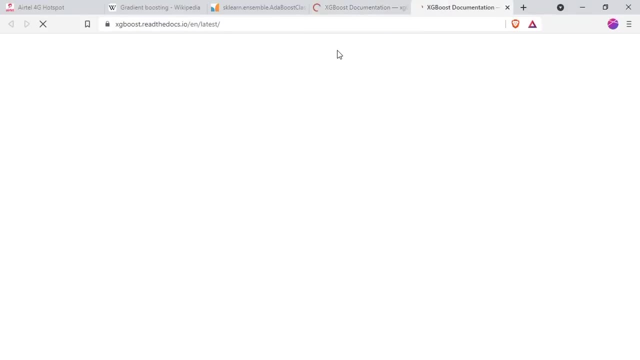 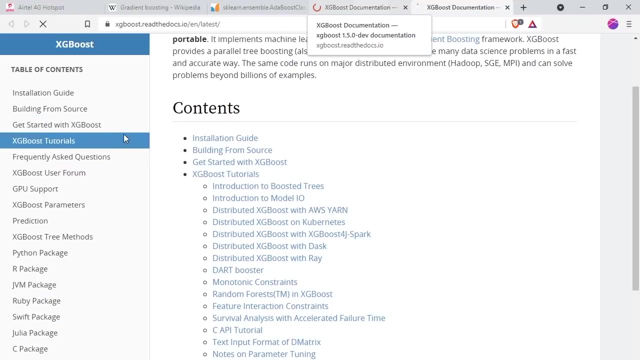 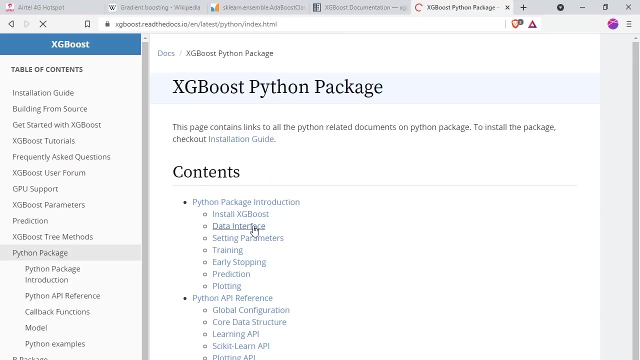 But it's very good to use because there this is fast. Actually it is fast. Actually. it's a very good to learn from here rather than there. Okay, so I think that we can found get us Python package, because we have different, different package now. 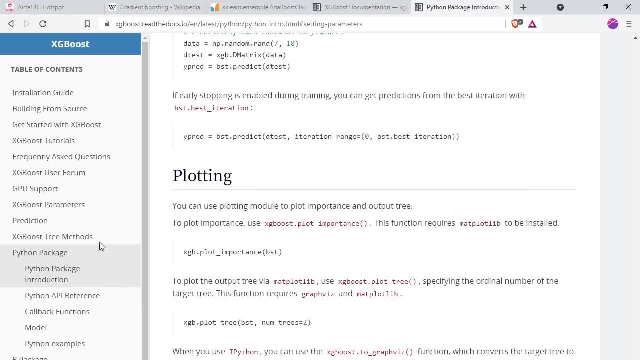 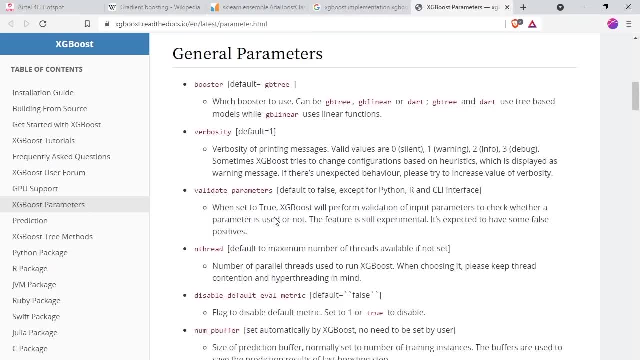 Setting parameters. Oops, where it is XG boost Python package. Okay, so here we have some parameters and XG boost. I think that my brave is not working after again switch to my favorite Chrome. why I have switched to this? It's bad. X brave is actually not good for me. 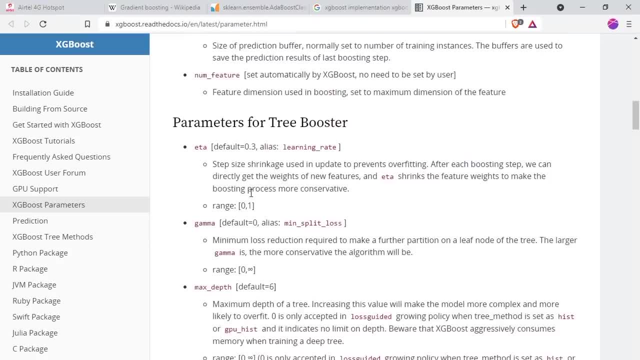 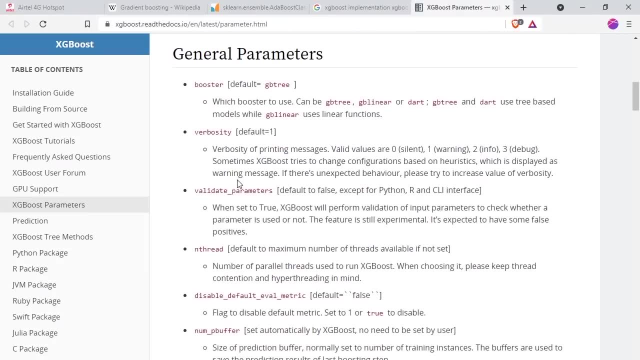 And since some kids actually I'm like who am I say to say bad but screw good, But it's all. of course sometimes it does very bad, Okay, so let's see some of the parameters. Let's see some of the parameters. so we have different, different packages that we 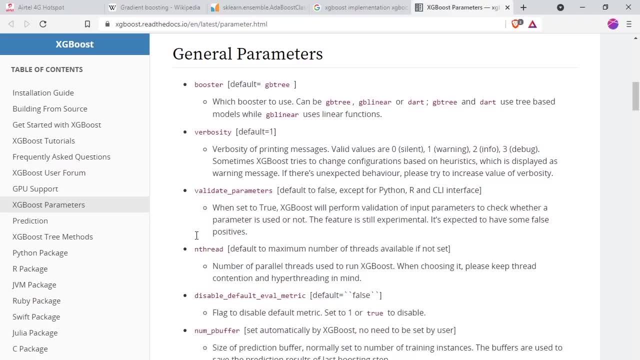 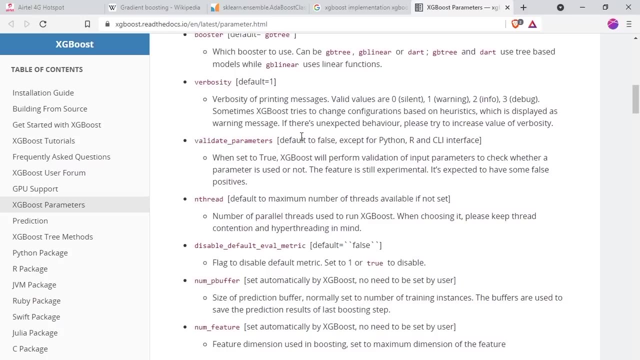 we had that already been implemented, this algorithm. so here you have booster, which is gb3 means gradient boosting tree. you can use a gb, linear or dart. the means we use will use gb3. then you have a validate parameters default to false means. it's just you want to validate your. 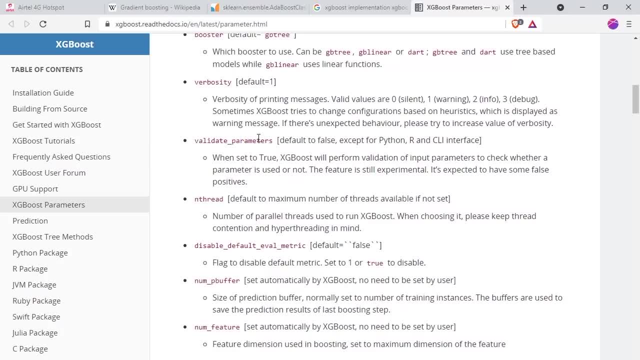 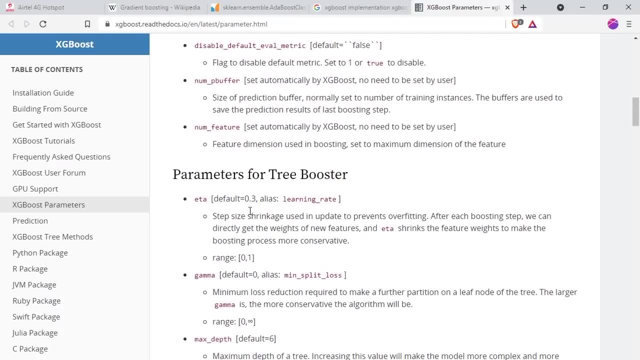 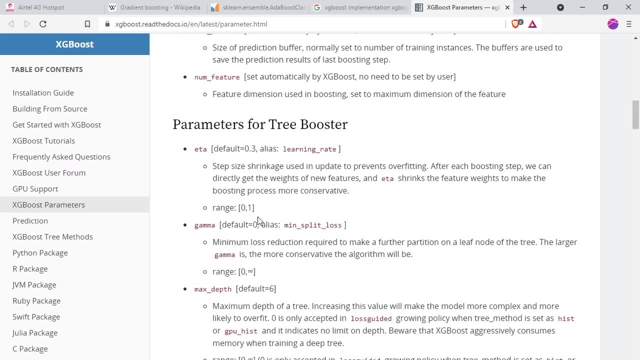 parameters or not. then default to maximum number of threads, then you have an evaluation metric. then, uh, etom is learning rate, okay, is 0.3. okay, gamma, which we have seen, which is the constant, which is zero as default, and it's just, uh, it's just randomly initialized means. and then we 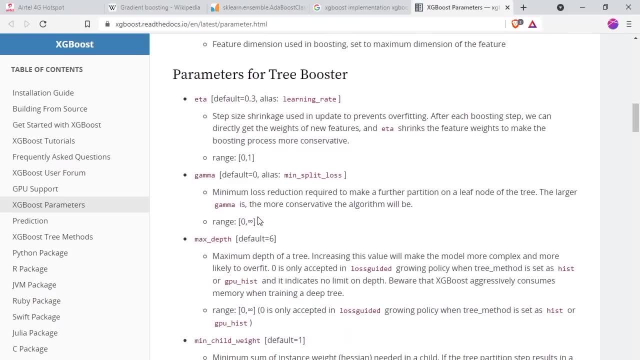 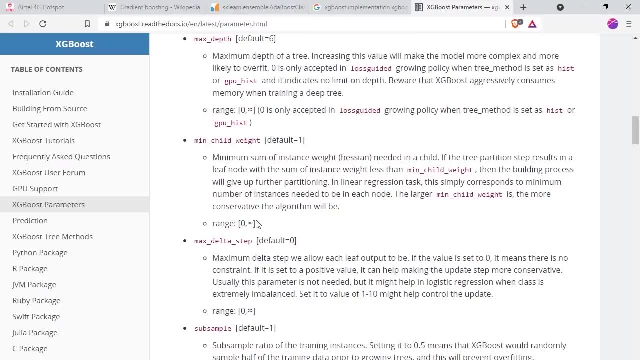 find a good like gamma. and then what is the max depth for each tree? and you can read the documentation of your more minimum child weight. minimum delta step means: what is the step should one uh maximum delta step we allow each leaf output to be? if it means there is no constraint, okay. if if means it's just like that, it's just uh. 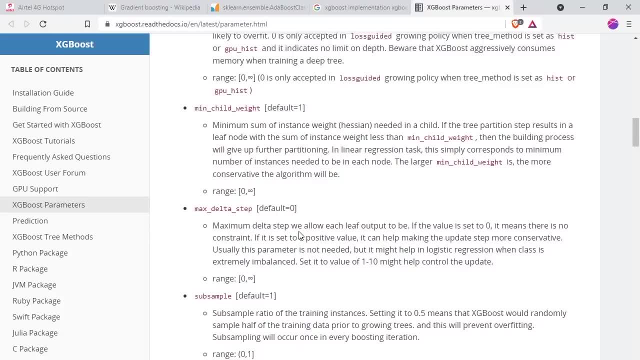 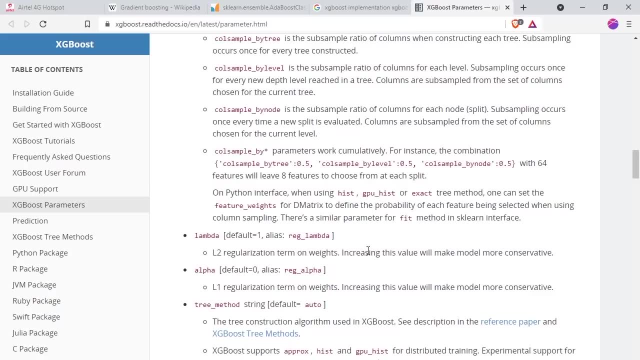 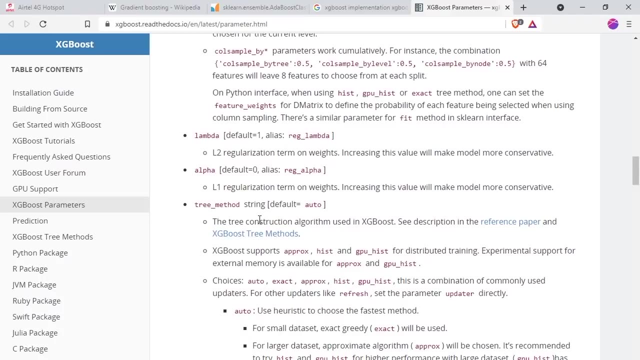 helping you to not too much proning to overfitting. it's a more robust model. okay, so you can see your lambda means l2 regularization like a lasso, and this is for regular uh regularization, that is, alpha regularization. okay, then we have a tree method which is exhibits construction uh algorithm. 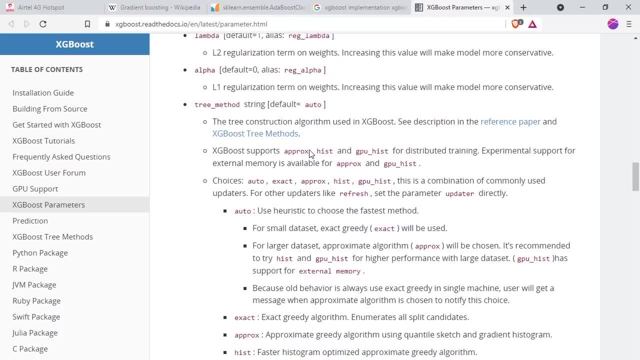 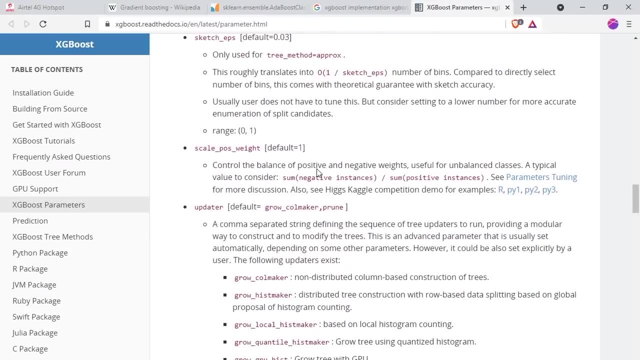 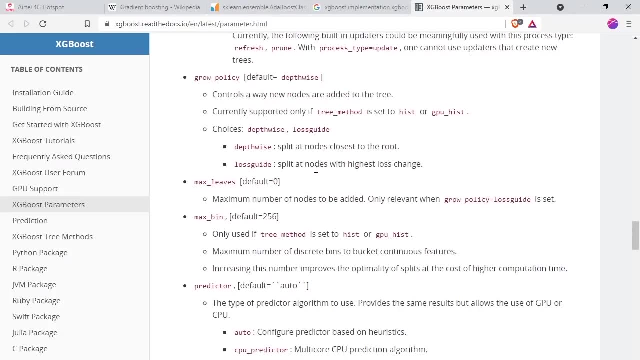 boost. you can see the reference. you can see, obviously, see the reference. it's also supports: uh, hist and etc. then it's a have a scale post weight updater which is process type, grow policy, maximum number of leaves, but it's default to zero to be added. okay, so max bin predictor. then we have 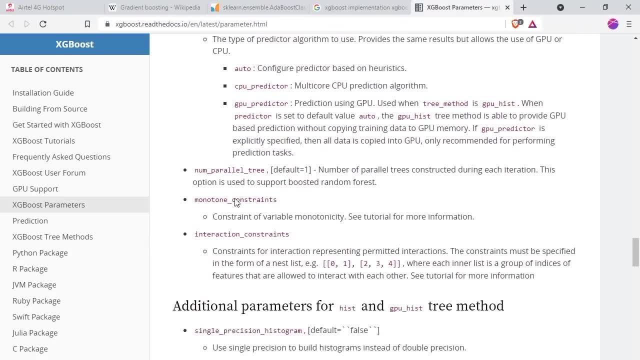 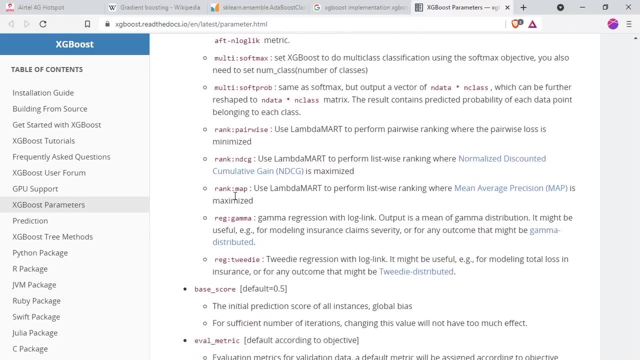 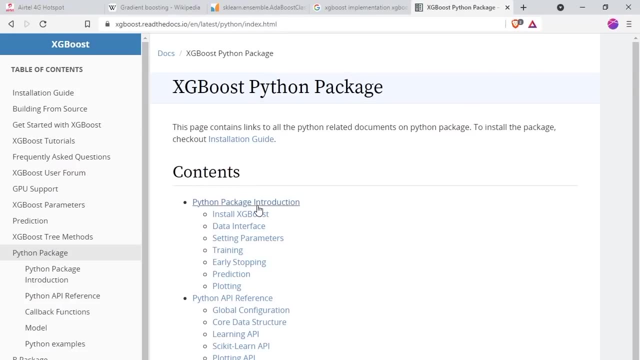 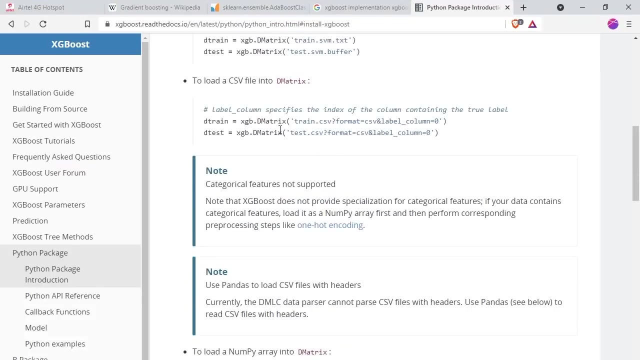 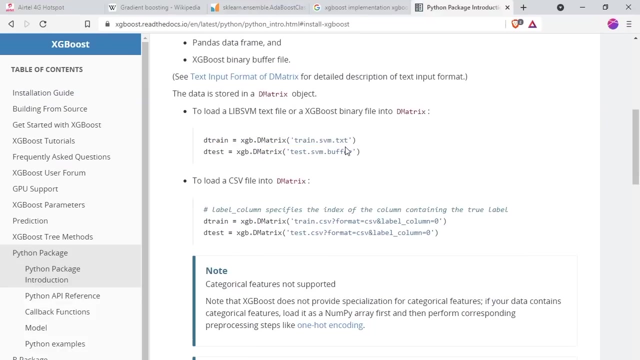 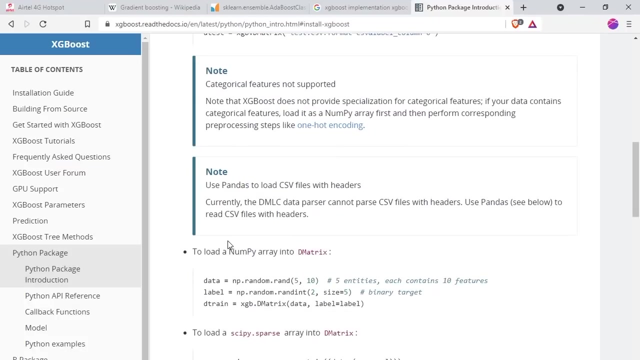 a gpu cpu, but this leads a lot of fine tuning. it takes a lot of time in cpu, okay, so we have this much and you can see more about this in the next video. so thanks for watching and i'll see you in the next video. okay to use it, but you can see over here implementation. 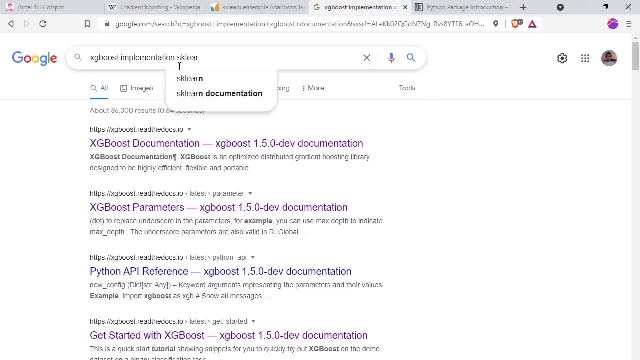 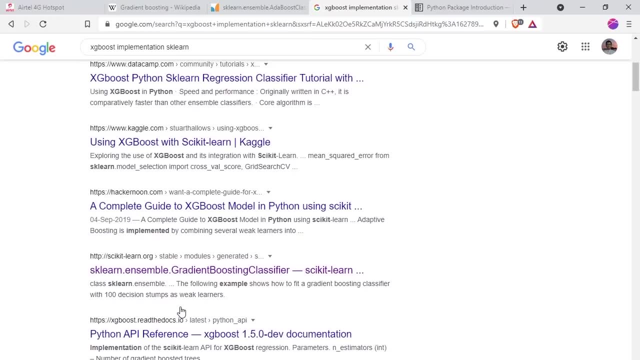 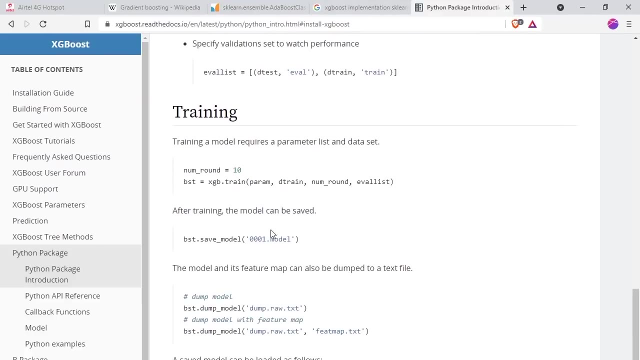 sk learn. it's also for a regressor that we have seen. i think that we had. they have removed. i think not. they have, they haven't removed. no, no worries, so you can see from here how it is used and how we train this model and how we save this model. uh, it's just like a neural. 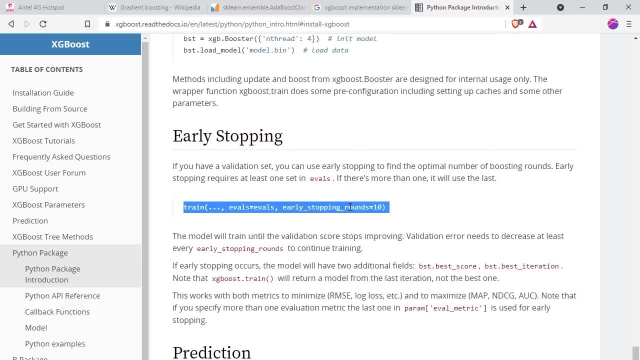 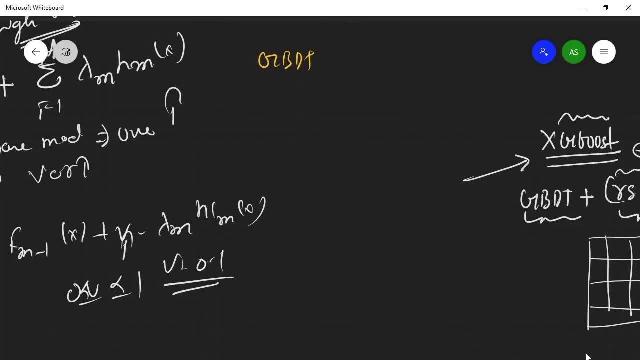 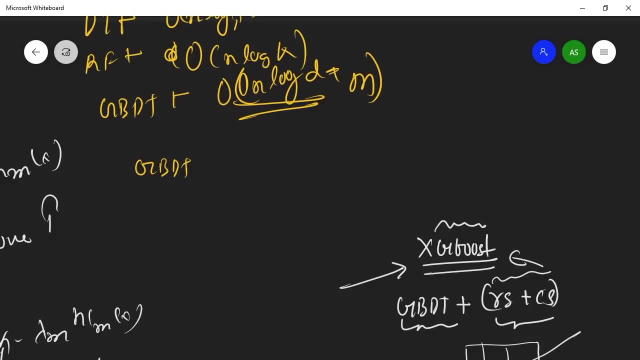 web, as you. as you know that uh, tensorflow has also added decision trees and, like that, in sample, started adding because one of the most powerful algorithm in sample learning- okay, so we have seen a lot in in in decision trees. okay, sorry, in ensemble learning I get bagging and boosting, okay, so now one last step is left is stacking. 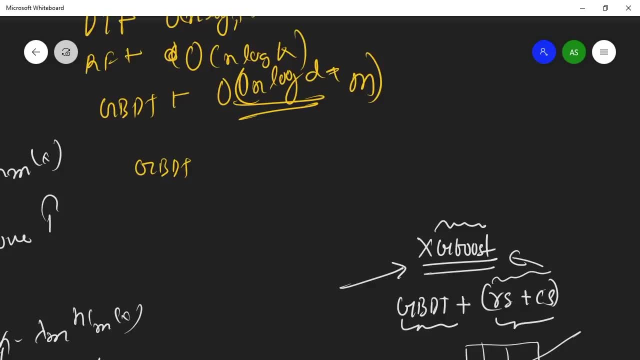 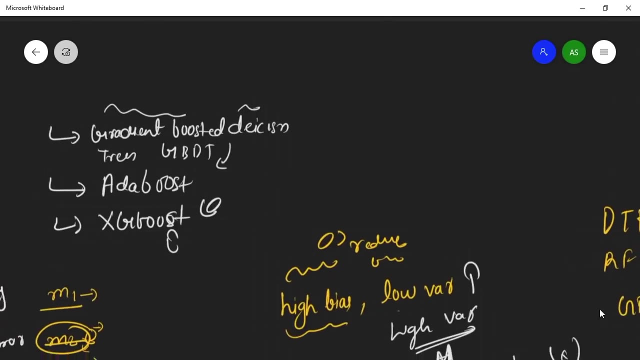 of your stacking. okay, so after this section, we will start with a stacking to help you to better understand what actually stacking is, and it will obviously help you. okay, so we have seen a lot of applications of this and I really hope that you enjoyed it also. okay, so this, this section, is just 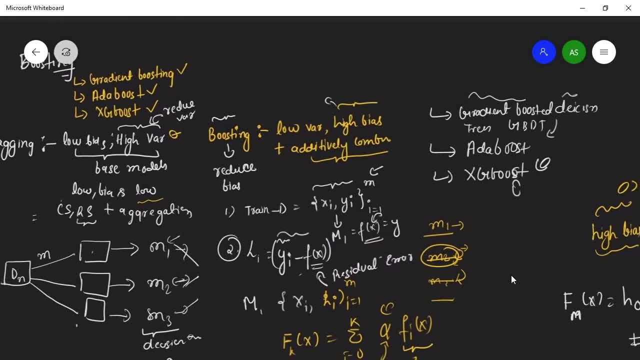 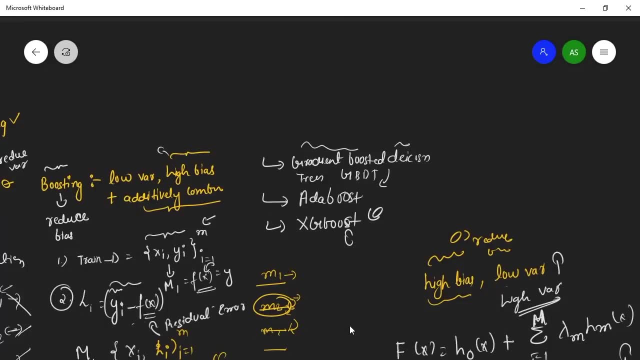 amazing. we have learned about boosting and we have learned about gradient boosting. they are adaptive boosting. then you learn about XG boost. okay, and so one of the project will fine-tune, will use XG boost at a boost with fine-tuning. okay, one of our project. 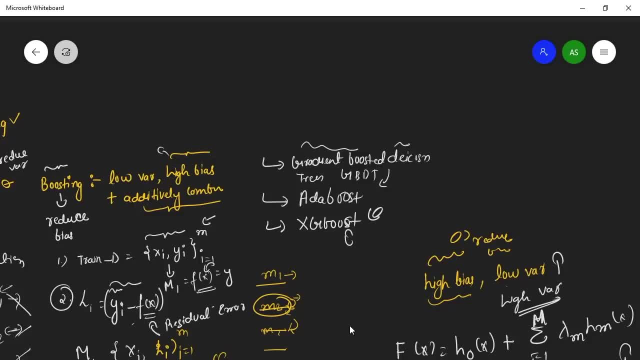 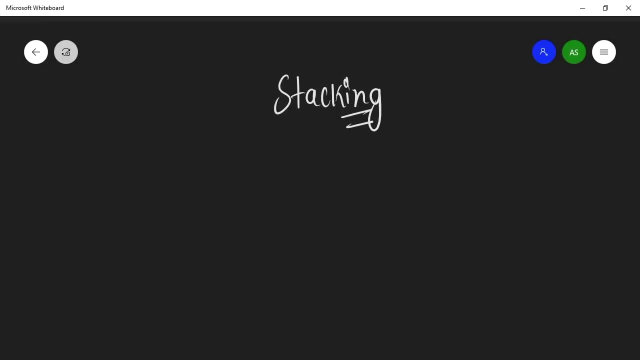 okay, so the that's it for this section. in the next section will start with a. stacking is up 118, 20 minutes section on stacking will take, and then we just with some other summary or revision of ensemble learning. okay so, let's meet at the next section. okay, so now we'll talk. 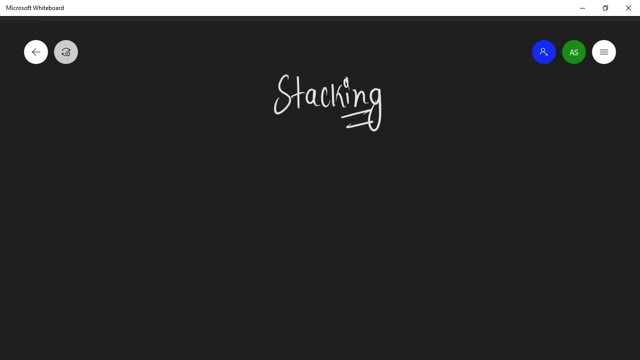 about our loss ensemble learning technique, which is called stacking of our models. okay, so we will see the implementations of stacking, so, and we will see how it works and how it changes your accuracy. okay, so let's recall something called as bias and variance of our bagging and boosting. 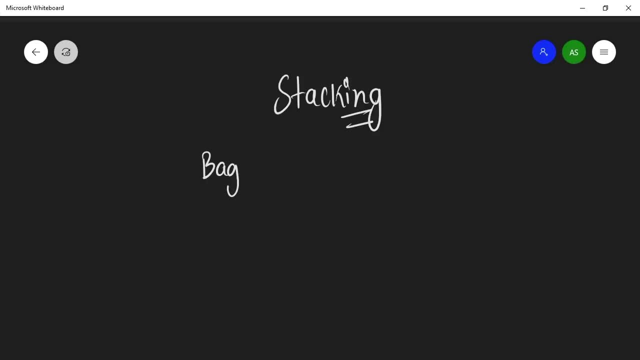 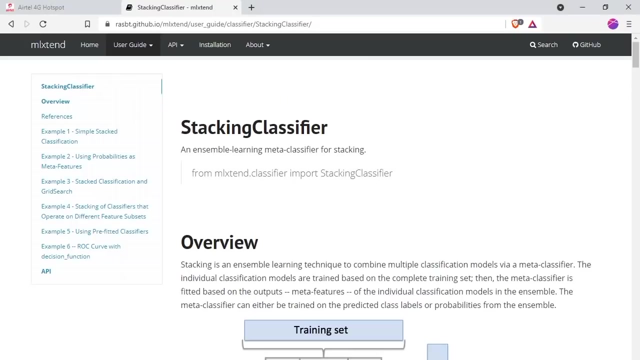 okay. so when bagging, in bagging, we have high variance, high variance and a low bias trade-off, okay. and in boosting, and in boosting, you have low by a high bias, high bias and low variance trade-off. okay, so remember these two for stacking, okay. so here I am. I am on my MLS to extend, which is a library for 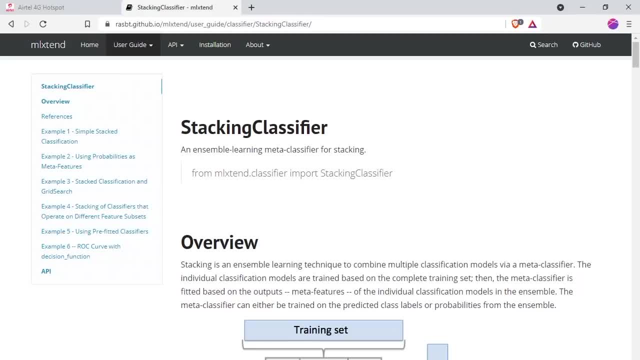 implementing the sacking classifier. okay, so you can. we will see the implementation of this stack inclusive fire, but before that we will learn well how actually stacking works. you can get to this page by just going on an MLS 10 stacking pacifier and click on the first link. okay, so let's start. so here is our data. 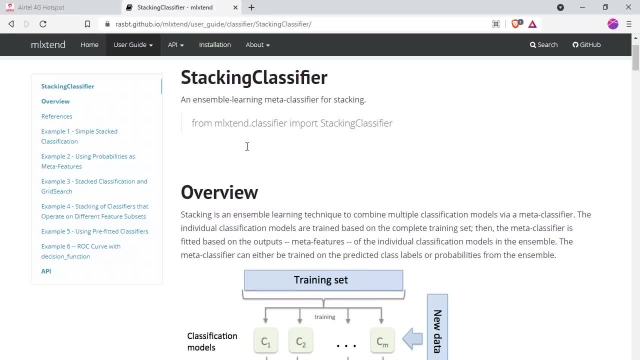 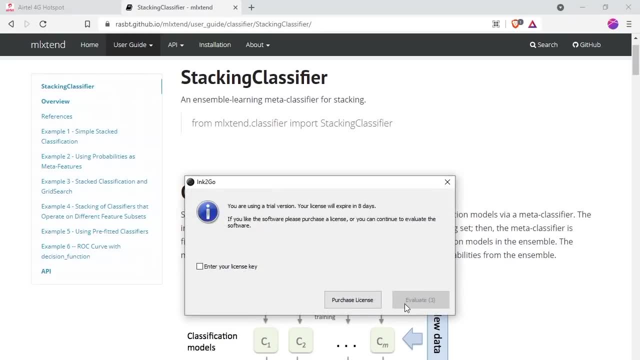 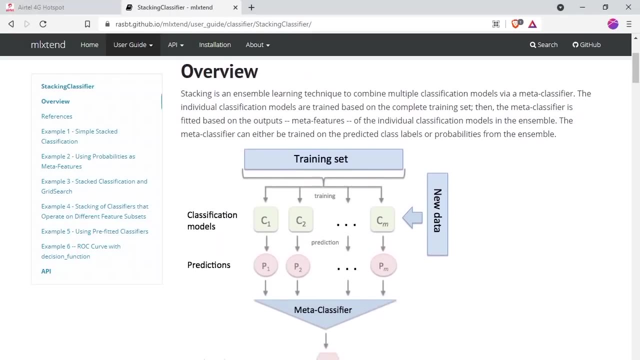 set. here is our data set. so let me take out my favorite in to go. I hope that you remember my favorite in to go. sometimes I roast it also, but here it is very good just for annotating these kind of things. Okay, so here let me take the pen. 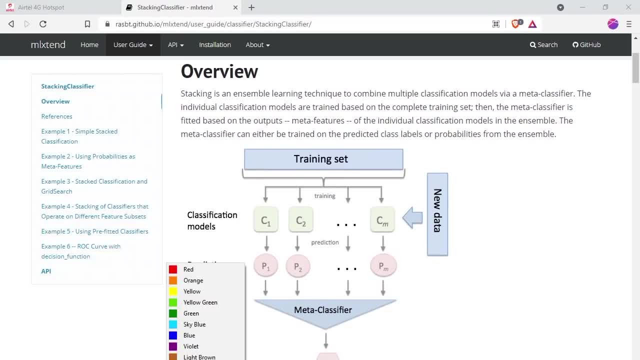 As of now. let's take red, which I like a lot. Let's take medium, Okay, great. So here, in bagging what we were doing, we have a large training data. We have a large training data And then you multiply. 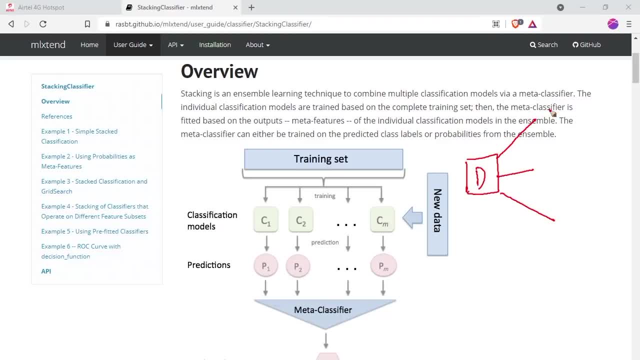 or you're just taking out a subset of this data- d and 1,, d and 2,, d and 3, with the replacement of training, the decision trees or maybe some same-based learners. Okay, so in the stacking we have different, different-based learners. 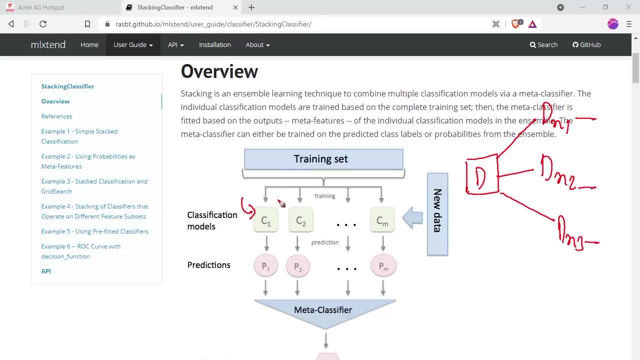 We take out the data, okay, and then we train our model different, different model under each data. Like C1 is a model which is trained on different data, Then again it's on the data D1. Then C2 is trained on D2,. 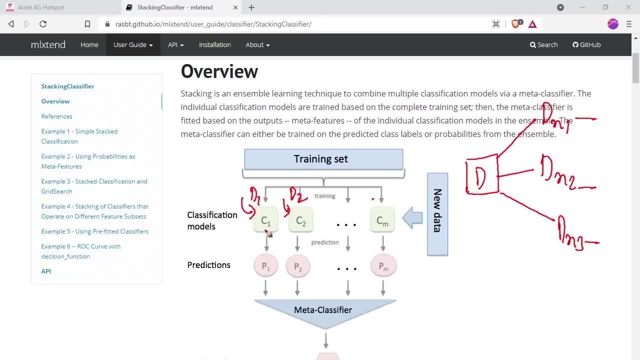 all the way down to the M. okay. So here, C1, C2, all the way down to the CM are different, are different models, okay? So what do I mean by are different models? It's quite simple. Let's take an example. 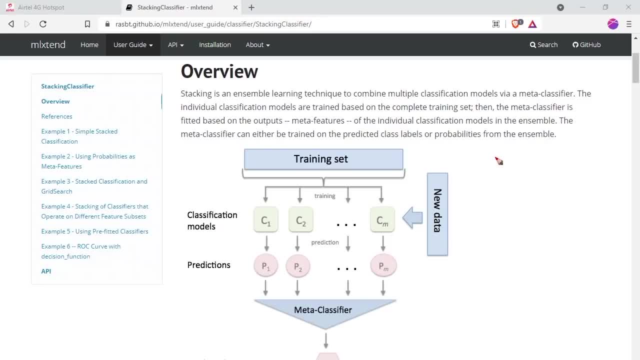 Let's take an example that you have your favorite logistic regression. Okay, you have a logistic regression. You have a logistic regression As a C1,. okay, as a C1.. Then you have your support vector machine as a C2.. 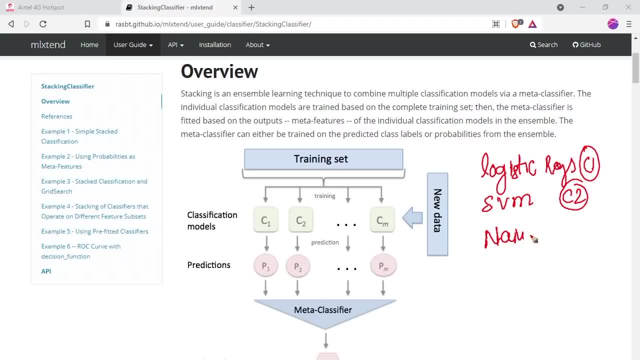 Then you have your favorite Naive Bayes algorithm. Naive Bayes algorithm with, maybe with extensive fine-tuning using grid search, okay. So here we have C3.. Here we have K- nearest neighbors, which is C4, okay. 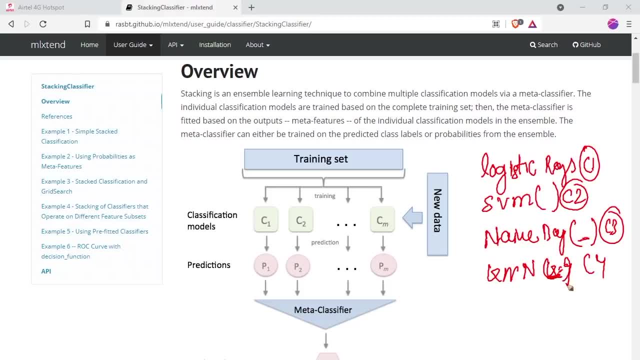 with extensive, with maybe K equals to 4, okay, with extensive fine-tuning, okay, Okay. So here we have four Bayes learners and we have a different logistic regression support vector machine: Naive, Bayes K: nearest neighbors. 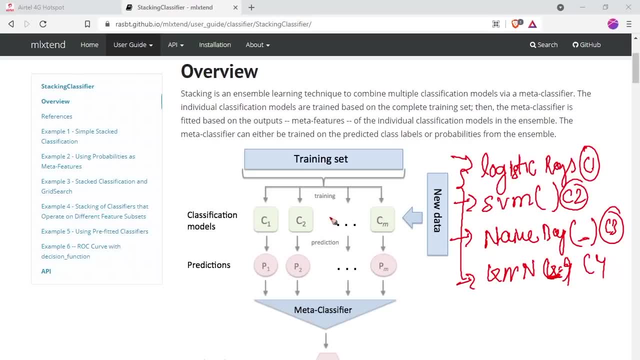 and there are four different models, okay, and a train of different different thing, okay, And the major difference between the bagging and boosting is in bagging. that I've told you to recall: bagging, bagging and stacking is in bagging. we have high variance. 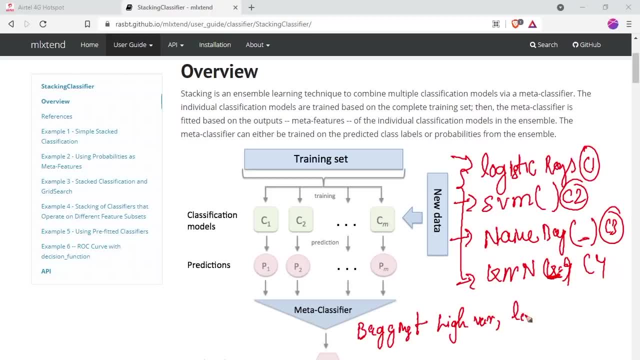 high variance and low bias, low variance, Okay. So we have low variance, low bias, models, which is a Bayes learners, which is a Bayes learners. and in and in bagging we use. we use bagging for reducing the high variance, okay. 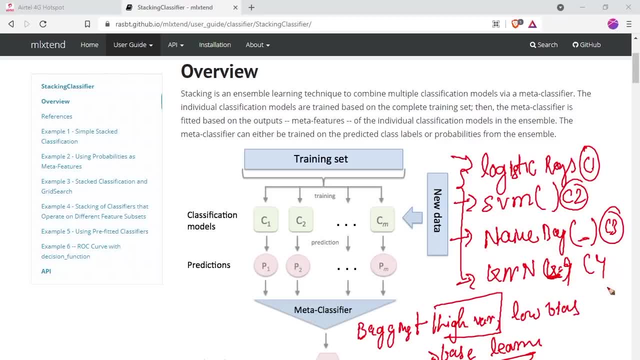 So Bayes learners are usually high variance and low bias and trade off between them. okay. So what is the difference between stacking In? stacking in stacking our Bayes, Bayes models or Bayes learners are highly tuned, are highly well-tuned okay. 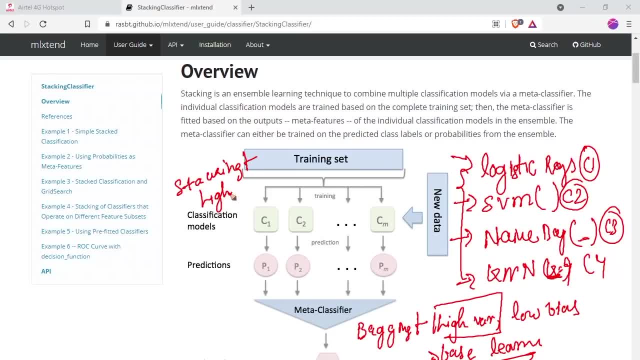 Highly well-parameter-tuned- okay, Highly well-parameter-tuned, and they have a good bias and variance trade-off- okay. So when boosting, so when bagging, we have high variance, we are our Bayes Bayes. learners are not that much good. 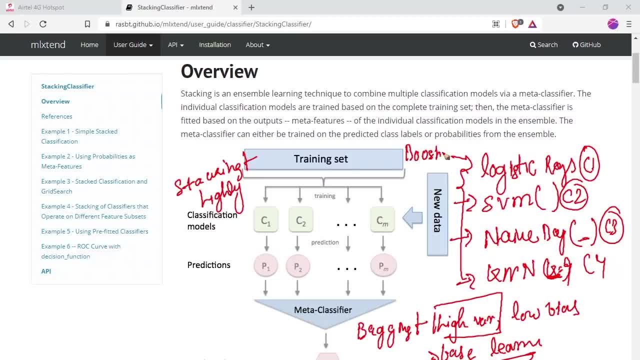 and also when boosting our Bayes, learners are not that much good. But in stacking our Bayes, learners are quite good, are quite good, are very good with extensive, fine fine tuning. So maybe you have changed the legislation- fine tuning with the learning rate. 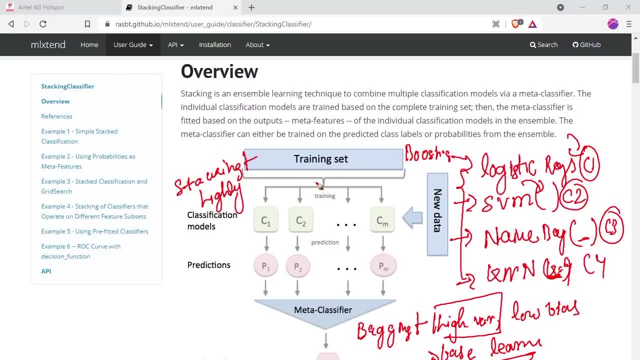 support vector machine like C, your regularization parameter and your gamma and then maybe some of the other parameters. okay, In nine Bayes algorithm we have also done. it's not required, but you have done some extensive fine tuning. You have kin, K, nearest neighbors. we have chosen what is the number for K. okay, 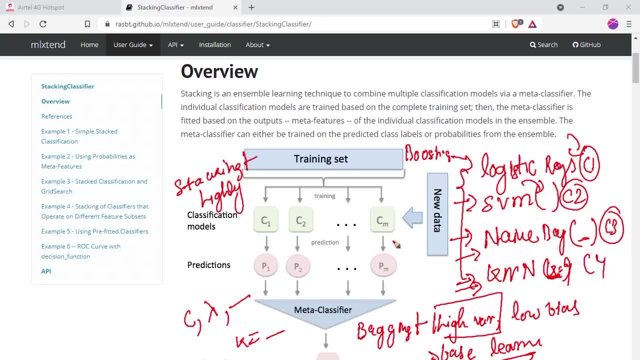 So you have done an extensive fine tuning of your model, okay, So that's part of what I mean Here. I'm taking what a classification example, okay, So here, what, what, what we are doing here. what what we are doing is just we are. 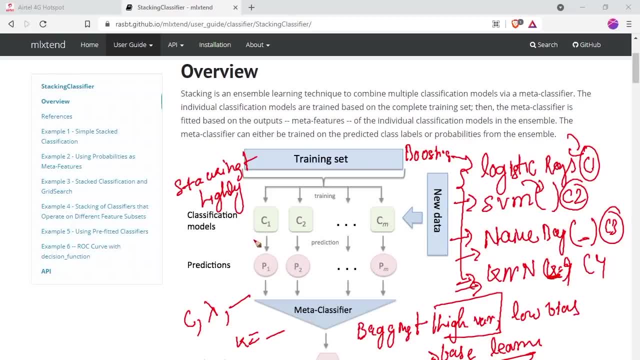 the models are highly trained means highly fine tuned. okay, Highly, very, very, very much a train. extensive, fine tuning are very good models. They do have a very good bias and variance trade off okay. And here it gives prediction. 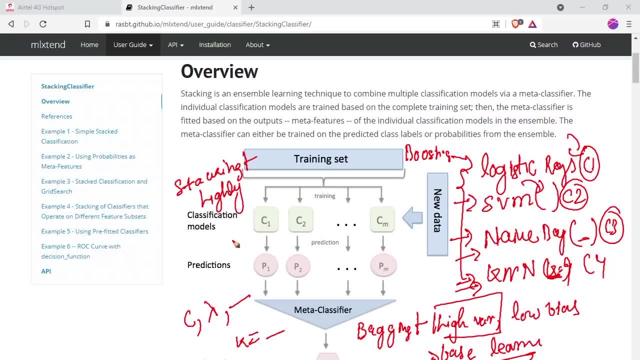 Let's take an example that Y C1 gives you a prediction as a Y hat 1, then C2 gives you a prediction as a Y hat 2. And all the way around to the Y hat M. okay, Each model gives your output, okay. 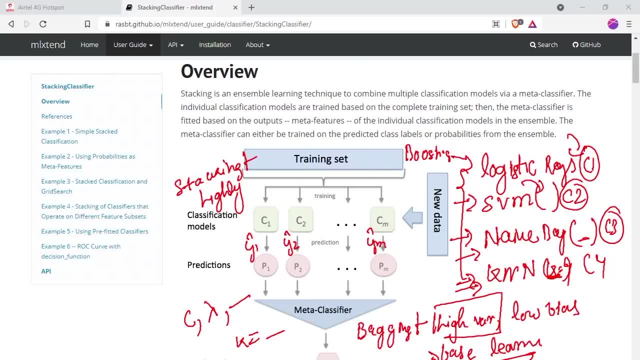 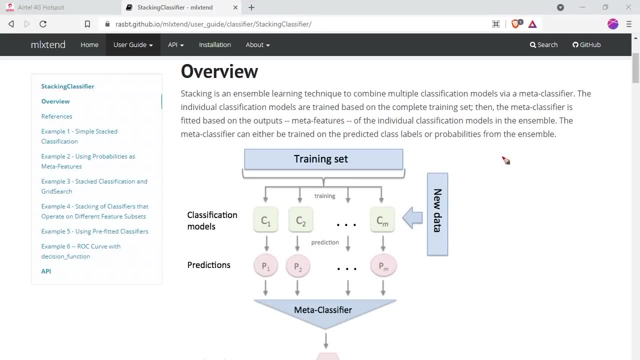 The prediction. okay, So what you are doing, so what you are doing, so, let me do this. So, as a motivating example: so can I delete this if I can? Yeah, let me, let me delete that. So what you are doing, so what you are actually doing, is simply taking your training data. 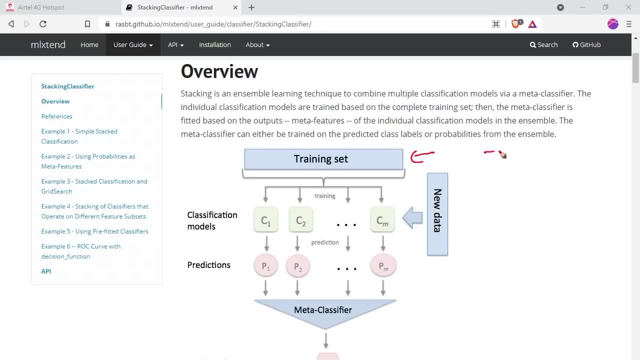 which is taking your training data. you are dividing your training data. you are dividing your training data into subsets of, into subset of training data D1,, D2, and D3.. For an example, let's take for D3, okay. 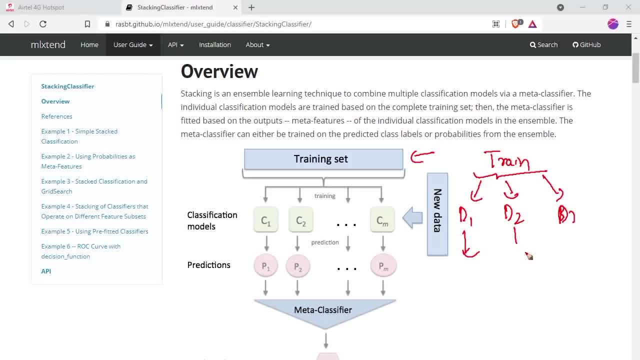 And you are training your base learners. which has a good bias and variance trade off? which has a good bias and variance trade off? okay, The base learners are very good bias and very good model. They are not either low bias or high bias. 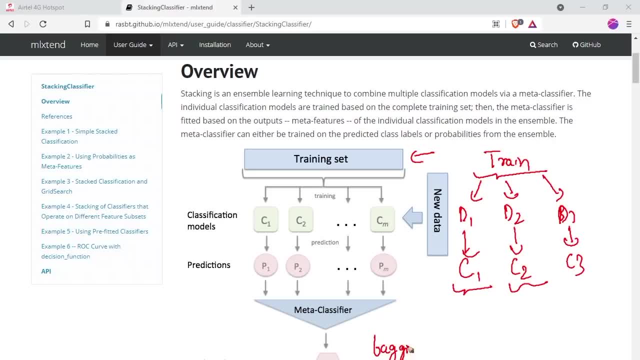 Because here in bagging again I'm saying: in bagging you have high variance, high variance and low bias model. And what do I mean by high variance? It means it performs very, very well under training data, but it fails to generalize well under the testing data. okay, 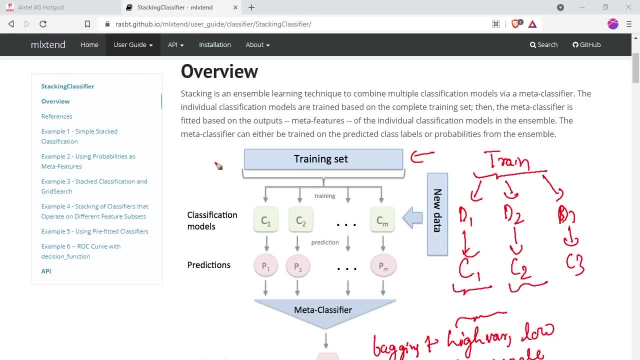 So that's why, and so that's why it's called high variance, And in boosting it is underfitting. It means that your model, your model, is either over, overfitting means underfitting because it has a low, high bias. 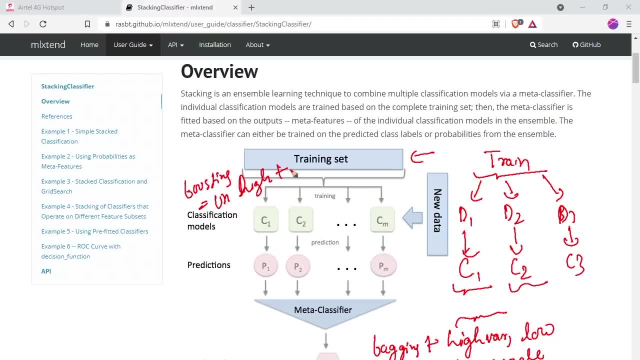 it's not performing well under training data and low variance like that. okay, So here we have an intuition about bagging and boosting. okay, So here we have a highly tuned model with extensive fine tuning. and then what you do? you take out the prediction. 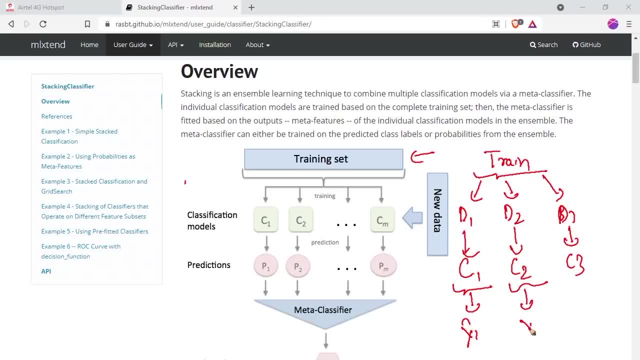 Y hat 1,, Y hat 2,, Y hat 3, Y hat 3,. okay, After you take out this, now what you do? you train your model, you train your model, you train your model, you train your meta classifier. 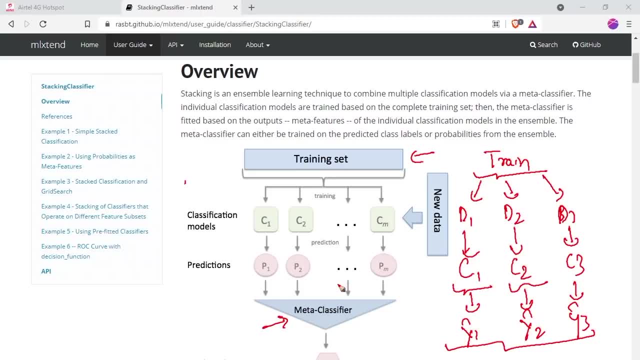 you train your meta classifier, which is just which is just trained to, on the, on the predicted class labels from the base learners or their probabilities from their ensemble. okay, So they are usually trained on these things, on these things, On the predicted class of our favorite classification. 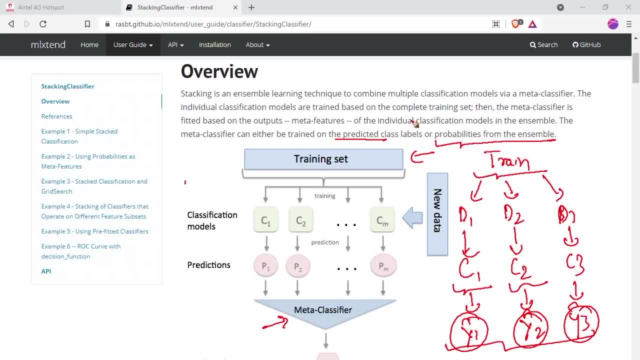 or base learners. Either they will either take the class labels or the probability of being that class. okay, So maybe 0.65, or in predicted class it may be 0, or 1, or 2, okay. 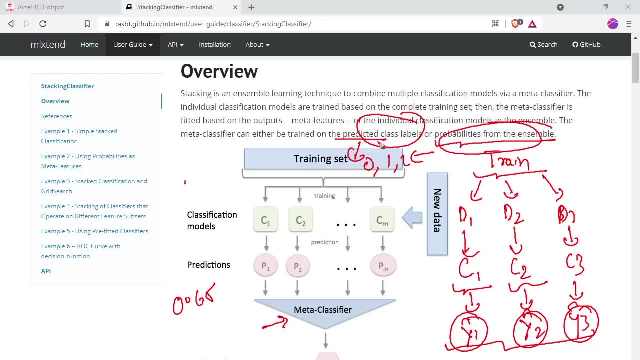 So that's what the basic intuition behind the this stacking. But again, I'm, I'm very just. I will recap to you so that it works. it makes sense again, okay, So what do you do In stacking? so let's just just for an example, 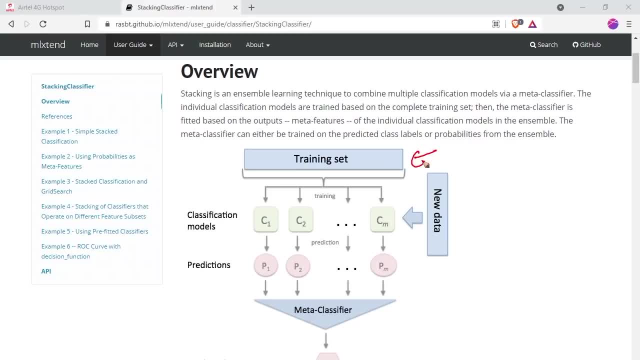 in the stacking. we are just taking a training data, okay, And then we are training, and then then we are dividing our data into a subset of a data and then we are training different, different classifier on that data. okay. 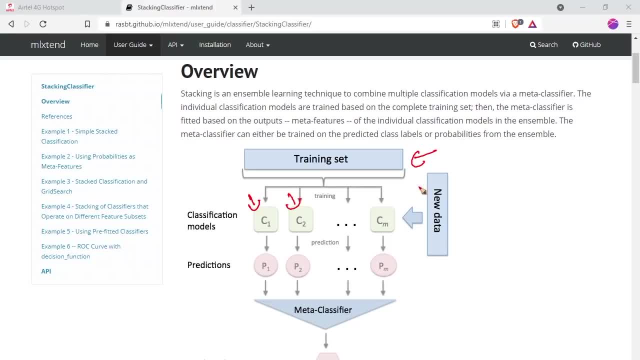 Here we have a C1,, here we have a C2, all the way down to the CM, which is new data. okay, New, new data we are training and and then what it happens and trains our C1,, C2,. 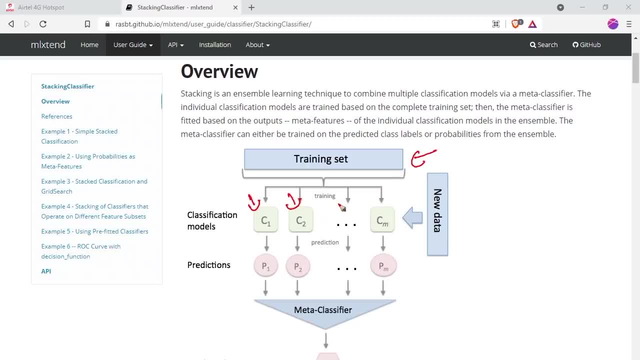 all the way down to the C3, and CM and CM onto the. that data and takes out predictions. And the major difference is: the first difference is that the the bias and variance trade-off- bias and variance trade-off, trade-off of. 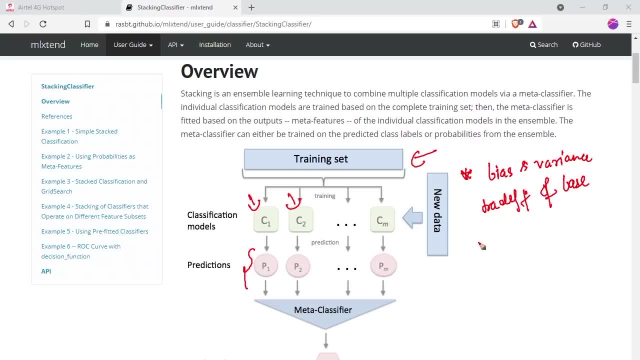 of the base learners in the stacking. base learners in the stacking is good, In the stacking is good, okay, It's good. Whereas in bagging we have high variance and low bias- okay, And in oops, what happened? 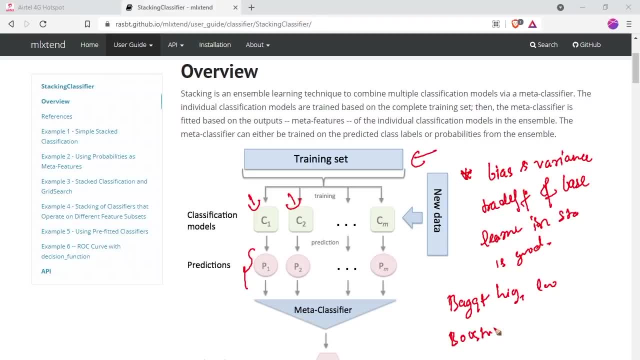 And in boosting, we have high bias and low variance. high bias and low variance. oops, what happened? High bias and low variance, low variance. okay, That's the major difference. Next thing is that, after you get the prediction from each of the model by 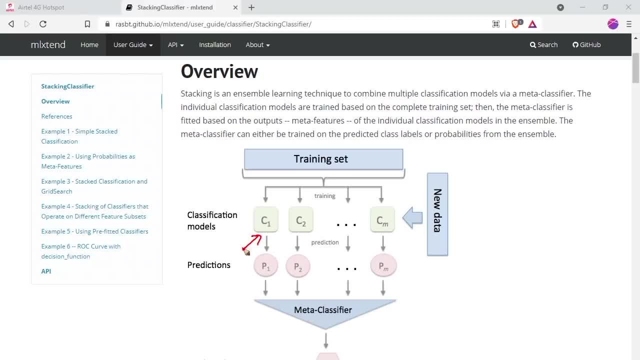 because you have done a lot more fine tuning of the hyperparameter. you get your P1, P2, all the way down to the PM. now you train a big or a meta-classifier, which you usually call as S dash. 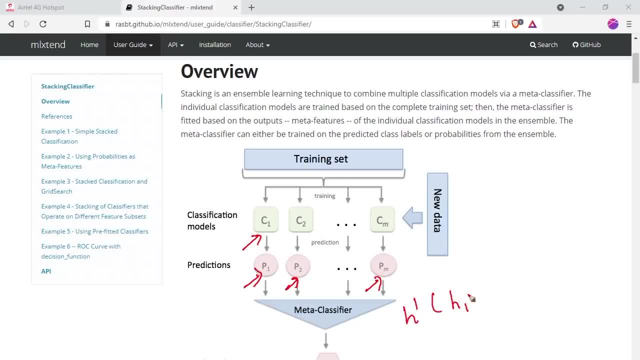 onto the prediction of H1 of X means the one classifier, second H2 of X, second classifier, all the way down to the HM of X. Either you train onto the, the probabilities, probabilities given by these models, probabilities, or the predicted class labels. 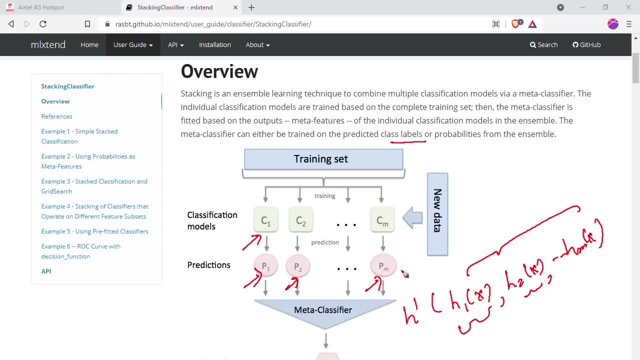 from these ensembles, okay, And in, whereas in bagging we are aggregating the majority of votes, we are aggregating, okay, the majority of votes of from that models. then you are taking that as a final prediction by hat. 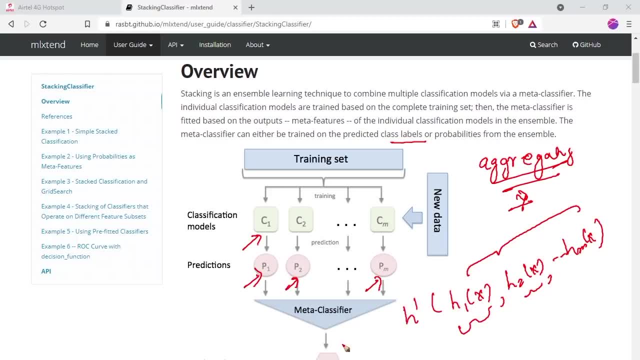 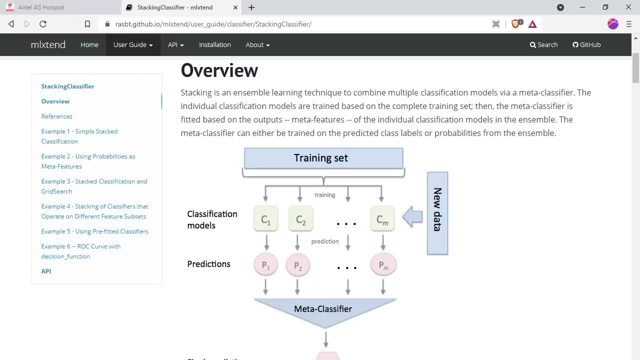 but we have a different chance of here. we have different approach, okay, So let's, let's take a quick, quick, quick look at the, at the stacking, at the stacking algorithm. but it's, I have already explained you. 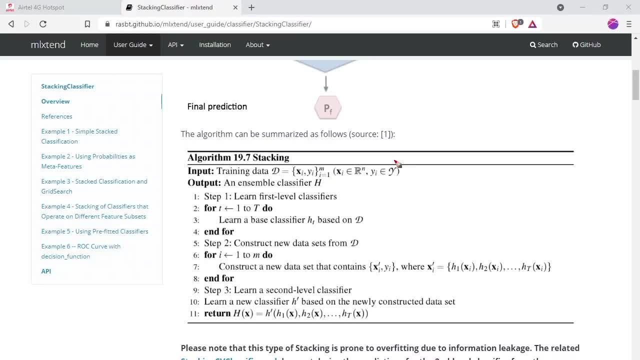 just just above, but as an just as a formal definition. Here you have your training data, which is usually XI and YI, which is, which goes from XI equals to 1, all the way down to the M, where XI is the member of R. 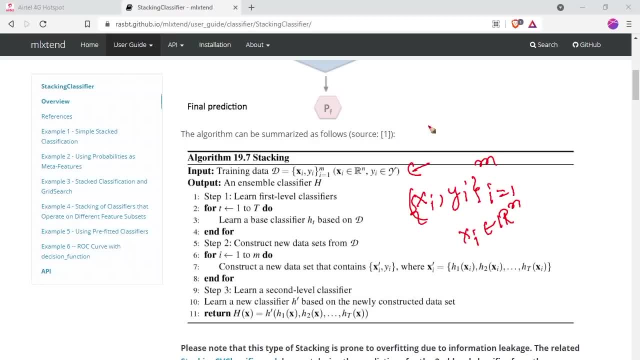 which has an N dimensional, maybe it can have a multiple field features, and, whereas the YI will be the member of the number of the classes of Y. okay, So that's the thing, and then what you do, and its output will be the ensemble classifier. 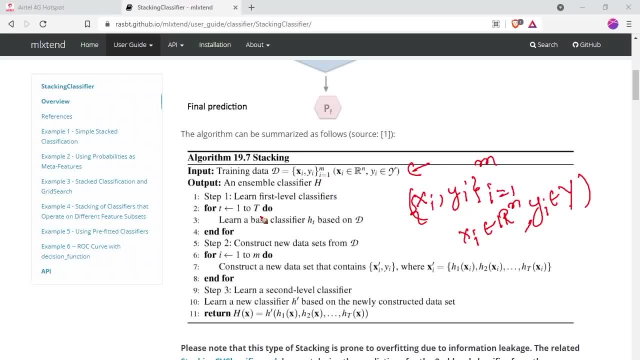 which is Y edge, dash or a big edge. okay, First what you do learn first level classifiers means you learn T T classifiers. maybe it can be logistic regression: 9 base, 9 base, it can be K: nearest neighbors. 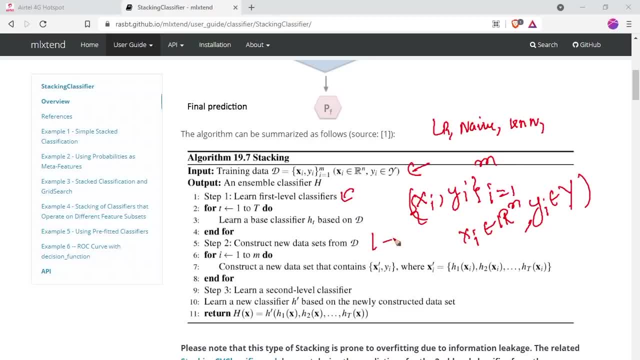 and 1, all the way down to the T and T. here is the number of base models. okay, Based on the distribution data D. Now you construct new data set. now you construct new data set. going from I equals to 1,. 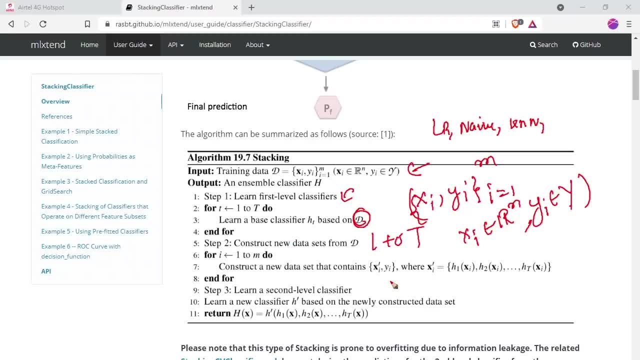 all the way down to the M, and then that contains XI, hat, prime YI, where XI is simply the prediction, the prediction from the edge, from the edge model, from the edge base learners model. okay, From the edge models. 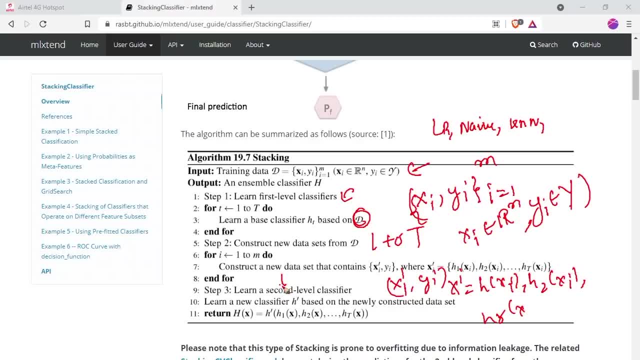 Now what you do? you train your second level classifier. first you train the first level, now you train your second level classifier and here it simply trains to get mega hypothesis of training onto these models and this meta classifier can be anything. 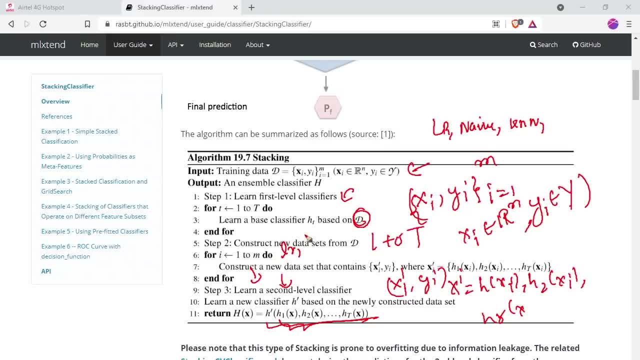 this meta classifier can be logistic regression, can be 9 base, can be, can be your neighbors, can be support with the machine and even model. and we are not aggregating, we are not taking mean, we are not taking anything. 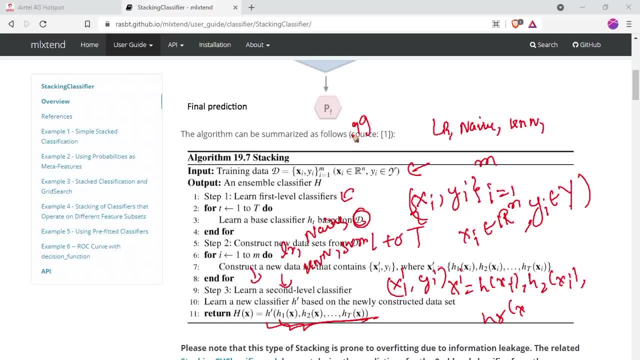 we are just training a second level classifier that is just trained on how to perform the base learners. and base learners have a good bias invariant trade off. okay, So that's the stacking, and I hope that you understood about the stacking. now I will just take a look at the 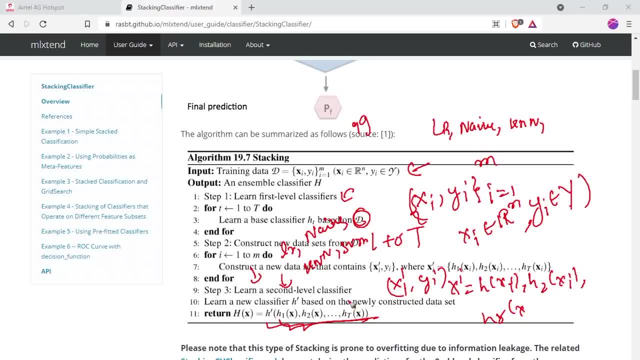 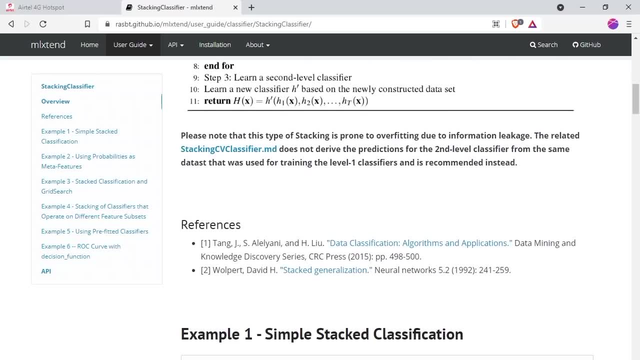 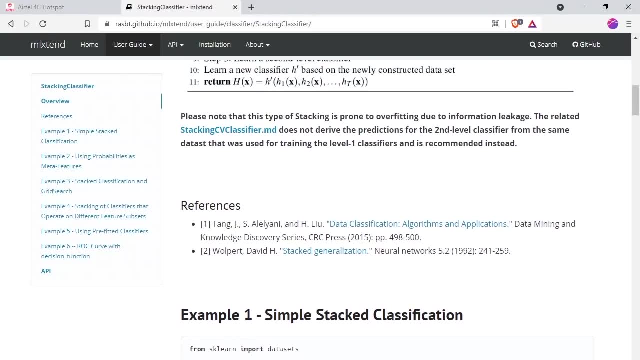 the formal, I would say the form, without doubt I could say the implementation of the stacking. the implementation of the stacking, okay, so you can see over here, you can see over here the people, which is in some of the research papers they usually call as a stacked generalization. you can some, some, some and some research. 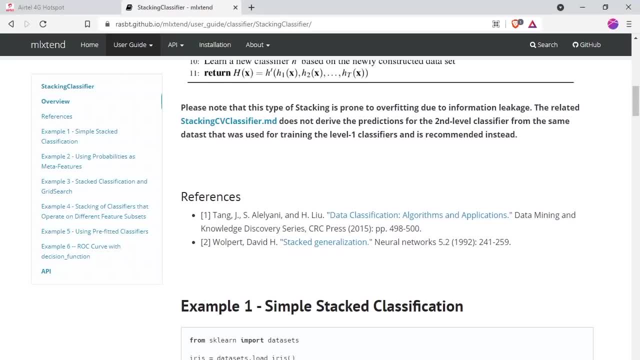 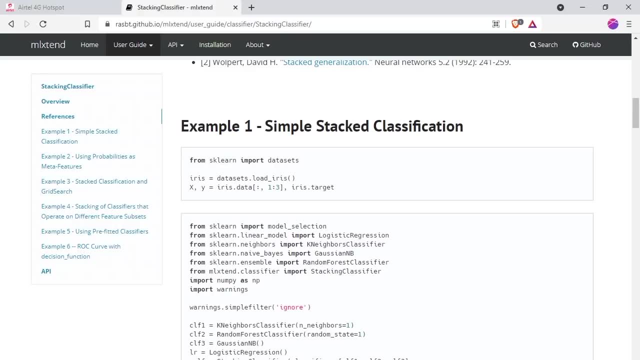 paper. we call that okay, okay. so let's make a simple stack classification first. what you have done over here: we have simply loaded the data set from the escalator data set, which is an iris data set, and iris data set is not too much hard. we have sepal, we have a sepal length, we have a sepal length petal. 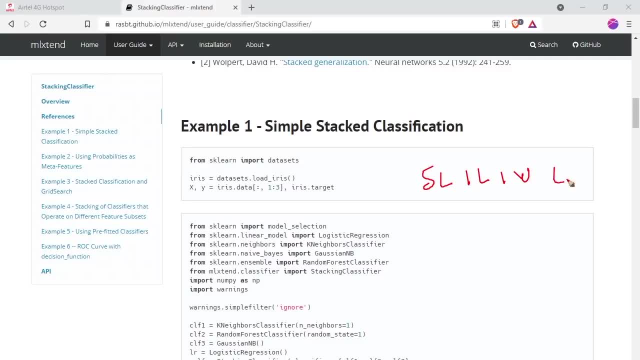 length, petal width and petal length. okay, so we have four features and basis on that, we have to predict what is this species of that flower which is either- can be set also versicolor or virginica. okay, so that's the, the that's the, that's our data set. now you can see. first we import the model. 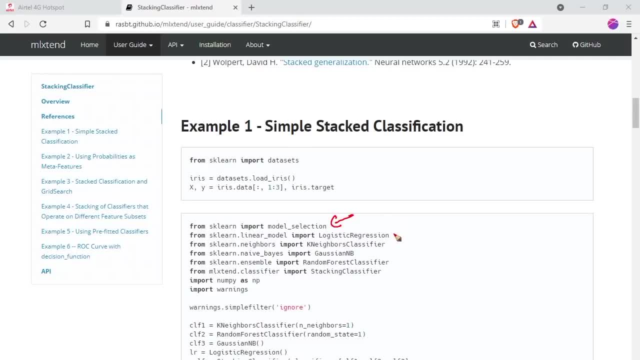 selection, which you'll see what it does. then we import the logistic regression from linear model, API and cycle learn. then we import KNE, KNN, which is a which is again from neighbor from neighbors, API and cycle learn and then you implode input Gaussian night base from night base either- not gone into too much. 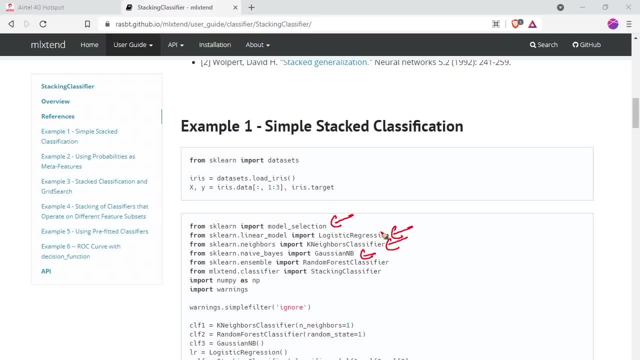 of algorithm, because learning algorithm can just. you can see the Wikipedia. you are now capable of learning any algorithm. okay, now you just import the random forest classifier from ensemble learning, ensemble API of cycle learn. now you import from MLA- extend library is flat classifier and put a second classifier. 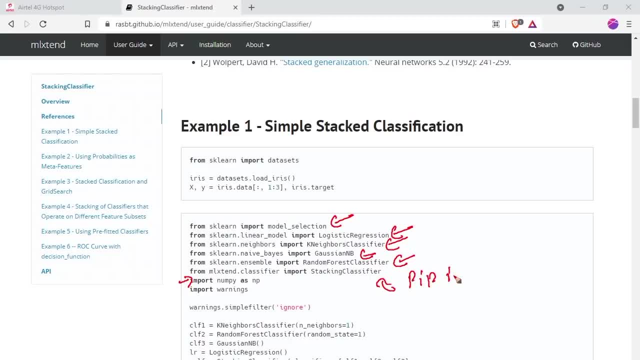 either you have to- first you have to install this using pip install if you have a biker and I like stand- but then again do this kind of thing. okay, where is my? let me delete this. okay, after that. after that, What we have to do? we have to simply import the numpy as np. 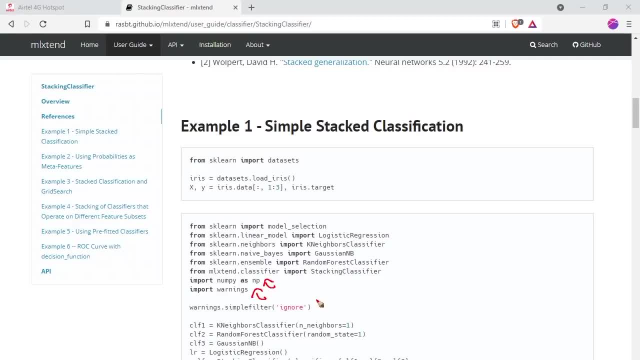 as alias and import warnings. Now you're going to ignore the warnings given by the models. Now, first, your first model is clf1, which is k neighbors with the neighbors of 1.. If it is bagging, if it was bagging, 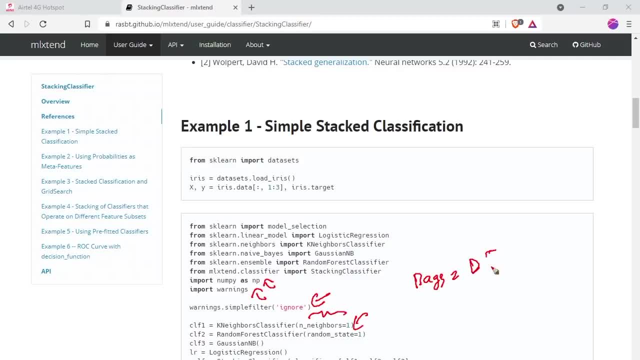 then we have to random forest. We have taken one decision tree, but we are taking different models, and that's what makes it perfect. Random classifier: Gaussian 9 base logistic regression. OK, Now what we have done? we instantiated our object. 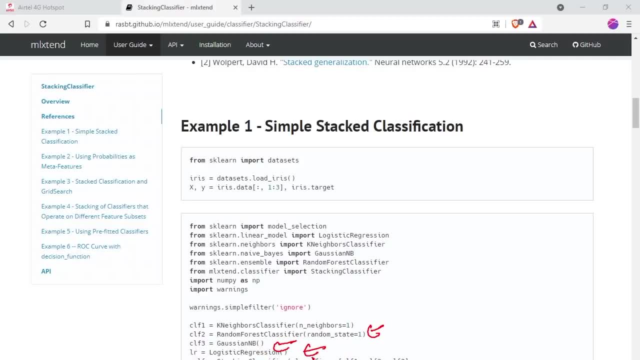 everything. Now we instantiate our stacking classifier, which is the number of the classifier, will be clf1, which is clf of k neighbors random forest, which is the clf2, and these three- These three are clf2, clf3- are the base learners. 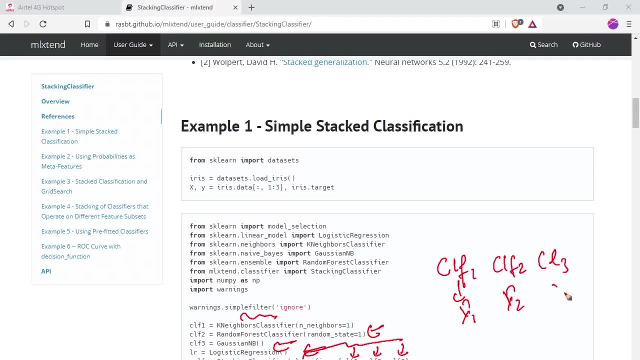 It will give output. It will give output like this. Now, what you will do? you want a meta classifier which will be the logistic regression, which will the logistic regression which will be Until you can take logistic regression as a meta classifier. 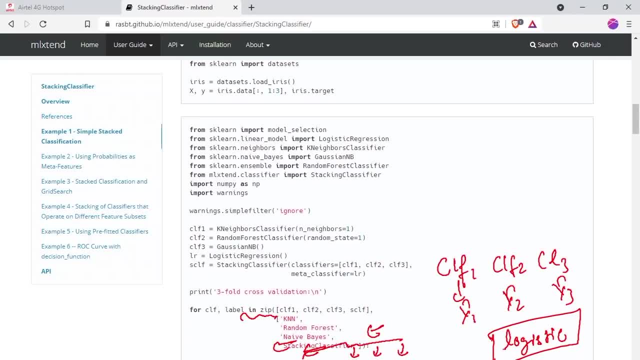 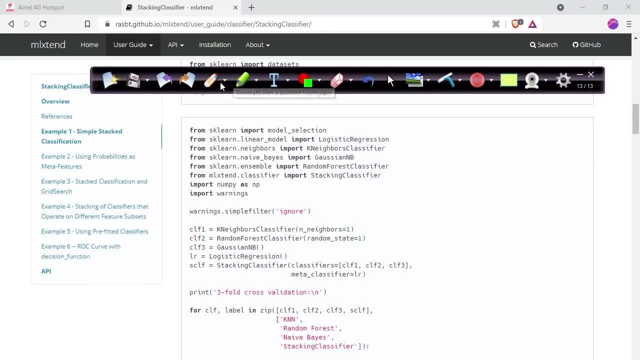 now you perform a 3-fold cross validation. and now you perform 3-fold cross validation. Now you perform 3-fold cross validation Now in 3-fold cross validation. you're are just looping through CLF as well as the label, it seems zipping the CLF 1, CLF 2, CLF 3 and SCLF. 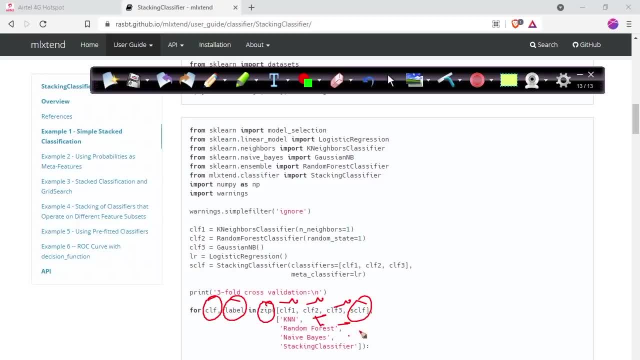 okay, now KNN, a random forest night base and stacking classifier. now you select the best model. you know you select the base model by training each other model. whether you are taking a scoring equals to accuracy. now you check the accuracy and you can see, and you can see, and. 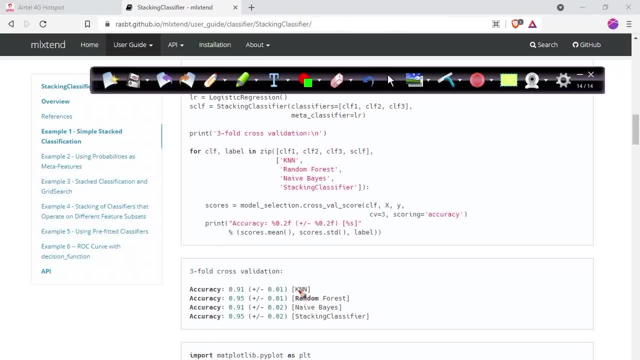 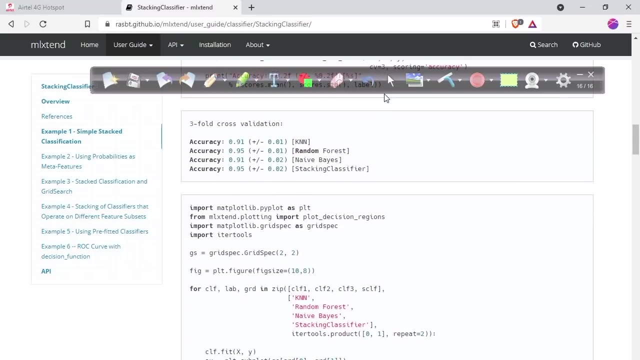 you can see that this stacking classifier has around point is 0.4 percent of increase. as is better? I mean, this is quite better than this. a random for the staggy festival works best in this case. okay, and now, what you can do, you can, what you can do, you can actually plot the KNN. 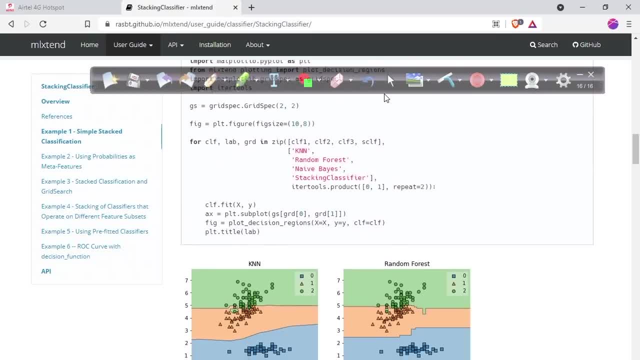 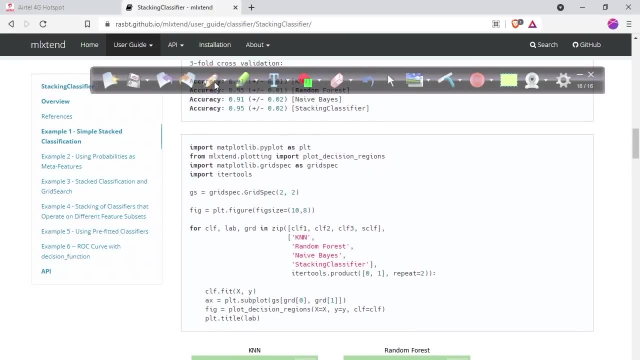 how it is plotting means the decision boundaries of the models, how they are plotted at decision boundaries or hyperplanes. okay, in the math plot, let so let me and annotate what is doing. first you import the math plot lib. then you have to import the plot decision regions from ML extend. 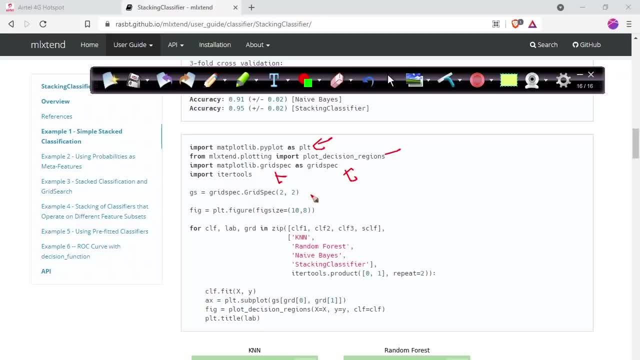 then flow. the grid is pick, then you include the iter tools, then you set the set the area, then you set the area again. you loop through by dipping, and then you take out the product and then you fit it and then you plot it and then you plot. 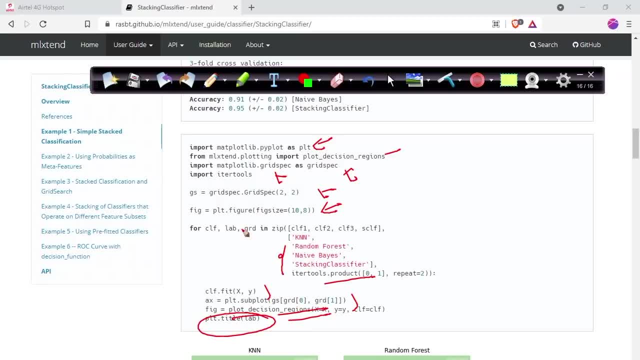 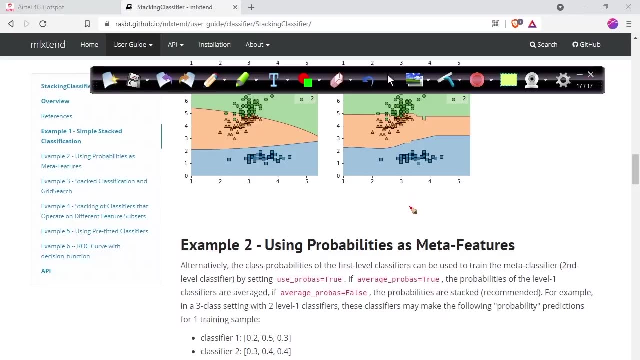 the decision boundary, then your title, the lab, and lab here is just KNN and random forest night base and stacking classifier. okay, after you plot it now you are done with a second classifier. okay, now I, as I've already stated you either for training, the meta classifier, you can use either this that I could say: 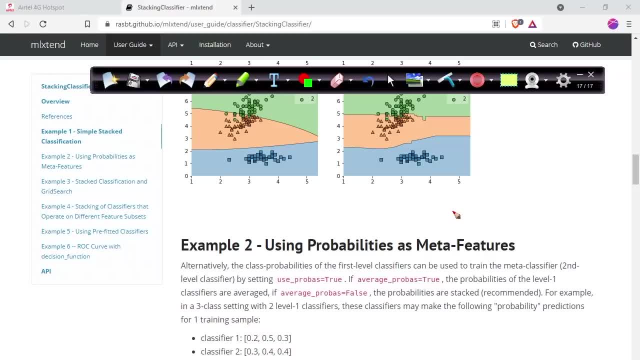 I could say that maybe let's see the prediction from the base learners so you can either take prediction class. you can either take prediction class. you can either take prediction class or the probabilities as the meta features, or the probabilities as the meta features, or the probabilities as the meta features. okay, so you can say that use proba use. 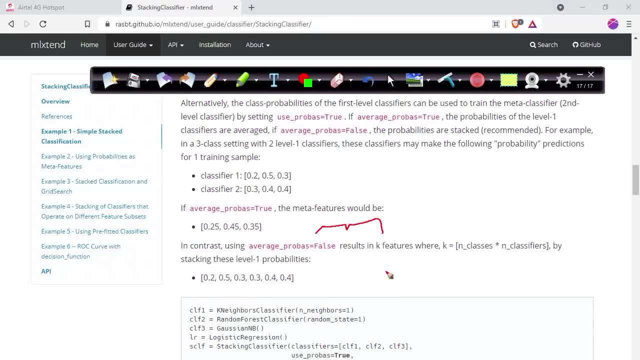 okay, so you can say that use proba use. okay, so you can say that use proba use. proba equals to true use. proba equals to proba equals to true use. proba equals to proba equals to true use. proba equals to true and average provide equals to false. 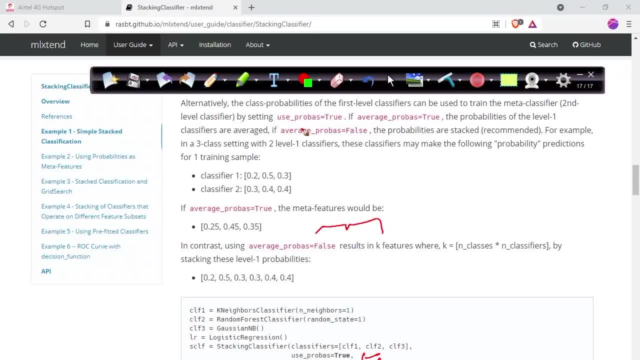 true and average provide equals to false. true and average provide equals to false. okay, and you can see here are a little okay and you can see here are a little okay and you can see here are a little bit of the documentation over there, okay, bit of the documentation over there, okay. 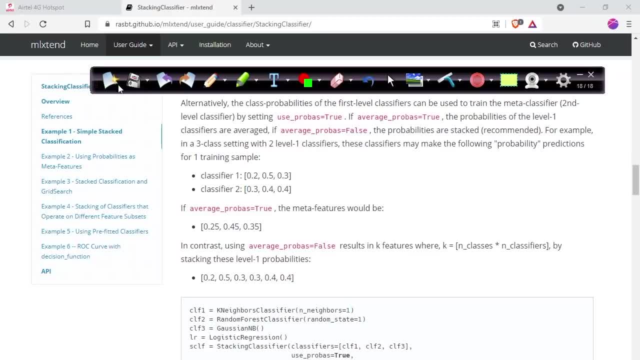 bit of the documentation over there. okay, great, now, we have seen this and again. great now we have seen this and again. great now we have seen this and again. the same thing is not too much harder. we, the same thing is not too much harder. we, the same thing is not too much harder. we are using the thing and now we will see. 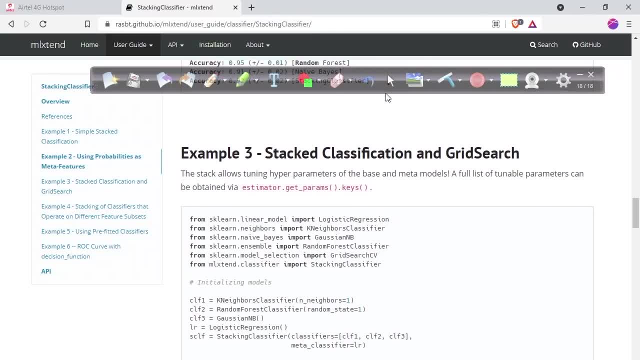 are using the thing and now we will see are using the thing, and now we will see. here is an example of static. here is an example of static. here is an example of static classification using grid search. it's your classification using grid search. it's your classification using grid search. it's your task is to do this, but I'm just going. 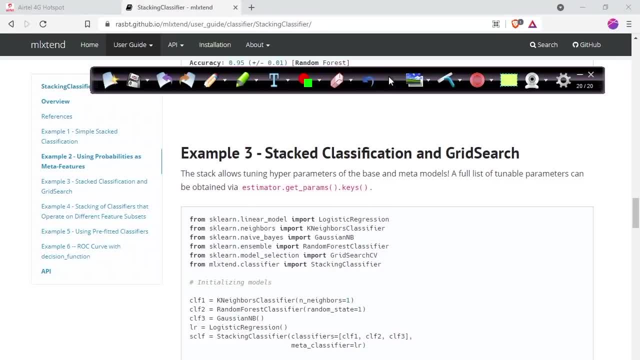 task is to do this, but I'm just going. task is to do this, but I'm just going to annotate what the this kind of thing to annotate what the this kind of thing to annotate what the this kind of thing will do. grid search. so here you are, just. 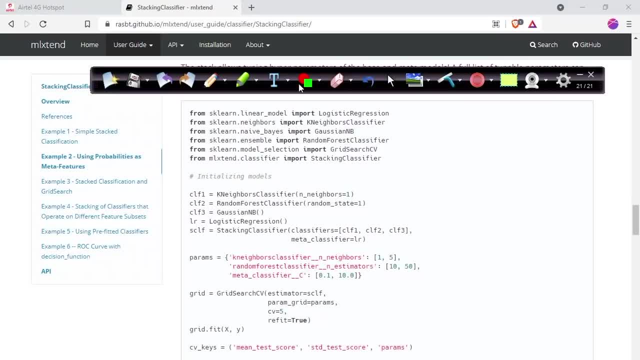 will do grid search. so here you are, just will do grid search. so here you are, just first of all. you are just you, now, you, first of all. you are just you, now, you, first of all, you are just you, now you will do. you will have a good bias. 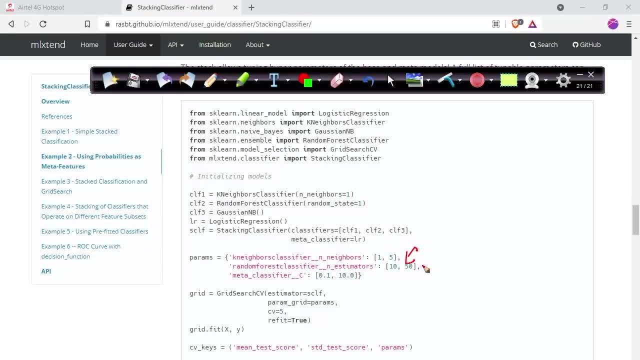 will do, you will have a good bias. will do, you will have a good bias- invariant straight off. so you are going invariant straight off. so you are going invariant straight off. so you are going to check between 1 to 5 and we're going to check between 1 to 5 and we're going. 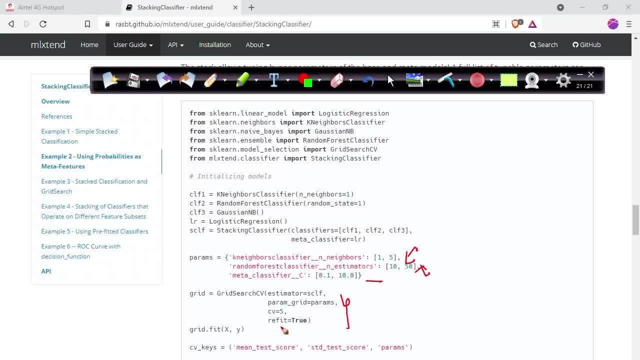 to check between 1 to 5 and we're going to check, and then that I classifier and to check, and then that I classifier and to check, and then that I classifier and it's fed a grid search, you find the. it's fed a grid search. you find the. 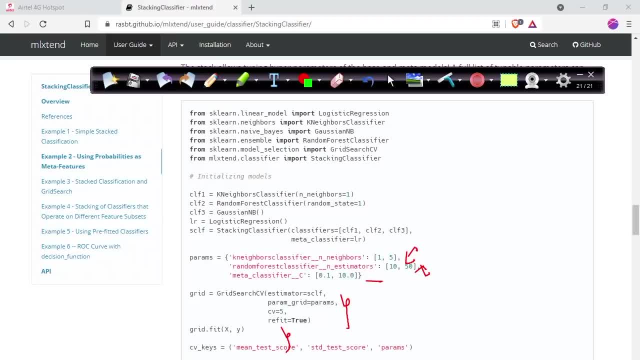 it's fed a grid search. you find the grids- best grid search. then you plot grids- best grid search. then you plot grids- best grid search. then you plot their results. means that you take out their results. means that you take out their results. means that you take out the results. what are the best parameters? 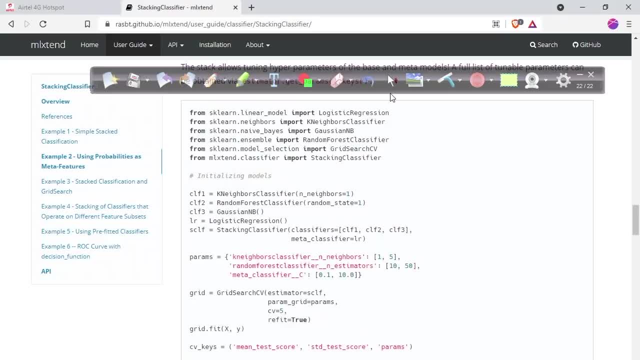 the results, what are the best parameters? the results, what are the best parameters? and accuracy. so, after applying that, you and accuracy. so, after applying that, you and accuracy. so, after applying that, you will get a set of values which are the will get a set of values which are the. 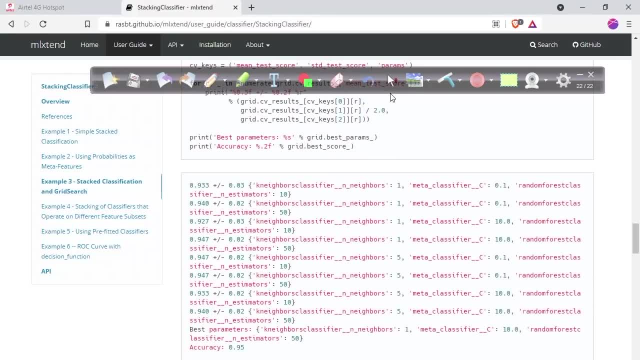 will get a set of values which are: the best of k nearest has these best. best of k nearest has these best. best of k nearest has these best features and like that. okay, now you can features and like that. okay, now you can features and like that. okay, now you can import the same thing for doing the. 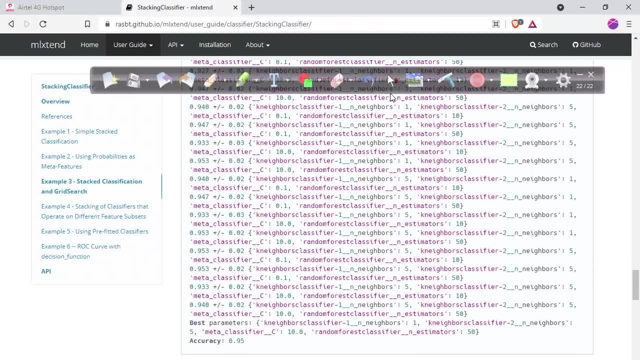 import. the same thing for doing the import, the same thing for doing the k-nearest neighbors and random forest k-nearest neighbors and random forest k-nearest neighbors and random forest classifier. and then we have one, one, one classifier. and then we have one, one one. 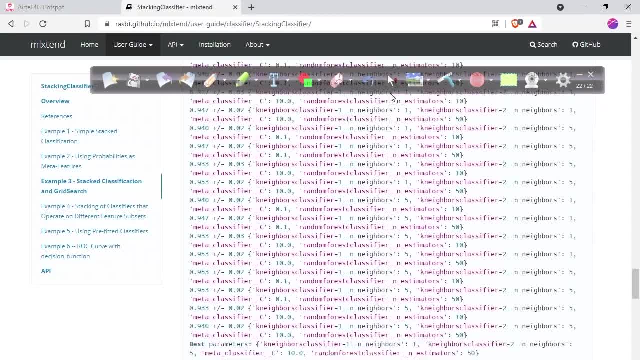 classifier. and then we have one one, one more, which is the meta classifier. okay, more, which is the meta classifier. okay, more, which is the meta classifier. okay, now, using the grid search stacking on. now using the grid search stacking on. now using the grid search stacking on that operate on different subset of. 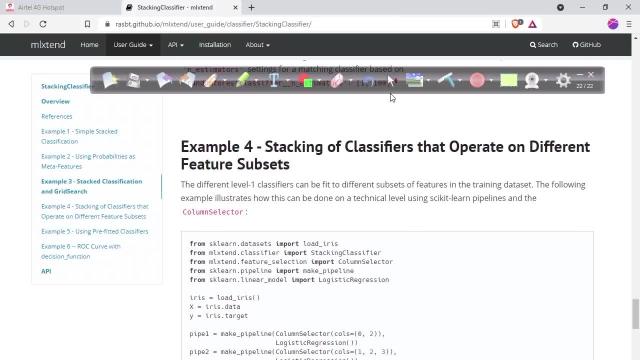 that operate on different subset of that operate on different subset of features. you can also do that by features. you can also do that by features. you can also do that by selecting the column separator, by selecting the column separator, by selecting the column separator by quality, the make pipeline that selects. 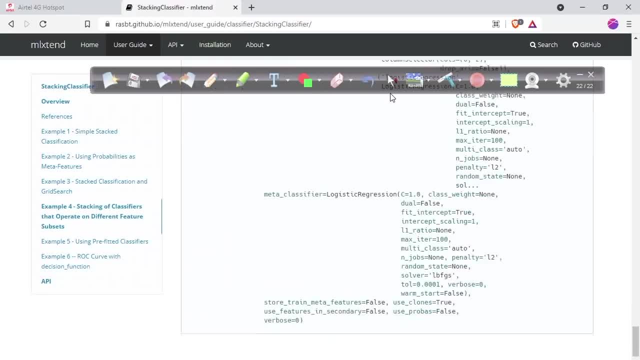 quality. the make pipeline that selects quality, the make pipeline that selects the two features. okay, so that's the that, the two features. okay. so that's the that, the two features. okay. so that's the that you can do and you can use pretty. you can do and you can use pretty. 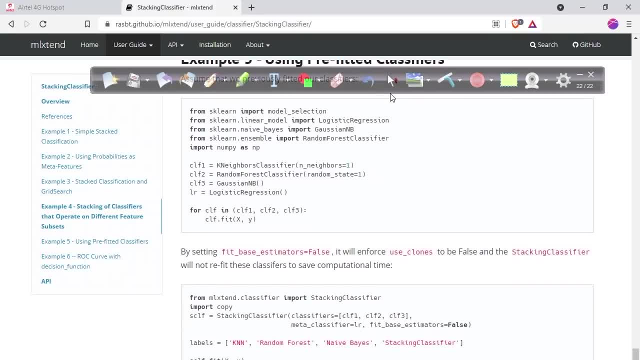 you can do and you can use pretty fitted classifiers which is already being fitted, classifiers which is already being fitted, classifiers which is already being fitted- we previously fitted our fitted. we previously fitted our fitted. we previously fitted our classifiers in your models- okay, fit base. classifiers in your models- okay, fit base. 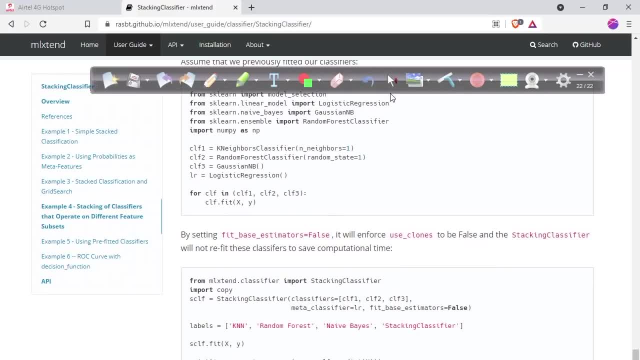 classifiers in your models. okay, fit. base estimator equals to false means you estimator equals to false means you estimator equals to false means you don't want to fit your base estimators. don't want to fit your base estimators. don't want to fit your base estimators? okay, then also plot ROC curve using and. 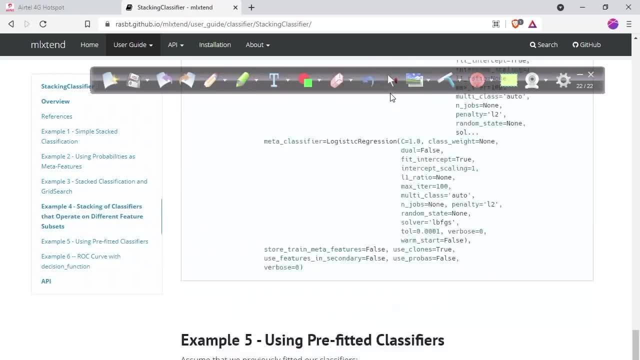 okay, then also plot ROC curve using: and okay, then also plot ROC curve using: and you can see the ROC curve like this, and you can see the ROC curve like this, and you can see the ROC curve like this, and, and this is the first of all these four: 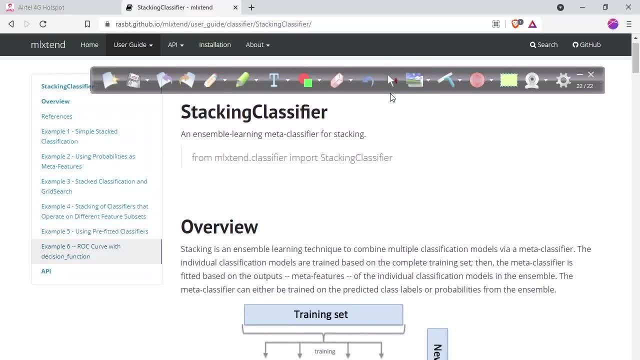 and this is the first of all. these four- and this is the first of all these four examples are very, very important. if you examples are very, very important, if you examples are very, very important. if you do you can see the ROC curve and in more do you can see the ROC curve and in more. 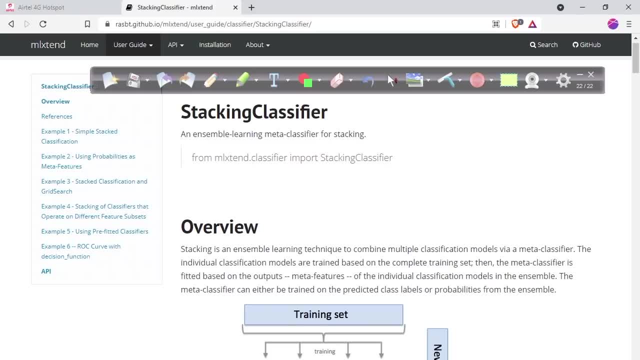 do. you can see the ROC curve and in more detail on the internet. okay, great, so now detail on the internet. okay, great, so now detail on the internet. okay, great, so now. we have talked a lot about stacking. we have talked a lot about stacking. we have talked a lot about stacking classifier. I showed you the. 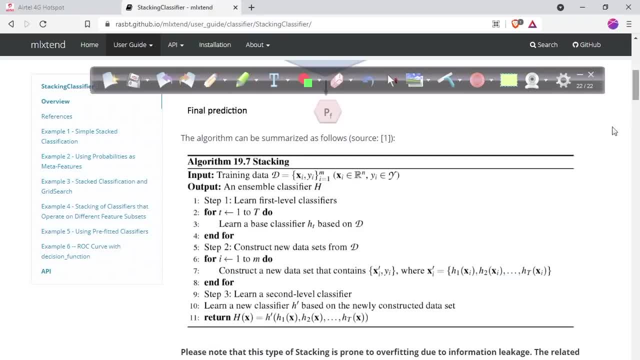 classifier. I showed you the classifier. I showed you the implementation of stacking classifier. implementation of stacking classifier, implementation of stacking classifier. here's it a very interesting and a here's it a very interesting and a here's it a very interesting and a brilliant diagram on a stacking or. 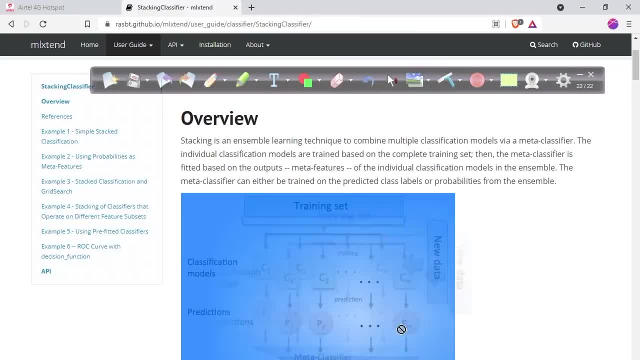 brilliant diagram on a stacking or brilliant diagram on a stacking or algorithm given on stacking. this is a algorithm given on stacking. this is a algorithm given on stacking. this is a good example on stacking that I want to. good example on stacking. that I want to good example on stacking that I want to give it to you. okay, thanks to the author. 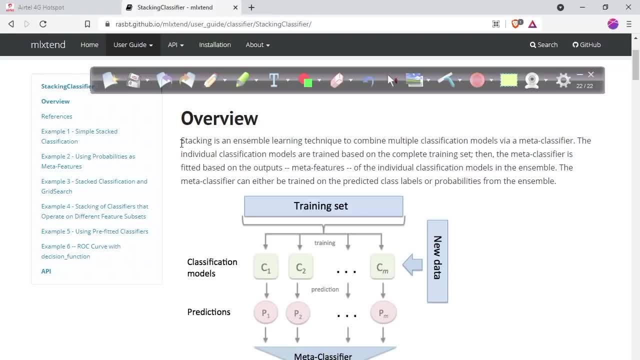 give it to you. okay, thanks to the author. give it to you, okay, thanks to the author. let's give it to you. full credit goes to. let's give it to you. full credit goes to. let's give it to you. full credit goes to them. okay, there's some, I just don't. 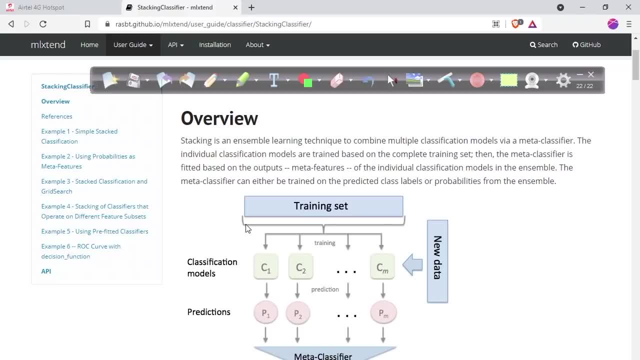 them. okay, there's some, I just don't them. okay, there's some I just don't. man annotating okay. so now we are done, man annotating okay. so now we are done, man annotating okay. so now we are done with these, with ensemble learning, so. 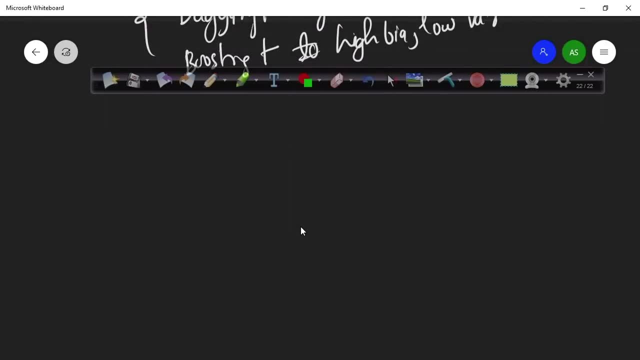 with these, with ensemble learning, so with these, with ensemble learning. so let's, let's recap to late what, what we let's, let's recap to late what, what we have seen so far, we have seen, we have have seen so far, we have seen, we have have seen so far, we have seen. we have said: we have completed, we have completed. 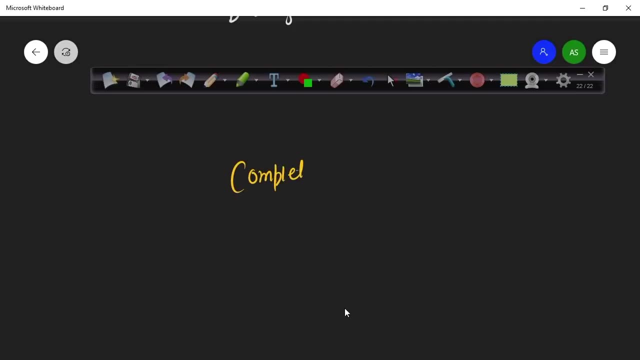 said we have completed, we have completed. said we have completed, we have completed. let me write a good accomplishment. let me write a good accomplishment, let me write a good accomplishment. completed ensemble learning: so what we completed. ensemble learning, so what we completed. ensemble learning: so what we have seen. we have seen bagging, so in 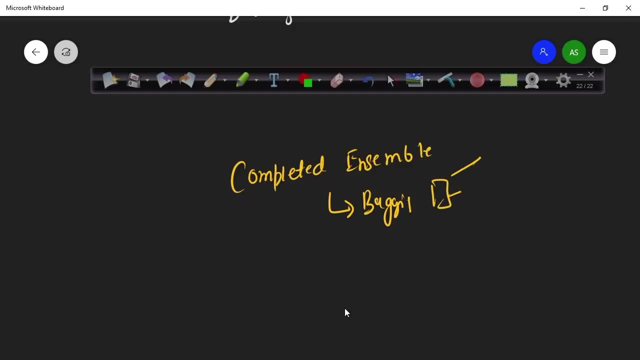 have seen, we have seen bagging. so in have seen, we have seen bagging. so in bagging, the basic intuition is: we have a bagging. the basic intuition is: we have a bagging. the basic intuition is: we have a data. we take out different, different. 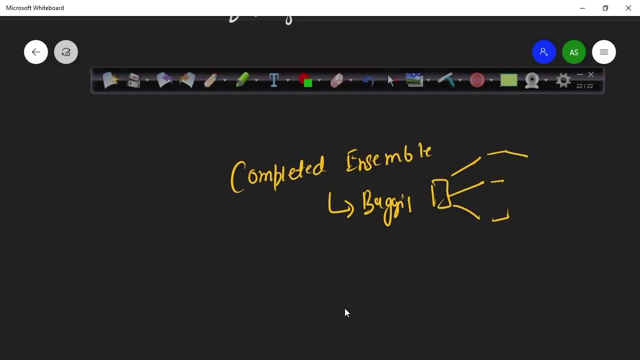 data. we take out different, different data. we take out different, different data. we train a different, different model data. we train a different, different model data. we train a different, different model. and then we aggregate the majority of, and then we aggregate the majority of, and then we aggregate the majority of votes from each of the model, then you. 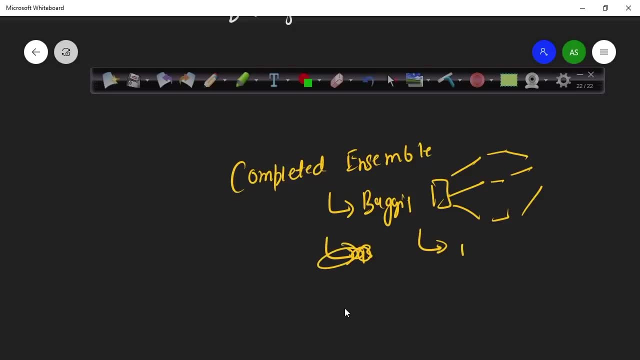 votes from each of the model, then you votes from each of the model, then you have then, in bagging, we have learned, have. then, in bagging, we have learned, have. then, in bagging, we have learned about one of the algorithm which is a, about one of the algorithm which is a. 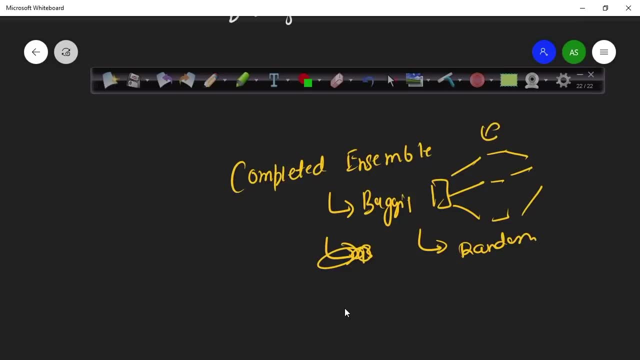 about one of the algorithm, which is a random forest that just use the base random forest. that just use the base random forest. that just use the base learners with rule sampling, with feature learners, with rule sampling, with feature learners, with rule sampling, with feature sampling. okay, feature bagging. and then we 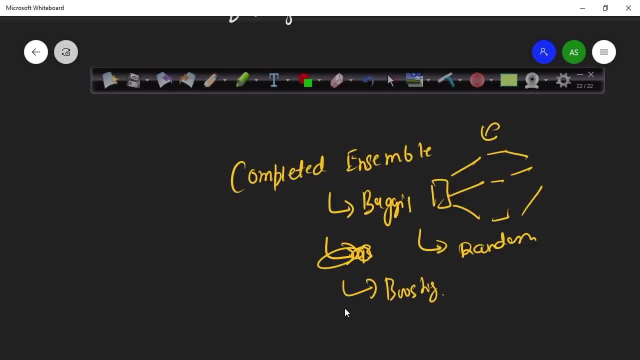 sampling- okay, feature bagging. and then we sampling- okay, feature bagging. and then we take out the boosting. then you learned: take out the boosting, then you learned, take out the boosting, then you learned about the boosting. we're in boosting you about the boosting, we're in boosting you. 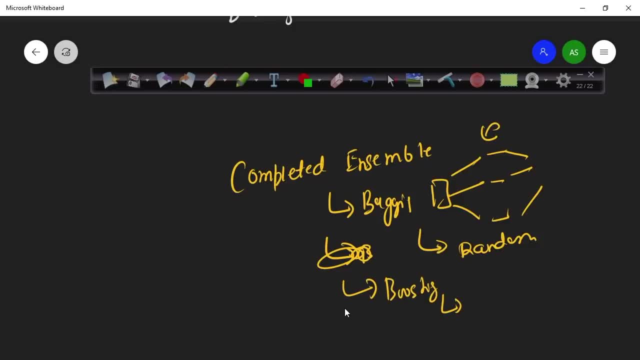 about the boosting we're in boosting. you learned about the technique okay and then learned about the technique okay and then learned about the technique okay, and then we kind of converting the weak, we kind of converting the weak, we kind of converting the weak learners to the strong learners. then let me talk. 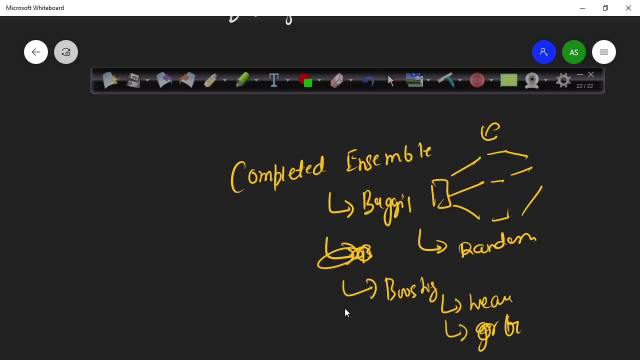 learners to the strong learners, then let me talk learners to the strong learners. then let me talk about the great deep radiant, about the great deep radiant, about the great deep radiant. boosting decision trees: then we have boosting decision trees. then we have boosting decision trees. then we have talked about adaptive boosting, which is: 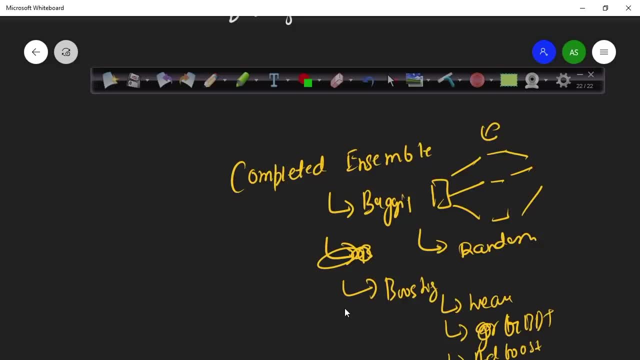 talked about adaptive boosting, which is talked about adaptive boosting, which is adapt boost, which is just with adapt boost, which is just with adapt boost, which is just with exponential it's a loss, and then we exponential it's a loss, and then we exponential it's a loss. and then we talked about xg boost. okay, now we are now. 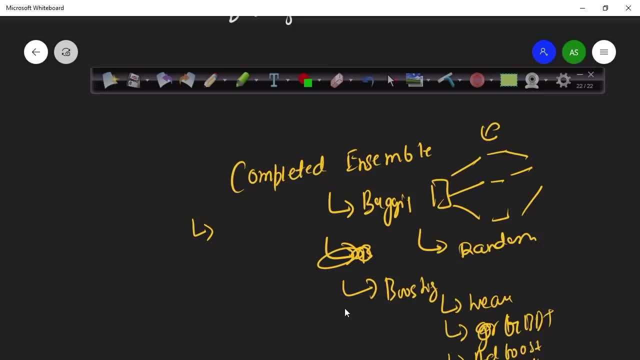 talked about xg boost. okay, now we are now talked about xg boost. okay, now we are now. we in this section in this subsection, we in this section in this subsection, we in this section in this subsection, we have talked about its stacking, we have. we have talked about its stacking, we have. 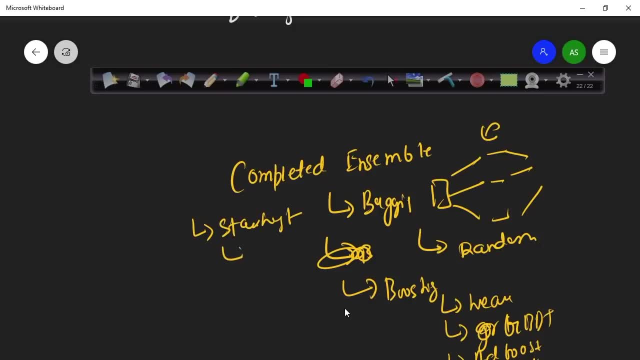 we have talked about its stacking. we have talked about the stacking there. we talked about the stacking there. we talked about the stacking there. we have seen a lot of examples. a lot of have seen a lot of examples. a lot of have seen a lot of examples. a lot of examples is a grid search and such. 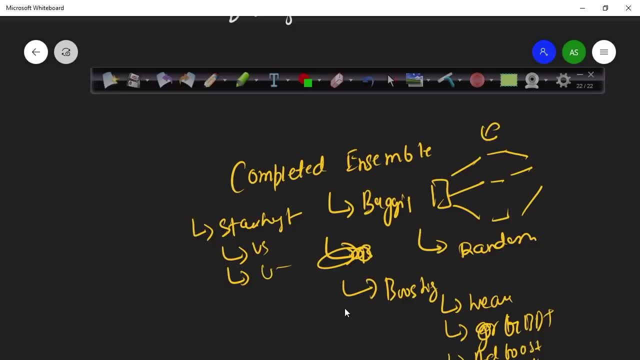 examples is a grid search and such examples is a grid search and such values, and that that that okay. so now I values. and that that that okay. so now I values. and that, that, that okay. so now I hope that you understood everything. hope that you understood everything. 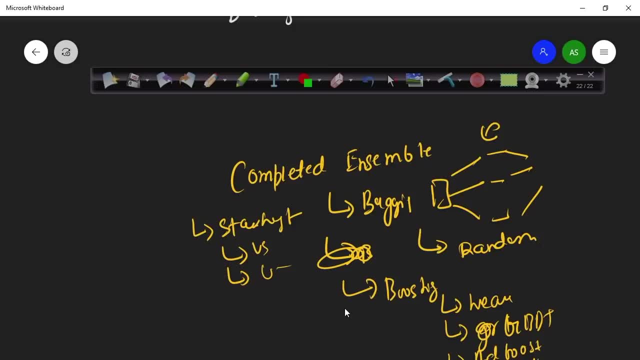 about machine learning, sorry, ensemble learning. okay. so if you're watching till now, I am saying that you know that you do everything about supervised learning, that you need to crack any kind of interview, okay. so just pack your bag and be sure to subscribe my YouTube channel. 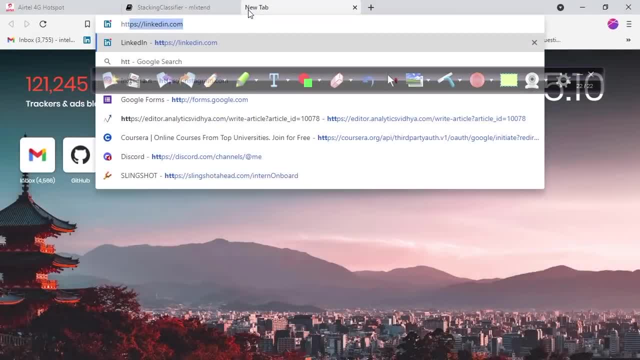 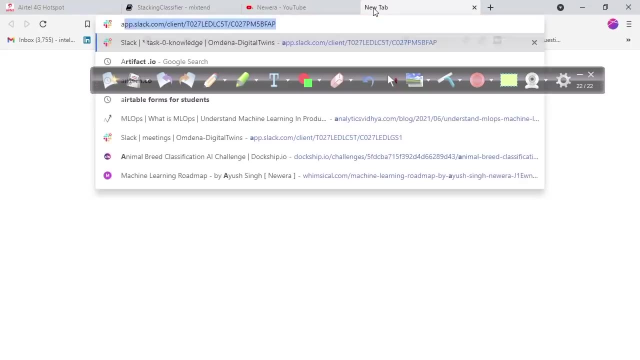 it just gives you a great motivation as the new deep learning course is coming soon. so you can pre-register there for free. you can pre-register there or, if you want. or, if you want, you can go to anternco for detailed CSO. there is CSO 1 course, which is 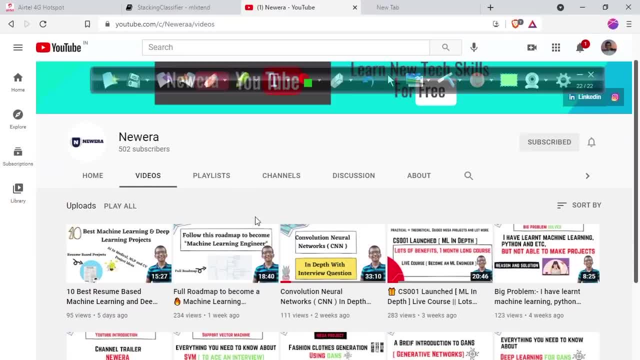 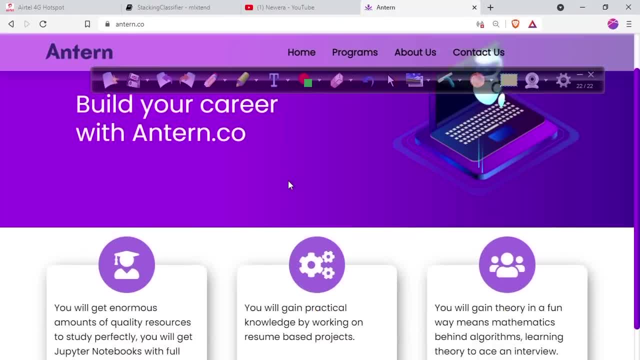 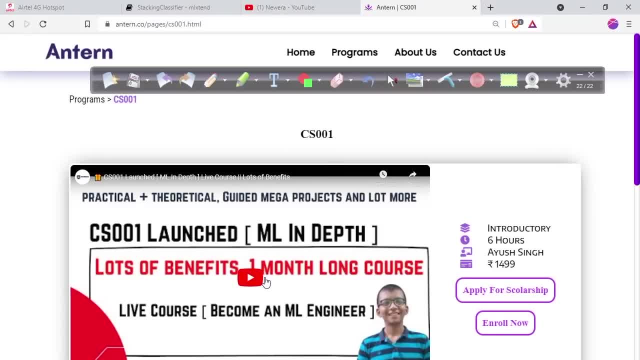 see the benefits, what are the course details and et cetera, and the launch video which is already being launched. okay, so I think that it's. you can also apply for a scholarship if you're a college student, but it's totally fine for giving, but the course prize is like this: 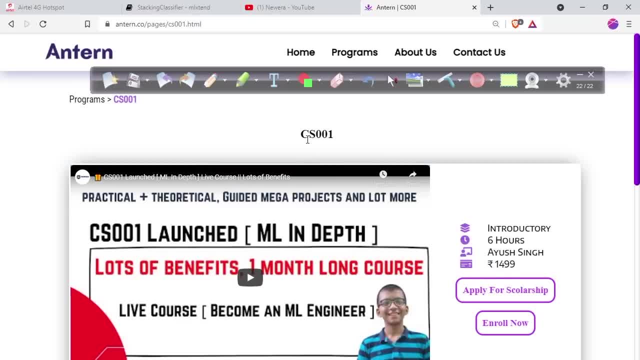 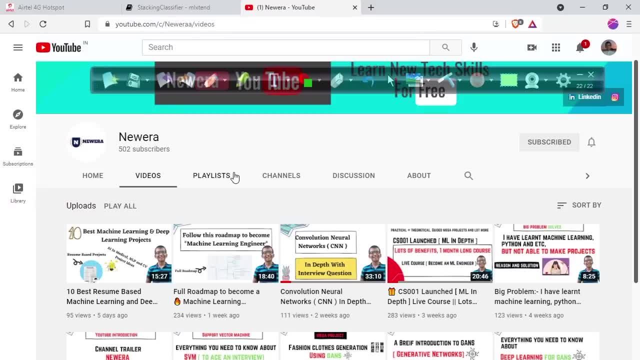 okay, but it's totally based upon you. if you want, you can definitely consider it just supports to make free content more okay. so that's just just to me ask a question: is this course the same as CSO 1,? yeah, it's yeah, but in that 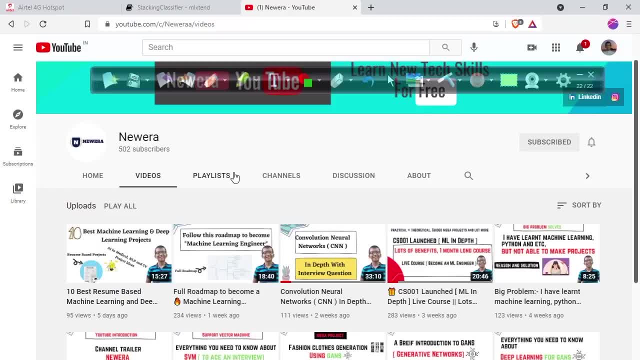 we have talked about about neural networks, then you have talked about GANs, convolutional neural networks. you have you will get a one-to-one session. you will get Jupyter notebooks, which are amazing Jupyter notebooks. you will get early access to my books. you will work with the team. 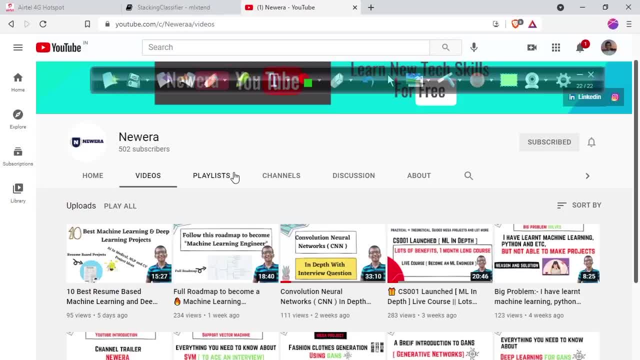 you will be getting an internship, you will work on a real-world project in Anturn, et cetera. okay, so you can consider Anturnco for this. okay, if you want the lab, but if you complete this this course, you'll all be very, very comfortable in machine learning. okay, so that's it for this. 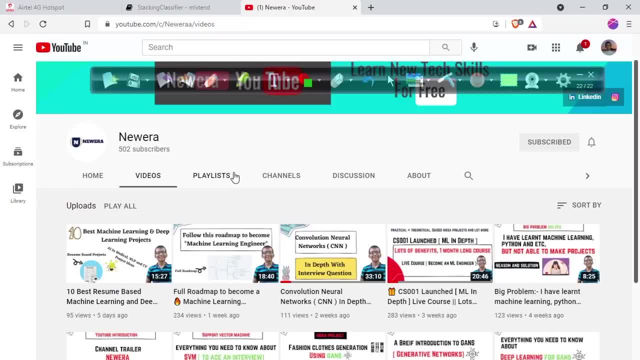 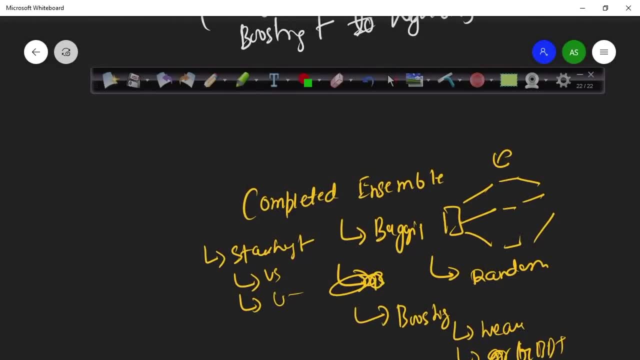 section for this whole section on ensemble learning. from the next section you can consider subscribing. obviously from the next section we'll be starting with, and in between we can do some projects. so from the next section we'll be starting with unsupervised learning and I 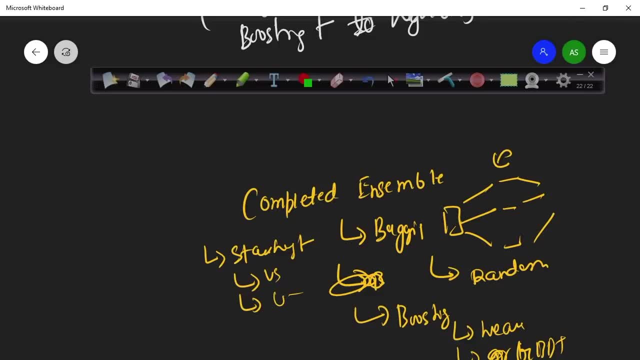 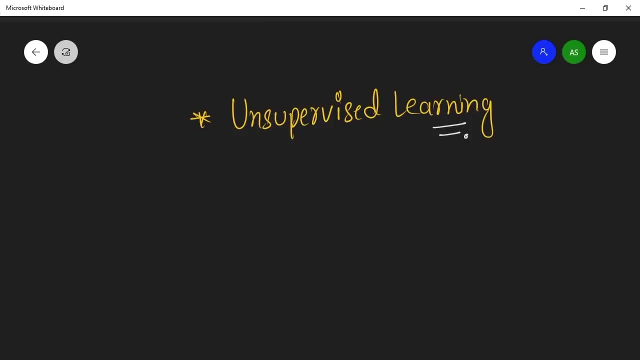 really hope that you will enjoy that series also. okay, so let's meet the next section. okay, so now we have covered supervised learning and you're going to now consider a comfortable and supervised learning yourself. supervised learning is one of the very 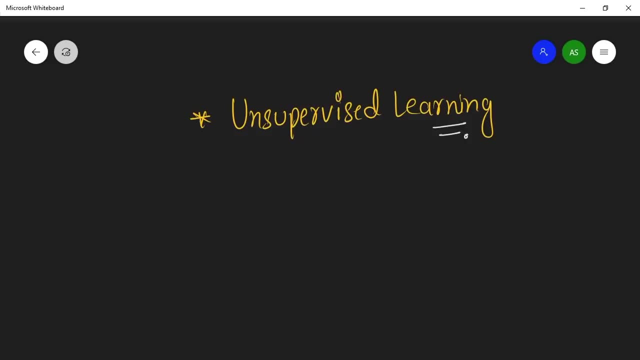 vast, vast topic in machine learning that we have covered very smoothly and I hope that you understood every, each and every thing about supervised learning. if you have any kind of doubt, you can either ask a newer or just start community, or you can ask over to the 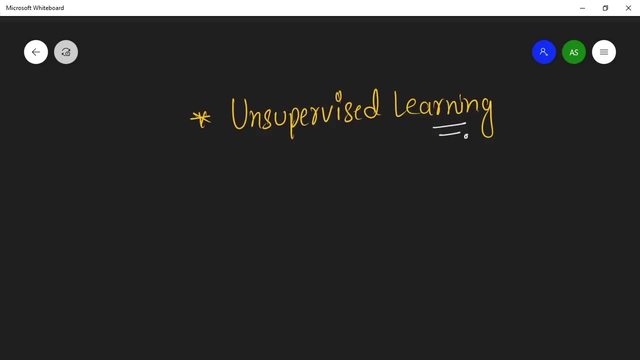 you can find the discord community or you can come comment and then we can answer your questions. okay, so that? so let's, let's start with unsupervised learning. so what, actually, in supervised learning, we are doing? we have our data set, which is xi as well as yi, and we have 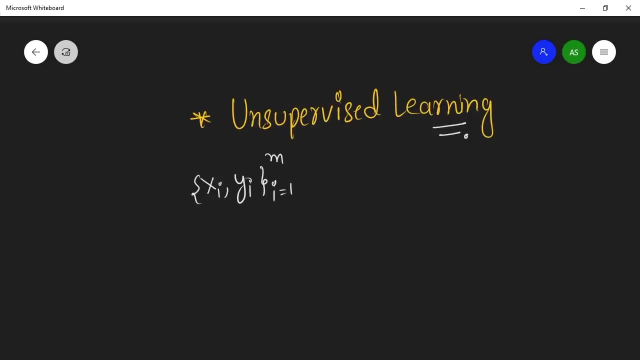 i equals to one all the way around to the n, and actually we have one supervisor, which is yi, and we know what our output should look like means we know what our output should look like and continuous value, which is either regression problem or a classification or a classification. 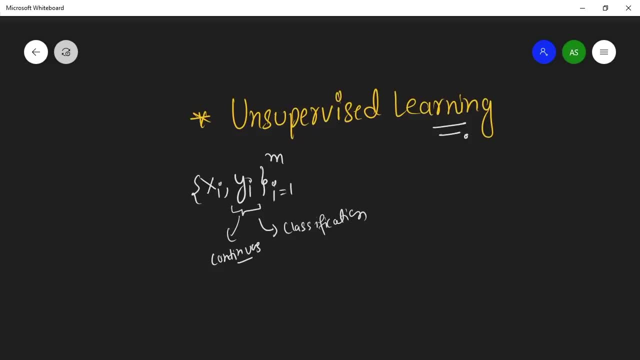 okay, so that that we know that what our output should look like. okay, so here, so we know what our output should look like. so now, in case of unsupervised learning, there is no supervisor. so in case of unsupervised learning, we have only xi. 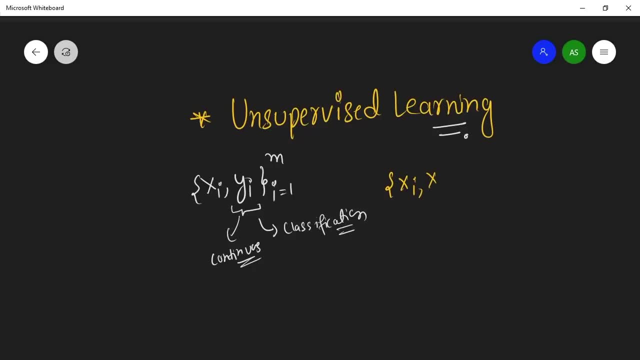 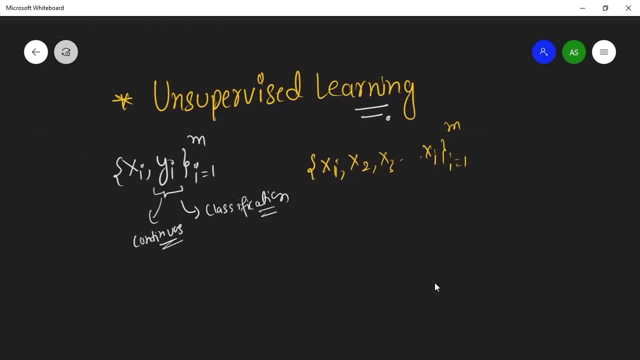 okay, so here in unsupervised learning we don't have any kind of supervisor. that will that? that will tell us what. what will be our either output or will help us to train our model? okay, and we? 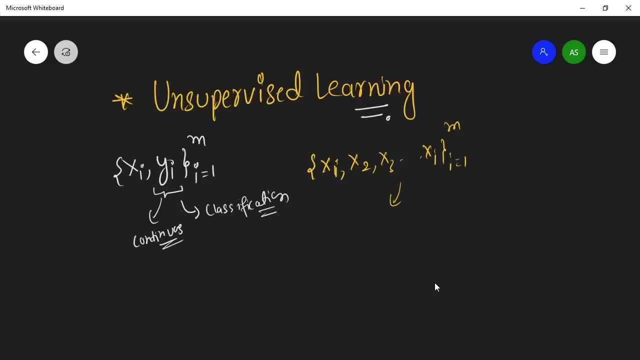 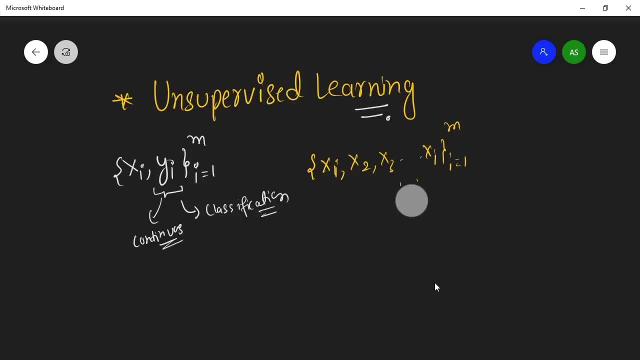 labels, then then you cannot frame, frame it in a supervised learning problem. so what I have to do, what, what we have to do? so but I'm going to do, just want to do is just specify that the data. 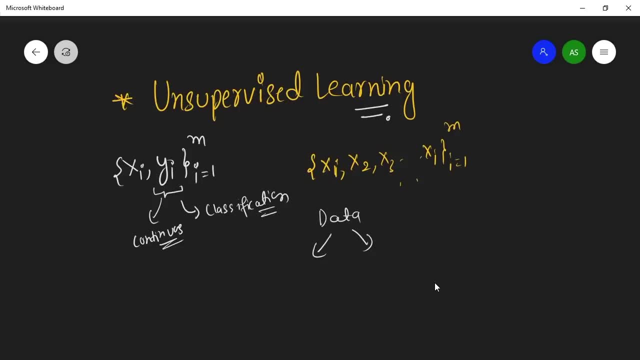 we we have a structured data as well as unstructured data, structured data as well as unstructured data, and a structured data is simply that which is in a table or for for a map, and unstructured data, which is just images, which which cannot be fed around tables. 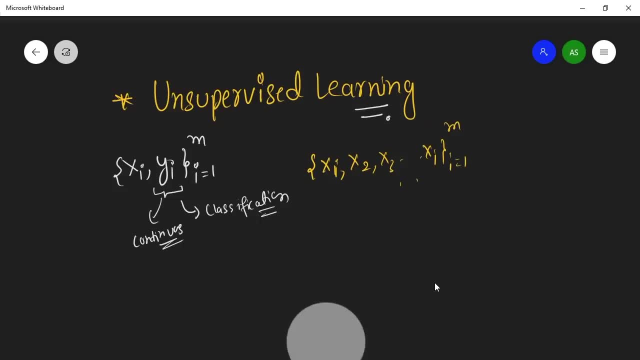 or CSV files, okay, or in Excel, okay. so here, so this is our unsupervised learning, because we we don't have our output okay, so what? what we have to do? this is the main question to ask. 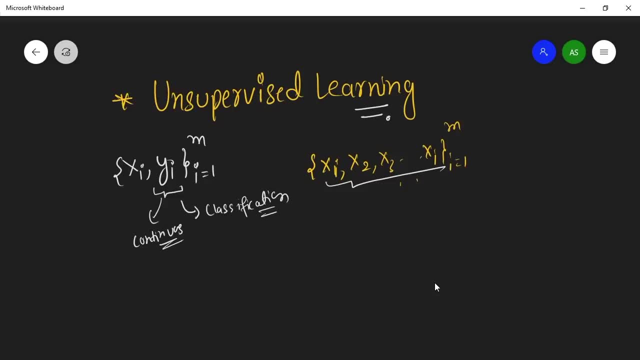 what we have to do if, if we don't have the labels. so let's consider, let's consider you have this, you have this X and Y plane. let me draw it very nicely, so the in this section, I'm just going to, in this subsection, I'm just going to give you an 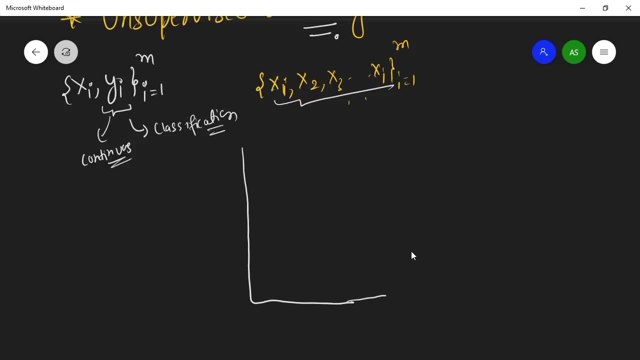 overview, understanding and some of the applications of unsupervised learning. okay, so consider that you are working on just just you have your data points, just you have your data points like this. you have your data points like this into an X and Y plane onto the 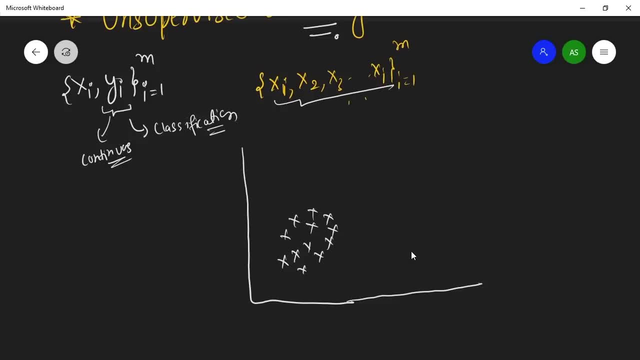 coordinate planes and you have another data points, which is like this: okay, which is like this. and you may ask: hey, Ayush, why can't we make a simple hyperplane? but you don't know, but you cannot frame it in classification problem, just as a motivating example, and I'm 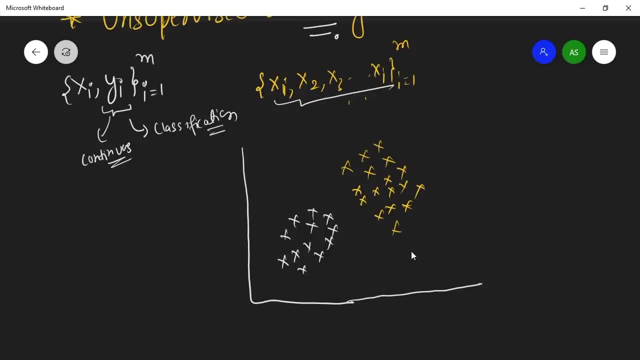 taking it as an example. okay, so here, just assume that you have this type of data set, okay, which is three-dimensional. either. you can make the three-dimensional also, you can make a three-dimensional also just by converting this. and now let's consider that. 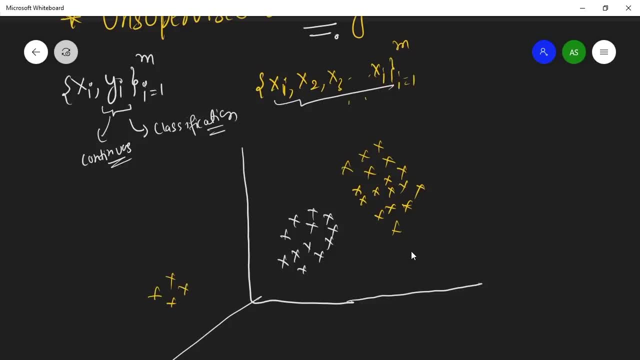 you have three-dimensional features, so here you have this. here you have another examples. okay, so you have this. so now you only have the these types of data points, which is this: this one is X1, X2, X3, these types of. okay, so in unsupervised learning. 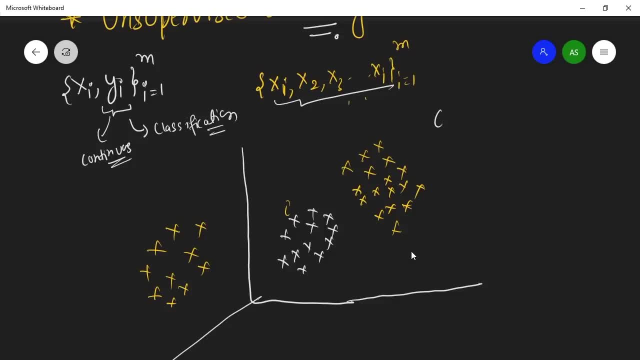 in unsupervised learning what you do. you make cluster of your data which is closest to one point. you make cluster of your data, of your data. make cluster of your data. so, as a motivating example, let's take an example of, let's take an example that you want to segment your. 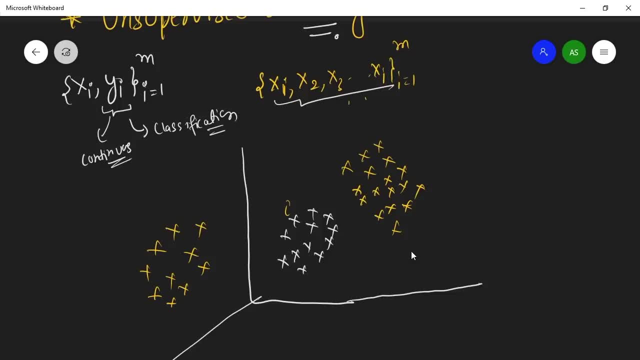 customers. okay, let's take an example: your data scientist at Amazon, some, some, some companies. so you're just wanted to segment your customers. so how you will segment your customers. so what? you will just segment your customers. we have this data, but you don't have the Y labels. so what you will do? you will make the 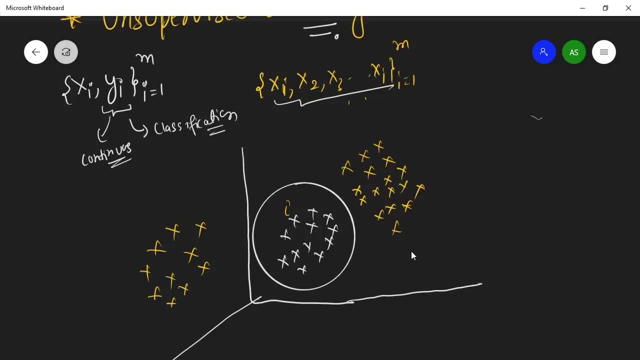 similar person into the one group. similar person into the other group- similar person. let me do that, my bad, okay. similar person and another group and similar person, similar person. similar person into the other- similar person. so what you would have done? you have divided your customers into segments. now, data scientists or business stakeholders- what they can do, they can. 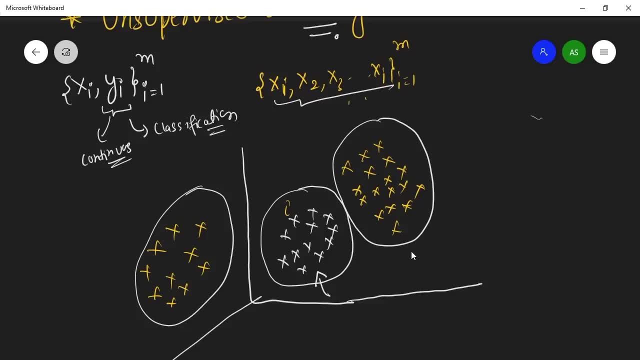 decide that, okay, we can give these, these customers are deal, these customers are deal basis on their activity, what they are doing. or we can make a sub on another machinery model that will detect what they are dealing, what they want, okay, and and we can recommend the products. we can recommend the products. they think these these 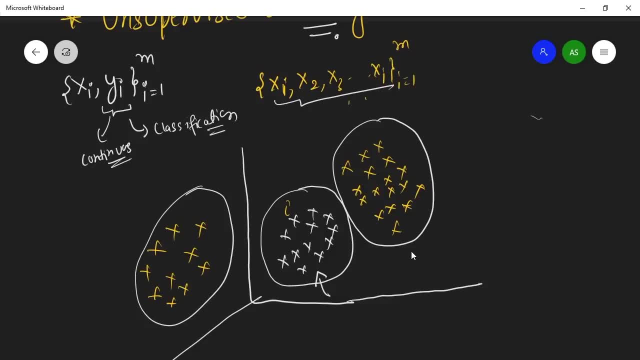 types of customers like milk or like watching the jewelry on that one, maybe an on Amazon, so here on, so on. here you it will show the products of books or maybe some jenneries which are interested, and here maybe they will show you some kitchen, kitchen groceries. maybe these customers are questioning these. 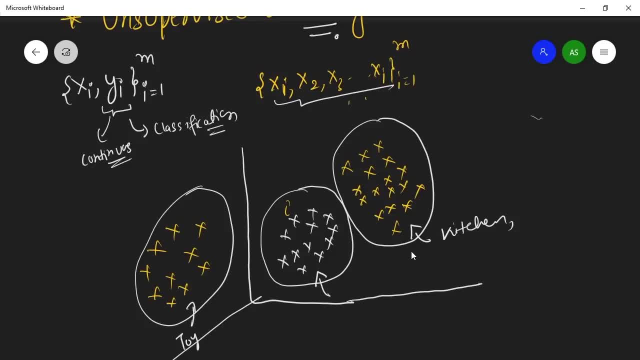 and then these customers can be toys, maybe some TVs, okay, so they will be recommended some products and, according to them, they are a huge amount of money from ads and cetera. okay, so so that's why you can see that how we walk, how we frame. 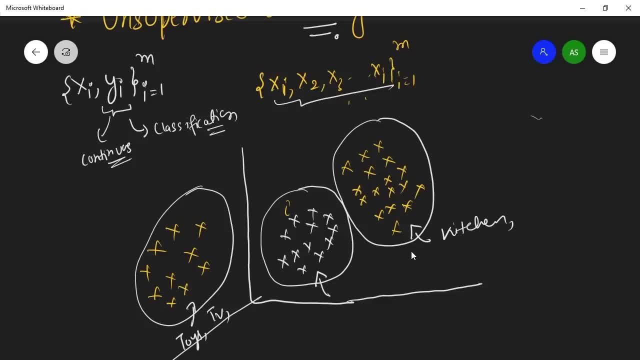 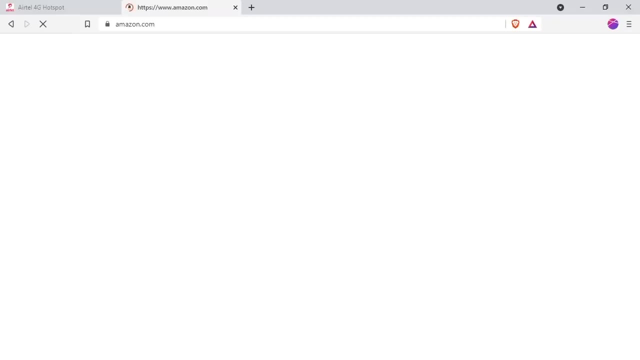 our problem and now you know it's quite clear to understand that as a motivating example of customer segmentation, customer segmentation in Amazon and- and if you may think, here you should- you see that let me go to amazoncom. you will see that I'm being I'm being really good at recommending and they know what I. 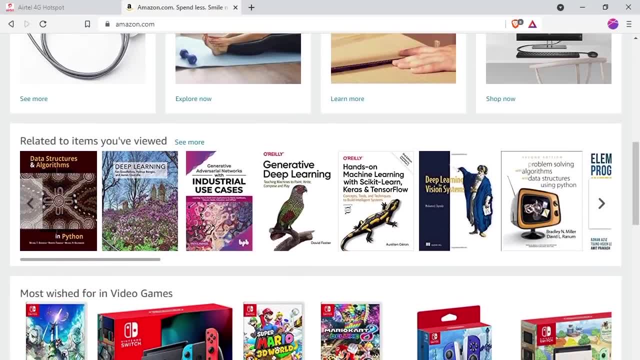 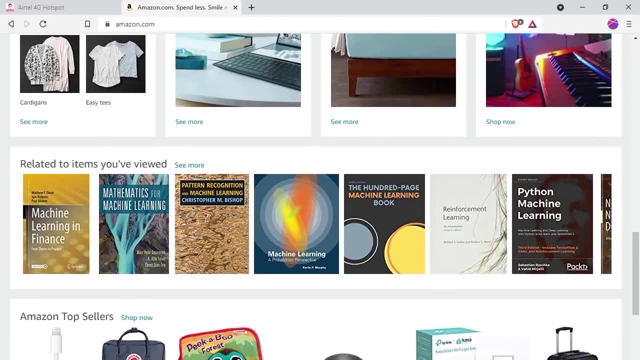 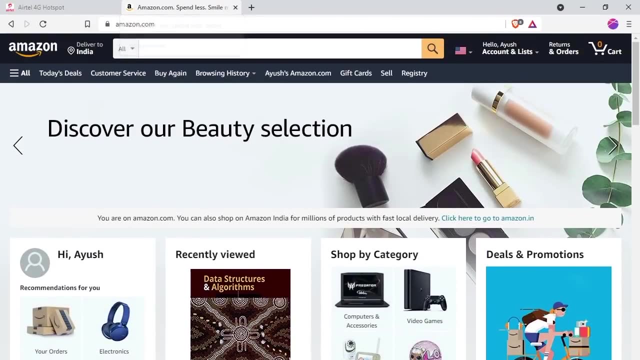 recently view, what I recently view, and they are recommending the products. they are recommending the products which you can see over here, that they are recommending the products basis on my views. okay, so I'm in some segment, I'm in some segment and they are simply recommending the basis products and I hope that you understood and I hope that 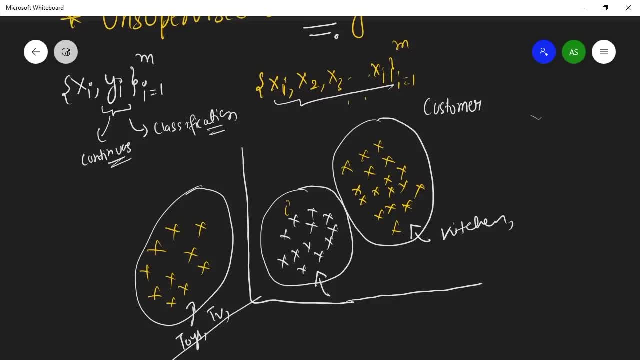 you are understanding what I'm saying as an unsupervised framing the problem, as an unsupervised learning. okay, so that's what the first customers segmentation of and recommendation engine that is happening in Amazon. okay, so I just just see that. just watch the too much talk videos on YouTube. now what YouTube will. 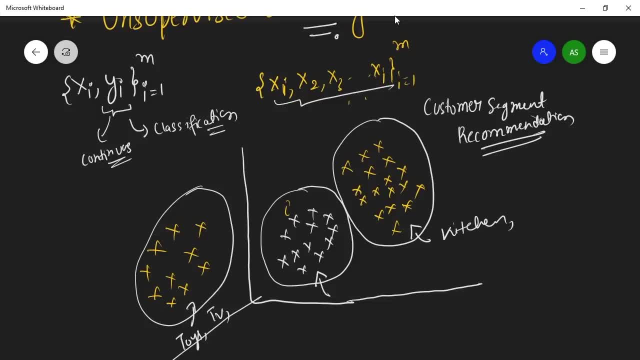 do you do it? take yourself and add it in a segment of the one who watches talks, and now they will show you dog ads- maybe pedigree or it's actually whatever the food of the dog is part of. it should recommend you the videos of dogs, okay, so 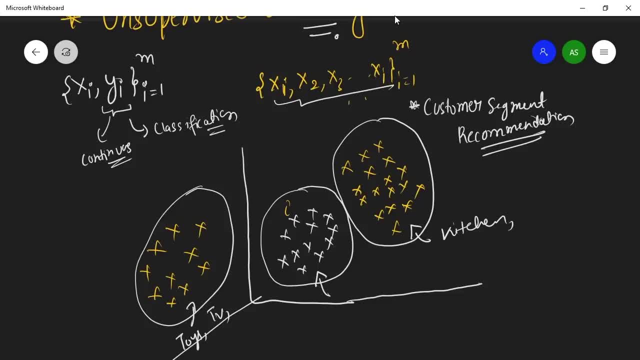 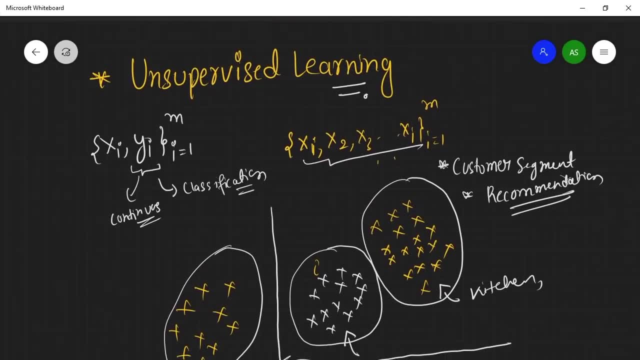 that's why we have the summer segmentation, as in. what a big example. I recommend a shun is an as a more motivating example. so now I hope that is start making sense to you. but why we call this as unsupervised learning? okay, now we. so there's a. this is a, in the end, a supervised learning and supervised. 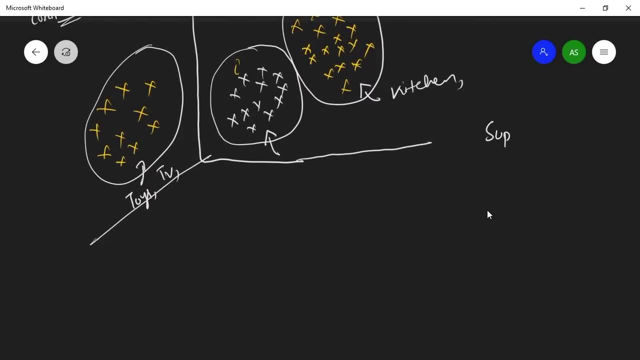 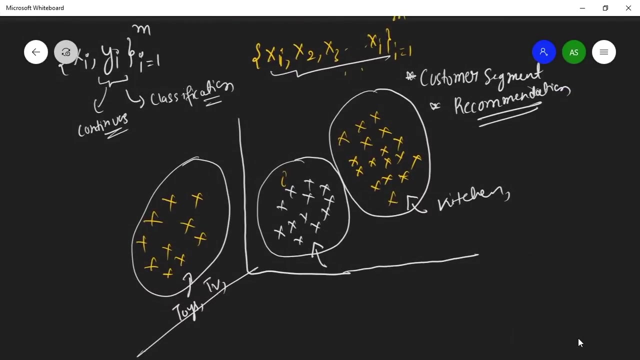 learning we have to two approaches. we have two approaches: which is the regression, which is the regression, and next one is specification. but in unsupervised learning we have something called as clustering. okay, we cluster our outputs with, and if you thought in high dimension of space, then you will imagine that the most similar items are close to each. 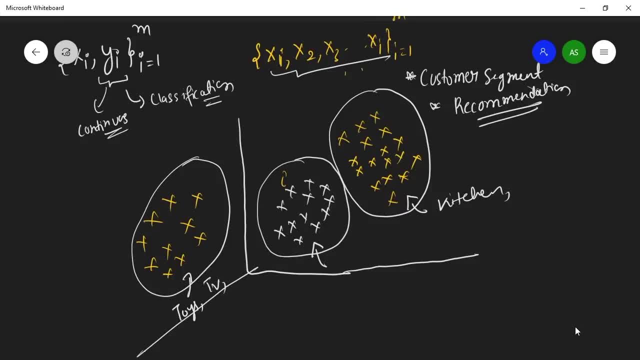 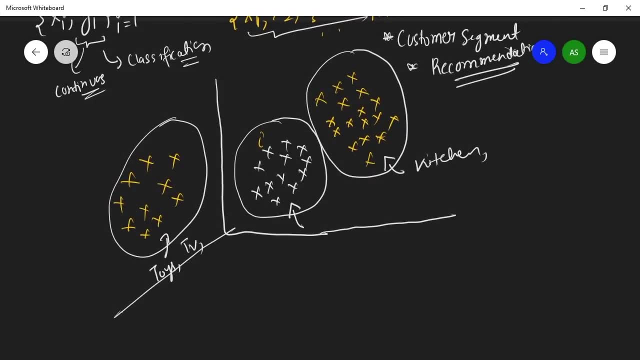 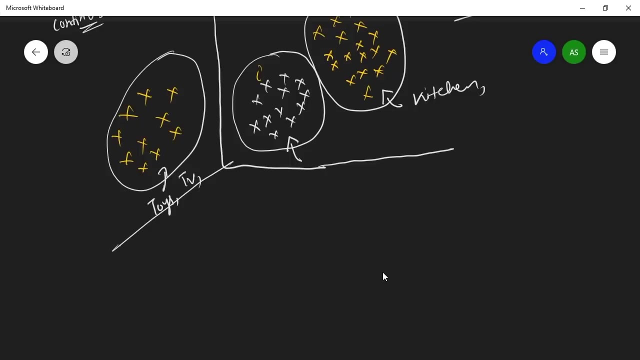 other and most decimal items are very much far away. okay, so you can under understand like this. okay so let's take a, let's take an, a motivating example again. so let's see some of the applications of unsupervised learning. so I will spend a little bit amount of time telling you about the applications of 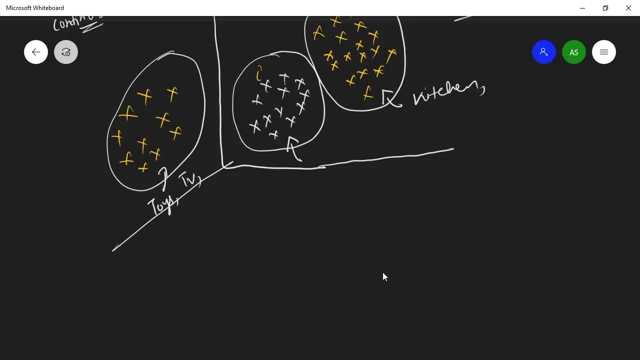 unsupervised learning. and in the next subject we will start with the making clusters. how, what is intro, what is enter, how we do we make the cluster, how do we evaluate our cluster, and cetera. okay, so here I'm not talked about detail of in clustering, about clustering, but I will definitely. but I just told 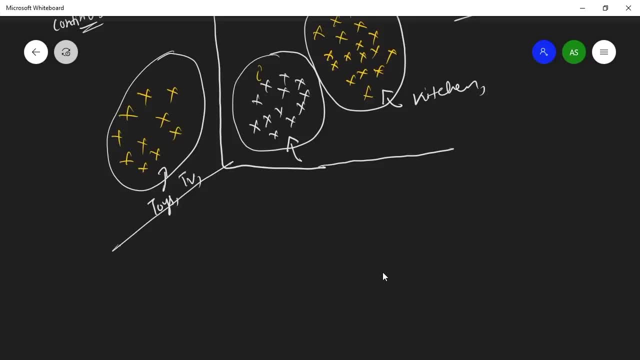 you that we divide our customer into segments. okay, so here here let's take an example we have. now we are taking the. now we are taking a look at the applications. now we are taking a look at the applications of unsupervised learning. so the first application of unsupervised learning is in biology, which I have. 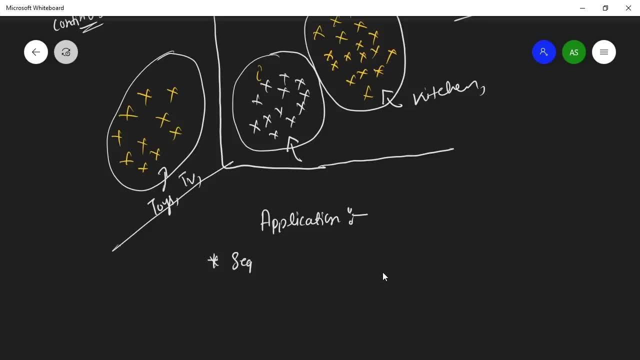 taken from Wikipedia, which is sequence analysis. okay, sequence analysis, and it's simply, it's just put your gene on just genes, into the particular segment and this will help you in various cases for biology student. then you will understand. then you will understand this concept, sequester analysis- because you don't have, Despite, 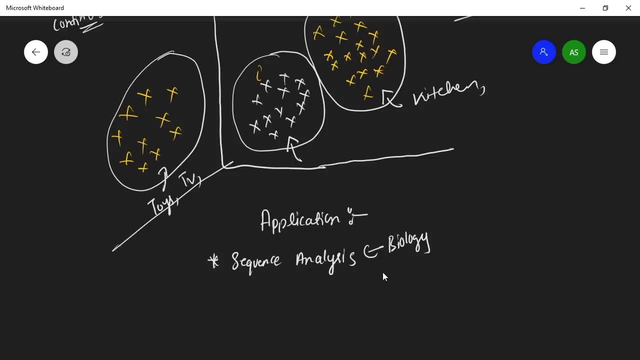 You segment your genes in a particular segment and you can diagnose if this person has any kind of problem. The next application, which is in business, may be grouping of similar clusters for business needs. So let's take an example that some company takes your data and then simply grouping the similar cluster. 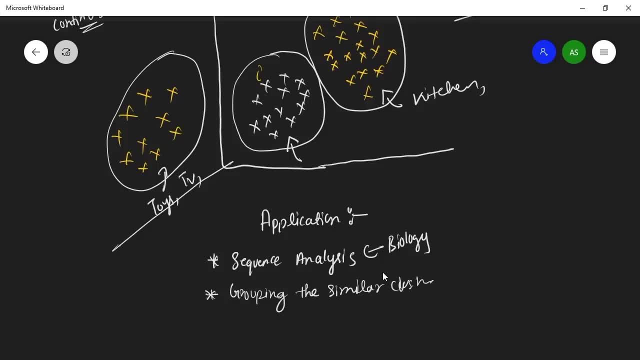 Clusters based on the business data, and they can see the clusters, what they are, what their activity is and they can provide deals, offers, according to their activity. Another thing is we have a recommendation engine that recommends the products that we have seen. So in recommendation you have content filtering- collaborative filtering- content filtering- content filtering- collaborative filtering. 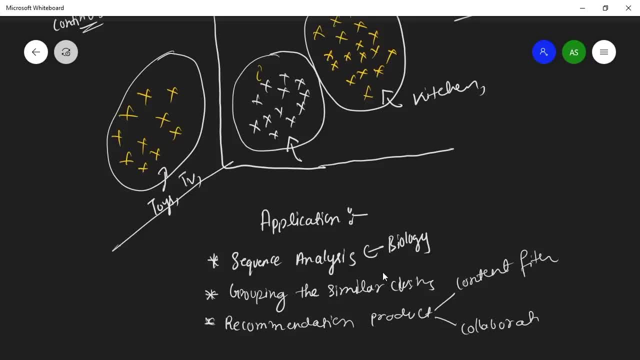 Okay, so which you can see, which is little advanced, but I am not going to talk about recommendation engine, but, as an example, that whatever you see in Amazon or Google, they just show you what you have seen so far. Because they have each and every, because if you search anything, they have that data. okay for making annual models. 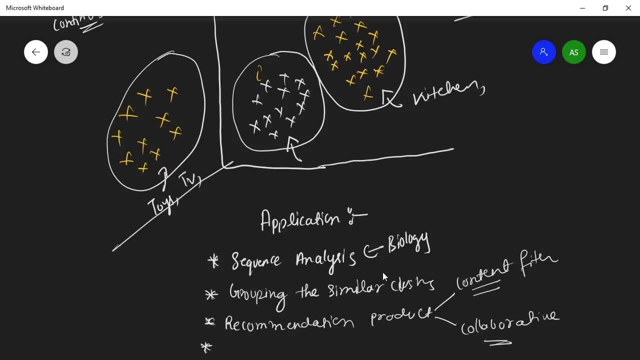 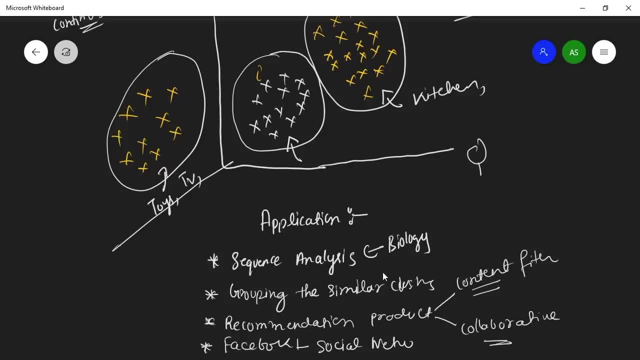 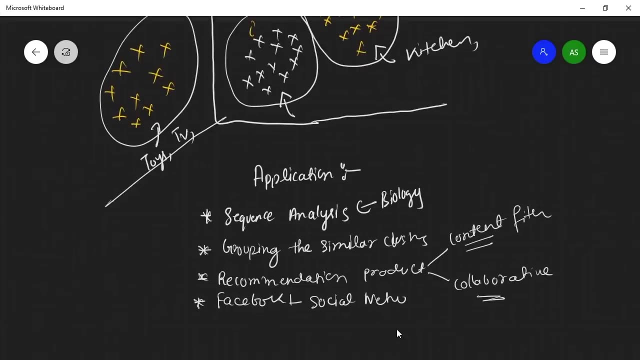 the means these, for they the group customers into the segments, the group customers into the segments, the group customers into segments and the core and they show the accordingly profiles. okay, another is: and we have in computers, computer systems is we have our favorite in computer science, we have image. 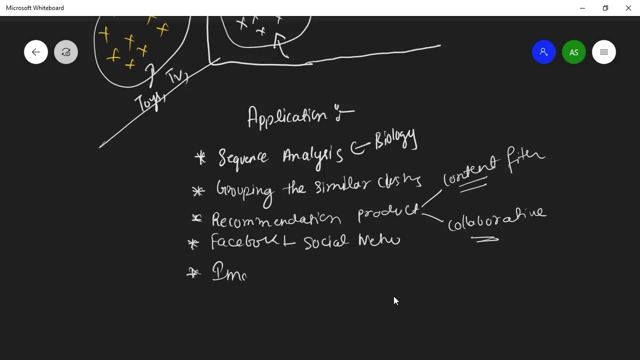 segmentation. so what do I mean by image segmentation? so you have a mage, you have an image and you segment your image, your segment, if you frame, this problem has unsupervised learning. so you have your image, so you have your image like this and some: someone is here, someone is here, someone is here, so you segment. 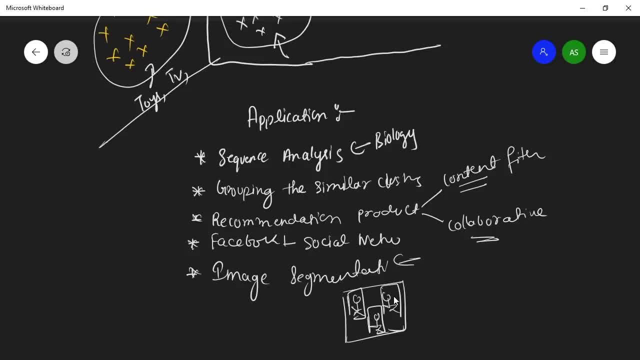 these images, seg, sekman, these images okay. segment, segment these images as a pixel vice. you see that they are. they are similar pixels was segmented and so. so that's where you're saying saying meeting, and then this can be used for classification or object detection. object detection okay. object detection like that, okay. so just grouping your images. 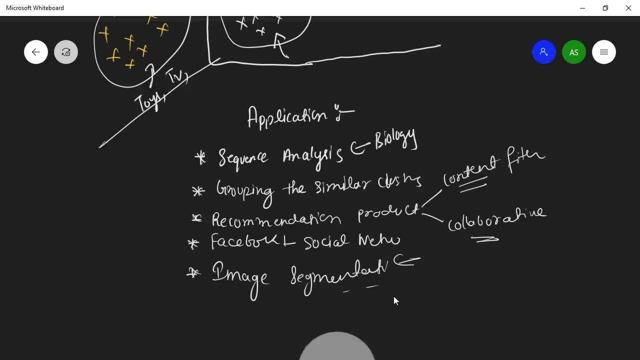 into segments by using maybe pixels and cetera. okay, because we don't have a legal score. by another motivating example- and that's trying, is processing and is sentiment analysis means just just seeing whether it be a negative or positive, okay, so what? let's take an example that you have. this, that is that 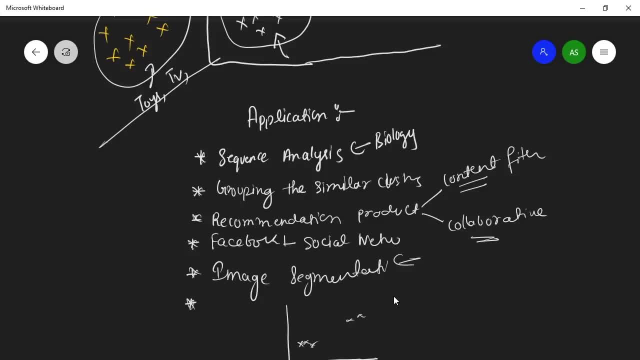 we have this sentence, okay, this sentence and another sentence, okay. so it will group the positive science sentence and the negative sentence, okay. so now you will see now. now you will see now what, what you will do. you will go and see one of the sentence. you will go and go and see one of the sentence. 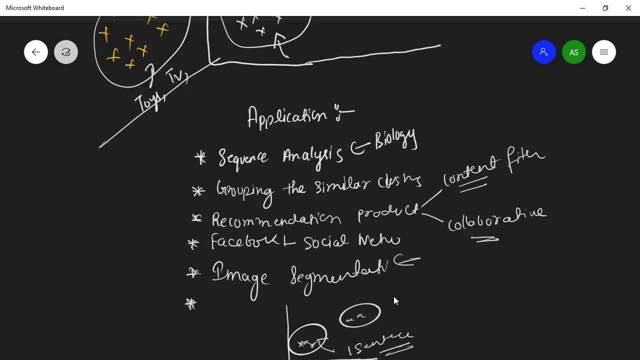 go and see the one of the sentence and see, okay, if it is positive, then you leave a whole, whole cluster which is maybe 10,000, 10,000 sentences as a positive and you date is to hold, then that maybe whatever the number of as a. 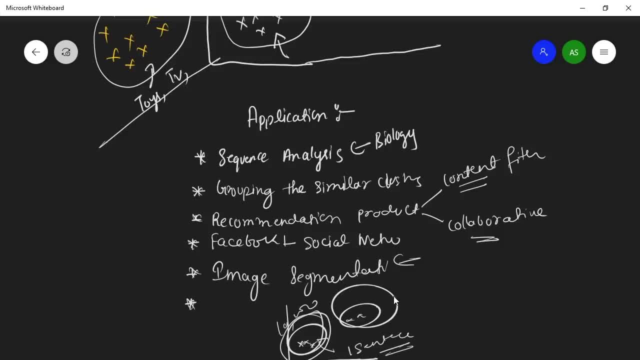 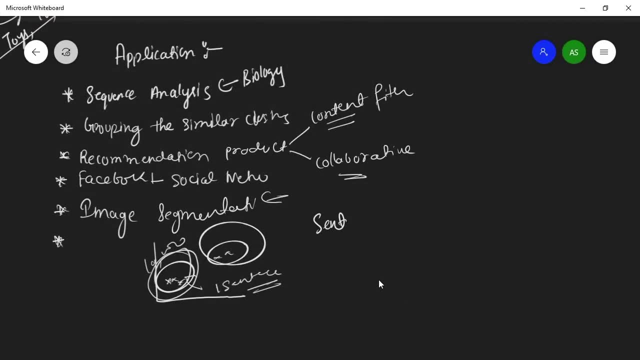 negative. so may let's please take over list. let me elaborate this NLP task of segment analysis. let's take an example: sentiment analysis. sentiment analysis. so for example, an example: assume that you have a 1 billion text, data points in text which are text text, textual, okay, so converter is a word, embeddings mean numbers. now, if 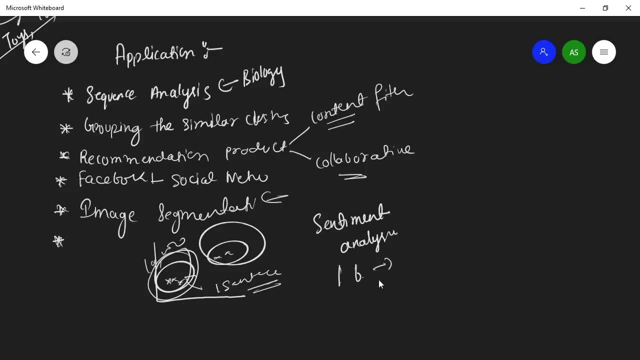 it is very, very hard to label. it will compute. if it will take time, it will take cost. it will take because if you hire some people, you have to give them money. okay, so you have to label 1 billion. so how you have to do so what? 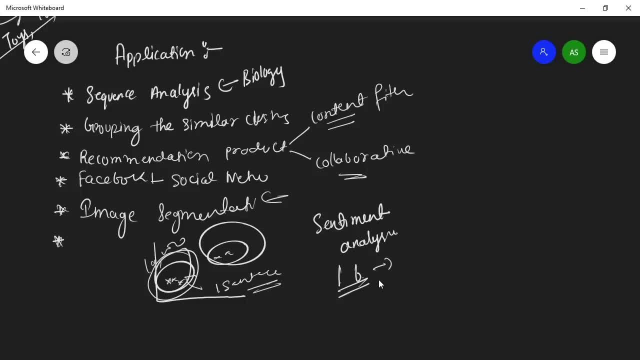 do you? do you convert them into a high dimensional space and you segment the closest text, which is called the word embeddings, closest word embeddings, the word embeddings and sentences are here, and then then you see one sentence is from this cluster with another sentence from this cluster. now assume that this: 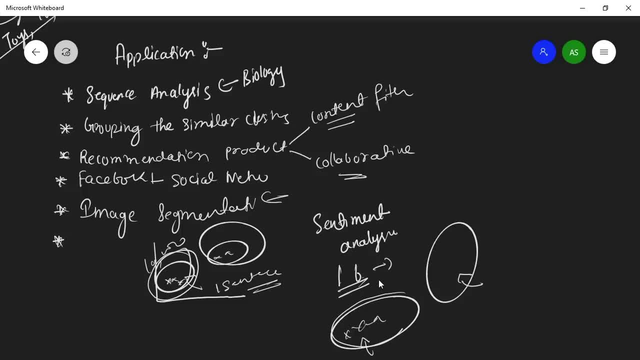 cluster is a positive sentence. to label all they say- 50 million- as a positive and hold 50 million as the negative, okay, so, uh, so you just require it to just you don't require a lot of time for working with NLP tasks, okay, so that's the. that's that's for NLP tasks. another is anomaly: 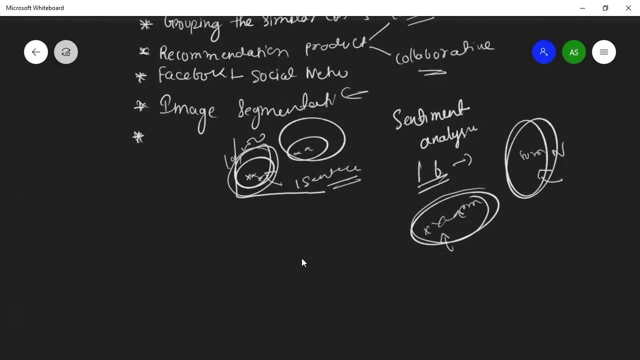 detection. okay, what is anomaly detection? and in anomaly detection, in anomaly, you have anomaly anomaly detection. anomaly detection where we determine outliers in your model. so, as an example, that you have the exact age like this: now assume that your data points is here. so this is actually outlier, this is actually outlier. so if 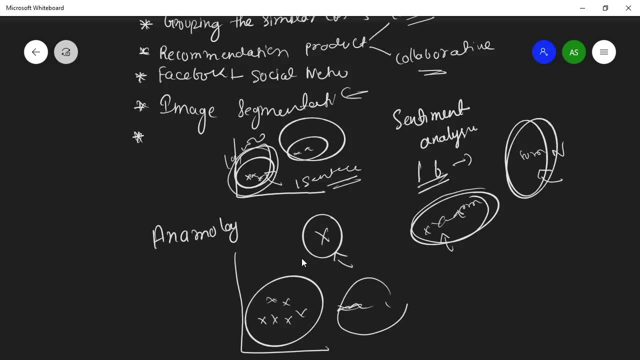 you cluster it. if you cluster here, then this will be ignored and this, this, this can help in in a removing button, but using maybe the TV scan, isolation forest they, but most many of them, maybe some k-means, just take that outlier into this cluster. okay, so let's assume there is a, then it is also closest to then they. 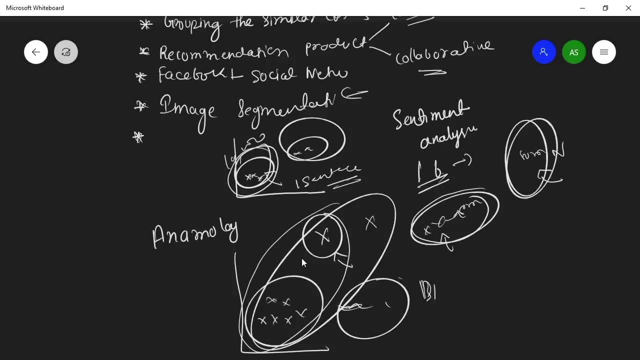 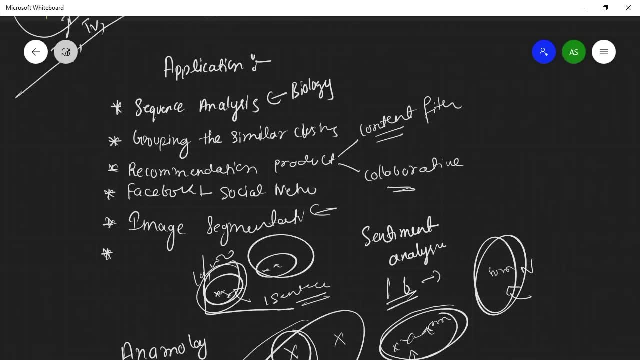 take that into that cluster. okay, so we have a TV scan which helps us into an arm which is actually, which is again our own supervised learning model. okay, in a dense based reasons, great, so we have seen a lot of applications of unsupervised learning. we have seen a lot and I hope that you understood really and 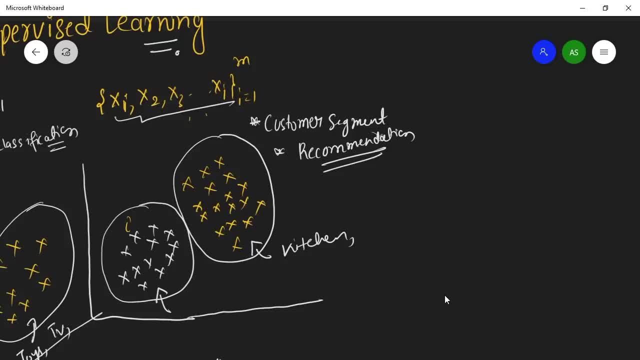 in the name. in the next subsection we were starting talking about clustering. okay, we will deep dive into the clustering to help you better understand the topic. we'll talk about clustering. we will talk about engine cluster and truck cluster, how we evaluate our cluster. okay, how we evaluate our data. 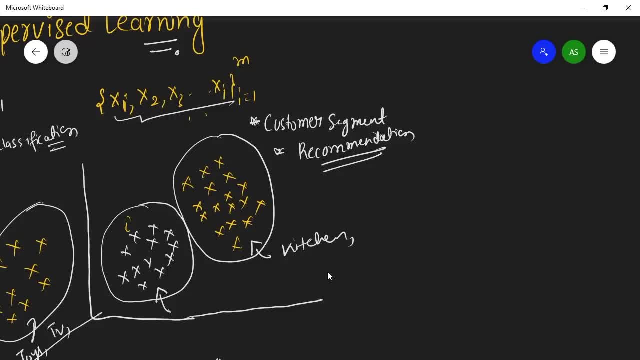 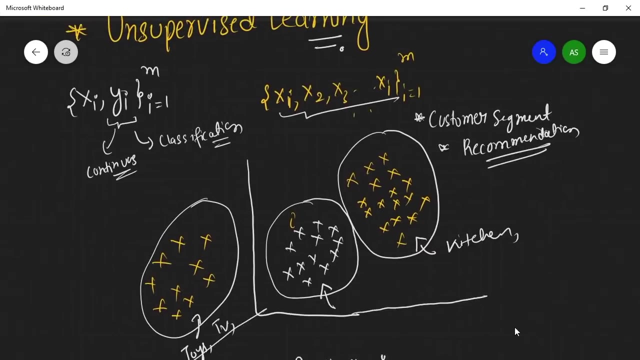 that's that we have a good clustering. what? what are the some of the types of clustering, like partial, hierarchical. okay, then we talked about center based, continuity based, density based, and then we'll talk about one formal center based algorithm, which is k-means clustering algorithm. okay, and then we are done with. 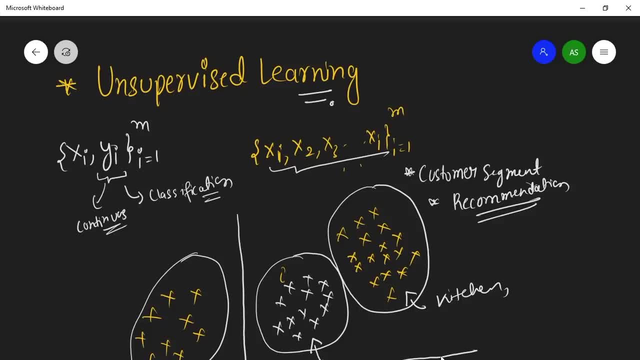 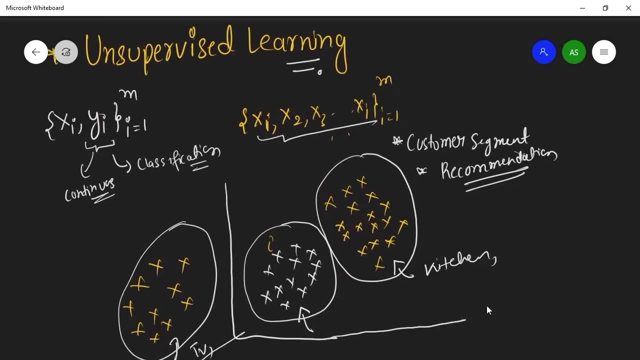 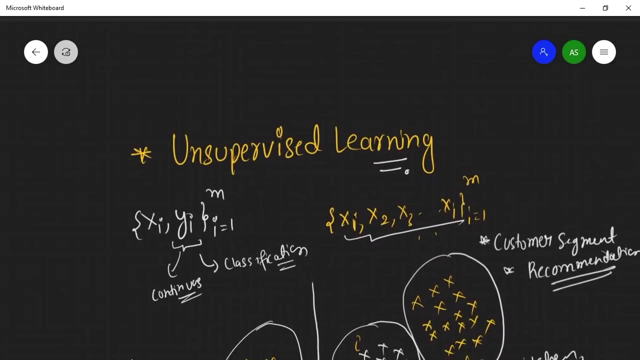 supervised, unsupervised learning, okay, and then I will give you a little bit overview of deep learning. okay, but as you could better understand your deep learning. a journey, just a evaluation, and then we will do some projects based on machine learning so that you could get more feel about machine learning and you are more comfortable and be sure to do. 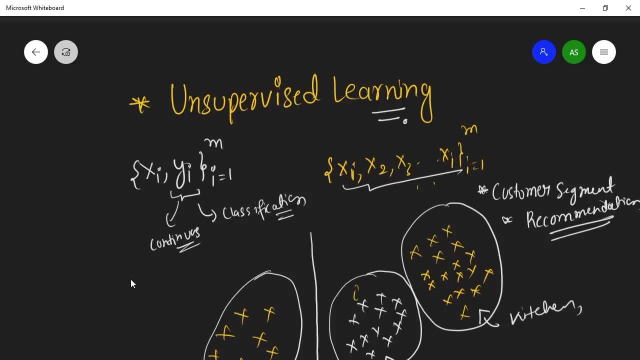 the problem sets which are uploaded and get top to help you want to understand the topic or master the topic. okay, so that's it for this section and I hope that you will, that we have enjoyed this section. okay, so now we'll start talking about clustering. we will get in the math and 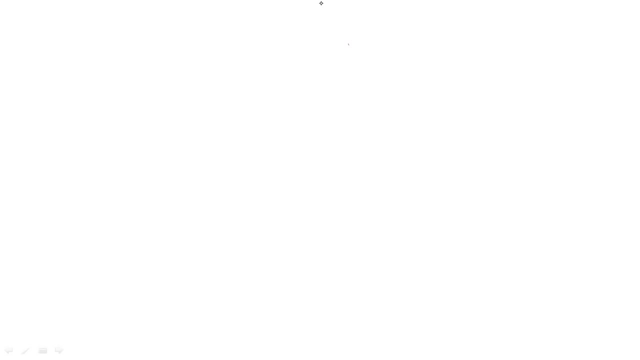 we will see some more algorithms like k-means clustering, then we will see hierarchical clustering algorithms, which is all glomerative and divisive, and then we are and bed unsupervised learning. so we are entering the last phases of this course and I really hope that you enjoyed this course a lot. okay, as I 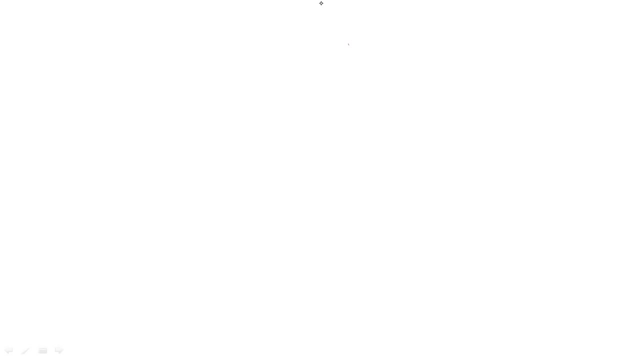 enjoyed making this course with very curiosity, with very energetic mood. so I think that you are also very energetic till now and, like me and you may also thinking: hey, are you sure, what about the projects? and the projects are in the last section to help you to get feel of everything about machine. 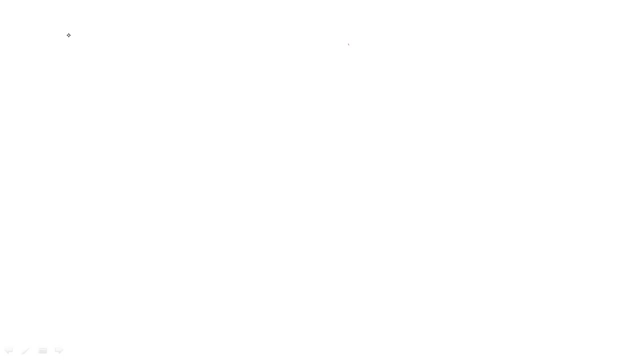 learning means, after you learn all of these things- performance matrix algorithms- now you will be able to build state-of-the-art models. okay, so I'm very excited to see you all there. and it means in this section, last section of building a back-to-back project, and the course website is also in the description. 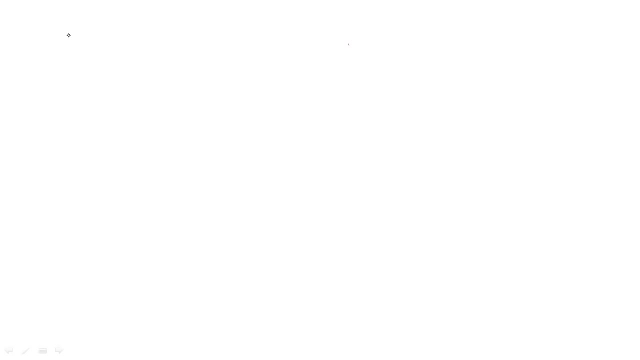 are not below, you can see what's what problem set is there and you can download and start working on that problem set. okay, so you- I hope that you're watching this video- did totally worth it. even I was making video, or was totally worth it. okay, so what we are going to start talking about? we are 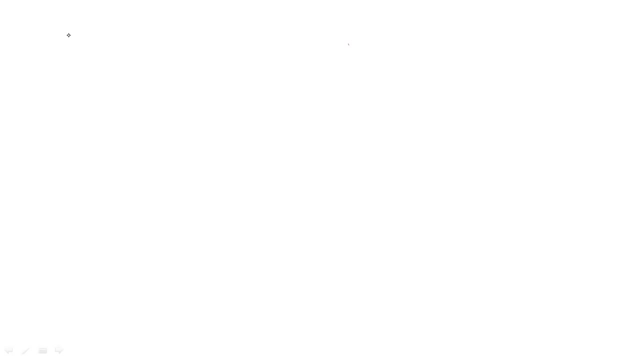 going to start talking about. we are going to start talking about clustering in the in our previous section will be. we have talked about some of the applications of clustering we have talked about. let let me choose a pen, a good pen. we have talked about applications. we have talked about applications of clustering. we have seen 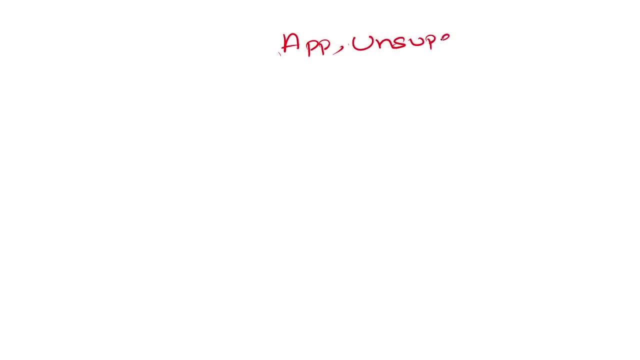 what unsupervised learning is, what unsupervised learning is, and we have seen the dagger and tiger, some a lot of applications like biology and business and cetera. I've seen the applications of unsupervised learning and then I've shown you the data, okay, and then I've given you an overview what we do in. 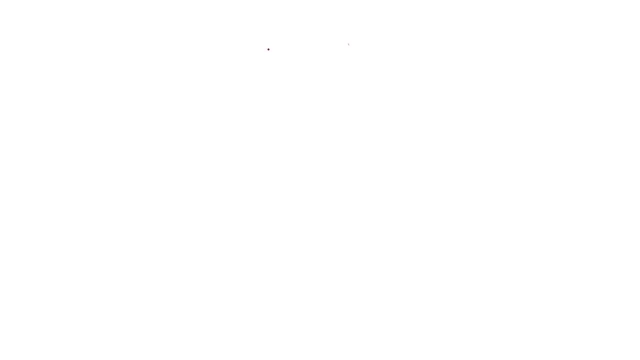 clustering. okay, so let's start with clustering. okay, so how, what, what, what we it, what the clustering is, what the clustering is. but don't just bear with me, but then with my handwriting, because I don't know what happened to my pen. it's very working bad, but no worries, let's start. so here, let's assume that you. 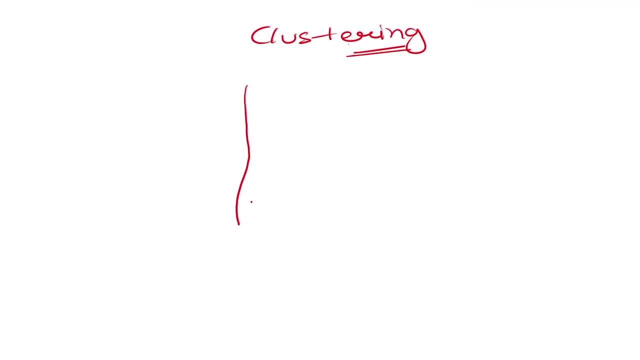 have this, you have this, you have the great. oops, let me why it is not being removed. let's assume that you have a X and Y plane where you have a, two, two features, where we have a, two features like this: if I draw a straight line, if I draw a straight line, okay, so here. so here you. 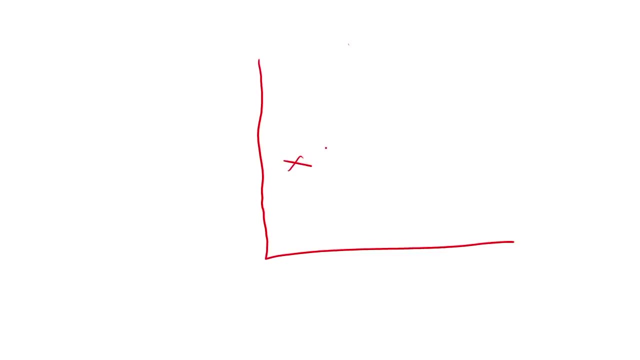 have this and let's assume that we have here as a point here, okay, you have this as a point. and Another point, and another point is green ones, which is here, okay, So no, in unsupervised learning and unsupervised learning, all data are same. by, I forgot. 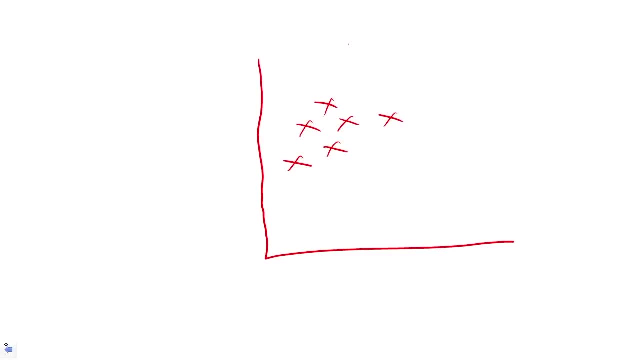 No worries, I usually forgot everything. okay, so what you have? you have these features, Red features, and you have this here. so what you usually do in in case of clustering: you segment your clusters, you Segment your data into different, different clusters. Oh, oh my God, Why it is not happening? Yes, 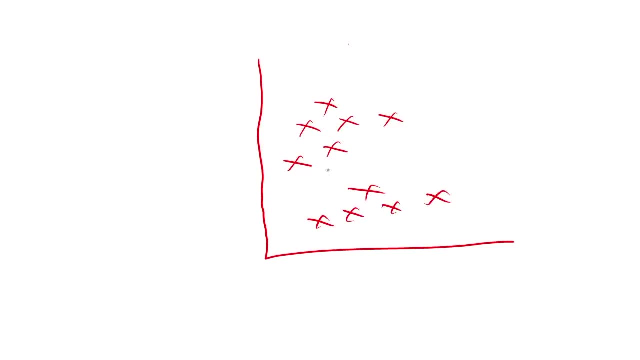 You segment your cluster, so you have this data, so you segment this cluster. you segment this cluster To be going into this and the second cluster We're going into this. Okay, so this is first cluster. This is your second cluster, okay. 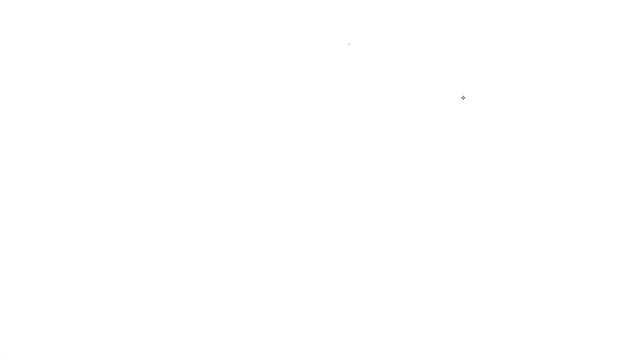 So this is your basic, inter basic thing about clustering. that that we have talked. okay, So we'll see some of the terminology In this, so let's draw a very good Representation of this diagram. so let me delete all this links now. Let me choose a black pen. it's works best in the in case of white. 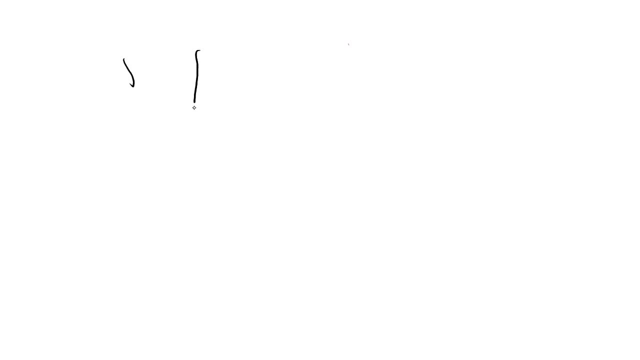 Okay, so you let me draw a straight line with X plane. okay, so you have X and Y plane, X and Y plane, and here you have the data point. Here you have the data point like this and here you have the data point like this. Okay, so what do you know? you segment your data points into clusters, use your cluster, it out. 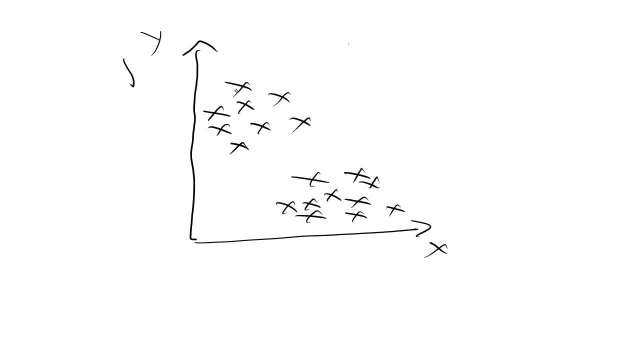 So some of the terminology is: you cluster this, you cluster this. let me draw a good Cluster. you cluster this and then you cluster this. Okay, so let's leave that. I don't want to make it like that. Let's leave that for now, okay. 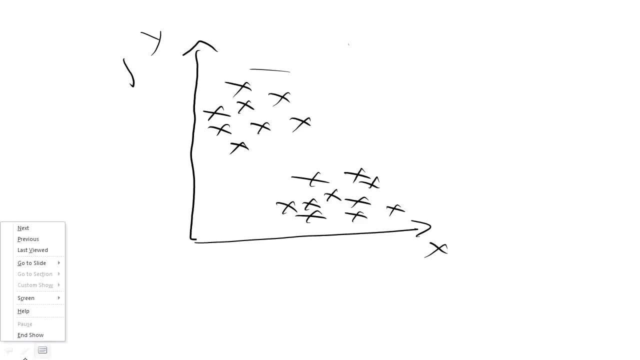 so you cluster this out, and Then what happens? so here is a terminology. alert means the. in terminology we have something called as Intracluster, we have something called as intracluster, Intracluster and intercluster- just us just listen to what I'm saying. intracluster and. 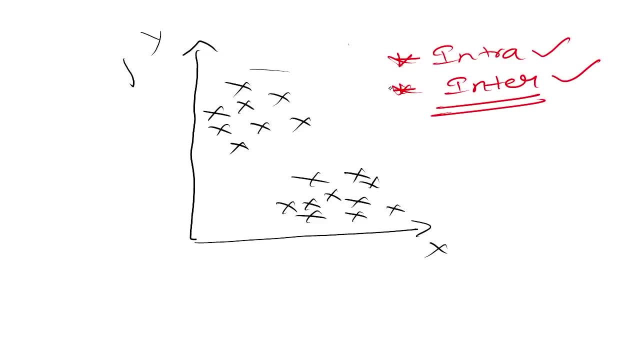 Intra and inter cluster. so what do I mean with these intra and inter? I mean with this entire and intra and inter is: Is Inter cluster is the distance between the cluster, okay, between between the clusters, Across all the clusters. so inter cluster is the difference, is the distance between across the clusters. so here we have one cluster. 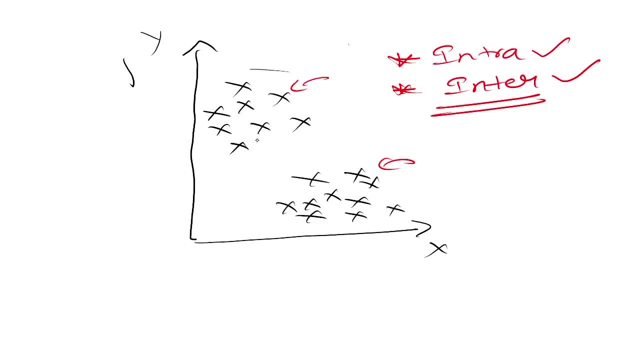 Here we have second cluster, so entering inter cluster is the distance between This cluster and this cluster. It's the distance between this cluster and this cluster, so that's why it's known as inter cluster. Okay, the second type of his intracluster, which is the distance between: 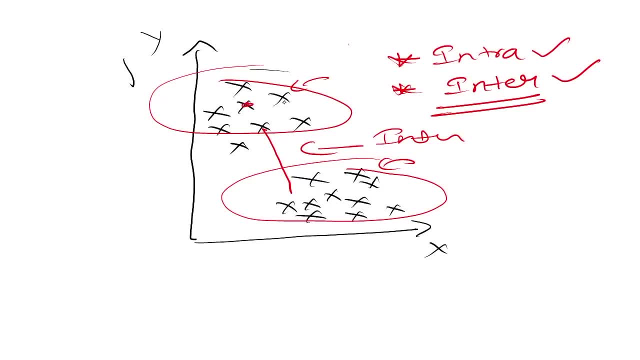 Within the cluster. that points within the cluster, within the cluster. so it may be like this: This is called, This is called the intracluster, This is called the intra Cluster. I hope that you are. that is making sense now, this x and y plane, and you have this, this kind of thing, and 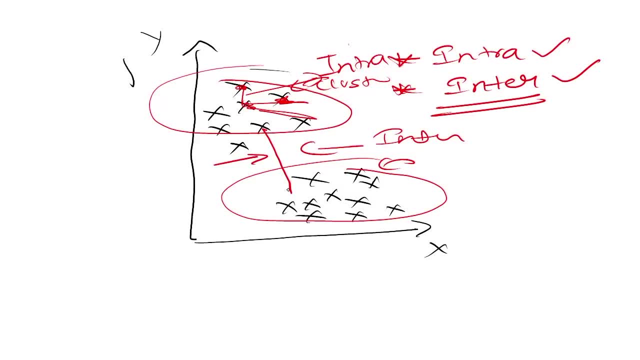 What to what we have to do. this is. this is called the intracluster, where we have the distance between two clusters, or maybe two or more than clusters across all the clusters, and Intracluster is the distance between the data points inside that cluster. Okay, great, so we can think. think something like that is. 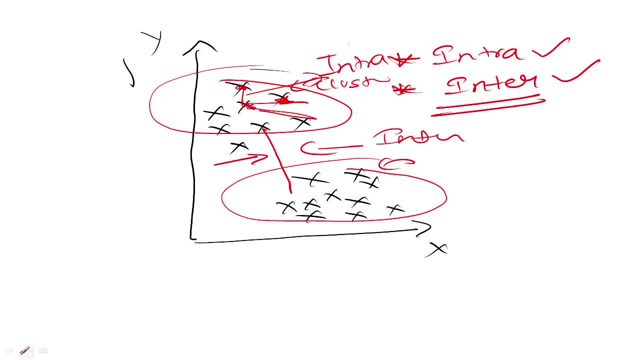 We want what we want in this case, if you're taking as a terminology that. so we want our Intracluster to be small, intracluster, intracluster to be small and intracluster, Intracluster, intracluster to be large. What do I mean with this small and large? I 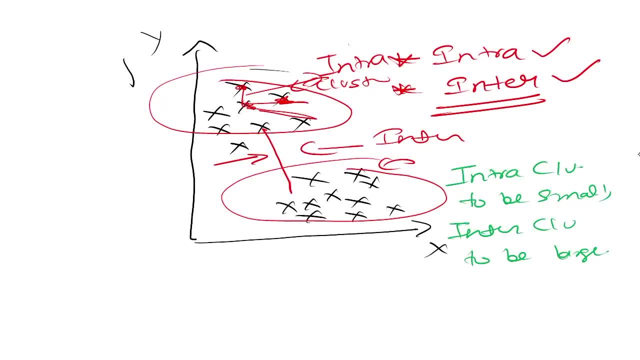 Mean with this small and large is you have this intracluster. Intracluster is the distance between this and this and the clusters takes whoever is similar. a group Is a cluster is, just as in is a grouping of the similar objects, that they are similar to one another, so they should. 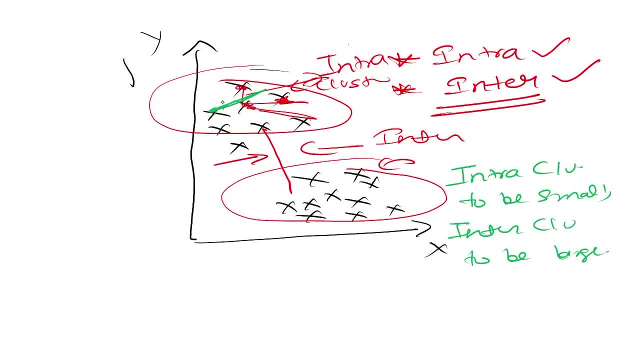 The data points should be closest. the data points should be closes and the intracluster of these should be closest, Okay, and the entire cluster, inter cluster, means the similarity between two clusters should be Maximum, okay, so here We have original optimization objective. We have we, we want our inter cluster. our inter cluster, which I did, is I n should be large and 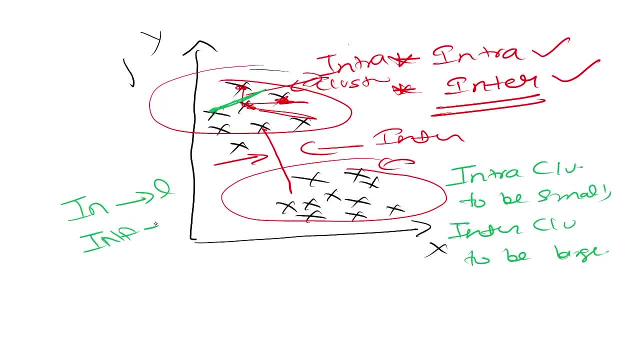 I n should be LARGE, and I am, and a should be intra cluster should be small. okay, so that's the, that's the basic definition of, that's the basic, basic terminology that we have seen and i hope that is making sense. okay, so we can frame some problem. we can frame something over here. what we can frame is: we can. 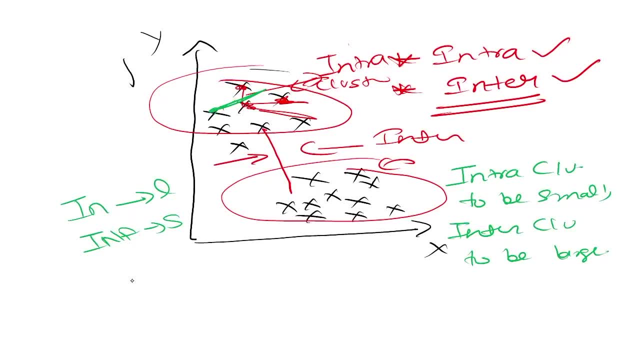 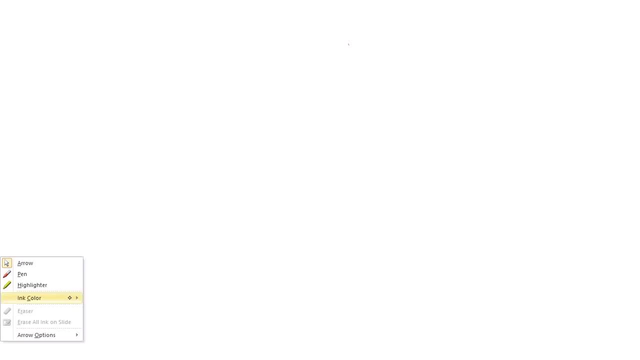 frame an optimization objective, we can frame a evaluation technique, but before that, why do we even need? so let's assume, let's assume that you have this, you have this cluster, you have this cluster, you have this cluster like this. you have this cluster one, two, three, four, five, six, seven, one. 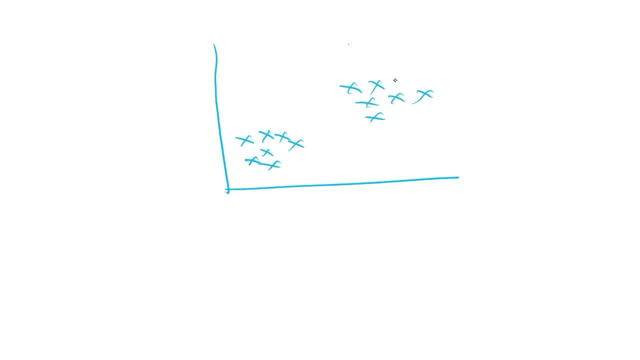 two, three, four, five, six, seven. okay, so here we have this, and who can tell you, who can tell you that these are the perfect clusters? these are the perfect clusters. either you will tell here you, i'm able to see, i can tell that these are the perfect clusters. 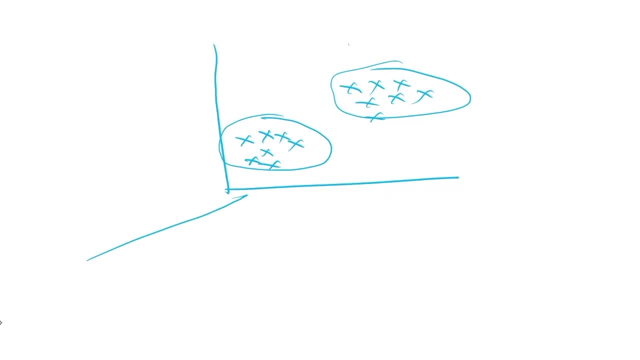 but assume that we have, uh, three dimensional, we have four dimensional, we have 50 dimensional, we have 80 dimensional, we have 100 dimensional, we have black dimensional. so what you will do in that case? so we have evaluation techniques. okay, we have optimum evaluation technique that will. 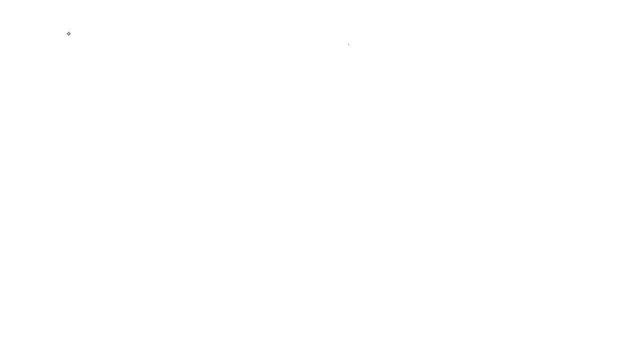 help us to identify, to evaluate our clustering or unsupervised learning, our clustering model, okay, clustering model that will help us, uh, ideally, to understand, to, to evaluate how good our clustering is. okay, so let's see how some of some of the evaluation uh techniques okay. so the first: 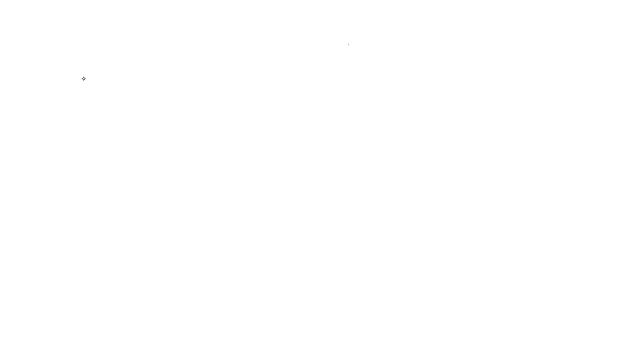 one we have which is called done index. okay, so the first one we have is called d u n n index. so this is: this is a very funny name, but it's this very guy. you can see, it's very funny name, but it's so read about in wikipedia page, so it's so let let me first write the equation. so d equals which: 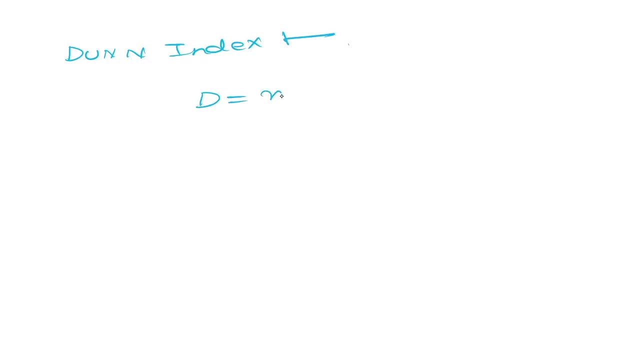 is a done index. equals to the maximum maximum of i and j, means the maximum. should maximum distance between i and j divided by or by maximum k, a maximum distance d dash between k. okay, so here what i'm telling. here we have this, we have this intra cluster. 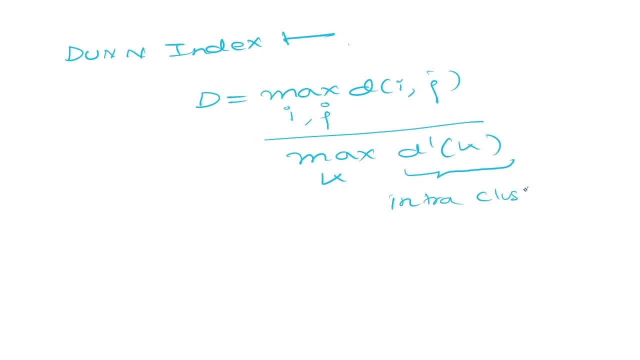 we have this intra cluster here. we have maximum inter cluster distance, maximum inter cluster distance, inter cluster distance. okay, so ideally it is framing our problem of intra and inter that our inter inter should be small. and also the answer is n. i should be small because the x and y are. 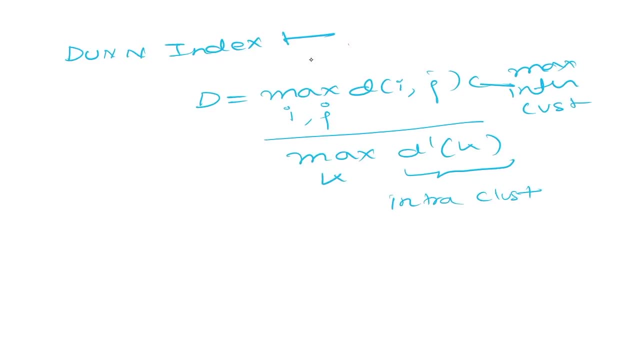 our interest should be large, okay, so here we are not assuming should be small, we are assuming what is the largest maximum distance? okay, so if every everyone is small, then the largest maybe 0.00 like that. okay, so maybe something like that will be there. so we are just changing this maximum, okay. 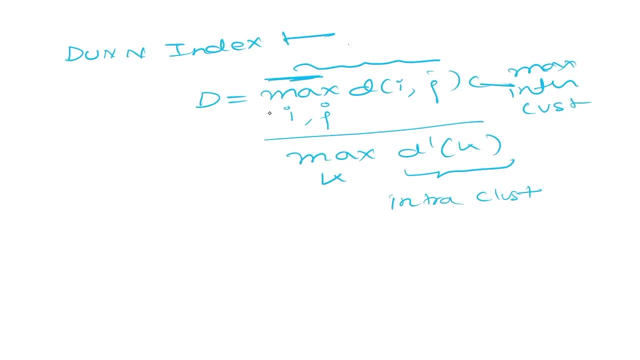 we have maximum over here. just don't be confused. we are telling minimum interest. that just ideally means that you want the distance between inter cluster to be small, so that's why you are taking the largest. whoever the largest have, whoever they have, a largest distance, okay, so that's why. 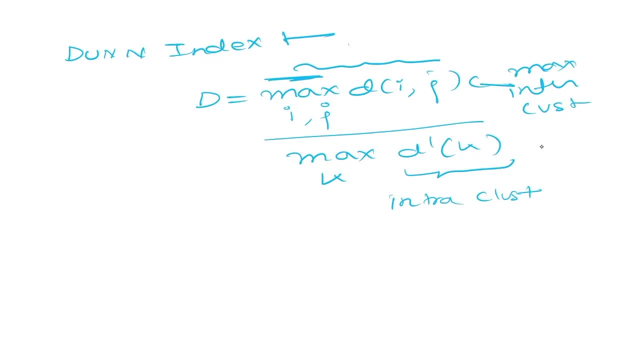 social, so you, so you can evaluate your model. and it's this, this sim, this the denominator simply means that: and the the distance between your intra cluster, okay, the distance between your clusters, the distance between it should be ideally large, not too much small. okay, so that's the, that's the. 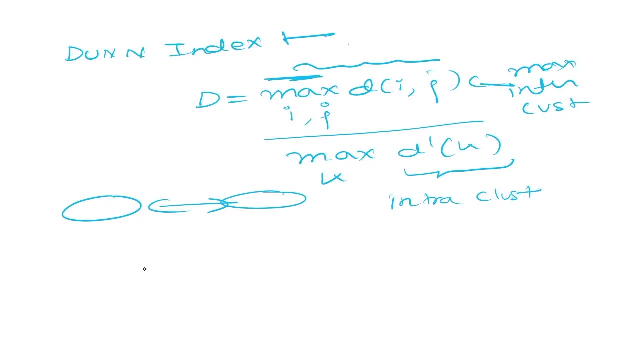 and if you feel, seen, if you see, if you sense it's math, mathematically you can see that D should be high. D should be high. to be a good, good cluster, D should be high. okay, so this is the evaluation technique for clustering your model and I think that you understood, done. 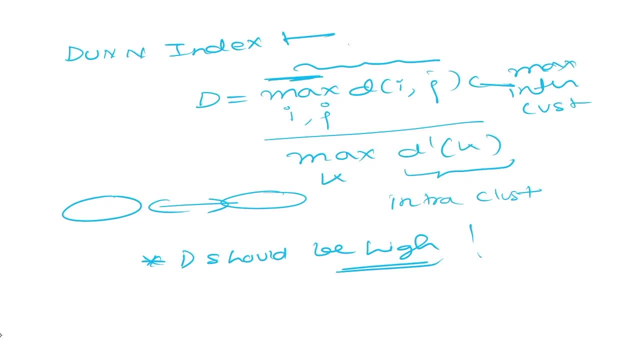 index. so let's recap to late. what we have seen so far is we have- let me remove this, let me remove this. so we have seen that we have some of some of the terminologies. so we have this small x and y plane where we have the 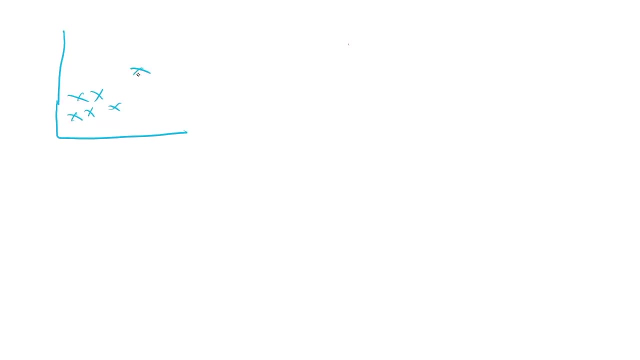 blotting Sch nous here. so we have a house two, we have this block space. maybe it is the. is thats be the sum of the in this ac vào here, coz the and you also, you have 11 times 12 is same thing with range 12. again also here you have to Trivis. You can take thisしょ to this courthouse on, because so it's very complicated that one part for a singleеры. distance between, Because both arethings between between two. the distance between the, the distance between two clusters. The distance between two clusters is called as intra cluster. Please, across all the clusters, maybe some cluster will be here, another cluster aynı. 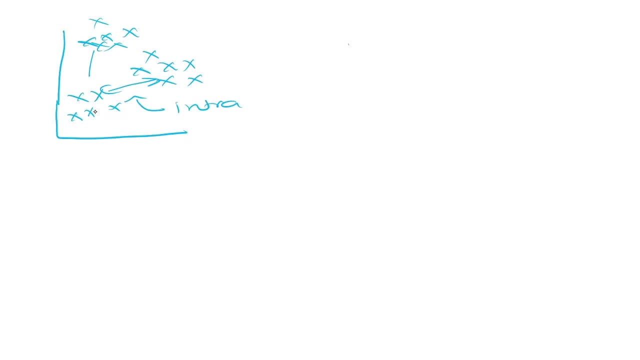 across all the clusters. maybe some cuse Raise help United. Wow, that is across all the clusters. the is прот��. This is called the intra cluster, and the distance between within the cluster, within the data points, is known as the inter cluster, is known as the inter cluster, and core idea is for any valuation matrix of your clustering model is: your intra cluster should be large, intra cluster should be large, large and inter cluster should be small. 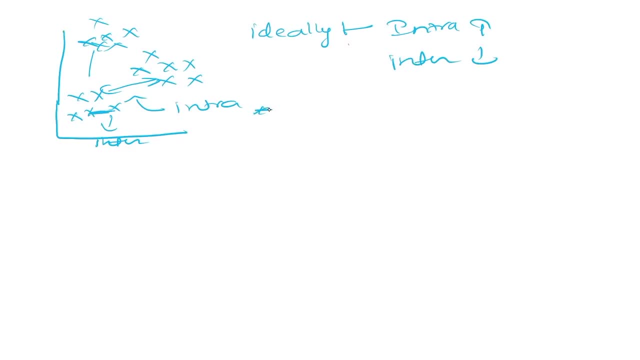 Okay, so we have the. we have talked about, about a done index, We have talked about a done index. We have talked about done index and done index is simply evaluation matrix. So the done index is written as: D equals to the max of the distance between I and J, which are two data points, which is obviously inter cluster, which is obviously the first numerator is: 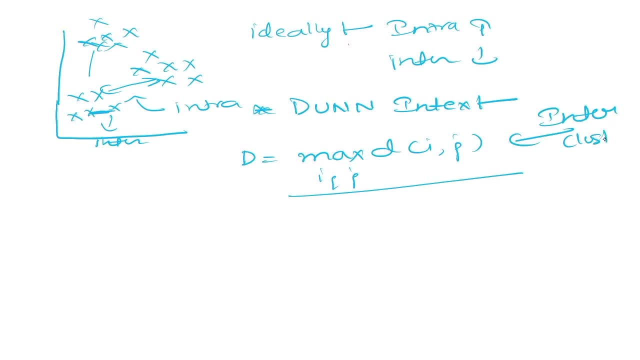 inter cluster, Okay, and the denominator is simply the intra cluster where you want the maximum distance, maximum distance between the values. Okay, so this, this is a basic definition and you may think here you should have told about entry. inter cluster should be small. but we are checking the maximum so that we can evaluate. we are checking the what is the maximum in that cluster that has the distance so we can evaluate. So everyone should middle, so our D should be high in that. 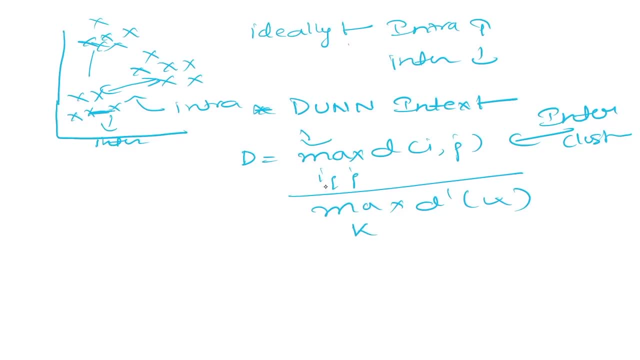 cluster case. Okay, so I think the two are understood, done, index also. So let's see one more, one more evaluation technique, which is for clustering, which is just just. I'm setting you just some, some constraints to be added, And I just have seen the equations, just some conditions to be added in ing where, here in I, here in I, I should be, I should be greater than I should be. 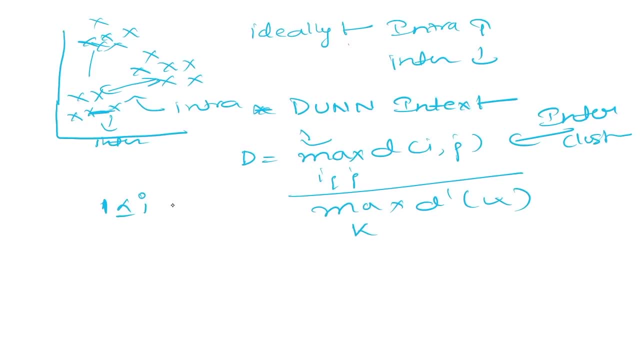 greater than or equals to one, or it should be, And it should be smaller than or equals to J And J should be smaller than or equals to n And n. here is a number of training samples And for K, constraints of K: is your K should be smaller than or equals to? is true, it should be at least a smaller should be smaller than or equals to n. Okay, so that's the. that's the basic definition of that's. that's the basic. 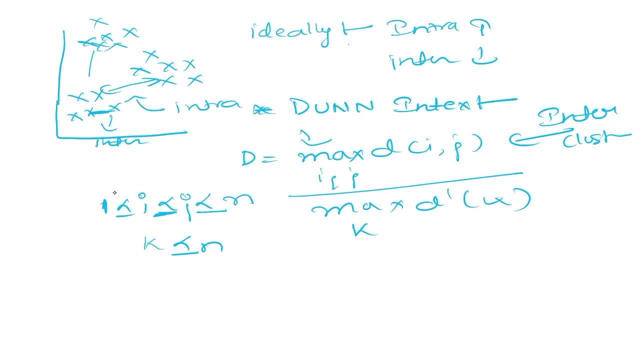 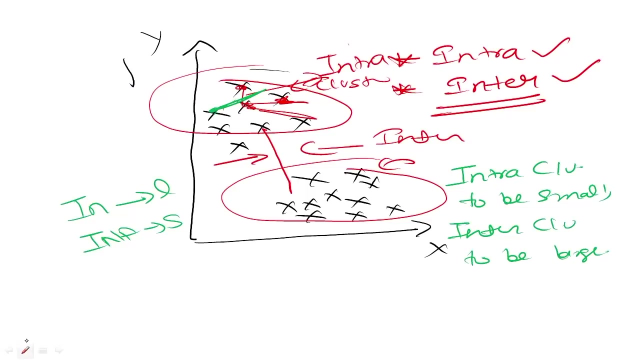 definition of that's. that's the basic definition of. that is the basic definition of. that is the same. Okay, so another way, evaluation technique, that that have seen so far. let me. let me go back, actually, okay. so here I am on my another thing and let me remove this, okay so. 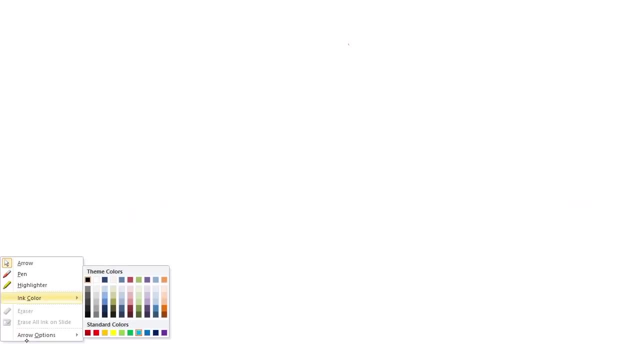 another tech technique. another technique is here in front of you, which is the Davis-Baldin index, Davis Davis-Baldin-Baldin index. this is also like done index. what do you want here? we denote is that DB equals 2. we take it as. 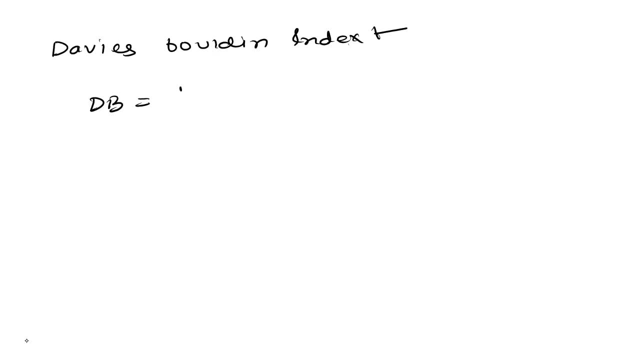 a DB equals 2, 1 over, and I equals to 1 all the way down to the N, and then you take out the maximum. take out a maximum where G is not equals to I, Sigma, I plus Sigma G, divided by the distance between CI and CG. okay, and this is just like the clusters and for more. 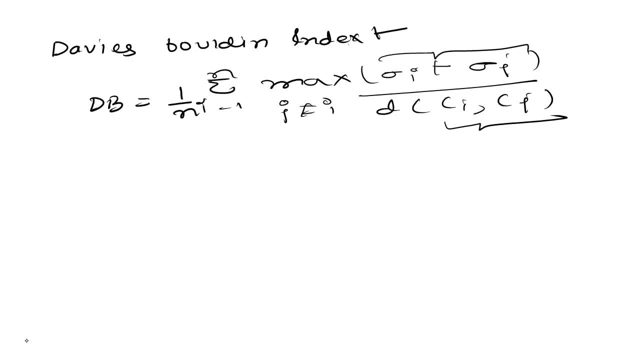 information about what is this. you can refer to and do a Wikipedia page. okay, there is a more derivation etc has been already done over there. okay, so that's the Davis-Baldin index, but most of most probably this: this: this the done index used properly in the country in the whole, except for evaluation of your of. 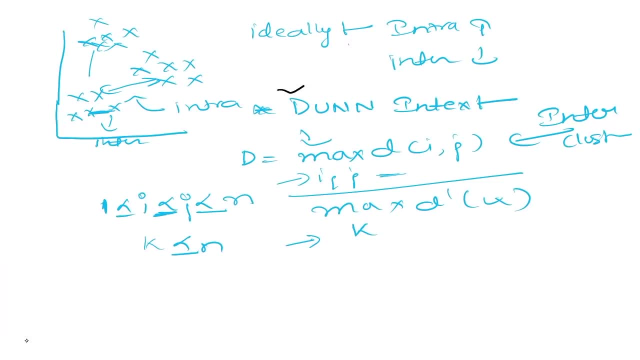 your model, so let me highlight it. this one. okay, so we have seen the Davis-Baldin index. now it's time for learning a little bit more in depth about what the, what, the approval means, what actually. the definitions of what was the definition of your favorite? 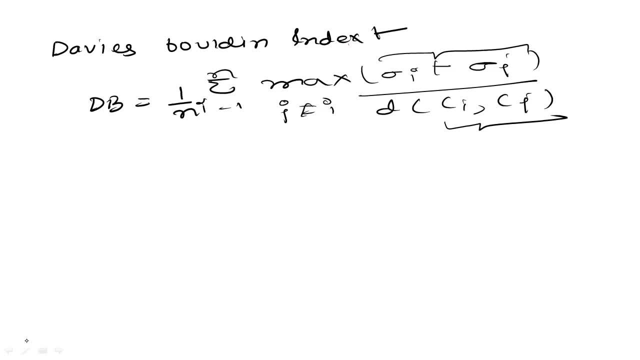 clustering, okay. so one line definition I could tell about clustering is in clustering you have and it's a, it's a grouping. can I write it? yeah, it's, it's better to write it. okay, it's better. better with me, our organ ride with me also. so a clustering is simply grouping, grouping. 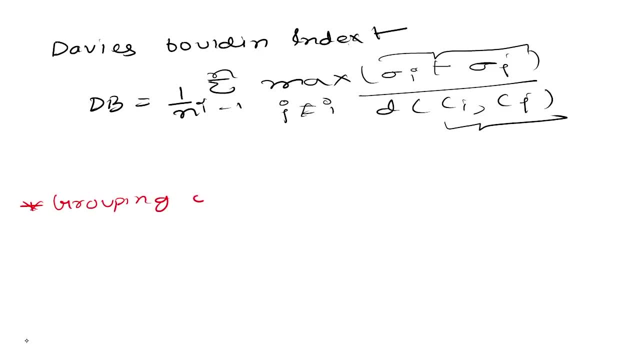 of objects, grouping of objects or elements, objects such that in such a way, I could say, in such a way, such a way, such such a way, our, our, our object, our object in a should be, should be similar, similar to each, to the, to each group, where it is in each group. 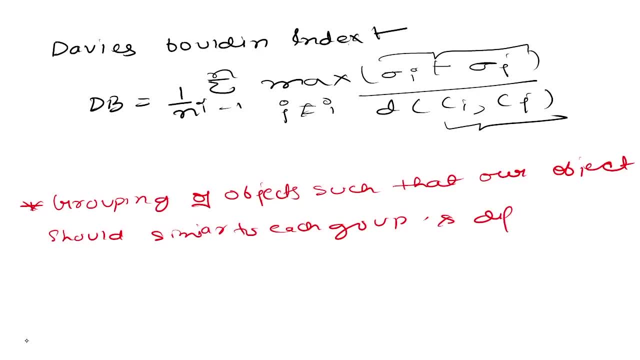 and differ from another cluster, cluster, differ from another cluster. okay, so that's the basic definition, basic definition of clustering and a very good definition. and from clustering in clustering we have two cases: intra-cluster and inter-cluster. where we want our, intra-cluster is the measure of distance between, just a distance within the cluster, and inter-cluster is difference. 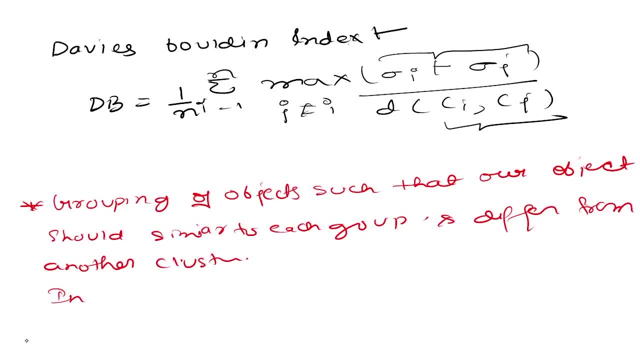 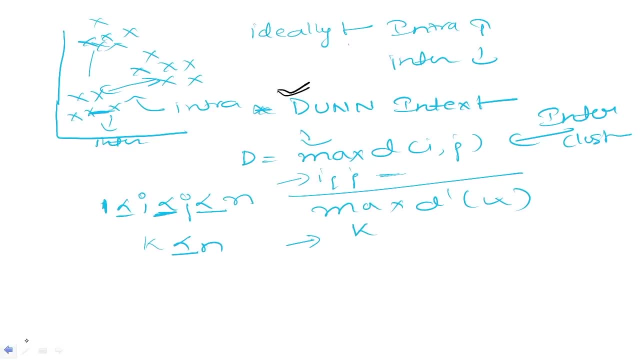 between across all the clusters. okay, so this is the basic definition of a clustering and i hope that you understood everything. okay, so now we have seen done index, we have seen clustering. now it's time for learning about getting into depth of clustering is about types of clustering. 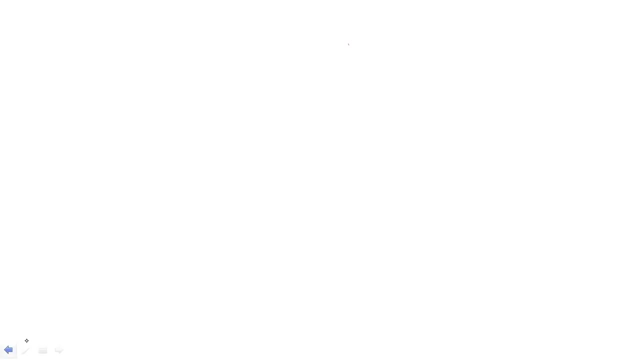 how many types of clustering we get in our life. and then we will, just after talking about types of clustering, we will end this subsection and in the next section we'll be talking about one algorithm, which is k-means, and the next subsection we'll be talking about a hierarchical 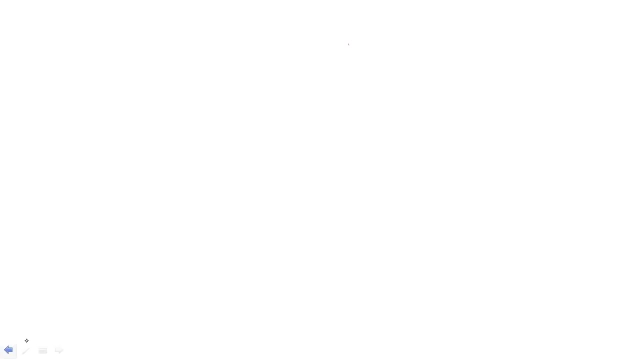 clustering which is agglomerative and divisive clustering. okay so, but before that, let's let's see some of the types of clustering. okay so, the types of clustering, which includes the types, the types of clustering. let me choose a it the color. so some some of the types of clustering are. first, one is partitional based. 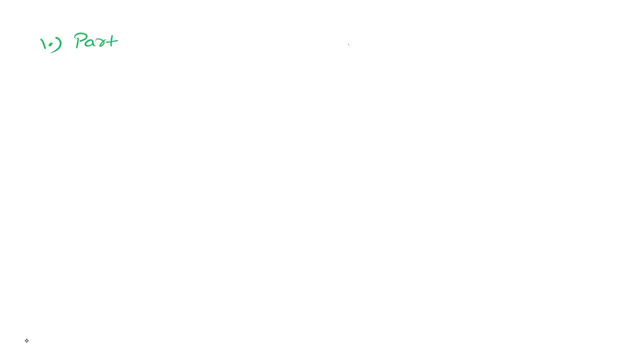 clustering, partitional- i'm just writing in short: partitional, partitional based approach or clustering. okay, so what is partitional based clustering? so assume, assume that you have this, that that you have this x and y plane and you have this data point like this and you have this data. 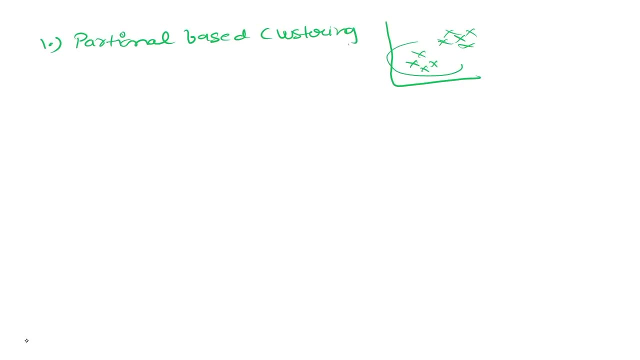 point like this: okay, so what do you will do? you will partition it. you will partition it into two clusters and you are done. okay, so here we have one algorithm, which is called k-means algorithm, that we'll study in our next subsection. okay, for in a partitional based approach. then we have hierarchical clustering: hierarchical. 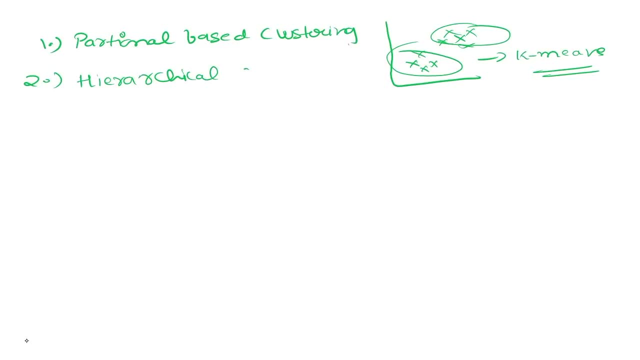 hierarchical clustering, clustering. okay. so in these types of hierarchical clustering we have like a dendogram. if you have seen a dendogram, then you know about a hierarchical clustering just just just as a just, if you know. so let's assume that you have this data point like this: you have this data point, let me do it here that you have this. 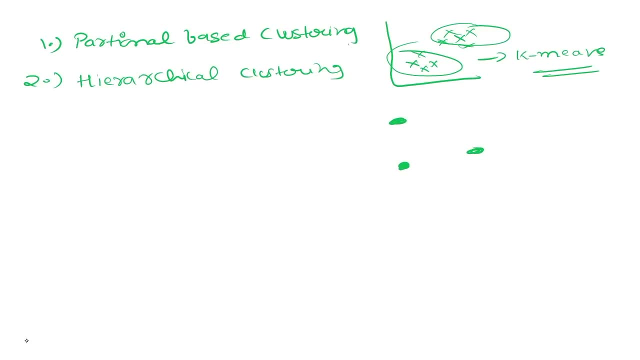 here like this: okay, so you have this four points, we have this four points, and again you have P 1, P 2, P 3, P 4 and, if you're plotted, the points looks like this: so these two, this P 1 and P 2, looks. 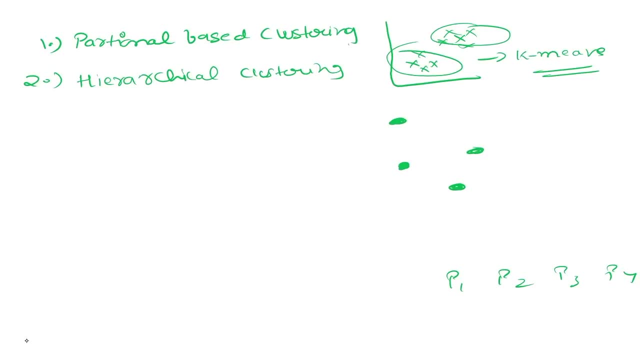 close this P 1 and P 2 periods, this p2 and p3? just just assume that this is a p2 and p3. this, this, this looks close, so you just cluster it out. okay, so the p2. so what you do? you just make a dendrogram, just like this. 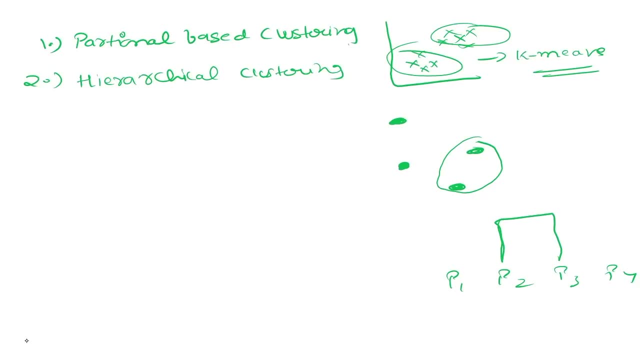 that p2 and p3 are now a cluster, which is the same, which which we can consider p2, union, p3. okay, now, these are the two clusters. now, if you see the closest structure, is this a p4. so what you will do? you will again make a nested cluster. now. now this: this will look like: 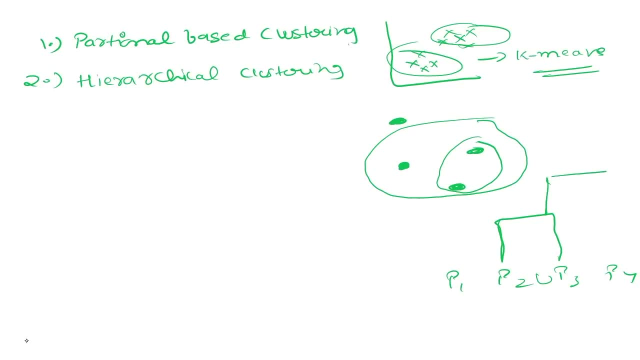 this. and now what you will do. you will attach p4 over here, pp4 as a dendrogram, okay, and then what you do then here is this: this is the p1 is the closest. then you cover it and then this hole and this hole. now, after that, you will be ended up being a dendrogram. you will be able to see a. 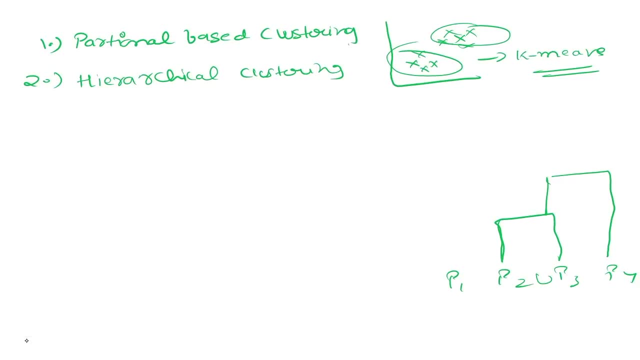 dendrogram which you can see over here, so here, after, which is p1, like this: okay, now you can see, now we cannot. we have a large cluster, which we have a large cluster. now we are done this, this, this is called the traditional dendrogram, because you can see. 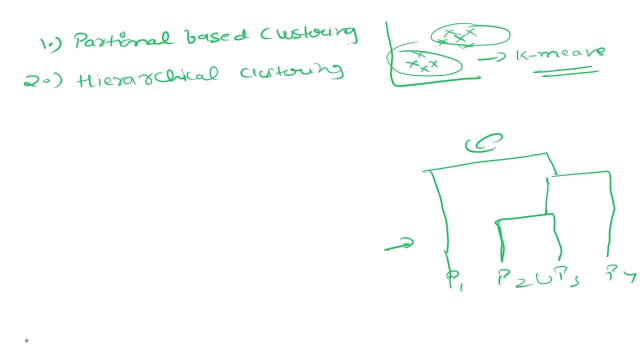 on internet about this. so what we have seen so far we have we have agglomerative structure. we are going up means we are just. we are going up like this means we have this p1, p2, p3, p4, we are we. these are own clusters by themselves and first these are their own clusters. we have four clusters over here. 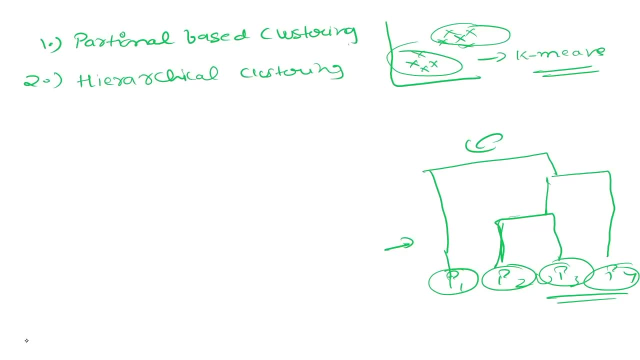 we have four clusters now. we cluster this p2 and p3, then we cluster cluster p3 and p4 because they are close to each other. then we construct p1 to p4. okay, so now we got our full dendrogram. okay, so that's. that is usually agglomerative, agglomerative cluster. we have something called. 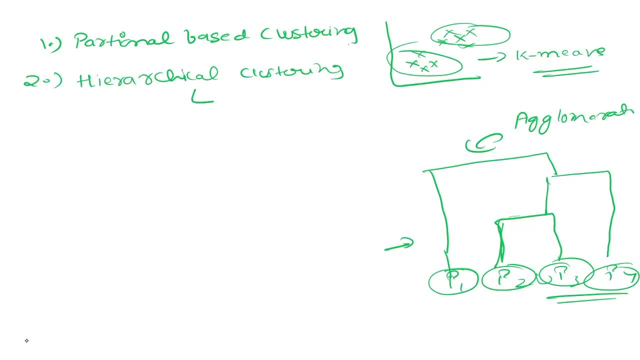 as divisive. we are in divisive and i'm talking about in hierarchical clustering, application uh, which is agglomerative and type divisive and divisive. we have given p1, uh, p2, p2, we have something called as p3. let's, let's assume that that, that we have a, b, c, d, okay. 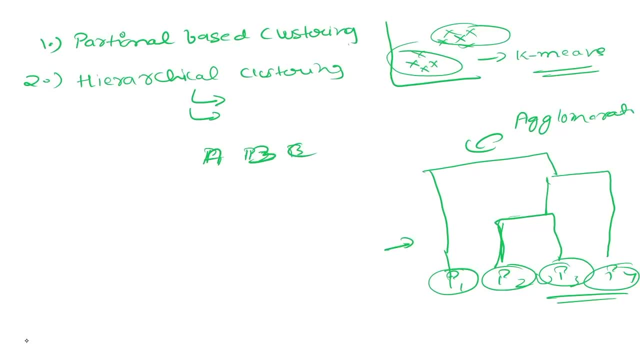 so a, it's just, it will match. if i do that, a, b, c, d, okay, so e, let's assume e also. so you divide this, okay. so what, what? what you do you? simply you divi visit, okay, like this: uh, first you divide this here, you divide a and b, a b as one cluster, then you divide c d e, then you have c d e, okay, then you. 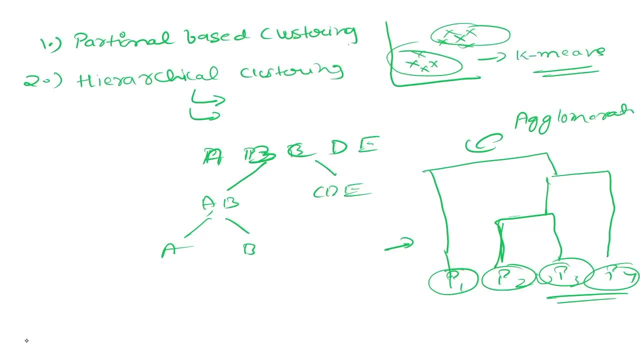 divide a and b into different, different cluster. so you have this whole dendrogram like structure, like this. now you are, now you are. this is just opposite of agglomerative. we are just here. we are making up here. we are making up here. we are making a different, different cluster. okay, now we 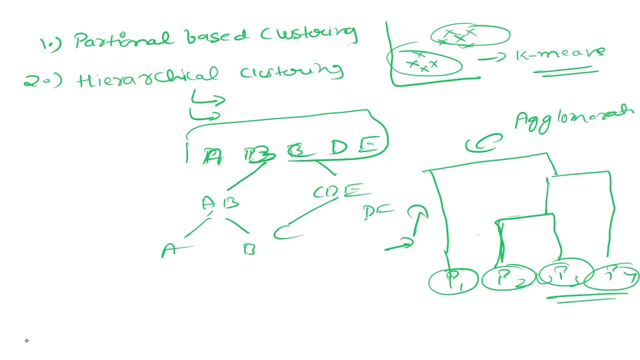 divide our c. then we have a, d, e. now we divide our d and e. now this is our divisive. okay, so we divide our whole cluster into different, different groups which are most closest to each other. okay, we will study in detail about this uh in in our uh next subsection, where we will talking about 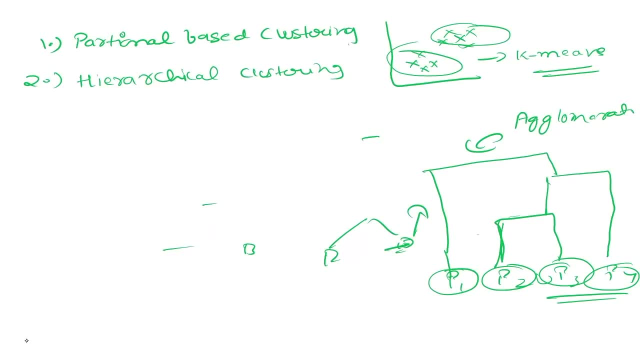 hierarchical clustering. okay, after that we have something known as. after that we have something known as well separated clusters. where it is well separated clusters, okay, just just i'm writing. it's well separated means we, you can easily, your model can easily- uh, separate well separated, well separated. then you have the fourth one, which is center based. 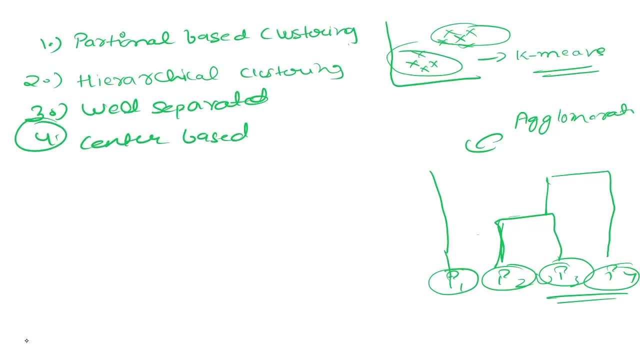 which is also k-minus clustering. is this center based algorithm? okay. continuity based, we have something called as nearest neighbors- k nearest neighbors- okay then. then we have density based, which is often known as db scan, which is often known as db scan. okay, which which you have? you will get in problem set to learn about this. 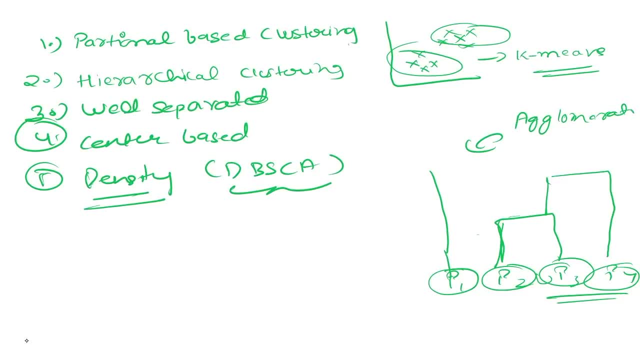 uh, db scan. okay, great. so we have seen a lot about clustering and i hope that you really enjoyed this session, this sub, sub subsection of clustering, and from the next section we'll be talking about lord's algorithm or k-minus clustering. but i will definitely try to complete in no time so that you can- you could get a more, more, a prone uh. 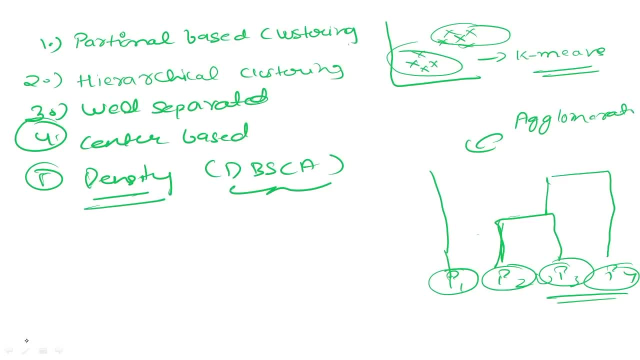 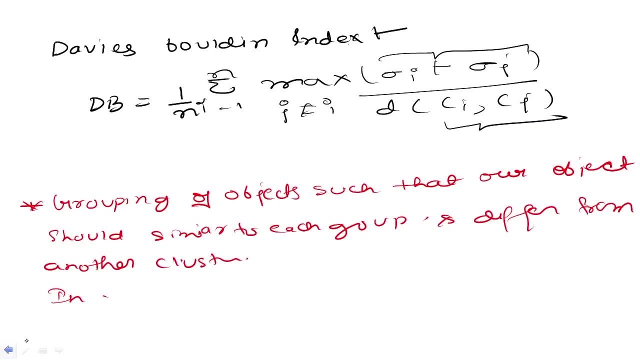 knowledge of clustering and uh able to make a unsurpassed learning models. okay, so let's see. so let's see, uh, as uh just re-recaptulate what, what you have seen so far, uh, we have seen what is clustering. clustering is just a grouping of similar objects in such a way that these objects 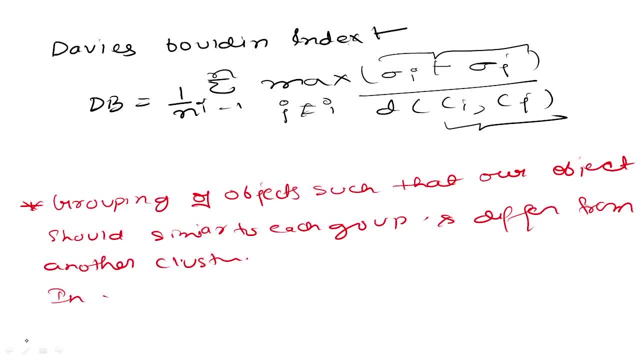 are similar to each other within the cluster or our inter-cluster, our inter-inter-cluster should be different, should be maximum and our intra-cluster should be small. what is the difference between inter, inter and intra? and inter? we have uh- the distance between uh across all the clusters, and that's why we need a maximum- and we have intra in which our points. 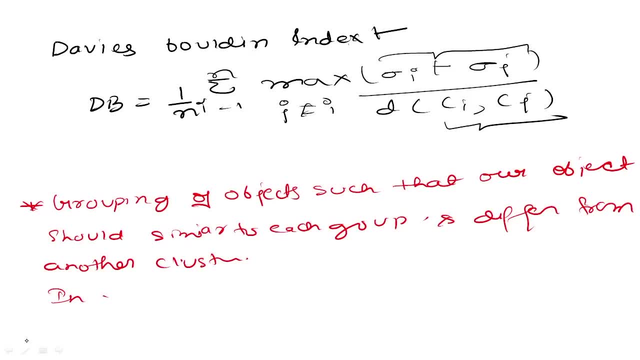 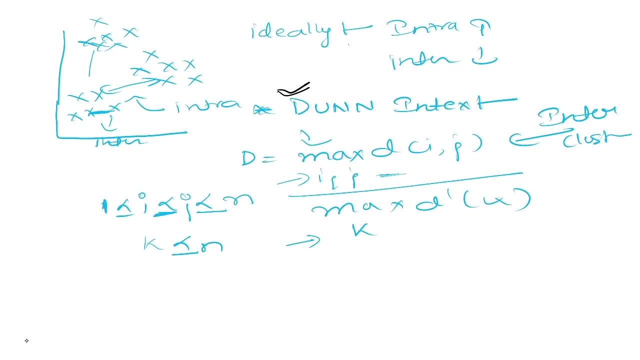 our points within the cluster should be minimum. okay means more similar, okay, other than the other clusters, okay. so that's, that's the, that's the basic intuition about this and, uh, clustering. then we have seen how we can evaluate. so i have talked about one index, which one evaluation index, which is a done index, okay, and done index it is used to. 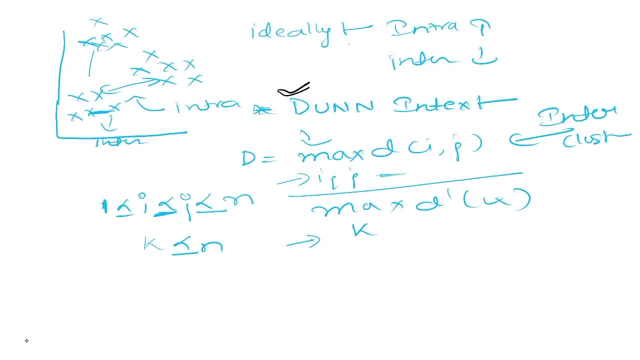 uh, take out the evaluate you. it is used to evaluate your clustering model. and what is what? what is what it does he? it takes out the maximum. what is the maximum inter cluster? what is the maximum to evaluate the performance? uh, between between two points, and it takes out the maximum. 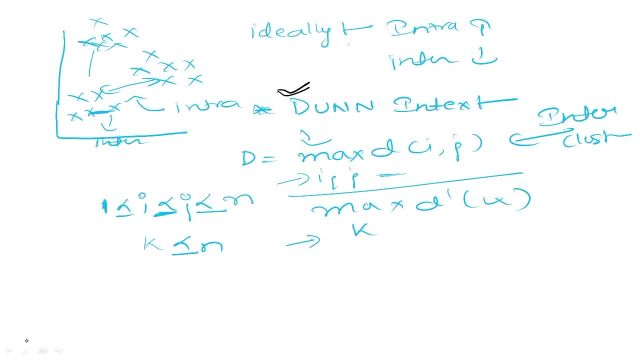 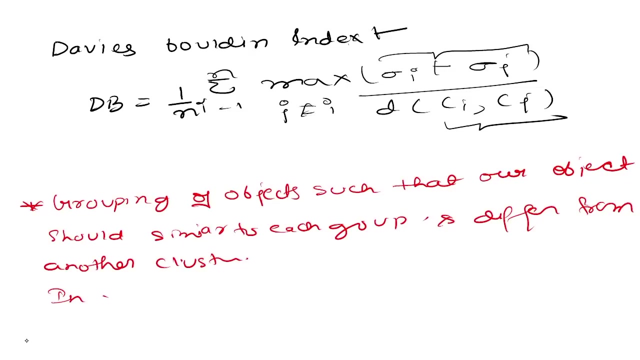 of the, uh, this, the. the denominator is uh- intra-cluster and um a numerator. sorry, yeah, the denominator is intra-clusters, is the numerator is intra-cluster and the denominator is inter-cluster. okay, and then we have something called as davis bounding, balding, block and index. this is just uh. it will take a lot of time to teach this, but it's out of. 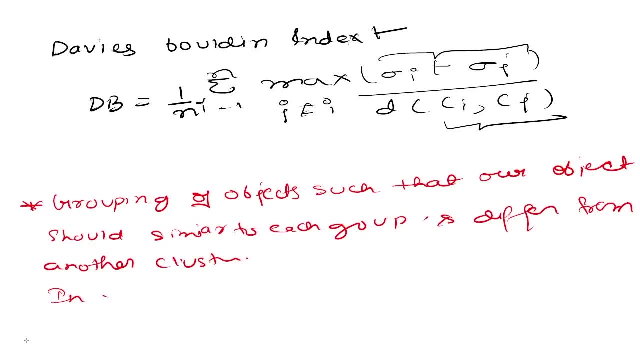 the boundary course, but it's just here, and is the number of clusters where we have a sigma i plus six sigma g and where i is not equals to g. we want the maximum and then we are taking out the distance between two clusters and then we are dividing it up. 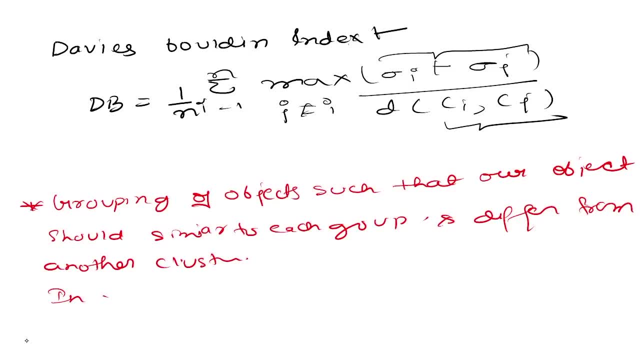 okay, so that's why and that's what the full uh clustering base models is now. i hope that you understood about clustering uh. now it's time. now. now it's time for learning about now, now. now it's time to learn about something new, which is in sub section where we will talk about. 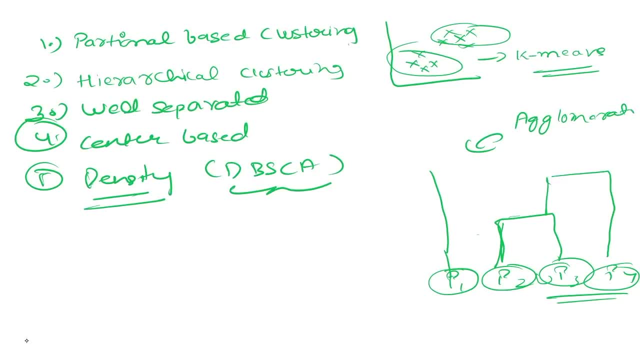 uh, where we have talked about four, five types of clustering, which is partitional based, hierarchical clustering and well separated and center based and db scan. okay, so we will talk about partitional. hierarchical and well separated is also, and center based, where you your prop problem set will be on db scan, okay, so here we are done with this. 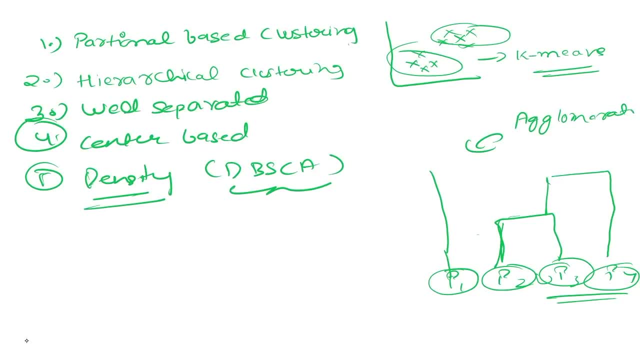 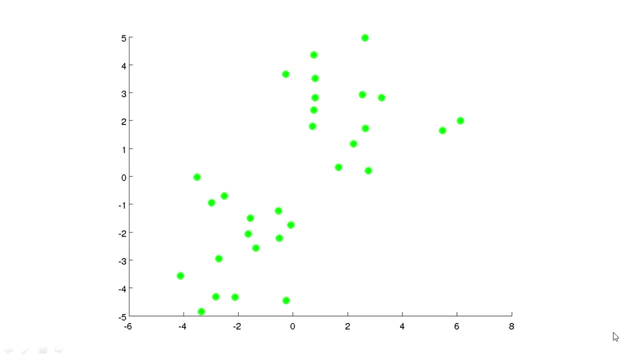 sub section. now, in the next section, we'll be start talking about k means. till then, have a good day, okay, so now we have talked about various things like clustering. we have given a part one in sub section. i've given you unsupervised learning applications, and then we have talked about various applications of unsupervised learning. 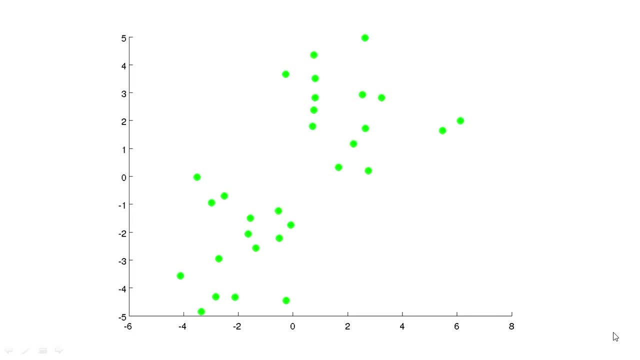 and then i've just given you an overview of clustering in this first subsection and the next subsection i've given you the intuition behind clustering, i've given a formal definition of a clustering. we have talked about inter cluster, intra cluster. we have talked about the evaluation matrix, like ton index, devious volume index, and i've made you understand each. 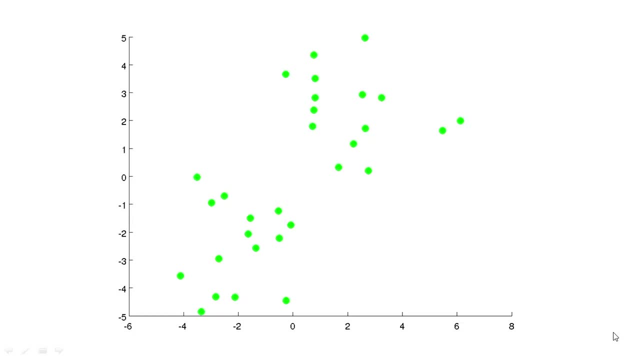 and every equations and i've also helped you to understand what are the types of of clustering which are available, like partitional based, hierarchical clustering. then you have a center based, world separated, density based, continuity based. okay, so we have this kind of clustering which are already available. now we will talk about a partitional and center center based. 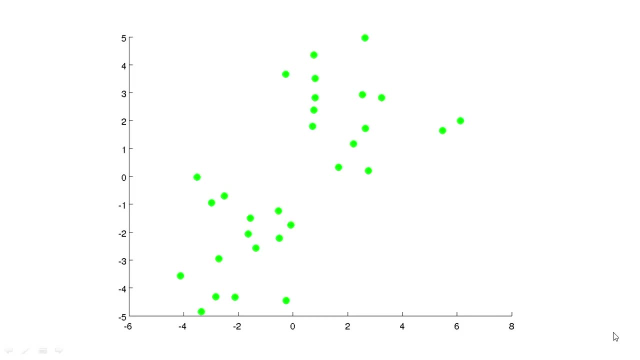 clustering, which is k, means algorithm, as this example was taken from andrew nong course of machine learning, but he has uh, but it's too much uh. j is seven years old, but i have. i have made it very, very updated for 2020, just that that this. 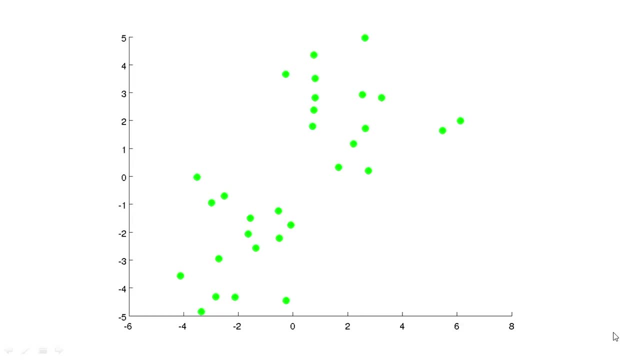 example is from andrew nong. okay, so i i have also included k means plus plus algorithm, what the k means plus plus algorithm does and some of the variations of k means. and then also i have talked about in detail what are the, what are the delimitations of k means, clustering what 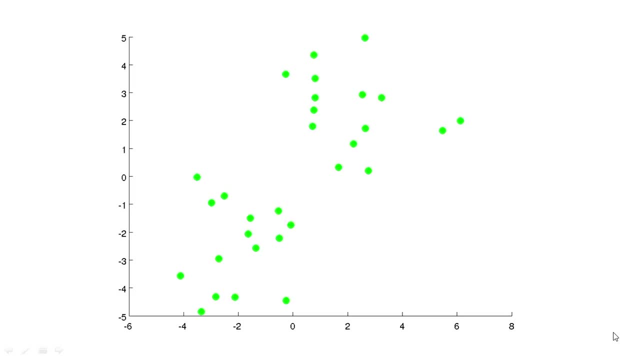 how we initialize the centroids, what are the time complexity of k means clustering. okay. so then we have talked about the full machine, full k-means clustering algorithm. how we evaluate our k-means clustering algorithm. okay, with the euclidean distance. so that's what we are going to start talk about. just be sure to just sit sit somewhere and see and take copy and 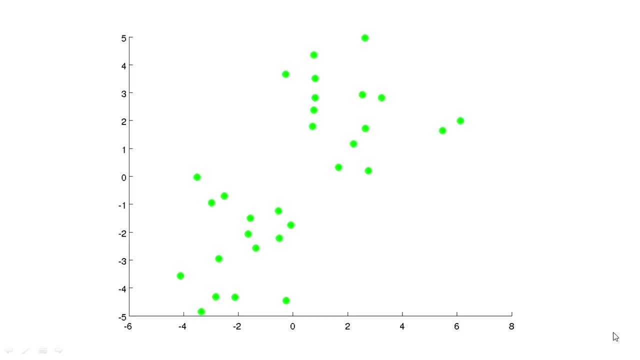 pen to understand. okay, but before that, what we are going to study is k-means clustering algorithm. sometimes, since the synonym of k-means clustering is lloyd's algorithm, it's something sometimes called lloyd's. it's sometimes called lloyd's algorithm, lloyd's algorithm. okay, so it's maybe. 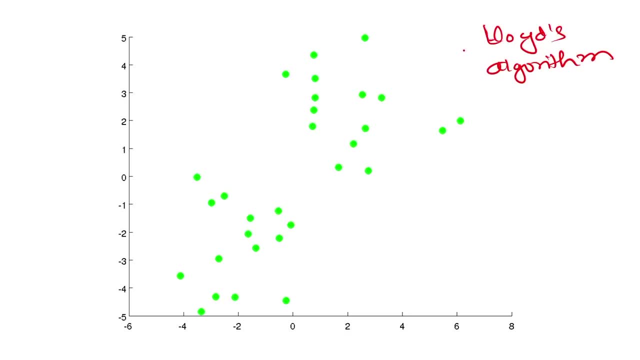 some people pronounce it as a lots algorithm or a k-means clustering algorithm. okay, but i like to pronounce with k means okay. so, uh, just just as an example, we have this data set. we have this data set over here. now, what? what we do when clustering? 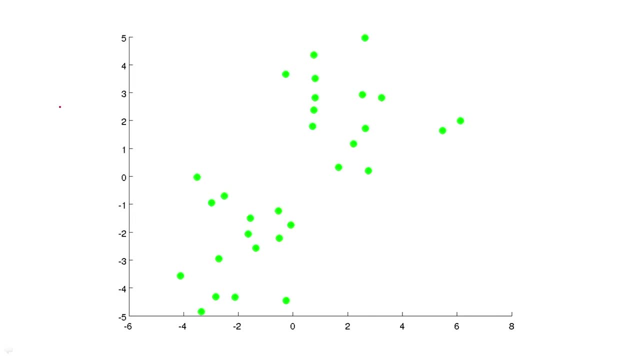 what we do in clustering: we initialize centroid, which is k. okay, we initialize centroid, which is denoted by k. so here what? it is a hyper parameter. so, what we are going to do, we are going to initialize k, we are going to initialize k, as we are going to initialize k, which is two. 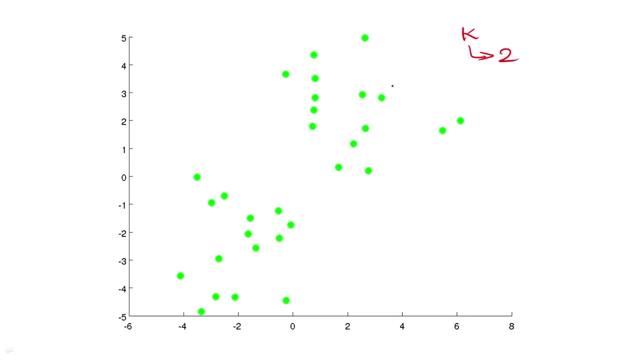 two centriodes and Centroids is just the initial. you will get to know with the visualization. So what you do, you initialize with two points onto this. So here you initialize two points like this: The first point is over here, The first point is over here And the second point is over here, And these are called the centroids. You will get to know why we call it as a centroids, But these are called the centroids. Okay, these are called the centroids And here in this example, 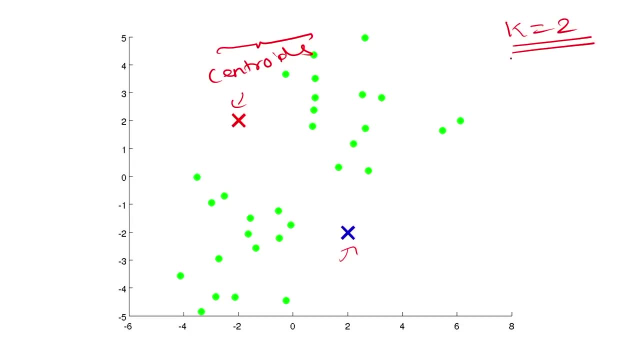 k is equals to two because we have taken k equals to two because, as we have a, two centroids and we randomly initialize these centroids. Okay, so we'll see the initialization. just after some PPTs, This has some slides. Okay, so you initialize your model now, And now- this is the first iteration, Now, in the first and first, to initialize. then what you do. you do the assignment step. What do I mean by assignment step? First you initialize. 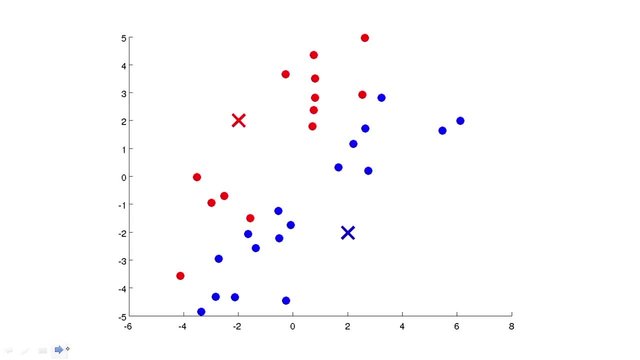 then what do you do? you do assignment step like this: you assign all the all. the particular value means red to red color and blue to blue color. you can see over here that we have that we have done red to all the red color which are closest to this center and centroid And this blue we have covered, that is, all the centroids which are closest to that blue. Okay now what? what we will do? we will take out the average of these points. we will take out the average of these whole blue points. 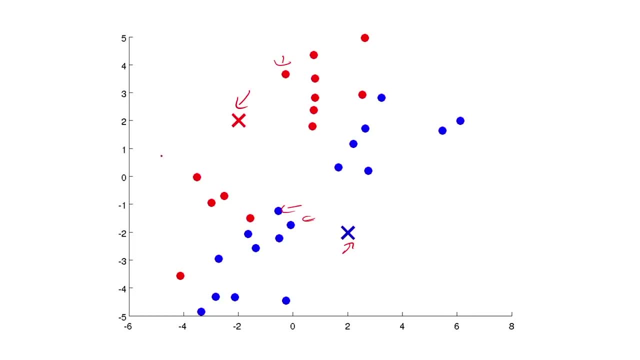 And then we will take out the average of this red points, And then what, and then what we will do. we will average it. we will average it like this: We will average it now. after averaging, We will make that percent right to at average, and then what we will do again. 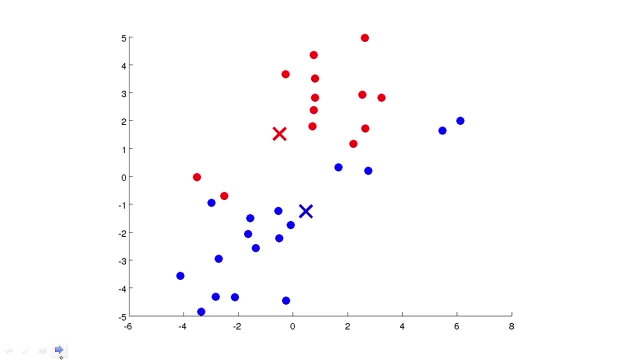 We take out the again, We do the assignment step like this: We just assign, we just update our values, which are so closest to this sense, and right now You can see that the blue becomes like this: now, Then what? and then what we will do? we will again move the centroid again. 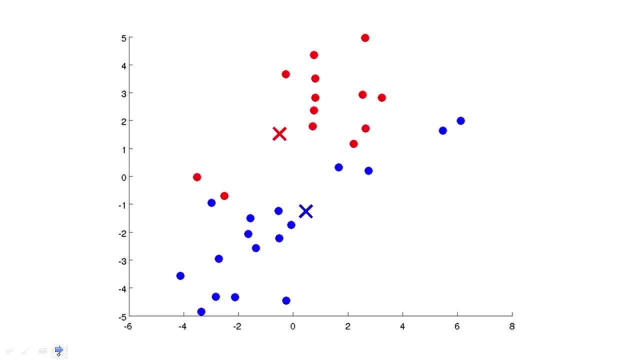 We will take, take out the average and move the centroid. like this: We will move, move the sand centroid and then we will make this red. red means who, those, those are closest to Blue, blue and these are two red. Okay, Then again you do, then again you do, like this as a taking of the average and making the color as blue and red. 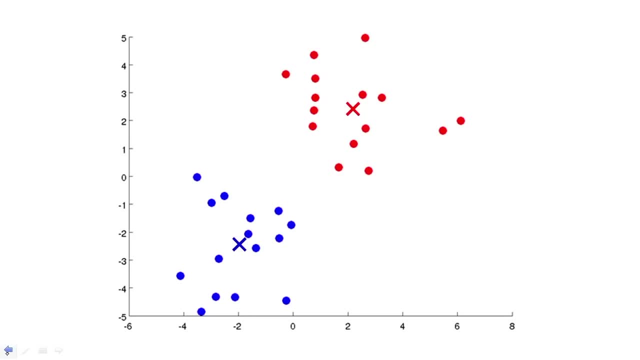 Okay, now you can see that you would that to what you have done. You have a very good Plus. I mean you have initialized here and then you taken out the average, then you move to that centroid and again you update the Updated cluster and then again you move that like that. Okay, so we have done like that. 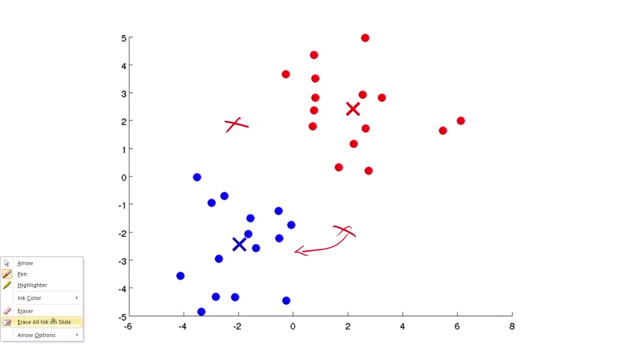 And I have just shown you a very good visualizations of this came in. So let's see again in a little bit more fundamental way. Okay, so here is our data and then you can see the data is looks like this. So here, what we had done, we had in the, we had simply 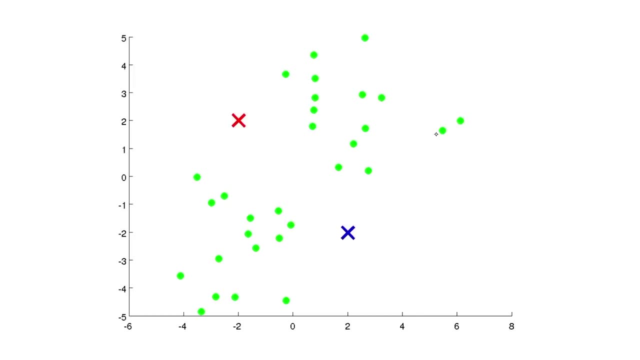 initialized two centroids like this. and then what we have done: we have a. we had just make the Make the points which are closer to that blue to blue and red to that red. Okay, you can see over here then what, what we have done. We had taken out the average and then we moved our centroid to that average. 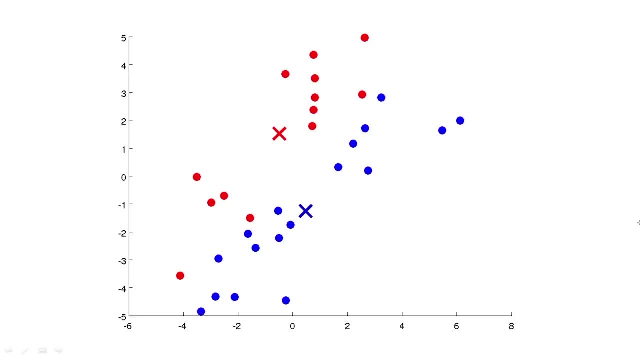 Okay, and how we take out? you do you all know How do we take out the average. you just take out the number of observations and then divide, or some the number, the sum over the observation, divided with a freak frequency over the Observation. you just do that and then you update in and then you again make the whole. 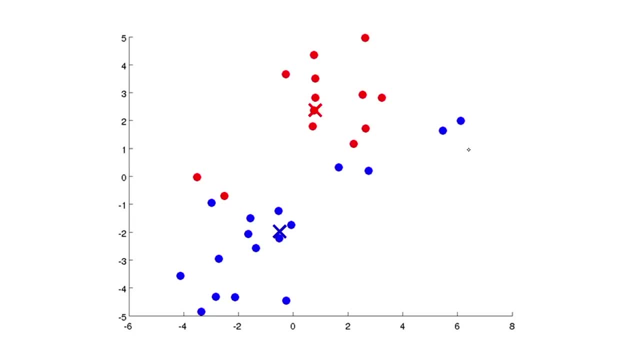 Assignment step. and then what you do. then you again up the make and take out the average. now you again update The points you can see like this: and then you again take the average. you again make the point says like this: Okay, and after, until and unless your centroids are not changing, you keep doing this. Okay, so here is an informal algorithm. 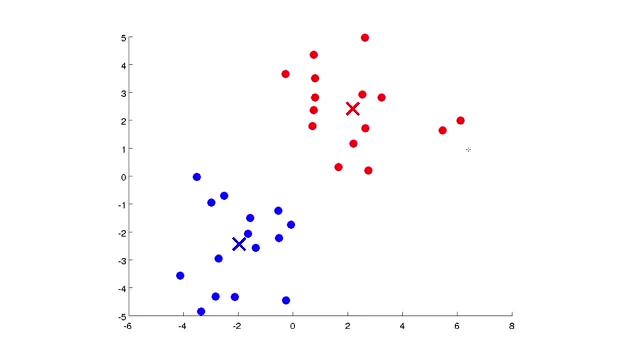 Here is an informal algorithm and you can see over here: after seven, It is not changing. So we converged, we, our algorithm is converged. Okay, so this is how whole k-means clustering algorithm works in Visualization. so let's see the algorithm in detail. Okay, so what you do? first of all, here's an algorithm. 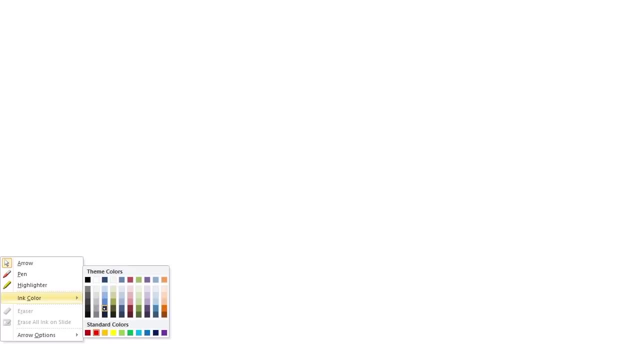 I'm writing, just bear with me, but just bear with my handwriting. So I'm just writing an algorithm. So here is my algorithm with the reds, right it with a red color. So Let let me write: here is your algorithm, algorithm, Algorithm. okay, so you do for key centroids, case for centroids. 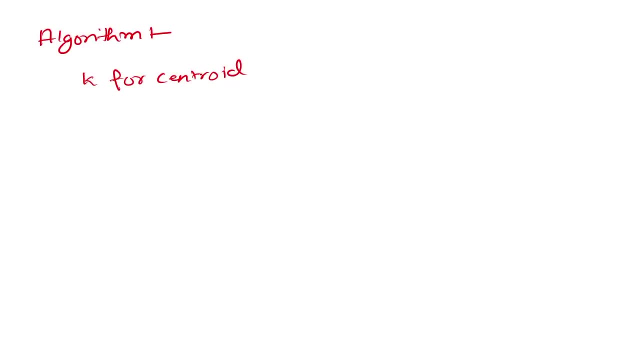 Okay, so you have to choose key. Okay, you have to choose key. which is key? There is a hyper parameter. Okay, then you repeat this to process, then you repeat this to process. The first process is cluster assignment, Cluster assignment. you assign all the clusters, you assign all the cluster, you assign all the cluster. 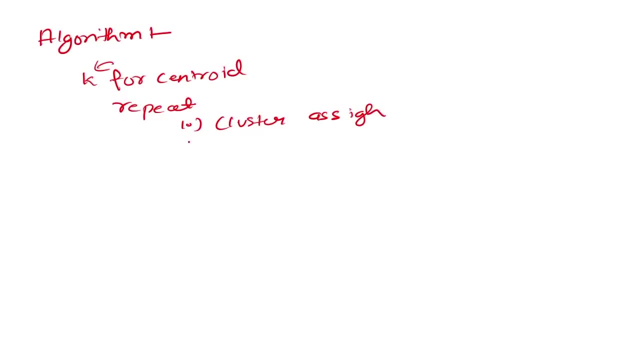 And then update tick, tick on average and then take out that cluster sign. You assign the clusters and then you take an average and then you make that point. So you went, then you do that updation of a cluster. Okay, then you up the compute, the centroids: 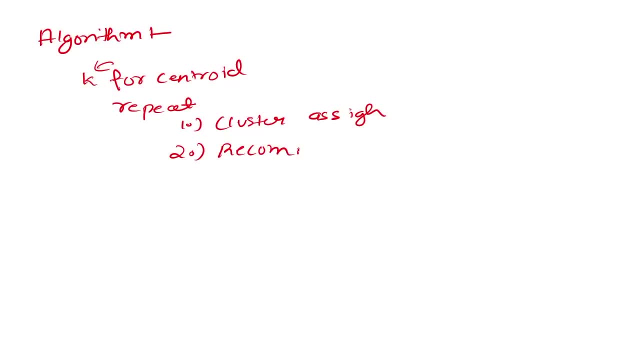 Okay, then you re-compute the centroid. okay, then you, how, you, how, you recompute the centroid, the Centroid, but simply means you make the, you take out the average and then you assign that cluster- Okay, that cluster two to two, the nearest data point. okay, again, you have to take out average until and. 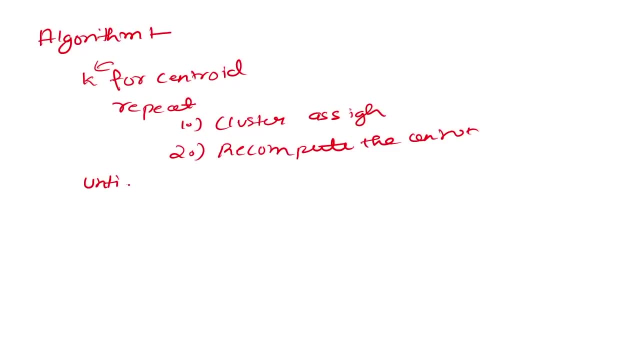 unless until you do, until you do, until your, your centroid are not changing, your centroid, your centroids, your centroids are not changing, are not changing. okay, where it's. it means that your algorithm is converged. now you don't need, okay, so you repeat these two process like clusters. cluster assignment means: 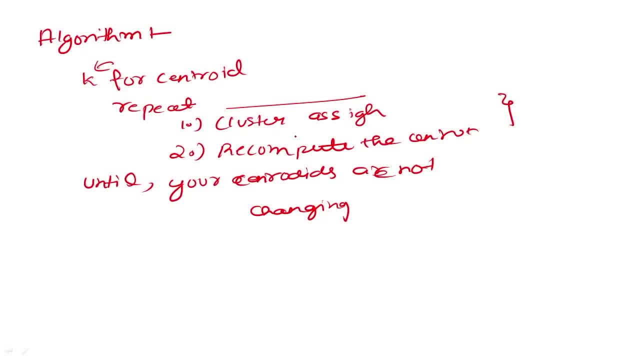 assign the cluster with blue or red, and then you update your centroid and take up by taking out the average, and then again doing doing this, taking out the average, again doing this, like that. okay, so this is the basic algorithm of K means clustering algorithm, and I hope that you understood about k-means, so let's under. 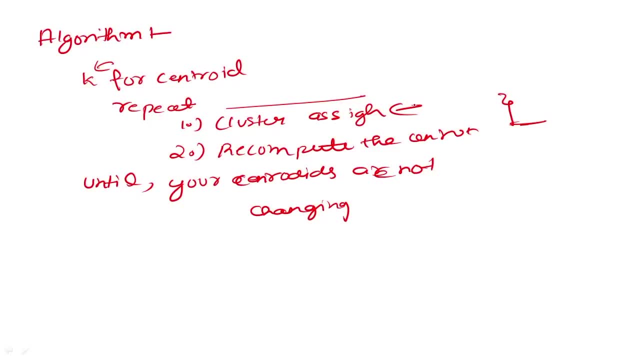 and let's understand a little bit more way is a little bit more further into just a recapitulation of k-means. k-means- clustering is an algorithm that also called the Lloyd's algorithm algorithm. then we what? what we do? so let's go back to our visualizations. okay, so here is our. 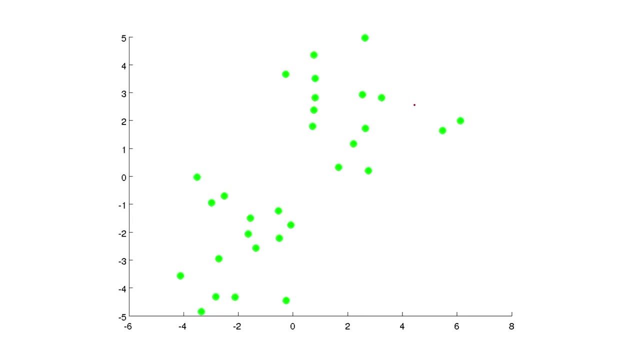 data and what? what we do is we randomly, we randomly initialize two centroids- okay, not every case, just just have taken, it is a hyper parameter. we have just taken two for this case. okay, then what you do? then you do the second step, which is, uh, which? first you do the cluster. 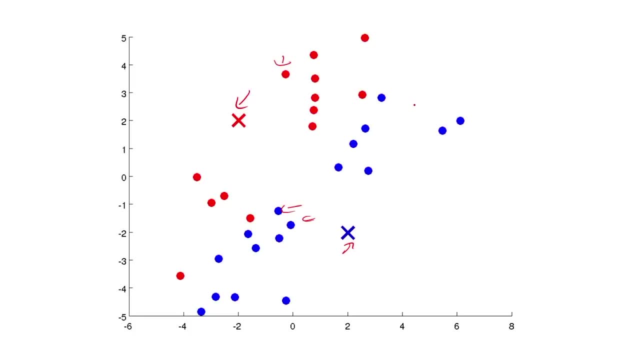 assignment. you assign all the cluster with the closest with the same points in into the cluster. then what you do? then you do this: recompute the centroid by taking out the average and moving the centroid. okay, then you do the cluster assignment. then you assign the cluster like this. then you: 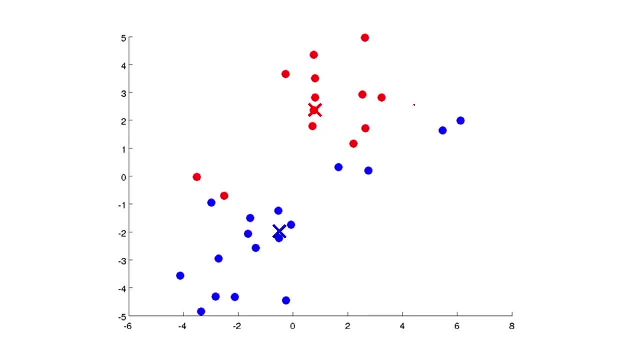 again, move the centroid. okay, recompute the centroid, then you assign the like, like that, and then you take out the average and again you, uh, again you do the same, you take out the average and then move your centroid. okay, now, now, in the next iteration, which is not changing, now your 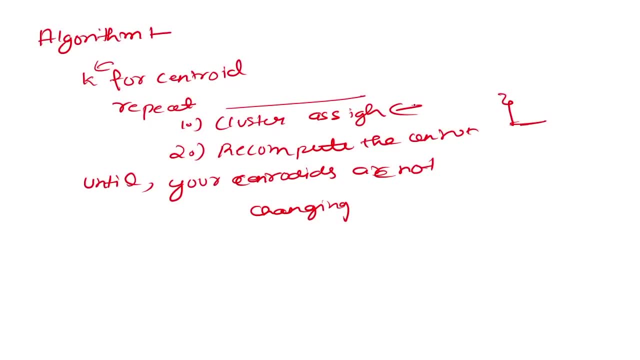 k-minus clustering is converged. now you are done. okay, so here's a good algorithm. you will be able to see on the internet. the same thing like: first you do you choose k, how many number of k clusters, then you assign the clusters, recompute and then, until and unless your centroids are not, are not, are not changing, okay, so this is whole about k-minus. 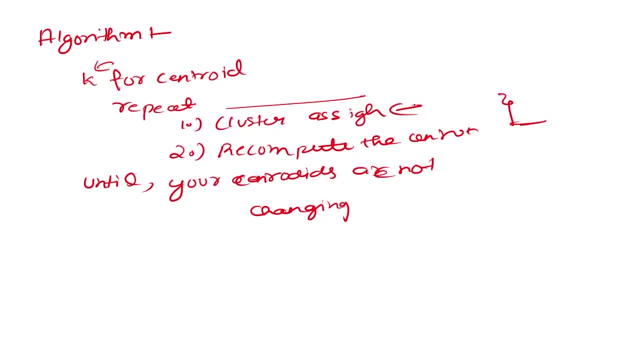 clustering algorithm and i really, really hope that you understood k-minus clustering algorithm. so now let's see some evaluation techniques of k-minus clustering algorithm. okay, evaluation technique: how do we evaluate our k-minus clustering algorithm? so for an example. so for an example. here is my example. so for for for an example: we are given, we are given. 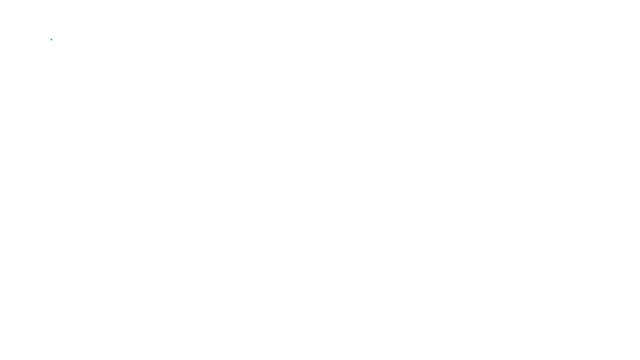 uh, no, not an foreign example, is just a, just just, i'm giving you the optimization objective, so you are given. so you are given x, d dimensional space, d dimensional space, as well as and the clusters which are this, uh, and set, i think the dictionary which is as, not, which is in. 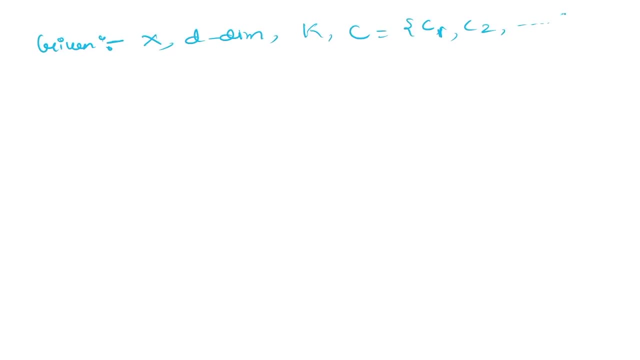 this c1, c2, all the way around to the ck. okay, we have k clusters. okay, then, what you do? you want your uh to optimize c. you want to minimize this cost function. you want to minimize this cost function. now, what you do? you take out i equals to one all the way around to the k, where, k, where. 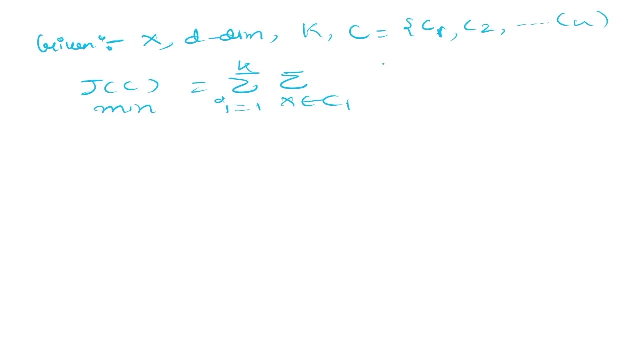 x be the member of c. i mean the cluster. now you take out the distance of x and c. okay, you want to minimize this cluster? okay, so, uh, just it, it will make sense, don't worry. here we have ci, which is equals to the centroid, so let's see. let's see what do, what do i mean with this? uh, distance between x and c. so what we are. 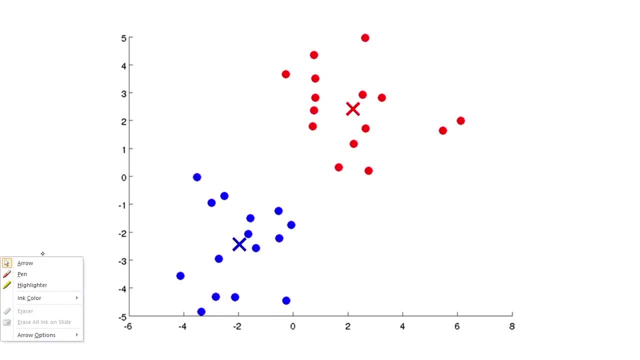 told that what? what we are told like: uh, we are. we are told that we have that, that we are given x, d dimensional space and we have clusters, which is c1, c2, all the way around to the ck, where we have cake clusters. now, what we have? then we have this equation: i equals to one all the way around to the. 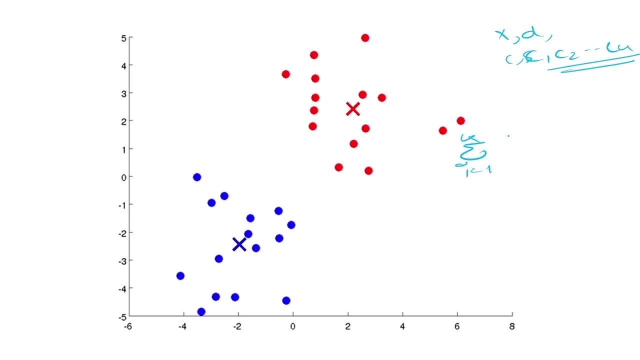 k. we are going to until every clusters where each, where each x, where each x is the member of cluster, means where this data point is the member of this cluster. okay, now you take out the distance between you, take out the distance between this data point cluster, this, this cluster. okay, and this should be. this should be minimized, your distance should be. 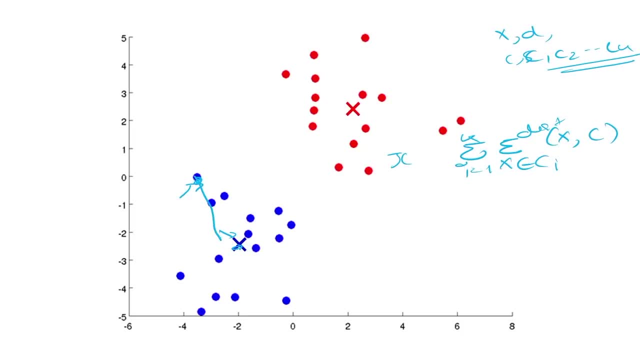 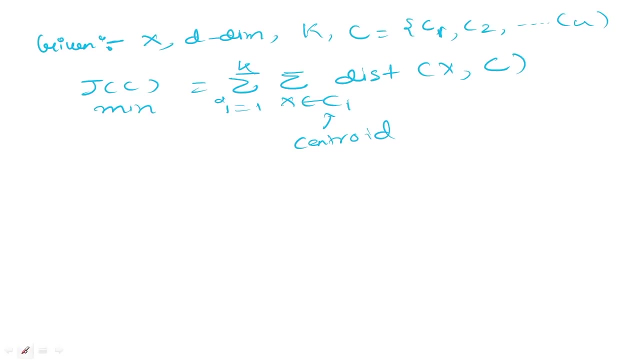 minimal. your distance should be minimal. as compared to this, your distance should be minimal. so that's what it is telling over here. okay, so i hope that you understood with the help of a visualization. okay, so ci is the centroid. okay, uh, cluster centroid. okay, so how do we take out? 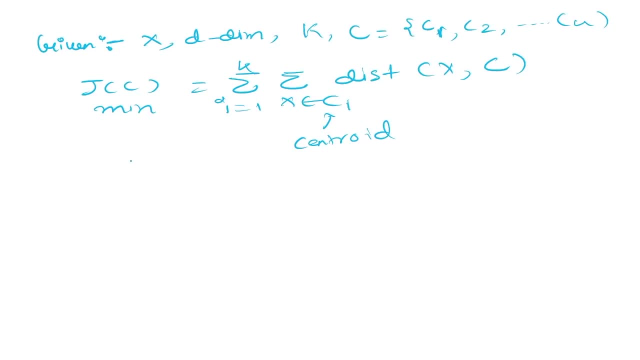 the distance for taking out the distance. we have something called this and you can take out the distance for taking out the distance for taking out the distance, we have something called you. there are a lot more distances which are already available. you can take a look at it online, but it's a very used euclidean distance. so what is euclidean distance? 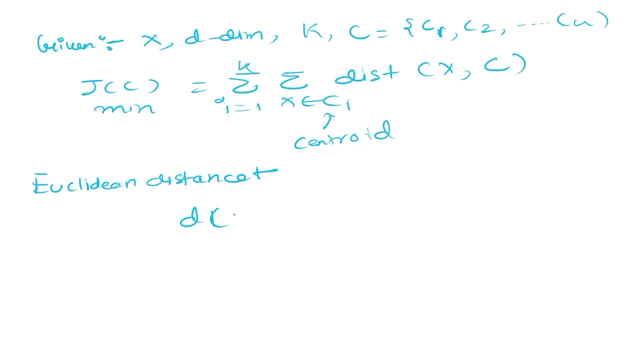 and euclidean distance. we have d. uh, we have two points, p and q. okay, since we are doing: for each and every point, i equals to one, all the way down to the n means number of training training. example: qi minus pi squared: okay, and it's taking out the square of the square root of that, okay. so this is the, this. 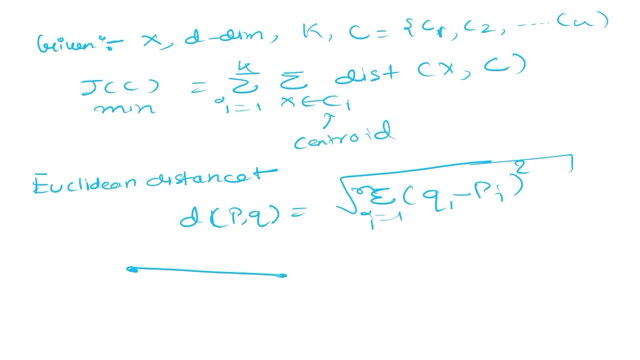 is the euclidean distance. that just measures the distance between two points, like this, and you can see some more about this onto the internet: how we derive this equation. what is this? well, who have found it? is that right, cetera, etc. okay, and sometimes, and this, this cost. function of k. 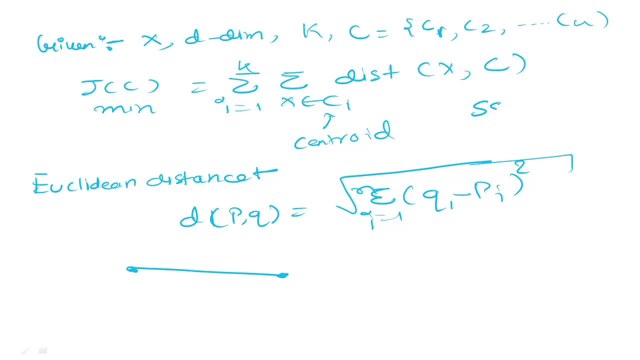 means close string is called, is called s. s. e means sum squared error, sum squared error. you can also see it is just like the done index following the inter and intra cluster. here we want to minimize our int, our intra cluster over. here we want to minimize our intra cluster, we. 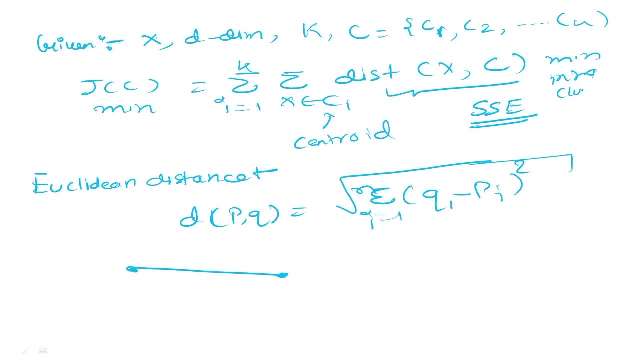 want to minimize our intra cluster. okay, so that's the basic definition and that's the whole thing about whole story about a k-means clustering algorithm, and i really hope that you understood k-means. and then we have talked about evaluation techniques for k-means and that's it for 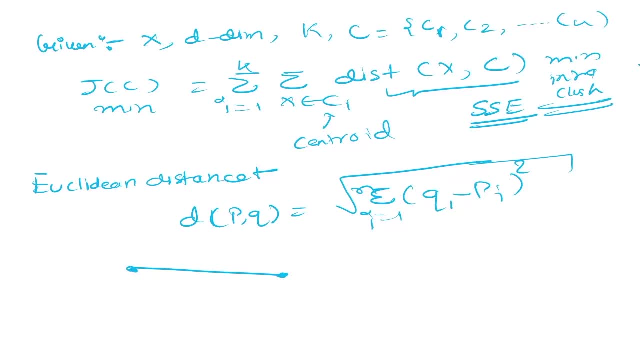 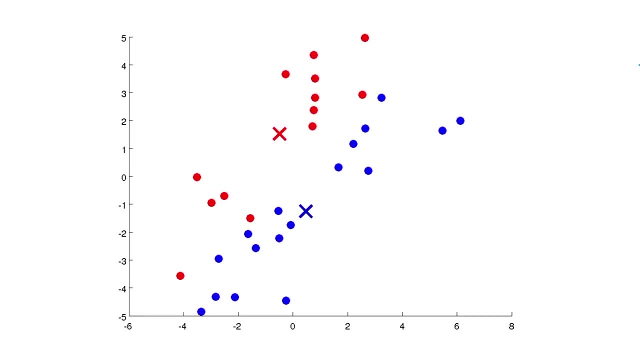 k-means. and now we will talk about why it matters. it's the basic definition of why it matters, with the random initialization as we have seen that we initialize our centroids. these centroids are randomly. you can see that we have initialized randomly. so why it matters, how it can cause the. 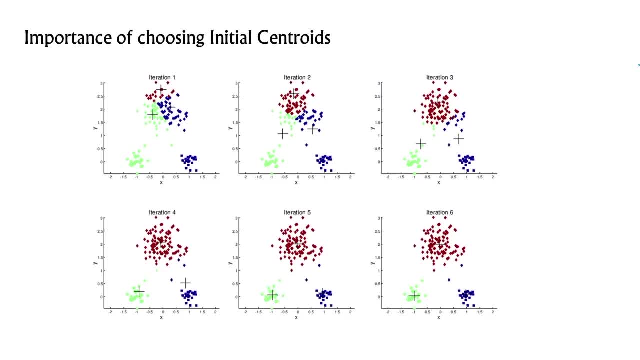 problem, it can cause the problem. so here we had just, we had just chosen here. you can see over here here, over here here, that we have: in iteration number one we have three centroids. iteration number two: we take another average compute, then we do the, we come, we, we simply what we have done, we cluster, we assign. 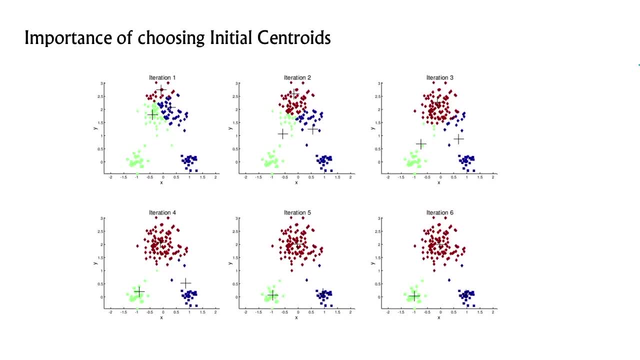 the cluster with the same centroid and then we recompute by taking out the average in the second iteration, then in a third iteration and the fourth iteration, the fifth iteration and the sixth iteration. you can see over here that how, uh, we? you can easily see that we have a good cluster over. 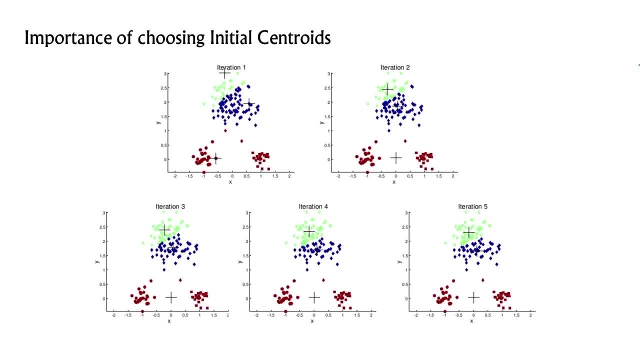 here, but you can see in here that you have you just hit. it can cause. how it can cause problem is into iteration about your engine. you have just randomly initialized. volume is 3. can see whole story changed. whole story changed. you can see over here. okay, so that's the big. 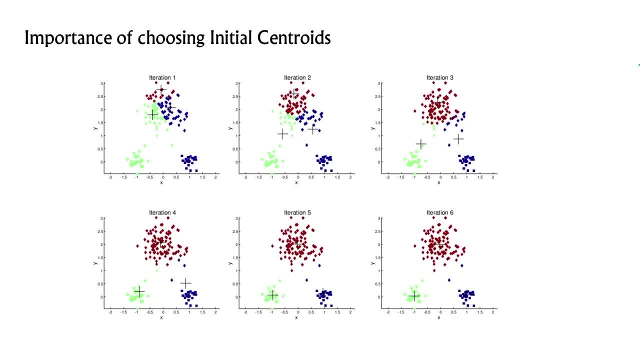 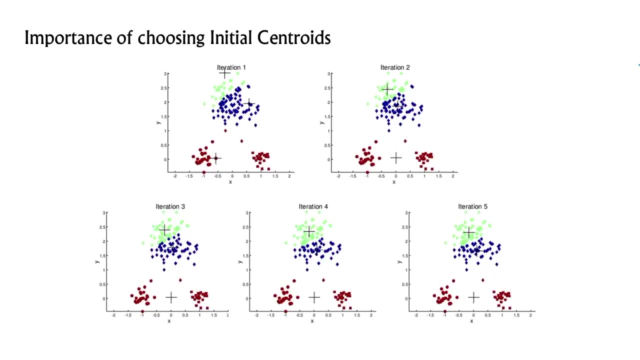 problem. so that's why we do, which is very not recommended to, to choose it randomly. so researchers discussed about it. the researchers had talked about it, how we can use it, how we can make something good. so we researchers found that k means plus plus, something called as k means plus plus algorithm works best. works best, uh, and which is which i'm, which i'm going to. 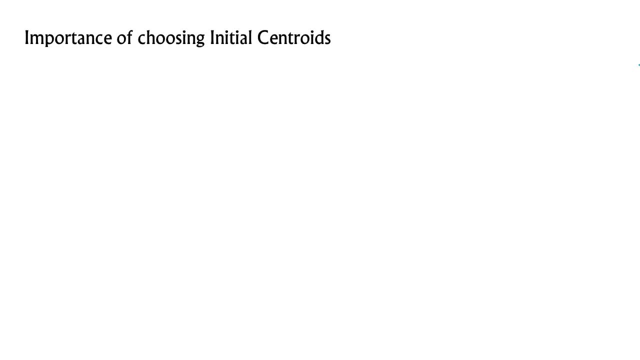 tell you, okay, so k means plus plus algorithm what it does. it simply select multiple numbers. it simply select multiple numbers, as in random we are, we are just taking any random, but it selects multiple numbers and select the smallest error. okay, so that's, that's what the k means, plus plus. 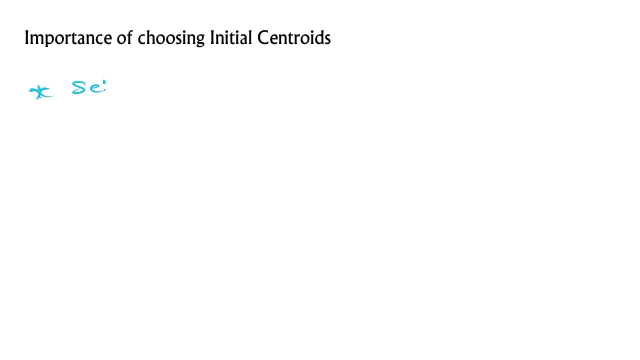 does it selects, selects multiple. multiple means it's just a, it's just a multiple. a sample from the numbers, multiple numbers, and checks and checks. which number? which number minimizes? which number minimizes? minimizes the sse, the sse, which is the which minimizes the into intra cluster distance. 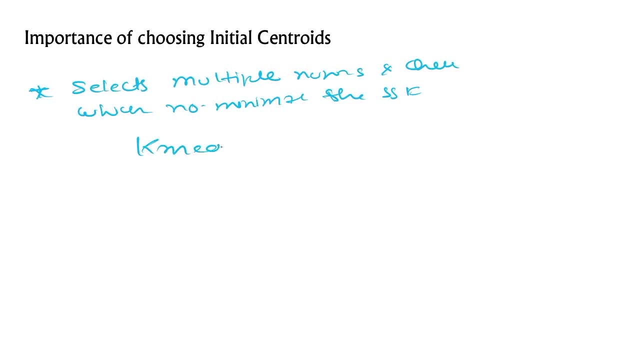 okay, so that's the k means plus, plus, and it is usually used in everywhere. okay, rather, rather than randomly. okay, so we have talked about uh why, why we choose importance, why we choose um over uh random, why we choose k means plus, plus over uh rand randomly, because 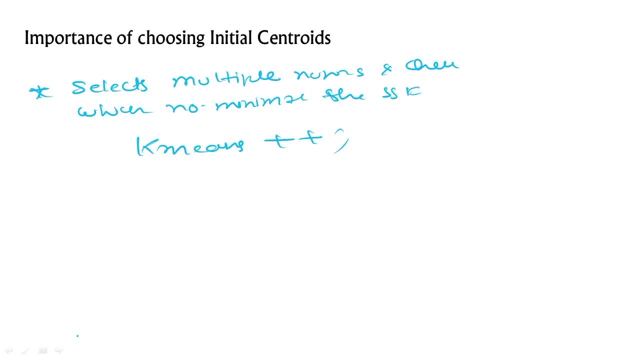 maybe it can happen sometimes. okay, a very good, a very cool god. if the luck is not with us, it can cause a big problem in further. okay, so how? how we have to deal with this kind of situations. for dealing with these kind of search situations, we have something called as kameez plus plus, which will help us to which, if it just selects. 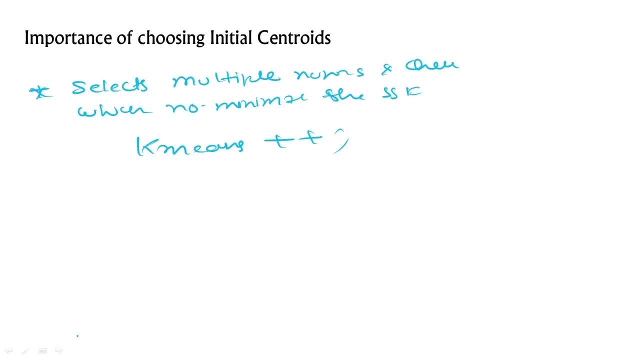 the multiple multipliers and selects. select the one, select the numbers which has a smallest error, okay, okay. so, uh, let's see, uh, you may, you may think, you may think, hey, i use, hey, i use. how do we select how many number of a centroid that we need? okay, so, that's the, that's, that's, that's also the best. 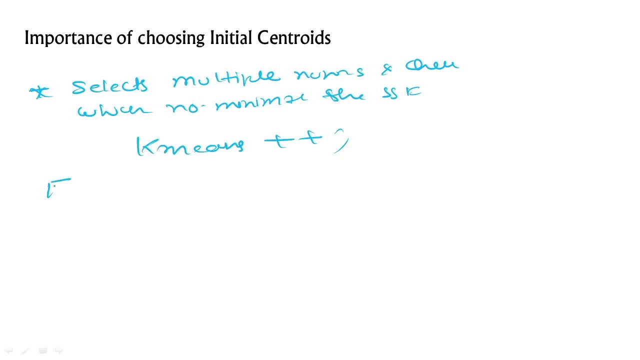 the big problem. so we have something called as elbow method. we have something called as elbow method, and what is does? we have elbow method like this: we have written the k clusters one, two, three, four, five, six. okay, now, and if you, if you have taken k equals to one, your error is high. two, uh. 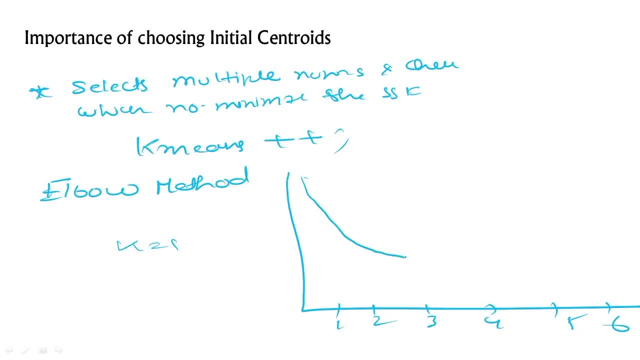 if you've taken a k equals to two, your error is going down like this: like an elbow, like an elbow, okay. so here you can see. the elbow turns around at three. so you select this elbow. you select k equals to three. okay, so this is your loss. this is the number of a k and this is your loss, which. 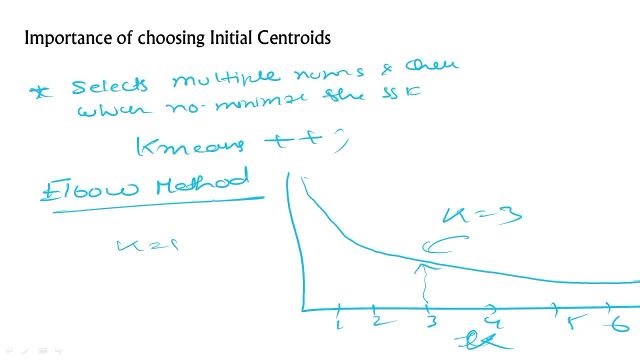 is decreasing ssc, ssc. okay, so that's why how we use elbow method: either you can use grits or cv or random randomized research to tune the this parameter. i think that will not work because, uh, we don't have labels, but uh, elbow method works. 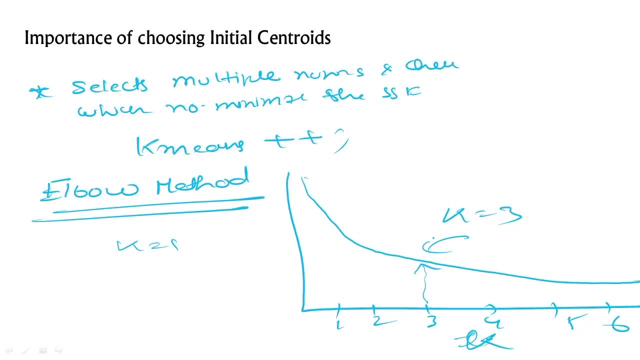 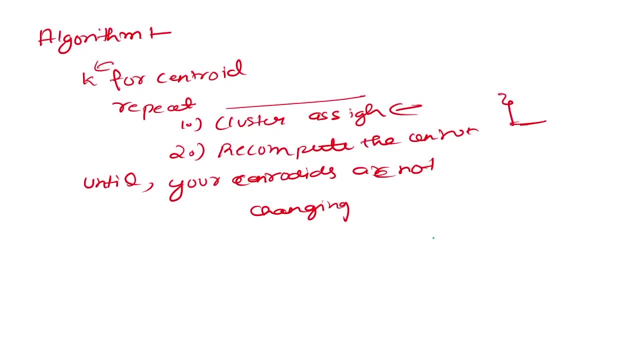 best when you plot it. you know when you plot it and see well what number of a k you need. okay, so that's it. that's, that's the following, and let's revise so that we are on the same pace. so what? what we do in k means clustering algorithm. we choose number of a k using the elbow method. 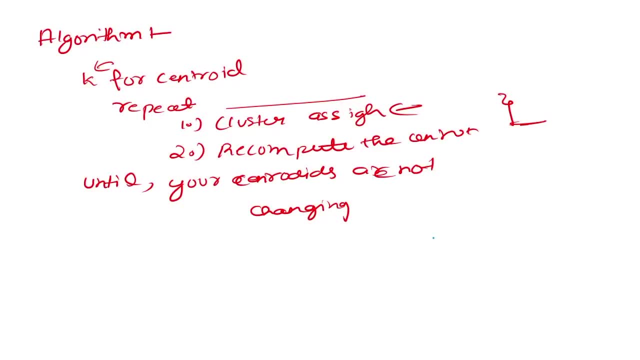 not now just just actually randomly, and then we plot it, and then then we choose the k and then what i've done, then we repeat like cluster assignment, like we assign all the cluster with the same clusters, then then we compute the centroid by taking out the average. okay, then you uh, then you keep repeating this until and. 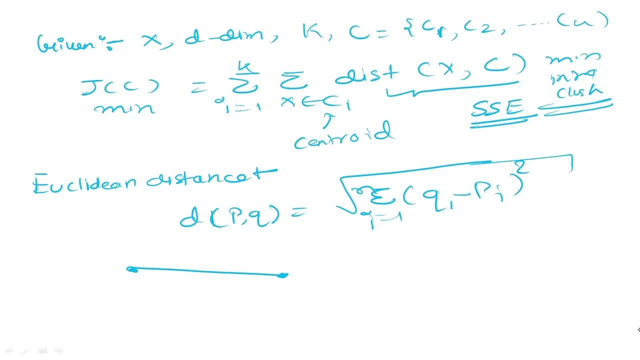 unless your centroids are not changing. and then, uh, the evaluation technique for your k means or loss function for your k means, is the, the. you want to minimize your intra cluster by just taking out the distance between two, this distance between the, the points, between points inside the cluster. 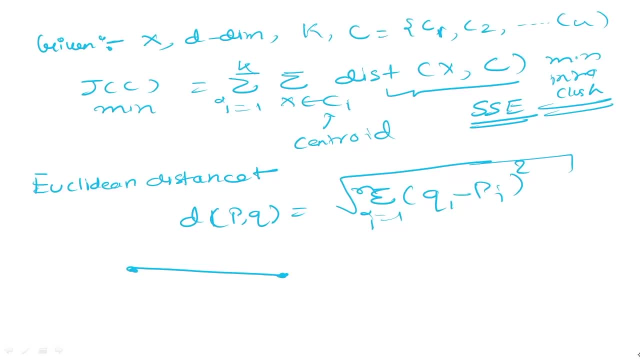 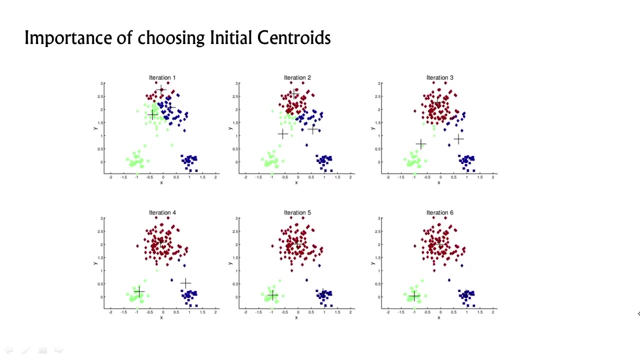 okay, and then that's called some square error. and here, and you take out the distance using the euclidean distance. that just that. just take out the difference between two points by doing the summation over there. okay, great, so uh, why, how, how, how we choose the in, how, how we choose the cent. 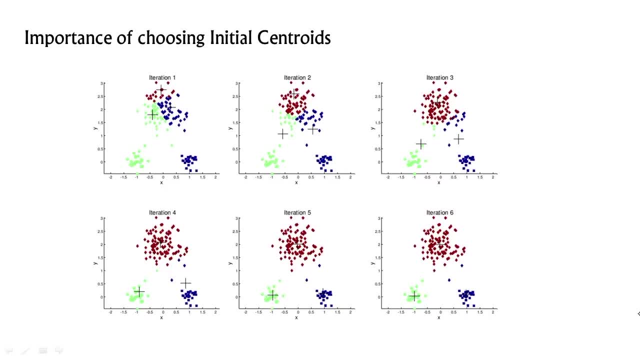 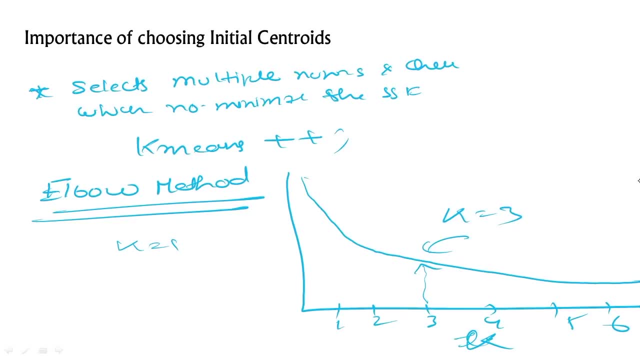 centroids: okay, the initializing of the centroids for initializing. we have seen over here that randomly initialized can cause a very big problem, so that's why we're going to use the centroids. okay, we have something called, as k means plus plus- which will help us to select a centroids using. 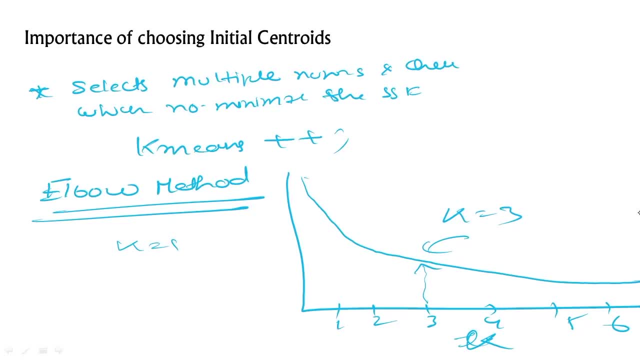 what it does, it select, it does for multiple runs and checks where uh and checks the numbers, who where uh. the sse is a low okay. and how we select the number of a k. we select the number of a k by using elbow method. we are uh, it the elbow is where elbow is turning around, like in as a hand. 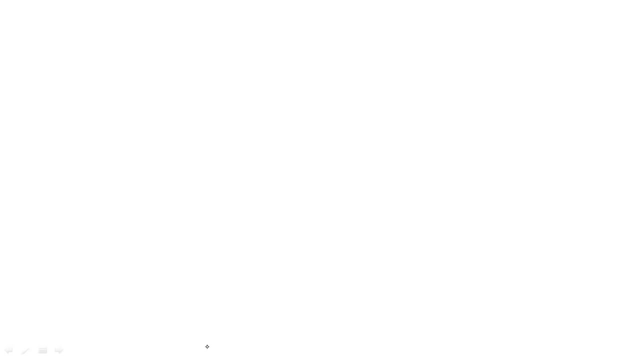 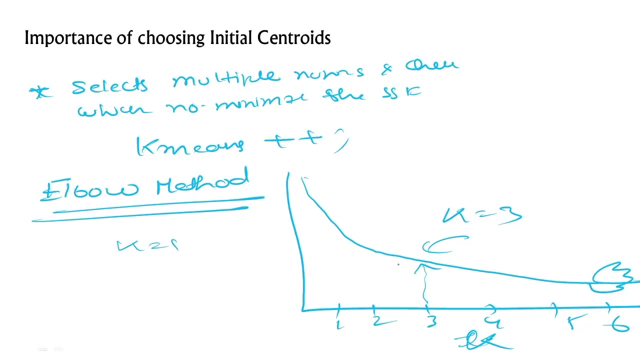 as a hand. if you draw it like this, if you draw it like this, if i draw a hand over here, if it draw it like this, okay, so your elbow is there, so your loss is decreasing. with k equals to one, is your losses this, this, this? okay, so you choose the elbow: k equals to. 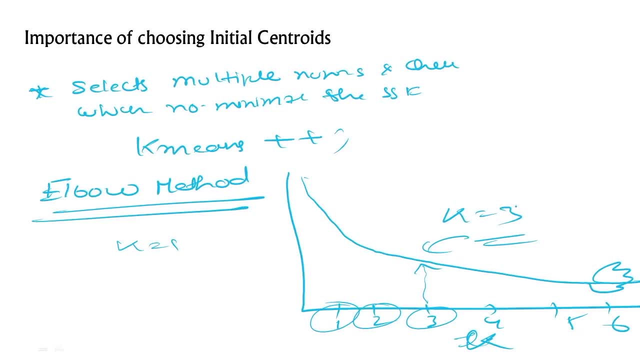 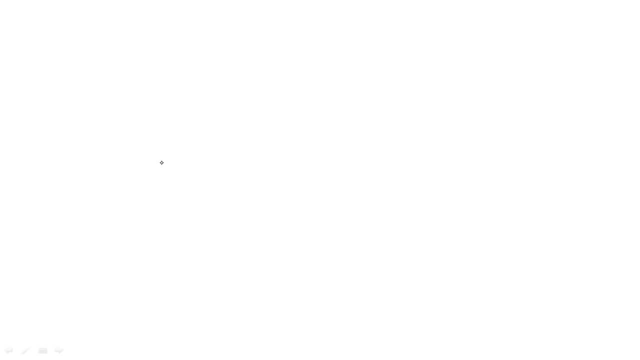 three, and it works best. okay, so we had talked about these things, and now it's time for ending up k-means clustering, the chapter of k-means clustering, which is uh, just, uh, just ending the topic with our favorite. what are the some of the limitations of k-means clustering? 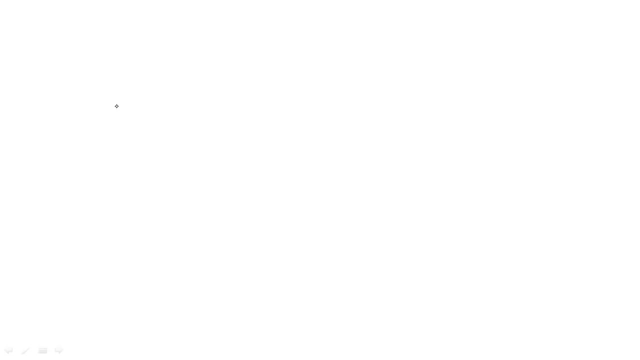 algorithm. and what is the first time? complexity. so the time complexity of k-means clustering algorithm, the time complexity, the time complexity of k-means clustering algorithm. if you don't know about from, if you don't know dsa, leave it okay, ignore this. the time complexity is order is time. 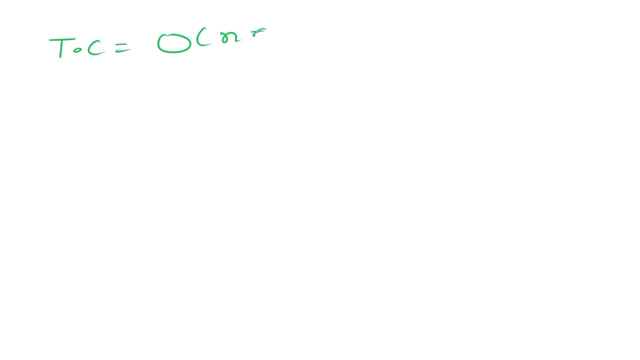 complexity order of n times k, and n is the input size, k, k is the number of clusters, i number of iterations, d the dimensions. okay, uh, this, this is our and this is this, this is what the time complexity of that? okay, this depends, because the time complexity depends upon your size. if you don't know about, 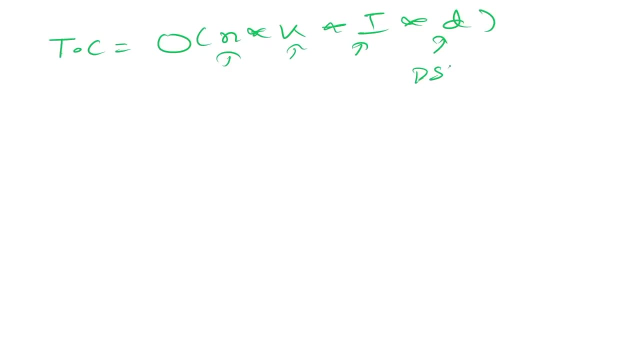 time complexity. i have one, something called as dsa mastery course. uh, soon we're putting putting putting videos onto that. so, um, first four lectures are based on time complexity. you can watch that. just go on anywhere. i will just show you where you can go. okay, uh, some, some of some of the limitations. 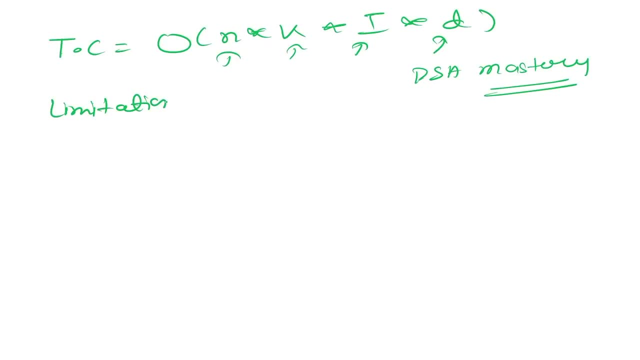 of k-means clustering algorithm. some of the limitations of k-means clustering algorithm is it's, it's very, it's very sensitive to outliers. okay, so let's assume that you have this, that that you have this. oops, like why, uh, powerpoint control z does not work. i don't know why. 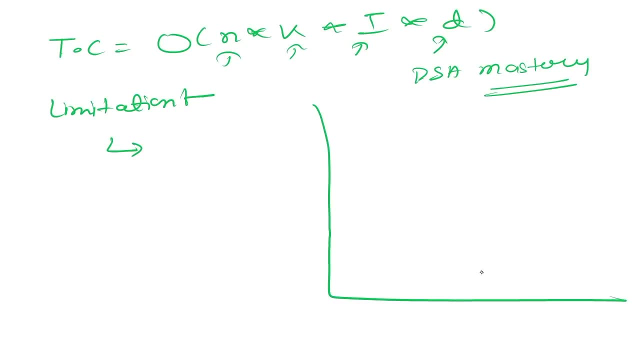 so, uh, here we draw an x and y plane and here we have x, here we have y and let's assume that we have made it, and here we have the outlier. here we have it is closer so it will take that outlier in that cluster, so we don't want that. so it is very prone to outlier means we have. we have to detect the. 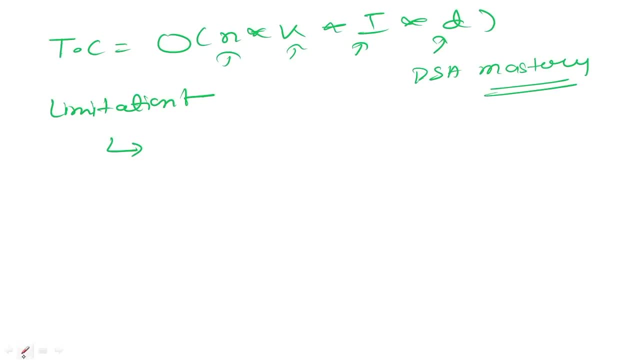 outlier and it can be solved using density based um even. i just don't know what s with what, what's there, so it can be solved. outliers problems can be solved using a db scan which you have a problem set to solve. okay means you have to read the wikipedia page. 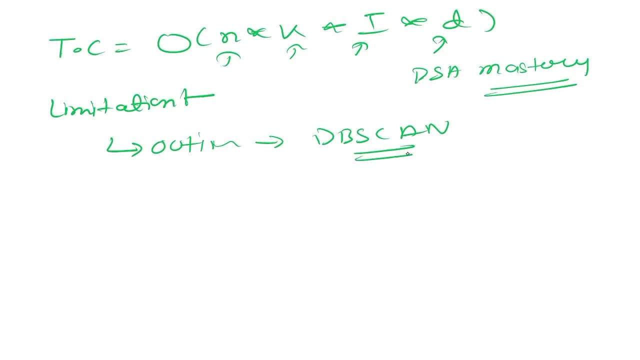 and uh write, uh go google docs onto the db, scan what you understood, okay, and then it's it's. it's like different sizes, different distances. maybe they're causing the problem, okay, but the main, main problem is outlier. okay, k-means says so. we have a. i have given you the thing that. 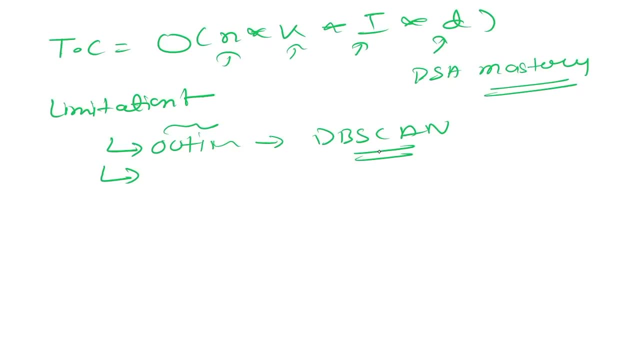 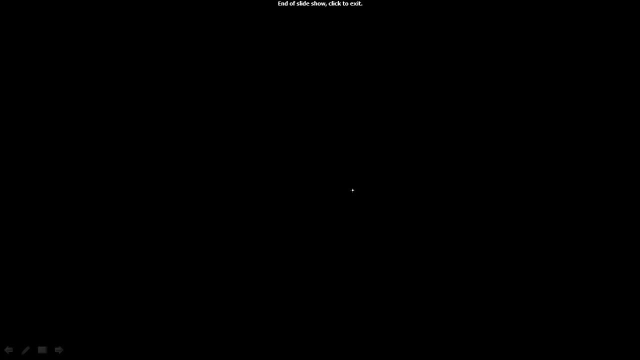 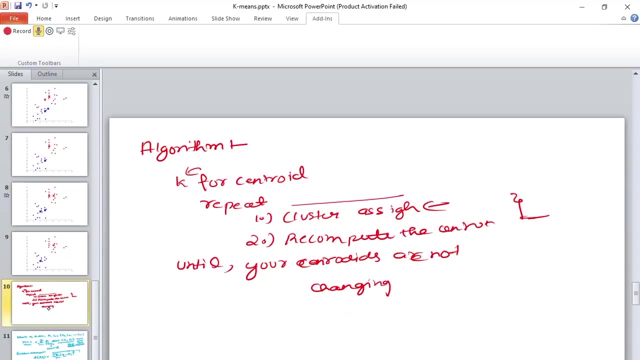 db scan. hierarchical clustering works on these types of issues. okay, so that's it for this k-means clustering algorithm and where you can uh record, where you can uh find the complexity videos, and it's very, very recommend. uh, just, it's a very, very helpful if you subscribe. 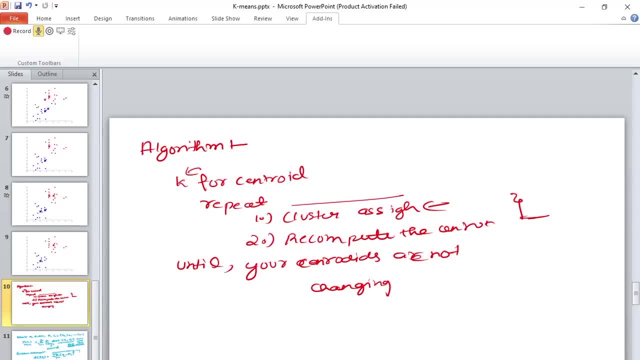 this youtube, uh, the new era youtube channel, which you can find um, which, which you can easily find onto the uh youtube just by writing. new era, where i have 500 to subscribers as of now. okay, so you can subscribe that and see the dsm mastery course, where we have more than 23 videos already uploaded. 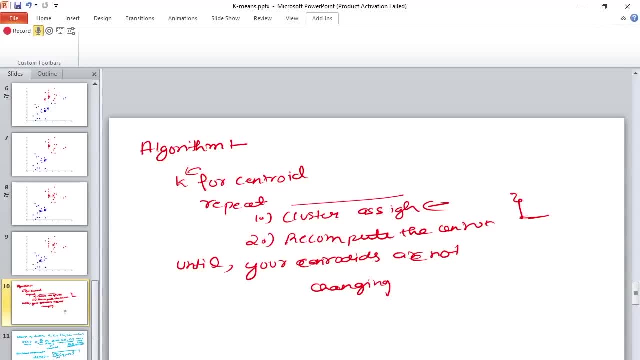 a long lecture so you can learn about time complexity from that also. okay, so that's it for this sub section. you now have a toolkit of various algorithms, various techniques, various things. okay, so now let's meet at the next section, where we'll be talking about hierarchical, hierarchical. 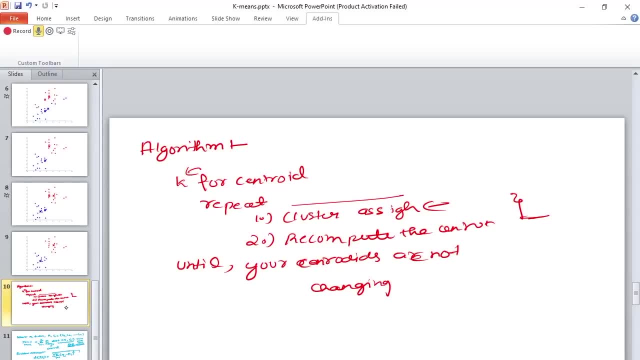 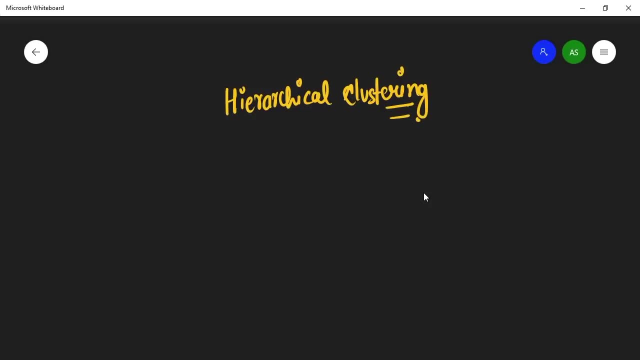 clustering. i will give it a thought so that it should make sense. okay, so let's meet at the next sub section. okay, so now we have talked about clustering, we have talked about unsupervised learning, we have talked about one of the particular functional based or center based approach, which is k means clustering with. k means plus, plus. 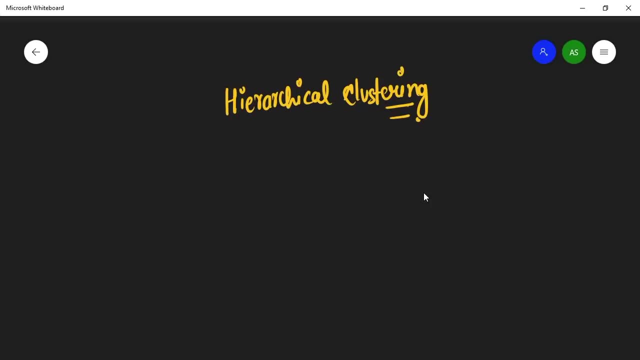 algorithm for random initialization. okay, so i hope that you understood everything in unsupervised learning and if you have gone so much further into unsupervised learning, now we are capable of learning hierarchical clustering, which is one of the most favorite- uh means one of the most. 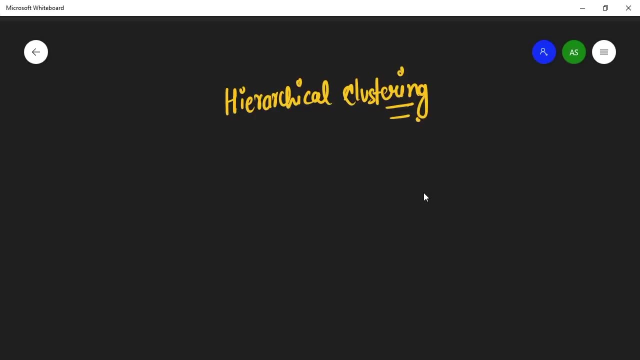 favorite uh and the best clustering techniques that include uh, including partition based, and then we have a hierarchy clustering. okay, so this is the. this is this. this is what we are going to do. we are going to start with an introduction to a hierarchical clustering to help you better understand what a hierarchical 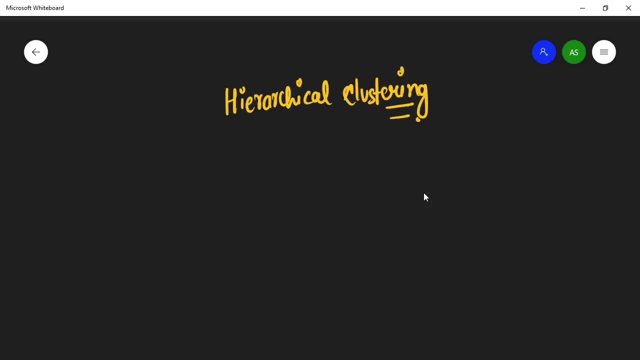 clustering is, then i will go further into different. i'm just just a quick recap onto partition based. okay, then i will show you the visual representation of hierarchical clustering and what's the dendrogram. okay, and then we will move further into understanding the two, two types of clustering, which is called agglomerative and divisive. okay, so agglomerative clustering. 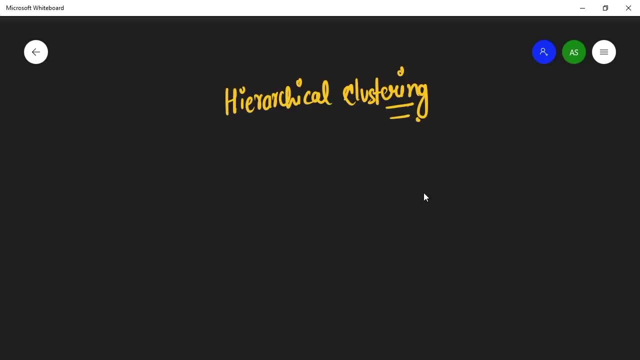 and diverse of clustering. we will dig dive in an agglomerative clustering and we will just take a look at the divisive, okay. and then we will go further into understanding the agglomerative clustering algorithm and then we will see: uh, then we'll compute that algorithm manually. 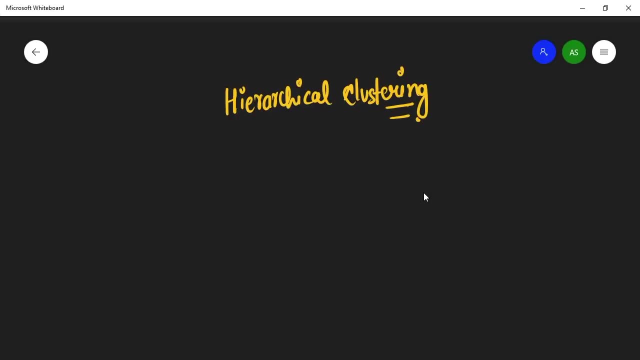 and then we will see the intercluster similarity between our two points. okay, but if, if, if you, if you all the words or technical terms are going above your mind, leave it means, uh, just ignore it the words. as of now. let's start with the hierarchical clustering. just introduction to hierarchical 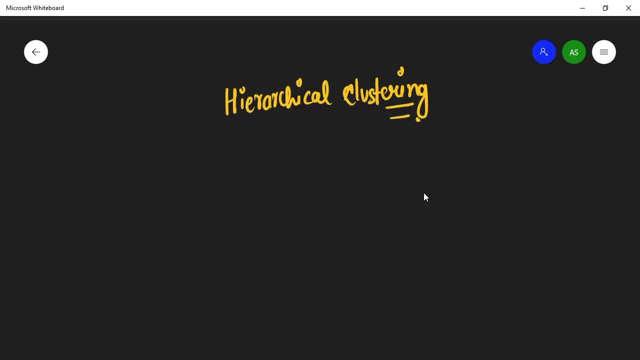 clustering. okay, so what is hierarchical clustering? hierarchical clustering is that you have a hierarchy of clusters. okay, so, for an example, what i'm going to do, what i'm going to do is i'm going to take four points. i'm going to take four points. points: p1: let's- let's not take it here. let's take p1 here. p1, then i'm going to take p2, then i'm going 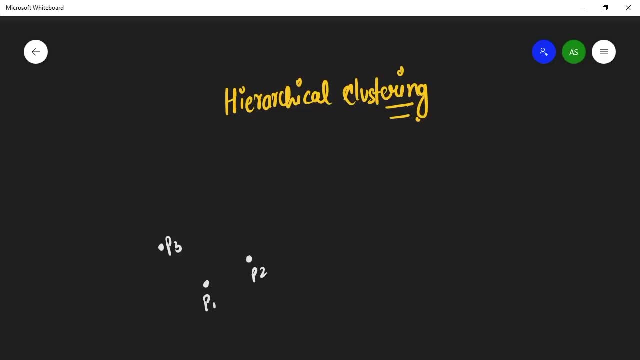 to take p3, then i'm going to take p4. okay, for an example, i've taken these four points and now we want to cluster it out. okay, now we want to cluster it out. so how do we cluster it? so for clustering, so for clustering, we have our favorite means. we can simply see: okay, this distance is small, these 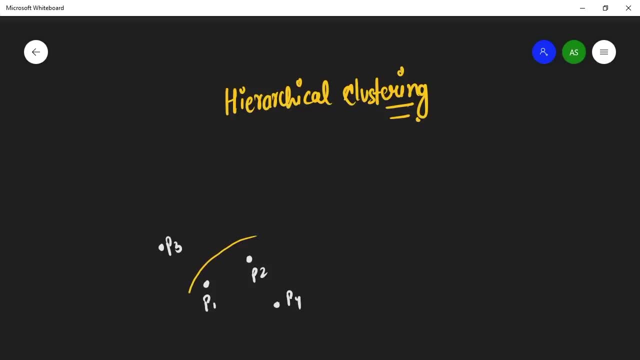 two points are similar. we are going to do this, we are going to cluster it out like this and we have this: uh, p3 and p4. how do we cluster? we cluster this. pp1 and p2 are are here, so we cluster we, we put another cluster. okay, because this, this cluster p1 and p2 is p1 union. p2 is now a one cluster now. 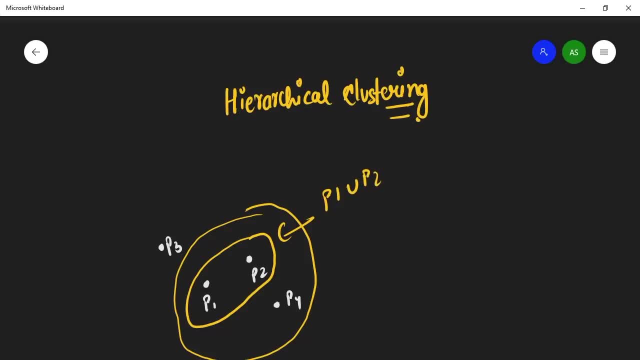 in nearest the data point, nearest point between or the nearest to these. these are their own clusters. initially these are their own clusters, so we are going to merge it, okay. and so here we have a p1 and p2. now the, now that this uh smallest distance is p4. now we attach means, now we make one more cluster. okay, now in this, 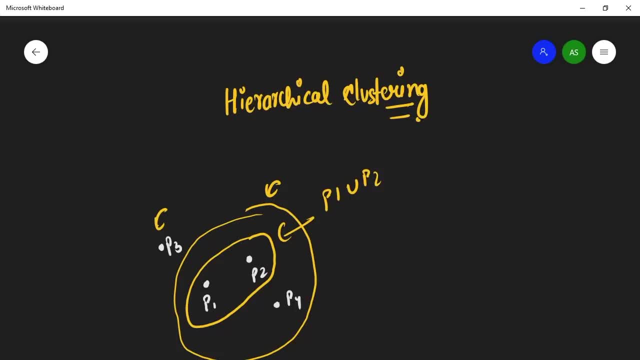 big cluster. in this cluster where we have three points, what is the nearest data point? now? the nearest state data point is p3. okay, so we'll make again one cluster, again one big cluster like this, until and unless we have one cluster at uh, one, one, one cluster uh. 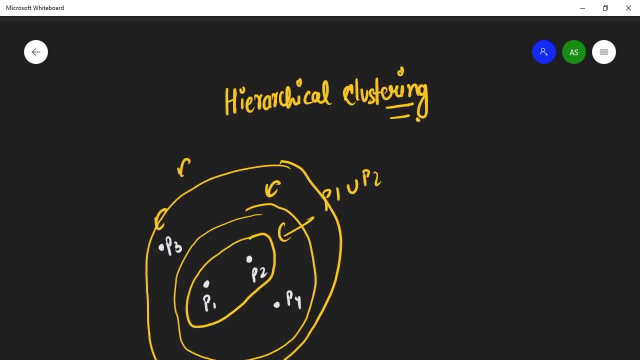 at a point. okay, so here we we are, ended up with one cluster. okay, so it is not making sense, i know, but we can. um, just just as a diagram, i have made this, so let's see how, how we do it using a dendrogram. that that will make more sense. okay, so here we have a p1, here we have a p2. oh, oops, let me. 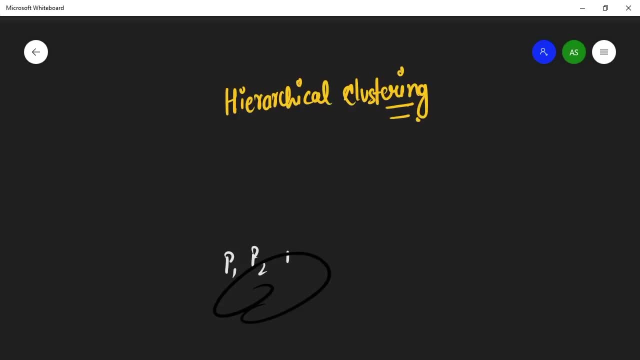 make a little bit more in good oops, what happens? okay, so here we have a p1, let's assume that we have. this is the point p1, this is a point p2, this is the point p2 and this is the point p3 and this is the point p4. 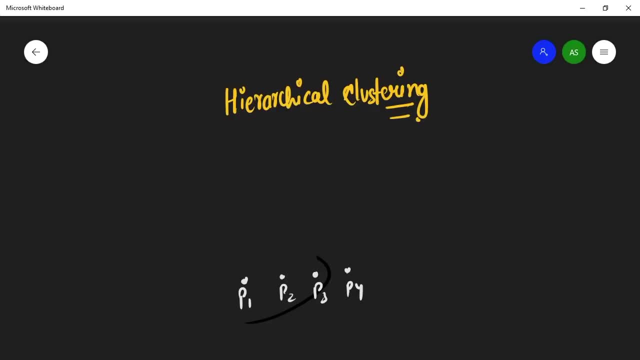 okay, now, these are the points, now what we will do with here. you can see, let's assume that, just assume that this is p1, p2, p3 and p4, and you can see this: p, p1 and p2 are smallest, so we can make. 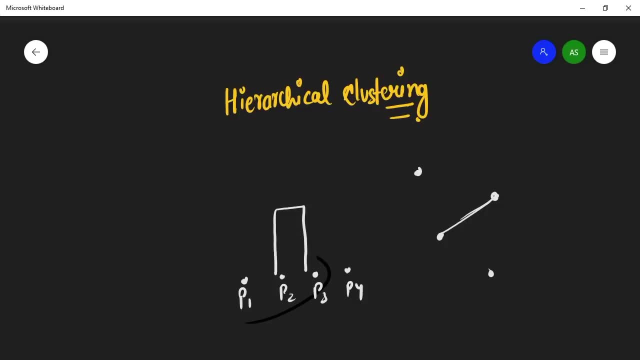 uh, we can attach this, we can make a dendro. uh, we can make like this, we can attach this. p2 and p3. okay, now these are one cluster. p2 and p3 are one cluster, which usually cause p2 union, p3. okay now. initially p1 is one cluster, c1, p2 is one cluster, c2, p3, c3 and p4, c4. okay, so these 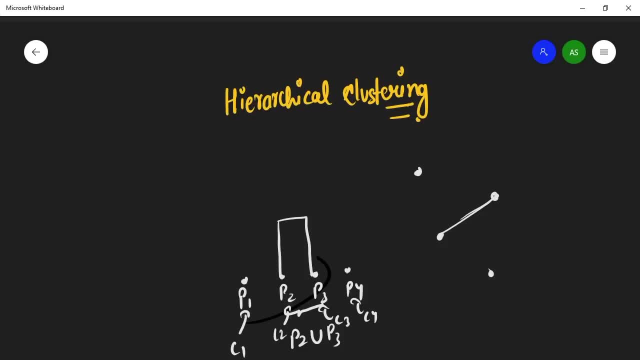 are initial clusters. now, what now? what we'll do. now, this is the one cluster which is c2. okay, so we've we, we found and attached it. okay, now, what now? what we will do. now, the nearest state data point is p4 over here. okay, so what? what we will do? we'll again attach p4 into this. 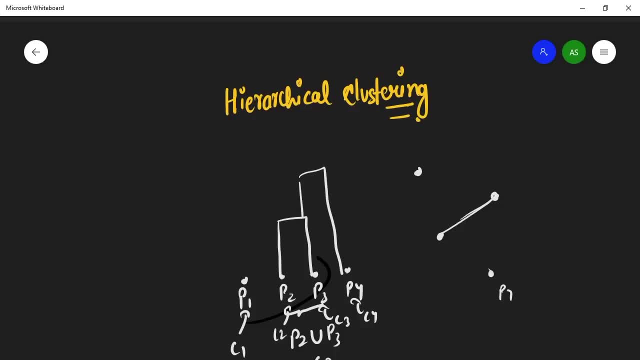 we'll again attach people. now we have. now we have p3 and p4 as one cluster over here. okay, now we are. now we can attach p1. now we can attach p1. now. now we can attach p1 like this: now we can attach p1. and now we have our dendrogram, which is actually a hierarchy of. 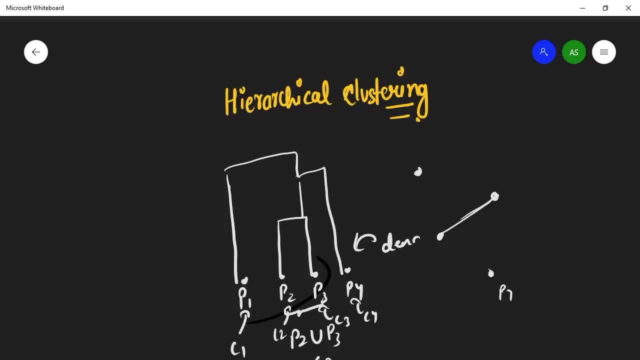 clusters. okay. so here we have a traditional dendrogram which, uh, which, which i think that you have all have seen in your journey. so this is your hub, this is your dendrogram. what you have done you have just who are most similar, you attach to it. okay, who are more similar? you attached it. 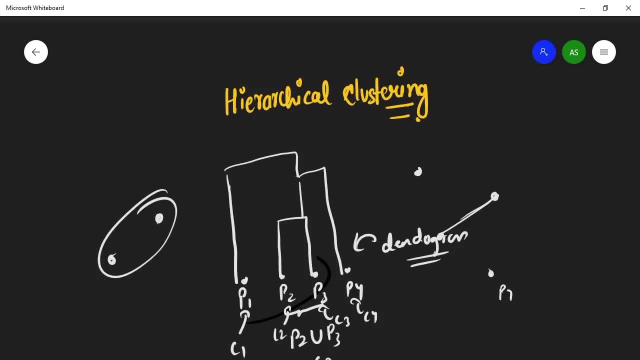 for an example, these are two similar. you attached it and then these: this is now what you attach it. okay, do not merge it. do not merge it. okay, so you have to do, do like this: now, here we have until and unless we have left with one cluster, okay, so that's the basic, uh, hierarchical clustering. 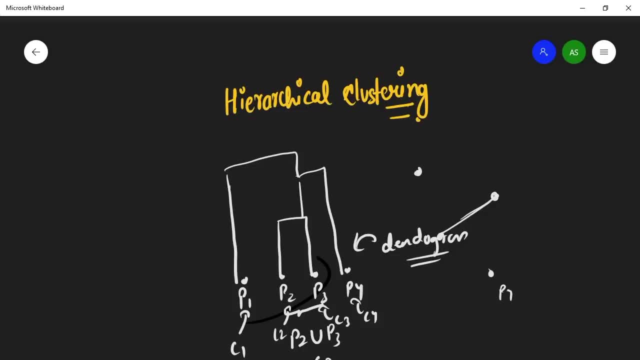 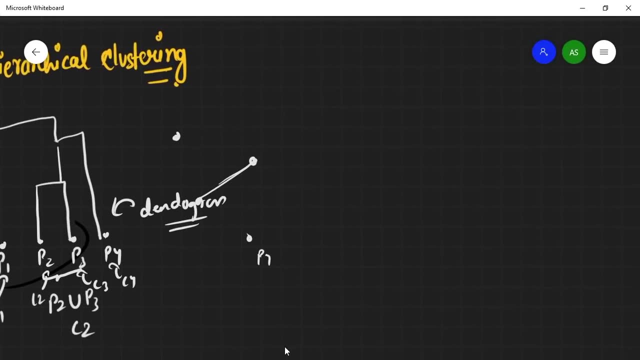 and i hope that you understood hierarchical clustering, the basic intuition. but if not, let's, let's try to again understand a little bit more further into a more sophisticated way. okay, not so for some, just just a easy way. okay, so for the example, i'm going to take a yellow color. so here, 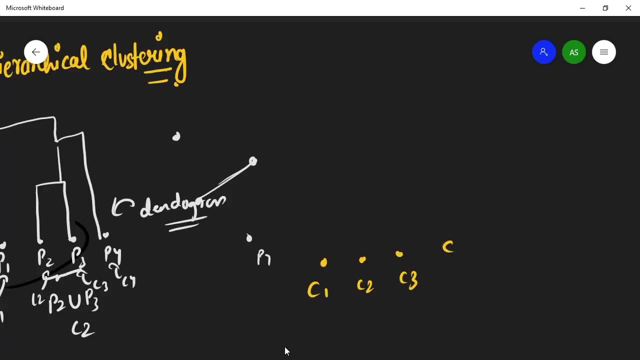 here you have a c2, here you have a c3, here you have a c4. okay, so these- uh, this is your c4. now you can this. c2 and c3 are your points. c2 and c3 are your points, okay. so these are two too much. 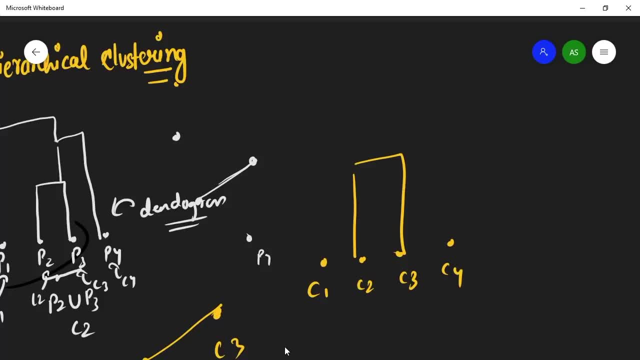 similar. so you will attach this like this. now, c4: here here's your, so will you make you? so you will make one one more now, p, c3 and c4 will be attached like this: and c1 will be attached onto the up of c4. 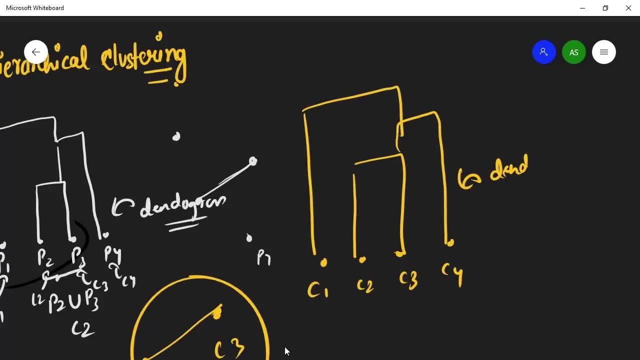 is a traditional dendrogram. this is a traditional dendrogram where you convert this cluster of numbers, where you convert cluster of numbers c1, these clusters clusters, to a hierarchy of clusters. okay, so for an intuition, what, what, what? i'm trying to see you here. so i have one example. 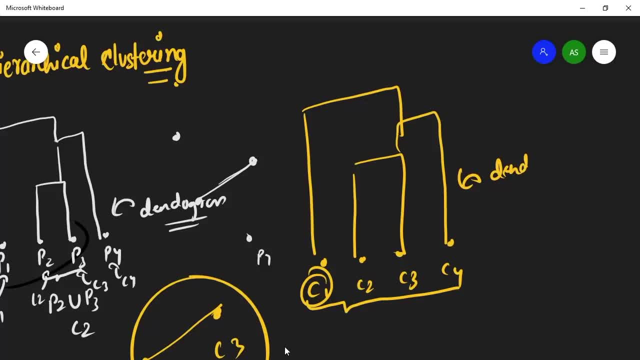 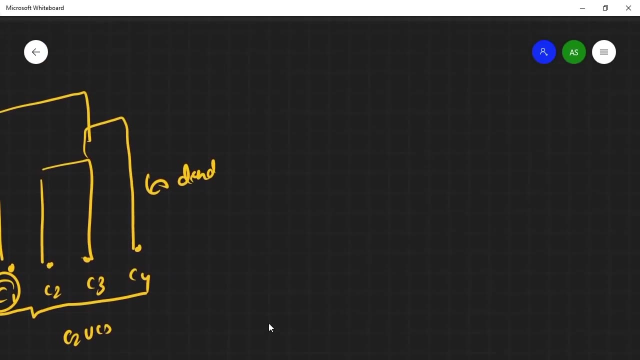 so, for intuition, what i'm trying to say you here that we have a c1, c2, c3, c4. now we're just making a attach, attaching as a cluster. so okay, so this is the basic intuition behind hierarchical clustering. so there are two types of hierarchical clustering. some of the types are: we have some something called as agglomerative. 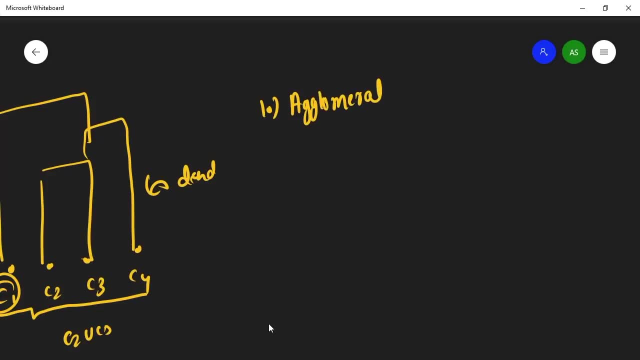 agglomerative clustering, and then we have, and then we have divisive clustering, and then we have divisive clustering. okay, so we will keep having an agglomerative clustering. i'll just give you an intuition behind divisive clustering. okay, so what is agglomerative clustering? so the agglomerative 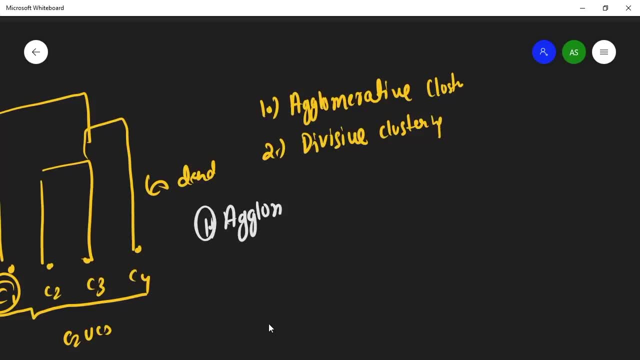 clustering, agglomerative clustering, okay, so, before that, let's understand, let's, let's see, let's, uh, let's, let's understand the divisive clustering to help you better understand that. so it is down to, it is up to down approach. sorry, it's a down to up approach, it's a agglomerative. 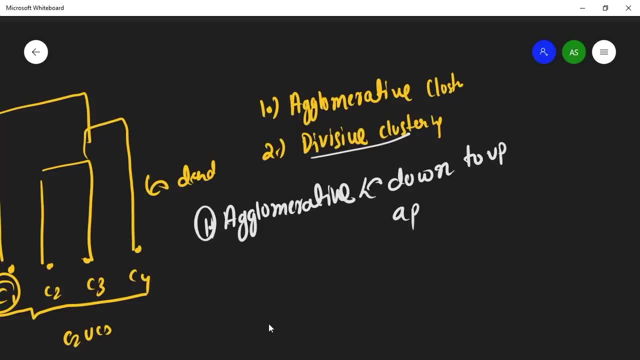 is a down to up approach and divisive is just opposite. it's just opposite where divisive, divisive is just up to down approach, up to down approach. so what do i mean by this? so, for an example, for an example, let's assume that you have a four points, we have a five points. 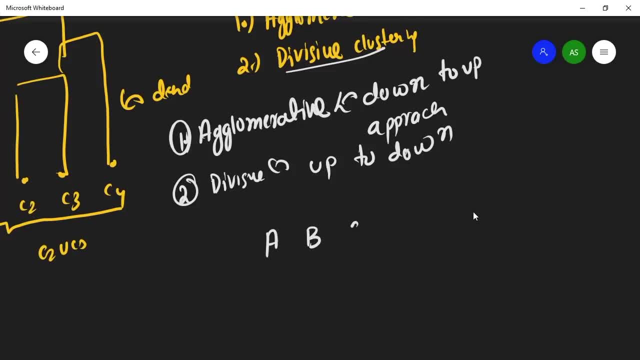 in the form of data: a, b, c and d and e. okay, so here what you, what you are going to do here. what you are going to do is you're going to divide this cluster of numbers, the cluster of, is you're going to divide this cluster of numbers, the cluster of numbers, into a different, different. 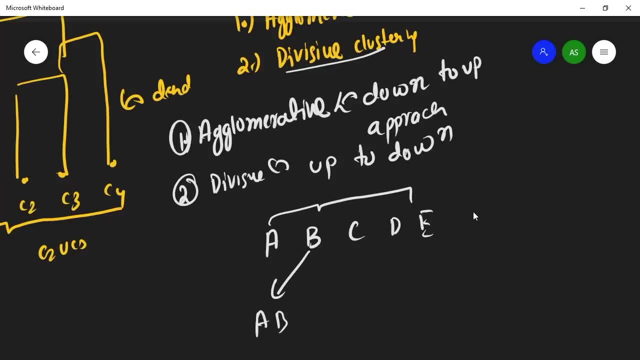 numbers, the cluster of numbers, into a different, different uh, a, b. let's assume that you are divided. uh, a b. let's assume that you are divided with a b. now this is your c, d, e, c, d, e, c, d e as a most similar with a b. now this is your c, d, e, c, d, e, c, d e as a most similar. okay, you divided this. now what you? 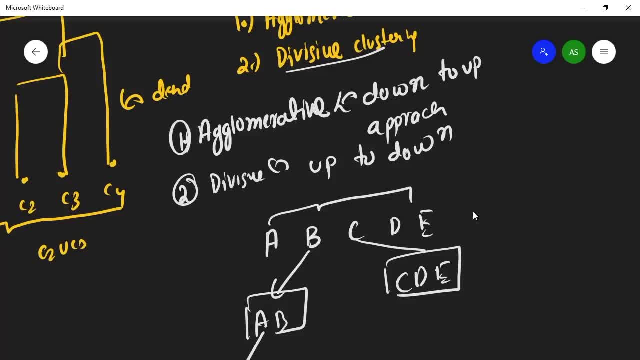 okay, you divided this. now, what you will do, you will devise this: a and b, a and b. now you will divide this: c, c and d, d, e. okay, now you will take the d and e. okay, so this is the basic. uh, this what? what you are doing? you are making the cluster of numbers into separate, separate numbers. you're. 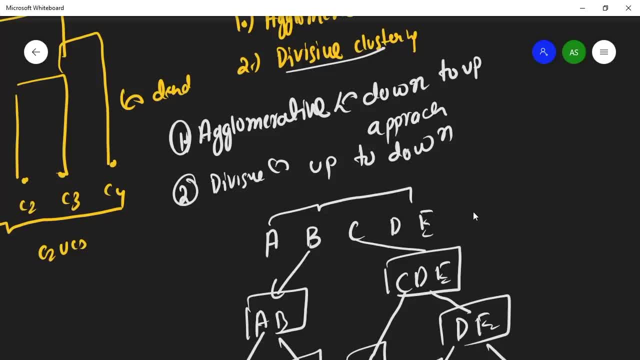 making the hierarchy of numbers. okay, hierarchy of numbers, and this is what you are doing. okay, so you're just making a die um hierarchy of numbers. it's like a, b, c, d, is you're going to up to down approach, from up to down approach, but in the case? but in the case of, but in the case of. 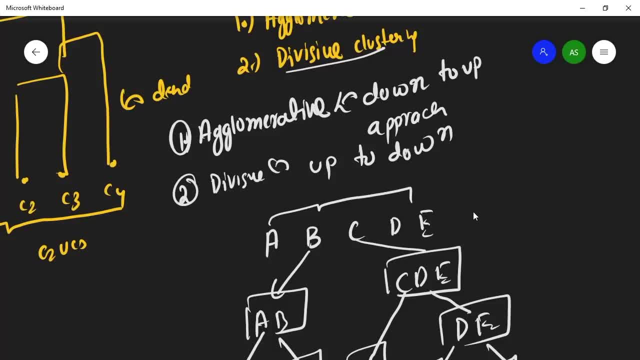 agglomerative. you're doing something different. you are here, you are going up to down, up to down, and agglomerative you will take. you will take because in agglomerative you have cluster one, c, two. they are unique clusters means only one cluster, so you do. 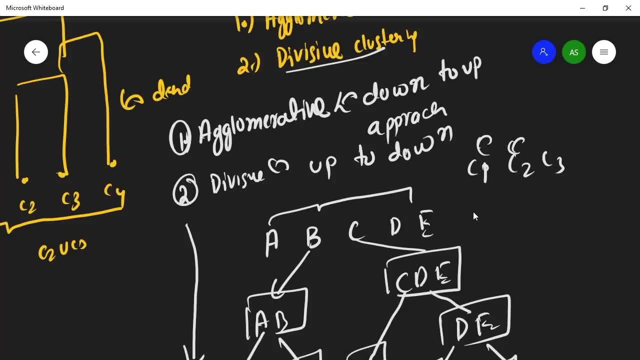 merge it okay, you do merge it okay. so it is agglomerative as up to down approach. sorry, down to approach, down to up. okay, so that's the basic intuition behind agglomerative and diversive clustering. okay, so we'll see in detail about agglomerative clustering and 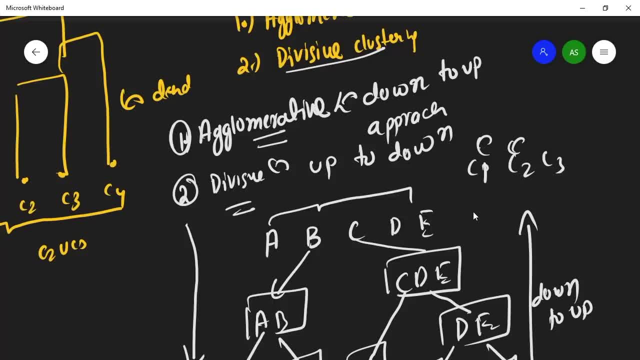 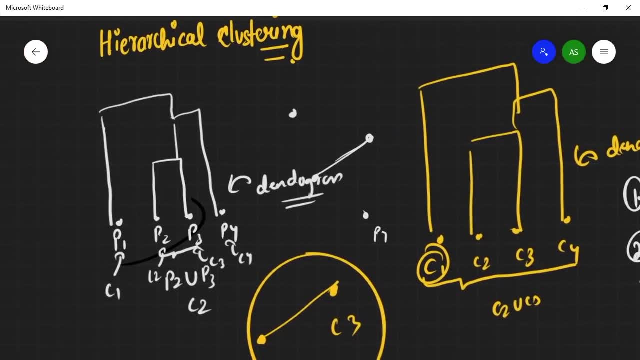 diversive clustering to help you better understand all of this algorithm: agglomerative and diversive. but the basic intuition behind hierarchical of clustering, hierarchy of clustering is that you have some points and what you do? you simply, you simply, you simply merge to cluster because these p1, p2, p3 are before our fourth cluster. initially you merge to cluster. 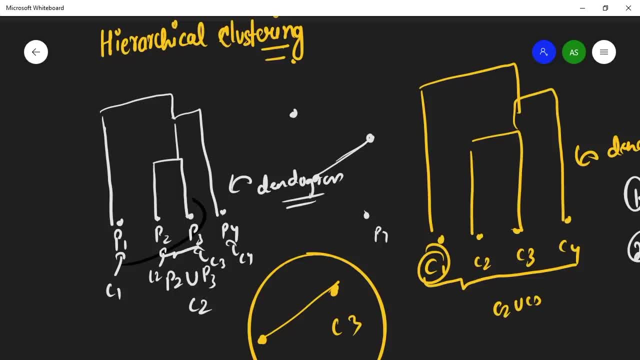 and then you have some kind of similarity matrix. okay, so you have some some kind of similarity matrix that that we'll see. according to that, you merge it and then you make a dendogram or hierarchy of clusters. okay, so that's the, that's, that's what the agglomerative and 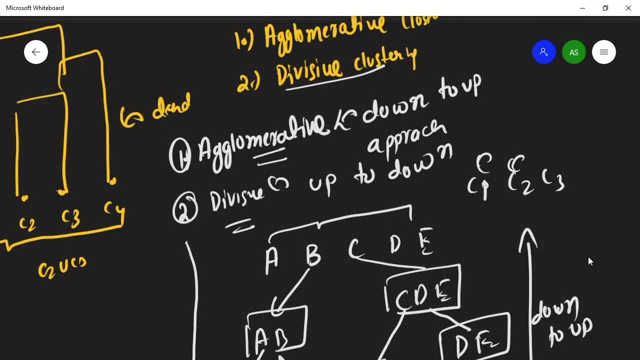 agglomerative is just down to approach where you are converting the, converting the clusters into by merging different different cluster until and unless you have one cluster left at the top, like this c1. okay, as an example, and in diversives you are actually going up to down approach when dividing the cluster into a single single group. okay, like a, b, c, d, e, okay, so 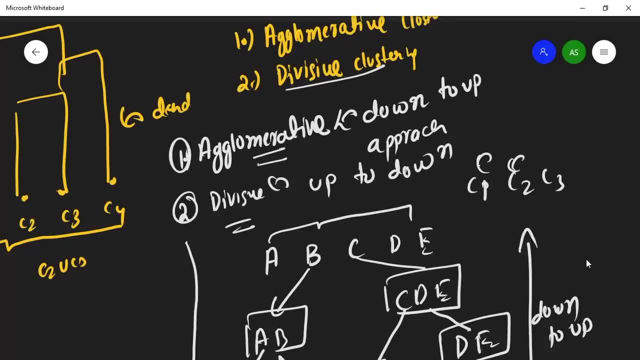 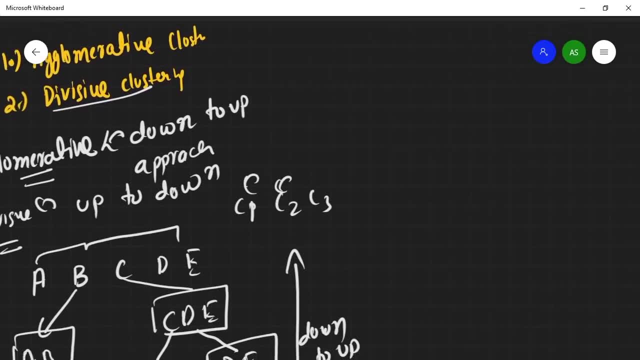 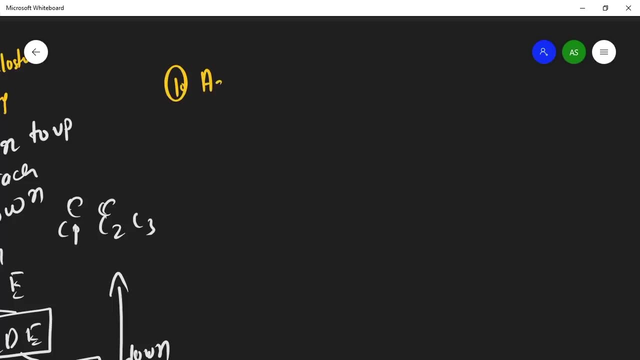 that's the basic intuition behind this. uh, agglomerative and diversive clustering. okay, so let's start with agglomerative clustering. deep divinator, agglomerative clustering- to help you better understand what an algorithm, agglomerative, agglomerative clustering does, and we will see a lot more about this. okay, we will not. 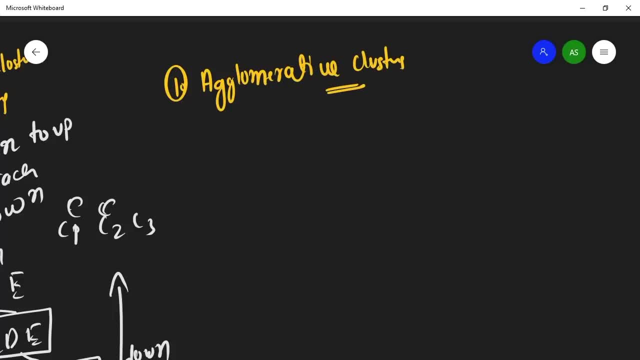 see the implementation as of now. we will see in another section where we now we are now after this, i think we are, we have, we have completed this theory part. all those stuffs means we have now have a good knowledge of everything. now, what, what we will do. we will make a lots of projects, okay. 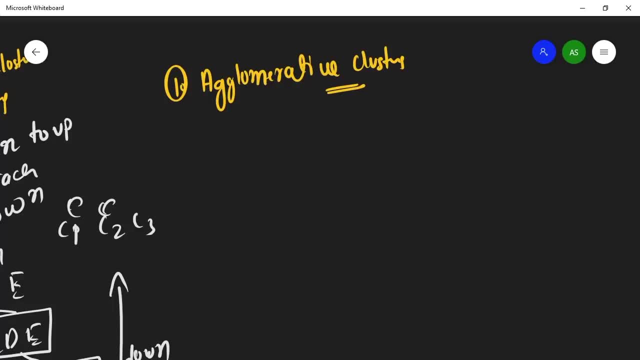 so here's an algorithm. so first, if you're so, first let, let me write an algorithm. i will write an algorithm and then i, then i will make you understand with the help of good examples that i've already listed over here. okay, okay. so here first what, what we will do, first you, we. 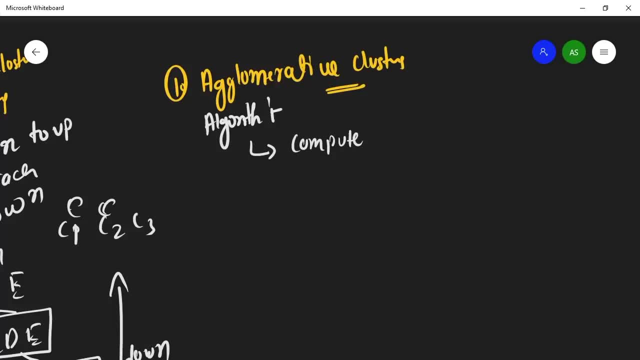 compute the proximity matrix. we compute the proximity matrix proxy midi matrix. that just tells you the similarity between two points. second: we will, we will see, we will see, we will see just as how it looks like, and then you repeat these two process, then, then you repeat these two. 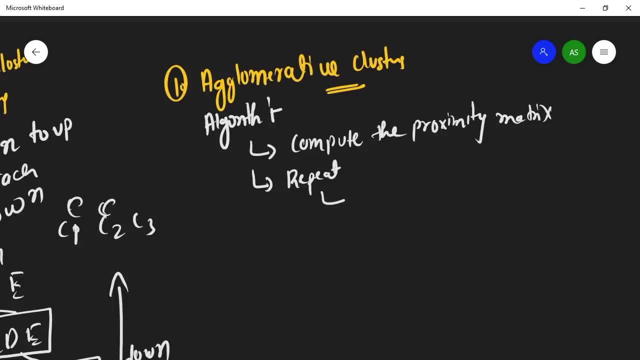 process. then you repeat these two process, merge, merge two clusters, merge two clusters and update the cluster, update the matrix, update the proximity matrix, proxy, midi matrix. okay, so that's the basic, that's the that you repeat in a for loop and then you, until and unless, until you have one cluster, you have one large cluster left, means until you. 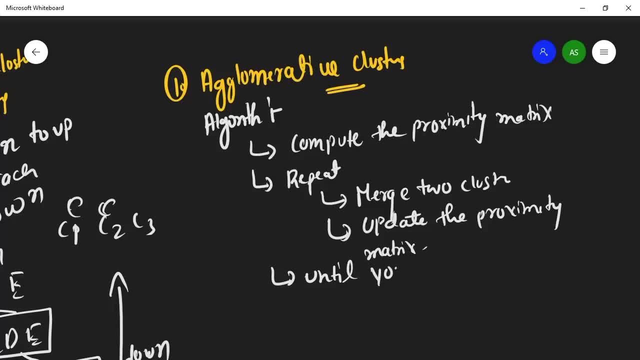 have left. you have covered all the cluster. okay. until you have covered all the cluster, okay, covered all the cluster. or we can say no clusters are left as a single cluster, okay, but this is, this is a more formal definition- until you have a good cluster, like as an example that I've showed to you, okay. so this is a 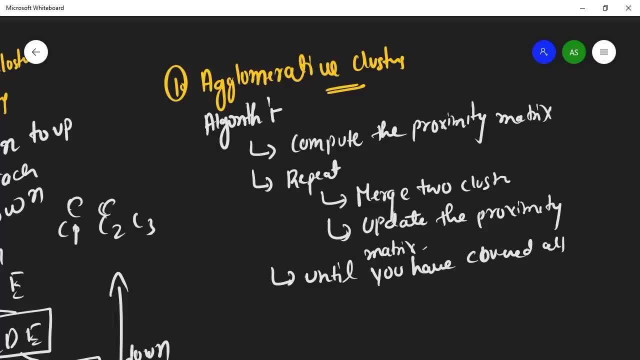 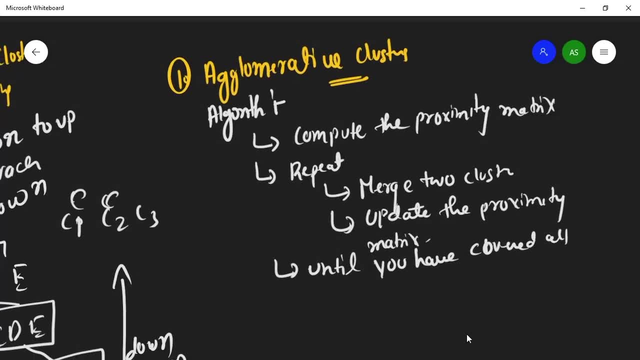 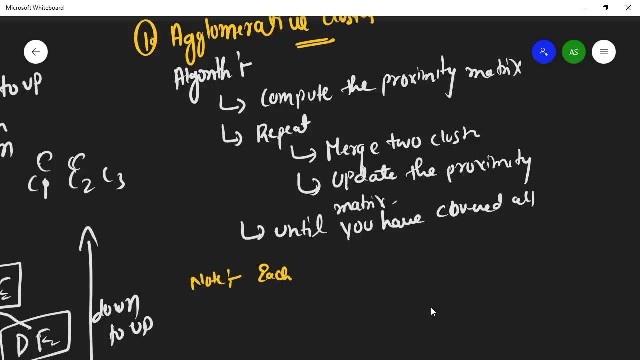 basic algorithm to understand an agglomerative clustering. now let's understand these in more detail. okay, so initially, what I've taught, what I've note here and what I'm going to note here- like I'm not going to write note- which is each, each cluster, or P 1, P 2, P 3, each are its own cluster. now we'll be. 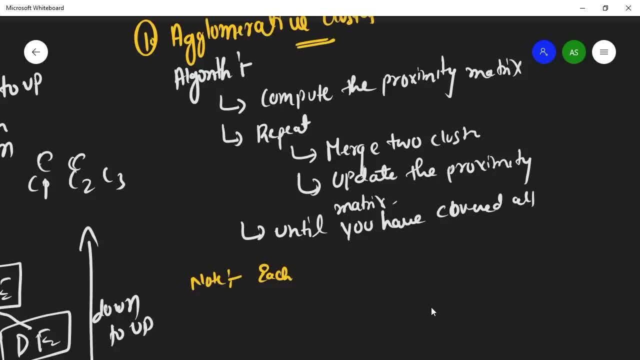 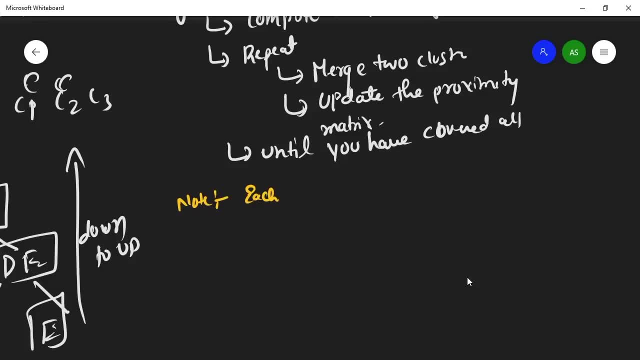 able to build a hierarchy of clusters. okay. so let's, let's build. let's build on proximity matrix how it looks like. so the proximity matrix looks like this: let's iron. let's assume that you have P 1, P 2, P 3, P 4. okay, 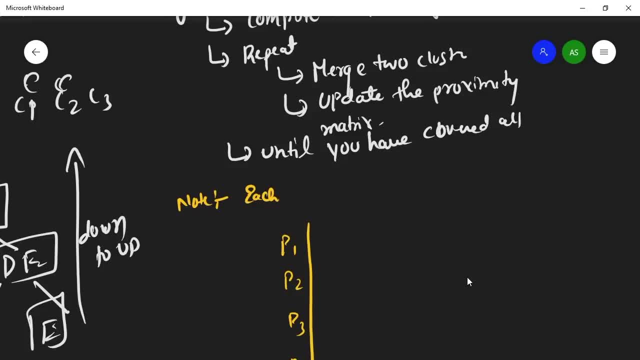 I just assume, as an example now, what you do you? you do this: P 1, P 2, P 3, P 4, okay, now you do this mean this: this is a proximity matrix, this is your proximity matrix, like this: okay, okay, and these diagonals are 0, these: 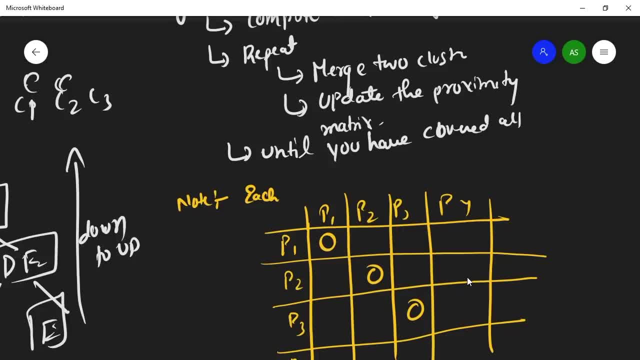 diagonals are 0. this diagonal, the diagonals are 0 because the distance between the distance between the P 1 and P 2 will be obviously 0. the distance between P 1 and P 2, maybe some poop 2.4. there is P 3, P 4, like that. so we have we. 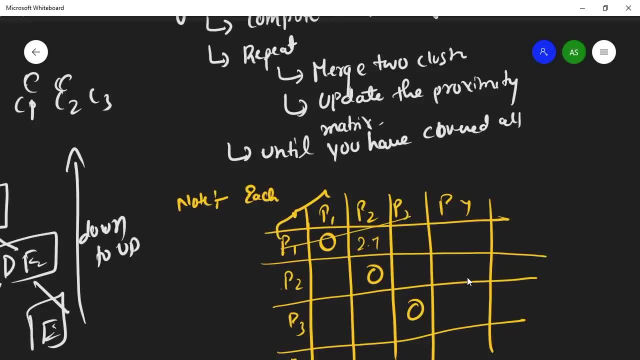 have written like that P did. the distance between P 1, P 2 and P 1 is maybe something like: and diagonal distance between P 2 and P 2 is obviously 0. okay, so this, this is what the basic. this is what the basic. 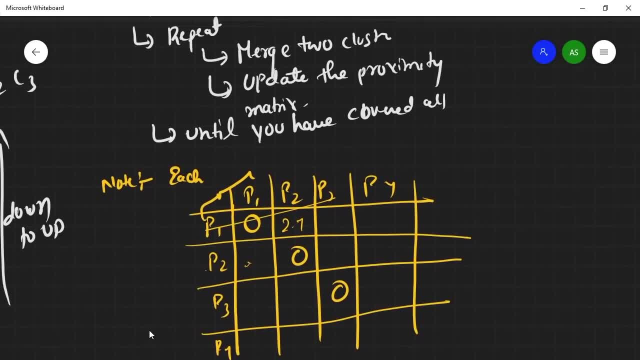 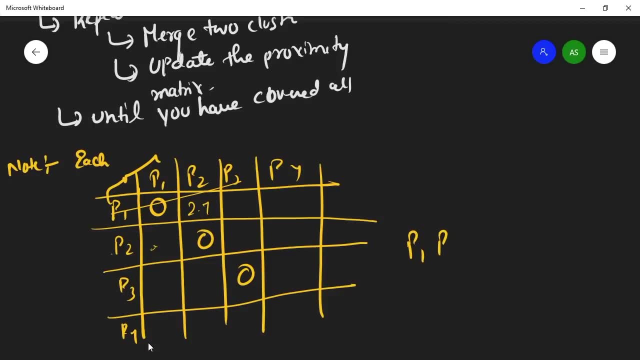 proximity matrix looks like. so let's see, let's see. and that how we, how we make a dendrogram. okay, so here we have P 1, P 2, P 3, P 4. now assume, now we will just assume that let's take an example- that this, this is four, point six to four, point two: 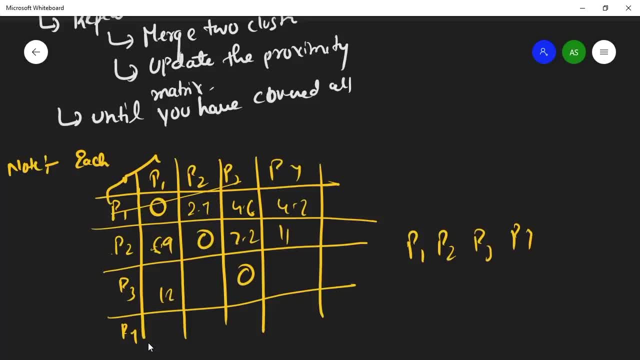 six point nine, seven point two, eleven, twelve, thirteen, fourteen, fifteen, sixteen, seventeen, eighteen. okay, it's a zero. okay, so the distance between P, P 4 is P 4 is obviously, is it okay? so the P 2, we, we will find the smallest one, we will find the smallest similarity here, you can see. 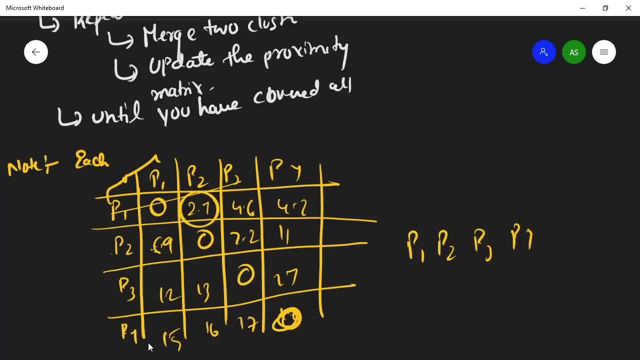 that this, this is the smallest similarity- P 2, and I think, oops, it's a, it's a P 2, and also I think that I'm not drawn a good mayor. I will tell you so here. let's, let's assume that you have this proximity matrix, that you have this. 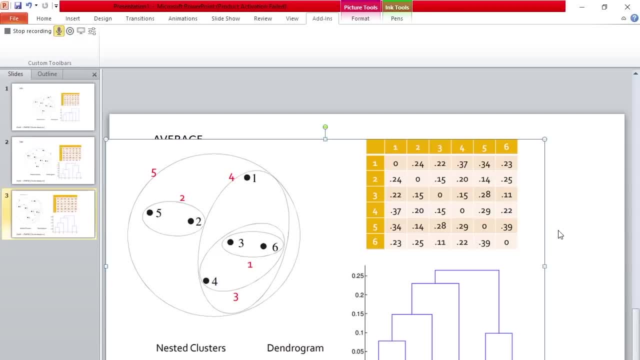 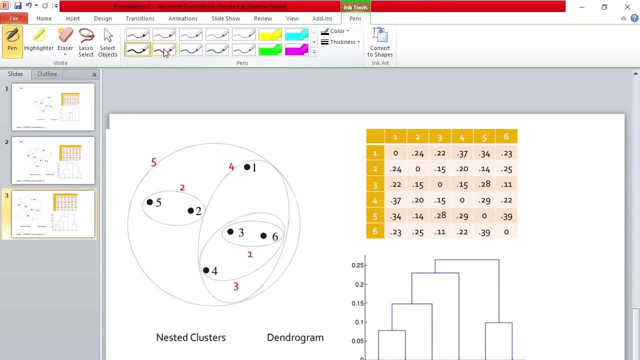 proximity matrix. just just don't take a look at this proximity matrix now. what you will find is smallest similarity. so the smallest similarity, so the smallest similarity over here is this: 3. here we have 3 and 6. okay, so here we have 3 and 6. that we have done first. 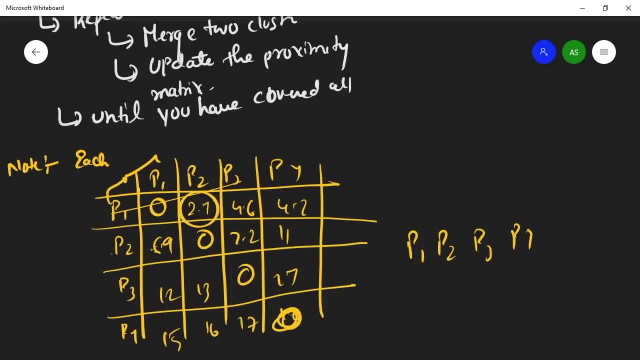 the smallest similarity. okay, so that's the. that's. that's what we haven't going to do, so assume that this is P 1 and P 2 has a small interest. now we have, now what. but now the next is. the next you can find over here is 4 means 6 and 4. 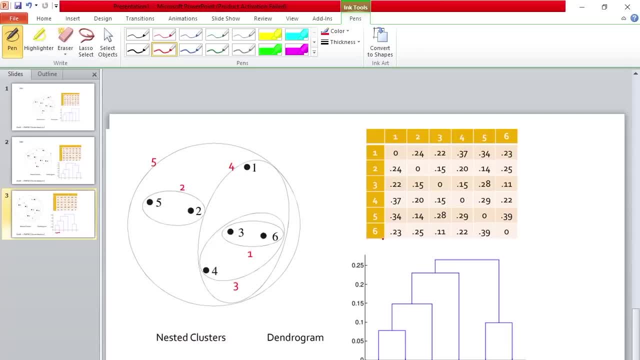 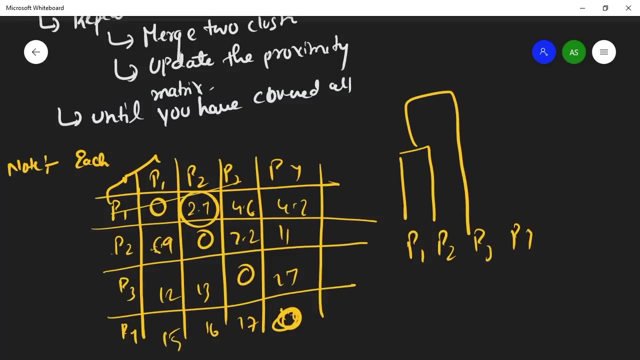 maybe let's see six and four, which is here. okay, so we can go over here also three and four. we can see this three and four also. okay, so we can take this three and four like this. it's okay. so just assume the next smallest is p3 and the next smallest is p4. okay, so now we have constructed. 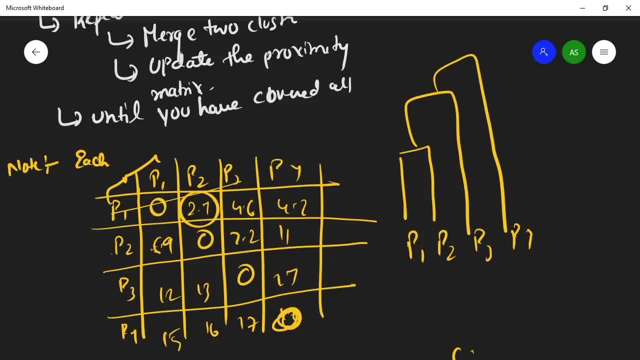 now, let's assume c2, p1, p2, p1, then we have a again maybe some p3 and p4. now first you do this, then you do this, then you make this like this: okay, so now we have now and now you have the hierarchy. 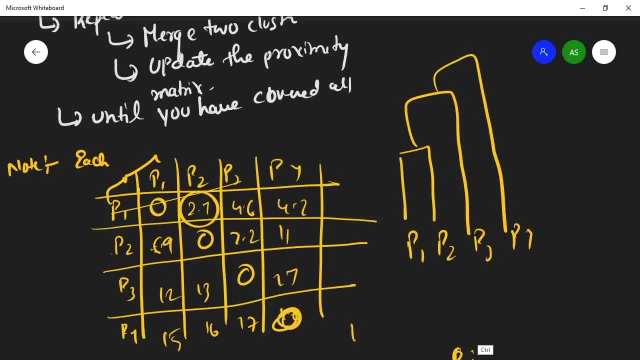 of clusters. okay. so that's the basic definition, that's the basic algorithm for proximity matrix. okay, and this is what you do and you update the proximity matrix. so how you update, now you merge the merge the cluster. now what you will do: p1 union, p2- okay, p1 union, p2, this one will be, let's assume, p1 and p2 are. 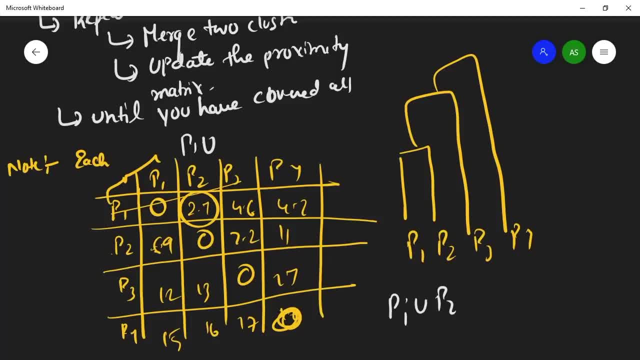 attached, then p1, union, p2, this will be the cluster. okay, now let's assume that the 2.7 and these are this are similar means: this 2.7 and maybe some, maybe like that, so we can combine the cluster like that. i think this is not the actual example. this is that example. okay, but here you can you. 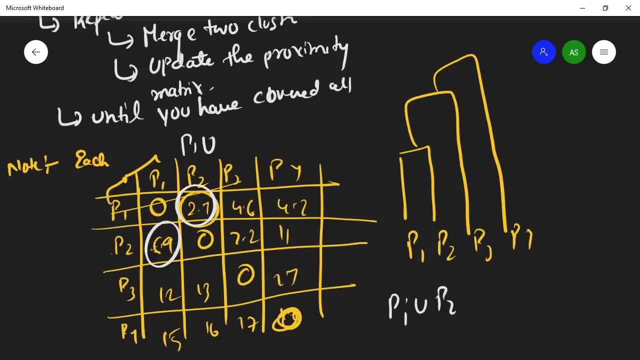 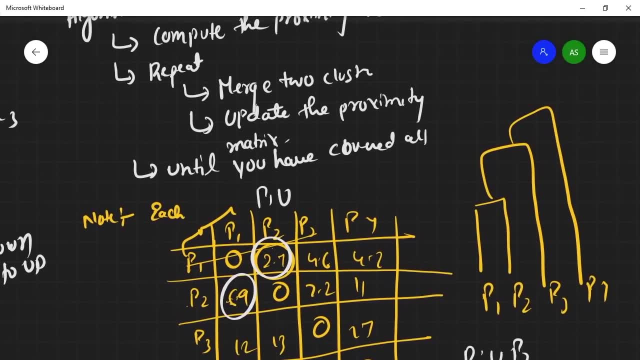 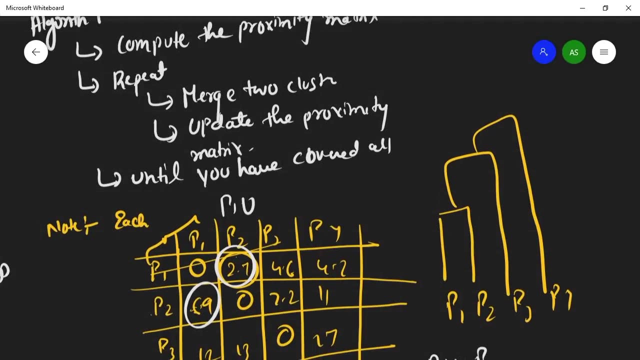 will be seeing one of one of the one of the, one of more, one more comprehensive example. okay, so how do we measure the similarity? how do we measure the similarity of the inter cluster similarity? we can measure the distance between two club, two points or clusters, these p1 and p2, using, maybe, euclidean distance, euclidean distance. 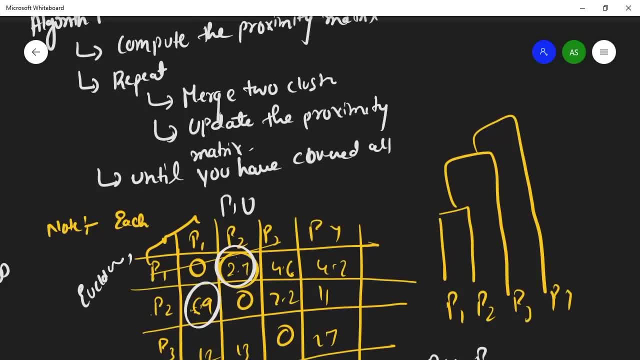 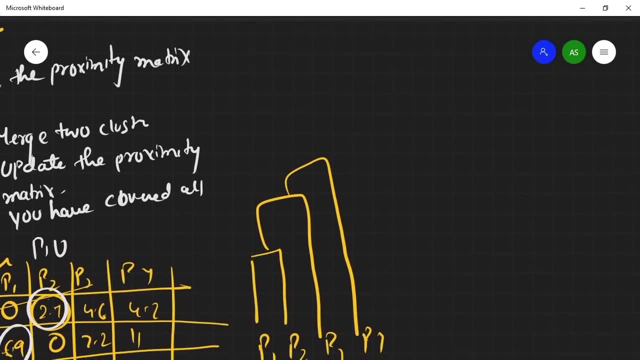 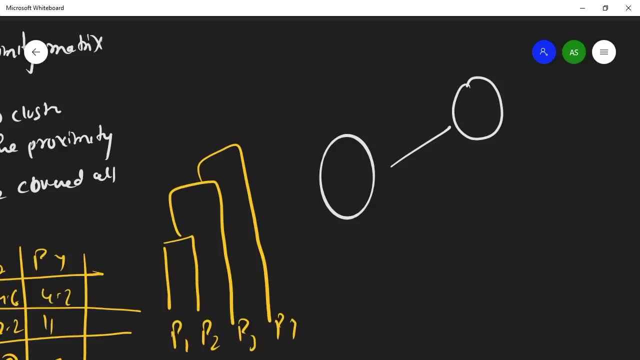 manhattan distance. we have different, different distance, similar. this distance, uh, distance measures. so how do we measure the, the similarity between two clusters or inter cluster? an inter cluster is nothing much. the similar the this: this is your one cluster and this is another cluster. so what's the distance, what the similarity between? to merge it, okay, so 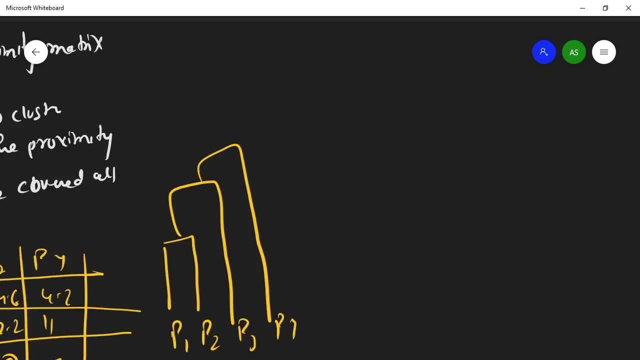 that's the, that's the inter cluster that we have already talked about in terminology sessions. so, let's see, so we have, so we have, let's, uh, let's, let's assume that you have this, let's assume that you have this cluster where we have x, this, this, this, this, this. let's do another cluster, this, this. 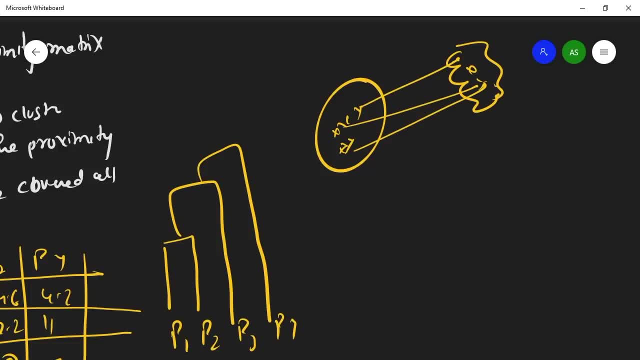 so how do we measure the similarity? how do we measure the similarity? so, for measuring the similarity we have, i'm going to talk about three methods. i'm going to talk about three methods: min. and the next method, max. the next method is group average. the next method is group average. 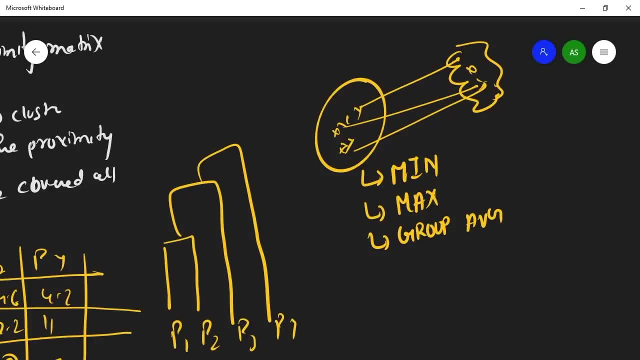 so let's start with min. so what do i'm doing in min? so let's assume that you have this, uh, so so you have this data point like this: we have this cluster, you have this cluster. now the second cluster is like this. second cluster is like this: okay, so what? 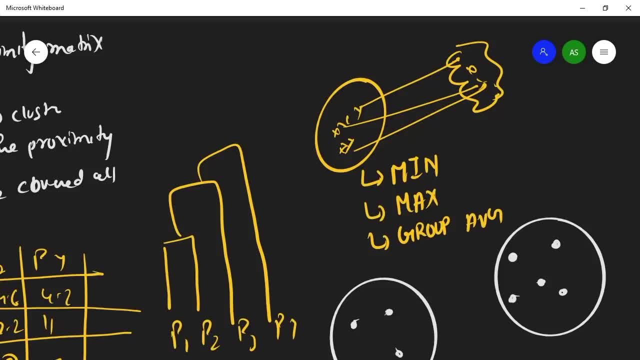 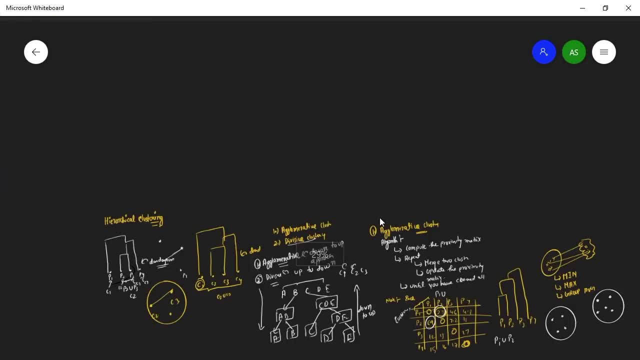 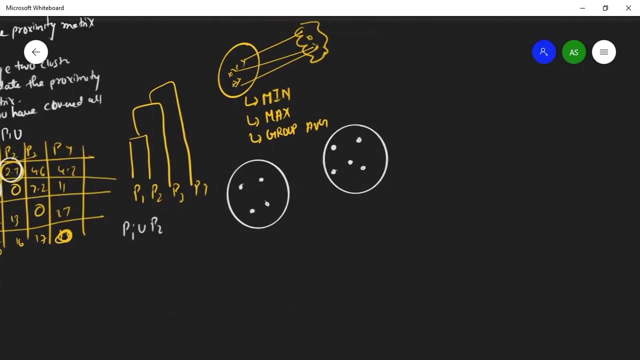 you do in minimum. what you do in minimum, you take out the minimum first to first. um, just just right room. let let me write it mathematically to make it more sense. oops, what i've done, okay, so what? what you have to do, what you have to do? so let's let let me write it mathematically for minimum. 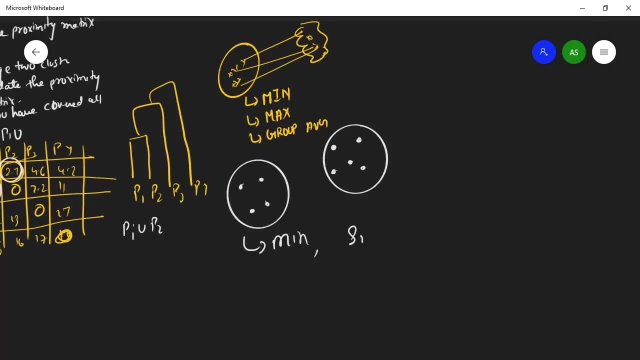 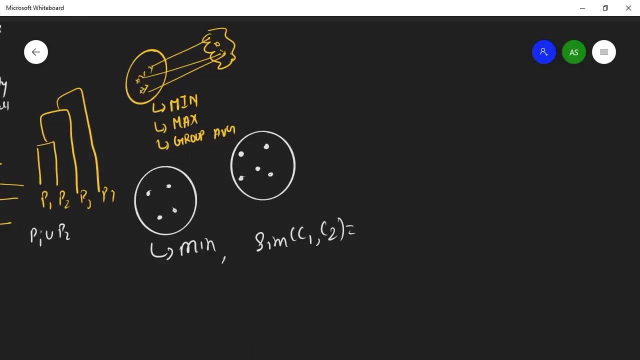 so minimum is is just the similarity between c1 and c2, which is nothing but equals to nothing but equals to minimum. minimum of p. i is mem member of c1 p i to be the member of c1. let's assume this is c1. so 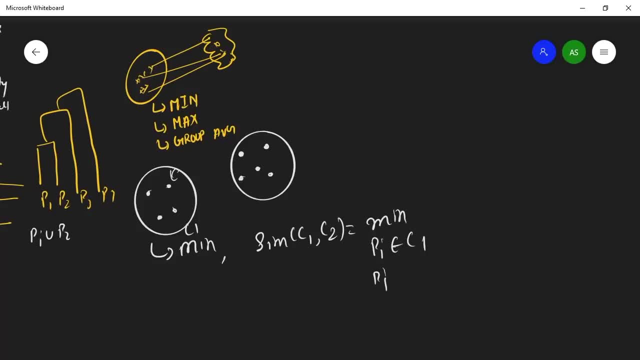 p, i may be this point- and pj, the another cluster, should be the member of c2. now, what you will do? you will take out the similarity, this, the similarity between c1 and c2, and this is the similarity of p, i and pg. okay, these two. okay, these two distance. okay, now you take out the distance. 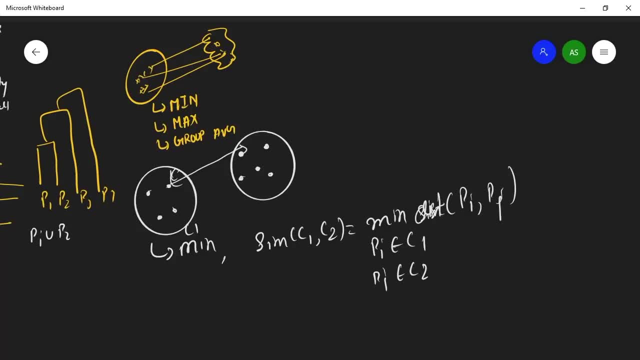 that you do. you take out the distance, i'm striking your distance and you, you take out the minimum point, minimum points. who have means here? you would this. the distance between these two points is is minimum as compared to this point, this point, this point. okay, so we will. we will, uh, just uh. 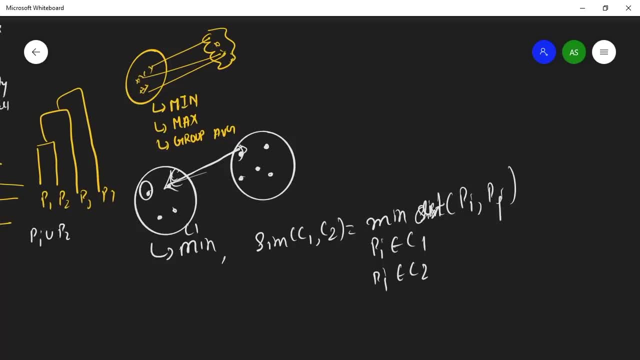 what? what we will do? we will simply, uh, merge it okay. so this is what the basic minimum, uh, minimum- approach does. it just takes out the similarity between c1 and c2 by the taking out a minimum of all the i and j's, by taking out the distance. 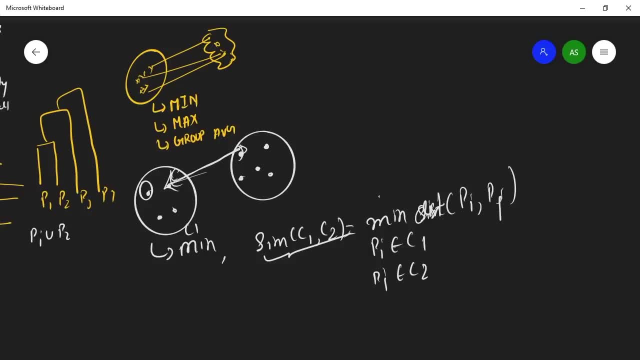 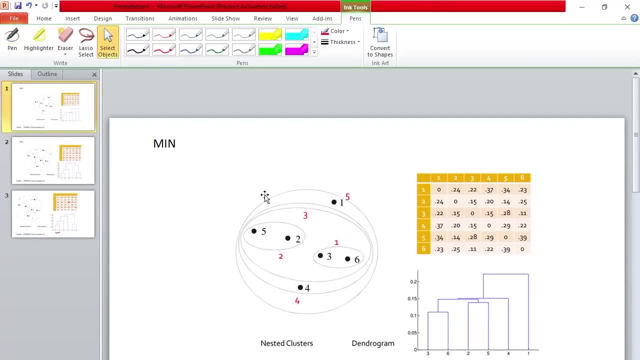 between all the minimum, taking out the minimum distance of all i and j's with a member of c1 and c2. okay, so that's the, that's the minimum. so let's see the basic, basic thing over here to under understand it a little bit further away. and this, this is the. 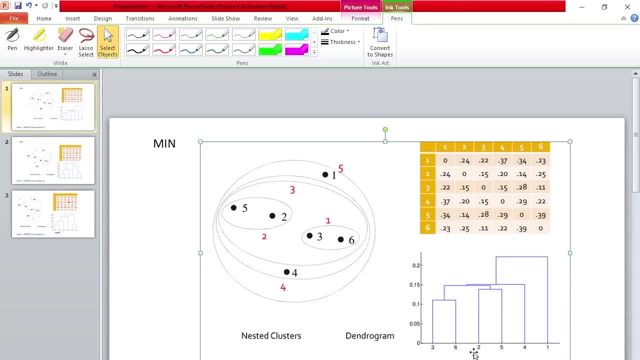 this. this example is taken from cs6530 by claustroanalysis class lecture notes. this, this, this example, okay, so here, here is your proximity matrix. here is your proximity matrix where you have one as a p12, as a p2, like that. okay, now you have the. here, you have a proximity matrix, here you. 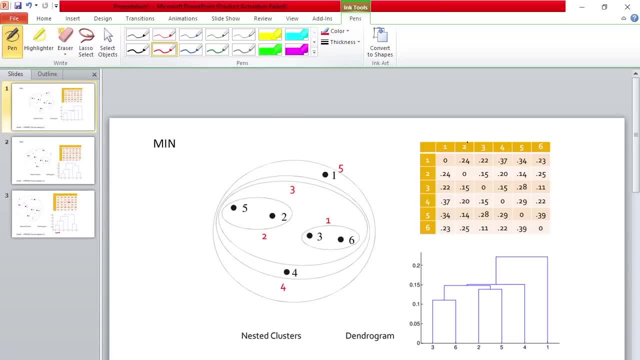 have a proximity matrix. now here, the distance between one and one is zero. the distance between one and two is the four point twenty four. the distance between one and three ends one point two. the distance between one and four is 0.37. the distance between one and five is like this and: 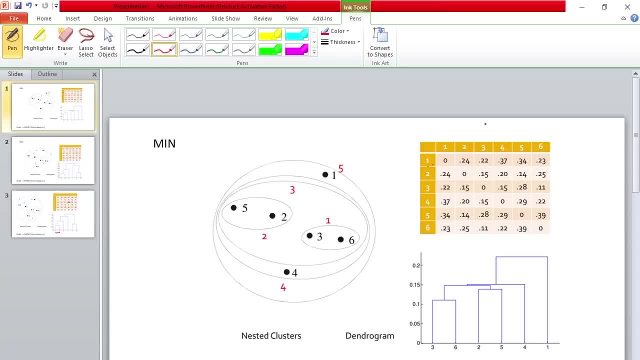 this in the same diagonal- are zero. okay, so you can see here the smallest similarity between, or smallest distance between, two points, i and j. here we have- let's assume this is i and this is j- the smallest distance is point eleven. point eleven and we have three and six. okay, so we merge three. 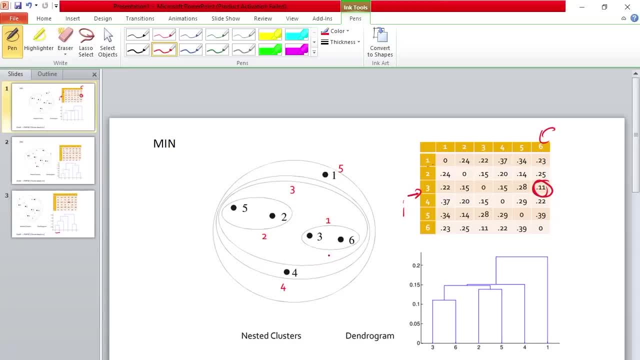 okay, now the next. now the next smallest similarity or the smallest distance is: is, uh, this one, uh, let me choose. yeah, this, this one, point fourteen. okay, so five and two. okay, so this is your next smallest. so now what you will do. you will merge it at the second cluster now. 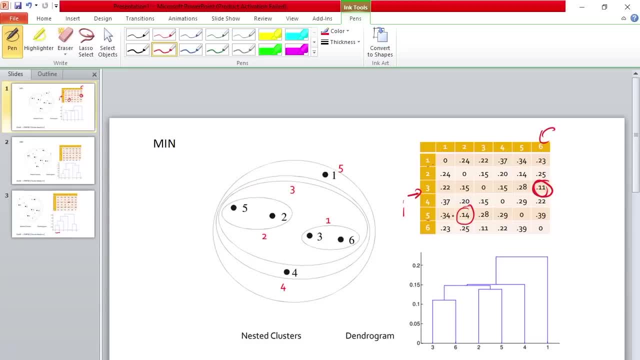 what you will do. you will find that this to cluster, this to cluster you, and this, this p five, union two and, and three, union six finds to be, uh fine, um has the smallest distance, so you merge the cluster three. next is you have one, you have one and four. now what? what you do? you? this first, 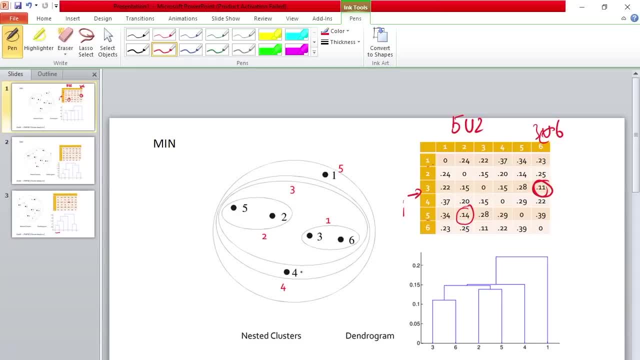 you take out the, just you, just, you can see. first you take a first. here we have four in which the this union, union and this four, and this four has the smallest distance. so you merge it at the first and then you make a big cluster again and then you are done. okay, so it might make sense, it might. 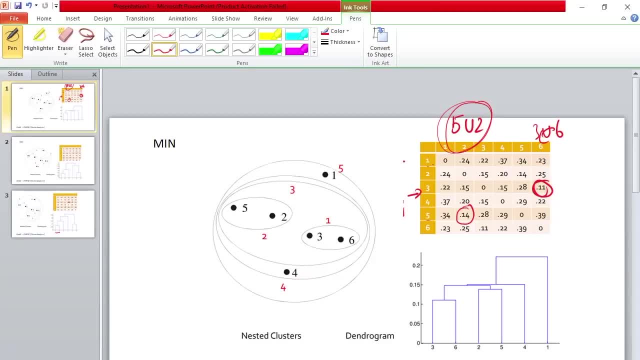 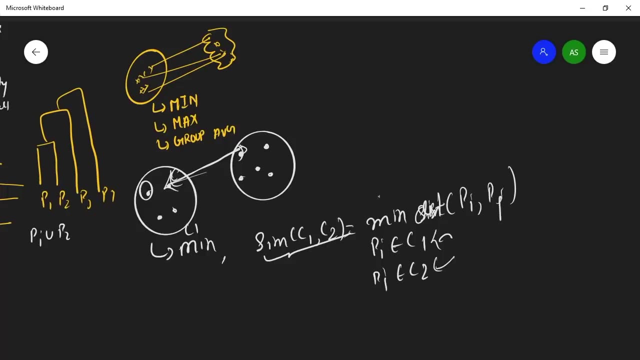 not make sense further, but i will walk you through. go through this example: make the dendrogram by yourself or necessary clusters by yourself. okay, that will make more sense. the next type of this is max. what do i mean with max? max is simply. max is taking out the similarity between c1 and c2, which 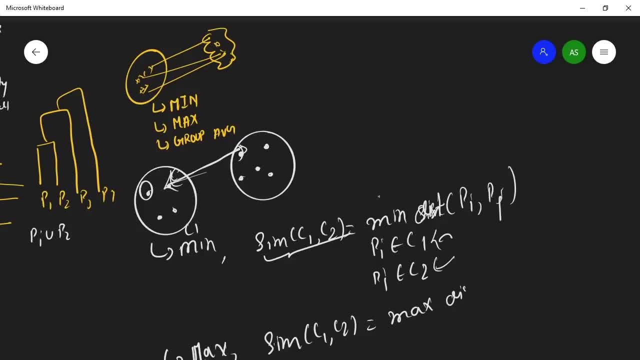 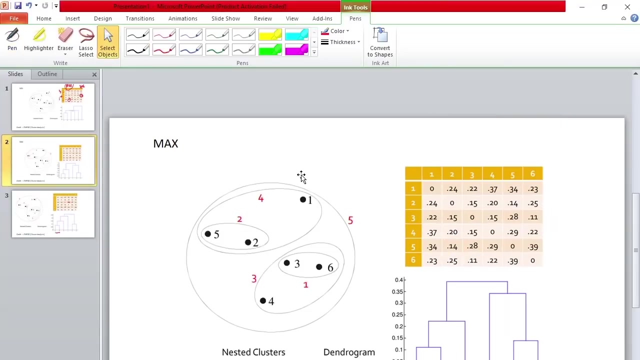 is the maximum which we want, the maximum distance, maximum distance between pi and pj, and pi be the member of c1 and pj pj may be the member of c2. so that's the. that's the basic definition. uh, that's the basic of this. instead of, we are taking the max. so what do i mean with max? so here we have an. 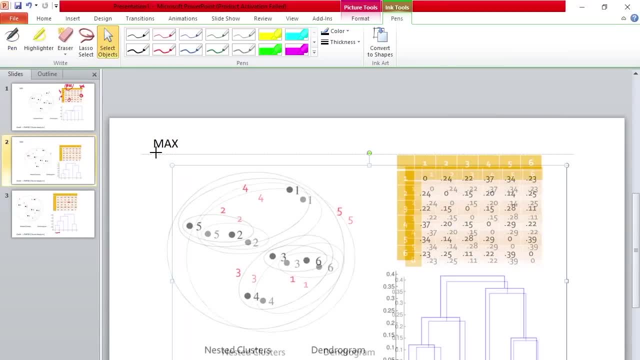 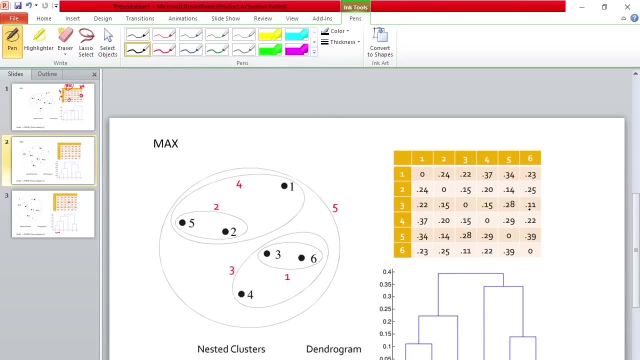 intuitive or a comprehensive example. so here you can see that we have again the same proximity. now you can see that the smallest distance is three, six, okay, you merge it. now how you will merge this four, how will more? why? why don't? don't we merge with five? okay, so the distance between 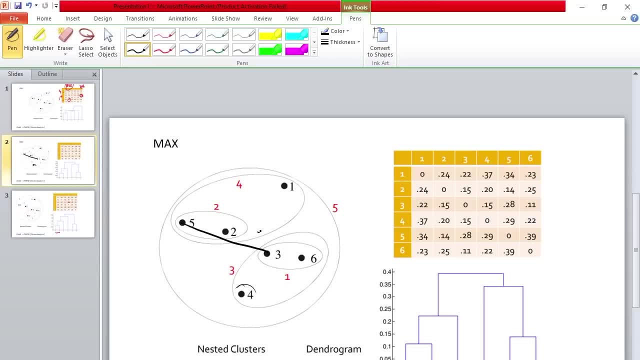 the distance between this five and two is a maximum. it's very large. so obviously, this, this one, obviously will be minimum. so you merge that. that's, that's makes sense. that's makes sense, obviously. okay. so this, this is what why you are you, you take minimum distance, but for a merge. 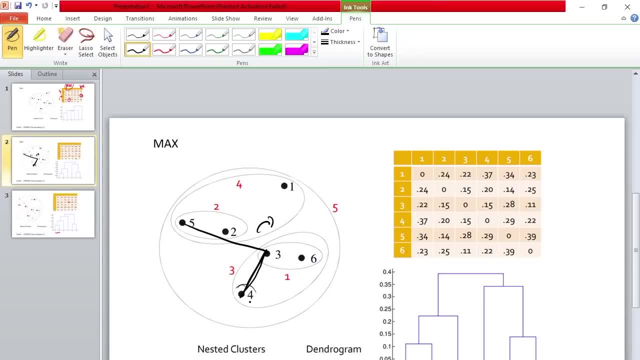 you take out a maximum, you take out the maximum to merge, and here you have taken the maximum. and that's how, and that's how, and that's how all it works. and here we have a maximum, here we have a minimum. so you take out a maximum and then you 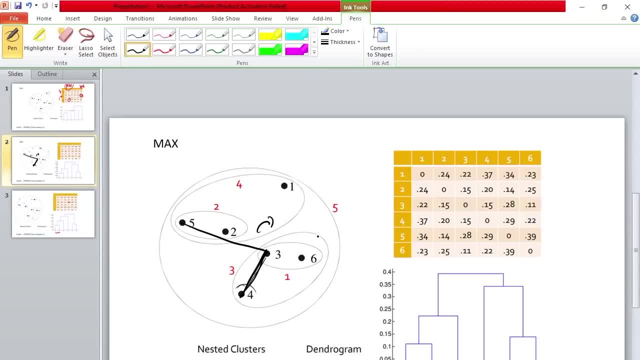 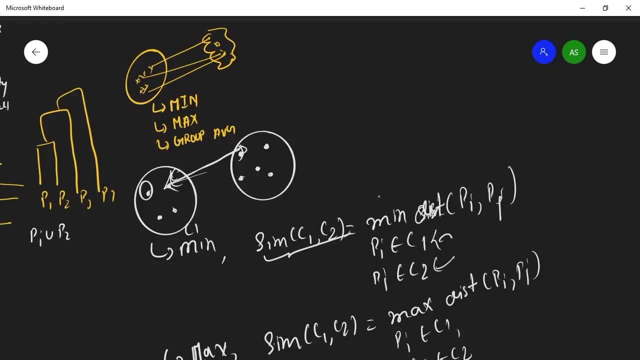 compare and then you take out a minimum and this is obviously will be minimum and then you and you can see this is the maximum here and this is the minimum from here. so you more shit, okay. so this is the basic and you can see the dendrogram over here how we made, okay, the next type of inter cluster. 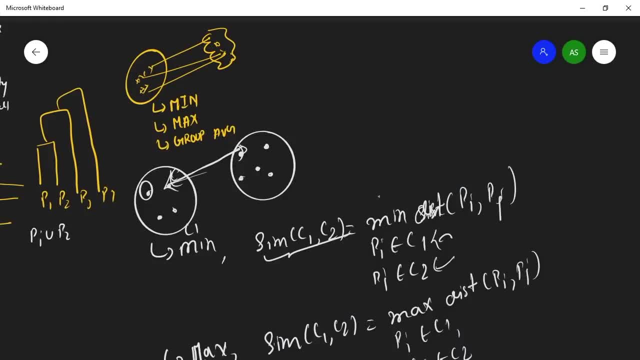 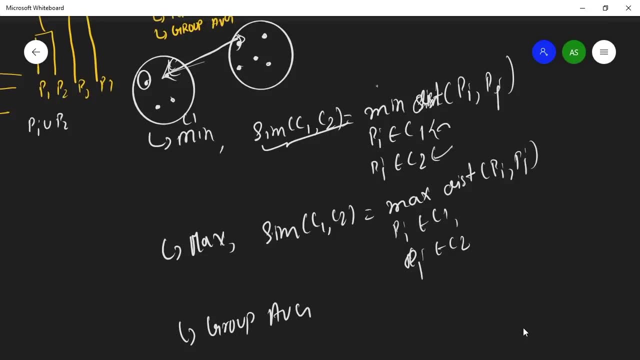 similarity measure. the next type of inter cluster similarity measure is a group average. what do I mean by group average? group average. so I'm just going to give you the intuitive, just as a simple equation, which is: PI with a member of C 1 and PJ with a member of C 2, PI with a member of C 1 and PJ with a. 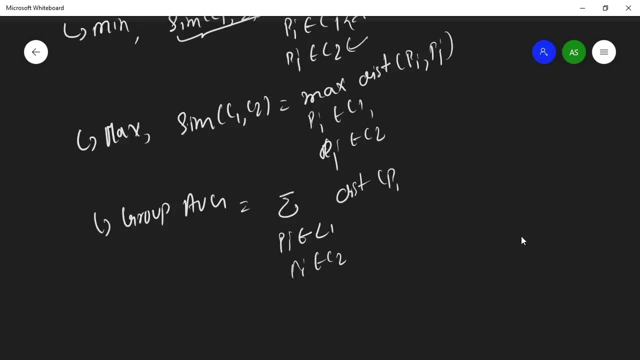 member of C 2. you take out the distance between PI and PJ divided- divided by the norm, because it's the fake frequency, divided by the norm of C 1, with whatever the number of points times, then I think, times the norm of C 2. okay, so this is. 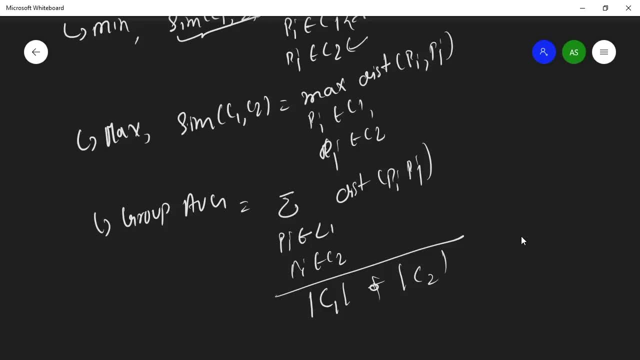 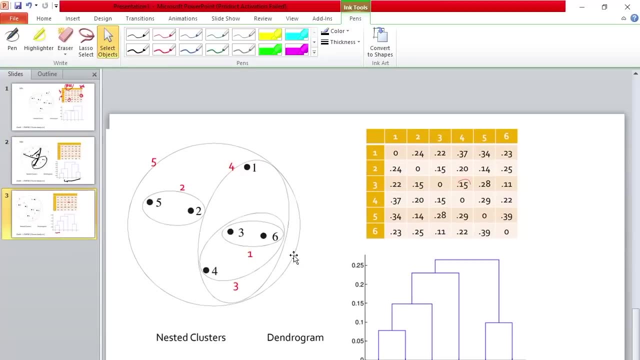 what you have to do, I think, is be a tip: maybe plus, yeah, it did. maybe plus, yeah. I guess we take out the norm of what is number of points, free frequency. okay, that's what you are going to do, so you can see over here that we have this. 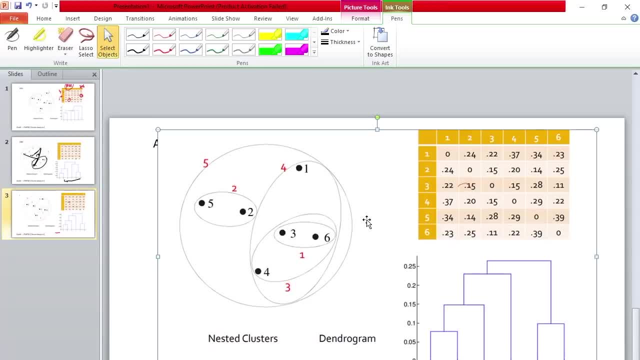 tender gram. we have this following. and then what you do? you take a new group. you group it little for, for example, you can see the same thing has been done. but I'm going to take another example to help you understand this much better. to help you understand this much better. so you have this first, and then you have 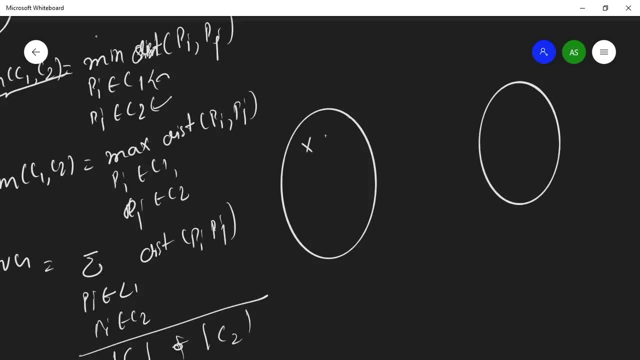 this second cluster. okay, now you have some points, we have some points in here, you have some points in here and some points in here. okay, you take each pair, you take each pair, each pair like this: you take each pair, okay, okay, then average it out, okay, and then you take out the distance, average it and then 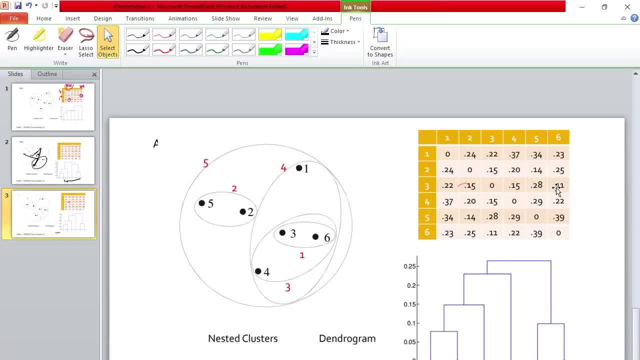 here you go, okay. so for an example, here you take out them in, the minimum distance is three and six, and then you have this four. then again you merge it using the and that's what what we, what we were doing, but here we are merging one, also, the reason being the average between will, it will, will be making 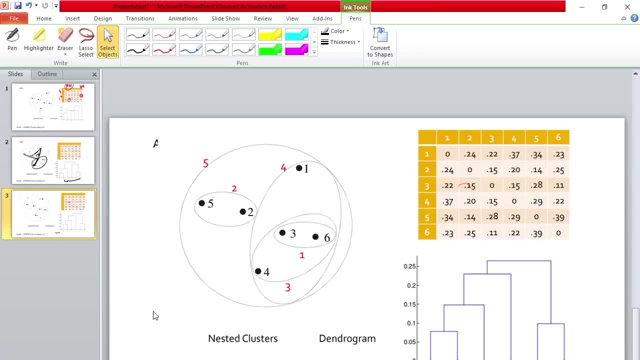 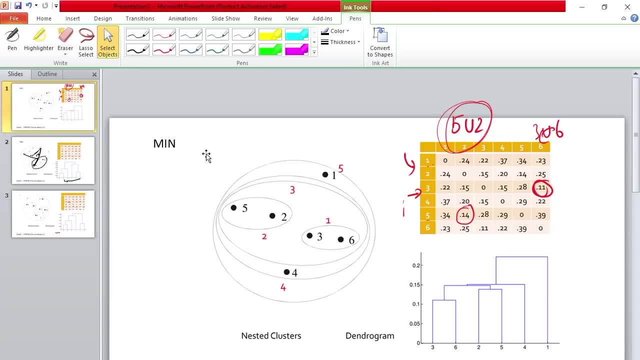 sense, if you sense it mathematically, okay, even to our closest, okay. so this is what you are doing in group min and let's see some of the some. just this minimum, this at this disadvantage, that minimum disadvantage is it. it simply did it, it is. it is sensitive to outliers, it is. 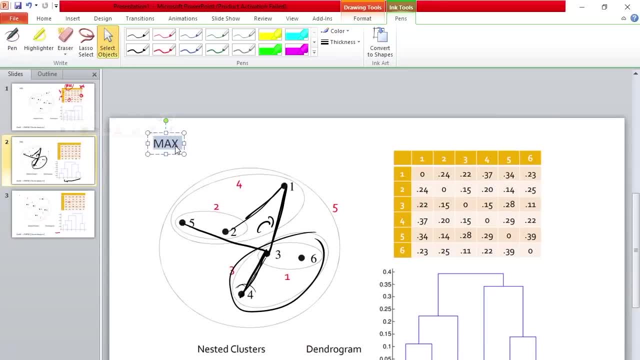 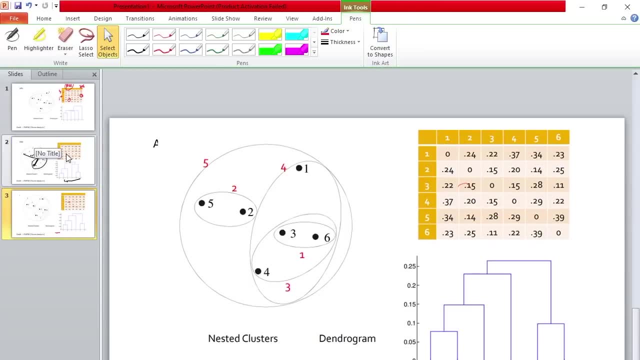 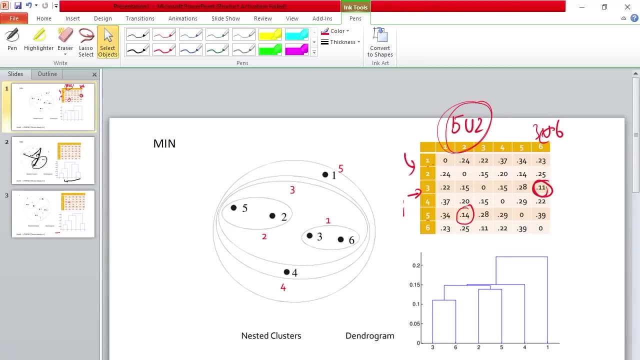 sensitive to outliers and bad wrath rather than max is will, will be less prone to outliers. okay, so that's the basic and this disadvantage that I've told to you, and you can see more on the CS six, four, fifth, five thirty cluster analysis lecture notes to understand it much better. okay, so this is what we are doing and if you have not, 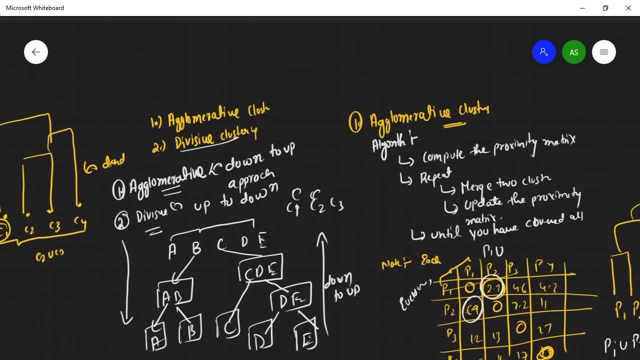 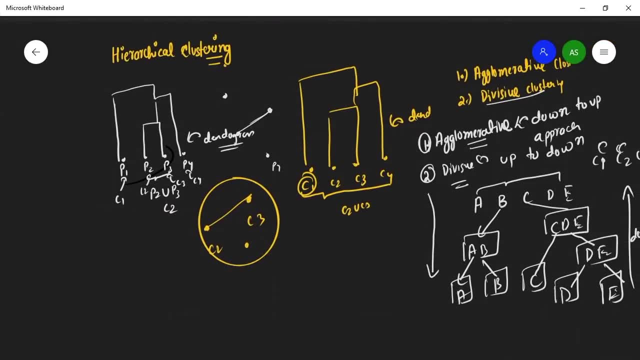 understood. it is a little bit advanced, but it it should make sense little bit what, what we do, what we do in this. we have make hierarchical clusters like this. okay, so now we have talked a lot about the hierarchical clustering and I hope that you really understood everything you need to know about. 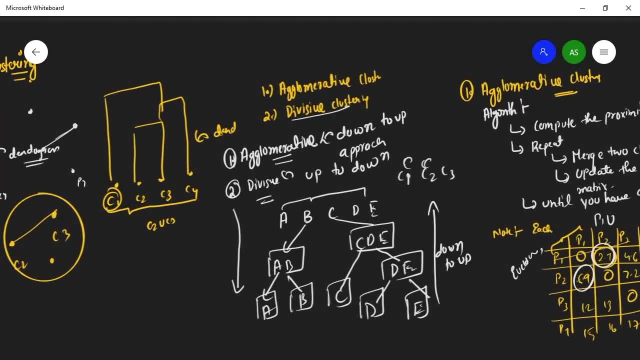 hierarchical clustering. now what I will do. I will just name some now. name some Now what I will do. I will name a time complexity and a space complexity. Now I'll name one time complexity and a space complexity for agglomerative clustering, just to make sure everyone is on the same pace. 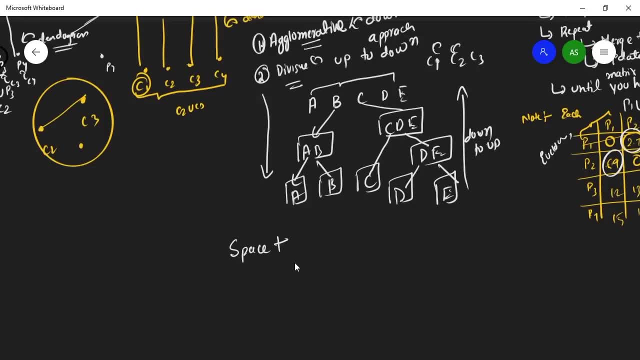 So the space complexity is order of n square okay, because we have approximated matrix 2.. And time complexity will be order, or maybe sometimes it's order of n cube- okay, But sometimes it goes to order of n square, log of n- okay. 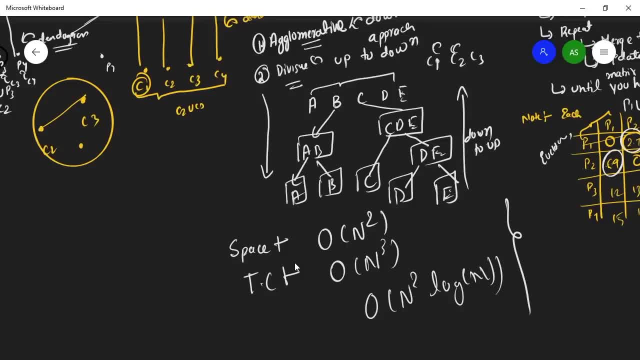 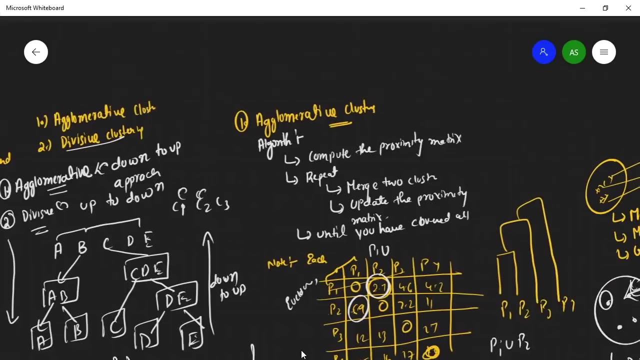 So this is your space and time complexity. to understand it much better, And you can see the limitations, pros, cons of these onto the Wikipedia pages. They are really well explained there. okay, So we are done with the hierarchical clustering and I really really hope that you understood everything. 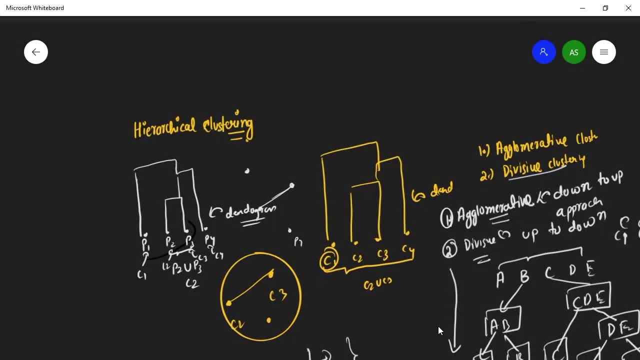 Now we are done with unsupervised learning. Now we will do logic, We will do a lot of process and then we will end up this course And I highly recommend you to do lots of projects also, okay, And then, after learning this machine learning, you can go to New Era. 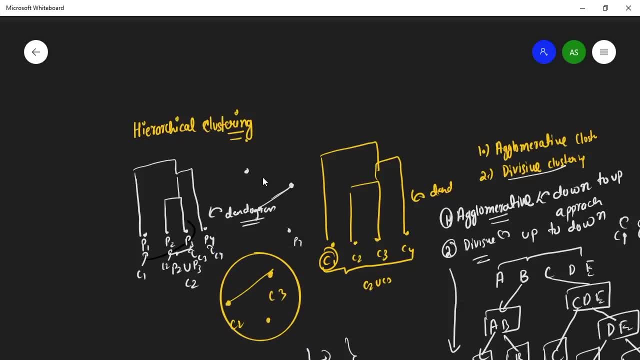 Again, I'm going to just navigate here the URL, https. you can slash youtubecom, slash New Era- okay, So you can find and just take a look at a newly launched deep learning series, okay, And from there you can learn advanced. 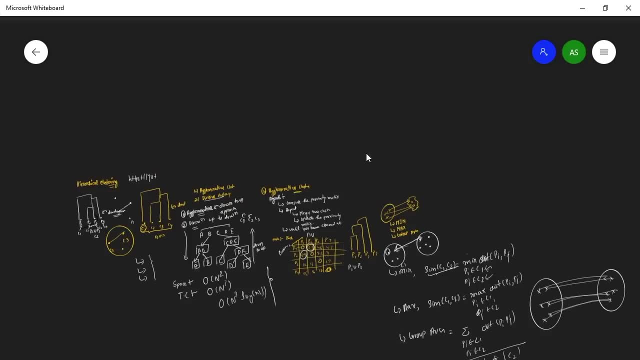 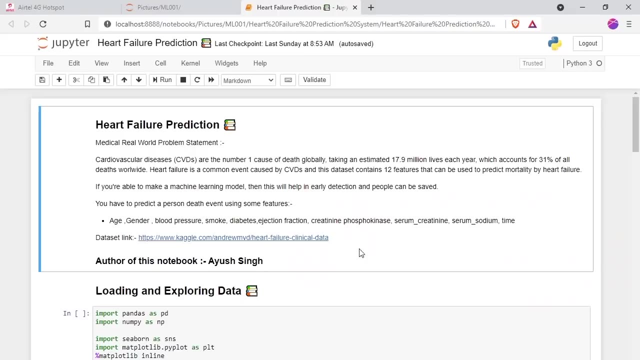 You can learn advanced machine learning or deep learning. okay, So that's it for this session. I'll be. so that's it for all this subsection. I'll be catching up your next section. Okay, so now we will build or start our last section of this course, which is project section. 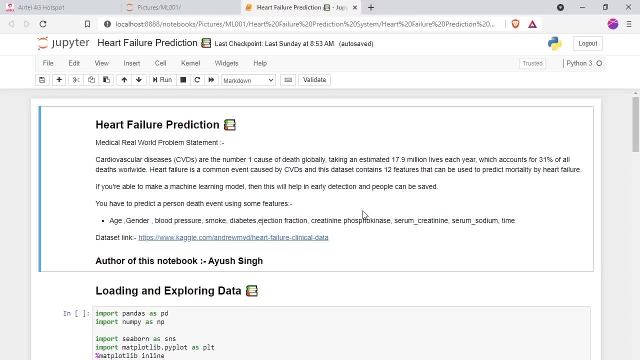 And in this section we will build two projects. maybe some more projects, But initially I planned for two projects. Maybe I can add more, But you can surely go to my YouTube channel For more projects. But these projects will tell you an overview of how a machine learning project would look like. 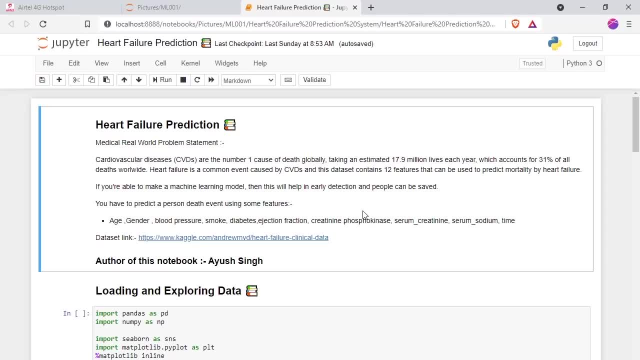 And the motivation for starting your new project, Because it's better to make your project by yourself, Just taking the inspiration from other people. okay, So in this project we will build a heart failure prediction model That will predict whether the person will die based on some of the features or not. 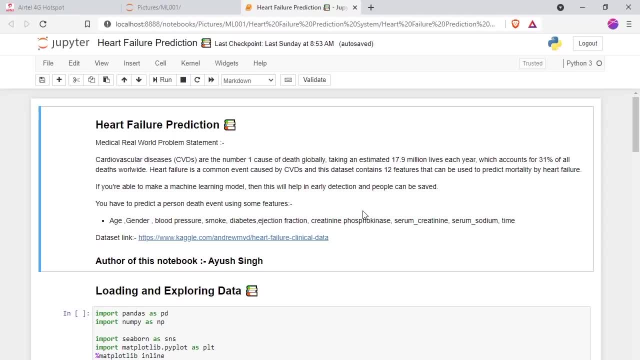 Okay, So this is the problem statement, And we have certain features like age, gender, blood pressure, smoke- whether a person has smoked or not, whether a person has diabetes or not, what is the injection fraction, what is the, and such. 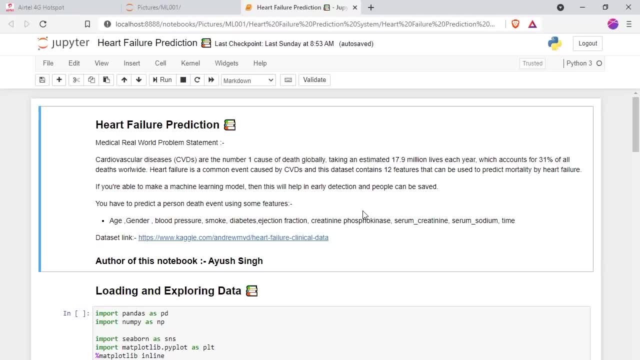 There is a long name which I can't pronounce, But this is the. this is a problem statement And I'm going to take a look at the data. I'm going to take a look at the data which is available at this link. 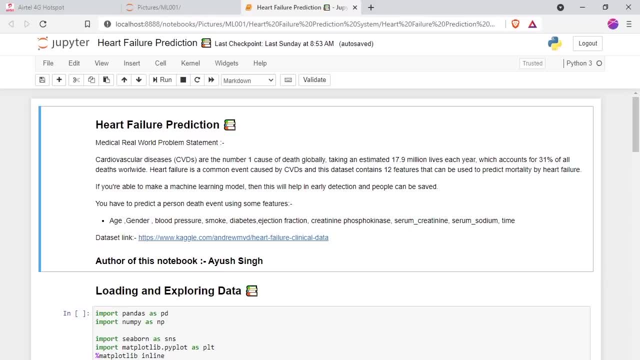 And I hope that you will understand. Okay, And I hope that you will understand this project. I have, I have made, I have I have run step by step to help you understand everything And as I have made, just I have not worked on this project. 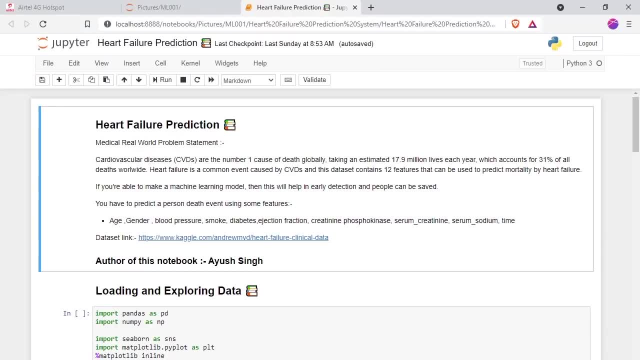 So I just want to pick up this heart failure detection system just to make sure that I will be making my own project also- And it will be- and narrating over through this project. Okay, So here, what I'm going to do is what I'm going to do is I'm going to make a heart failure detection based on these features and the target variable. 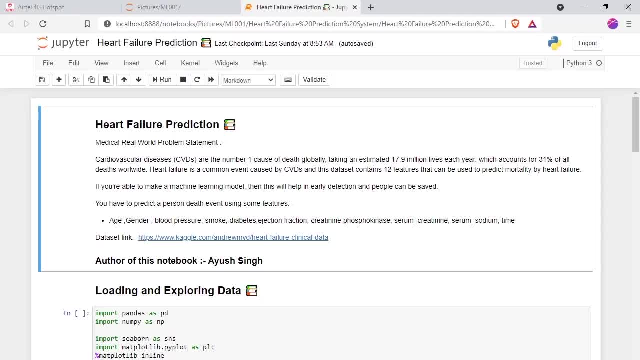 So I'm going to pass these, I'm going to pass these tags And I'm going to write a little dot And then I will take all the and I'm going to pass daily red tags on top like handheld tags. Okay, 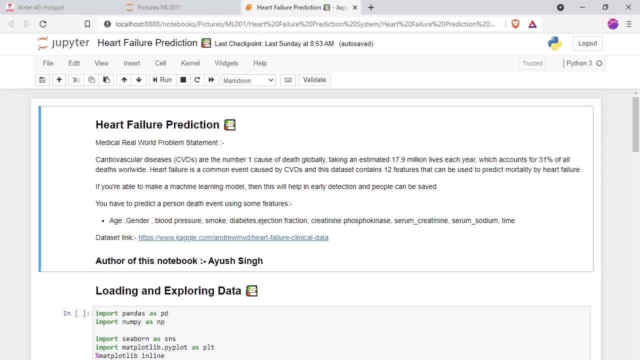 But what I'm going to do is I'm going to assign that category to the International Provincial University Okay model that will help you in early detection of the person based on particular features and help the person can be saved. so that's why we are going. 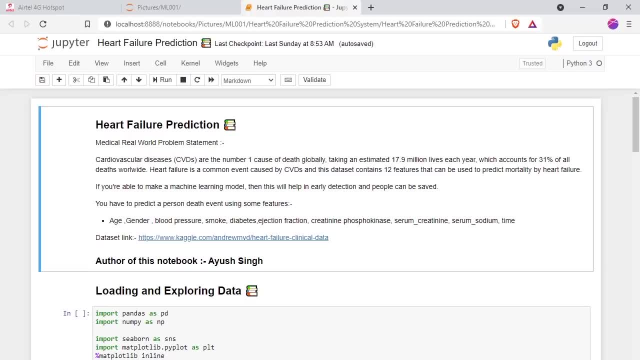 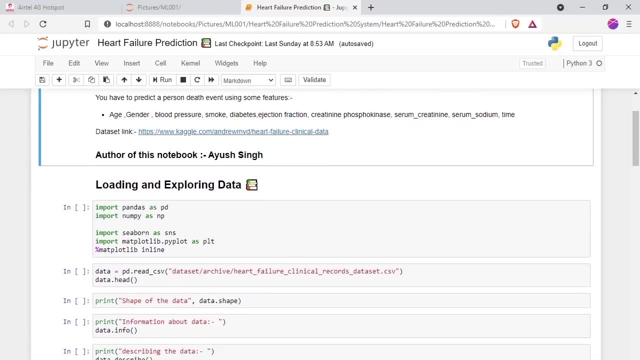 to build that model to help you better understand the AI healthcare. we'll be building one more project, which is spam detection system, that is, whether the email or messages are spam or not. okay, so let's start with this notebook and first of all, I've divided. first of all, I'm going to load the data and sorry. 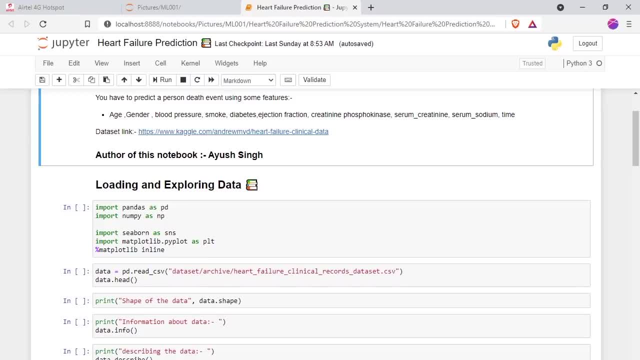 load those or import the libraries. so I'm going to import pandas, numpy, seaborn, matplotlib and this. okay, so I will run it down, I will run it out and then I will load my data. so I don't know why the second time. so now I will load the. 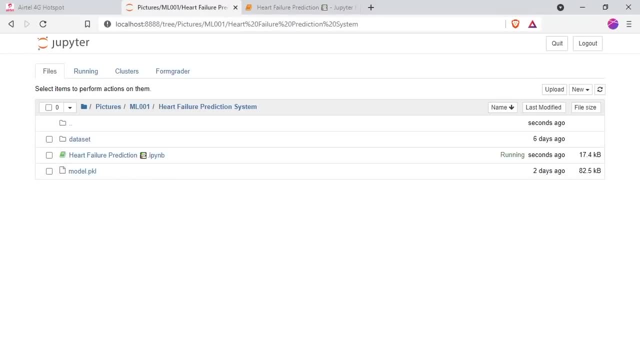 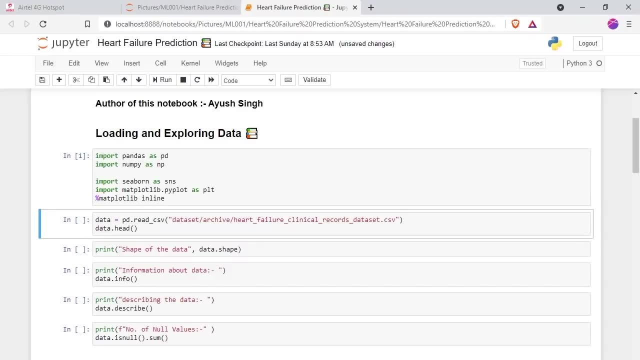 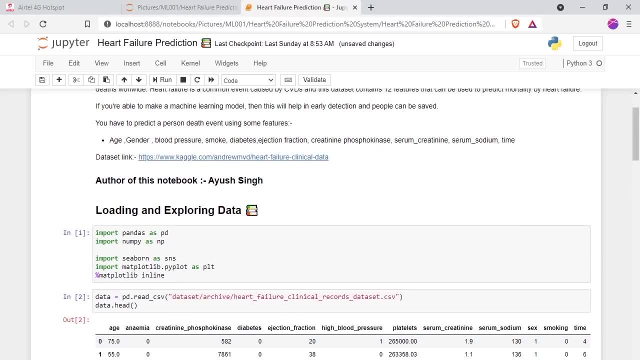 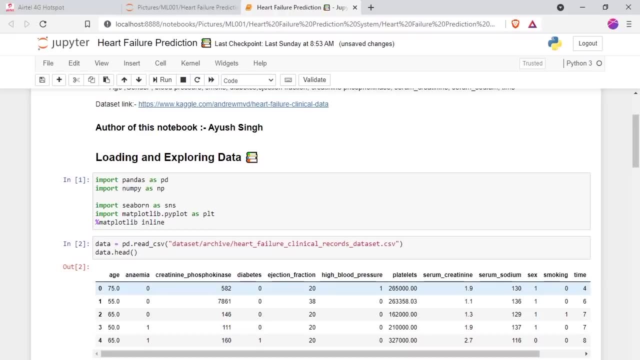 out head. and one, one more thing that I'm to clarify over the reason why I'm not writing or coding by it here, because I thought like it will be better if I narrate the code, if I can. if I'm writing the code, maybe I forget something, or 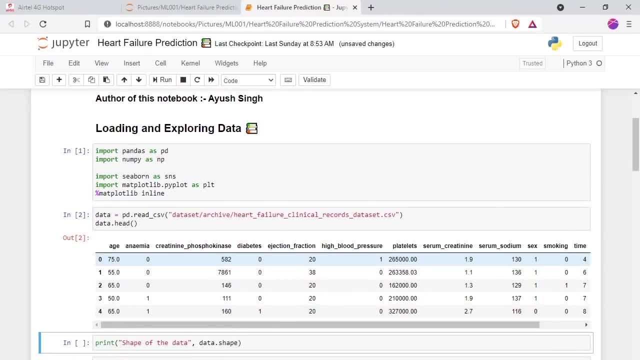 maybe the code is not annotated too much. so that's the for a few further references. I just took to just write it down over here and then I'm only going to just an add it over there. okay, most of them because, because maybe while writing the code I may forget to narrate some of the code. 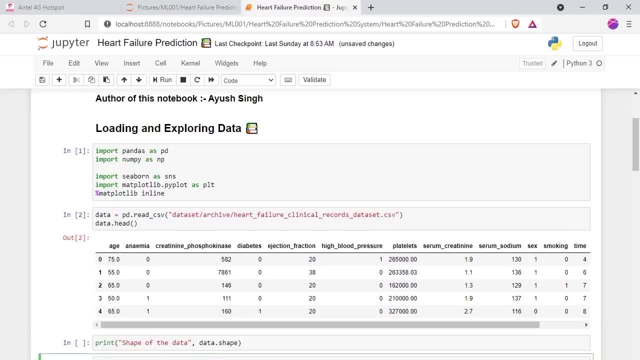 but yeah, let let me know what you like, whether I should write a code or not. okay, so I'm going to print it out of the shape of the data, and one of the shape of the data is 29913, which is 13 columns, and here we have H anemia creatinine. 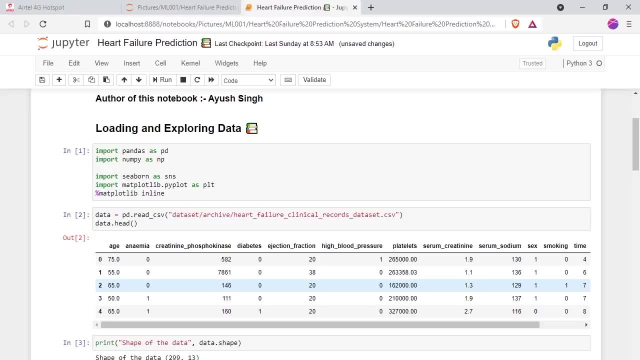 phosphoquiness, diabetes, injection fraction, HP, then battle it serum. then what is the gender, smoking time and that even okay, and that event is our target variable that we need to detect, okay, so that's our basic intuition, that's our basic data exploration. now I'm going to do is we will see how much the data we 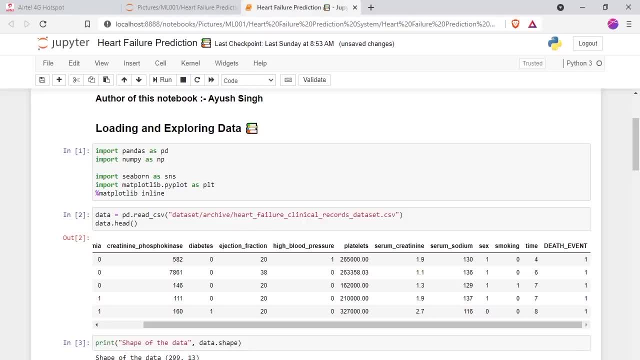 have means we will see what's the shape of the data we have. so here we are, given the shape of the data, which is two, nine, nine rows and 13 columns. okay, now using day data, don't shape, you can do. now I'm going to take a look at the 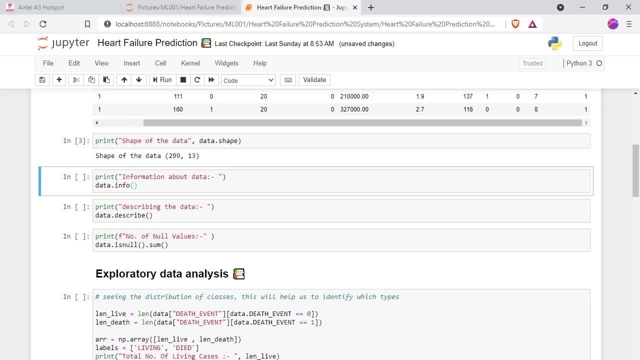 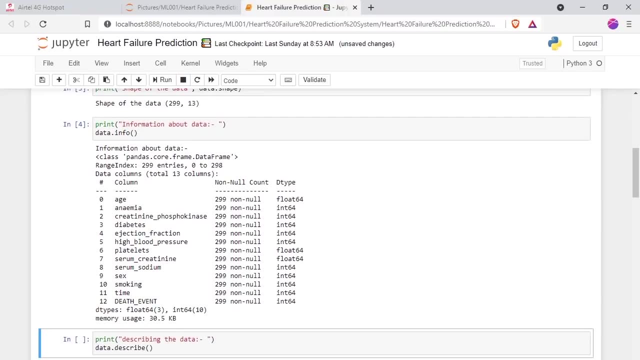 information about the data. you can calculate or you can take out the information from about the data, from the data to info method, and you can if you steel. we hope that it will tell you whether the particular column has no values, what is the data type and what is the memory usage, and it will also tell 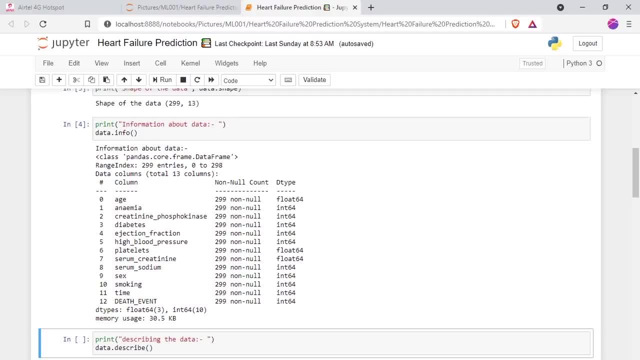 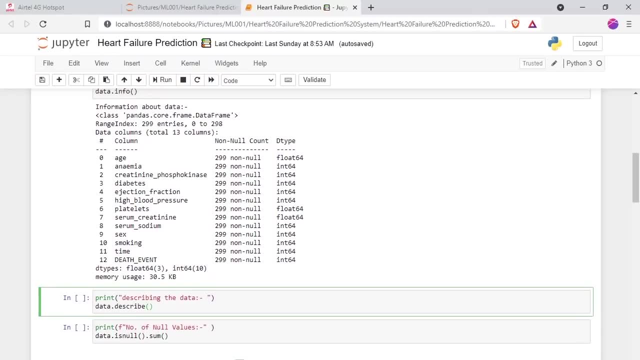 you what's the shape of the data data. by just taking, you can also take a look at this and you can see that it starts with zero indexing. so we have 13 columns. you can also take a look at the description. it will simply tell you whoever is the numerical column. it will 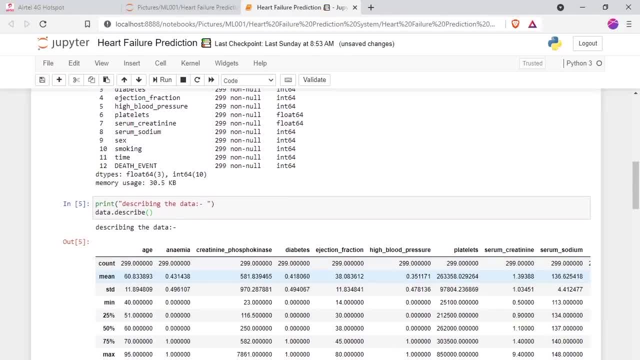 tell you the describing means. what is the count? what is the mean of the particular column? what is the standard deviation? what is the minimum? what is a 25% of that column and 50% of that column and 75% of the column and max in. 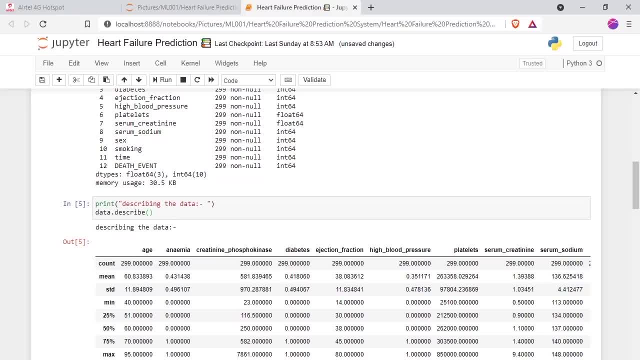 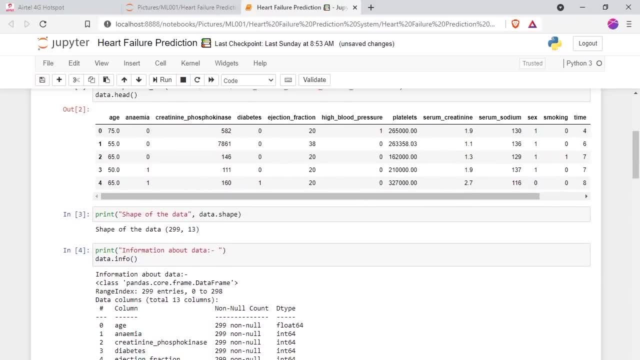 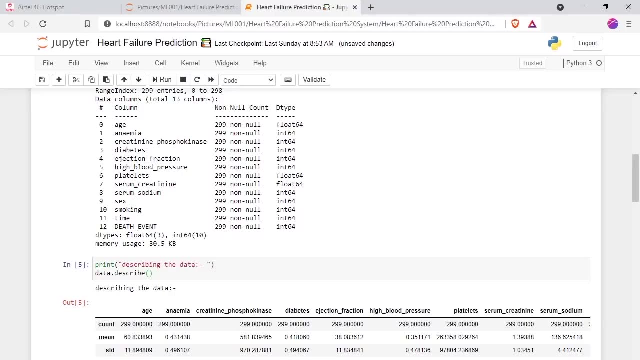 that column, it will surely help. and photo means when it's a data scientist, it will surely help. maybe something that you are exploring: what's the maximum? you can take a look at this. you can take a look at what is the standard deviation, what does it mean? maybe you're formulating some problem based on. 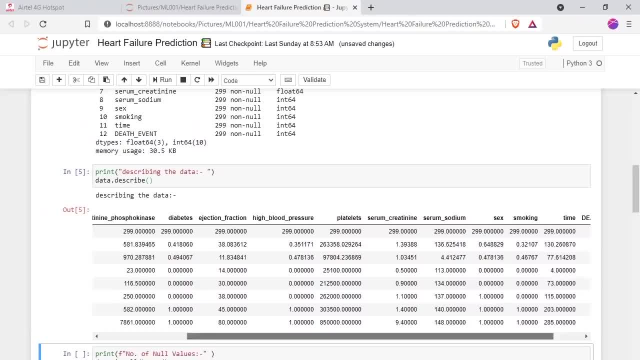 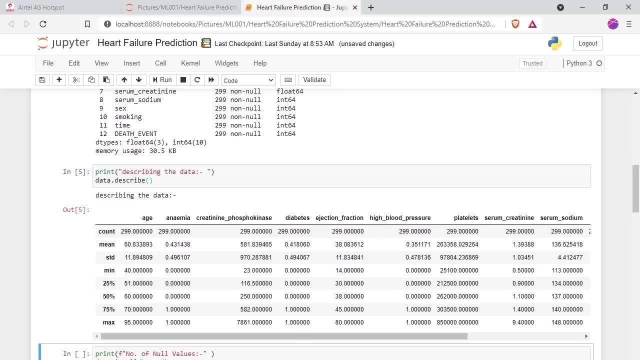 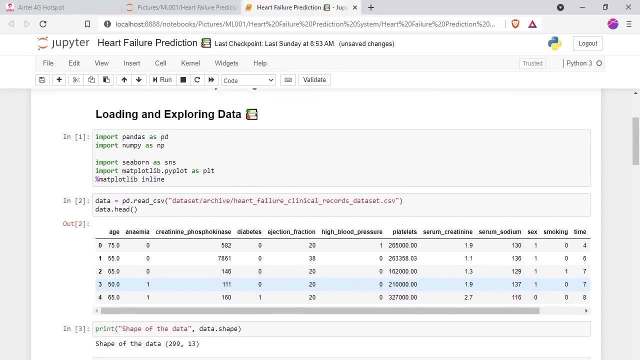 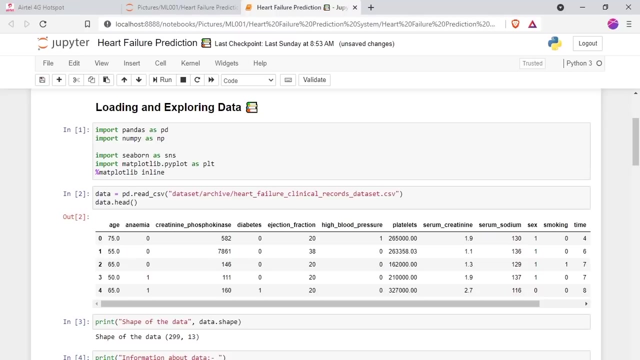 machine learning. so it is very helpful. this: there's a data frame you can do, can have a day, spend five minutes understanding what, what space, and it's very easy. it will tell you the count, minimum standard deviation, etc. Okay, so what we have seen so far, we have loaded, we have imported the libraries, we have loaded the data from a local directory. I'm going to take a look at the shape of the data and I'm going to take a look at information about the data. 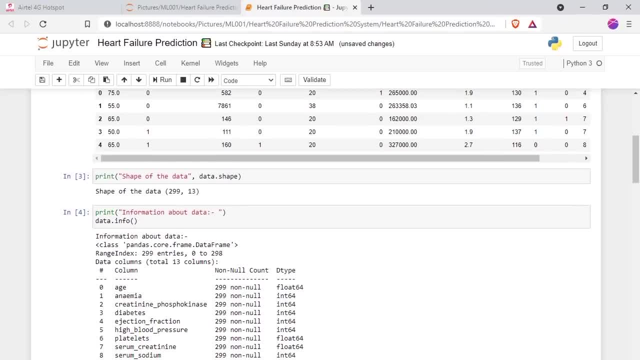 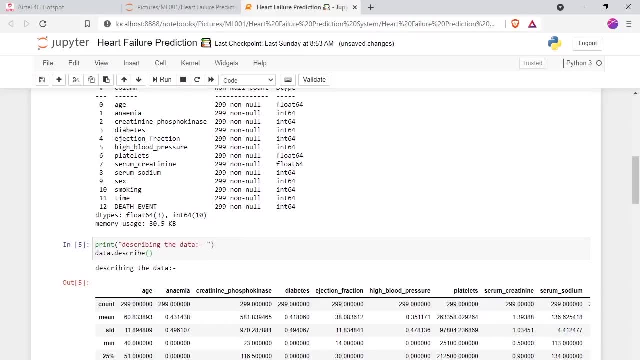 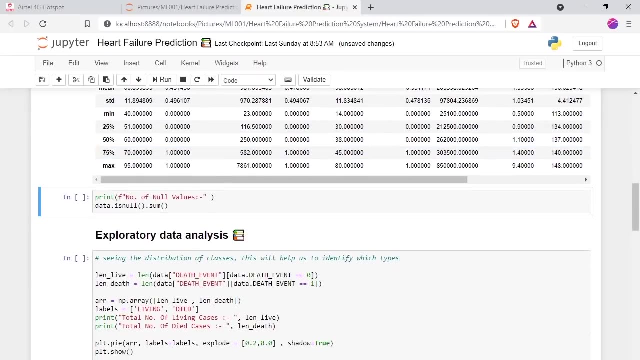 Okay, so here I'm going to datainfo and that will give me the information about the data. Okay, then I'm going to take a look at the distribution. what is the? it will describe our numerical data, and then I'm going to take a look at what is the number of null values. 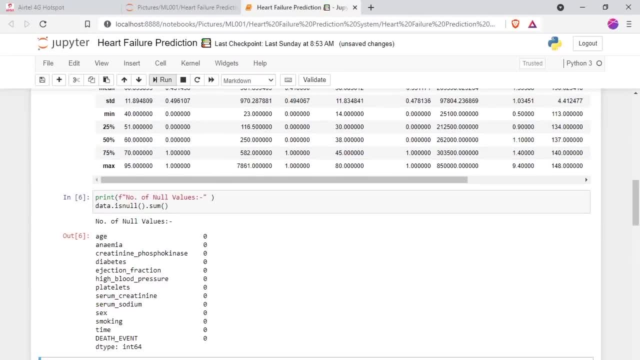 So here, this will tell you, this will tell you in all the columns how many number of null values are, and here we have 0,, 0, 0 null values in each and every column. Okay, but if you let's say, let's say, let's take an example that you want. no, I don't want this. 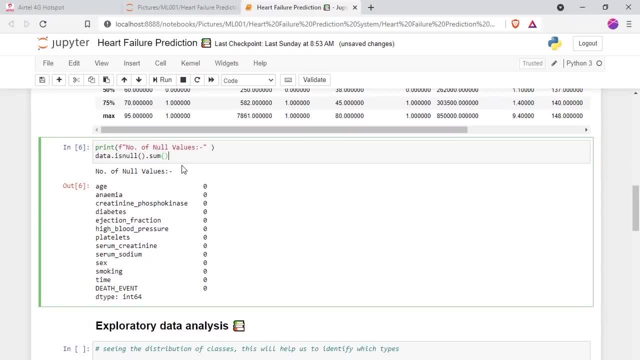 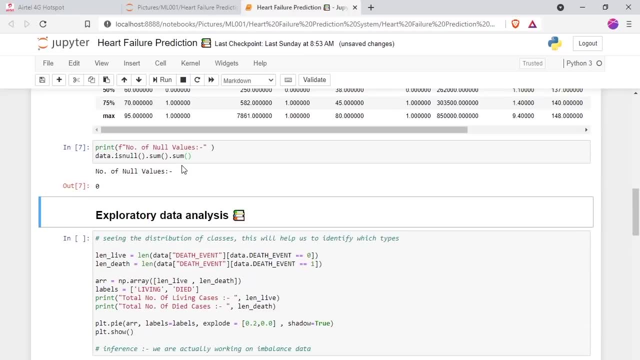 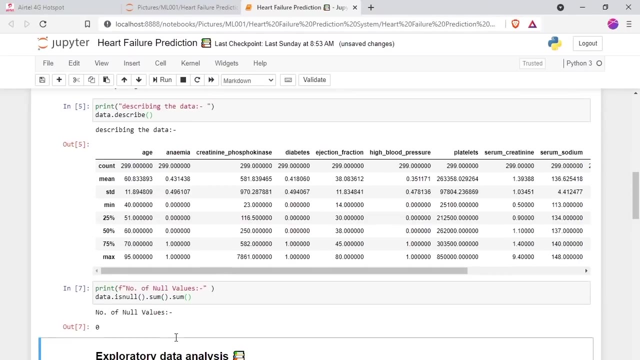 I just only want that: how many, how many numbers, so you can add a sum and then you can run it down to see how it works. So you can see that we have a total of 0, null values. Okay, so this is the basic exploration, as I can do about the data. a little bit of exploration about the data. 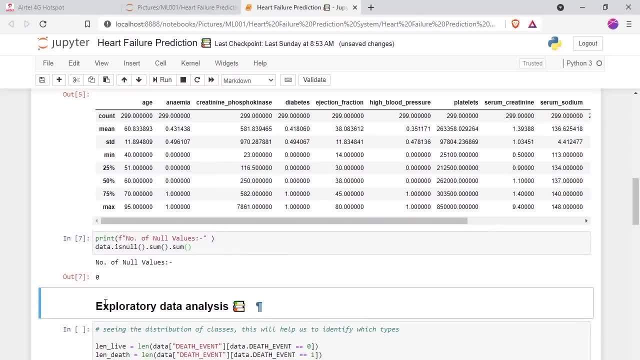 Okay, now the main part will come in exploration data analysis, when we do the so much of EDA and a lot more. So we will see how we all have We do the exploratory data analysis, and here, what do I mean by exploratory data analysis? 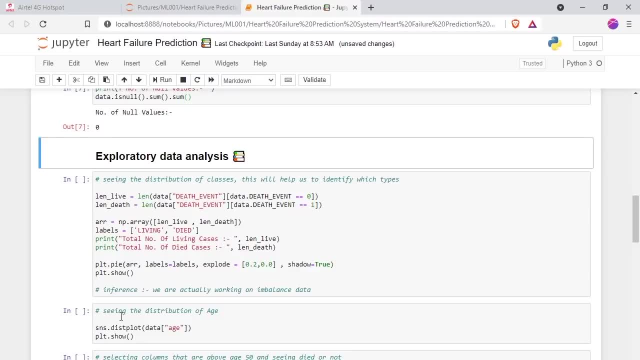 In EDA. it does not mean that it is a very, very hard, but it does not also mean that it is very, very easy. It's a very, very crucial step in machine learning. You should know your data, how it is working, what's the what's, the distribution of the data is the data is balanced? 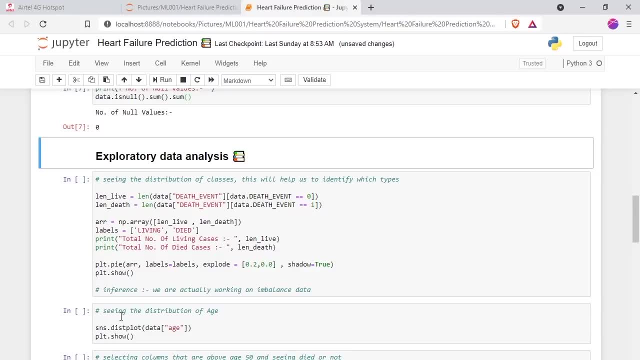 You have certain question to ask, which we will see over here. Okay, so you have certain questions to ask. You have to use some data that should be your, that using maybe some plots, maybe some numbers- We'll see that- and you have to find answers of your coach, of your company. 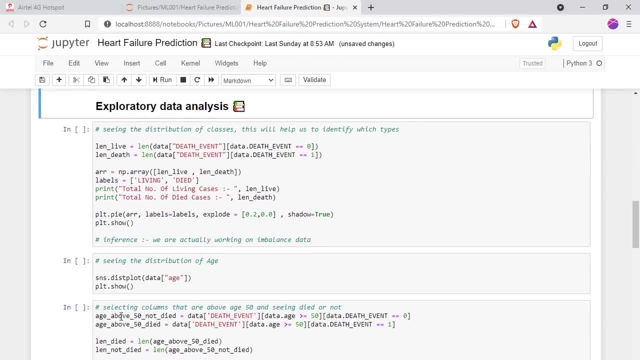 Because if you're a data scientist or data analyst at some company, you should work mostly on to understanding and finding your business solutions. As I'm a data scientist, I used to see I used to work a lot more with the data. I used to work a lot more with the data because I think that I should be able to. 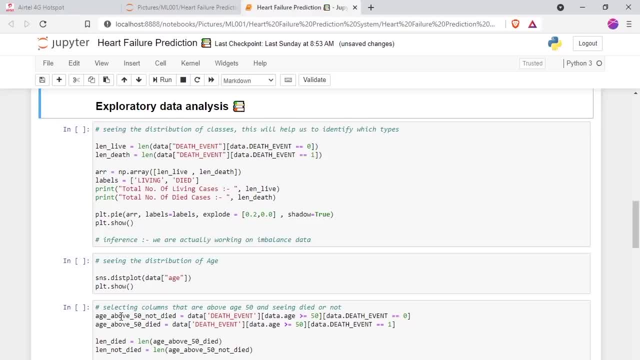 What the actual data is, my data is, and what the business objectives are, and what's this, what's the answer they want from my data. okay, so that's what I do: a lot of data, exploratory, data analysis there- so that's why I picked up this problem. I. 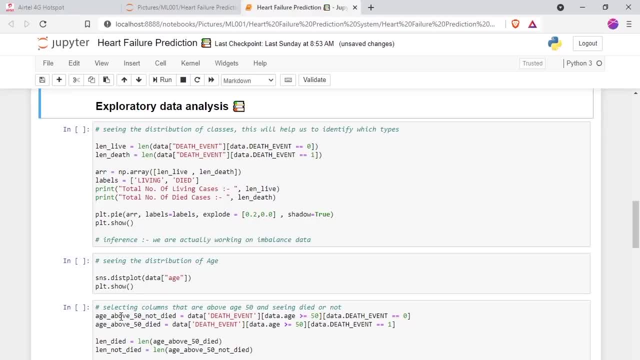 found it very interesting and not picked so much apart because it should be conserved like advanced house price predictor, diabetes prediction system, which I already made, which is available in my in my github. but I want you to try out, make your unique project and showcase on your resume, okay, so then 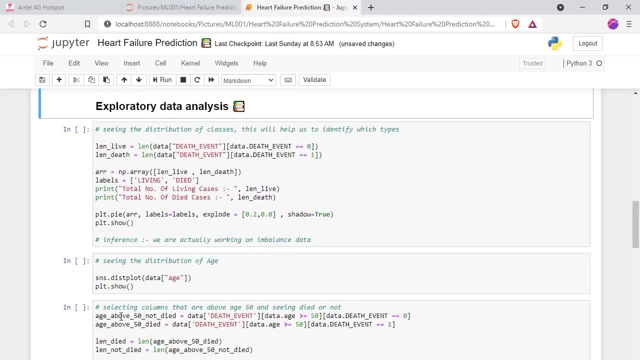 what? what we will do then? we will simply see the distribution of our class, assess. what do I mean? the class is above here. for this example we have. we have a binary classification problem and this binary classification problem we are given one and zero. okay, so whether it is one, then a person died. if it is zero, 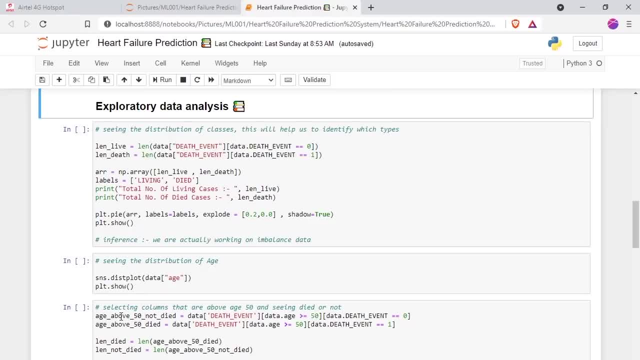 then a person does not die. I think I have to see. okay, so it's sometimes. yeah, so the person is leaving is zero, and the person is that is one. so we have two classes, which is a binary classification problem. okay, so I'm going to take a. 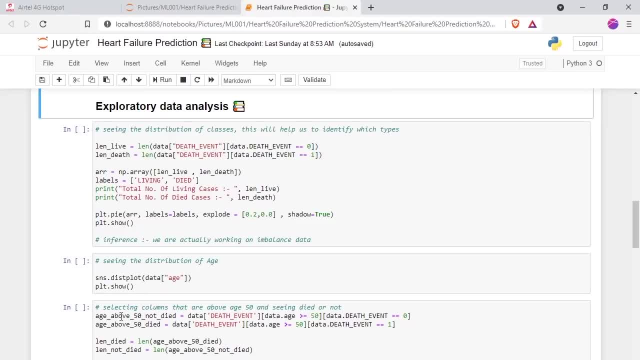 little first what I will do. I will take a look at the distribution of my data and you can see I'm highlighting the code from here. I'm taking a look at the distribution of my data and here it simply means that I'm just going to take. 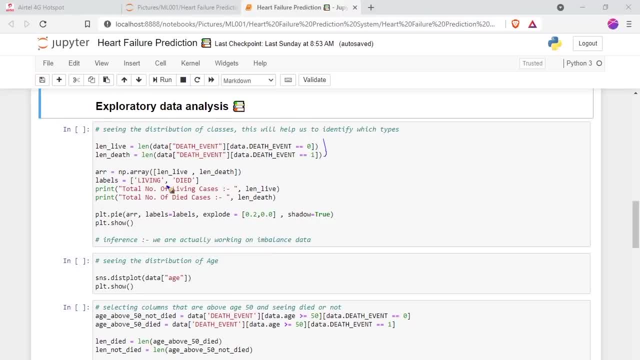 that's just just one of data. then bracket. I will take a look at the event. I'm going to count the number of event where the event is equal- equals to zero. I'm going to count the same where the event is equal, equals to one, by taking out the length of. 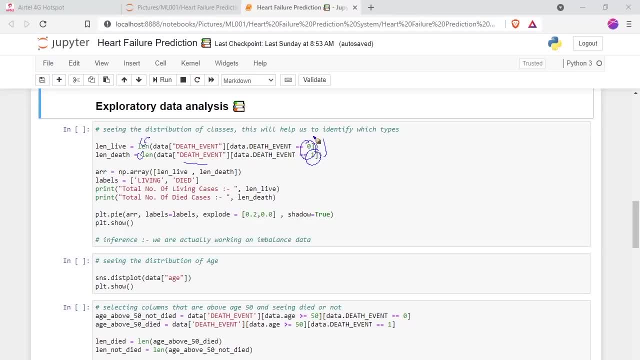 Each arrays or CDs. okay then, and also, the PI PI takes an array, So I'm going to put in an arrow like this: I'm going to put in an arrow, So let let me choose that red color and this Medium. that works good. I'm going to put in a array and then I'll just label it, just just to make sure everything is right. 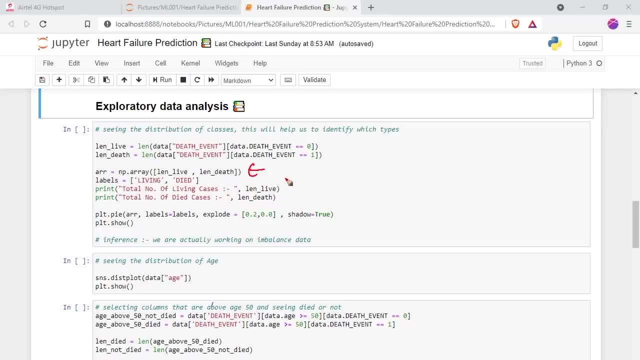 So I'm gonna label it with living in data. I'm going to print it out: What is the total number of a living case cases And what is the total number of a diet cases? Okay, and then I'm going to plot it out by just PLT PI. 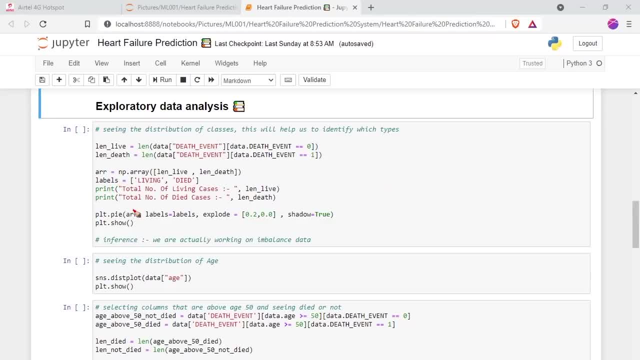 I'm going to lot it a pie chart by giving our AR. our AR will contain the length of life and length of that like this: okay, and then labels will be the same, like living and died, exploit. this is how much to explode our and shadow. what do you do? you want your. 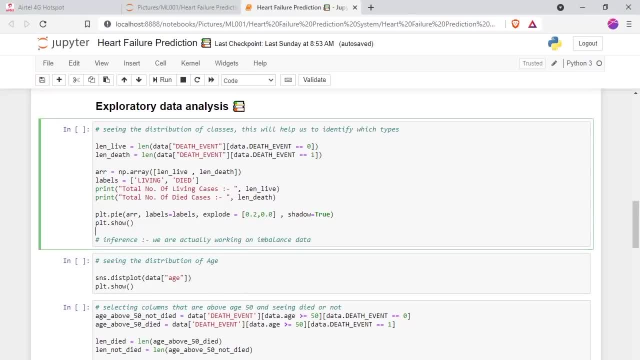 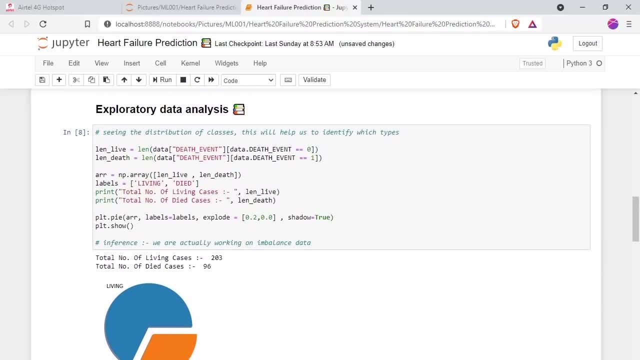 shadow. yeah, sure, I want the shadow, so I'm going to run it now. so I just hope that I've run the previous. I'm going to run it now and you can see over here that to you that your data is imbalanced. we are actually working out, we are our. 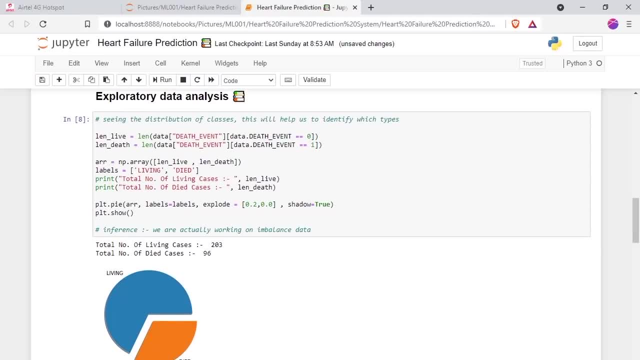 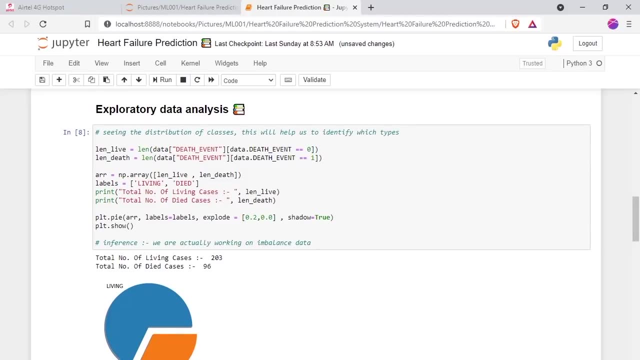 data is imbalanced data. so I will tell you why I like this, this. this data is imbalanced. but first of all, what is? first of all, you can still be all that we have total of two hundred three living cases and ninety six, which is type cases, and it makes sense also because in real world, living cases is 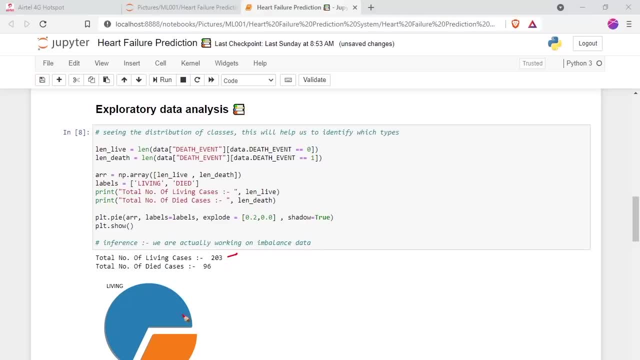 more than the death cases. I don't know, actually I'm not, but I think so. okay, so now let's let let me show it to you in particular, to help you get a feel that what is imbalanced data? okay, oops, why there's not working? 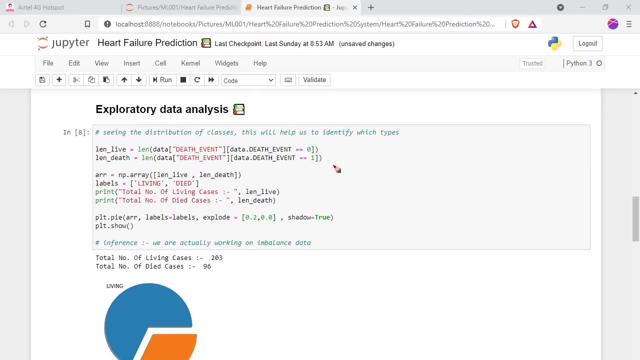 what is imbalanced data? okay, what is imbalanced data? okay, what is imbalanced data? so imbalanced data means- let's take an example- that you have two classes, for an example, here we have two classes, living, and that okay. so you have more examples of living. which is here: two hundred three, two hundred three. 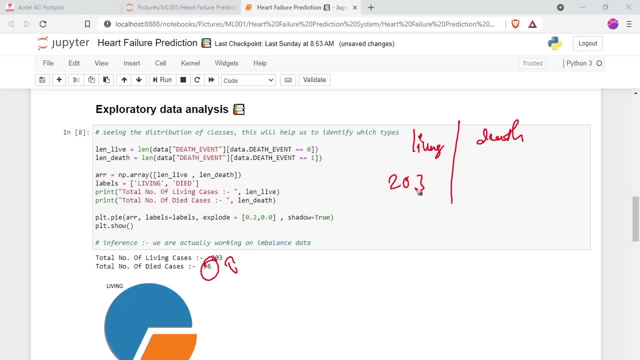 examples, but you have a far lesser, two times lesser, the lesser than examples of ninety six. okay, so here you were actually working on a balance data. what? what can be the issue of this? issue of this can be that your model, in most of the model, is most trained on this living. so 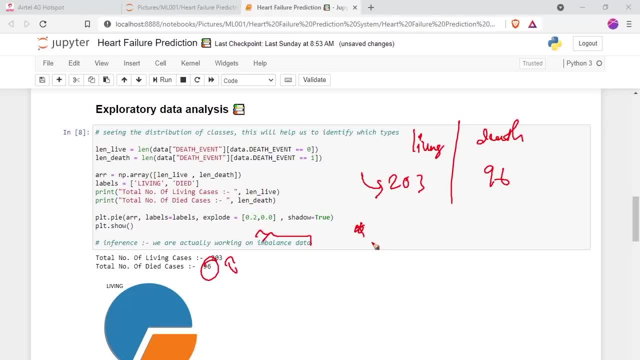 your. you can assume that you're that the output of the most of the output of a model will be zero, rather than one in some cases, actual print one, but it will be most of the cases it will be zero, okay, so here we have some examples. so 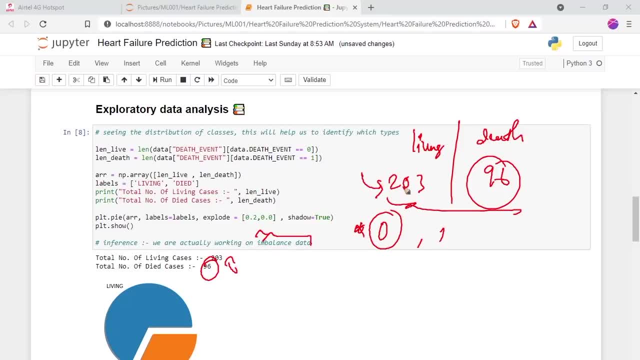 maybe it can, but your model is more poorly trained under two hundred three and your model may maybe get biased towards. problem means your model and can be like this: print zero. your model is this, this model, and it's funny, printing zero at every time. so this happens when you have. 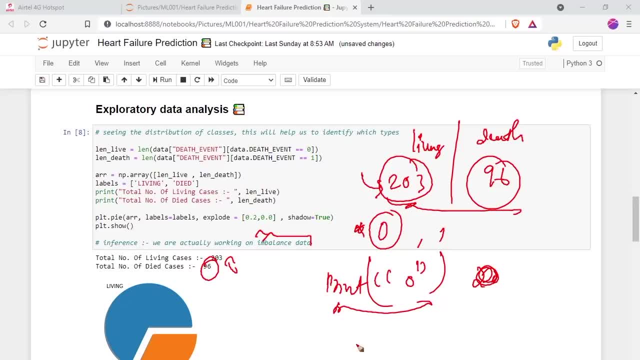 for one cases. we have two and the. let's take an example that you have a four hundred examples. so for one cases you have three, nine, nine examples and one, one example for for death. okay, so that is causing that will cause the problem. okay, a big problem. this is a big problem which comes as a something called, as we 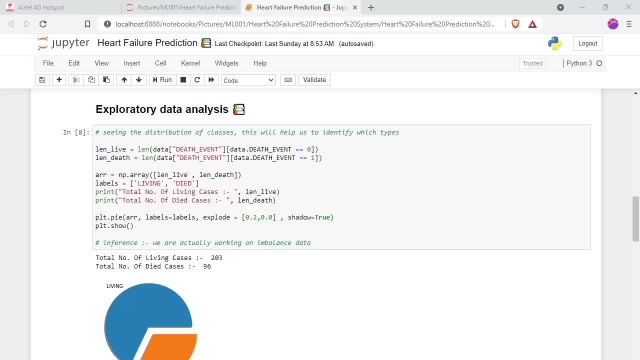 were starting in deep learning, which is working with imbalanced data. okay, so this- this is what I'm going to highlight- that just I'm just want to take a take, a take, take, take. my answer is: my data is imbalanced. how much examples for each case do I have? so I need to answer my question that we are actually working. 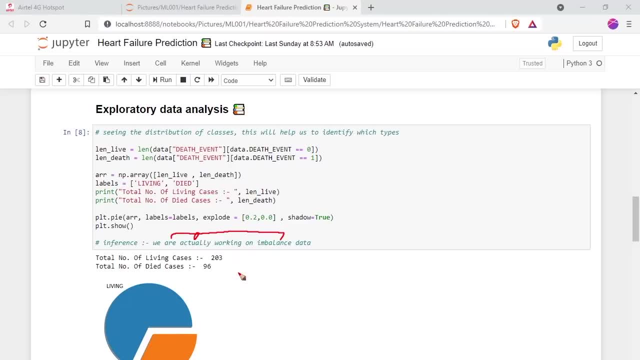 we are actually working on imbalanced data. which is actually working here? on imbalanced data where we have a living cases equals to two hundred three and died cases equals to ninety six. so imbalance, simply imana or equal required. imbalanced means that your classes, at your classes, are not equally distributed. 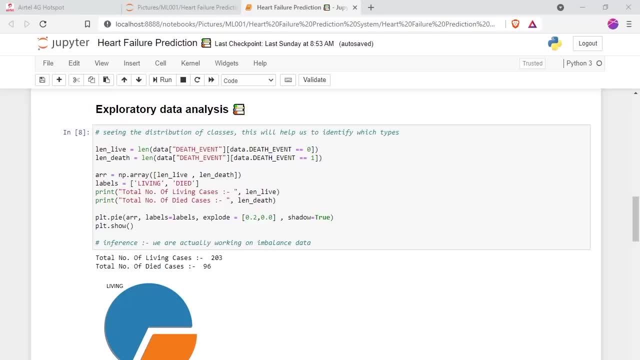 and not equally distributed. so can I write you down now? yeah, so let's write the definition. so those is going to ambient out is to imbalance means, and balance means that your data is data is not equally distributed between classes, distributed losses. okay, so it may happen that if in balance data, our data is equal. the 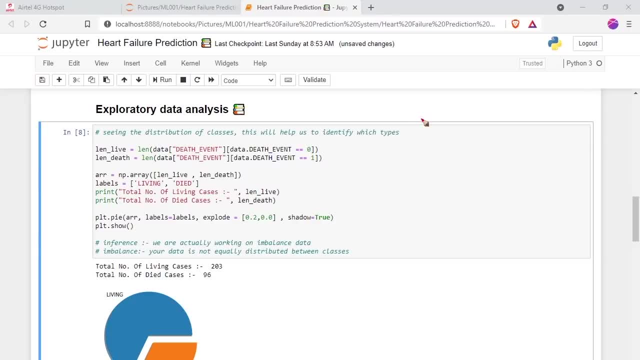 distributors. so for an example, for a particular example. so for example, let's say you have a training length maybe 400, so if you have a training length to be the 400, so assume. so assume 200 is for death examples, 200 is for life example. 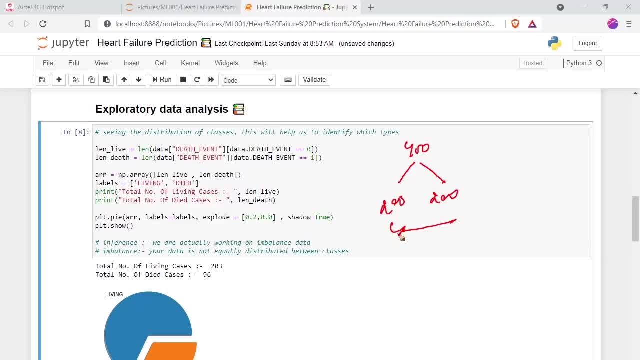 so we have. we have equal number of examples in both living and death cases. death cases- okay. so this is. this is an example of balance data and our model works best here. okay, isn't more robust, it is not biased towards anything, okay. so this is the basic, this is the business, this is our. 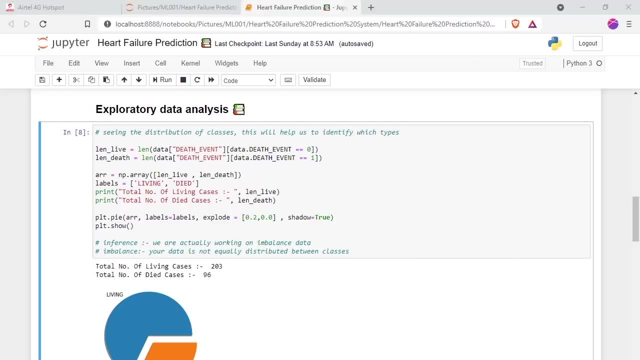 four sticks for a way to didn't analysis take taking out their reference. so what, what we have done so far? we have simply taken to have simply drawn some EDA from here by taking out the length and taking out the length of each event differently. so we are simply taking out the length and taking out the length of 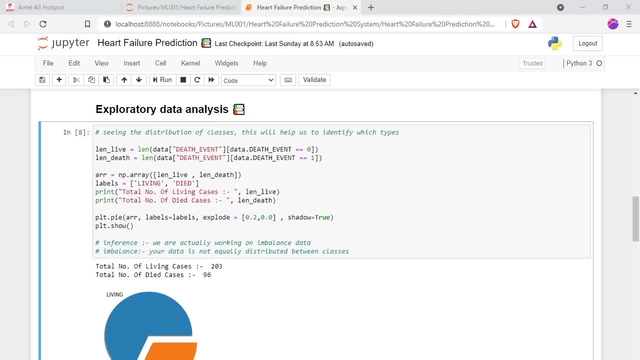 0 and 1, and then I, then I put in an array and then I'm, then I have labels, Which is living in dots and printed something, and then I'm gonna plot the pie chart with that. this, this, this, this, This explode comes with explored and shadow. We want the shadow, So you might be seeing the shadow over here. 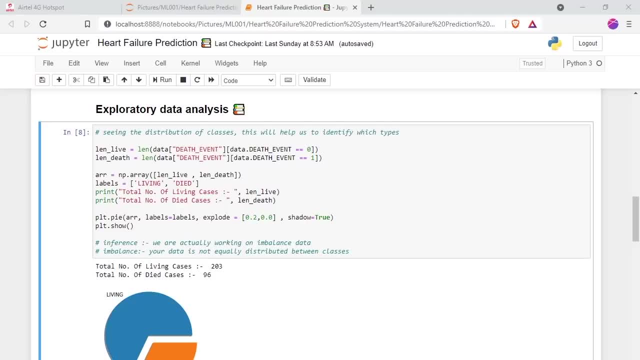 Okay, and you can see that. what the inference? so I answered my question. Am I working on imbalanced data? Yes, how much here? Okay, two times, just an approximate. So our bypass is two times lesser than the living cases, or we can put in a percentage. 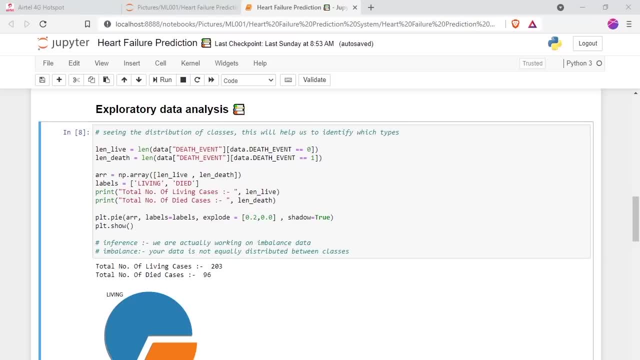 We're just dividing it down by just dividing it down to the total length of our data. Okay, so you can, you can take, you can try it out more mathematically, But this is what I'm going to show you, to you, about this inference. Okay, let's move on to the next inference. in the next sense, we enter inference. 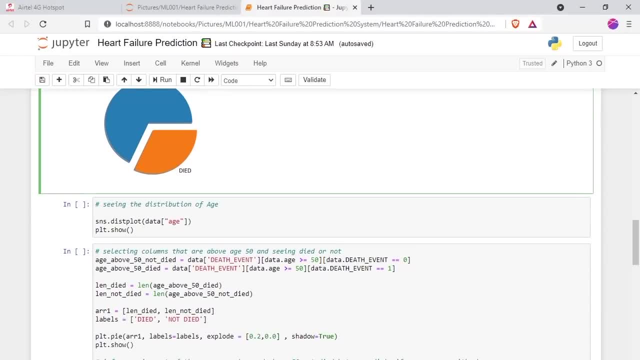 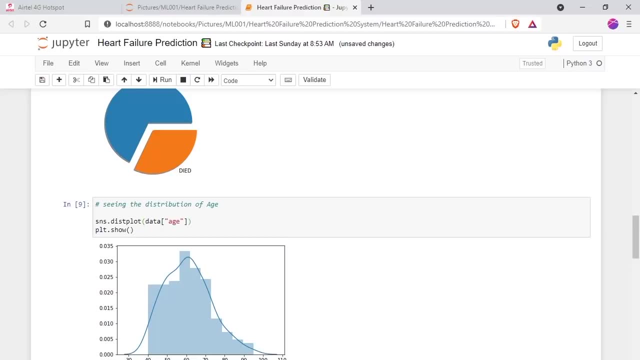 I'm going to take a look at the distribution of our age. This, this, this will tell you whether your data is when. what range, most of your most of them, the central tendency, I think that is that is here the mean, the most of the cases, most of the edges, like from 40 to. 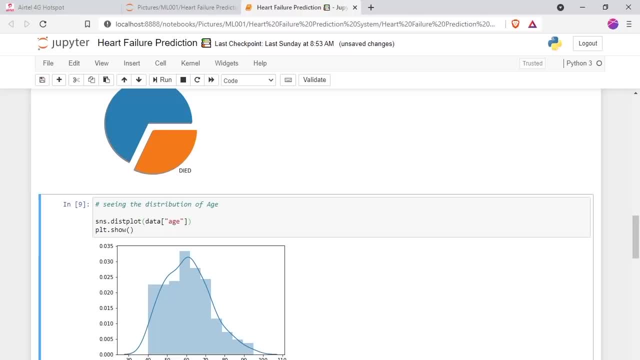 95. okay, most of the cases 40 to 95 examples. examples are starting from 40 to 95, 95 and then you can see most of the cases are in around 16. Okay. Okay. So this is the distribution of your data. You can try out for different different. you can try out for definitely for different, different. 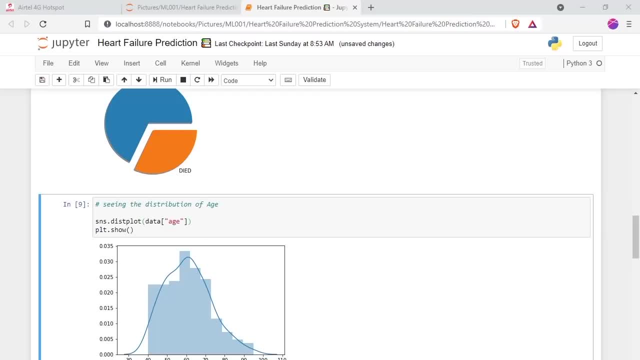 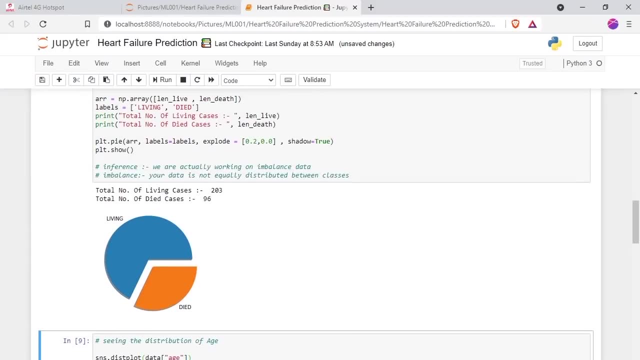 Okay, so this is the distribution of your data. you can try out for different, different. you can try out for definitely for different, different Numbers which I've already shown to you. There are a lot more numbers, You can definitely try it out. Okay, make a pie chart for class club, for binary columns like high blood pressure. 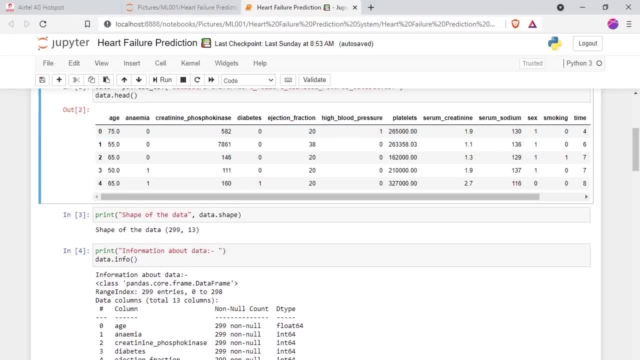 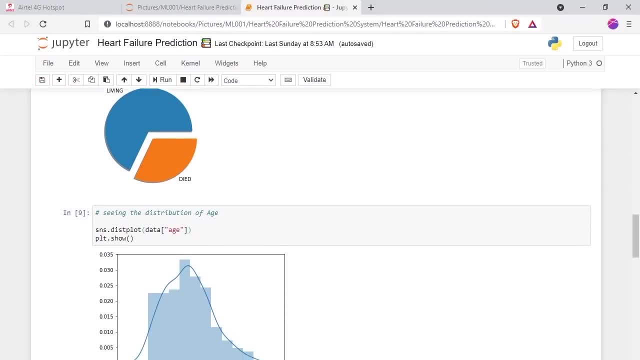 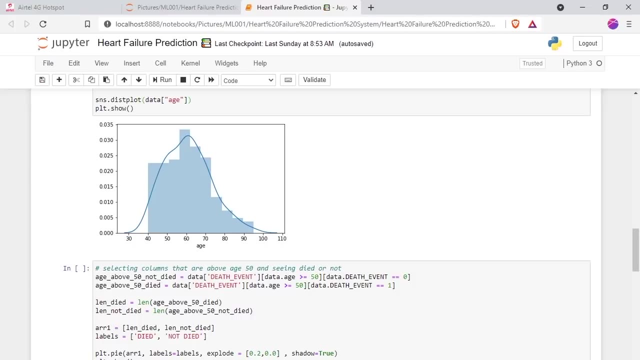 It was or not, or maybe gender, make that column and see if it works. So I will show you how to filter out the columns from there. okay, So now we have seen the distribution of our data. So now what I want? I just want to check. so maybe my business objective is, maybe my, some my, my lead to tip told. 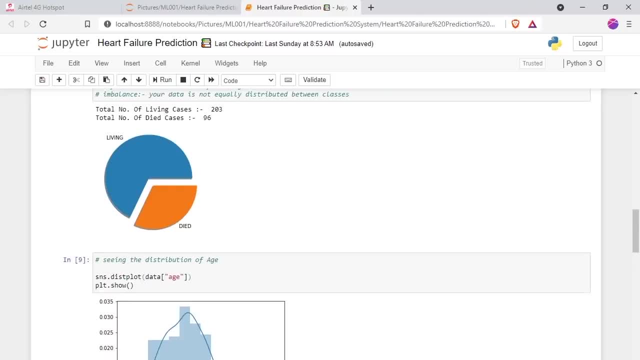 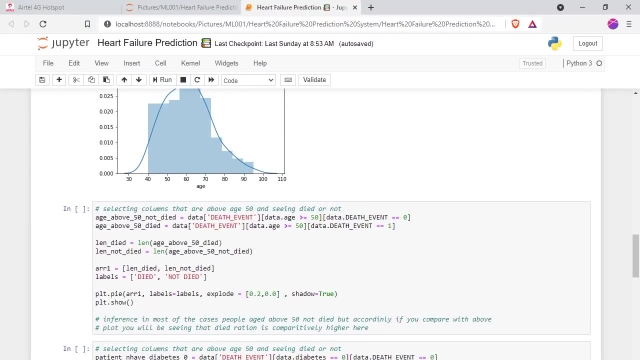 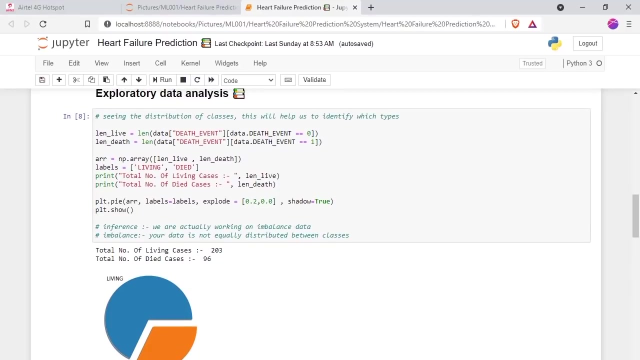 To me. hey up, if your data to your data dashboard, like this, should be answering lots of questions, Should be answering lots of your questions about the data. Okay, so here the answer that you're working on. this data means the total number of type type cases is less than the living cases. 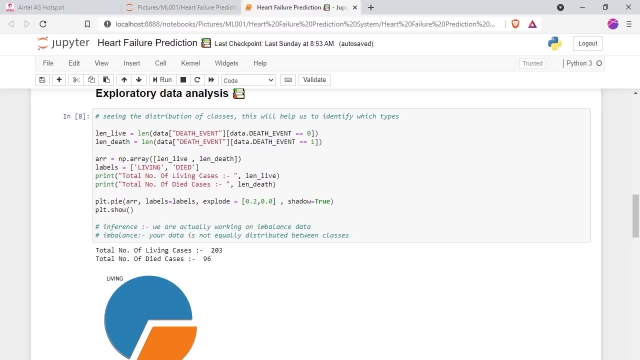 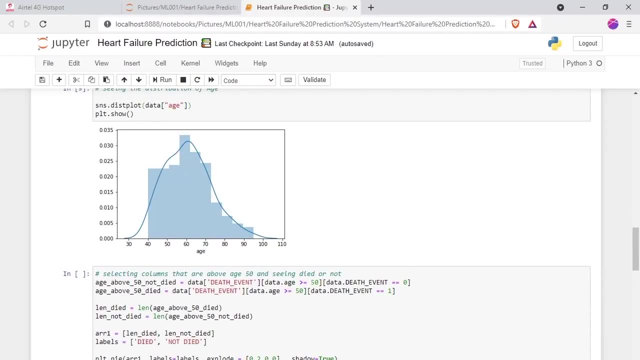 Okay, which is two times less than the tipping living cases, okay. So that's the, that's the, that's how you do, and here you can see, you can say to your Stakeholder, or whatever the leave, that most of the a most of the age rise from 40 to 95. 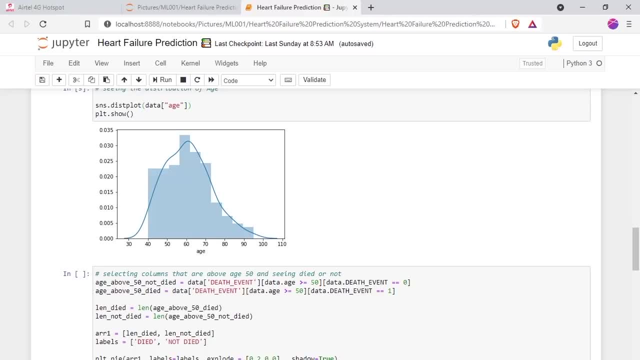 Okay, so you can see from this and see and you can tell. most of the cases fly around from 50 to 70, like that. Okay, that is the distribution of a day. So now say that you wanted to check. you wanted to check Select, you want to select the columns that are above age 50 and see their died or not. 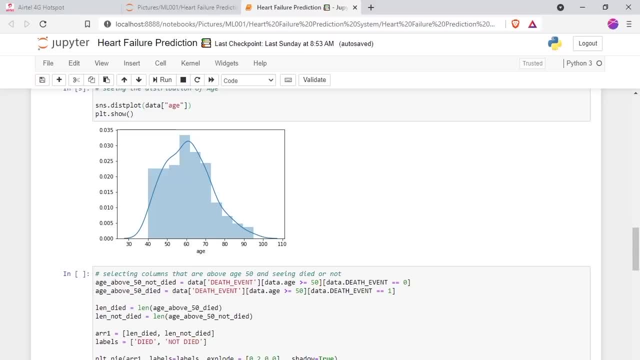 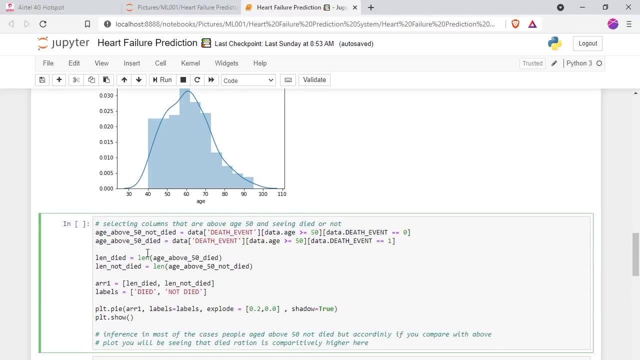 Again, the very great secret. it can be solved, it It can be put as a sequel query forum, But maybe you just just just think about you want to do in pandas or you want to do in like that. Okay, so it is possible and seek, well, but it's not why I- just as an example- Yeah, I've made it a Python. 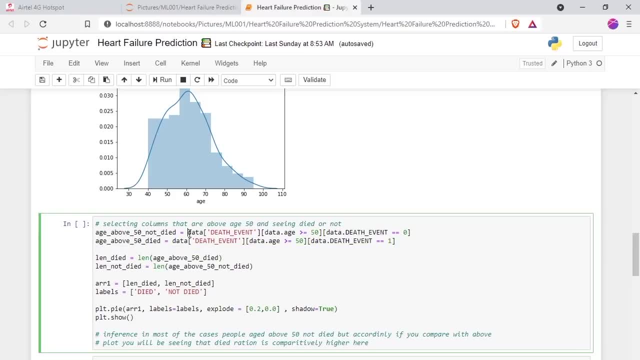 Okay. So what I'm going to do, my business objective Is select the columns. select the columns- Sorry, number of examples, I think better write it. Select rows that are above age 50 and seeing that are they are died or not. So here what I'm going to do: I want the death event. 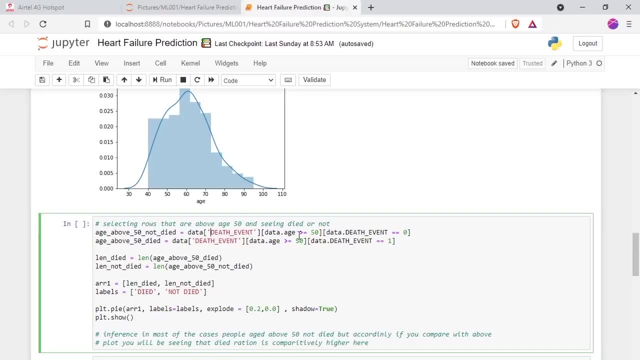 I want the death, even because I don't want any column over the death- even whose age is above or equals to 50, and They are living, okay. and then Again the same thing, and then again I'm going to take out the length of the same as above, and then I'm going to put in: 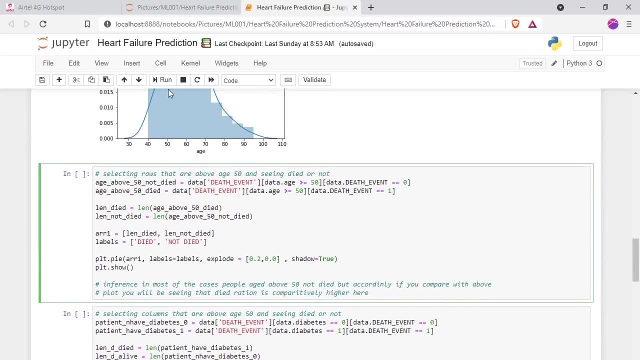 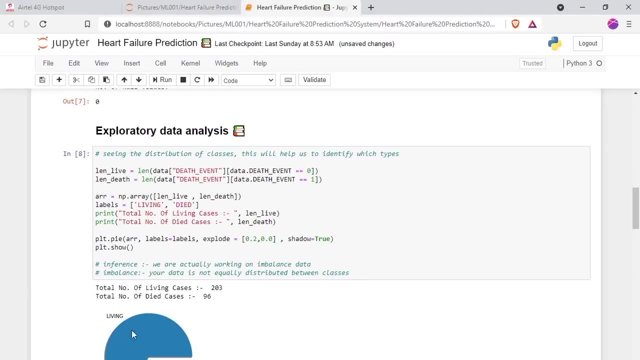 An array labels and I'm going to plot it, Okay. So if you can, if I run this, you can again see. you can see here that here you have living cases here. Here we have the living is a lot and you have a small, but you can see the died cases, died cases. 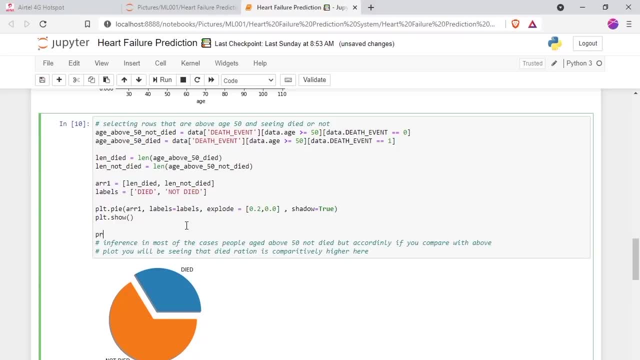 So if, if I write it out, I just want to write it out like this. So I'm gonna write a total number of total total number of It's a diet cases, died cases. I'm going to take out the length, length of died, Length of data I'm gonna do for total number of. 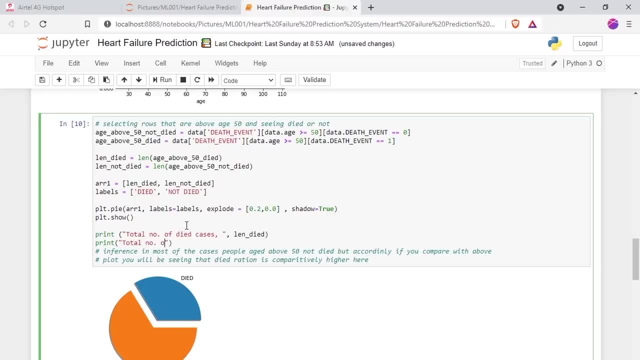 total number of non died cases. not died cases. just just, I'm not able to write because I have two tabs in front of me. it's very difficult for me to table right over here. okay, so here. length not died. okay, so here, if you can see that you can, you are able to see that we have total. 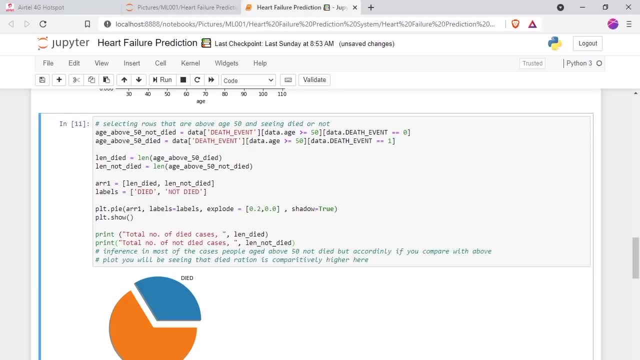 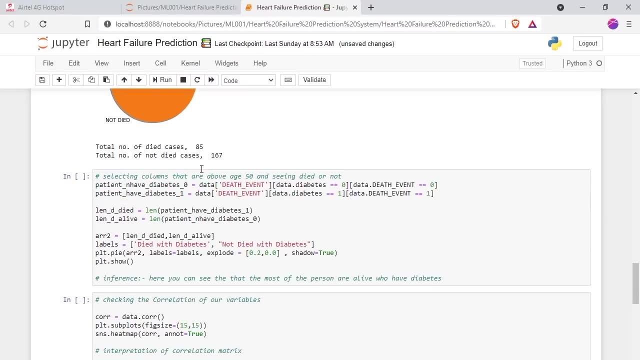 number five is 85 and total number for not at 167. so just see over here that in total, in total we have 203, which is two times lesser than- and here this is fairly one times less than. okay, so here you can see, and most of the cases are: 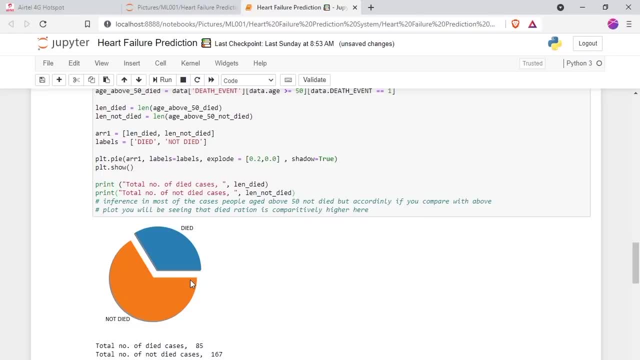 green died, but most of the cases of over 50 died. okay, as comparatively to of a plot, maybe not not making sense, but again I'm sorry going to say let's assume that just let's listen me what I'm saying. I'm saying like you can see. 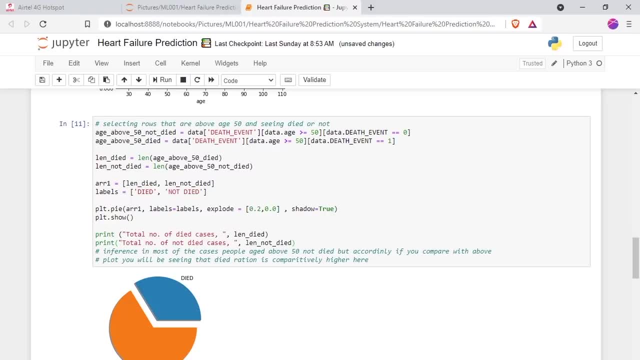 that of the number plot. we have total number of our died cases in two times our died cases, our died cases. you can see that in our plot we have total number of our died cases in two times our died cases. our died cases in two times lesser is two times lesser than our living cases. and here our died 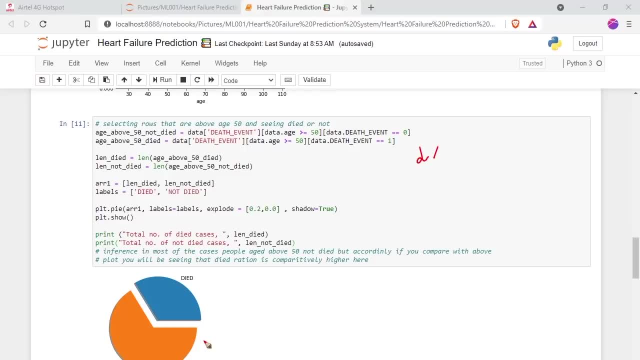 cases is one times lesser than not died cases. so here you can, we can see, obviously this is low, but here you can see, most of the people that are above age 50 died. okay, from this inference, comparatively from the upper plot, okay. so here that's how we answer the questions from the data and I hope that. 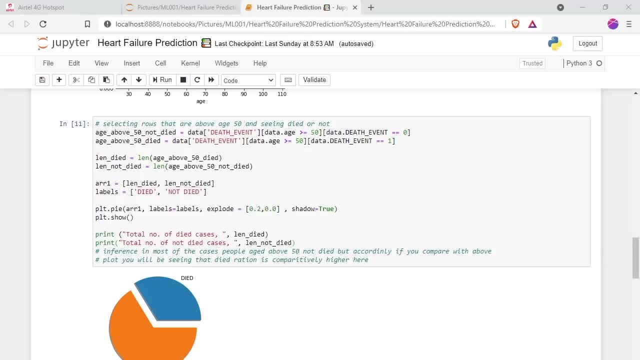 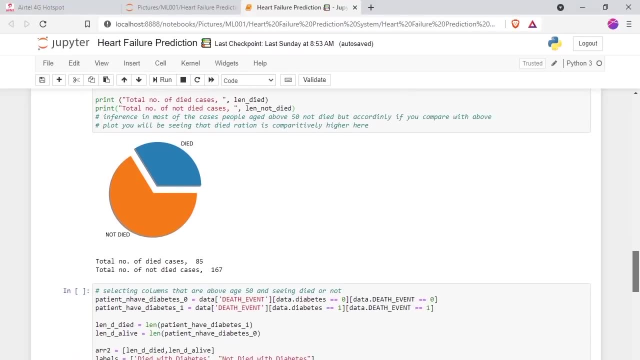 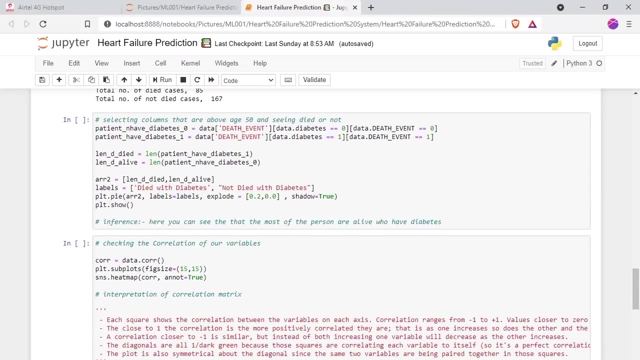 you understand, understood everything, and I think that you will be taking out more inference. okay, great. so let's see one, one more, one more column which is very fairly good, column which I think, oops, cut out. I'm just going to: yeah, here it is, oops, yeah. 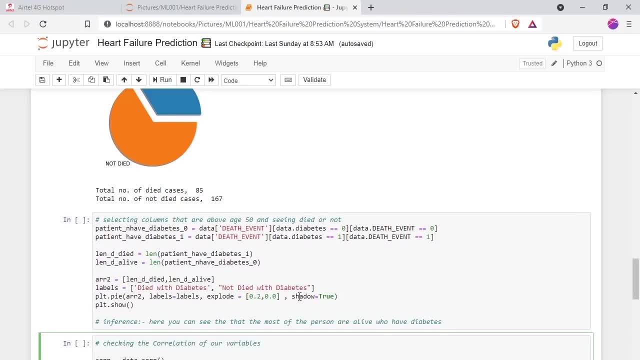 here. it is okay. so now, now just assume that you want the columns that are of above age 50 and you just see whether they are died or not. I think that the I have already okay, so you want they have that there are above age 50, oops, I. 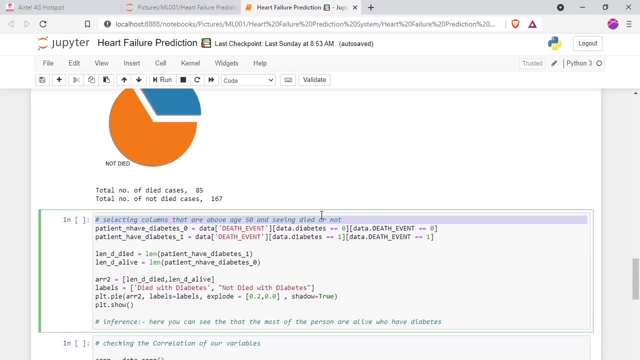 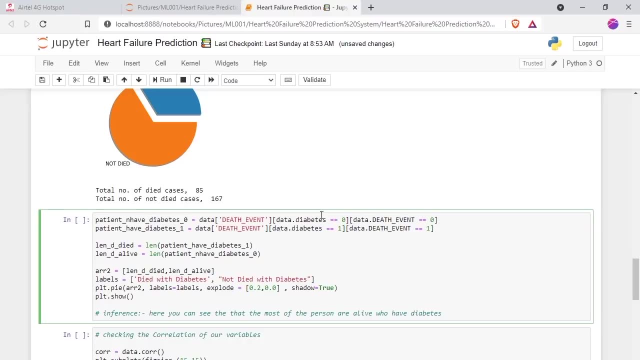 think this is, this is for diabetes. so yeah, so what you have to see, you have to see, you have to answer the question that the person is having diabetes, that a person is having diabetes. how many numbers, how many numbers or patient, what died are having diabetes and how many numbers of patient this don't dies there. 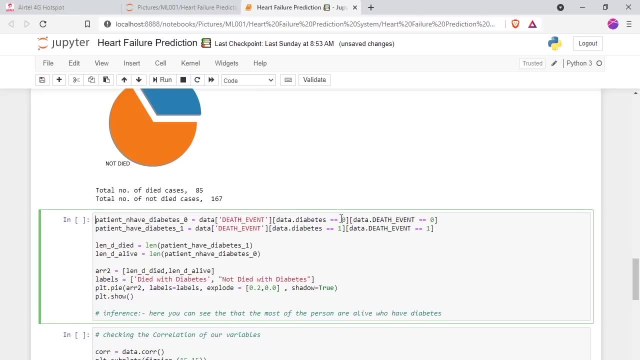 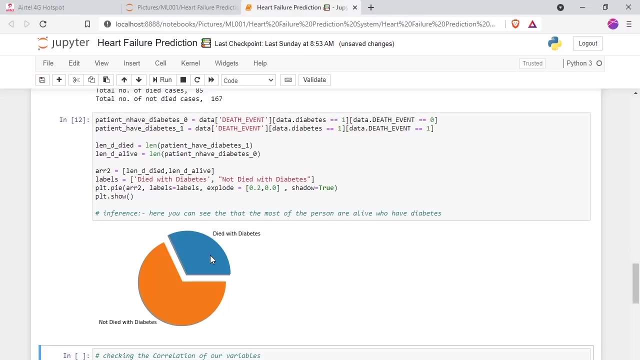 did not dies having diabetes, okay, so diabetes isn't where the person is not having diabetes and having diabetes, okay. so maybe i've done a little bit wrong over here. the diabetes should be there. the diabetes should be there and we have to see whether the person had died or not. okay, so you can see: died with diabetes, is this and not died. 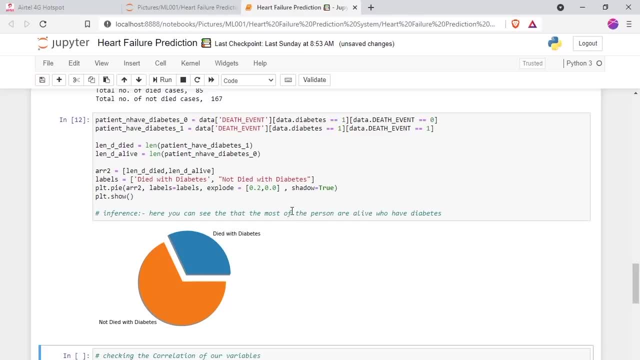 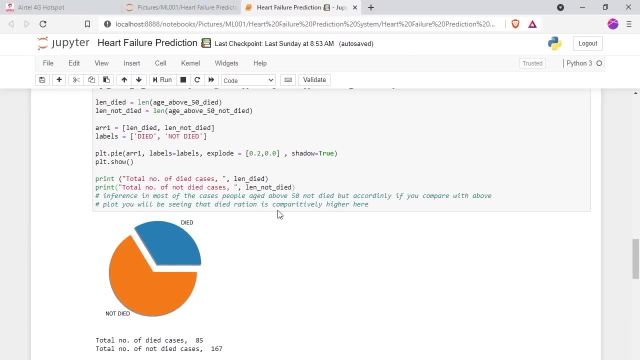 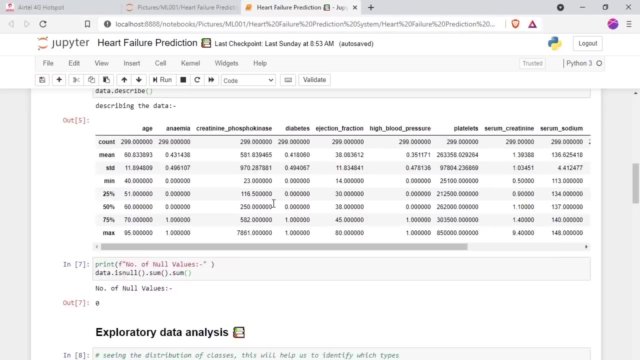 with diabetes is this. so there are a lot more, but you can again compare with the other plot over here. then it will start making more sense. okay, so we have done extensive data experiment today, data analysis- a lot more can be done to answer a particular business problem like this. you can see. 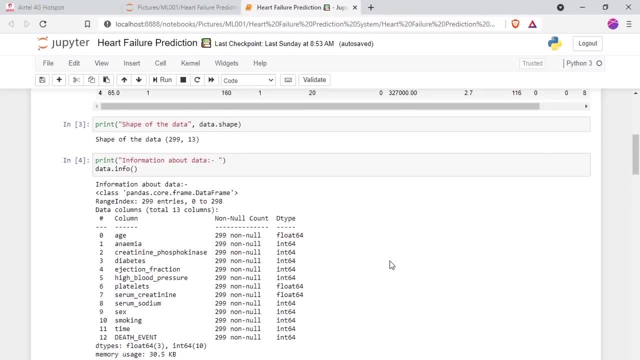 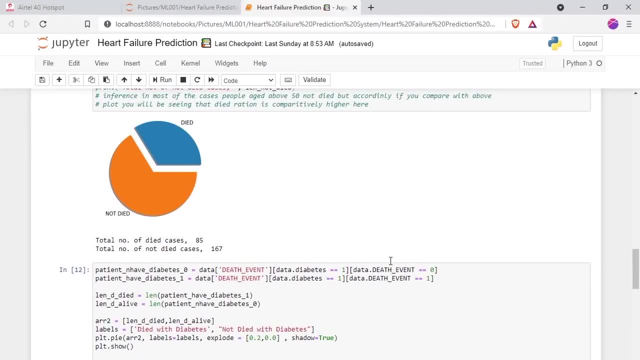 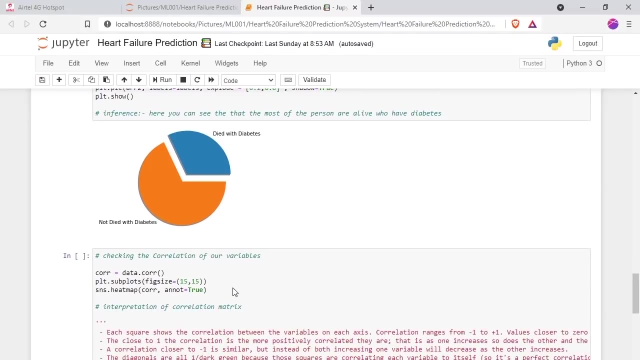 over here you can answer some more questions from the data. but as to give you a taste of this, how i do, how i like to do the answer the problem using my favorite visualizations, okay, so you can answer this. uh, it's, it's very good to answer this all uh, by just uh. 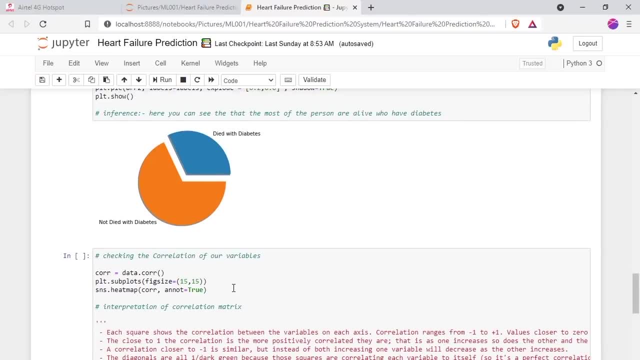 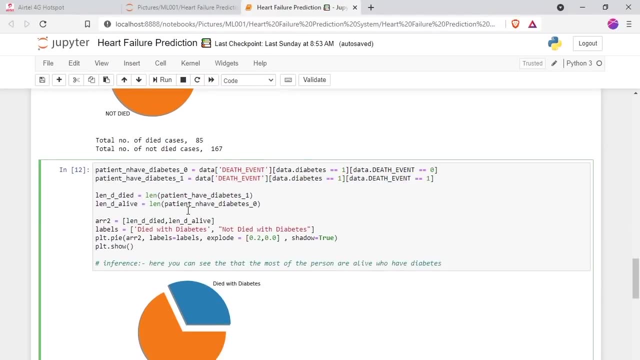 visualizing it down and saying to the lead: okay, so now, now we have seen a lot more things. we have seen that more of the visualization. just don't worry about this. these are again in the course website, mlo1.netifyapp. it's a very, very, uh easy, easy to get all these notebooks. 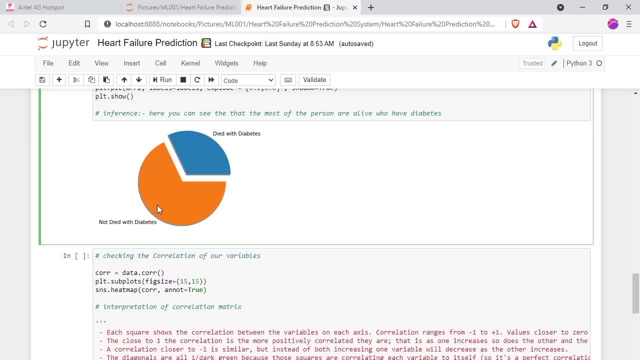 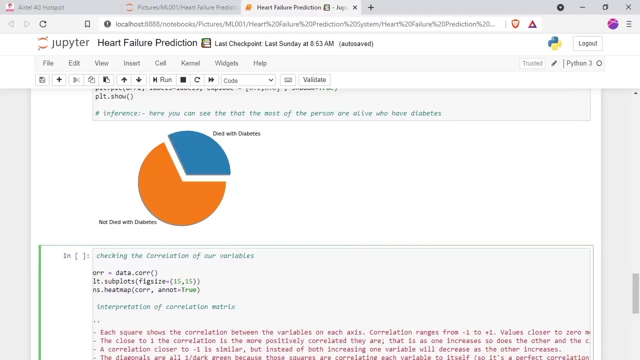 okay, so now you will check the correlation of our variable. so what do i mean by take checking the correlation of our variables? it simply means, if you don't do, um, that, how your, how your features, how your features are correlated. so here you have a very good reference. i've taken from a style of the. they have explained very much extensively. maybe some 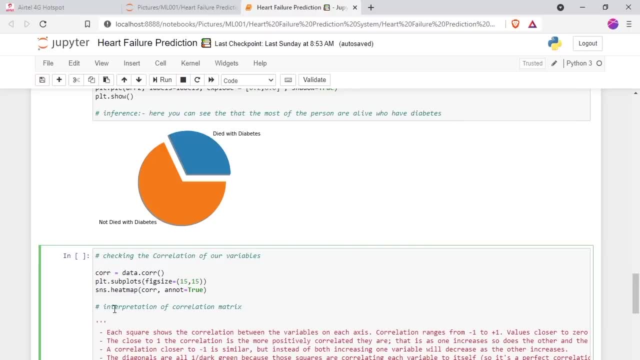 online. so here what it's telling: it shows the correlation between variables on each axis and the it's means. it just shows that i i will give you the uh plot over here, but what is just what it does? it simply shows you the correlation ranges from minus one to plus one. okay, minus one to plus one. it simply means that if your 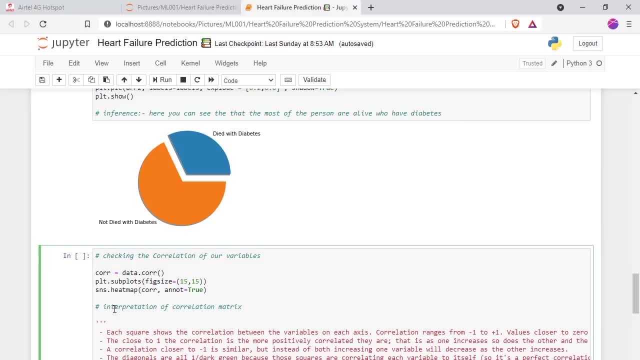 variable is closer to minus one, then it's very, very similar. okay, if you're is is very, very similar, so you can see: value closer to zero means there is a no linear trend, means clean linear thing is not there, so you can. you can't use linear regression over there between two variables. 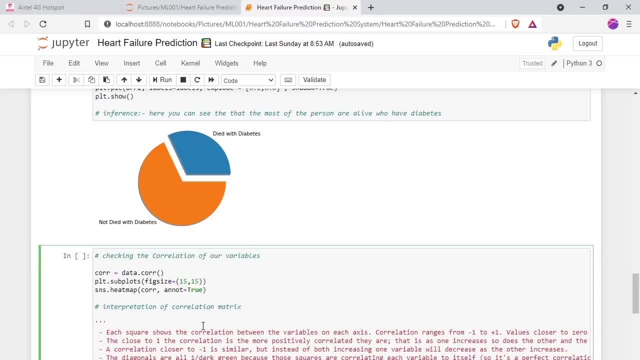 means we can each this correlation tell us whether your data is a linear or a transverse 송 or not, and the close to one, the correlation is more positively correlated. okay, more positive means correlation and correlation between these things, and you can read about Pearson correlation coefficient over here, because this uses 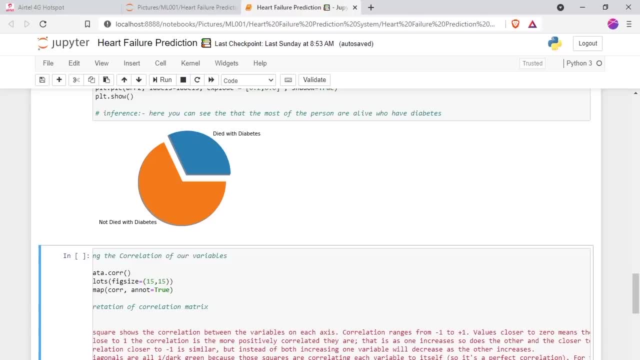 something kind of that. okay, that is one increase so that the other and close to close to one, to the strongest this relationship is means the the one is closer to one, the stronger the relationship is. the diagonals are all one. that simply indicates that the V squares are correlating with each. 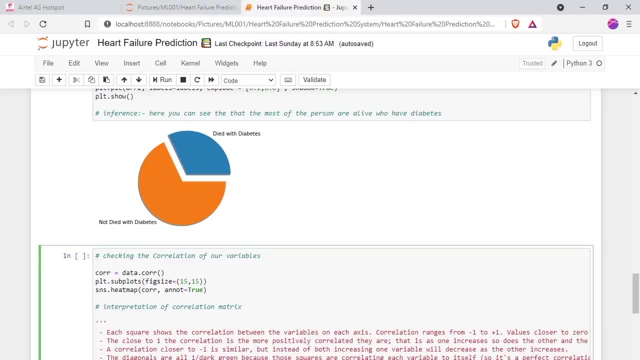 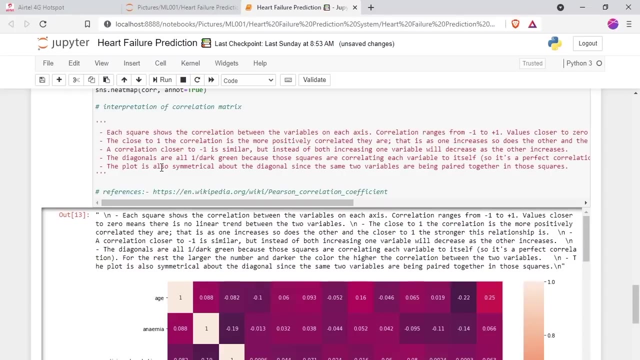 variable to itself, so it's a perfect correlation. so if you have all the data, all the all, the all the diagonals are one to the perfect, sign of perfect correlation. and the plot is also symmetrical, and I know that you know about symmetrical so you can see over here, but I'm going to just put it in a 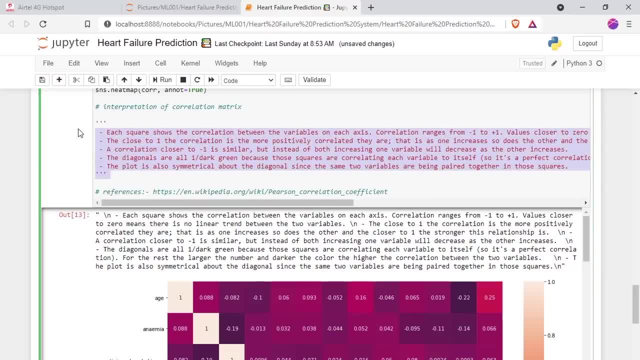 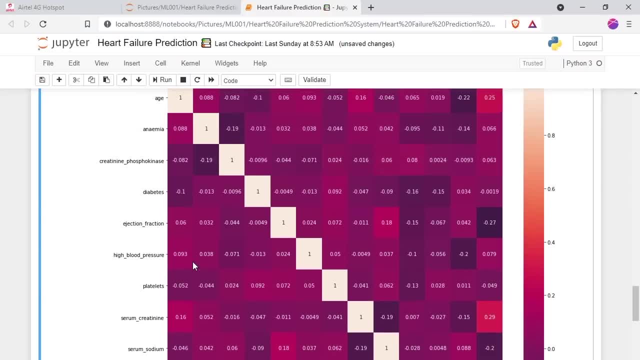 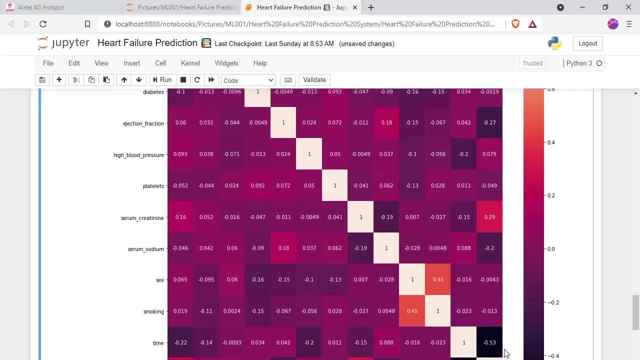 form of this. I just hope that. okay, so I'm going to run it out and here you can see that our data is perfect correlation: more the dark is minus 5.3, like that is the is the more correlated. okay, so you can read that. it's very I explained and also you can. 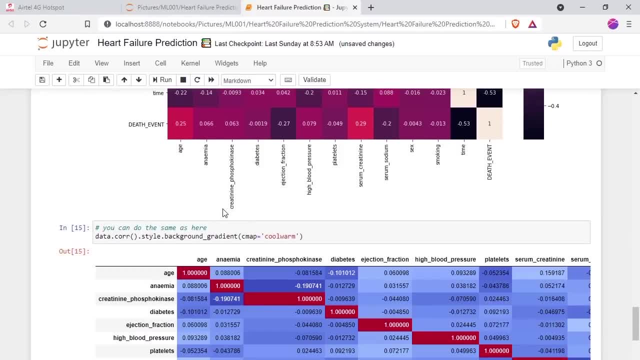 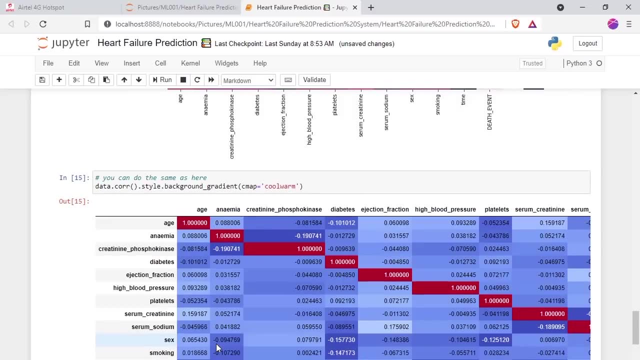 do the same as you like, if you want to do it with the pen, as so here you are going to do, and your diagonals are again one and cetera. okay, so we have talked about various things you have under understood: data and such right, such right. 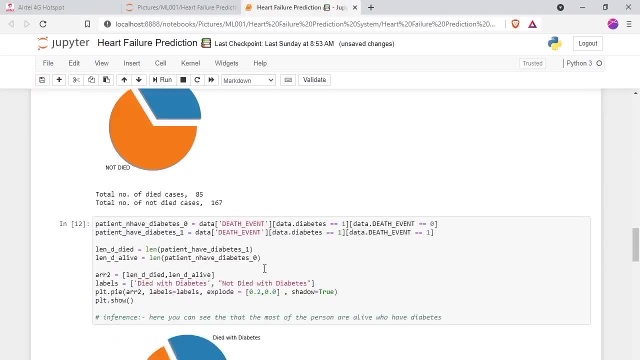 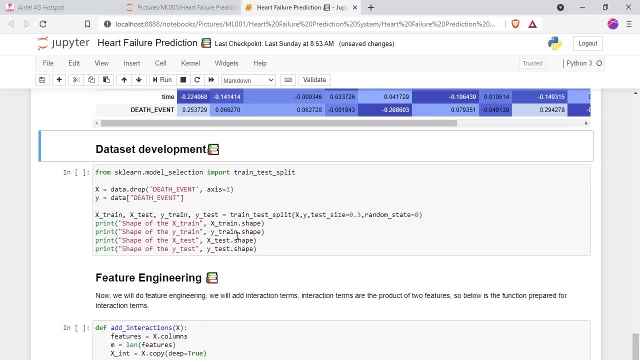 everything okay. so now I hope that you got an idea about how we process. so now what I will do. I will start with data set development, as I've talked about that. you should apply your data and the training on testing set, because for testing, you have to check some you have to. you don't have real example, so for 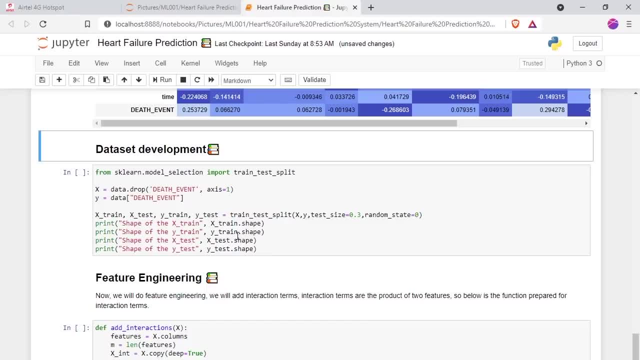 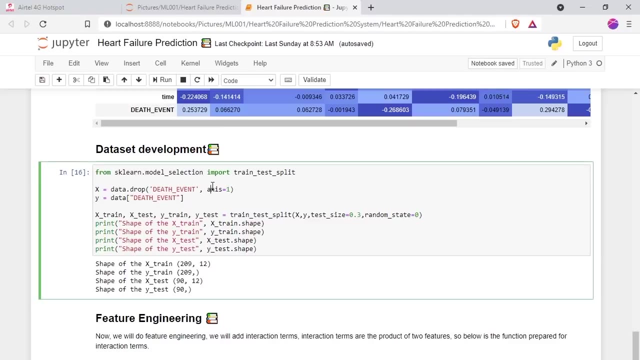 validating your model works best. so what you will do, you will divide your data and do. validation set means training, and validation set where you are dividing 70-30- okay, so 70% of training and 20% for testing. okay, so you can run this out. here we are using the escalon API from, while 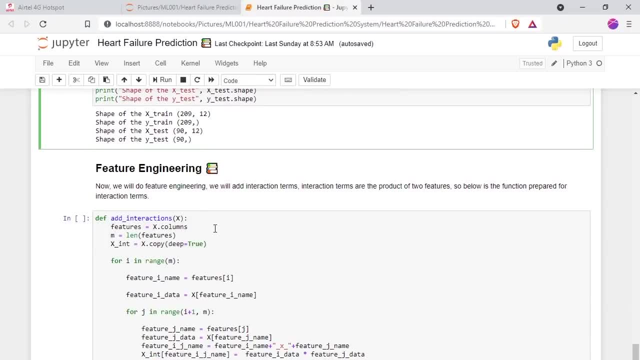 importing. the trend is split. okay, so now we have done this and I hope that you understood this also. so now we will do, now we will. I will not do feature engineering over here, but I will just showcase to you what's the what, what we do. just a one example of feature engineering. okay, so in feature. 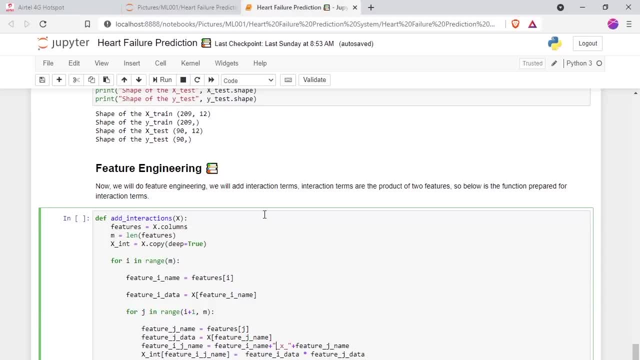 engineering. we add more features, we encode our variable, we put our categorical variables, we apply some transformations on our data just to insert our feature. okay, so here is the example of adding the feature. okay, so here what we here, what, what, what we are doing, we are adding in the interaction. 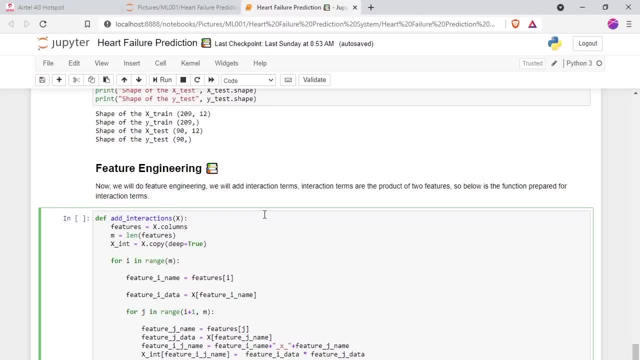 term. okay, so what is interaction term? interaction terms means interaction terms means lists. for a forensic, of example, assume that you have this data set, this data set which is gender and age- okay for an example. so it will add again one new form by taking on the product of G is Z and not less, taken a BP. okay, everything is in numerical, so it. 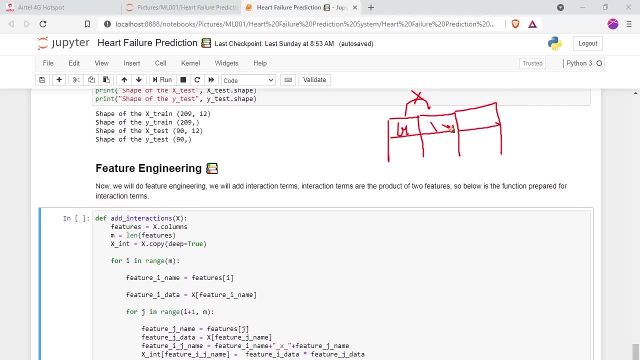 will take the product and add: okay. so it is just doing the product of two features and making that column okay. so maybe that that will not make sense, but this is what the interaction term means means. we are just adding the product of two features, okay. so here is a function for that. so first of all we are taking the columns names, then 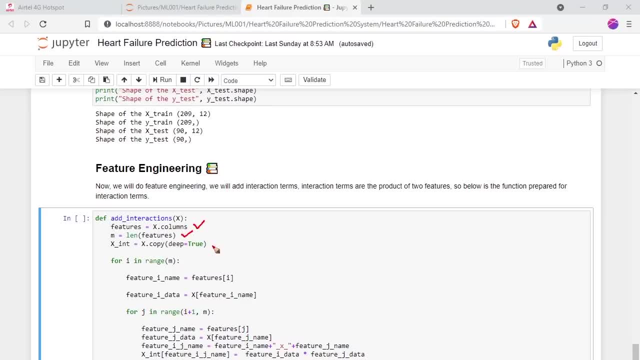 then we are taking the length because we have to see, we have to iterate through and and and then I'm going to copy it out so that we can change anything to X and I'm going to just iterate through all the columns and I column represent the represent of first column and this feature, I name that, this where it is. 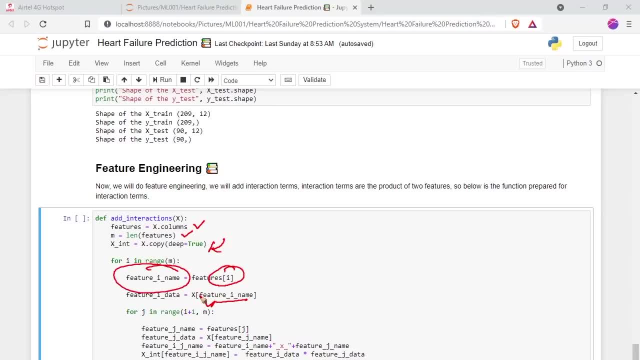 this, this column going to ask access using X and then range through G, because I want to multiply these two. so here again the same thing, and again I'm going to take out the data. and it was just to make it this, to just show the name of the column like this: that's definitely multiplied. 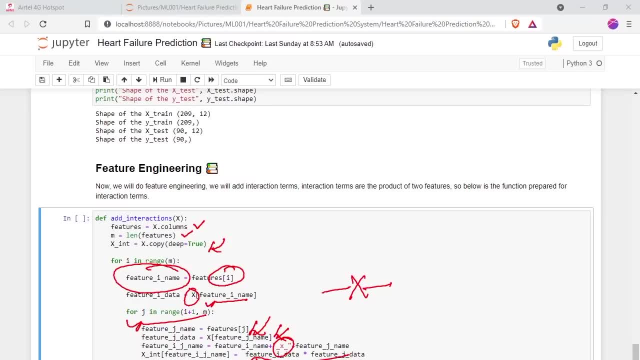 and actually you're multiplying the sound and then we are returning the X and okay, so this is what. and then we are calling on X train and X test and we are done, okay, so here, if you run it out now you can see if, if I show you the code, you 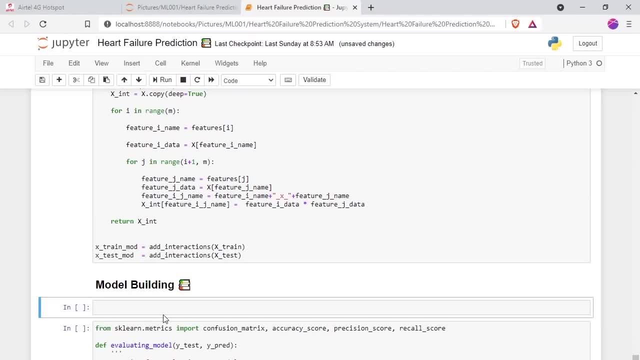 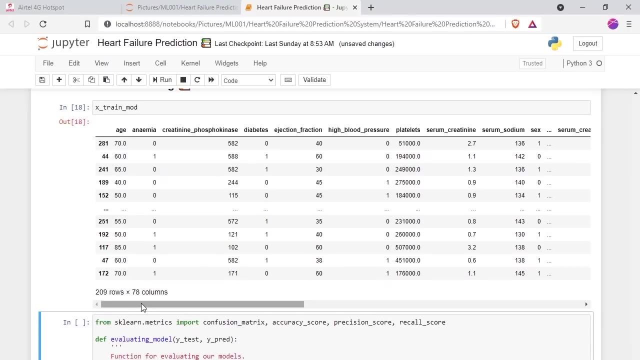 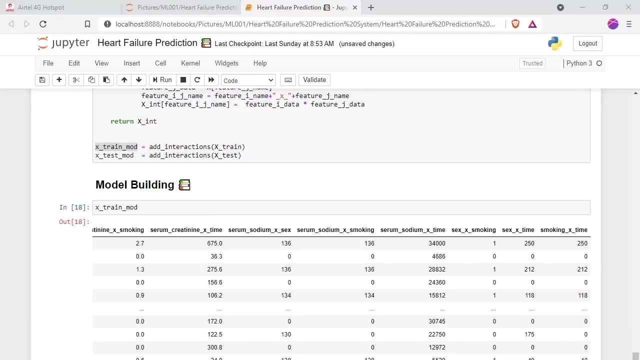 if I show you the X train mod- X train mod- do I run it? yeah, let me run it again. you can see that we have 78 columns. yes, 78 columns. from your 30 call, 13 columns to 78 columns. you can try the result, how it is working, and let me know. 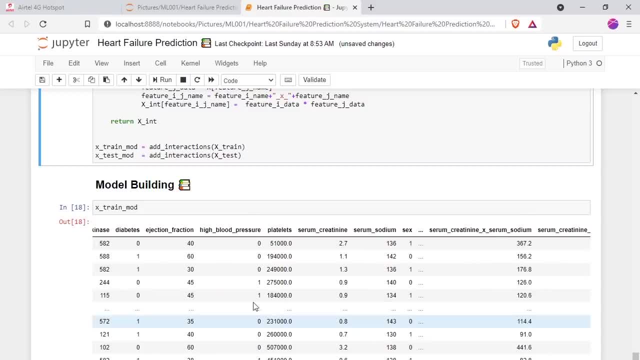 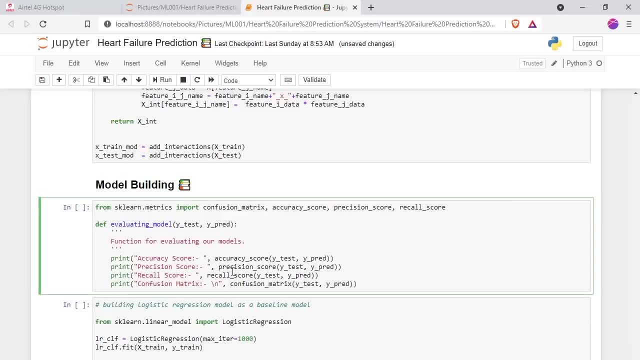 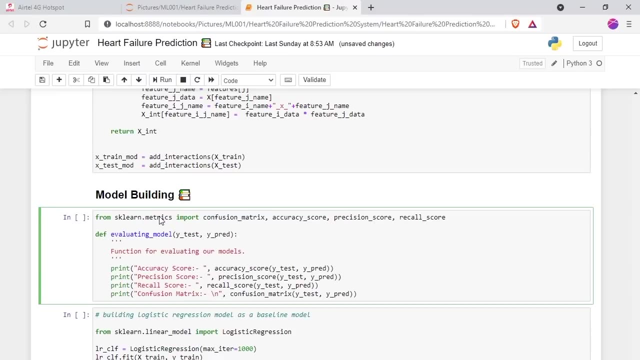 in the comment box below on our on in our desktop community. okay, so this is what what we are doing, and by adding the interaction term, we are filtering to explore more. okay, now what we'll do, we will. now we'll start building our model. so how do we build? just just, we will start building our 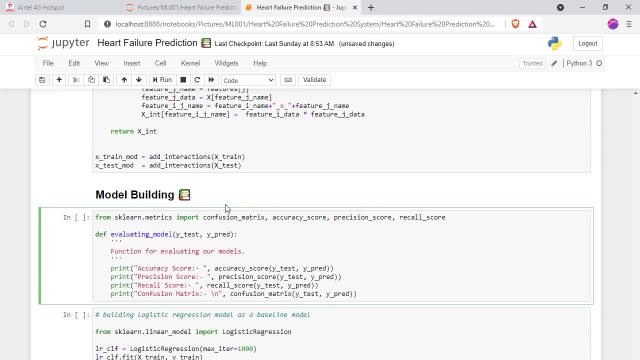 model. so first I'm going to make a model for evaluating our models. so first I will take a look at the accuracy, the season recall and confusion matrix. so again, if I run it over here now, now it will give, and we are giving the ground truth, as well as our predictor. okay, 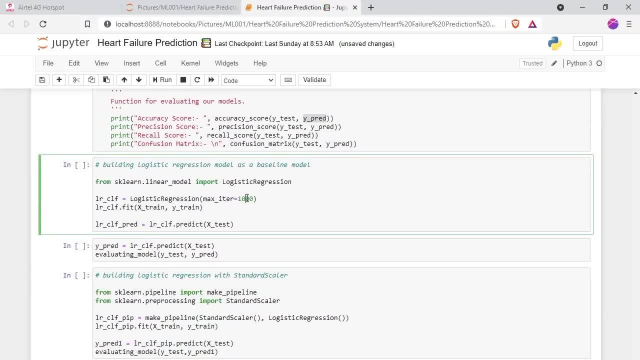 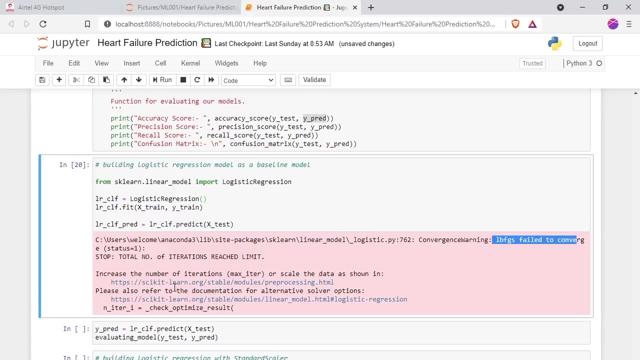 so let me update you basic caliber. you can enter this to and you will see this is much packed. you can so simply, as I just showed you elements when I track with 함- oxygen- and we set that scalability and they work very well together. it should function very well together, but you just need to. 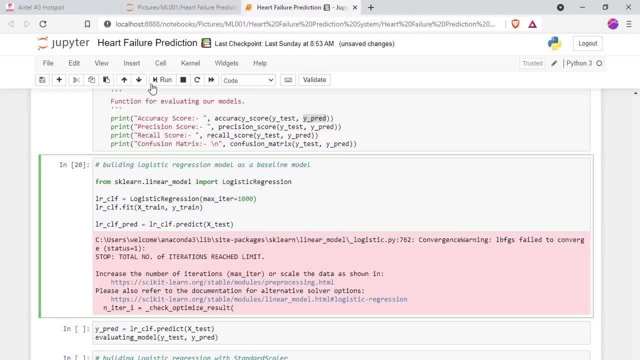 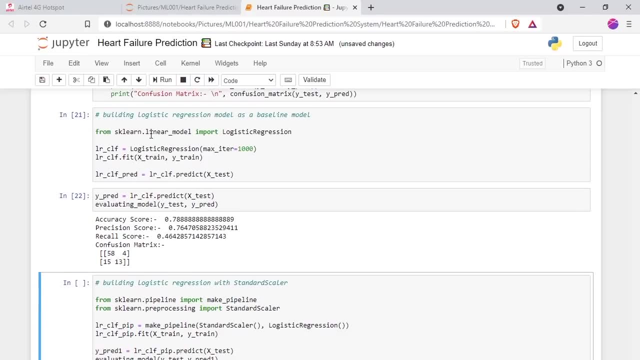 take a look here. ok, first of all, I'm start with registration when max iteration to be 1000, the reason why I had given over your, because if you, it is not converging, So increase the iterations to 1000 and it worked. But it is also telling a process to standardize your data or to scale your data. 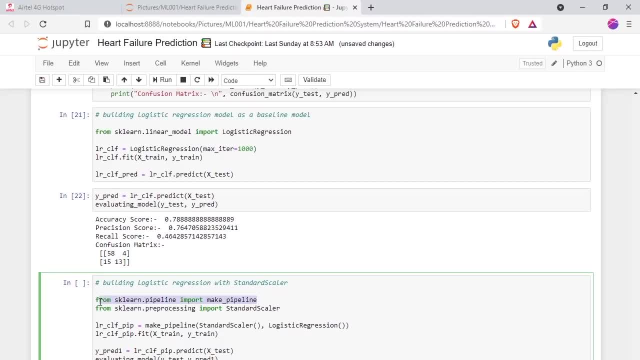 So here for standardizing as well as building the model, we have something called as make pipeline. So what it will do for any coming example is to standardize and then it will apply the logistic regression over there. So we are just doing a small number of and you can compare the result of the standardization. 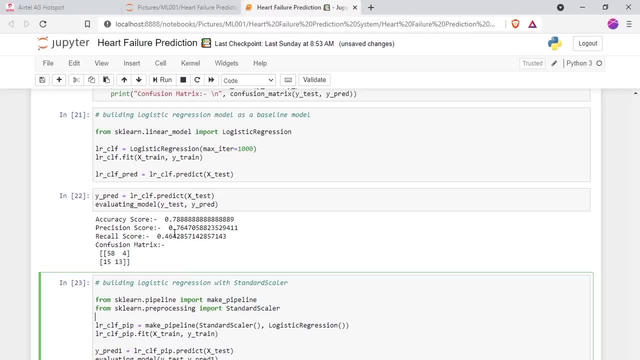 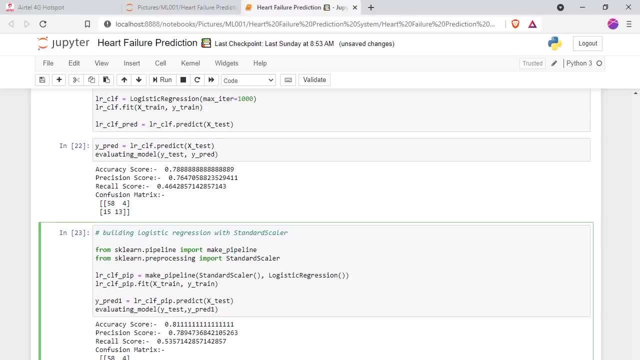 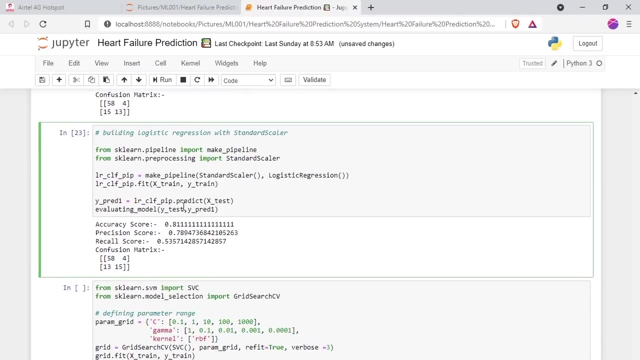 and that max iteration, So the accuracy is actually better. precision is also better, recall is also better and this is also better confusion matrix. So I hope that you watched my session on precision and recall, but let me show you what those precision and recall are. 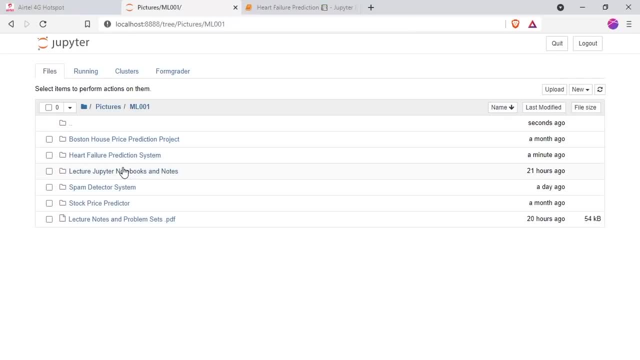 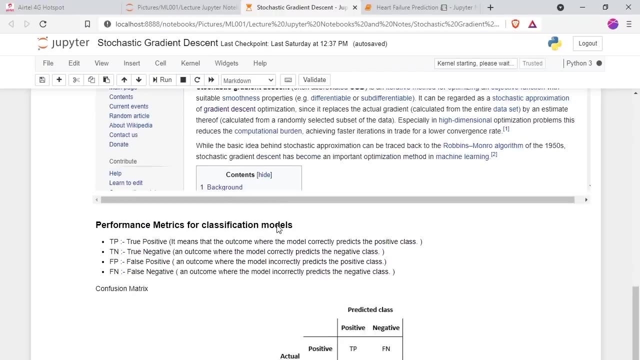 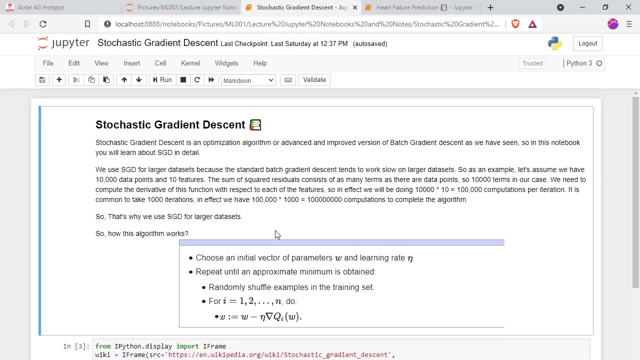 What does one recall? confusion matrix mean. So maybe I have this stochastic gradient descent, So we just want to make sure that you are on the same base. So here I am going to highlight one algorithm, which is optimization algorithm, which is same as our favorite gradient descent. 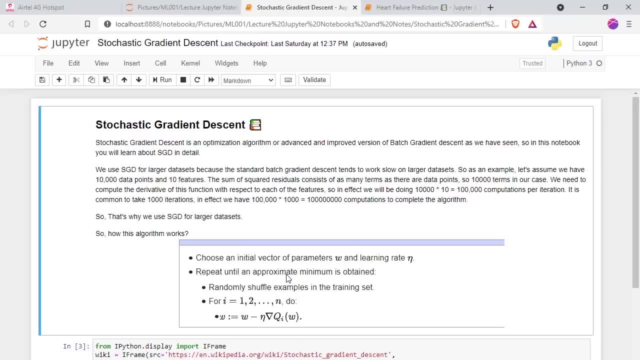 But here in gradient descent, what we were doing, it is taking a lot of time. Why it is taking a lot of time? So here, assume this example. Assume this example. I'm going to narrow it over here. Let's assume that you have a 10,000 data points, 10,000 data points, 10,000 data points and 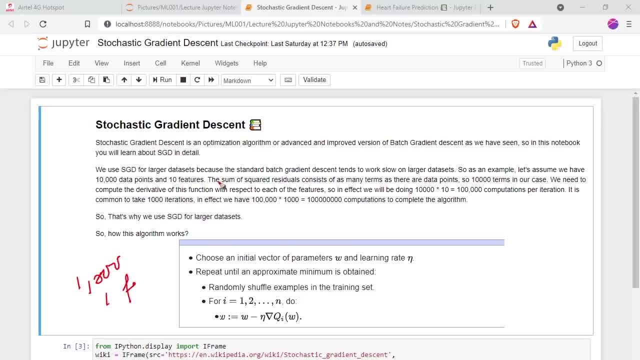 you have a 10 features. So here you have 10 features and the residuals consist of as many terms as their data points. So you have 10,000 residuals because we are taking the difference between your predicted and our model predicted model output value. 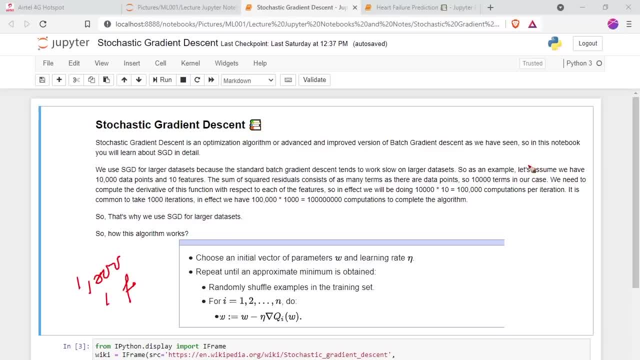 So you have around 10,000 terms, in our case, residuals, So we need to compute the derivative. We need to compute the derivative of the 10,000 terms. We need to compute the derivative of the 10,000 terms with respect to our features, which 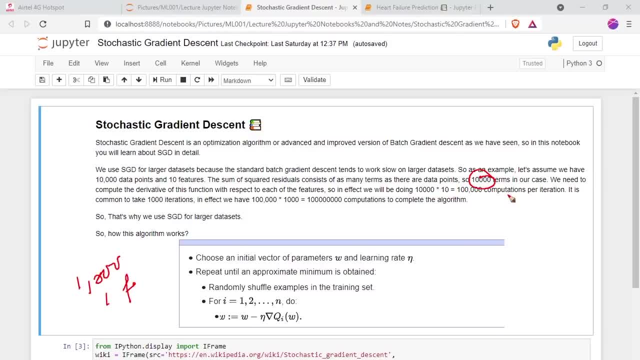 is 10,000 times 10, which is 1 lakh computation per iteration. That is so so much higher. So that's why we have something called as stochastic gradient descent. So what would we do in stochastic gradient descent? We choose simply, as the same thing happens. 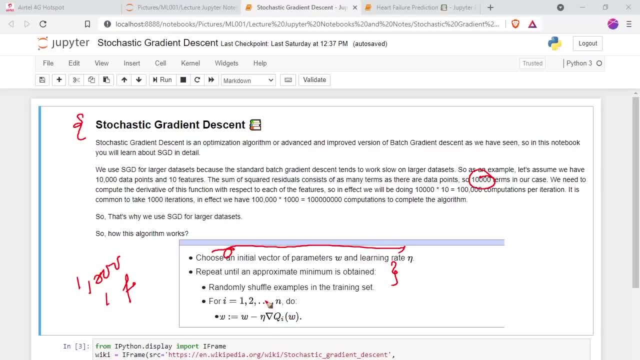 We repeat until and unless our approximation is minimized, and then we randomly shuffle, and then we do at each step. It means we act at only a step, So we don't update. We do updation, as well as the derivation, at each step and we are doing for each training. 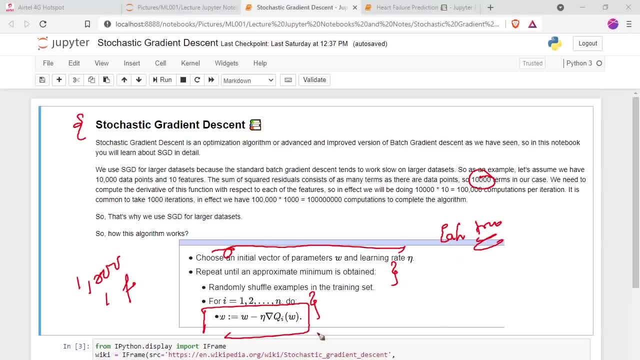 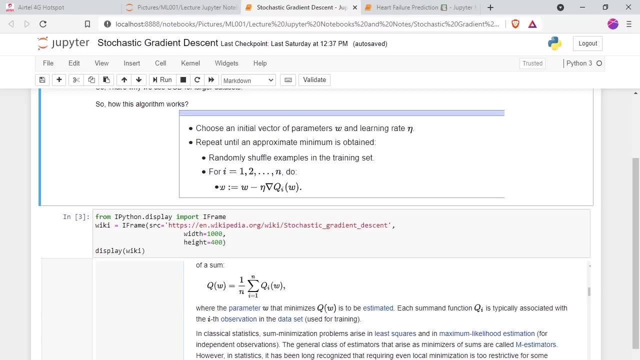 examples for each training examples. So it is a little bit out of the course. It is usually taught, maybe in deep learning, but I would highly recommend to learn this. This is just equal equals to batch gradient descent, So you will be able to see what's the difference. 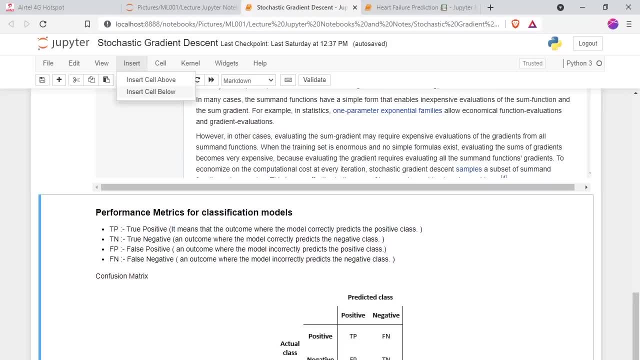 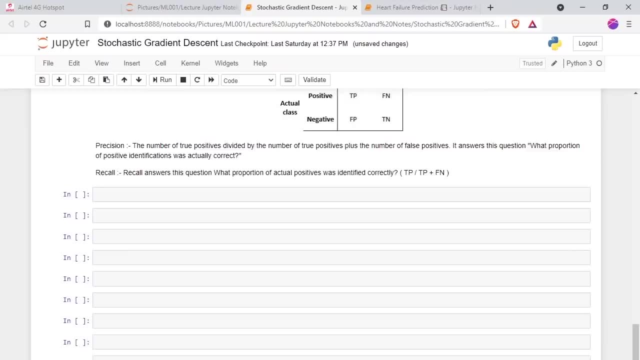 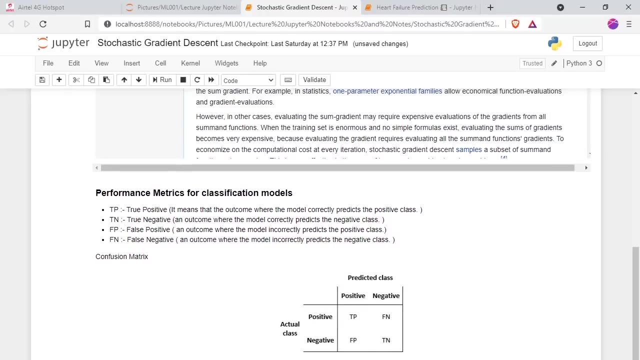 So now, as I have talked to you that we have something called as precision, recall, accuracy, So we have not talked about that, So let's talk about just to spend a little bit of amount of time on that. So here TP means true, positive. 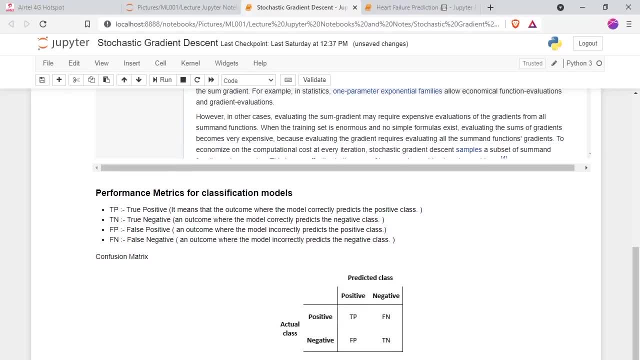 True. positive means that your outcome, That your outcome, That your model outcome, correctly predicts the positive class. So you have, in any model you have two positive and negative classes: Positive, negative classes, Like zero is a positive and one is a negative. So your model predicts the same output as your ground truth in a positive. for a positive. 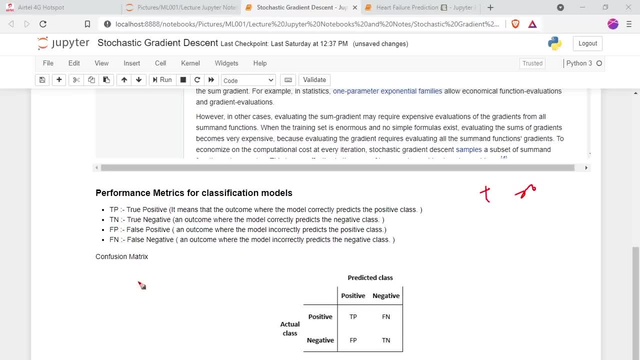 class. True negative is where your model predicted one and your output is also one. So you have positive and negative classes. True positive means zero and zero. These are positive class and these are negative class. Here you have false positive, which is your model. incorrectly, your model predicted your. 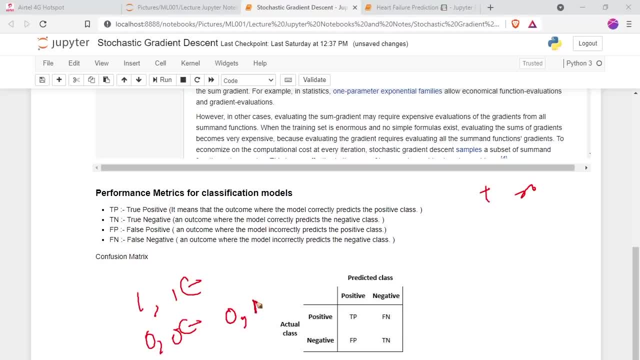 model predicted your zero and actually the output is one, So it is false. positive means positive and false because they are not matching False. negative is just the. it's your model. your model predicted. your model predicted wrongly, So your model predicted one and your output is actually zero. means negative and positive. 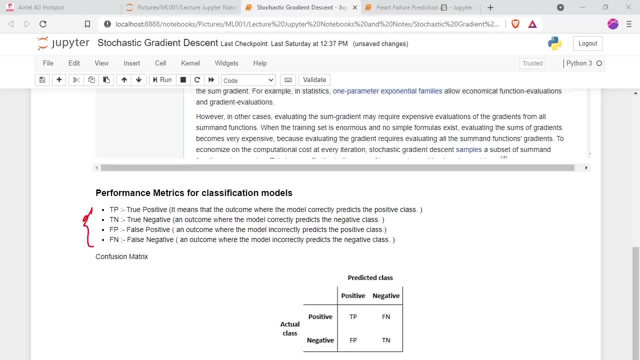 class. Okay, So that's the that's. that's the true, positive and negative and confusion matrix is simply like this: First we have a true positive, false negative, false positive and true negative That we have just seen. It will tell you how many number of are correctly classified as in a positive class, in a negative. 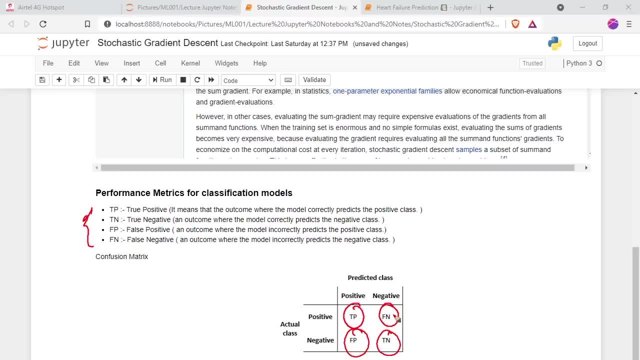 class, in a in a, but in the model model failed, in a positive class where the model failed. So again this, this is the true negative where the model actually worked. Okay, So you can see the we will. we have seen. 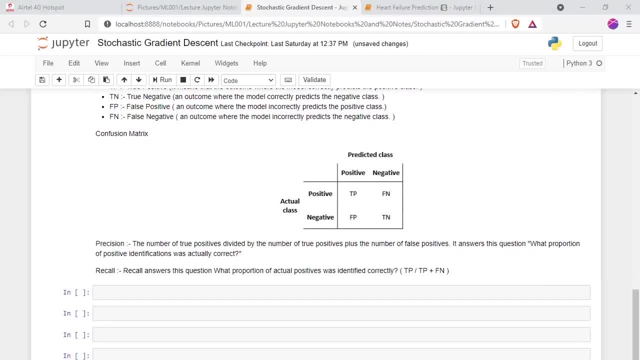 Okay, So Precision, Recall, As we have talked about Precision and Recall, the number of a true positive divided by the number of a true positive, divided by the number of a true positive plus the number of a false positive. So true positives, Tp plot by Tp divided by the number of a true positive plus the number. 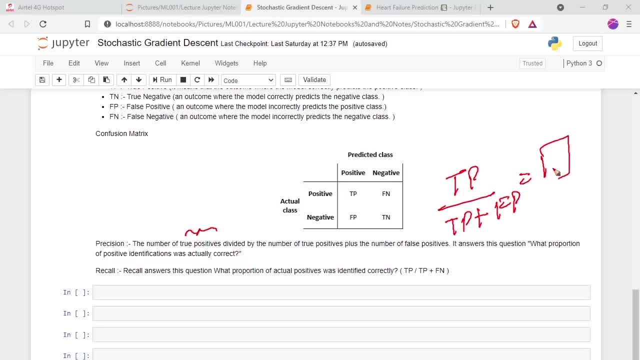 of a false positive. Okay, your output. this is your output of the preseason. it simply answer the question: what proportion of positive indications was actually correct? okay, so it answer what proportion. so here we have 0.73, which actually good proportion, but we had. it can be improved. the equal answer the question: what proportion of actual 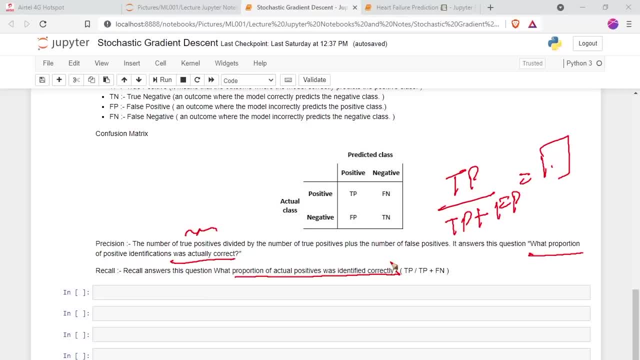 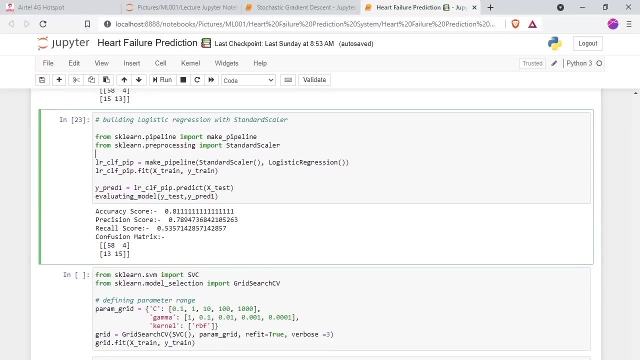 positive was identified correctly, okay, okay, so it will tell you that what is the proportion of actual positives was identified correctly, okay, so this is the easy recall of our model. okay, so now we will see. now we will see, just just we will see the back, that the preseason we call confusion, matrix, and cetera. okay so, 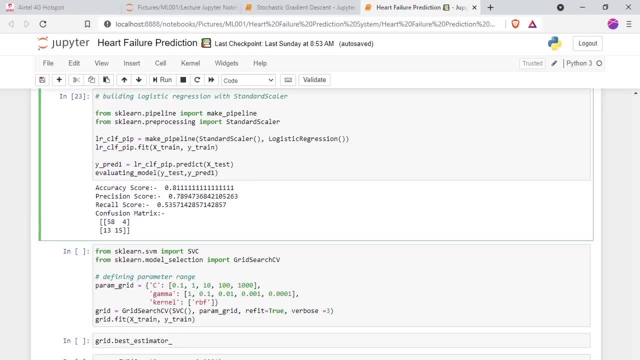 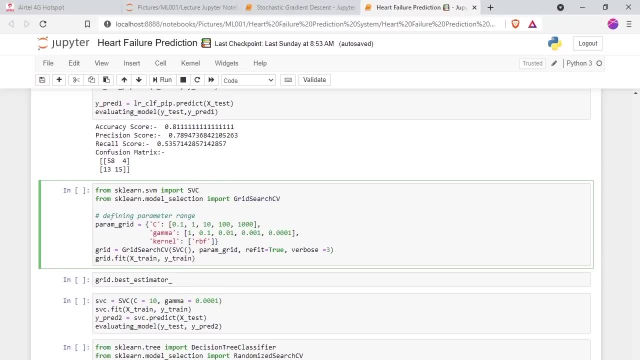 now you'll see, now we have built all the determination with some standardization. now we'll build a support, better classifier with the grid search CV, with extensive fine-tuning. we have to see which is lambda, which switcher equipment controls the width of the margin. so it is very easy to define the condition of the model. so it has since. 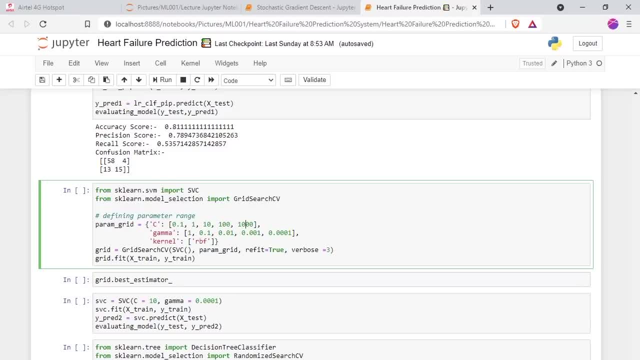 So we'll try different differences: 0.1, 1, 10, 100, 1,000, gamma: 1, 0.1, 0.1, 0, 0, 0.1, and kernel to be RBF kernel. 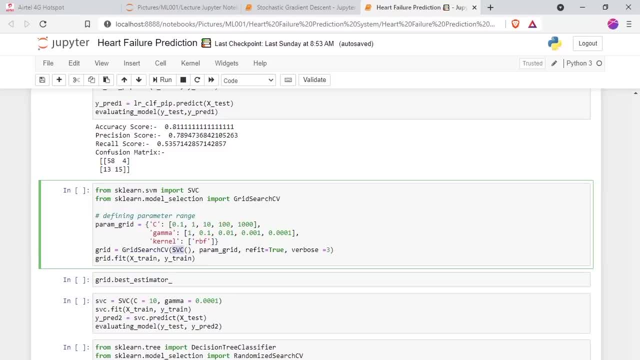 And then I will call the grid source instantiate with SVC classifier: RAM: grid ref equals to verbose, equals to 3.. I'm going to fit it. It will try for each entry and check the score, And this is what the thing is. 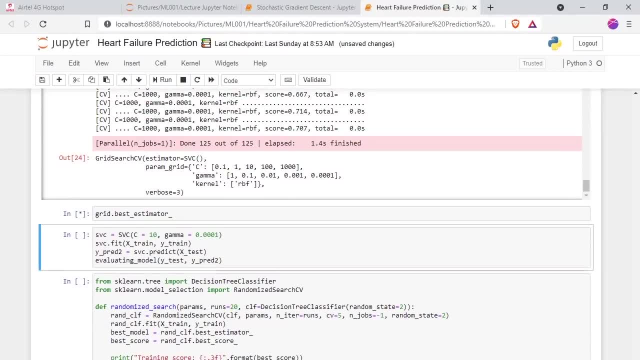 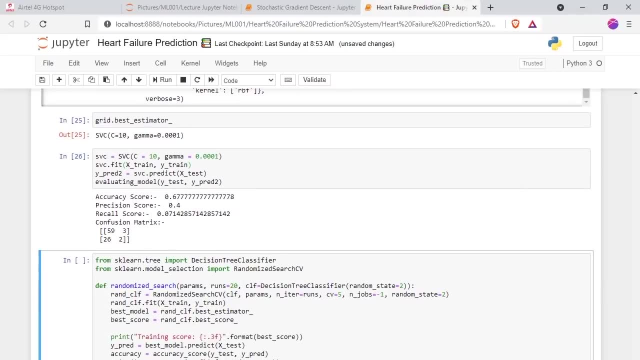 They have done, They have checked And you can find the best parameter that the model found where C equals to 10 and gamma equals to 0.001.. You can see it far performs a little bit less compared to logistic regression, but it worked. 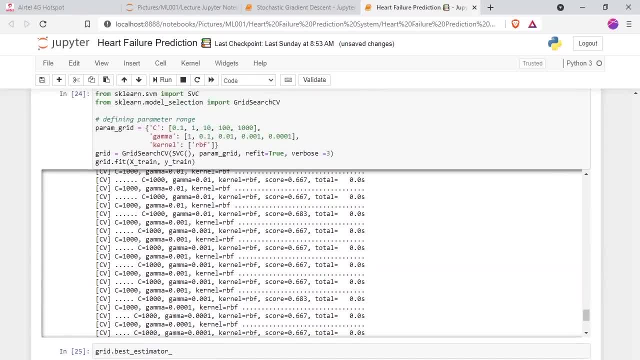 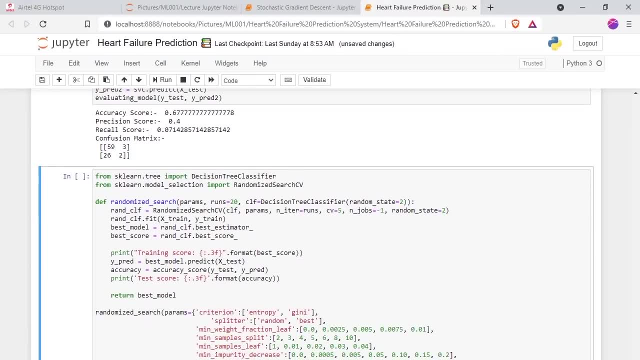 So we have done with the support vector-vector classifier as well as logistic regression classifier. Now, what we will do, we will make a decision tree classifier. So what do I mean? What I mean by decision tree classifier is: I'm going to import- as we have already talked in detail, I'm going to import a randomized search. 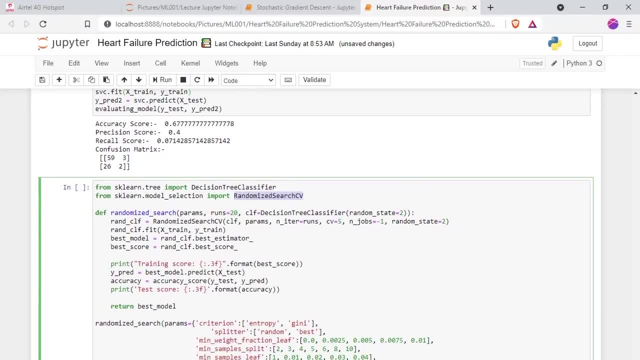 We have talked about grid search. Randomized search is the same. So I'm going to define a function that takes the parameters, takes how many runs to CLF, what the classifier to use. Then we will call a randomized on CLF. 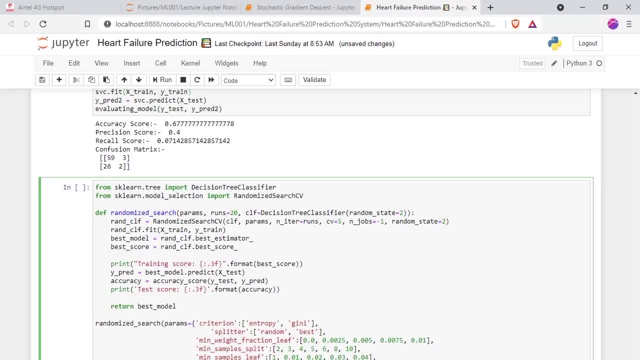 First we will give the CLF, which is classification, number of iterations, et cetera, Then we will fit it, Then we will find the best parameter, Then we will find the best score, And then we will say this: and this is just a custom model, but you can surely remove that and just use that randomized search and then put all these. 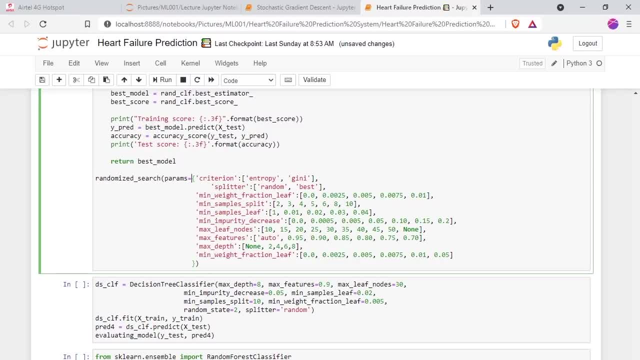 So I have already done it in some of my projects. I've just taken out from there and it's working great. So it will tell which is the best, which criterion is the best, whether it's entropy or Gini or splitter or mean weight. 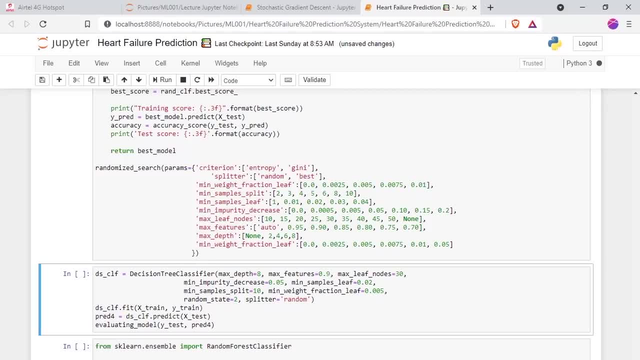 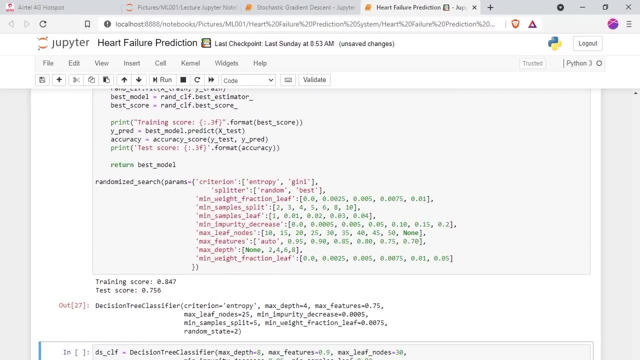 I have done a lot of fine tuning. I will run it. It will take a little bit of time trying all the values and checking This score and you can see the training score is 0.84, and the test score is 0.75, okay. 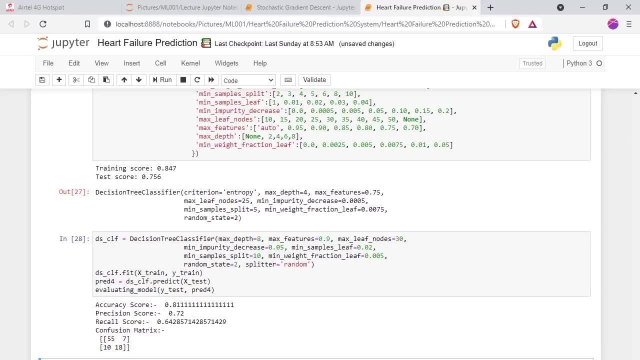 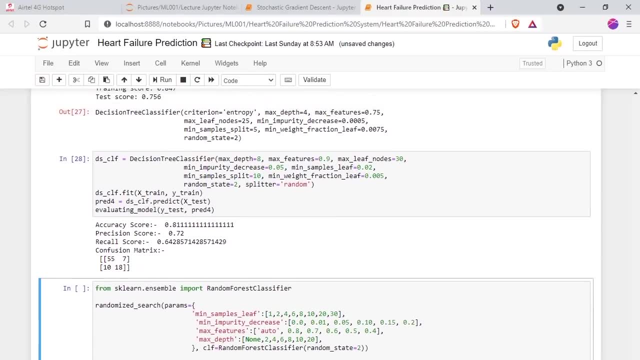 Now we will run this classifier with the same, with these features. okay, So it will give me the output like this: Now I will, oops, now I will run it out. Maybe you can see. okay, So you can see how well it is performing. 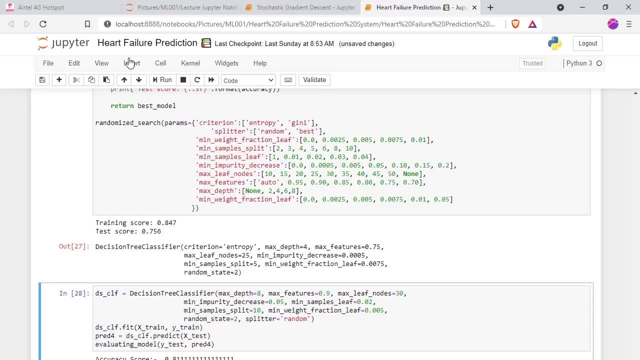 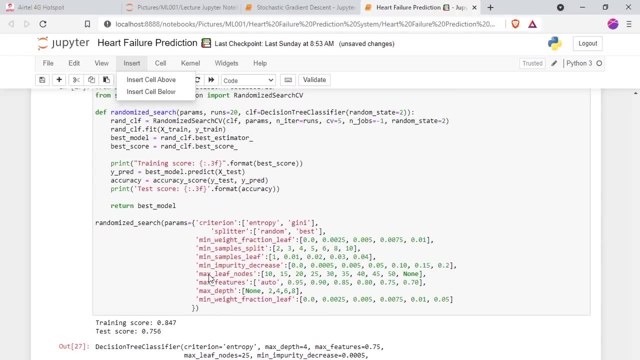 Maybe I have not. Let's see the best score. randomized search: best score: Okay, maybe. yeah, so that's the basic and you can also try it out. Maybe I'm a little bit, you can see. let's see if it is not good or not. 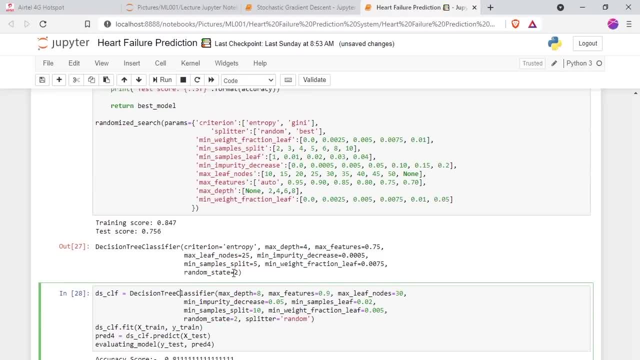 Oops, I have to also show okay, So it is showing the best classifier, so I have to put it over here. I don't know why I put it over here, but what I have put it now in what mine. but I will let me put it. 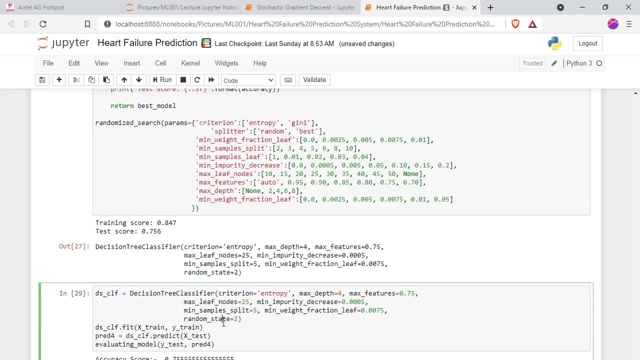 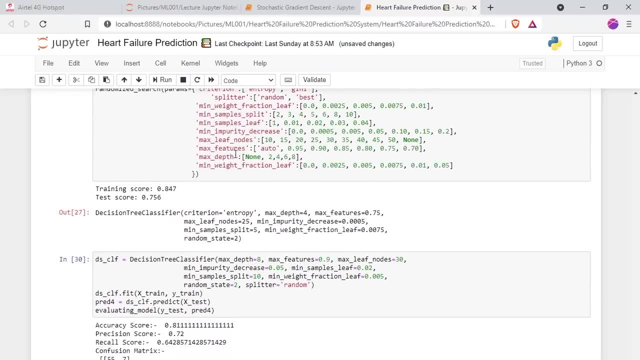 Okay, let's run it. It's actually 0.75, so I have. I have obviously done some fine tuning and here what I got with a good parameter okay. So it's not always this works best. In some of the cases it worked okay. 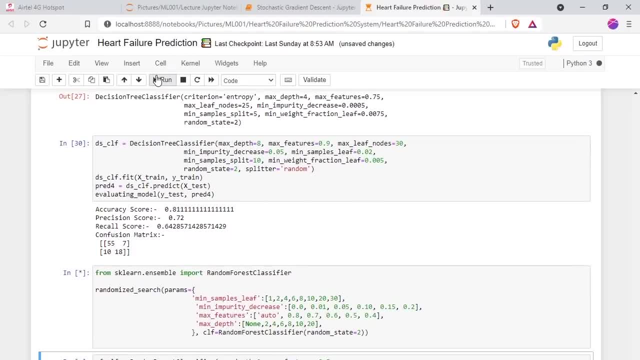 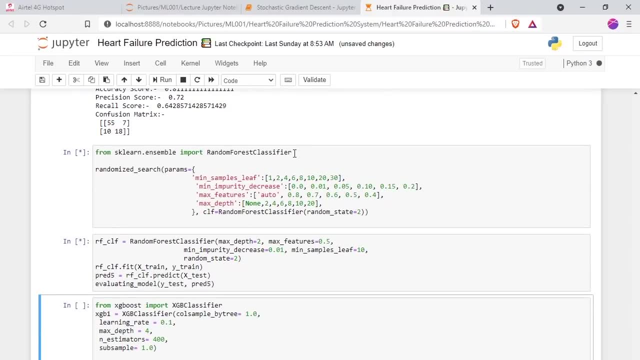 So now, with a little bit of fine tuning, I'm going to call a random forest classifier, Then I'm going to run it with a parameter stack that we got with a random forest. okay, It will evaluate my model, and then 0.86, 0.10, actually good, okay. 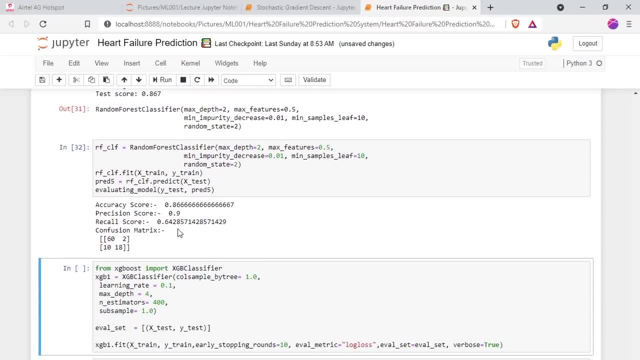 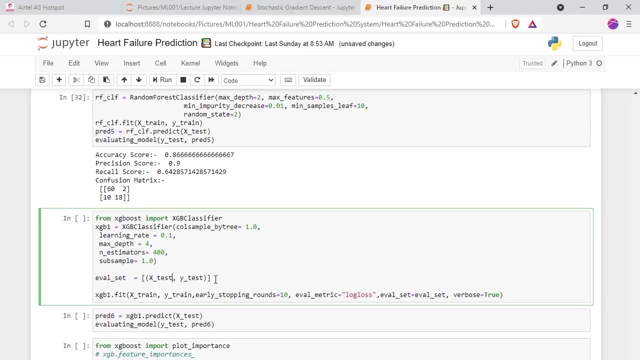 Now what we'll do. we will use XGBoost. Okay, XGBoost is another we have talked about. We're learning by 0.1 max step. what is the number of parameters? Then I'm going to put evaluation set into one array, okay. 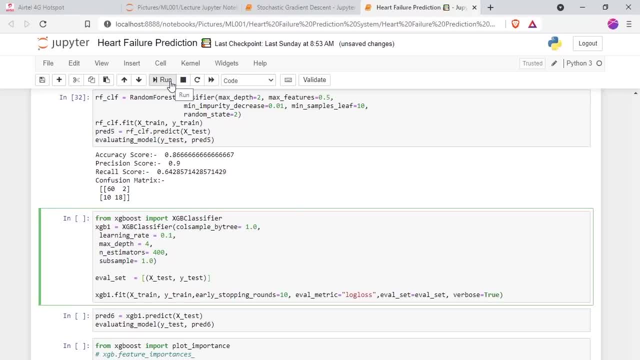 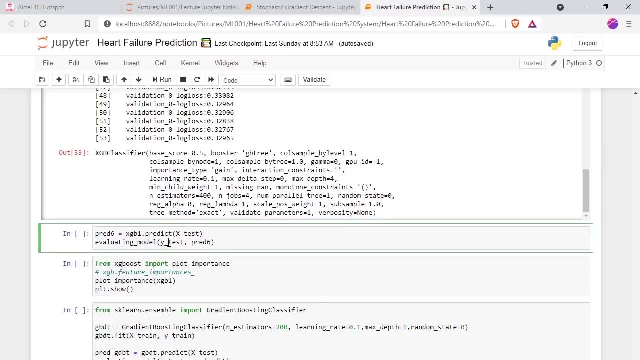 So just see the log loss at the same time and then I'm going to run it So it will tell at the log loss of the zero iteration and 0.32 is the log loss, validation loss: okay, Now it will evaluate and here again, 0.85 is more robust model, okay. 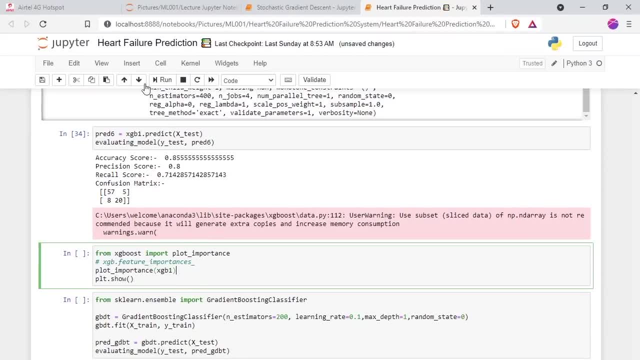 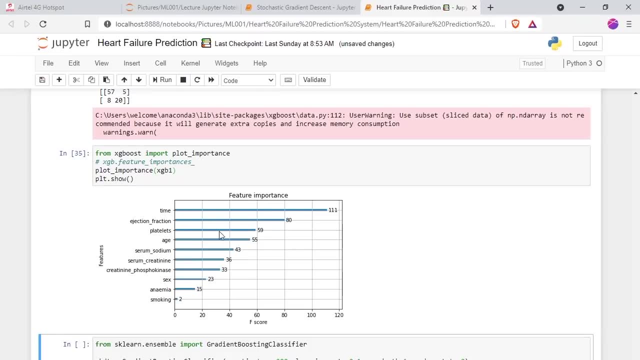 It is a robust model. If you can see the importance, it will show what features are more important. So time is very important, injection is very important. So in this way you can select, you can discriminate. so maybe smoking, anemia, sex, creatine, 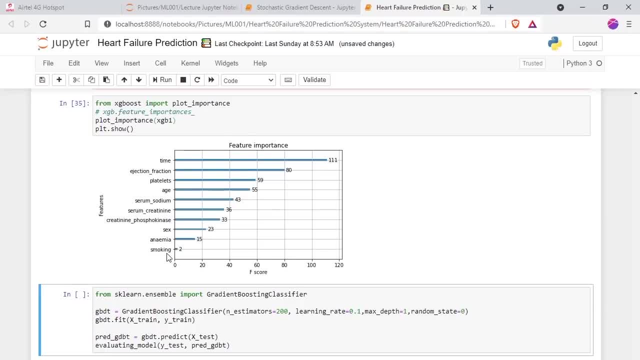 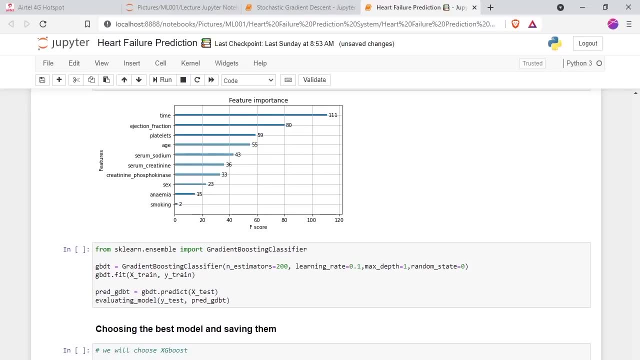 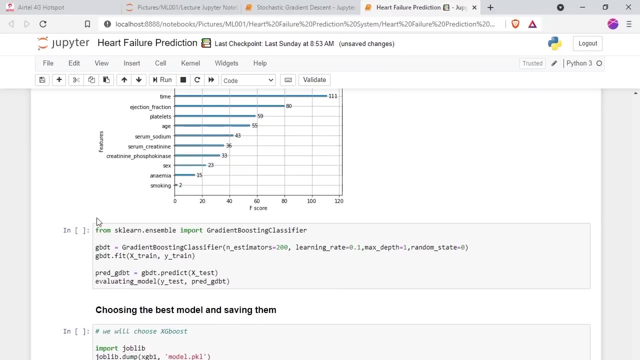 and then these three you can remove as a feature selection. okay, The last thing that we are going to use is a Gervarion boosting classifier. Gervarion boosting is mostly used in cases of- in many cases, but let's see here how well it works with these hyperparameters. 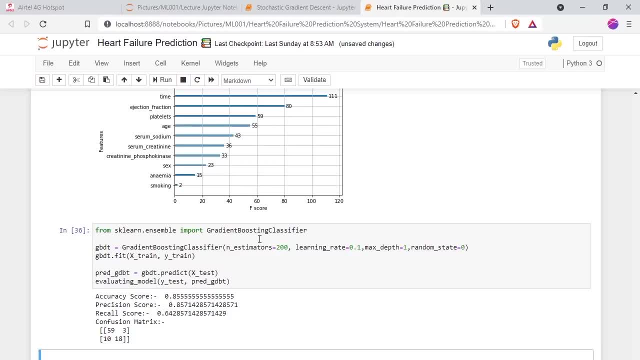 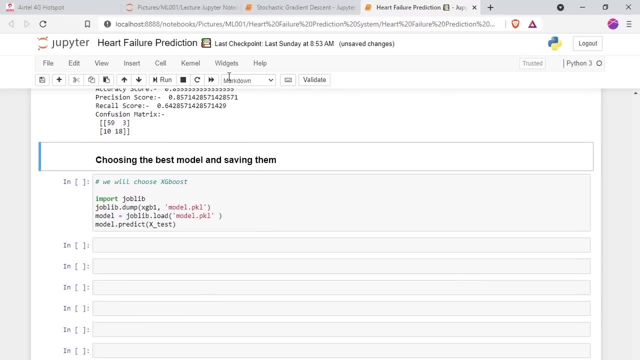 You can also fine tune it to get better results than me, and it actually worked. okay, Now what I will do? I will save my XGBoost model because XGBoost is more robust, So I will save my model by just calling for joblib- joblibdump. 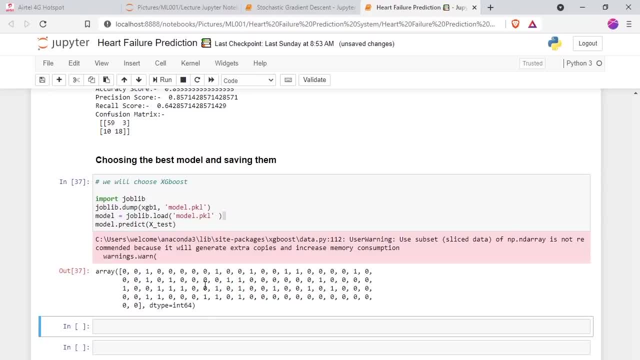 I'm going to load my joblib If you can see if I run it now. you can see that 0, 0, 1.. And you can see if I go over here, if I go over my word failure. 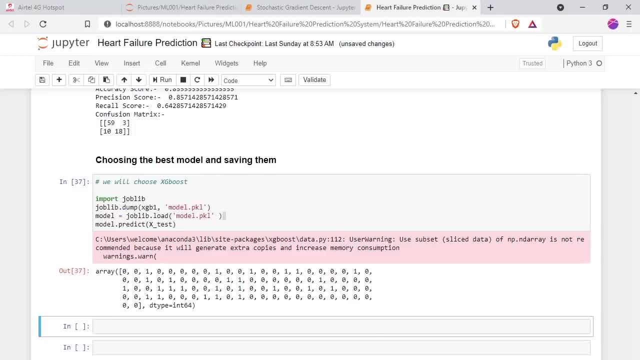 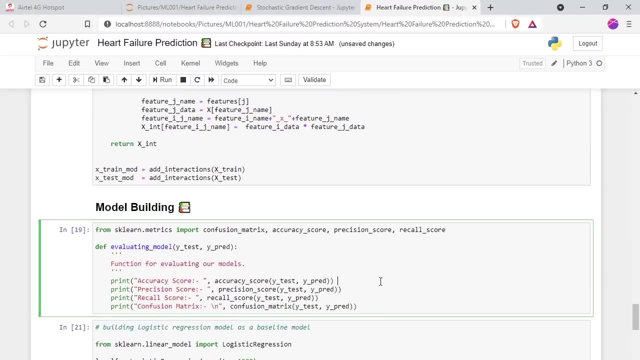 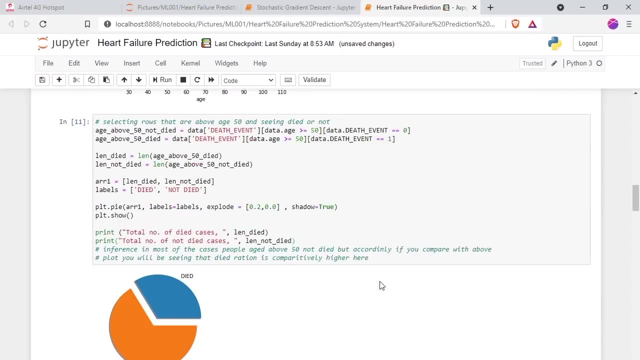 and modelpkl file and you can load this modelpkl file to make a good model, okay. So that's the, that's our. that's a basic thing that we need to understand about that. we need to understand about this hot failure detection system. 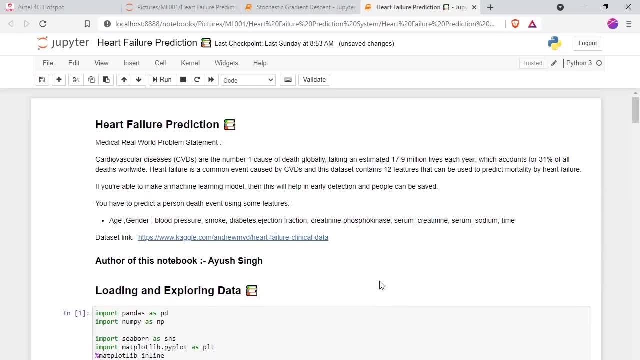 and I hope that you have understood a lot from this. Okay, so thank you for seeing this section and I really hope that you enjoyed this and you have covered this project. We'll see you in 42 minutes. In the next project, we will be talking about a small project. 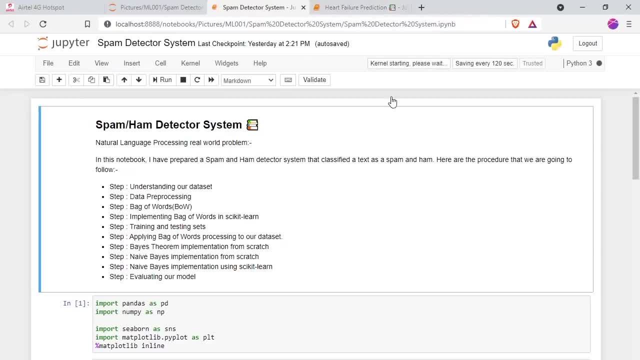 Spam Detector System, which is again a very cool project, which is understanding, problem statement and building a good model. okay, So let's meet at the next project. Till then, have a good day. So now we'll talk about, or we will make one project. 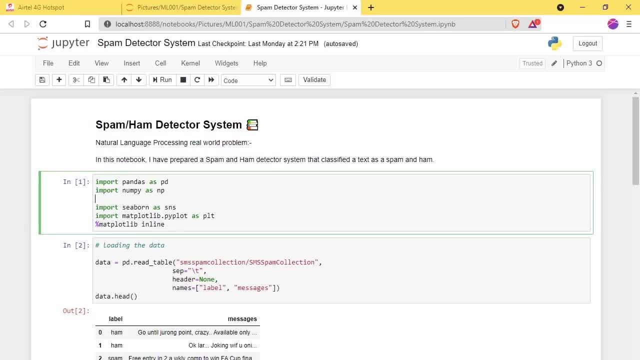 which is Spam Enhanced Detector System. So if you have seen your Gmail or Google Gmail or Microsoft Outlook there, you are seeing that there may be. you have a tab which is Spam tab, where all your spam emails are there. So in the same way, we are going to build a Spam Enhanced Detector System. 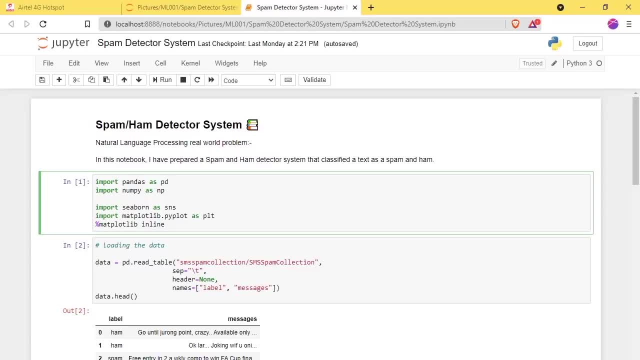 So Spam means means that a particular message may be corrupt, and Ham means not a spam, just opposite to spam, okay. So just Ham means not a spam. I don't know why it does not work for the first time. not a spam, okay. 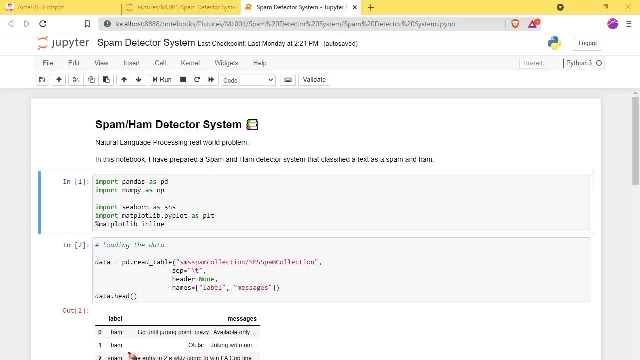 And here you can see that that we have a label means we are given a message. we are given a message and we are given the target label, which is our Y. okay, So this is our message. maybe go until journey point- crazy. 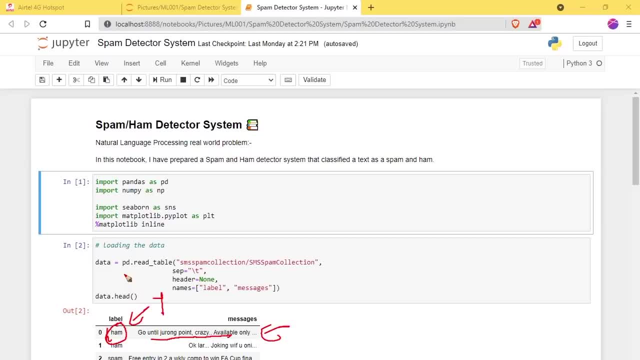 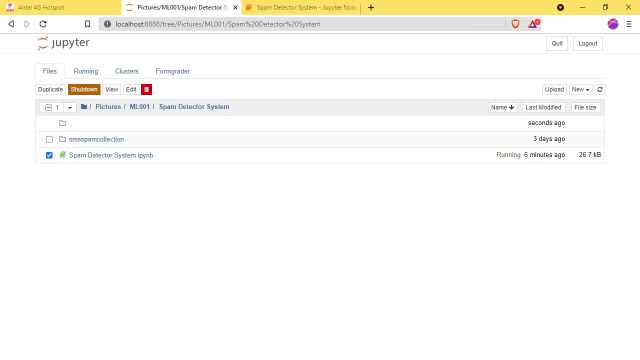 and then there is a label which is given over there, okay, And this data set is downloaded. this data set is downloaded from UCI repository and here is our data data set. So it is in table. so I'm not going to use CSV. 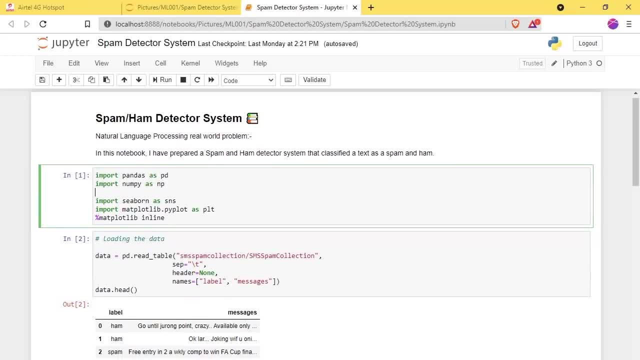 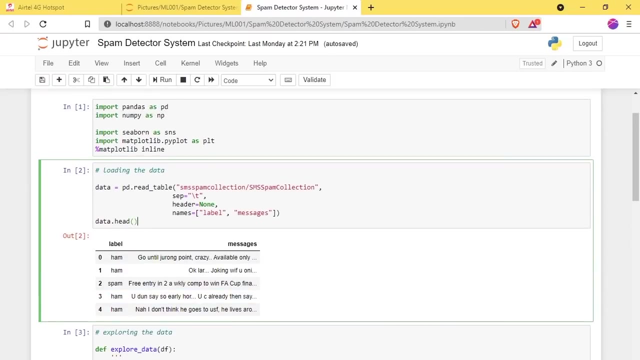 I'm going to use table to read that I'm going to separate by a tab. header should be none and the names of the columns should be labeled and messages. Okay, so let's take a look at. we will take a look at the first few data points. 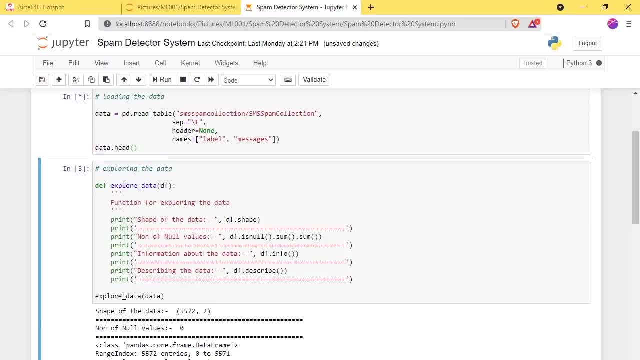 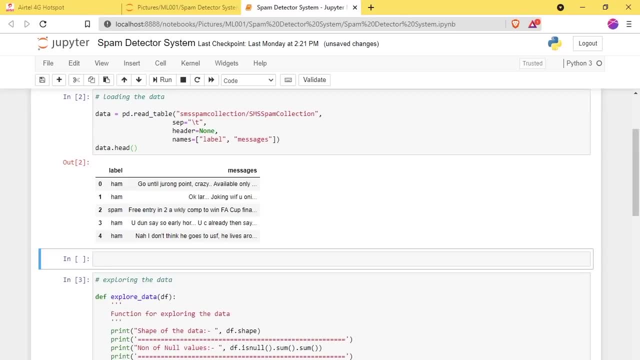 So let me run this out: first of all this, and then this, And then I'm going to show you one of the messages there, so it should start making sense to you. So here, data- oops, what happened? Data, and then this is the messages. it will take a little bit of time. 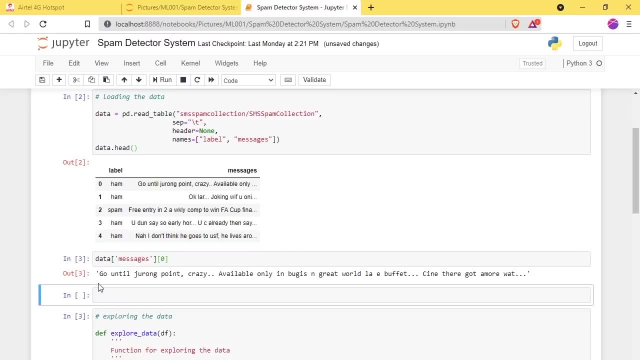 then zero position. so you can see that go until journey point crazy available one, et cetera, et cetera. and here it says that this is a ham, which means not a spam. So for an example, let's assume this second number. 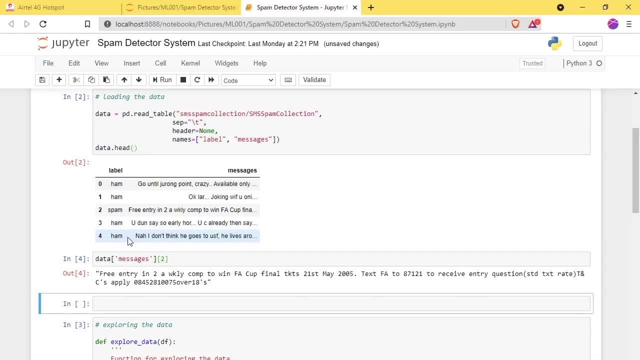 because in second number we have it labeled as a spam, so free entry. it's looking like a spam, like it's free entry or like that. Okay, So that is the. that's. that's the basic. that's the basic exploration of our data. 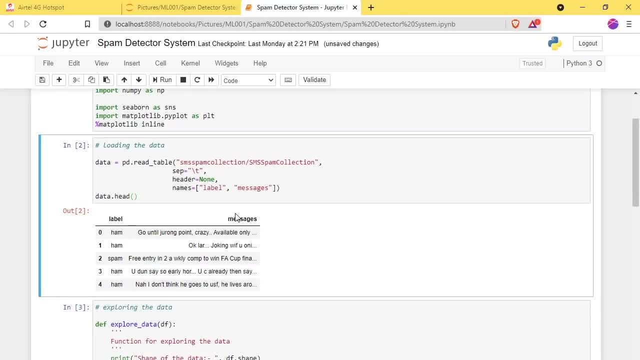 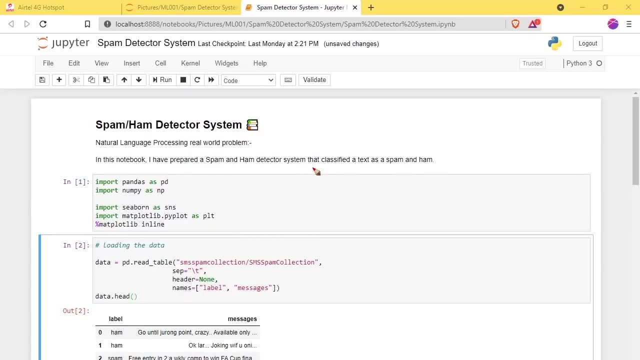 and this is downloaded from UCI repository. Okay, So I think that you, that you understood. we are given a corpus for test, so here we are not given any numbers Here, and we are given here, Okay, Here we are not given any number. 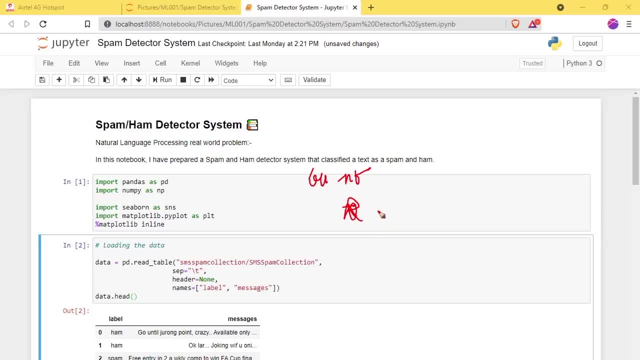 We are given: oops, what happened? what is happening? We are given a messages which is X as a messages which is in text format. So your neural network or, I'm sorry, machine learning model, does not work with text. 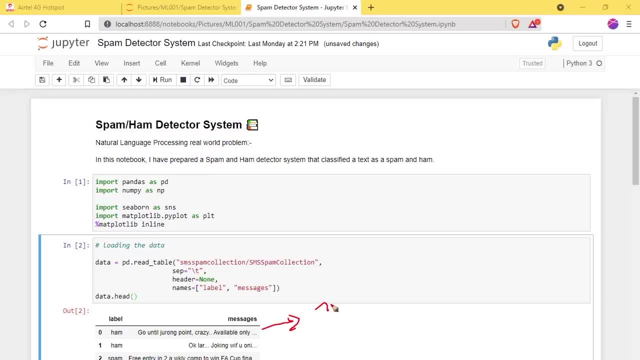 So you have to convert the text into numbers. So we will see some of our favorite text text: a vectorizer to convert this corpus of a test into a matrix or a vector or a number of vectors. We will see that. We will see that. 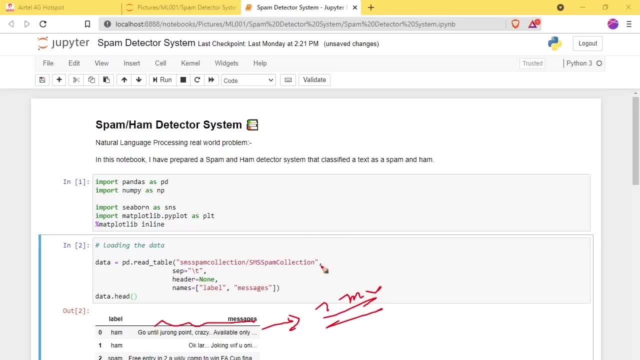 Okay, So here you can see that what here we are given a data which is text and this one, and then we have a label. Okay, So now we'll see. now we'll start exploring our data set. So now we have got our problem statement that we are given a corpus called text. 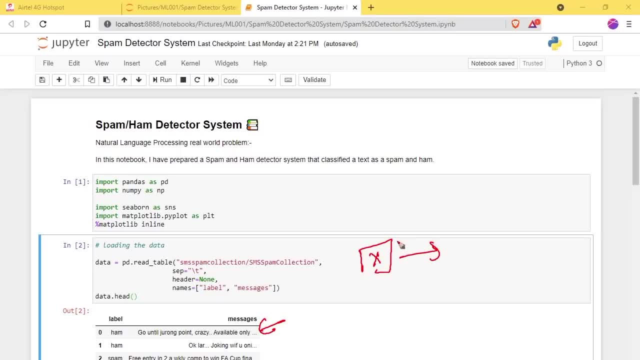 We are given a text and we need to. we need to pass it to pipeline and give it to our output, whether it is a ham or a spam, or ham and zero Okay. spam means one okay, so that's that's that. that's the our favorite given now. 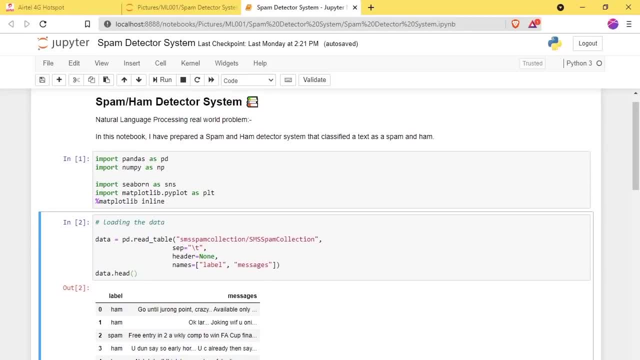 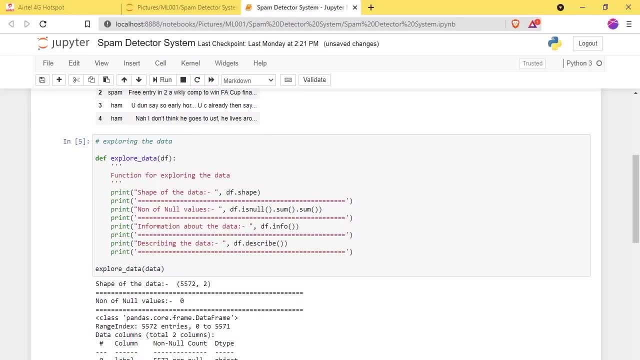 we will move forward now, and I will move forward- and to exploring our data. so I've already explored it, so let me read on it again. so here, I hope that you all are able to see this, so maybe you- and if you cannot, don't, don't worry, I will just 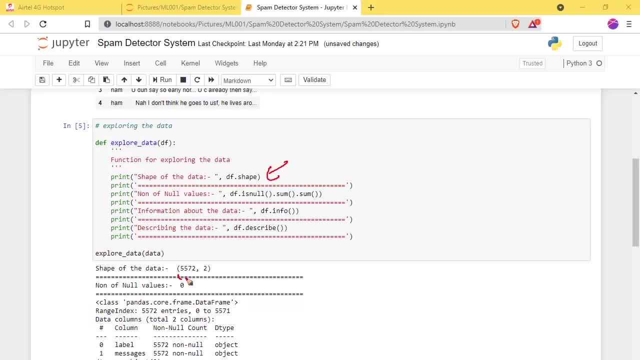 we're going to take a look at a shape of the data which is five thousand seven hundred and seventy two. five thousand five hundred and seventy two with two columns, and then we have a no values to be zero, because we don't have any no values. we have two inflows and here, which is a count, unique values. what is? 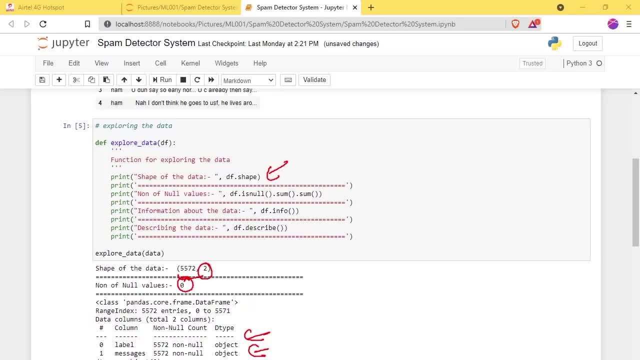 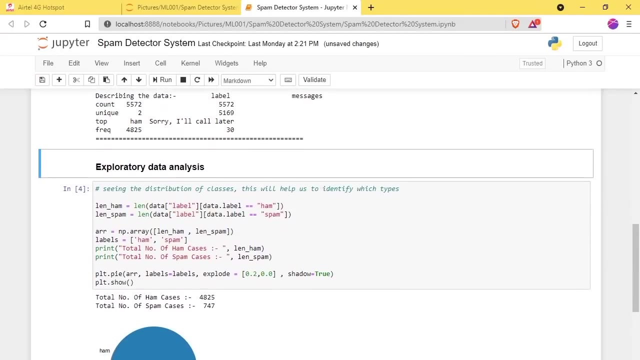 the frequency and set right, obviously, the text. we do. you don't have numerical things, so that's why it's it's empty. okay, great, so we explored the data very much. now it's time to again start with Explorer. it's exploratory data analysis. okay, so in exploratory data. 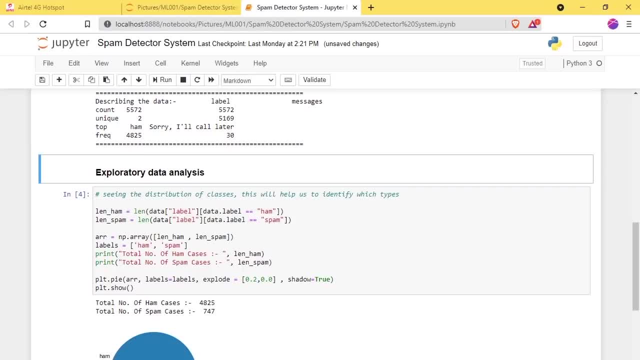 analysis we end up in our previous project. we have seen that. we have seen that we have to see the distribution. we have to see the distribution. you have to see the distribution of the classes. okay, so here we are seeing the distribution of the classes by just taking out the length and converting that into a length. 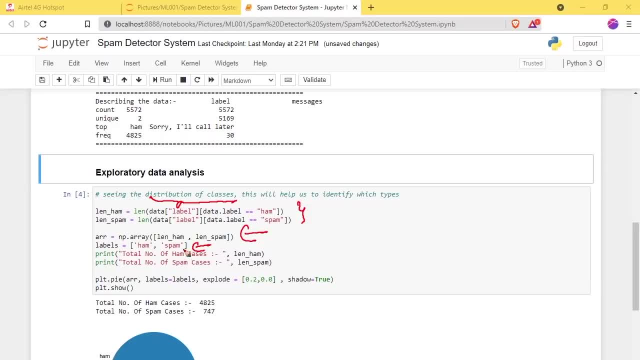 now, now, here you can see the labels, which is hammer, spam, and it will tell what is the number of the total labels. with the plotting, the pie chart, and you can see OBO, that the number of ham examples is four thousand eight hundred and twenty five and spam examples at seven hundred and forty seven. so we are 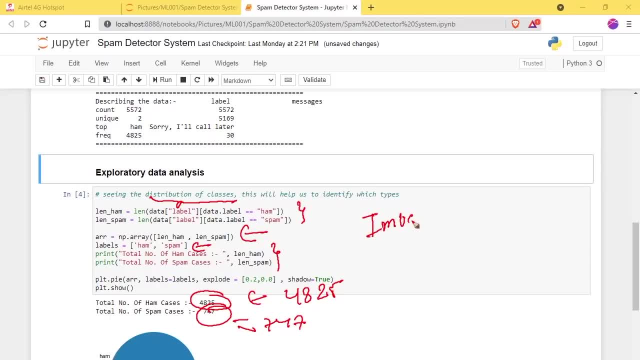 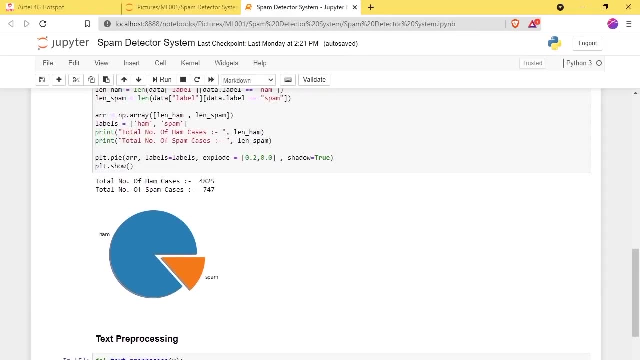 actually working on imbalanced. we are actually working on imbalanced data, so your model will learn a more about time rather than spam, okay, so be sure to keep that in mind. next we will. now it's it's very, very important, like for an example. so let's, let's under understand the 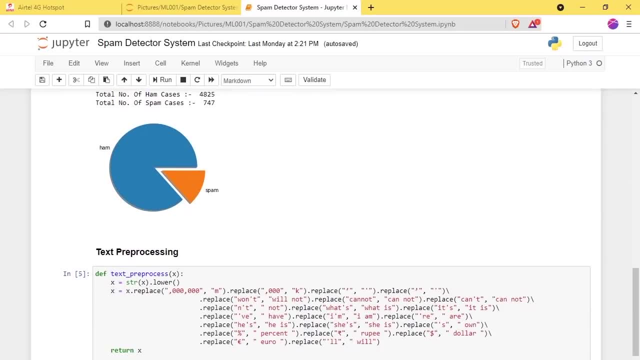 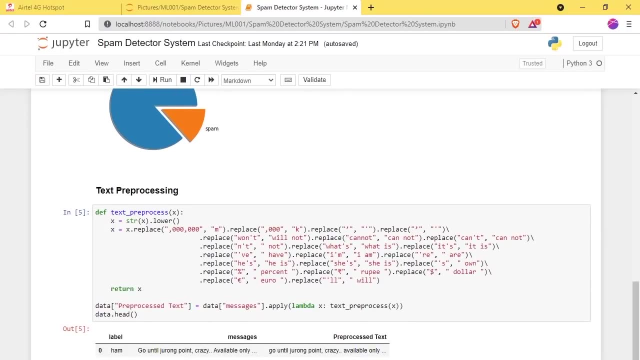 processing of a text, how well how we clean our text and why it is. why it is there a lot more need. so why do I mean like? what do I mean? my cleaning is, for an example, let's assume that you have a goal, okay. so here you have go, oops, go, okay, small g. I don't know why it is not working. 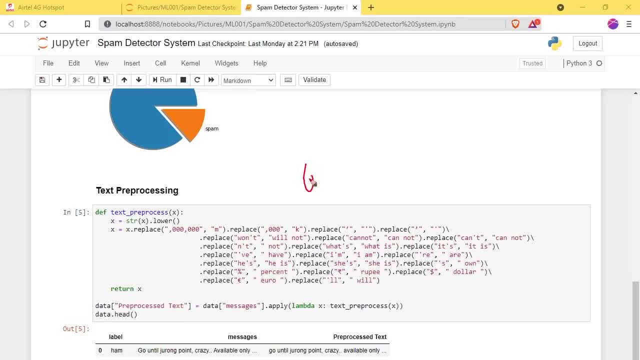 again, I like: okay, so here you have go, here you have go. okay, says this: this small: oh okay, so these two will be considered different. these two will be considered different, but this is the same. this two will can will be considered different, but this is, this is the same, or maybe this hashtag will be considered. 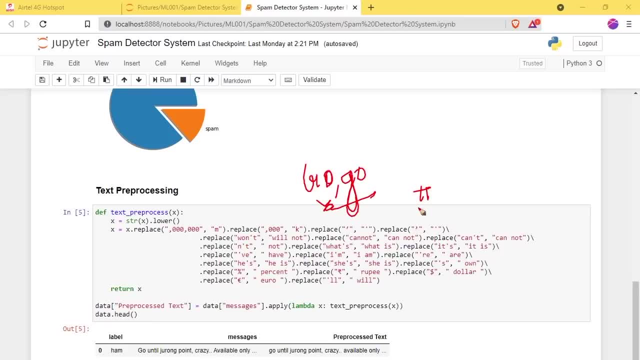 different, or maybe this hashtag will be considered different, but this is the same. so you have to think before you go here. okay, so let's say here: so maybe this hashtag does not need an essential bio, so why do we need hashtag over you all? maybe we don't need like this, we don't need emojis, but here, but in some cases, 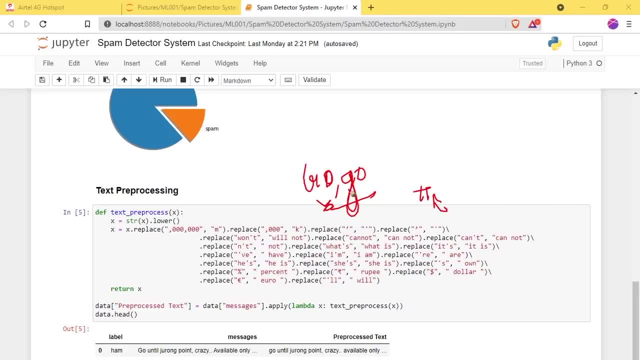 like incentive analysis, we space in a modern role. but here we are, go and go are similar thing. maybe here we have a bit, here we have a these, this team, if we, if it needs to be model, these two would be considered differently. so that's, that's not a good thing. 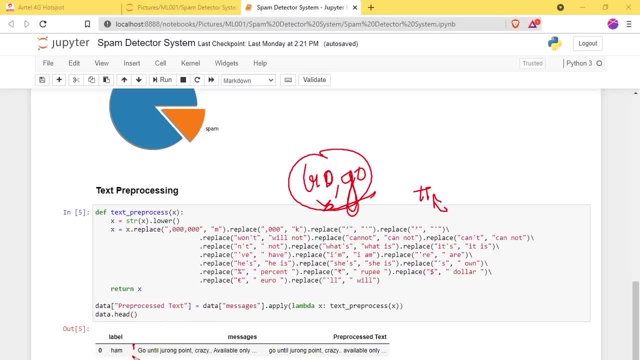 what we will do. we will convert all our text and to lower text. okay, now here we are doing some text pre-processing that you need to know. okay, just just using re, okay, rejects, okay. so I'm going to replace here and I'll be given one simple message. I'll be given one simple message first of all. okay, I'm going to 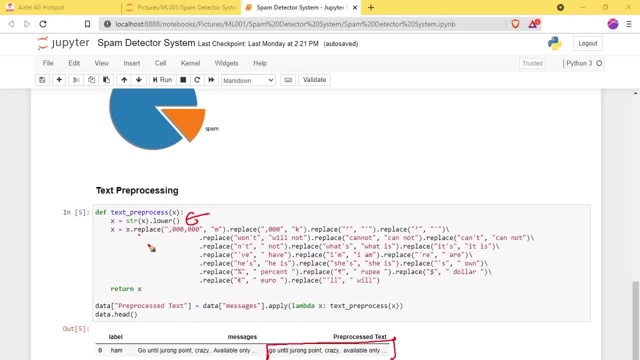 first lower it down by converting that into a string. then I'm going to replace this: this 0- if there is any- 0 to the text will be replaced by M. okay, and this: this 3 will be replaced by K, and K is thousand K or 100 K or what whatever. 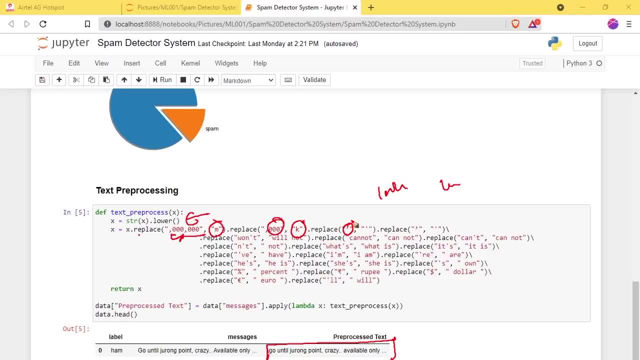 this. this comma will be replaced by this: sorry, the above I am NOT recalling was the name and is. I'm sorry it's it's, I'm not recalling, but yeah, you can see. okay, so then you have won't will be here. it will become different, so will not. okay, can not, should be, can not, can't. 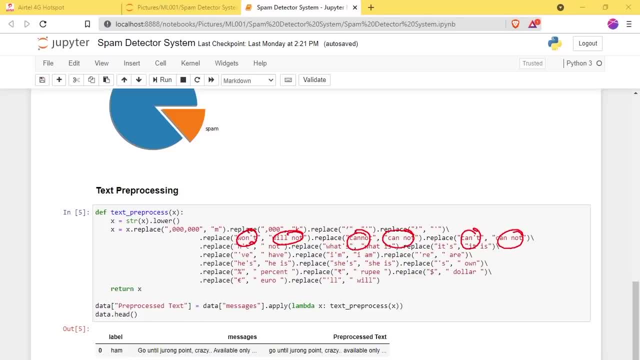 should be, cannot. okay, he we have, we are just doing and not he was not what's, what is, is it's, it is. then every is he is, she is, she is s own percentage, then etc. and then here L will okay. so this is the big. this is the basic text, pre-processing. 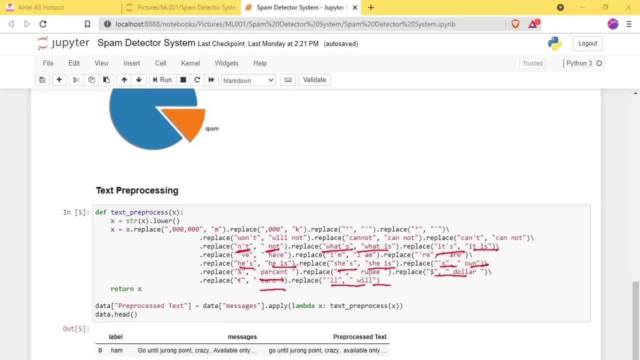 Reprocessing that I've done over here, but one thing that I can also do over here, one thing that I can also do over here, Like for stemming: stemming, okay, stemming, lemmatization, Lemmatization, lemmatization. so I would like you to explore this. 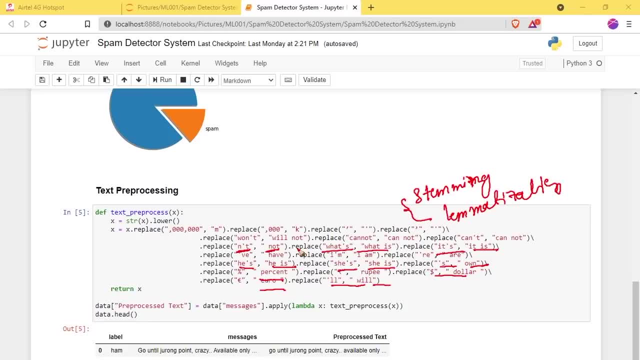 I would like you to explore both of them in implement of a hope. okay, and Why? what? first of all, let let let me tell you what is stemming okay. So stemming, it simply means, and it's, it's in stemming. it simply means that, For an example, for an example: so, if I go to some website, 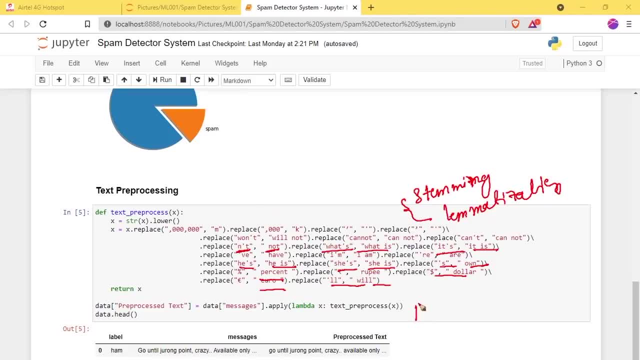 Let's take an example: that I write play, that I write play, I write P, l, a, y, e, d, then I write player. Okay, so it will. it will the other stemming will give play and means these three quote can become will. will become It to this single word, because they make a similar sense. 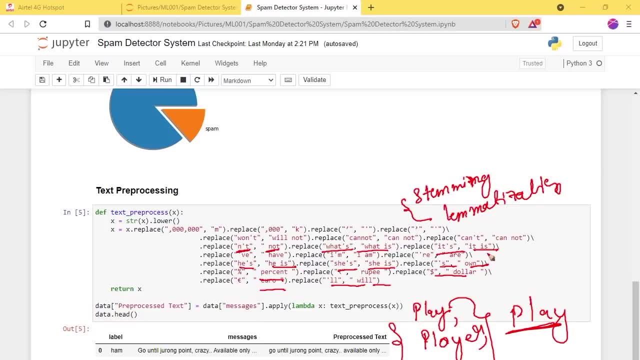 Okay, so that's the stemming, and Lemmatization is just a bigger version of that. it makes a meaningful some. sometimes a stemming does not make a meaningful Word, so for making a meaningful, meaningful word we have lemmatization. but again Lemmatization. what is just so? for example, plays: 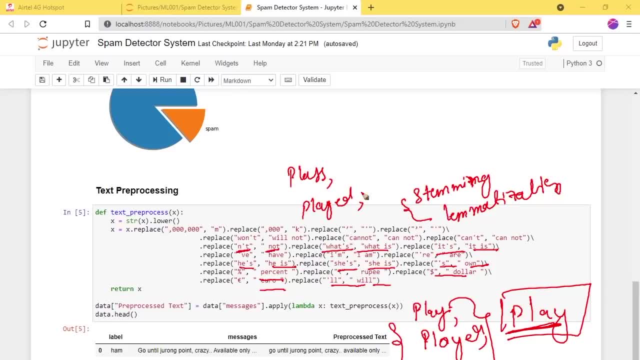 plays, plates played and players. so it will convert in play and Simultaneously the stemming will convert in plot. okay, so it does not make a sense, But this lemmatization is making sense. after we lemon eyes, our word, What will avoid? or be? convert our part into a word, into a single word. okay, 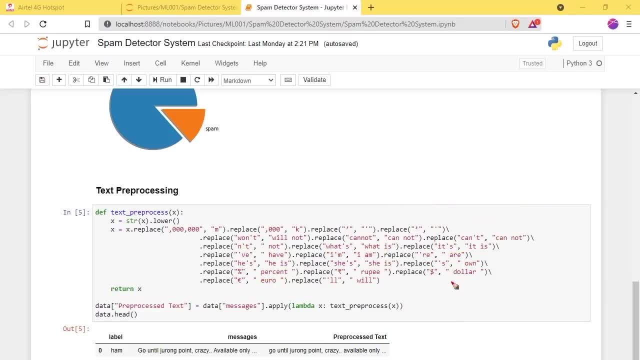 So that's the semi-laboratization, but I want you to explore stemming the word Systemic Lemmatization using an L? p library. you can reference some of my get up. I've already done that, but I want you to do this, okay. 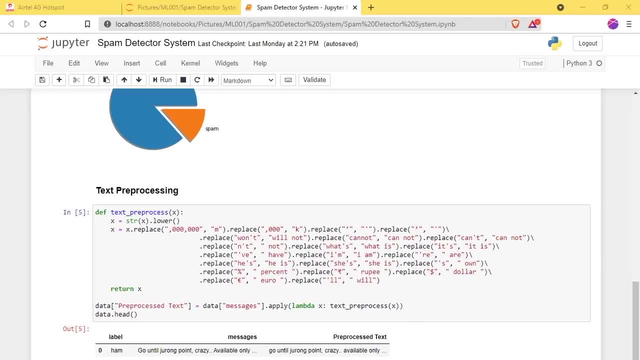 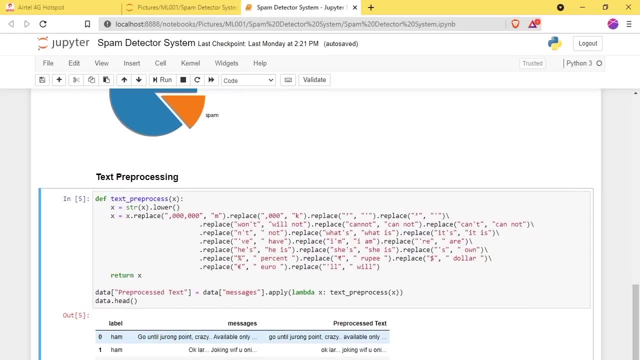 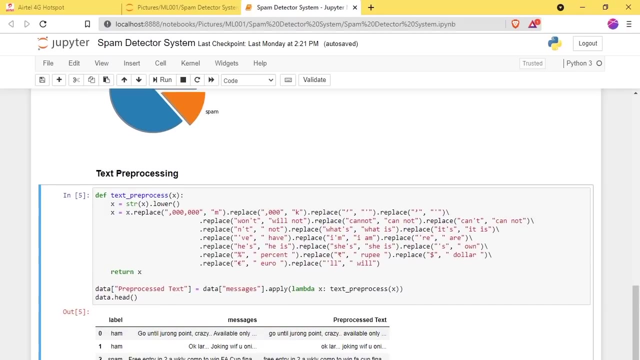 So otherwise no task will be left for you in this task. okay, So here then what we'll do. then you apply to each messages by making a new column. you apply to each messages, these text preprocessing, by doing this all by calling the lambda. 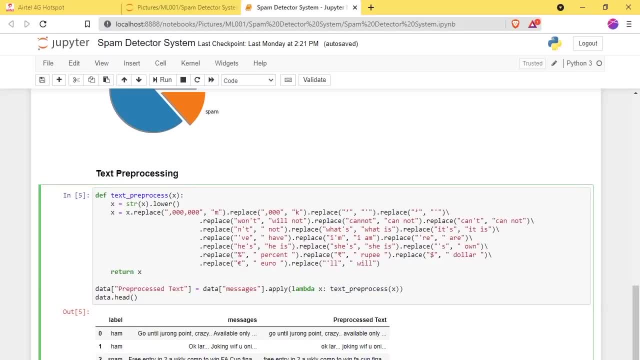 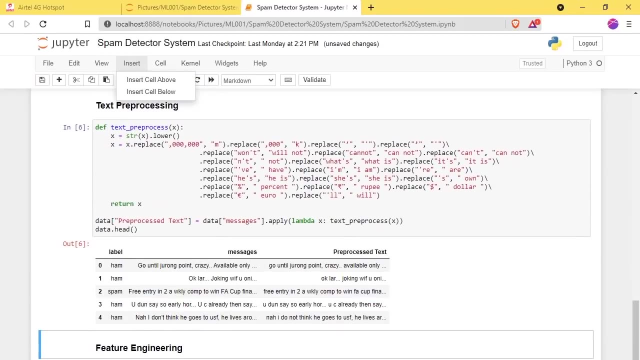 and calling the lambda. it will go to each step. it will go to each step and apply the function onto each messages and put that into a processed text. So let's take an example of that. it will start making more sense if you take a little. 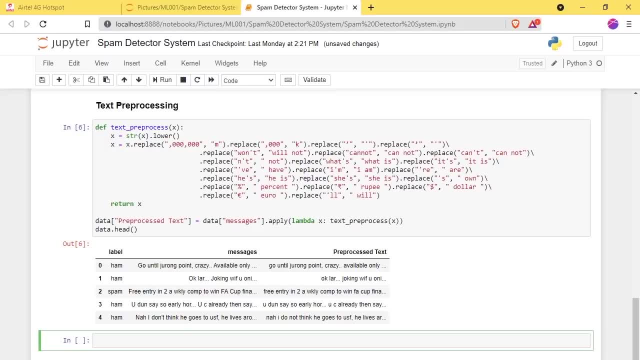 bit of example, okay, So what I'm going to do is I'm going to print out. I'm going to print out not first, which will be our favorite- not processed text, so I'm going to print out first, which is: 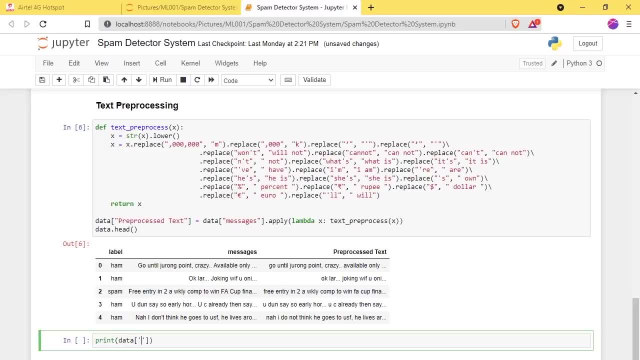 not processed text. so this is our data and then I'm going to post over here. now I want to zero element, and now I'm going to make a simple line. I'm going to make a simple line. oops, what happened? I'm going to make a simple line. 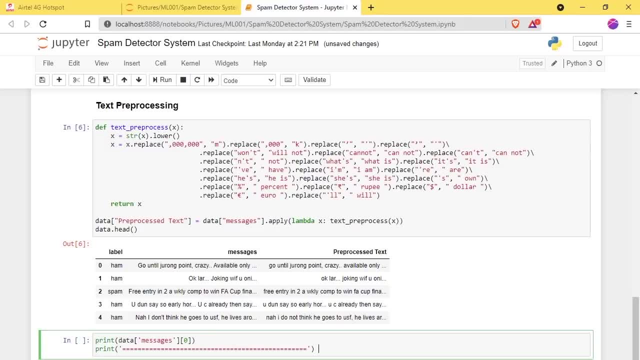 so it just makes this and I'm not, and then I'm going to just paste it over like this: okay, So it will show you what is the preprocessed text. so this preprocessed text is converted like this: okay. 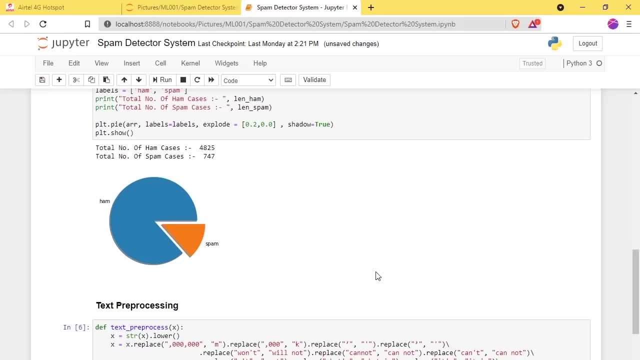 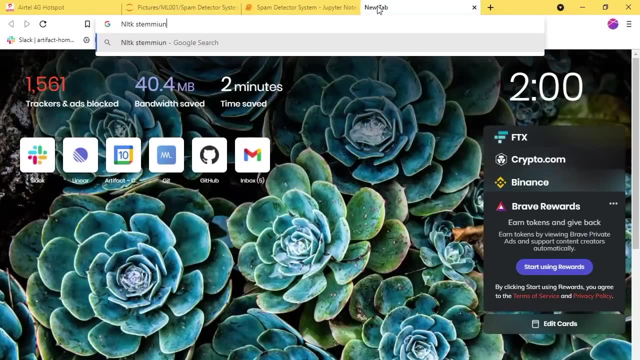 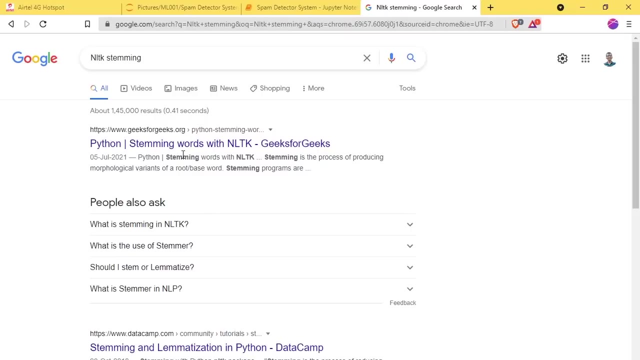 So apply stemming. okay, by using the poorer stemmer you can go to NLTK. NLTK stemming. oops, stemming okay. there is something called a lemmatization so you can see some of the tutorials which are available in Geeks, for Geeks, etc. so read it out means you. 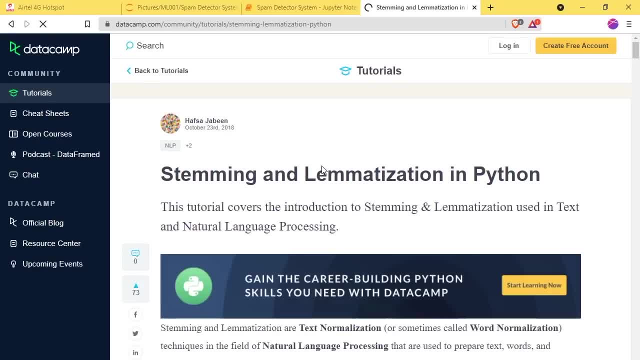 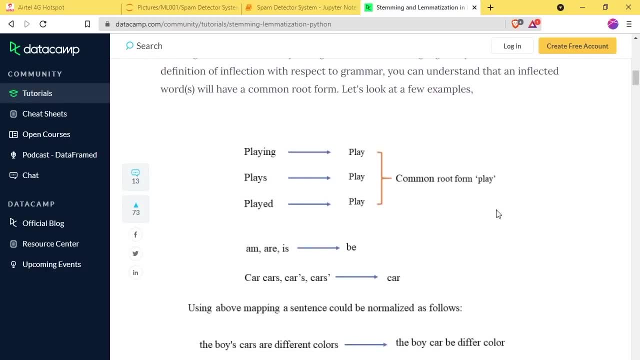 can go to any of them whatever you like. it just converts the words into yeah. here is a good example: so playing, played, played. so it will come common root from played. okay, So this will convert it like this: like stemming is the process of reducing your inflection. 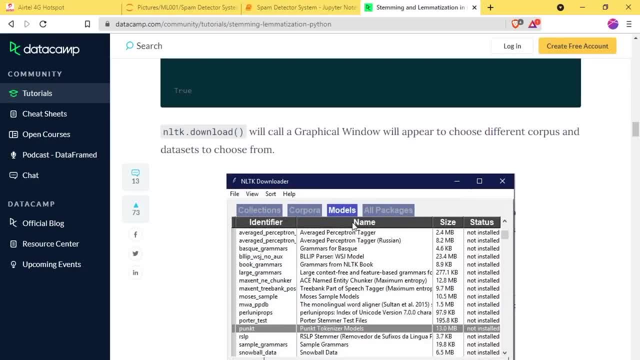 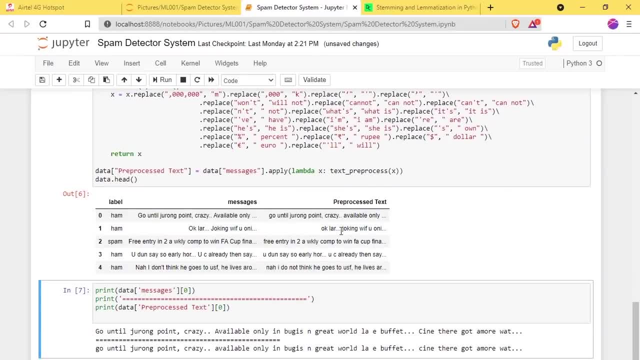 into words. okay, So you can read this, read this sound. this is a very good documentation provided by DataCamp and you will get to know much better about this. but I have been bringing up one full course on to national language processing. just this is a sample: how to work with a text. 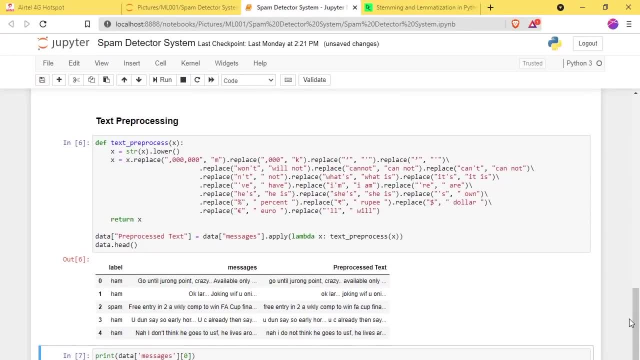 but on new era, on new era, one full course on deep learning. where we will be talking on deep learning, we will cover text working with a textual data. okay, Now we will go further into. now, we will go further into, we will go further into we. 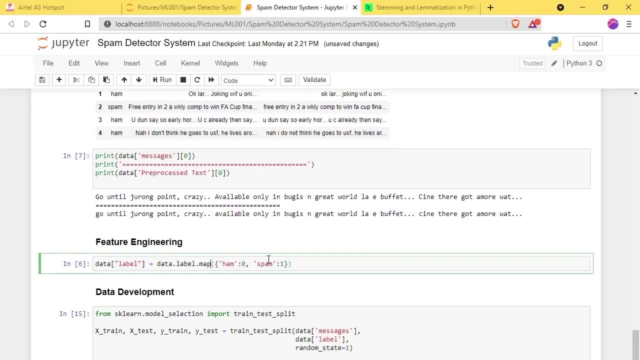 will go further into now. we will go further into now. we will go further into now. we will go further into feature engineering. what is feature engineering Here? we are not going to add any features. we are just going to encode our ham to zero. 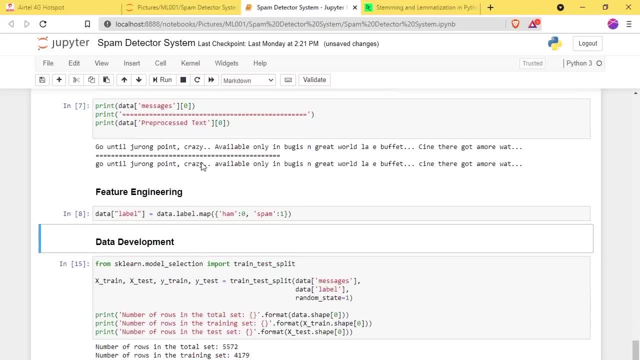 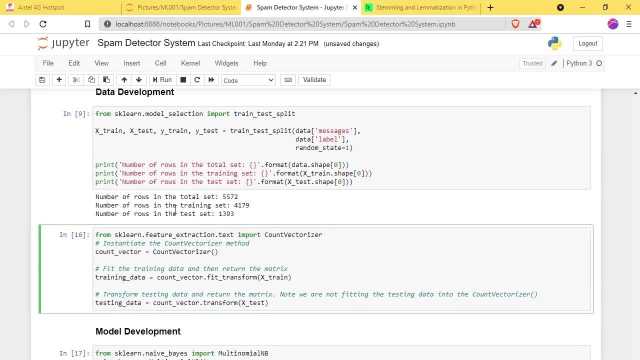 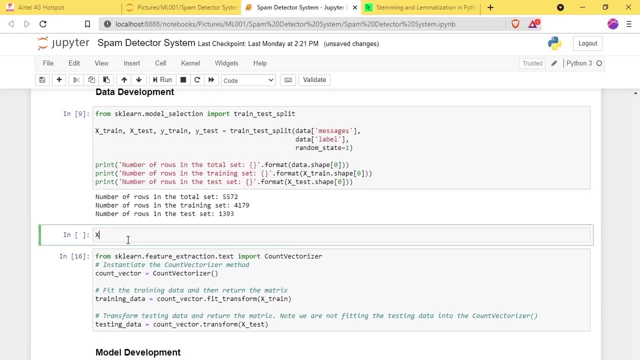 and expand to one by calling our map method. that's done. now we'll divide up our data into train to split. now, if I run it here, we have total number of this and then what we will do now. just assume, now, just see, now just see over here that in training set. 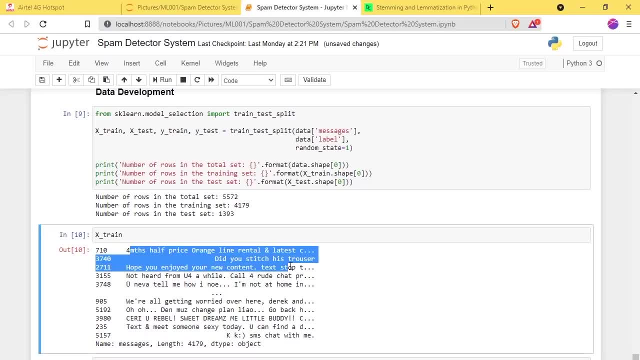 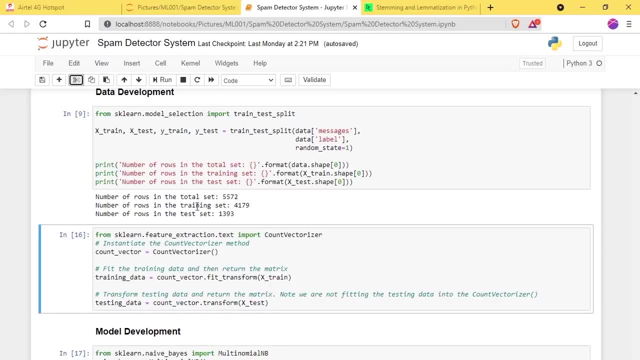 in training set. we have our. we have our data set. we have our data set, we have our text. but neural machine learning will not accept the string or whatever the textual data. so what we have to do there is modern means, word embeddings. then we 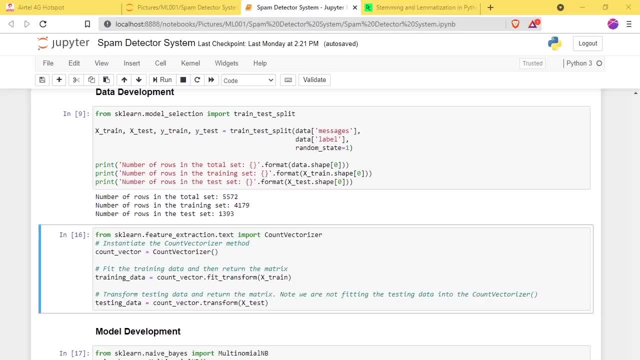 convert our word and then we convert our word into, maybe this word, into some numbers, into some numbers, into some numbers. there are a lot more techniques: count, vectorizer, TF, IDF, vectorizer- bag of words which I'm not going to again talk about again. it's time for you to explore as of now. you can just think of: 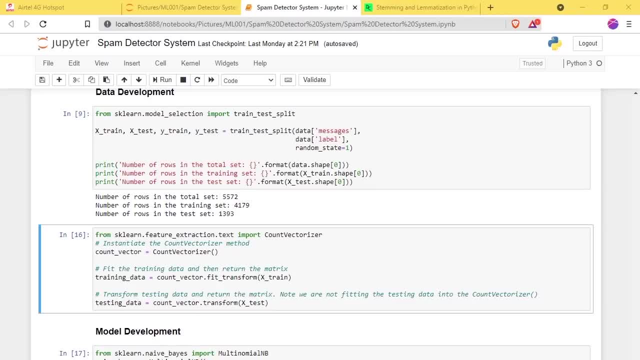 it as you can see there. you can see that what's the mathematical equation for? that is a single mathematical equation, but is what it does. it's simply. you can go to a skill, learn feature extraction: just extract the feature from the text. miss converts your text into the numbers. okay, 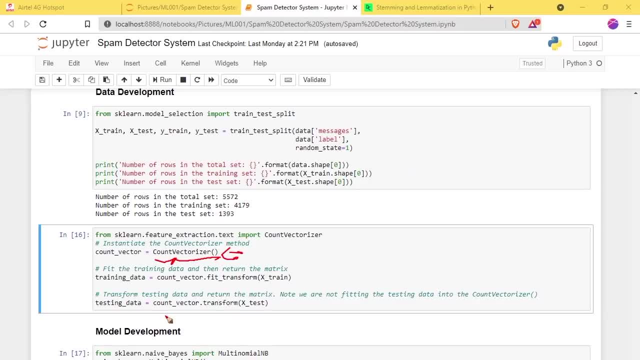 bye. just you instantiate over here now. now, what now? what is it will do? it will fit the training data means and return the matrix. and there is. we don't want to fit the time text test testing, so that's why we are just transforming our text test. 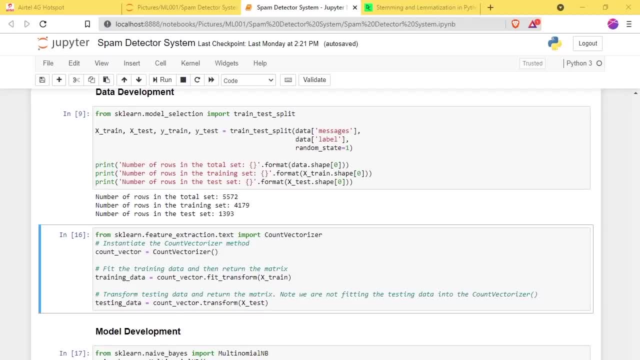 with the numerical into the matrix. okay, that's it. okay, so this is what we use to convert our text into. on vector of numbers: okay, so if I show you the training data, how is the training data? is a sparse matrix. okay, it's a sparse matrix, which is with a five thousand fifty five thousand two hundred nine. 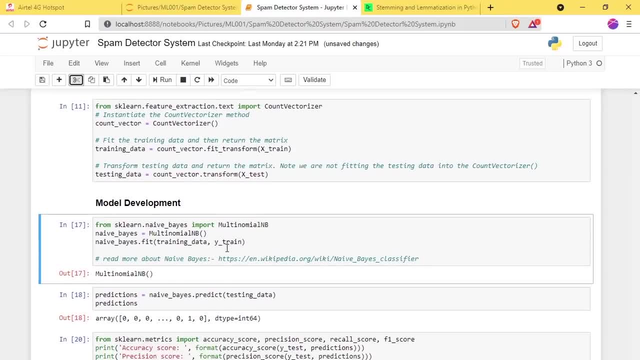 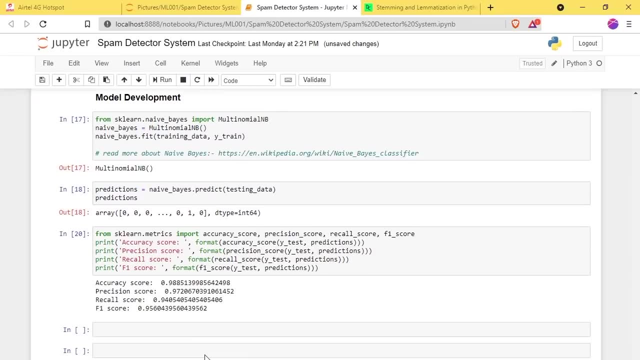 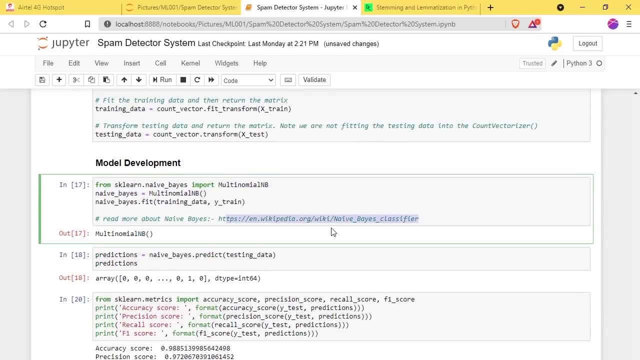 stored elements into that. okay, now we will use nine base. I hope that you understood and I hope that you had a look there on nine days on this, as you have told to do the assignment. so you hope that you had a look at nine days. you can read more about nine. base is just a 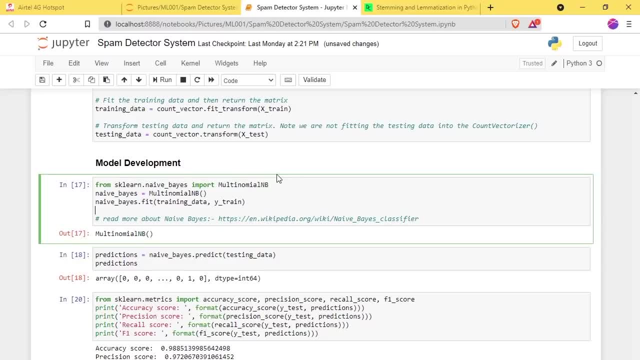 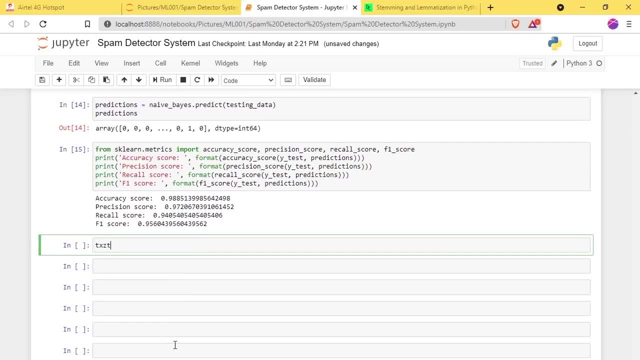 take and take. take an example you have here. you have a text here. you have a text and I'm going to write a. my usage is a good boy, I think. let's see it is if it is a spam or not spam. okay, so I'm gonna just want to convert that. this is: 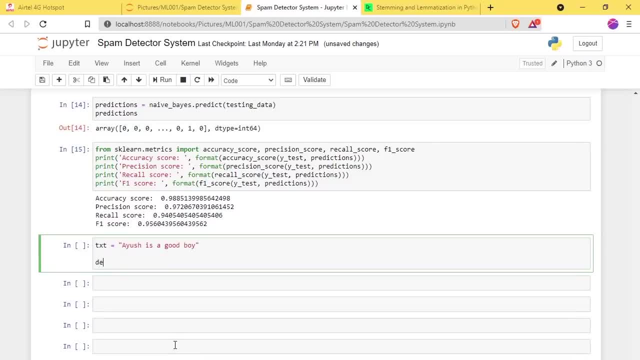 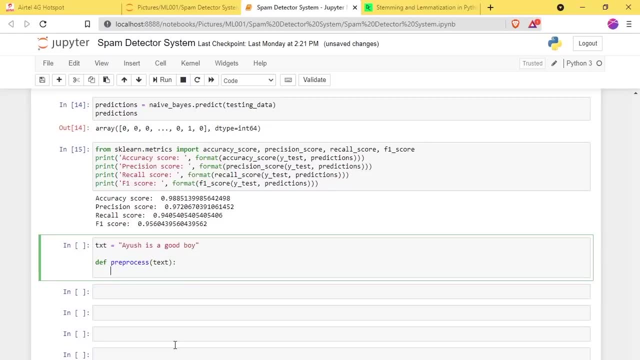 it in, in production, what we do? we write the function process. we write the function will take a text as an input. then what it will do we, we, instead we call our compact riser, which is which we, which we call over here. so I'm going to 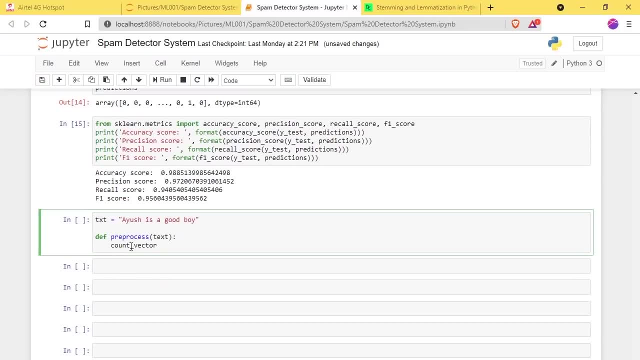 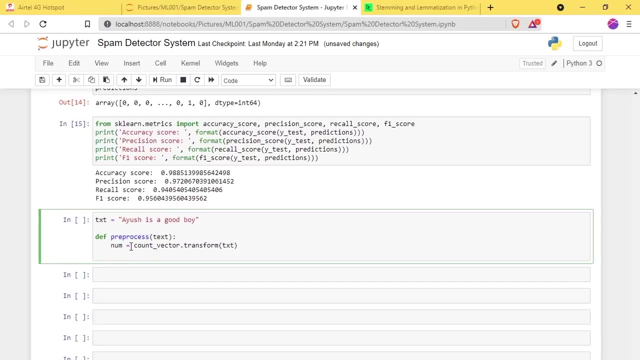 call my count vectorizer, like this count vector dot to transform. I'm going to transform my text: giving, giving, giving this. I'm going to this num, okay, so it will contain the basis of vectors. now I'm going to just call my model, which is maybe it will take a model, so I'm going to call my. 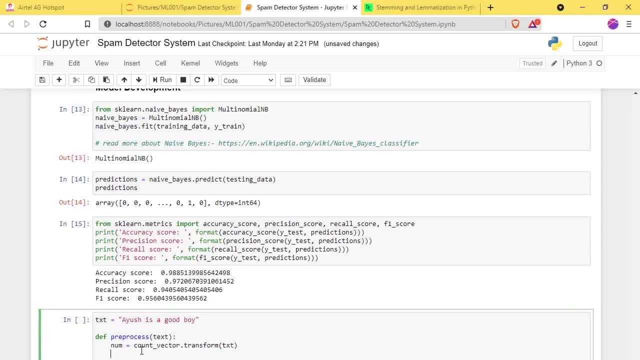 model which is here and I base, and then it will simply dot predict. now it will simply predict my txt, okay, and then I'm going to: oops, it's nom, nom. I have just convert that into a num, so it's the prediction. and what is the prediction? 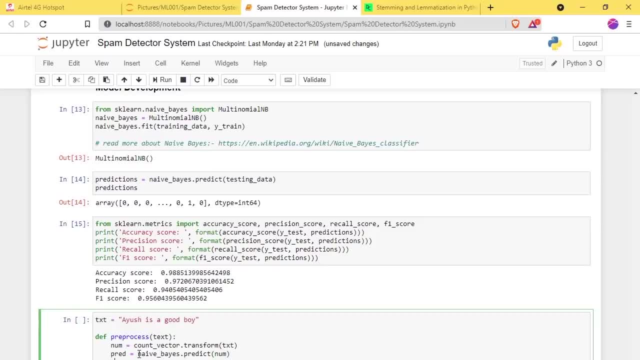 and then what I'm going to do. I'm going to return the prediction. okay, so here, if you call pre process and then pre process and predict so it will be, it will take text as an input and it will return. maybe it may be some problem and maybe I. 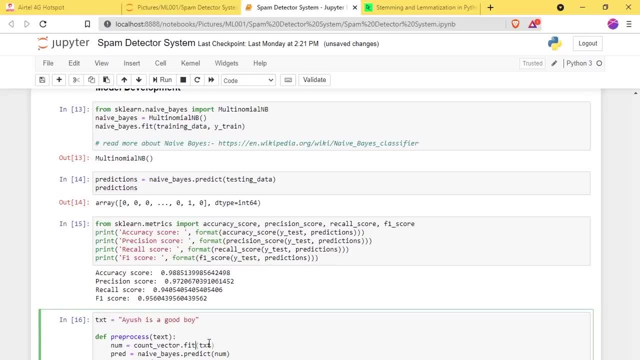 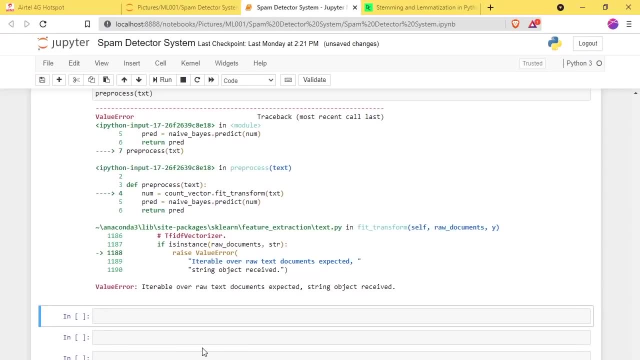 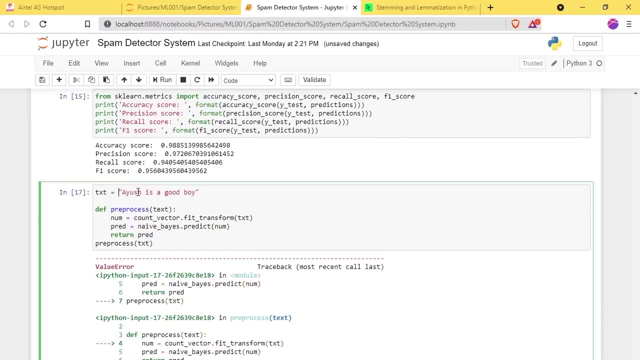 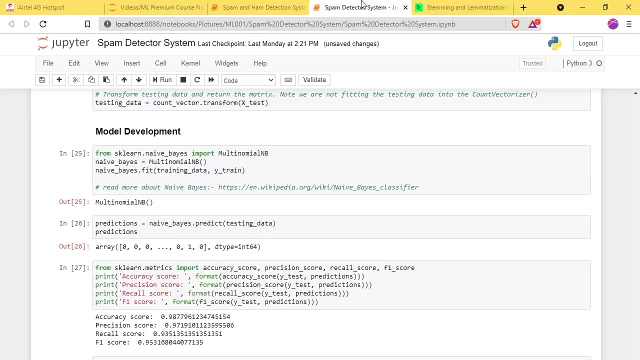 have to do count vector dot fit, transform what happened, the process iteratable over raw documents. a string object received. okay, no worries, so maybe you do call counter on odd element. okay, feel free to connect that to your reference. please don't extensively press ctrl to skip forward team. 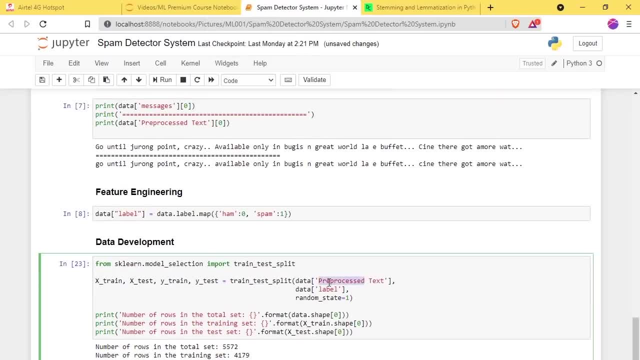 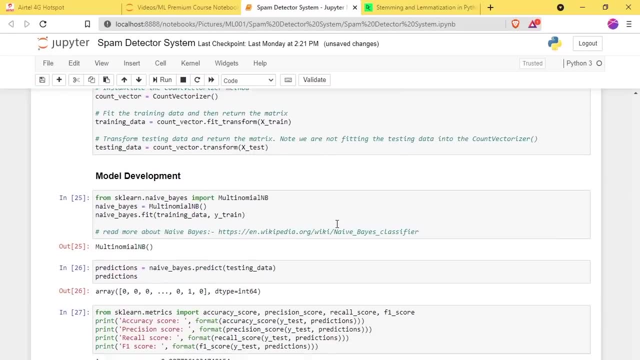 and here you have any another media. Huh, what's the problem was causing is is I'm given messages and in St 8 of this pre process, but we need to be the process text and steer of messages. so here we are, given the messages. now we are just. 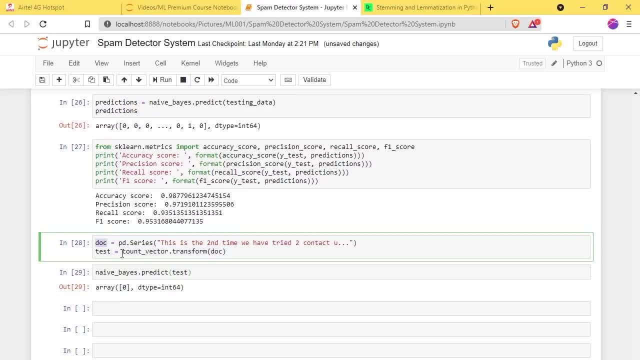 going to protect the cd's and then I'm gonna do count vector dalam transform. I'm giving this talk and then providing nine base dot protect and this, this, this, this will protect this. this, this will predict whether that it will. it is a spam or a non spam. okay.